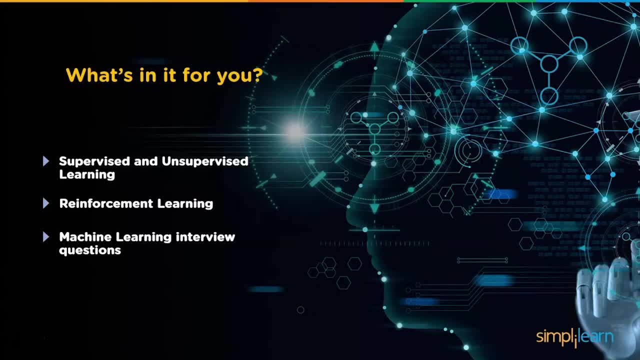 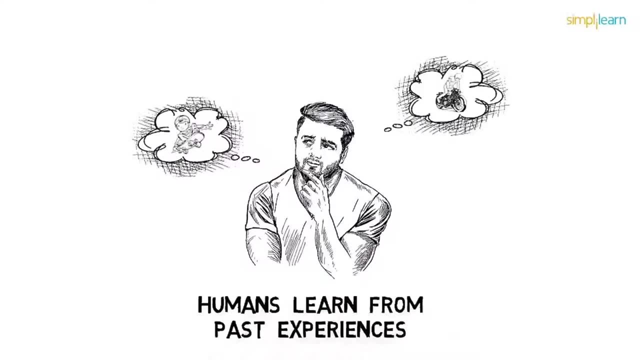 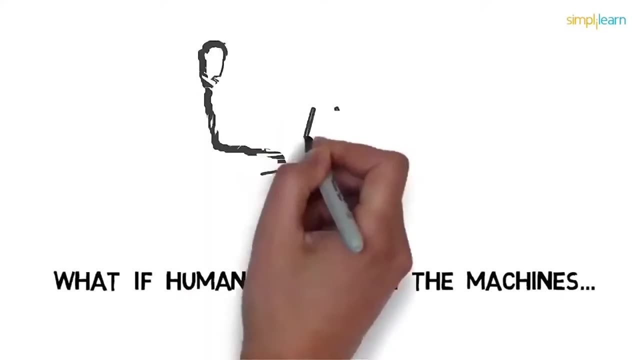 algorithms, all with the help of hands-on demos. So let's get started. We know humans learn from their past experiences and machines follow instructions given by humans. But what if humans can train the machines to learn from their past data and do what humans can do, and much faster? Well, that's called machine learning, But it's a lot more. 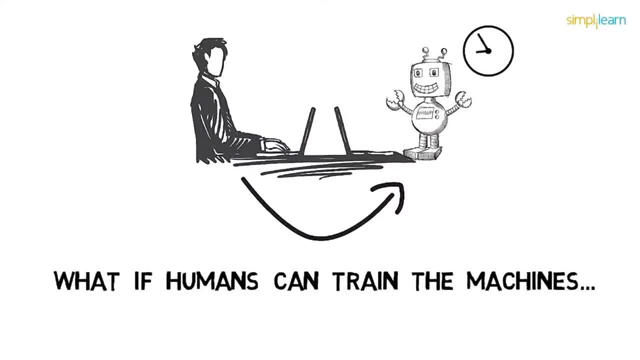 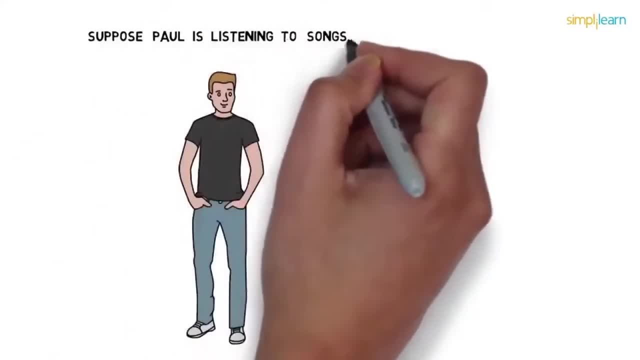 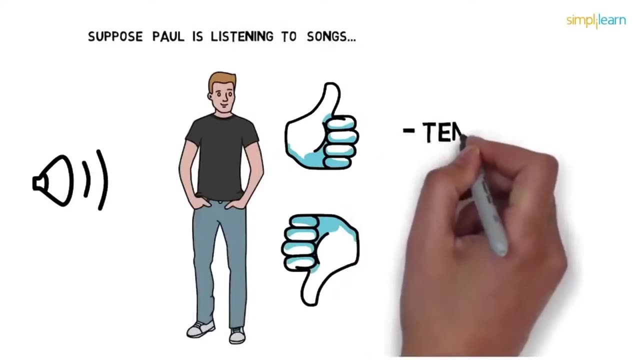 than just learning. It's also about understanding and reasoning. So today we will learn about machine learning. So that's Paul. He loves listening to new songs. He either likes them or dislikes them. Paul decides this on the basis of the song's tempo, genre, intensity. 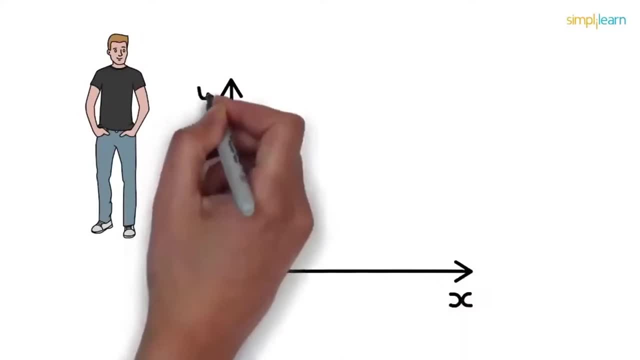 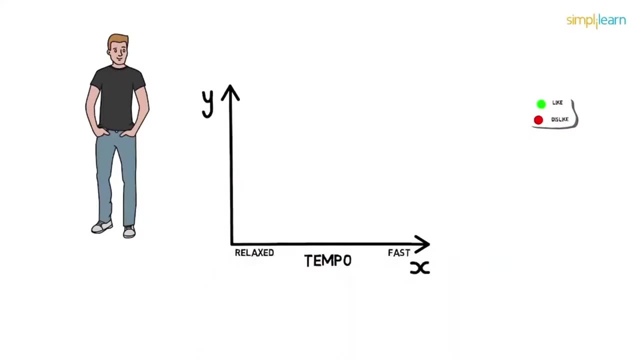 and the gender of voice. For simplicity, let's just use tempo and intensity for now. So here, tempo is on the x-axis, ranging from relaxed to fast, whereas intensity is on the y-axis, ranging from light to soaring. Let's say that Paul likes the song with fast tempo and soaring intensity, while he dislikes 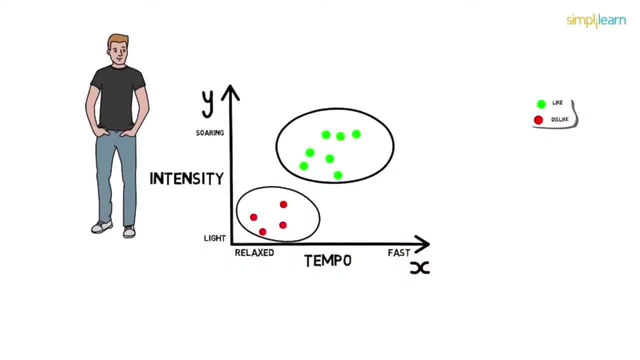 the song with relaxed tempo and light intensity. So now we know Paul's choices. Let's say Paul listens to a new song. Let's name it as song A. Song A has fast tempo and a soaring intensity, So it lies somewhere here. Looking at the data, can you guess whether Paul will like? 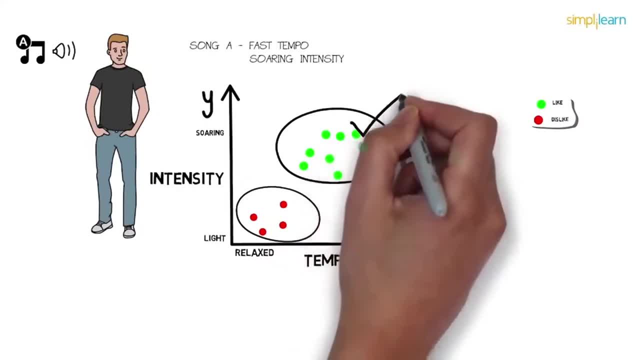 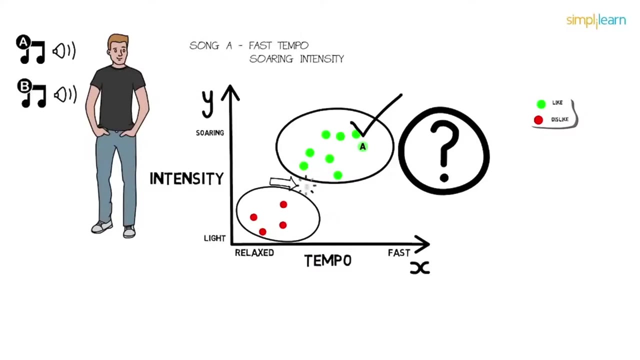 the song or not. Correct. So Paul likes this song. By looking at Paul's past choices, we were able to classify the unknown song very easily, Right? Let's say now Paul listens to a new song, Let's label it as song B. So song B lies somewhere here with medium. 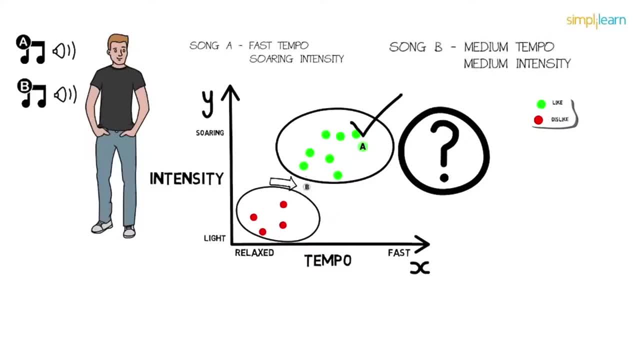 tempo and medium intensity, Neither relaxed nor fast, neither light nor soaring. Now can you guess whether Paul likes it or not? Not able to guess whether Paul will like it or dislike it, Are the choices unclear, Correct? We could easily classify song A, But when? 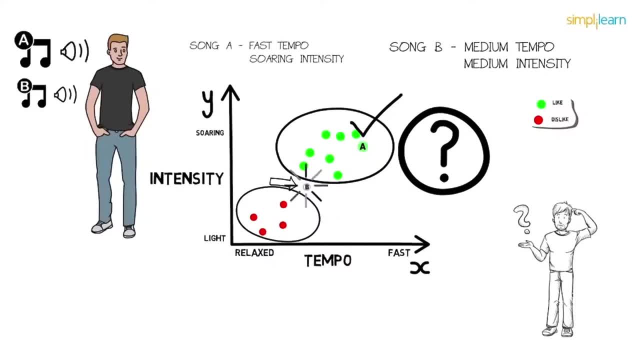 choice became complicated, as in the case of song B. yes, and that's where machine learning comes in. Let's see how. In the same example for song B, if we draw a circle around the song B, we see that there are 4 votes for like, whereas 1 vote for dislike. If we go, 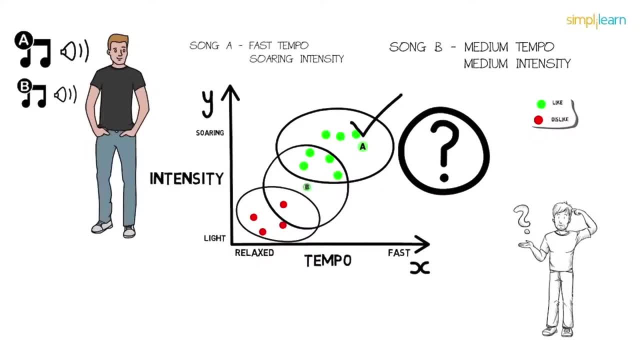 for the majority votes. we can say that Paul will definitely like the song. That's all. This was a basic machine learning algorithm. also, It's called k-nearest neighbours, So this is just a small example in one of the many machine learning algorithms. 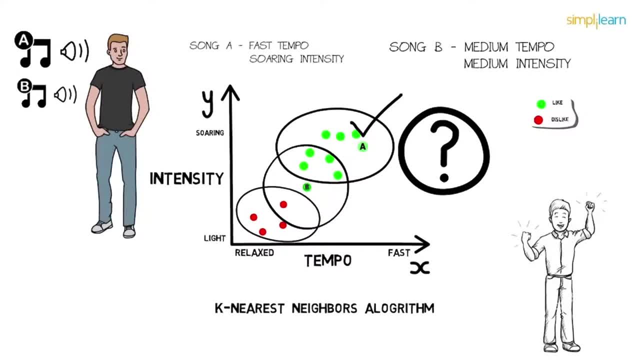 Quite easy right, Believe me it is. But what happens when the choices become complicated, as in the case of song B? That's when machine learning comes in. It learns the data, builds the prediction model, and when the new data point comes in, it can easily predict for. 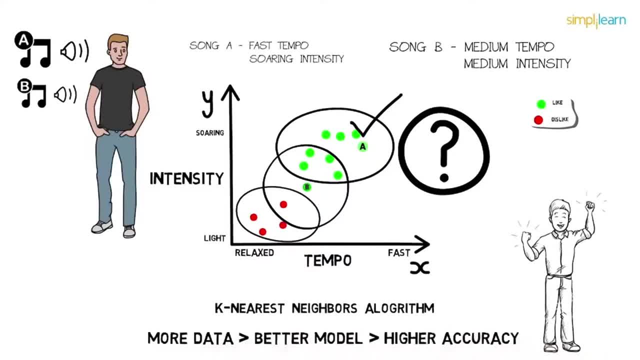 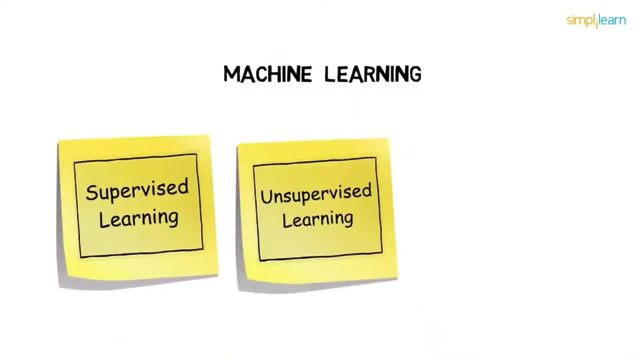 it. More the data, better the model, higher will be the accuracy. There are many ways in which the machine learns. It could be either supervised learning, unsupervised learning or reinforcement learning. Let's first quickly understand supervised learning. Suppose your friend gives you one million. 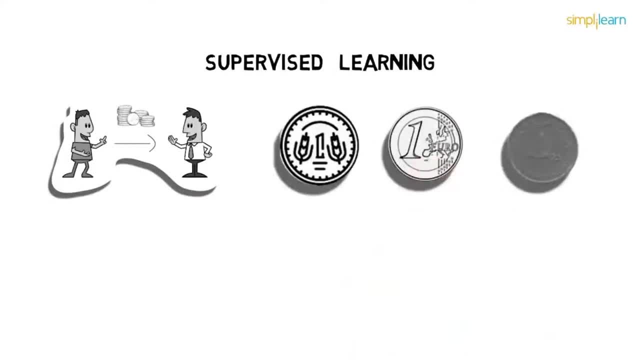 coins of three different currencies, say one rupee, one euro and one dirham. Each coin has different weights. For example, a coin of one rupee weighs 3 grams, one euro weighs 7 grams and one dirham weighs 4 grams. Your model will predict the currency of the coin. 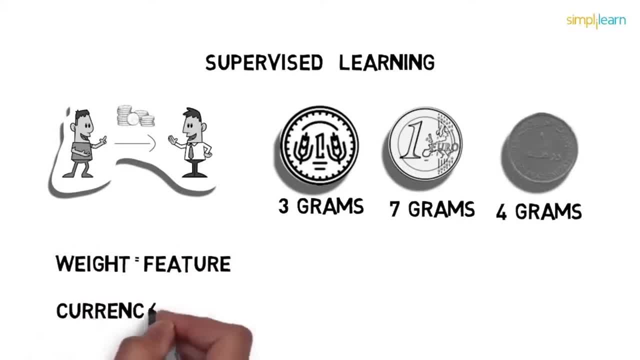 Here, your weight becomes the feature of coins, while currency becomes their label. When you feed this data to the machine learning model, it learns which feature is associated with which label. For example, it will learn that if a coin is of 3 grams, it will be a one. 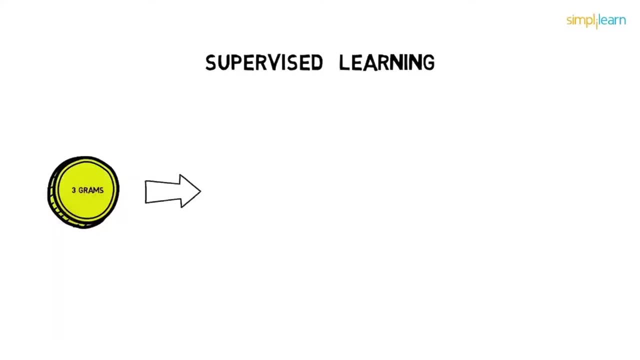 rupee coin. Let's give a new coin to the machine. On the basis of the weight of the new coin, your model will predict the currency. Hence supervised learning uses labeled data to train the model. Here the machine knew the features of the. 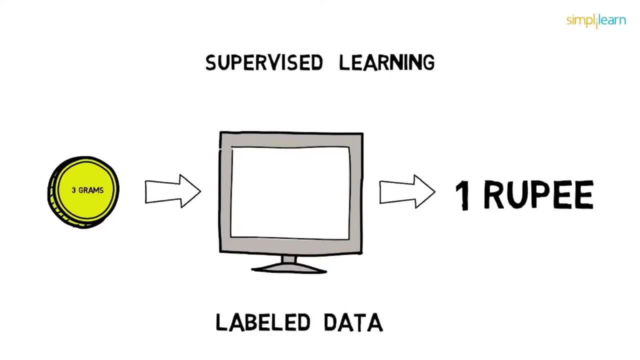 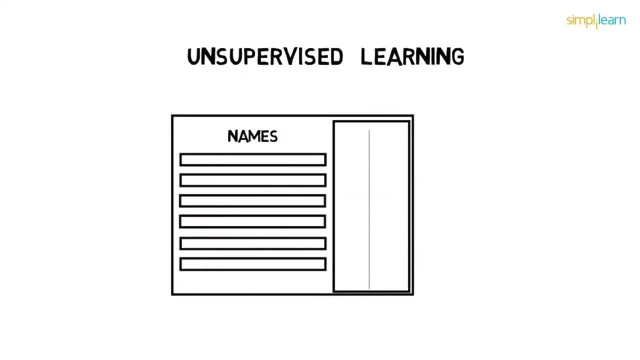 object and also the labels associated with those features. On this note, let's move to unsupervised learning and see the difference. Suppose you have a cricket dataset of various players with their respective scores and the wickets taken. When we feed this dataset to the machine, the machine identifies the pattern. 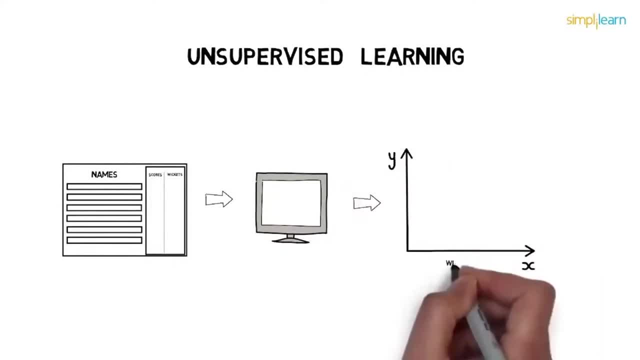 of player performance. So it plots this data with the respective wickets on the x-axis while runs on the y-axis. While looking at the data, you will clearly see that there are two clusters. The one cluster are the players who scored high runs and took less. 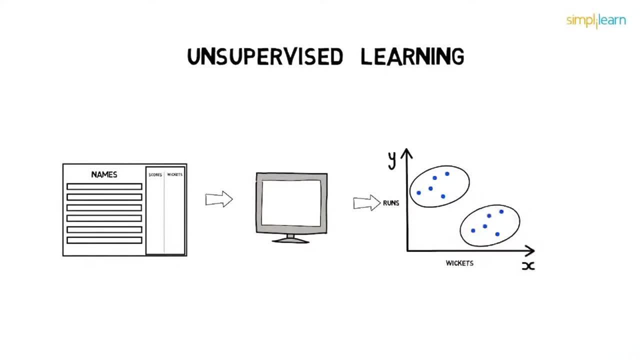 wickets, while the other cluster is of the players who scored less runs but took many wickets. So here we interpret these two clusters as batsmen and bowlers. The point to note here is that there were no labels of batsmen and bowlers, Hence the 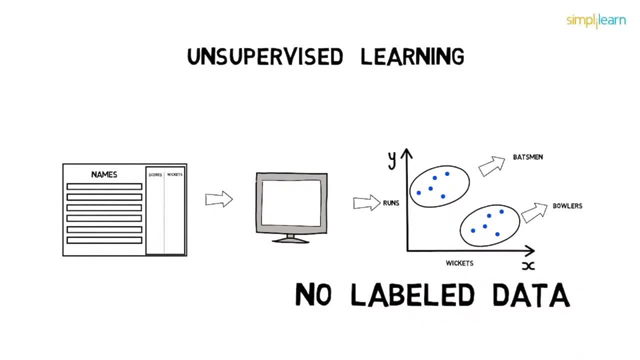 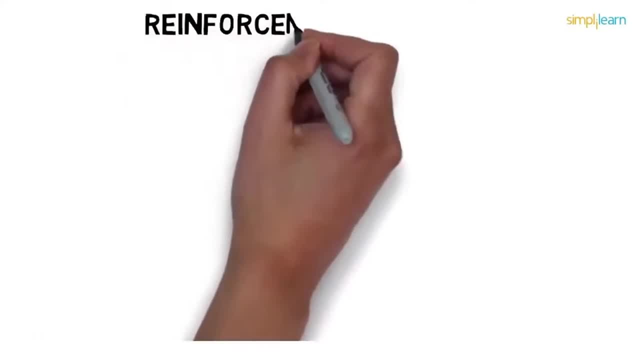 learning with unlabeled data is unsupervised learning. So we saw supervised learning where the data was labeled, and the unsupervised learning where the data was unlabeled. And then there is reinforcement learning, which is reward-based learning. or we can say: 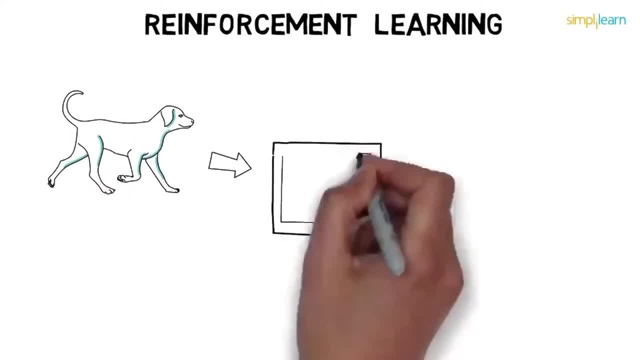 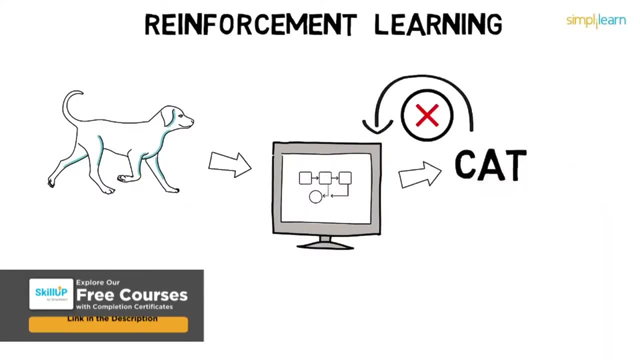 that it works on the principle of feedback Here. let's say you provide the system with an image of a dog and ask it to identify it. The system identifies it as a cat, So you give a negative feedback to the machine, saying that it's a dog's image. 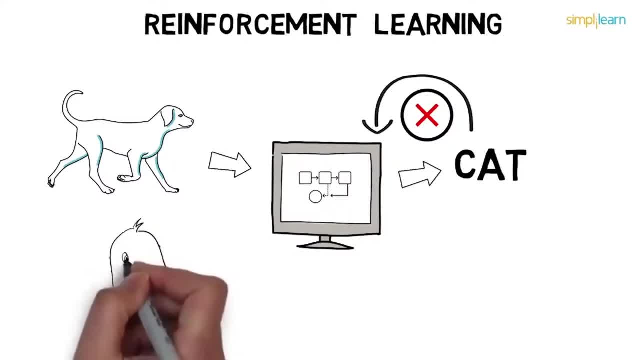 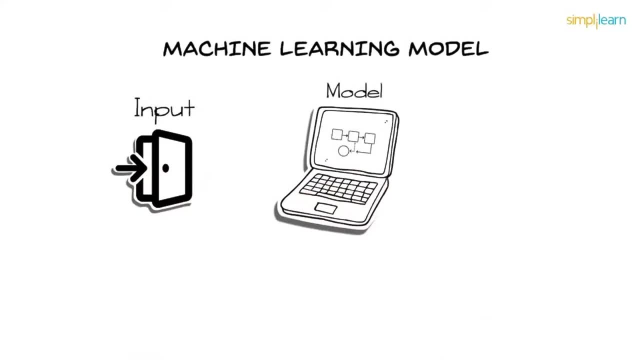 The machine will learn from the feedback and finally, if it comes across any other image of a dog, it'll be able to classify it correctly. That is reinforcement learning. To generalize machine learning model, let's see a flowchart. Input is given to a machine learning model. 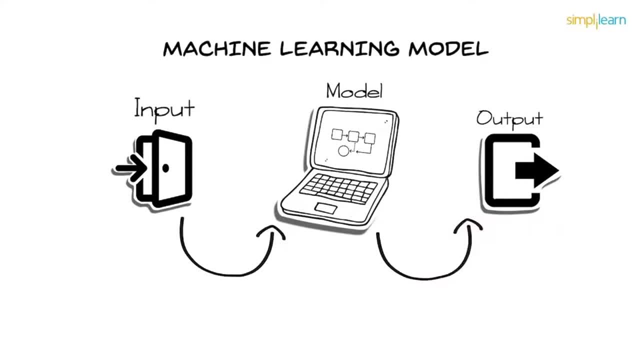 which then gives the output according to the algorithm applied. If it's right, we take the output as our final result. Else, we provide feedback to the training model and ask it to predict until it learns. I hope you've understood supervised and unsupervised learning. 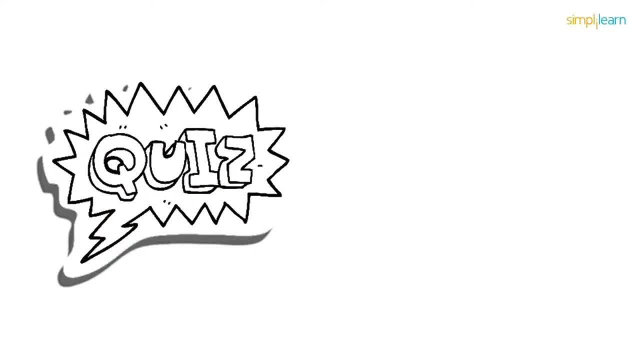 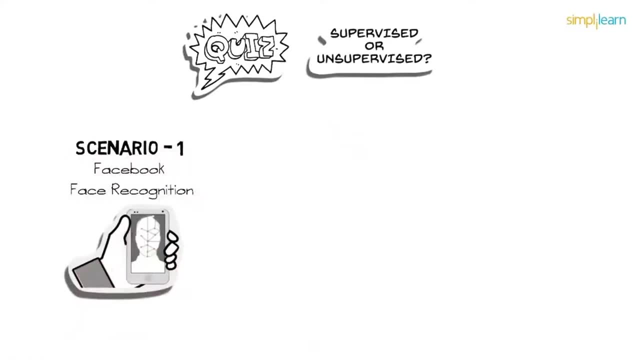 So let's have a quick quiz. You have to determine whether the given scenarios uses supervised or unsupervised learning. Simple right. Scenario 1.: Facebook recognizes your friend in a picture from an album of tagged photographs. Scenario 2.: 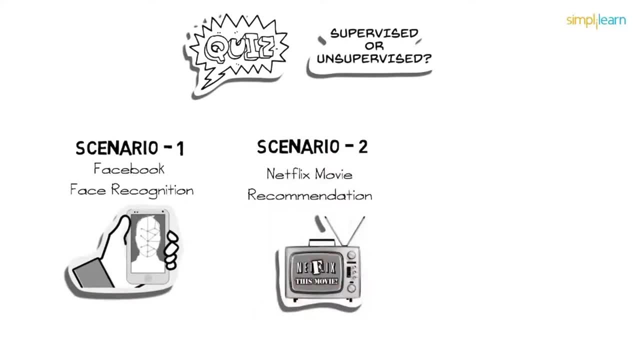 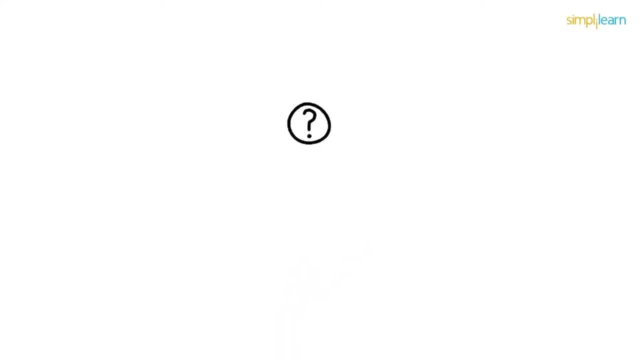 Netflix recommends new movies based on someone's past movie choices. Scenario 3. Analyzing bank data for suspicious transactions and flagging the fraud transactions. Think wisely and comment below your answers Moving on. don't you sometimes wonder how is machine learning possible in today's era? 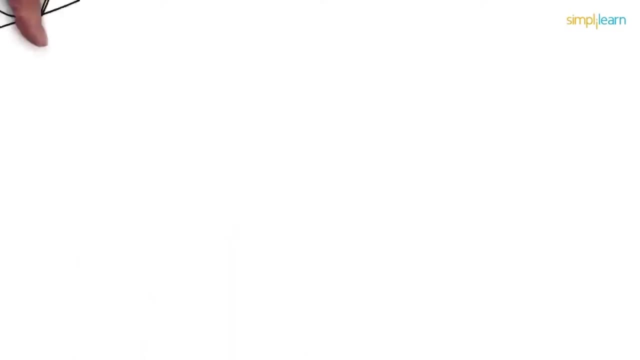 Well, that's because today we have humongous data available. Everybody's online, either making a transaction or just surfing the internet, and that's generating a huge amount of data every minute. And that data, my friend, is the key to analysis. 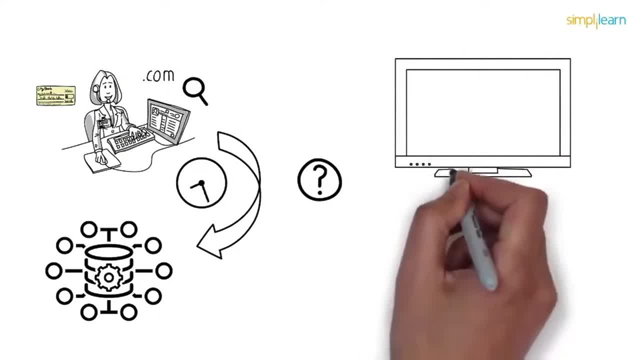 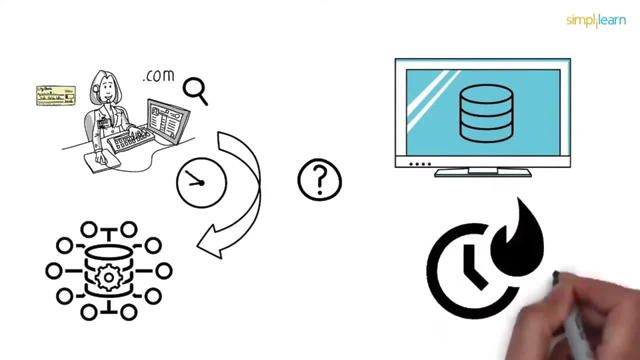 Also, the memory handling capabilities of computers have largely increased, which helps them to process such a huge amount of data at hand. Scenario 4. Without any delay, And yes, computers now have great computational powers, So there are a lot of applications of machine learning out there. 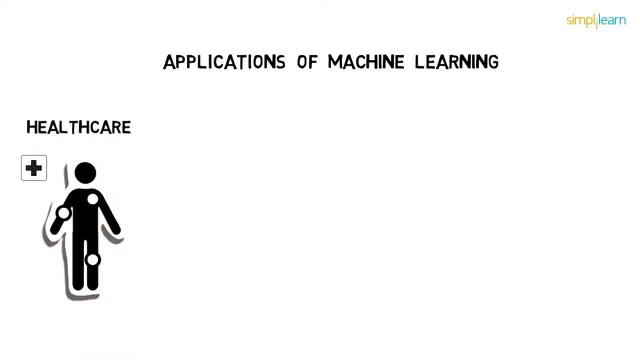 To name a few. machine learning is used in healthcare where diagnostics are predicted for doctor's review. The sentiment analysis that the tech giants are doing on social media is another interesting application of machine learning: Fraud detection in the finance sector and also to predict customer churn in the e-commerce sector. 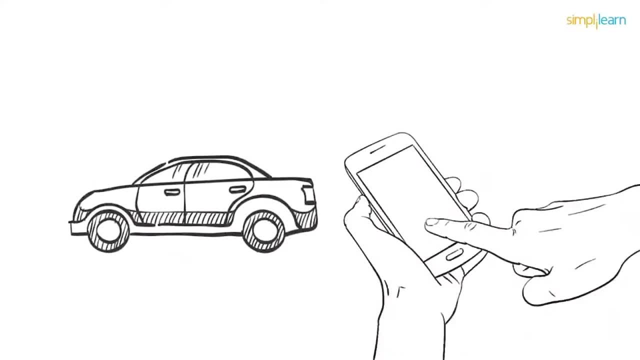 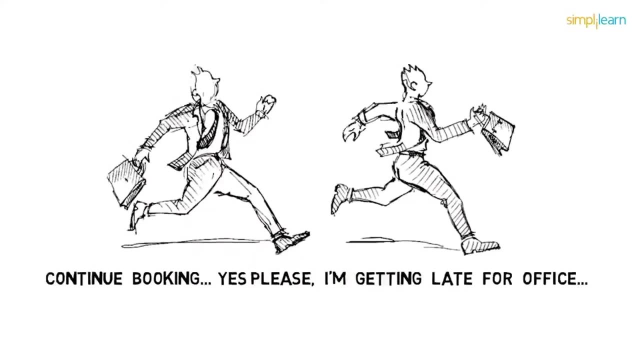 While booking a cab, you must have encountered surge pricing, often where it says the fare of your trip has been updated. Continue booking. Yes, please, I'm getting late for office. Well, that's an interesting machine learning model which is used by global taxi giant Uber and others. 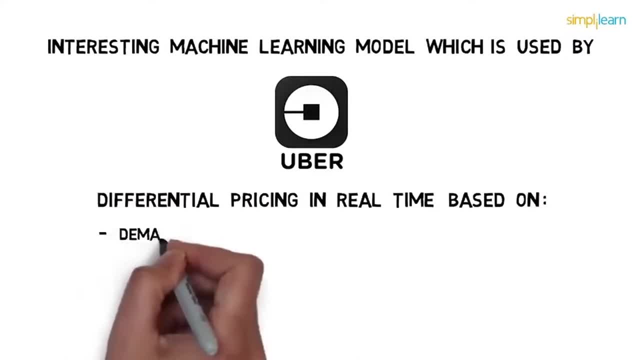 where they have differential pricing in real time based on demand, the number of cars available, bad weather, rush hour, etc. So they use the surge pricing model to ensure that those who need a cab can get one. Also, it uses predictive modeling. 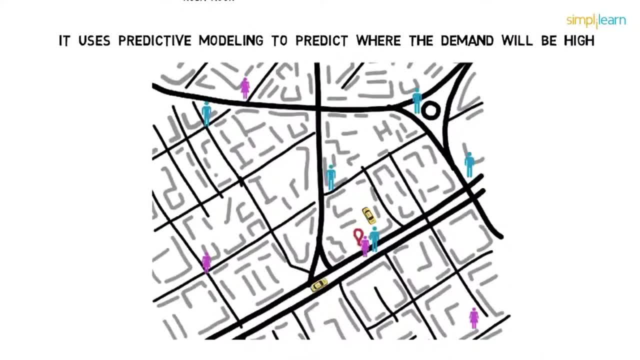 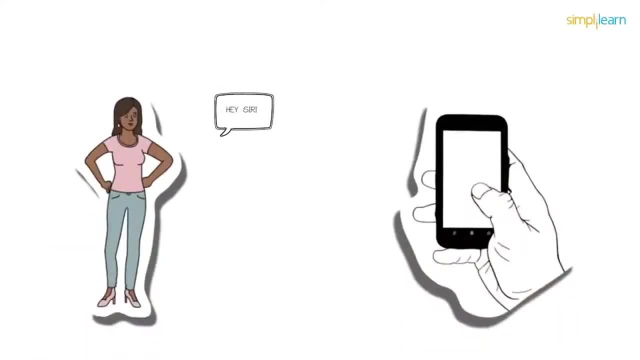 to predict where the demand will be high, with a goal of getting a cab. It's a whole that drivers can take care of the demand and surge pricing can be minimized. Great Hey Siri. can you remind me to book a cab at 6PM today? 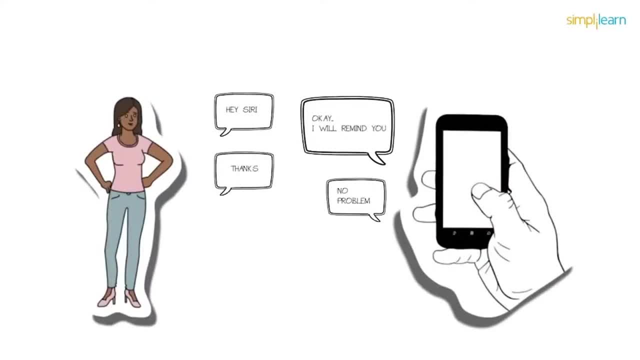 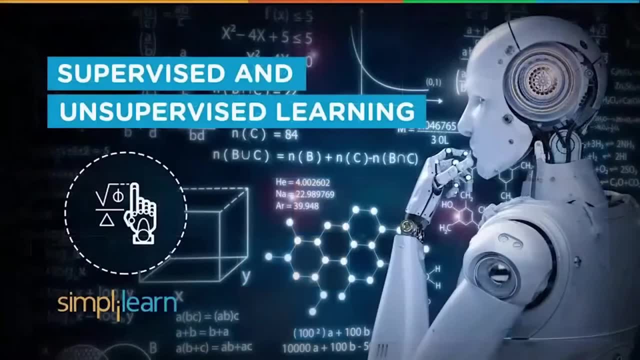 Ok, I will remind you. Thanks, No problem. Comment below some interesting everyday examples around you where machines are learning and doing amazing jobs. Hi Guys, This is a picture from Simply Learn, and we are going to talk about the two types of machine learning. 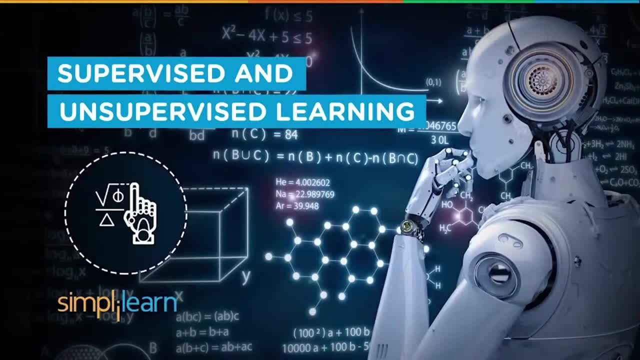 Supervised and Unsupervised learning their types and applications. But before we talk about them, But before we talk about them, let's quickly understand what is machine learning. These days, applications use artificial intelligence in machine learning to optimize speech recognition. I usually ask Siri things I want to know, like: hey Siri, how far is the nearest subway? 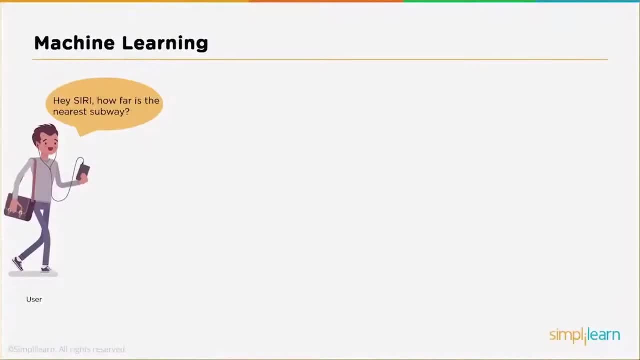 So whenever we ask something to Siri, a powerful speech recognition kicks off and converts the audio into its corresponding textual form, which is then sent to the Apple servers for further processing. Then neural language processing algorithms are run to understand the user's intent, And then, finally, Siri tells you the answer. 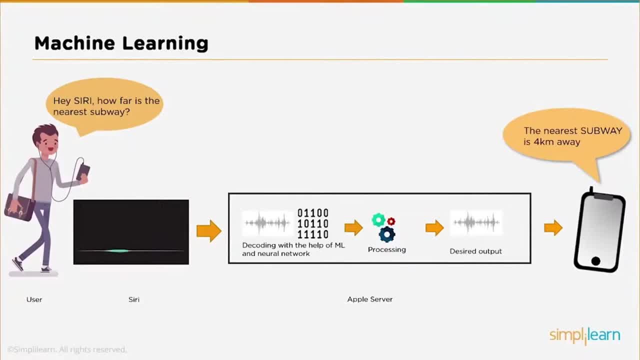 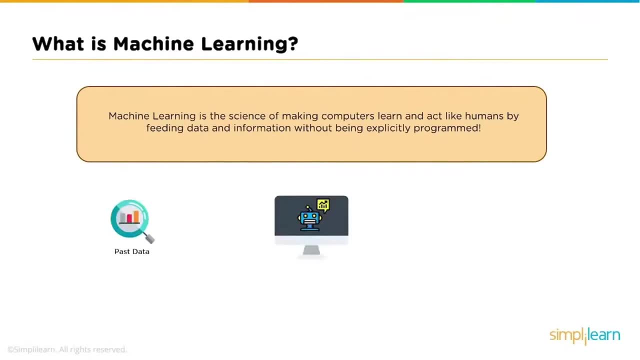 Well, this is what machine learning is all about: making the machines learn and act like humans by feeding them with data and information without being explicitly programmed. As we saw in the previous example, when the data comes in, machines immediately starts analyzing the data and eventually gets trained on it and learns it. 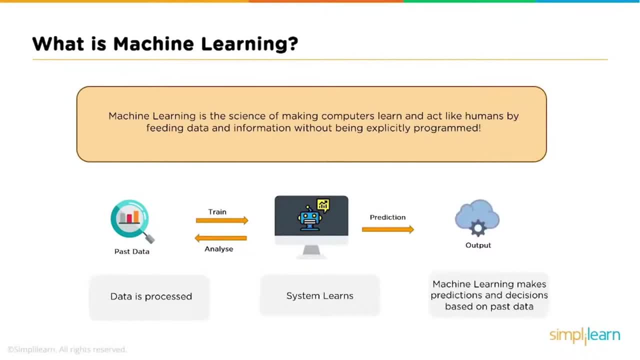 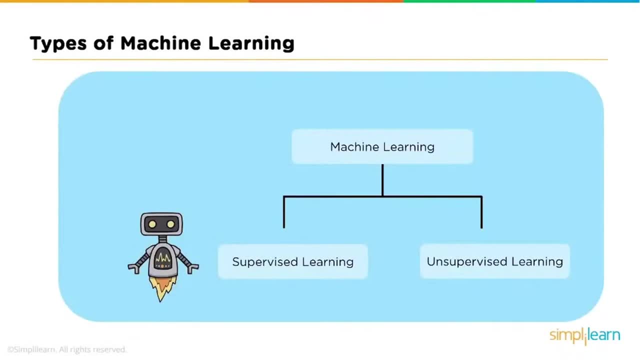 Now, when a new data point comes in, Machine accurately makes predictions and decisions based on the past data. Now that you know what is machine learning, let's talk about supervised and unsupervised learning. Supervised learning, as the name suggests, works under supervision, that is, it's a 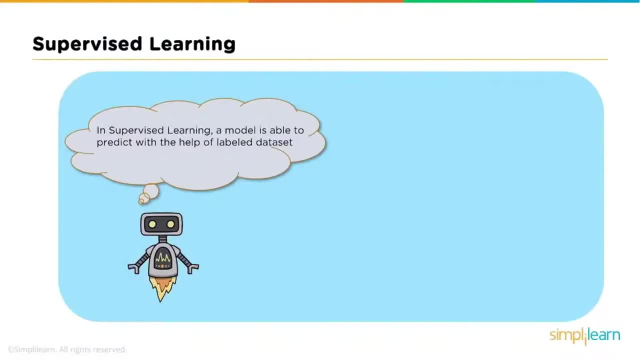 learning, in which machine is trained with data which is well labelled and then predicts with the help of the labelled dataset. But what is a labelled dataset? Data for which you already know the target answer is called a labelled data, Like I show you an image and tell you that it's a dog. 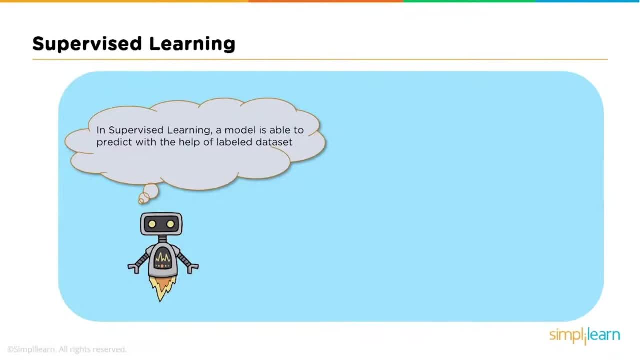 Then it's a labelled data, while if I show you an image without telling you what exactly it is, then it's an unlabelled data. Now let's say we have images which are labelled as spoon or knife. We then feed it to the machine, which analyzes and learns the association of these images. 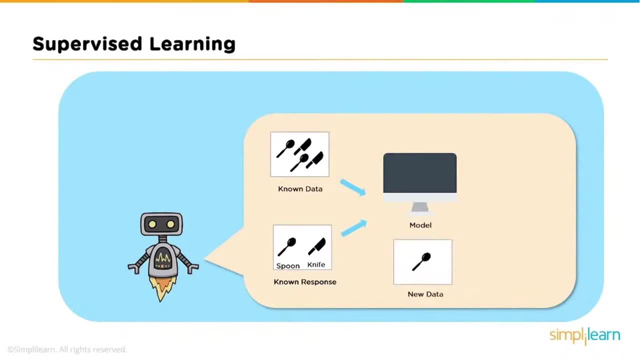 with its labels based on its features, such as shape, size, sharpness, etc. Now, when a new image is fed to the machine without any label, with the help of the past data, The model is able to predict accurately and tell that it's a spoon. 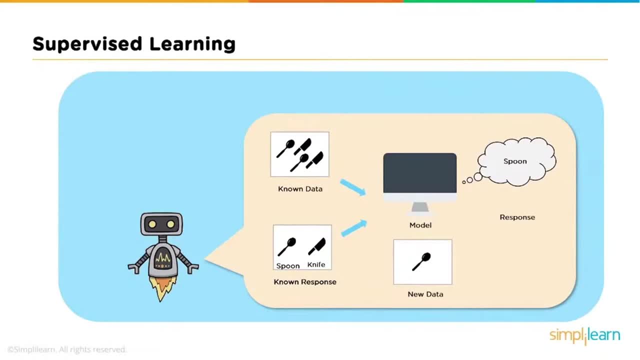 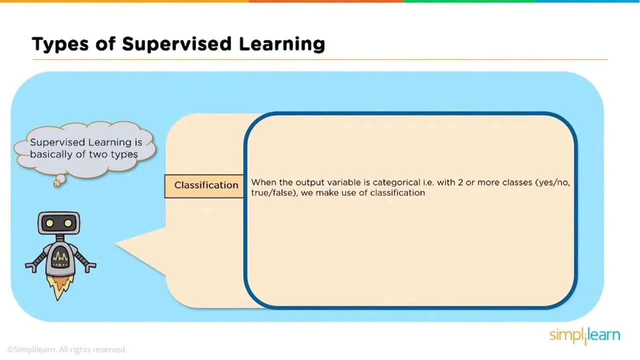 Hence, in supervised machine learning, the algorithm teaches the model to learn from the labelled example that we provide. So supervised learning can be further divided into classification and regression. It is a classification problem when the output variable is categorical, such as red or blue. 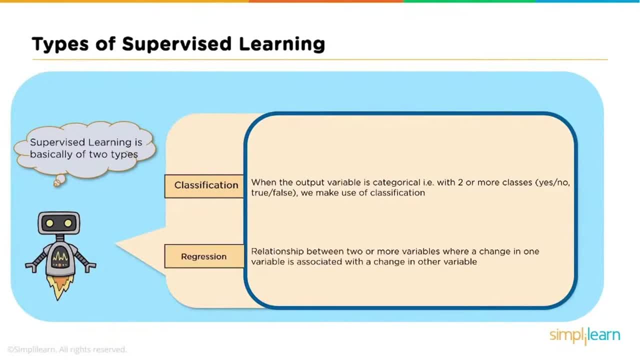 disease or no disease, male or female, whereas it's a regression problem when the output variable is a real or continuous value, For example salary based on work experience, weight based on height. So it creates a predictive model showing trends and data. 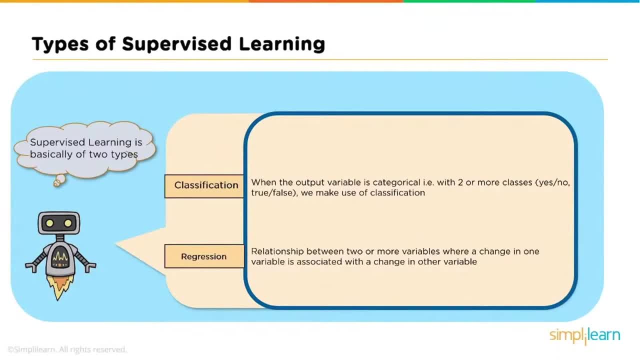 So now, if I say, will I get a salary raise or not, That's classification. But if I say, how much salary raise will I get, That is regression. Now let's understand classification with the help of an example, In order to predict whether an email is a spam or not. first we need to teach our machine. 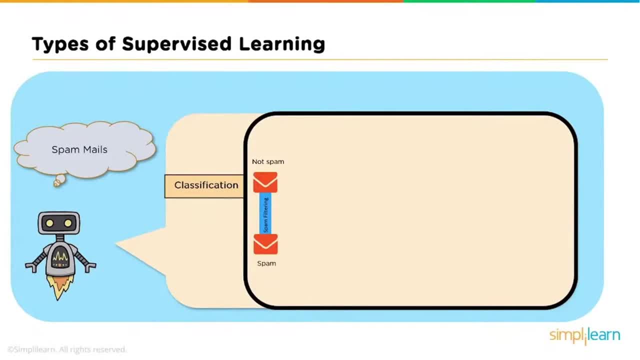 what a spam mail looks like. This is done based on a lot of spam facts. So, for example, if I say I will get a salary raise or not, that's classification. But if I say I will get a salary raise or not, that's classification. 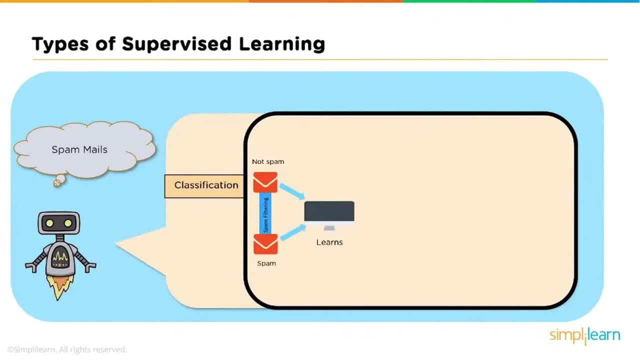 This is done based on a lot of spam filters like firstly reviewing the content of the email, then review the email header and search if it contains any falsified information. This is done based on some keywords like free lottery, price claim, etc. 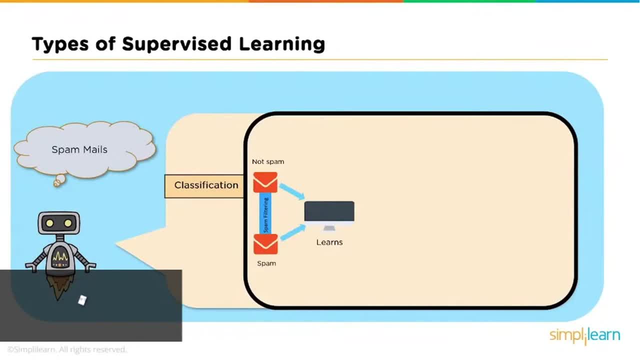 Then general blacklist filters to stop emails that come from already blacklisted known spammers and etc. So all these filters scores the email, which is known as spam score. The lower the total spam score of the email, it is more likely that the email will land. 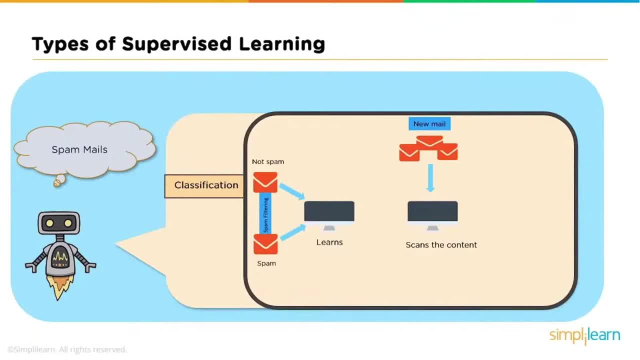 in subscribers' inboxes. So based on the content labels and spam score of the new incoming mail, the algorithm decides whether it should land in inbox or the spam folder. Now let's quickly understand regression. So let's say we have two variables, that is, temperature and humidity. where temperature 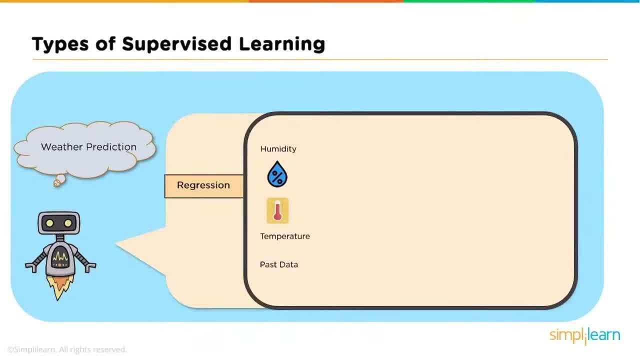 is the independent variable and humidity is the dependent variable, Such that as the temperature increases, humidity decreases. hence they are correlated. When we feed this data to a regression model, it will understand the relationship between these two variables and how one variable depends on the other. 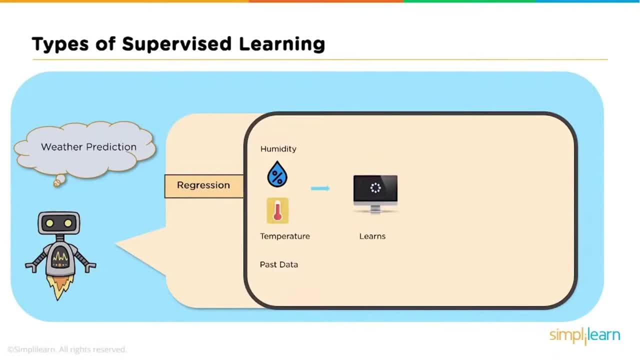 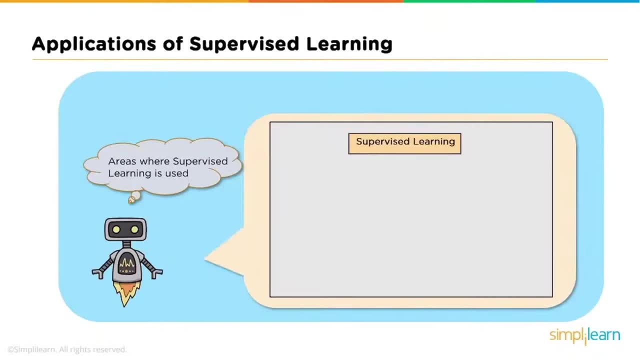 After the machine is trained, it can easily predict the humidity based on the given temperature. Well, that was about regression. Now let's see some real life applications where supervised learning is used. So supervised learning is used in risk assessment To assess risk in financial services or an insurance domain, to minimize the risk portfolio. 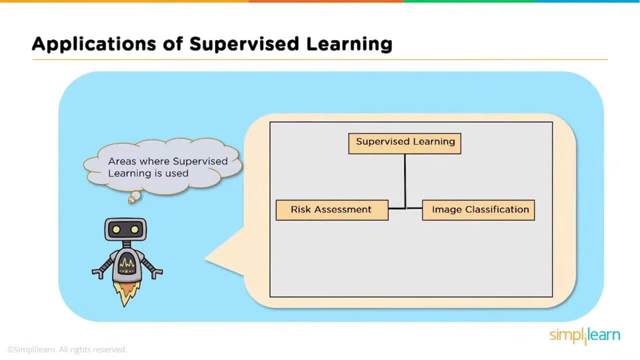 of the companies. Image classification: Facebook recognizes your friend in a picture from an album of tagged photos. So image classification is one of the key use cases of demonstrating supervised machine learning algorithms. Obviously, a lot more goes into all these, like convolutional neural networks, etc. 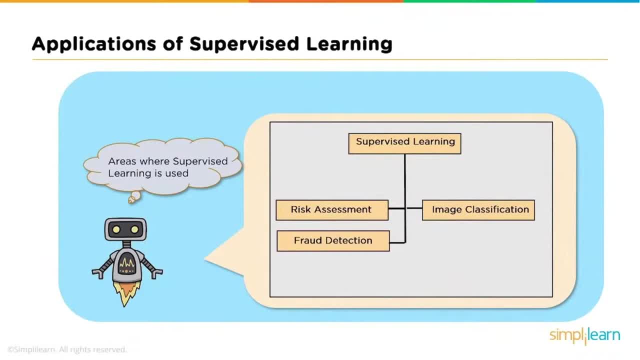 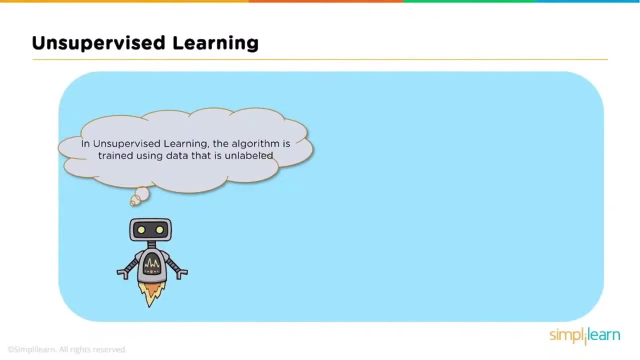 Fraud detection- Whether the transactions made by the user are authentic or not. And visual recognition- The ability of a machine learning model to identify objects, places, people and actions and images. Now let's quickly talk about unsupervised learning. In unsupervised learning, there is no supervision, ie no training will be given to the machine. 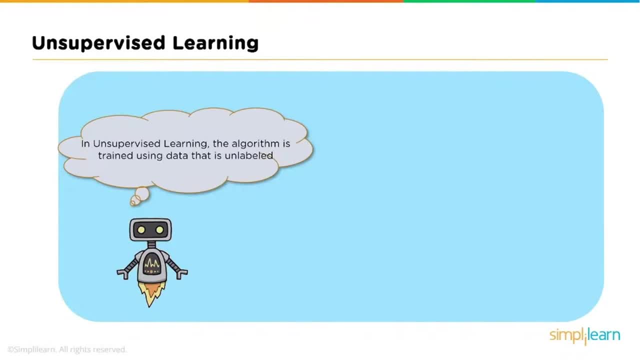 allowing it to act on the data which is not labeled. Hence machine tries to identify patterns and gives the response. Let's take a similar example as before, but this time we do not tell the machine whether it's a spoon or a knife. The machine identifies patterns from the given set and groups them based on their patterns. 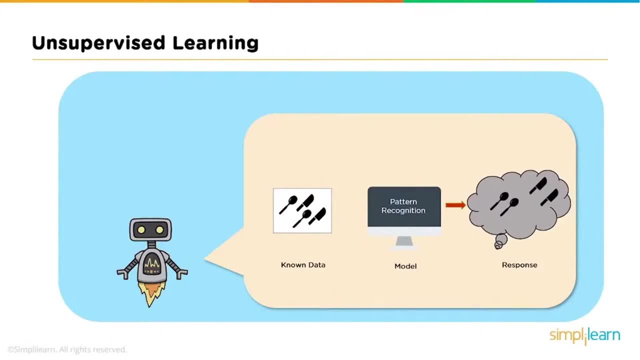 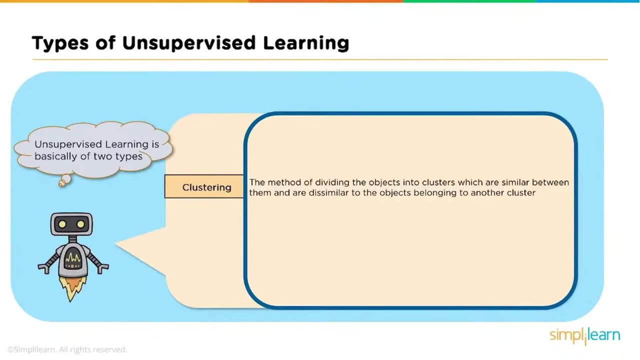 similarities, etc. Again, unsupervised learning can be further grouped into clustering and association. Clustering is basically where the machine forms groups based on the behavior of the data. Secondly, association: It is a rule-based machine learning to discover interesting relation between variables in 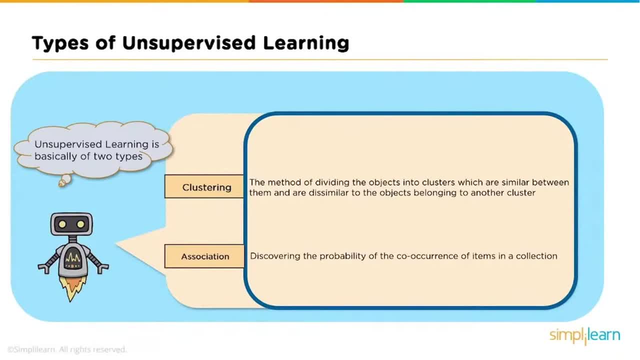 large datasets, For example, which customer made similar product products. Here the machine identifies patterns from the given set and groups them based on the behavior of the data. Thanks for listening. and from the end of day 13 we come to closing ClusteringAdvantages. 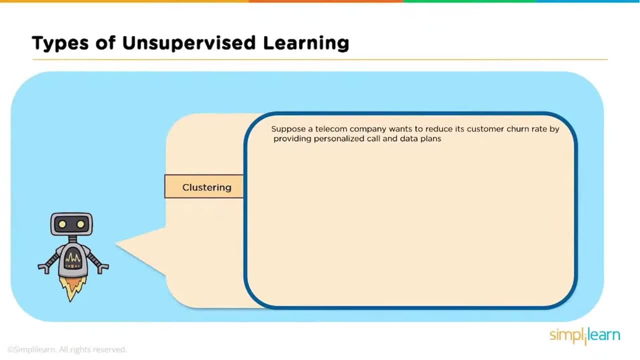 Reducing e-churn combined era To reduce their churn rate. A telecom company studies the behavior of the customers based on average call duration and internet usage and observes that while some customers' call duration is quite high, others have heavy internet usage. The customers are grouped based on their observed behavior and a strategy is adopted to minimize. 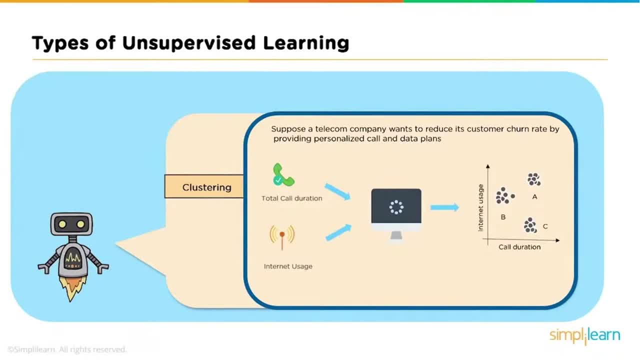 the tricks: minimized churn rate and maximized profit via suitable promotions and campaigns. As you can see in the chart on the right hand side, customers in Group A uses more data and also have high call duration. Group B customers are heavy internet users, while Group 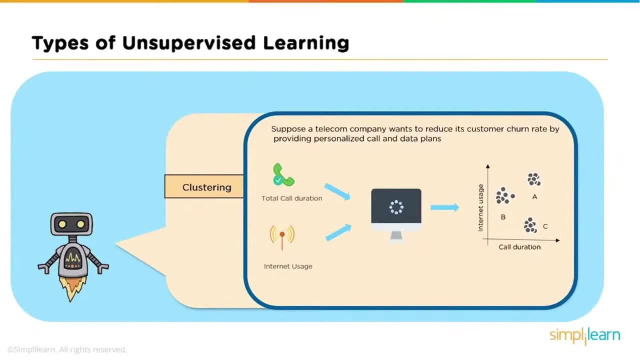 C customers have high call duration. So Group B will be given more data benefit plans, while Group C will be given cheaper call rates to buy their loyalty. So this was the example of clustering. Now let's understand association with another example. Let's say customer 1 goes to a supermarket. 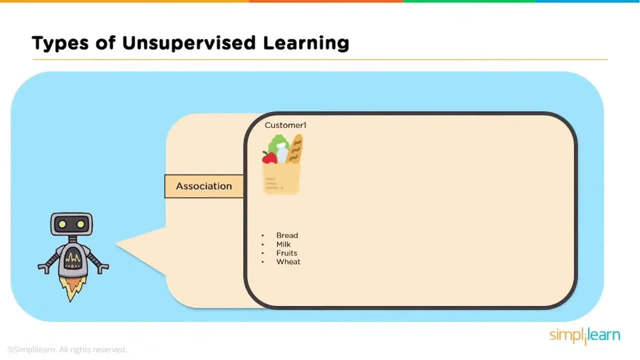 and buys these products- say bread, milk, fruits, wheat- Then customer 2 goes and buys bread, milk, rice and butter. Now, when customer 3 goes and buys bread, it is highly likely that he will also buy milk. Hence relationship is established based on customer behaviour, and recommendations are. 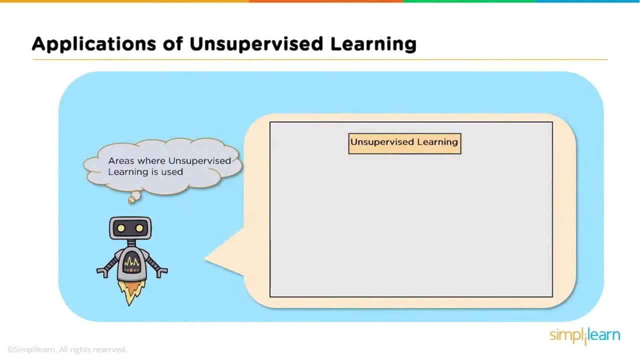 made. Now let's look at some real-life applications of unsupervised learning. Market basket analysis is a machine learning model based on the algorithm that if you buy a certain group of items, you are less or more likely to buy another group of items. 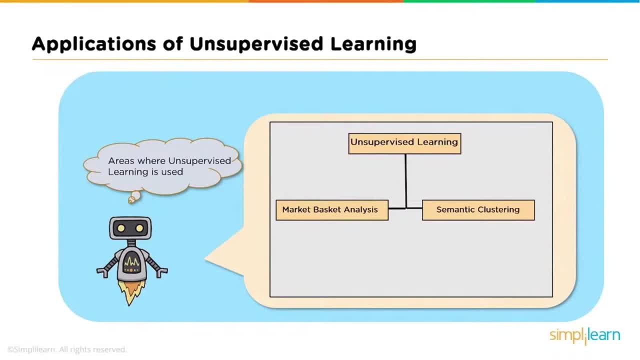 Semantic clustering: Semantically, similar words share similar contexts. People post their queries on websites in their own ways. Semantic clustering groups all responses in a cluster with same meaning to ensure that the customer finds the information they want quickly and easily. It plays an important role in information retrieval, good browsing experience and comprehension. 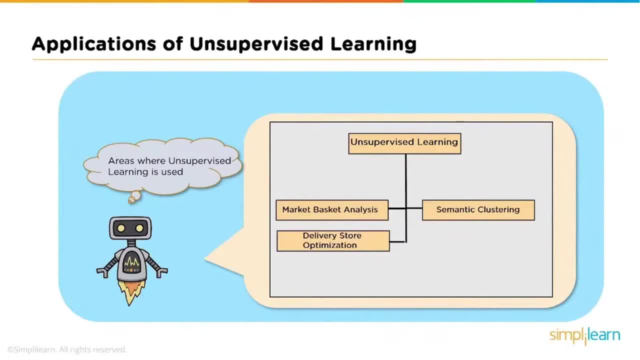 Delivery store optimization. Machine learning models are used to predict the demand and keep up with the supply, Also to open stores where demand is more and optimizing routes for more efficient deliveries according to past data and behaviour. We can also use unsupervised machine learning models to identify accident-prone areas based 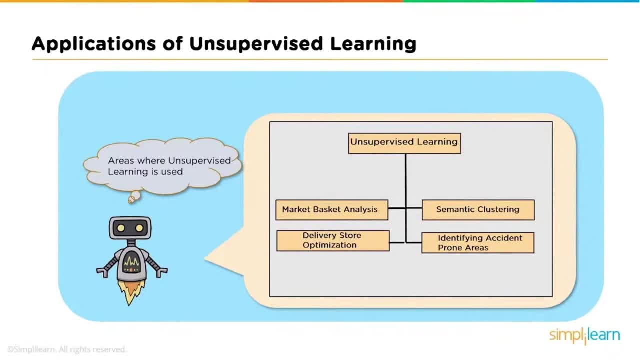 on the intensity of those accidents and the area in order to introduce success. So in this example, we can use unsupervised machine learning models to identify accident-prone areas based on the intensity of those accidents and the area in order to introduce success. 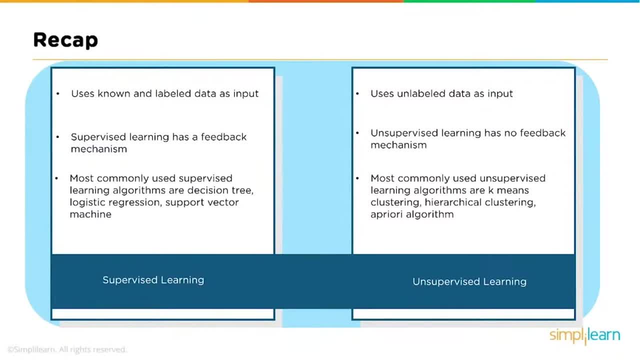 safety measures. by now i hope you've understood supervised and unsupervised learning. for a quick recap, let's see a few differences between the two. the most fundamental difference is that supervised learning uses known and label data and unsupervised learning uses unlabeled data as their input. 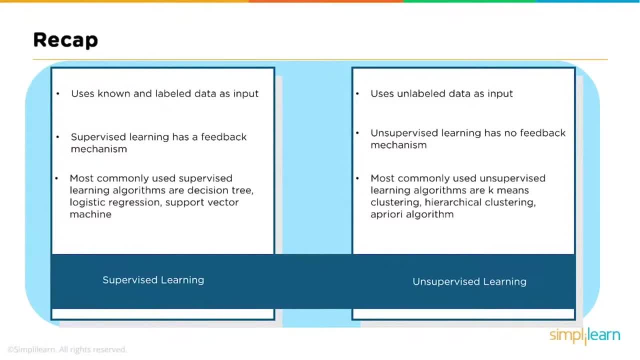 secondly, supervised learning follows a feedback mechanism, while unsupervised learning does not. also, the most commonly used algorithms in supervised learning are decision tree, logistic regression, support vector machine, etc. and in unsupervised learning there k-means clustering, hierarchical clustering, a priori algorithm and many more. welcome to linear regression. my name is richard kirschner. 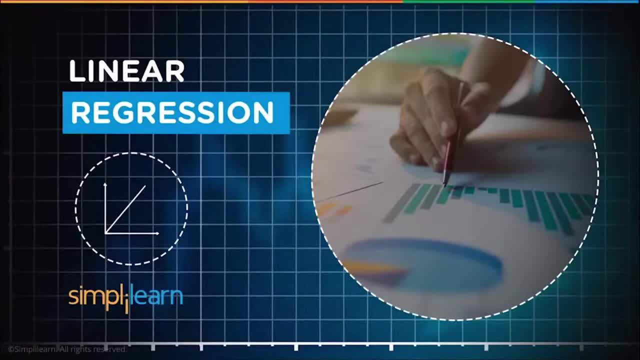 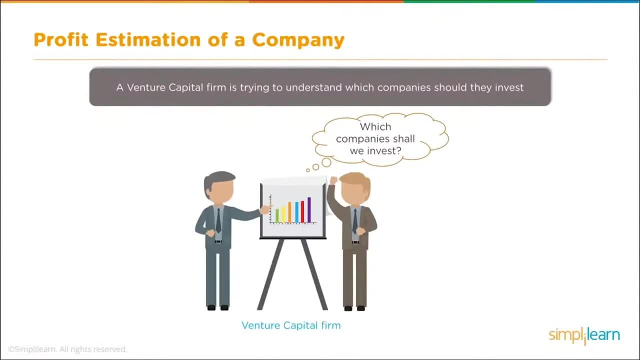 i'm with, simply learn. let's look at an example of a common use for linear regression profit estimation of a company. if i was going to invest in a company, i would like to know how much money i could expect to make. so we'll take a look at a venture capitalist firm. 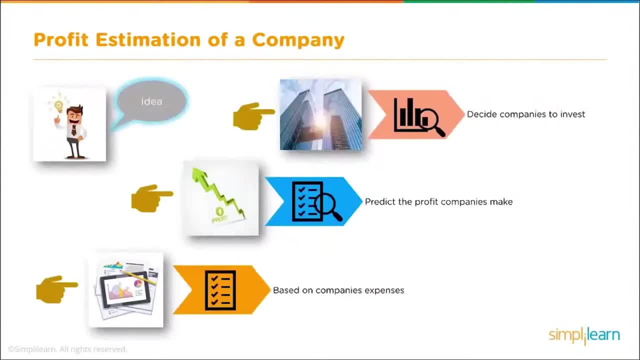 and try to understand which companies they should invest in. so we'll take the idea that we need to decide the companies to invest in. we need to predict the profit the company makes, and we're going to do it based on the company's expenses, and even just a specific expense in this. 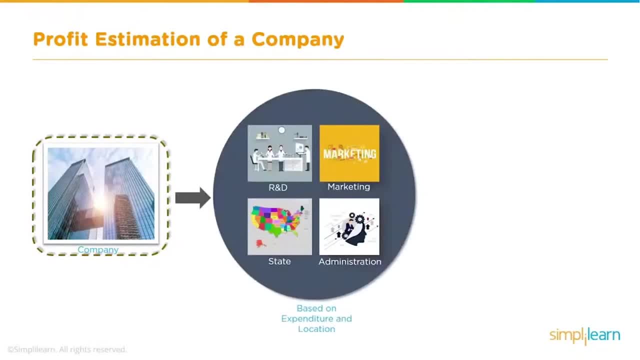 case, we have our company. we have the different expenses. so we have our r? d, which is your research and development. we have our marketing. we might have the location. we might have what kind of administration is going through? based on all this different information, we would like to 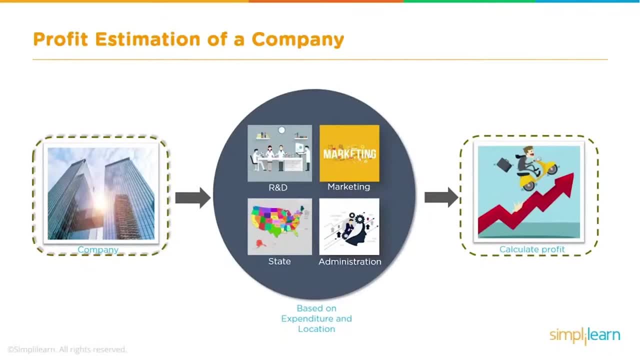 calculate the profit now. in actuality, there's usually about 23 to 27 different markers that they look at if they're a heavy duty investor. we're only going to take a look at one basic one. we're going to come in and, for simplicity, let's consider a single variable: r d. 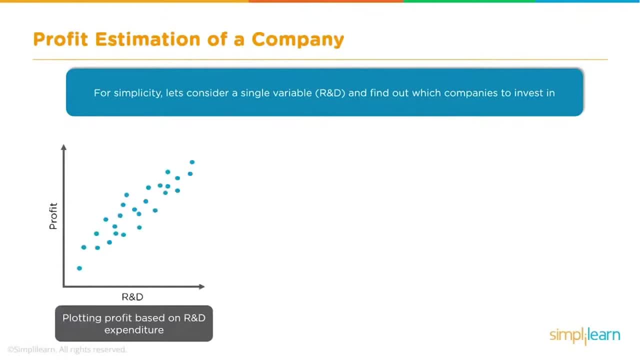 and find out which companies to invest in based on that. so we take our r? d, we're plotting the profit based on the r? d expenditure- how much money they put into the research and development, and then we look at the profit that goes with that. we can predict a line to estimate the. 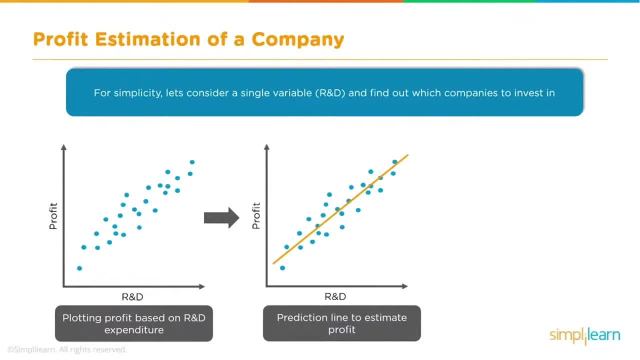 profit. so we draw a line right through the data. when you look at that, you can see how much they invest in the r? d is a good marker as to how much profit they're going to have. we can also note that companies spending more on r d. 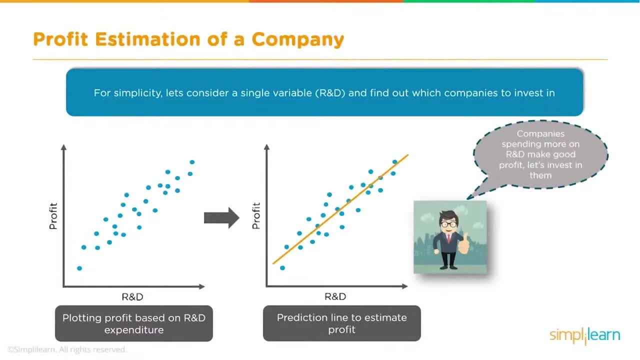 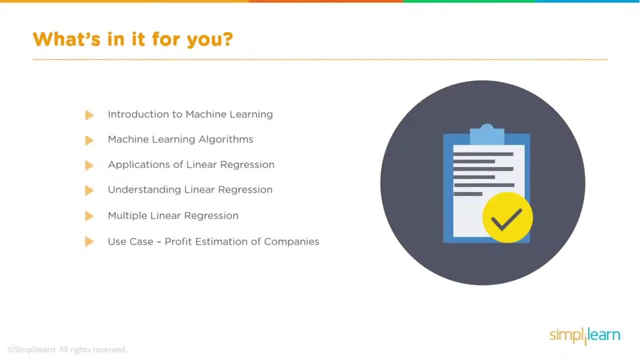 make good profit, so let's invest in the ones that spend a higher rate in their r? d. what's in it for you? first, we'll have an introduction to machine learning, followed by machine learning algorithms. these will be specific to linear regression and where it fits into the 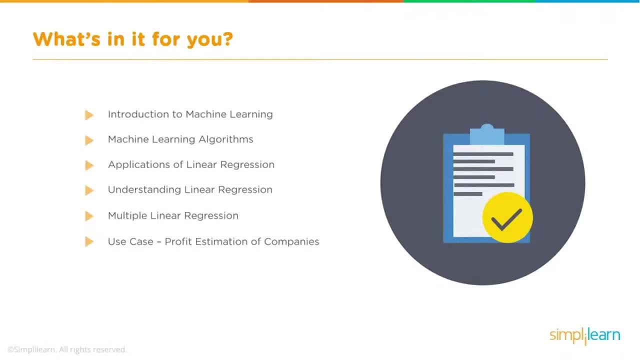 larger model. then we'll take a look at applications of linear regression, as in rumaha, computer programming, money management. alphastar went down higher. college went up higher, always. this cliff rise becomes axel confederate. enough for me each case. so the answer is yeah. we expressed it vertically in our 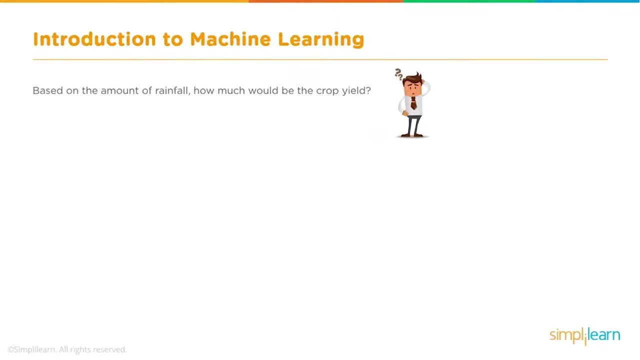 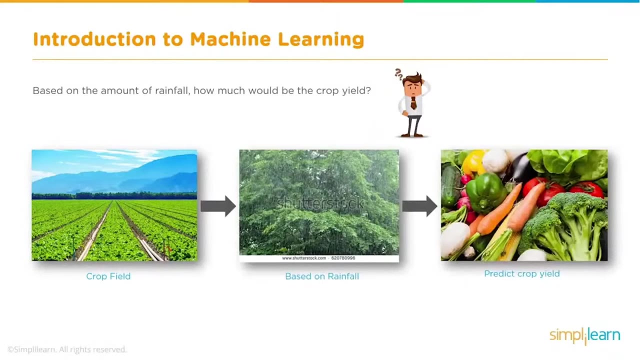 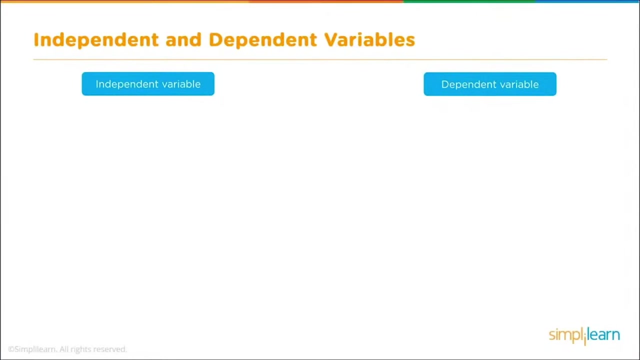 business rates are duly important, and one of the things that gives us an advantage over what others do is: you take a look underneath our comparison strategy and what goes out of the box is how much profit we make or how much we could make from fish year. So we're going to introduce two variables: independent and dependent. The independent variable: 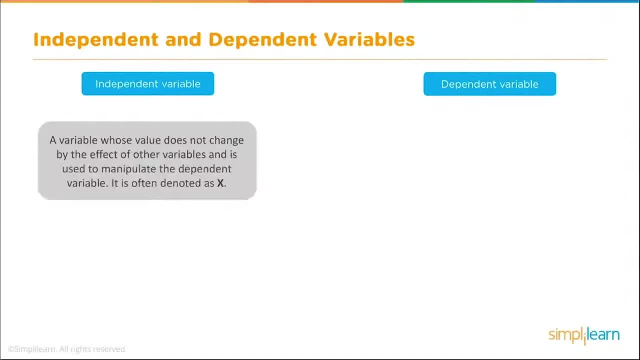 is a variable whose value does not change by the effect of other variables and is used to manipulate the dependent variable. It is often denoted as x. In our example, rainfall is the independent variable. This is a wonderful example, because you can easily see that we can't control. 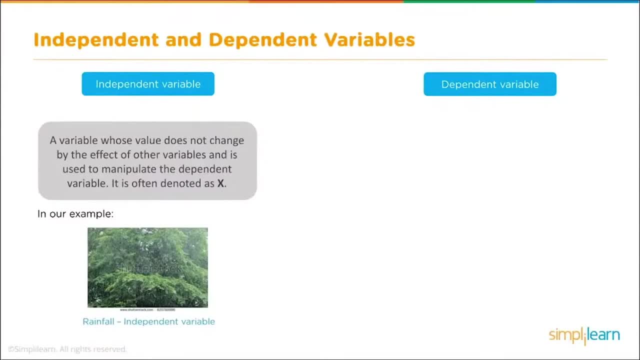 the rain, but the rain does control the crop. So we talk about the independent variable controlling the dependent variable. Let's define dependent variable as a variable whose value change. when there is any manipulation of the values of the independent variables, It is often denoted: 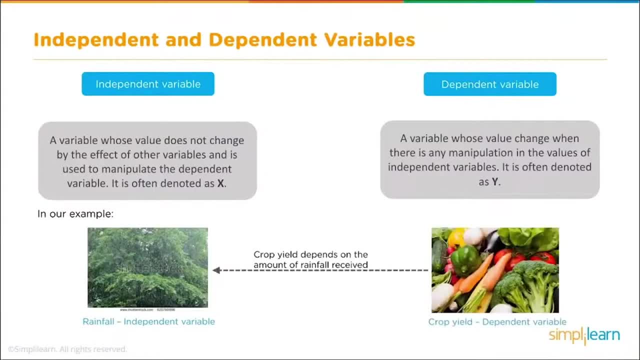 as y, And you can see here our crop yield is dependent variable and it is dependent on the amount of rainfall received. Now that we've taken a look at a real life example, let's go a little bit into the theory and some definitions on machine learning and see how that fits together. 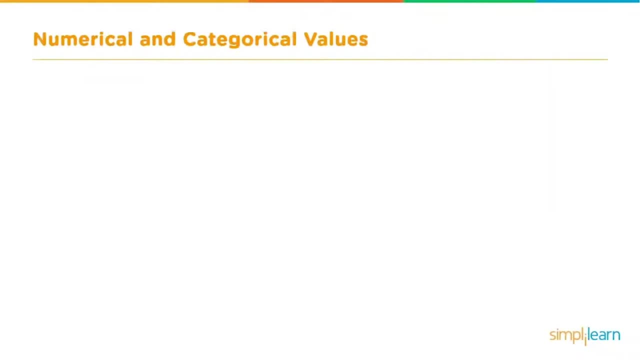 with linear regression, Numerical and categorical values. Let's take our data coming in. This is kind of random data from any kind of project. We want to divide it up into numerical and categorical. So numerical is numbers- age, salary, height- where categorical would be. 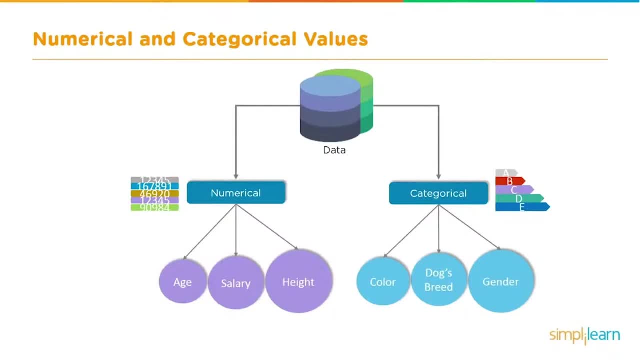 a description, the color a dog's breed, gender. Categorical is limited to very specific items, where numerical is a range of information. Now that you've seen the difference between numerical and categorical data, let's take a look at some different data. Let's take a look at some different data. Let's take a look at some. 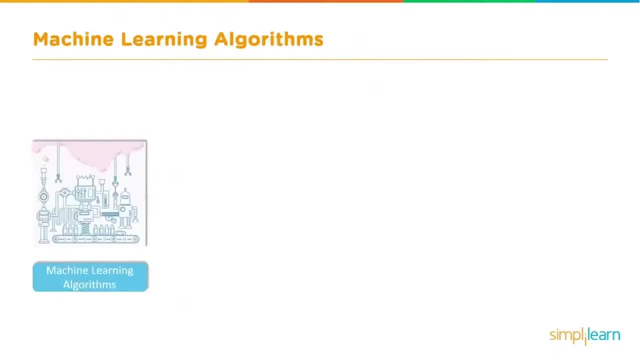 different machine learning definitions. When we look at our different machine learning algorithms, we can divide them into three areas: Supervised, unsupervised, reinforcement. We're only going to look at supervised today. Unsupervised means we don't have the answers. 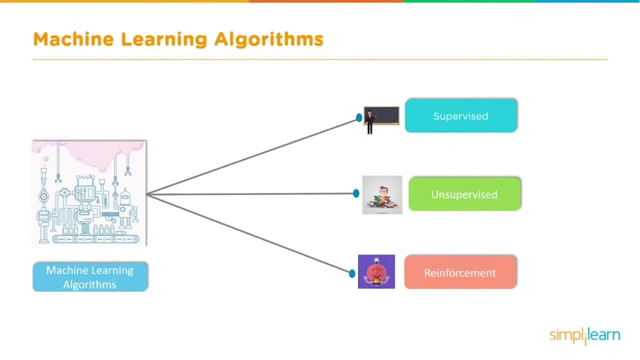 and we're just grouping things. Reinforcement is where we give positive and negative feedback to our algorithm to program it, and it doesn't have the information until after the fact. But today we're just looking at supervised, because that's where linear regression fits in In the 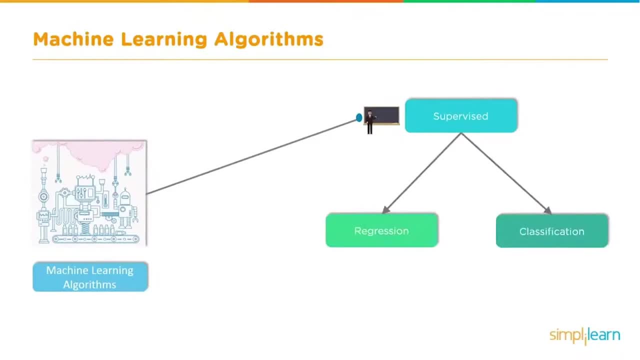 supervised data. we have our data already there and our answers for a group and then we use that to program our model and come up with an answer. The two most common uses for that is through the regression and classification. Now we're doing linear regression, so we're just going to focus on 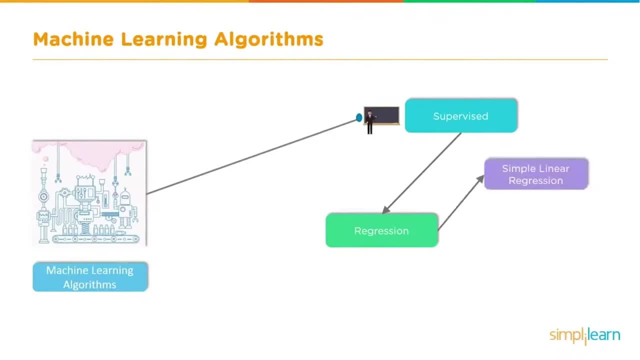 the regression side, And in the regression we have simple linear regression, we have multiple linear regression and we have polynomial linear regression. Now, on these three, simple linear regression is the examples we've looked at so far, where we have a lot of data and we draw a straight line through it. Multiple linear regression means: 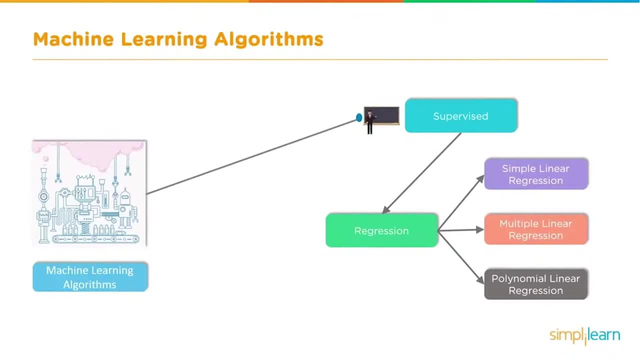 we have multiple variables. Remember where we had the rainfall and the crops. We might add additional variables in there, like how much food do we give our crops? When do we harvest them? Those would be additional information add into our model and that's why it'd be multiple linear. 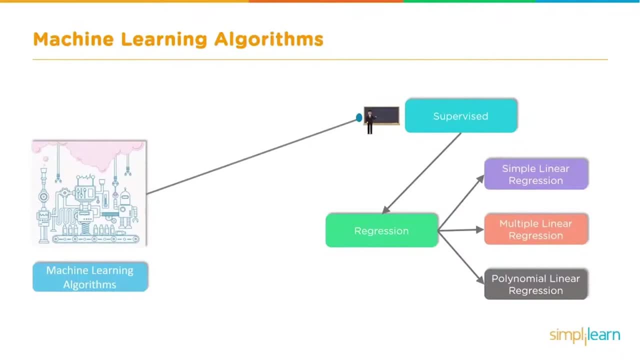 regression. And finally, we have polynomial linear regression. That is, instead of drawing a line, we can draw a curved line through it. Now that you see where regression model fits into the machine algorithm and we're specifically looking at linear regression, let's go ahead and take a look. 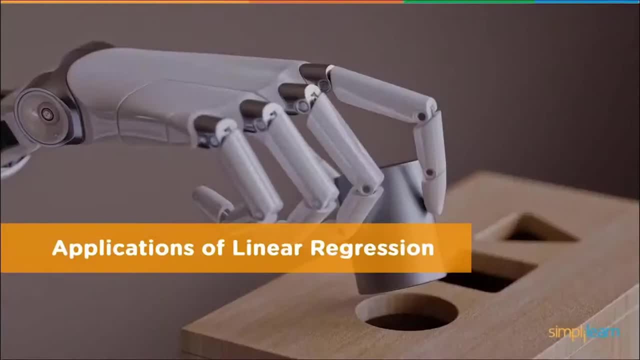 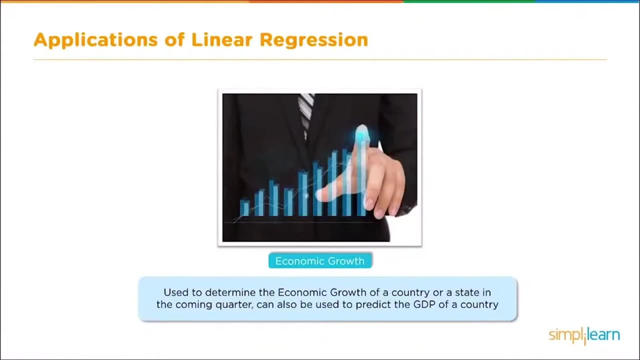 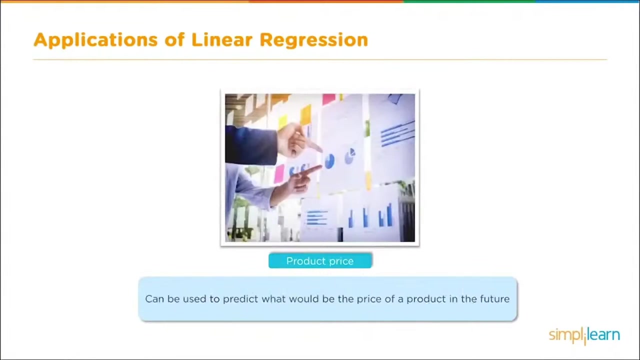 at applications for linear regression. Let's look at a few applications of linear regression. Economic growth used to determine the economic growth of a country or a state in the coming quarter. can also be used to predict the GDP of a country. Product price can be used to predict. 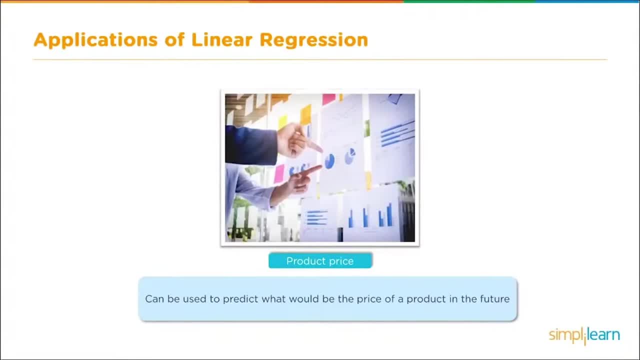 what would be the price of a product in the future. We can guess whether it's going to go up or down, or should I buy it today? Housing sales to estimate the number of houses a builder would sell and what price in the coming months. 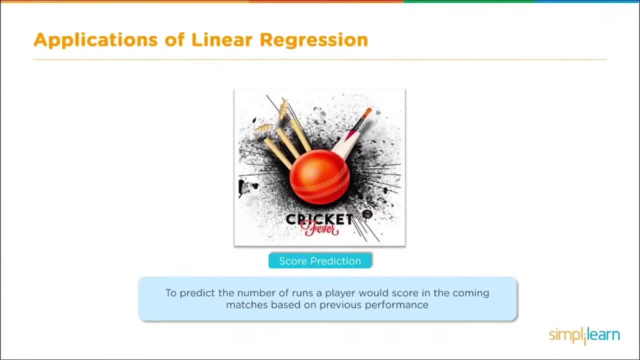 Score predictions- cricket fever- to predict the number of runs a player would score in the coming matches based on the previous performance. I'm sure you can figure out other applications you could use linear regression for. So let's jump in and let's understand linear regression and 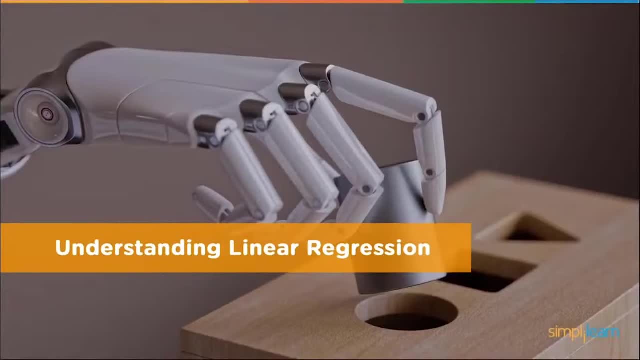 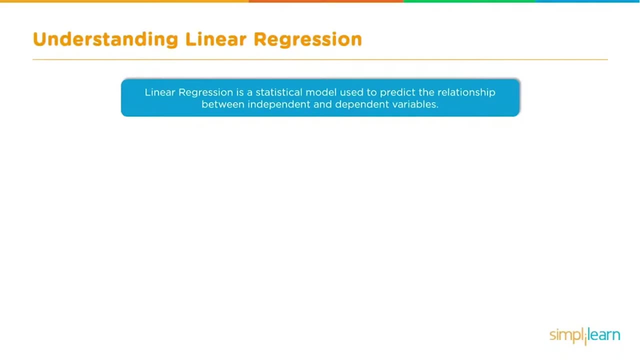 dig into the theory Understanding linear regression. Linear regression is the statistical model used to predict the relationship between independent and non-independent houses. Linear regression is a method of measuring the relationship between independent and dependent variables by examining two factors. The first, important one is which variables in particular? 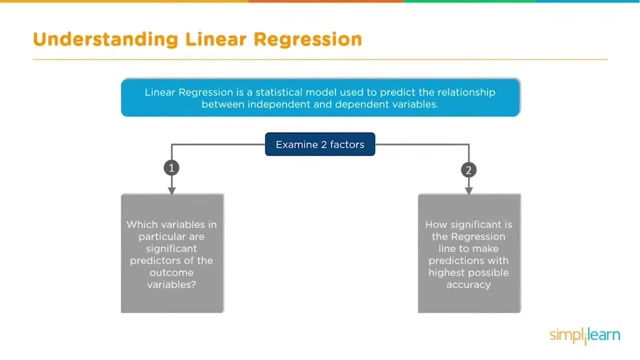 are significant predictors of the outcome variable. And the second one that we need to look at closely is how significant is the regression line to make predictions with the highest possible accuracy. If it's inaccurate, we can't use it, So it's very important we find out the most accurate line. we 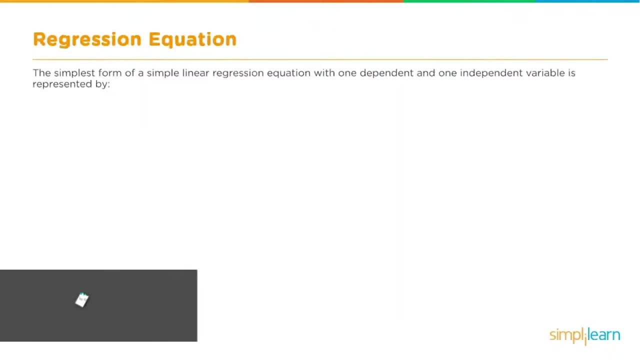 can get. Since linear regression is based on drawing a line through data, we can't use it. So let's go back and take a look at some Euclidean geometry, The simplest form of a simple linear regression equation with one dependent and one independent. 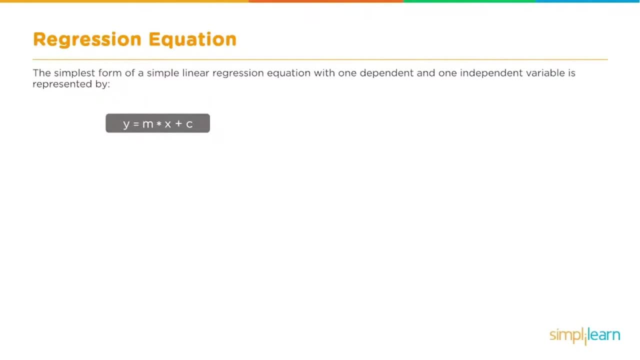 variable is represented by. y equals m times x plus c. And if you look at our model here, we plotted two points on here: x1 and y1,, x2 and y2, y being the dependent variable- remember that from before- and x being the independent variable. So y depends on whatever. 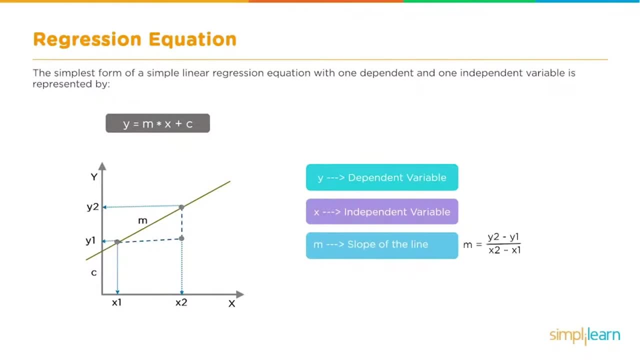 the dependent variable is So m, in this case, is the slope of the line, where m equals the difference in the y2 minus y1 and x2 minus x1. And finally we have c, which is the coefficient of the line, or where it happens to cross the zero axes. Let's go back and look at an example we used earlier of 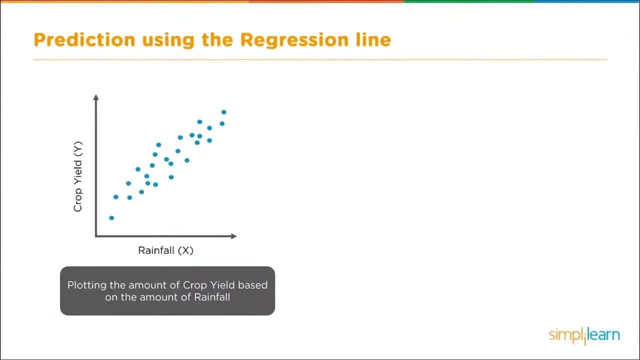 linear regression. We're going to go back to plotting the amount of crop yield based on the amount of rainfall, And here we have our rainfall And we have our crop yield, which is dependent on the rainfall. So we have our independent and our 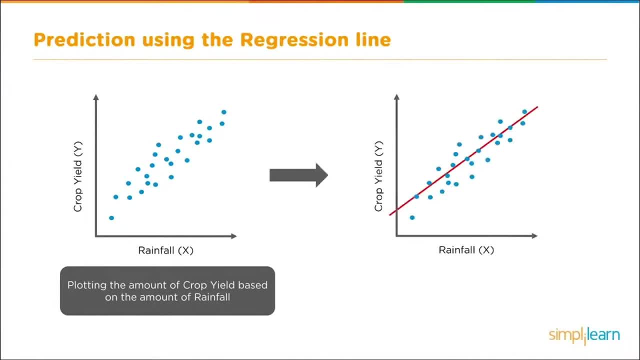 dependent variables. We're going to take this and draw a line through it, as best we can through the middle of the data, And then we look at that. we put the red point on the y-axis is the amount of crop yield you can expect for the amount of rainfall represented by the green dot. So if 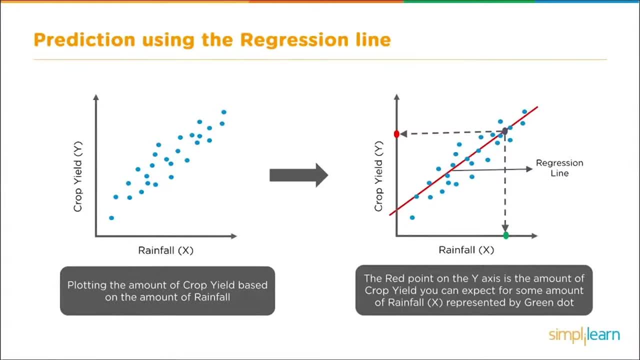 we have an idea what the rainfall is for this year and what's going on, then we can guess how good our crops are going to be. And we've created a nice line right through the middle to give us a nice mathematical formula. Let's take a look and see what the math looks like behind this. Let's look at. 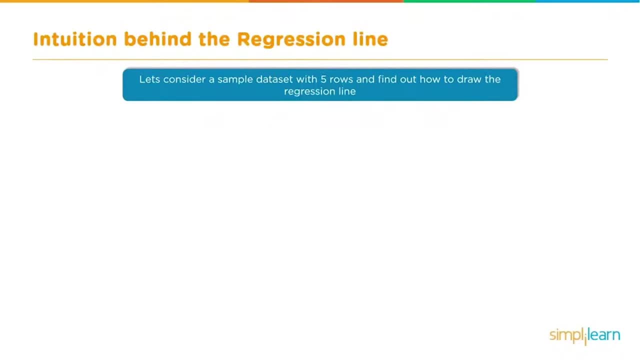 the intuition behind the regression line. Now, before we dive into the math and the formulas that go behind this and what's going on behind the scenes, I want you to note that when we get into the case study and we actually apply some Python script, that this math you're going to see. 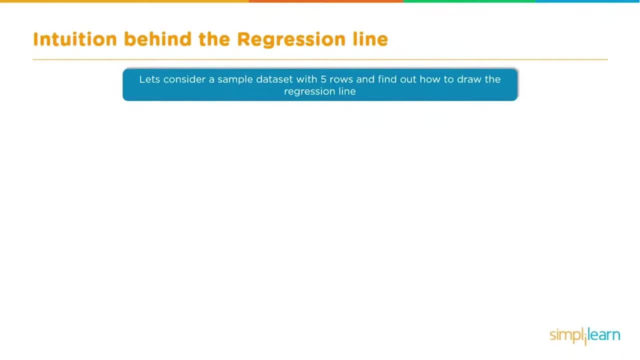 here is already done automatically for you. You don't have to have it memorized. It is, however, that you're going to be able to see what's going on, So if people reference the different terms, you'll know what they're talking about. Let's consider a sample data set with five rows and find: 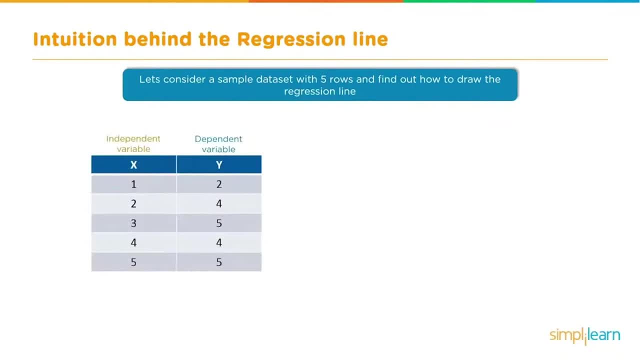 out how to draw the regression line. We're only going to do five rows because if we did like the rainfall with hundreds of points of data, that would be very hard to see what's going on with the mathematics. So we'll go ahead and create our own two sets of data And we have our independent. 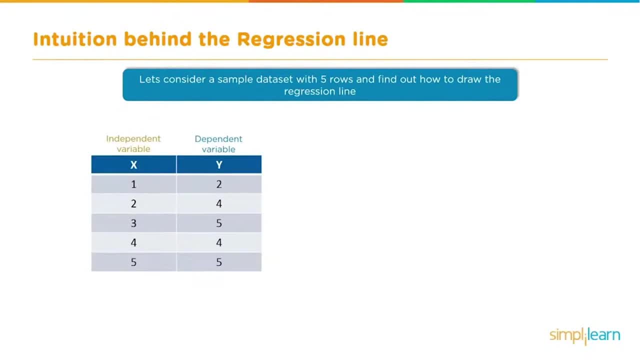 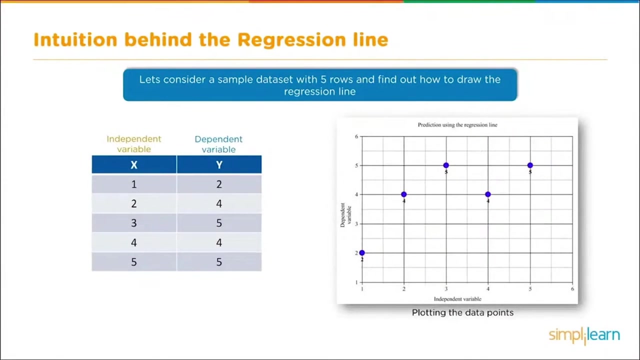 variable x and our dependent variable y, And when x was one we got y equals two, And x was two, y was four, and so on and so on. If we go ahead and plot this data on a graph, we can see how it forms a nice line. through the middle. You can see where it's kind of grouped. 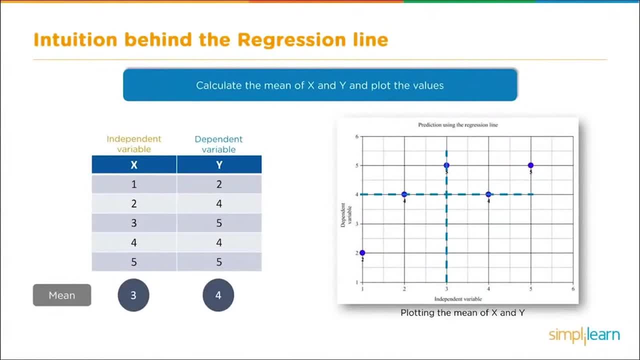 going upwards to the right. The next thing we want to know is what the means is of each of the data coming in the x and the y. The means doesn't mean anything other than the average. So we add up all the numbers and divide by the total. So one plus two plus three plus four plus five over five. 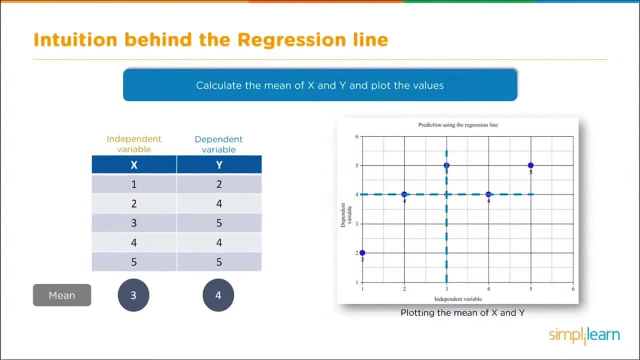 is three And the same for y, we get four. If we go ahead and plot the means on the graph, we'll see we get three comma four, which draws a nice line down the middle, A good estimate Here. we're going to dig deeper into the math behind the regression line. Now remember before: 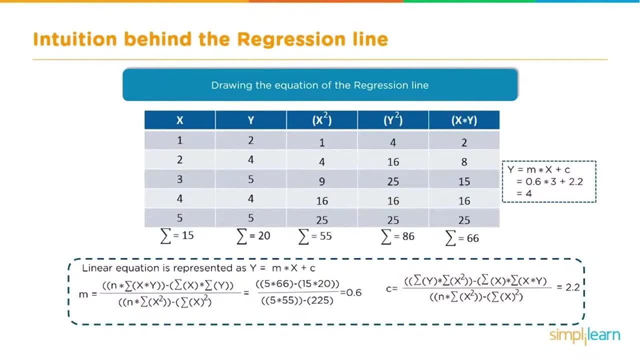 I said, you don't have to have all these formulas memorized or fully understand them, even though we're going to go into a little more detail of how it works. And if you're not a math whiz and you don't know, if you've never seen the sigma character before, which looks a little bit like. 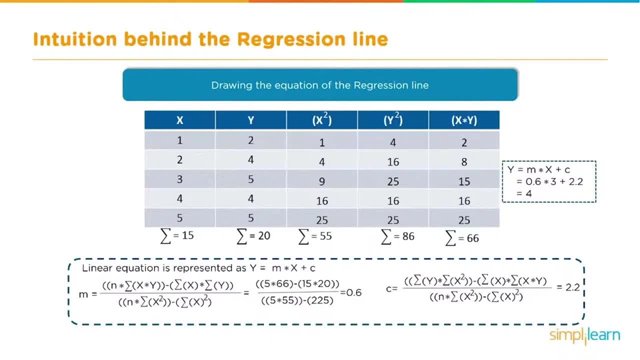 an e that's opened up. that just means summation. That's all that is. So when you see the sigma character, it just means we're adding everything in that row. And for computers this is great because as a programmer you can easily iterate through each of the xy points and create all the 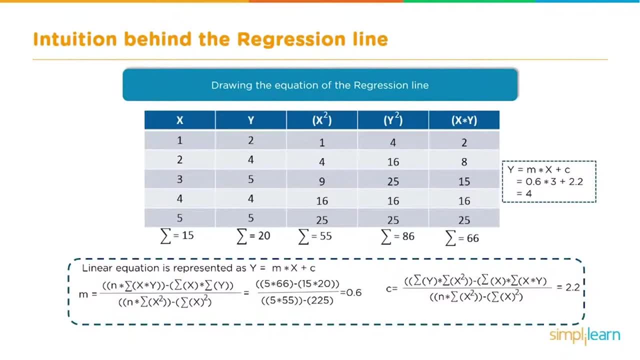 information you need. So in the top half you can see where we've broken that down into pieces. And as it goes through the first two points, it computes the squared value of x, the squared value of y and x times y, And then it takes all of x and adds them up all of y. 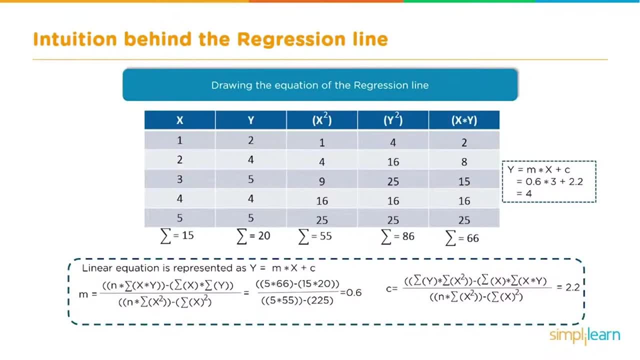 adds them up, all of x squared adds them up, and so on and so on, And you can see we have the sum of equal to 15, the sum is equal to 20, all the way up to x times y, where the sum equals 66.. 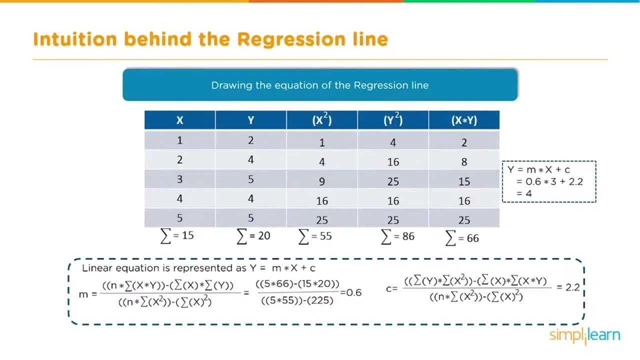 This all comes from our formula for calculating a straight line, where y equals the slope times, x plus the coefficient c. So we go down below and we're going to compute more like the averages of these And we'll explain exactly what that is in just a minute and where that information comes. 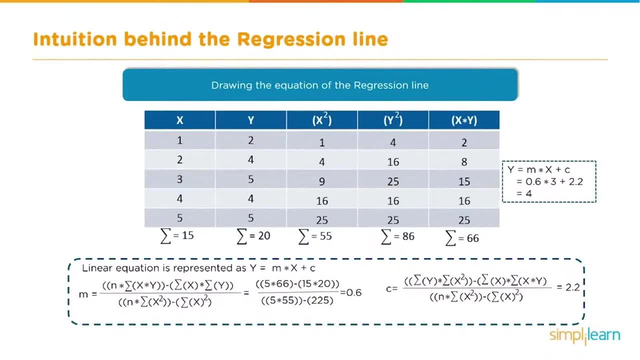 from. It's called the square-means equation, And we're going to do that in detail in a few minutes. All you need to do is look at the formula and see how we've gone about computing it line by line, instead of trying to have a huge 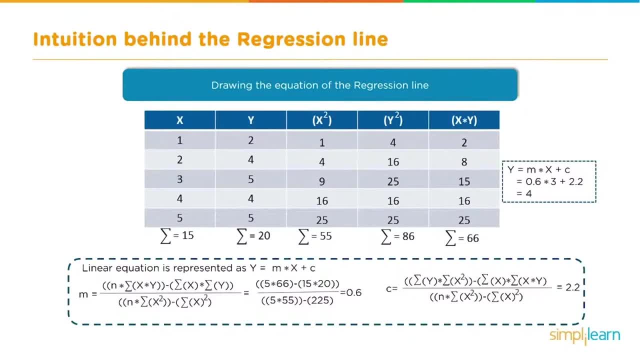 set of numbers pushed into it And down here you'll see where the slope m equals. and in the top part, if you read through the brackets, you have the number of data points times the sum of x times y, which we computed one line at a time there, and that's just the 66. And take 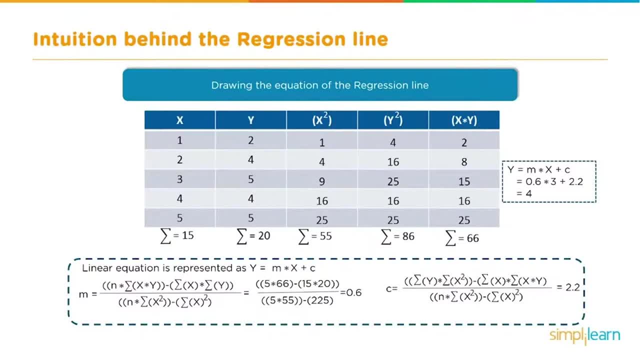 all that and subtract it from the sum of x times the sum of y, And those have both been computed, So you have 15 times 20.. And on the bottom we have the number of lines times the sum of x squared, easily computed as 86 for the sum minus. I'll take all that and subtract the sum of x squared. 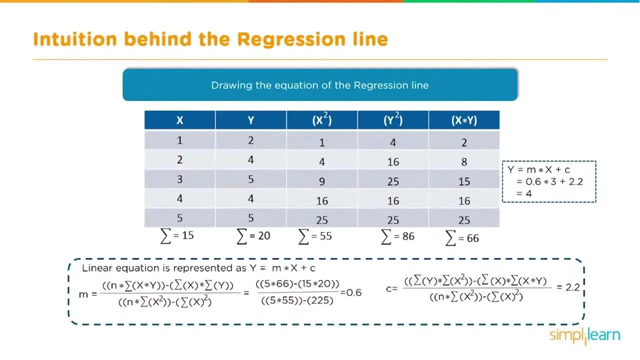 And we end up as we come across with our formula. you can plug in all those numbers, which is very easy to do in the computer- You don't have to do the math on a piece of paper or calculator- and you'll get a slope of 0.6, and you'll get your c-coefficient. 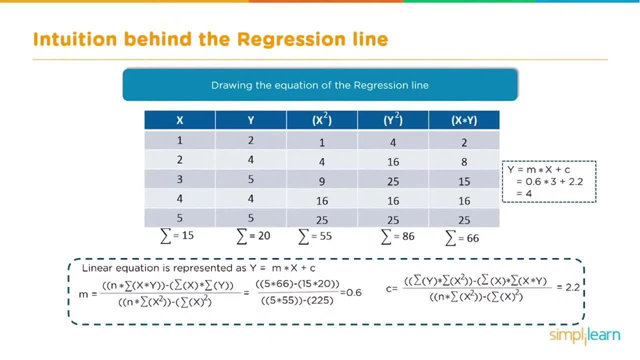 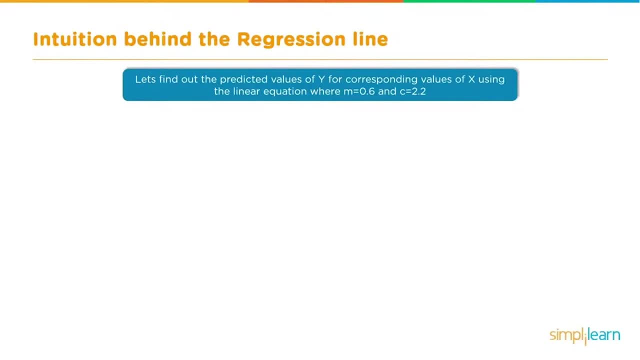 If you continue to follow through that formula, you'll see it comes out as equal to 2.2.. Continuing deeper into what's going behind the scenes, let's find out the predicted values of y for corresponding values of x using the linear equation, where m equals 0.6 and c equals 2.2.. 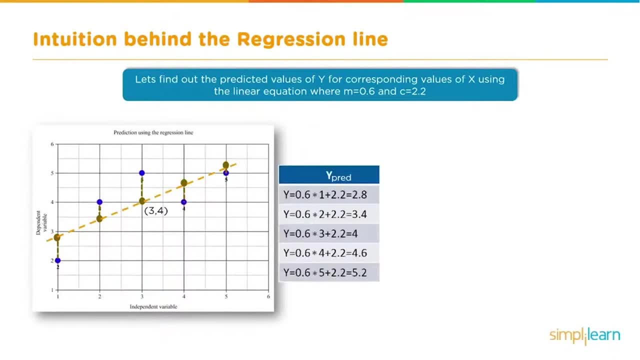 We're going to take these values and we're going to go ahead and plot them, We're going to predict them. so y equals 0.6 times where x equals 1, plus 2.2 equals 2.8, and so on and so on. 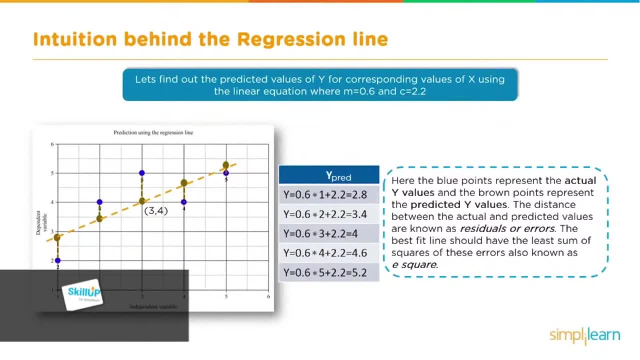 And here the blue points represent the actual y values and the brown points represent the predicted y values. based on the model we created, The distance between the actual and predicted values is known as residuals or errors. The best-fit line should have the least sum of squares of these errors, also known as e-square. 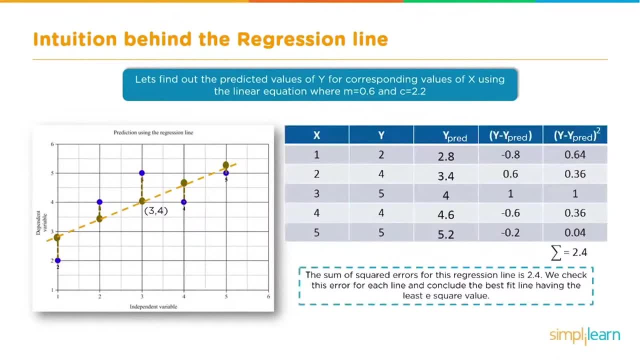 If we put these into a nice chart where you can see x and you can see y- what the actual values were, and you can see y predicted, you can easily see where we take y minus y predicted and we get an answer. 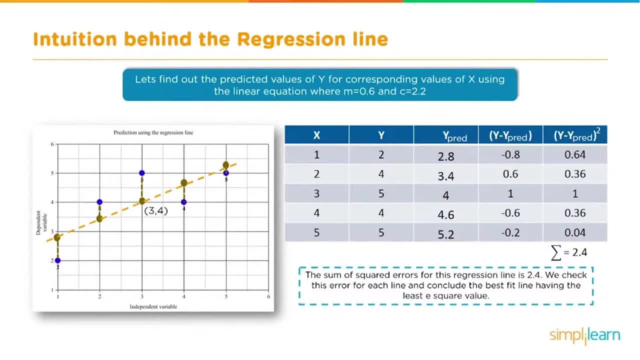 What is the difference between those two? And if we square that y minus y prediction squared, we can then sum those squared values. That's where we get the 0.64 plus the 0.36 plus 1,, all the way down until we have a summation equals 2.4.. 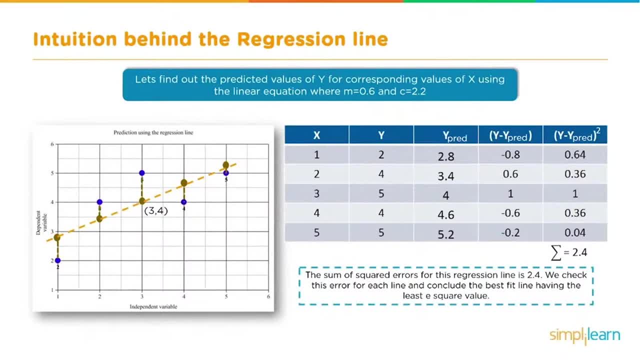 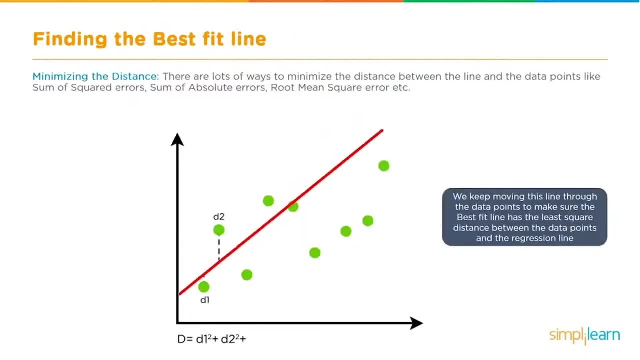 So the sum of squared errors for this regression line is 2.4.. We check that, We check this error for each line and conclude the best-fit line having the least e-square value In a nice graphical representation. we can see here where we keep moving this line through the data points. 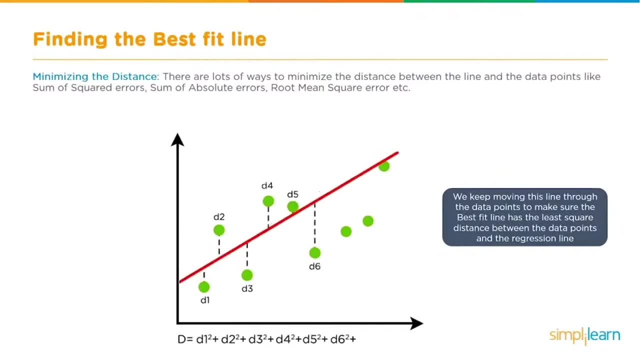 to make sure the best-fit line has the least squared distance between the data points and the regression line. Now we only looked at the most commonly used formula for minimizing the distance. There are lots of ways to minimize the distance between the line and the data points. 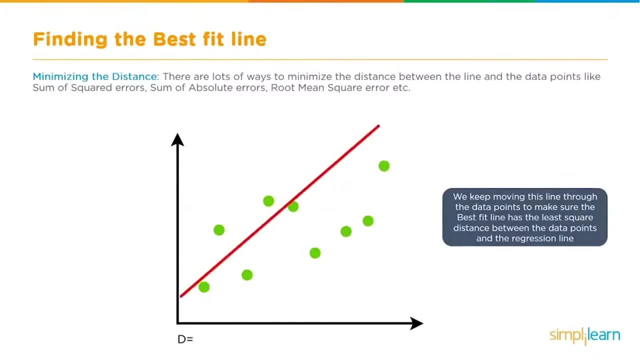 like sum of squared errors, sum of absolute errors, root mean square error, etc. What you want to take away from this is, whatever formula is being used, you can easily, using a computer programming and iterating through the data, calculate the different parts of it. 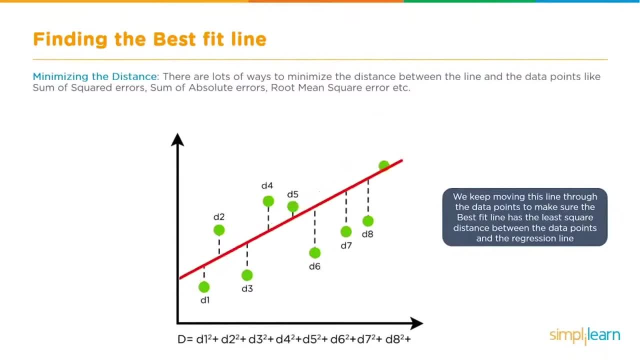 That way, these complicated formulas you see, with the different summations and absolute values, are easily computed one piece at a time. Up until this point we've only been looking at two values: x and y. Well, in the real world it's very rare that you only have two values. 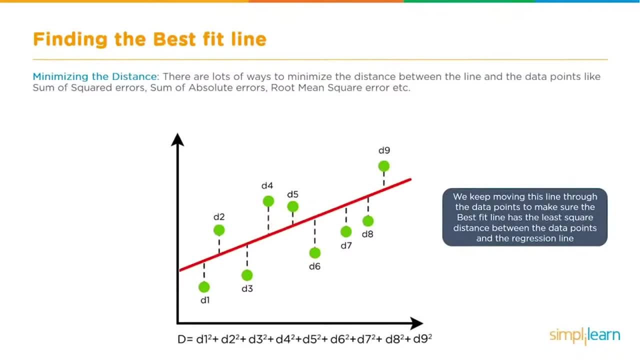 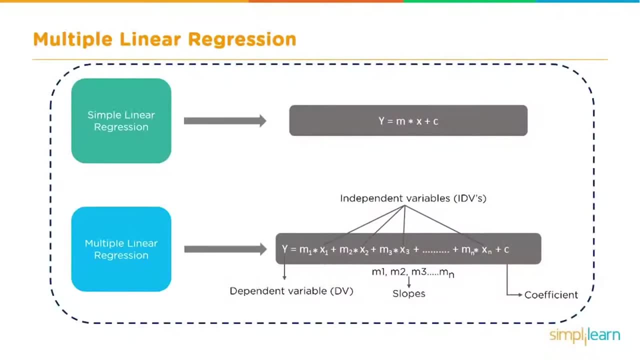 when you're figuring out a solution. So let's move on to the next topic, multiple linear regression. Let's take a brief look at what happens when you have multiple inputs. So in multiple linear regression we have. well, we'll start with the simple linear regression. 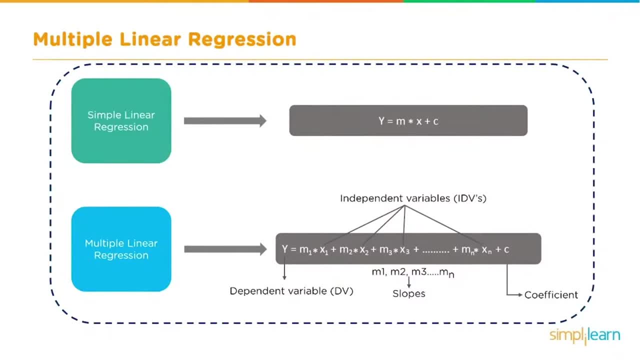 where we had y equals m plus x plus c, And we're trying to find the value of y. Now, with multiple linear regression, we have multiple variables coming in, So instead of having just x, we have x1,, x2, x3.. 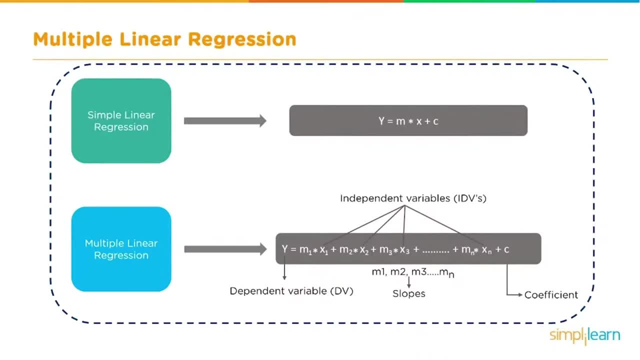 And instead of having just one slope, each variable has its own slope attached to it. As you can see, here we have m1, m2, m3. And we still just have the single coefficient. So when you're dealing with multiple linear regression, 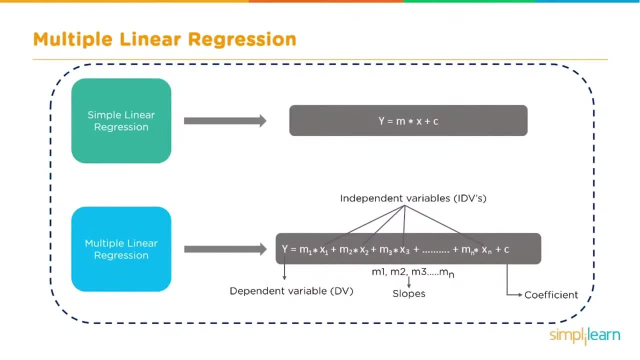 you basically take your single linear regression and you spread it out. So you have: y equals m1 times x1 plus m2 times x2, so on all the way to m to the nth, x to the nth, and then you add your coefficient on there. 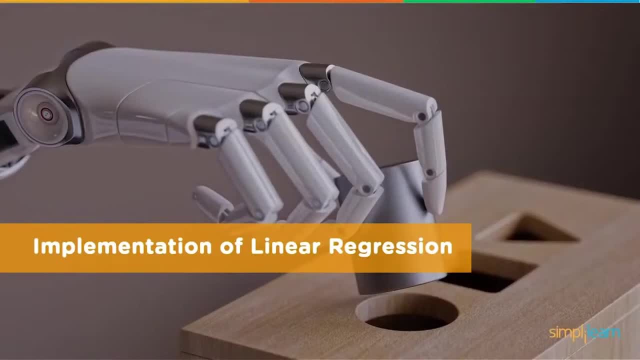 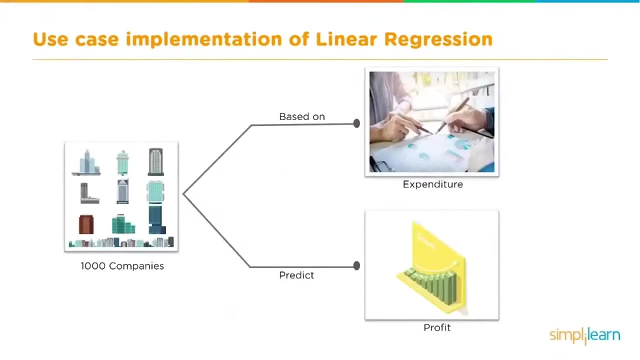 Implementation of linear regression. Now we get into my favorite part. Let's understand how multiple linear regression works by implementing it in Python. If you remember, before we were looking at a company and, just based on its R&D, trying to figure out its profit. 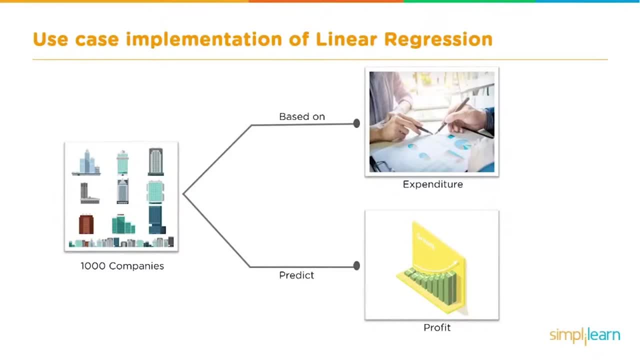 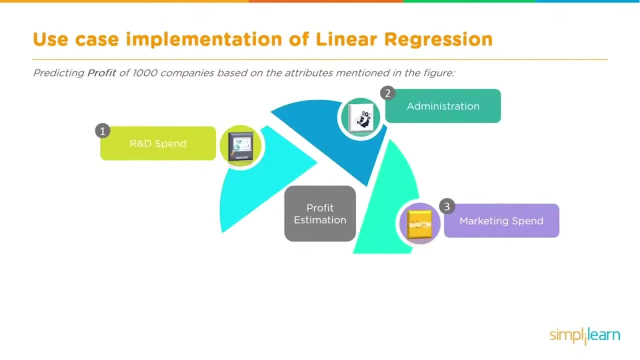 We're going to start looking at the expenditure of the company. We're going to go back to that. We're going to predict its profit, But instead of predicting it just on the R&D, we're going to look at other factors like administration costs, marketing costs and so on. 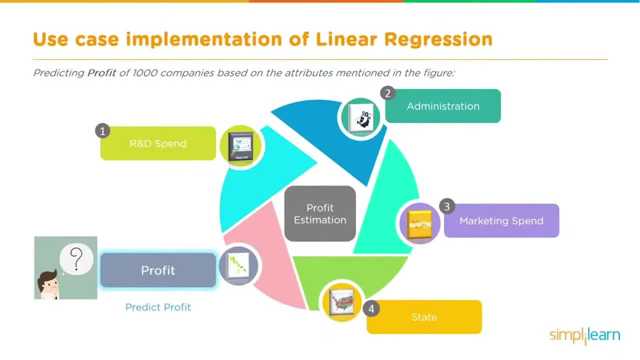 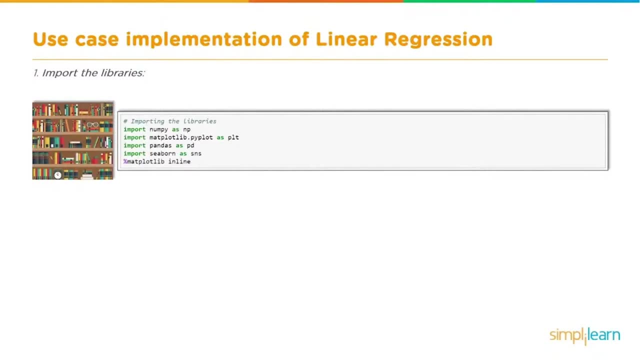 And from there we're going to see if we can figure out what the profit of that company is going to be. To start our coding, we're going to begin by importing some basic libraries And we're going to be looking through the data before we do any kind of linear regression. 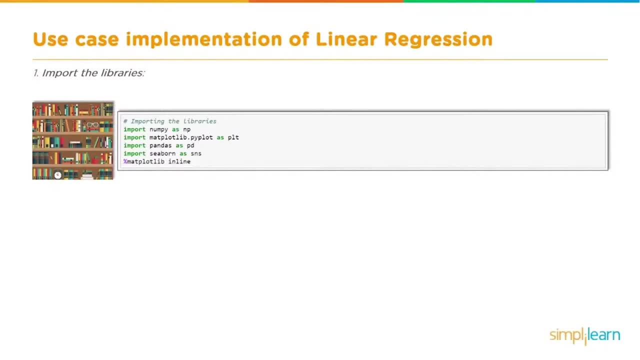 We're going to take a look at the data to see what we're playing with. Then we'll go ahead and format the data to the format we need to be able to run it in the linear regression model And then from there we'll go ahead and solve it and just see how valid our solution is. 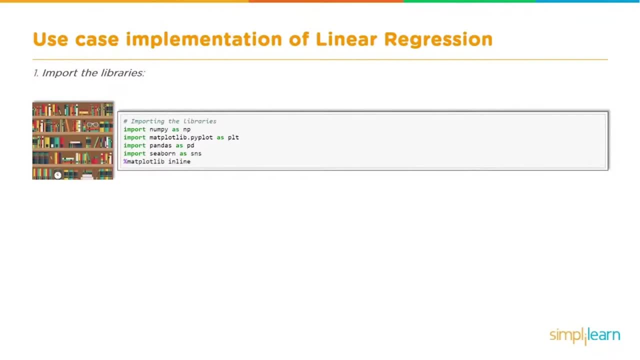 So let's start with importing the basic libraries. Now I'm going to be doing this in Anaconda Jupyter Notebook. It's a very popular IDE. I enjoy it because it's such a visual to look at and it's so easy to use. 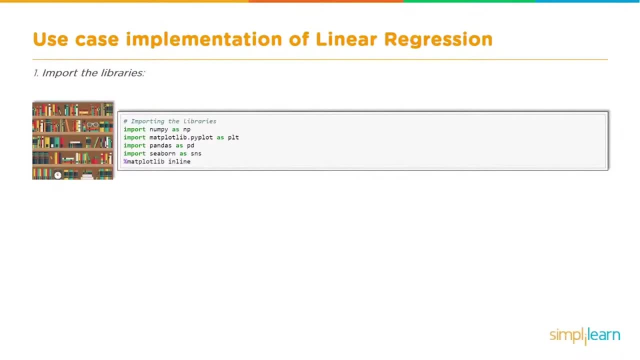 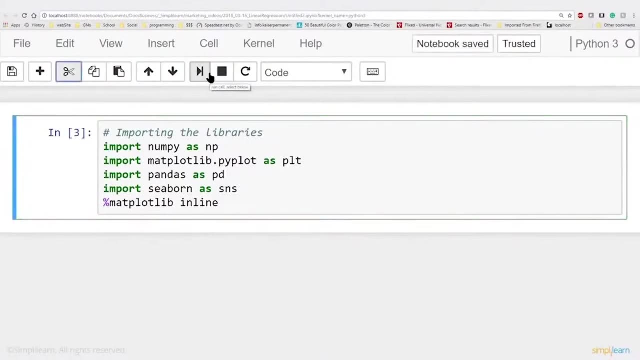 Just any IDE for Python will work just fine for this, So break out your favorite Python IDE. So here we are in our Jupyter Notebook. Let me go ahead and paste our first piece of code in there And let's walk through what libraries we're importing. 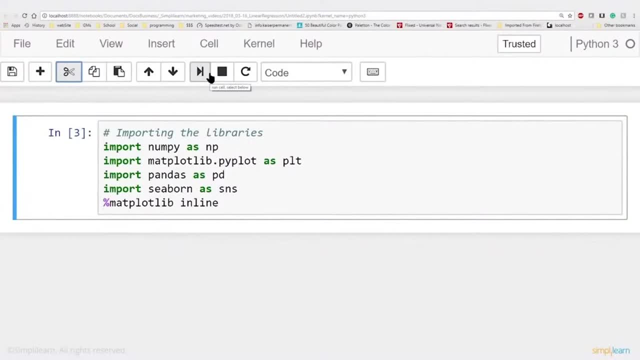 First we're going to import numpy as np And then I want you to skip one line and look at import pandas as pd. These are very common tools that you need with most of your linear regression. The numpy, which stands for number Python, is usually denoted as np. 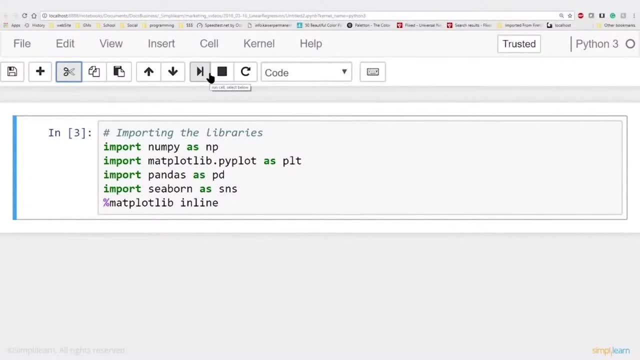 And you have to almost have that for your sklearn toolbox. You always import that right off the beginning, Pandas, although you don't have to have it for your sklearn libraries, it does such a wonderful job of importing data, setting it up into a data frame, so 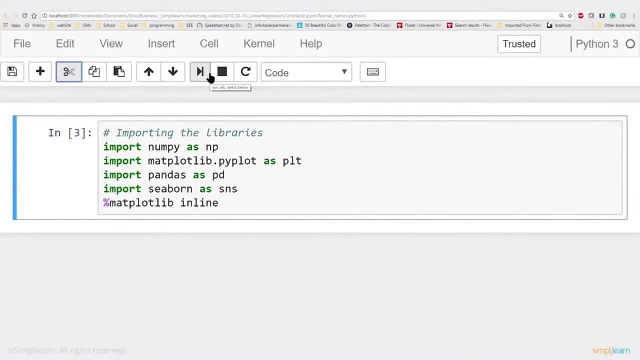 we can manipulate it rather easily and it has a lot of tools also in addition to that. So we usually like to use the pandas when we can, And I'll show you what that looks like. The other three lines are for us to get a visual of this data and take a look at it. 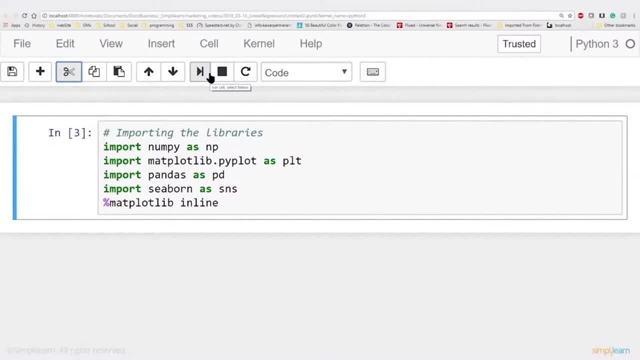 So we're going to import matplotlibrarypyplot as plt and then seaborn as sns. Seaborn works with the matplotlibrary, So you have to always import matplotlibrary and then seaborn sits on top of it, And we'll take a look at what that looks like. 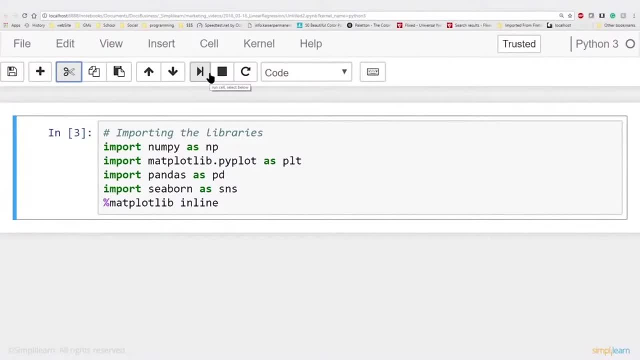 You could use any of your own plotting libraries you want. There's all kinds of ways to look at the data. These are just very common ones, And the seaborn is so easy to use that it just looks beautiful. It's a nice representation that you can actually take and show somebody. 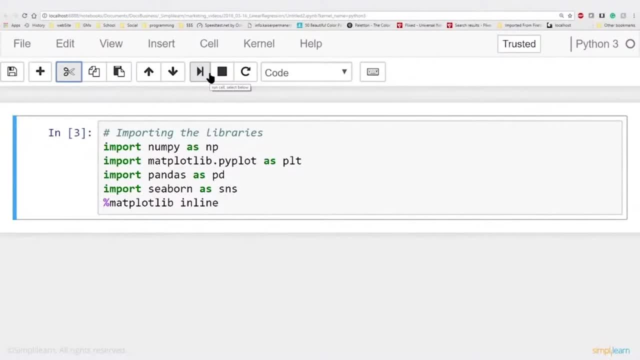 And the final line is the amber signed matplotlibrary inline. That is only because I'm doing an inline IDE. My interface in the Anaconda Jupyter Notebook requires I put that in there Or you're not going to see the graph when it comes up. 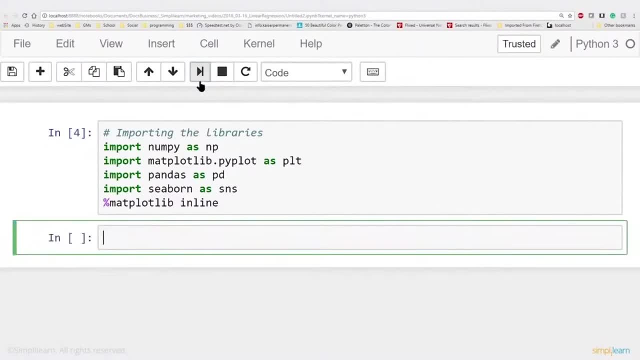 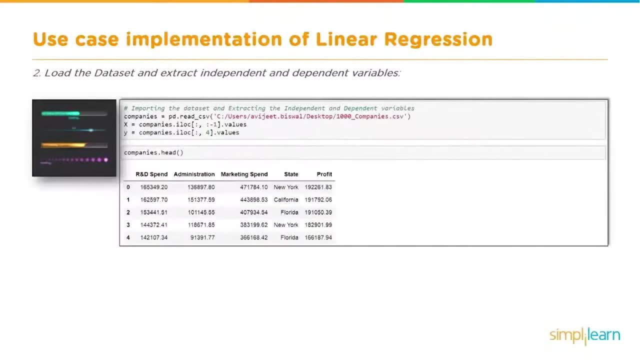 Let's go ahead and run this. It's not going to be that interesting, So we're just setting up variables. In fact, it's not going to do anything that we can see, But it is importing these different libraries and setup. The next step is load the dataset and extract independent and dependent variables. 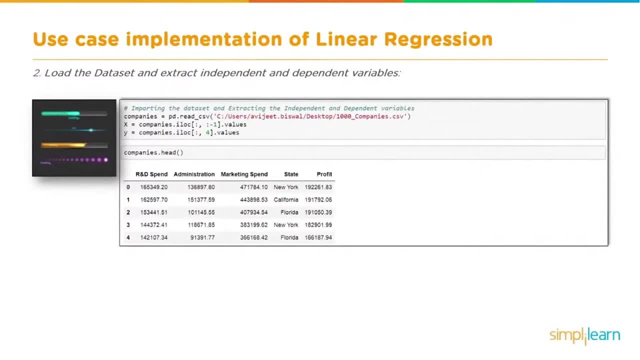 Now here in the slide you'll see companies equals PD dot read CSV And it has a long line there with the file at the end, 1000 companies dot CSV. You're going to have to change this to fit whatever setup you have in the file itself. 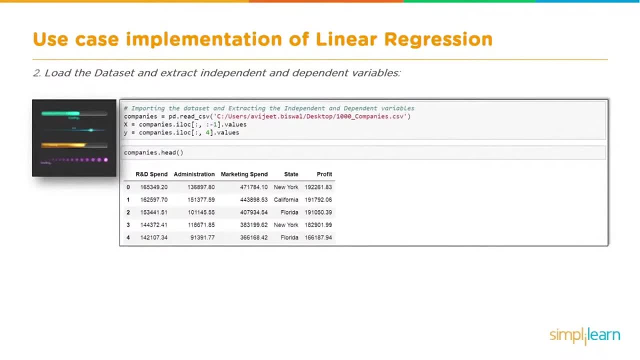 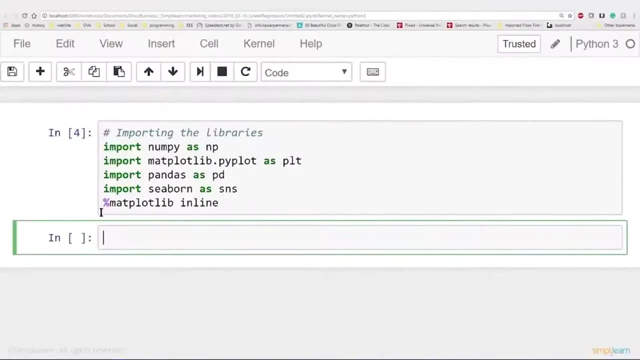 You can request. just go down to the commentary below this video and put a note in there and simply learn. will try to get in contact with you and supply you with that file so you can try this coding yourself. So we're going to add this code in here and we're going to see that I have 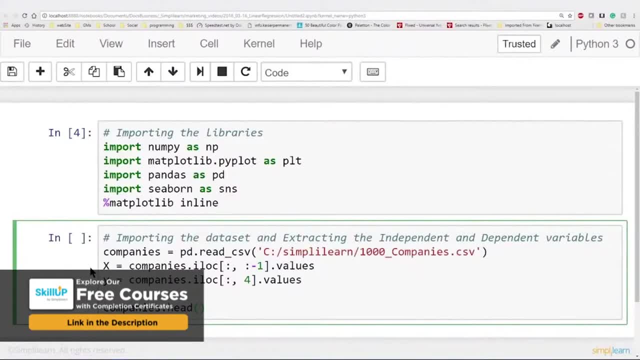 companies equals PD dot reader underscore CSV. And I've changed this path to match my computer, See colon slash. simply learn: slash 1000: underscore companies, dot CSV And then below there we're going to set the X: equals to companies under the I location. 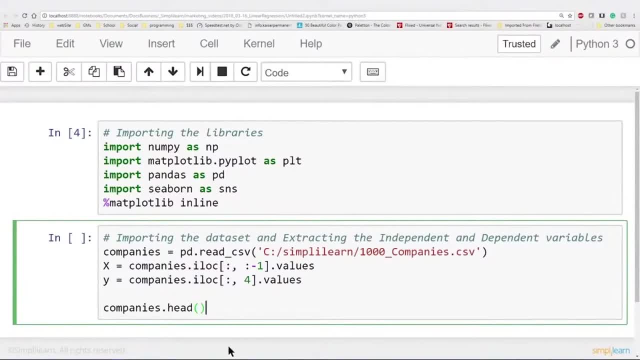 And because this is companies is a PD data set, I can use this nice notation that says: take every row. That's what the colon, the first colon, is comma, except for the last column. That's what the second part is, where we have a colon minus one. 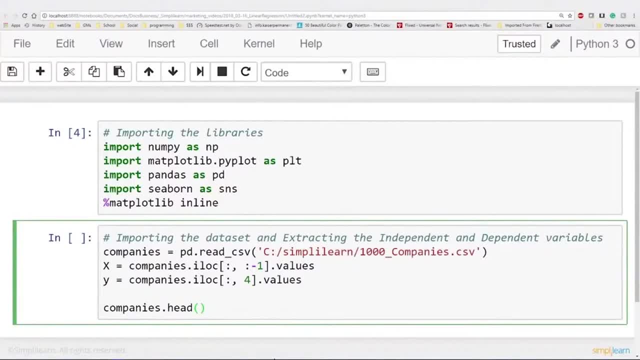 And we want the values set into there. So X is no longer a data set, It's a Pandas data set, But we can easily extract the data from our Pandas data set with this notation. And then Y we're going to set equal to the last row. 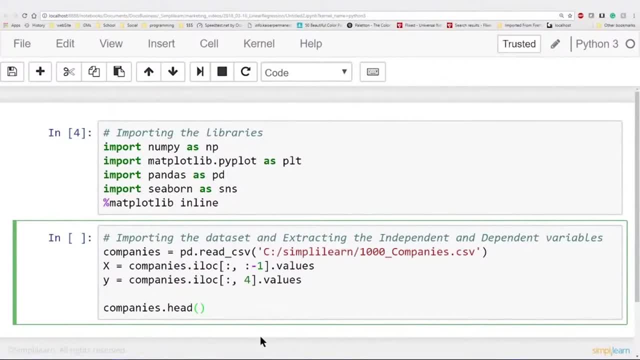 Well, the question is going to be: what are we actually looking at? So let's go ahead and take a look at that, And we're going to look at the companies dot head, which lists the first five rows of data, and I'll open up the file in just a second so you can see where that's coming from. 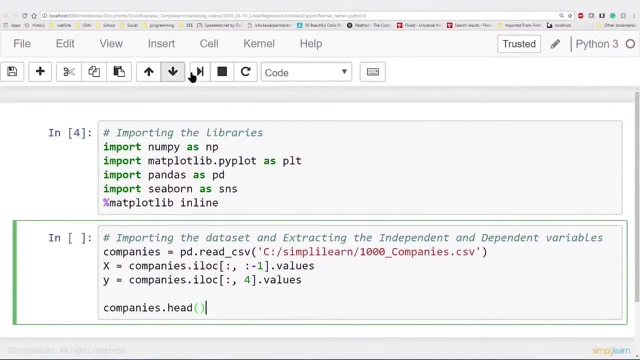 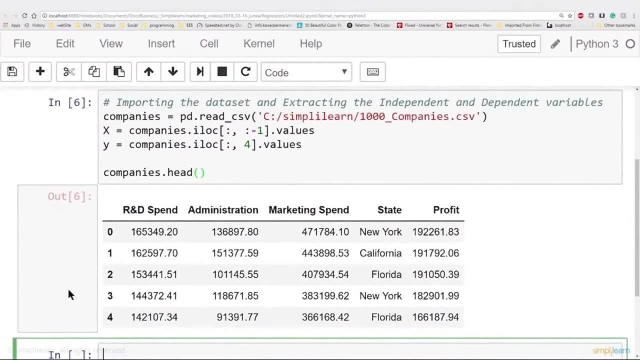 But let's look at the data in here. as far as the way the Pandas sees it, When I hit run, you'll see it breaks it out into a nice setup. This is what Pandas- It means Pandas is really good about, is? it looks just like an Excel spreadsheet. 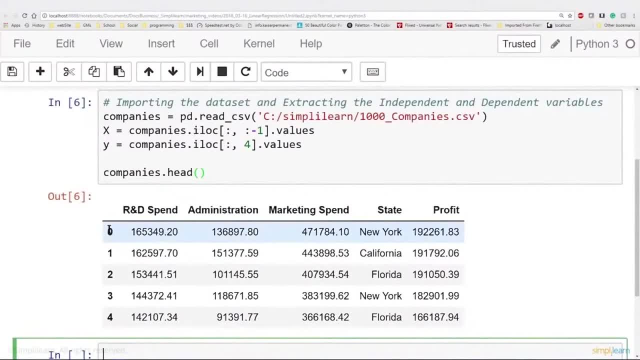 You have your rows And remember when we're programming we always start with zero, We don't start with one. So it shows the first five rows- zero: one, two, three, four- And then it shows your different columns. 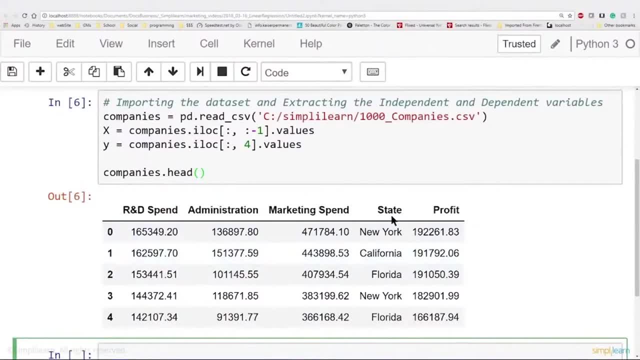 R&D spend, administration, marketing spend, state profit. It even notes that the top are column names. It was never told that, but Pandas is able to recognize a lot of things that they're not the same as the data rows. 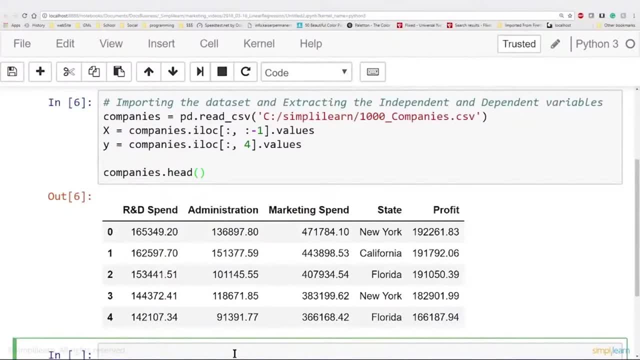 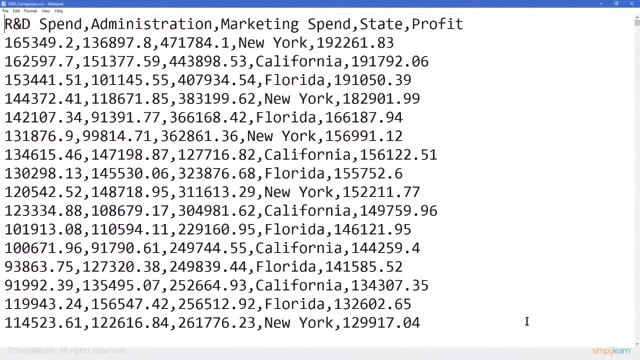 Why don't we go ahead and open this file up in a CSV so you can actually see the raw data? So here I've opened it up as a text editor and you can see at the top we have R&D spend, administration, marketing spend, state profit carries return. 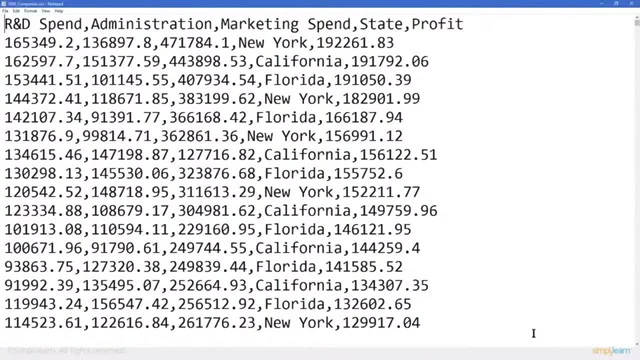 I don't know about you, but I'd go crazy trying to read files like this. That's why we use the Pandas. You could also open this up in an Excel and it would separate it, since it is a comma separated variable file. 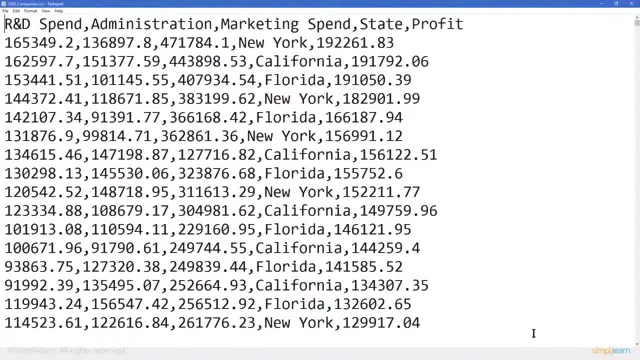 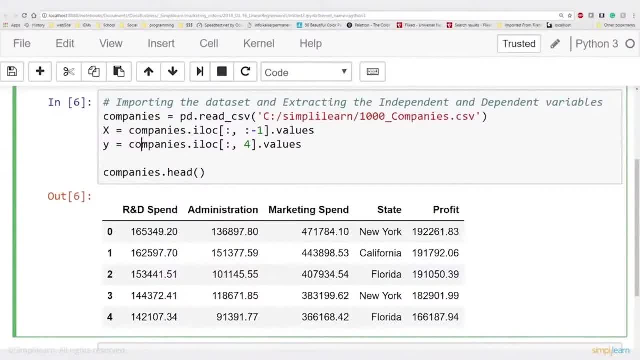 But we don't want to look at this one. We want to look at something we can read rather easily. So let's flip back and take a look at that top part, The first five rows. Now, as nice as this format is where I can see the data, to me it doesn't mean a whole lot. 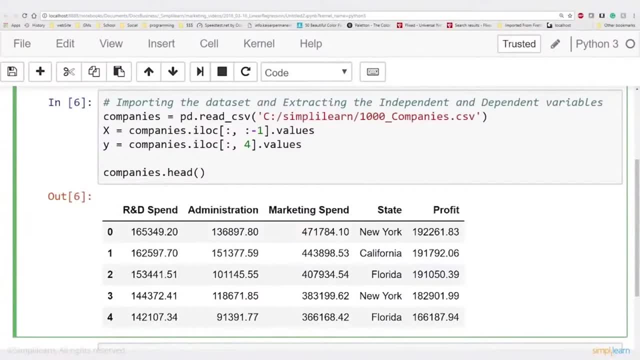 Maybe you're an expert in business and investments and you understand what one hundred and sixty five thousand three hundred forty nine dollars and twenty cents, compared to the administration cost of one hundred and thirty six thousand eight hundred ninety seven dollars and eighty cents, so on, so on, helps to create the profit of one hundred ninety two thousand. 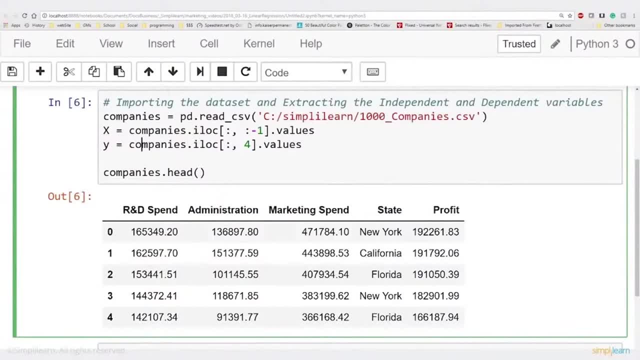 two hundred sixty one and eighty three cents. That makes no sense to me whatsoever, No pun intended. So let's flip back here and take a look at our next set of code, where we're going to graph it, so we can get a better understanding of our data and what it means. 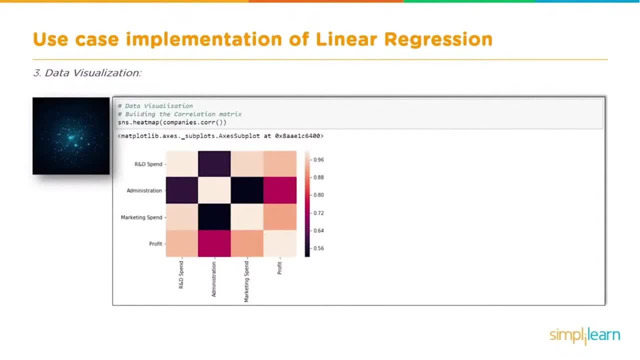 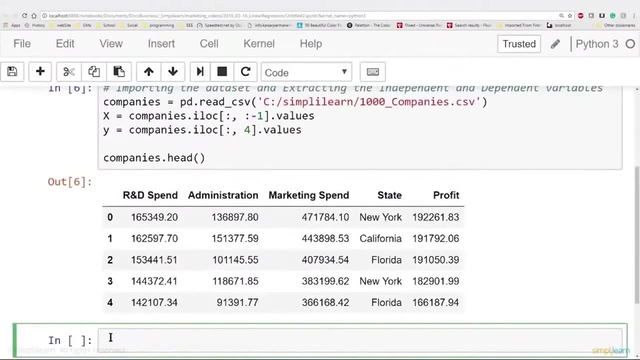 So at this point we're going to use a single line of code to get a lot of information so we can see where we're going with this. Let's go ahead and paste that into our notebook and see what we got going, And so we have the visualization. 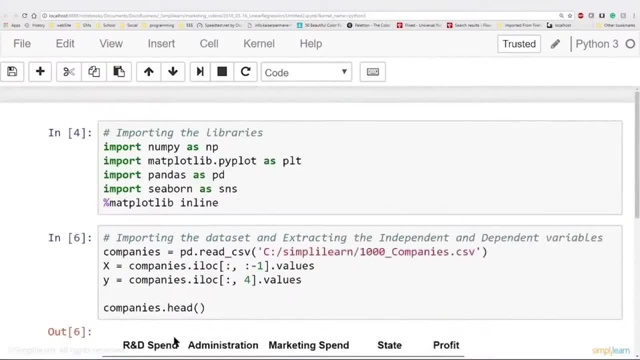 And again we're using SNS, which is Pandas. As you can see, we imported the matplotlibrarypyplot as PLT, which then the Seaborn uses, And we imported the Seaborn as SNS, And then that final line of code helps us show this in our inline coding. 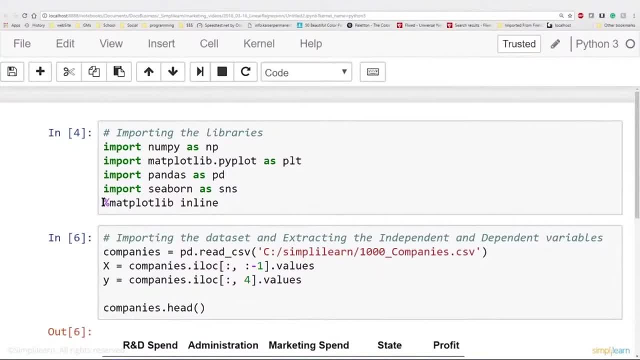 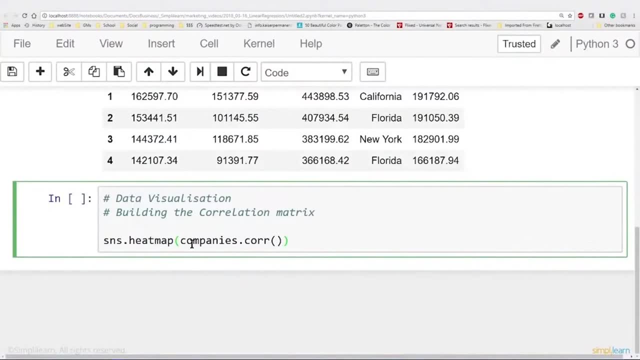 Without this it wouldn't display and you could display it to a file and other means And that's the matplotlibrary inline with the amber sign at the beginning. So here we come down to the single line of code. Seaborn is great because it actually recognizes the Panda data frame. 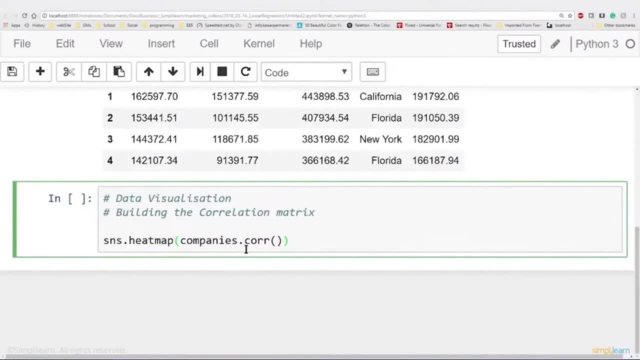 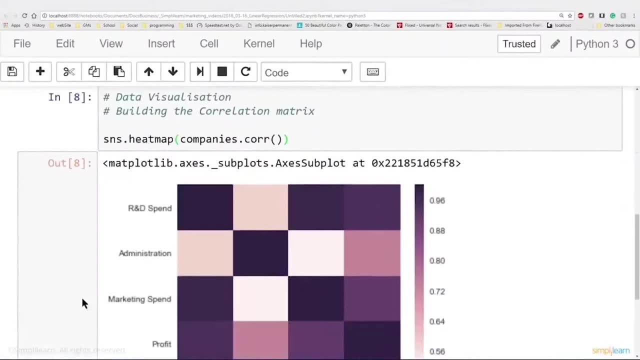 So I can just take the companiescore for coordinates and I can put that right into the Seaborn And when we run this we get this beautiful plot And let's just take a look at what this plot means. If you look at this plot on mine, 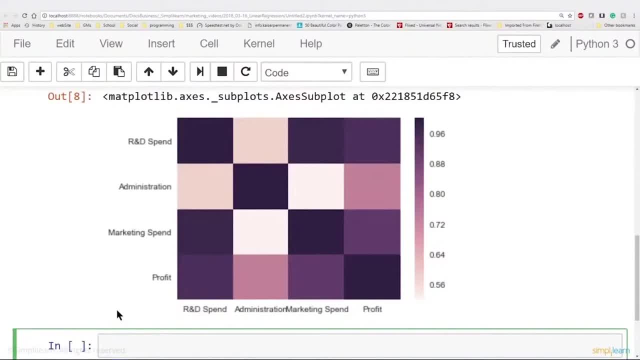 the colors are probably a little bit more purplish and blue than the original one. We have the columns and the rows, We have R and D spending, We have administration, we have marketing spending and profit And if you cross, index any two of these, since we're interested in profit. 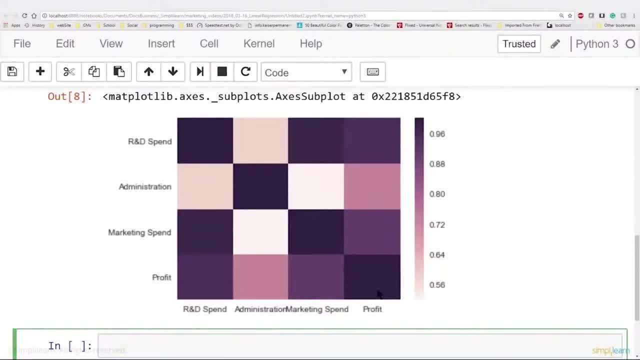 if you cross index profit with profit, it's going to show up if you look at the scale on the right way up in the dark. Why? Because those are the same data. They have an exact correspondence. So R and D spending is going to be. 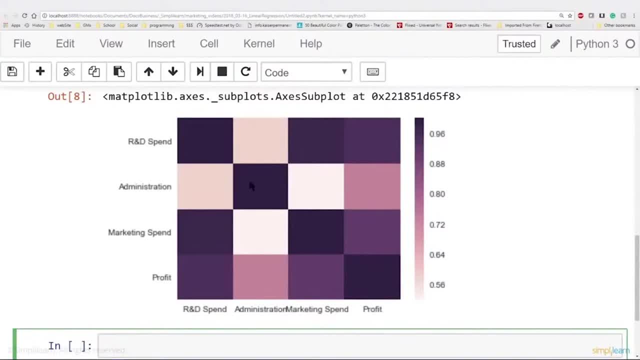 the same as R and D spending and the same thing with administration costs. So right down the middle you get this dark row or dark diagonal row that shows that this is the highest corresponding data. That's exactly the same, And as it becomes lighter there's less connections between the data. 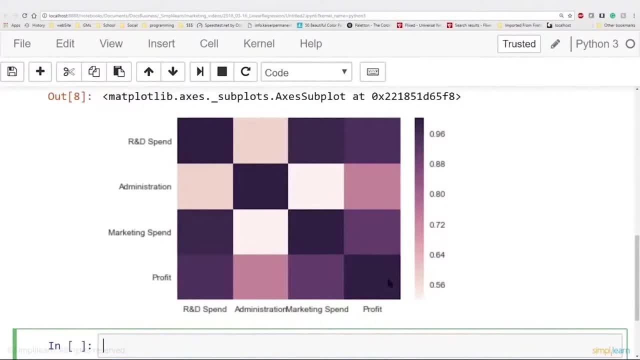 So we can see, with profit, obviously profit is the same as profit. And next, it has a very high correlation with R and D spending, which we looked at earlier, And it has a slightly less connection to marketing spending and even less to how much money we put into the administration. 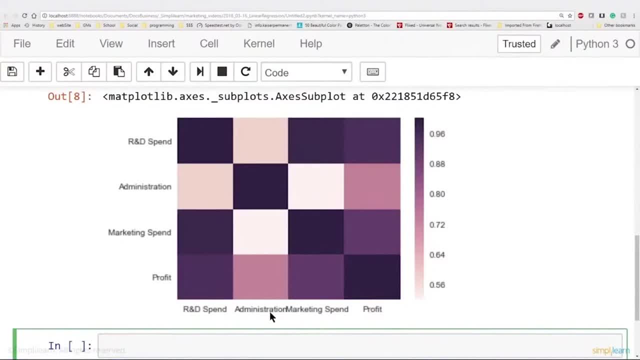 So, now that we have a nice look at the data, let's go ahead and dig in and create some actual, useful linear regression models so that we can predict values and have a better profit. Now that we've taken a look at the visualization of this data, we're going to move on to the next step. 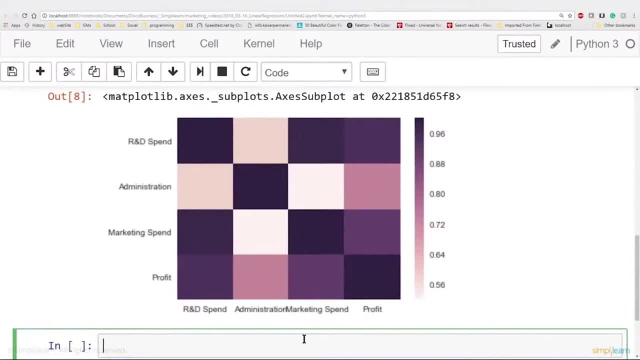 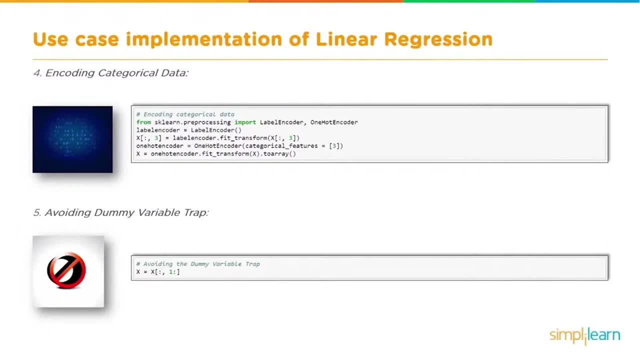 Instead of just having a pretty picture, we need to generate some hard data, some hard values. So let's see what that looks like. We're going to set up our linear regression model in two steps. The first one is we need to prepare some of our data so it fits correctly. 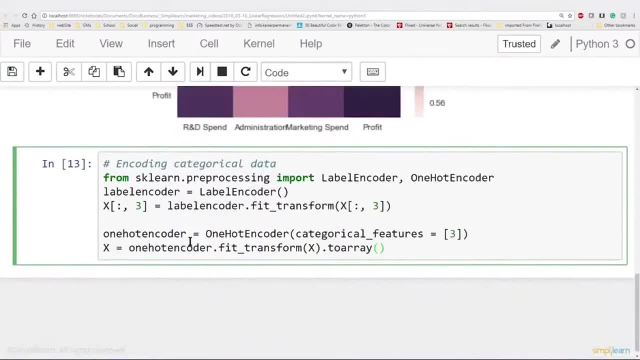 And let's go ahead and paste this code into our Jupyter notebook. And what we're bringing in is: we're going to bring in the sklearn preprocessing. We're going to import the label encoder and the one hot encoder. To use the label encoder, we're going to create a variable called 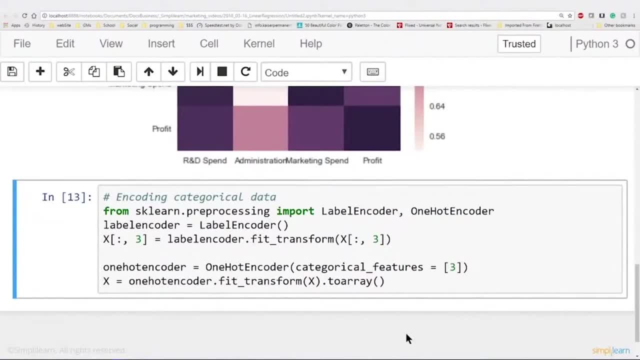 label encoder and set it equal to capital L label, capital E encoder. This creates a class that we can reuse for transferring the labels back and forth. Now about now, you should ask: what labels are we talking about? Let's go take a look at the data we processed before and see what I'm talking about here. 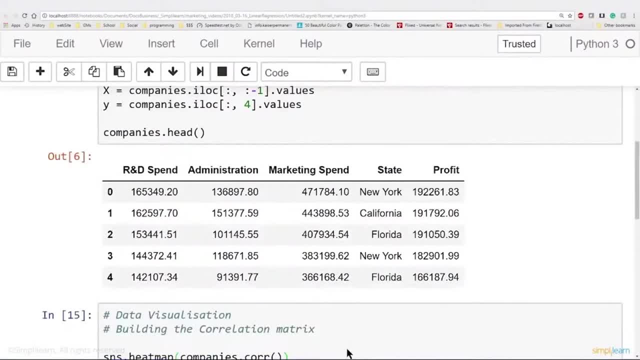 If you remember when we did the companies dot head and we printed the top five rows of data. we have our columns going across and we have column zero, which is R&D spending, column one, which is administration, column two, which is marketing spending, and column three is state. 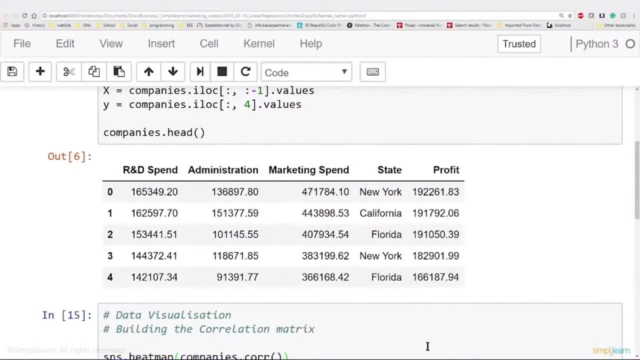 And you'll see, under state we have New York, California, Florida. Now to do a linear regression model. it doesn't know how to process New York. It knows how to process a number. So the first thing we're going to do is we're going to change that New York. 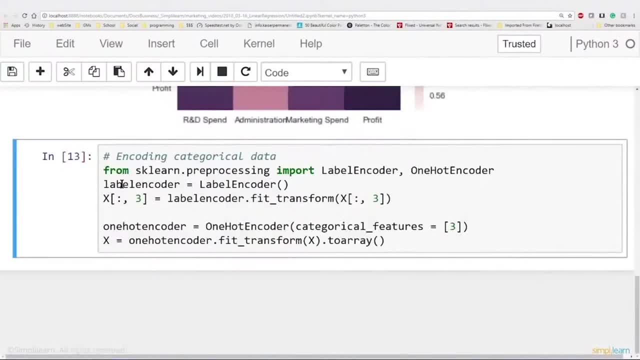 California and Florida, and we're going to change those to numbers. That's what this line of code does. here, X equals, and then it has the colon comma, three in brackets, The first part. the colon comma, means that we're going to look at all the different. 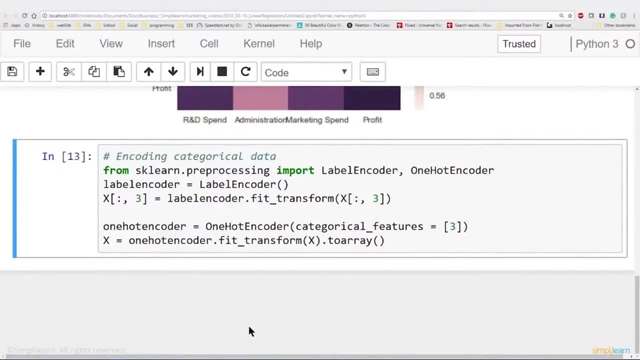 rows, so we're going to keep them all together. But the only row we're going to edit is the third row And in there we're going to take the label coder and we're going to fit and transform X, also the third row. 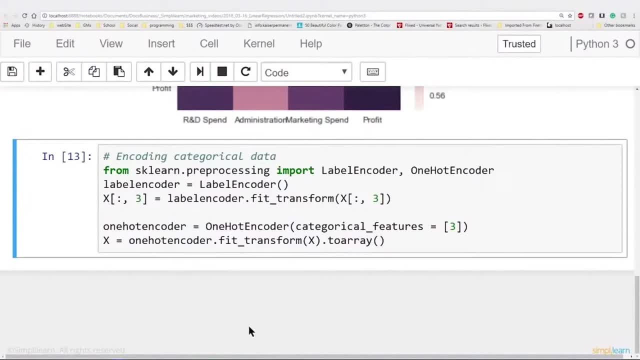 So we're going to take that third row, We're going to set it equal to a transformation And that transformation basically tells it that instead of having a New York, it has a zero or one or a two. And then, finally, we need to do a one hot encoder. 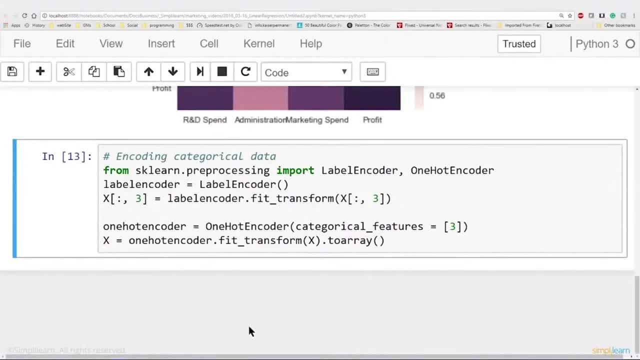 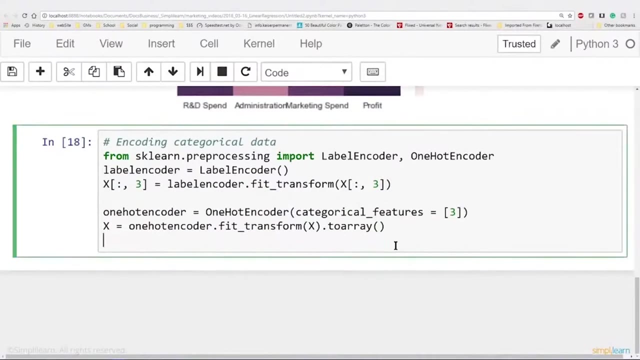 which equals one hot encoder. categorical features equals three. And then we take the X and we go ahead and do that. equal to one hot encoder. fit. transform X to array. This final transformation preps our data for us. So it's completely set The way we need. it is just a row of numbers, even though it's not in here. 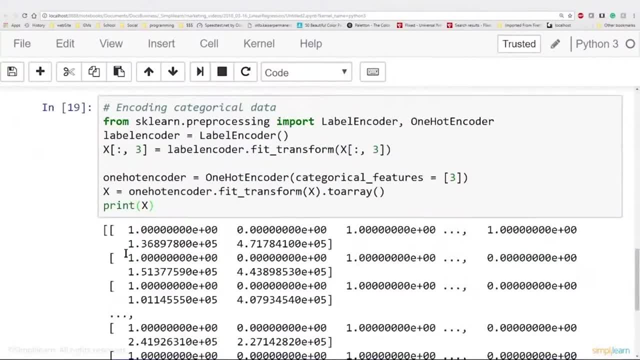 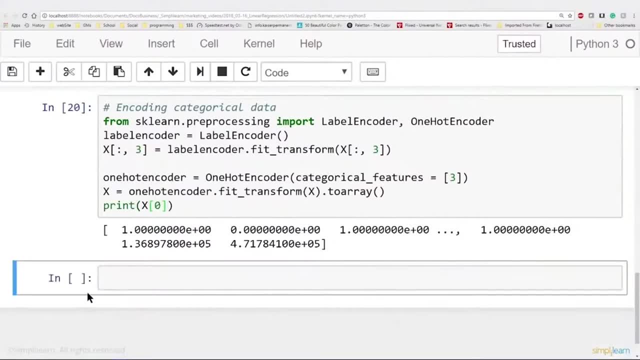 Let's go ahead and print X and just take a look at what this data is doing, You'll see you have an array of arrays and then each array is a row of numbers. And if I go ahead and just do row zero, you'll see I have a nice organized row of numbers that the computer now understands. 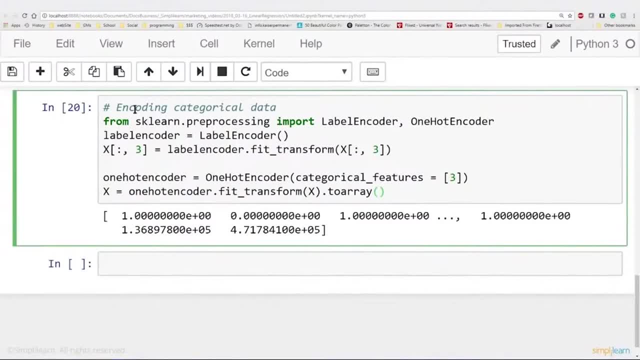 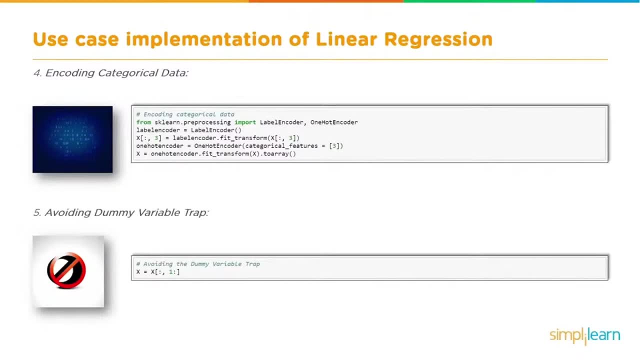 We'll go ahead and take this out there, because it doesn't mean a whole lot to us. It's just a row of numbers. Next, on setting up our data, we have avoiding dummy variable trap. This is very important. Why? Because the computer is automatically. 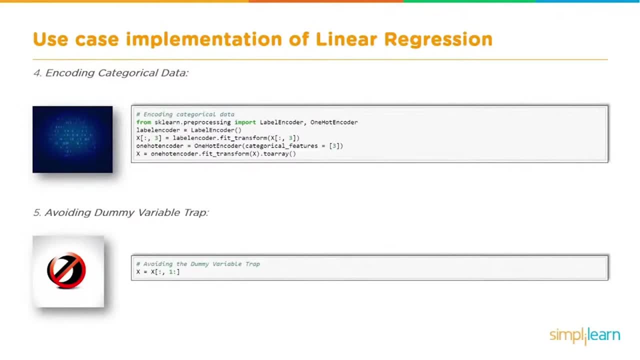 transformed our header into the setup and it's automatically transferred all these different variables. So when we did the encoder, the encoder created two columns And what we need to do is just have the one, because it has both the variable and the name. That's what this piece of code does here. 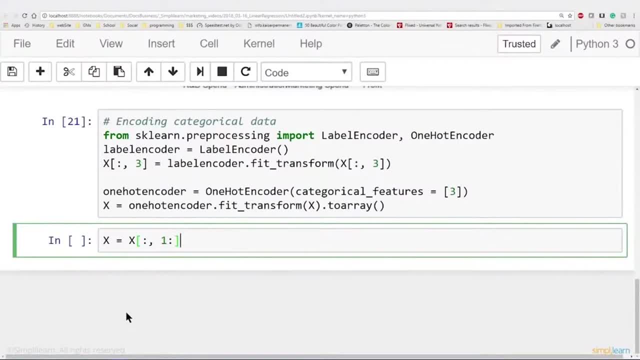 Let's go ahead and paste this in here. We have X equals X, colon, comma one colon. All this is doing is removing that one extra column We put in there when we did our one hot encoder and our label encoding. 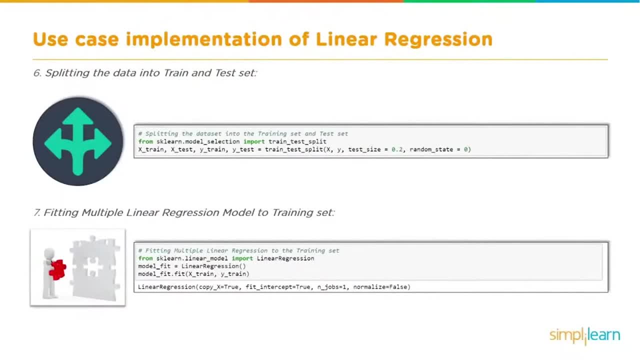 Let's go ahead and run that, And now we get to create our linear regression model And let's see what that looks like here. We're going to do that in two steps. The first step is going to be in splitting the data. 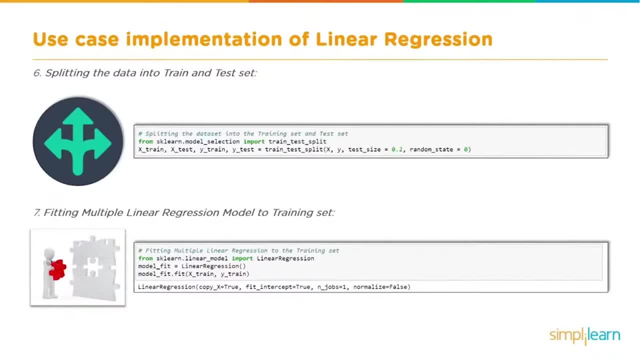 Now, whenever we create a predictive model of data, we always want to split it up. So we have a training set and we have a testing set. That's very important, Otherwise we'd be very unethical without testing it to see how good our fit is. 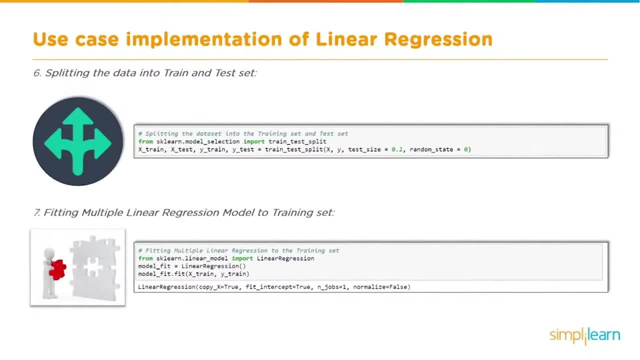 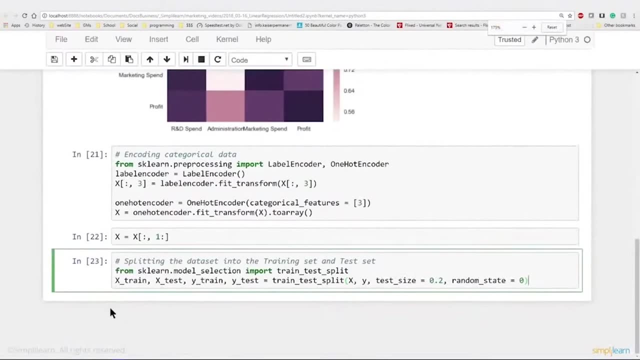 And then we'll go ahead and create our multiple linear regression model and train it and set it up. Let's go ahead and paste this next piece of code in here and I'll go ahead and shrink it down a size or two so it all fits on one line. 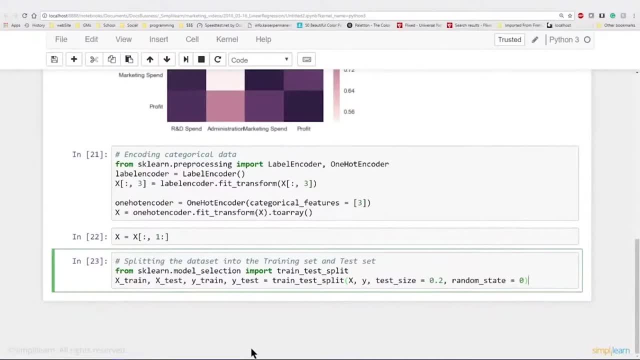 So from the SKLearn module selection we're going to import train test split And you'll see that we've created four completely different variables. We have capital X train. capital X test. smallercase y train. smallercase y test. 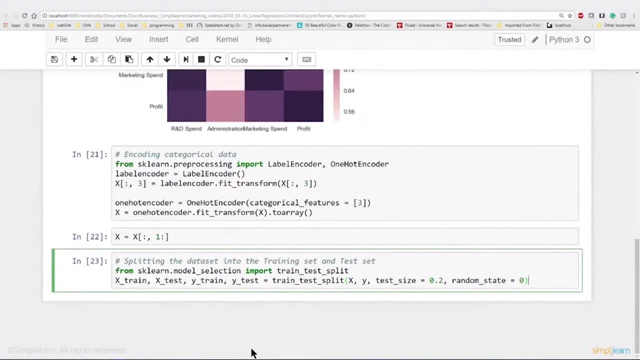 That is the standard way that they usually reference these. when we're doing different models, You usually see that a capital X. You see the train and the test and the lowercase y. What this is is X. is our data going in? That's our R&D spin, our administration, our marketing. 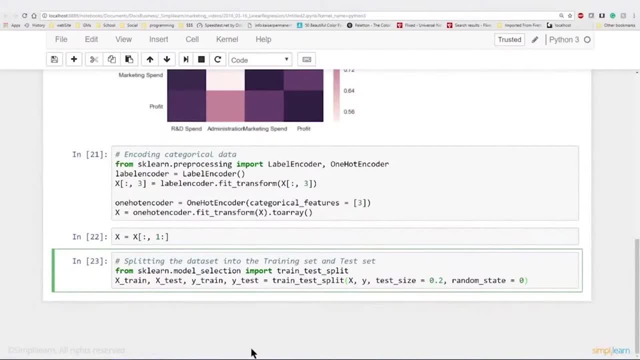 And then Y, which we're training, is the answer. That's the profit, because we want to know the profit of an unknown entity. That's what we're going to shoot for in this tutorial. The next part, train test split. We take X and we take Y. 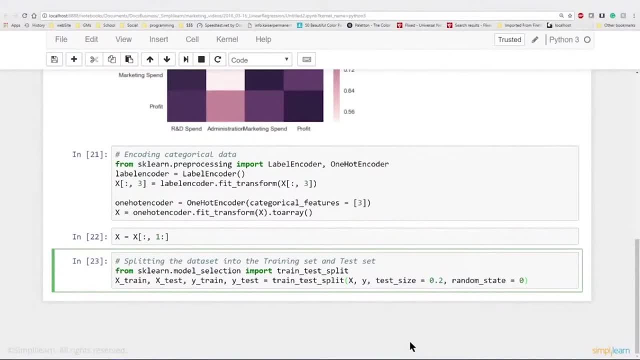 We've already created those. X has the columns with the data in it, and Y has a column with profit in it, And then we're going to set the test size equals 0.2.. That basically means 20 percent. So 20 percent of the rows are going to be tested. 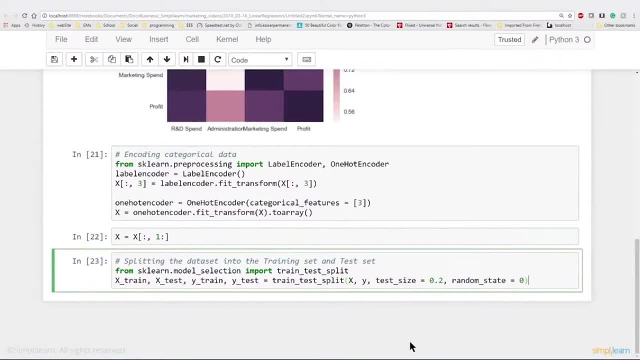 We're going to put them off to the side. So since we're using a thousand lines of data, that means that 200 of those lines we're going to hold off to the side to test for later, And then the random state equals zero. 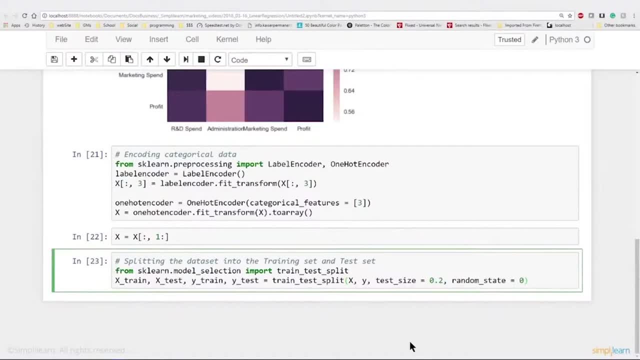 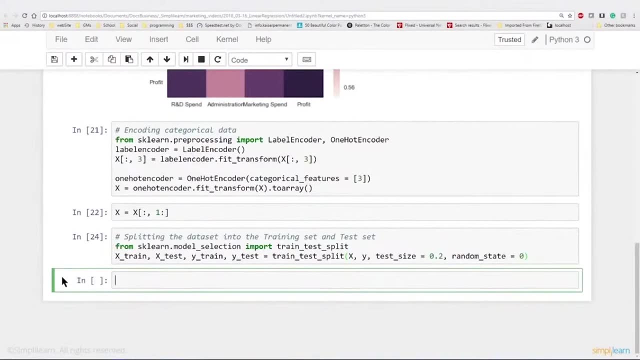 We're going to randomize which ones it picks to hold off to the side. We'll go ahead and run this. It's not overly exciting because it's setting up our variables, But the next step is the next step. We actually create our linear regression model. 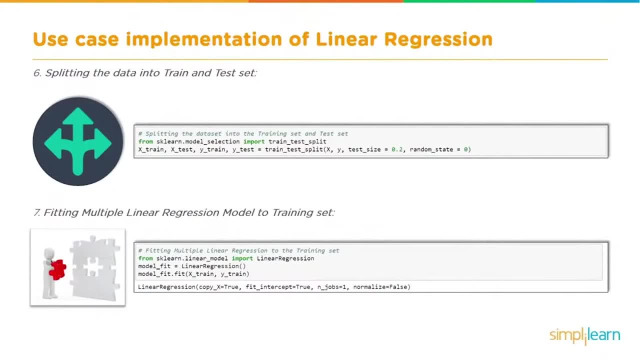 Now that we got to the linear regression model, we get that next piece of the puzzle. Let's go and put that code in there and walk through it. So here we go: We're going to paste it in there And let's go ahead. 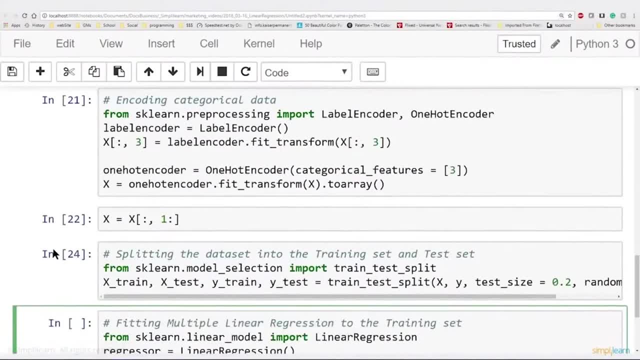 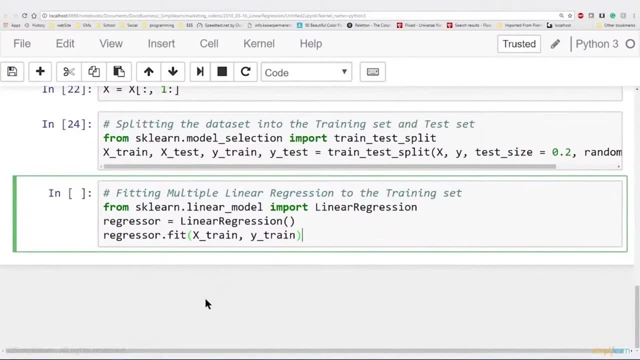 And since this is a shorter line of code, let's zoom up there so we can get a good look. and we have from the sklearn dot linear underscore model. We're going to import linear regression. Now I don't know if you recall from earlier when we were doing all the math. 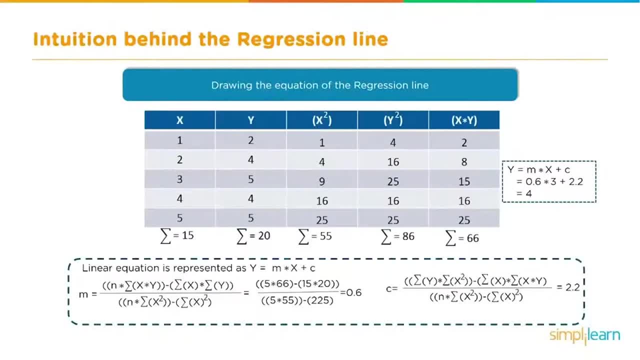 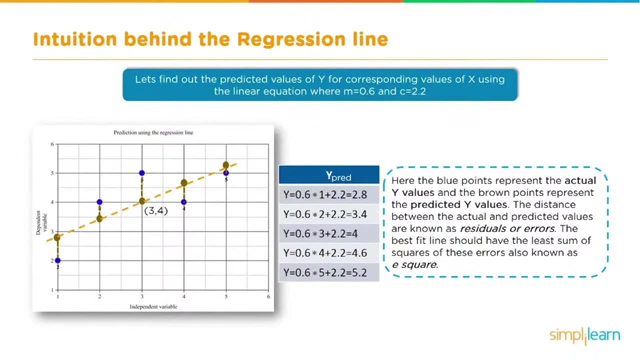 Let's go ahead and flip back there and take a look at that. Do you remember this, where we had this long formula on the bottom and we were doing all this summation and then we also looked at setting it up with the different lines, and then we also looked all the way down to multiple linear regression. 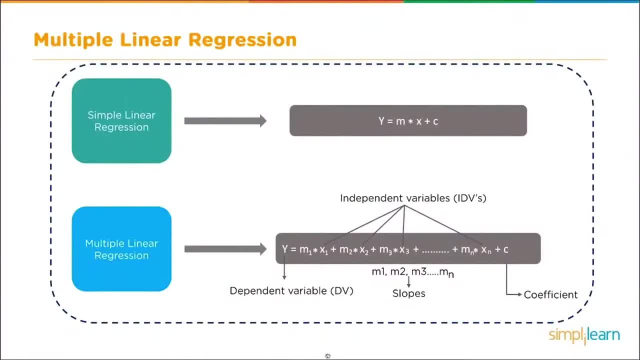 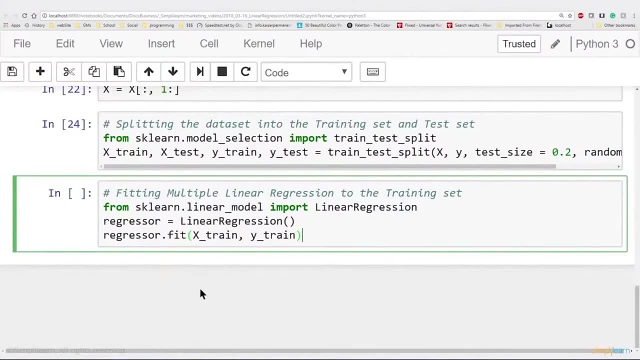 We're adding all those formulas together. All of that is wrapped up in this one section. So what's going on here is I'm going to create a variable called regressor, and the regressor equals the linear regression. That's a linear regression model that has all that math built in. 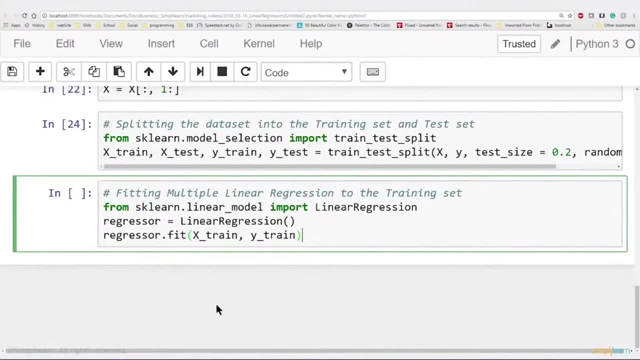 So we don't have to have it all memorized or have to compute. We can do it individually. and then we do the regressor dot fit. In this case, we do X train and Y train because we're using the training data, X being the data in and Y being profit. what we're looking at 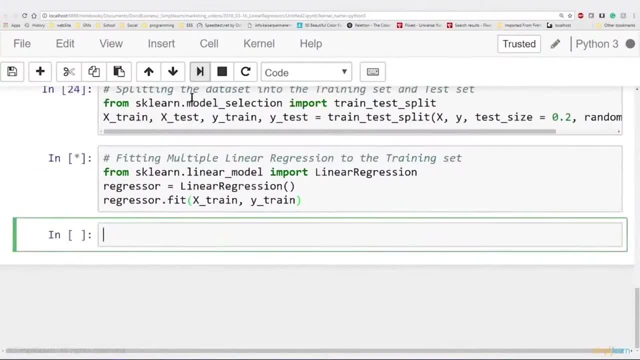 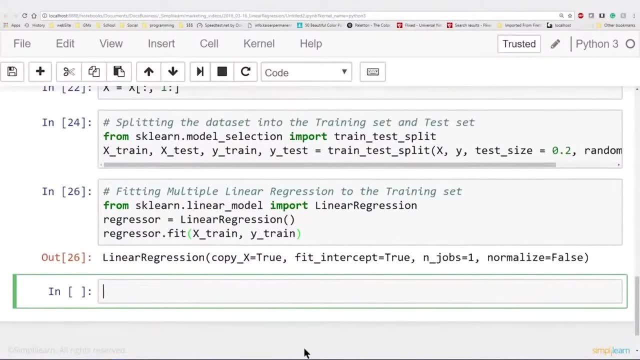 And this does all that math for us. So within one click and one line we've created the whole linear regression model and we fit the data to the linear regression model And you can see that when I run the regressor it gives an output linear. 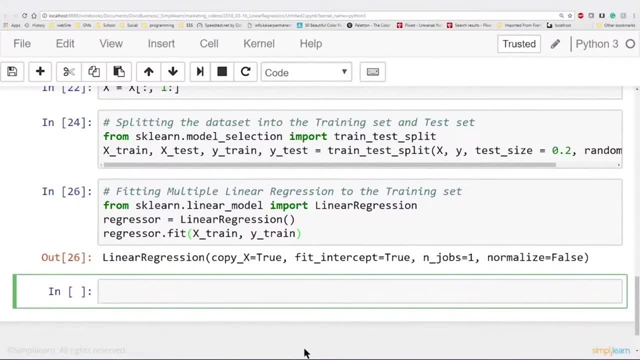 regression. it says: copy X equals true, fit intercept equals true. in jobs equal one false. It's just giving you some general information on what's going on with that regressor model. Now that we've created our linear regression model, let's go ahead and use it. 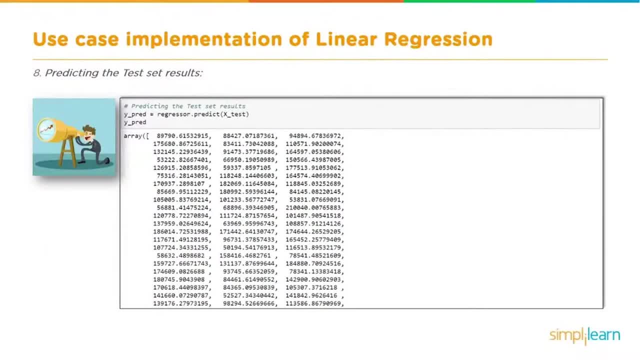 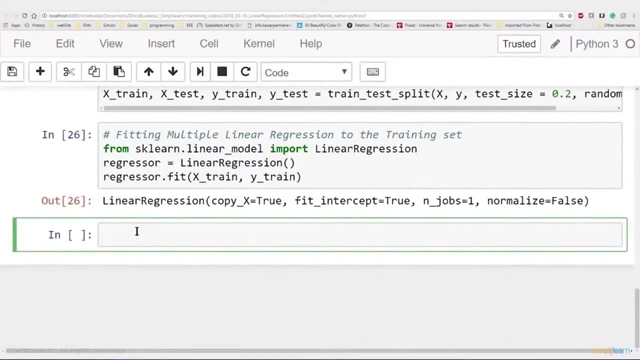 And, if you remember, we kept a bunch of data aside. So we're going to do a Y predict variable and we're going to put in the X test And let's see what that looks like. Scroll up a little bit, Paste that in here. predicting the test set results. 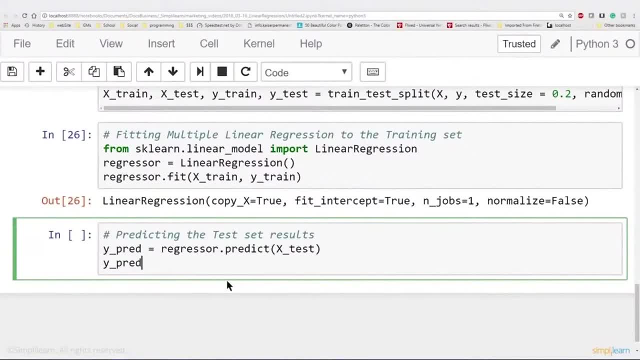 So here we have Y predict equals regressor dot predict X test going in And this gives us Y predict. Now, because I'm in Jupyter inline, I can just put the variable up there And when I hit the run button it'll print that array out. 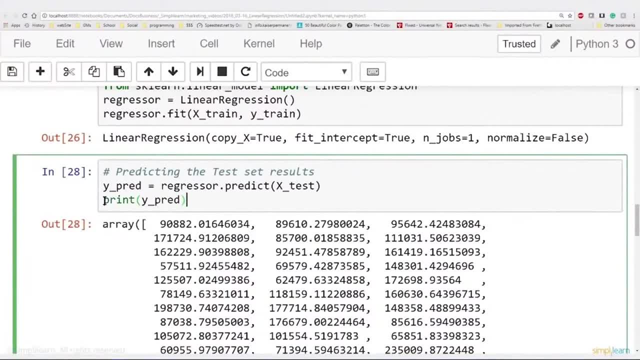 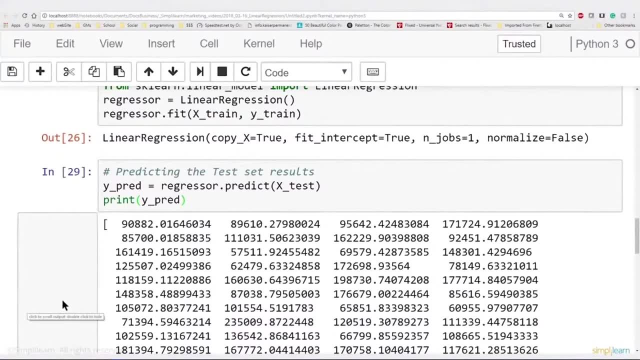 I could have just as easily done print Y predict. So if you're in a different IDE that's not an inline set up like the Jupyter notebook, you can do it this way: Print Y predict And you'll see that for the 200 different. 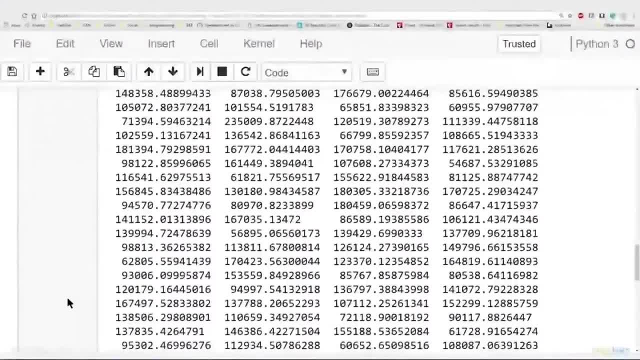 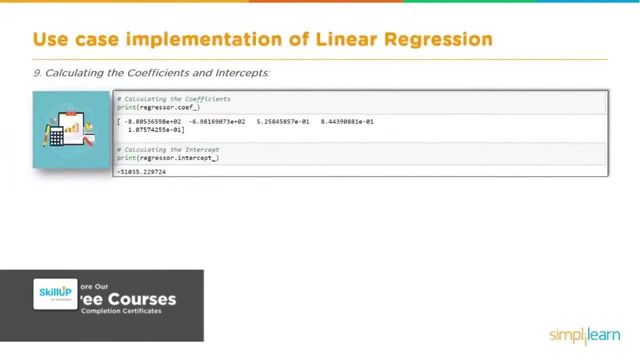 test variables. we kept off to the side. it's going to produce 200 answers. This is what it says. the profit are for those 200 predictions. But let's don't stop there. Let's keep going and take a couple. look, We're going to take just a short detail. 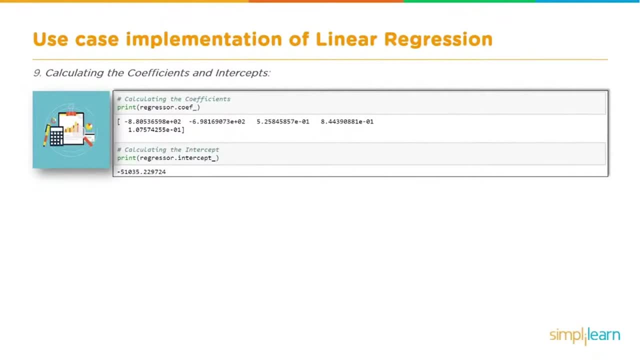 here and calculating the coefficients and the intercepts. This gives us a quick flash at what's going on behind the line. We're going to take a short detour here and we're going to be calculating the coefficient and intercepts So you can see what those look like. 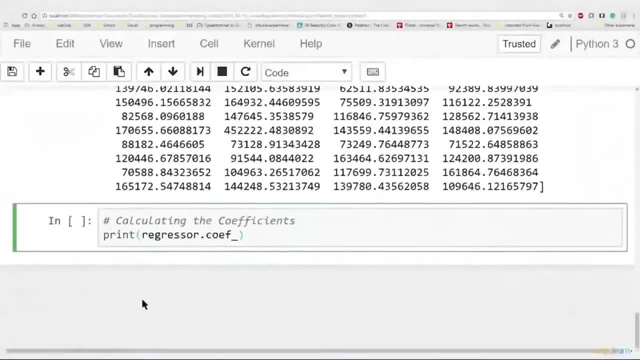 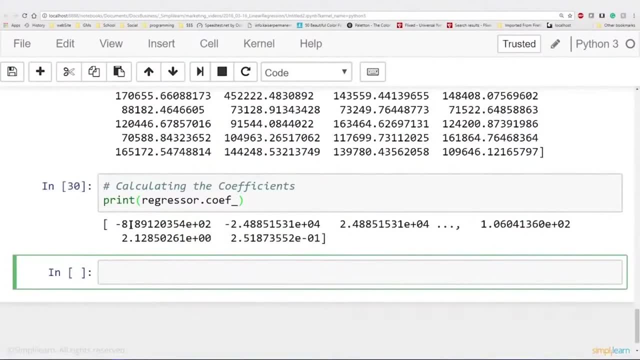 What's really nice about our regressor we created is it already has a coefficients for us. We can simply just print regressor dot coefficient underscore. When I run this you'll see our coefficients here And if we can do the regressor coefficient. 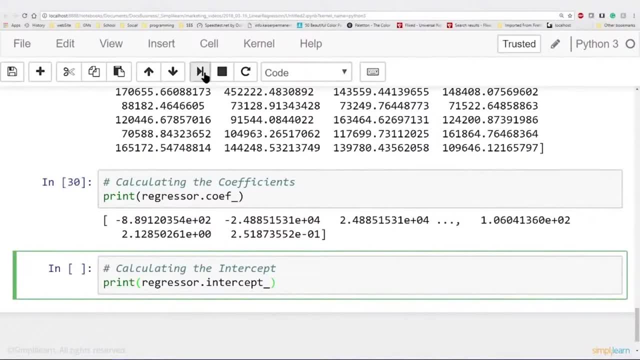 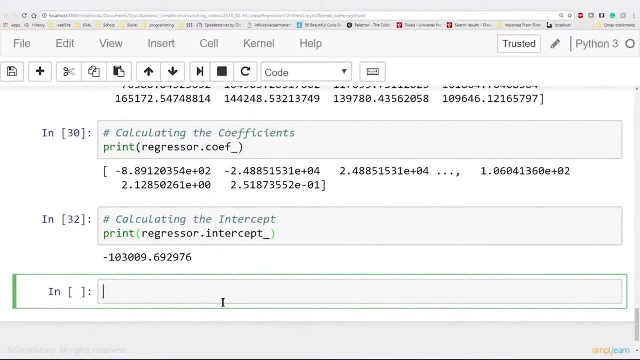 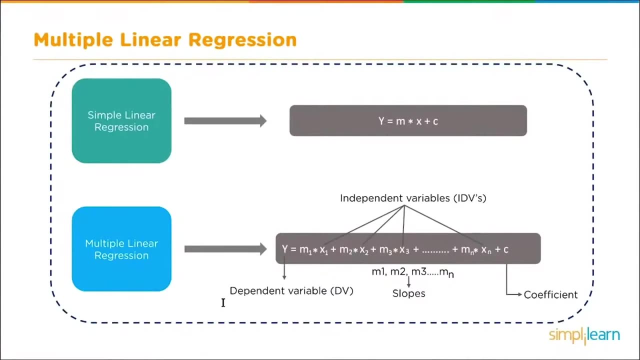 we can also do the regressor intercept and let's run that and take a look at that. This all came from the multiple regression model. We'll flip over so you can remember where this is going into, where it's coming from. You can see the formula down here, where Y equals M1 times X1 plus M2 times X2, and so 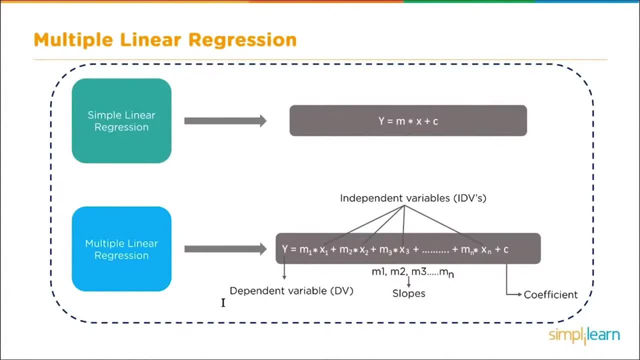 on and so on, plus C, the coefficient. So these variables fit right into this formula: Y equals slope one times column, one variable, plus slope two times column, two variable, all the way to the M, into the N, and X to the N plus C. 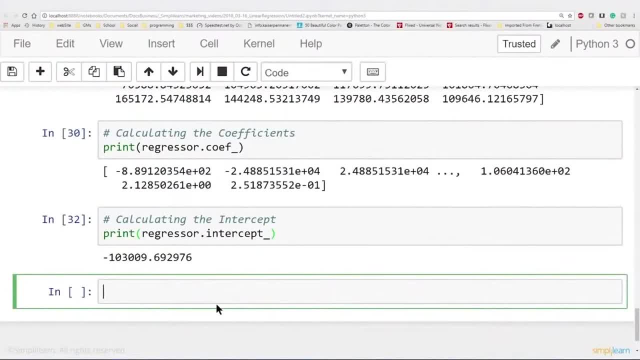 the coefficient, Or in this case you have minus eight point eight, nine, to the power of two, et cetera, et cetera, times the first column and the second column and the third column, And then our intercept is the minus one, zero, three, zero, zero, nine point. 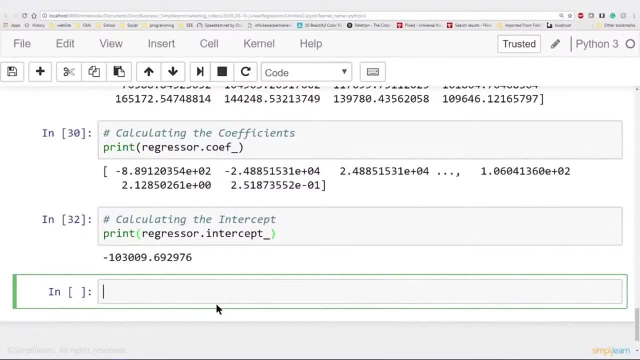 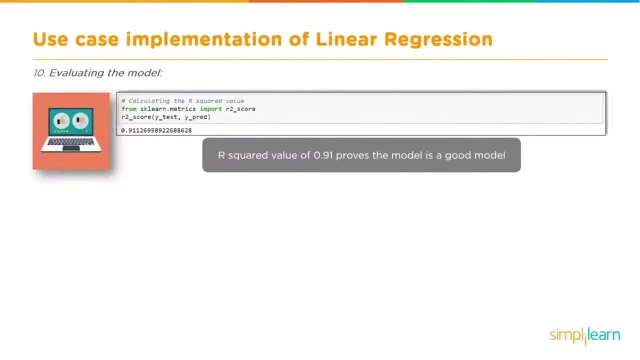 Boy, it gets kind of complicated when you look at it. This is why we don't do this by hand anymore. This is why we have the computer to make these calculations easy to understand and calculate. Now, I told you that was a short. 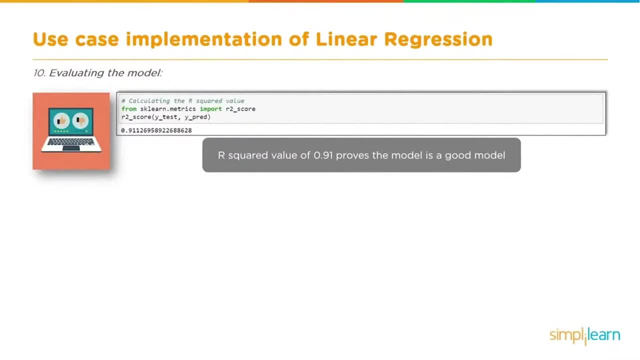 detour and we're coming towards the end of our script. As you remember, from the beginning I said if we're going to divide this information, we have to make sure it's a valid model, that this model works and understand how good it works. So, calculating the R squared value. 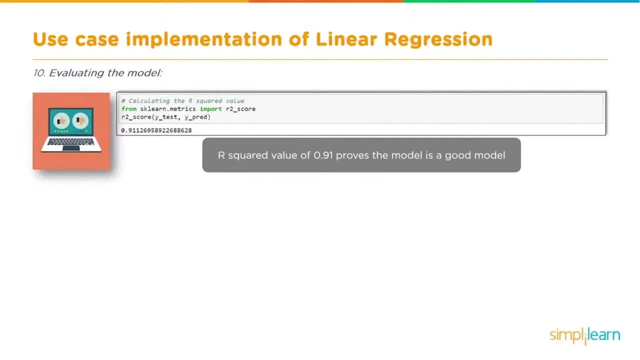 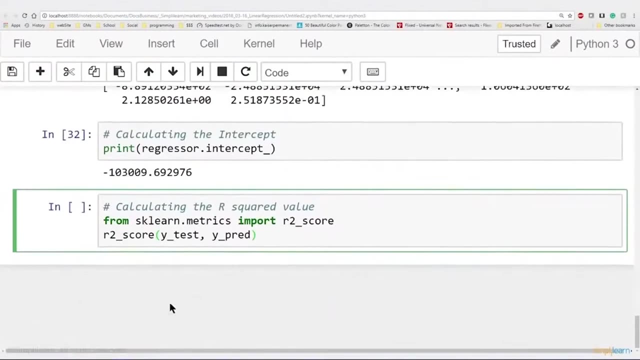 that's what we're going to use to predict how good our prediction is, And let's take a look at what that looks like in code. And so we're going to use this from sklearnmetrics. We're going to import R2 score. 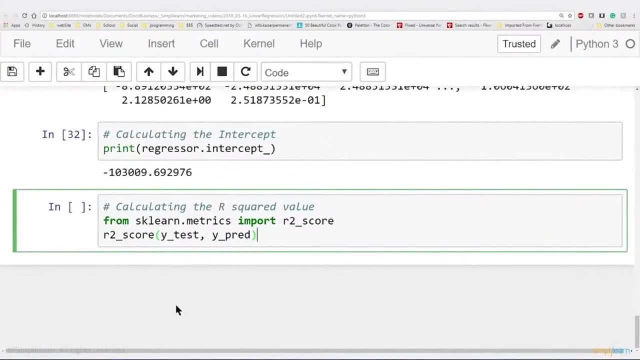 That's the R squared value. We're looking at the error. So in the R2 score we take our Y test versus our Y. predict Y test is the actual values we're testing. That was the one that was given to us that we know are true. 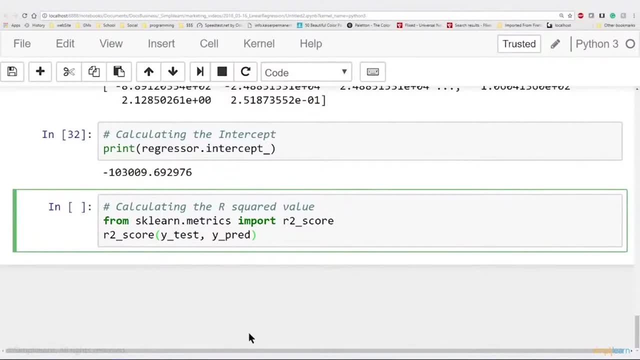 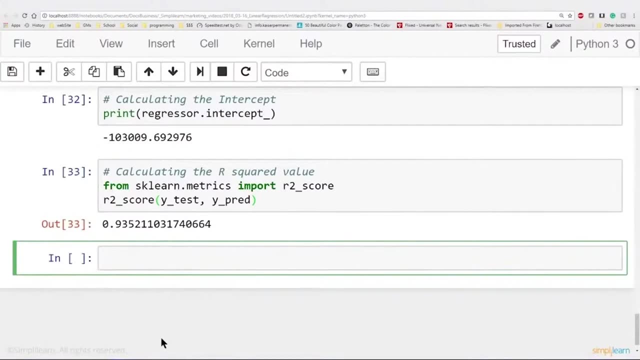 The Y predict of those 200 values is what we think it was true, And when we go ahead and run this we see we get a .9352.. That's the R2 score. Now, it's not exactly a straight percentage. 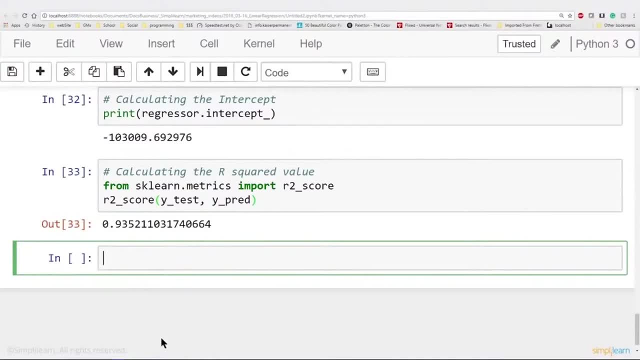 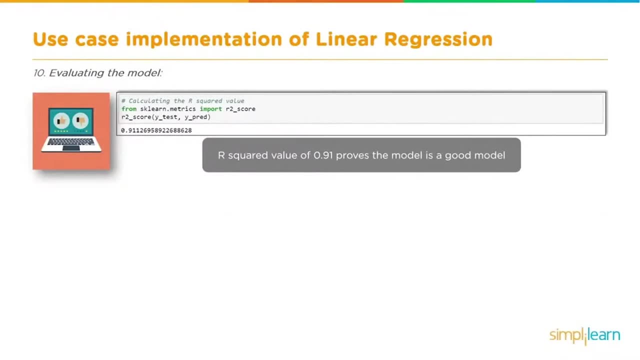 So it's not saying it's 93 percent correct, But you do want that in the upper 90s and higher, which shows that this is a very valid prediction based on the R2 score And if R squared value of .91 or 92, as we got on our model. 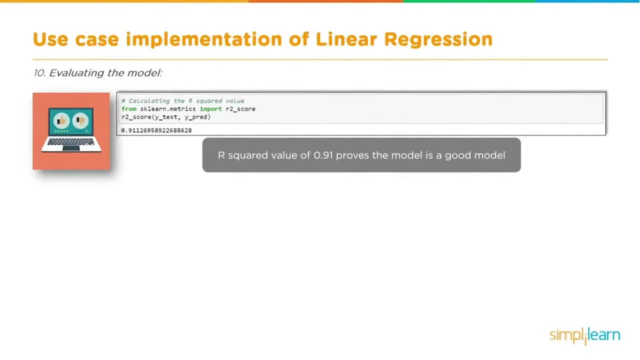 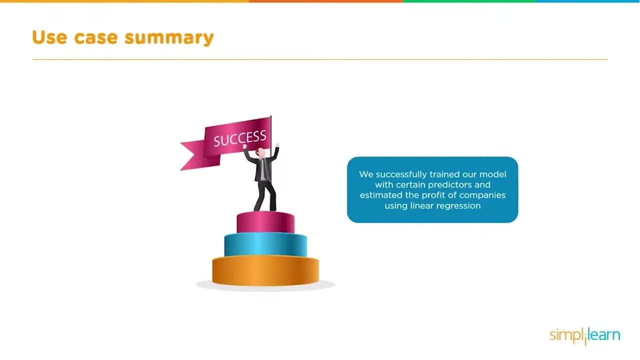 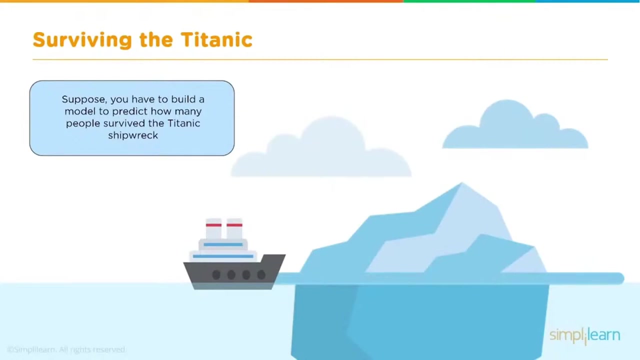 remember it does have a random generation involved. This proves the model is a good model, which means success. Yay, We successfully trained our model with certain predictors and estimated the profit of the companies using linear regression. What is logistic regression? Let's say we have to build a predictive model or a machine learning model to predict. 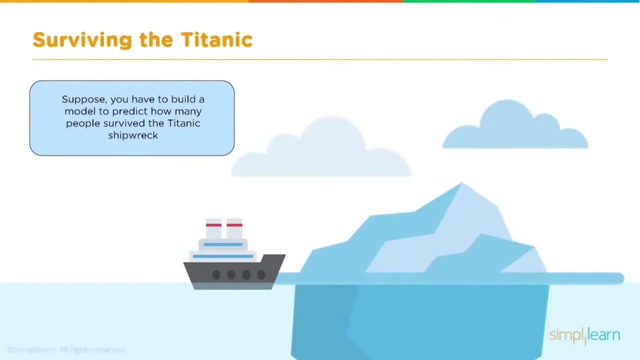 whether the passengers of the Titanic ship have survived or not the shipwreck. So how do we do that? So we use logistic regression to build a model for this. How do we use logistic regression? So we have the information about the passengers, their ID. 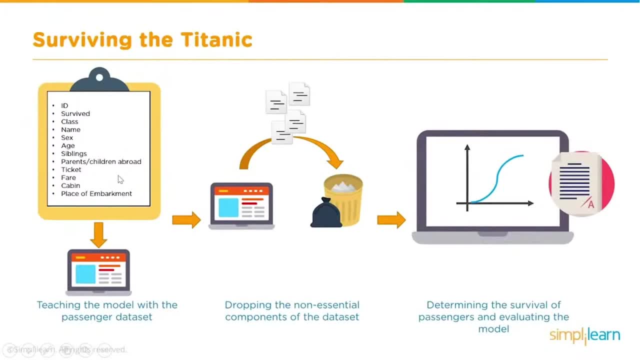 whether they have survived or not, their class and name and so on and so forth, And we use this information where we already know whether the person has survived or not. That is the labeled information, And we help the system to train based on this information, based on this labeled data. 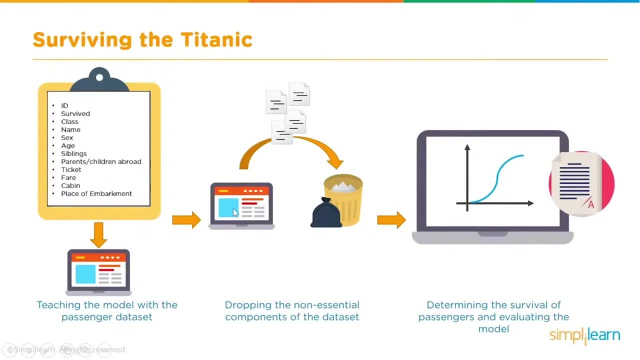 This is known as labeled data, And during the process of building the model we probably remove some of the non-essential parameters or attributes. here We only take those attributes which are really required to make these predictions, And once we train the model, we run new data through it, whereby the model 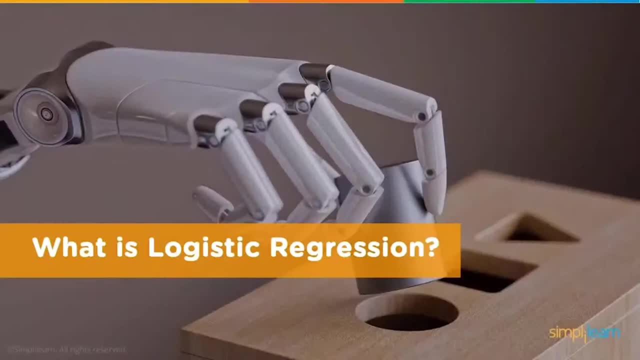 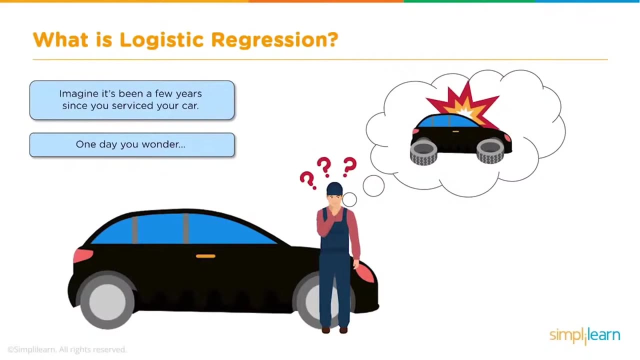 will predict whether the passenger has survived or not. All right, What is logistic regression? As I mentioned earlier, logistic regression is an algorithm for performing binary classification. So let's take an example and see how this works. Let's say your car has not been serviced for quite a few years and now you want 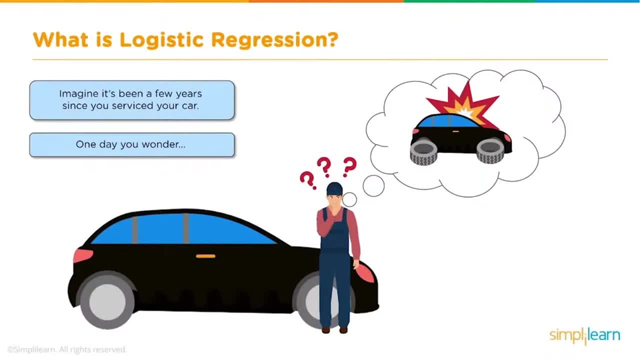 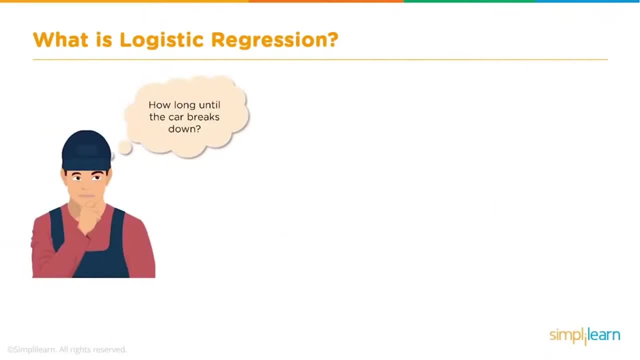 to find out if it is going to break down in the near future. So this is like a classification problem: Find out whether your car will break down or not. So how are we going to perform this classification? So here's how it looks. 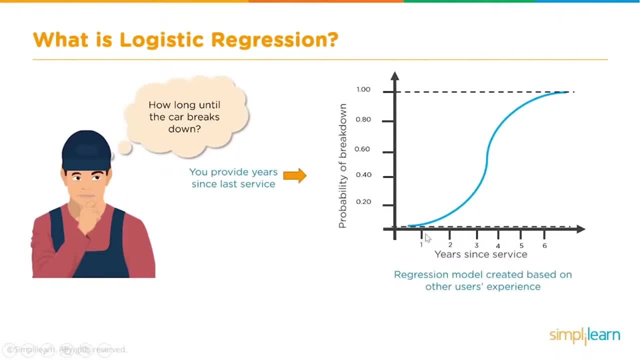 If we plot the information along the X and Y axis, X is the number of years since the last service was performed and Y is the probability of your car breaking down. And let's say, this information was this data that was collected from several car users. it's not just your car, but several car users. 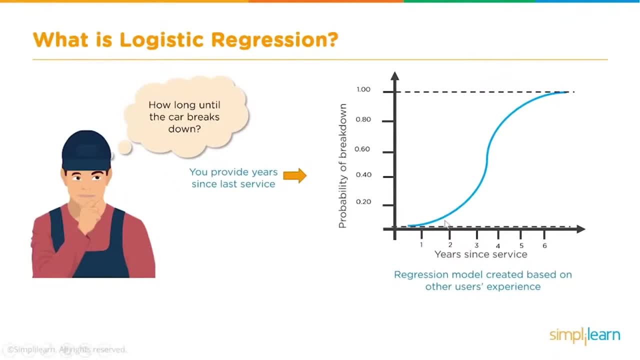 So that is our labeled data, So the data has been collected and for the number of years and when the car broke down, What was the probability? And that has been plotted along X and Y axis. So this provides an idea from this graph. 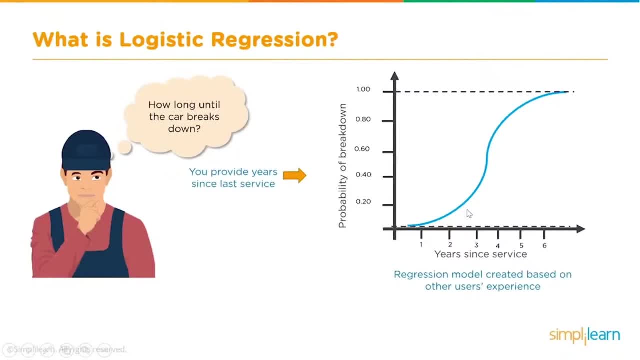 We can find out whether your car will break down or not. We'll see how. So, first of all, the probability can go from zero to one. As you're aware, probability can be between zero and one And, as we can imagine, it is intuitive as well, as the number of years are on the lower side, maybe one year. 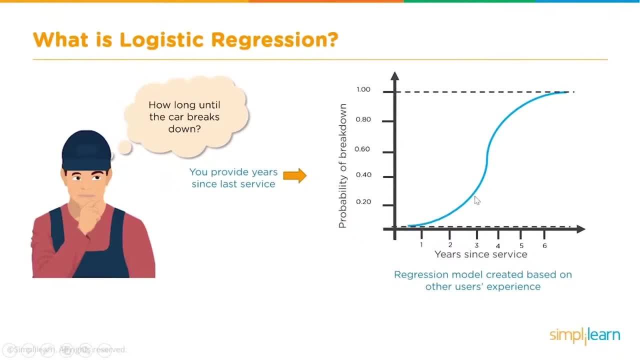 two years or three years to after the service, The chances of your car breaking down are very limited. So, for example, the chances of your car breaking down, the probability of your car breaking down within two years of your last service, are point one. 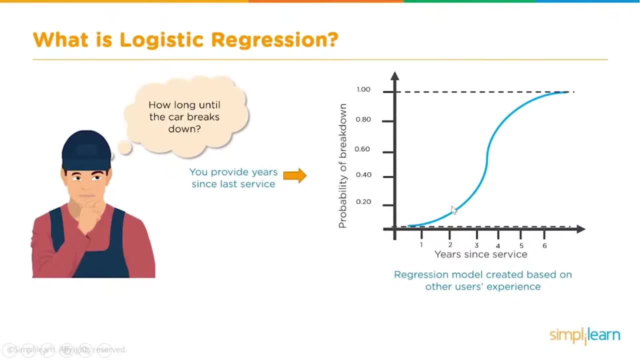 Similarly, three years is maybe point three and so on, But as the number of years increases- let's say six or seven years- there is almost a certainty that your car is going to break down. That is what this graph shows. So this is an example of an application of the classification algorithm. 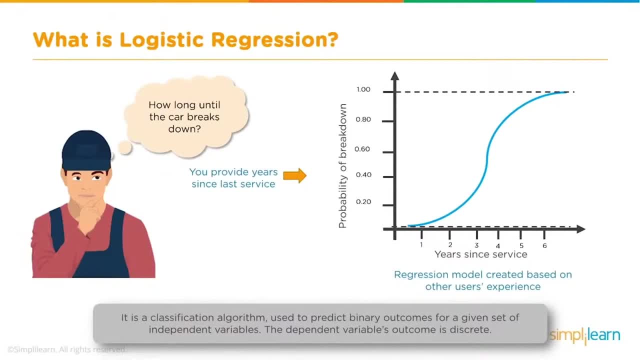 And we will see in little details how exactly logistic regression is applied here. One more thing needs to be added here is that the dependent variables outcome is discrete. So if we are talking about whether the car is going to break down or not, So that is a discrete value. 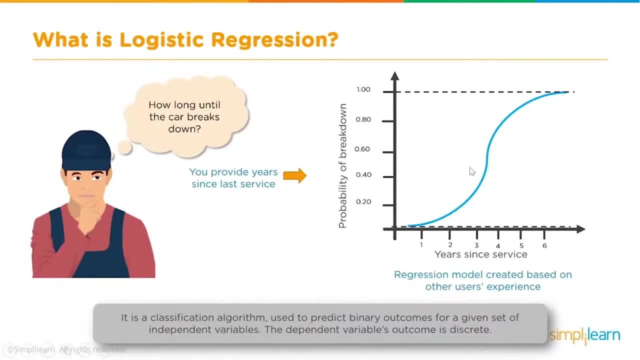 The Y that we are talking about, the dependent variable that we are talking about. What we are looking at is whether the car is going to break down or not, Yes or no. That is what we are talking about. So here the outcome is discrete and not a continuous value. 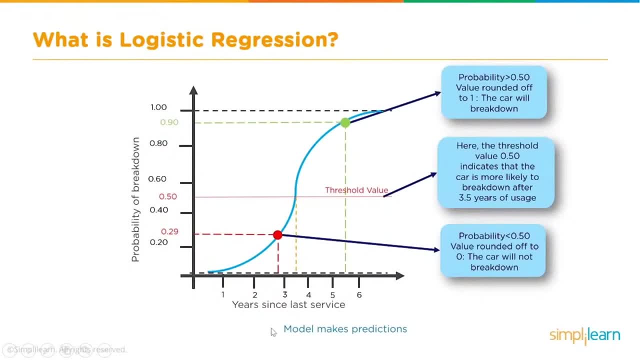 So this is how the logistic regression curve looks. Let me explain a little bit what exactly, and how exactly we are going to determine the class outcome. rather So, for a logistic regression curve, a threshold has to be set, saying that, because this is a probability calculation. remember, this is a probability calculation. 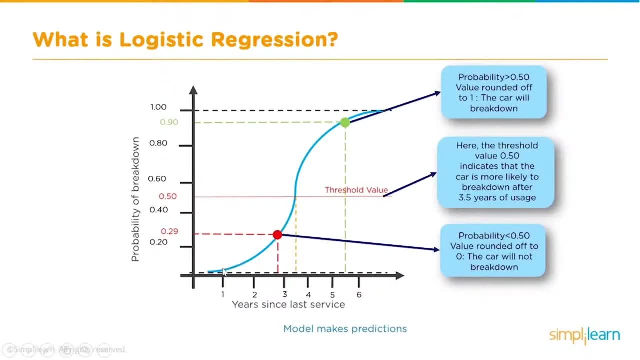 and the probability itself will not be zero or one, But based on the probability we need to decide what the outcome should be. So there has to be a threshold, like, for example, 0.5 can be the threshold Let's say in this case, 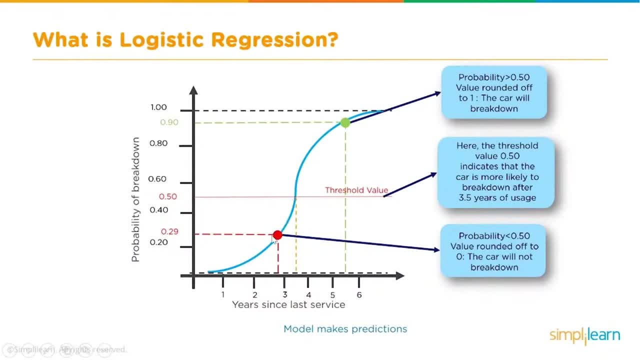 So any value of the probability below 0.5 is considered to be zero And any value above 0.5 is considered to be one. So an output of, let's say, 0.8 will mean that the car will break down, so that is considered as an output of one. 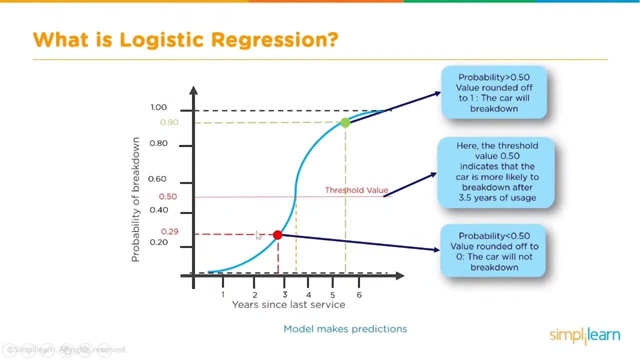 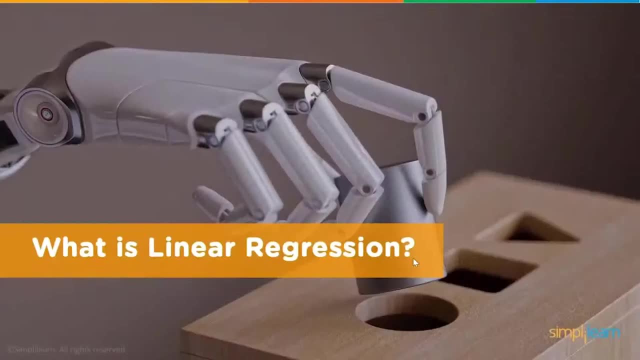 And let's say, an output of 0.29 is considered as zero, which means that the car will not break down. So that's the way logistic regression works. Now let's do a quick comparison between logistic regression and linear regression, because they both have the term regression in them. 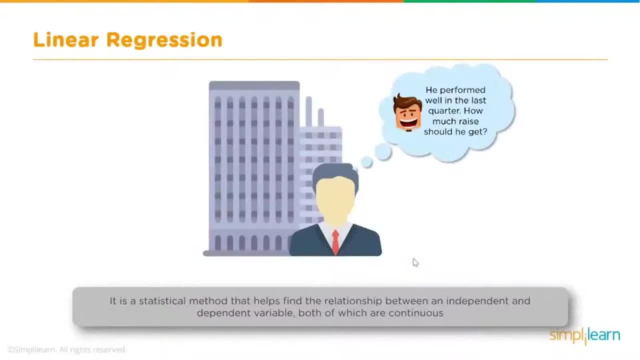 So it can cause confusion. So let's try to remove that confusion. So what is linear regression? Linear regression is a process. It's, once again, an algorithm for supervised learning. However, here you're going to find a continuous value. You're going to determine a continuous value. 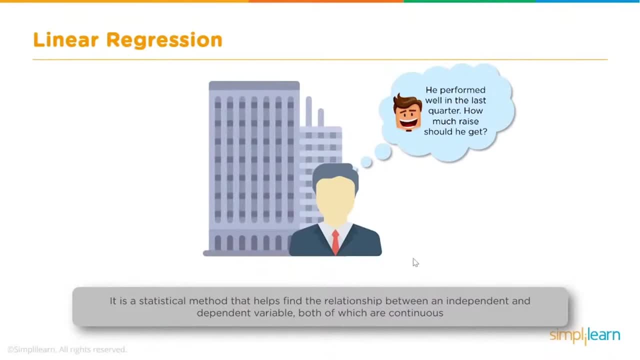 It could be the price of a real estate property. It could be your hike- how much hike you're going to get- or it could be a stock price. These are all continuous values. These are not discrete compared to a yes or no kind of response that we are looking for in logistic regression. 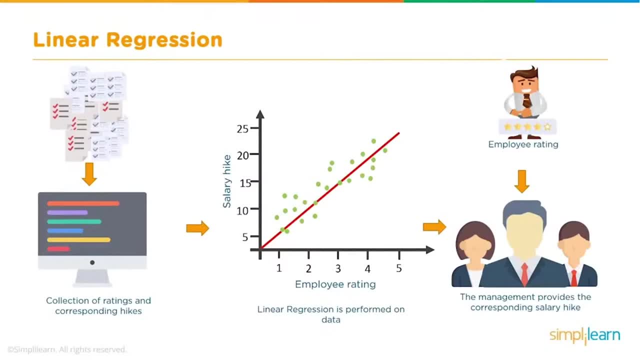 So this is one example of a linear regression. Let's say, at the HR team, A company tries to find out what should be the salary hike of an employee. So they collect all the details of their existing employees, their ratings and their salary hikes. what has been given? 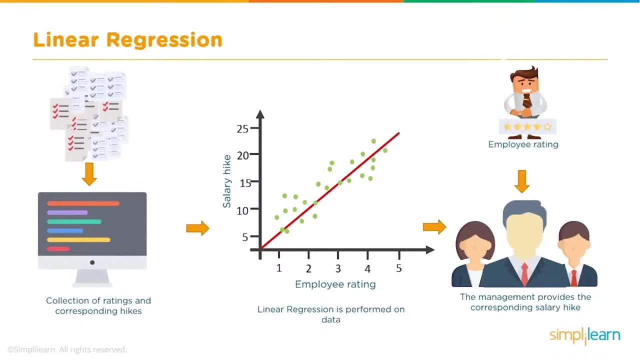 And that is the labeled information that is available And the system learns from this. It is trained and it learns from this labeled information so that when a new employee's information is fed, based on the rating, it will determine what should be the high. 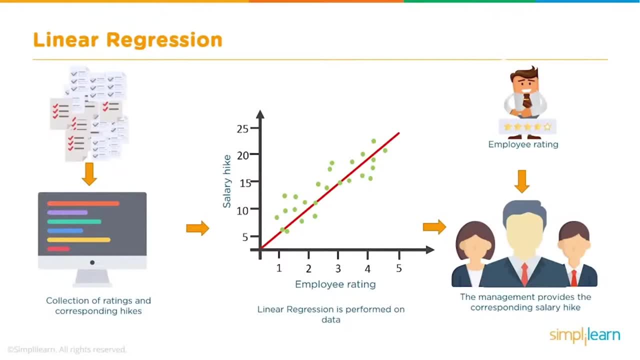 So this is a linear regression problem and linear regression- For example now salary- is a continuous value. You can get five thousand, five thousand, five hundred, five thousand, six hundred. It is not discrete, like a cat or a dog, or an apple or a banana. 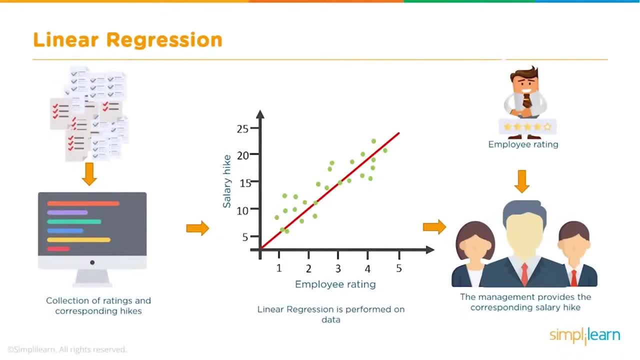 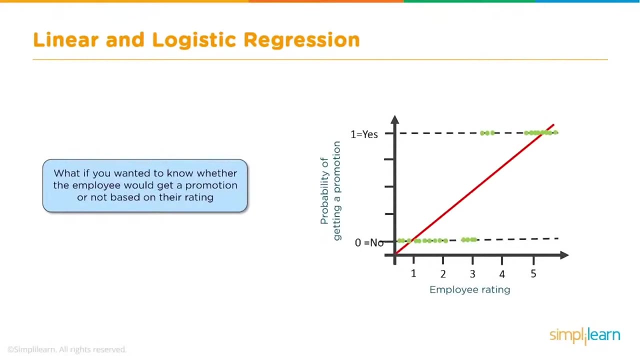 These are discrete, or a yes or a no, These are discrete values. So this way you're trying to find continuous values is where we use linear regression. So let's say, just to extend on this scenario, we now want to find out whether this employee is going to get a promotion or not. 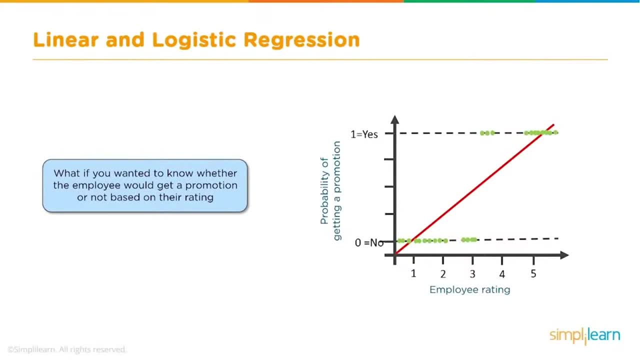 So we want to find out that is a discrete problem, Right, Yes, or no Kind of a problem. In this case, we actually cannot use linear regression, even though we may have labeled data. So this is the label data. So, based on the employee rating, these are the ratings. 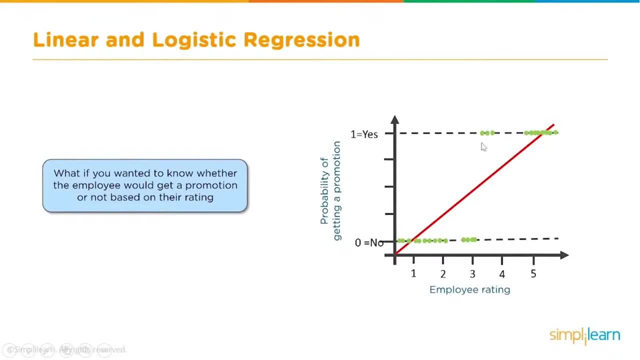 And then some people got the promotion and this is the ratings for which people did not get promotion. that is a no and this is a Rating for which people got promotion. We just plotted the data about whether a person has got an employee has got promotion or not. Yes, no. 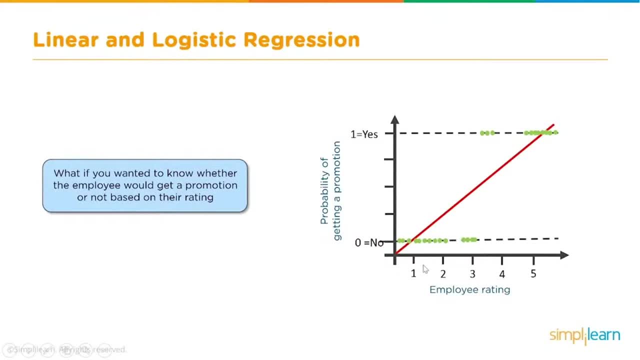 Right. So there is nothing in between. And what is the employee's rating? And ratings can be continuous, That is not an issue. But the output is discrete in this case, whether employee got promotion, Yes, no. So if we try to plot that and we try to find a straight line, this is how it would look. 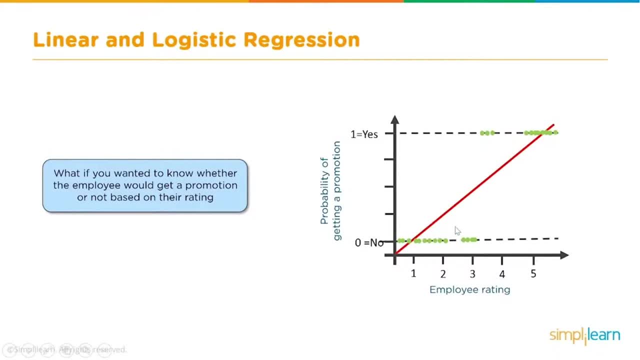 And, as you can see, it doesn't look very right because it looks like there will be a lot of errors. this root mean square error, If you remember, for linear regression would be very, very high And also the values cannot go beyond zero or beyond one. 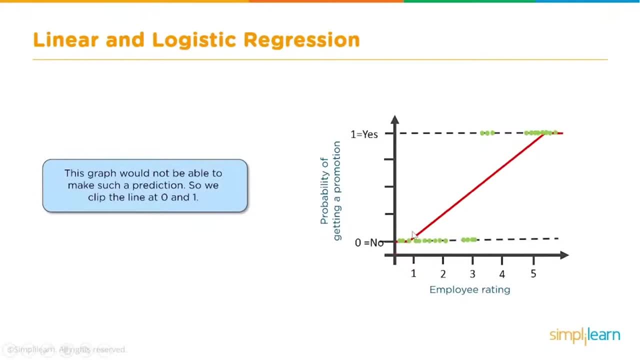 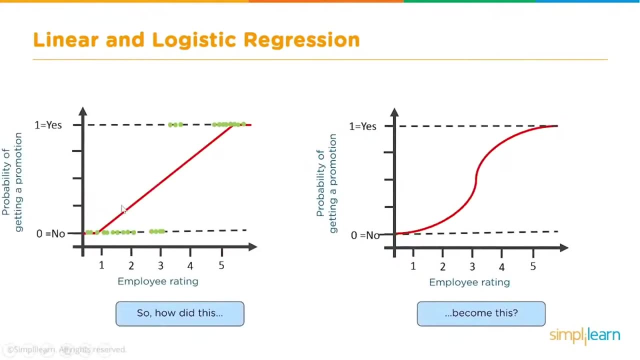 So the graph should probably look somewhat like this, at zero and one, But still the straight line doesn't look right. Therefore, instead of using a linear equation, we need to come up with something different, and therefore the logistic regression Model looks somewhat like this: 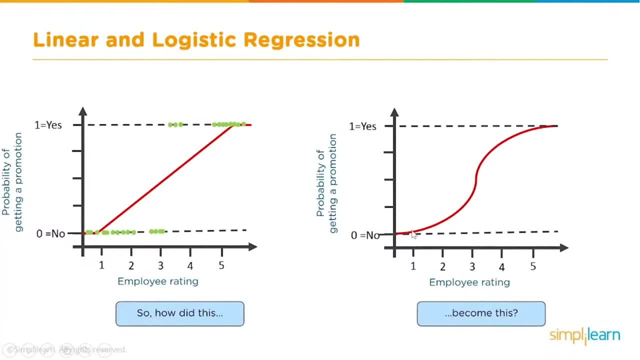 So we calculate the probability, and if we plot that probability- not in the form of a straight line, but we need to use some other equation- We will see very soon what that equation is- Then it is a gradual process. So you see here, people with some of these ratings are not getting any promotions. 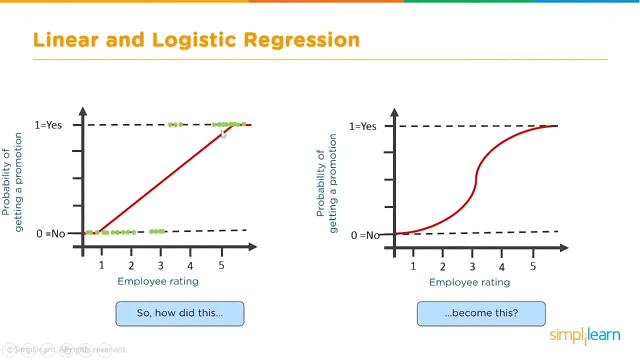 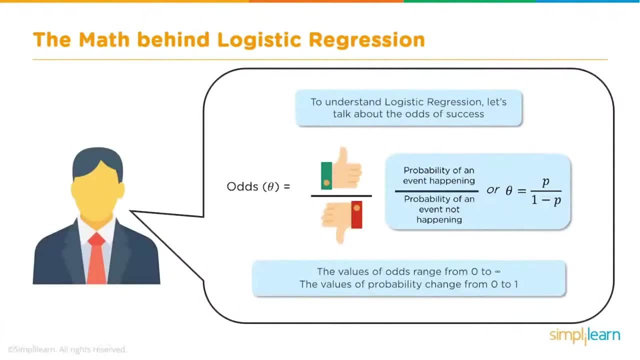 and then slowly, at certain rating, they get promotion. So that is a gradual process And this is all the math behind. This is how logistic regression looks. So we are trying to find the odds for a particular event happening, And this is the formula for finding the odds. 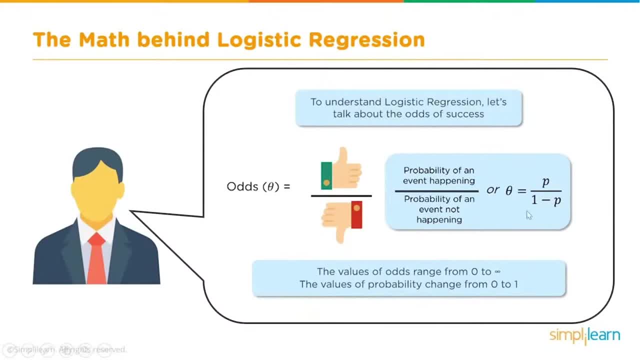 So the probability of an event happening divided by the probability of the event not happening, So P. if it is the probability of the event happening, probability of the person getting a promotion, and divided by the probability of the person not getting a promotion, that is one minus P. 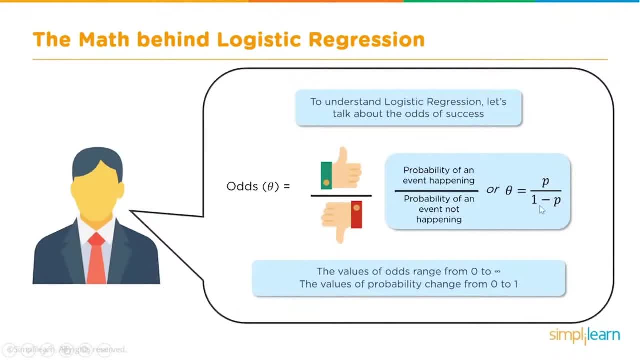 So this is how you measure the odds. Now. the values of the odds range from zero to infinity. So when this probability is zero, then the odds with the value of the odds is equal to zero, And when the probability becomes one, then the value of the odds is one by zero. that will be infinity. 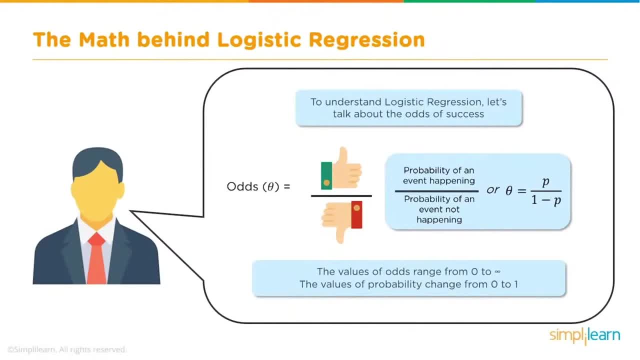 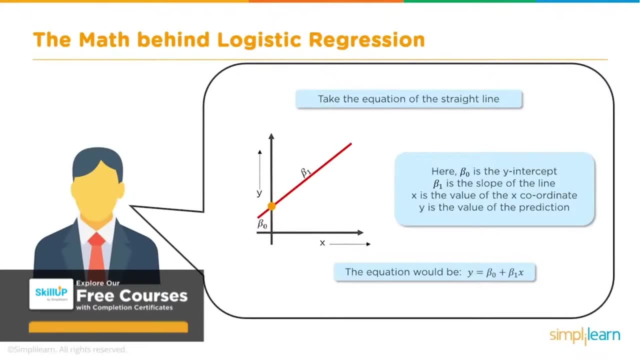 But the probability itself remains between zero and one. Now this is how an equation of a straight line looks. So y is equal to beta zero plus beta one, x, where beta zero is a y intercept And beta one is the slope of the line. 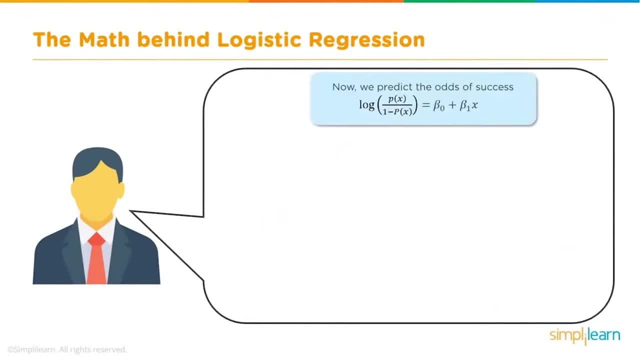 If we take the odds equation and take a log of both sides, then this would look somewhat like this, and the term logistic is actually derived from the fact that we are doing this. we take a log of Px by one minus Px. This is an extension of the calculation of odds that we have seen. 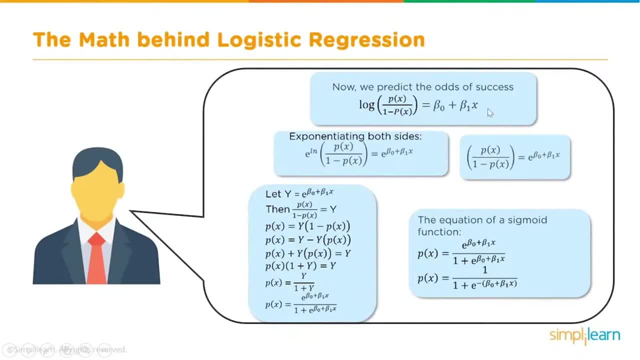 And that is equal to beta zero plus beta one, x, which is the equation of the straight line. And now from here, if you want to find out the value of Px, you will see we can take the exponential on both sides And then, if we solve that equation, we will get the equation of Px like this: 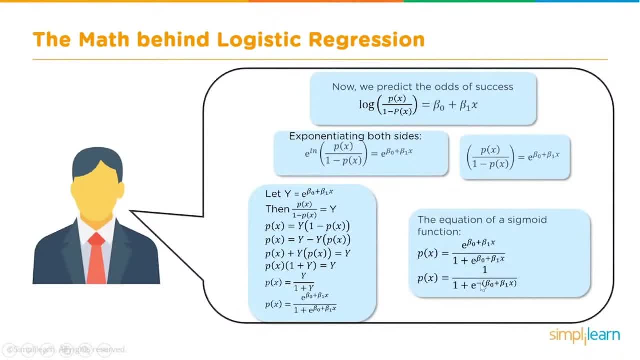 Px is equal to one by one plus e, to the power of minus beta zero plus beta one x. And recall, this is nothing but the equation of the line which is equal to y. y is equal to beta zero plus beta one x. 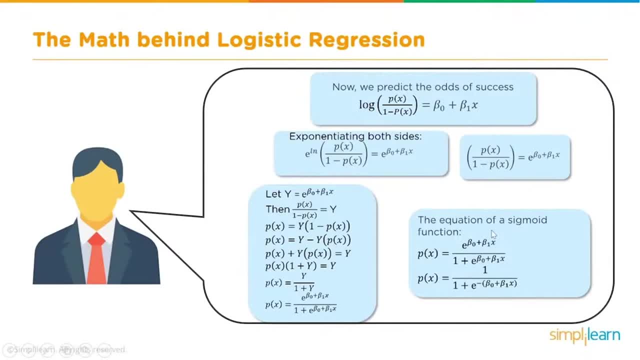 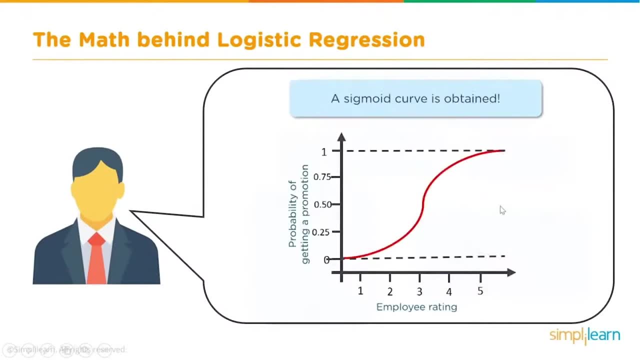 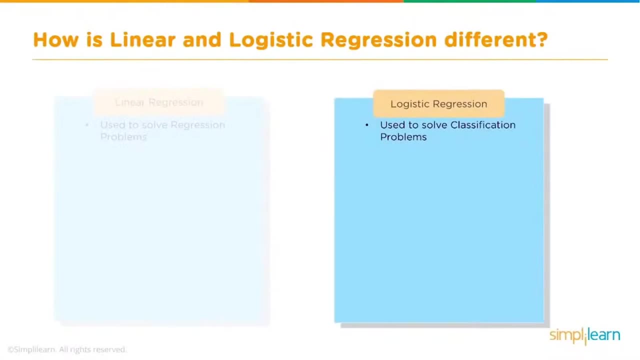 So that this is the equation also known as the sigmoid function And this is the equation of the logistic regression. And if this is plotted, this is how the sigmoid curve is obtained. So let's compare linear and logistic regression, how they are different from each other. 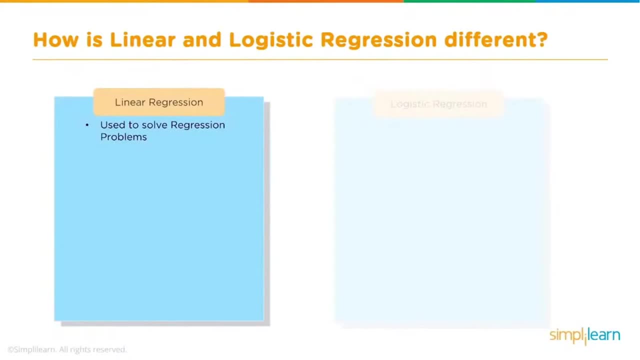 Let's go back. So linear regression is solved or used to solve regression problems And logistic regression is used to solve classification problems. So both are called regression. but linear regression is used for solving regression problems where we predict continuous values, whereas logistic regression is used for solving classification problems where we have had 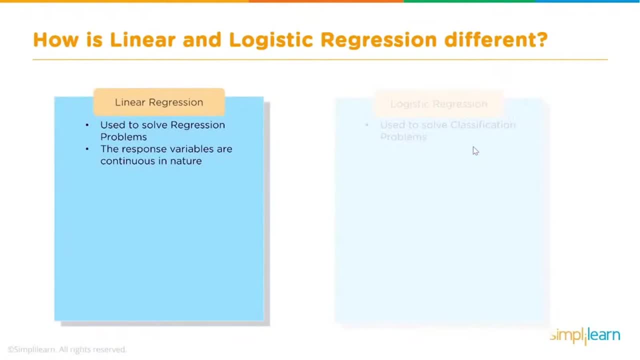 to predict discrete values. the response variables in case of linear regression are continuous in nature, whereas here they are categorical or discrete in nature. And linear regression helps to estimate the dependent variable when there is a change in the independent variable, Whereas here, in case of logistic regression, it helps to 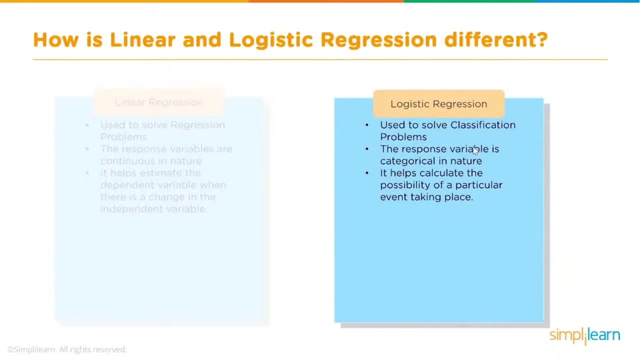 calculate the probability or the possibility of a particular event happening, And linear regression, as the name suggests, is a straight line. That's why it's called linear regression, whereas logistic regression is a sigmoid function and the curve is the shape of the curve is an S-shaped curve. 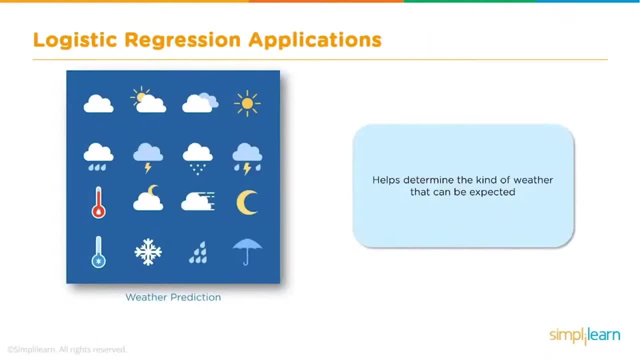 This is another example of application of logistic regression in weather prediction: whether it's going to rain or not rain. Now, keep in mind both are used in weather prediction If we want to find the discrete values like whether it's going to rain or not rain. 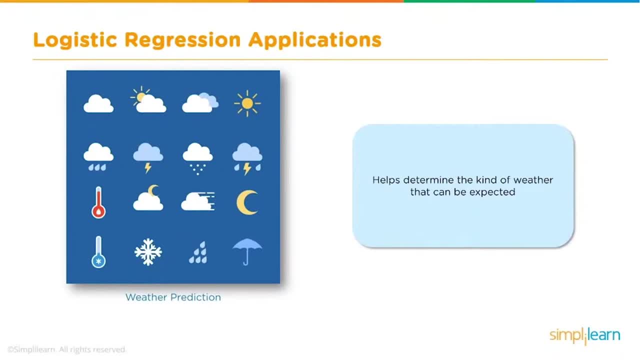 that is a classification problem. we use logistic regression. But if we want to determine what is going to be the temperature tomorrow, then we use linear regression. So just keep in mind that in weather prediction we actually use both. But these are some examples of logistic regression. 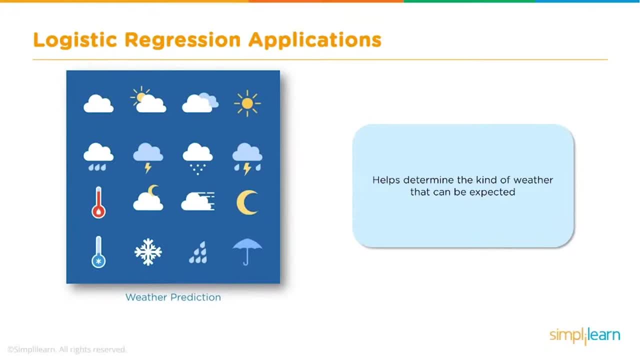 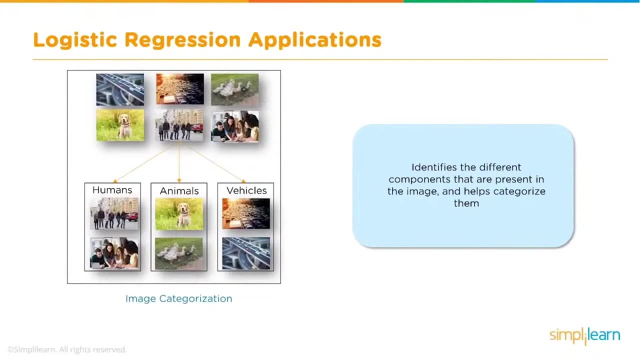 So we want to find out whether it's going to rain or not, whether it's going to be sunny or not, whether it's going to snow or not. These are all logistic regression examples. A few more examples: Classification of objects. This is again another example of logistic regression. 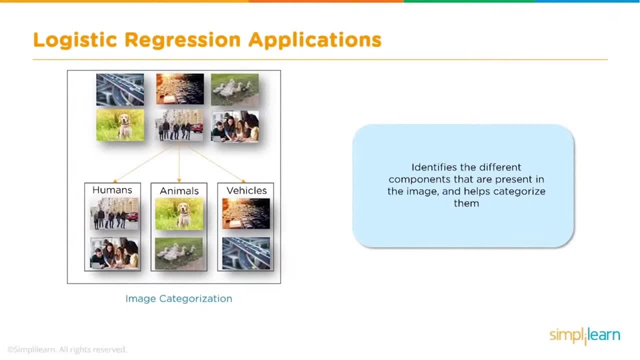 Now here, of course, one distinction is that these are multi-class classification, So logistic regression is not used in its original form, but it is used in a slightly different form. So we say: whether it is a dog or not a dog. 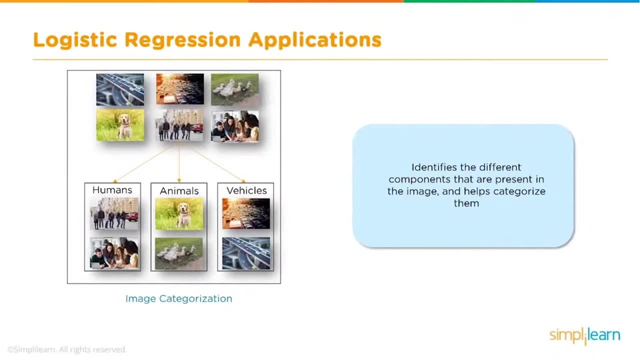 I hope you understand. So instead of saying is it a dog or a cat or elephant, we convert this into saying so, because we need to keep it to binary classification. So we say: is it a dog or not a dog, Is it a cat or not a cat? 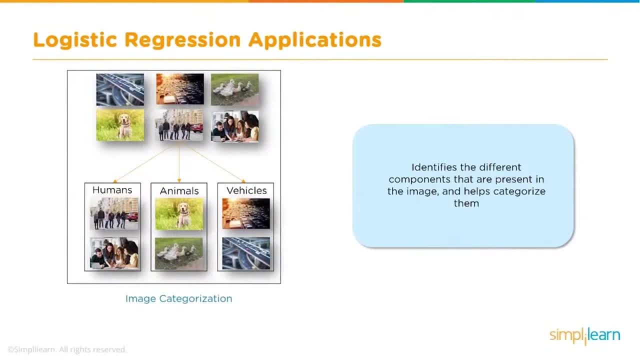 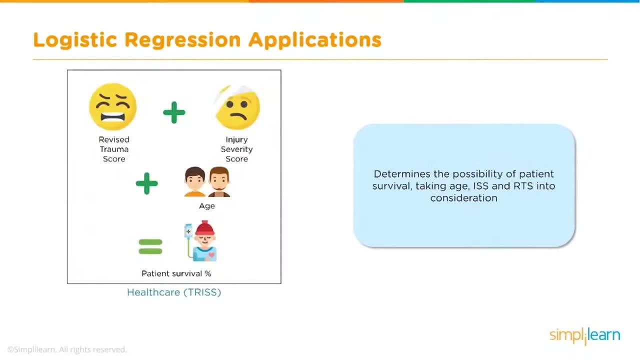 So that's the way logistic regression can be used for classifying objects. Otherwise, there are other techniques which can be used for performing multi-class classification. In healthcare, logistic regression is used to find the survival rate of a patient, So they take multiple parameters like trauma score and age, and so on and so forth. 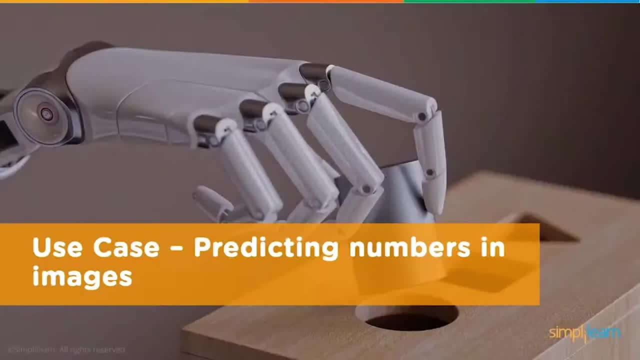 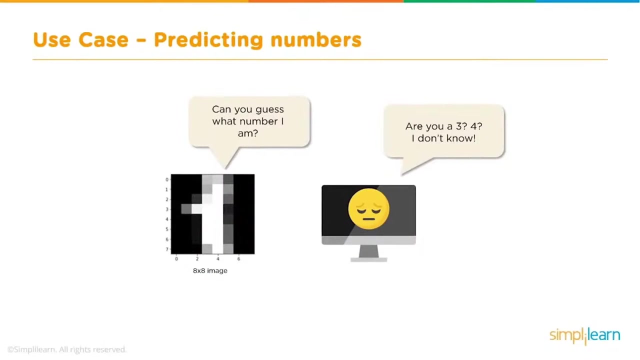 And they try to predict the rate of survival All right. Now, finally, let's take an example and see how we can apply logistic regression to predict the number that is shown in the image. So this is actually a live demo. I will take you into Jupyter Notebook and show the code. 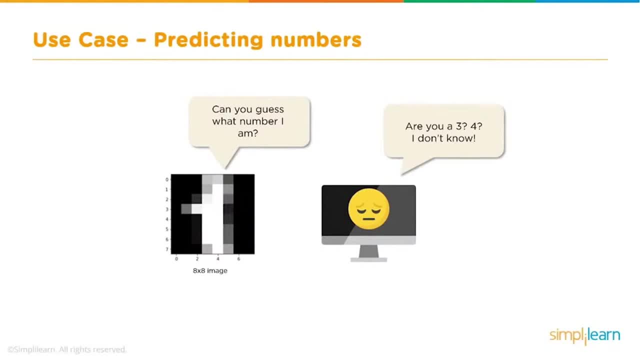 But before that let me take you through a couple of slides to explain what we are trying to do. So let's say you have an eight by eight image and the image has a number one, two, three, four, And you need to train your model to. 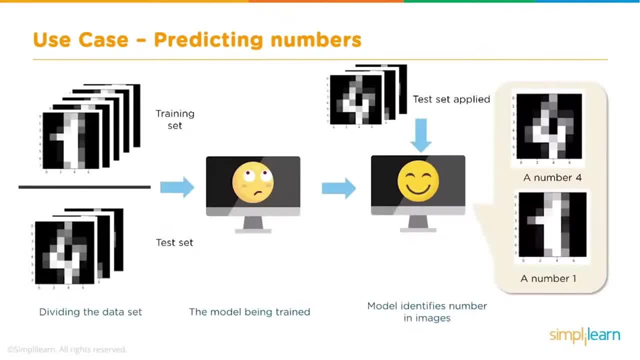 predict what this number is. So how do we do this? So, the first thing is obviously many machine learning process. You train your model. So in this case, we are using logistic regression, So, and then we provide a training set to train the model, and then we test how. 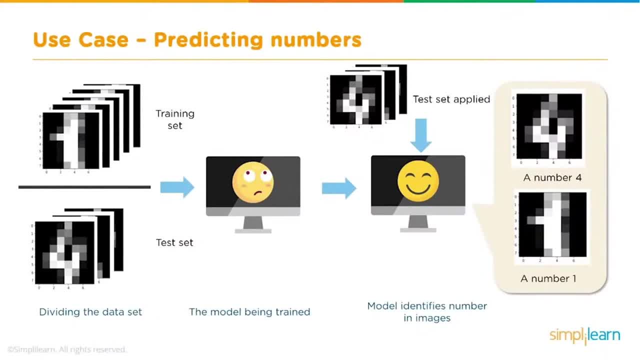 accurate. our model is with the test data, which means that, like any machine learning process, we split our initial data into two parts: training set and test set. With the training set, we train our model and then, with the test set, we test the model till we get good accuracy and then we use it for inference. 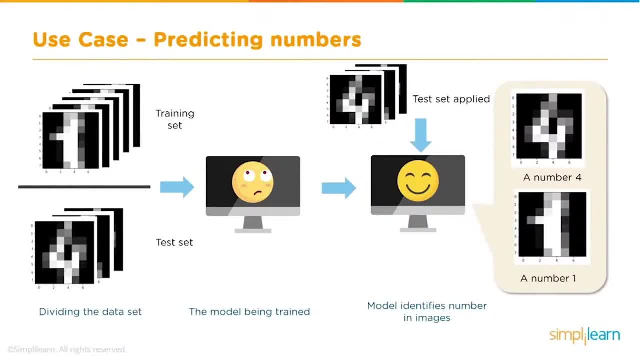 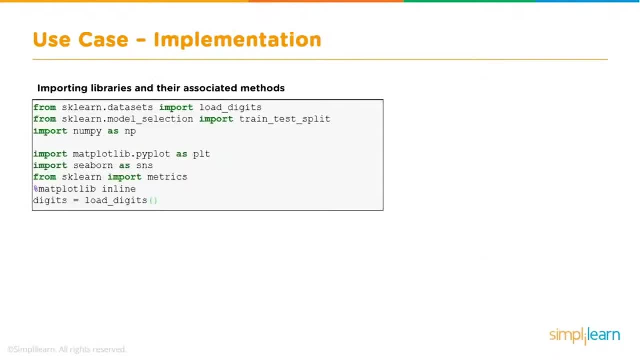 So that is typical methodology of training, testing and deploying of machine learning models. So let's take a look at the code and see what we are doing. So I will not go line by line, but just take you through some of the blocks. 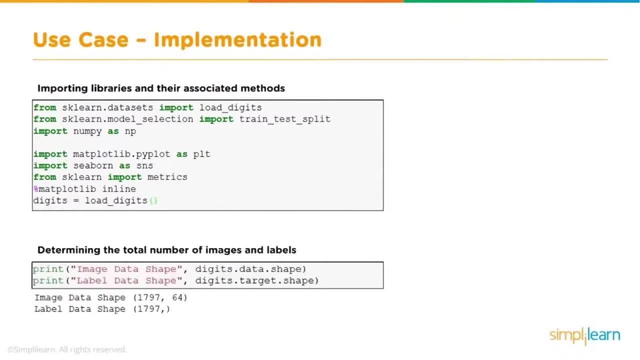 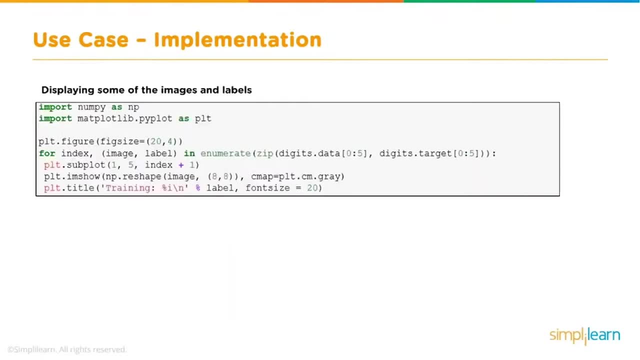 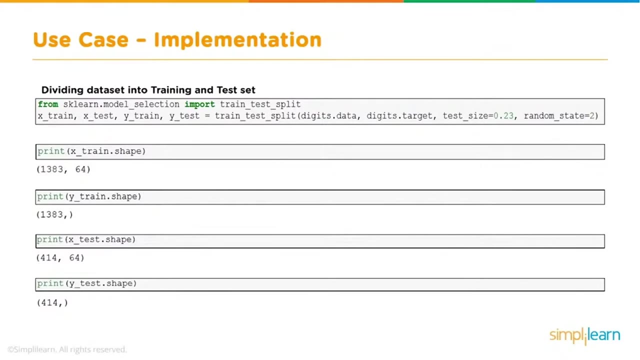 So first thing we do is import all the libraries and then we basically take a look at the images and see what is the total number of images we can display using Matplotlib- Some of the images are a sample of these images- And then we split the data into training and test, as I mentioned earlier. 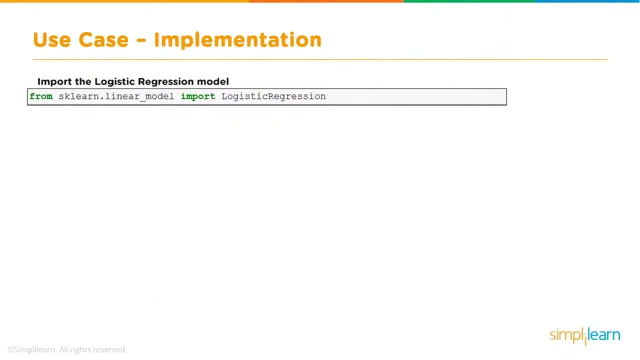 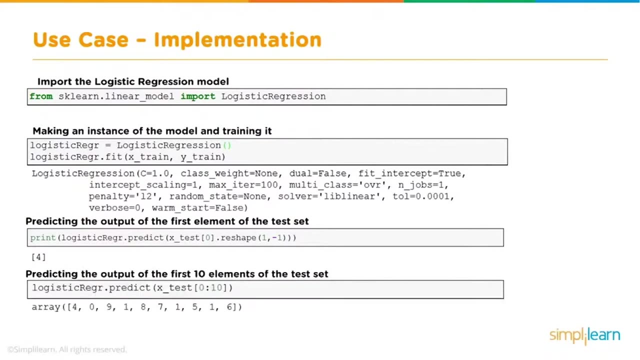 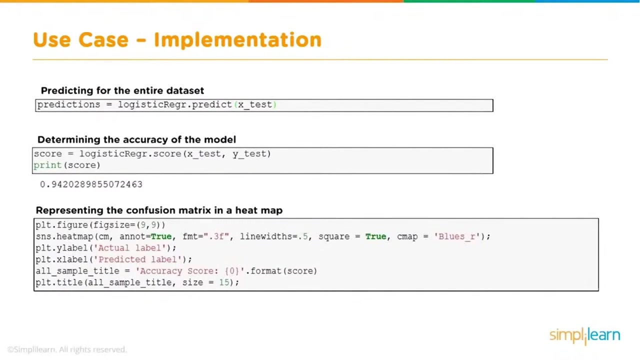 And we can do some exploratory analysis and then we build our model, We train our model with the training set and then we test it with our test set and find out how accurate our model is using the confusion matrix, the heat map, and use heat map for visualizing this. 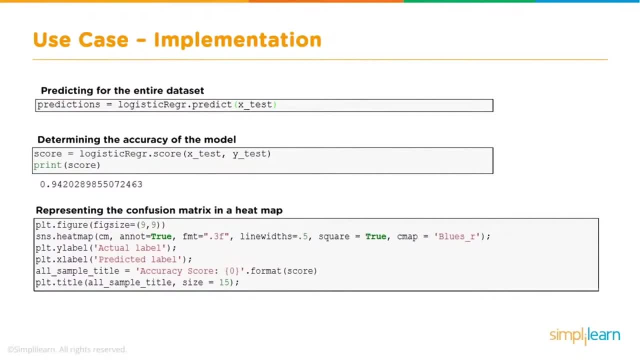 And I will show you in the code what exactly is the confusion matrix and how it can be used for finding the accuracy. In our example, we get an accuracy of about 0.94,, which is pretty good, or 94%, which is pretty good. 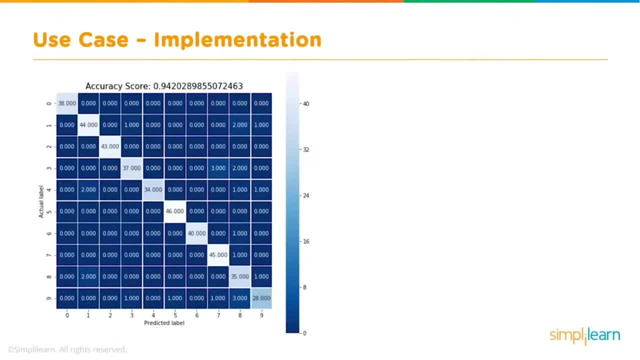 All right. So what is the confusion matrix? This is an example of a confusion matrix, and this is used for identifying the accuracy of a classification model, like a logistic regression model. So the most important part in a confusion matrix is that. first of all, this: as you 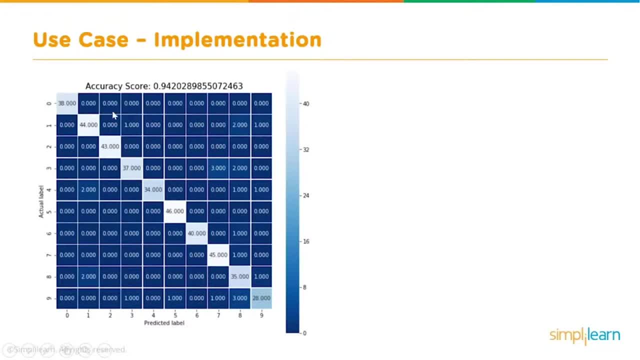 can see, this is a matrix, and the size of the matrix depends on how many outputs we are expecting, Right. So the most important part here is that the model will be most accurate when we have the maximum numbers in its diagonal, like in this case. 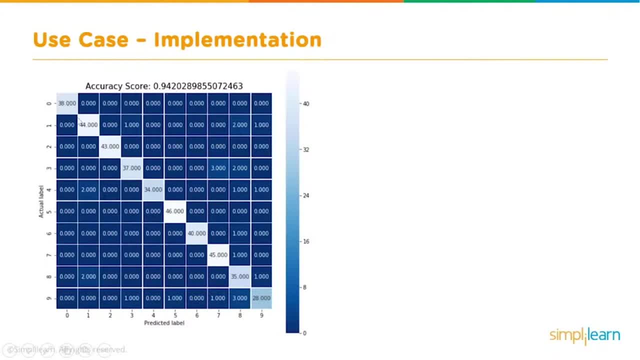 That's why it has almost 93, 94%, because the diagonal should have the maximum numbers And the others, other than diagonals, the cells other than the diagonal, should have very few numbers. So here that's what is happening. So there is a two here. 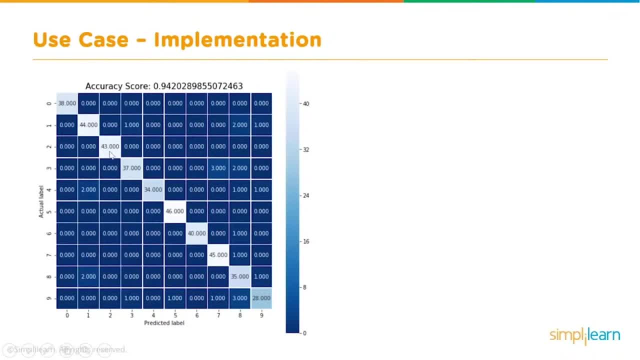 There are. there's a one here, but most of them are along the diagonal This. what does this mean? This means that the number that has been fed is zero and the number that has been detected is also zero, So the predicted value and the actual value are the same. 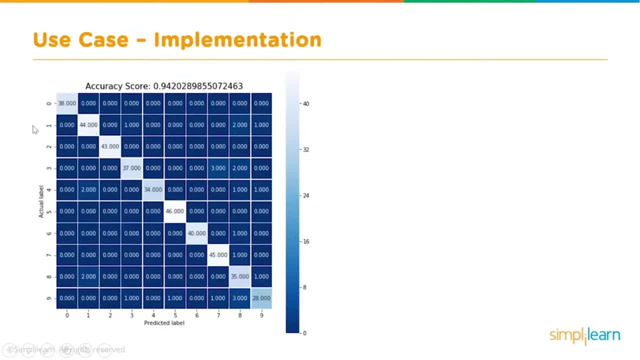 So along the diagonals. that is true, Which means that let's, let's take this diagonal Right. If the maximum number is here, that means that, like here, in this case, it is 34, which means that 34 of the images. 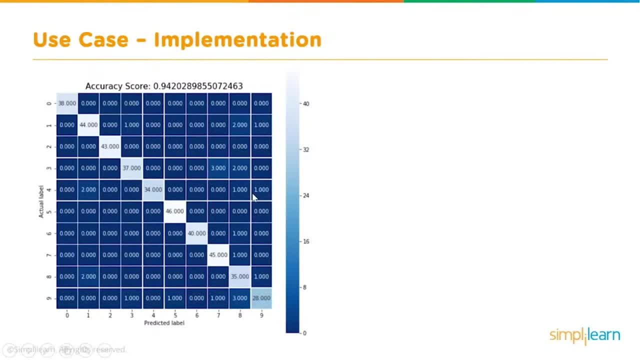 that have been fed, or rather, actually there are two misclassifications in there. So 36 images have been fed which have number four, and out of which 34 have been predicted correctly as number four and one has been predicted as number eight. 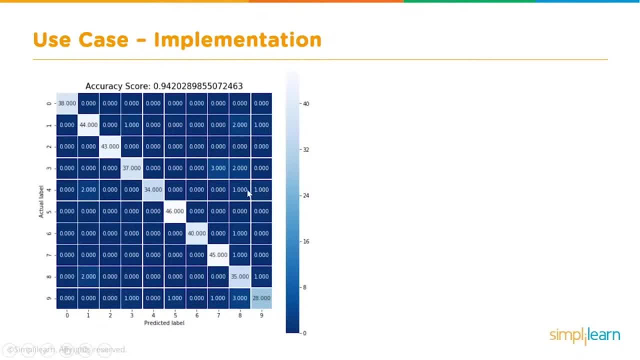 and another one has been predicted as number nine. So these are two misclassifications. OK, so that is the meaning of saying that the maximum number should be in the diagonal. So, if you have all of them, so for an ideal model which has, let's say, 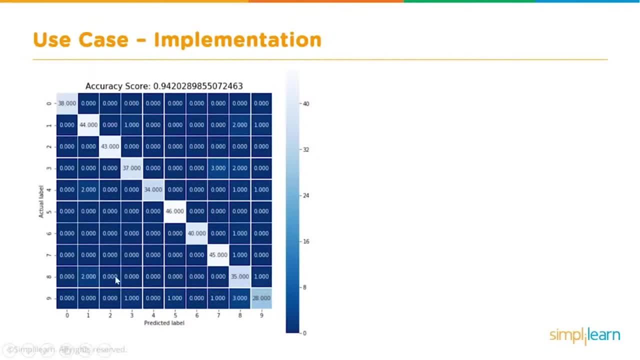 100 percent accuracy. everything will be only in the diagonal. There will be no numbers other than zero in all other cells. But that is like 100 percent accurate model. OK, so that's just how to use this matrix, how to use this confusion matrix. 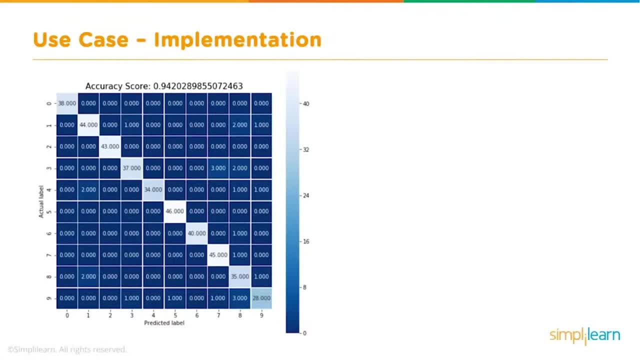 I know the name is a little funny sounding- confusion matrix- but actually it is not very confusing, It's very straightforward. So you are just plotting what has been predicted and what is the label, information or what is the actual data. that's also known as the ground truth sometimes. 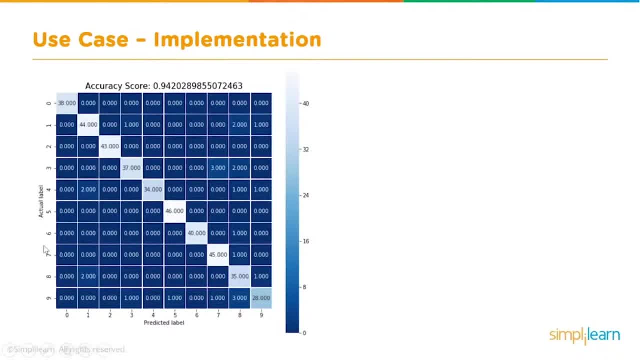 These are some fancy terms that are used: predicted label and the actual label. that's all it is OK. yeah, so we are showing a little bit more information here. So 38 have been predicted, and here you will see that all of them have been predicted correctly. 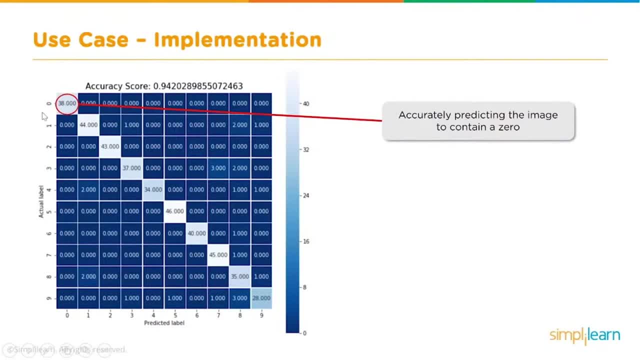 There have been 38 zeros and the predicted value and the actual value is exactly the same, Whereas in this case, right it has. there are, I think, 37 plus five. Forty two have been fed the images. Forty two images are of digit three and the accuracy is only 37 of them have been accurately predicted. 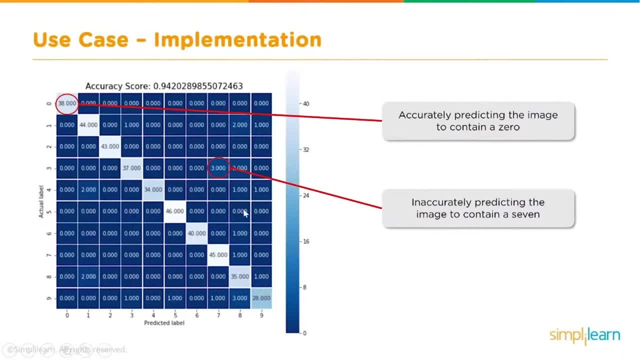 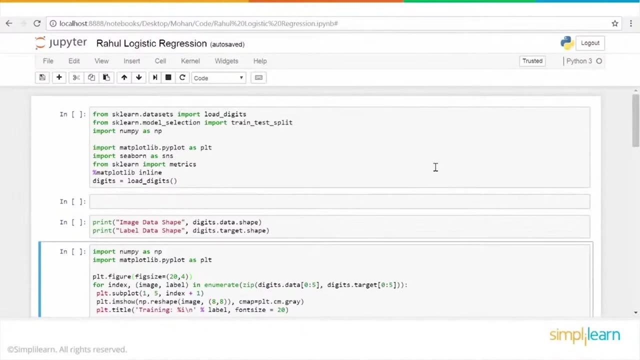 Three of them have been predicted as number seven, and two of them have been predicted as number eight, and so on And so forth. OK, All right. So with that let's go into Jupyter Notebook and see how the code looks. So this is the code in in Jupyter Notebook for logistic regression. 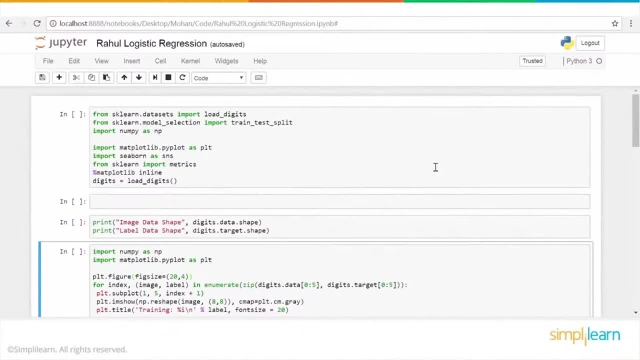 In this particular demo, what we are going to do is train our model to recognize digits, which are the images which have digits from, let's say, zero to five or zero to nine, And and then we will see how well it is trained. 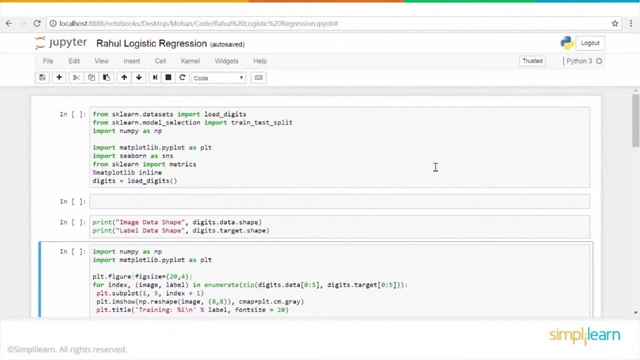 Whether it is able to predict these numbers correctly or not. So let's get started. So the first part is as usual- we are importing some libraries that are required- And then the last line and this block is to load the digits. So let's go ahead and run this code. 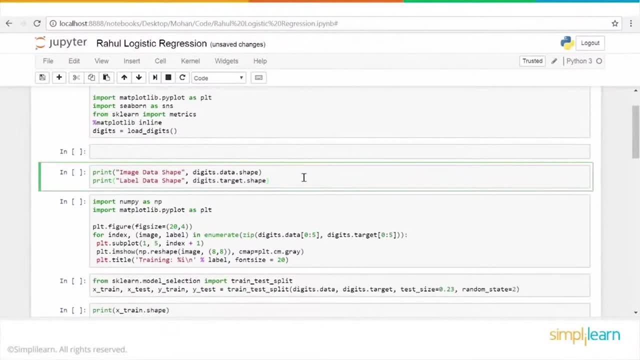 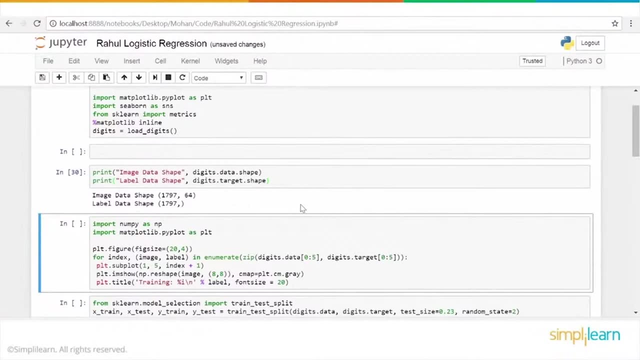 Then here we will visualize the shape of these digits. So we can see here, if we take a look, and this is how the shape is: So 1797 by 64. These are like eight by eight images. So that's, that's what is reflected in this shape. 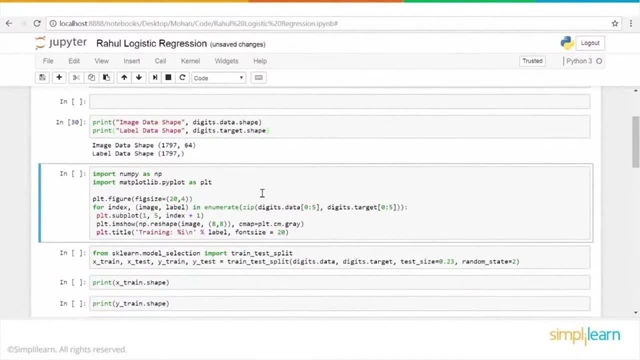 Now, from here onwards, we are basically once again importing some of the libraries that are required, like NumPy and Matplot, And we will take a look at some of the sample images that we have loaded. So this one, for example, creates a figure. 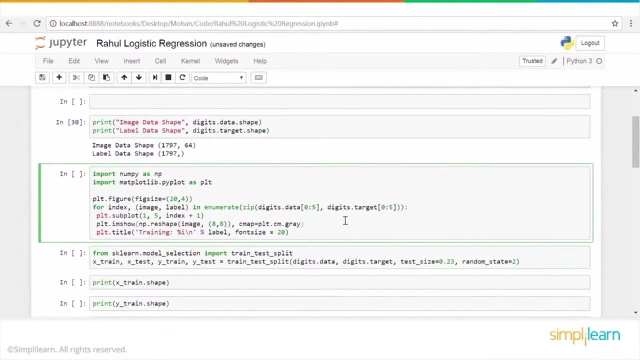 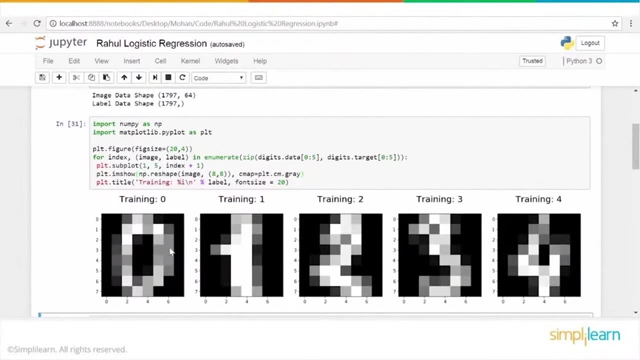 And then we go ahead and take a few sample images to see how they look. So let me run this code so that it becomes easy to understand. So these are about five images, sample images that we are looking at: Zero, one, two, three, four. 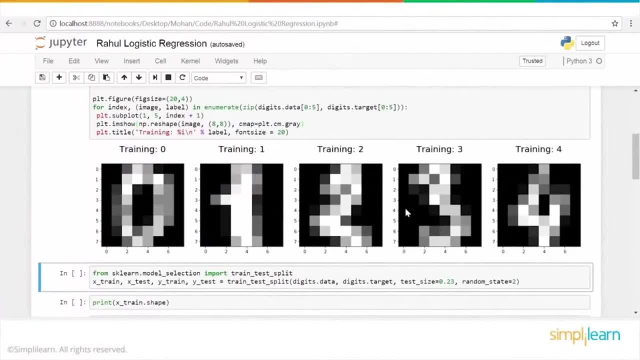 So this is how the images, this is how the data is OK, and based on this we will actually train our logistic regression model and then we will test it and see how well it is able to recognize. So the way it works is the pixel information. 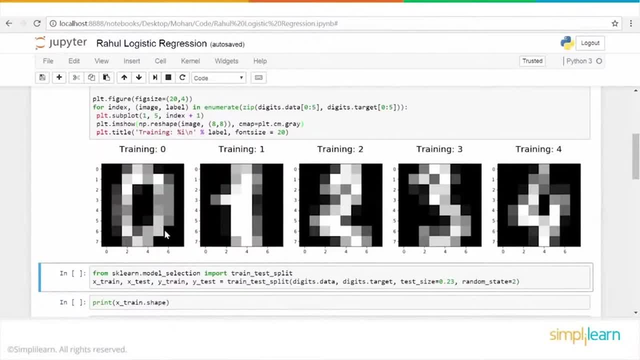 So, as you can see here, this is an eight By eight pixel kind of image and the each pixel whether it is activated or not activated. that is the information available for each pixel. Now, based on the pattern of this activation and non activation of the various pixels, this will be identified. 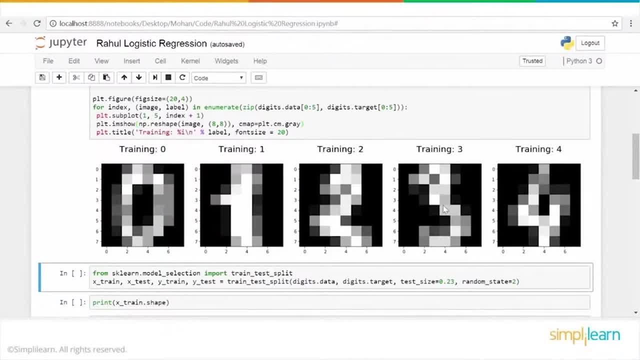 as a zero, for example. right, similarly as you can see. So overall, each of these numbers actually has a different pattern of the pixel, and that's pretty much that our model needs to learn. for which number? What is the pattern of the activation of the pixels? 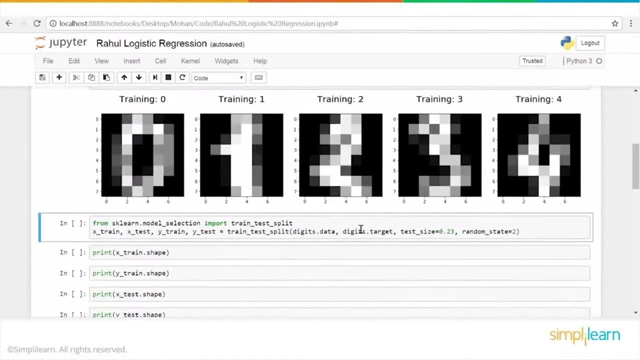 Right, So that is what we are going to train our model. OK, so the first thing we need to do is to split our data into training and test data set, Right? So whenever we perform any training, we split the data into training and tests so that the training data set is used. 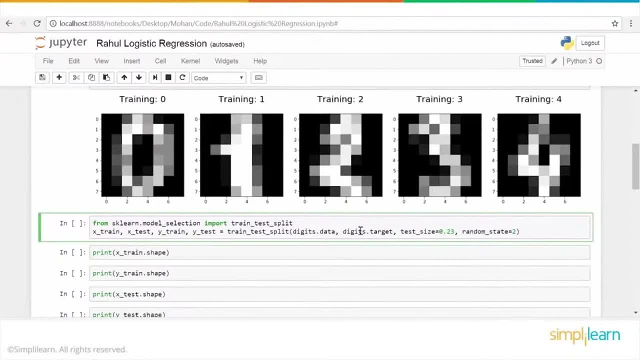 to train the system. So we pass this probably multiple times and then we test it with the test data set And the split is usually in the form of that, And there are various ways in which you can split this data. It is up to the individual preferences. 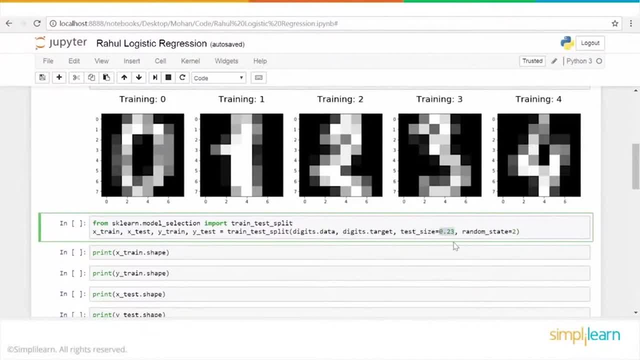 In our case, here we are splitting in the form of twenty three and seventy seven. So when we say test size as twenty point two, three, that means twenty three percent of that entire data is used for testing and the remaining seventy seven percent is used for training. 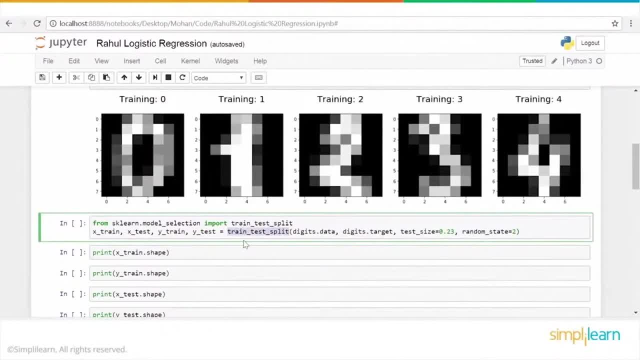 So there is a readily available function which is called train test split. So we don't have to write any special code for the splitting. It will automatically split the data based on the proportion that we give here, which is test size. So we just give the test size automatically. 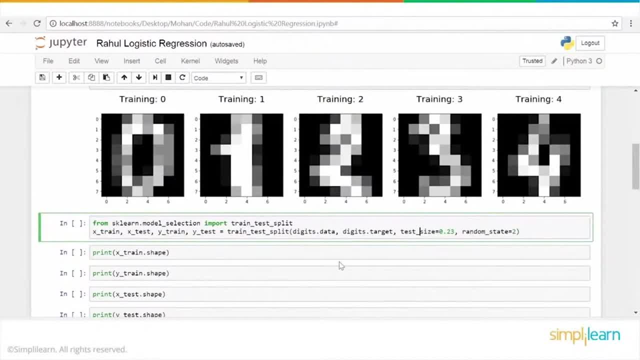 Training size will be determined and we pass the data that we want to split And the results will be stored in X underscore train and Y underscore train for the training data set. And what is X underscore train? These are, these are the features, right. 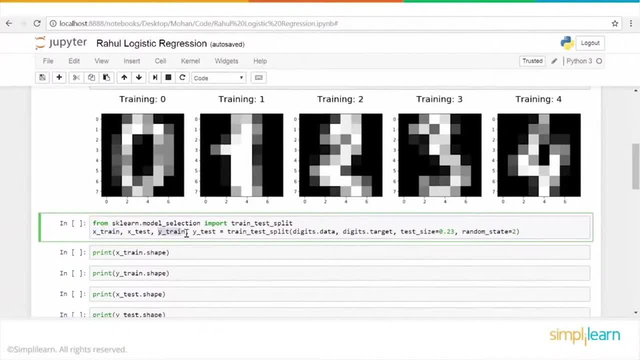 Which is like the independent variable, and Y underscore train is the label Right. So in this case, what happens is we have the input value, which is all the features value, which is in X underscore train, And since this is the labeled data for each of them, each of the observations, 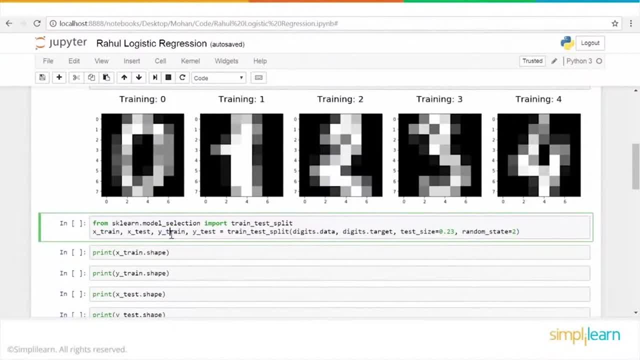 we already have the label information saying whether this digit is a zero or a one or a two, so that this is what will be used for comparison to find out whether the system is able to recognize it correctly or there is an error. for each observation, it will compare with this Right. 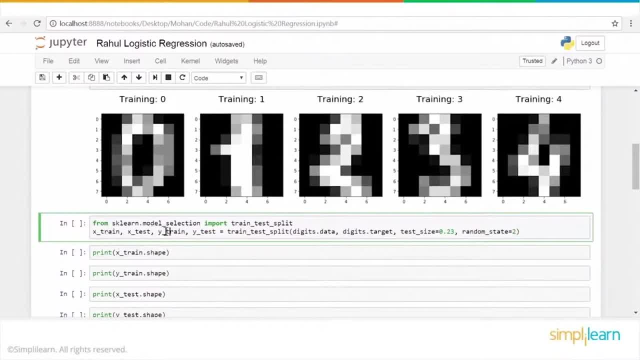 So this is the label. So the same way, X underscore train, Y underscore train is for the training data set, X underscore test, Y underscore test is for the test data set. OK, so let me go ahead and execute this code as well. 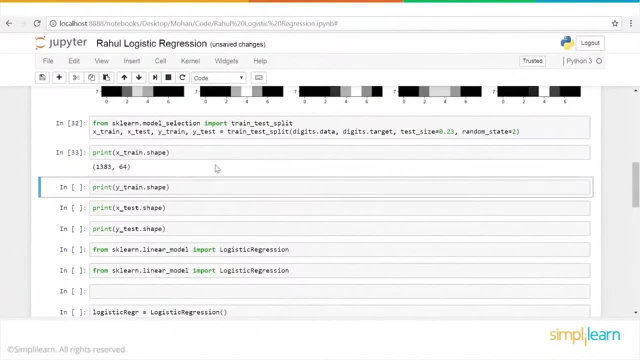 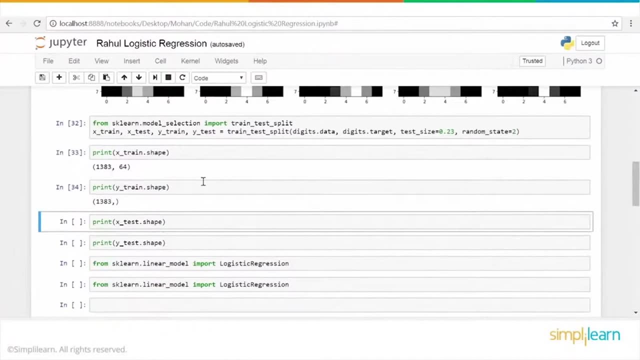 And then we can go and check quickly what is the, how many entries are there, And in each of these X underscore train the shape is 1383 by 64. And Y underscore train has 1383. because there is nothing like the second part is not required here. 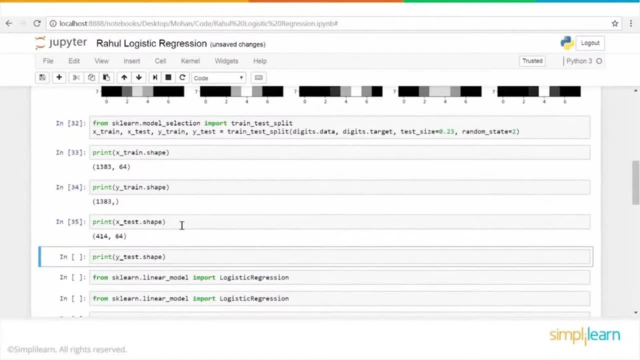 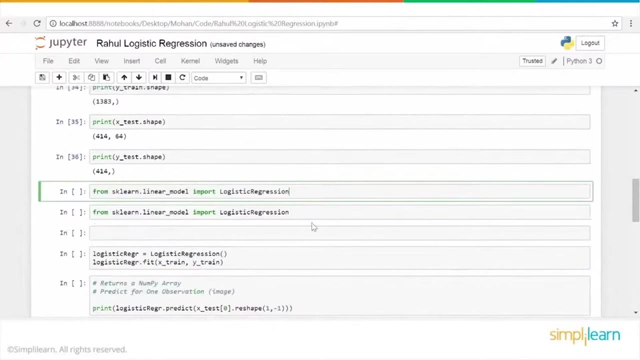 And then X underscore test shape we see is 414.. So actually there are 414 observations in test and 1383 observations in train. So that's basically what these four lines of code are saying. OK, Then we import the logistic regression library and which is a part of scikit-learn. 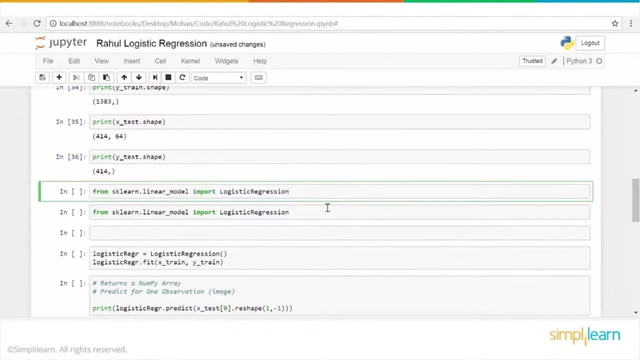 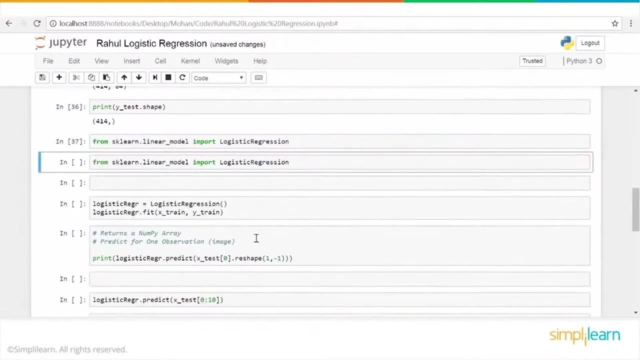 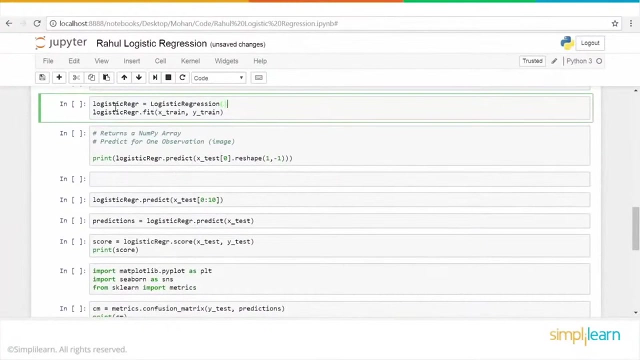 So we don't have to implement the logistic regression process itself. We just call these the function, And let me go ahead and execute that so that we have the logistic regression library imported. Now we create an instance of logistic regression. So logistic REGR is is an instance of logistic regression. 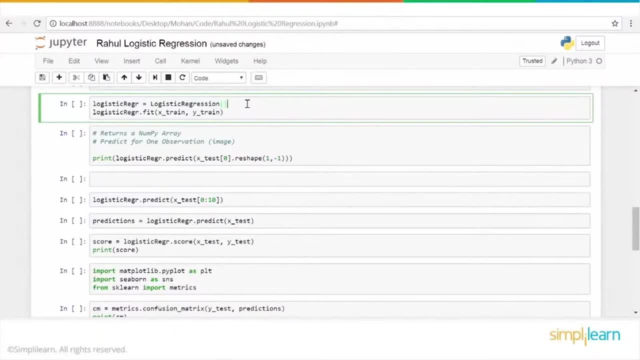 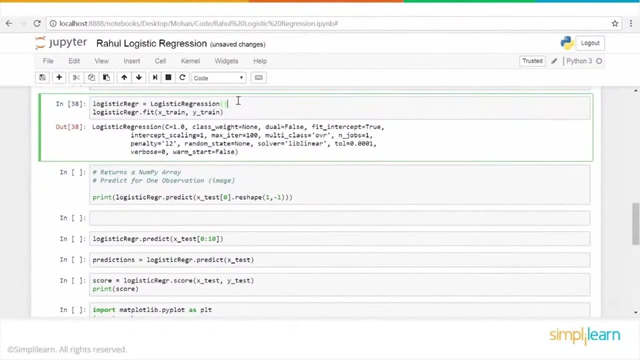 And then we use that for training our model. So let me first execute this code, So these two lines. So the first line basically creates an instance of logistic regression model, And then the second line is where we are passing our data, the training data set. 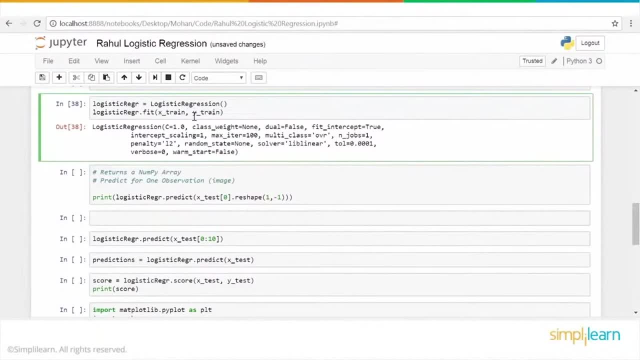 And this is our, the predictors, And this is our target. We are passing this data set to train our model, All right. So once we do this, in this case the data is not large, But by and large, the training is what takes usually a lot of time. 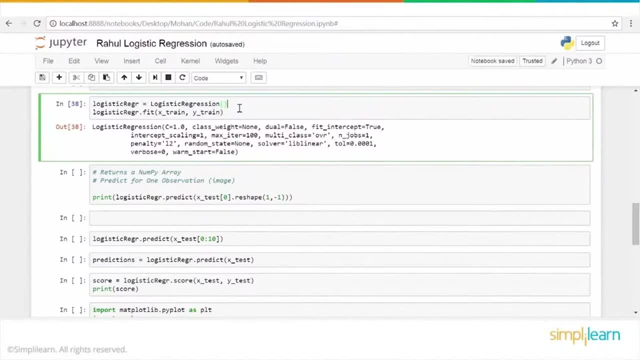 So we spend in machine learning activities and machine learning projects. We spend a lot of time for the training part of it. OK, so here the data set is relatively small, So it was pretty quick. So all right. So now our model has been trained using 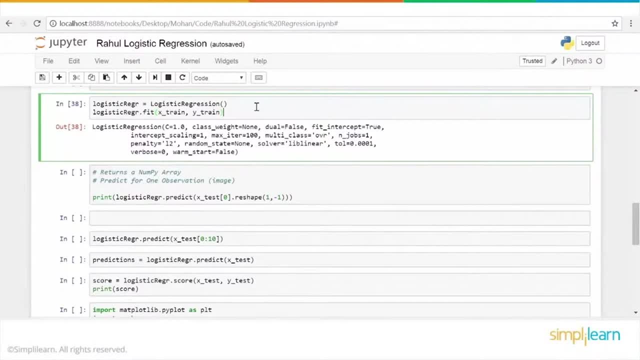 the training data set and we want to see how accurate this is. So what we'll do is we will test it out in probably phases, So let me first Check out how well this is working for one image. OK, I'll just try it out with one image. 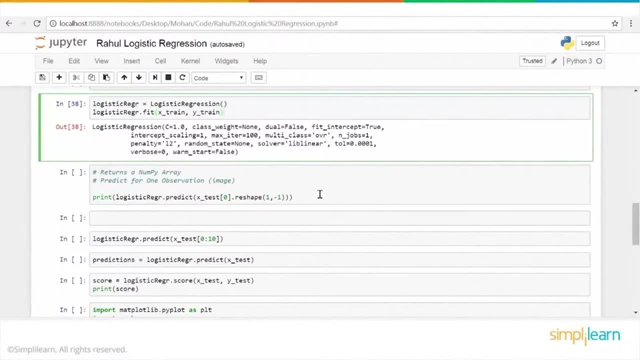 My the first entry in my test data set and see whether it is correctly predicting or not. So, and in order to test it, So for training purpose, we use the fit method. There is a method called fit, which is for training the model. 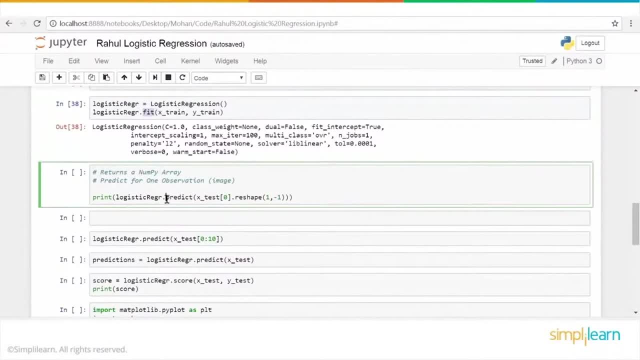 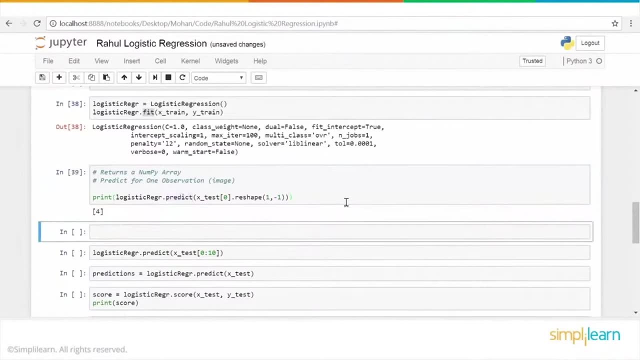 And once the training is done, if you want to test for a particular value- new input- you use the predict method. OK, So let's run the predict method and we pass this particular image And we see that the shape is or the prediction is four. 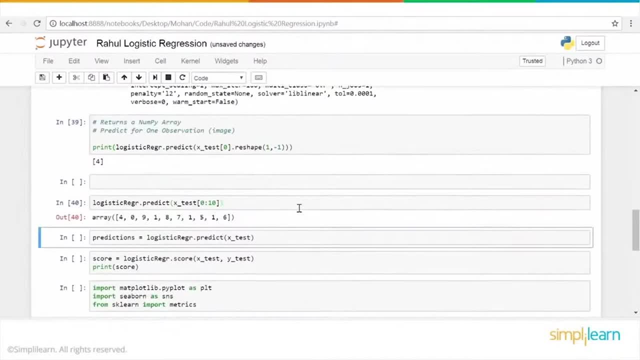 So let's try a few more. Let me see for the next 10 seems to be fine, So let me just go ahead and test the entire data set. OK, that's basically what we will do, So now we want to find out how accurately this has performed. 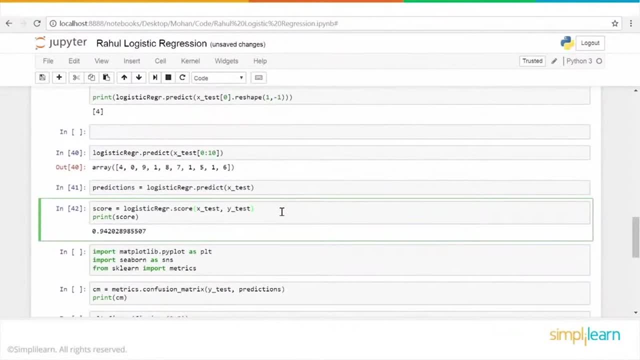 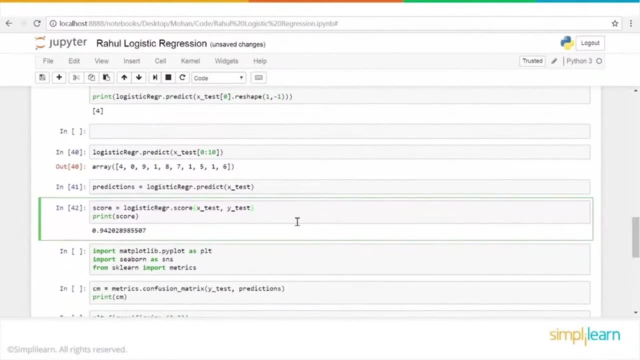 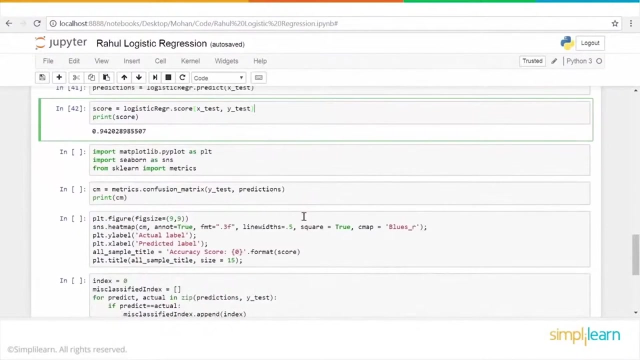 So we use the score method to find what is the percentage of accuracy, and we see here that it has performed up to ninety four percent accurate. OK, so that's on this part. Now, what we can also do is we can also see this accuracy using what is known as. 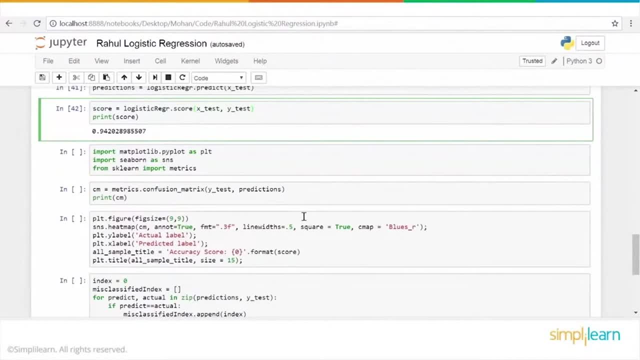 a confusion matrix. So let us go ahead and try that as well, so that we can also visualize how well this model has done. So let me execute this piece of code, which will basically import some entries that are required, and we basically create a confusion matrix. 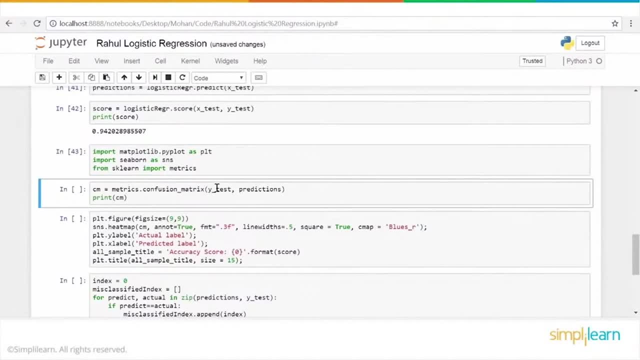 an instance of confusion matrix by running confusion matrix and passing these values. So we have. so this confusion underscore matrix method takes two parameters: One is the Y underscore test and the other is the prediction. So what is the Y underscore test? These are the labeled values which we already know for the test data set. 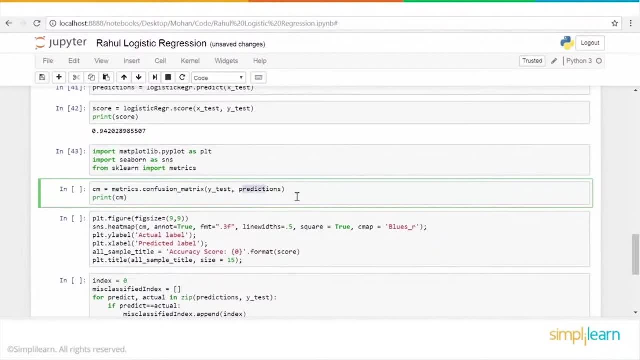 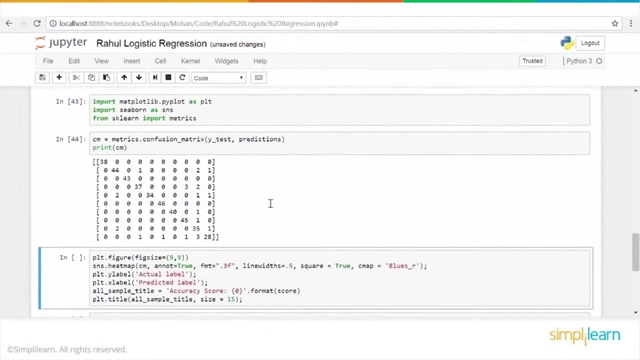 And predictions are what the system has predicted for the test data set. OK, so this is known to us and this is what the system has, The model has generated. So we kind of create the confusion matrix and we will print it. And this is how the confusion matrix looks. 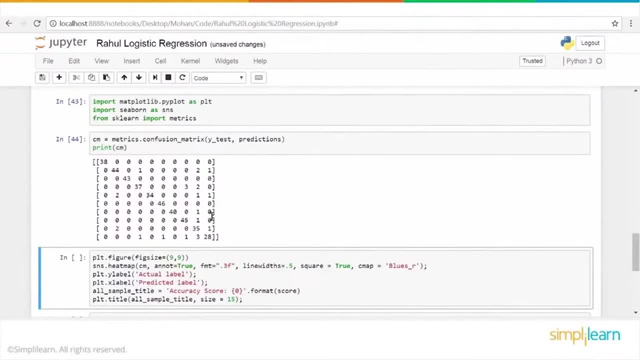 As the name suggests, it is a matrix And the key point out here is that the accuracy of the model is determined by how many numbers are there in the diagonal. The more the numbers in the diagonal, the better the accuracy is. OK. and first of all, the total sum of all the numbers in this. 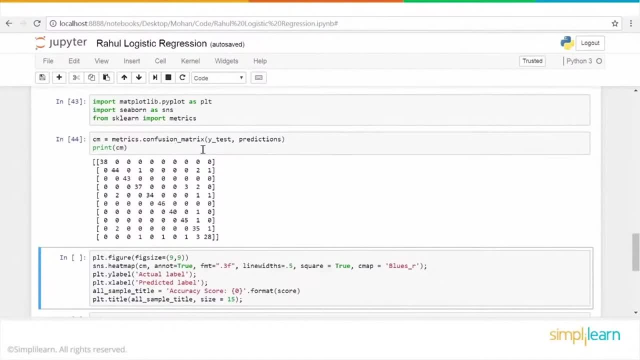 whole matrix is equal to the number of observations in the test data set. That is the first thing. So if you add up all these numbers, that will be equal to the number of observations in that test data set, And then out of that the maximum number of them should be in the diagonal. 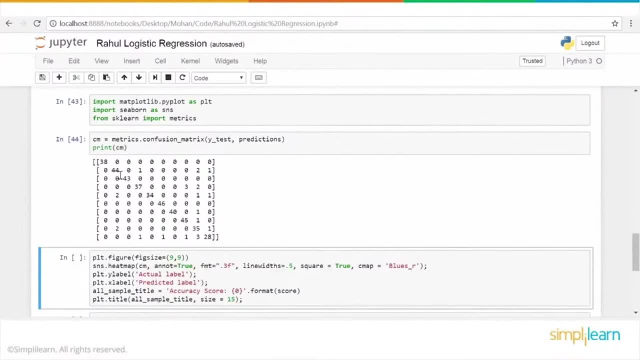 That means the accuracy. The accuracy is pretty good if the numbers in the diagonal are less And in all other places there are a lot of numbers, which means the accuracy is very low. The diagonal indicates a correct prediction. This means that the actual value is same as the predicted value. 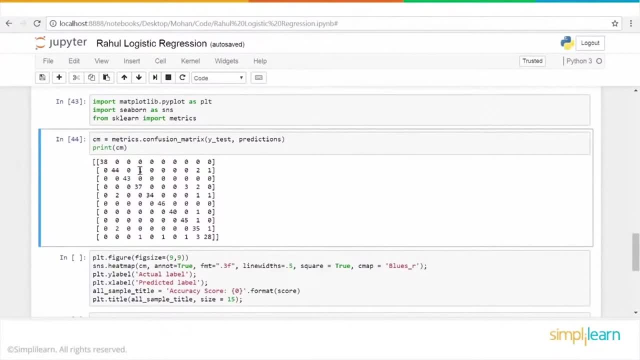 Here again, actual value is same as the predicted value, and so on. Right? So the moment you see a number here, that means the actual value is something and the predicted value is something else, Right? Similarly, here, the actual value is something and the predicted value is. 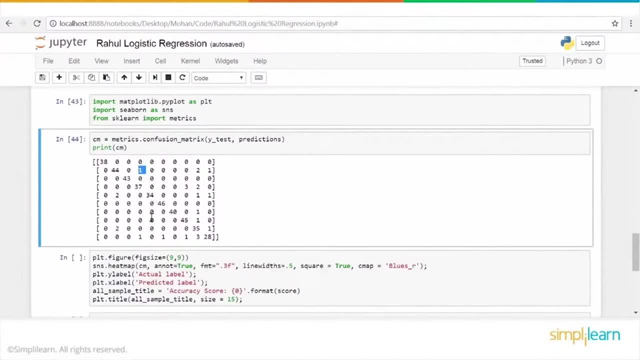 something else. So that is basically how we read the confusion matrix. Now how do we find the accuracy? You can actually add up the total values in the diagonal, So it's like 38 plus 44 plus 43 and so on. 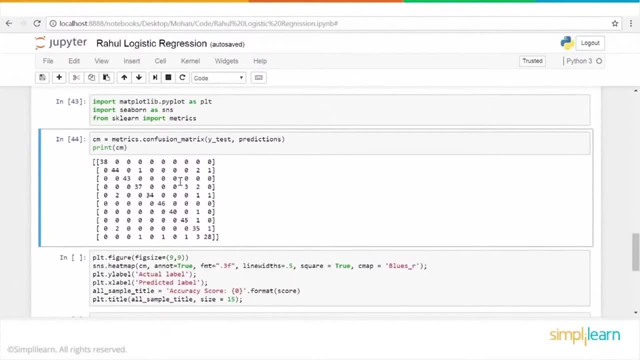 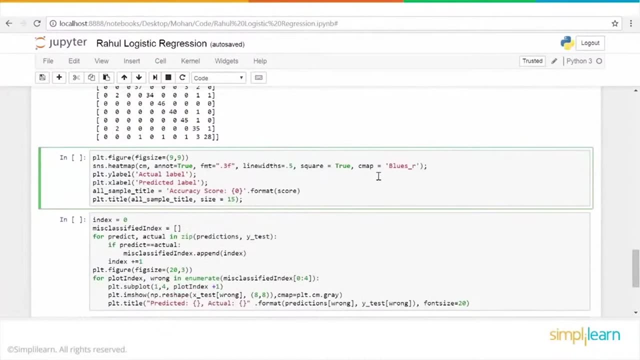 And divide that by the total number of test observations. that will give you the percentage accuracy using a confusion matrix. Now let us visualize this confusion matrix in a slightly more sophisticated way, using a heat map. So we will create a heat map with some. we'll add some colors as well. 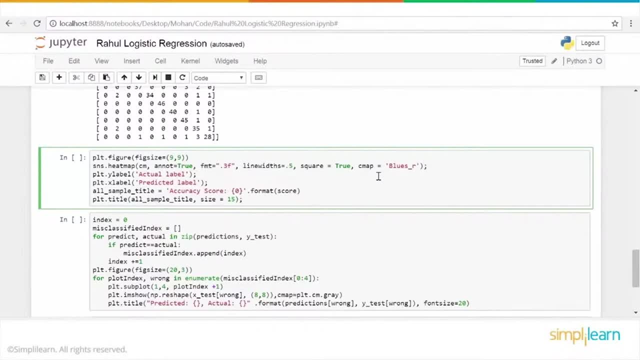 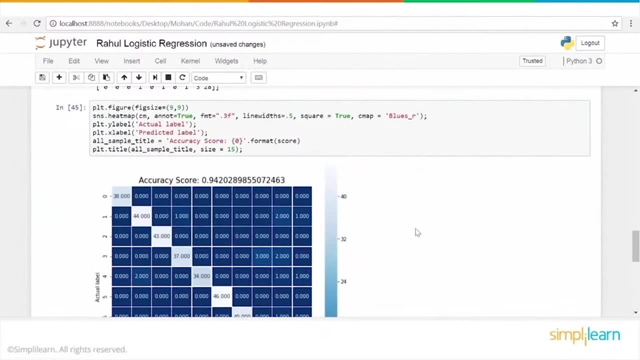 It's, it's like a more visually, visually more appealing. So that's the whole idea. So if we let me run this piece of code and this is how the heat map looks, And as you can see here, the diagonals again are all the values are here: 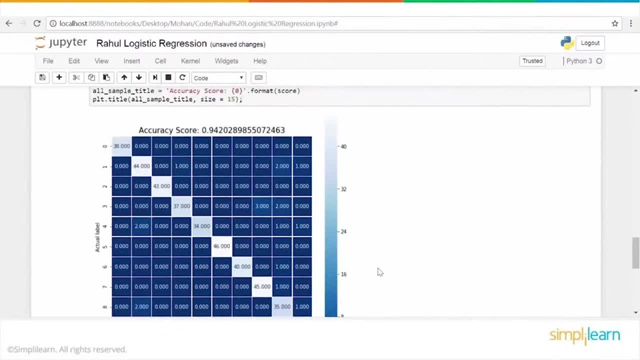 Most of the values. So, which means reasonably, this seems to be reasonably accurate And, yeah, basically the accuracy score is 94 percent. This is calculated, as I mentioned, by adding all these numbers divided by the total test values or the total number of observations in test data set. 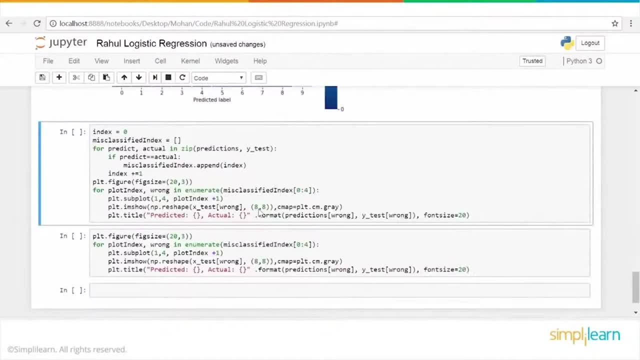 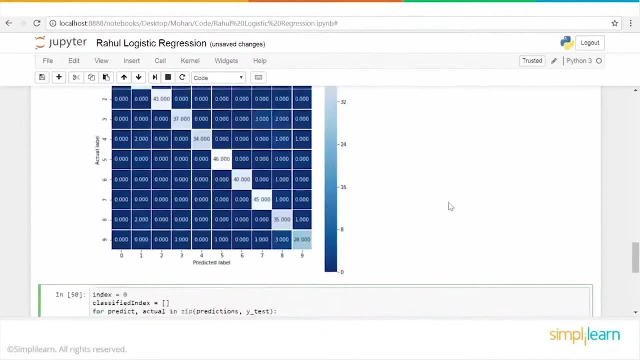 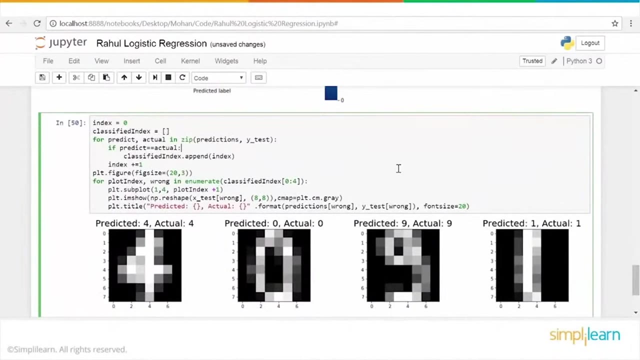 OK, so this is the confusion matrix for logistic regression. All right, so now that we have seen the confusion matrix, let's take a quick sample and see how well the system has classified and we will take a few examples of the data. So if we see here, we picked up randomly a few of them. 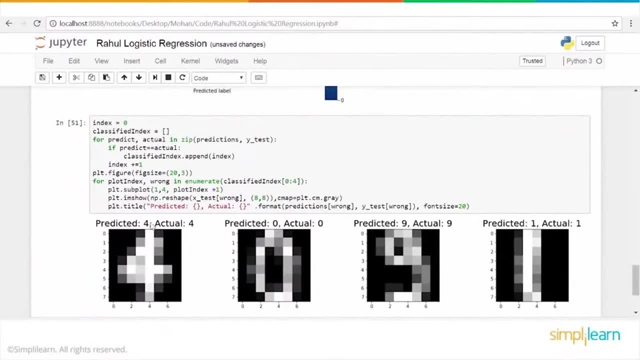 So this is number four, which is the actual value and also the predicted value. Both are four. This is an image of zero, So the predicted value is also zero. Actual values, of course, zero. Then this is the image of nine. 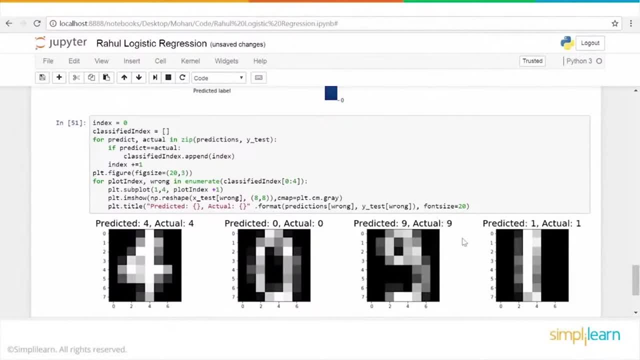 So this has also been predicted correctly: Nine and actual value is nine, And this is the image of one And again, this has been predicted correctly, as like the actual value. OK, so this was a quick demo of logistic regression: How to use logistic regression to identify images. 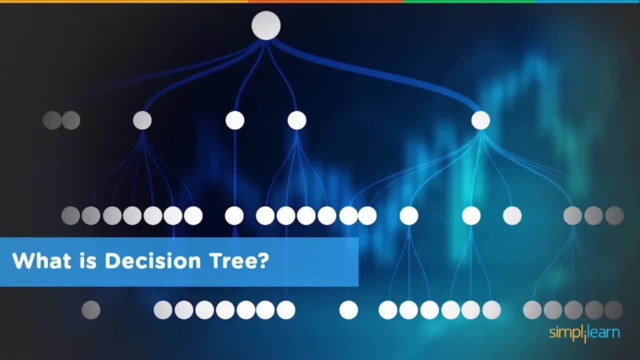 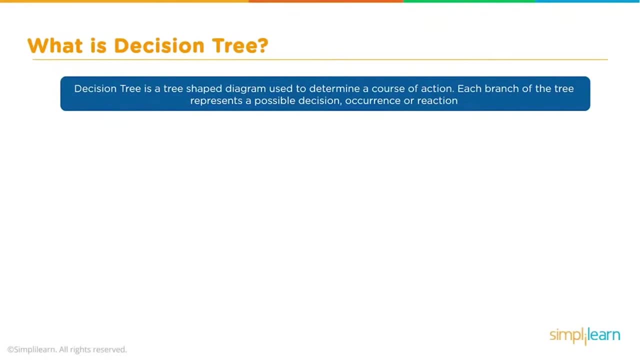 What is a decision tree? Let's go through a very simple example before we dig in deep. Decision tree is a tree shaped diagram used to determine a course of action. Each branch of the tree represents a possible decision or occurrence, or reaction. Let's start with a simple question. 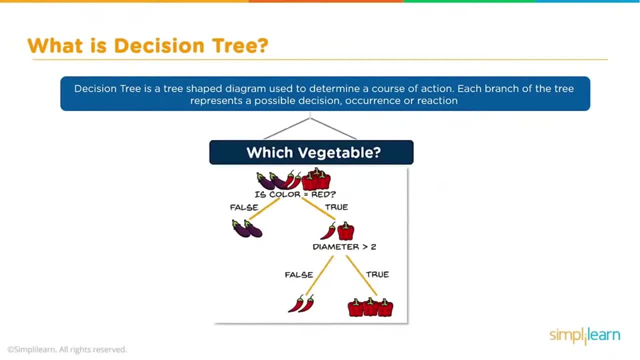 How to identify a random vegetable from a shopping bag. So we have this group of vegetables in here. We can start off by asking a simple question: Is it red? And if it's not, then it's going to be the purple fruit to the left. 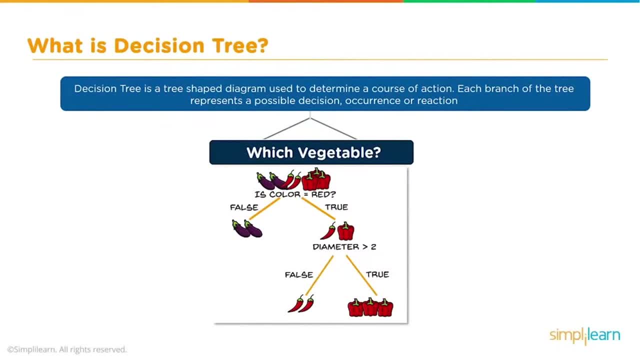 Probably an eggplant. If it's true, it's going to be one of the red fruits. Is a diameter greater than two? If false, it's going to be a what looks to be a red chili. And if it's true, it's going to be a bell pepper from the capsicum family. 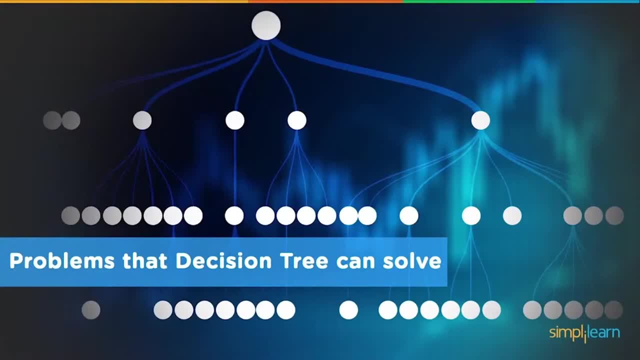 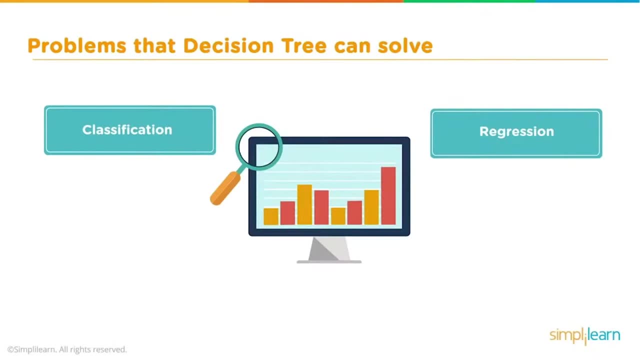 So it's a capsicum- Problems that decision tree can solve. So let's look at the two different categories the decision tree can be used on. It can be used on the classification- Is it true, false, yes, no. And it can be used on regression, where we 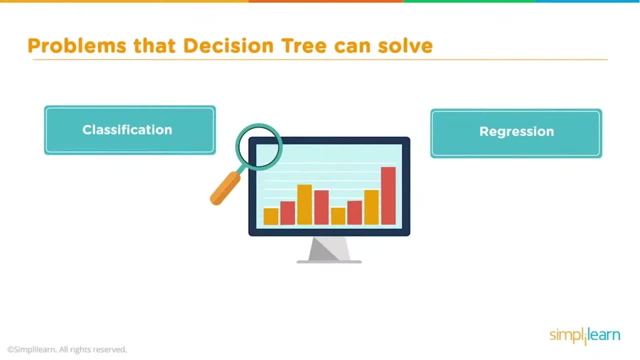 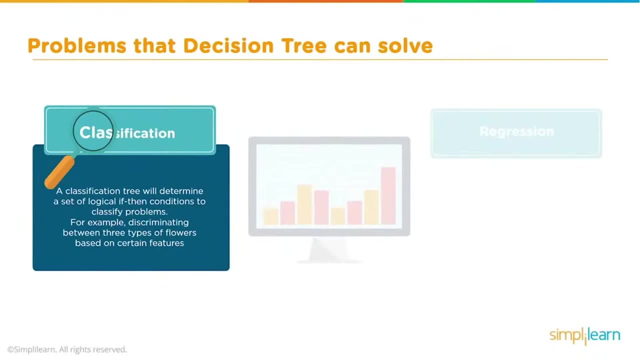 figure out what the next value is in a series of numbers or a group of data In classification. the classification tree will determine a set of logical, if then conditions to classify problems, For example, discriminating between three types of flowers based on certain features. 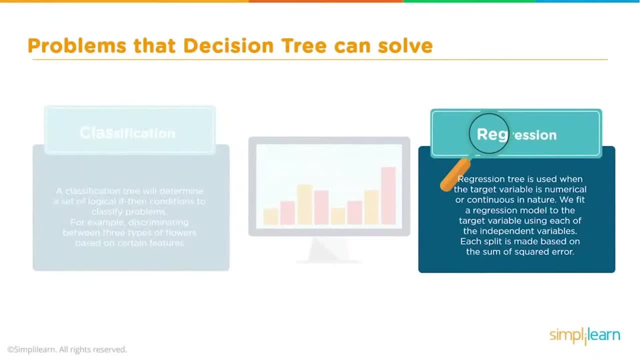 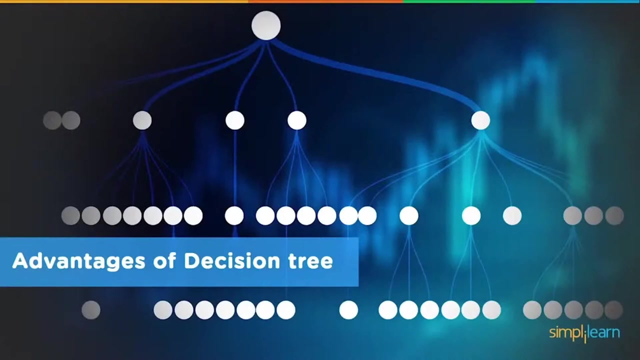 In regression. a regression tree is used when the target variable is numerical or continuous in nature. We fit the regression model to the target variable using each of the independent variables. Each split is made based on the sum of squared error. Before we dig deeper into the mechanics of the decision tree, 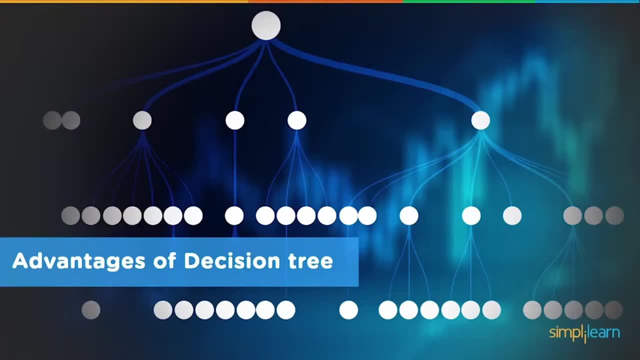 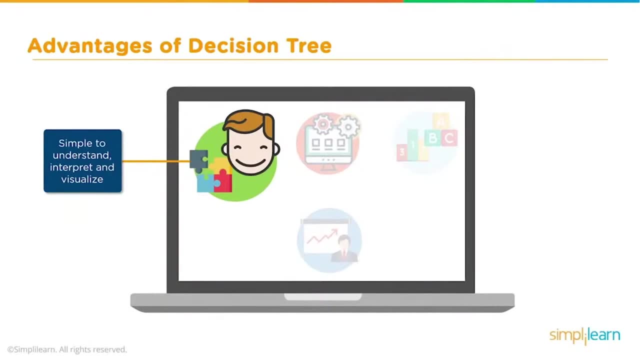 let's take a look at the advantages of using a decision tree And we'll also take a glimpse at the disadvantages. The first thing you'll notice is that it's simple to understand, interpret and visualize. It really shines here because you can see exactly what's going on in a decision tree. 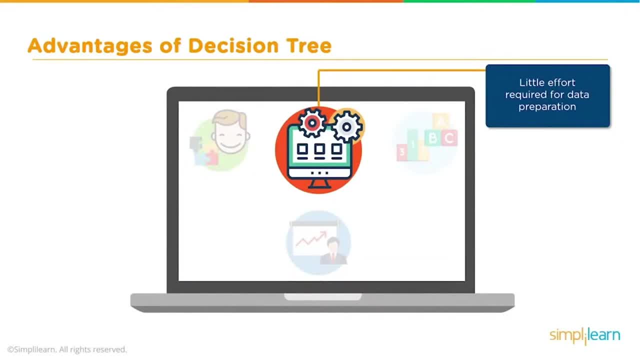 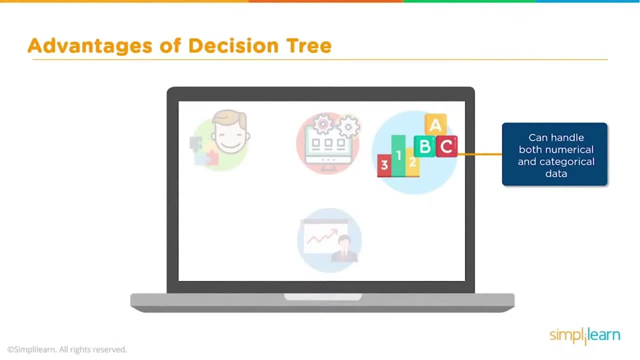 Little effort is required for data preparation, So you don't have to do special scaling. There's a lot of things you don't have to worry about when using a decision tree. It can handle both numerical and categorical data, as we discovered earlier. 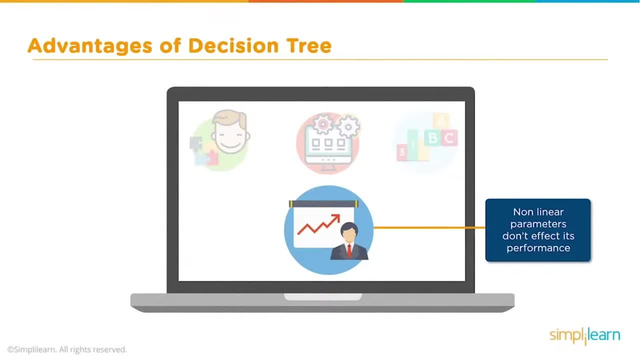 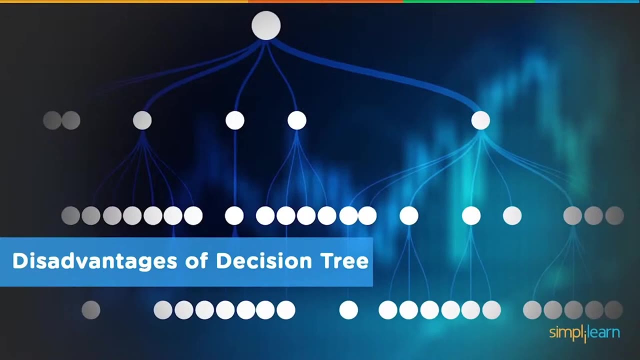 And nonlinear parameters don't affect its performance. So even if the data doesn't fit an easy curved graph, you can still use it to create an effective decision or prediction. If we're going to look at the advantages of a decision tree, we also need to understand the disadvantages of a decision tree. 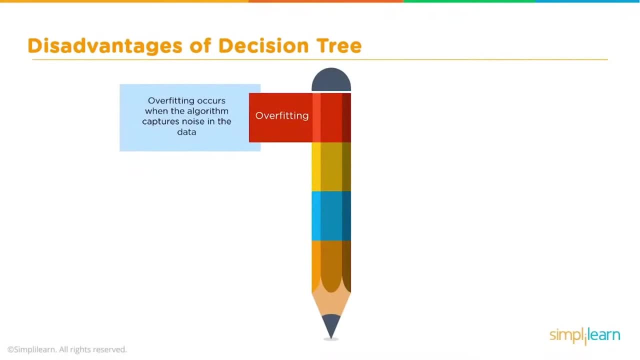 The first disadvantage is overfitting. Overfitting occurs when the algorithm captures noise in the data. That means you're solving for one specific instance instead of a general solution for all the data. High variance: The model can get unstable due to small variation in data. 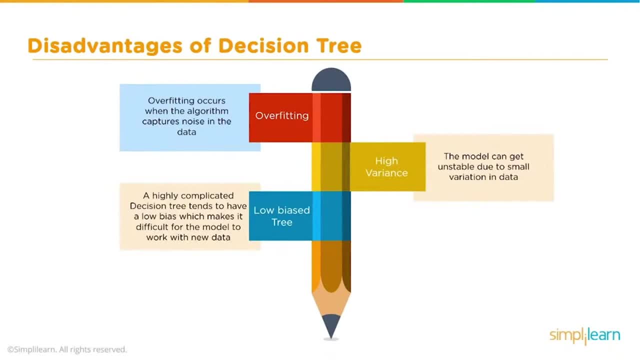 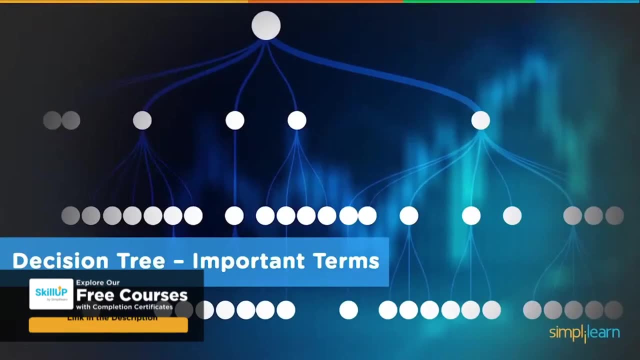 Low bias tree. A highly complicated decision tree tends to have a low bias, which makes it difficult for the model to work with new data Decision tree. important terms. Before we dive in further, we need to look at some basic terms. We need to have some definitions. 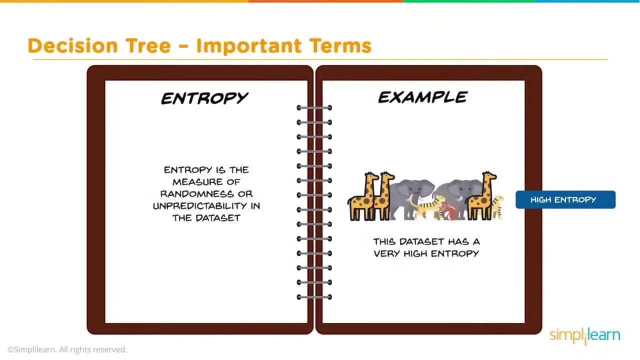 To go with our decision tree and the different parts we're going to be using. We'll start with entropy. Entropy is a measure of randomness or unpredictability in the data set. For example, we have a group of animals in this picture. 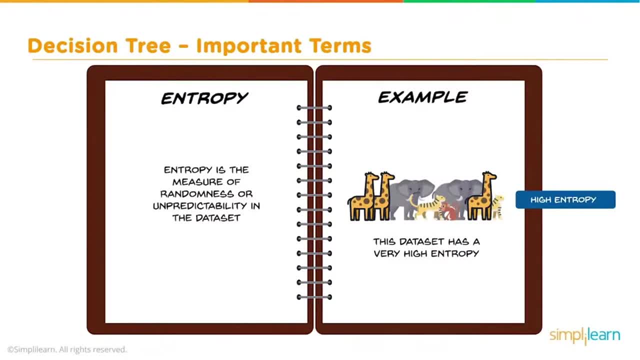 There's four different kinds of animals And this data set is considered to have a high entropy. You really can't pick out what kind of animal it is based on looking at just the four animals as a big clump of entities. So as we start splitting it into subgroups, we come up with our second. 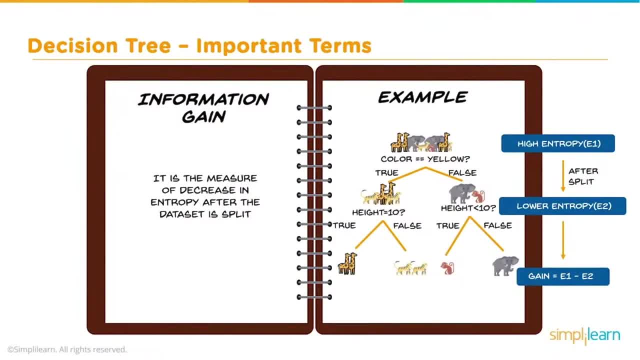 definition, which is information gain. information gain: It is a measure of decrease in entropy after the data set is split. So in this case, based on the color yellow, we've split one group of animals on one side as true and those who aren't yellow as false. 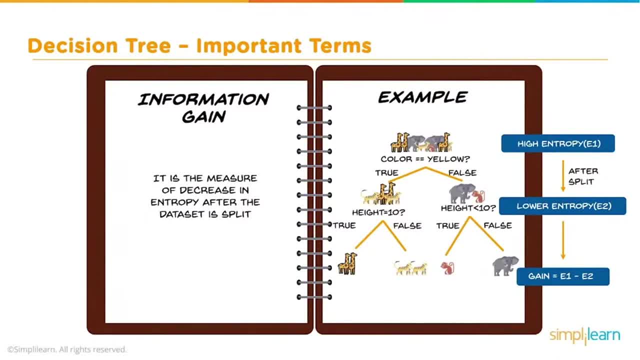 As we continue down the yellow side, we split based on the height- true or false equals 10.. And on the other side, height is less than 10,- true or false. And as you see, as we split it, the entropy continues to be less and less and less. 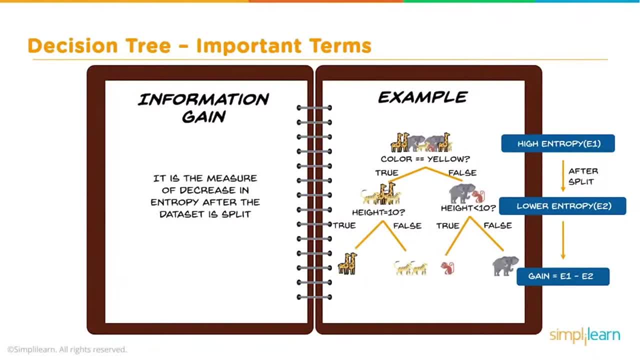 And so our information gain is simply the entropy E1 from the top and how it's changed to E2 in the bottom, And we'll look at the deeper math, although you really don't need to know a huge amount of math when you actually do the programming in Python, because they'll 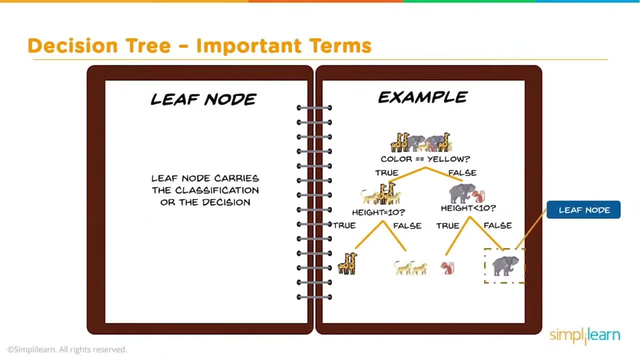 do it for you, but we'll look on the actual math at how they compute entropy. Finally, we went to the different parts of our tree and they call the leaf node. Leaf node carries the classification or the decision. So it's the final end at the bottom. 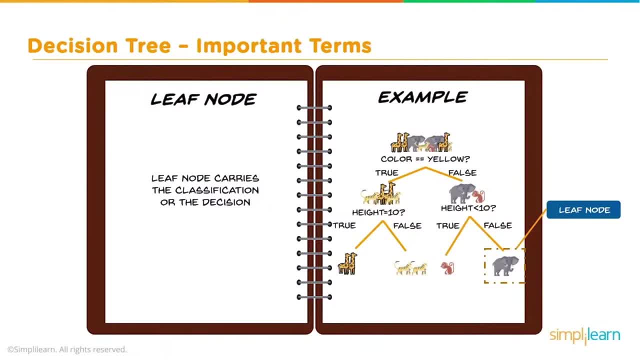 The decision node has two or more branches. This is where we're breaking the group up into different parts And finally you have the root node. The topmost decision node is known as the root node. How does a decision tree work? Wonder what kind of animals I'll get the jungle today. 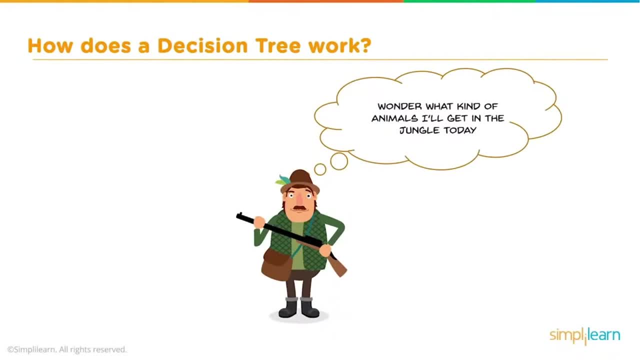 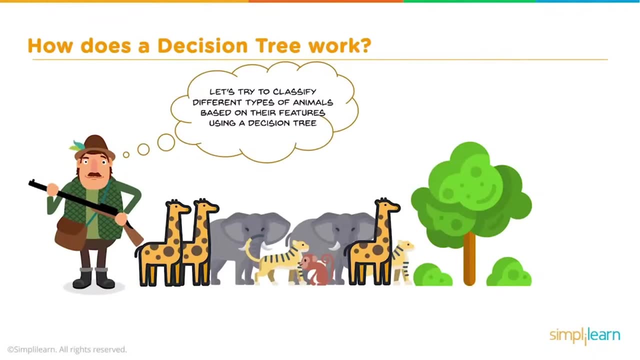 Maybe you're the hunter with the gun, or if you're more into photography, you're a photographer with a camera. So let's look at this group of animals and let's try to classify different types of animals based on their features, using a decision tree. 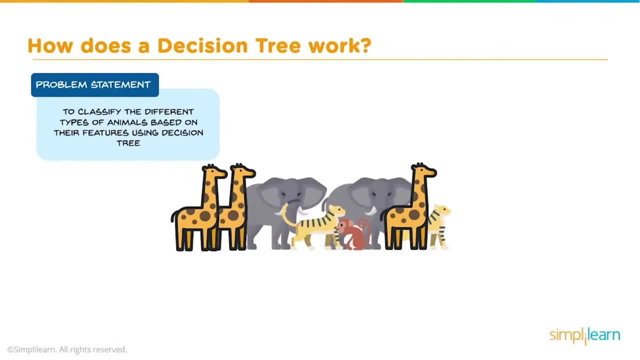 So the problem statement is to classify the different types of animals based on their features using a decision tree. The data set is looking quite messy and the entropy is high in this case, So let's look at a training set or a training data set. 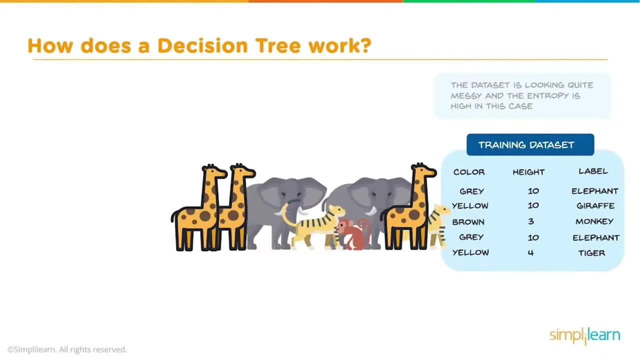 And we're looking at color, We're looking at height, And then we have our different animals. We have our elephants, our giraffes, our monkeys and our tigers, And they're of different colors and shapes. Let's see what that looks like. 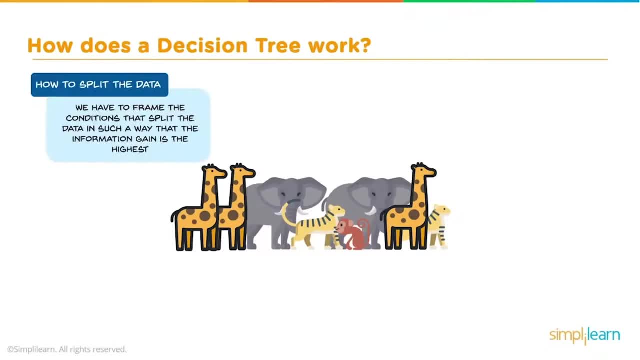 And how do we split the data? We have to frame the conditions that split the data in such a way that the information gain is the highest. Note gain is a measure of decrease in entropy after splitting, So the formula for entropy is the sum. 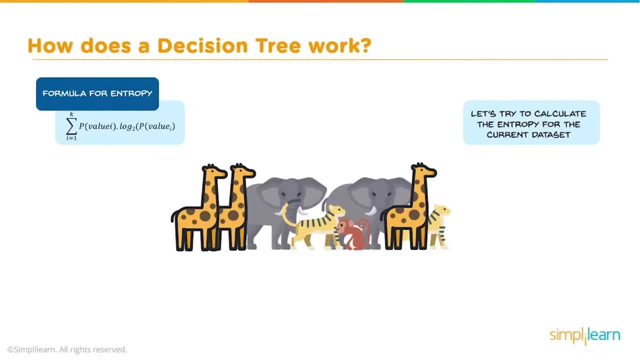 That's what this symbol looks like. It looks like kind of like a e funky e of k. where i equals 1 to k, K would represent the number of animals, the different animals in there, where value or p value of i would be the percentage of that animal times the log base 2. 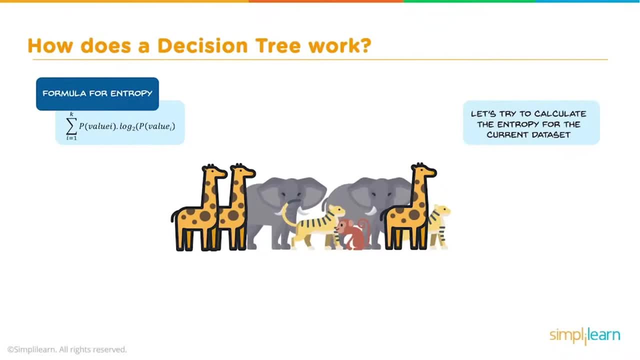 of the same, the percentage of that animal. Let's try to calculate the entropy for the current data set and take a look at what that looks like. And don't be afraid of the math. You don't really have to memorize this math. 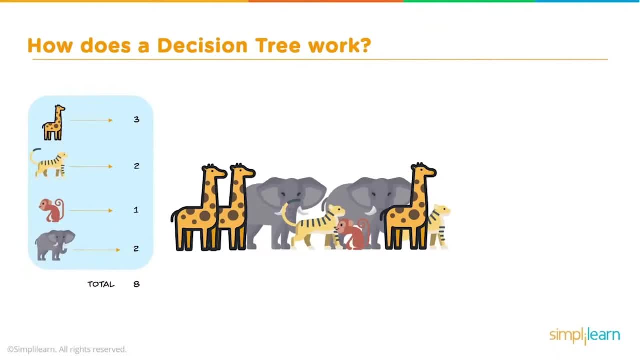 Just be aware that it's there, And this is what's going on in the background. And so we have three giraffes, two tigers, one monkey, two elephants, a total of eight animals gathered. And if we plug that into the formula, 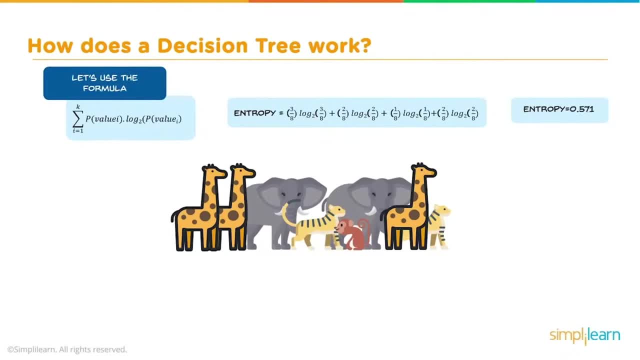 we get an entropy that equals 3 over 8.. So we have three giraffes, a total of 8 times the log. Usually they use base 2 on the log, So log base 2 of 3 over 8 plus. in this case let's say it's the elephants. 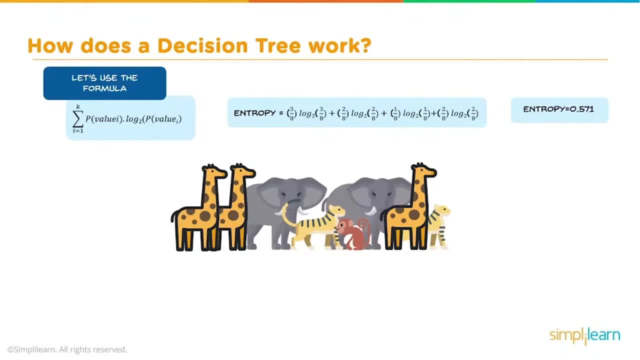 2 over 8, 2 elephants over a total of 8 times log base 2.. Log base 2,: 2 over 8 plus one monkey over total of 8.. Log base 2,: 1 over 8 and plus 2 over 8 of the tigers. 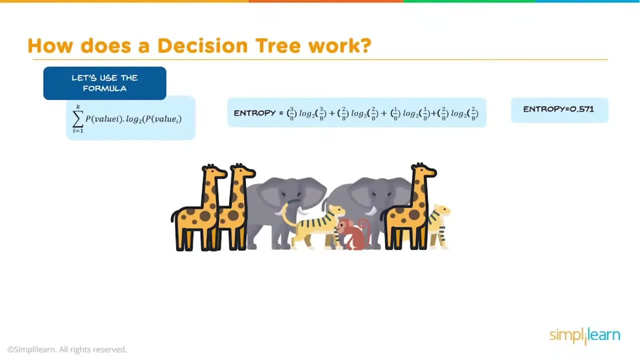 Log base 2 over 8.. And if we plug that into our computer, our calculator- I obviously can't do logs in my head- we get an entropy equal to 0.571.. The program will actually calculate the entropy of the data set. similarly, 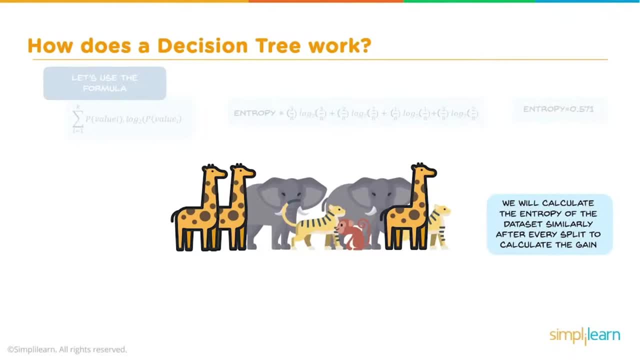 after every split to calculate the gain. Now we're not going to go through each set, one at a time, to see what those numbers are. We just want you to be aware that this is a formula or the mathematics behind it. Gain can be calculated by finding the difference. 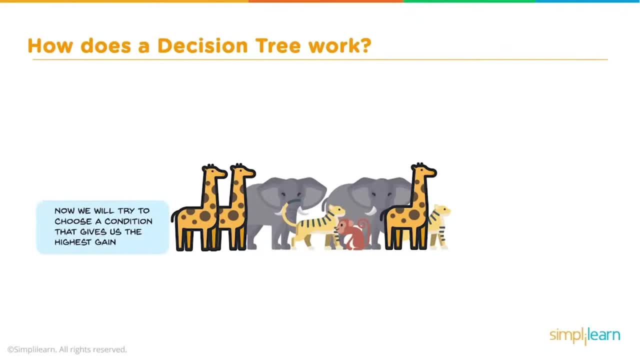 of the subsequent entropy values after a split. Now we will try to choose a condition that gives us the highest gain. We will do that by splitting the data using each condition and checking that the gain we get out of them The condition that gives us the highest. 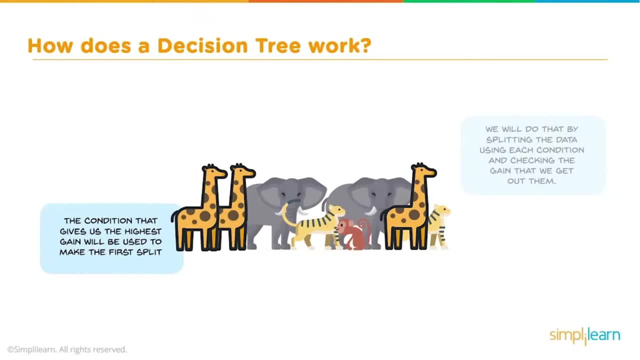 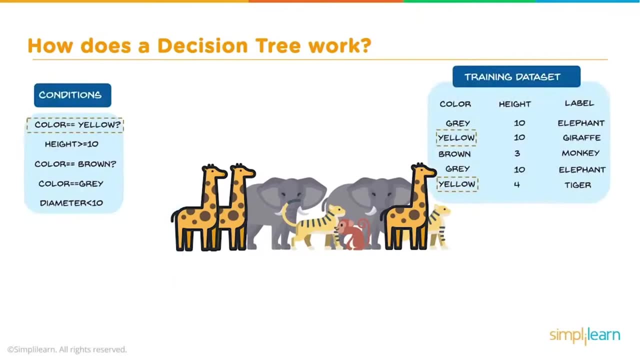 gain will be used to make the first split. Can you guess what that first split will be? just by looking at this image, As a human, it's probably pretty easy to split it. Let's see if you're right, If you guessed the color. 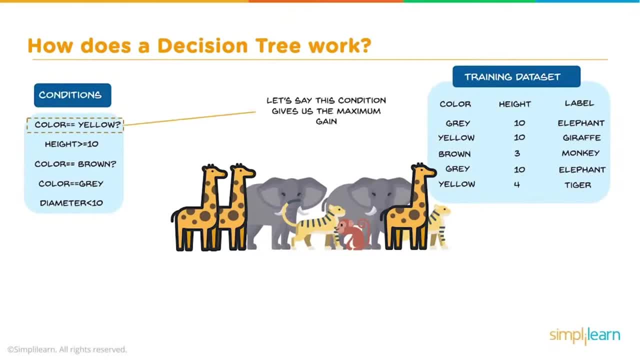 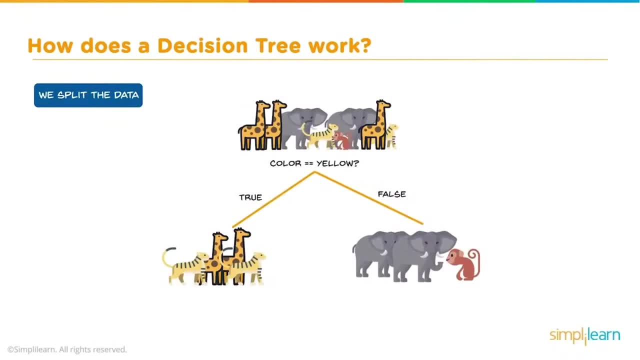 yellow. you're correct. Let's say, the condition that gives us the maximum gain is yellow. So we will split the data based on the color yellow. If it's true, that group of animals goes to the left. If it's false, it goes to the right. 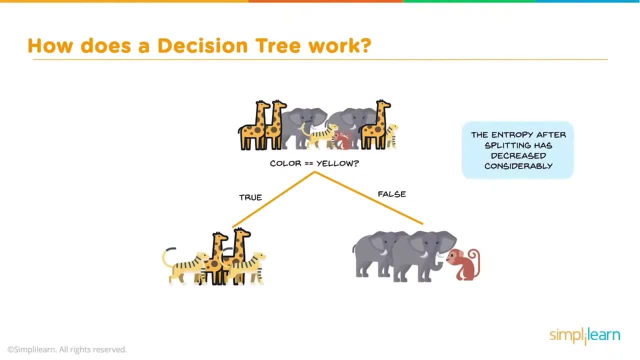 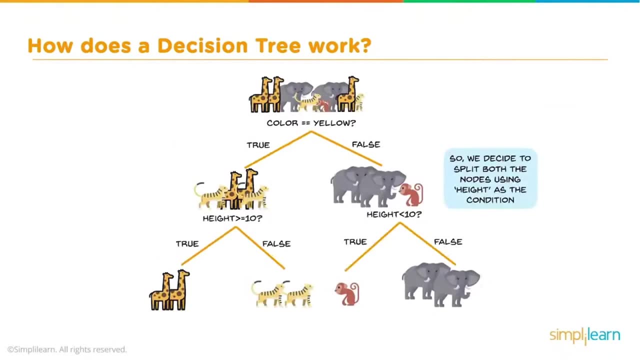 The entropy after the splitting has decreased considerably. However, we still need some splitting at both the branches to attain an entropy value equal to zero. So we decided to split both the nodes using height as a condition. Since every branch now contains single label type, we can say that entropy in this 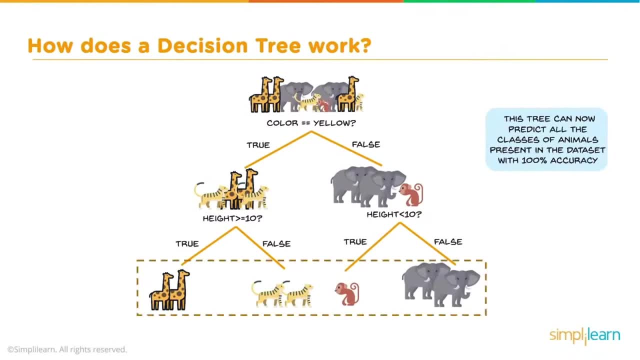 case has reached the least value. And here you see, we have the giraffes, the tigers, the monkey and the elephants, all separated into their own groups. This tree can now predict all the classes of animals present in the dataset with 100 percent accuracy. 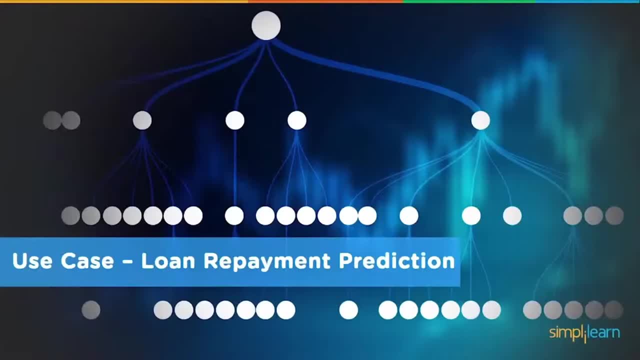 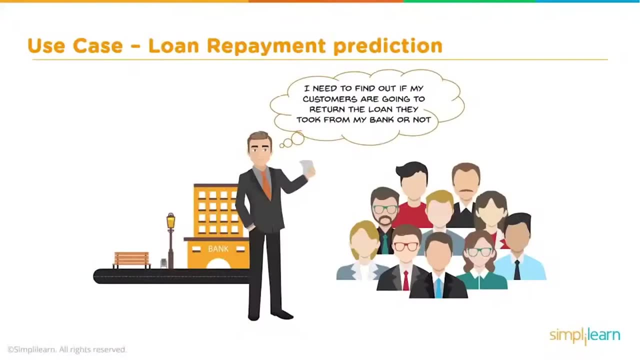 That was easy. Use case: loan repayment prediction. Let's get into my favorite part and open up some Python and see what the programming code and the scripting looks like. In here we're going to want to do a prediction and we start with this. 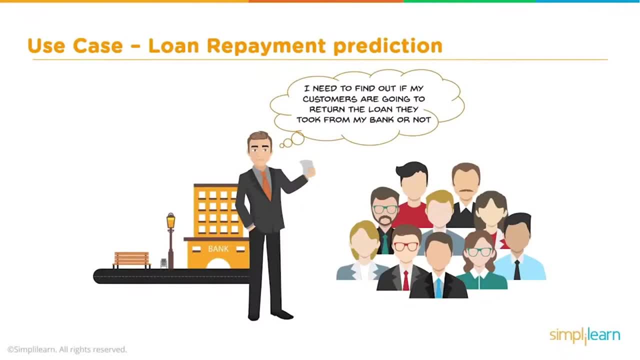 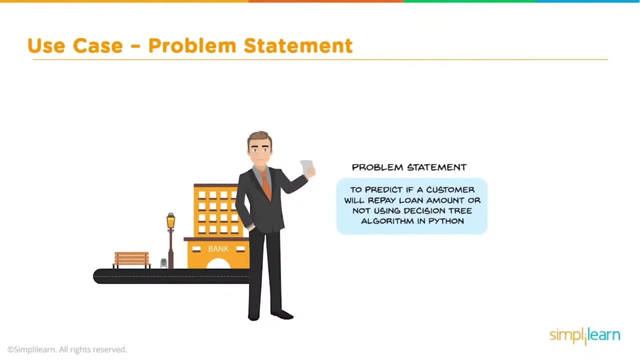 individual here who's requesting to find out how good his customers are going to be, whether they're going to repay their loan or not for his bank. And from that we want to generate a problem statement to predict if a customer will repay loan amount or not. and then we're going to be using the 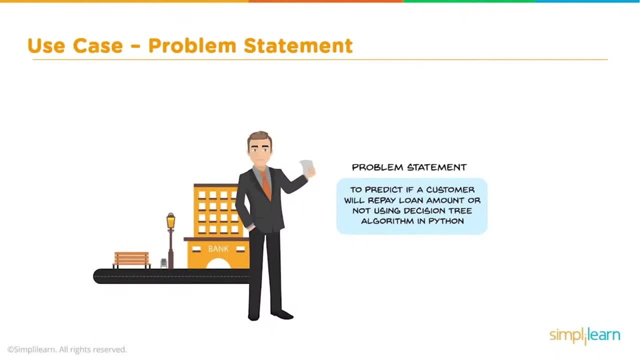 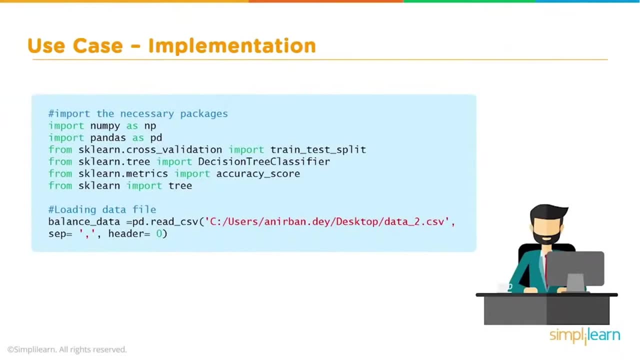 decision tree algorithm in Python. Let's see what that looks like and let's dive into the code. In our first few steps of implementation, we're going to start by importing the necessary packages that we need from Python and we're going to load up our data and take a look at what the data looks like. 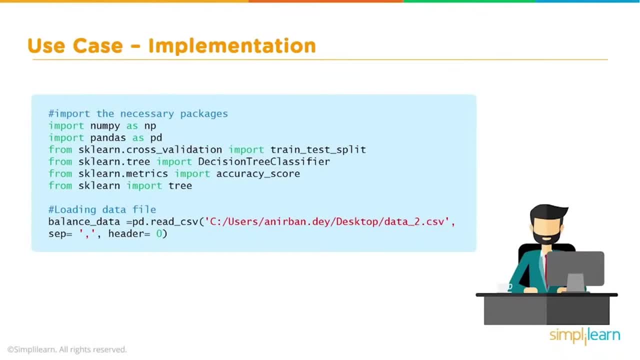 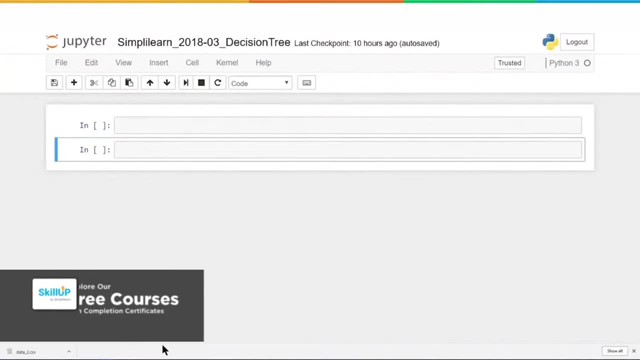 So the first thing I need is I need something to edit my Python and run it in. So let's flip on over, And here I'm using the Anaconda Jupyter Notebook. Now you can use any Python IDE you like to run it in. 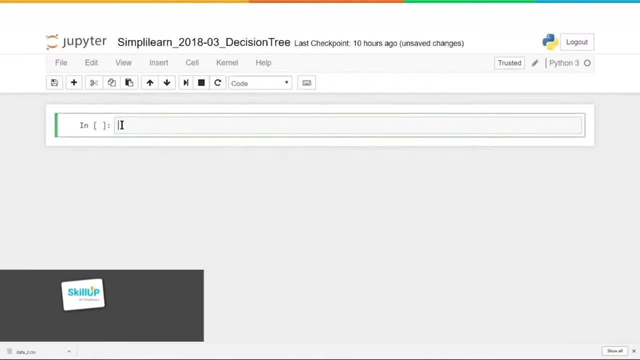 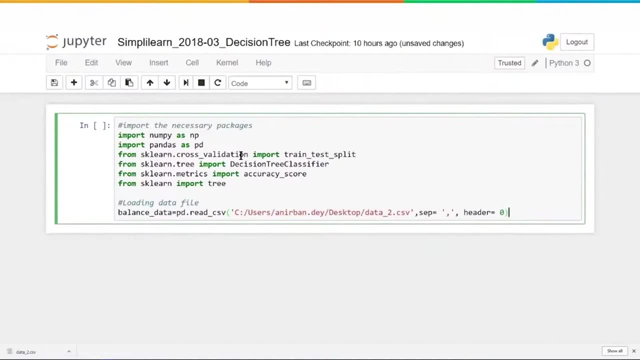 But I find the Jupyter Notebook's really nice for doing things on the fly, And let's go ahead and just paste that code in the beginning And before we start let's talk a little bit about what we're bringing in, And then we're going to do a couple of things in here. 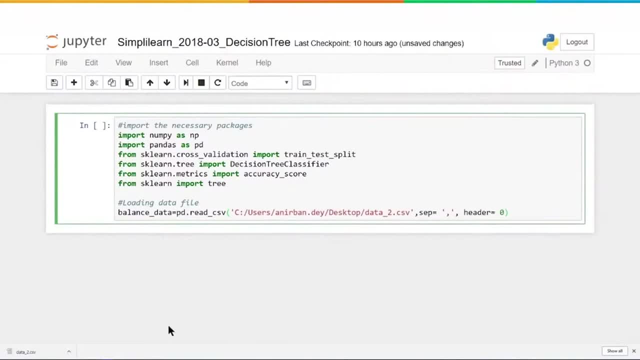 We have to make a couple of changes as we go through this first part of the import. The first thing we bring in is numpy as np. That's very standard when we're dealing with mathematics, especially with very complicated machine learning tools. You almost always see the numpy come in for your numbers. 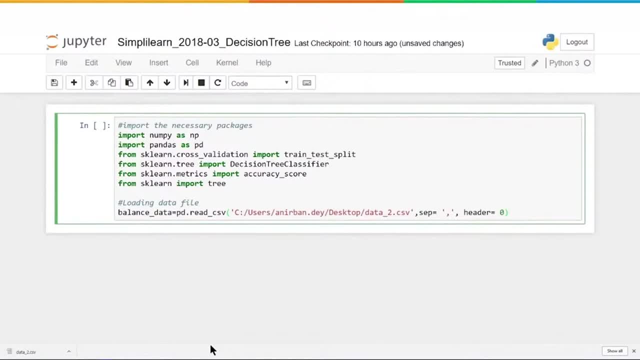 It's called number Python. It has your mathematics in there. In this case we actually could take it out, But generally you'll need it for most of your different things you work with, And then we're going to use pandas as pd. 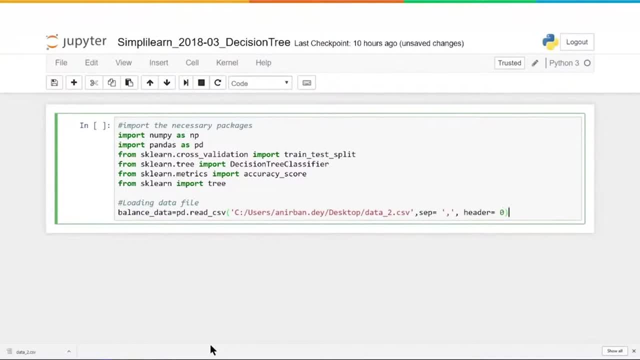 That's also a standard. The pandas is a data frame setup And you can liken this to taking your basic data and storing it in a way that looks like an Excel spreadsheet. So, as we come back to this, when you see np or pd, 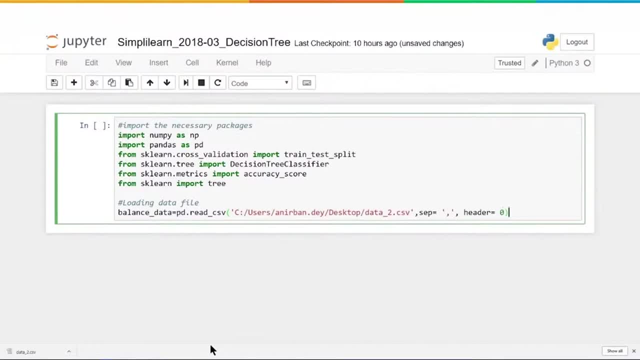 which are very standard uses. you'll know that that's the pandas And I'll show you a little bit more. when we explore the data in just a minute, Then we're going to need to split the data, So I'm going to bring in our train, test and split. 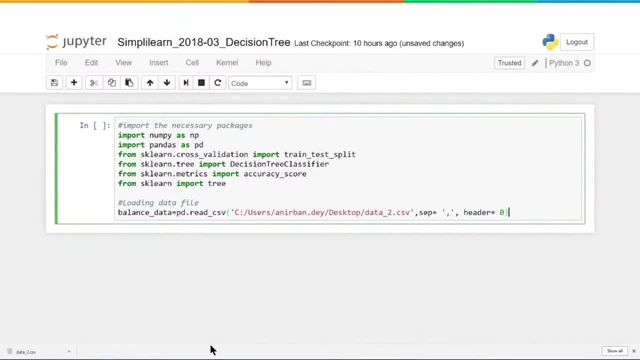 And this is coming from the sklearn package: cross-validation. In just a minute we're going to change that and we'll go over that too. And then there's also the sktree import decision tree classifier. That's the actual tool we're using. 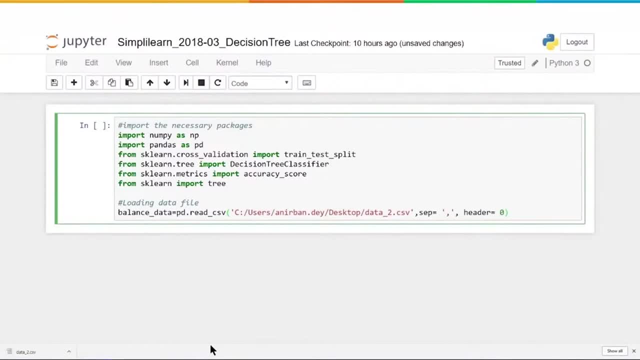 Remember I told you don't be afraid of the mathematics, It's going to be done for you. Well, the decision tree classifier has all that mathematics in there for you, so you don't have to figure it back out again. And then we have sklearnmetrics for accuracy score. 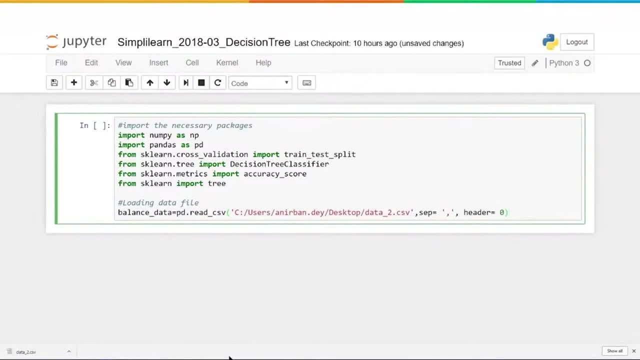 We need to score our setup. That's the whole reason. we're splitting it between the training and testing data And finally, we still need the sklearn import tree, And that's just the basic tree function is needed for the decision tree classifier. And finally, we're going to load our data down here and I'm going to run this. 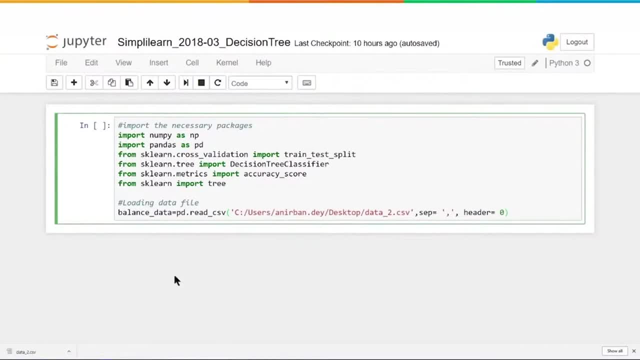 And we're going to get two things on here. One, we're going to get an error and two, we're going to get a warning. Let's see what that looks like. So the first thing we had is we have an error. 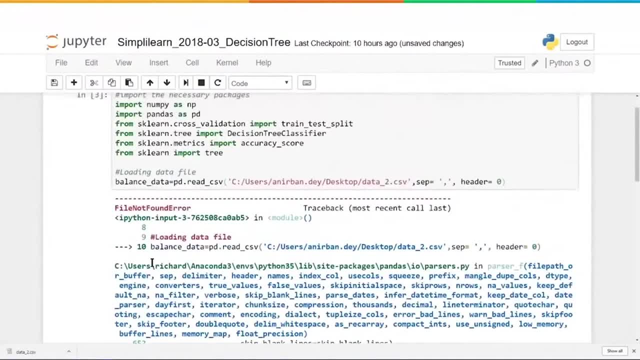 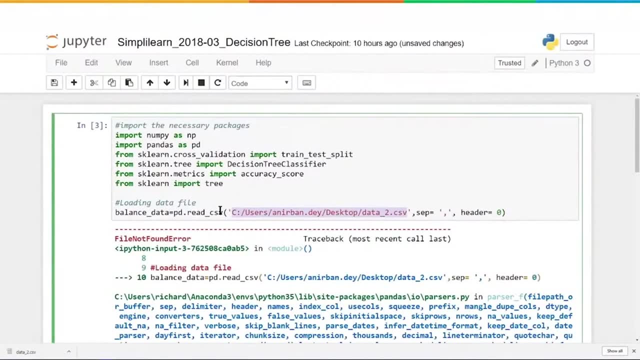 Why is this error here? Well, it's looking at this and says: I need to read a file, And when this was written, the person who wrote it. this is their path, where they stored the file, So let's go ahead and fix that. 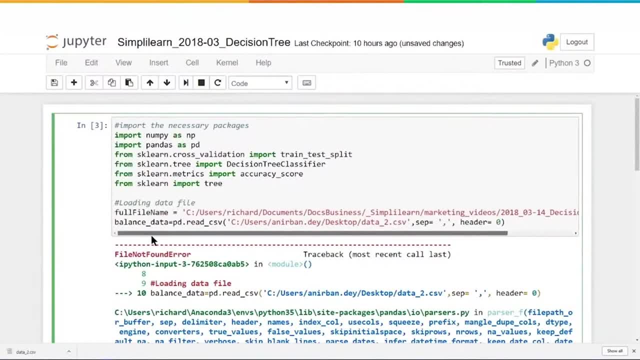 And I'm going to put in here my file path. I'm just going to call it full file name and you'll see it's on my C drive And this is very lengthy setup on here where I stored the data2.csv file. 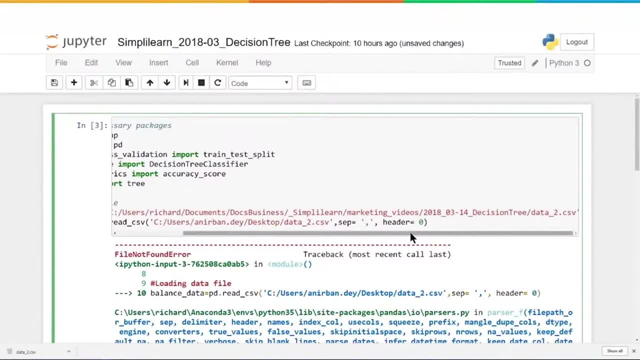 Don't worry too much about the full path, because on your computer it'll be different. The data.2.csv file was generated by SimplyLearn. If you want a copy of that, you can comment down below and request it here in the YouTube. 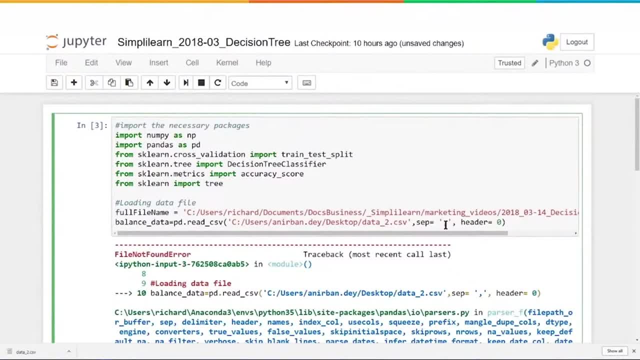 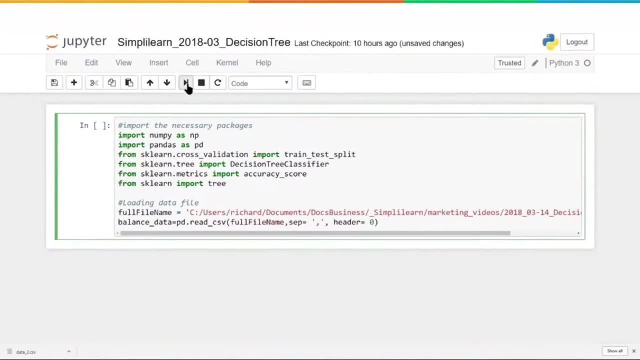 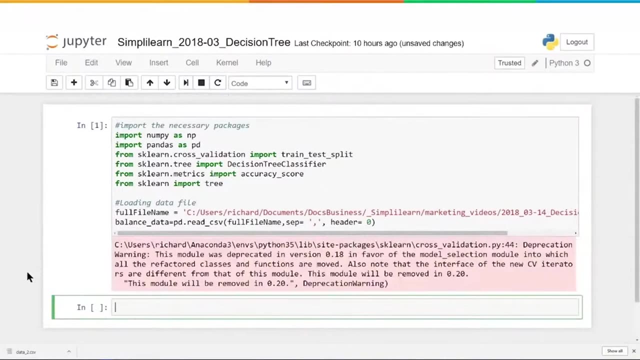 And then, if I'm going to give it a name- full file name- I want to go ahead and change it here to full file name. So let's go ahead and run it now and see what happens, And we get a warning When you're coding. understanding these different warnings and these, 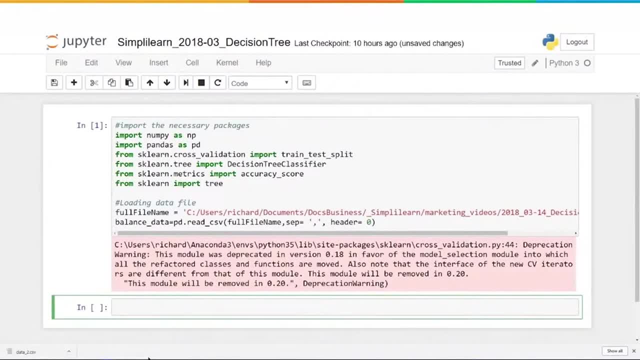 different errors that come up is probably the hardest lesson to learn. So let's just go ahead and take a look at this and use this as a opportunity to understand what's going on here. If you read the warning, it says the cross validation is depreciated. 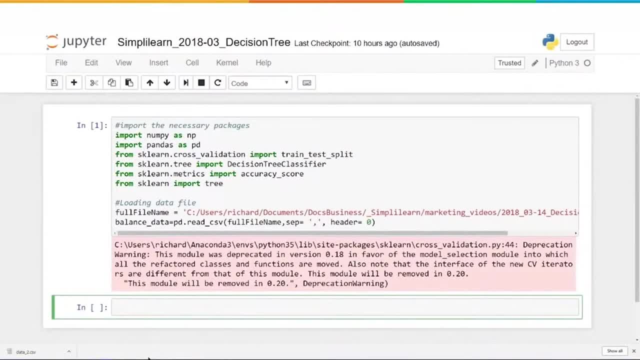 So it's a warning on it's being removed and it's going to be moved in favor of the model selection. So if we go up here, we have SKLearn Cross validation And if you research this and go to the SKLearn site, 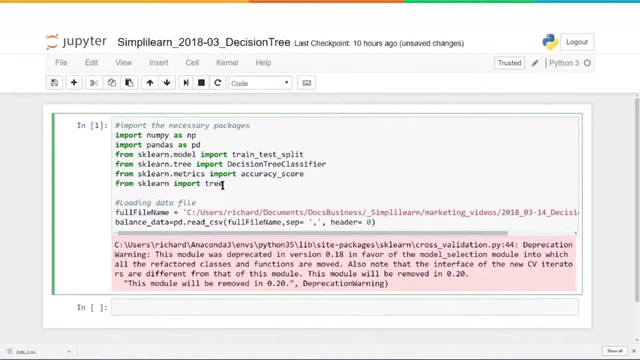 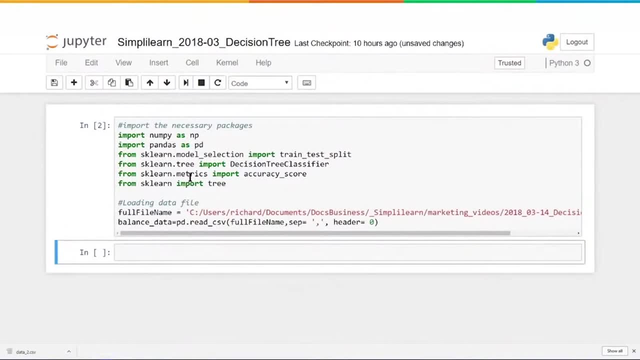 you'll find out that you can actually just swap it right in there with model selection, And so when I come in here and I run it again, That removes a warning. What they've done is they've had two different developers develop it in two different branches. 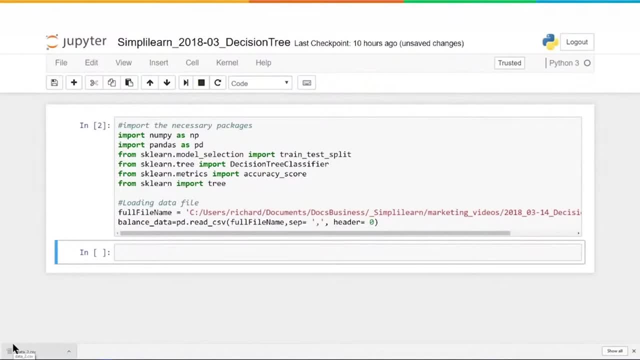 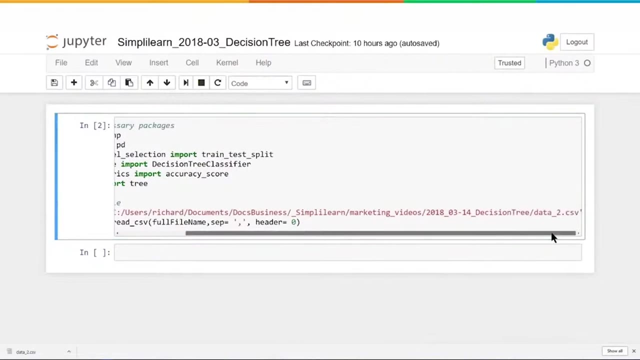 And then they decided to keep one of those and eventually get rid of the other one. That's all that is, And very easy and quick to fix. Before we go any further, I went ahead and opened up the data from this file. Remember the data file we just loaded on here? the data underscore two dot CSV. 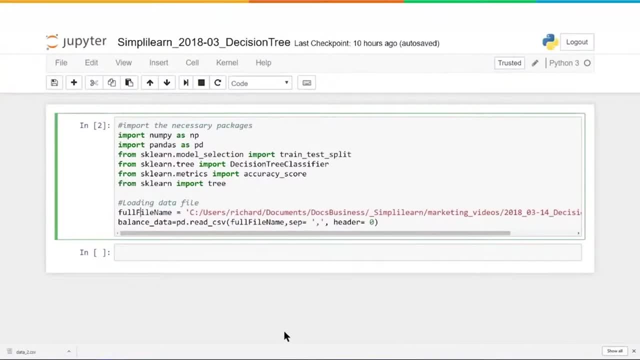 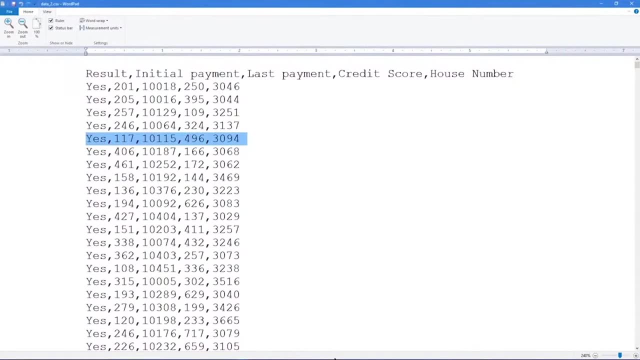 Let's talk a little bit more about that and see what that looks like both as a text file- because it's a comma separated variable file- and in a spreadsheet. This is what it looks like as a basic text file. You can see at the top they've created a header. 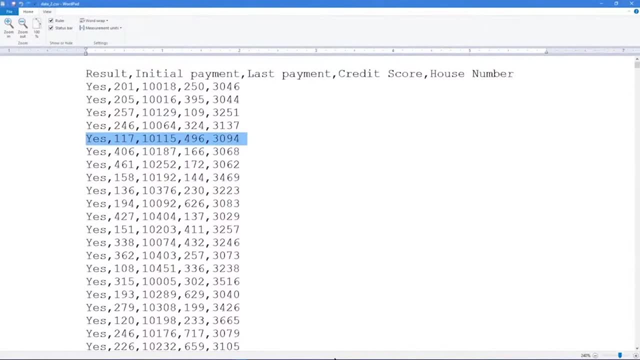 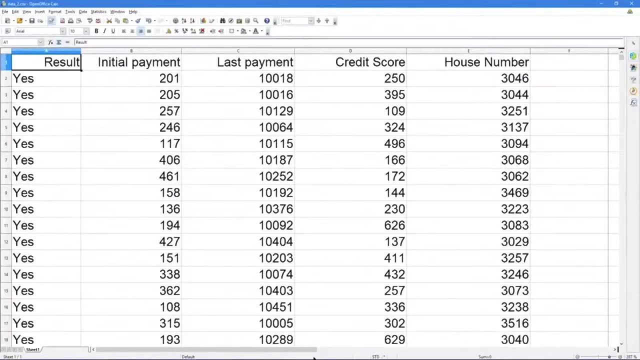 It's got one, two, three, four, five columns and each column has data in it. And let me flip this over, because we're also going to look at this in an actual spreadsheet and see what that looks like. And here I've opened it up in the open office, calc. 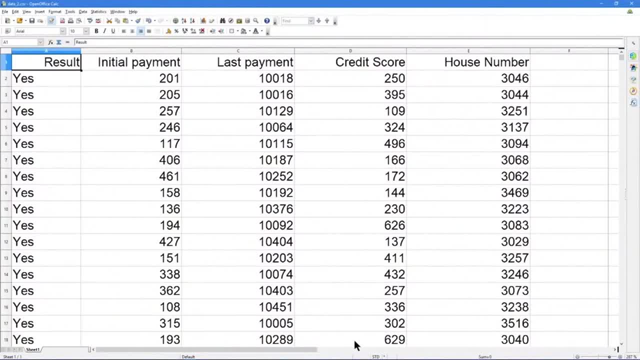 which is pretty much the same as Excel, and zoomed in And you can see we've got our columns and our rows of data a little easier to read. in here We have a result. Yes, yes, no, We have initial payment. last payment: credit score, house number. 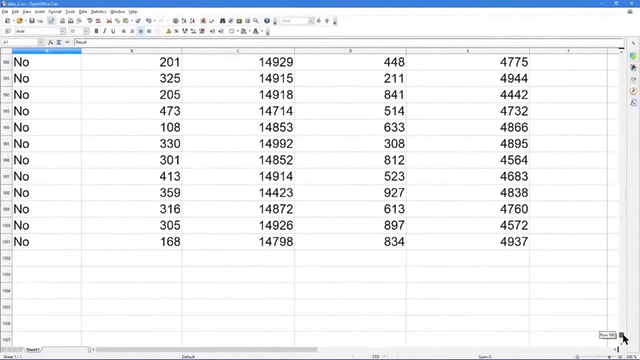 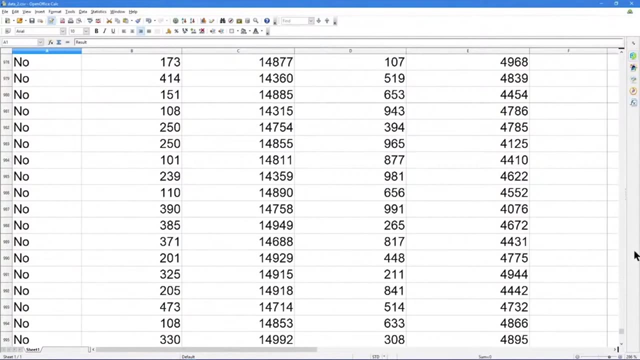 If we scroll way down, We'll see that this occupies a thousand and one lines of code or lines of data, But the first one being a column and then one thousand lines of data. Now, as a programmer, if you're looking at a small amount of data, 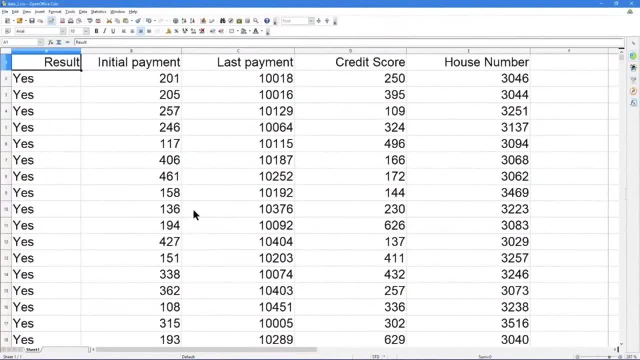 I usually start by pulling it up in different sources and see what I'm working with. But in larger data you won't have that option. It would just be too, too large. You need to either bring in a small amount that you can look at it like we're doing. 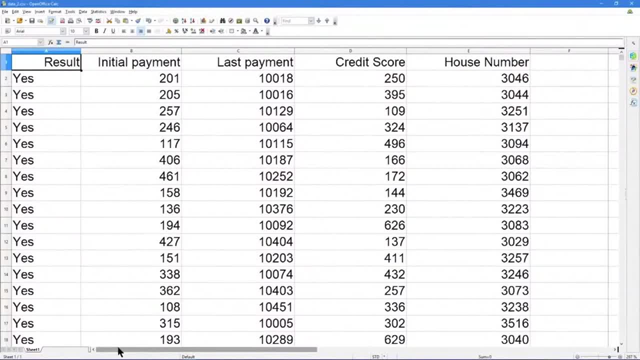 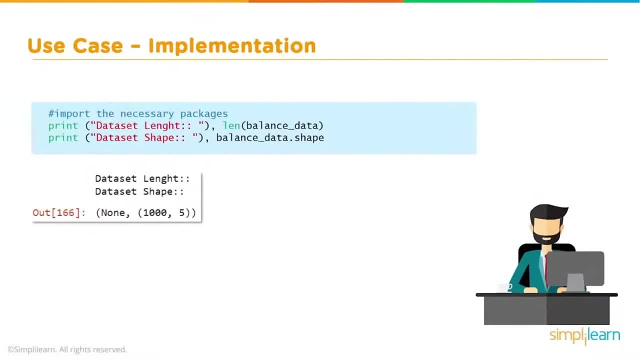 right now, or we can start looking at it through the Python code. So let's go ahead and move on and take the next couple of steps to explore the data using Python. Let's go ahead and see what it looks like in Python to print the length and the shape of the data. 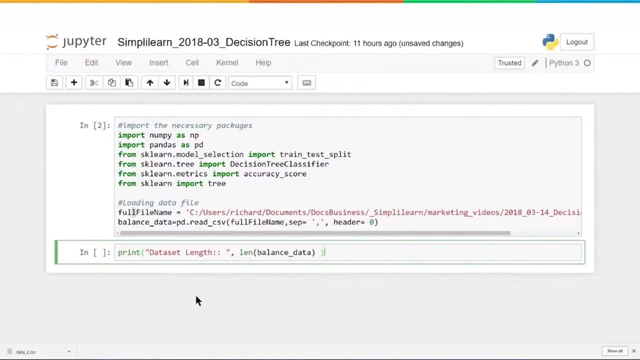 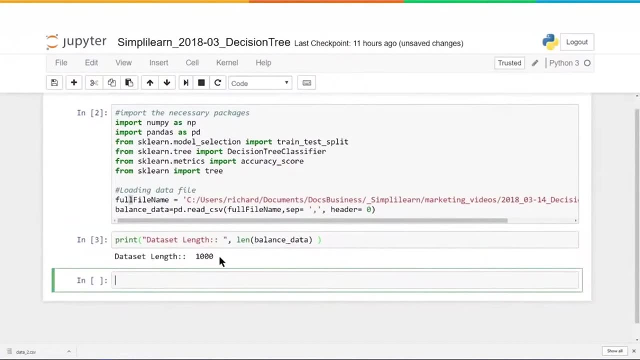 So let's start by printing the length of the database. We can use a simple lin function from Python, And when I run this, you'll see that it's a thousand long, and that's what we expected. There's a thousand lines of data in there if you subtract the column head. 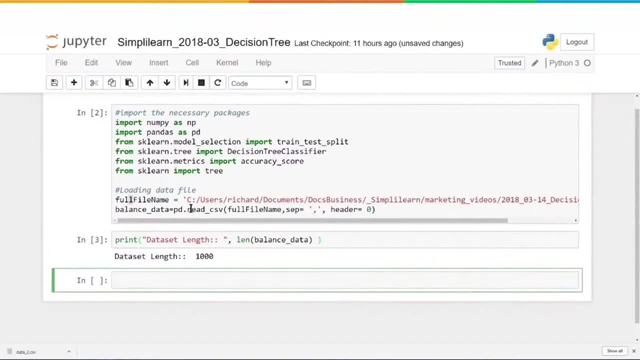 This is one of the nice things when we did the balance data from the Panda. read In CSV: you'll see that the header is row zero, So it automatically removes a row And then shows the data separate. It does a good job sorting that data out for us. 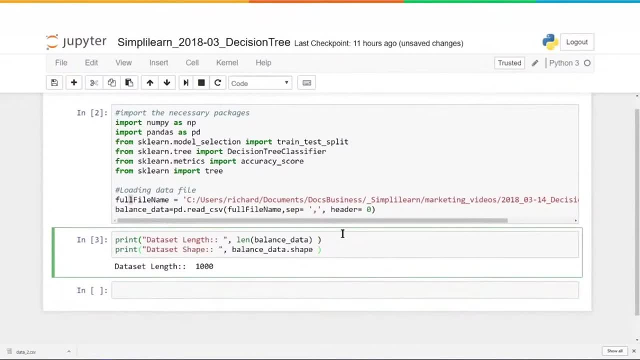 And then we can use a different function and let's take a look at that. And again, we're going to utilize the tools in Panda And since the balance underscore data was loaded as a Panda data frame, We can do a shape on it and let's go ahead and run the shape and see what that looks like. 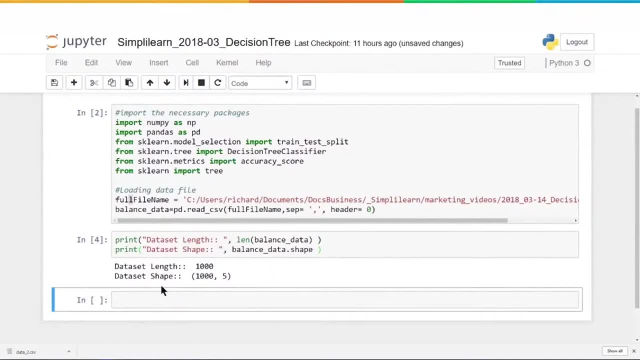 What's nice about the shape is not only does it give me the length of the data- We have a thousand lines- It also tells me there's five columns. So we were looking at the data. We had five columns of data. And then let's take one more step to explore the data using Python. 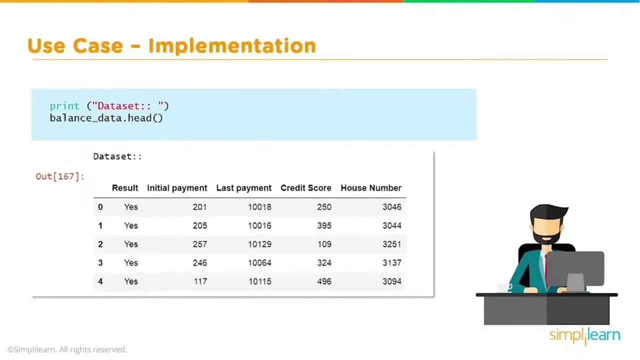 And now that we've taken a look at the length and the shape, let's go ahead and use the Pandas module for head- Another beautiful thing in the data set that we can utilize. So let's put that on our sheet here and we have print data set and. 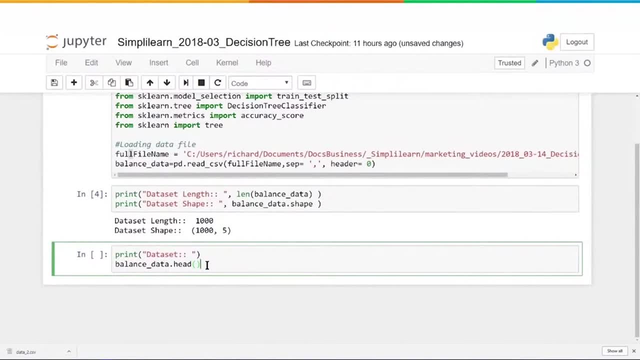 balance data dot head And this is a Pandas print statement of its own, So it has its own print feature in there. And then we went ahead and gave a label for a print job here of data set, just a simple print statement. 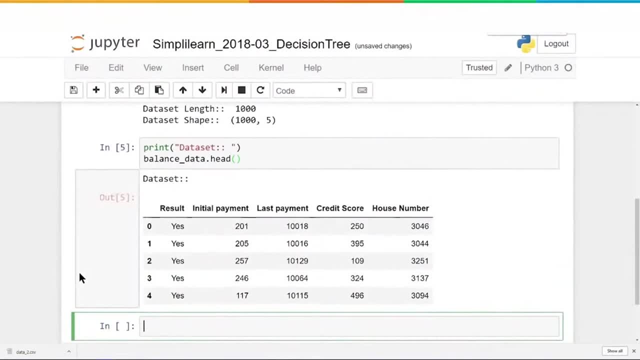 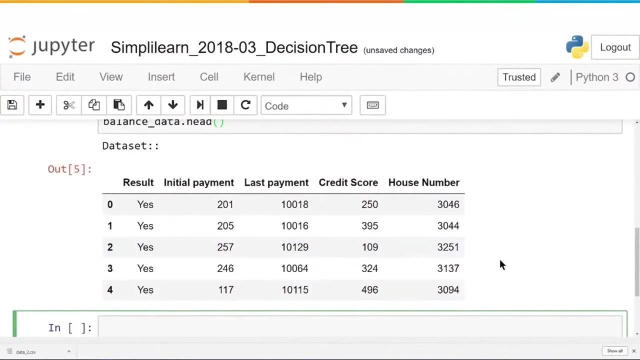 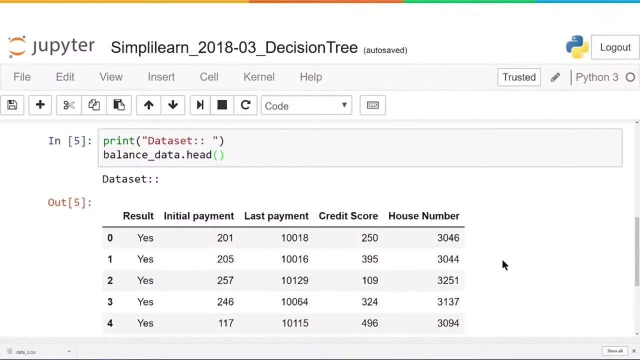 And we run that, and let's just take a closer look at that. Let me zoom in here. There we go. Pandas does such a wonderful job of making this a very clean, readable data set So you can look at the data, you can look at the column headers, you can have it. 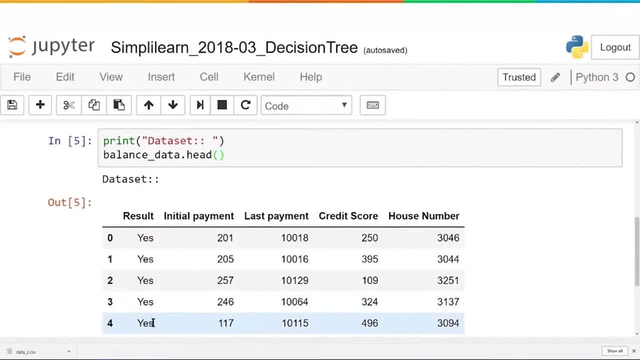 When you put it as the head, it prints the first five lines of the data And we always start with zero. So we have five lines. We have zero. one, two, three, four instead of one, two, three, four, five. 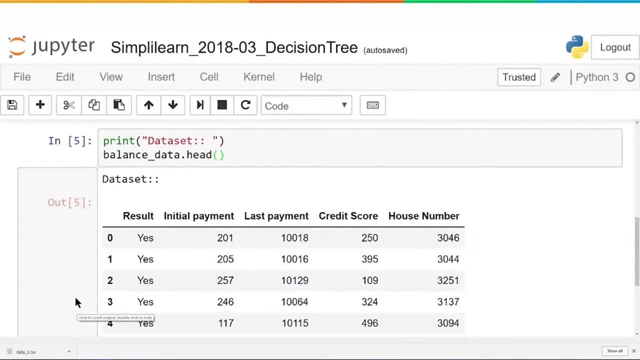 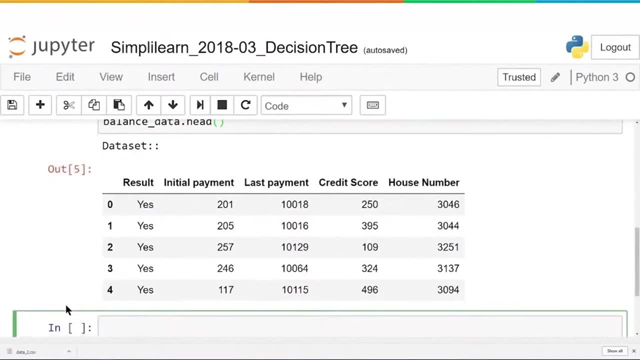 That's a standard scripting and programing set. is you want to start with the zero position? And that is what the data head does. It pulls the first five rows of data, puts it in a nice format that you can look at and view. very powerful tool to view the data. 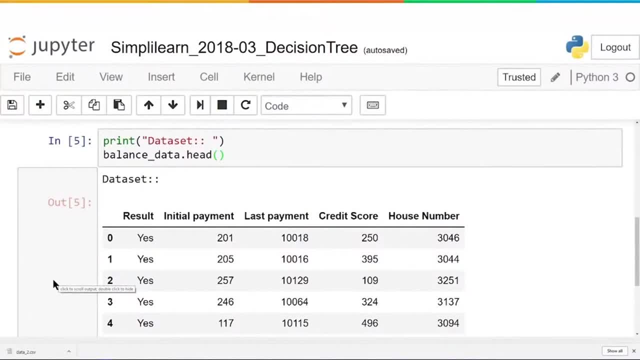 So instead of having to flip and open up an Excel spreadsheet or open Office Cal, or trying to look at a Word doc where it's all scrunched together and hard to read, you can now get a nice open view of what you're working with. 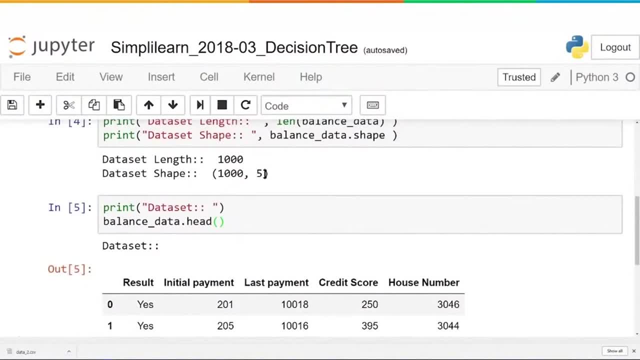 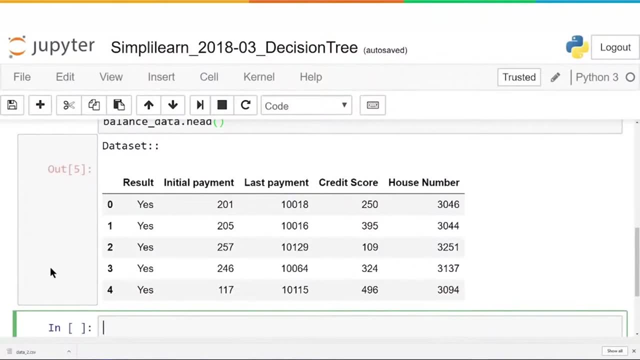 We're working with a shape of a thousand long, five wide, So we have five columns and we do the full data head. You can actually see what this data looks like: the initial payment, last payment, credit scores, house number. So let's take this, now that we've 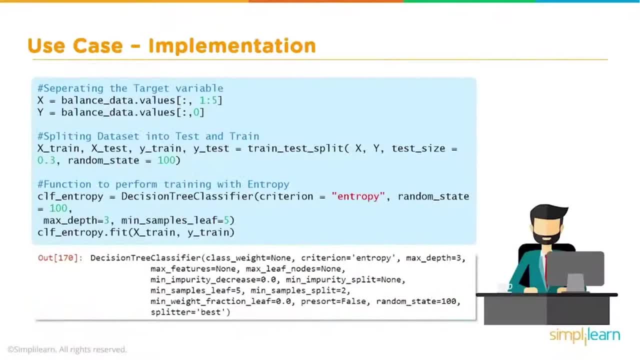 explored the data and let's start digging into the decision tree. So in our next step we're going to train and build our data tree, And to do that we need to first separate the data out. We're going to separate into two groups so that we have something to actually train. 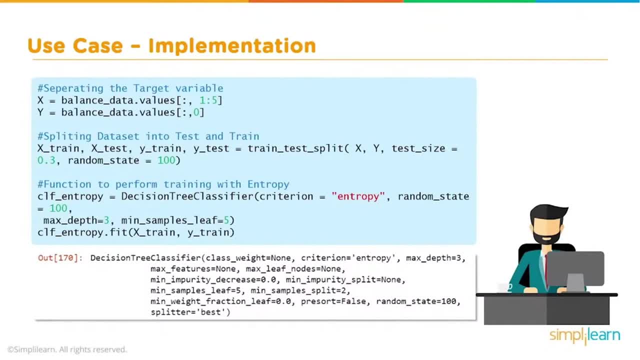 the data with, and then we have some data on the side to test it, to see how good our model is. Remember, with any of the machine learning you always want to have some kind of test set to weigh it against. So you know how good your model is when you distribute it. 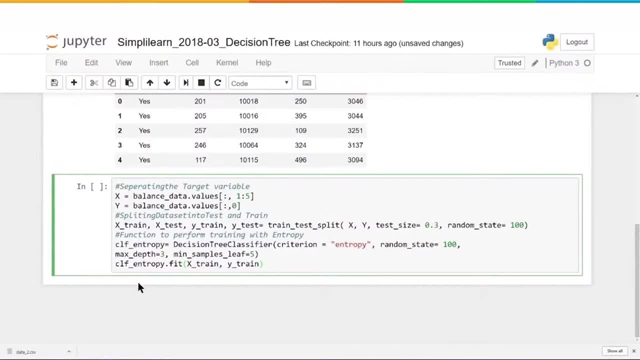 Let's go ahead and break this code down and look at it in pieces. So first we have our X and Y. Where do X and Y come from? Well, X is going to be our data and Y is going to be the answer or the target. 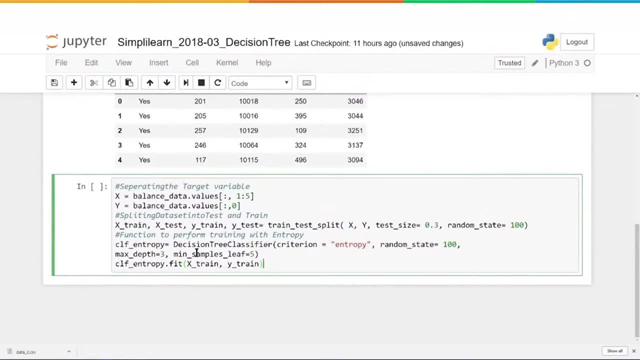 You can look at it as source and target. In this case, we're using X and Y to denote the data in and the data that we're actually trying to guess what the answer is going to be, And so to separate it we can simply put in: X equals the balance of the data dot values. 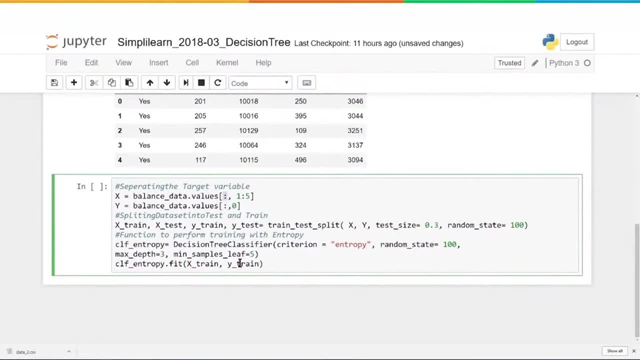 The first brackets means that we're going to select all the lines in the database, So it's all the data, And the second one says we're only going to look at columns one through five. Remember, we always start with zero. Zero is a yes or no. 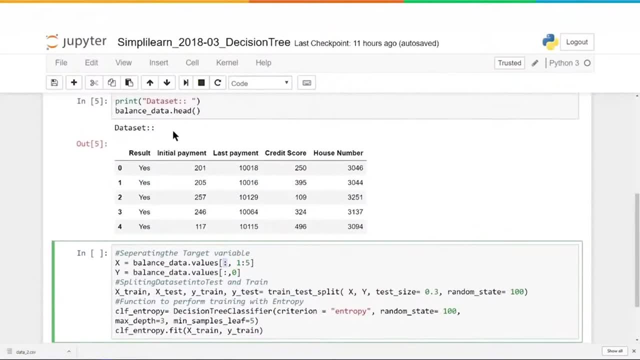 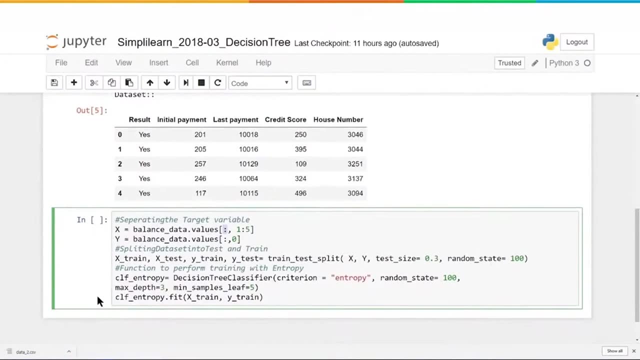 And that's whether the loan went default or not. So we want to start with one. If we go back up here, that's the initial payment And it goes all the way through the house number. Well, if we want to look at one through five, we can do the same thing for Y. 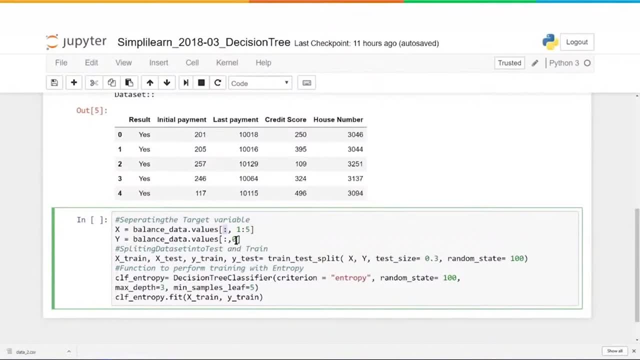 which is the answers, and we're going to set that just equal to the zero row. So it's just the zero row and then it's all rows going in there. So now we've divided this into two different data sets, One of them with the data going in and one with the answers. 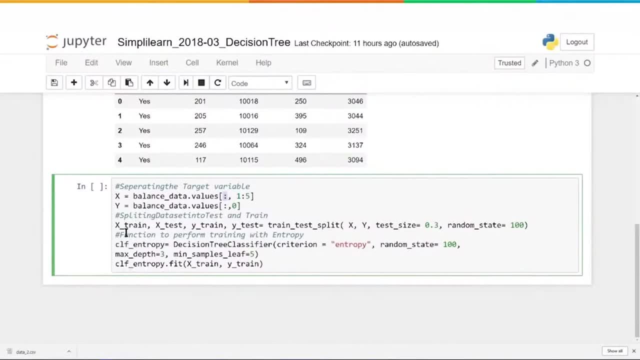 Next we need to split the data, And here you'll see that we have it split into four different parts. The first one is your X training your X test. your Y train, your Y test. Simply put, we have X going in where we're going to train it and we have 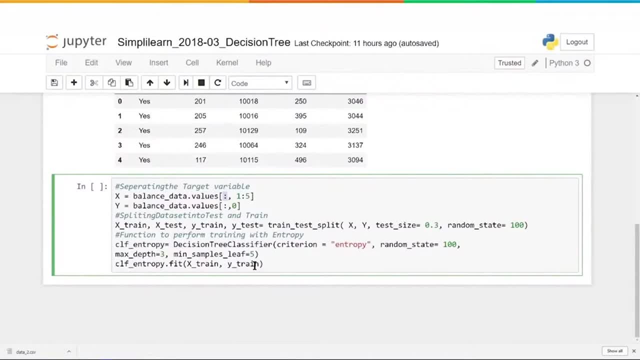 to know the answer to train it with. And then we have X test, where we're going to test that data And we have to know in the end what the Y was supposed to be. And that's where this train test split comes in that we loaded earlier in the modules. 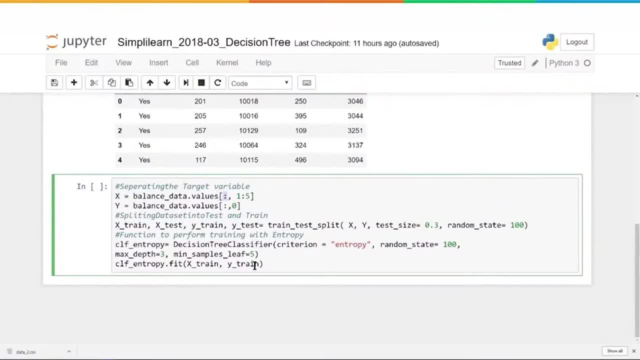 This does it all for us And you can see they set the test size equal to 0.3.. So it's roughly 30% will be used in the test, And then we use a random state. So it's completely random which rows it takes out of there. 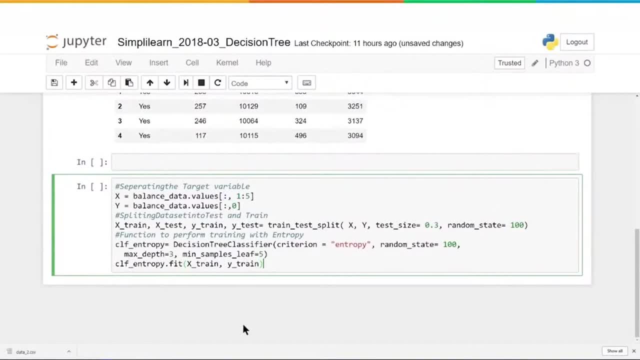 And then finally we get to actually build our decision tree And they've called it here CLF, underscore, entropy, That's the actual decision tree, or decision tree classifier, And in here they've added a couple of variables which we'll explore in just. 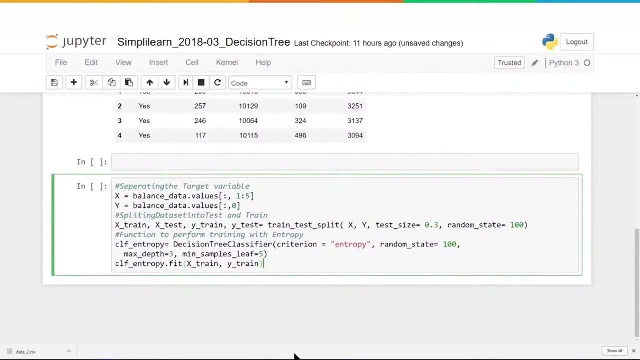 a minute And then, finally, we need to fit the data to that. So we take our CLF entropy that we created and we fit the X train And since we know the answers for X train or the Y train, we go and put those in and let's go ahead and run this. 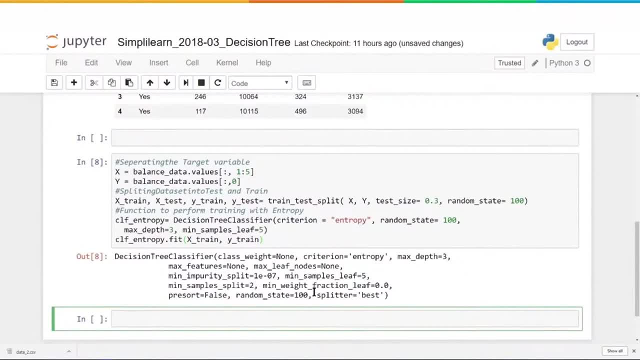 And what most of these SKLearn modules do is when you set up the variable- in this case we set the CLF entropy equal decision tree classifier- It automatically prints out what's in that decision tree. There's a lot of variables you can play with in here. 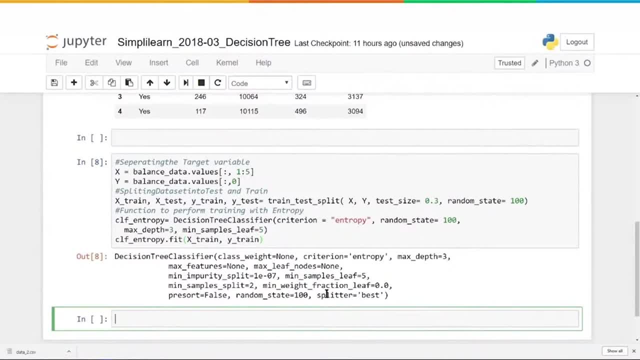 And it's quite beyond the scope of this tutorial to go through all of these and how they work. But we're working on entropy. That's one of the options We've added that it's completely a random state of 100, so 100%. 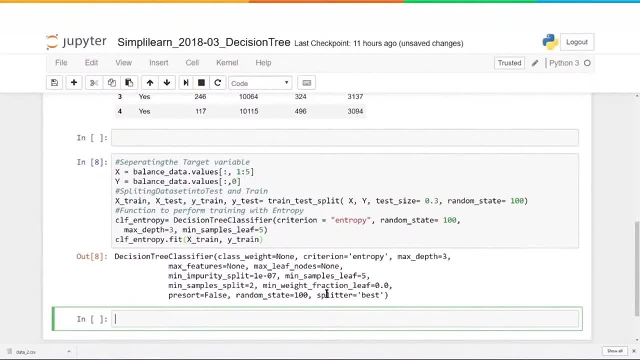 And we have a max depth of three. Now, the max depth, if you remember above when we were doing the different graphs of animals, means it's only going to go down three layers before it stops. and then we have minimal samples of leafs as 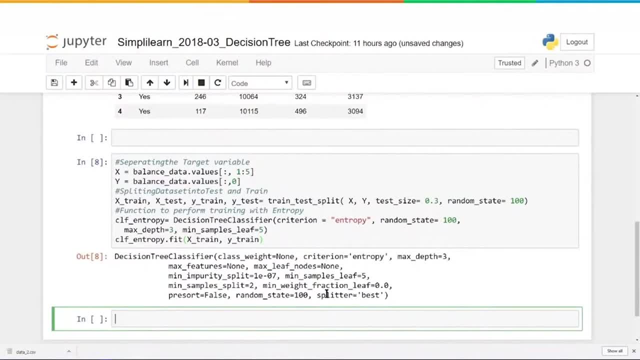 five. So it's going to have at least five leafs at the end. So we'll have at least three splits. We'll have no more than three layers and at least five in leafs, with the final result at the bottom, Now that we've created our decision tree. 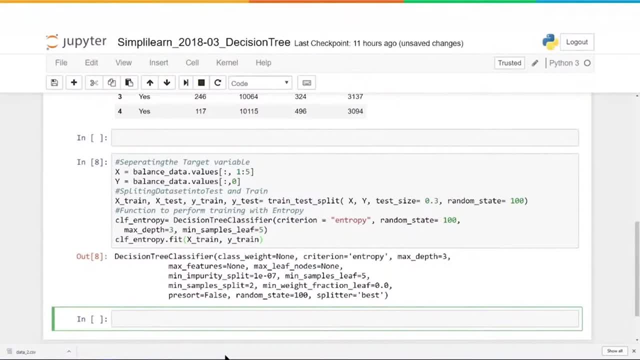 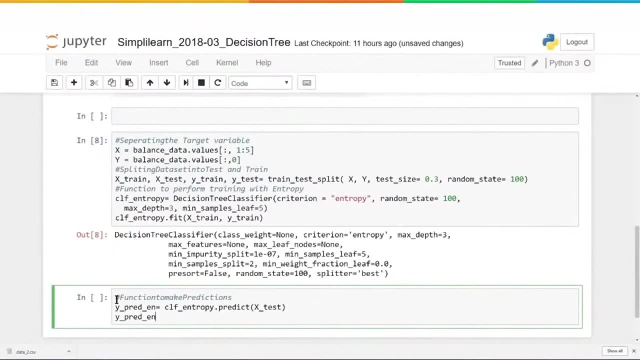 classifier not only created it, but trained it. Let's go ahead and apply it and see what that looks like. So let's go ahead and make a prediction and see what that looks like. We're going to paste our predict code in here. 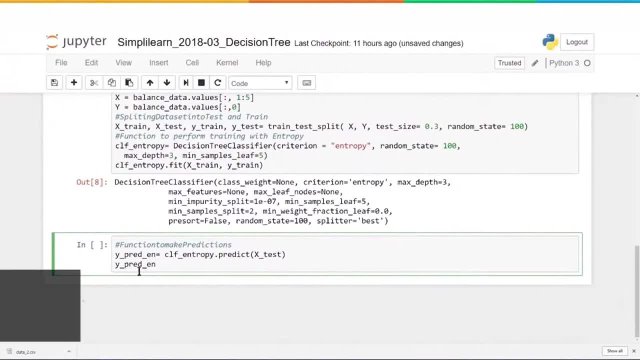 And before we run it, let's just take a quick look at what it's doing. here We have a variable Y predict that we're going to do And we're going to use our variable CLF entropy that we created, And then you'll see dot predict. 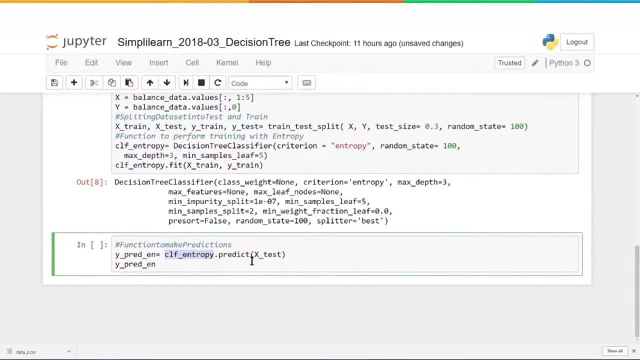 And it's very common in the SK learn modules that they're different tools- have the predict when you're actually running a prediction. In this case, we're going to put our X test data in here Now, if you delivered this for use- an actual commercial use- and distributed it. 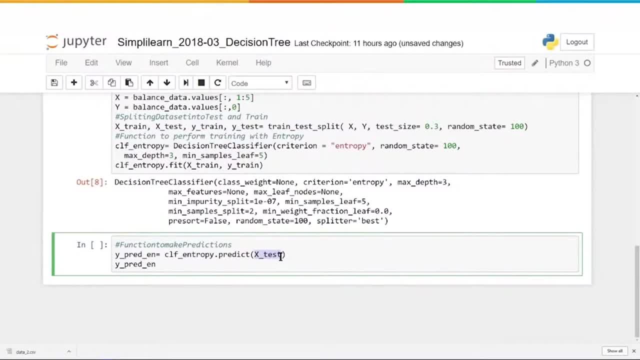 this would be the new loans you're putting in here. to guess whether the person is going to be pay them back or not. In this case, we need to test out the data and just see how good our sample is, how good of our tree does at predicting the loan payments. 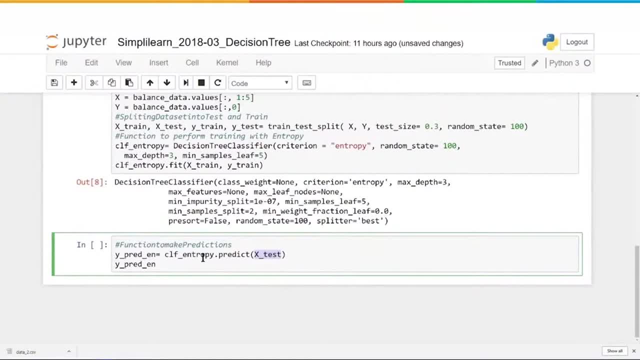 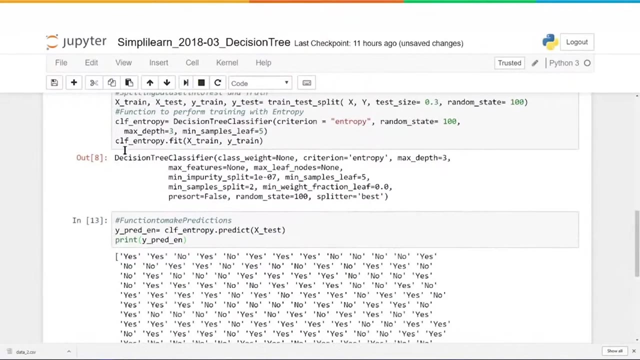 And finally, since Anaconda Jupyter Notebook works as a command line for Python, we can simply put the Y predict to print it. I could just as easily have put the print and put brackets around Y predict to print it out. I'll go ahead and do that. It doesn't matter which way you do it. 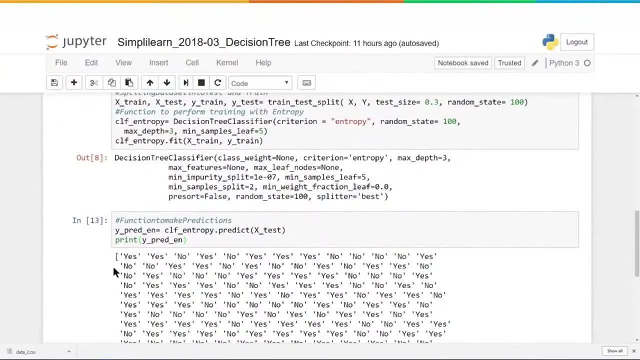 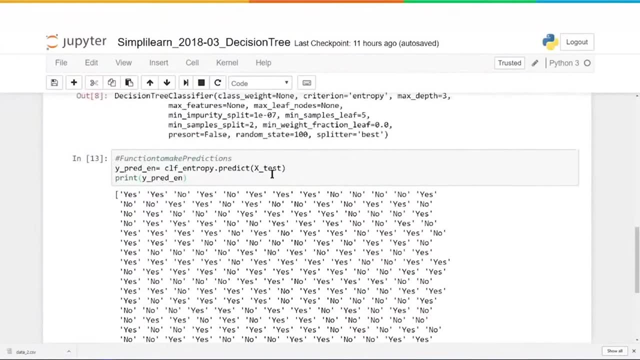 And you'll see right here that it runs a prediction. This is roughly 300 in here. Remember it's 30 percent of a thousand. So you should have about 300 answers in here And this tells you which each one of those lines of our test went in there. 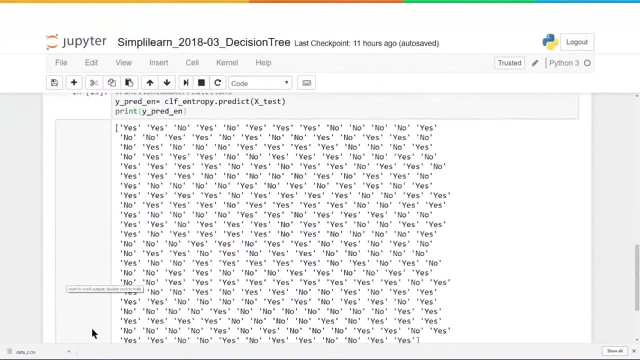 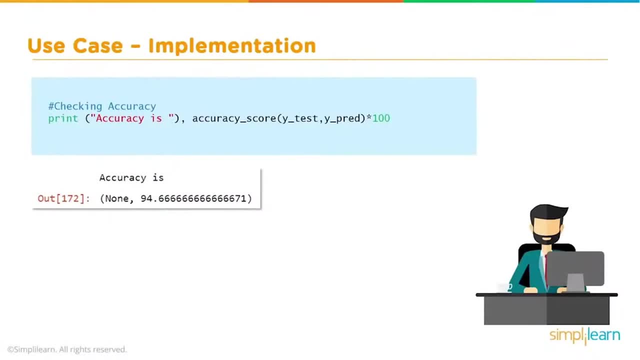 And this is what our Y predict came out. So let's move on to the next step. We're going to take this data and try to figure out just how good a model we have. So here we go. since SK learn does all the heavy lifting for you and all the math, we have a simple line of code. 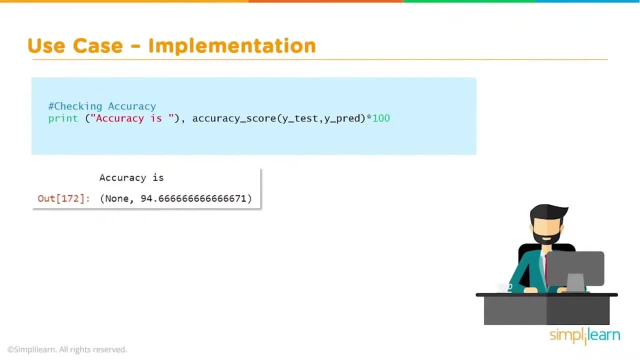 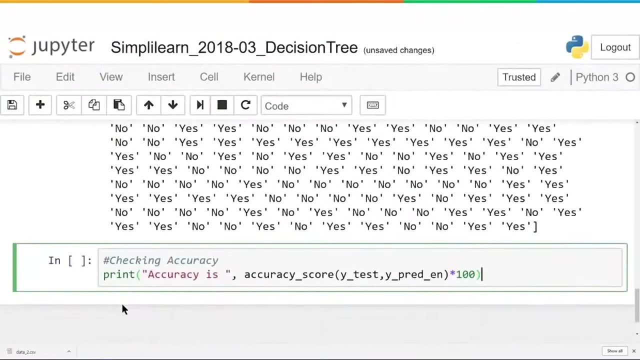 to let us know what the accuracy is. And let's go ahead and go through that and see what that means and what that looks like. Let's go ahead and paste this in and let me zoom in a little bit. There we go, So you have a nice full picture. 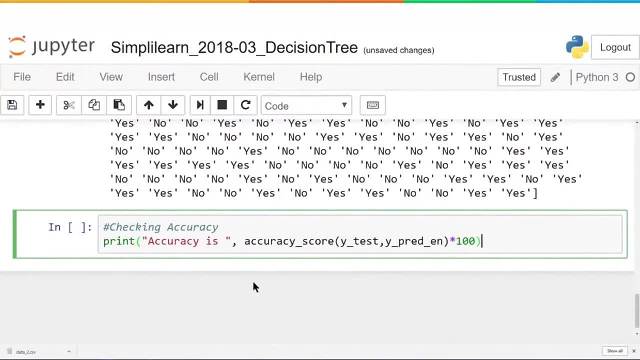 And we'll see here. we're just going to do a print. accuracy is, And then we do the accuracy score And this was something we imported earlier, If you remember, at the very beginning. Let me just scroll up there real quick so you can see where that 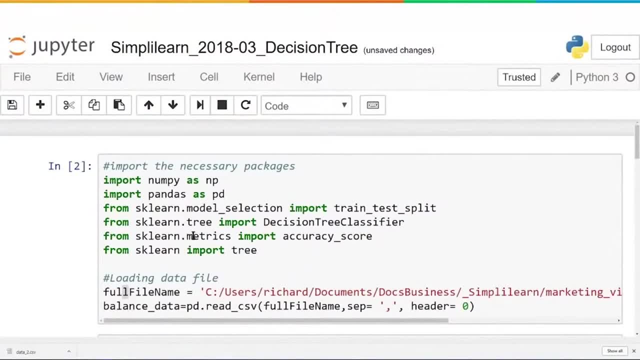 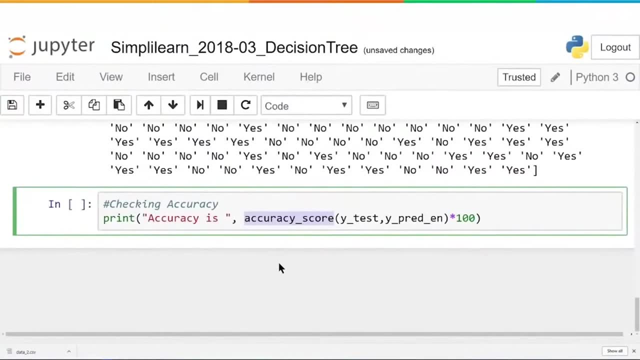 is coming from, That's coming from here, down here from sklearnmetrics import accuracy score And you could probably run a script, make your own script, to do this very easily. How accurate is it? How many out of 300 do we get right? 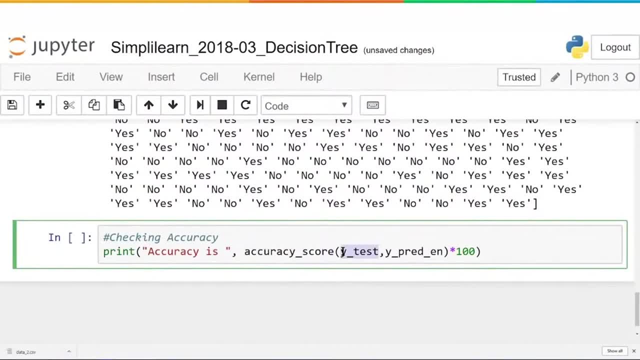 And so we put in our Y test- That's the one we ran the predict on- And then we put in our Y predict EN. That's the answers we got, And we're just going to multiply that by 100, because this is just going to give us. 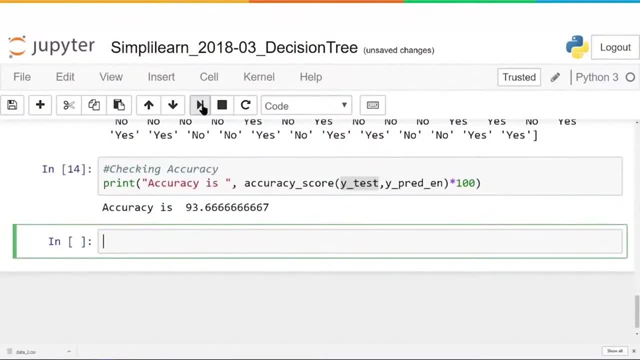 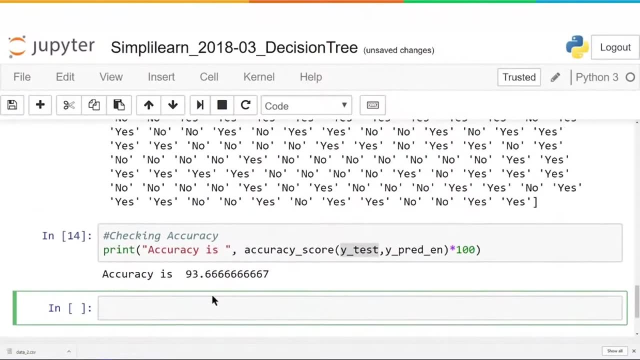 an answer as a decimal and we want to see it as a percentage. So let's run that and see what it looks like. And if you see, here we got an accuracy of 93.66667.. So when we look at the number of loans and we look at how good our model fit, 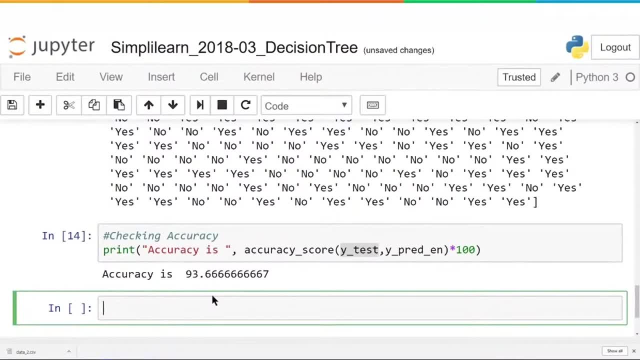 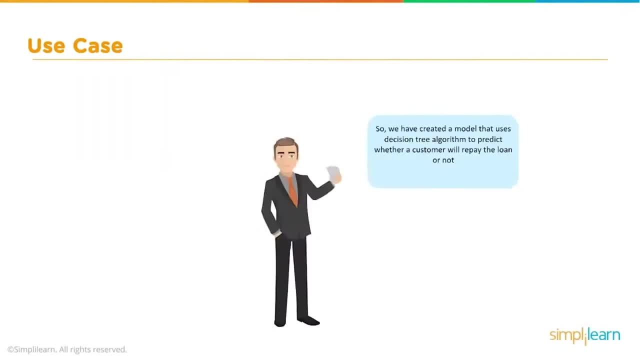 we can tell people it has about a 93.6 fitting to it. So just a quick recap on that. We now have accuracy set up on here, And so we have created a model that uses the decision tree algorithm to predict whether a customer will repay the loan or not. 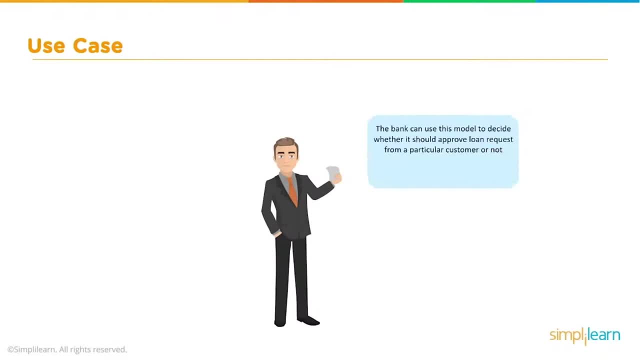 The accuracy of the model is about 94.6 percent. The bank can now use this model to decide whether it should approve the loan request from a particular customer or not, And so this information is really powerful. We may not be able to as individuals. 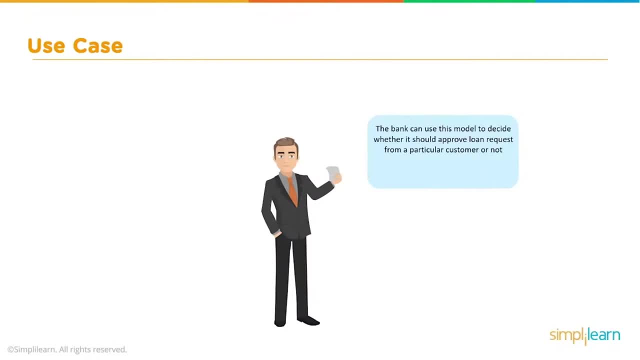 understand all these numbers because they have thousands of numbers that come in, But you can see that this is a smart decision for the bank to use a tool like this to help them to predict how good their profits going to be off of the loan balances and how many are going to default or not. 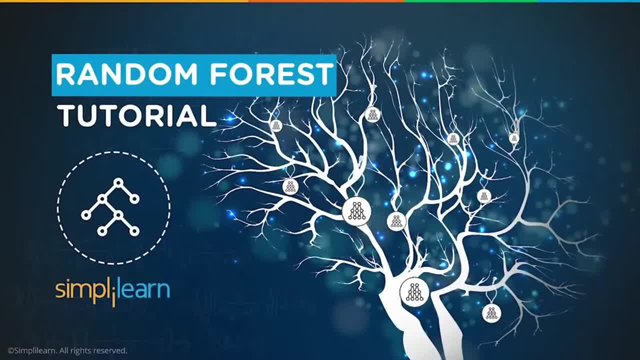 We're going to be looking at Random Forest, one of the many powerful tools in the machine learning library. Before we dive into the topic, let's start by looking at a few of the uses for Random Forest Currently. today is used in remote sensing. 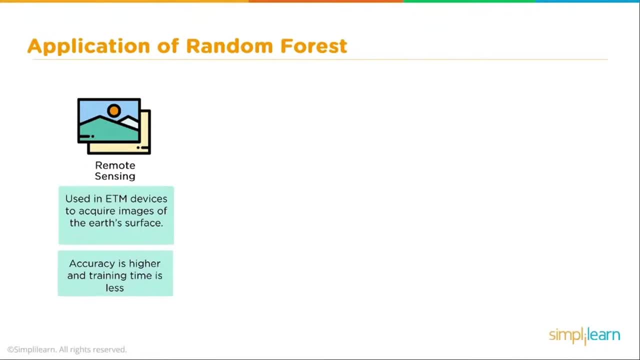 For example, they're used in the ETM devices. If you're a space buff, that's the Enhanced Thermatic Mapper. they use on satellites which see far outside the human spectrum for looking at land masses and they acquire images of the Earth's surface. 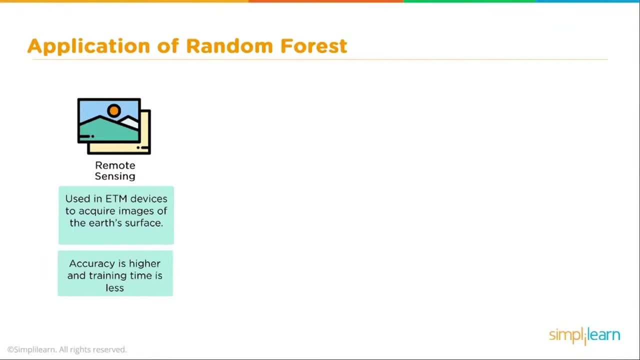 The accuracy is higher and training time is less than any other machine learning tools out there. Also, object detection. multi-class object detection is done using Random Forest algorithms. A good example is traffic. We try to sort out the different cars, buses and things and it provides a better detection in complicated environments. 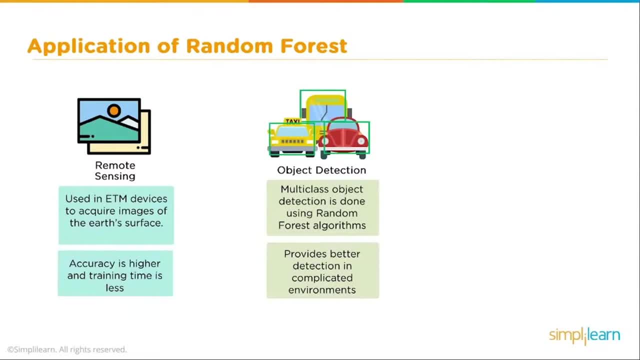 It's very complicated up there. And then we have another example, Connect, And let's take a little closer look at Connect. Connect, they use a Random Forest as part of the game console, And what it does is it tracks the body movements and it recreates it in the game. 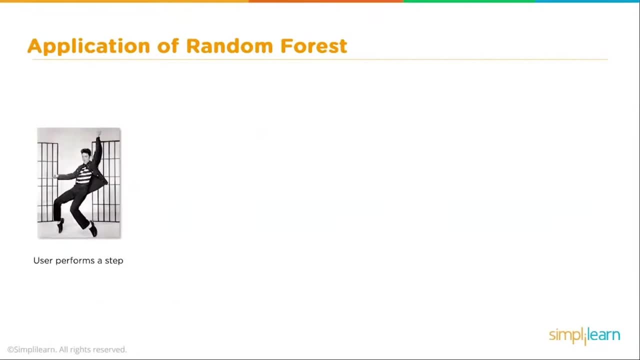 And let's see what that looks like. We have a user who performs a step. In this case it looks like Elvis Presley going there. That is then recorded, So the Connect registers the movement and then it marks the user based on accuracy. 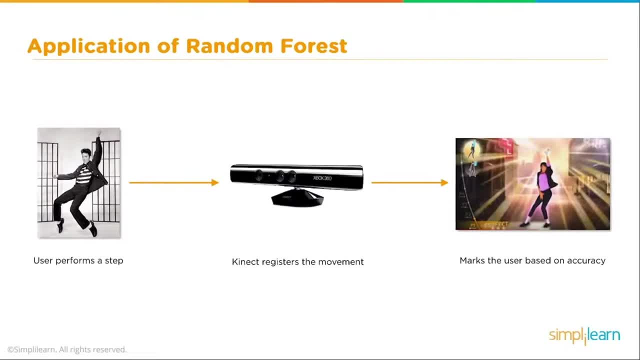 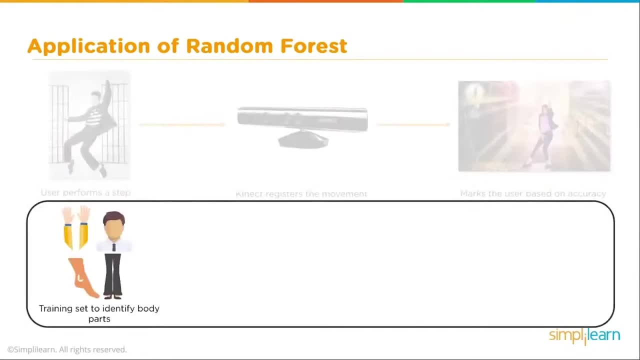 And it looks like we have Prince going on. this one from Elvis Presley to Prince, It's great. So it marks the user based on the accuracy. If we look at that a little closer, we have a training set to identify body parts. 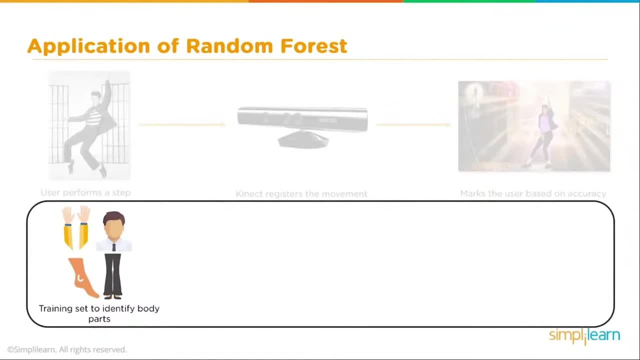 Where are the hands? Where are the feet? What's going on with the body? That then goes into a Random Forest classifier that learns from it. Once we train the classifier, it then identifies the body parts while the person's dancing. It's able to represent that in a computer format. 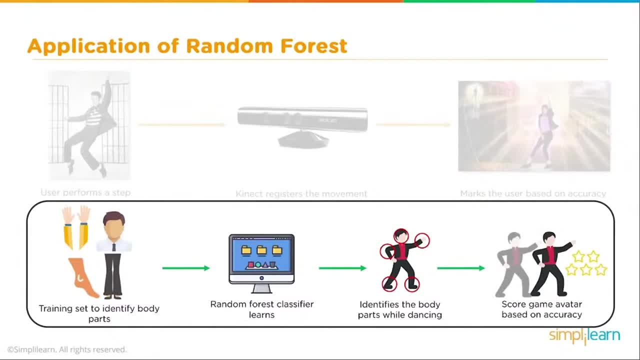 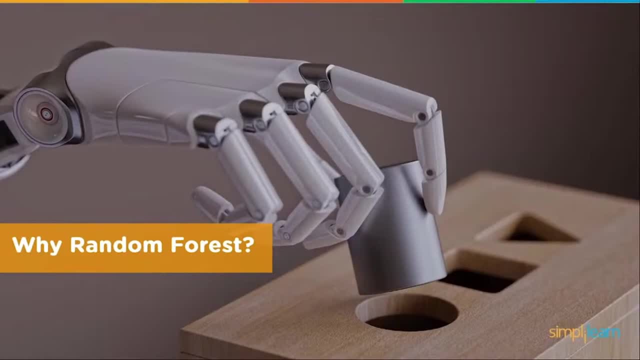 And then, based on that, it scores the game and how accurate you are as being Elvis Presley or Prince and you're dancing. So why Random Forest? It's always important to understand why we use this tool over the other ones. What are the benefits here? 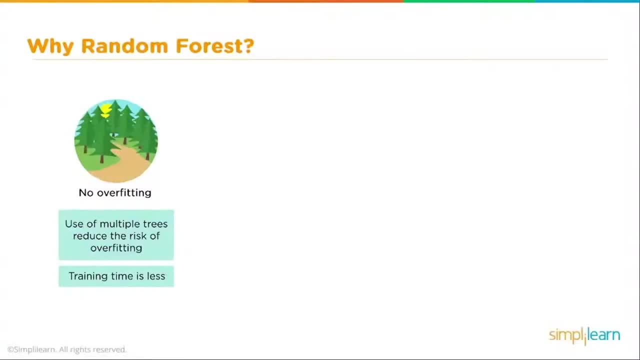 And so with the Random Forest. the first one is: there's no overfitting. If you use of multiple trees, reduce the risk of overfitting. Training time is less Overfitting means that we have fit the data so close to what we have as our. 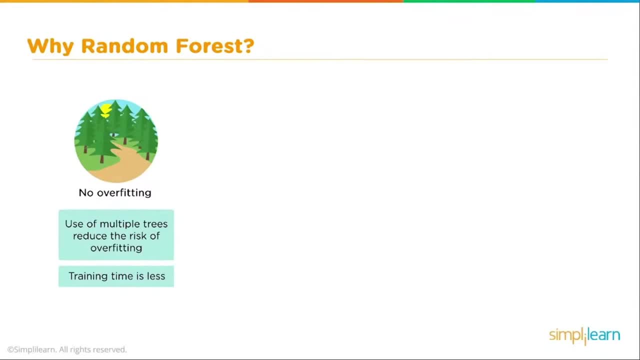 sample that we pick up on all the weird parts And, instead of predicting the overall data, you're predicting the weird stuff which you don't want. High accuracy Runs efficiently on large database. For large data it produces highly accurate predictions. 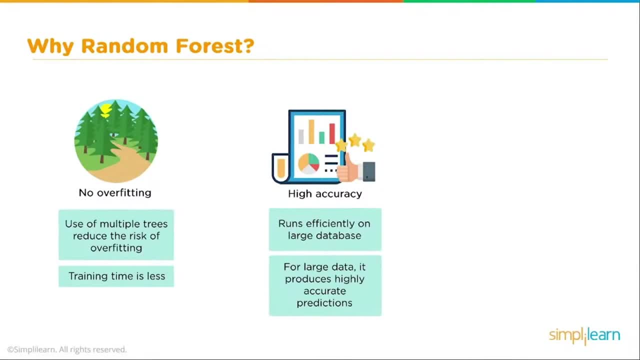 In today's world of big data, this is really important And this is probably where it really shines. This is where why Random Forest really comes in. It estimates missing data. Data in today's world is very messy, So when you have a Random Forest, 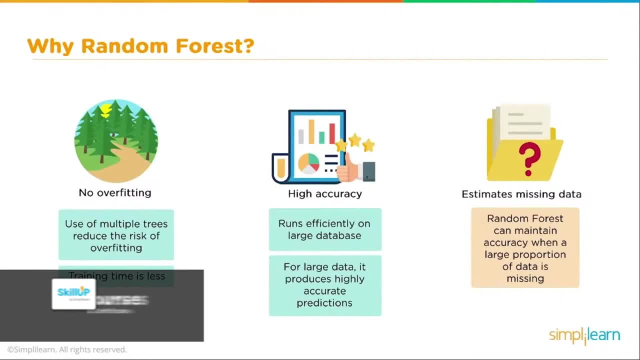 it can maintain the accuracy when a large proportion of the data is missing. What that means is if you have data that comes in from five or six different areas and maybe they took one set of statistics in one area and they took a slightly different set of statistics in the other. 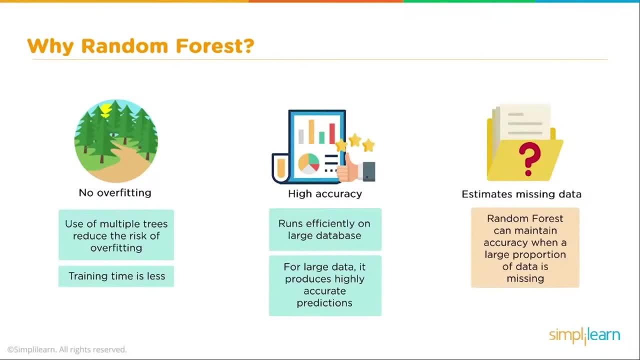 So they have some of the same shared data, but one is missing, like the number of children in the house, If you're doing something over demographics, and the other one is missing- the size of the house. it will look at both of those separately and build two different trees and then it can do a very good job. 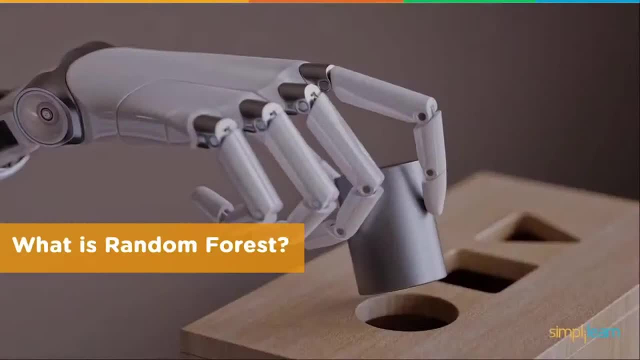 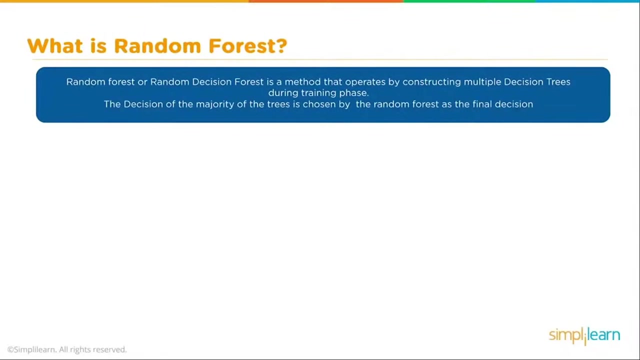 of guessing which one fits better, even though it's missing that data. Let us dig deep into the theory of exactly how it works and let's look at what is Random Forest. Random Forest or Random Decision Forest is a method that operates by constructing multiple decision trees, The decision of the majority of the trees. 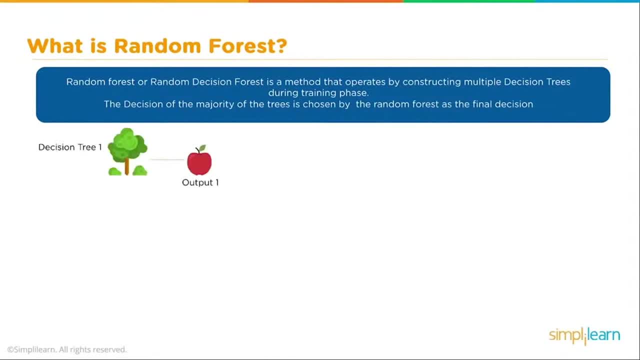 is chosen by the Random Forest as the final decision. And we have some nice graphics here. We have a decision tree and they actually use a real tree to denote the decision tree, which I love, And given a random some kind of picture of a fruit. 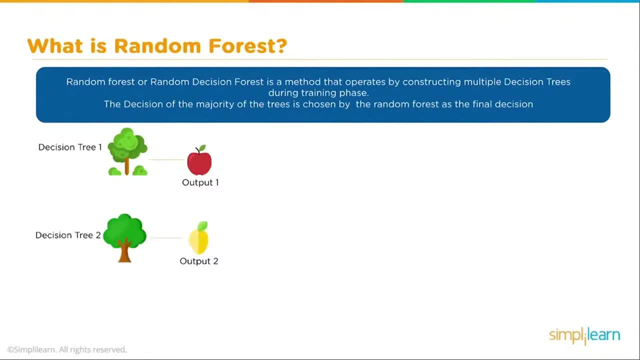 this decision tree decides that the output is it's an apple. And we have a decision tree too, where we have a picture of the fruit goes in and this one decides that it's a lemon. and the decision tree tree gets another image and it decides it's an apple. 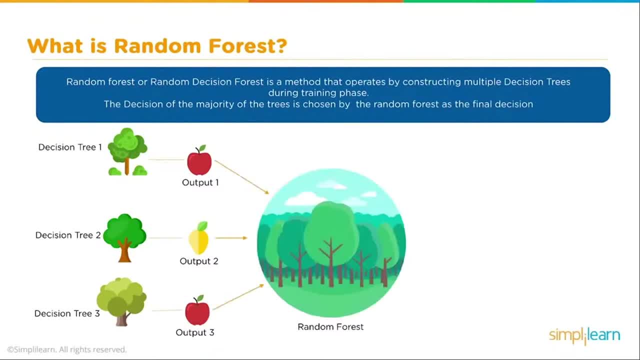 And then this all comes together in what they call the random forest. And this random forest then looks at it and says: OK, I got two votes for apple, one vote for lemon. the majority is apples, So the final decision is apples. 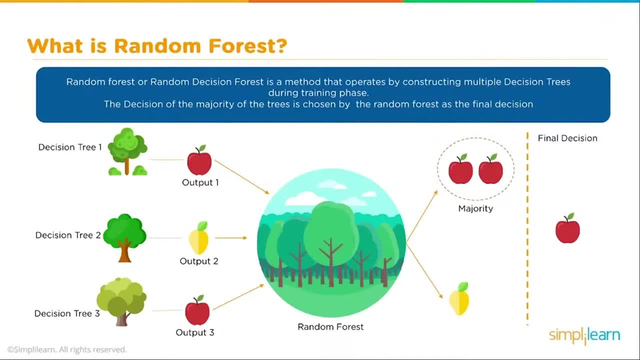 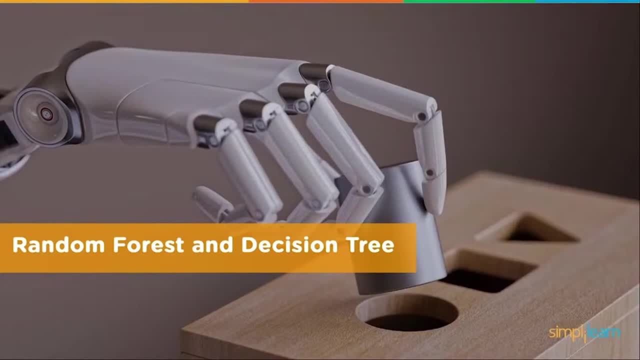 To understand how the random forest works, we first need to dig a little deeper and take a look at the random forest and the actual decision tree and how it builds that decision tree. in looking closer at how the individual decision trees work, We'll go ahead and continue to use the fruit example, since we're talking about 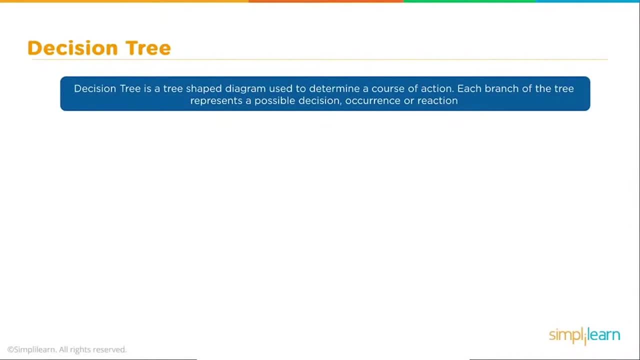 trees and forests. a decision tree is a tree shaped diagram used to determine a course of action. Each branch of the tree represents a possible decision, occurrence or reaction. So in here we have a bowl of fruit And if you look at that it looks like they switched from lemons to oranges. 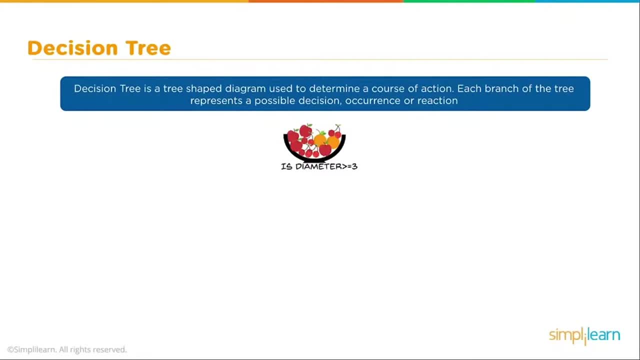 We have oranges, cherries and apples, And the first decision of the decision tree might be, as a diameter, greater than or equal to three, And if it says false, it knows that they're cherries because everything else is bigger than that, So all the cherries fall into that decision. 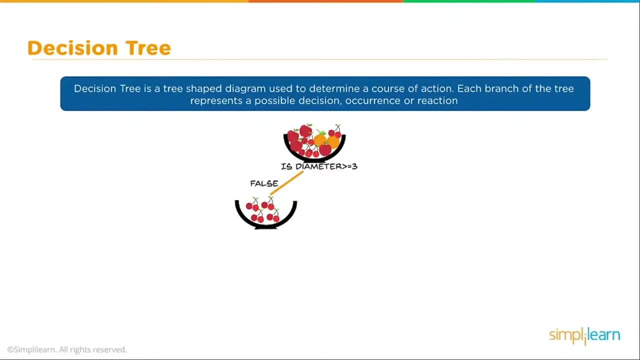 So we have all that data, we're training, We can look at that. We know that that's what's going to come up. Is the color orange? Well, it goes. hmm, orange or red? Well, if it's true, then it comes out as the orange. 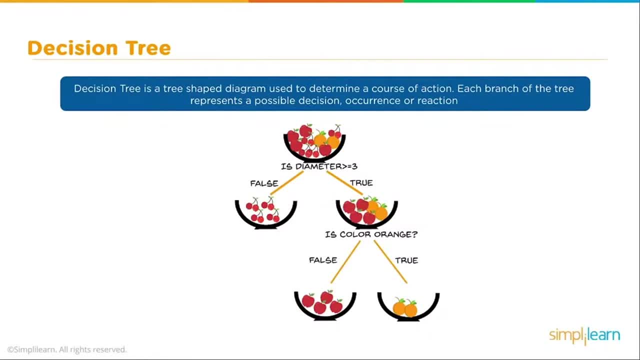 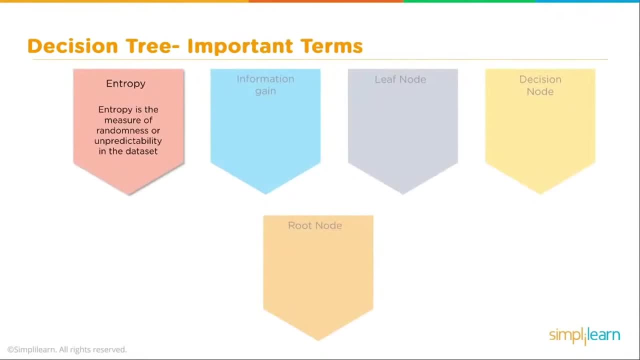 And if it's false, that leaves apples. So in this example, it sorts out the fruit in the bowl or the images of the fruit A decision tree. These are very important terms to know because these are very central to understanding the decision tree and when working with them. 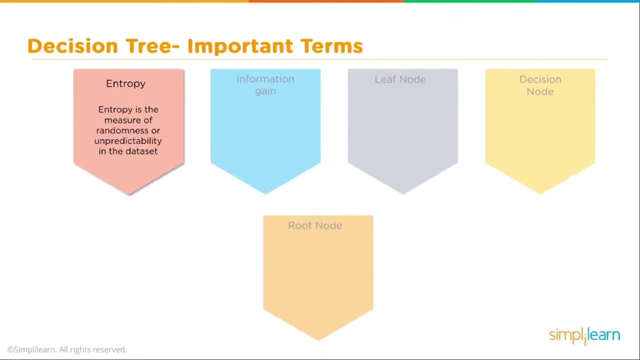 The first is entropy. Everything on the decision tree and how it makes a decision is based on entropy. Entropy is a measure of randomness or unpredictability in the data set. Then they also have information gain: the leaf node, the decision node and the root node. 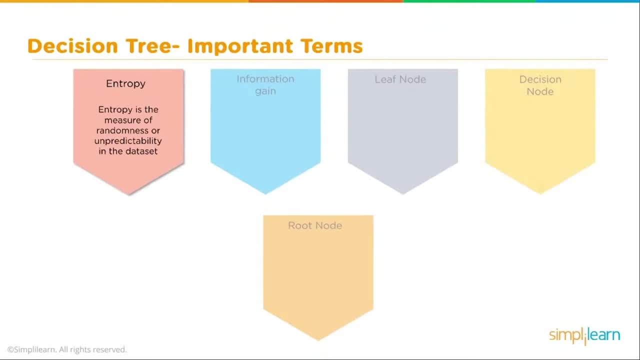 We'll cover these other four terms as we go down the tree, But let's start with entropy. So, starting with entropy, we have here a high amount of randomness. What that means is that, whatever is coming out of this decision, if it was going to guess based on this data, 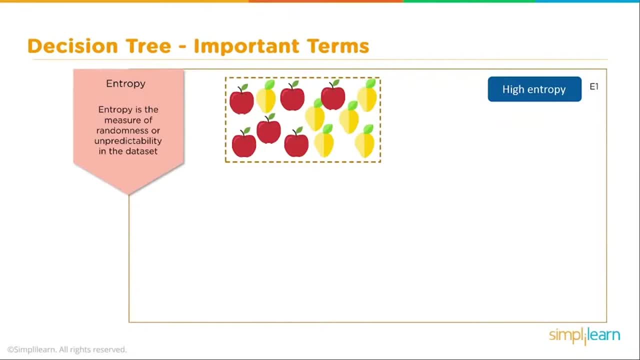 it wouldn't be able to tell you whether it's a lemon or an apple. It would just say it's a fruit. So the first thing we want to do is we want to split this apart and we take the initial data set. we're going to create a data set one and a data set two. 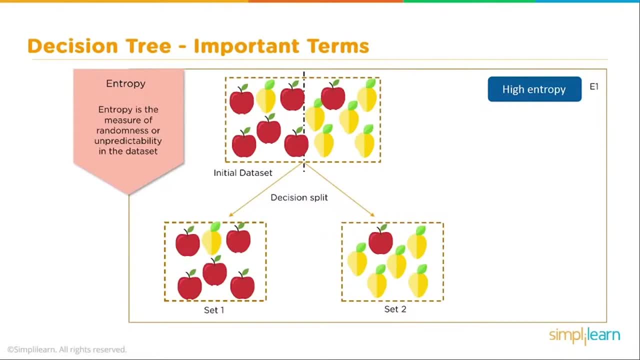 We just split it in two And if you look at these new data sets after splitting them, the entropy of each of those sets is much less. So for the first one, whatever comes in there, it's going to sort that data and it's going to say OK. 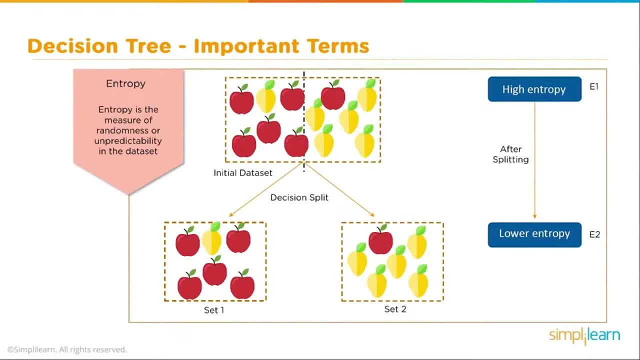 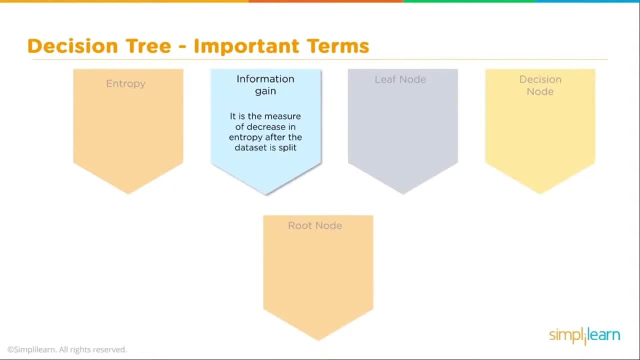 if this data goes this direction, it's probably an apple, And if it goes into the other direction, it's probably a lemon. So that brings us up to information gain. It is the measure of decrease in the entropy after the data set is split. 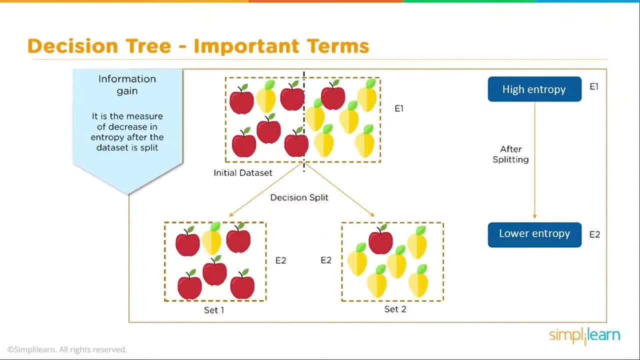 What that means in here is that we've gone from one set which has a very high entropy to two lower sets of entropy And we've added in the values of E1 for the first one and E2 for the second, two which are much lower. 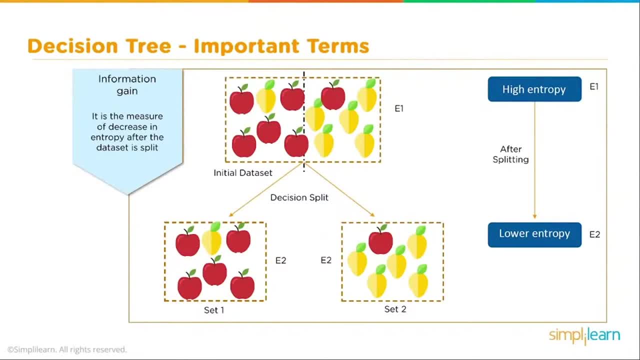 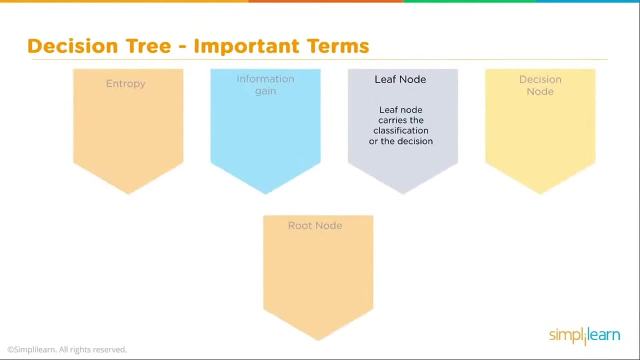 And so that information gain is increased greatly in this example, And so you can find that the information gain simply equals decision E1 minus E2.. As we're going down our list of definitions, we'll look at the leaf node, and the leaf node carries the classification or the decision. 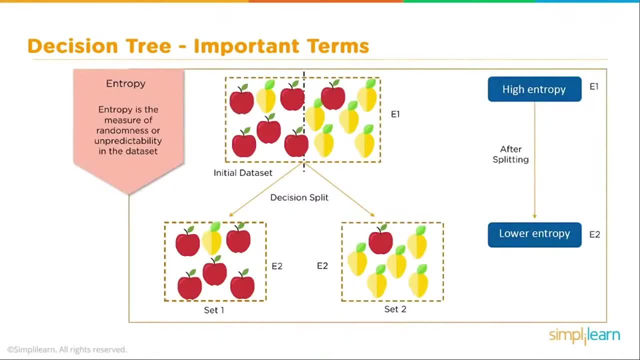 So we look down here to the leaf node, We finally get to our set one or our set two. When it comes down there and it says, OK, this object's gone into set one. If it's gone into set one, it's going to be split by some means. 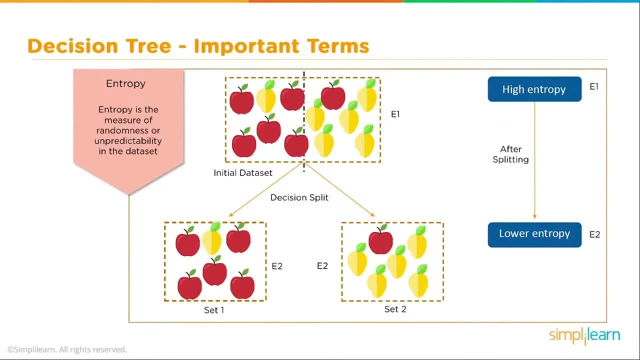 And we'll either end up with apples on the leaf node or a lemon on the leaf node, And on the right it'll either be an apple or lemons. Those leaf nodes are those final decisions or classifications. That's the definition of leaf node in here. 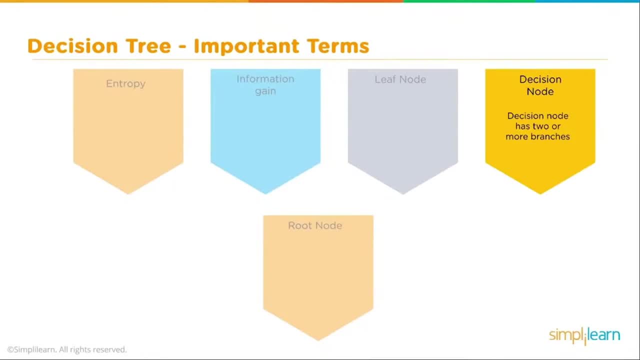 If we're going to have a final leaf where we make the decision, we should have a name for the nodes above it And they call those decision nodes A decision node. decision node has two or more branches And you can see here where we have the five apples and one lemon. 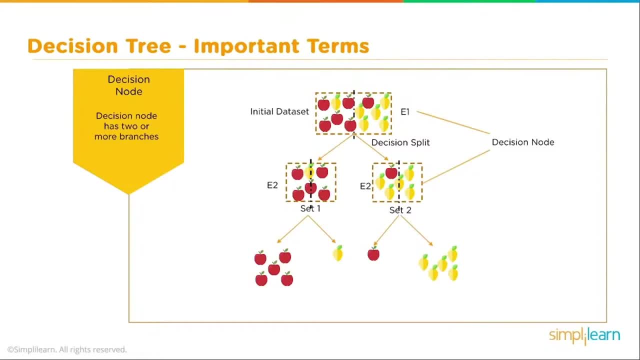 And in the other case, the five lemons and one apple. They have to make a choice of which tree it goes down, based on some kind of measurement or information given to the tree. And that brings us to our last definition: the root node, the top, most decision node. 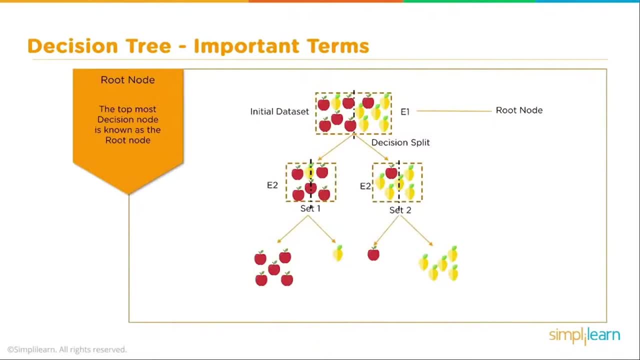 is known as the root node, And this is where you have all of your data and you have your first decision it has to make, or the first split in information So far. we've looked at a very general image, with the fruit being split. 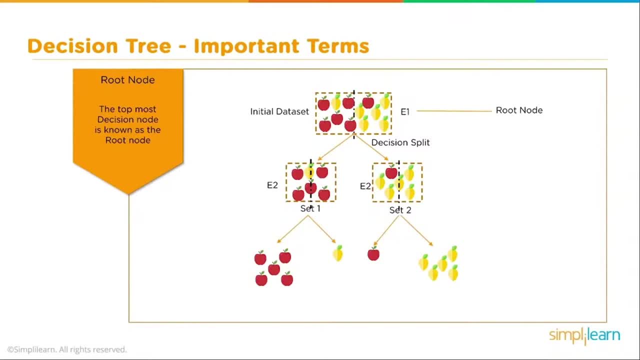 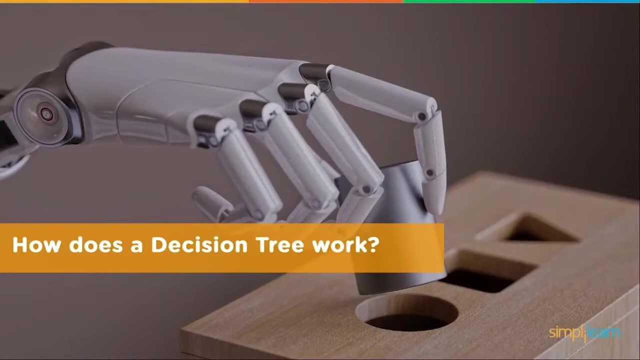 Let's look and see exactly what that means to split the data And how do we make those decisions on there? Let's go in there and find out. how does a decision tree work? So let's try to understand this and let's use a simple example. 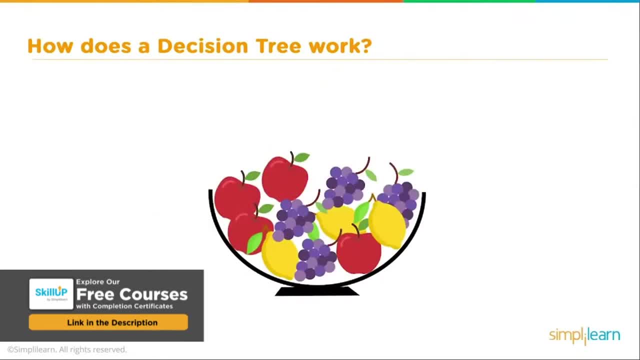 And we'll stay with the fruit. We have a bowl of fruit, And so let's create a problem statement, And the problem is we want to classify the different types of fruits in the bowl based on different features. The data set in the bowl is looking quite messy and the entropy is high in this case. 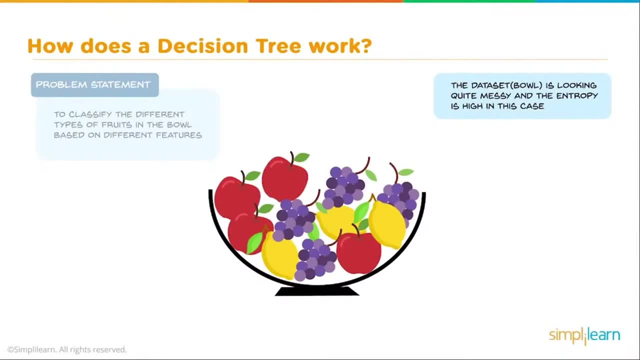 So if this bowl was our decision maker, it wouldn't know what choice to make. It has so many choices. Which one do you pick? Apple, grapes or lemons? And so we look in. here we're going to start with a training set. 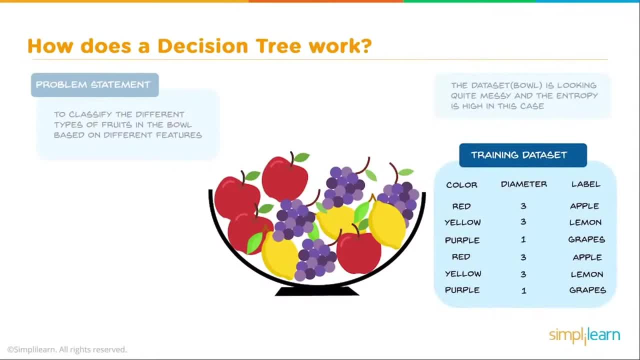 So this is our data, that we're training our data with, And we have a number of options. here We have the color and under the color we have red, yellow, purple. We have a diameter: three, three, one, three, three one. 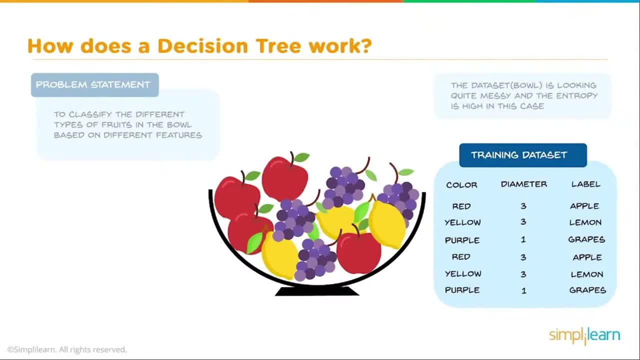 And we have a label- apple lemon grapes, apple lemon grapes. And how do we split the data? We have to frame the conditions to split the data in such a way that the information gain is the highest. It's very key to note that we're looking for the best gain. 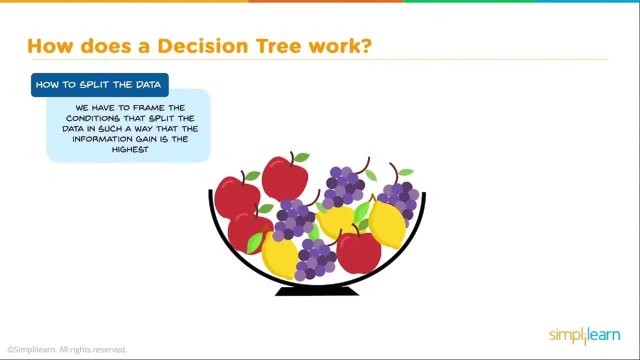 We don't want to just start sorting out the smallest piece in there. We want to split it the biggest way we can, And so we measure this decrease in entropy. That's what they call it Entropy. There's our entropy after splitting. 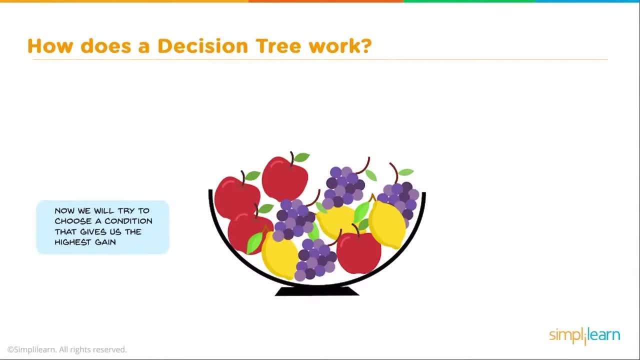 And now we'll try to choose a condition that gives us the highest gain. We will do that by splitting the data, using each condition and checking the gain that we get out of them. The conditions that give us the highest gain will be used to make the first split. 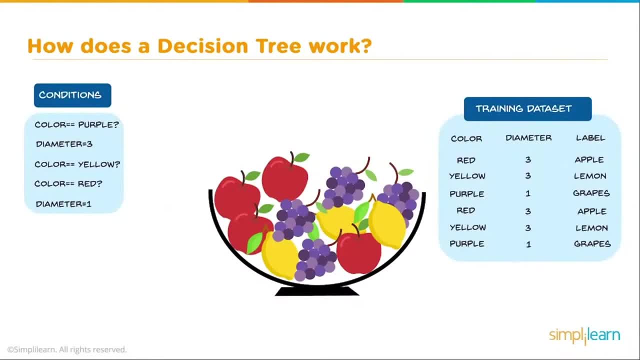 So let's take a look at these different conditions. We have color, we have diameter And if we look underneath that, we have a couple of different values. We have: diameter equals three, color equals yellow, Red, diameter equals one, And when we look at that you'll see over here we have one, two, three, four, threes. 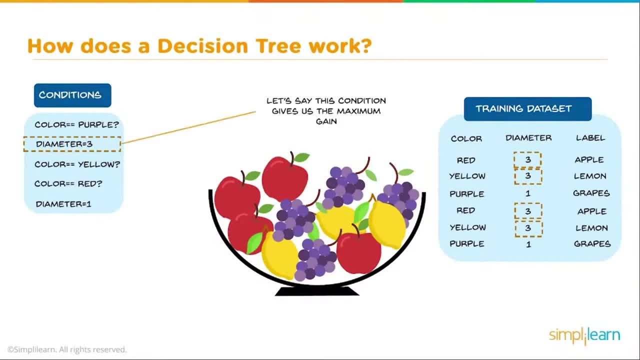 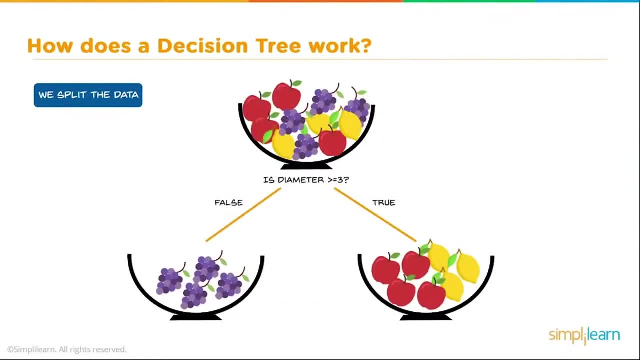 That's a pretty hard selection. So let's say the condition gives us the maximum gain of three, So we have the most pieces fall into that range. So our first split from our decision node is we split the data based on the diameter. Is it greater than or equal to three? 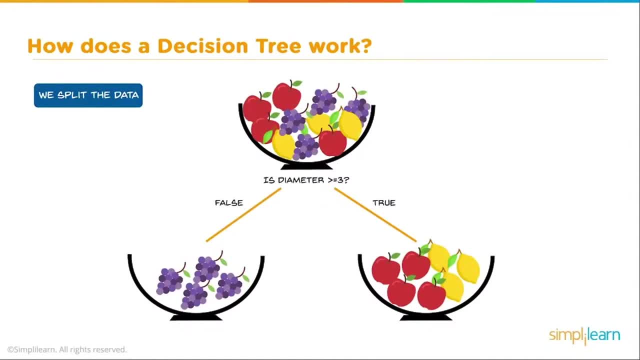 If it's not- that's false- It goes into the great bowl, And if it's true, it goes into a bowl full of lemon and apples. The entropy after splitting has decreased considerably, So now we can make two decisions. If you look at, they're very much less chaos going on there. 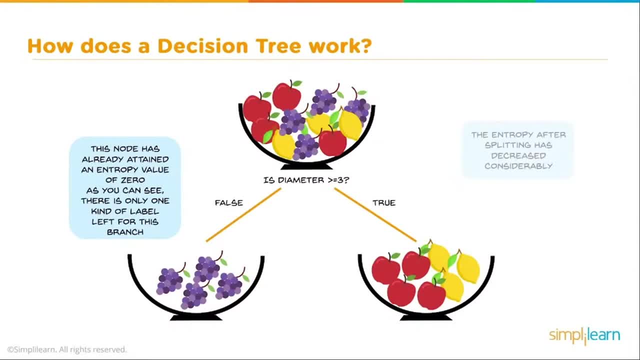 This node has already attained an entropy value of zero. As you can see, there's only one kind of label left for this branch, So no further splitting is required for this node. However, this node on the right is still requires a split to decrease the entropy further. 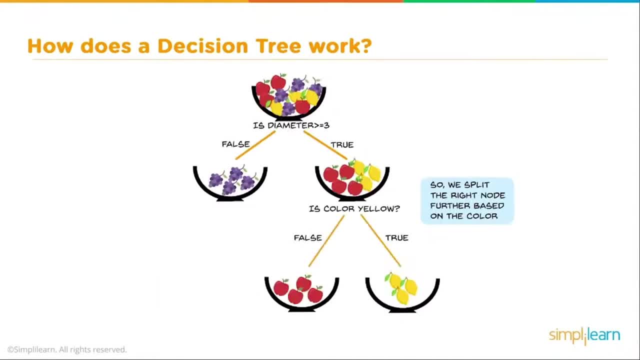 So we split the right node further based on color. If you look at this, if I split it on color, that pretty much cuts it right down the middle. That's the only thing we have left in our choices of color and diameter too. 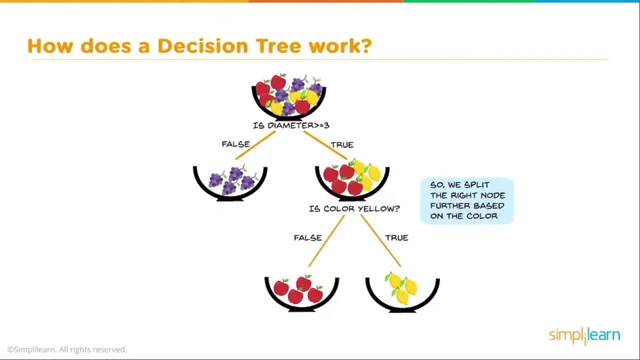 And if the color is yellow, it's going to go to the right bowl, And if it's false, it's going to go to the left bowl. So the entropy in this case is now zero. So now we have three bowls with zero entropy. 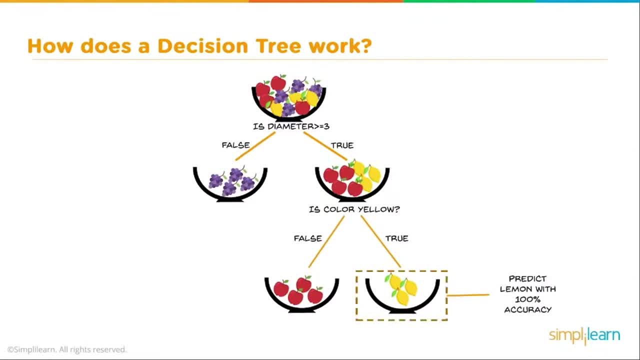 There's only one type of data in each one of those bowls. So we can predict a lemon with 100 percent accuracy And we can predict the apple also with 100 percent accuracy, along with our grapes up there. So we've looked at kind of a basic tree in our forest. 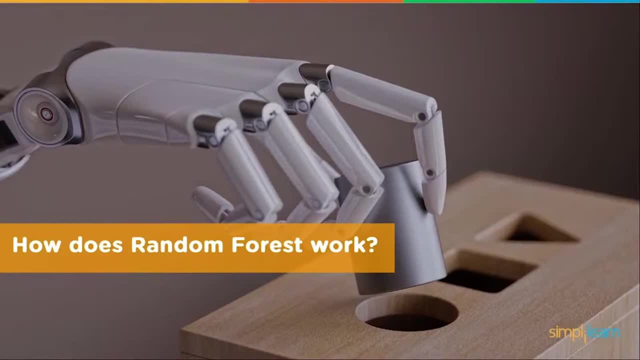 But what we really want to know is: how does a random forest work as a whole? So to begin our random forest classifier, let's say we already have built three trees And we're going to start with the first tree that looks like this: 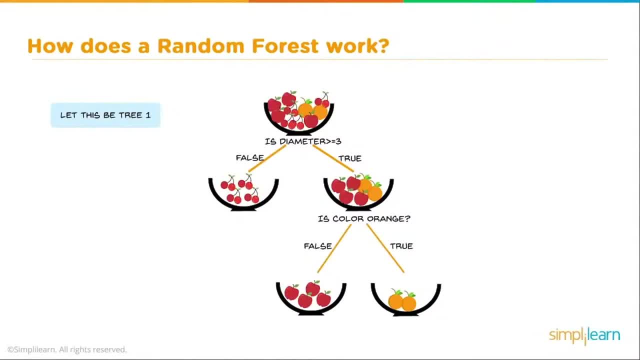 Just like we did in the example, this tree looks at the diameter. If it's greater than or equal to three, it's true. Otherwise it's false. So one side goes to the smaller diameter, one side goes to larger diameter. 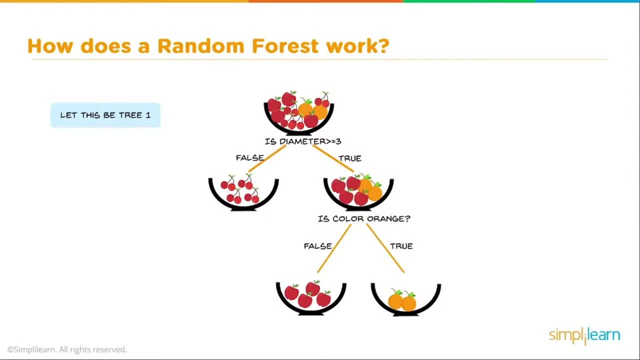 And if the color is orange, it's going to go to the right. true, We're using oranges now instead of lemons. And if it's red, it's going to go to the left. false, We build a second tree, very similar, but it's split differently. 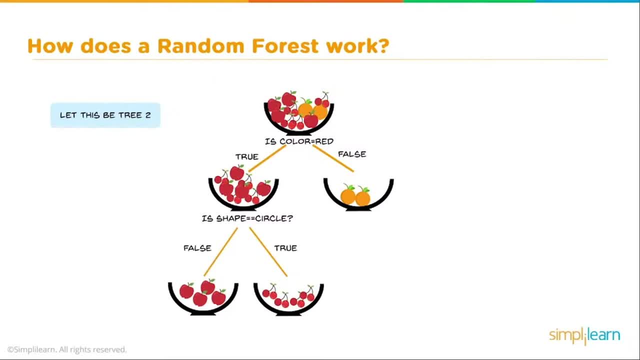 Instead of the first one being split by a diameter, this one when they created it. if you look at that first bowl, it has a lot of red objects. So it says, is the color red because that's going to bring our entropy down the fastest? 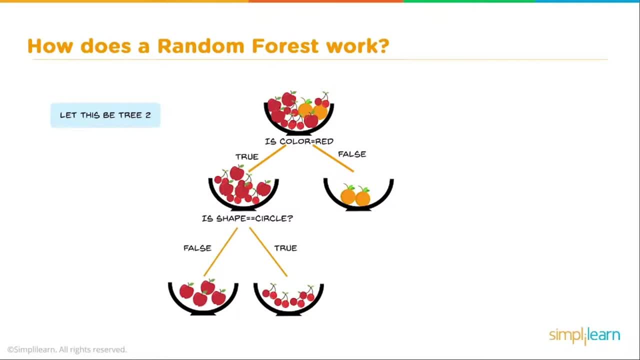 And so, of course, if it's true, it goes to the left, If it's false it goes to the right, And then it looks at the shape: false or true, and so on and so on. And tree three is the diameter equal to one. 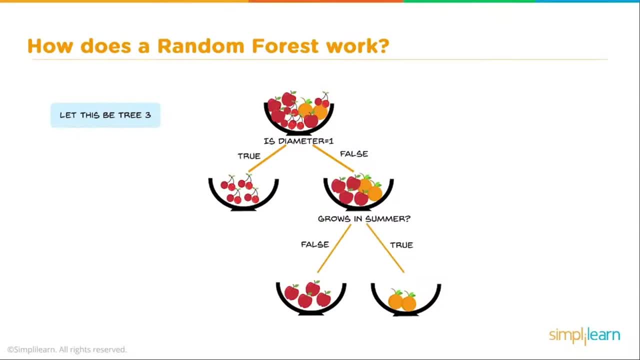 And it came up with this because there's a lot of cherries in this bowl, So that would be the biggest split on there is is the diameter equal to one. That's going to drop the entropy the quickest And, as you can see, it splits it into true. 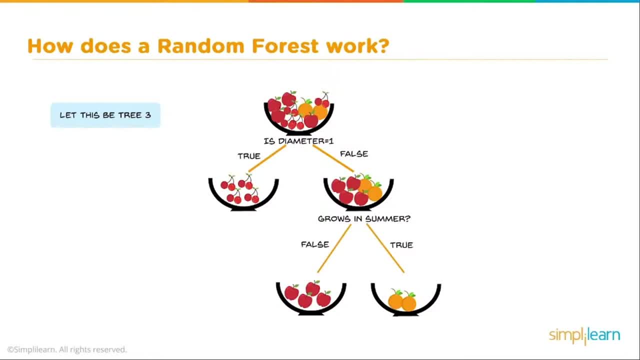 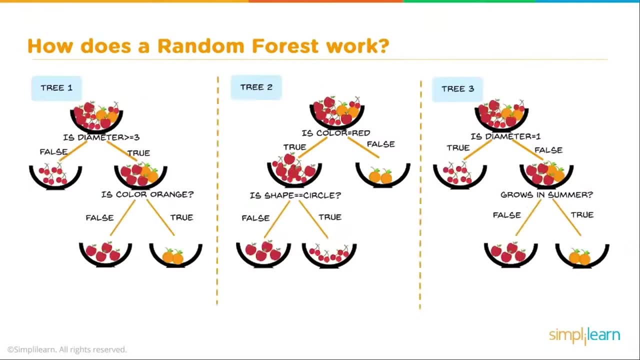 If it goes false- and they've added another category- does it grow in the summer? And if it's false, it goes off to the left. If it's true, it goes off to the right. Let's go ahead and bring these three trees, so you can see them all in one image. 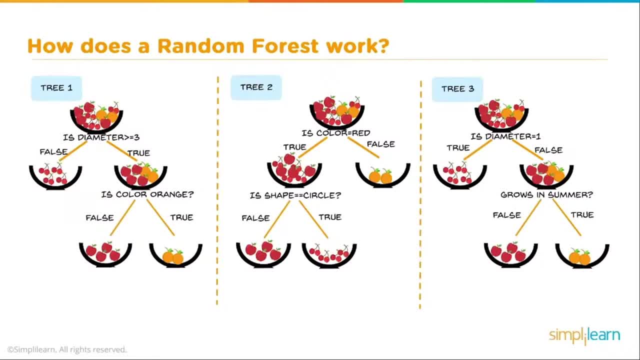 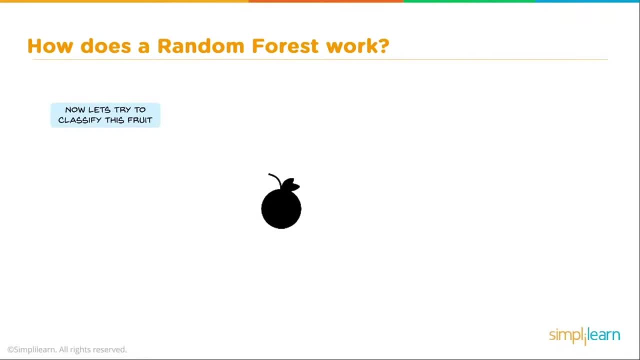 So this would be three completely different trees categorizing a fruit. And let's take a fruit. Now let's try this And this fruit. if you look at it, we've blackened it out. You can't see the color on it, so it's missing data. 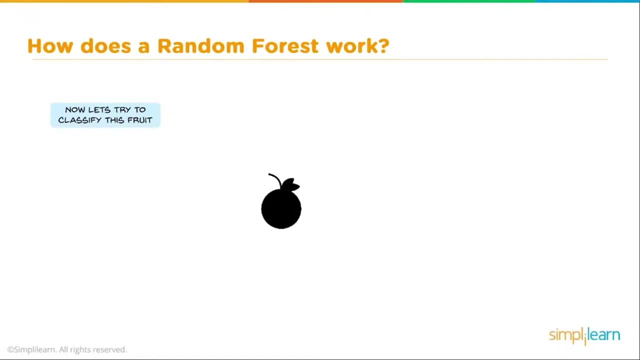 Remember, one of the things we talked about earlier is that a random forest works really good if you're missing data, if you're missing pieces. So this fruit has an image. the person had a black and white camera when they took the picture. 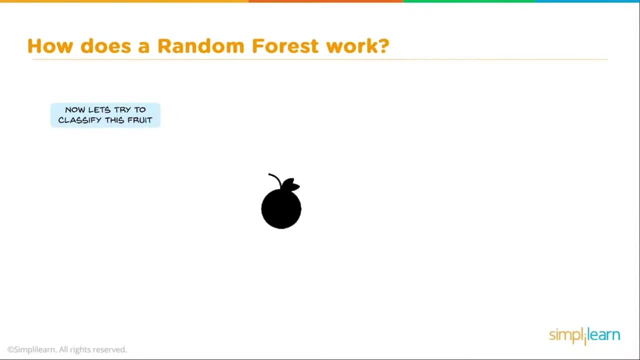 And we're going to take a look at this and it's going to have they put the color in there, so ignore the color down there. But the diameter equals three, We find out it grows in the summer. equals yes, And the shape is a circle. 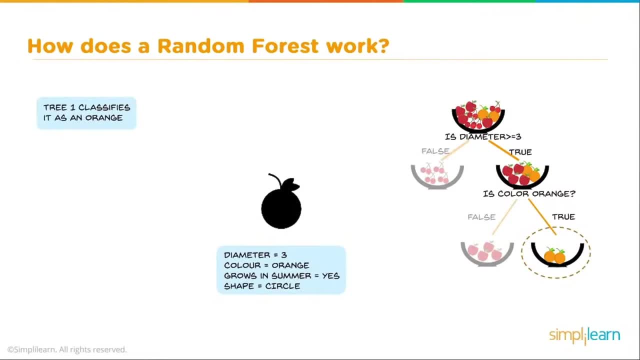 And if you go to the right, you can look at what one of the decision trees did. This is the third one. Is the diameter greater than equal to three? Is the color orange? Well, it doesn't really know on this one. 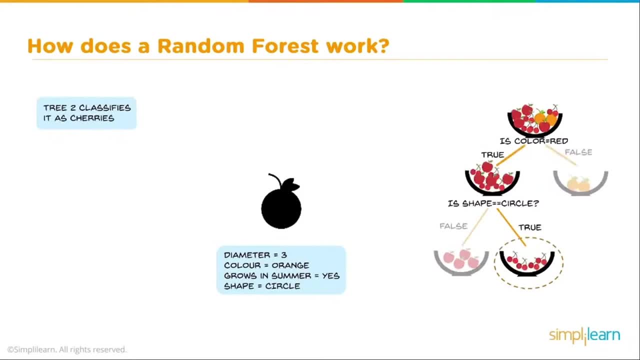 but if you look at the value, it'd say true and it'd go to the right Q classifies it as cherries. Is the color equal red. Is the shape a circle? True, It is a circle. So this would look at it and say, oh, that's a cherry. 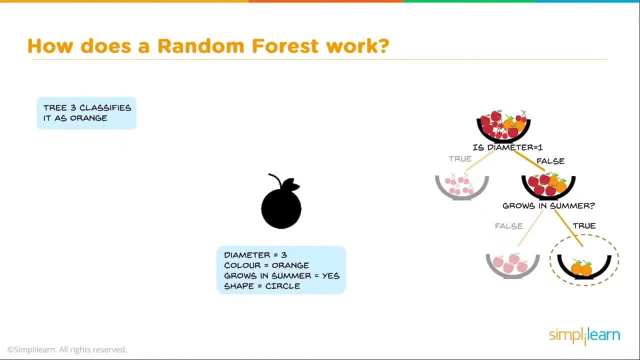 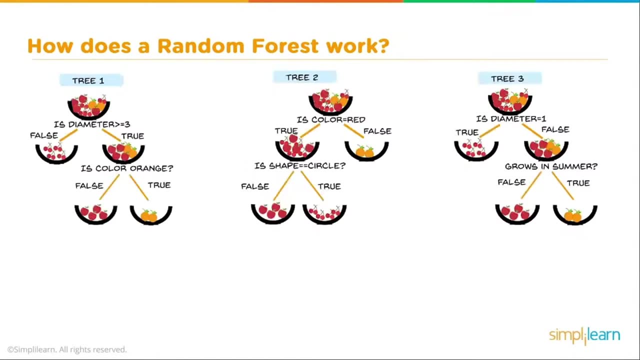 And then we go to the other classifier and it says: is the diameter equal one? Well, that's false. Does it grow in the summer? True, So it goes down and looks at as oranges. So how does this random forest work? 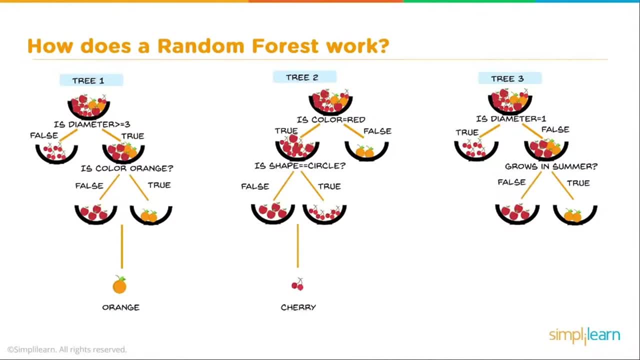 The first one says it's an orange, The second one said it was a cherry And the third one says it's an orange. And you can guess that if you have two oranges and one says it's a cherry, when you add that all together, 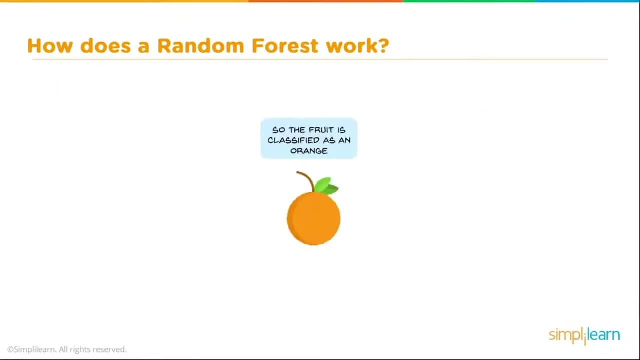 the majority of the vote says orange, So the answer is: it's classified as an orange, even though we didn't know the color and we're missing data on it. I don't know about you, but I'm getting tired of fruit, So let's switch. 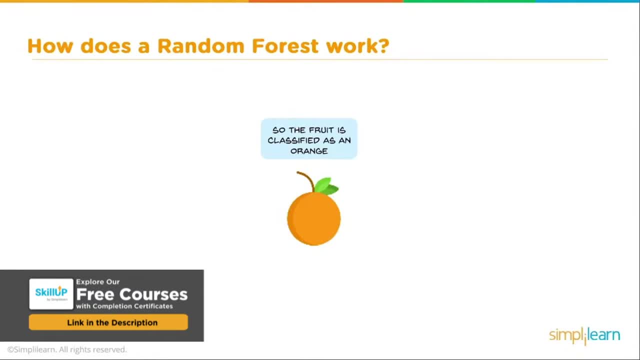 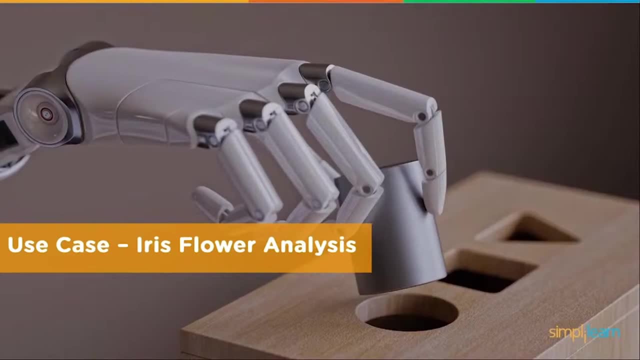 And I did promise you we'd start looking at a case example and get into some Python coding. Today we're going to use the case the Iris Flower Analysis. This is the exciting part, as we roll up our sleeves and actually look at some Python coding. before we start the Python coding: 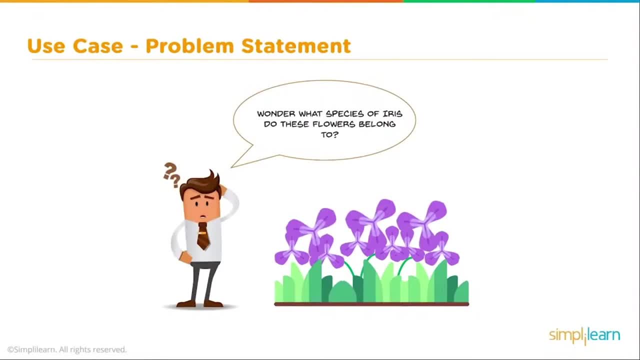 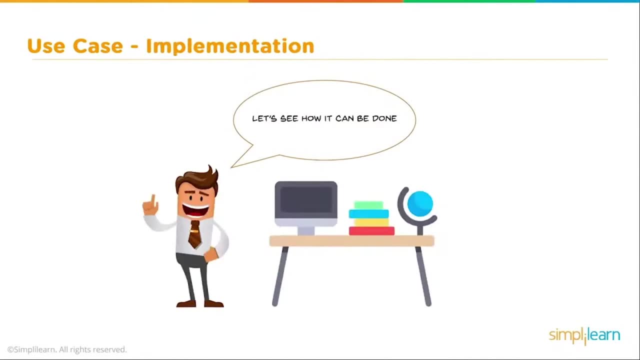 We need to go ahead and create a problem statement, Wonder: what species of Iris do these flowers belong to? Let's try to predict the species of the flowers using machine learning in Python. Let's see how it can be done. So here we begin to go ahead and implement our Python code. 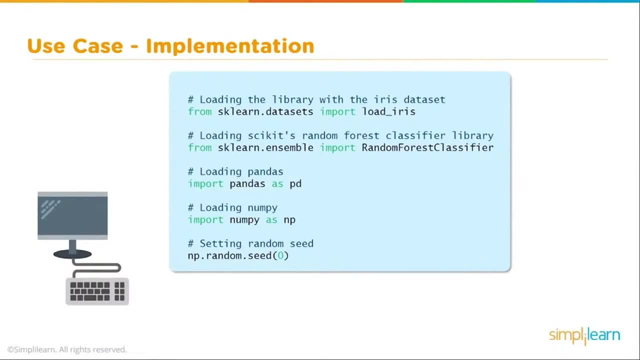 And you'll find that the first half of our implementation is all about organizing and exploring the data coming in. Let's go ahead and take this first step, which is loading the different modules Into Python, and let's go ahead and put that in our favorite editor. 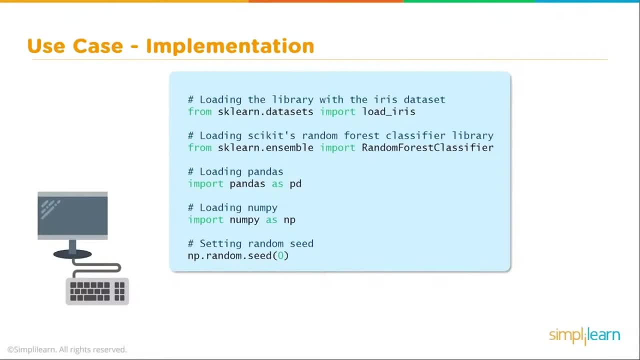 whatever your favorite editor is- In this case I'm going to be using the Anaconda Jupyter Notebook, which is one of my favorites. Certainly there's Notepad++ and Eclipse and dozens of others, or just even using the Python terminal window. 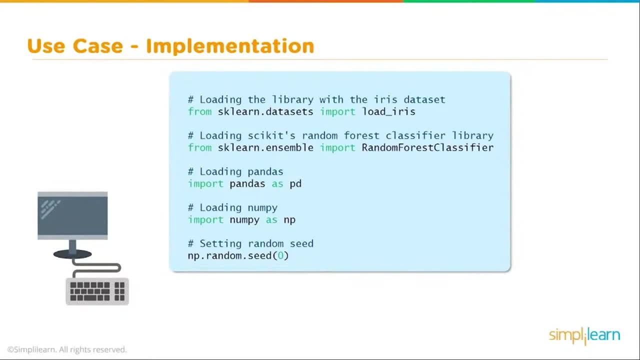 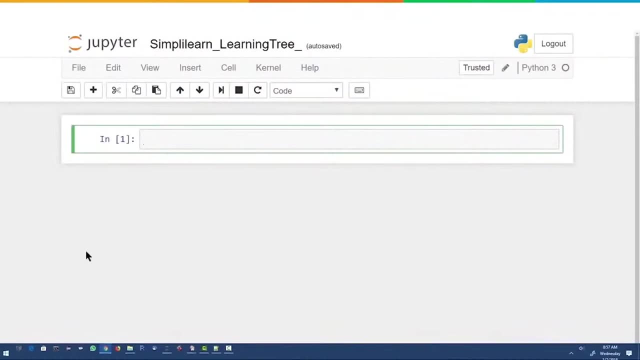 Any of those will work just fine to go ahead and explore this Python coding. So here we go. Let's go ahead and flip over to our Jupyter Notebook, And I've already opened up a new page for Python 3 code and I'm just going to paste this right in there. 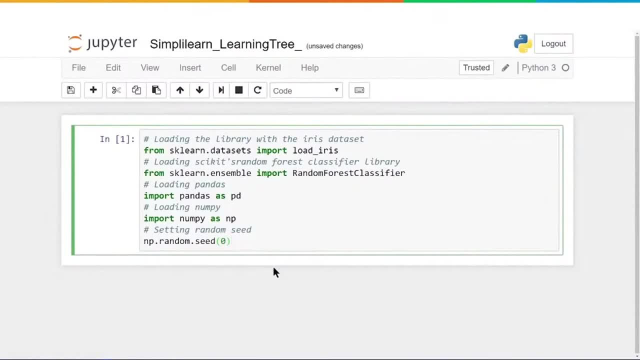 And let's take a look and see what we're bringing into our Python. The first thing we're going to do is, from the sklearndatasets, import load iris. Now, this isn't the actual data. This is just the module that allows us to bring in the data, the load iris. 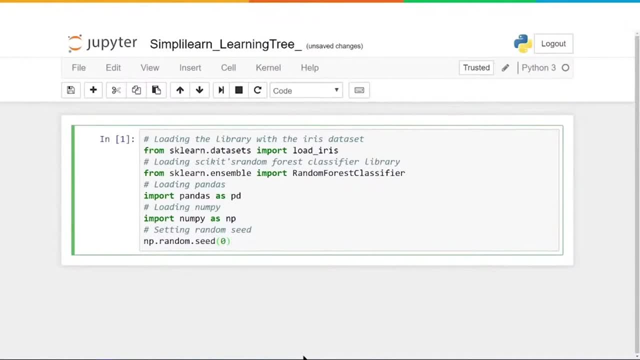 And the iris is so popular- it's been around since 1936 when Ronald Fisher published a paper on it- and they're measuring the different parts of the flower And, based on those measurements, predicting what kind of flower it is. and then, if we're going to do a random forest classifier, 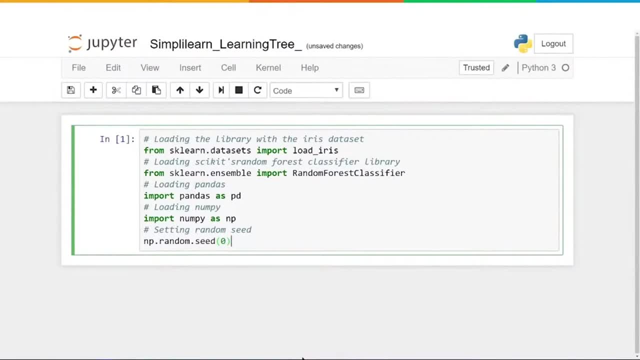 we need to go ahead and import a random forest classifier from the sklearn module, So sklearnensemble- import random forest classifier. And then we want to bring in two more modules And these are probably the most commonly used modules in Python and data science. with any of the other modules that we bring in. 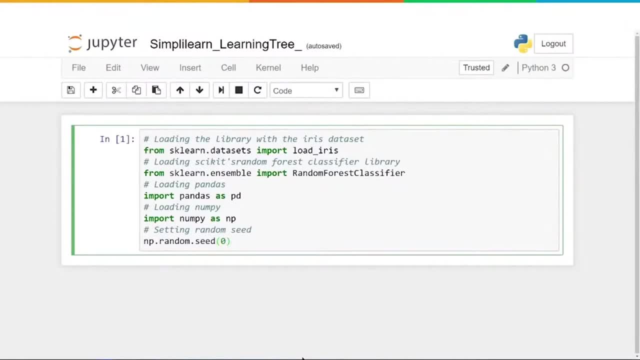 And one is going to be pandas. We're going to import pandas as pd. pd is a common term used for pandas And pandas is basically creates a data format for us where, when you create a pandas data frame, it looks like an Excel spreadsheet and you'll see that in a minute when we start. 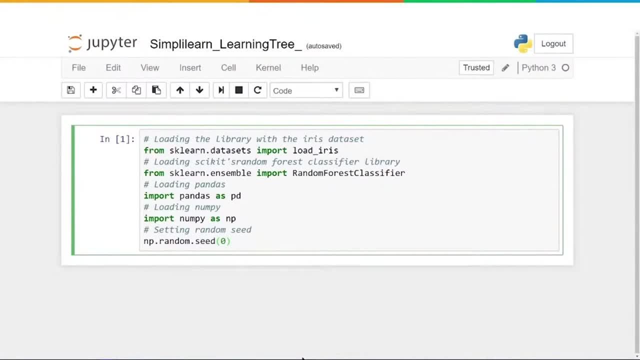 digging deeper into the code. pandas is just wonderful because it plays nice with all the other modules in there. And then we have numpy, which is our numbers Python, And the numbers Python allows us to do different mathematical sets on here. We'll see right off the bat. 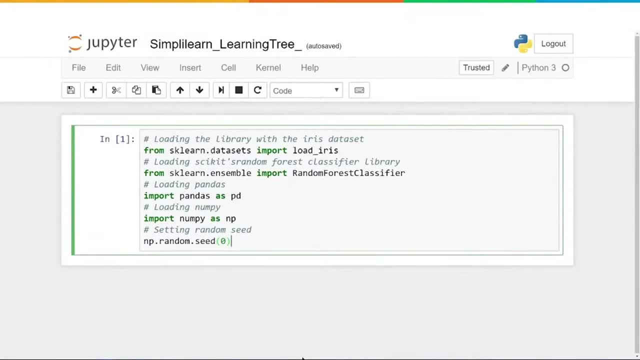 We're going to take our NP and we're going to go ahead and seed the randomness with it, with zero. So NPrandomseed is seeding that is zero. This code doesn't actually show anything. We're going to go ahead and run it because I need to make sure I have all those loaded. 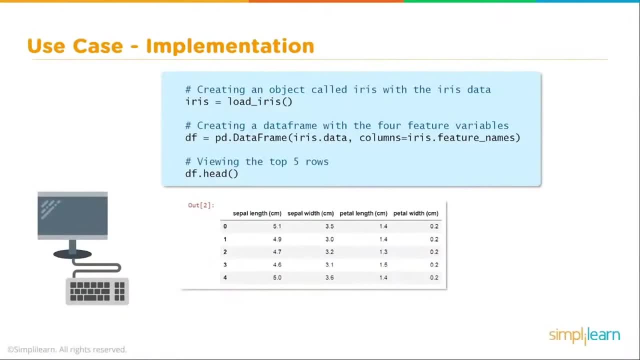 And then let's take a look at the next module on here. The next six slides, including this one, are all about exploring the data. Remember, I told you half of this is about looking at the data and getting it all set. So let's go ahead and take this code right here: the script. 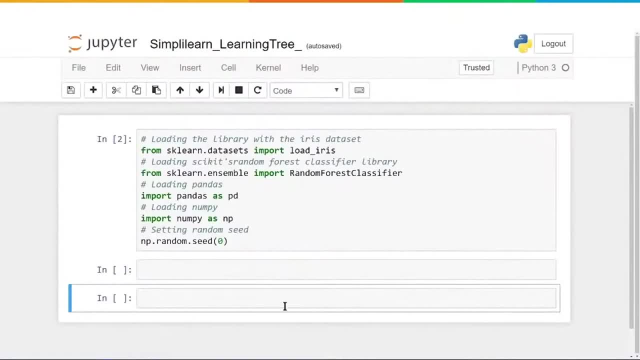 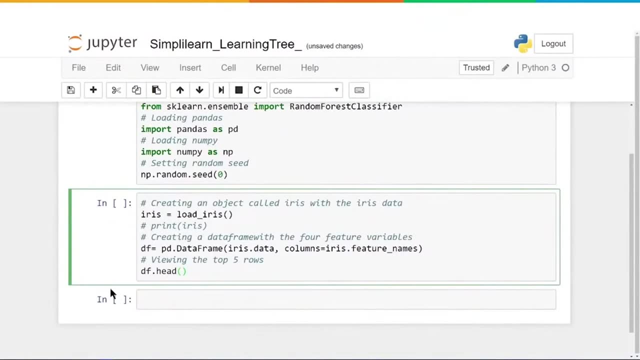 And let's get that over into our Jupyter notebook. And here we go. We've gone ahead and run the imports and I'm going to paste the code down here And let's take a look and see what's going on. The first thing we're doing is we're actually loading the iris data. 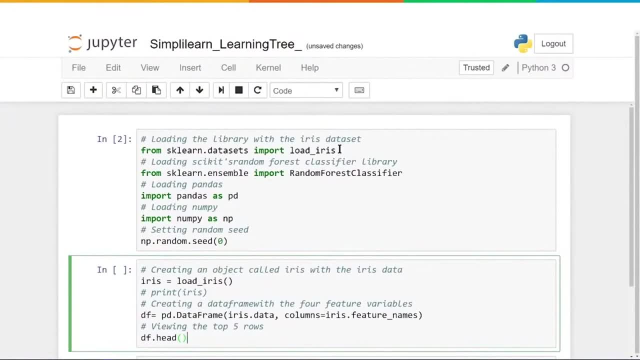 And, if you remember, up here we loaded the module that tells it how to get the iris data. Now we're actually assigning that data to the variable iris And then we're going to go ahead and use the DF to define data frame And that's going to equal PD. 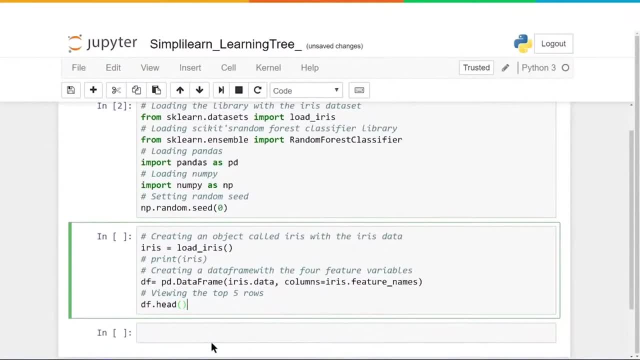 And, if you remember, that's pandas as PD, So that's our pandas And panda data. And then we're looking at iris data and columns equals iris feature names, And we're going to do the DF head and let's run this. 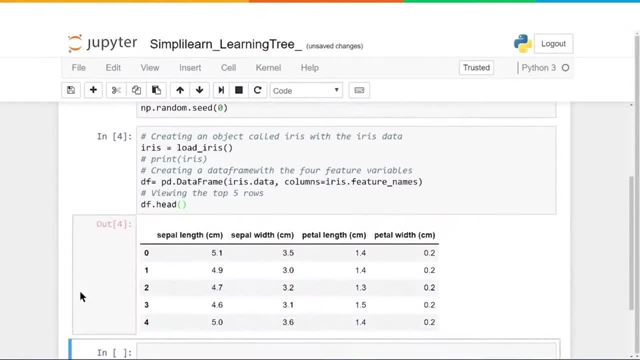 You can understand what's going on here. The first thing you want to notice is that our DF has created what looks like an Excel spreadsheet And in this Excel spreadsheet we have set the columns, So up on the top you can see the four different columns. 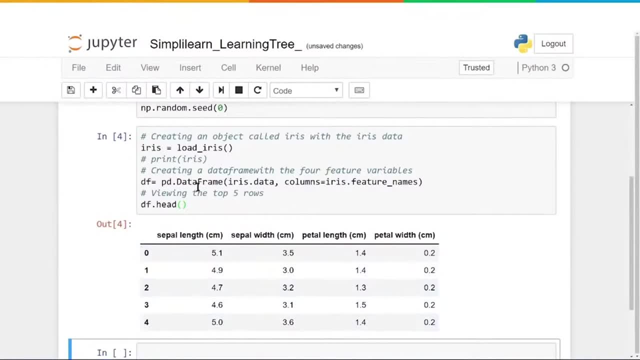 And then we have the data- iris data- down below. It's a little confusing without knowing where this data is coming from. So let's look at the bigger picture and I'm going to go print. I'm just going to change this for a moment. 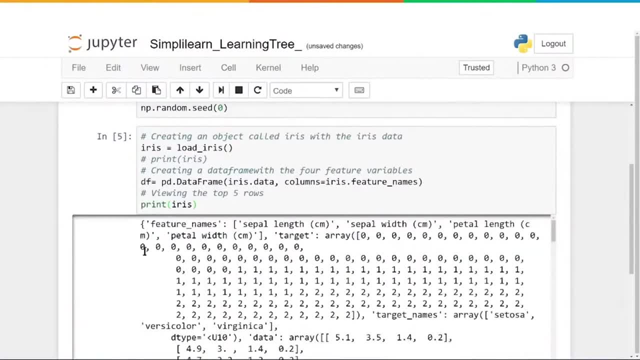 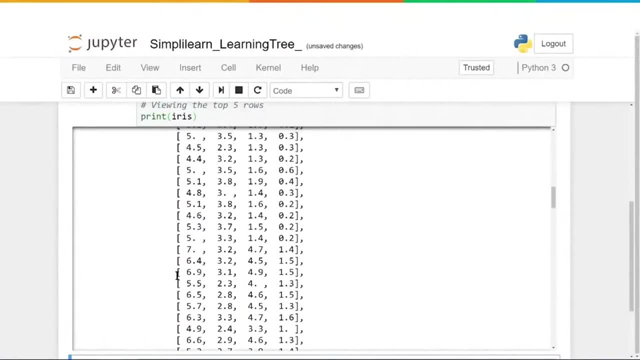 And we're going to print all of iris and see what that looks like. So when I print all of iris, I get this long list of information And you can scroll through here and see all the different titles on there. What's important to notice is that, first off, there's a brackets at the beginning. 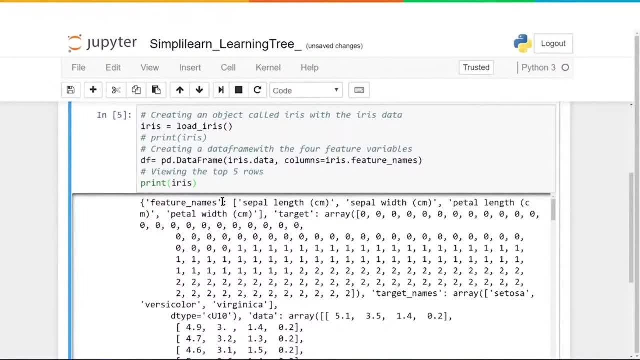 So this is a Python dictionary, And in a Python dictionary you'll have a, a key or a label, and this label pulls up whatever information comes after it. So feature names which we actually used over here under columns- is equal to an array of sepal length, sepal width, petal length, petal width. 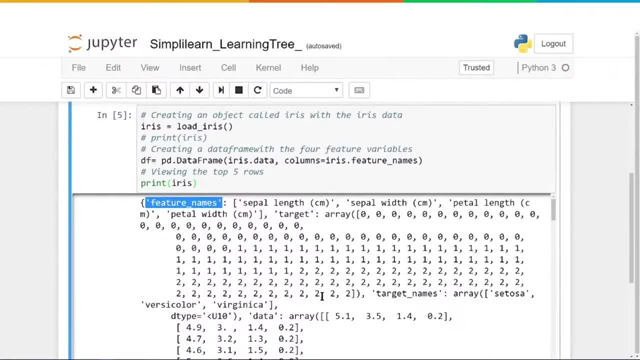 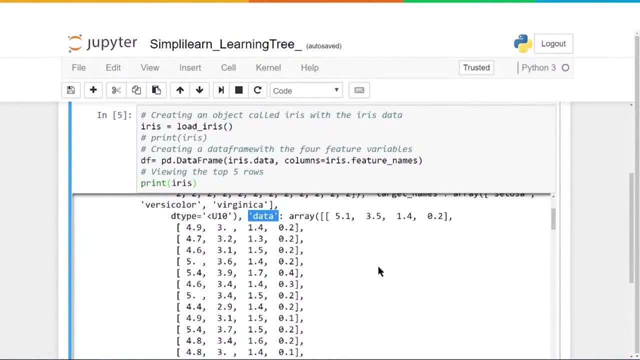 These are the different names they have for the four different columns And if you scroll down far enough, you'll also see data down here. Oh goodness, it came up right towards the top And data is equal to the different data we are looking at. 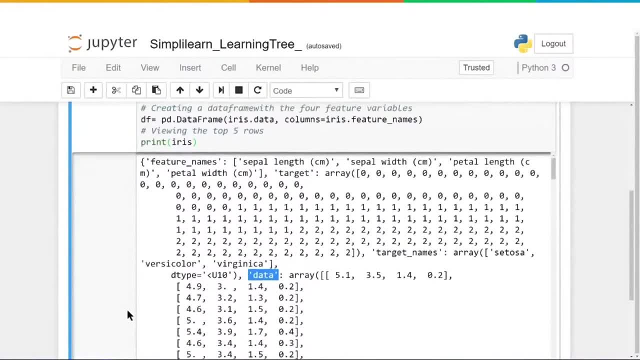 Now there's a lot of other things in here, like target- we're going to be pulling that up in a minute- And there's also the names, the target names, which is further down, And we'll show you that also in a minute. 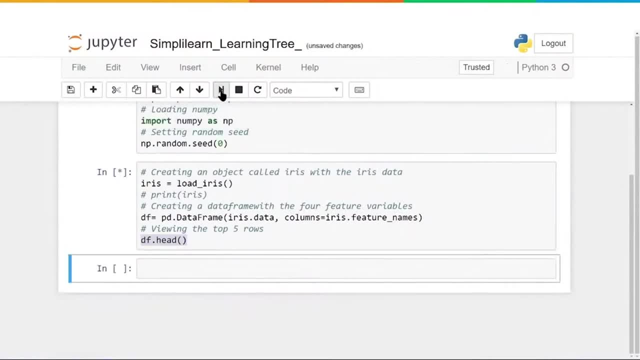 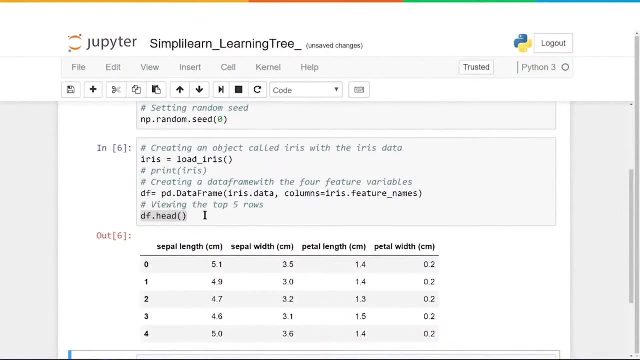 Let's go and set that back To the head. And this is one of the neat features of pandas and panda data frames is, when you do DF dot head or the panda data frame dot head, it'll print the first five lines of the data set in there, along with the headers. 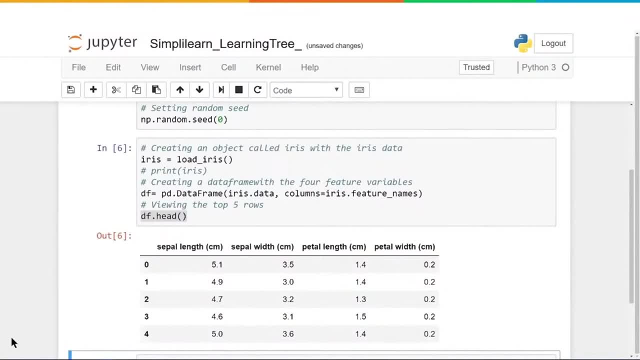 If you have it. in this case we have the column header set to iris, And then you can look at the other one to see how it works with the first features, And in here you'll see that we have 0, 1, 2, 3, 4.. 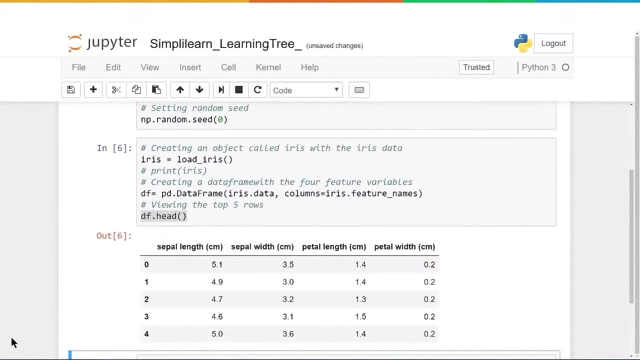 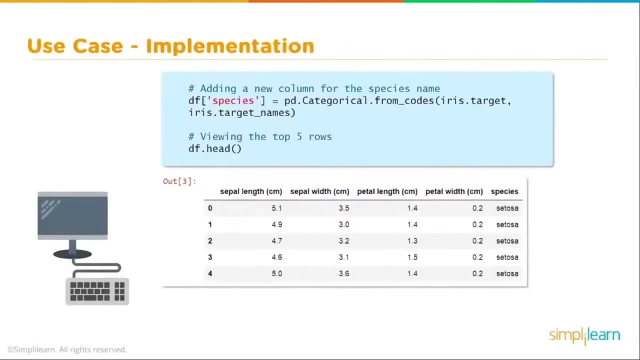 In Python, most arrays always start at zero. So when you look at the first five, it's going to be 0, 1, 2, 3, 4, not 1, 2, 3, 4, 5.. So now we've got our iris data imported into a data frame. 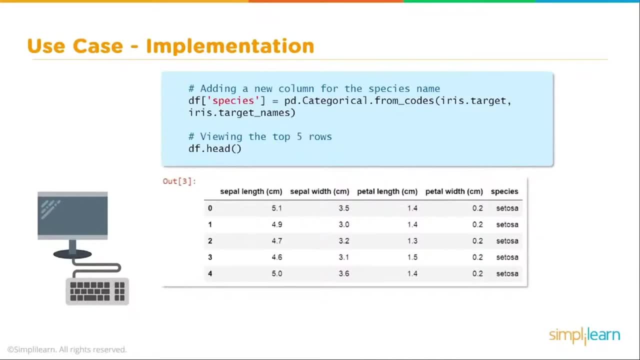 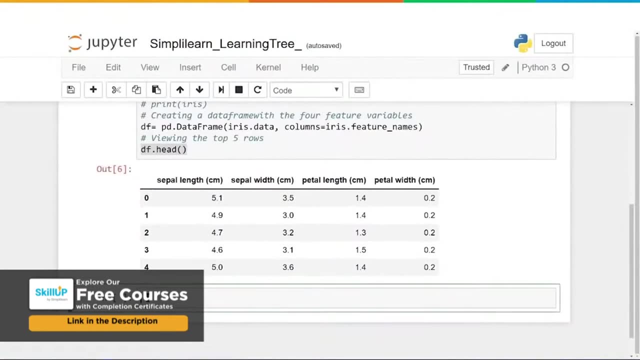 Let's take a look at the next piece of code in here, And so in this section here of the code, we're going to take a look at the target little bit more in detail. So here we are. in our Jupyter notebook, I'm going to put: 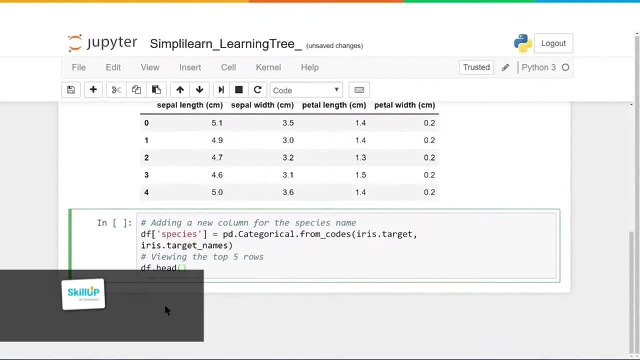 the code in here and before I run it, I want to look at a couple things going on. So we have DF species- and this is interesting because right here you'll see where I have DF species in brackets, which is the key code for creating another column- and here we have iris dot target. Now these are both in the pandas. 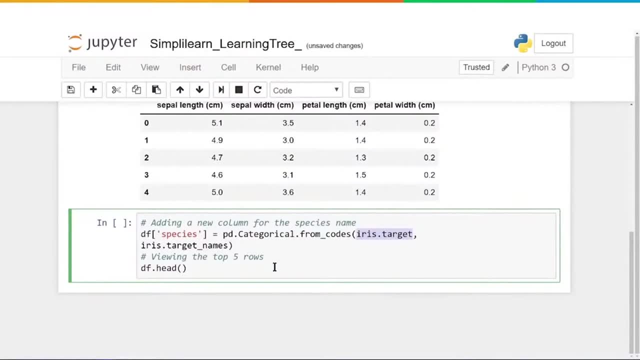 setup on here. So in pandas we can do either one. I could have just as easily done iris and then in brackets, target, depending on what I'm working on. Both are acceptable. Let's go ahead and run this code and see how this changes and 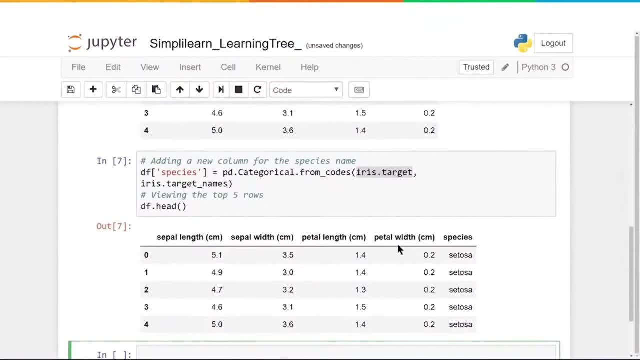 what we've done is we've added the target from the iris data set as another column on the end. Now, what species is? this is what we're trying to predict. So we have our data, which tells us the answer for all these different pieces, and then we've added a column with the answer. that way, when we do our final, 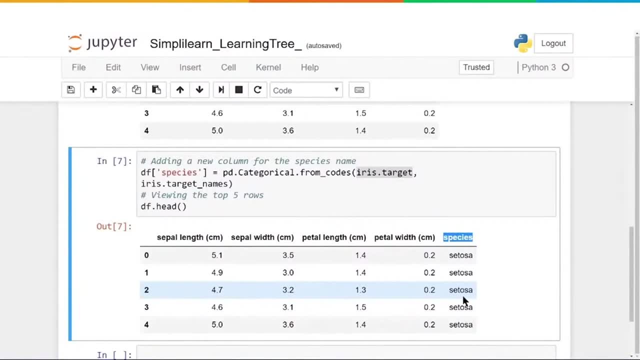 setup, we'll have the ability to program our neural network to look for these, this different data, and know what a setosa is, or a vericolor, which we'll see in just a minute, or virginica. Those are the three that are in there. And now? 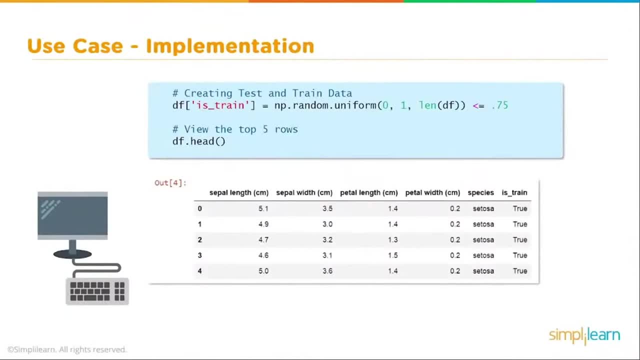 we're going to add one more column. I know we're organizing all this data over and over again. it's kind of fun. There's a lot of ways to organize it. What's nice about putting everything on to one data frame is that you can see what data you're organizing and what data you're. 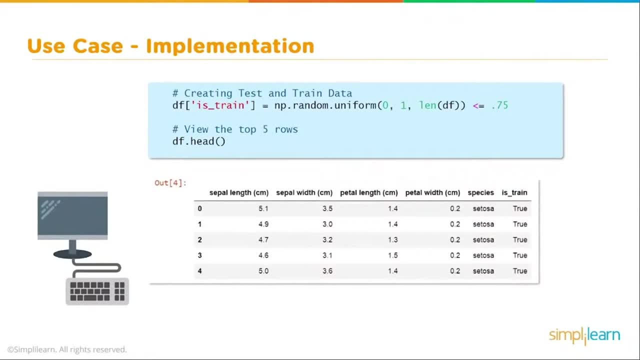 using. So if I want to do this, I can then do a printout and it shows me exactly what I'm looking at And I'll show you that where you, where that's different, where you can alter that and do it slightly differently. But let's go. 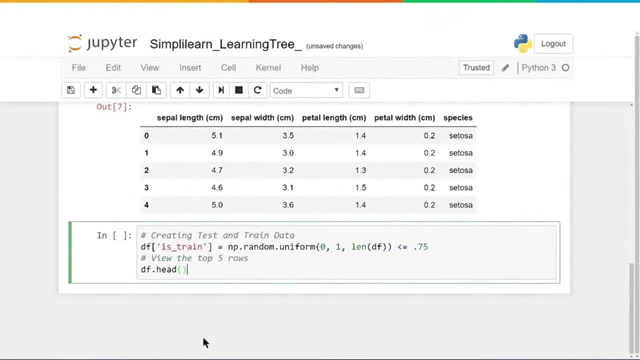 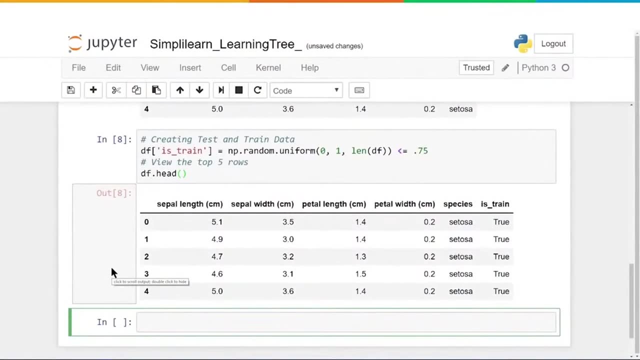 ahead and put this into our script up to that now. And here we go, we're gonna put that down here and we're gonna run that, and let's talk a little bit about what we're doing Now. we're exploring data and one of the challenges is knowing how. 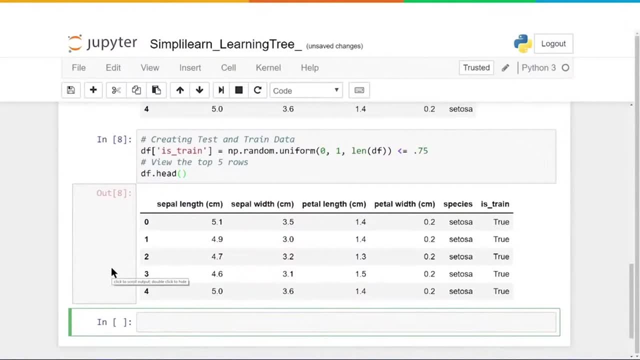 good your model is. Did your model work? And to that we need to know that you're using the right model. So let's go ahead and put this into our script And if we go into our project library and we're going to put in the data And we split it into two different parts- They usually call it. 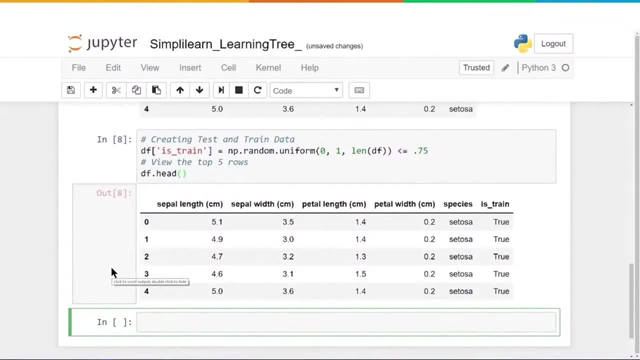 the training and the testing, And so in here we're gonna go ahead and put that in our database so you can see it clearly, And we've set it DF. Remember you can put brackets. This is creating another column Is trained, so we're going. 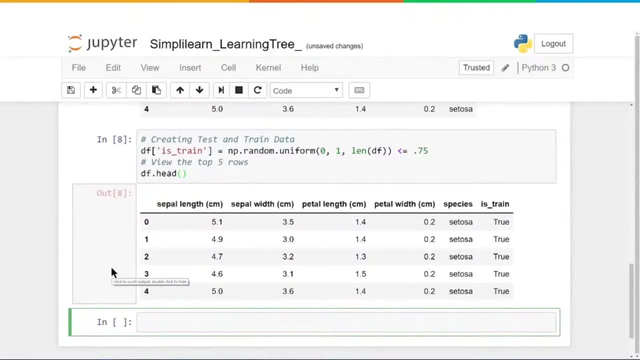 to use part of it for training, And this equals NP. Remember that stands for numpyrandomuniform. So we're generating a random number between zero and one, and we're going to do it for each of the rows. That's where the length DF equals. 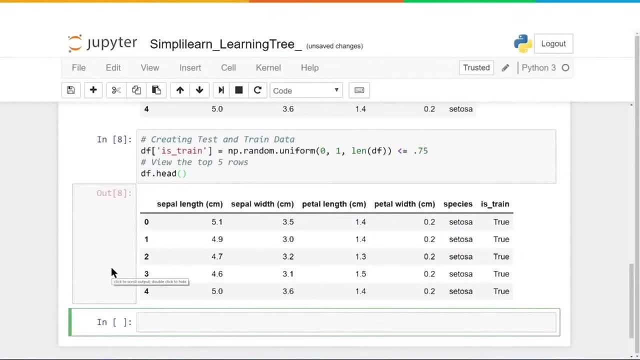 comes from. So each row gets a generated number, and if it's less than 0.75 it's true, and if it's greater than 0.75 it's false. This means we're going to take 75% of the data roughly, because 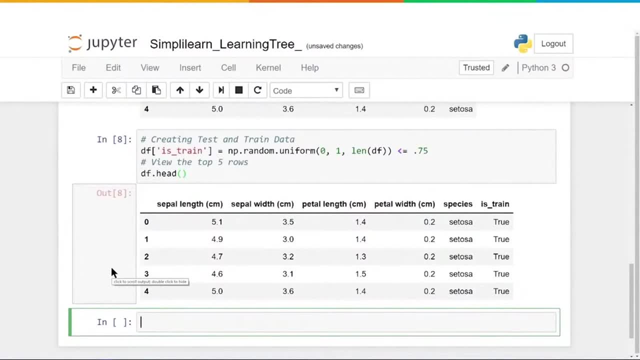 there's a randomness involved and we're going to use that to train it, and then the other 25% we're going to hold off to the side and use that to test it later on. So let's flip back out over and see what the next step is. So, now that we've labeled our database for which is training, and 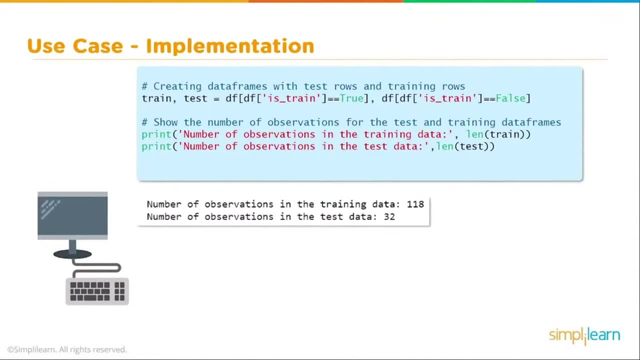 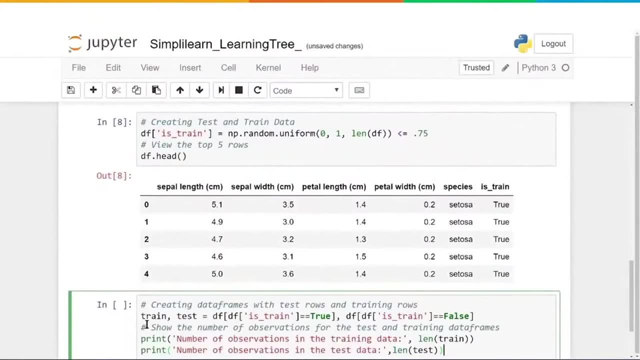 which is testing. let's go ahead and sort that into two different variables- train and test, and let's take this code and let's bring it into our project. Here we go, let's paste it on down here, and before I run this, let's just take a quick look at what's going on. here We have up. 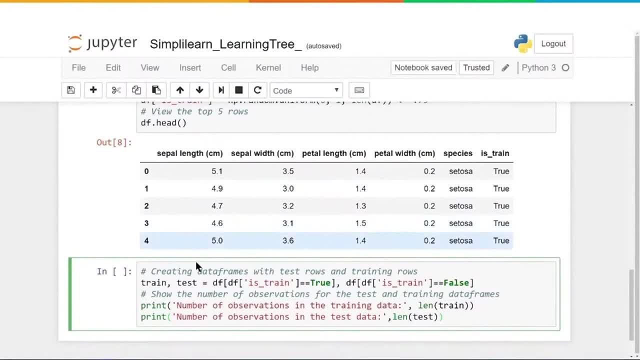 above. we created- remember, there's our defhead which prints the first five rows, and we've added a column: is train at the end. So we're going to take that. we're going to create two variables, we're going to create two new data frames. One's called train. 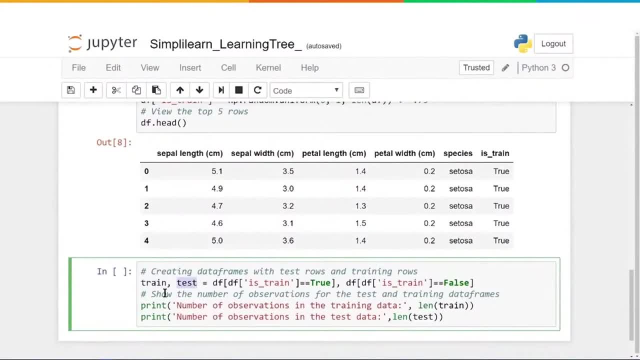 one's called test, 75% in train, 25% in test. and then to sort that out, we're going to do that by doing df, our main original data frame, with the iris data in it. and if df is train equals true. 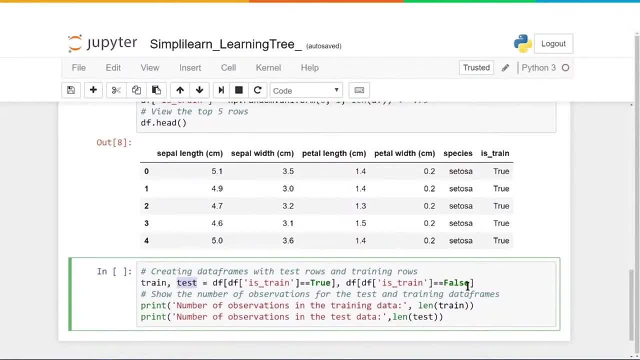 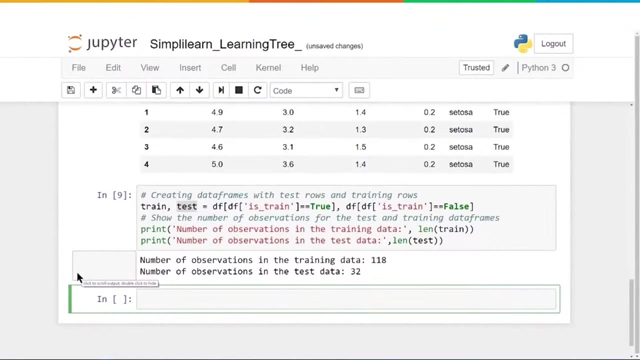 that's going to go in the train, and if df is train equals false, it goes in the test, and so when I run this, we're going to print out the number in each one. Let's see what that looks like. and it puts 118 in the training module and it puts 32 in the testing module, which lets us know that. 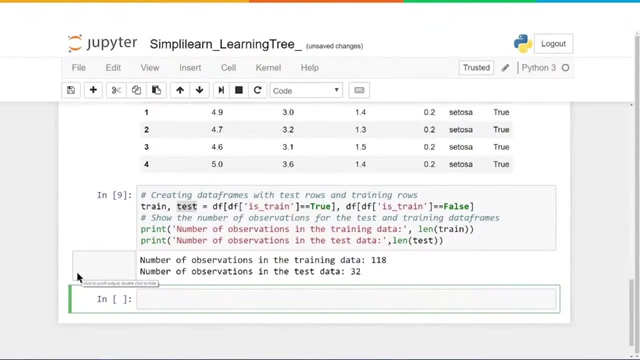 there was 150 lines of data in here. so if you went and looked at the original data, you could see that there's 150 lines and that's roughly 75% in one and 25% for us to test our model on afterward. So let's jump back to our code and see where this goes. In the next two steps we want to 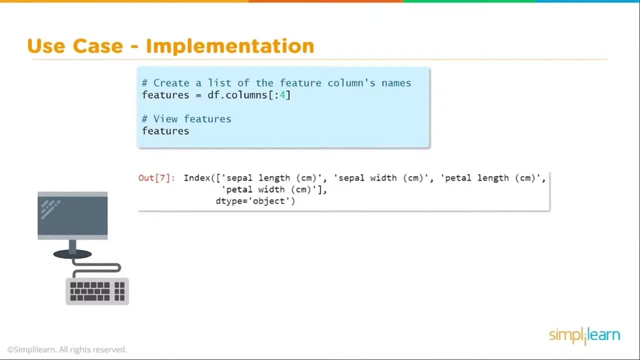 do one more thing with our data and that's make it readable to humans. I don't know about you, but we're going to do one more thing with our data and that's make it readable to humans. So let's go ahead and take those and make those readable to humans and let's put that in our code. 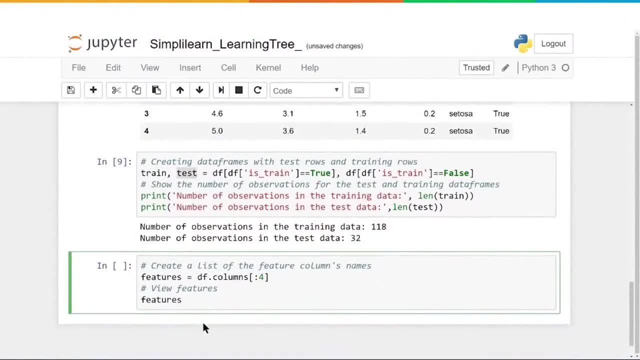 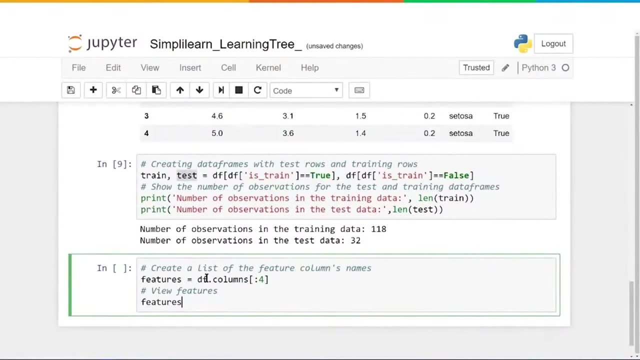 Let's see, here we go, paste it in and you'll see, here we've done a couple very basic things. We know that the columns in our data frame- again this is a panda thing- the df columns, and we know the first four of them: zero one, two, three, that'd be the first four. 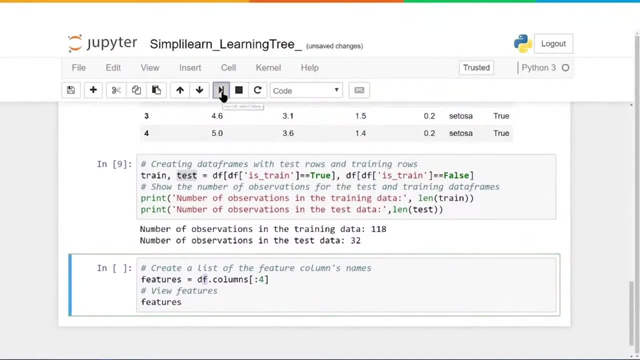 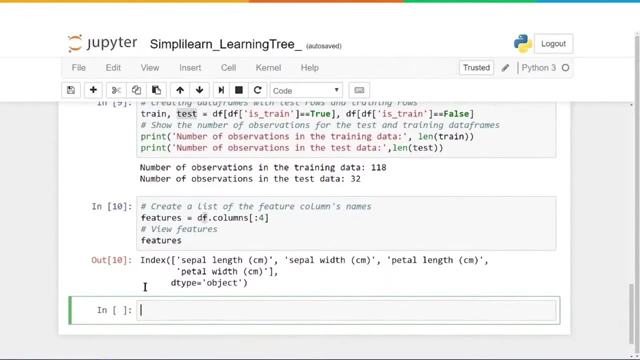 are going to be the features or the titles of those columns, And so when I run this, you'll see down here that it creates an index: sepa length, sepa width, petal length and petal width. And this should be familiar because if you look up here, here's our column titles going. 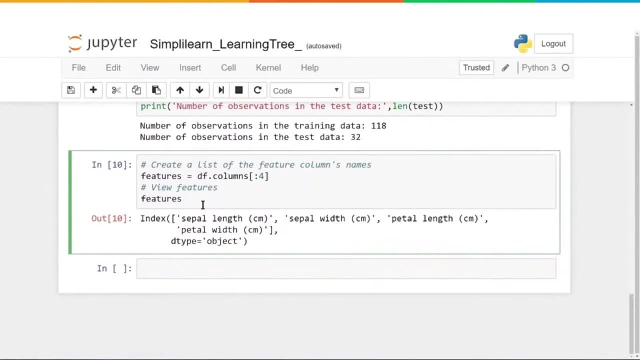 across, and here's the first four. One thing I want you to notice here is that when you're in a command line- whether it's Jupyter Notebook or you're running command line in the terminal window- if you just put the name of it it'll print it out. This is the same as 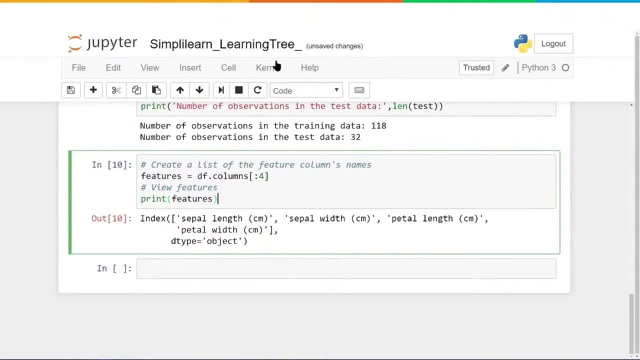 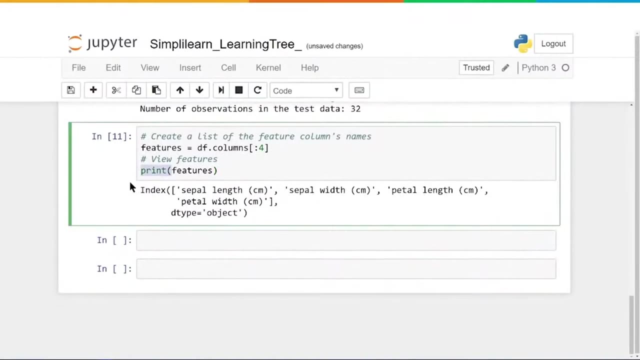 doing print features And the shorthand is you just put features in here. If you're actually writing a code and saving the script and running it by remote, you really need to put the print in there. But for this. when I run it, you'll see it gives me the same thing, But for this. 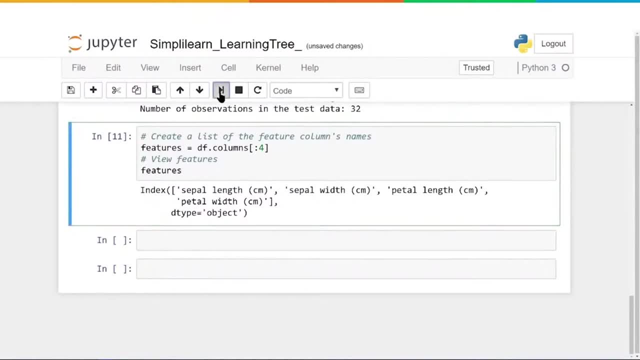 we want to go ahead and we'll just leave it as features because it doesn't really matter, And this is one of the fun things about Jupyter Notebooks is I'm just building the code as we go, And then we need to go ahead and create the labels for the other parts. 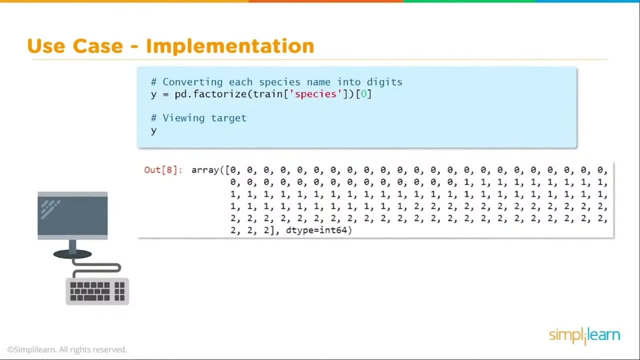 So let's take a look and see what that looks like For our final step in prepping our data before we actually start running the training and the testing is we're going to go ahead and convert the species on here into something the computer understands. So let's put this code: 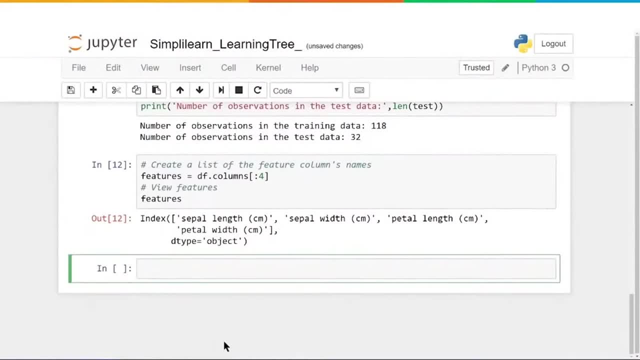 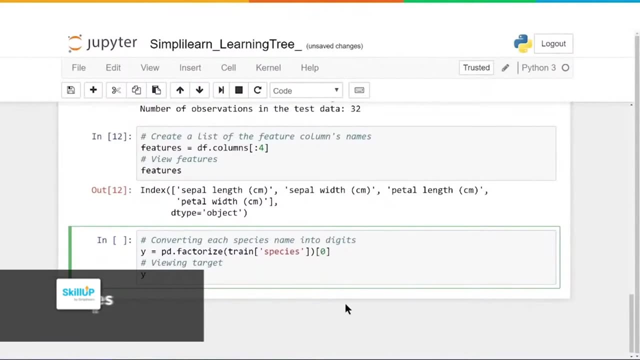 into our script and see where that takes us All. right, here we go. We've set y equal to pdfactorize- train species of zero. So let's break this down just a little bit. We have pandas right here. pd factorize- What is factorize doing? I'm going to come back to that. 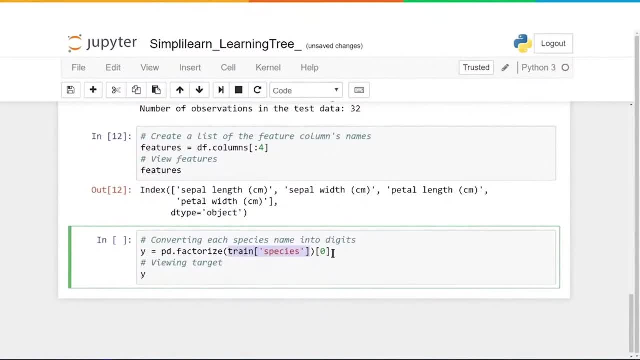 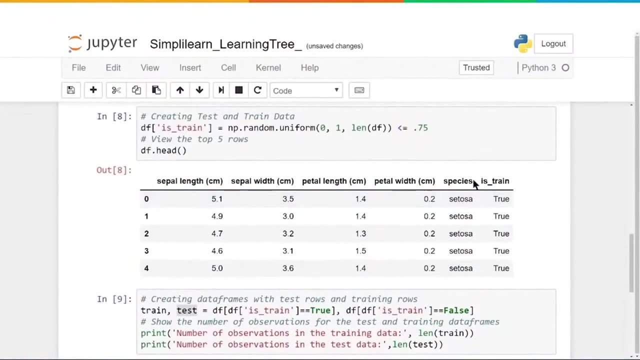 in just a second. Let's look at what train species is and why. we're looking at the group zero on there And let's go up here And here is our species. Remember this: We created this whole column here for species And then it has setosa, setosa, setosa, setosa, And if you scroll down, 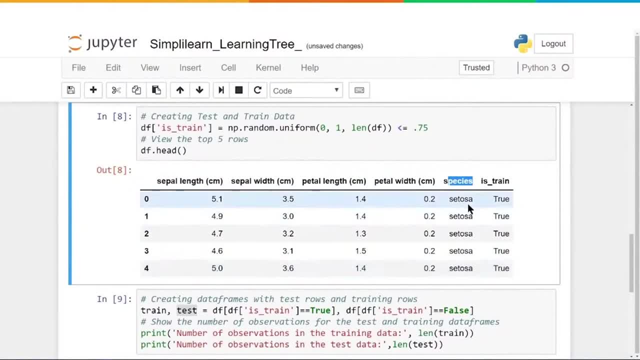 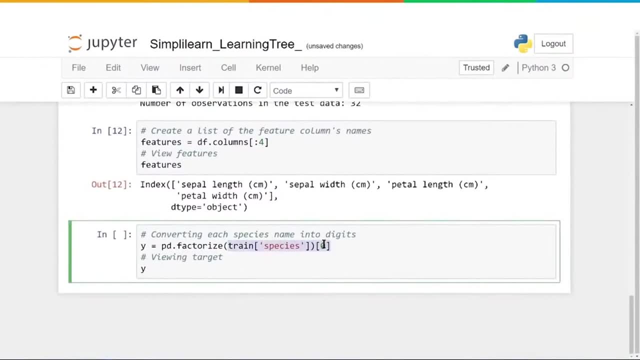 enough. you'd also see virginica and vericolor. And then we need to convert that into something. the computer understands zeros and ones, So the train species of zero, because this is in the format of an array, of arrays, so you have to have the zero on the end And then species is just that: column Factorize. 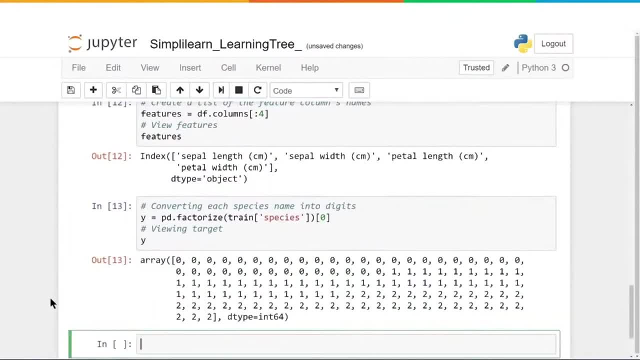 goes in there and looks at the fact that there's only three of them. So when I run this, you'll see that y generates an array that's equal to- in this case it's the training set, and it's zeros, ones and twos represented by pdfactorize. So we're going to go ahead and 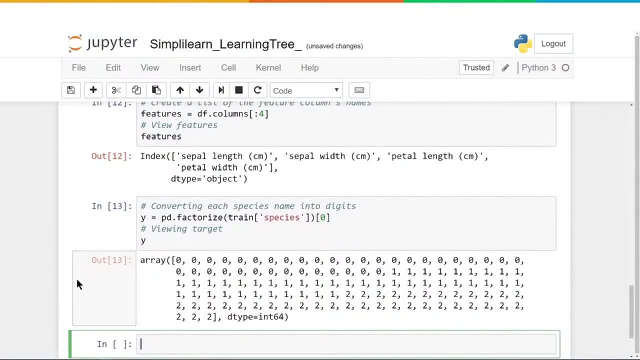 add in the three different kinds of flowers we have. So now we have something the computer understands, and we have a nice table that we can read and understand, And now, finally, we get to actually start doing the predicting. So here we go, We have 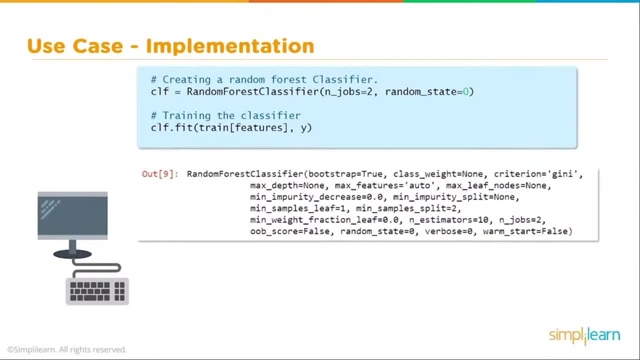 two lines of code. Oh my goodness, that was a lot of work to get the two lines of code, But there is a lot in these two lines of code, So let's take a look and see what's going on here and put this into our full script that we're running. Let's paste this in here. 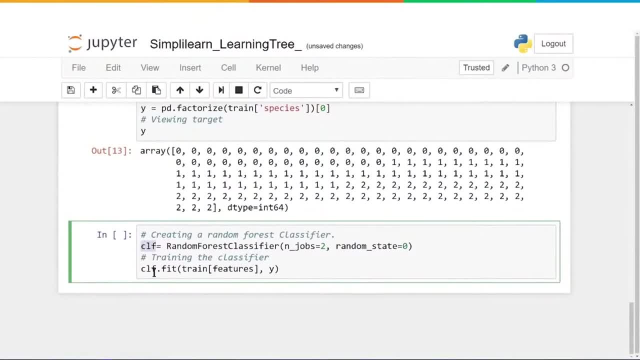 Let's take a look and see what this is. We're creating a variable f and we're going to set this equal to the random forest classifier. We're passing two variables in here and there's a lot of variables you can play with. 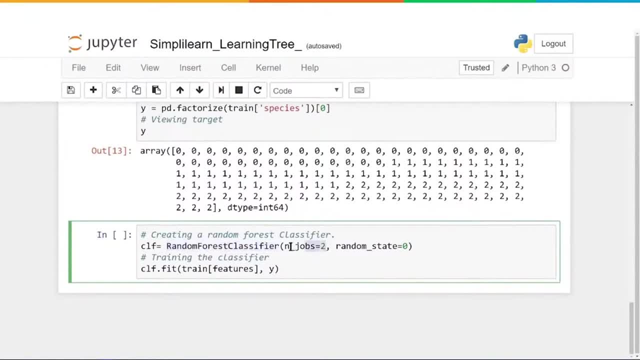 As far as these two are concerned, they're very standard In jobs. all that does is to prioritize it, Not something to really worry about. Usually, when you're doing this on your own computer, you do in jobs equals two. If you're working in a larger or big data and you need to prioritize it differently, this is what that number does. 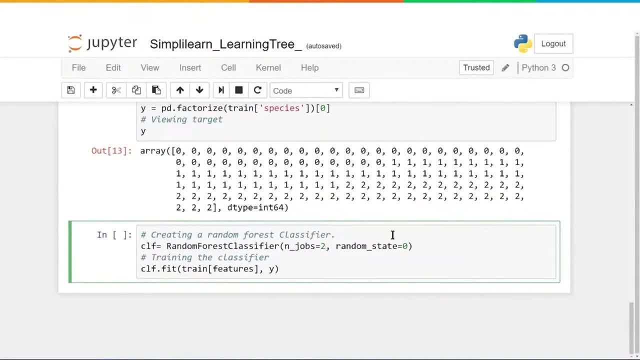 It changes your priorities and how it's going to run across the system and things like that. Then the random state is just how it starts. Zero is fine for here, but let's go ahead and run this. We also have clffit train features y. 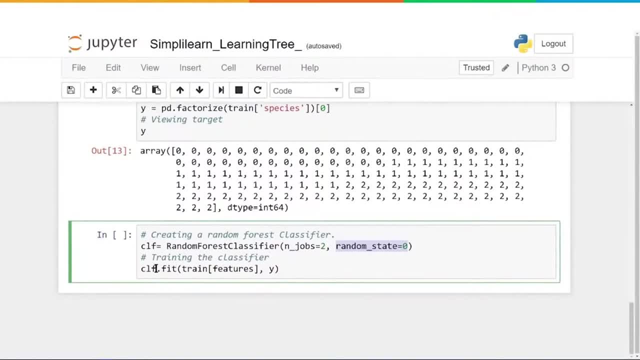 Before we run it, let's talk about this a little bit more clffit. We're fitting, We're training it. We are actually creating our random forest classifier right here. This is the code that does everything. We're going to take our training set. Remember, we kept our test off to the side. 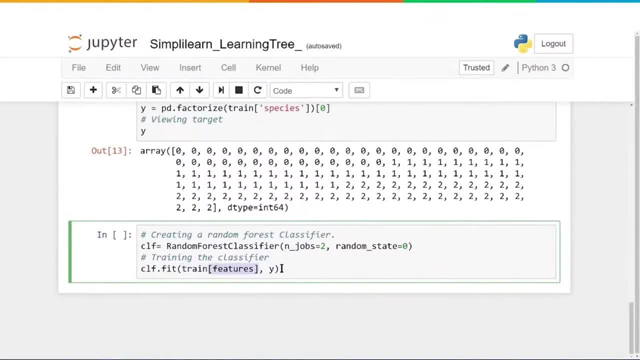 We're going to take our training set with the features and then we're going to go ahead and put that in. Here's our target. the y, The y is 0,, 1, and 2 that we just created. The features is the actual data going in that we put into the training set. 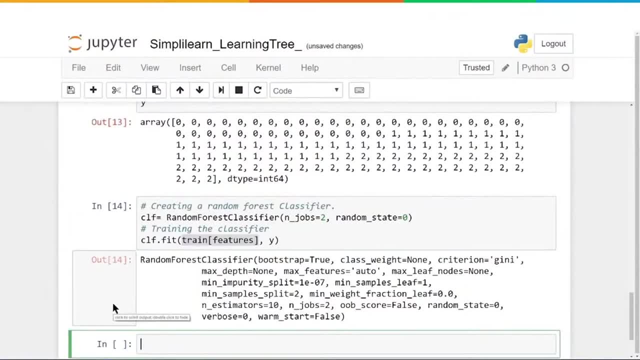 Let's go ahead and run that. This is kind of an interesting thing because it printed out the random forest classifier And everything around it. When you're running this in your terminal window or in a script like this, this automatically treats this, just like when we were up here. 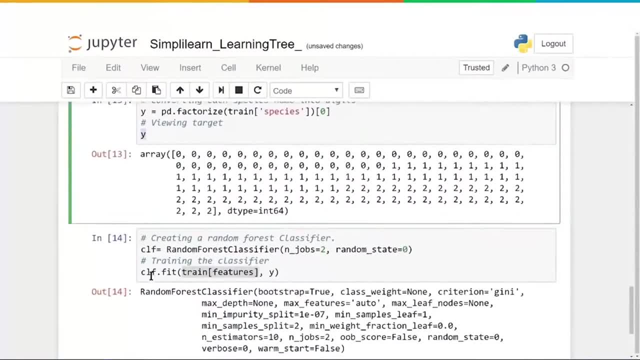 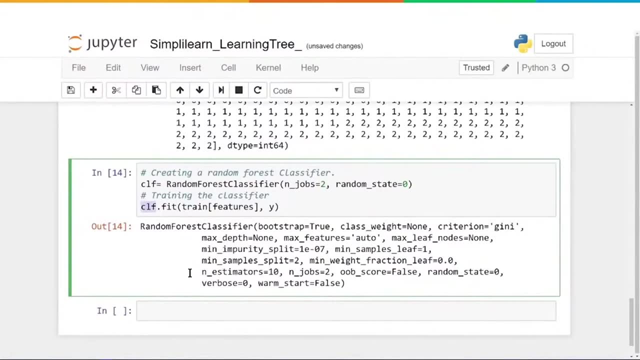 and I typed in y and it printed out y instead of print y. This does the same thing. It treats this as a variable and prints it out. But if you were actually running your code, that wouldn't be the case. What it's printed out is: it shows us all the different variables we can change. 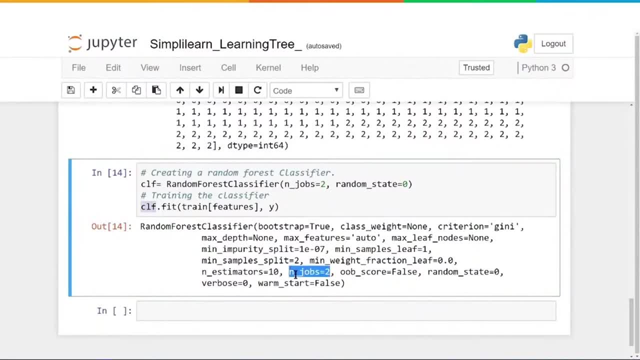 If we go down here you can actually see it. You can see in: jobs equals 2.. You can see the random state equals 0. Those are the two that we sent in there. You would really have to dig deep to find out all these different meanings of all these different settings on here. 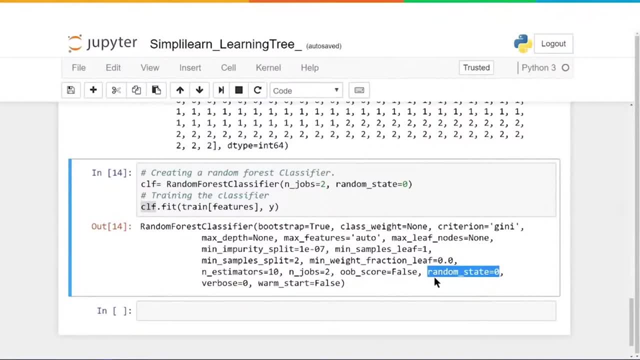 Some of them are self-explanatory, if you kind of think about it. a little bit like max features is auto, So all the features that we're putting in there is just going to automatically take all four of them. Whatever we send it, it'll take. 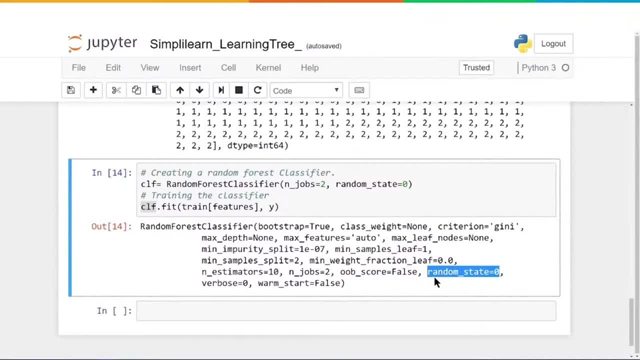 Some of them might have so many features because you're processing words. there might be like 1.4 million features in there because you're doing legal data And that's how many different words are in there. At that point, you probably want to limit the maximum features that you're going to process. 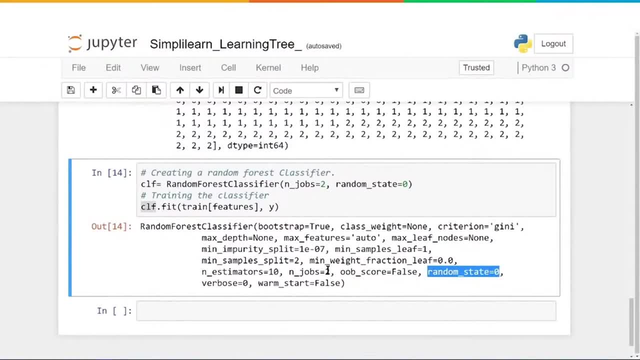 And leaf nodes. that's the end nodes. Remember we had the fruit and we're talking about the leaf nodes. Like I said, there's a lot in this. We're looking at a lot of stuff here, So you might have in this case there's probably only, I think, three leaf nodes, maybe four. 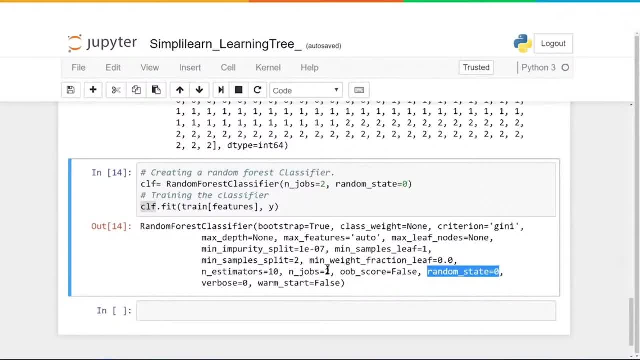 You might have thousands of leaf nodes, at which point you do need to put a cap on that and say, okay, you can only go so far, and then we're going to use all of our resources on processing this, And that really is what most of these are about. 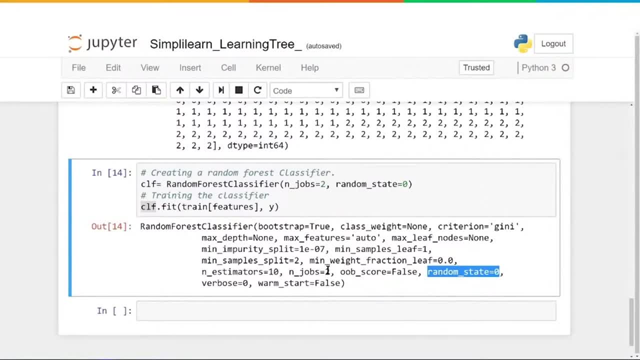 is limiting the process and making sure we don't overwhelm a system. And there's some other settings in here. Again, we're not going to go over all of them. Warm start equals false. Warm start is if you're programming it one piece at a time externally. 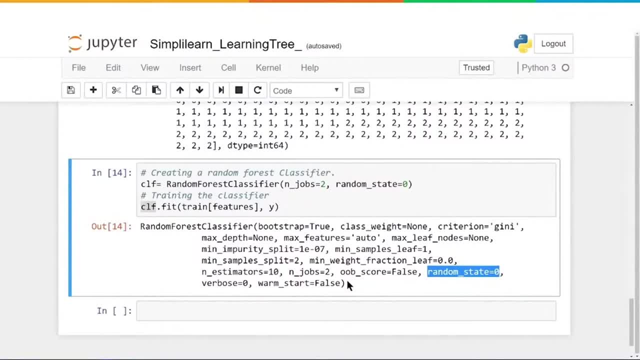 Since we're not. we're not going to continually detrain this particular learning tree And again, like I said, there's a lot of things in here that you'll want to look up more detail from the sklearn And if you're digging in deep and running a major project on here. 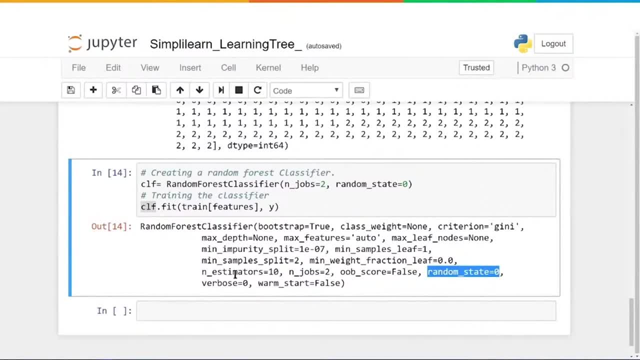 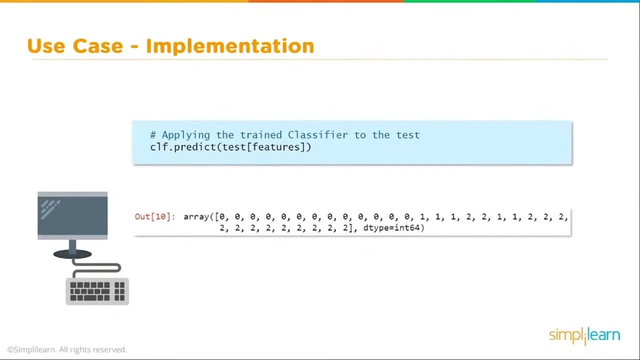 For today, though, all we need to do is fit or train our features and our target Y. So now we have our training model. What's next? If we're going to create a model, we now need to test it. Remember, we set aside the test feature, test group- 25% of the data. 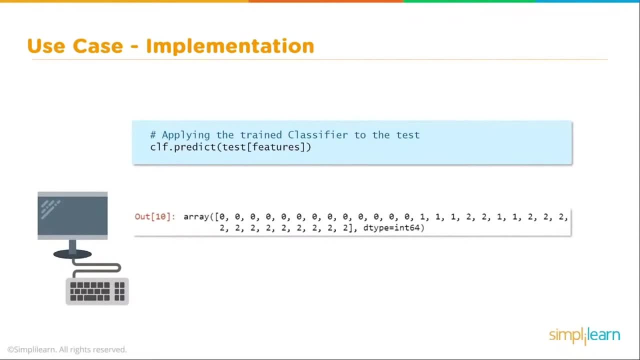 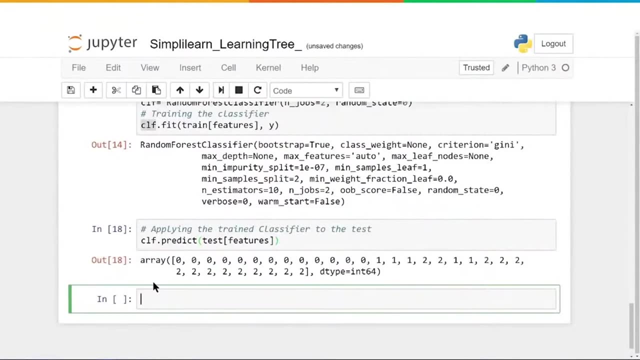 So let's go ahead and take this code and let's put it into our script and see what that looks like. Okay, here we go And we're going to run this And it's going to come out with a bunch of zeros, ones and twos. 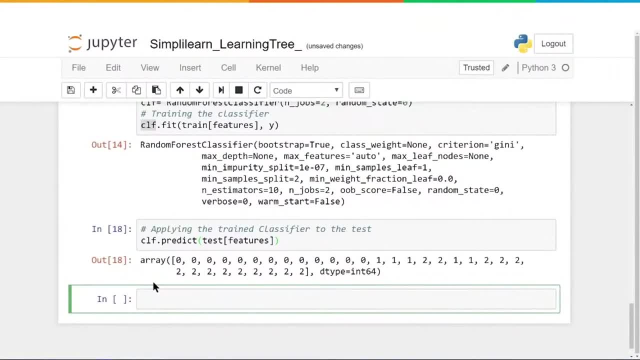 which represents the three type of flowers: the setosa, the virginica and the versicolor. And what we're putting into our predict is the test features, And I always kind of like to know what it is I am looking at. So, real quick, we're going to do test features. 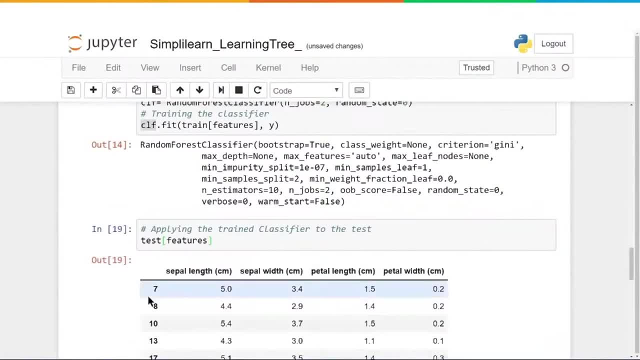 And remember, features is an array of sepal length, sepal width, petal length, petal width. So when we put it in this way, it actually loads all these different columns that we loaded into features. So if we did just features, 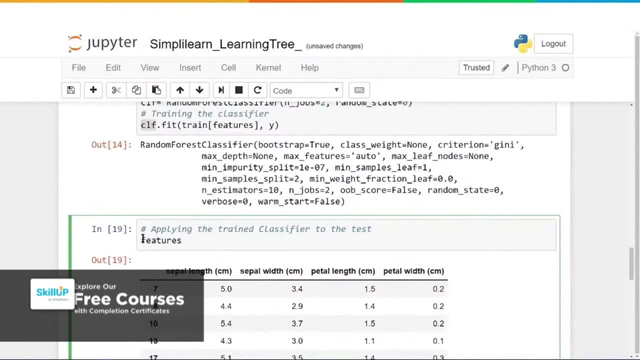 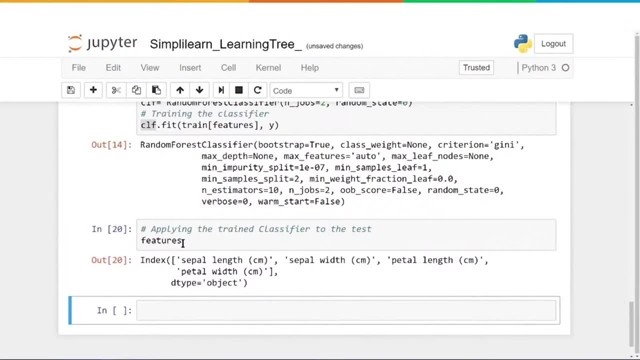 let me just do features in here, see what features looks like. This is just playing with Panda's data frames. You'll see that it's an index. So when you put an index in like this into test features, into test, it then takes those columns and creates a Panda data frames from those columns. 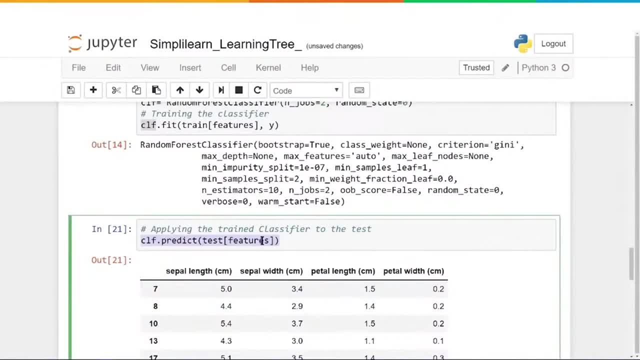 And in this case we're going to go ahead and put those into our predict. So we're going to put each one of these lines of data- the 5.0,, 3.4, 1.5, 0.2.. 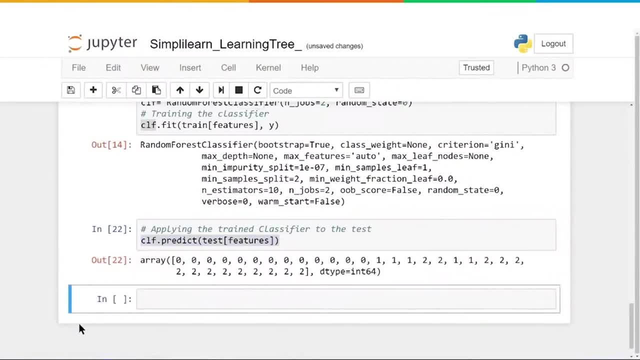 And we're going to put those in and we're going to predict what our new forest classifier is going to come up with. And this is what it predicts. It predicts 0, 0, 0, 1, 2, 1, 1, 2, 2, 2.. 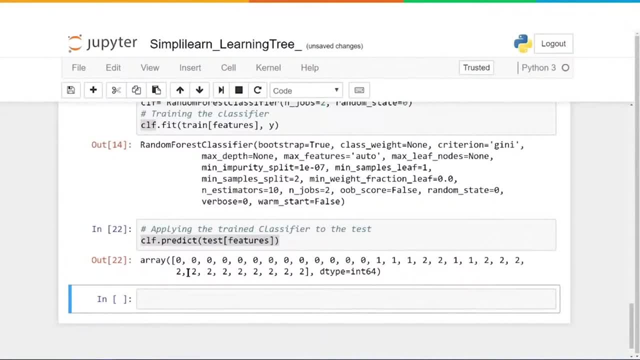 And again, this is the flower type: setosa, virginica and versicolor. So now that we've taken our test features, let's explore that, Let's see exactly what that data means to us. So the first thing we can do with our predicts: 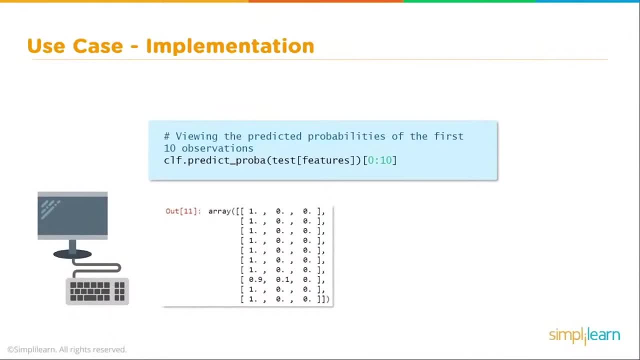 is, we can actually generate a different prediction model. When I say different, we're going to view it differently. It's not that the data itself is different. So let's take this next piece of code and put it into our script. So we're pasting it in here. 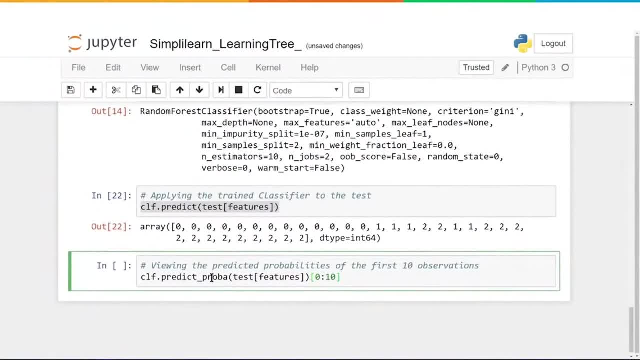 And you'll see that we're doing predict and we've added underscore proba for probability. So there's our CLF. This is our CLFpredict probability. So we're running it just like we ran it up here, But this time, with this, we're going to get a slightly different result. 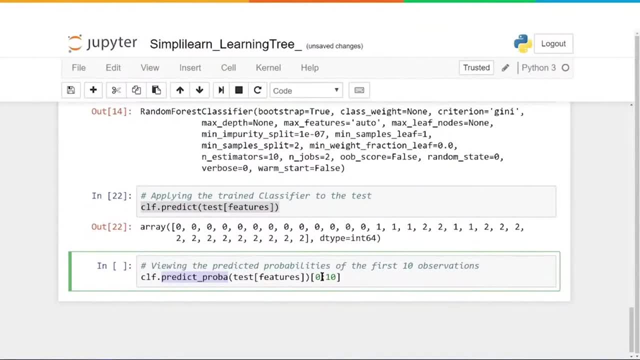 And we're only going to look at the first 10.. So you'll see down here, instead of looking at all of them, which was what? 27,? you'll see right down here that this generates a much larger field on the probability. 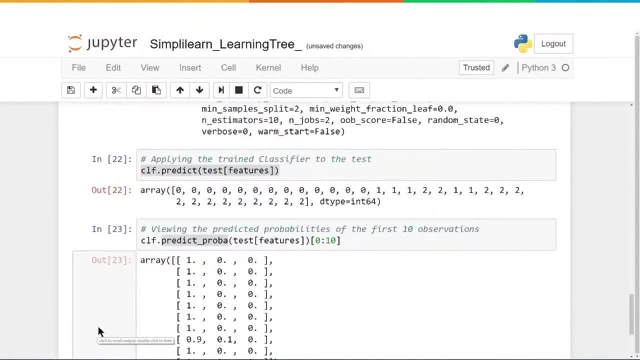 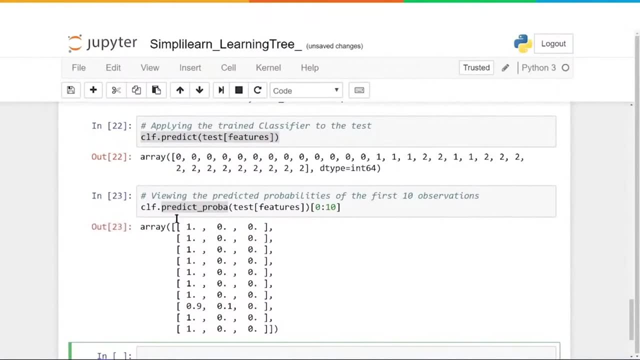 And let's take a look and see what that looks like and what that means. So when we do the predict underscore, proba for probability, it generates three numbers. So we had three leaf nodes at the end And if you remember from all the theory we did, 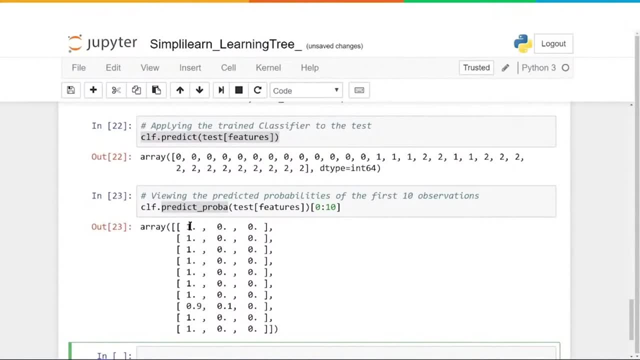 this is the predictors. The first one is predicting a 1 for setosa, It predicts a 0 for virginica, And it predicts a 0 for versicolor, And so on, and so on, and so on. And let's you know what? I'm going to change this just a little bit. 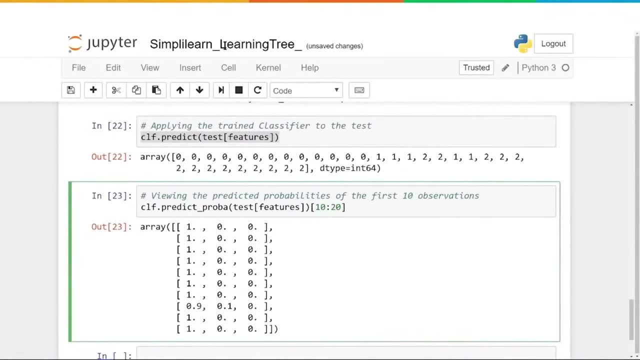 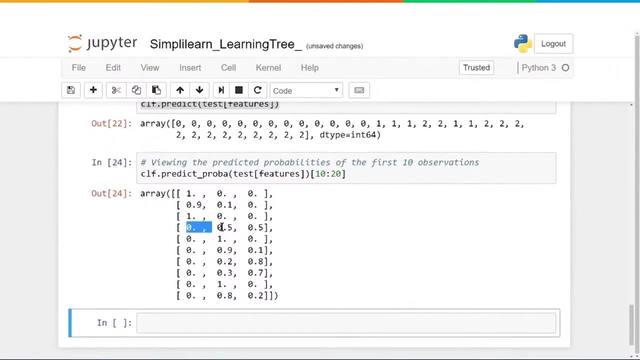 Let's look at 10 to 20, just because we can And we start to get a little different of data And you'll see right down here it gets to this one, this line right here, And this line has 0,, 0.5,, 0.5.. 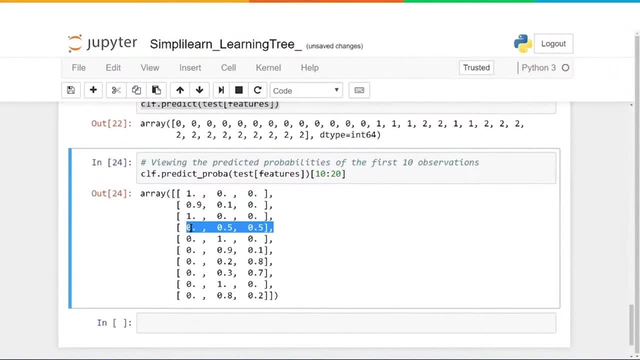 And so if we're going to vote and we have two equal votes, it's going to go with the first one. So it says setosa gets 0 votes, virginica gets 0.5 votes, versicolor gets 0.5 votes. 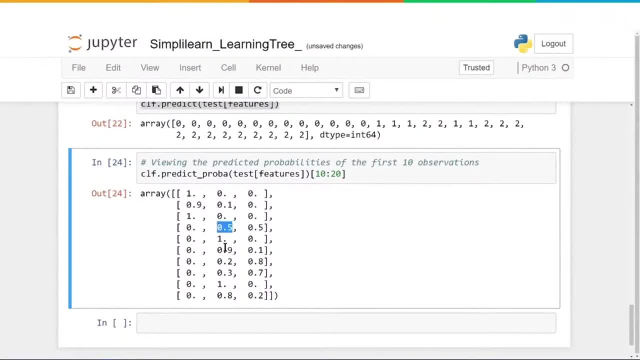 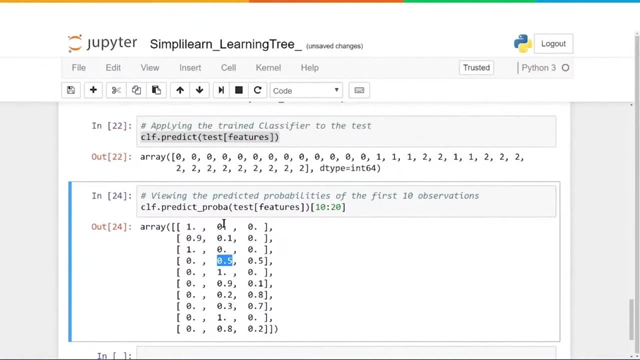 But let's just go with the virginica, since these two are equal, And so on and so on down the list. Let's see how they vary on here. So now we've looked at both. how to do a basic predict of the features. 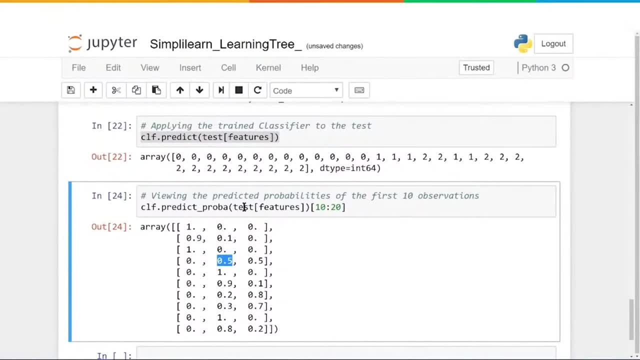 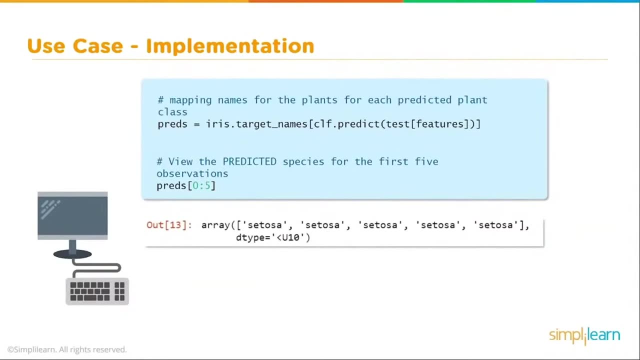 and we've looked at the predict probability. Let's see what's next on here. So now we want to go ahead and start mapping names for the plants. We want to attach names so that it makes a little more sense for us, And that's what we're going to do in these next two steps. 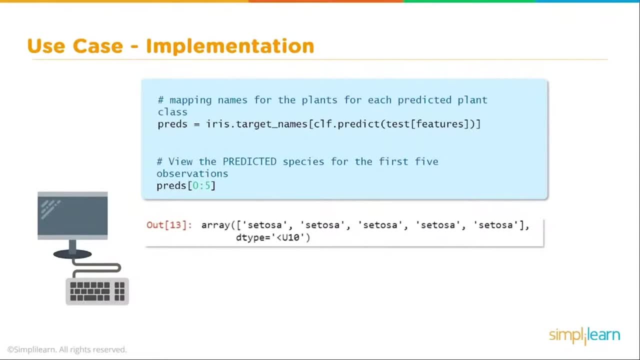 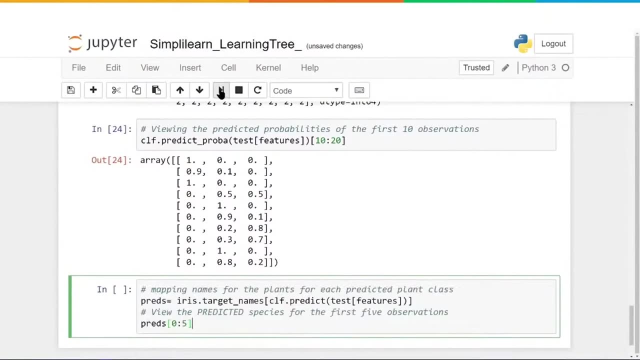 We're going to start by setting up our predictions and mapping them to the names. So let's see what that looks like And let's go ahead and paste that code in And run it. And this goes along with the next piece of code. 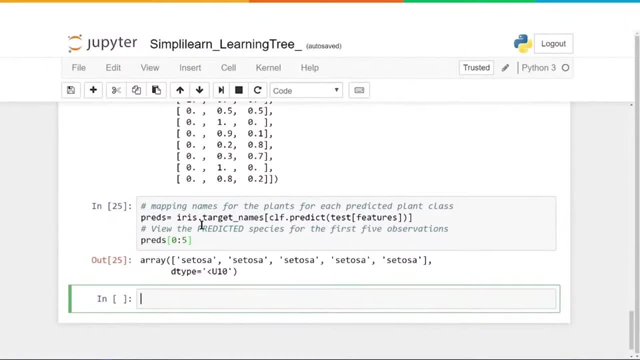 So we'll skip through this quickly and then come back to it a little bit. So here's iristargetNames And, if you remember correctly, this was the names that we've been talking about this whole time: the setosa virginica versicolor. 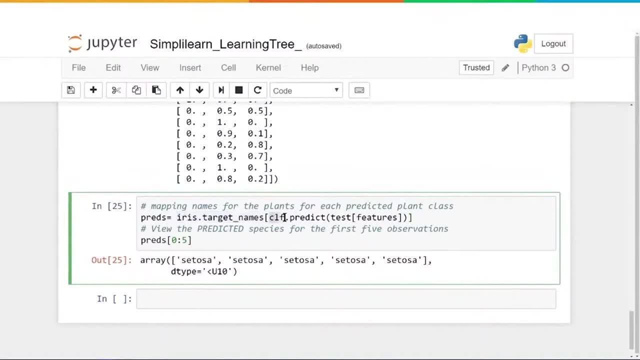 And then we're going to go ahead and do the prediction again. We could have just set a variable equal to this instead of re-running it each time, But we're going to go ahead and run it again. clfpredictTestFeatures- And remember that returns the 0s, the 1s and the 2s. 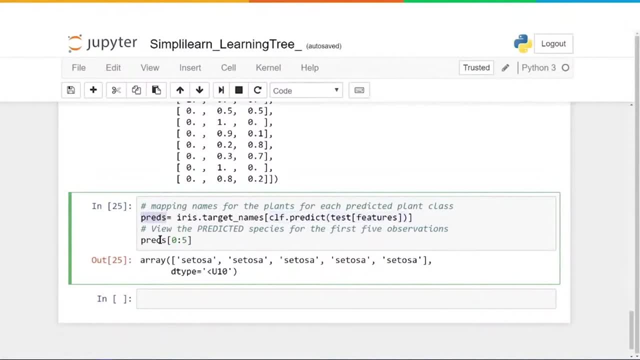 And then we're going to set that equal to predictions. So this time we're actually putting it in a variable And when I run this it distributes and it comes out as an array And the array is: setosa, setosa, setosa, setosa, setosa. 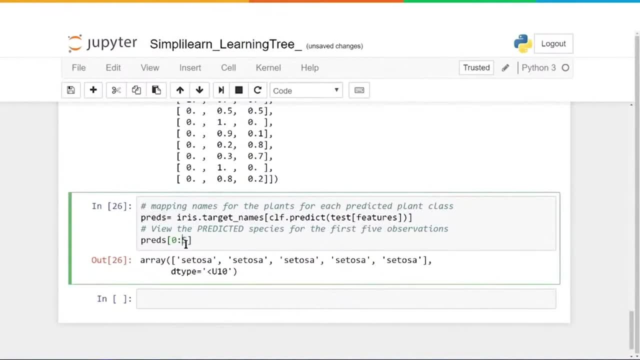 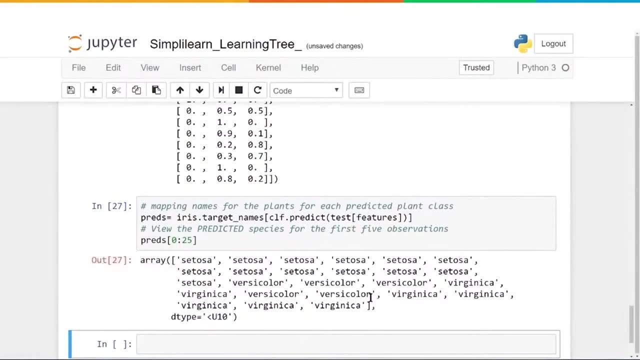 We're only looking at the first 5. We could actually do- let's do the first 25, just so we can see a little bit more on there- And you'll see that it starts mapping it to all the different flower types. 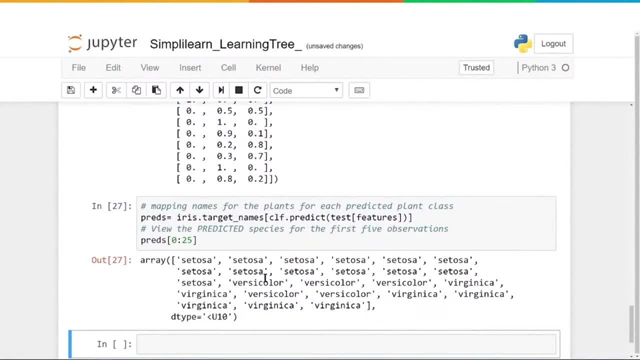 the versicolor and the virginica in there And let's see how this goes with the next one. So let's take a look at the top part of our species in here And we'll take this code and put it in our script. 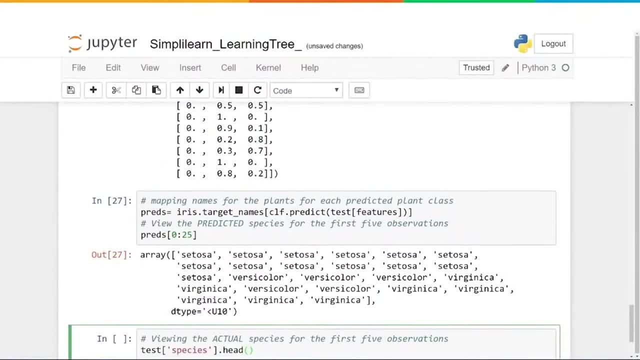 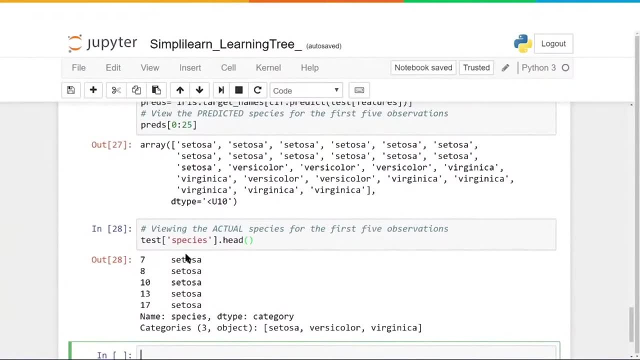 And let's put that down here and paste it. There we go And we'll go ahead and run it, And let's talk about both these sections of code here and how they go together. The first one is our predictions, And I went ahead and did predictions through 25.. 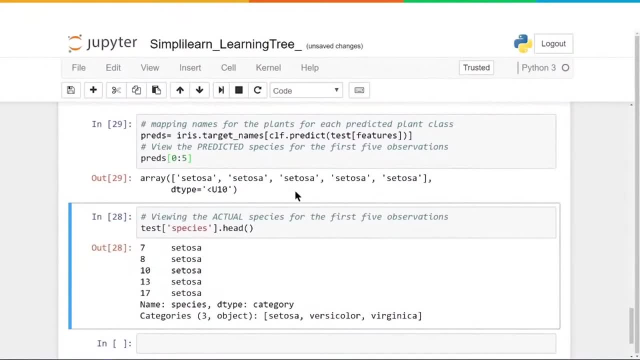 Let's just do 5. And so we have setosa, setosa, setosa, setosa, setosa. That's what we're predicting from our test model. And then we come down here and we look at test species And remember I could have just done testspecieshead. 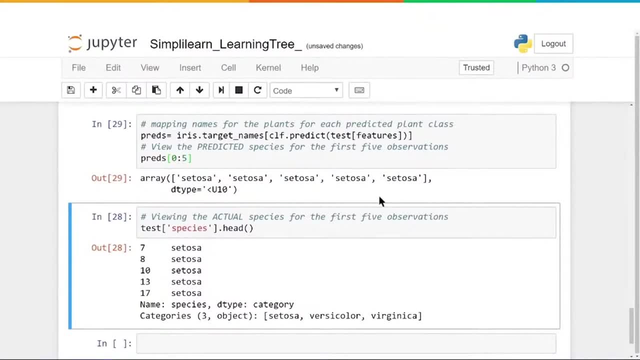 And you'll see, it says setosa setosa, setosa, setosa, And they match. So the first one is what our forest is doing And the second one is what the actual data is. Now we need to combine these so that we can understand what that means. 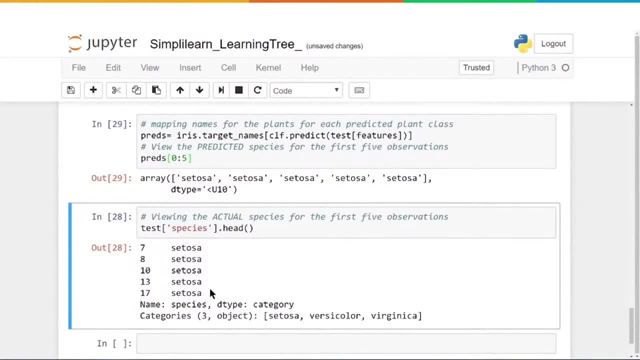 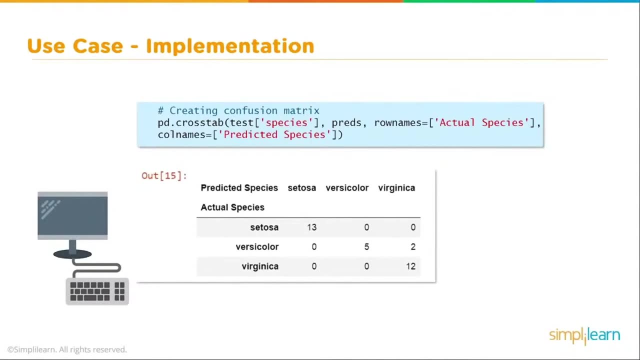 We need to know how good our forest is, how good it is at predicting the feature. So that's where we come up to the next step, which is lots of fun. We're going to use a single line of code to combine our predictions and our actuals. 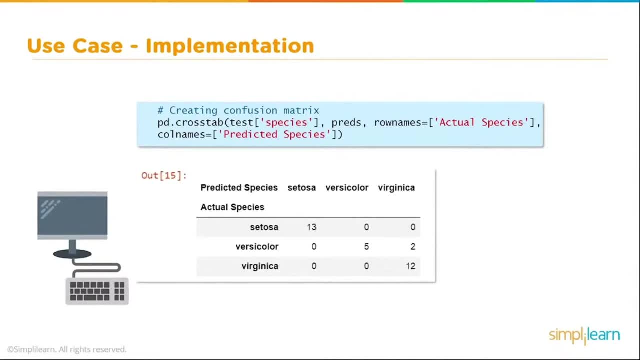 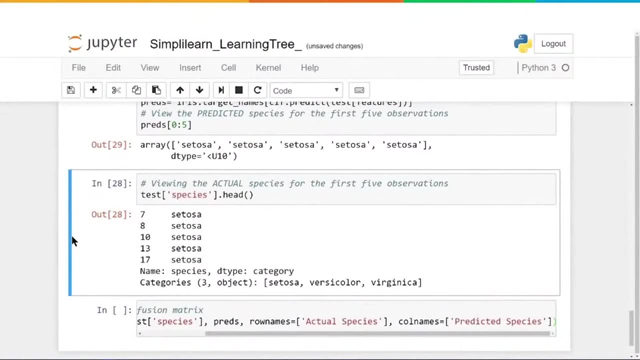 so we have a nice chart to look at And let's go ahead and put that in our script, in our Jupyter Notebook here. Let's see, let's go ahead and paste that in. And then I'm going to- because I'm on the Jupyter Notebook- 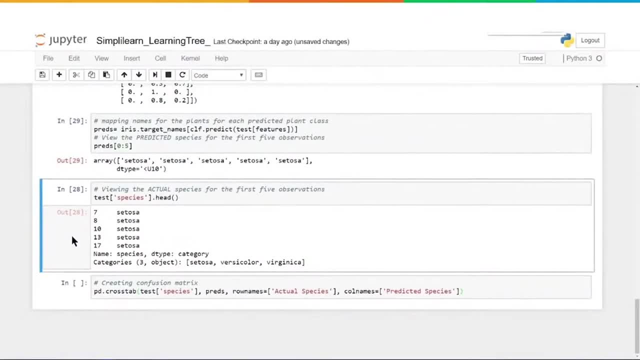 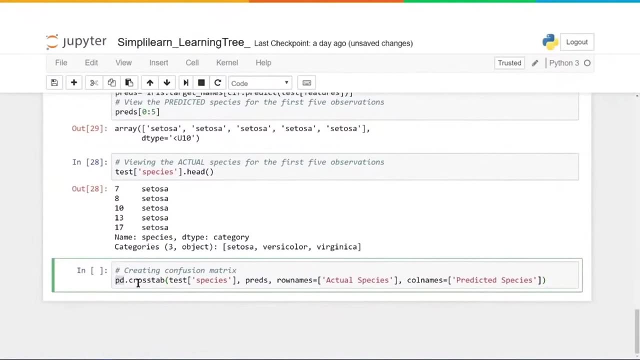 I can do a control minus. You can see the whole line there. There we go, resize it And let's take a look and see what's going on here. So we're going to create in pandas- Remember, PD stands for pandas. 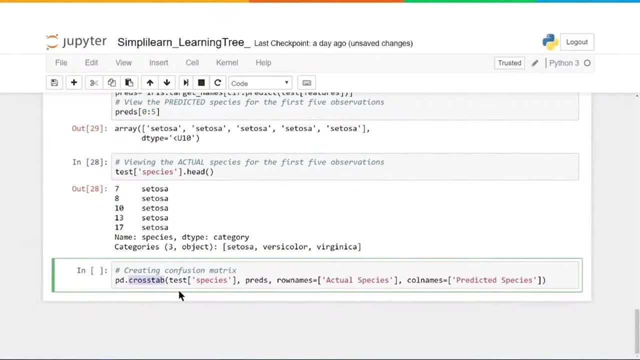 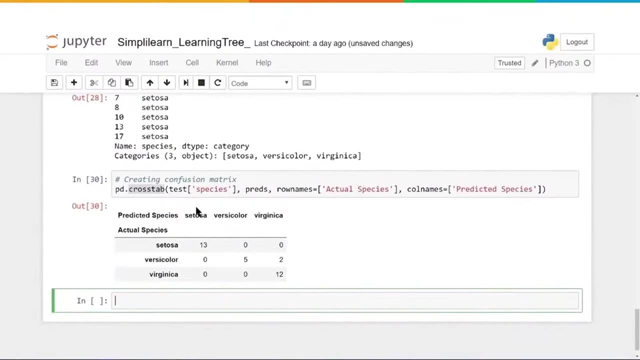 And we're doing a crosstab. This function takes two sets of data and creates a chart out of them. So when I run it you'll get a nice chart down here And we have the predicted species. So across the top you'll see the Cetosa versicolor virginica. 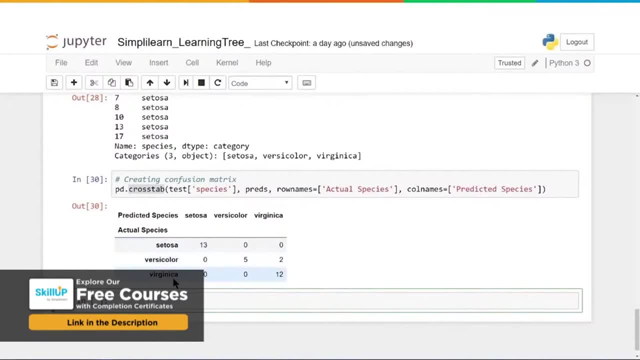 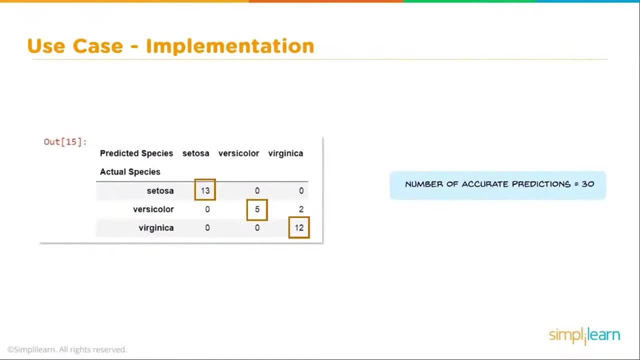 And the actual species, Cetosa versicolor virginica. And so the way to read this chart, and let's go ahead and take a look at how to read this chart here: When you read this chart, you have Cetosa where they meet. 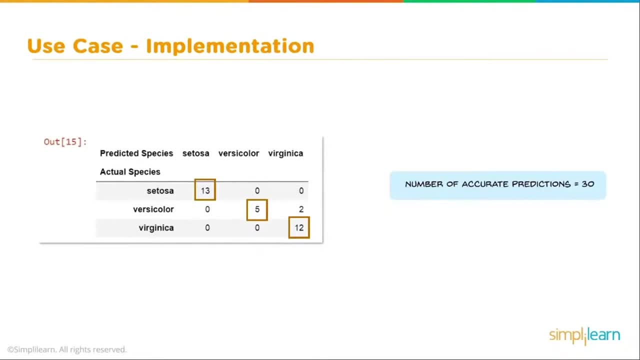 you have versicolor where they meet, and you have virginica where they meet, And they're meeting where the actual and the predicted agree. So this is the number of accurate predictions. So in this case it equals 30.. If you add 13 plus 5 plus 12, you get 30. 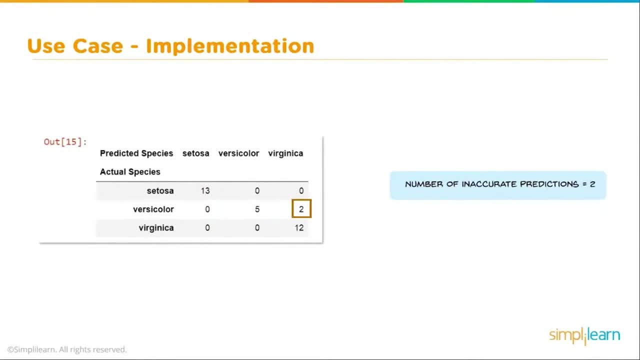 And then we notice here where it says virginica, but it was supposed to be versicolor. This is inaccurate. So now we have two: two inaccurate predictions and 30 accurate predictions. So we'll say that the model accuracy is 93.. 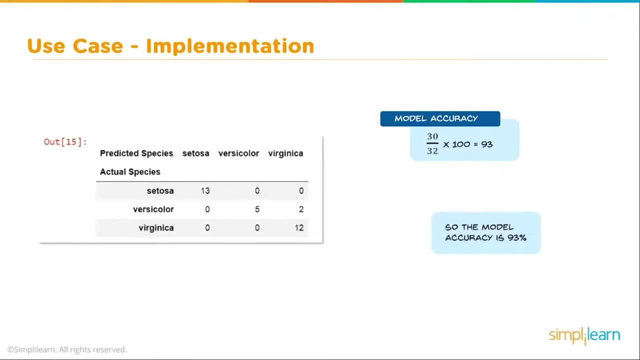 That's just 30 divided by 32.. And if we multiply it by 100, we can say that it is 93% accurate. So we have a 93% accuracy with our model. I did want to add one more quick thing in here on our scripting. 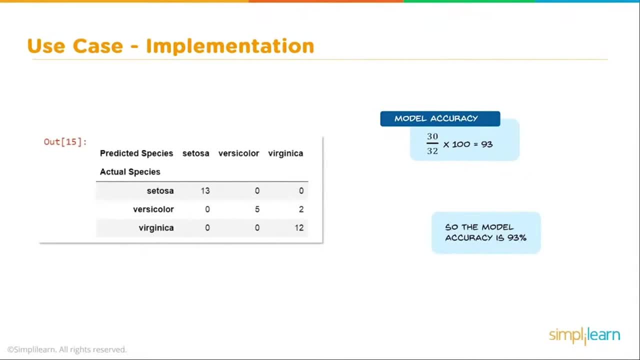 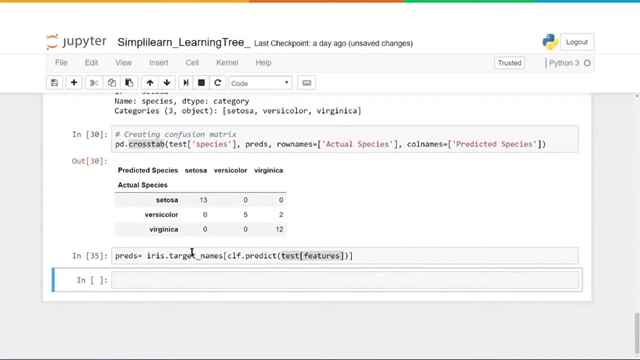 before we wrap it up. So let's flip back on over to my script. In here we're going to take this line of code from up above. I don't know if you remember it, but it predicts equals the iris dot target underscore names. 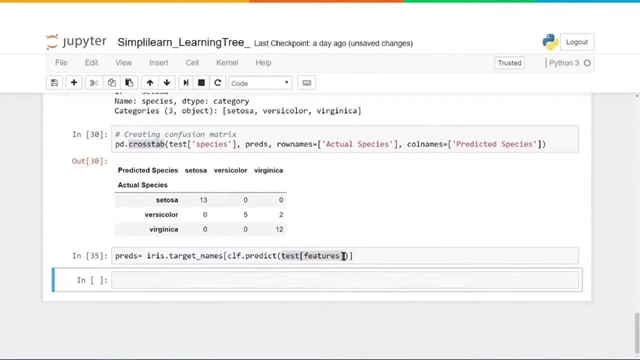 So we're going to map it to the names And we're going to run the prediction And we read it on test features. But you know, we're not just testing it, We want to actually deploy it. So at this point I would go ahead and change this. 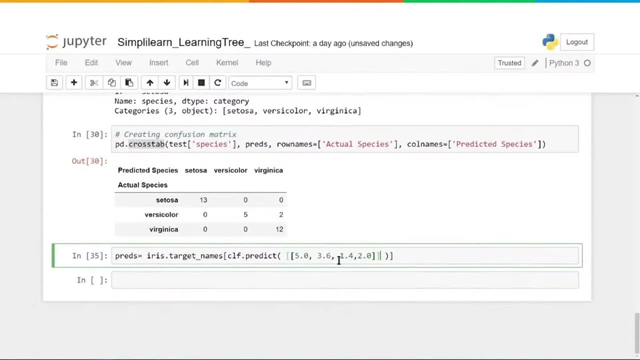 And this is an array of arrays. This is really important when you're running these to know that. So you need the double brackets And I could actually create data. Maybe let's just do two flowers, So maybe I'm processing more data coming in. 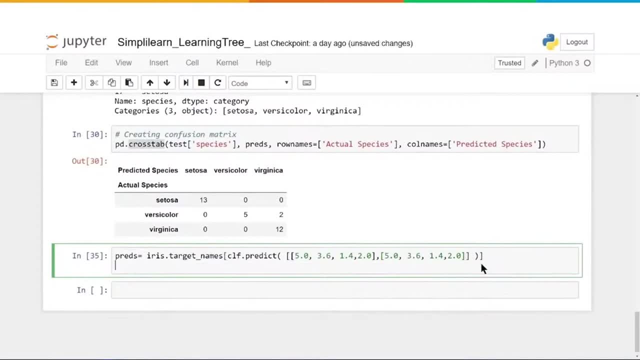 And we'll put two flowers in here, And then I actually want to see what the answer is. So let's go ahead and type in preds and print that out, And when I run this you'll see that I've now predicted two flowers. 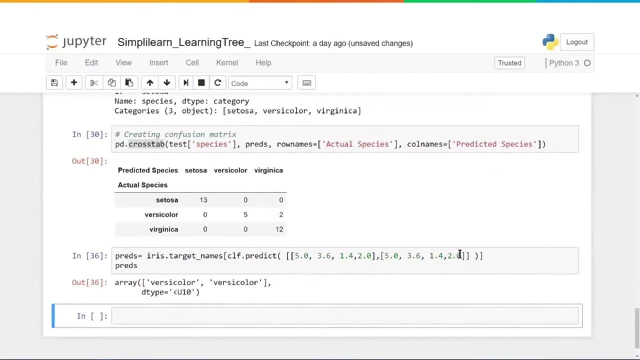 that maybe I measured in my front yard as versicolor and versicolor. Not surprising, since I put the same data in for each one. This would be the actual end product going out to be used on data that you don't know the answer for. 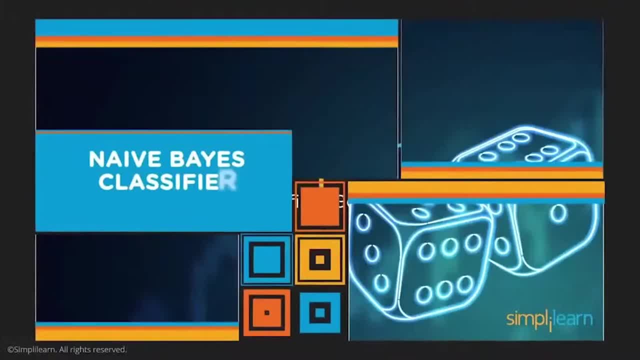 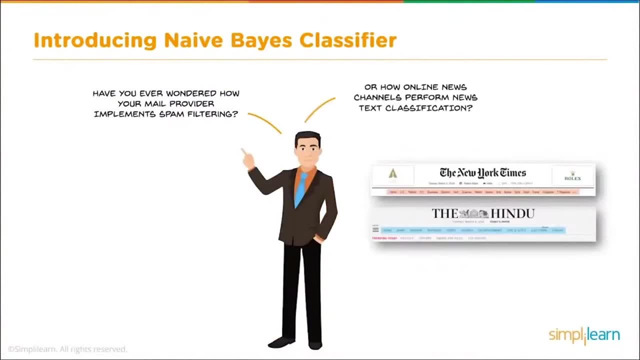 So that's going to conclude our scripting part of this Introducing Naive Bayes Classifier. Have you ever wondered how your mail provider implements spam filtering, Or how online news channels perform news text classification, Or how companies perform sentimental analysis of their audience on social media? 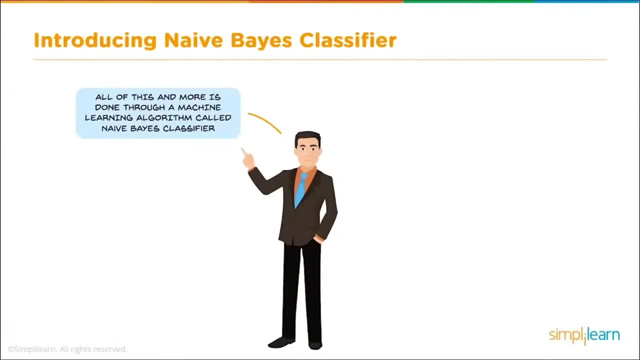 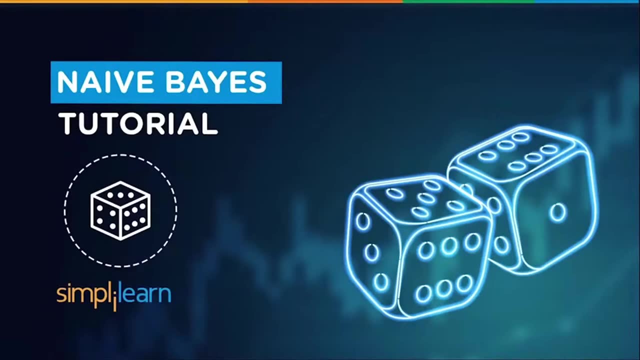 All of this and more is done through a machine learning algorithm called Naive Bayes Classifier. Welcome to Naive Bayes Tutorial. My name is Richard Kirshner. I'm with the Simply Learn team That's wwwsimplylearncom. 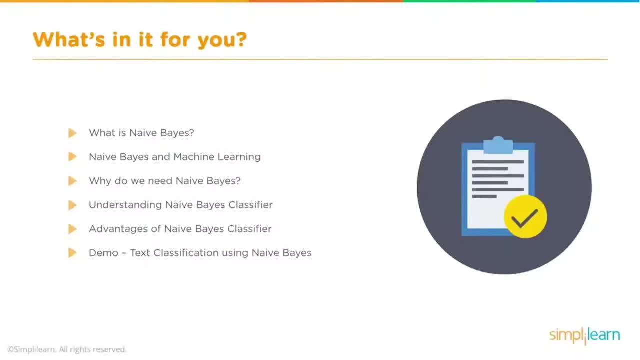 Get certified, Get ahead. What's in it for you? We'll start with what is Naive Bayes: A basic overview of how it works. We'll get into Naive Bayes and machine learning, where it fits in with our other machine learning tools. 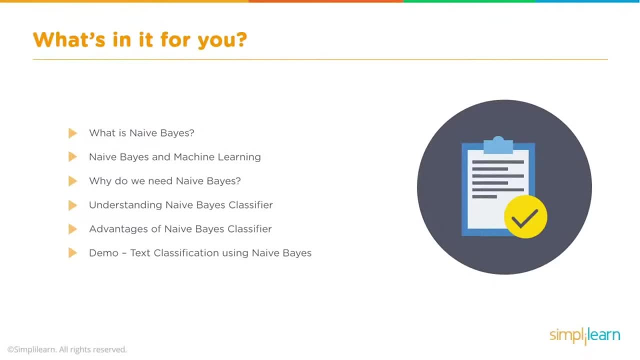 Why do we need Naive Bayes And understanding Naive Bayes Classifier in much more in-depth of how the math works in the background. Finally, we'll get into the advantages of the Naive Bayes Classifier in the machine learning setup. 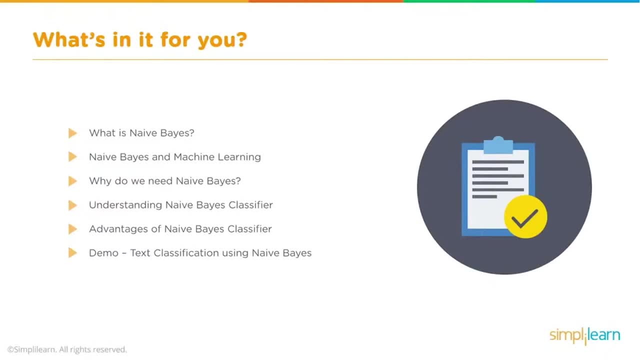 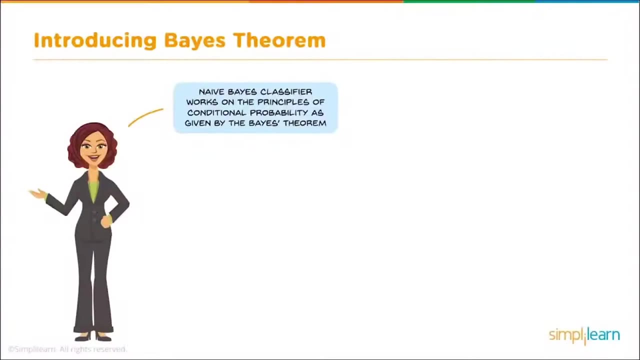 And then we'll roll up our sleeves and do my math. For my favorite part, we'll actually do some Python coding and do some text classification using the Naive Bayes. What is Naive Bayes? Let's start with a basic introduction to the Bayes Theorem. 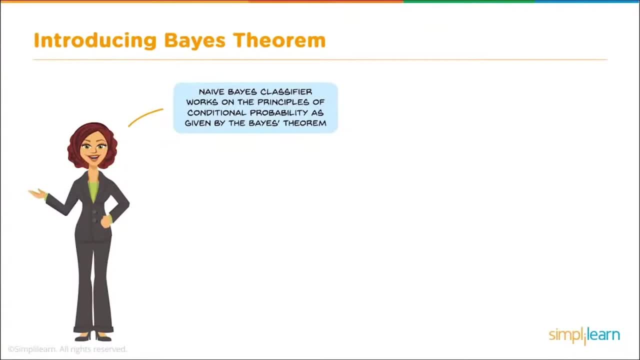 named after Thomas Bayes from the 1700s, who first coined this in the Western literature. Naive Bayes Classifier works on the principle of conditional probability as given by the Bayes Theorem. Before we move ahead, let us go through some of the simple concepts. 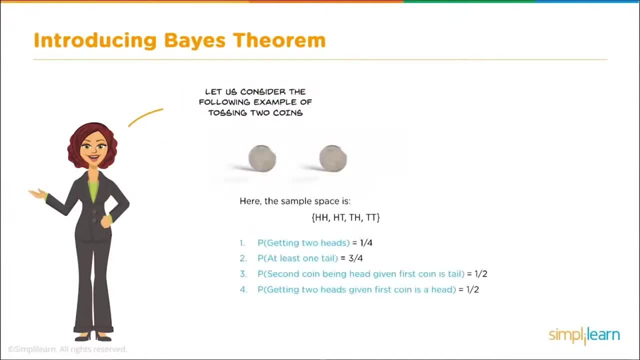 and the probability that we will be using. Let us consider the following example of tossing two coins. We have two quarters and if we look at all the different possibilities of what they can come up, as we get that, they can come up as head-heads. 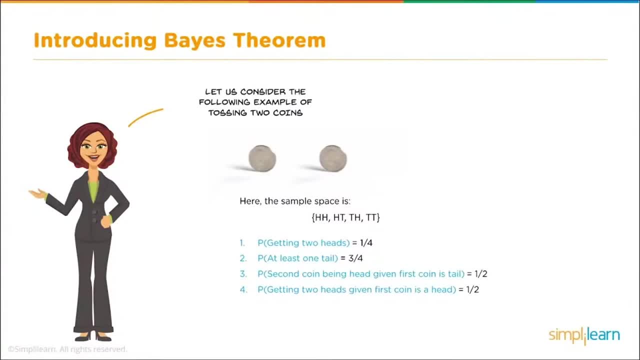 come up as head-tell, tell-head and tell-tell. When doing the math on probability, we usually denote probability as a P, a capital P. So the probability of getting two heads equals one-fourth. You can see on our data set: we have two heads. 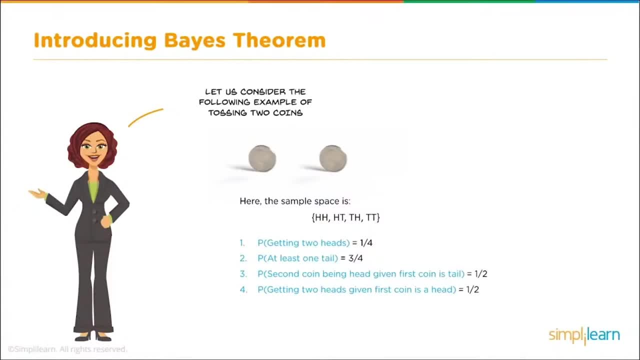 and this occurs once out of the four possibilities. And then the probability of at least one tell occurs three-quarters of the time. You'll see, on three of the coin tosses we have tells in them, And out of four that's three-fourths. 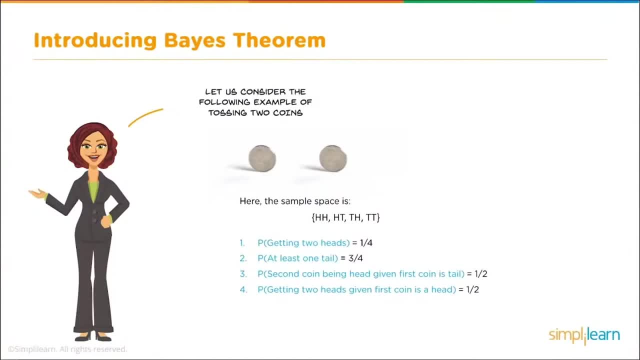 And then the probability of the second coin being head, given the first coin is tell, is one-half, And the probability of getting two heads, given the first coin is a head, is one-half. We'll demonstrate that in just a minute and show you how that math works. 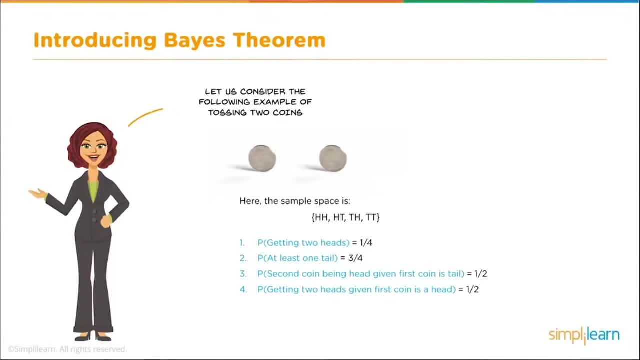 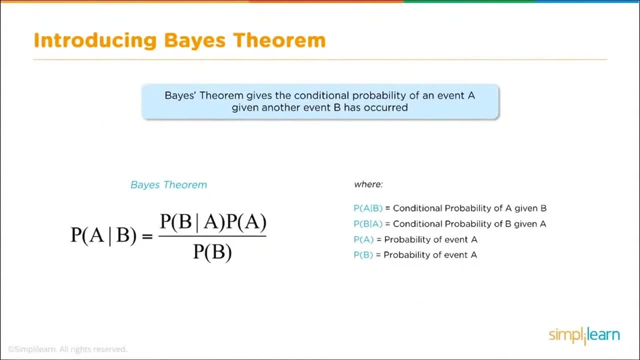 Now, when we're doing it with two coins, it's easy to see, But when you have something more complex, you can see where these formulas really come in and work. So the Bayes Theorem gives us the conditional probability of an event A given another event A. 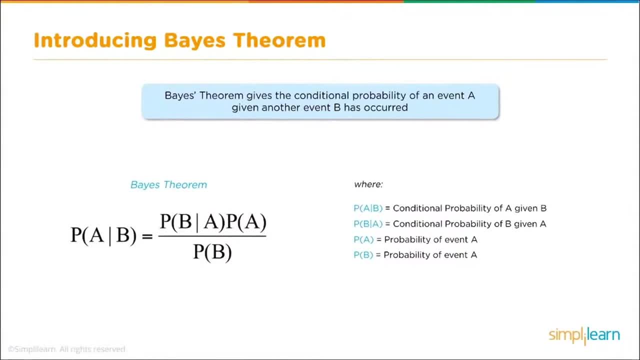 given another event, B has occurred. In this case, the first coin toss will be B and the second coin toss A. This could be confusing, because we've actually reversed the order of them and go from B to A instead of A to B. You'll see this a lot when you work in probabilities. 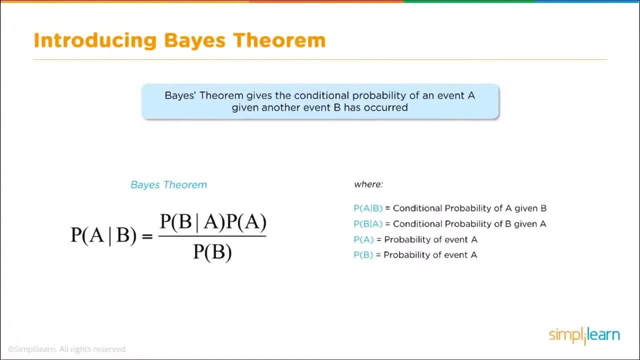 The reason is: we're looking for event A, We want to know what that is, So we're going to label that A, since that's our focus, And then, given another, event B has occurred In the Bayes Theorem, as you can see on the left. 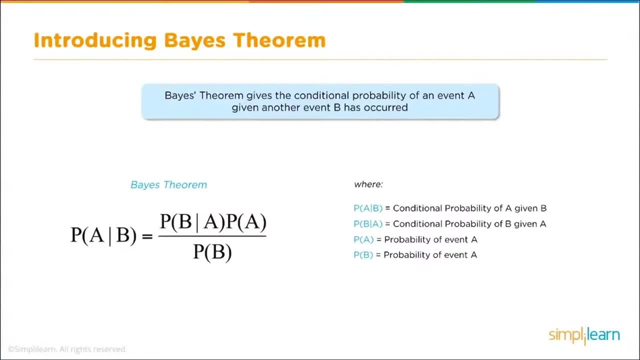 the probability of A occurring given B has occurred equals the probability of B occurring given A has occurred, times the probability of A over the probability of B. This simple formula can be moved around just like any algebra formula And we could do the probability of A after a given B. 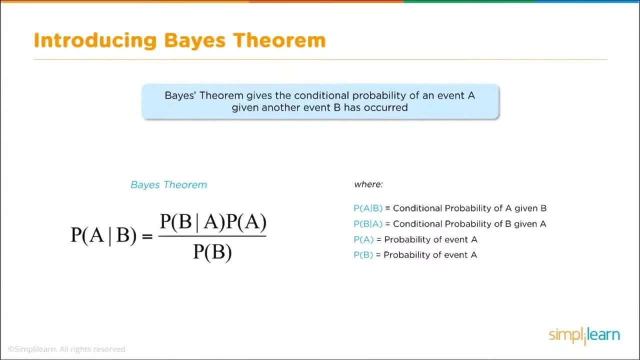 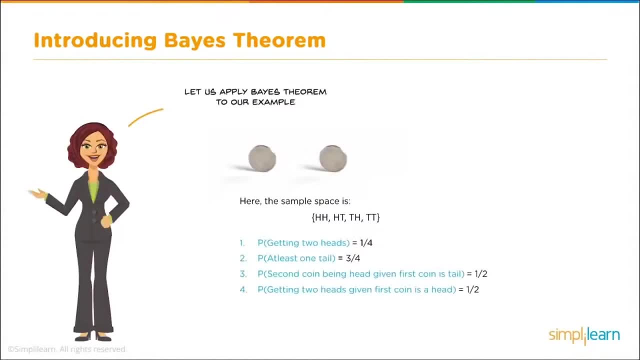 times probability of B equals the probability of B given A times probability of A. You can easily move that around and multiply it and divide it out. Let us apply Bayes Theorem to our example. Here we have our two quarters And we'll notice that the first two probabilities 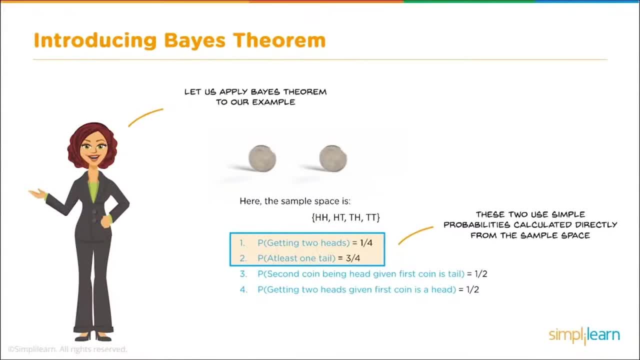 are getting two heads and at least one tail. We compute directly off the data, So you can easily see that we have one example HH out of four, one fourth And we have three with tails in them, giving us three quarters or three fourths- 75%. 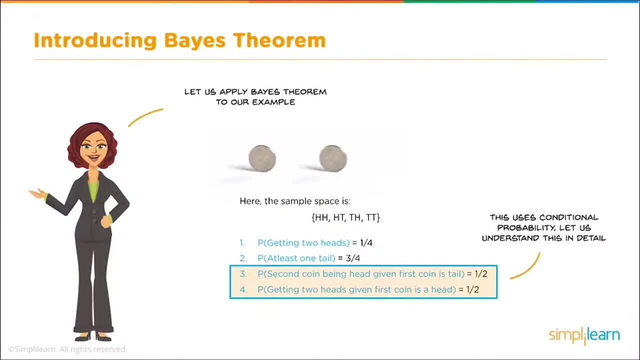 The second condition, the second set, three and four. we're going to explore a little bit more in detail Now. we stick to a simple example with two coins, because you can easily understand the math. The probability of throwing a tail doesn't matter what comes before it. 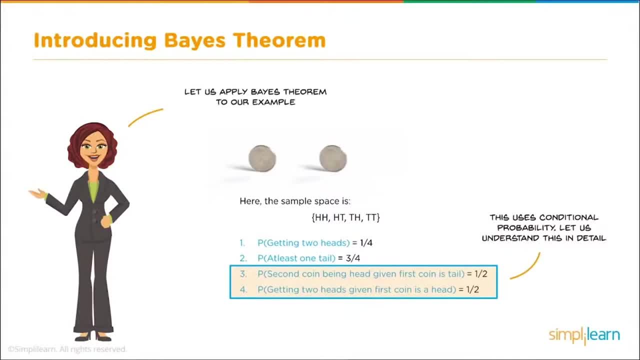 And the same with the heads. So it's still going to be 50% or one half. But when that probability gets more complicated- let's say you have a D6 dice or some other instance- then this formula really comes in handy. 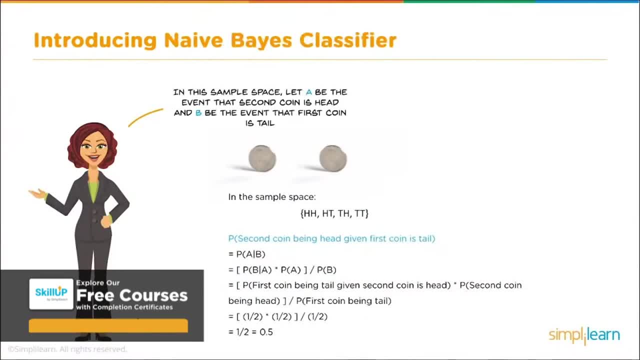 But let's stick to the simple example for now, In this sample space, let A be the event that the second coin is head and B be the event that the first coin is tails. Again, we reversed it because we want to know what the second event is going to be. 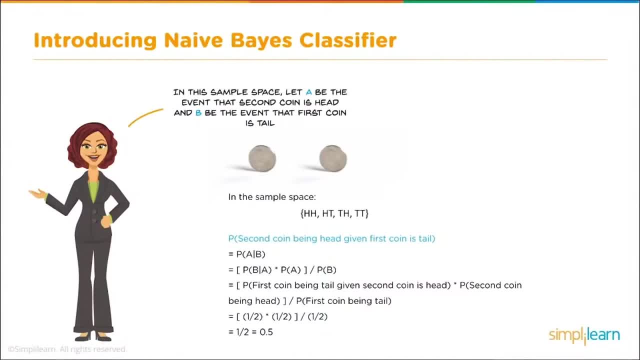 So we're going to be focusing on A And we write that out as the probability of A given B And we know this from our formula, that that equals the probability of B given A times the probability of A over the probability of B. And when we plug that in, 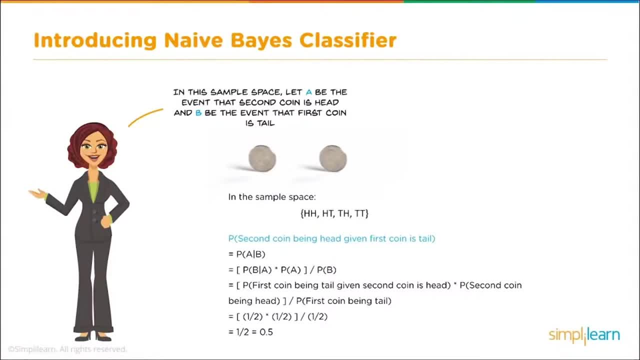 we plug in the probability of the first coin being tails, given the second coin is heads, and the probability of the second coin being heads, given the first coin being over the probability of the first coin being tails. When we plug that data in and we have the probability of the first coin being tails. 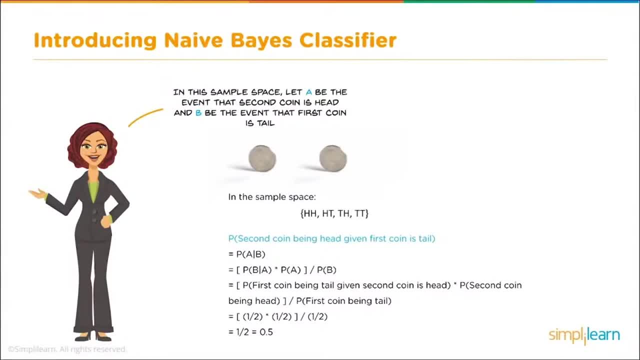 given the second coin is heads times the probability of the second coin being heads over the probability of the first coin being tails. You can see it's a simple formula to calculate. We have one-half times one-half, over one-half, or one-half equals .5 or one-fourth. 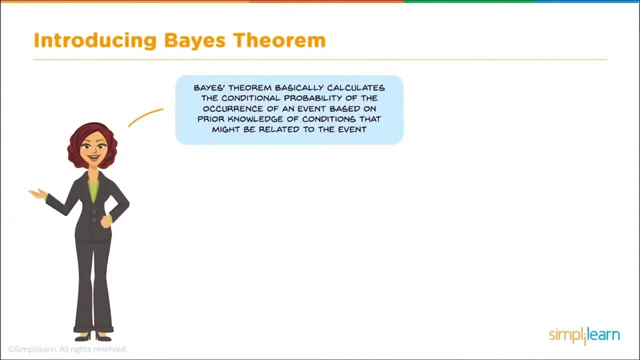 So the Bayes Theorem basically calculates the conditional probability of the occurrence of an event based on prior knowledge of conditions that might be related to the event. We will explore this in detail when we take up an example of online shopping further in this tutorial. 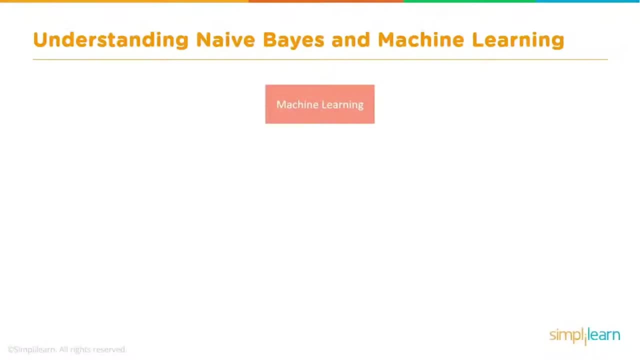 Understanding Naive Bayes and Machine Learning. Like with any of our other machine learning tools, it's important to understand where the Naive Bayes fits in the hierarchy. So under the Machine Learning, we have Supervised Learning and there is other things like Unsupervised Learning. 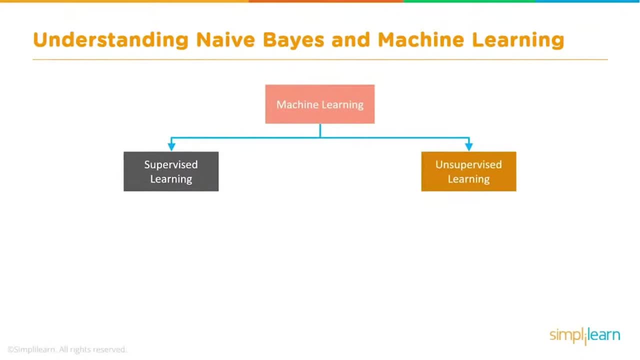 there's also Reward System. This falls under the Supervised Learning. and then under the Supervised Learning there's Classification, there's also Regression, but we're going to be in the Classification side. and then under Classification, is your Naive Bayes. Let's go ahead and glance into where is Naive Bayes used. 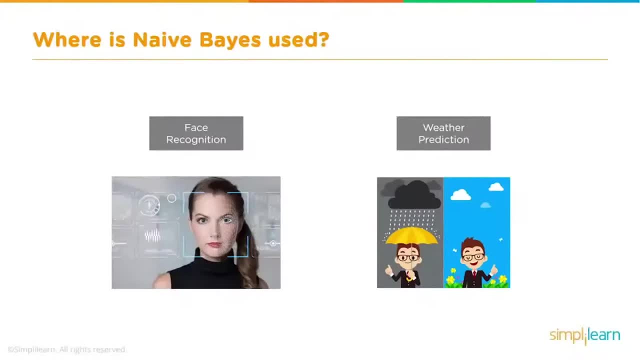 Let's look at some of the used scenarios for it. As a classifier. we use it in face recognition- is this Cindy, or is it not Cindy? or whoever? or it might be used to identify parts of the face that they then feed into another part of the face recognition program. 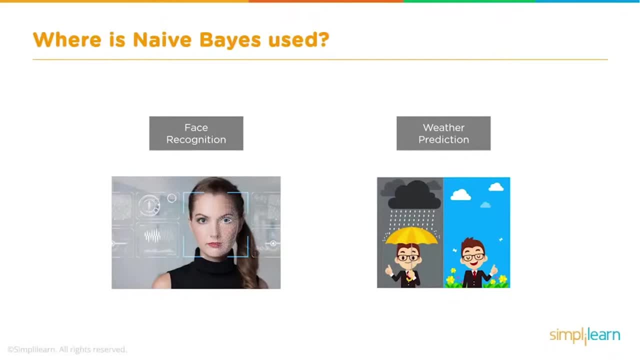 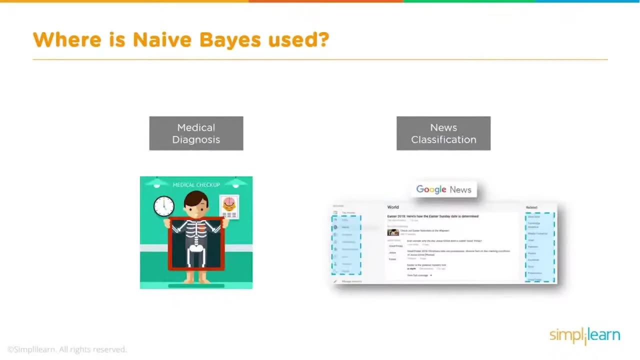 this is the eye, this is the nose, this is the mouth. weather prediction: is it going to be rainy or sunny? medical recognition news prediction. it's also used in medical diagnosis. we might diagnose somebody as either as high risk or not as high risk. 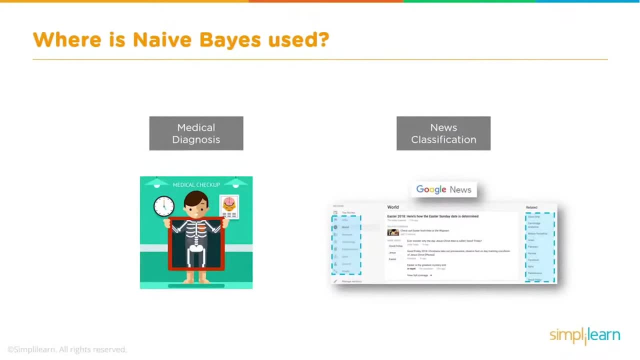 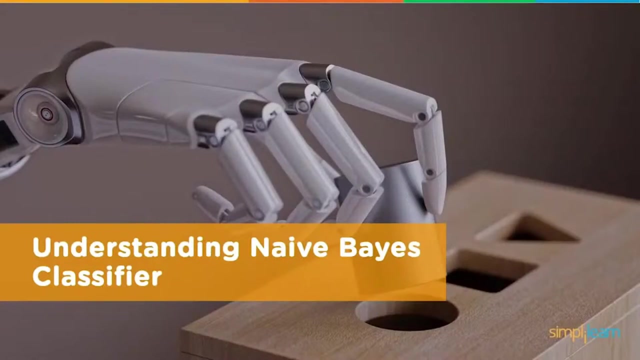 for cancer or heart disease or other ailments, and news classification. when you look at the Google News and it says: well, is this political or is this world news? or a lot of that's all done with the Naive Bayes Understanding Naive Bayes Classifier. Now we already went through a basic understanding. 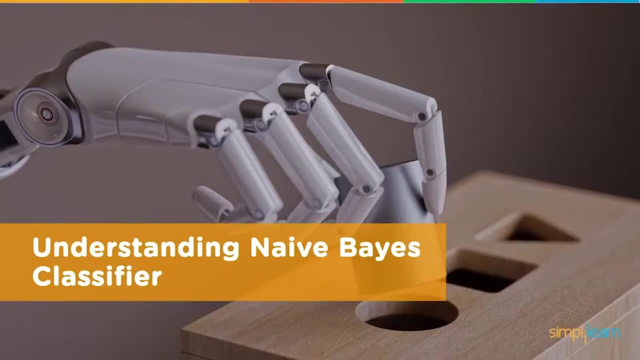 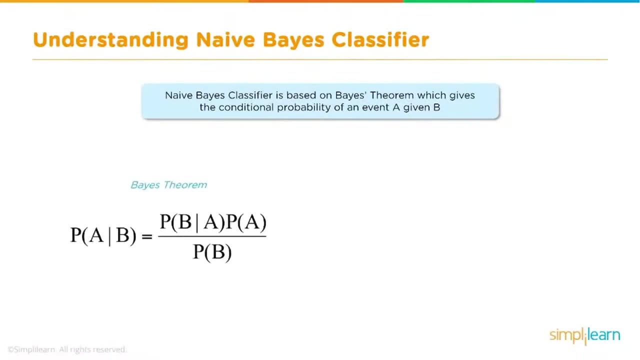 with the coins and the two heads and two tells, and head tell, tell heads, etc. We're going to do just a quick review on that and remind you that the Naive Bayes Classifier is based on the Bayes Theorem, which gives a conditional probability of event A given event B. 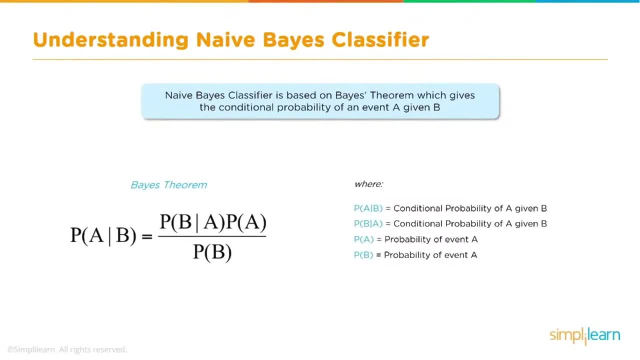 and that's where the probability of A given B equals the probability of B given A times the probability of A over the probability of B. remember, this is an algebraic function so we can move these different entities around. we can multiply by the probability of B, so it goes to the left hand side. 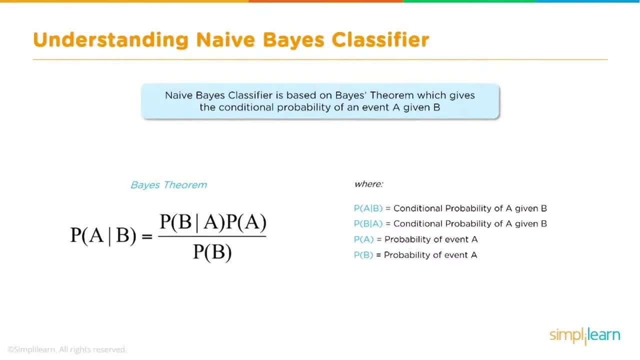 and then we can divide by the probability of A given B and just as easily come up with a new formula for the probability of B. to me, staring at these algebraic functions kind of gives me a slight headache. it's a lot better to see if we can actually understand. 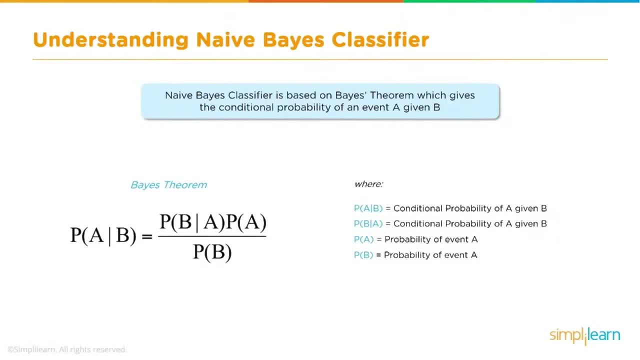 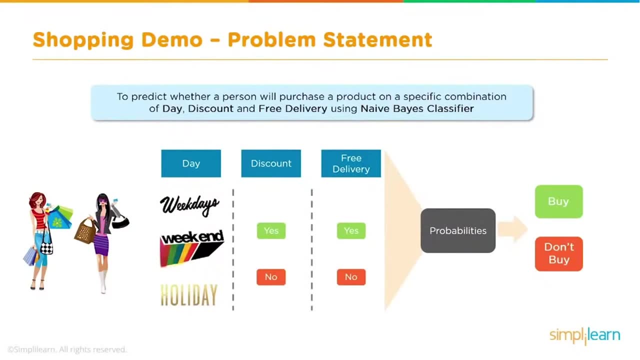 how this data fits together in a table and let's go ahead and start applying it to some actual data so you can see what that looks like. so we're going to start with the shopping demo problem statement and remember we're going to solve this first in table form. 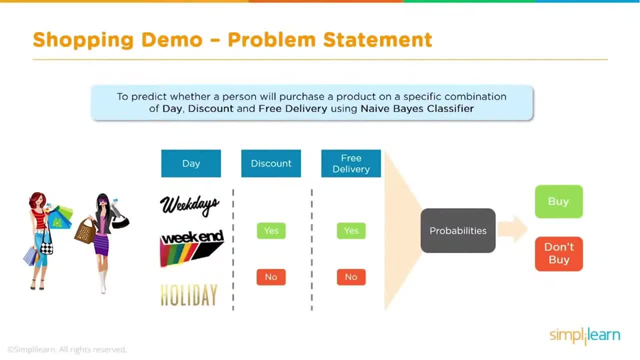 so you can see what the math looks like, and then we're going to solve it in Python and in here we want to predict whether the person will purchase a product. are they going to buy or don't buy? very important: if you're running a business, you want to know how to maximize your profits. 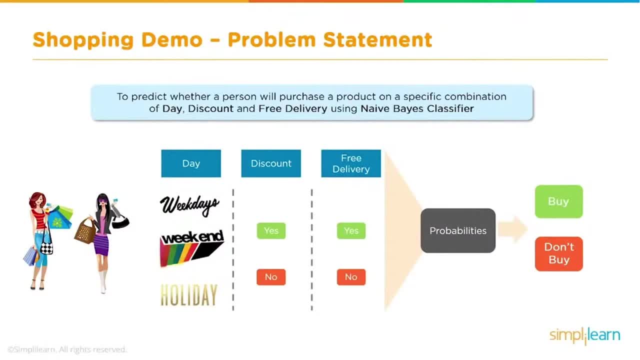 or at least maximize the purchase of the people coming into your store. and we're going to look at a specific combination of different variables. in this case, we're going to look at the day, the discount and the free delivery, and you can see here under the day. 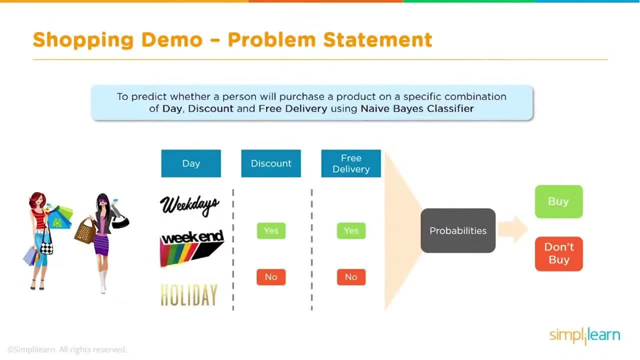 we want to know whether it's on the weekday. you know somebody's working. they come in after work or maybe they don't work weekend. you can see the bright colors coming down there celebrating not being in work or holiday. and did we offer a discount that day? 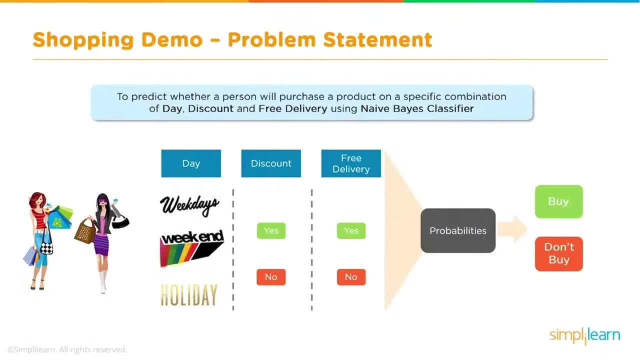 yes or no. did we offer free delivery that day, yes or no? and from this we want to know whether the person's going to buy based on these traits, so we can maximize them and find out the best system for getting somebody to come in and purchase our goods and products from our store. 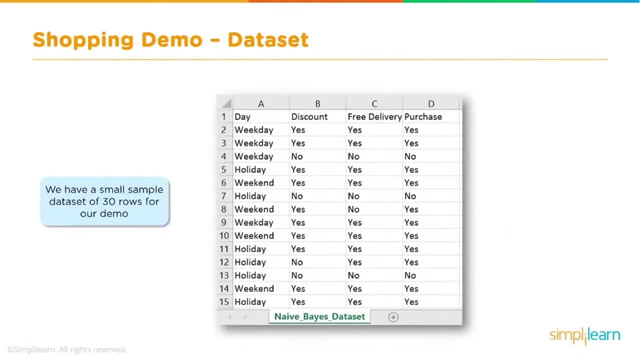 now. having a nice visual is great, but we do need to dig into the data. so let's go ahead and take a look at the data set. we have a small sample data set of 30 rows. we're showing you the first 15 of those rows. 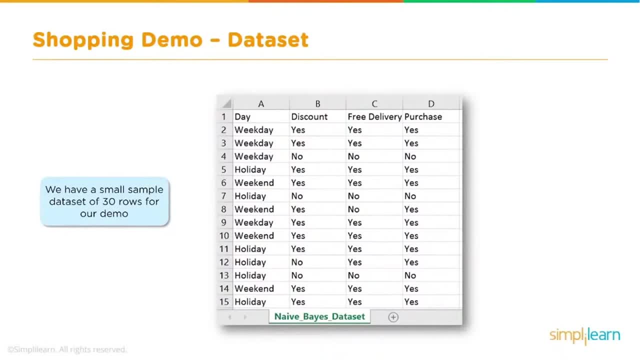 for this demo. now the actual data file you can request, just type in below under the comments on the YouTube video and we'll send you some more information and send you that file. as you can see here, the file is very simple: columns and rows. we have the day. 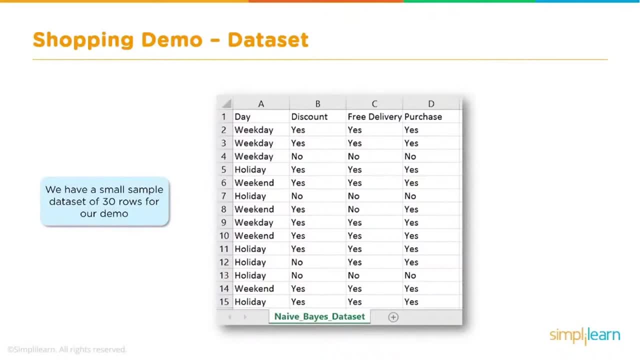 the discount, the free delivery, and did the person purchase or not? and then we have under data the day, whether it was a weekday, a holiday, was it the weekend? this is a pretty simple set of data and long before computers, people used to look at this data and calculate this all by hand. 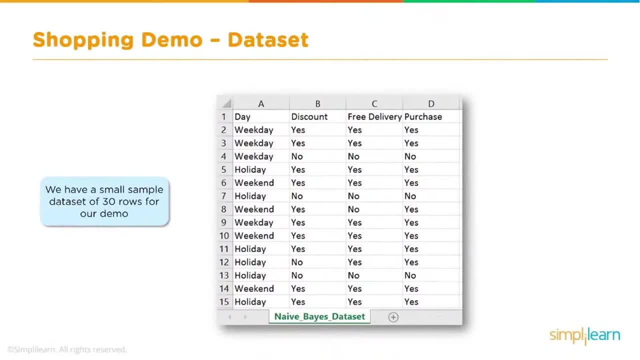 so let's go ahead and walk through this and see what that looks like, and we put that into tables. also, note: in today's world, we're not usually looking at three different variables in 30 rows. nowadays, because we're able to collect data so much, we're usually looking at 27,- 30 variables. 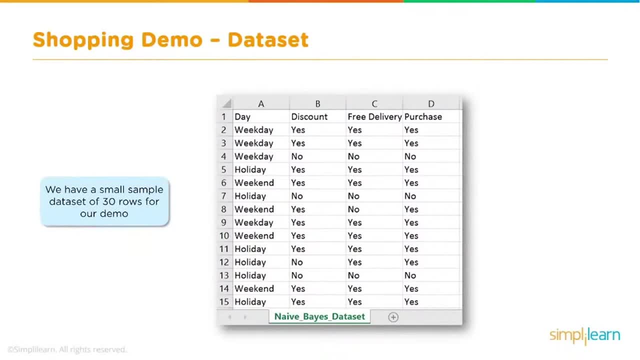 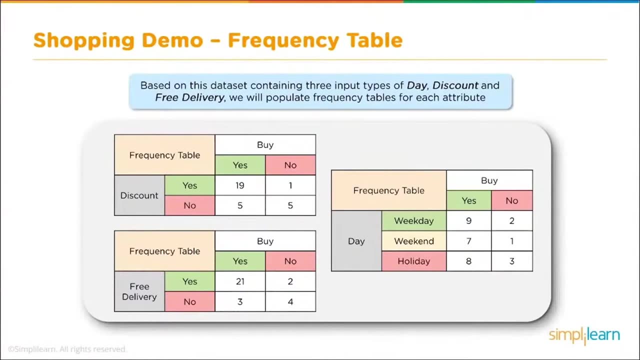 across hundreds of rows. the first thing we want to do is we're going to take a look at this data and, based on the data set containing our three inputs- day discount and free delivery- we're going to go ahead and populate that to frequency tables for each attribute. 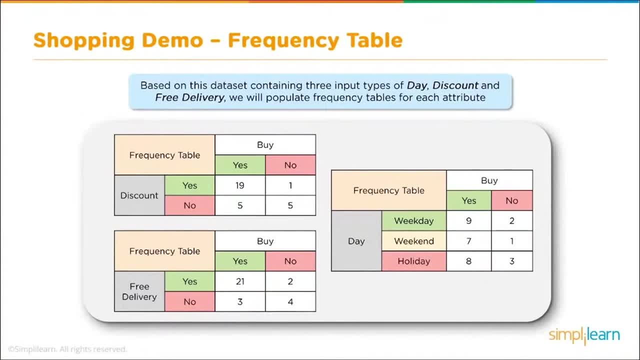 so we want to know if they had a discount. how many people buy and did not buy. did they have a discount, yes or no? do we have a free delivery, yes or no? on those days, how many people made a purchase and how many people didn't? and the same with the three days of the week. 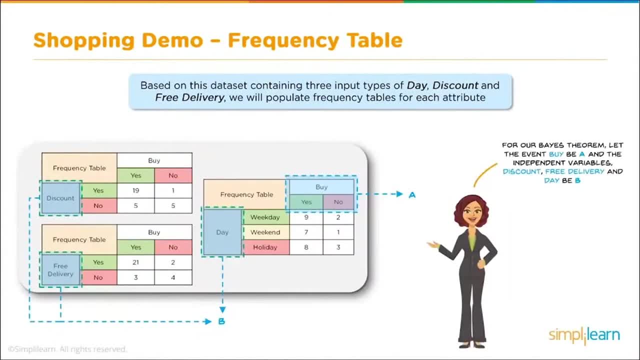 was it a weekday, a weekend, a holiday? and did they buy, yes or no? we're going to use the probability table for our Bayes theorem. let the event buy be A now. remember when we looked at the coins I said we really want to know what the outcome is. 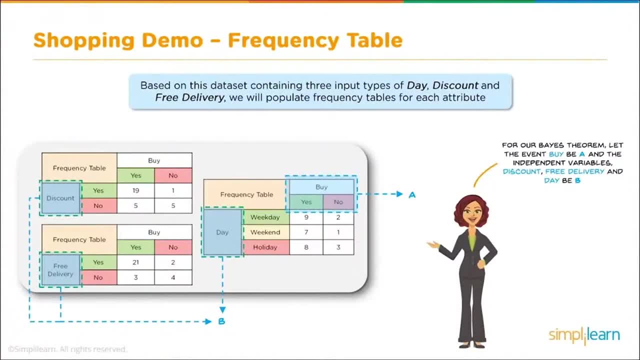 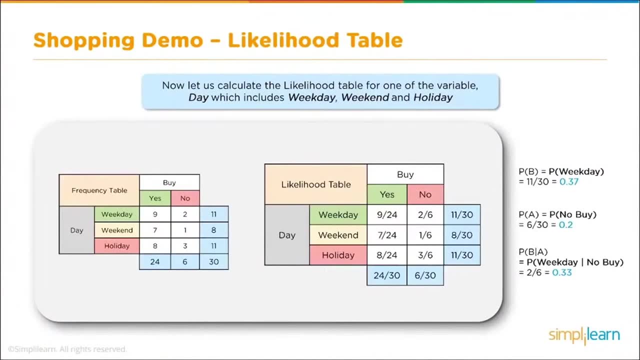 did the person buy or not, and that's usually event. A is what you're looking for, and the independent variables- discount, free delivery and day be B, so we'll call that probability of B. now let us calculate the likelihood table for one of the variables. 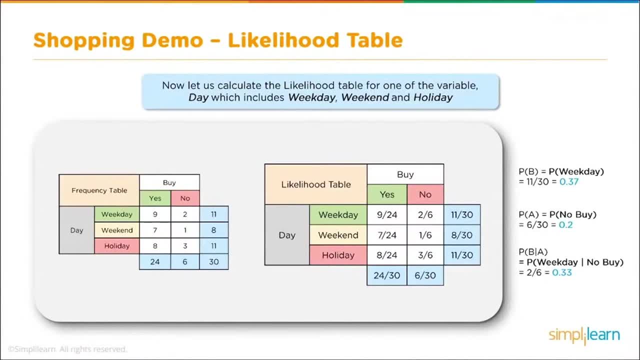 let's start with day which includes weekday, weekend and holiday, and let us start by summing all of our rows. so we have the weekday row and out of the weekdays there's 9 plus 2, so there's 11 weekdays. there's 8 weekend days. 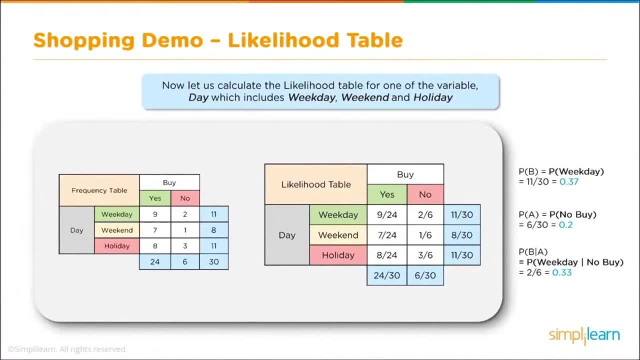 and 11 holidays. that's a lot of holidays. and then we want to sum up the total number of days, so we're looking at a total of 30 days. let's start pulling some information from our chart and see where that takes us and when we fill in the chart on the right. 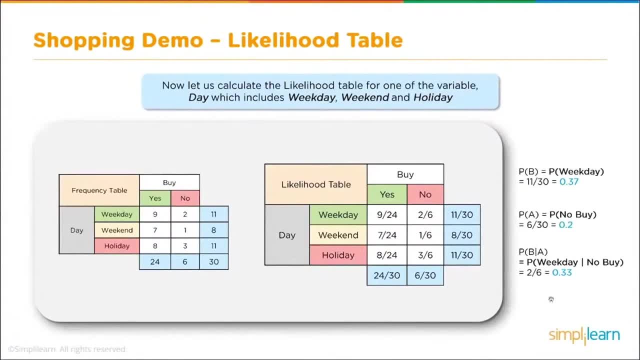 you can see that 9 out of 24 purchases are made on the weekday, 7 out of 24 purchases on the weekend and 8 out of 24 purchases on a holiday and, out of all the people who come in, 24 out of 30 purchase. 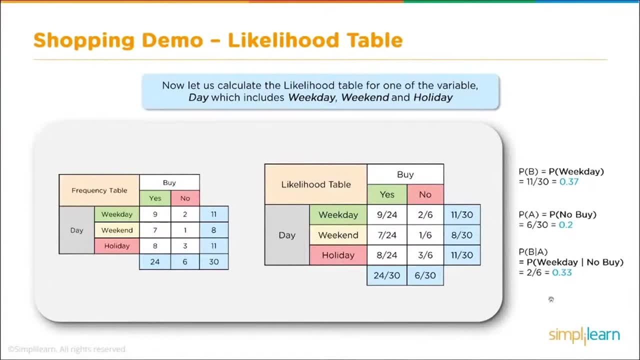 you can also see how many people do not purchase on the weekday. it's 2 out of 6 didn't purchase, and so on and so on. we can also look at the totals and you'll see. on the right we put together some of the formulas. 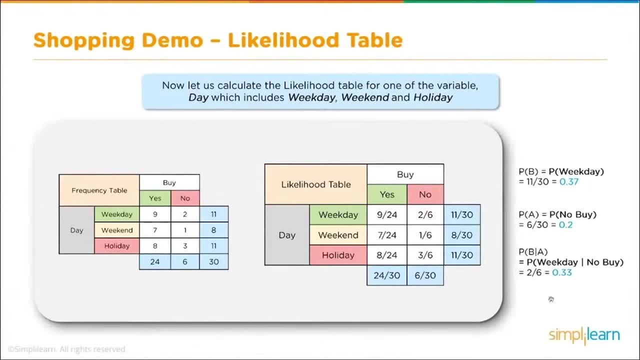 the probability of making a purchase on the weekend comes out at 11 out of 30. so out of the 30 people who came into the store throughout the weekend, weekday and holiday, 11 of those purchases were made on the weekday. and then you can also see the probability. 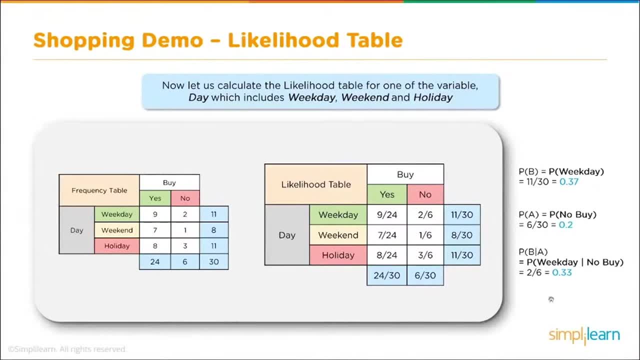 of them not making a purchase, and this is done for it doesn't matter which day of the week, so we call that probability of no buy would be 6 over 30 or 0.2, so there's a 20% chance that they're not going to make a purchase. 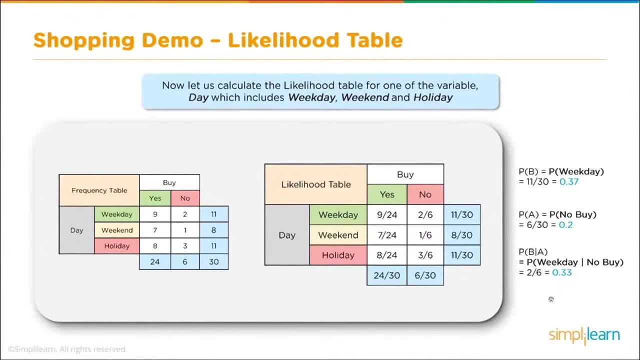 no matter what day of the week it is. and finally we look at the probability of B of A. in this case, we're going to look at the probability of the weekday and not buying. 2 of the no buys were done out of the weekend. out of the 6 people who did not make purchases: 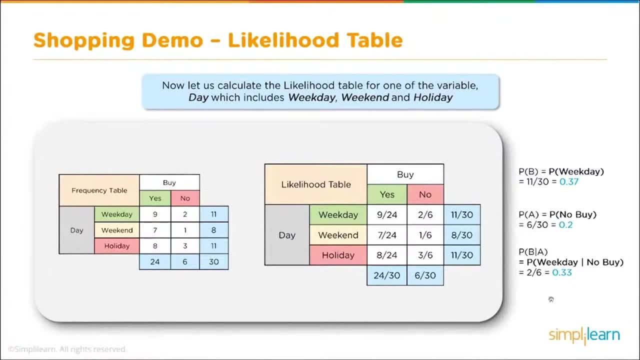 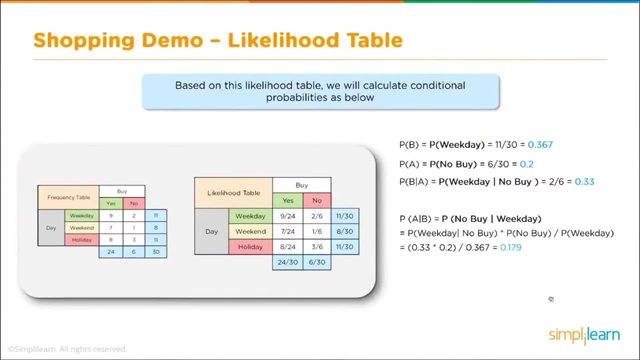 so when we look at that probability of the weekday without a purchase is going to be 0.33 or 33%, let's take a look at this, at different probabilities, and, based on this likelihood table, let's go ahead and calculate conditional probabilities as below. 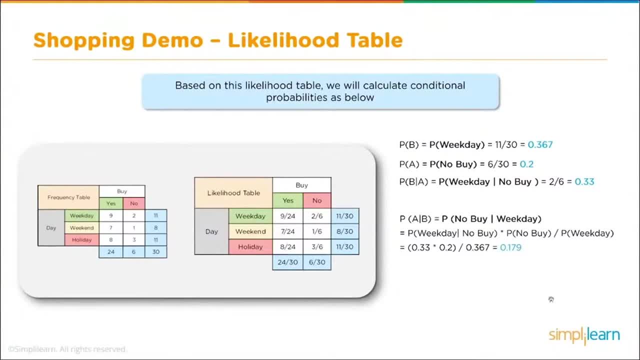 the first three we just did. the probability of making a purchase on the weekday is 11 out of 30, or roughly 36 or 37%, 0.367. the probability of not making a purchase at all doesn't matter what day of the week. 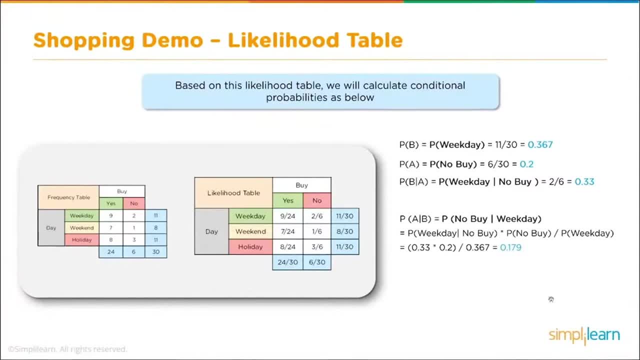 is roughly 0.2 or 20%, and the probability of a weekday no purchase is roughly 2 out of 6. so 2 out of 6 of our no purchases were made on the weekday. and then, finally, we take our P of AB. 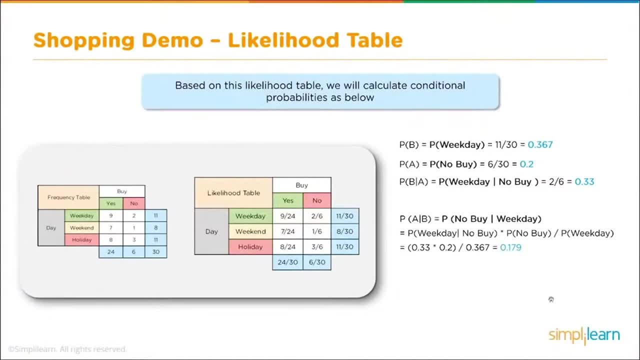 if you look- we've kept the symbols up there- we've got probability of B, probability of A, probability of B if A. we should remember that the probability of A if B is equal to the first, one times the probability of no buys over the probability of the weekday. 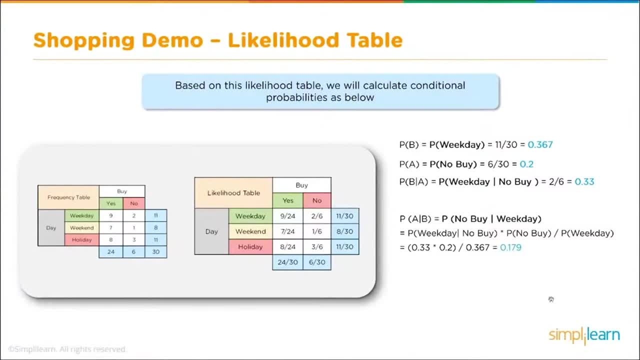 so we could calculate it both off the table we created. we can also calculate this by the form and we get the 0.367, which equals 0.33 times 0.2, over 0.367, which equals 0.179 or roughly. 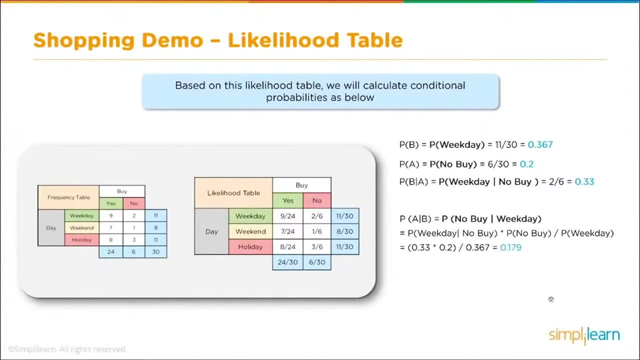 17 to 18% and that would be the probability of no purchase done on the weekday. and this is important because we can look at this and say, as the probability of buying on the weekday is more than the probability of not buying on the weekday, we can conclude: 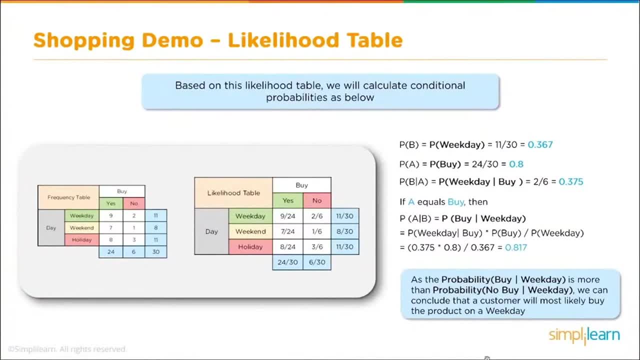 that customers will most likely buy the product on a weekday. so we've kept our chart simple and we're only looking at one aspect, so you should be able to look at the table and come up with the same information or the same conclusion. that should be kind of intuitive at this point. 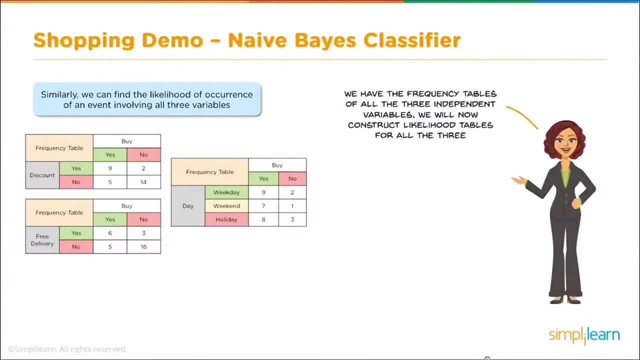 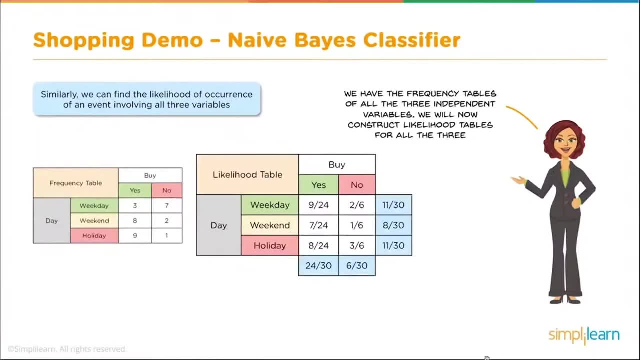 next we can take the same setup. we have the frequency tables of all three independent variables. now we can construct the likelihood tables for all three of the variables we're working with. we can take our day like we did before: we have weekday, weekend and holiday. 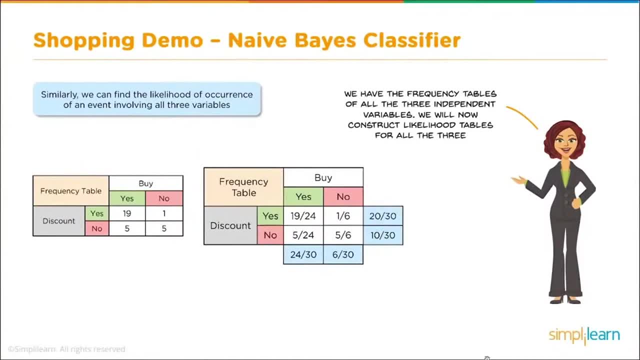 and we filled in this table, and then we can come in and also do that for the discount- yes or no- and we fill in that full table. so now we have our probabilities for a discount and whether the discount leads to a purchase or not, and the probability for free delivery. 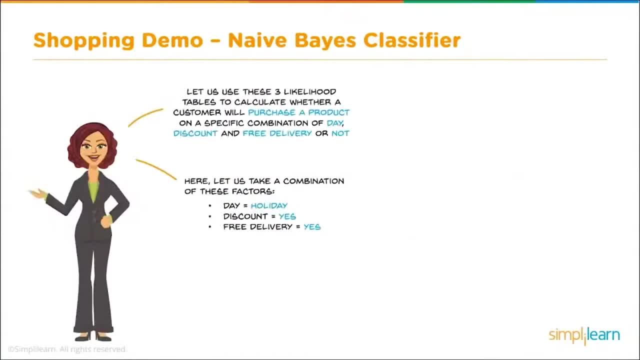 does that lead to a purchase or not? and this is where it starts getting really exciting. let us use these three likelihood tables to calculate whether a customer will purchase a product on a specific combination of day discount and free delivery or not purchase. here let us take a combination of these factors. 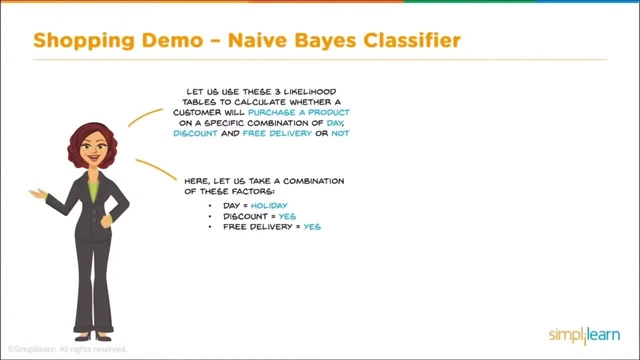 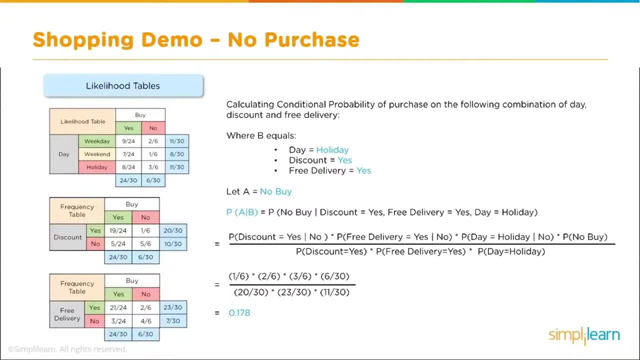 day equals holiday discount equals yes. free delivery equals yes. let's dig deeper into the math and actually see what this looks like, and we're going to start with looking for the probability of them not purchasing on the following combinations of days. we're actually looking for the probability of A. 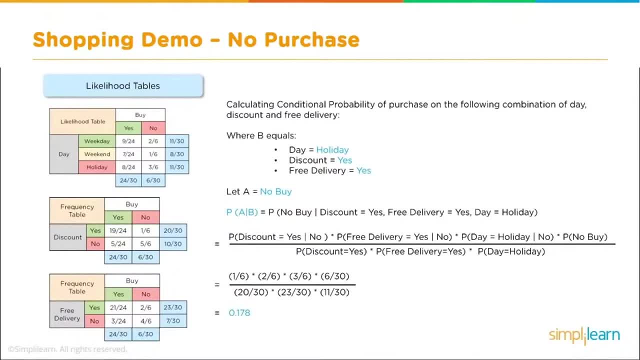 equals no buy, no purchase, and our probability of B we're going to set equal to: is it a holiday? did they get a discount? yes, and was it a free delivery? yes, before we go further, let's look at the original equation. the probability of B equals the probability of B. 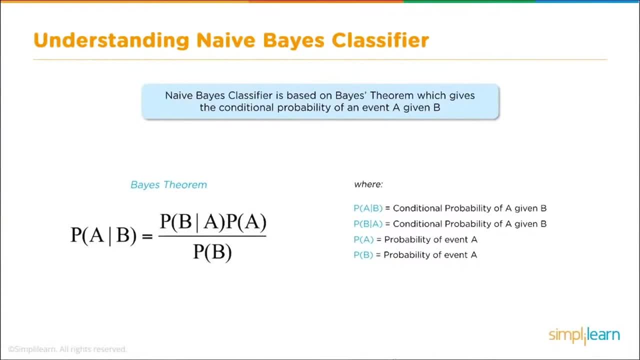 given the condition, A times the probability of A over the probability of B occurring. now this is basic algebra, so we can multiply this information together. so when you see the probability of A given B, in this case the condition is B, C and D, or the three different variables we're looking at. 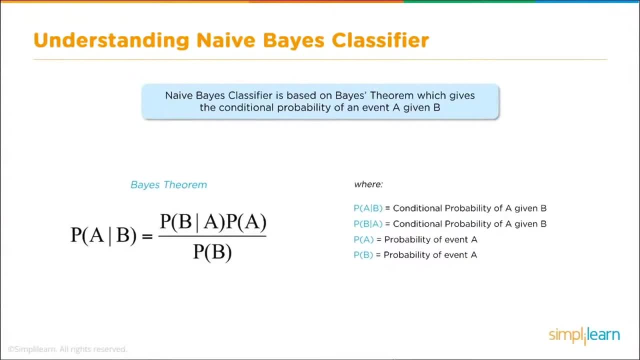 and when you see the probability of B, that would be the conditions. we're actually going to multiply those three separate conditions out. you'll see that in just a second in the formula times the full probability of A over the full probability of B. so here we are, back to this. 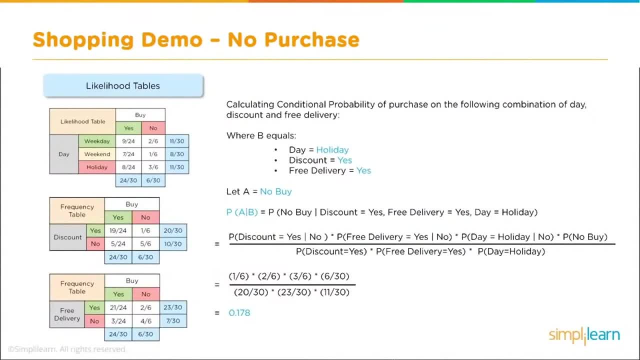 and we're going to have let A equal no purchase and we're looking for the probability of B on the condition A, where A sets for three different things. remember that equals the probability of A given the condition B and in this case we just multiply those three different variables together. 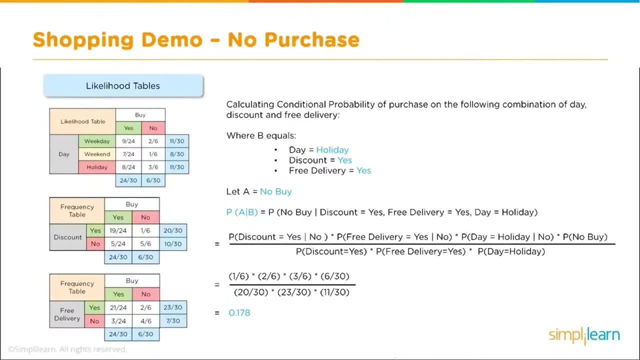 so we have the probability of the discount times, the probability of free delivery times, the probability is the day equal a holiday. those are our three variables of the probability of A, if B, and then that is going to be multiplied by the probability of them not making a purchase. 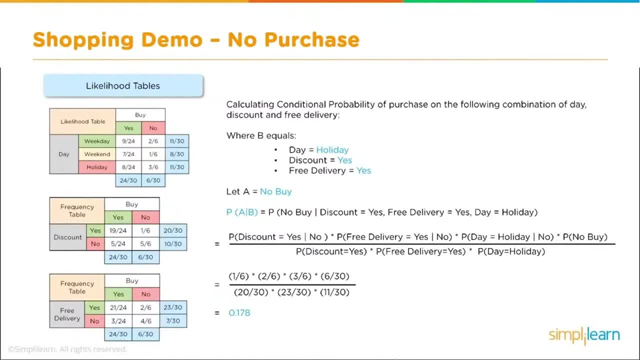 and then we want to divide that by the total probabilities and they're multiplied together so we have the probability of a discount, the probability of a free delivery and the probability of it being on a holiday. when we plug those numbers in, we see that one out of six were no purchase. 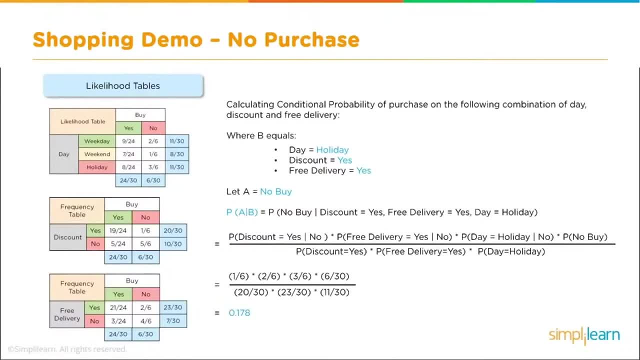 on a discounted day, two out of six were a no purchase on a free delivery day and three out of six were a no purchase on a holiday. those are our three probabilities of A if B multiplied out, and then that has to be multiplied by the probability of a no purchase. 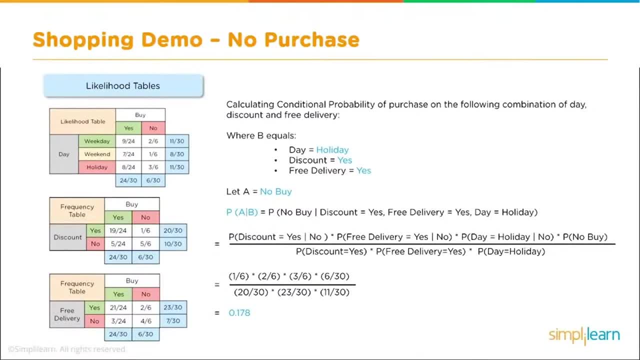 and remember the probability of a no buy is across all the data. so that's where we get the six out of thirty. we divide that out by the probability of each category over the total number. twenty-three out of thirty had a discount. twenty-three out of thirty had a yes for free delivery. 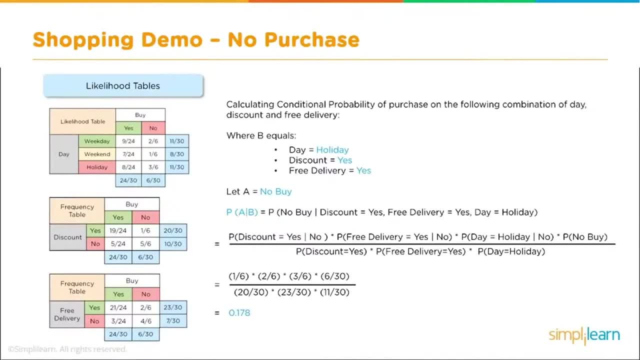 and eleven out of thirty were on a holiday. we plug all those numbers in, we get point one, seven, eight. so in our probability math we have a point one, seven, eight. if it's a no buy for a holiday, a discount and a free delivery, let's turn that around. 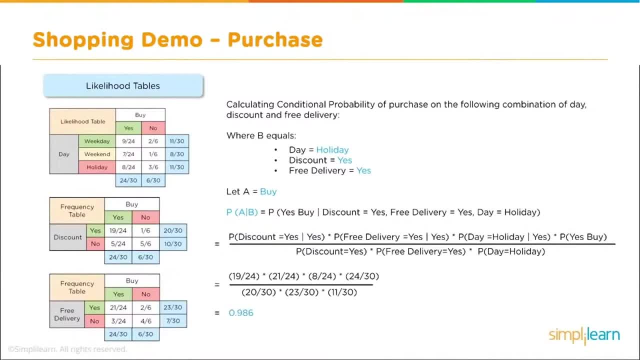 and see what that looks like if we have a purchase. I promise this is the last page of math before we dig into the Python script. so here we're, calculating the probability of the purchase using the same math we did to find out if they didn't buy. 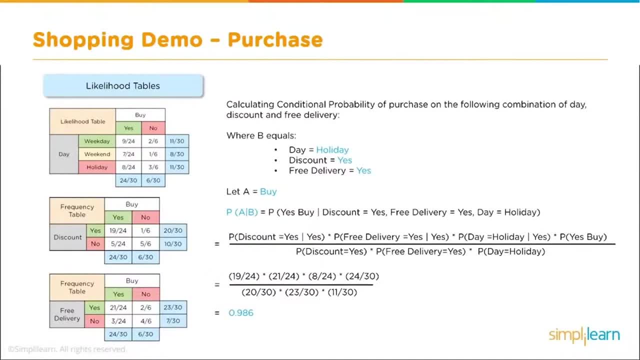 now we want to know if they did buy. and again we're going to go by the day: equals a holiday discount equals yes, free delivery equals yes, and let A equal buy. now, right about now, you might be asking: why are we doing both calculations? why would we want to know the? 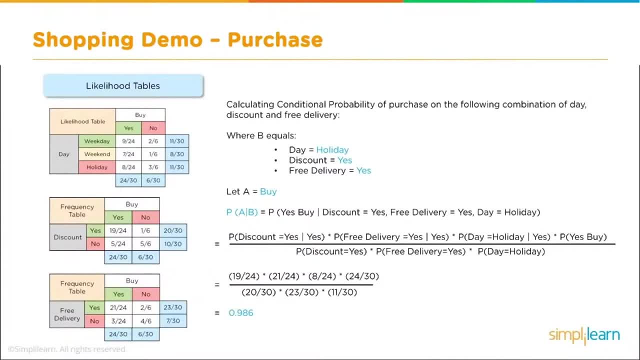 no buys and buys for the same data going in. well, we're going to show you that in just a moment. but we have to have both of those pieces of information so that we can figure it out as a percentage as opposed to a probability equation, and we'll get to that normalization. 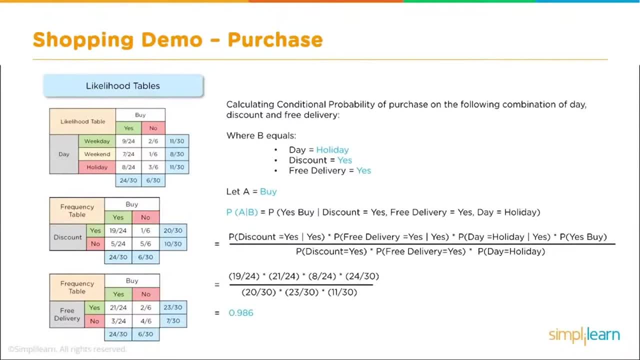 here in just a moment. let's go ahead and walk through this calculation and, as you can see here, the probability of A on the condition of B, B being all three categories, did we have a discount with a purchase? do we have a free delivery with a purchase? 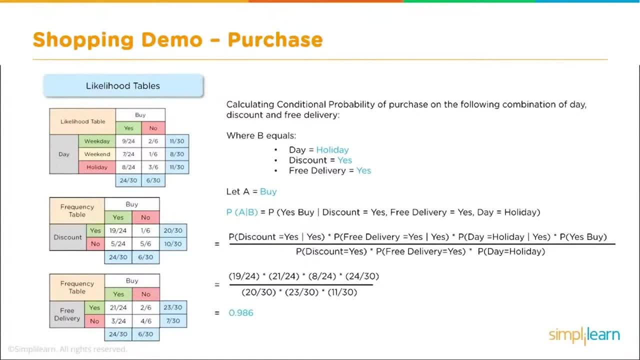 and is a day equal to holiday. and when we plug this all into that formula and multiply it all out, we get our probability of a discount, probability of a free delivery, probability of the day being a holiday times, the overall probability of it being a purchase multiplied by 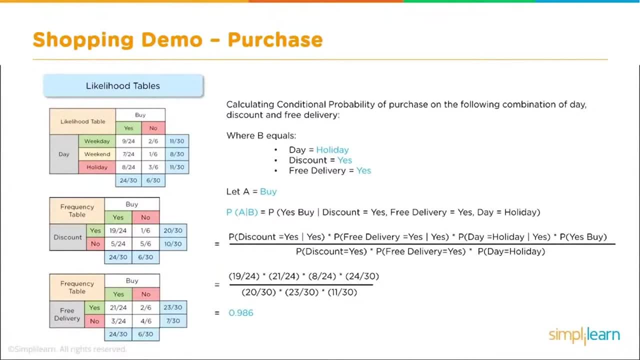 multiplying the three variables out: the full probability of there being a discount, the full probability of it being a free delivery and the full probability of there being a day equal holiday- and that's where we get this: 19 over 24 times 21 over 24. 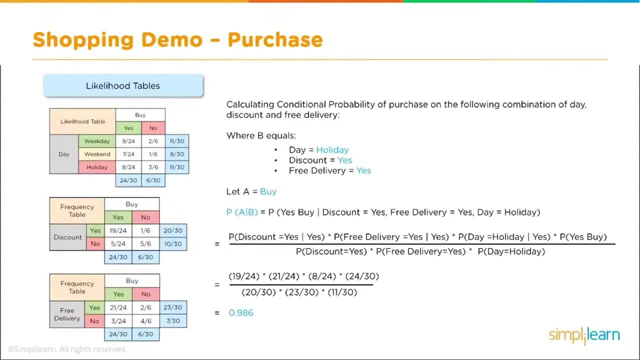 times 8 over 24, times the P of A, 24 over 30 divided by the probability of the discount, the free delivery times the day, or 20 over 30, 23 over 30 times 11 over 30: .986. so what are we going to do with these two pieces of data? 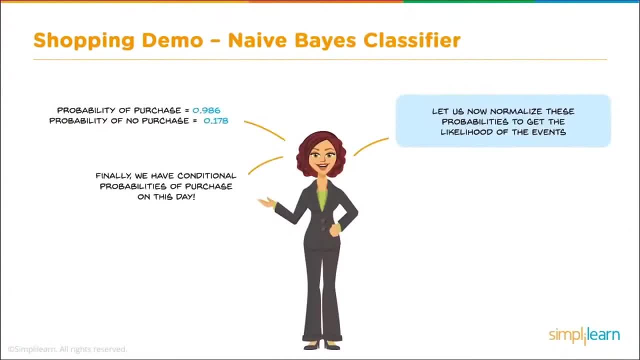 that we've just generated. well, let's go ahead and go over them. we have a probability of purchase- .986. we have a probability of no purchase- 0.178. so, finally, we have conditional probabilities of purchases on this day. lets take that and normalize it, and we are going to take these probabilities. 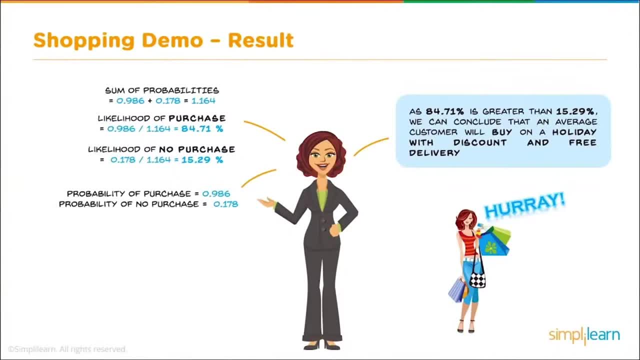 and turn them into percentages. this is simply done by taking the sum of probabilities, which equals 0.98686 178, and that equals the 1.164.. If we divide each probability by the sum, we get the percentage, and so the likelihood of a purchase is 84.71 percent and the likelihood of no purchase is 15.29 percent. 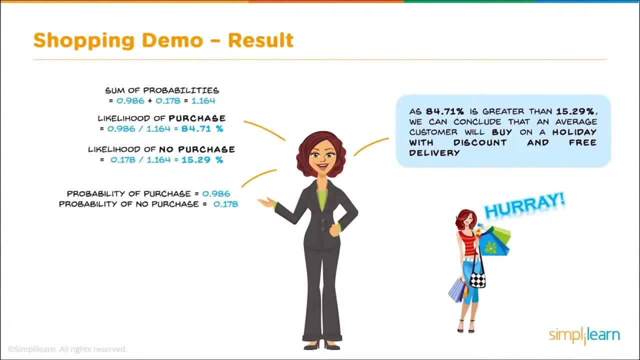 given these three different variables. So if it's on a holiday, if it's with a discount and has free delivery, then there's an 84.71 percent chance that the customer is going to come in and make a purchase. Hooray, They purchased our stuff. We're making money. If you're owning a shop, that's like 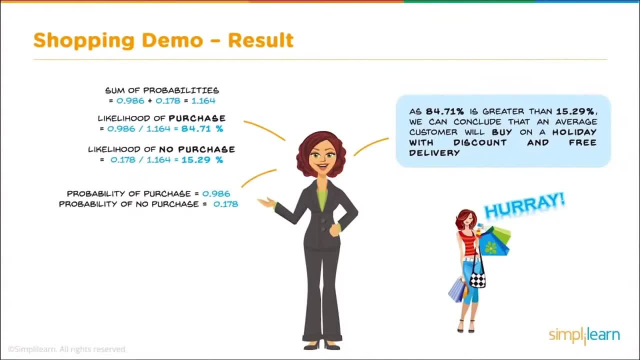 is the bottom line is you want to make some money so you keep your shop open and have a living. Now I promised you that we were going to be finishing up the math here with a few pages, So we're going to move on and we're going to do two steps. The first step is: I want you to understand why you 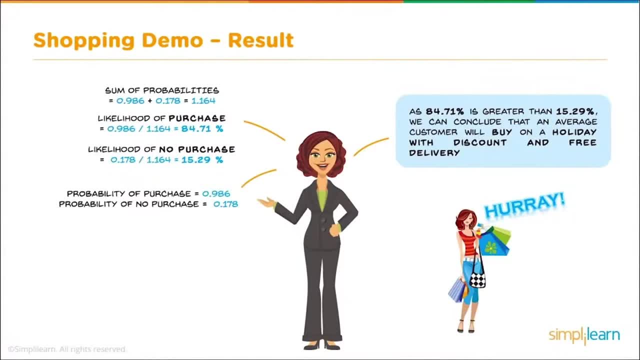 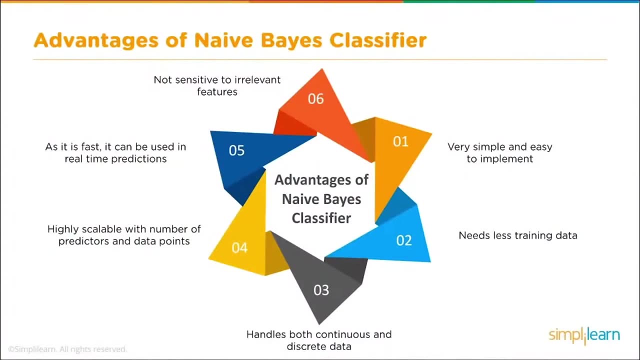 want to use the naive Bayes. What are the advantages of naive Bayes? And then, once we understand those advantages, we'll just look at that briefly. then we're going to dive in and do some Python coding: Advantages of naive Bayes classifier. So let's take a look at the six advantages of the naive Bayes. 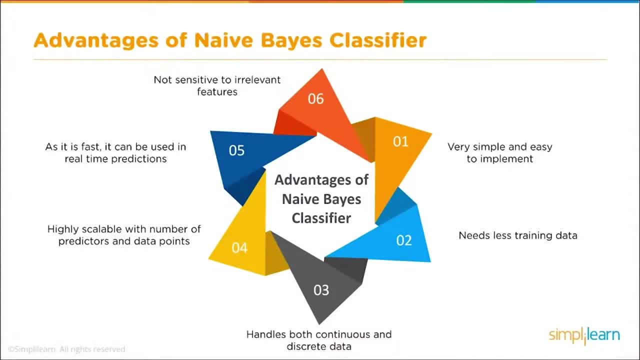 classifier And we're going to walk around this lovely wheel. It looks like an origami folded paper. The first one is very simple and easy to implement. Certainly you could walk through the tables and do this by hand. You got to be a little careful because the notations can get confusing. 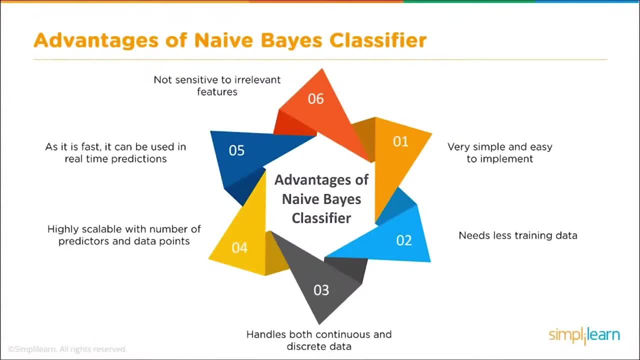 You have all these different probabilities and I certainly mess those up as I put them on. you know, is it on the top or the bottom? You got to really pay close attention to that. When you put it into Python, you're going to have a lot of problems. You're going to have a lot of problems. 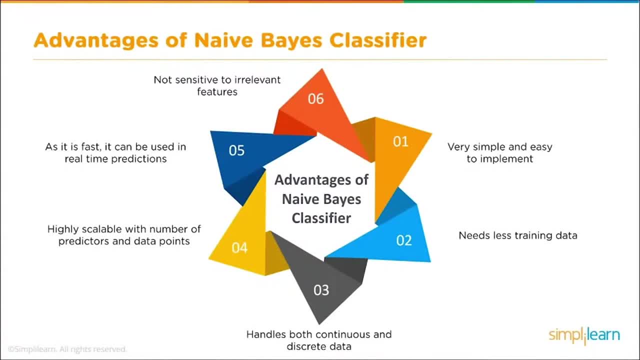 It's really nice because you don't have to worry about any of that. You let the Python handle that, the Python module. But, understanding it, you can put it on a table and you can easily see how it works. And it's a simple algebraic function. It needs less training data. So if you have smaller 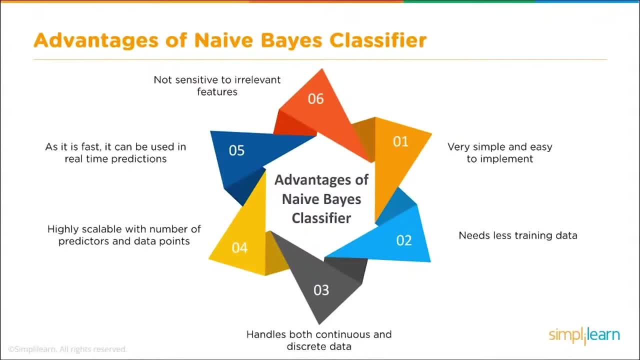 amounts of data. this is great powerful tool for that Handles both continuous and discrete data. It's highly scalable with number of predictors and data points. So, as you can see, you just keep multiplying different probabilities in there and you can cover not just three different variables. 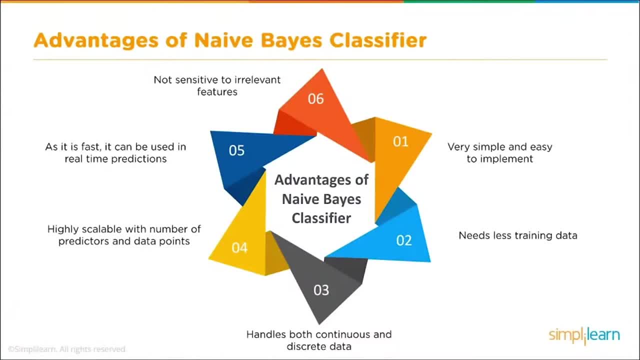 or sets. You can now expand this to even more, So you don't have to worry about any of that. Number five: it's fast. It can be used in real-time predictions. This is so important. This is why it's used in a lot of our predictions on online shopping carts, referrals, spam filters is because 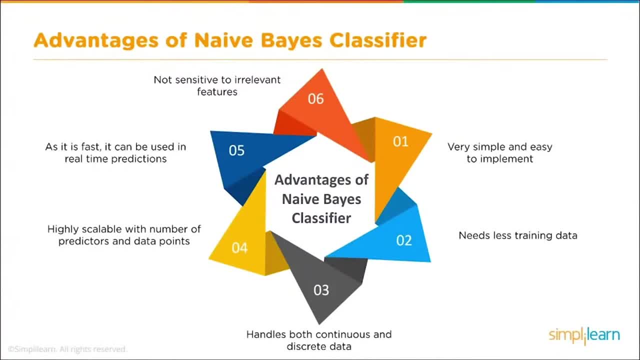 there's no time delay as it has to go through and figure out a neural network or one of the other mini setups where you're doing classification. And certainly there's a lot of other tools out there in the machine learning that can handle these, but most of them are not as fast as the 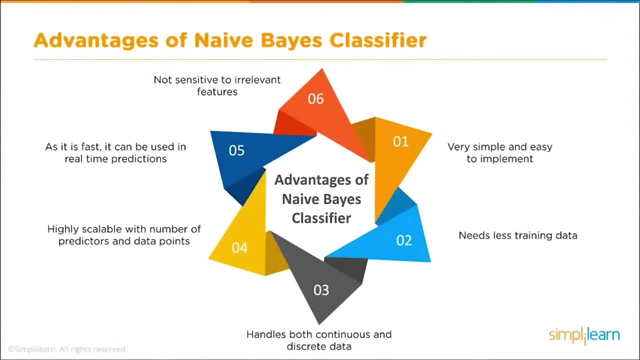 Naive Bayes. And then, finally, it's fast, It can be used in real-time predictions, So you can see that it's not sensitive to irrelevant features. So it picks up on your different probabilities and if you're short on data on one probability you can kind of automatically adjust for that. 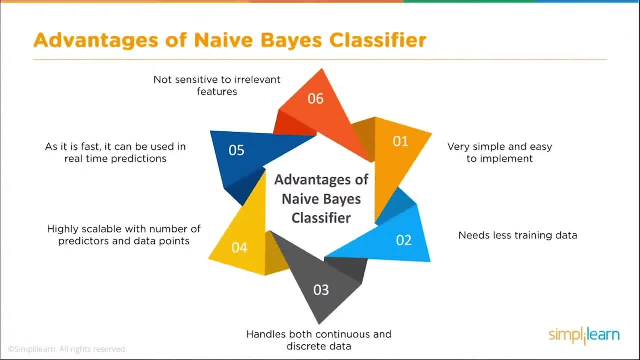 Those formulas are very automatic, and so you can still get a very solid predictability even if you're missing data or you have overlapping data for two completely different areas. We see that a lot in doing census and studying of people and habits, where they might have. 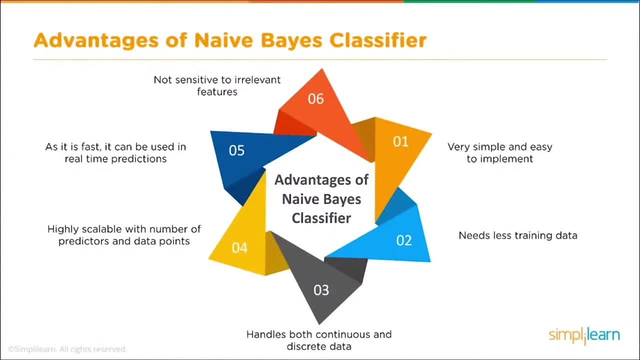 one study that covers one aspect, another one that overlaps, And because the two overlap, they can then predict the unknowns for the group that they haven't done the second study on, or vice versa. So it's very powerful in that it is not sensitive to the irrelevant features and in fact you can use it to help. 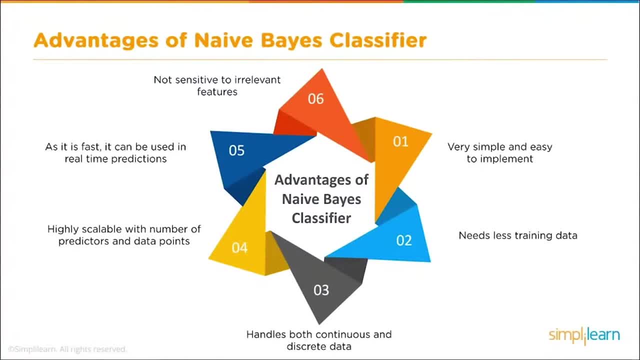 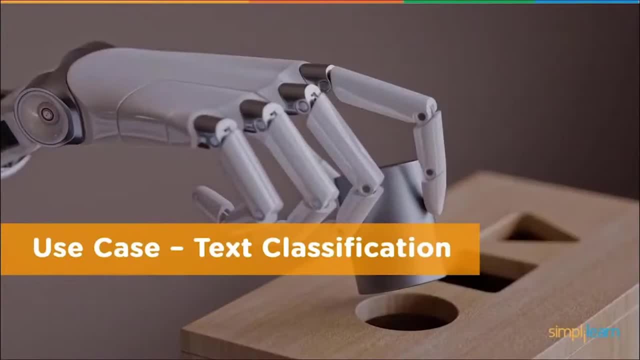 predict features that aren't even in there. So now we're down to my favorite part. We're going to roll up our sleeves and do some actual programming. We're going to do the use case text classification. Now I would challenge you to go back and send us a note on the notes below underneath the video and request the data for the. 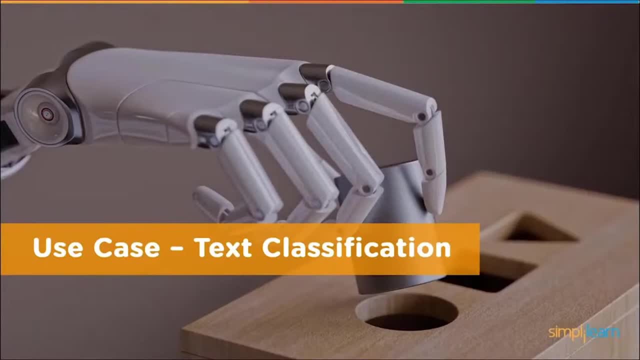 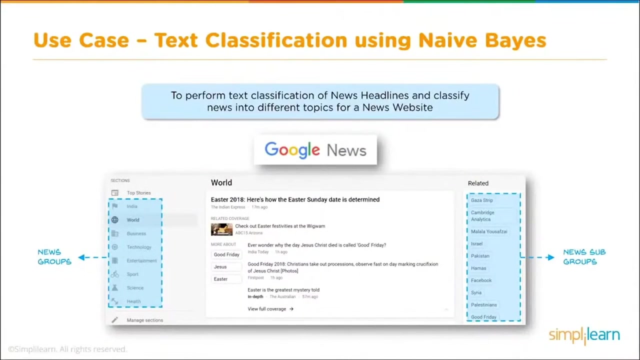 topic there. One of the more loops on webpages is the copying cart, where you can plug data into Python code and do that on your own time so we can walk through it, since we walked through all the information on it. But we're going to do a similar test using Python code doing text classification- very popular for doing the naive react. 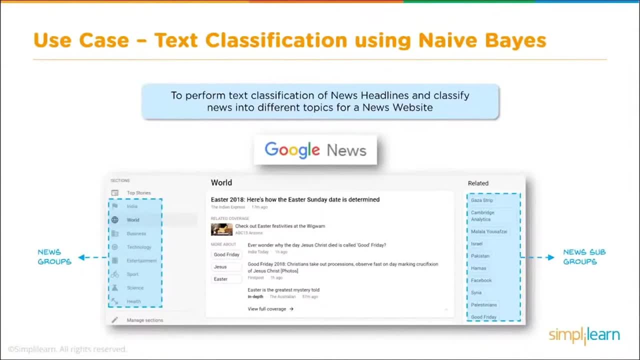 So we're gonna use our new tool to perform a text classification of news headlines and classify news into different topics for our news website. As you can see here we have a nice image of the Google news actual data we're going to use from. It's one of the standard sets, But certainly this can be used. 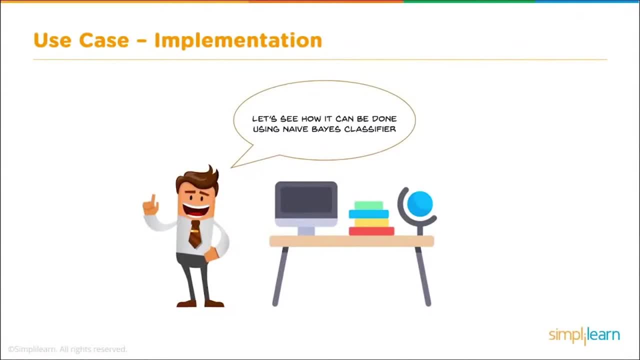 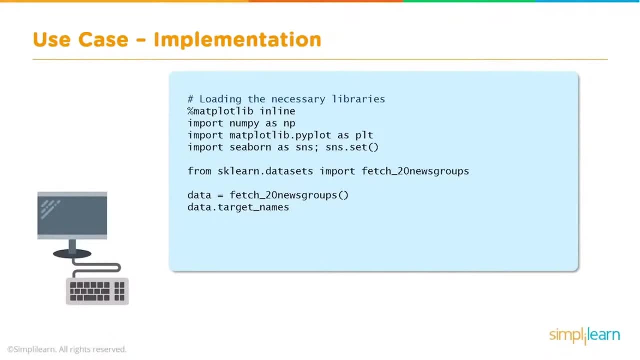 on any of our news headlines and classification. So let's see how it can be done using the Naive Bayes classifier. Now we're at my favorite part. We're actually going to write some Python script, Roll up our sleeves And we're going to start by doing our imports. These are very basic imports. 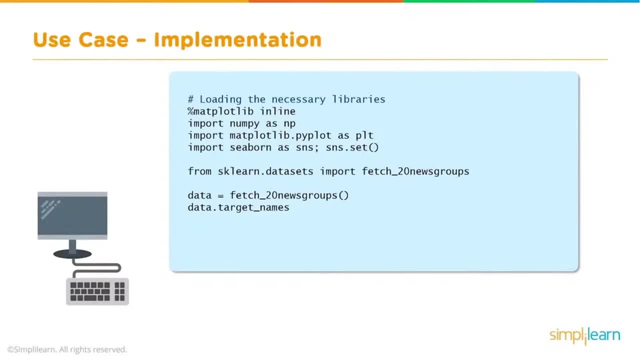 including our news group, And we'll take a quick glance at the target names. Then we're going to go ahead and start training our data set and putting it together. We'll put together a nice graph, because it's always good to have a graph to show what's going on. And once we've trained it, 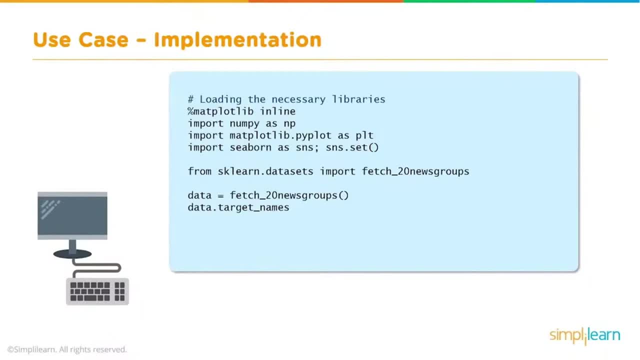 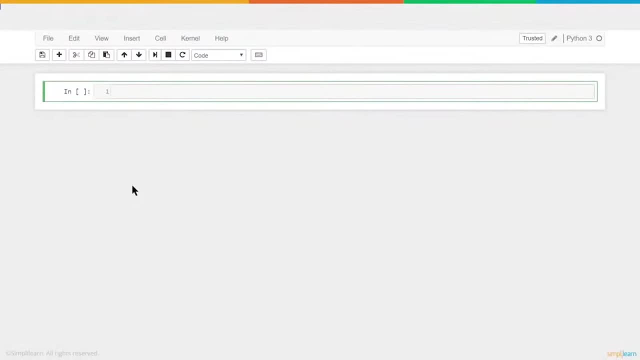 and we've shown you a graph of what's going on. then we're going to explore how to use it and see what that looks like. Now I'm going to open up my favorite editor, or inline editor for Python. You don't have to use this. You can use whatever your editor that you like, Whatever interface IDE you. 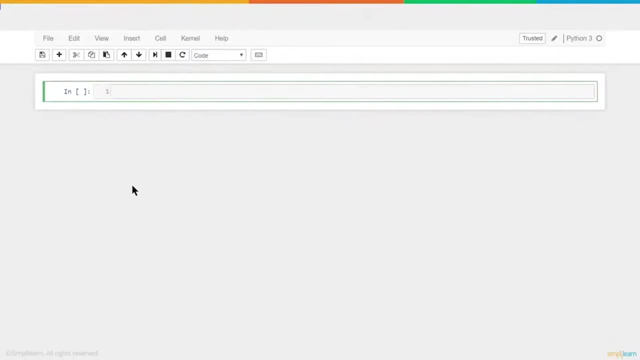 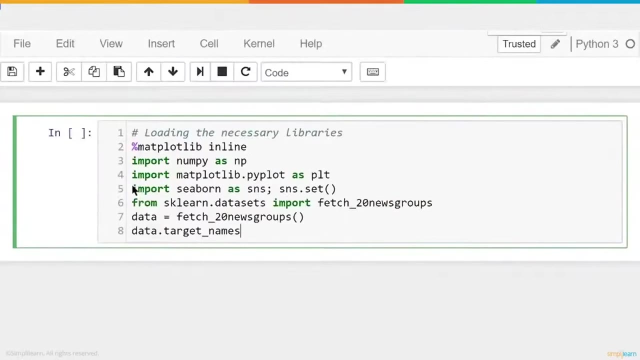 want. This just happens to be the Anaconda Jupyter notebook, And I'm going to paste that first piece of code in here so we can walk through it. Let's make it a little bigger on the screen so you have a nice view of what's going on. 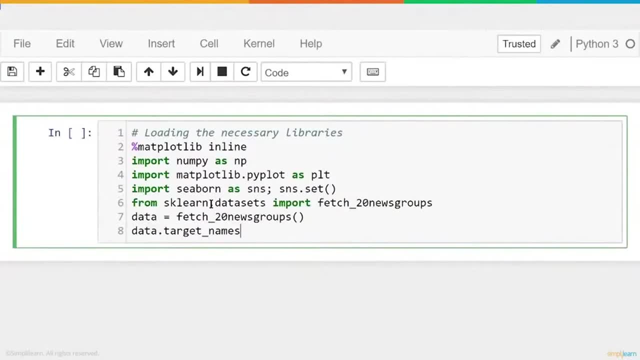 And we're using Python 3, in this case 3.5. So this would work in any of your 3x. If you have it set up correctly, it should also work in a lot of the 2x. You just have to make sure all of the versions of 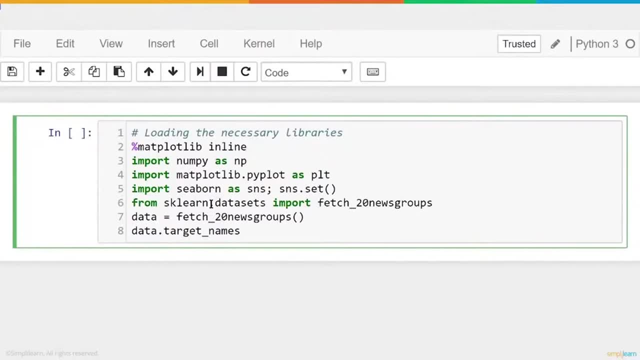 the modules match your Python version And in here you'll notice. the first line is your percentage matplotlibrary inline. Now three of these lines of code are all about plotting the graph. This one lets the notebook know, since this is an inline setup, that we want the graphs to show up. 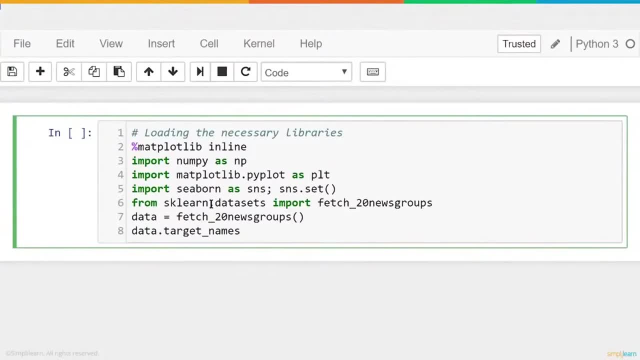 on this page. Without it, in a notebook like this, which is an explorer interface, it won't show up. Now, a lot of IDEs don't require that. A lot of them like if I'm working on one of my other setups. 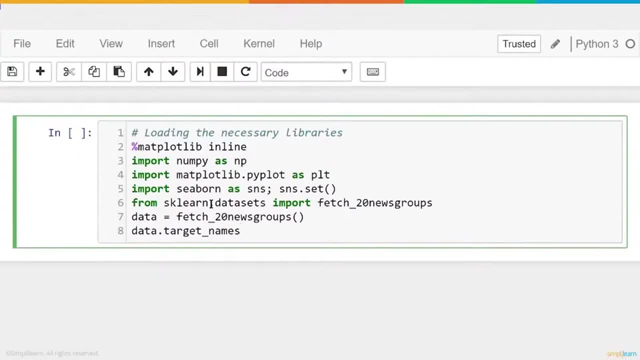 it just has a pop-up and the graph pops up on there. So you have that setup also. But for this we want the matplotlibrary inline, And then we're going to import numpy as np, That's number python, which has a lot of different formulas in it that we use for both of our sklearn module And we also 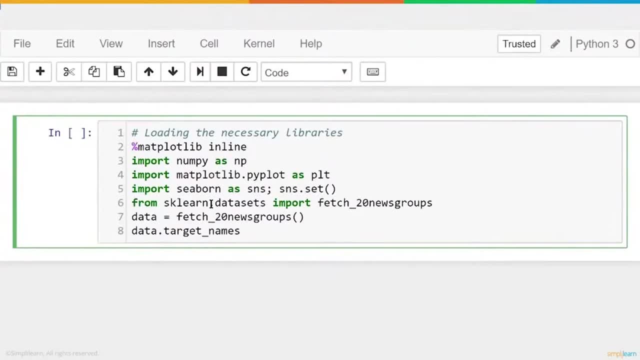 use it for any of the upper math functions in Python And it's very common to see that as np, numpy as np. The next two lines are all about our graphing. Remember I said three of these were about graphing. Well, we need our matplotlibrarypyplot as plt And you'll see that plt is a. 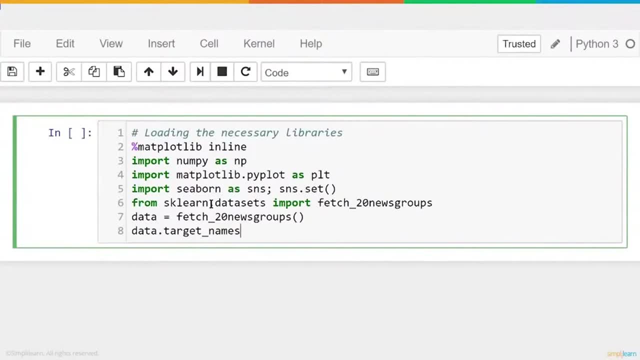 very common setup, as is the sns, and just like the np, And we're going to import sklearn as sns And we're going to do the snsset. Now, sklearn sits on top of pyplot And it just makes a really nice heatmap. It's really good for heatmaps And if you're not familiar with heatmaps, that just means 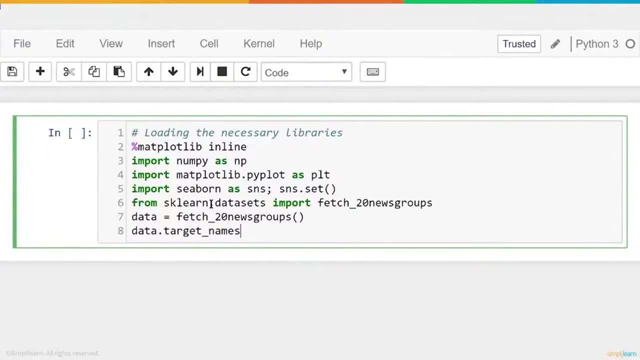 we give it a color scale. The term comes from the brighter red, it is the hotter. it is in some form of data And you can set it to whatever you want And we'll see that later on. So those you'll see. 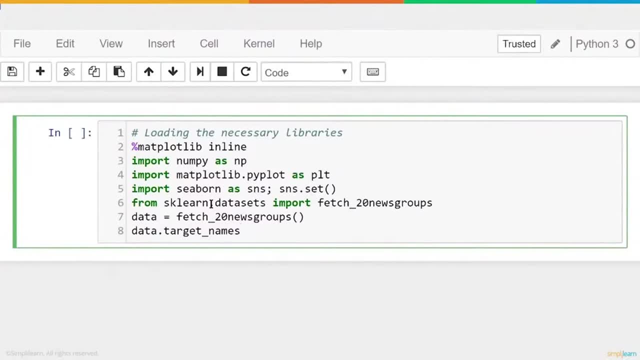 that those three lines of code here are just importing the graph function so we can graph it And as a data scientist, you always want to graph your data and have some kind of visual. It's really hard just to shove numbers in front of people and they look at it and it doesn't mean. 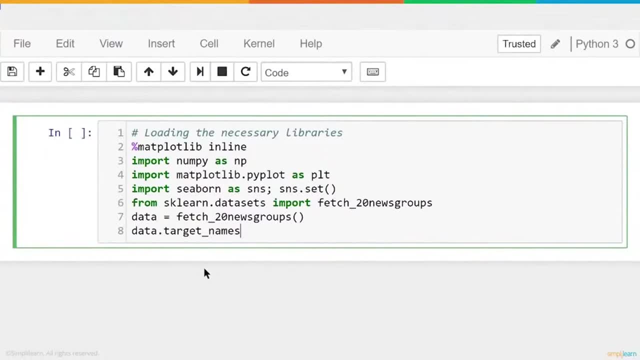 anything. And then from the sklearndatascientist, we're going to import the graph function And we're going to import the fetch20newsgroups- Very common one for analyzing, tokenizing words and setting them up and exploring how the words work and how do you categorize different things when 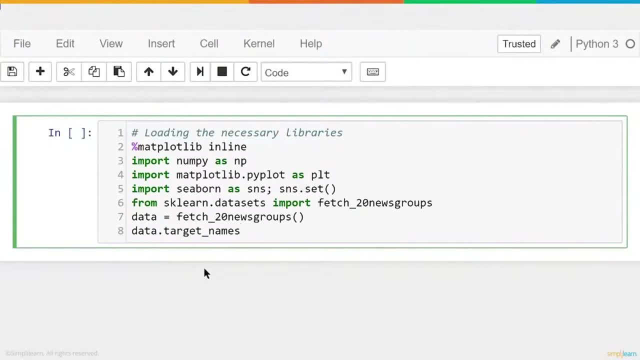 you're dealing with documents And then we set our data equal to fetch20newsgroups, So our data variable will have the data in it And we're going to go ahead and just print the target names- datatargetnames- And let's see what that looks like And you'll see, here we have alt atheism. 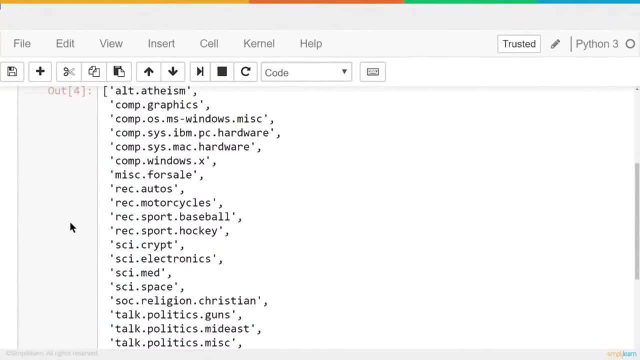 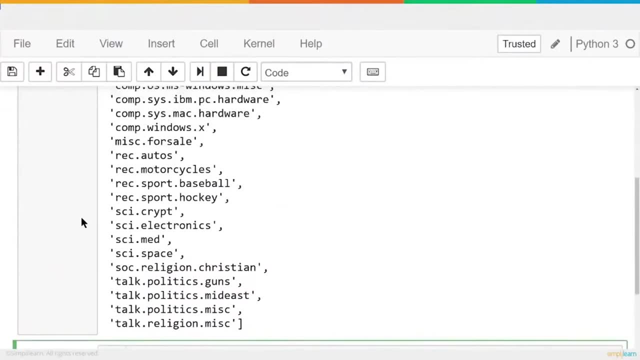 comp graphics, comp os, ms, windowsmiscellaneous. And then we're going to import the fetch20newsgroups And it goes all the way down to talkpoliticsmiscellaneous, talkreligionmiscellaneous. These are the categories they've already assigned to this news group And it's called fetch20. 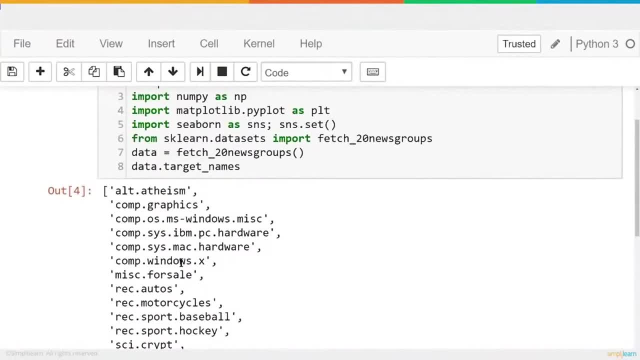 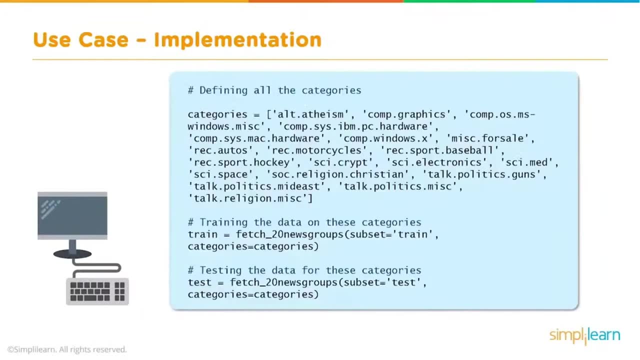 because you'll see, there's- I believe there's- 20 different topics in here, or 20 different categories as we scroll down. Now we've gone through the 20 different categories and we're going to go ahead and start defining all the categories and set up our data. So we're actually 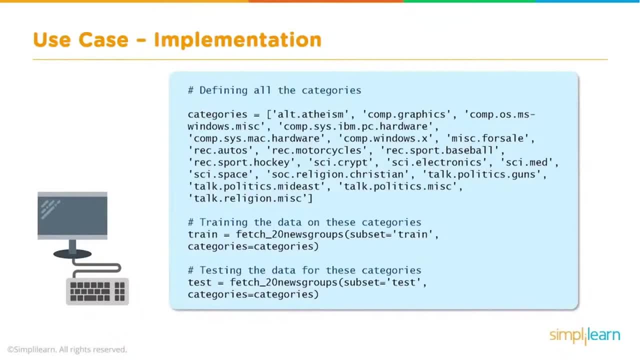 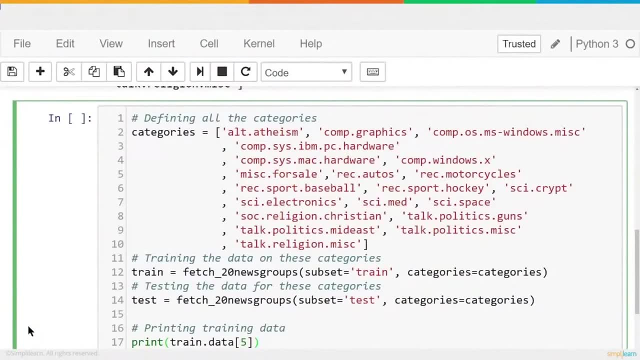 in here, going to go ahead and get the data all set up and take a look at our data And let's move this over to our Jupyter notebook And let's see what this code does. First, we're going to set our categories. Now, if you noticed up here, I could have just as easily set this equal to datatarget. 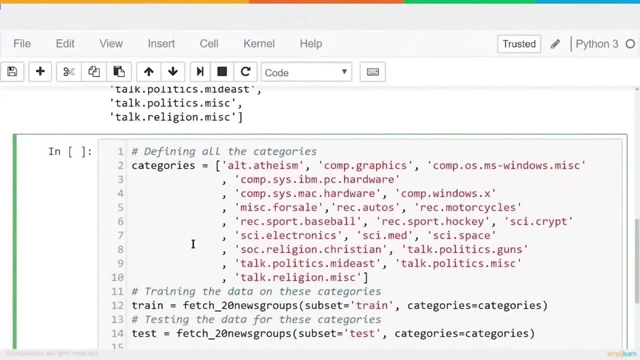 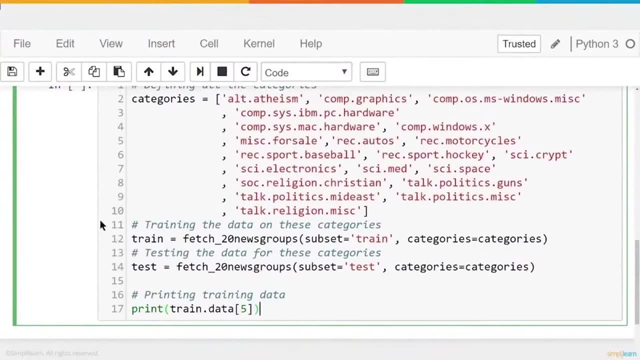 underscore names because it's the same thing, But we want to kind of spell it out for you so you can see the different categories. It kind of makes it more visual so you can see what your data is looking like in the background. Once we've created the categories, we're going to open up a train set. 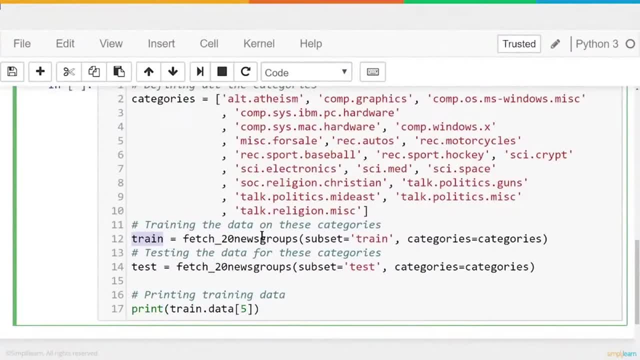 So this training set of data is going to go into the training set of data And we're going to go to fetch 20 news groups And it's a subset in there called train And categories equals categories. So we're pulling out those categories that match And then, if you have a train set, 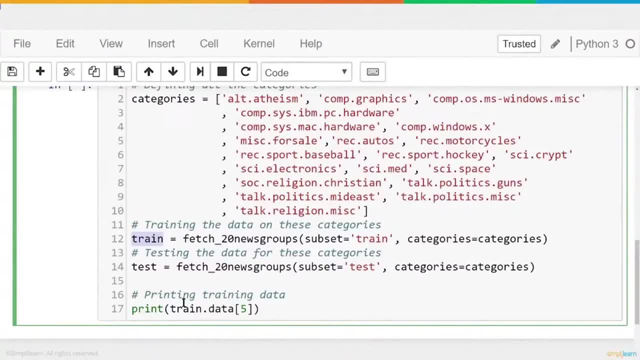 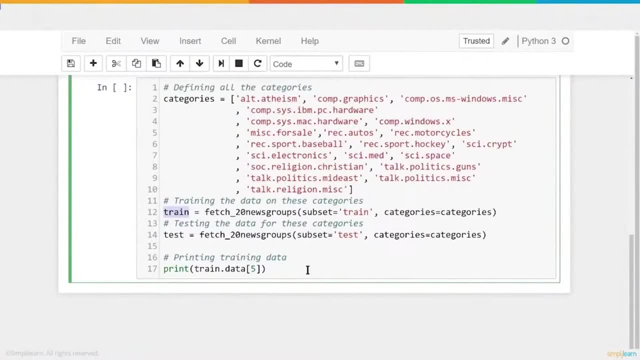 you should also have the testing set. We have test equals fetch, 20 news groups, Subset equals test And categories equals categories. Let's go down one size so it all fits on my screen. There we go, And just so we can really see what's going on, let's see what happens when we print out. 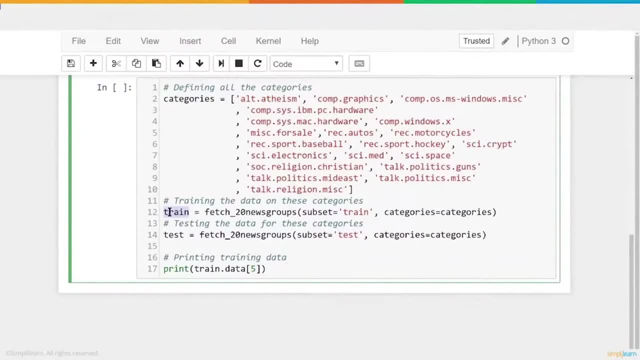 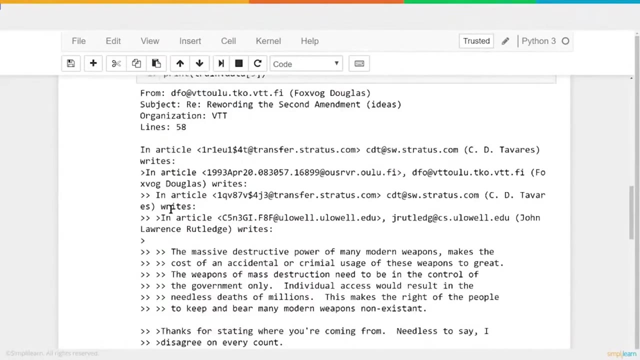 one part of that data. So it creates train And under train it creates train dot data. And we're just going to look at data piece number five And let's go ahead and run that and see what that looks like. And you can see, when I print train dot data number five under train, it prints out. 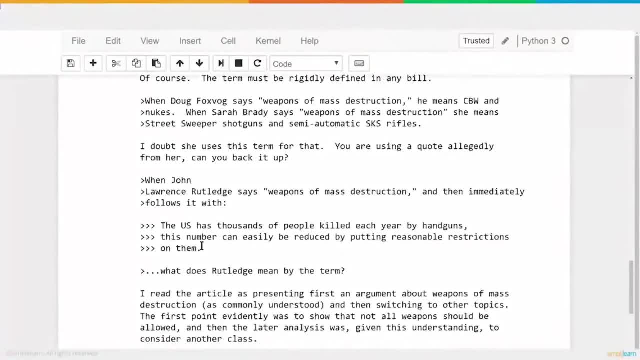 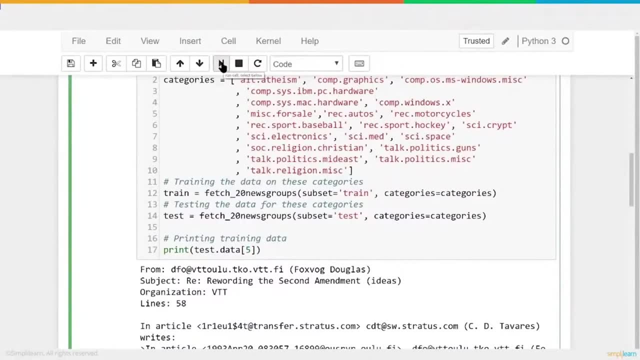 one of the articles. This is article number five. You can go through and read it on there And we can also go in here and change this to test, which should look identical because it's splitting the data up into different groups: train and test And we'll see test. number five is a different article. 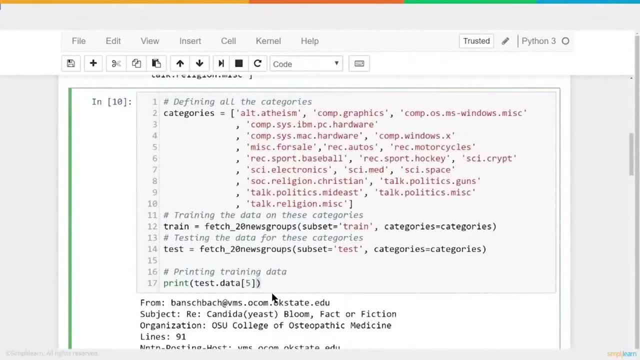 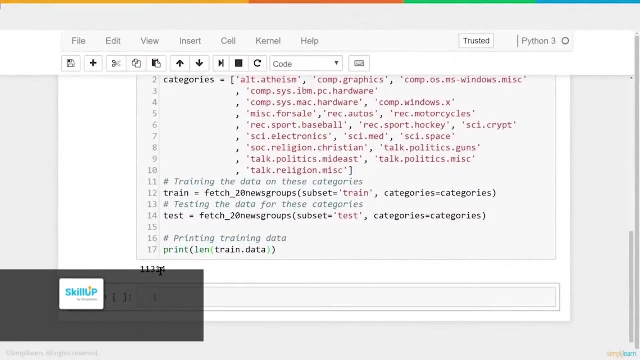 but it's another article in here And maybe you're curious and you want to see just how many articles are in here. We could do length of train dot data And if we run that you'll see that the training data has 11,314 articles. So we're not going to go through all. 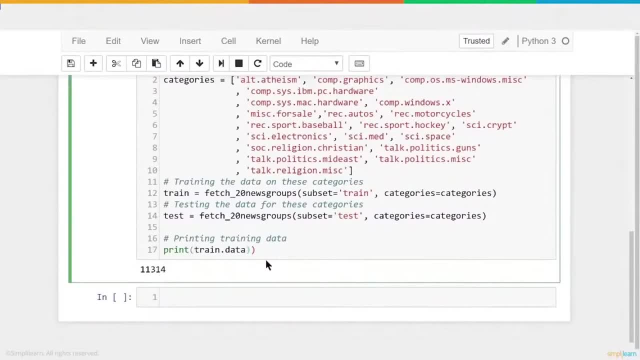 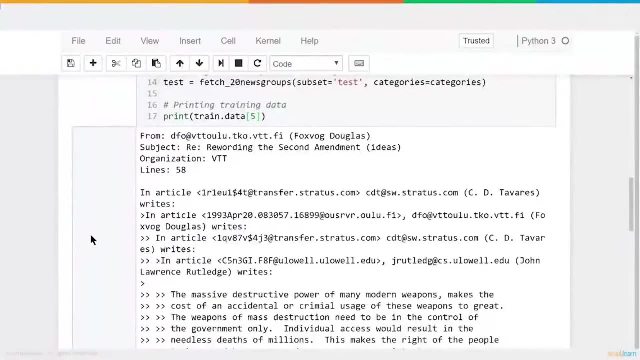 those articles. That's a lot of articles, But we can look at one of them just so you can see what kind of information is coming out of it and what we're looking at. And we'll just look at number five for today. And here we have it, rewording the second amendment: IDs VTT, line 58, lines 58 in. 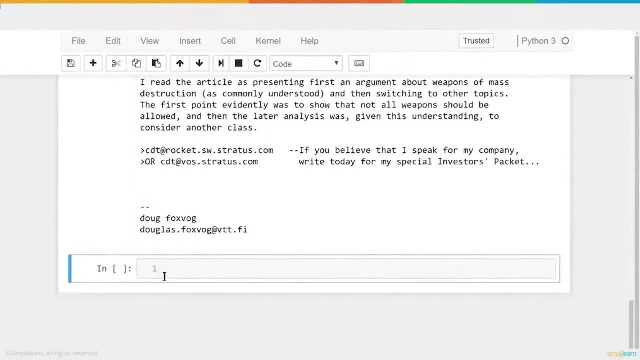 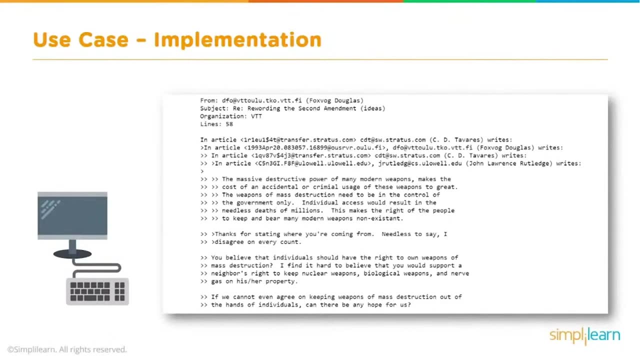 the middle, et cetera. You can scroll all the way down and see all the different parts to there. Now, we've looked at it and that's pretty complicated when you look at one of these articles to try to figure out how do you weight this. If you look down here we have different. 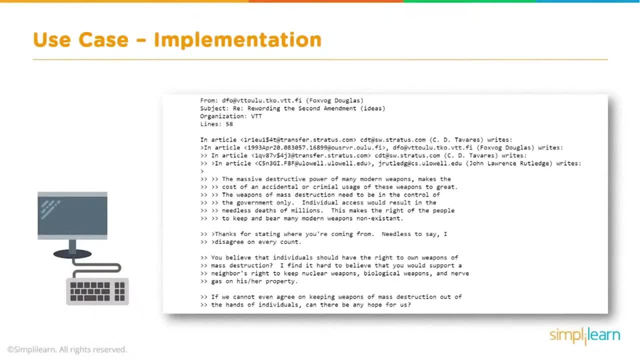 words and maybe the word from- Well, from- is probably in all the articles, so it's not going to have a lot of meaning as far as trying to figure out whether this article fits one of the categories or not. So trying to figure out which category it fits in based on these words is where 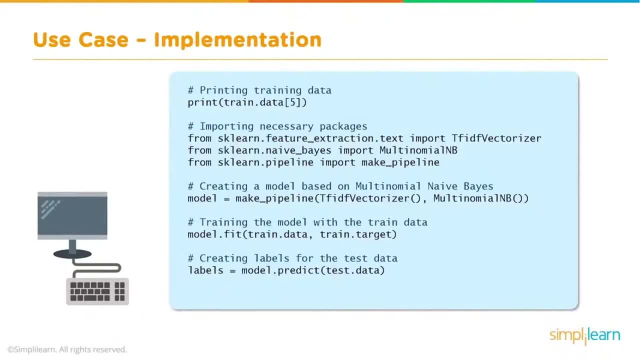 the challenge comes in Now that we've viewed our data. we're going to dive in and do the actual predictions. This is the actual naive base And we're going to throw another model at you or another module at you here in just a second. We can't go into too much detail, but it deals. 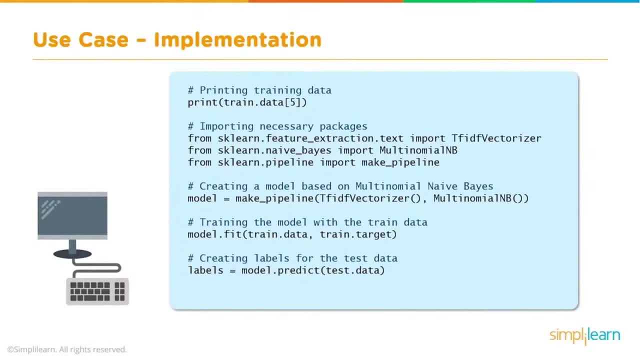 specifically working with words and text and what they call tokenizing those words. So let's take this code and let's skip on over to our Jupyter notebook and walk through it. And here we are in our Jupyter notebook. Let's paste that in there And I can run this code right off the bat. It's: 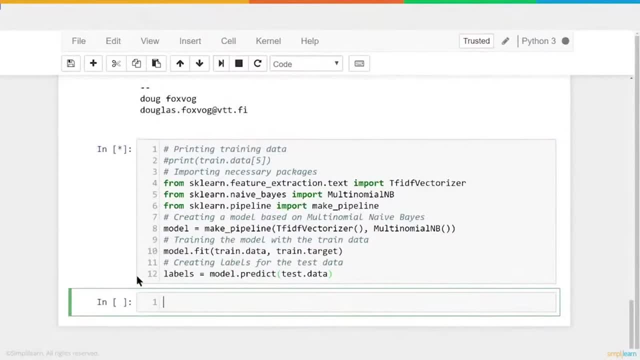 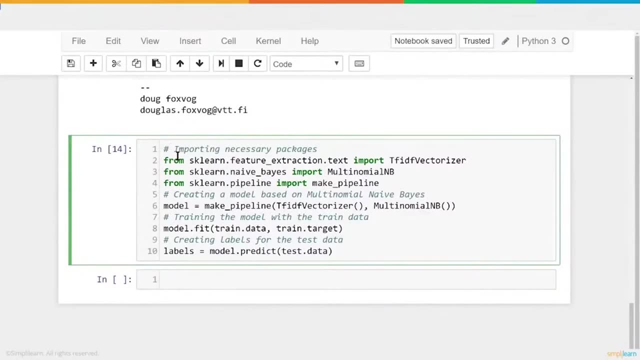 not actually going to display anything yet, but it has a lot going on. in here We have the print module from the earlier one. I didn't know why that was in there. So we're going to start by importing our necessary packages And from the sklearnfeaturesextractiontxt. 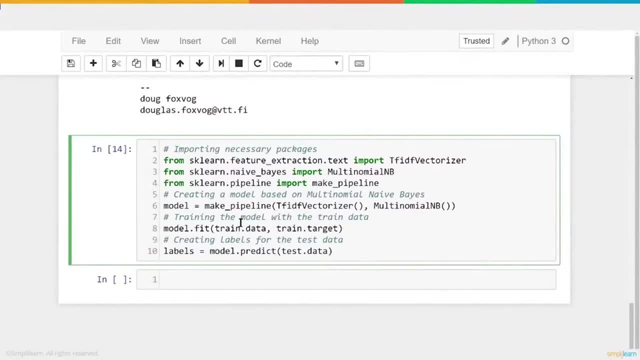 we're going to import tfidfvectorizer. I told you we're going to throw a module at you. We can't go too much into the math behind this or how it works. You can look it up. The notation for the math is: 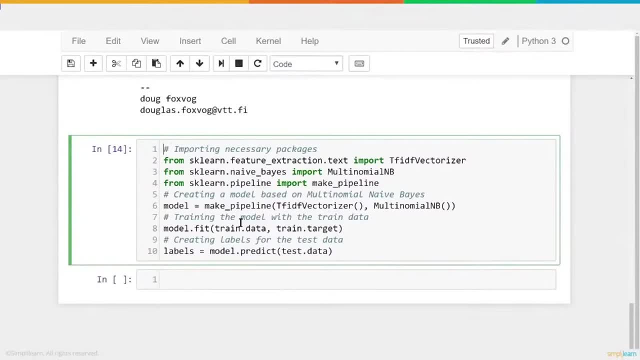 usually tfidf, And that's just a way of weighing the words. And it weighs the words based on how many times you're going to have to write the words. And that's just a way of weighing the words. And it's a well-used formula. It's been around for a while. It's a little confusing to put this in. 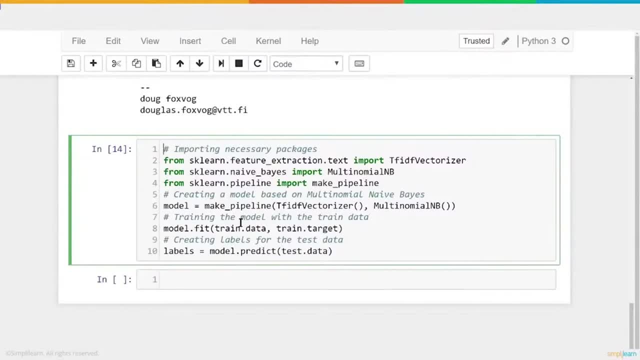 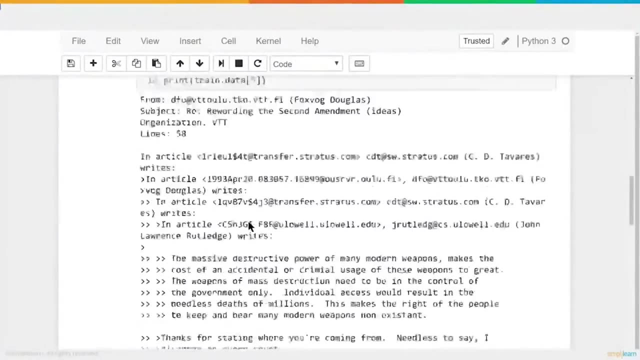 here, But let's let her know that it just goes in there and weights the different words in the document for us. That way we don't have to wait And if you put a weight on it- if you remember I was talking about that up here earlier- If these are all emails, they probably all have. 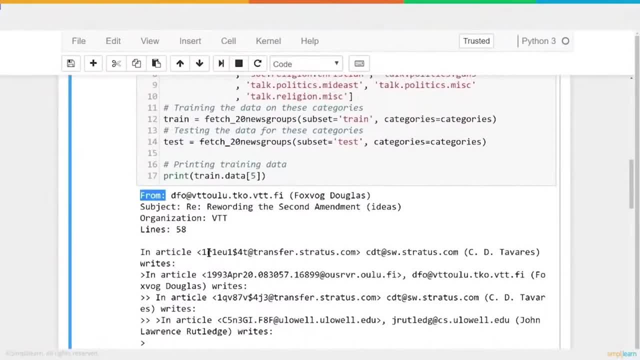 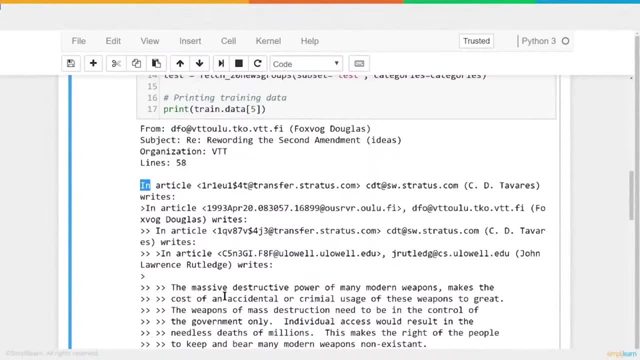 the word from, in them, From probably has a very low weight. It has very little value in telling you what this document's about. Same with words like in an article, in articles in cost of, on, maybe cost might, or where words like criminal. 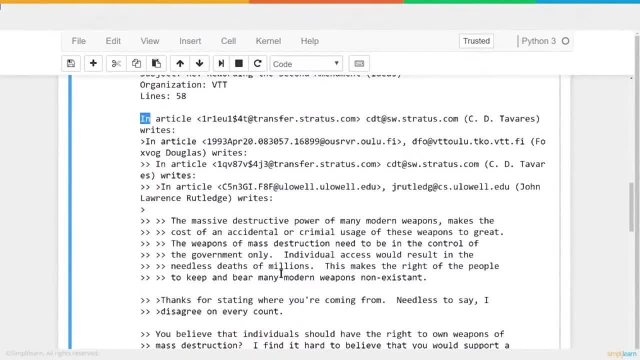 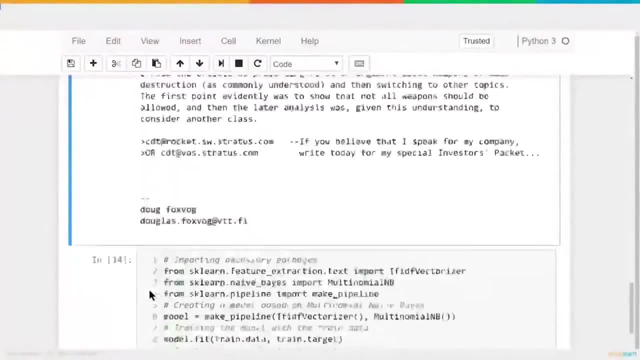 weapons destruction. these might have a heavier weight because they describe a little bit more what the article's doing. Well, how do you figure out all those weights in the different articles? That's what this module does. That's what the tfidf vectorizer is going to do for us. And then 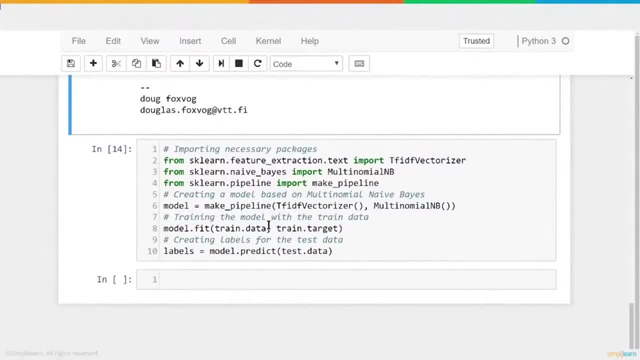 we're going to import our sklearnnaivebase And that's our multinomial NB, multinomial naive base, which is a very easy to understand that where that comes from. And then, finally, we have the sklearn pipeline, import make pipeline. Now, the make pipeline is just a cool piece of code because 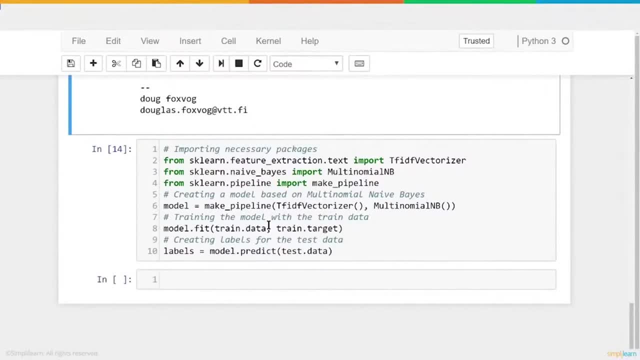 we're going to take the information we get from the tfidf vectorizer and we're going to pump that into the multinomial NB. So a pipeline is just a way of organizing how things flow. It's used commonly. You probably already guessed what it is If you've done any businesses. they talk about the. 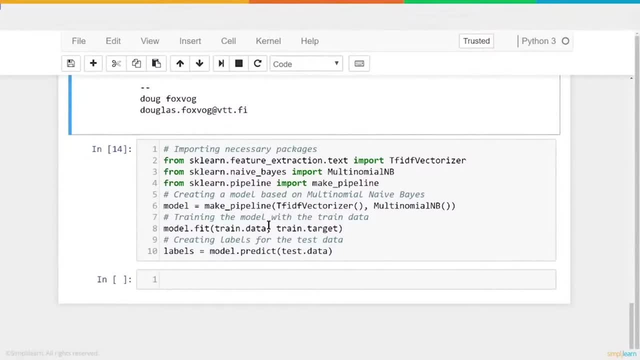 sales pipeline. If you're on a work crew or project manager, you have your pipeline of information that's going through or your projects and what has to be done in what order That's all this pipeline is. We're going to take the tfidf vectorizer and then we're going to push that into the multinomial NB Now. 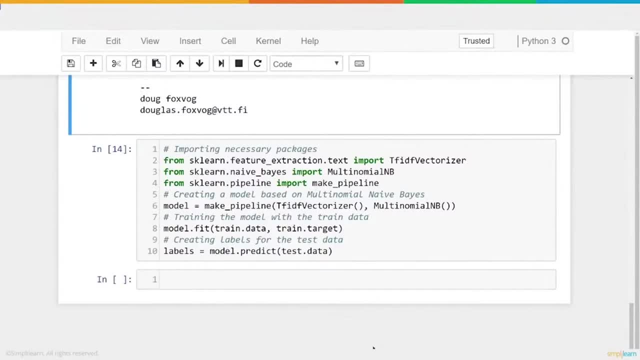 we've designated that as the variable model. We have our pipeline model And we're going to take that model. And this is just so elegant. This is done in just a couple lines of code: Modelfit, And we're going to fit the data. 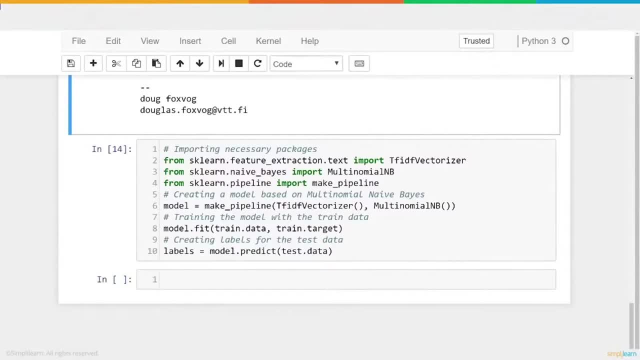 And first we're going to take the model. And we're going to take the model And we're going to first the train data and then the train target. Now the train data has the different articles in it. You can see the one we were just looking at And the traintarget is what category they already 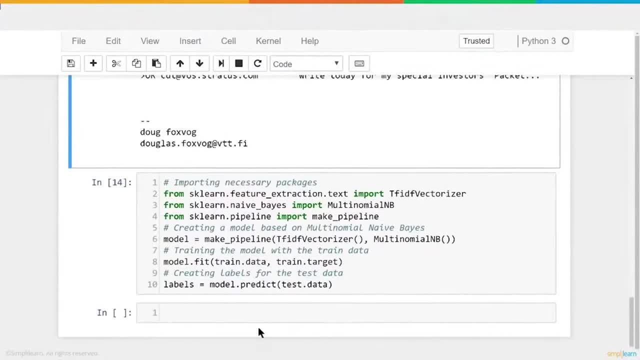 categorized that particular article as: And what's happening here is the train data is going into the tfid vectorizer, So when you have one of these articles, it goes in there. It weights all the words in there. So there's thousands of words with different weights on them. I remember once running 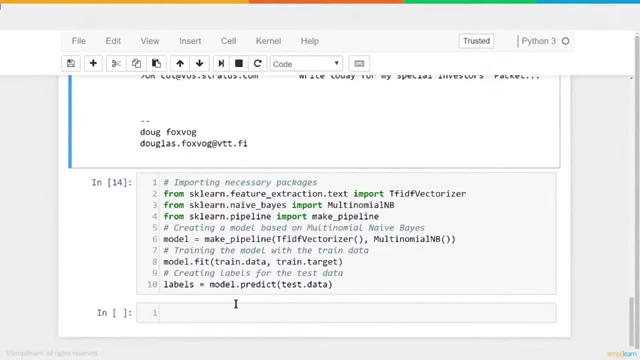 a model on this And I literally had 2.4 million tokens go into this. So when you're dealing with large document bases, you can have a huge number of different words. It then takes those words, gives them a weight And then, based on that weight, based on the words and the weights, it then puts that into. 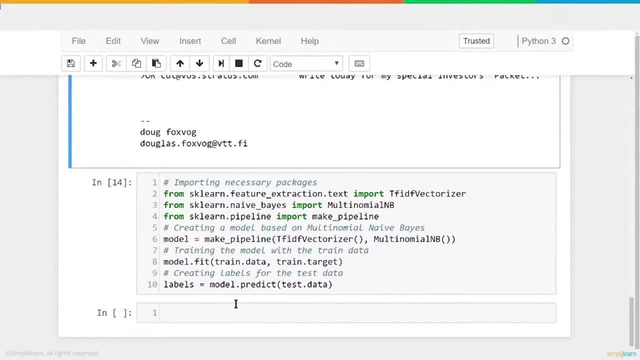 the multinomial NB And once we go into our naive base, we want to put the train target in there. So the train data that's been mapped to the tfid vectorizer is now going through the multinomial NB, And then we're telling it: well, these are the answers. These are the answers to the different. 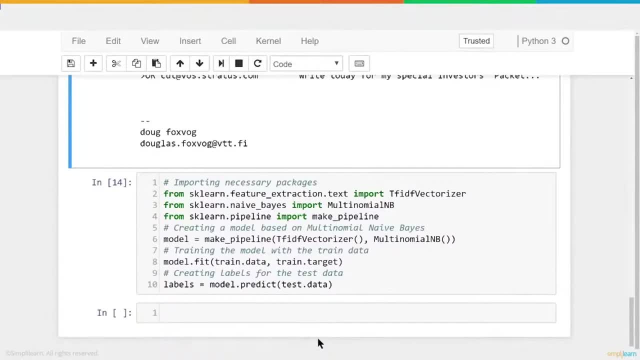 documents. So this document that has all these words with these different weights from the first part is going to be- whatever category it comes out of- Maybe it's the talk show or the article on religion- miscellaneous. Once we fit that model, we can then take labels And we're going to set. 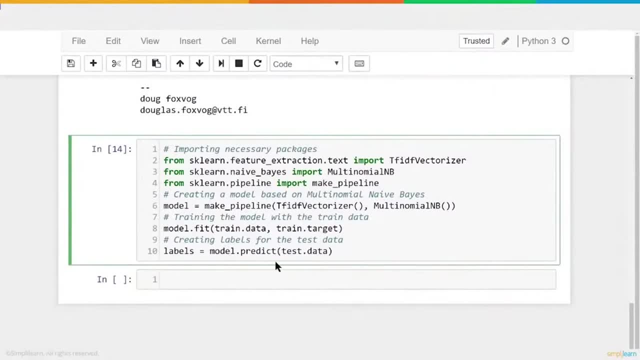 that equal to modelpredict. Most of the sklearn use the term predict to let us know that we've now trained the model And now we want to get some answers And we're going to put our test data in there, because our test data is the stuff we held off to the side. We didn't train it on there. 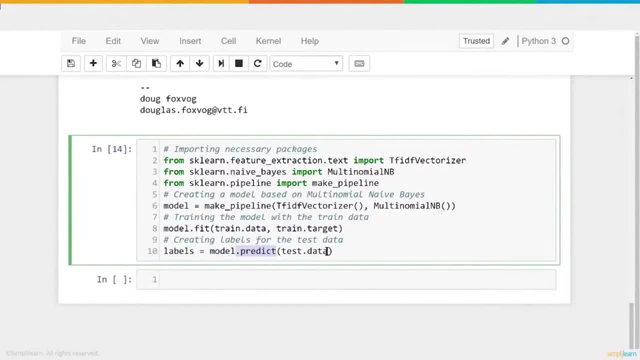 and we don't know what's going to come up out of it, And we just want to find out how good our labels are. Do they match what they should be? Now, I've already run this through. There's no actual output to it to show. This is just setting it all up. This is just training our 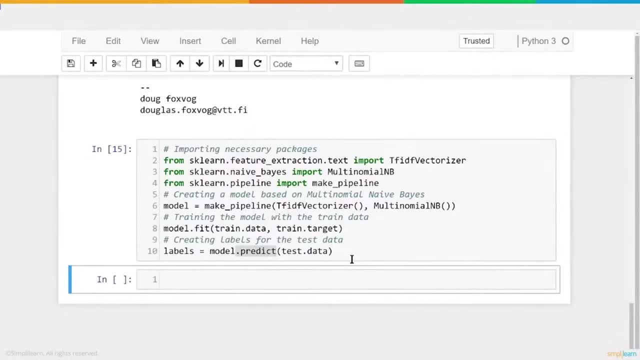 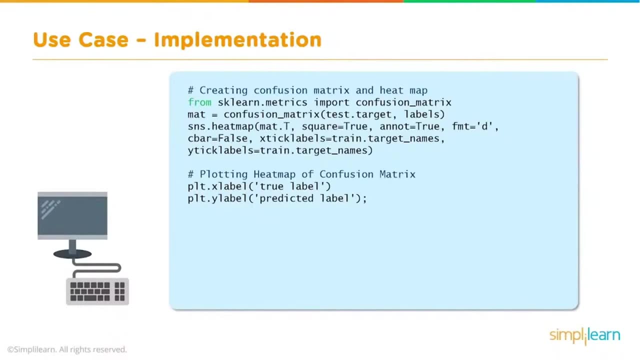 model, creating the labels, so we can see how good it is. And then we move on to the next step, to find out what happened. To do this, we're going to go ahead and create a confusion matrix and a heat map. So the confusion matrix, which is confusing just by its very name. 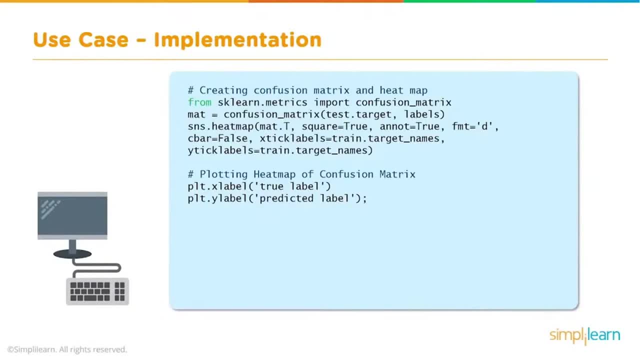 is basically going to ask: how confused is our answer? Did it get it correct Or did it miss some things in there or have some missed labels? And then we're going to put that on a heat map, so we'll have some nice colors to look at to see how that plots out. Let's go ahead and take this. 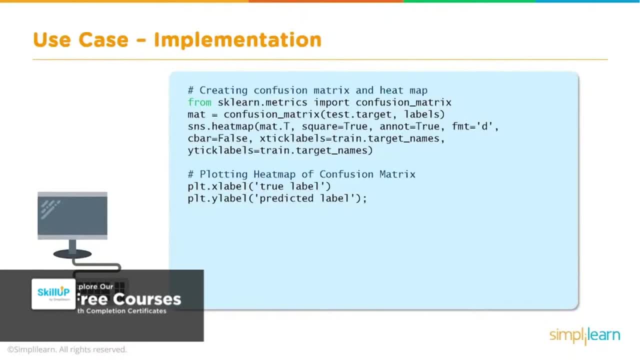 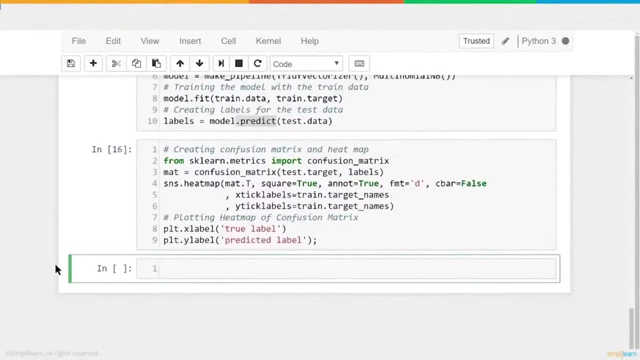 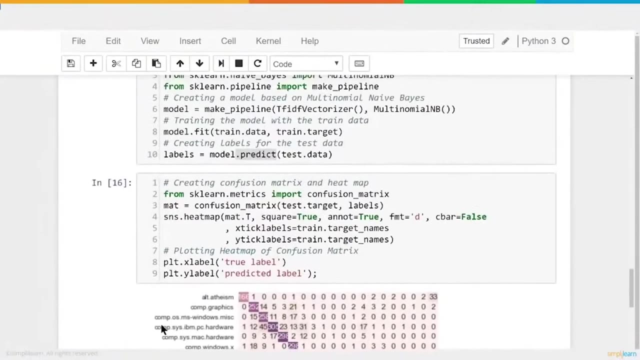 code and take a walk through it and see what that looks like. So back to our Jupyter notebook. go ahead and run that code. Take it just a moment And remember we had the inline. That way my graph shows up on the inline here And let's walk through the code and then we'll look at this. 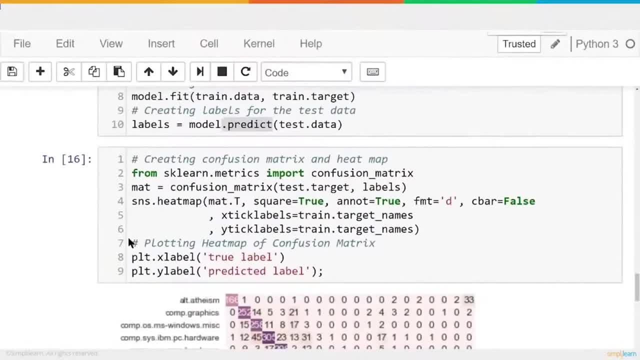 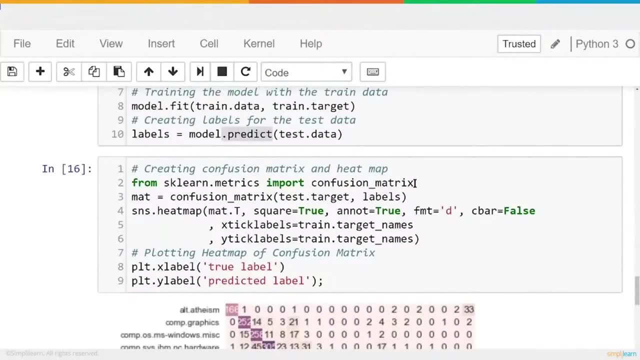 and see what that means. So make it a little bit bigger. There we go. No reason not to use the whole screen Too big. So we have here from sklearnmetrics import confusion matrix And that's just going to generate a set of data that says the prediction was such the actual truth was. 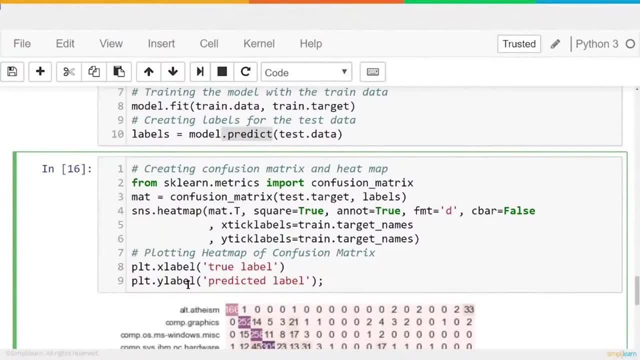 either agreed with it or is something different. And it's going to add up those numbers so we can take a look and just see how well it worked. And we're going to set a variable mat equal to confusion matrix. We have our test target, our test data. that was not part of the training. 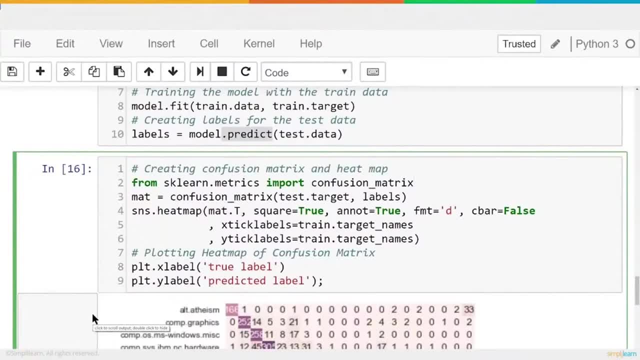 Very important in data science. we always keep our test data separate, Otherwise it's not a valid model if we can't properly test it with new data. And this is the labels we created from that test data. These are the ones that we predict it's going to be. So we go in and we create our SN. 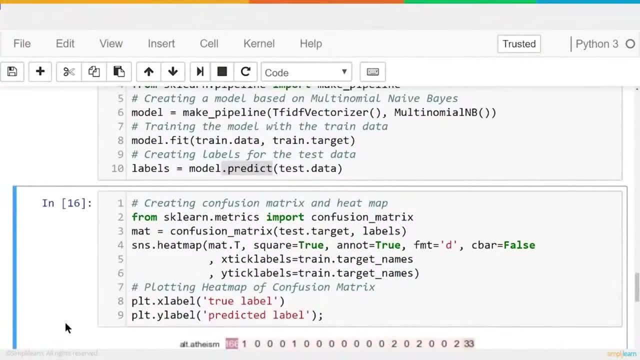 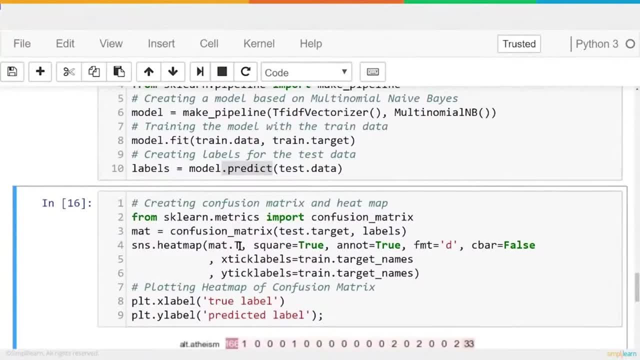 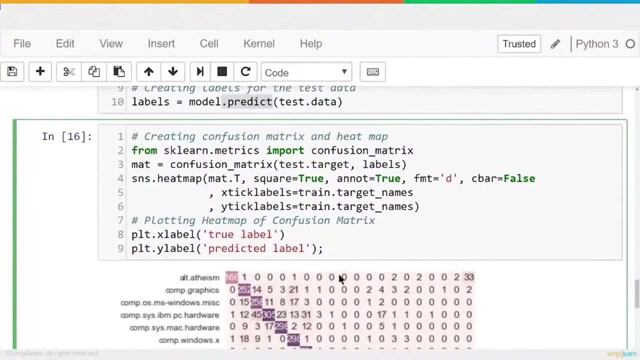 So we create a SNS dot heat map. we take our confusion matrix and it's going to be Matt dot t, And do we have other variables that go into the SNS dot heat map? We're not going to go into detail what all the variables mean. the annotation equals true. that's what tells it to put the numbers here. 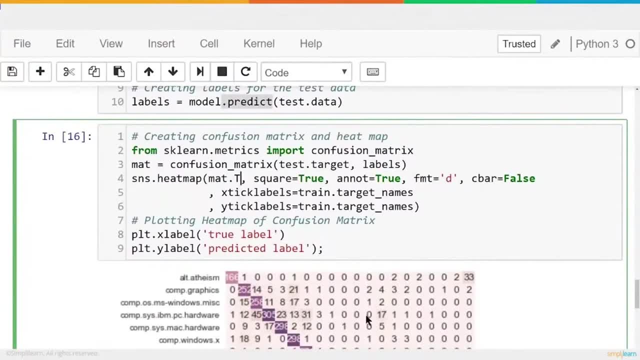 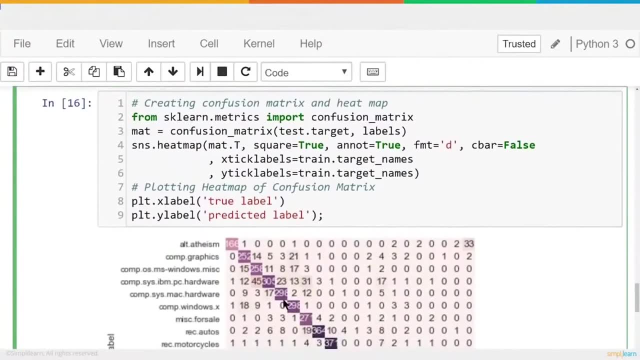 So you have the 166, the one the 0001, format d and c bar equals false, have to do with the format. if you take those out you'll see that some things disappear. and then the X tick labels and the Y tick labels. those are our target names and you can. 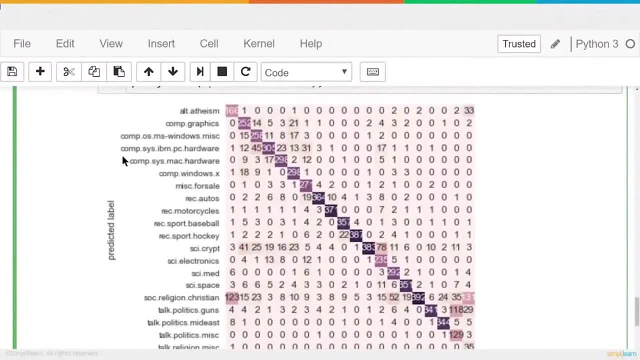 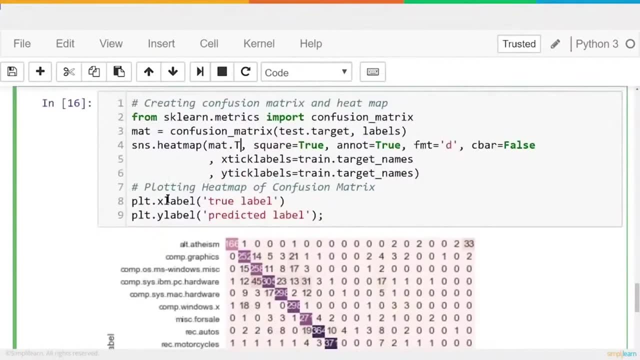 see right here, that's the alt atheism comp, graphics, comp, OSMS, windows, dot, miscellaneous. and then, finally, we have our PLT dot X label. remember the SNS or the seaborn sits on top of our matplotlib, our PLT, and so we want to just tell it: X label equals a true, is is true, the labels are true. and then the Y. 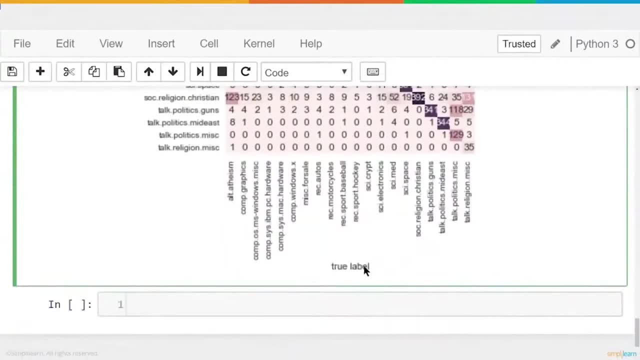 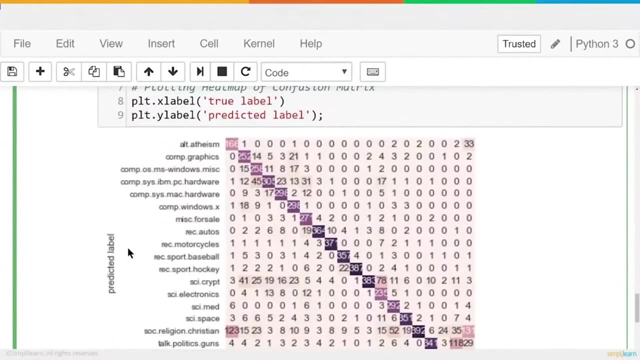 label is prediction label, so we say a true, this is what it actually is, and the prediction is what we predicted. and let's look at this graph, because that's probably a little confusing the way we rattled through it, and what I'm gonna do is I'm gonna go ahead and flip back to the slides, because they have a black. 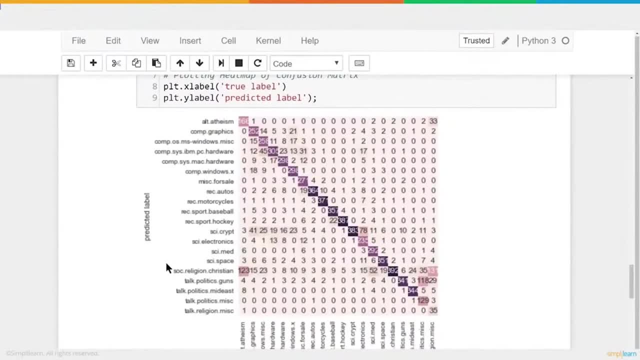 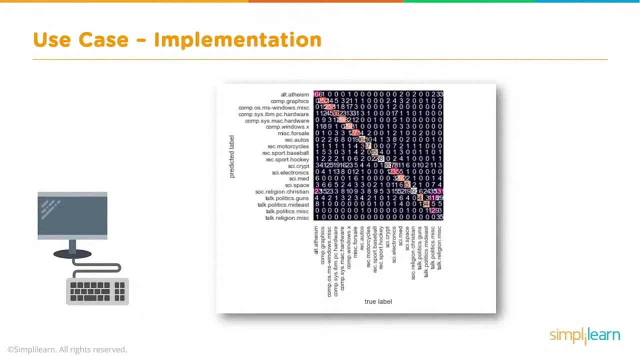 background they put in there. that helps it shine a little bit better, so you can see the graph a little bit easier. so in reading this graph, what we want to look at is how the color scheme has come out, and you'll see a line right down the 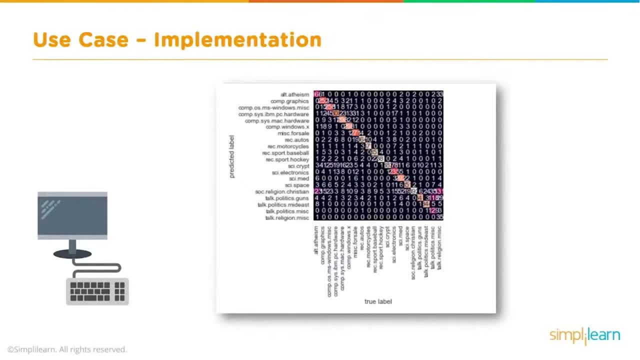 middle, diagonally from upper left to bottom right. what that is is, if you look at the labels, we have our predicted label on the left and our true label on the right. those are the numbers where the prediction and the true come together, and this is what we want to see, is we want to see those lit up. that's what. 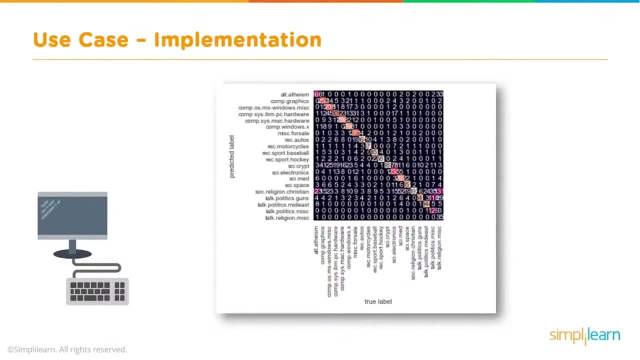 that heatmap does is. you can see that it did a good job of finding those data and you'll notice that there's a couple of red spots on there where it missed. you know it's a little confused. we talk about talk religion- miscellaneous- versus talk politics- miscellaneous. 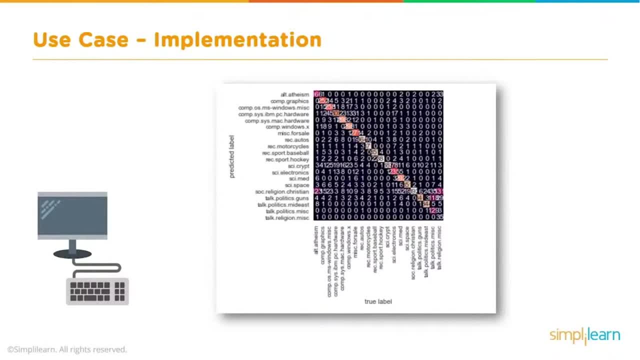 social religion, Christian versus alt atheism. it mislabeled some of those, and those are very similar topics. you could understand why it might mislabel them, but overall, it did a pretty good job. if we're gonna create these models, we want to go ahead and be able to use them, so let's see what that looks like to do. 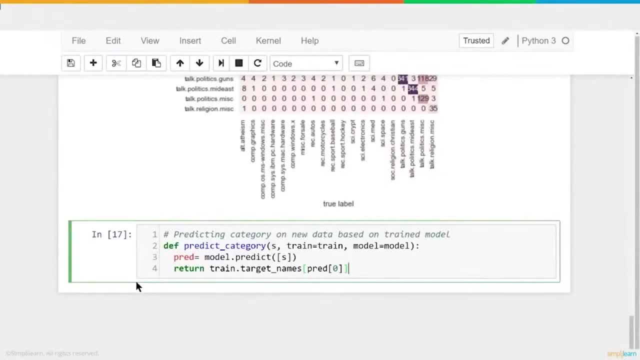 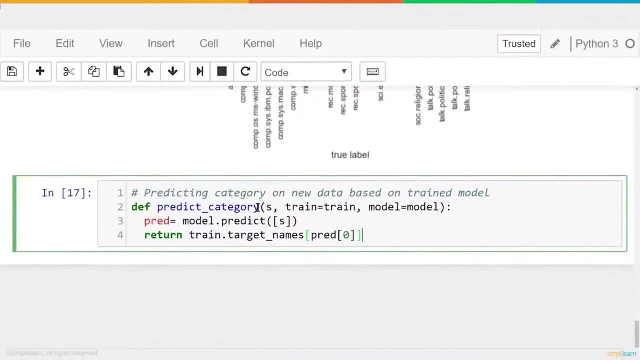 this: let's go ahead and create a definition, a function to run, and we're going to call this function. let me just expand that just a notch here. there we go. I like mine, in big letters: predict categories. we want to predict the category, to send it s a string, and then we're sending it. train equals train. we have our training model and 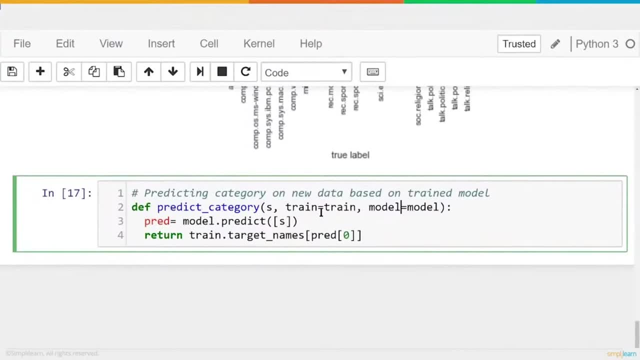 then we had our pipeline model equals model. this way we don't have to resend these variables each time. the definition knows that, because i said train equals train and i put the equal for model and then we're going to set the prediction equal to the model. dot predict s, so it's going to send. 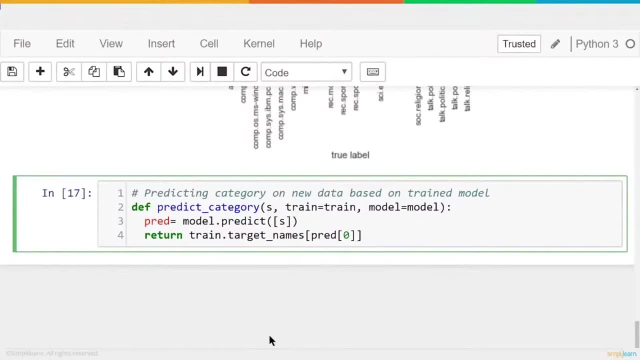 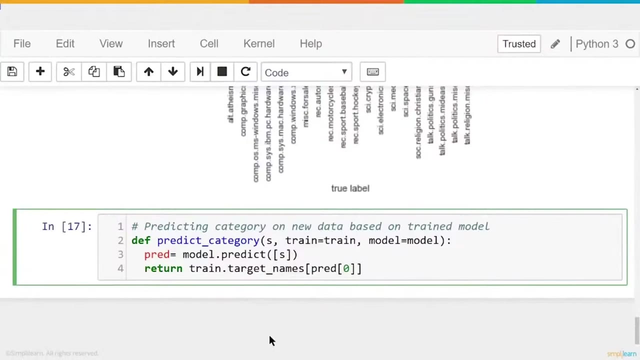 whatever string we send to it, it's going to push that string through the pipeline, the model pipeline. it's going to go through and tokenize it and put it through the tf, idf, convert that into numbers and weights for all the different documents and words and then it'll put that through our naive. 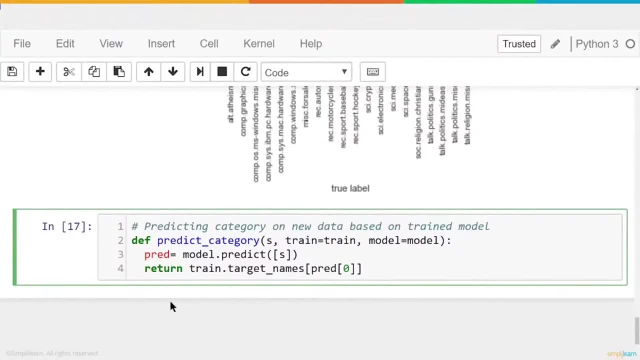 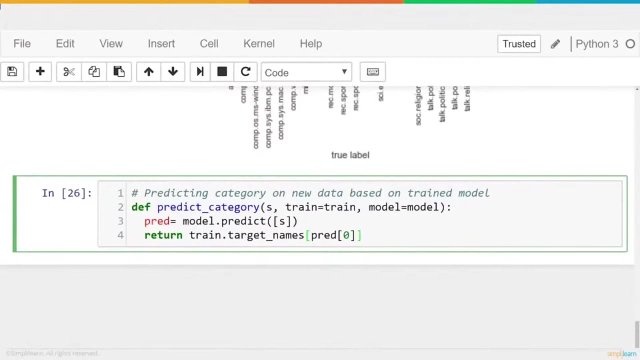 bays and from it we'll go ahead and get our prediction. we're going to predict what value it is and so we're going to return train dot target names, predict of zero, and remember that the train dot target names, that's just categories. i could have just as easily put categories in there. 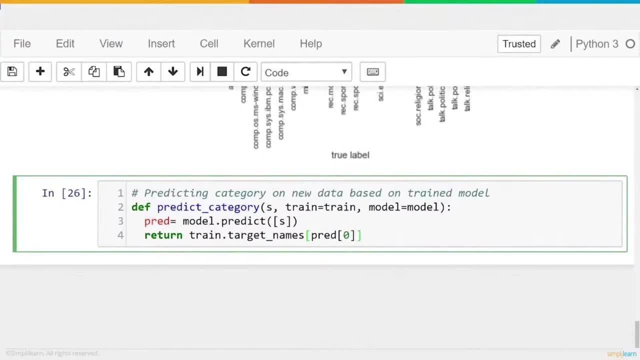 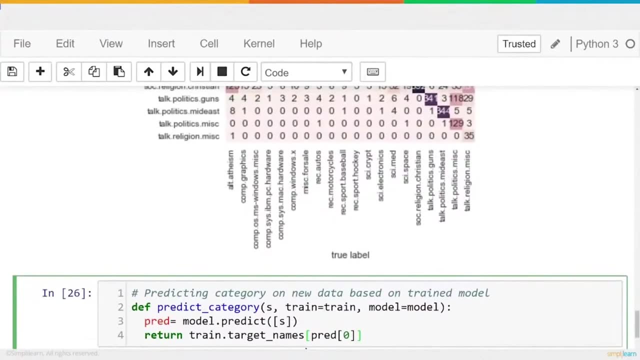 dot predict of zero. so we're taking the prediction, which is a number, and we're converting it to an actual category. we're converting it from i don't know what the actual numbers are. let's say zero equals alt atheism. so we're going to convert that zero to the word or one. maybe it equals comp. 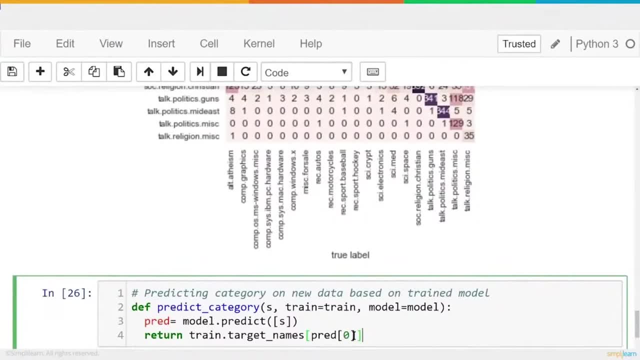 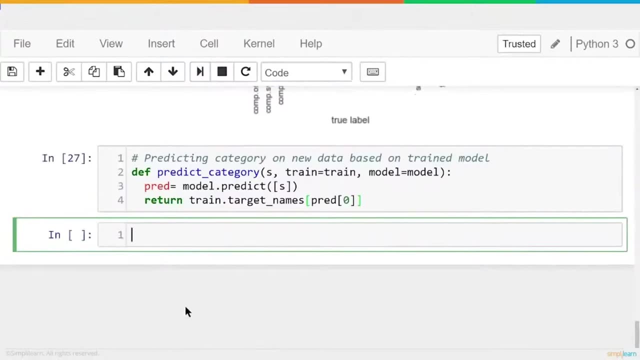 graphics. so we're going to convert number one into comp graphics. that's all that is. and then we got to go ahead and and then we need to go ahead and run this, so i load that up and then, once i run that, we can start doing some predictions. 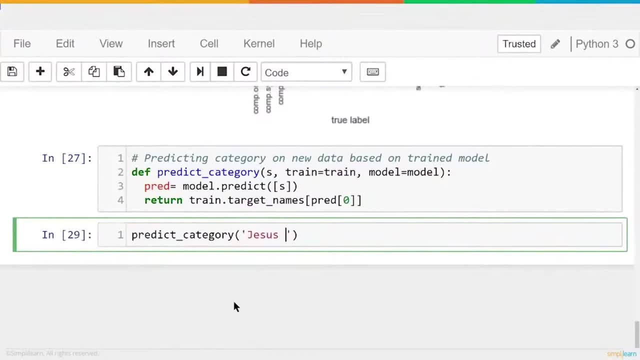 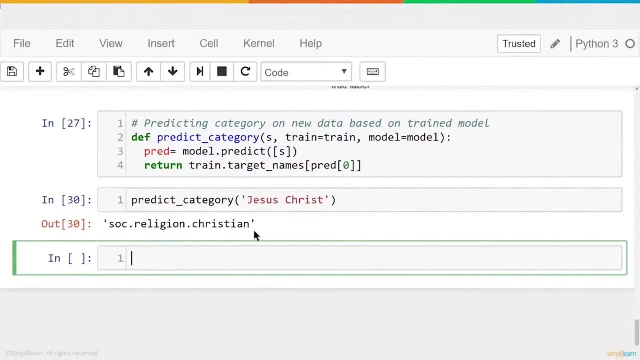 let me go ahead and type in predict category and let's just do predict category jesus christ and it comes back and says it's social religion- christian. that's pretty good. now note i didn't put print on this. one of the nice things about the jupyter notebook editor and a lot of inline. 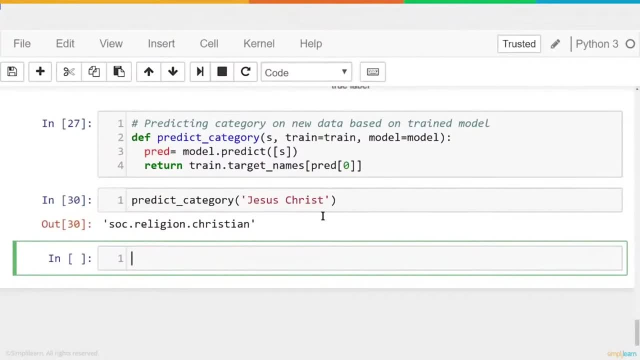 editors is if you just put the name of the variable out as returning the variable train dot target underscore names, it'll automatically print that for you in your own id. you might have to put in print. let's see where else we can take this. and maybe you're a space science buff. so how about sending load to international space station and 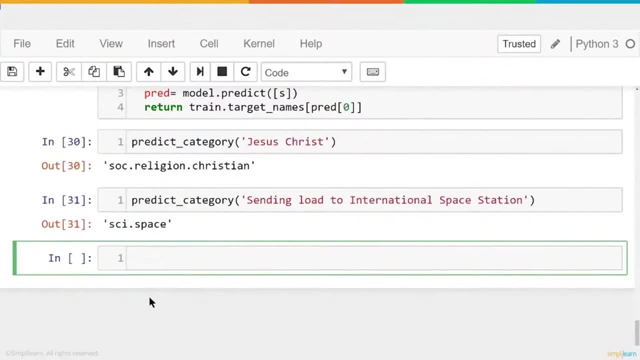 if we run that we get science, space. or maybe you're a automobile buff and let's do um. they were going to tell me audi is better than bmw. but i'm going to do bmw is better than an audi. so maybe you're a car buff and we run that and you'll see it says bmw is better than an audi. so maybe you're. 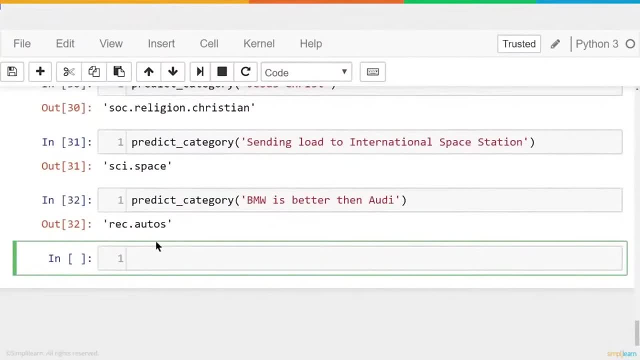 a car buff and we run that and you'll see it says recreational. i'm assuming that's what rec stands for autos. so i did a pretty good job labeling that one. how about if we have something like a caption running through there, president of india? and if we run that it comes up and says: talk politics. 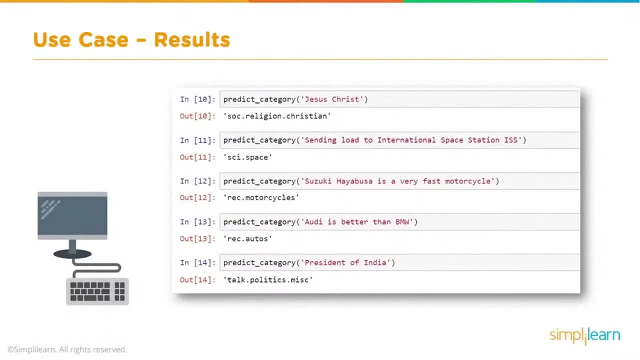 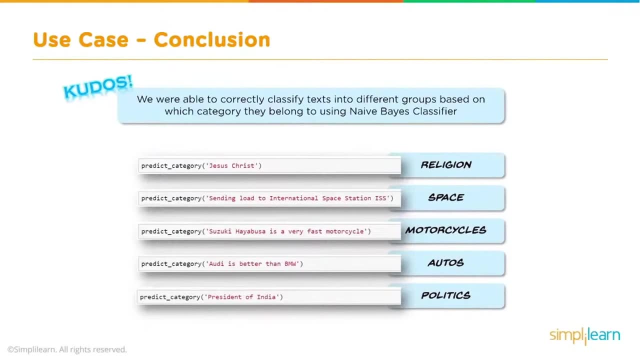 miscellaneous. so when we take our definition, our function and we run all these things through kudos, we made it. we were able to correctly classify texts into different groups based on which category they belong to, using the naive based classification. we're able to classify text into different groups based on which category they belong to, using the naive based classification. based on which category they belong to, using the naive based 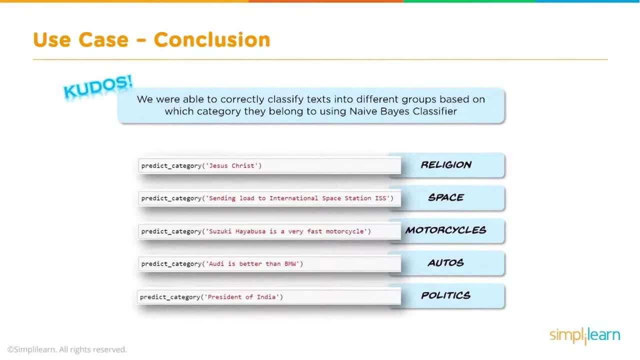 classifier. Now, we did throw in the pipeline the TF IDF vectorizer, we threw in the graphs. Those are all things that you don't necessarily have to know to understand that the Naive Bayes setup or classifier, but they're important to know. 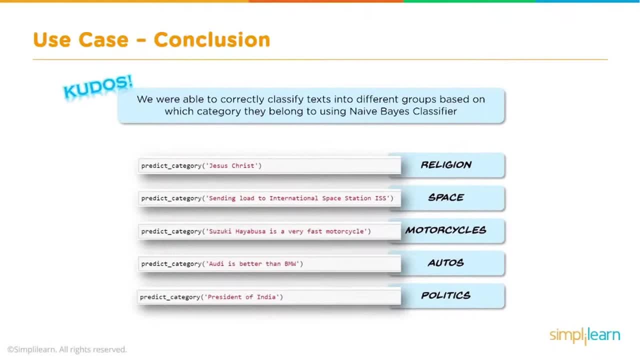 One of the main uses for the Naive Bayes is with the TF, IDF tokenizer or vectorizer, where it tokenizes the word and has labels, And we use the pipeline because you need to push all that data through and it makes it really easy and 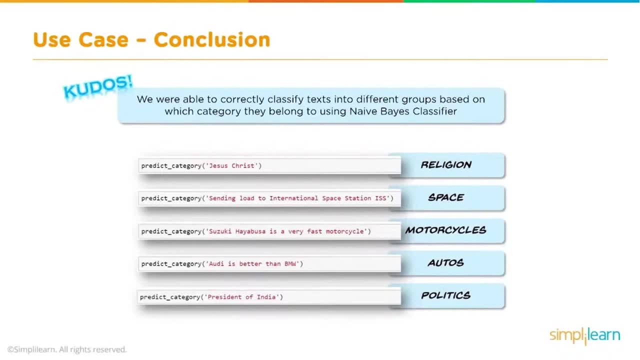 fast. You don't have to know those to understand Naive Bayes, but they certainly help for understanding the industry and data science. And we can see our categorizer, our Naive Bayes classifier. we were able to predict the category- religion, space, motorcycles, autos, politics- and properly classify all. 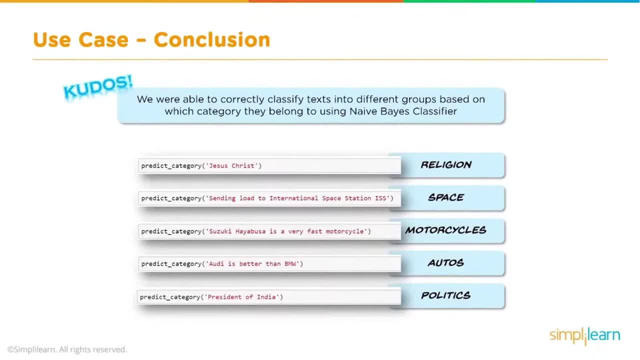 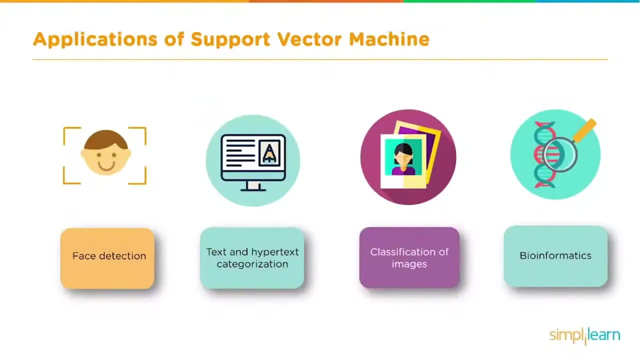 these different things we pushed into our prediction and our trained model. Before we dive into the SVM, let's take a look at applications of the support vector machine, at least some general ones that are commonly used With it: face detection, text and hypertext categorization, classification of 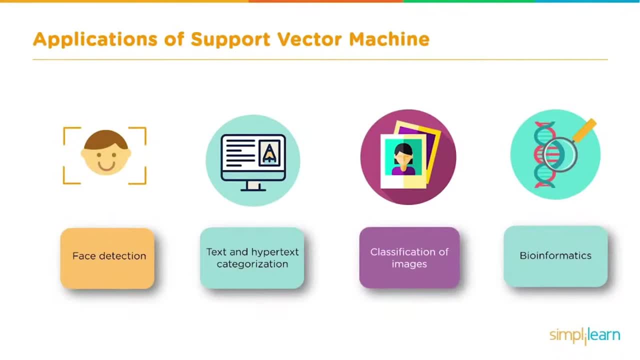 images and bioinformatics. These are only about a few of those that are used with this SVM. As we go through this lesson, see if you can figure out what other ones you could apply it to and also what you would want to use some. 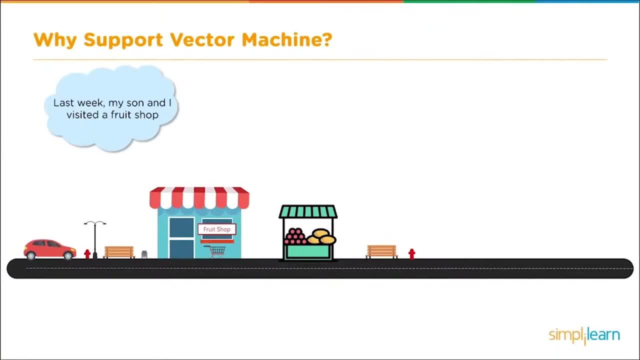 other tools for. So in this example, last week my son and I visited a fruit shop. Dad, is that an apple or a strawberry? So the question comes up: what fruit did I just pick up from the fruit stand? After a couple of seconds you can figure. 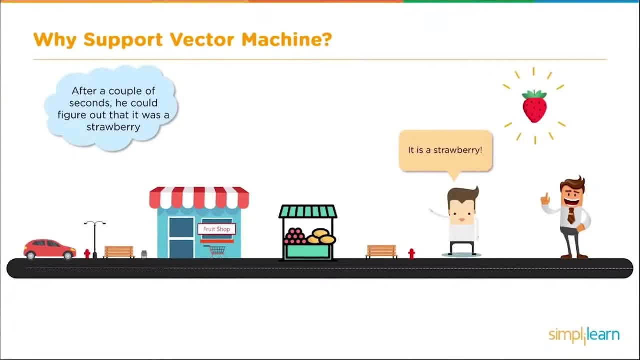 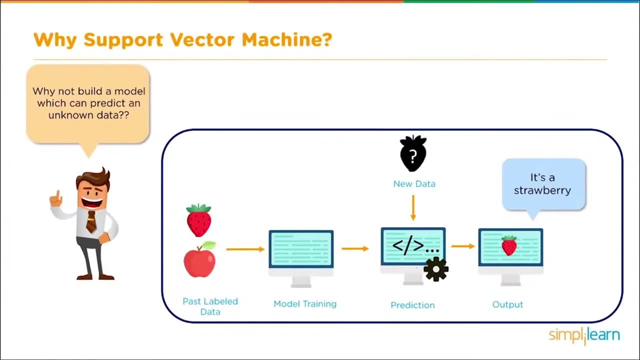 out that it was a strawberry. So let's take this model a step further and let's- why not? build a model which can predict an unknown data, And in this we're going to be looking at some sweet strawberries or crispy apples. We want it to be able. 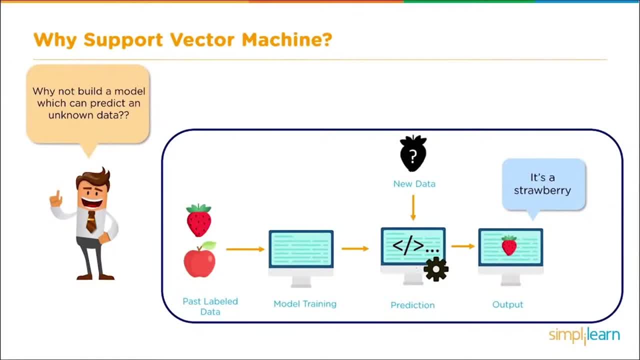 to label those two and decide what the fruit is. And we do that by having data already put in. So we already have a bunch of strawberries: we know our strawberries and they're already labeled as such. We already have a bunch of apples: we know our apples and are labeled as such. Then, once we train our 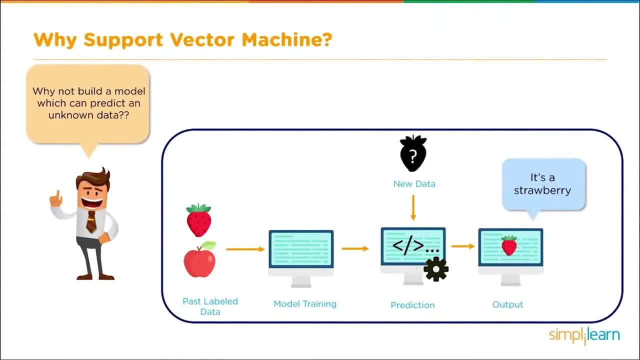 model. that model then can be given the new data, And the new data is this image. In this case, you can see a question mark on it and it comes through and goes. it's a strawberry. In this case, we're using the support vector machine. model SVM is. 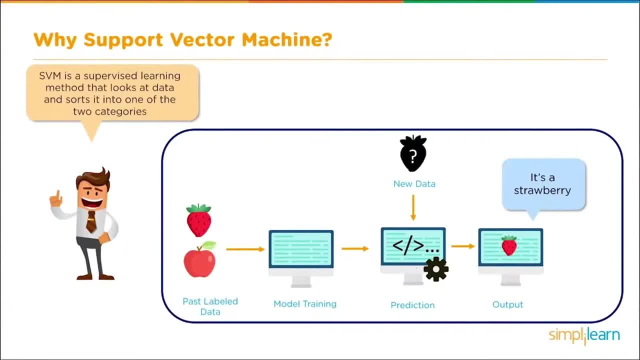 a supervised learning method that looks at data and sorts it into one of two categories, And in this case we're sorting the strawberry into the strawberry side. At this point, you should be asking the question: how does the prediction work? Before we dig into an example with numbers, let's apply this. 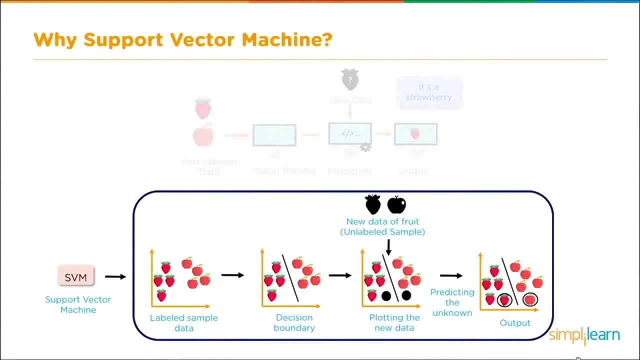 to our fruit scenario. We have our support vector machine. We've taken it and we've taken labeled sample of data- strawberries and apples- and we draw on a line down the middle between the two groups. This split now allows us to take new data- in this case an apple and a strawberry- and place them in the 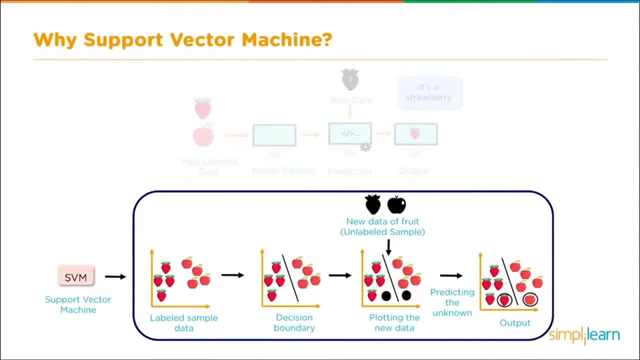 appropriate group based on which side of the line they fall in, And that way we can predict the unknown. As colorful and tasty as a fruit example is, let's take a look at another example with some numbers involved, And we can take a closer look at how the math works. 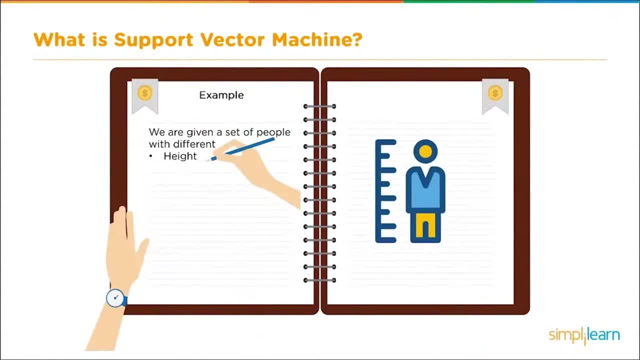 In this example, we're going to be classifying men and women And we're going to start with a set of people with a different height and a different weight, And to make this work, we'll have to have a sample data set of female, where. 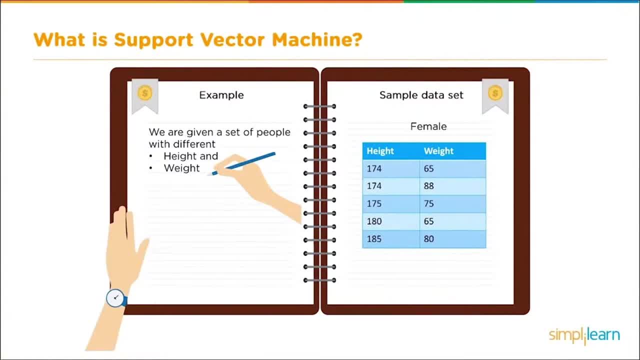 you have their height and weight- 174,, 65,, 174,, 88, and so on- And we'll need a sample data set of the male. They have a height: 179,, 90,, 180 to 80, and so on. Let's. 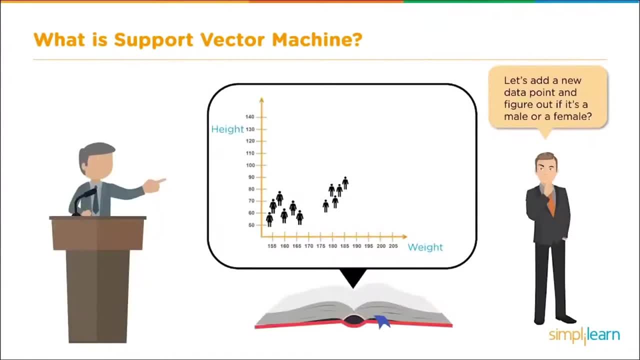 go ahead and put this on a graph so you have a nice visual. So you can see, here we have two groups based on the height versus the weight, And on the left side we're going to have the women. On the right side we're going to 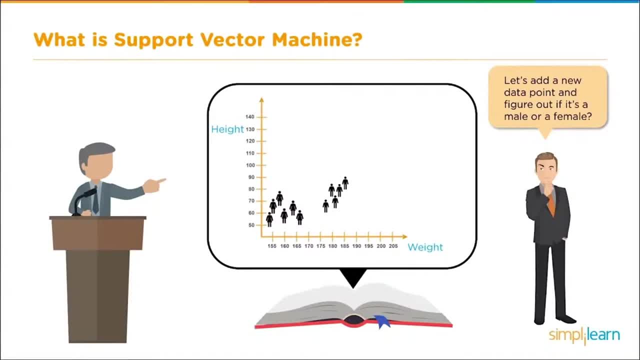 have the men. Now, if we're going to create a classifier, let's add a new data point and figure out if it's male or female. So before we can do that, we need to split our data first. We can split our data by choosing any of these lines In this case: 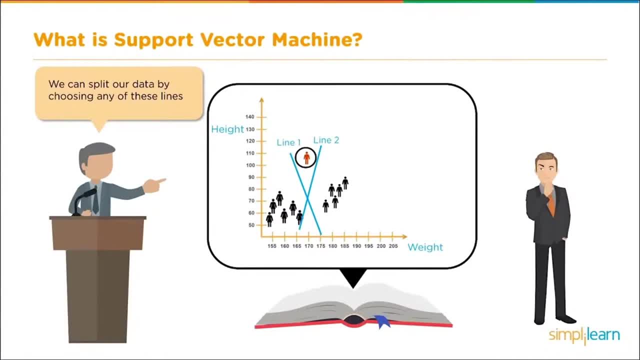 we draw in two lines through the data in the middle. that separates the men from the women. But to predict the gender of a new data point, we should split the data in the best possible way. And we say the best possible way because this line is: 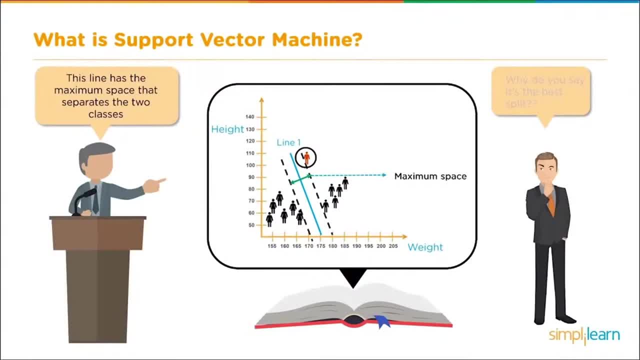 the maximum space that separates the two classes. Here you can see there's a clear split between the two different classes And in this one there's not so much a clear split. This doesn't have the maximum space that separates the two. That is why this line 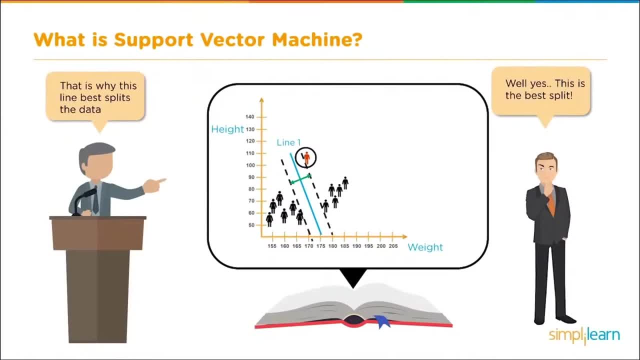 best splits the data. We don't want to just do this by eyeballing it. And before we go further, we need to add some technical terms to this. We can also say that the distance between the points in the line should be as far as possible. In technical terms, we can. 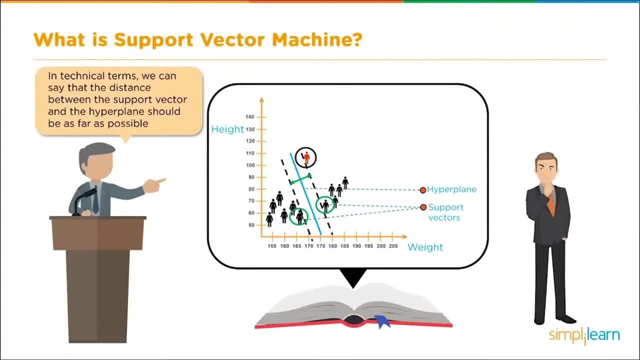 say, the distance between the support vector and the hyperplane should be as far as possible, And this is where the support vectors are the extreme points in the data set. And if you look at this data set, they have circled two points which seem to be right on the outskirts. 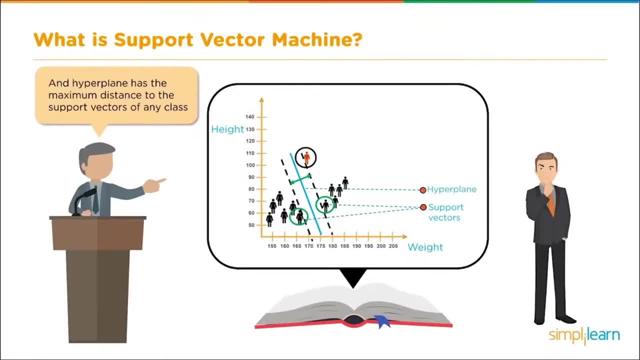 of the women and one on the outskirts of the men, And hyperplane has a maximum distance to the support vectors of any class. Now you'll see the line down the middle, And we call this the hyperplane, because when you're dealing with multiple dimensions, it's really not. 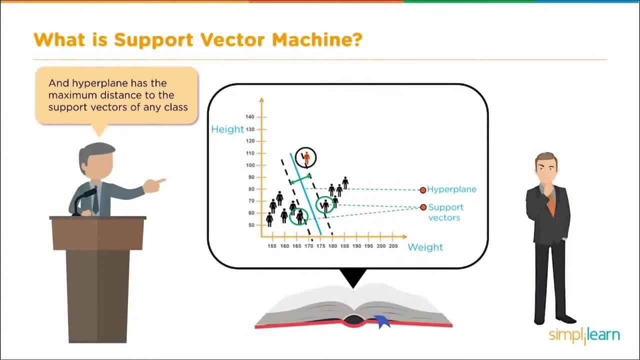 just a line but a plane of intersections, And you can see here where the support vectors have been drawn in dashed lines. The math behind this is very simple. We take D plus, the shortest distance to the closest positive point, which would be on the men's side, and D minus is the shortest distance to the closest. 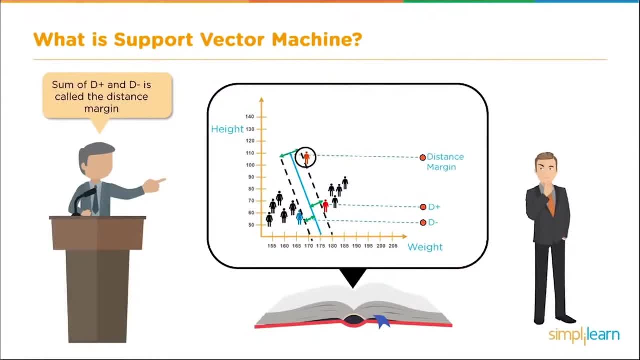 negative point, which is on the women's side. The sum of D plus and D minus is called the distance margin, or the distance between the two support vectors that are shown in the dashed lines, And then, by finding the largest distance margin, we get the optimal hyperplane. Once we've created an optimal hyperplane, we can easily 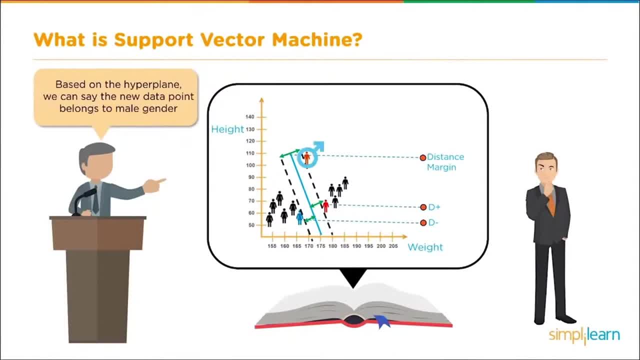 see which side the new data fits in And, based on the hyperplane, we can say the new data point belongs to the male gender. Hopefully that's clear how that works on a visual level. As a data scientist, you should also be asking what happens if the hyperplane is not optimal. 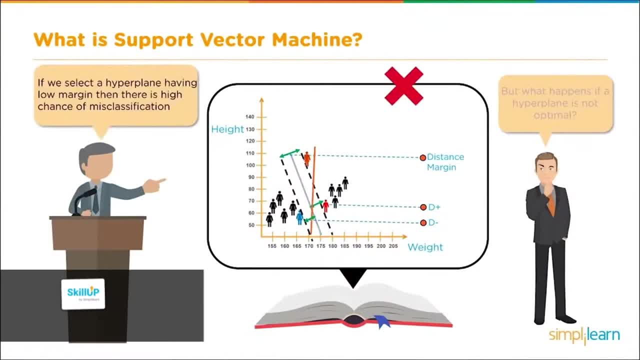 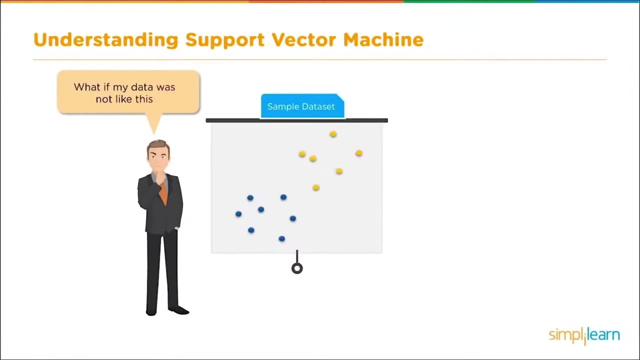 If we select a hyperplane having low margin, then there is a high chance of misclassification. This particular SVM model, the one we discussed so far, is also called or referred to as the LSVM. So far, so clear. but a question should be coming up. We have our sample data set. 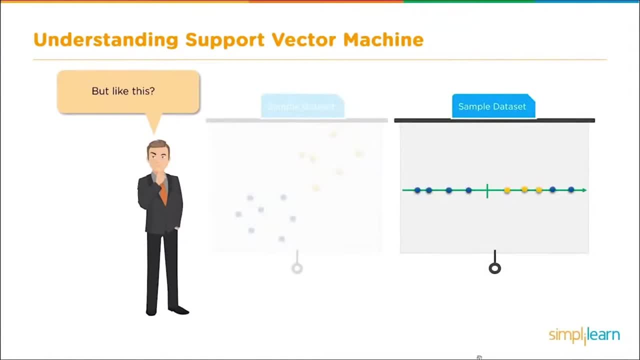 but instead of looking like this, what if it looked like this: where we have two sets of data, but one of them occurs in the middle of another set. You can see here where we have the blue and the yellow and then blue again on the other side of our data line. 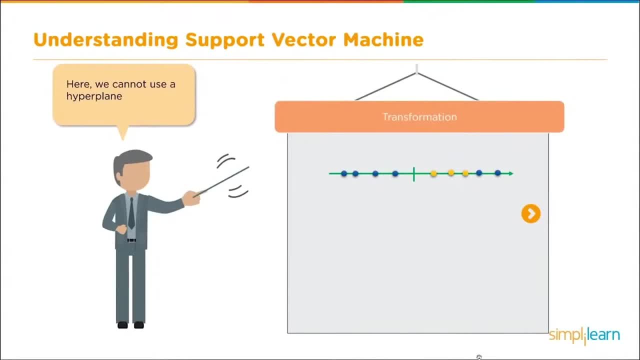 In this data set. we can't use a hyperplane. So when you see data like this, it's necessary to move away from a 1D view of the data to a two-dimensional view of the data, And that's what we're going to do here: We're going to use a hyperplane and we're going to use a. 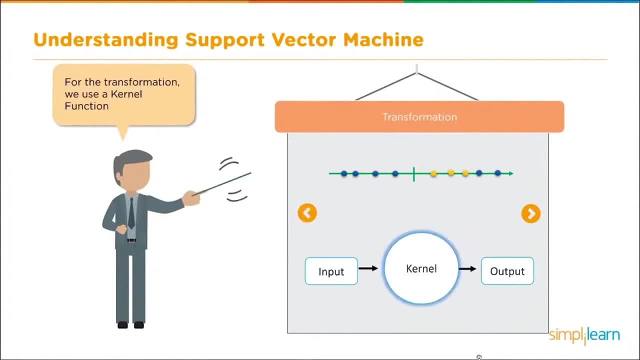 two-dimensional view of the data And for the transformation we used what's called a kernel function. The kernel function will take the 1D input and transfer it to a two-dimensional output. As you can see in this picture here, the 1D when transferred to a two-dimensional. 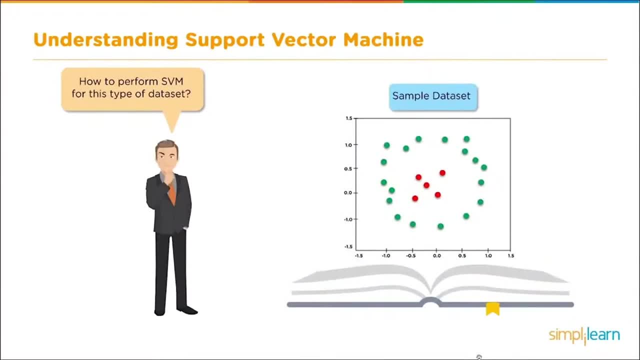 makes it very easy to draw a line between the two data sets. What if we make it even more complicated? How do we perform an SVM for this type of data set? Here you can see we have a two-dimensional data set where the data is in the middle, surrounded by the green. 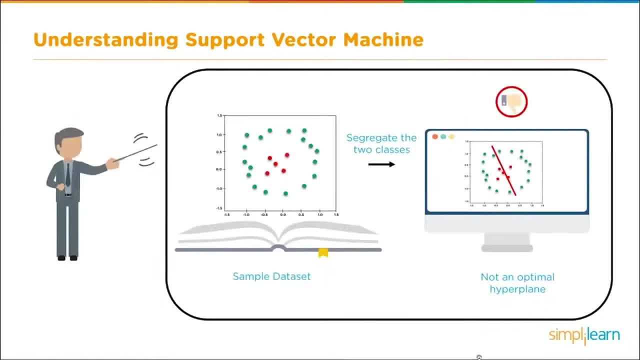 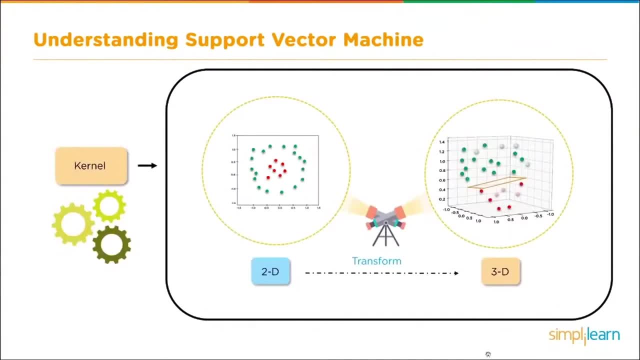 data on the outside. In this case we're going to segregate the two classes. We have our sample data set and if you draw a line through, it's obviously not an optimal hyperplane in there. So to do that, we need to transfer the 2D to a 3D array And when you translate 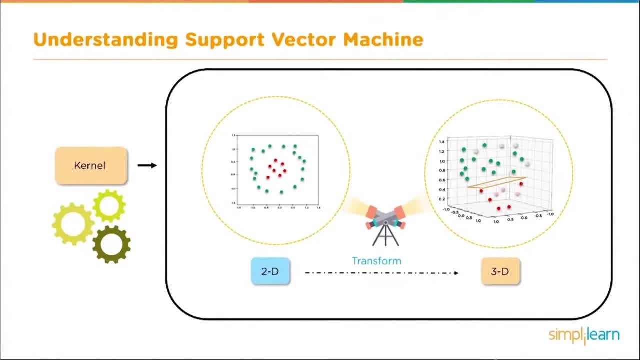 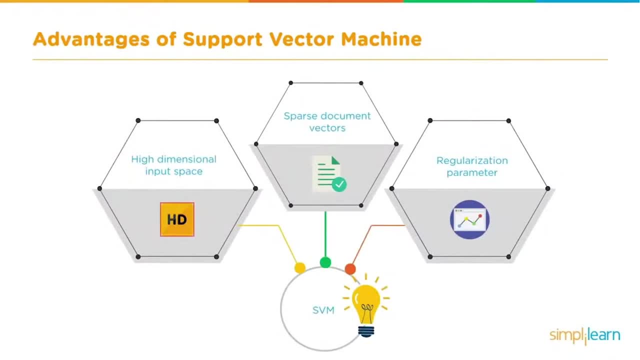 it into a three-dimensional array. using the kernel, you can see where you can place a hyperplane right through it and easily split the data. Before we start looking at a programming example and dive into the script, let's look at the advantage of the support vector machine. 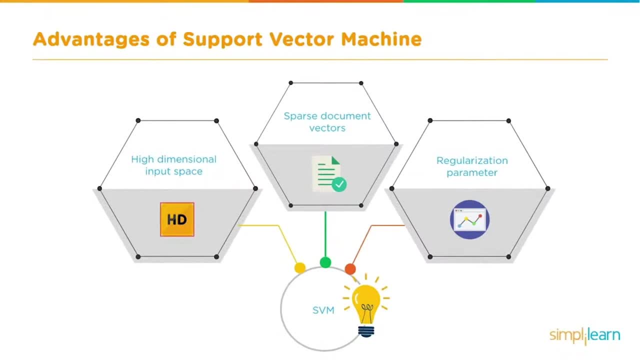 First of all, we need to know what the output space is, or sometimes referred to as the curse of dimensionality. We looked at earlier 1D, 2D, 3D. When you get to a thousand dimensions, a lot of problems start occurring with most algorithms that have to be adjusted for The 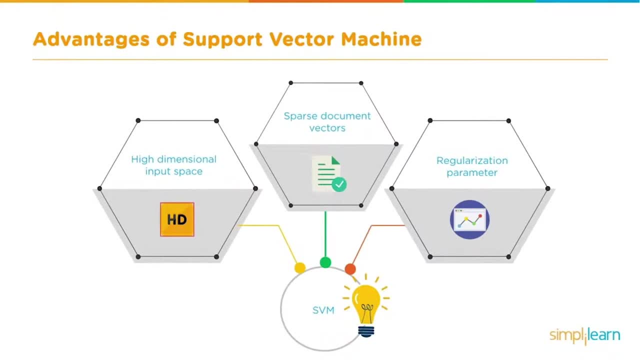 SVM automatically does that in high-dimensional space. One of the high-dimensional space, one high-dimensional space that we work on, is sparse document vectors. This is where we tokenize the words and documents so we can run our machine learning algorithms over them. And finally we have regularization parameter. The regularization parameter, or lambda, is 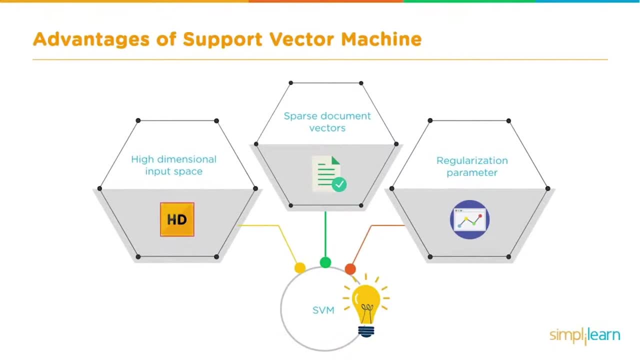 a parameter that helps figure out whether we're going to have a bias or overfitting of the data, whether it's going to be overfitted to a very specific instance or it's going to be biased to a high or low value. With the SVM, it naturally avoids the overfitting. 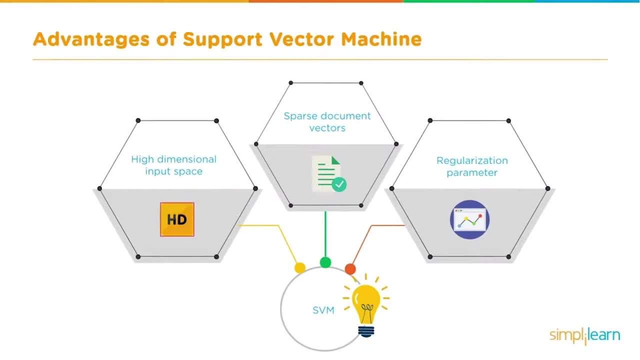 and bias, problems that we see in many other algorithms. These three advantages of the support vector machine make it a very powerful tool to use. It's a very powerful tool to add to your repertoire of machine learning tools. Now we did promise you a use case study. We're actually going to dive into some Python programming. 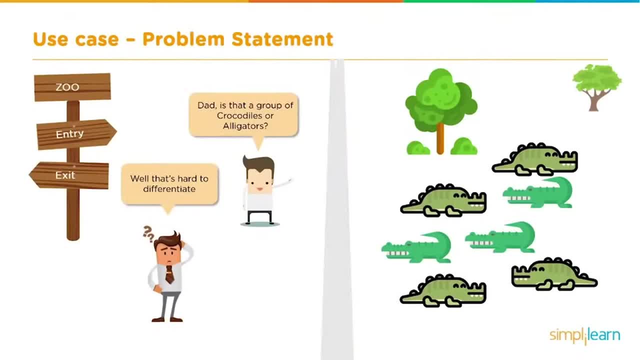 And so we're going to go into a problem statement and start off with the zoo. So in the zoo example, we have family members going to the zoo. We have the young child going Dad, is that a group of crocodiles or alligators? Well, that's hard to differentiate. 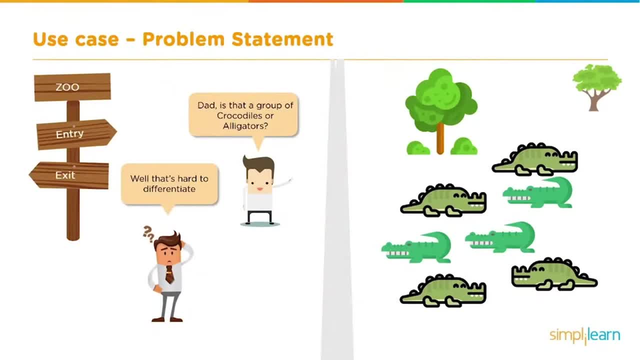 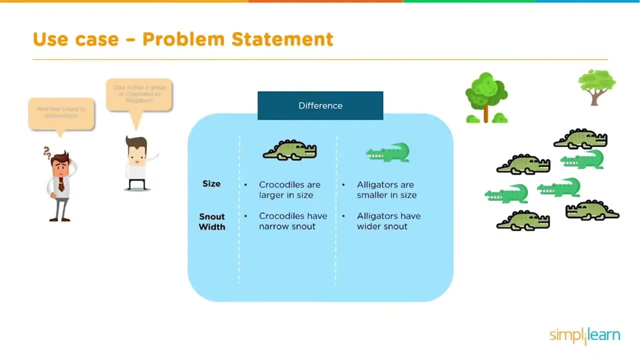 And zoos are a great place to start looking at science and understanding how things work, especially as a young child. And so we can see the parents sitting here thinking, well, what is the difference between a crocodile and an alligator? Well, one, crocodiles are. 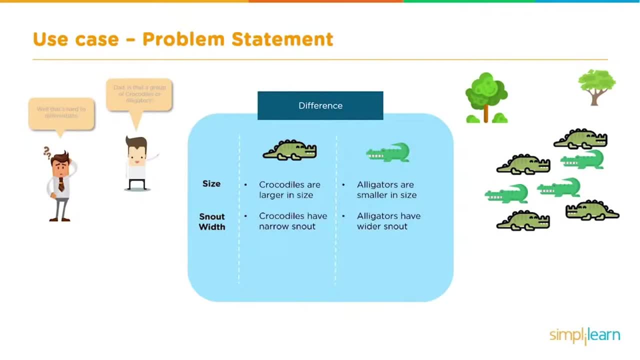 larger in size. Alligators are smaller in size. Snout width: the crocodiles have a narrow snout and alligators have a wider snout. And, of course, in the modern day and age, the father is sitting here is thinking how can I turn this into a lesson for my son? And 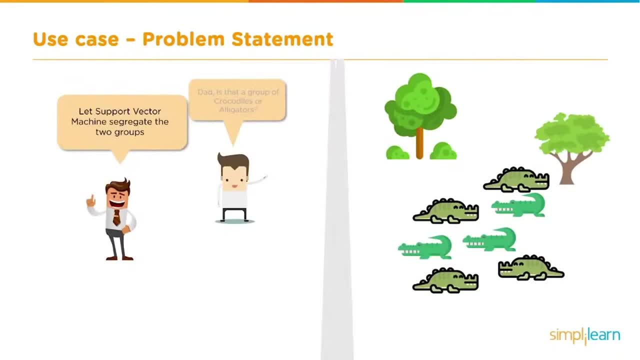 he goes: let a support vector machine segregate the two groups. I don't know if my dad ever told me that, but that would be funny. Now, in this example, we're not going to use actual measurements and data, We're just using that for imagery. 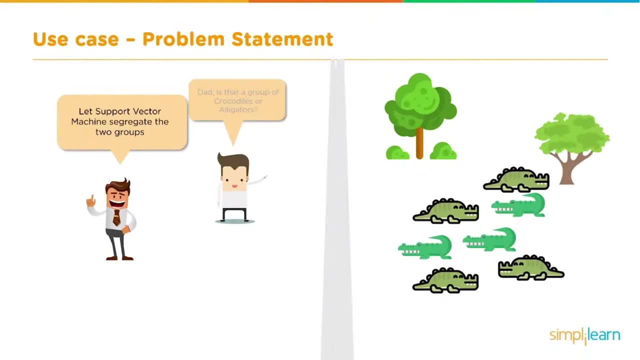 We're just using that for imagery. Now, if we were to take a look at this, we're going to see that this is a very common and a lot of machine learning algorithms and setting them up. But let's roll up our sleeves and we'll talk about that more in just a moment. 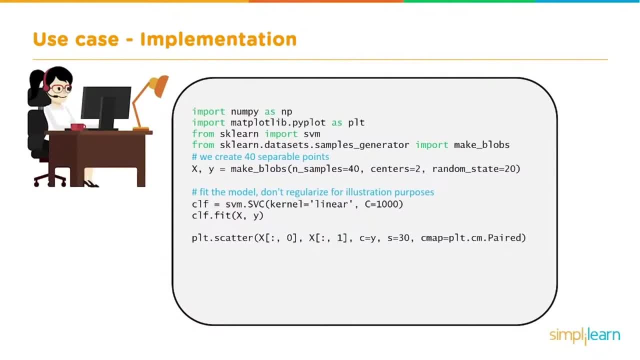 as we break into our Python script. So here we arrive in our actual coding, And I'm going to move this into a Python editor in just a moment. But let's talk a little bit about what we're going to cover First. we're going to cover in the code, the setup, how to actually 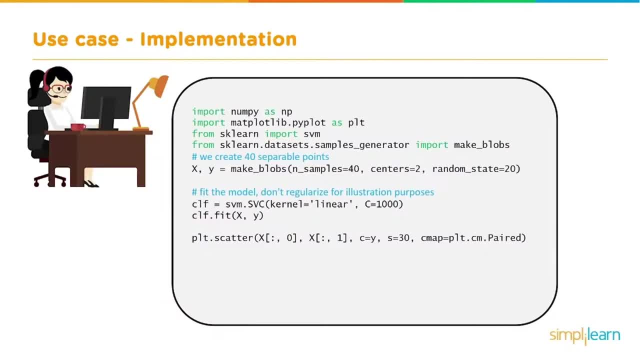 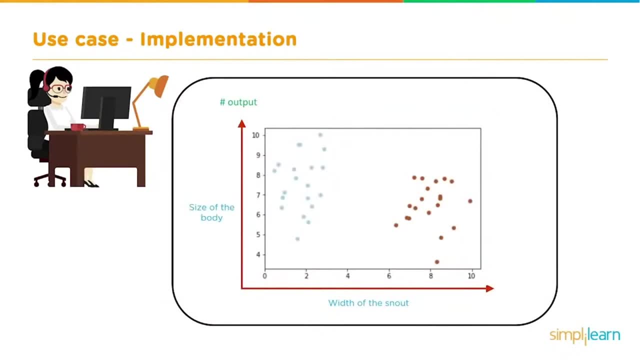 create our SVM And you're going to find that there's only two lines of code that actually appear on the first page, And we'll show you what that looks like as far as our data. So we're going to create some data. I talked about creating data just a minute ago And 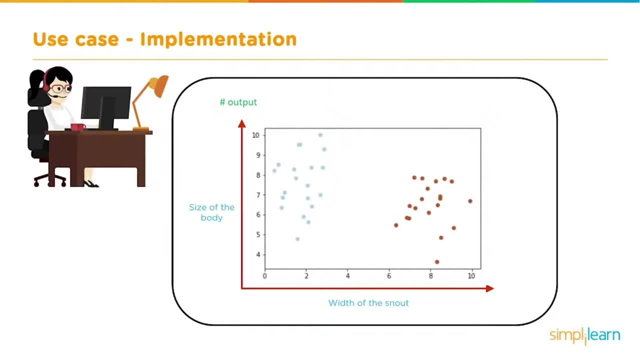 so we'll get into the creating data here And you'll see this nice correction of our two blobs And we'll go through that in just a second. And then the second part is: we're going to take this and we're going to bump it up a notch. We're going to show you what. 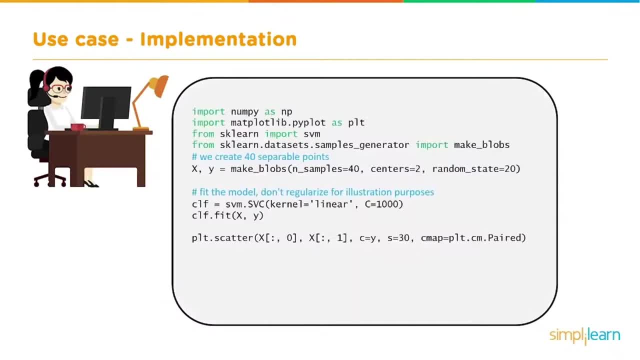 it looks like behind the scenes, But let's start with actually creating our setup. I like to use the Anaconda Jupyter notebook because it's very easy to use, But you can use any of your favorite Python editors or setups and go in there. 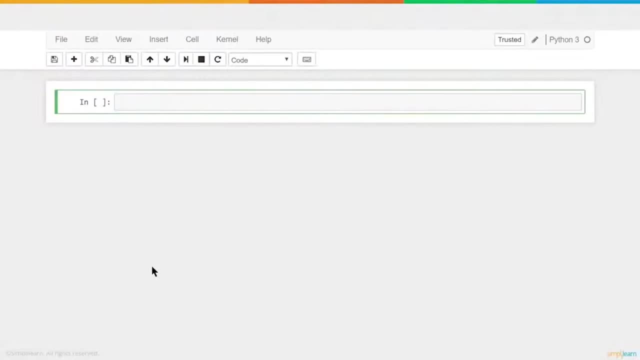 Go ahead and switch over there and see what that looks like. So here we are in the Anaconda Python notebook or Anaconda Jupyter notebook. with Python, We're using Python 3.. I believe this is 3.5, but it should be work in any of your 3x versions. 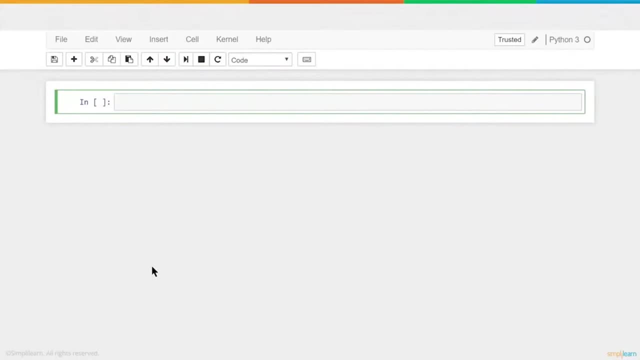 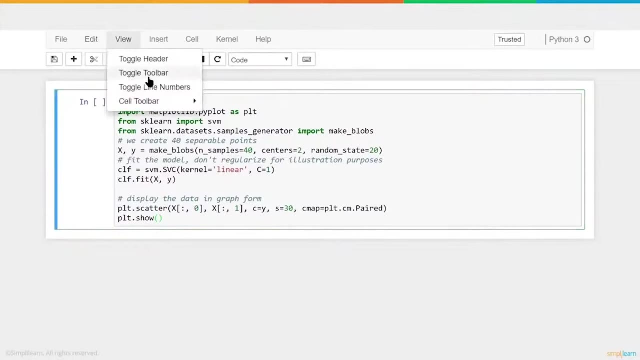 And you'd have to look at the sklearn to make sure if you're using a 2x version or an earlier version. Let's go ahead and put our code in there, And one of the things I like about the Jupyter notebook is I can go up to view And I'm going to go ahead and toggle the line. 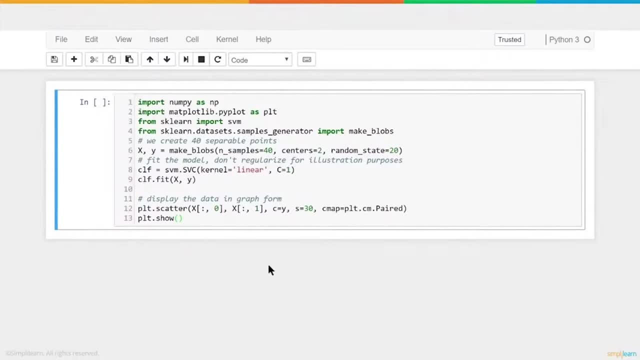 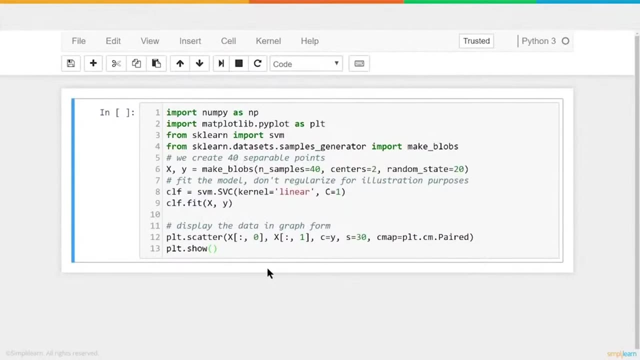 numbers on to make it a little bit easier to talk about, And we can even increase the size, because this is edited in. in this case, I'm using Google Chrome Explorer and that's how it opens up for the editor. Although anyone like I 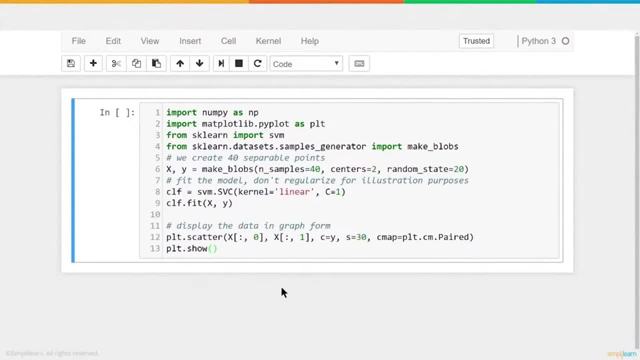 said, any editor will work. Now the first step is going to be our imports, And we're going to import four different parts. The first two I want you to look at are line 1 and line 2 are numpy as np and matplotlibrarypyplot. 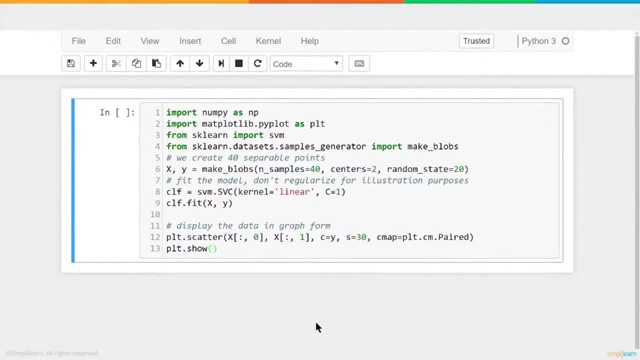 as plt. Now, these are very standardized imports when you're doing work. The first one is the numbers in Python. We need that because part of the platform we're using uses that for the numpy array, And I'll talk about that in a minute so you can understand why we want to use a. 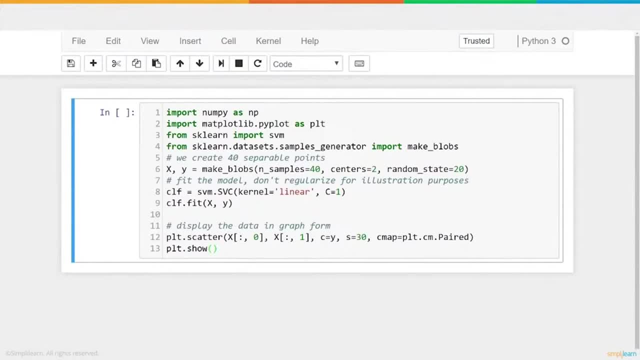 numpy array versus the standard Python array And normally it's pretty standard setup to use np for numpy. The matplotlibrary is how we're going to view our data. So this has. you do need the np for the sklearn module, But the matplotlibrary is purely for our use for visualization And 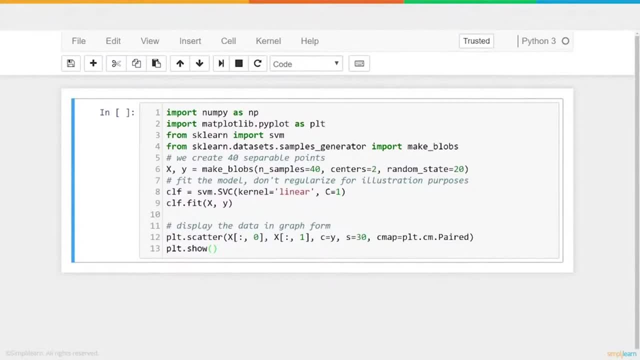 so you really don't need that for the SVM, But we're going to put it there so you have a nice visual aid And we can show you what it looks like. That's really important at the end when you finish everything, so you have a nice display for everybody to look at. 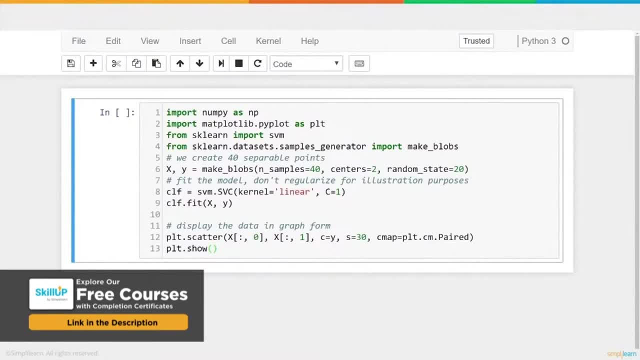 And then, finally, we're going to- I'm going to jump one ahead- to line number 4.. That's the sklearndatasetssamplesgenerator import makeblobs. And I told you that we were going to make up data And this is a tool that's in the sklearn to make up data. I personally, 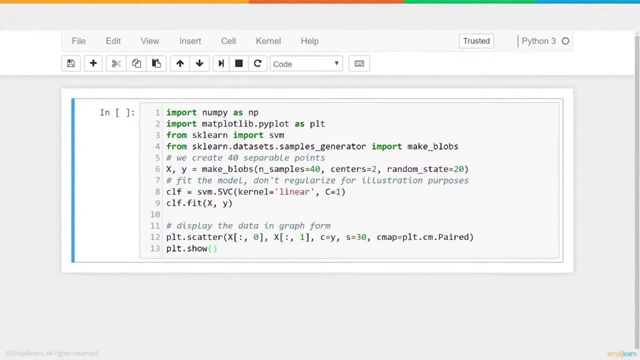 don't want to go to the zoo, get in trouble for jumping over the fence and probably get eaten by the crocodiles or alligators as I work on measuring their snouts and width and length. Instead, we're just going to make up some data And that's what that makeblobs. 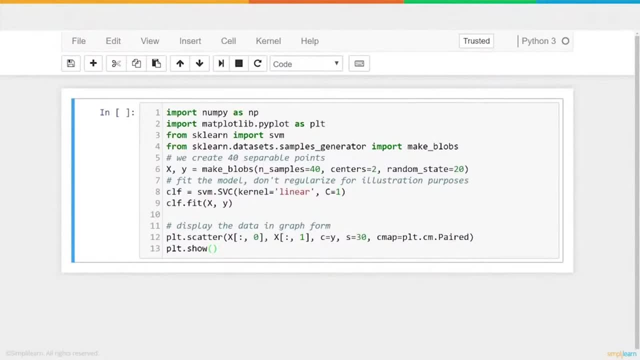 is. It's a wonderful tool. if you're ready to test your setup and you're not sure about what data you're going to put in there, You can create this blob and it makes it real easy to use. And finally, we have our actual SVM- the sklearn import svm- on line 3.. So that covers all our. 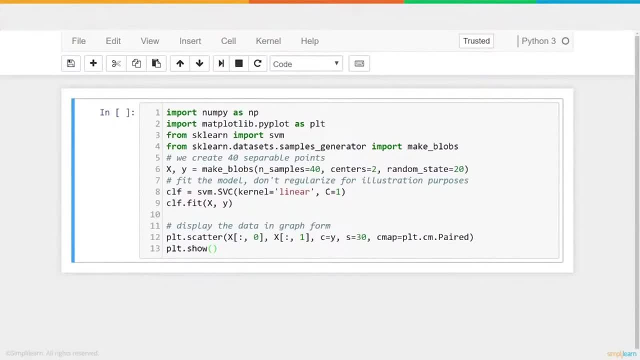 imports We're going to create- remember, I used the makeblobs to create data And we're going to create a capital X and a lowercase y equals makeblobs in samples- equals 40.. So we're going to make 40 lines of data. It's going to have two centers with a random state. 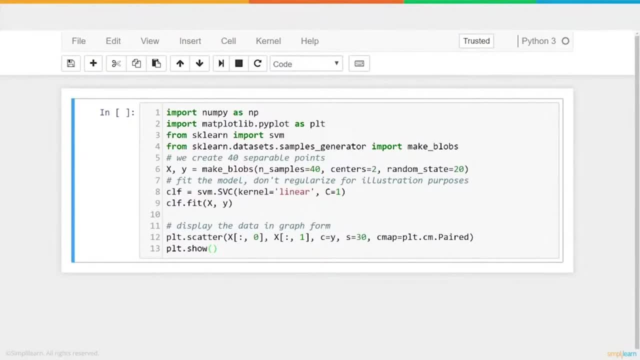 equals 20.. So each group's going to have 20 different pieces of data in it And the way that looks is it will have under x an xy plane. So it'll have two numbers under x, And y will be 0 or 1.. That's the two different centers. So we have yes or no in this case, alligator. 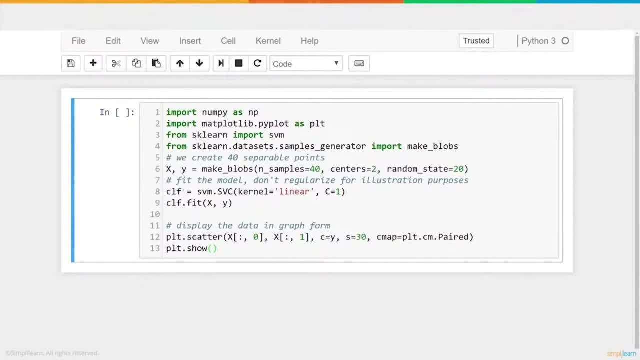 or crocodile. That's what that represents. And then I told you that the actual sklearn, or the SVM, is in two lines of code. And we see it right here with: clf equals svm, dot, svc, kernel equals linear And I set c equal to 1.. Although in this example, since we are not regularizing the data, since we want it, 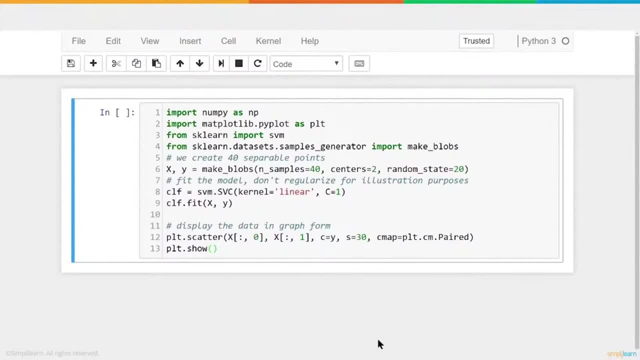 to be very clear and easy to see, I went ahead. you can set it to a thousand a lot of times when you're not doing that, But for this thing- linear because it's a very simple linear example- We only have the two dimensions and it'll be a nice linear hyperplane. It'll be a nice. 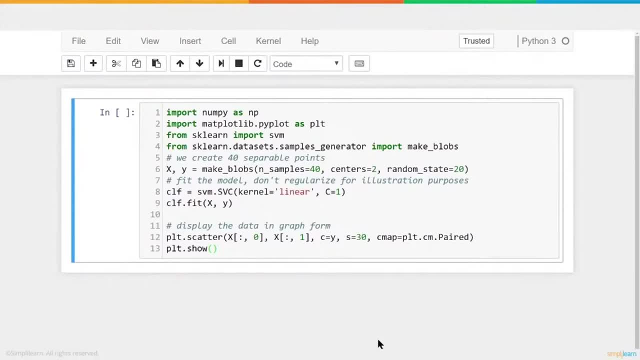 linear line instead of a full plane, So we're not dealing with a huge amount of data, And then all we have to do is do clf, dot fit x, comma y, And that's it. Clf has been created, And then we're going to go ahead and display it, And I'm going to talk about this display. 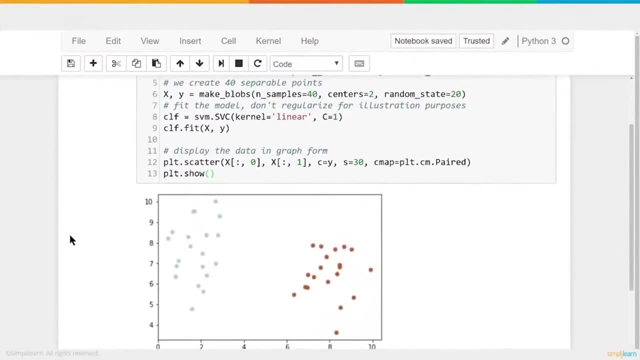 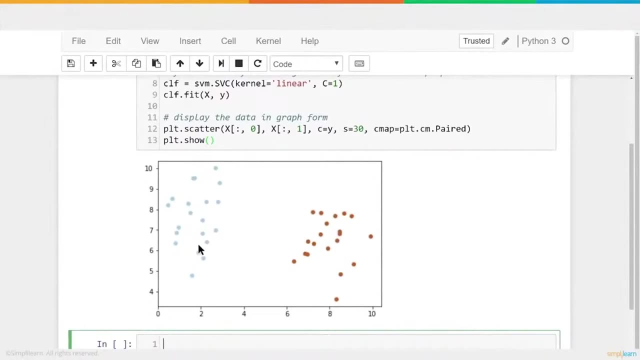 here in just a second, But let me go ahead and run this code, And this is what we've done is we've created two blobs. You'll see the blue on the side and then kind of an orangish on the other side. That's our two sets of data They represent. one represents crocodiles. 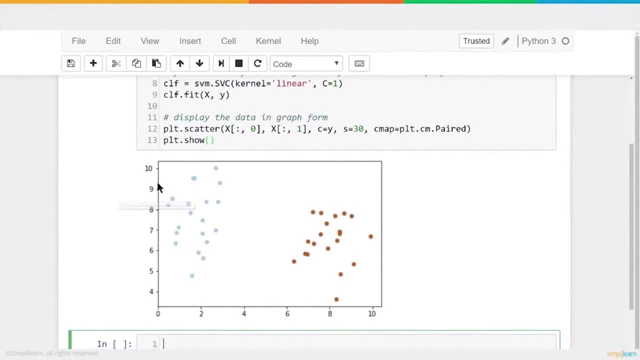 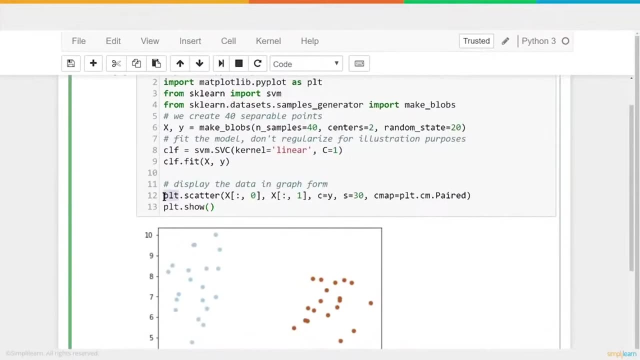 and one represents alligators. And then we have our measurements. In this case we have like the width and length of the snout. And I did say I was going to come up here and talk just a little bit about our plot And you'll see, plt, That's what we imported. We're going to do a scatter plot. That means 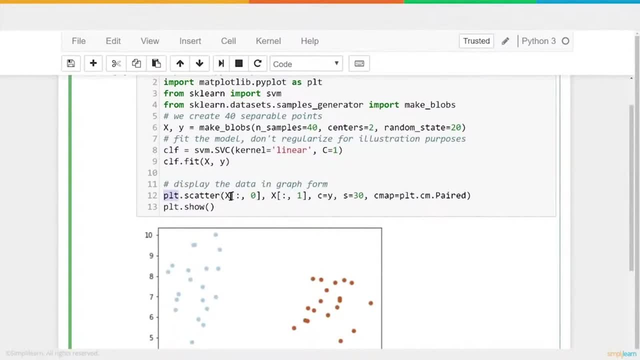 we're just putting dots on there And then look at this notation: I have the capital x and then in brackets I have a colon, comma, zero. That's from numpy. If you did that in a regular array, you'll get an error in a Python array. You have to have that in a numpy. 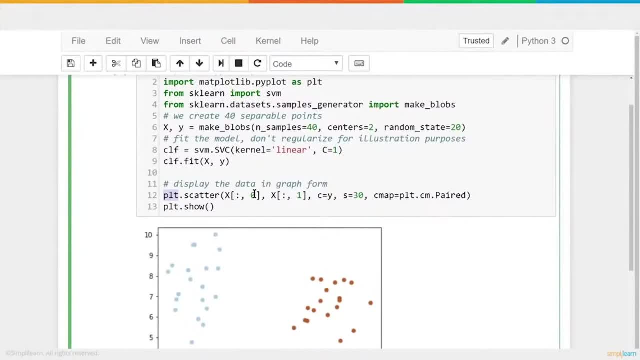 array. It turns out that our make blobs returns a numpy, And this notation is great because what it means is the first part is the colon. It means we're going to do all the rows. That's all the data in our blob we created under capital. 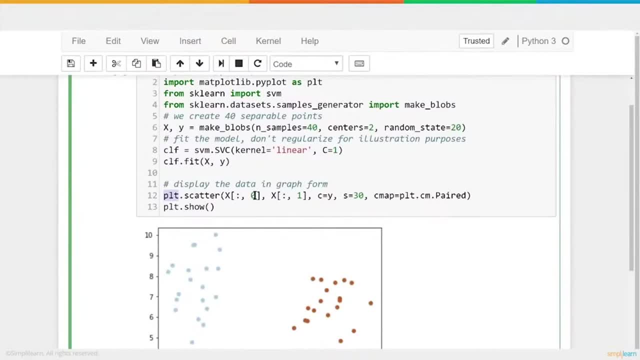 x, And then the second part has a comma zero. We're only going to take the first value And then, if you notice, we do the same thing but we're going to take the second value. Remember, we always start with zero and then one, So we have column zero and column one. 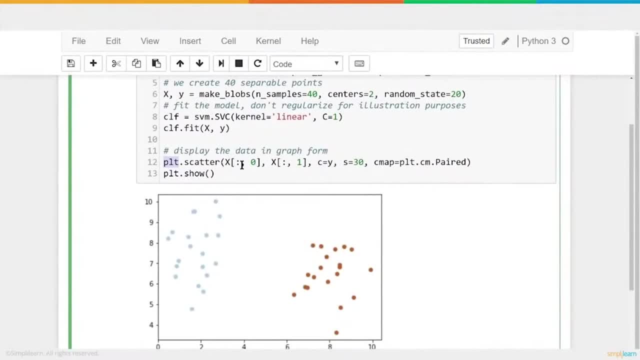 And you can look at this as our xy plots. The first one is the x plot and the second one is the y plot. So the first one is on the bottom zero, two, four, six, eight and ten, And then the second. 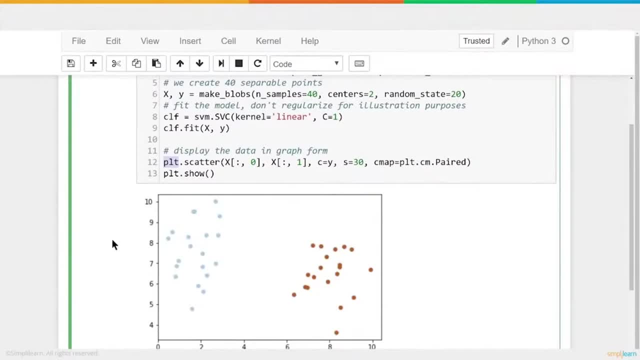 one x of the one is the four, five, six, seven, eight, nine, ten. going up the left hand side, S equals 30, is just the size of the dots. We can see them. It says real tiny dots And. 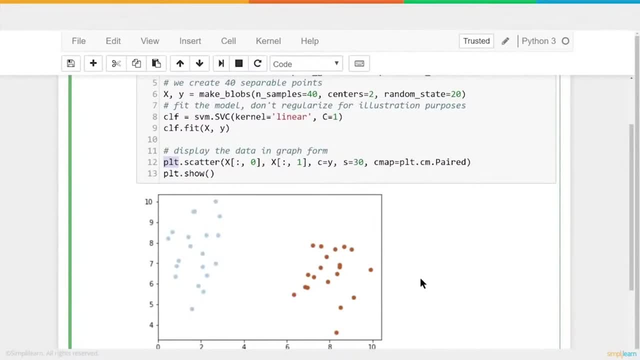 then cmap equals pltcmpaired And you'll also see the c equals y. That's the color We're using, two colors, zero one, and that's why we get the nice blue and the two different colors for the alligator. 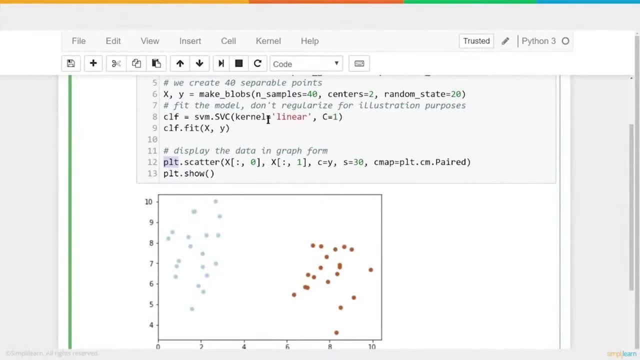 Now you can see here that we did this. the actual fit was done in two lines of code. A lot of times there will be a third line where we regularize the data, We set it between like minus one and one and we reshape it. But for this it's not necessary And it's 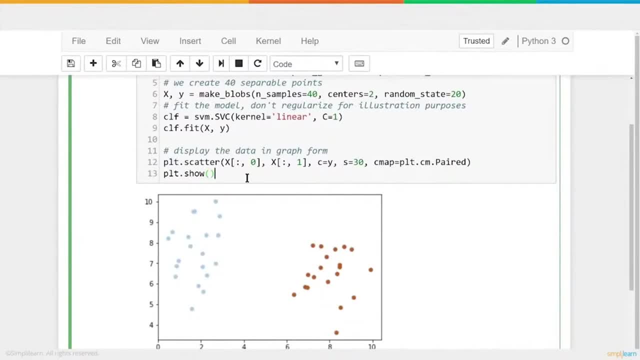 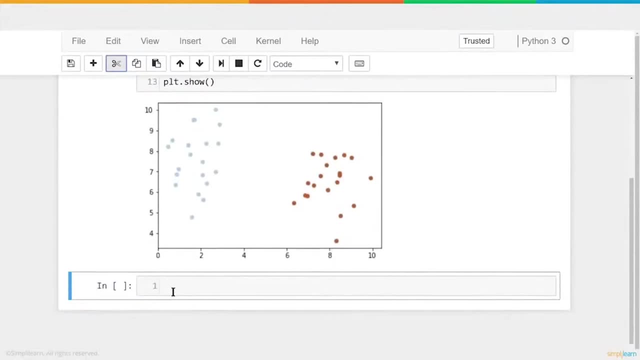 also kind of nice because you can actually see what's going on. And then, if we wanted to, we wanted to actually run a prediction- let's take a look- and see what that looks like- And to predict some new data, and we'll show this again as we get towards the end of digging. 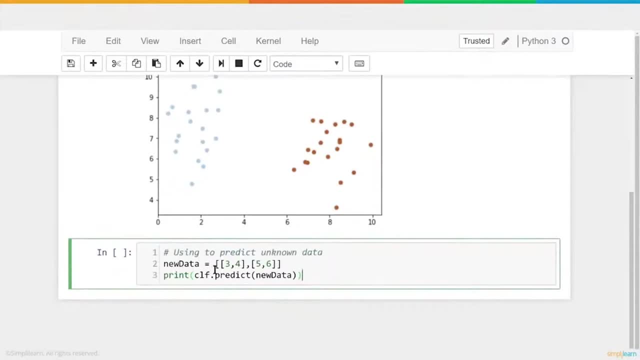 in deep. You can simply assign your new data. In this case, I am giving it a width and length three, four and a width and length five, six, And note that I put the data as a set of brackets, and then I have the brackets inside, And the reason I do that is because when we're looking 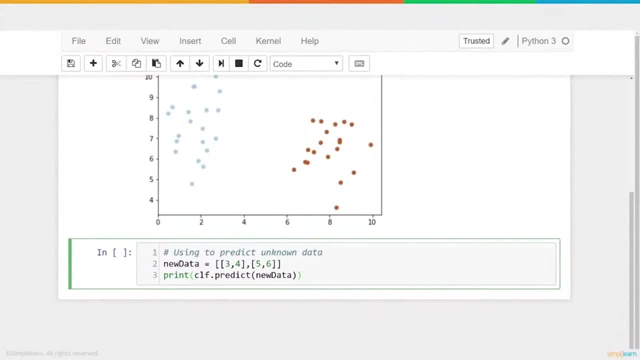 at data. it's designed to process a large amount of data coming in. We don't wanna just process one line at a time, And so in this case I'm processing two lines and then I'm just gonna print And you'll see clfpredict new data. So the clfpredict new data will actually do the. 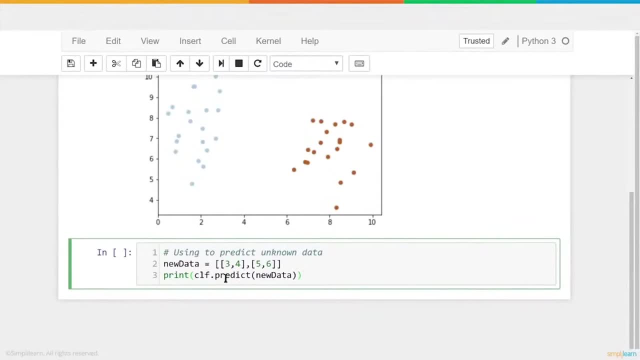 same thing And then I'm just gonna print and you'll see that I did a good job of connecting the data and then we have a little bit of data that's going to be in the same space that we recorded earlier- new data. So the CLF and the dot predict part is going to give us an answer and 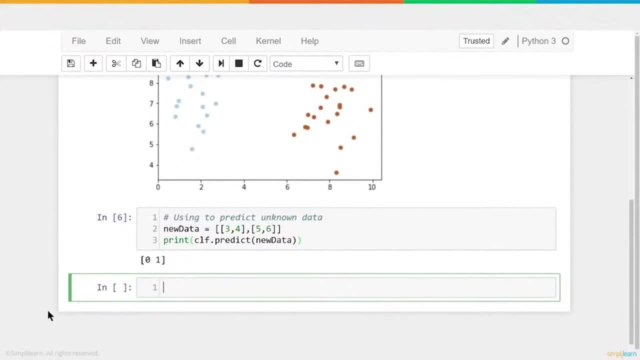 let's see what that looks like And you'll see 0, 1. so predicted the first one, the 3, 4, is going to be on the one side and the 5- 6 is going to be on the other side. So one came out as an alligator and one came out as a. 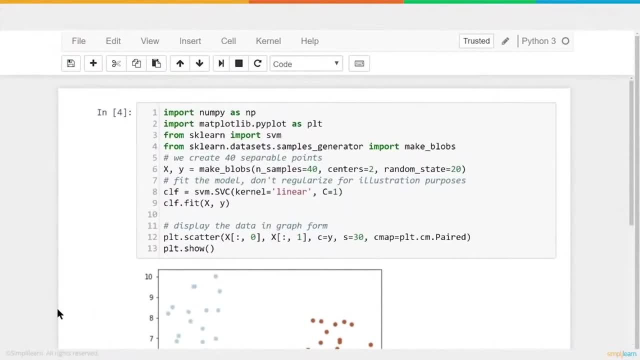 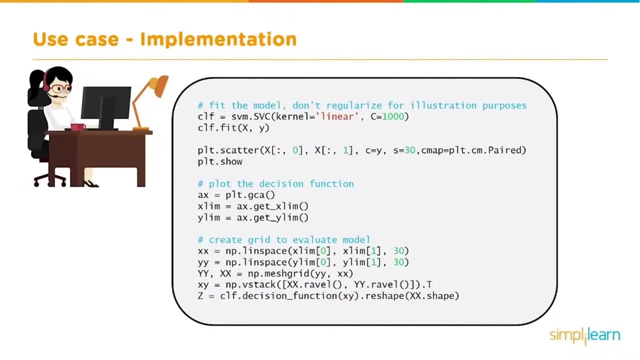 crocodile. Now that's pretty short explanation for the setup, but really we want to dig in and see what it's going on behind the scenes and let's see what that looks like. So the next step is to dig in deep and find out what's going on. 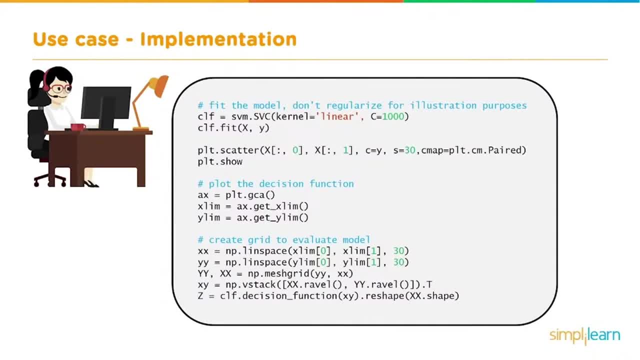 behind the scenes and also put that in a nice, pretty graph. We're going to spend more work on this- and we did actually generating the original model, and you'll see here that we go through a few steps and I'll move this over to our editor in. 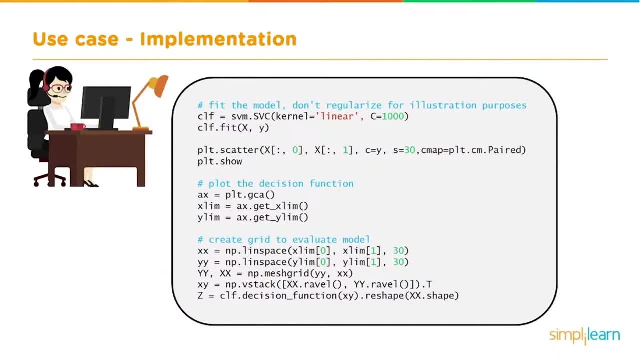 just a second. We come in, we create our original data. it's exactly identical to the first part and I'll explain why we redid that and show you how not to redo that. And then we're going to go in there and add in those lines. We're going to 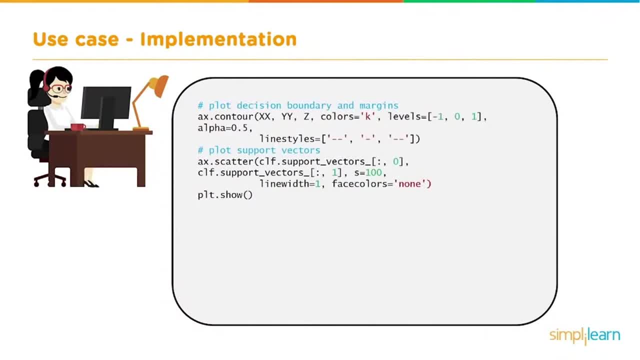 see what those lines look like and how to set those up. And finally, we're going to plot all that on here and show you how to do that. So we're going to do that and we're going to show it, And you'll get a nice graph with. 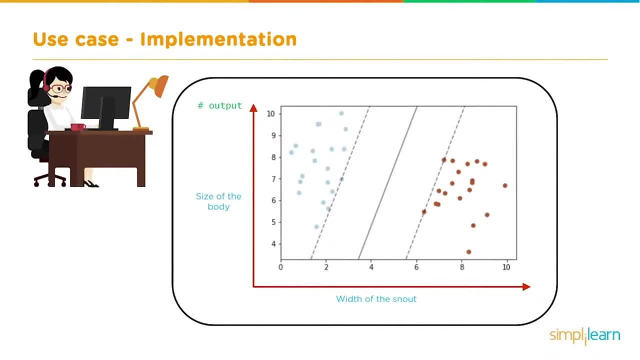 the what we saw earlier when we were going through the theory behind this, where it shows the support vectors and the hyperplane And those are done, where you can see the support vectors as the dashed lines and the solid line, which is the hyperplane. Let's get that into our Jupiter notebook Before I scroll down to 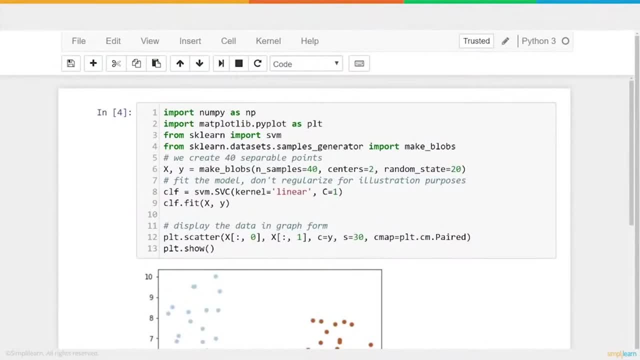 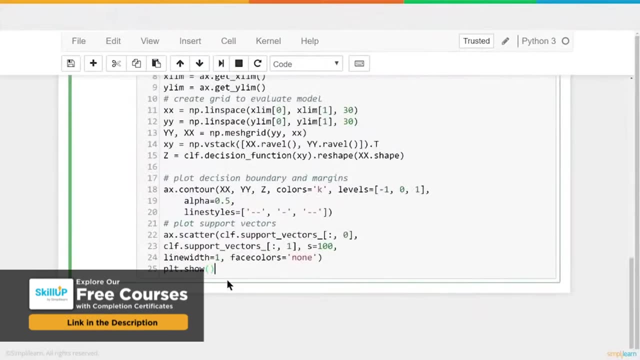 a new line. I want you to notice line 13. it has plot show And we're going to talk about that here in just a second. but let's scroll down to a new line down here, that code in, and you'll see that the plot show has moved down below. Let's scroll up a little. 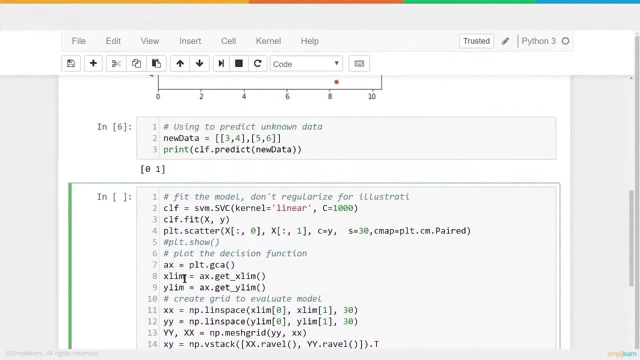 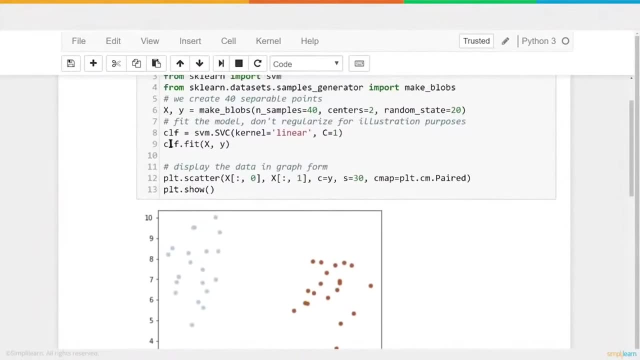 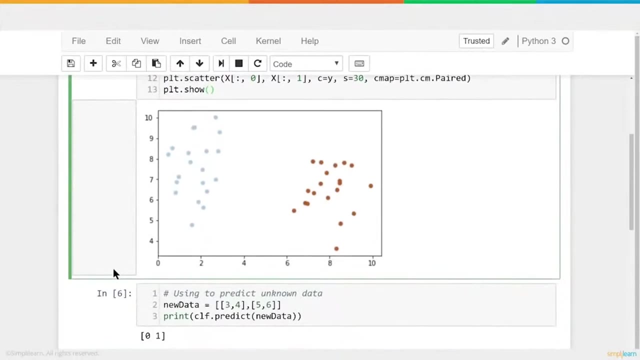 bit. and if you look at the top here of our new section, one, two, three and four is the same code we had before. and let's go back up here and take a look at that. We're gonna fit the values on our SVM and then we're gonna plot, scatter it and then we're gonna do a plot show. So you should be. 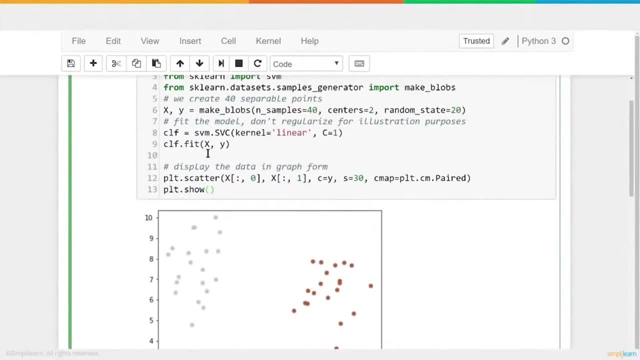 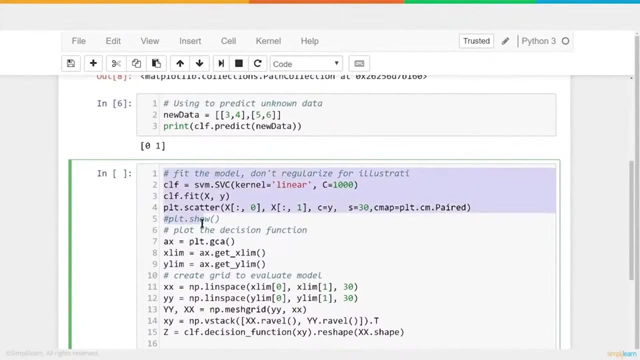 asking: why are we redoing the same code? Well, when you do the plot show, that blanks out what's in the plot. So once I've done this plot show, I have to reload that data. Now we could do this simply by removing it up here, rerunning it and then coming down here, and then we wouldn't have to rerun these. 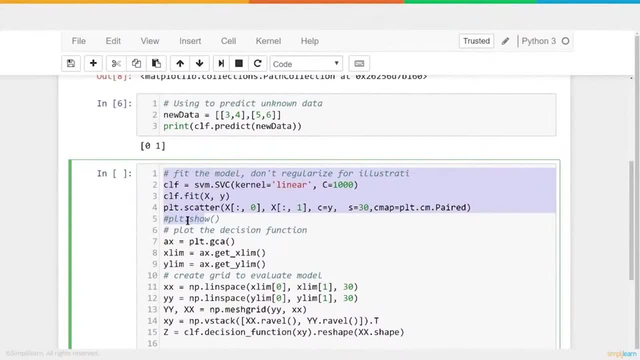 first four lines of code. Now in this it doesn't matter too much and you'll see the plot show was down here and then removed right there on line five. I'll go ahead and just delete that out of there, because we don't want to blank out our screen. We want to move on to the next setup. So 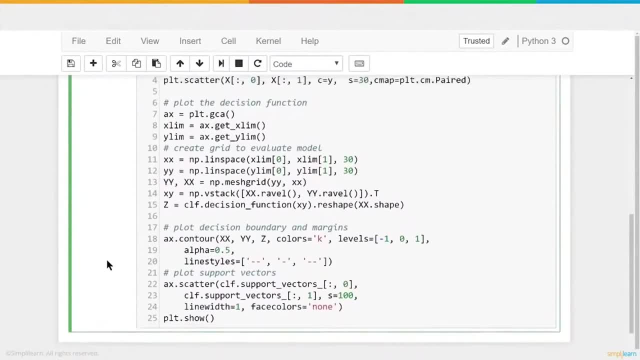 we can go ahead and just skip the first four lines, because we did that before, and I'll just skip the first four lines because we did that before. So we can go ahead and just skip the first four lines, because we did that before. and- And let's take a look at the ax equals pltgca. 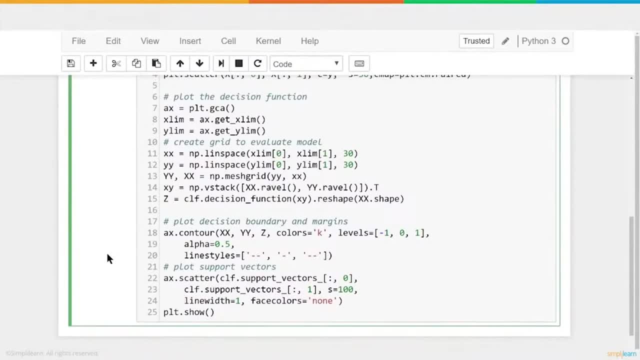 Now, right now, we're actually spending a lot of time just graphing. That's all we're doing here. So this is how we display a nice graph with our results and our data. Ax is a very standard used variable when you're talking about plt. 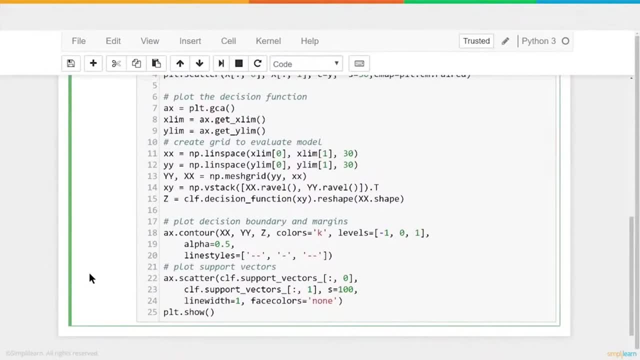 And it's just setting it to that axis, the last axis in the plt. It can get very confusing if you're working with many different layers of data on the same graph And this makes it very easy to reference the ax. So this reference is looking at the plt that we created. 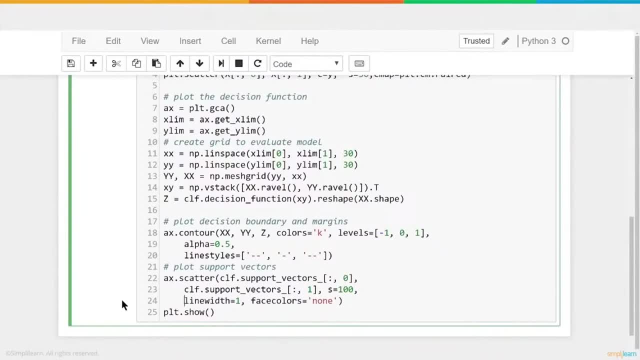 And we already mapped out our two blobs on. And then we want to know the limits, So we want to know how big the graph is. We can find out the x limit and the y limit simply with the get x limit and get y limit commands, which. 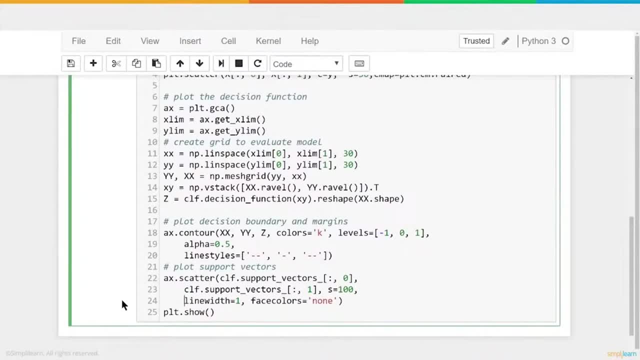 is part of our matplot library, And then we're going to create a grid And you'll see down here we've set the variable xx equal to nplinespace, x, limit 0,, x, limit 1, comma 30. And we've done the same thing for 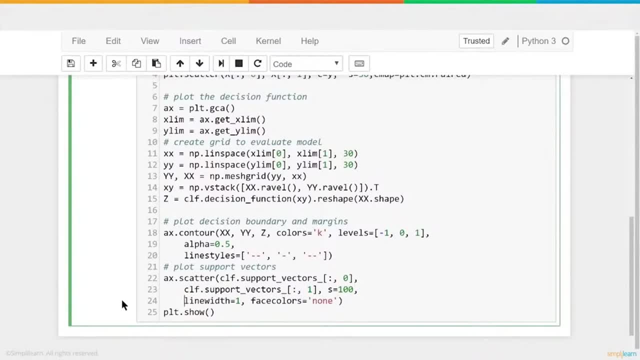 the y space. And then we're going to go in here and we create a mesh grid And this is a numpy command. So we're back to our numbers, Python. Let's go through what these numpy commands mean with the line space and the mesh grid. 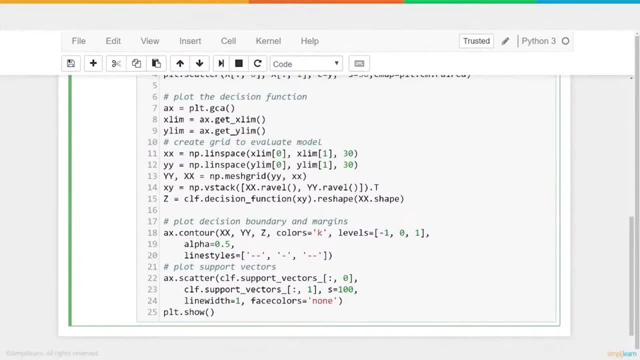 We've taken xx small xx equals nplinespace, And we have our x limit 0 and our x limit 1.. And we're going to create 30 points on it, And we're going to do the same thing for the y axes. 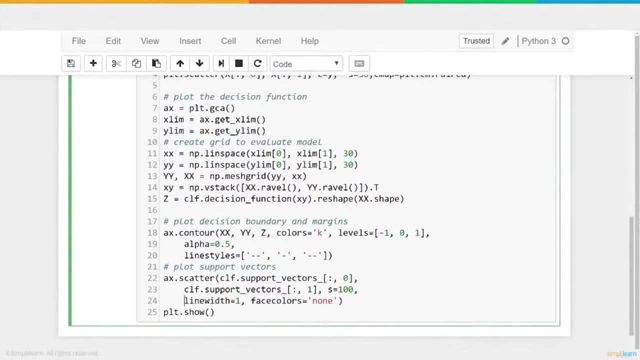 Now, this has nothing to do with our evaluation. It's all we're doing. What we're doing is we're creating a grid of data, And so we're creating a set of points between 0 and the x limit. We're creating 30 points, and the same thing with the y. 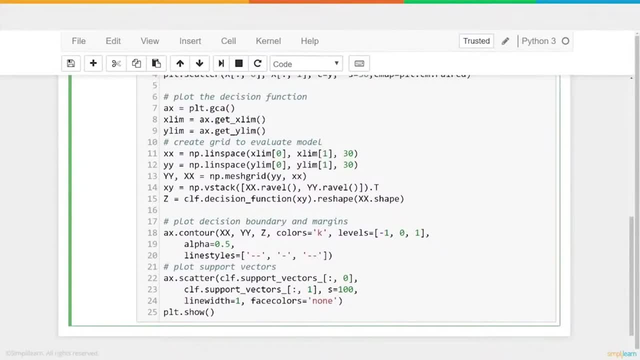 And then the mesh grid loops those all together so it forms a nice grid. So if we were going to do this, say between the limit 0 and 10, and do 10 points, we would have a 0, 0, 1, 1, 0, 1, 0, 2,, 0, 3,. 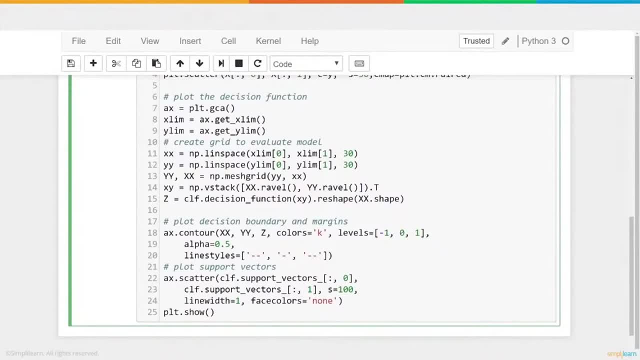 0,, 4 to 10, and so on. You can just imagine a point at each corner of one of those boxes And the mesh grid combines them all. So we take the y1.. y1 and the xx we created and creates the full grid. 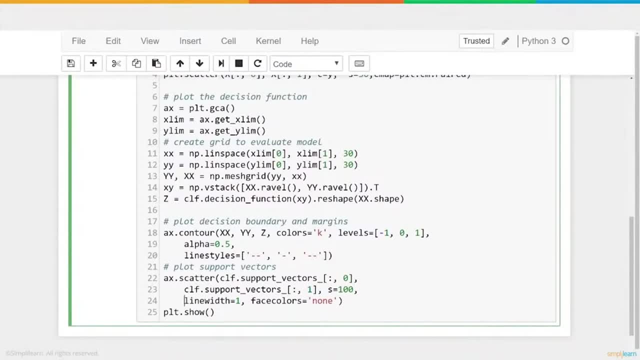 And we've set that grid into the yy coordinates and the xx coordinates. Now, remember we're working with Numbi and Python. We like to separate those We like to have instead of it being x comma 1, x comma y. 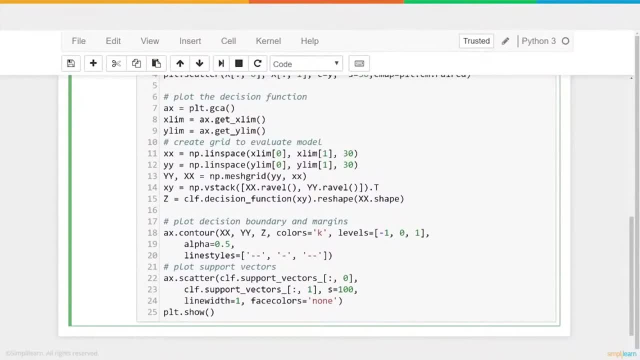 and then x2 comma y2. in the next set of data it would be a column of x's and a column of y's, And that's what we have here is we have a column of y's, And we put it as a capital yy, and a column of x's capital. 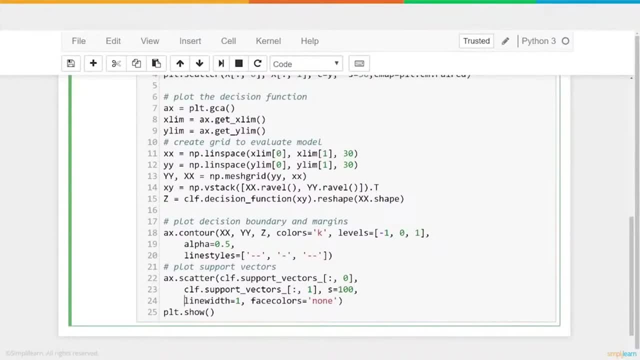 xx, With all those different points being listed, And finally we get down to the Numbi VStack. Just as we created those in the mesh grid, we're now going to put them all into one array, xy array, Now that we've created the stack of data points. 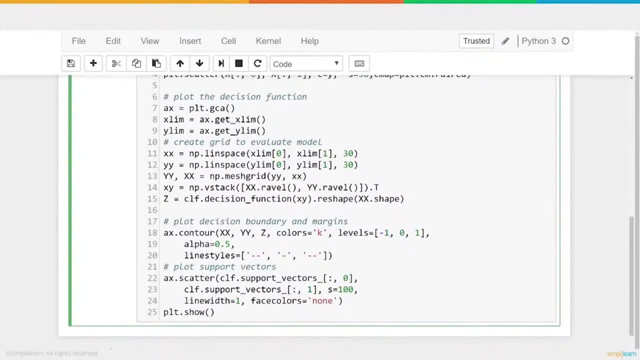 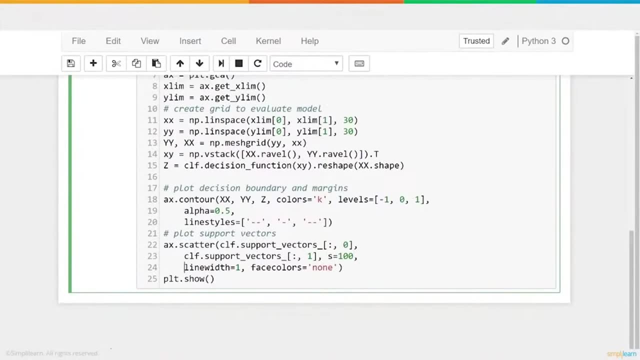 we're going to do something interesting here. We're going to create a value, z, And the z equals the CLF. That's our support vector machine. we created and we've already trained And we have a dot decision function And we're going to put the xy in. 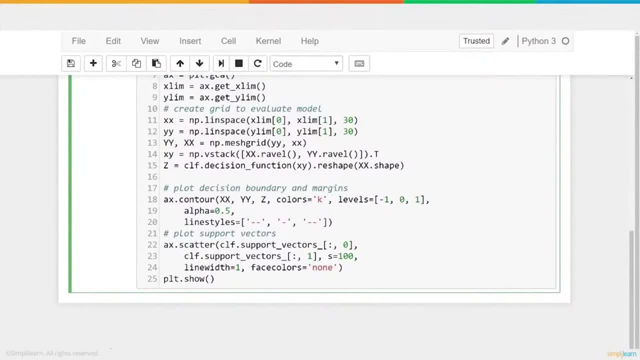 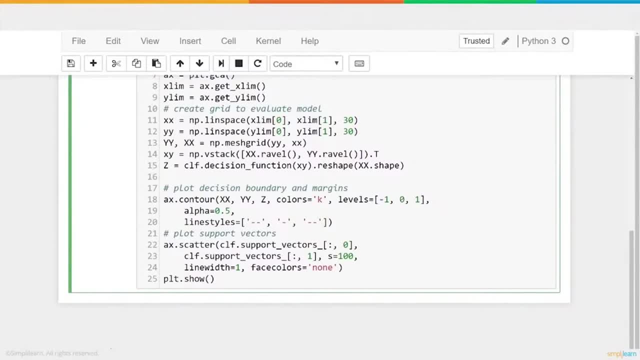 We're going to reshape it And you'll see that we have the xx dot shape in here. This literally takes the xx, resets it up connected to the y And the z value lets us know whether it is the left-hand side. 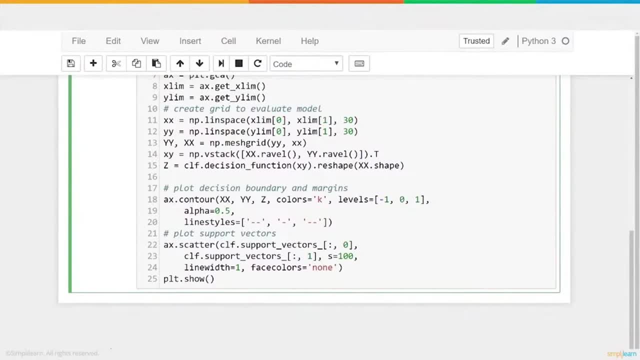 It's going to generate three different values. the z value does And it'll tell us whether that data is a support vector to the left, the hyperplane in the middle or the support vector to the right. So it generates that. It generates three different values for each of those points. 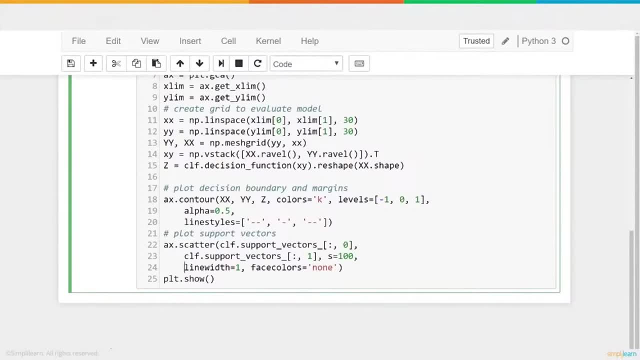 And those points have been reshaped so that they're right on the line, on those three different lines. So we've set all of our data up, We've labeled it to three different areas And we reshaped it And we've just taken 30 points in each direction. 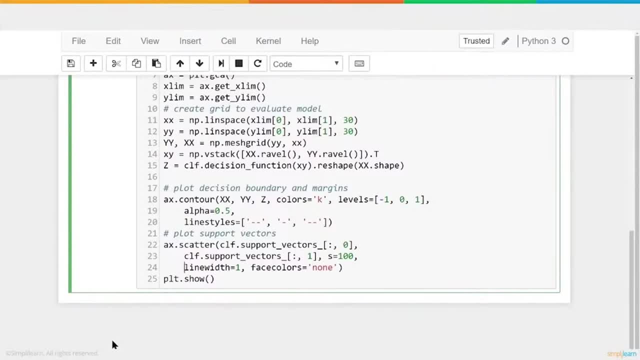 If you do the math, you have 30 times 30. So that's 900 points of data, And we separated it between the three lines and reshaped it to fit those three lines. We can then go back to our map plot library. 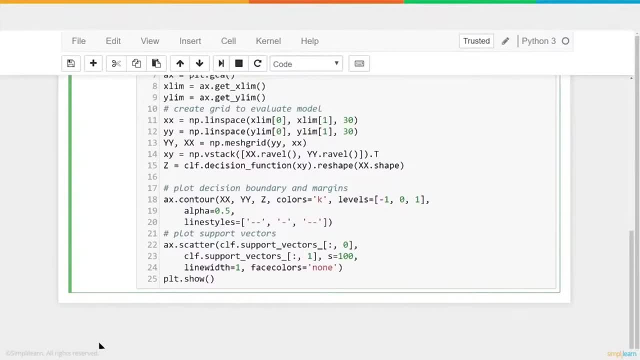 We've created the ax And we're going to create a contour And you'll see, here we have contour Capital XX, capital YY. These have been reshaped to fit those lines. Z is the labels. So now we have the three different points. 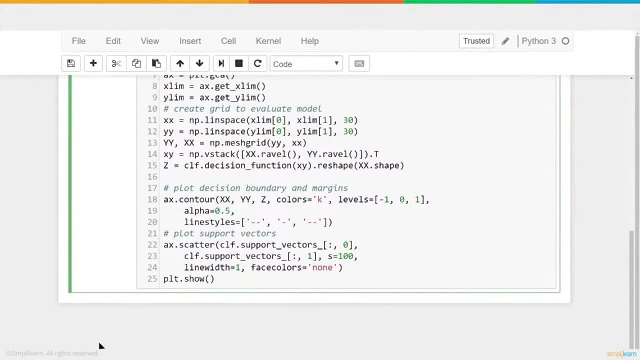 with the labels in there And we can set the colors. equals K And I told you we had three different labels But we have three levels of data. The alpha just makes it kind of see-through, So it's only 0.5 of the value in there. 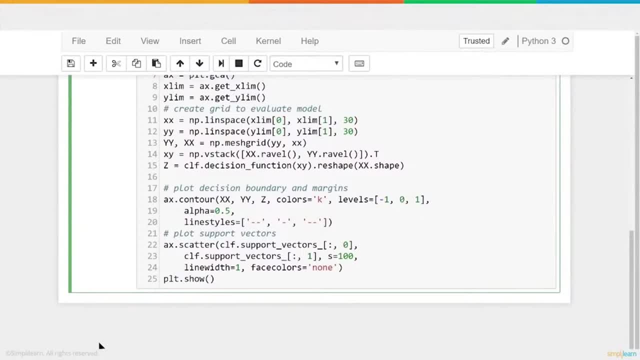 So when we graph it, the data will show up from behind it wherever the lines go. And finally, the line styles. This is where we set the two support vectors to be dash, dash lines, And then a single one is just a straight line. 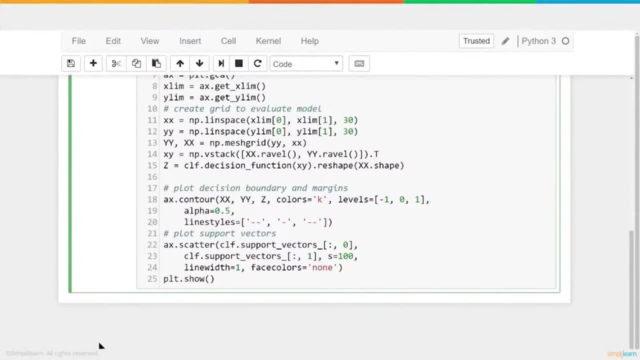 That's what all that setup does. And then, finally, we take our axscatter. We're going to go ahead and plot the support vectors, But we've programmed it in there so that they look nice like the dash, dash line and the dash line on that grid. 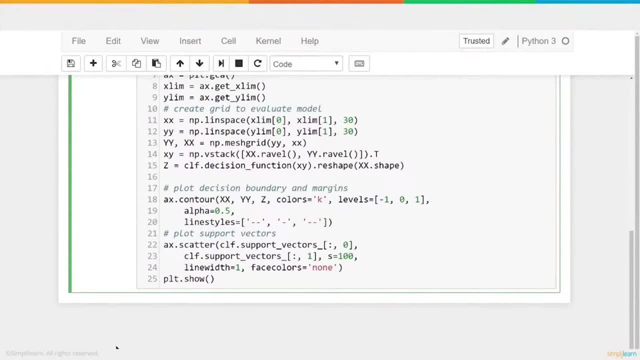 And you can see here, when we do the clfsupportvectors, we are looking at column 0 and column 1.. And then again we have the s equals 100.. So we're going to make them larger And the line width equals 1.. 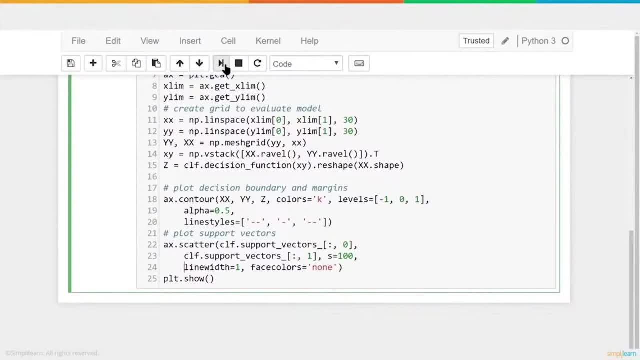 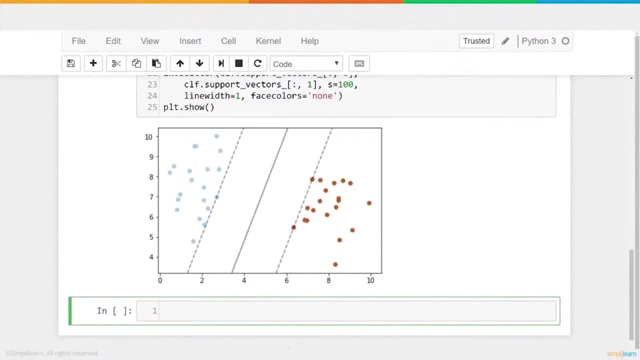 Face colors equals none. Let's take a look and see what that looks like when we show it And you can see when we get down to our end result. it creates a really nice graph. We have our two support vectors and dash lines. 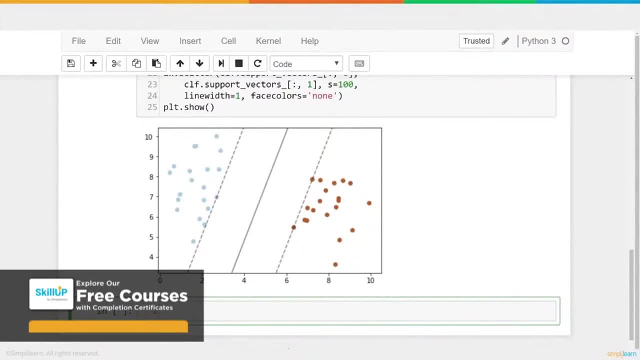 And they have the near data. So you can see those two points, or in this case the four points where those lines nicely cleave the data, And then you have your hyperplane down the middle, which is as far from the two different points as possible. 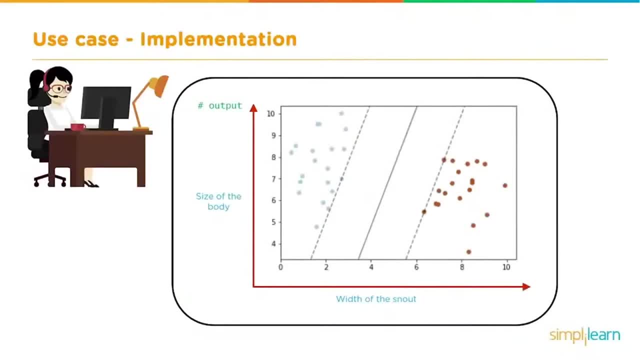 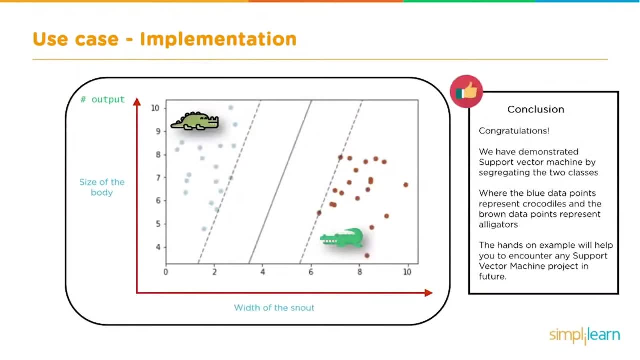 creating the maximum distance. So you can see that we have our nice output for the size of the body and the width of the snout, And we've easily separated the two groups of crocodile and alligator. Congratulations, You've done it. 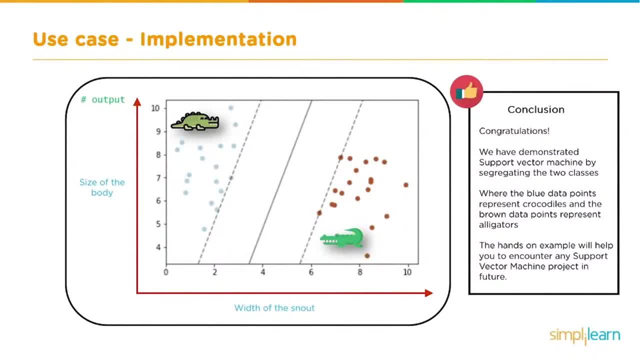 We've made it. Of course, these are pretend data for our crocodiles and alligators, But this hands-on example will help you to encounter any support vector machine projects in the future And you can see how easy they are to set up and look at. 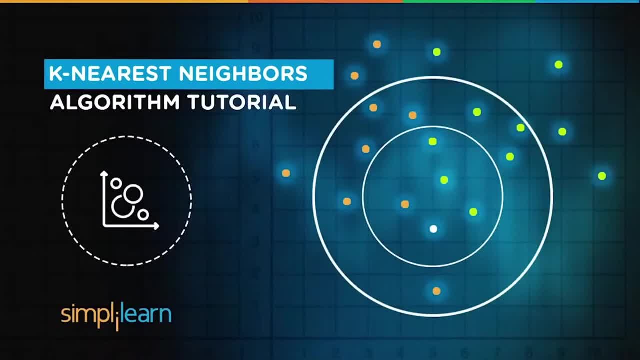 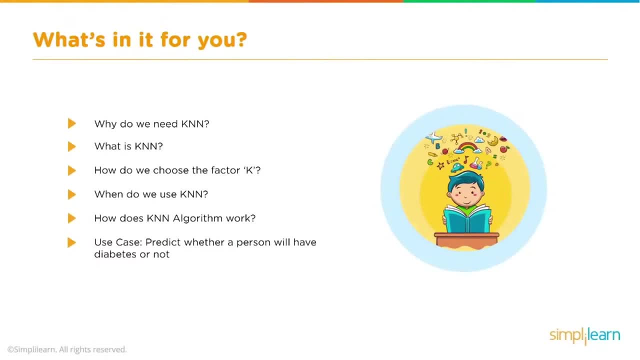 in depth And we're going to cover the k nearest neighbors. a lot referred to as knn And knn is really a fundamental place to start in the machine learning. It's the basis of a lot of other things And just the logic behind it is easy to understand. 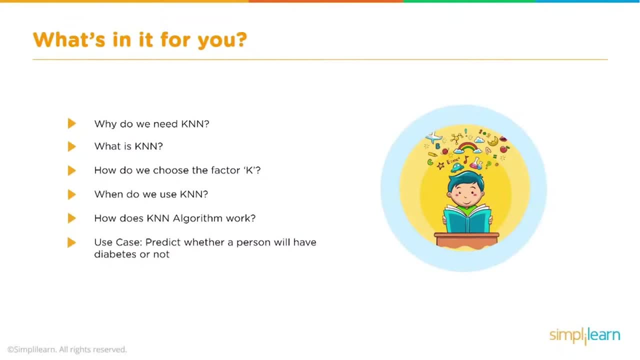 and incorporated in other forms of machine learning. So, today, what's in it for you? Why do we need knn? What is knn? How do we choose the factor k? When do we use knn? How does knn algorithm work? 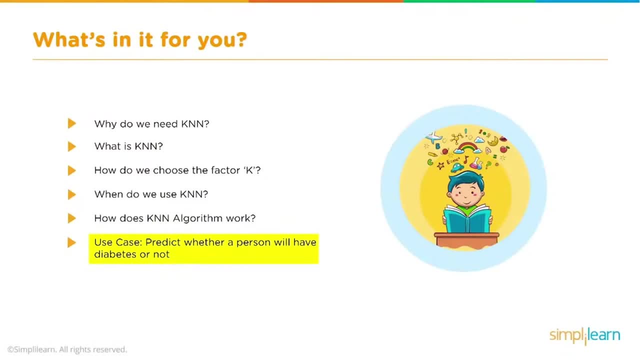 And then we'll dive into my favorite part: the use case Predict whether a person will have diabetes or not. That is a very common and popular used data set. as far as testing out models and learning how to use the different models in machine learning, 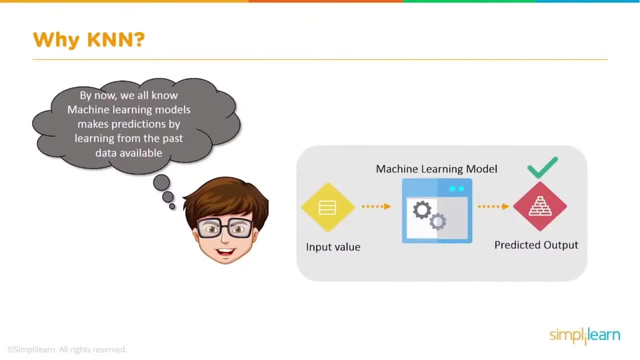 By now we all know machine learning models make predictions by learning from the past data available. So we have our input values. Our machine learning model builds on those inputs of what we already know And then we use that to create a predicted output. 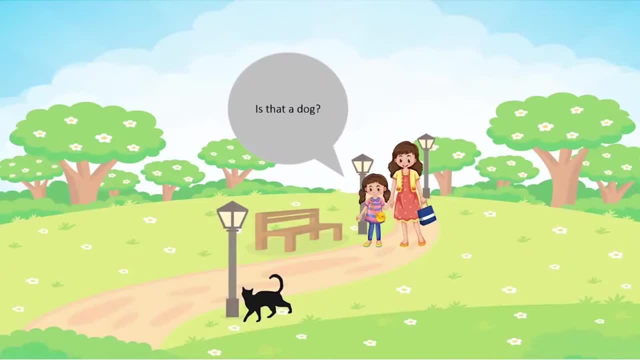 Is that a dog? Little kid looking over there watching the black cat cross their path? No dear, You can differentiate between a cat and a dog based on their characteristics: Cats. Cats have sharp claws, uses to climb, smaller length of ears. 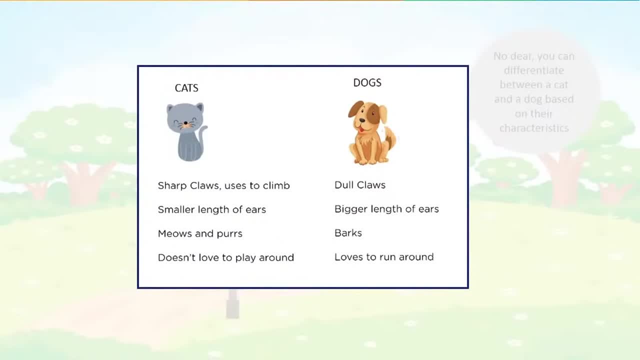 meows and purrs, doesn't love to play around. Dogs have dull claws, bigger length of ears, barks. loves to run around. You usually don't see a cat running around people, although I do have a cat that does that where dogs do. 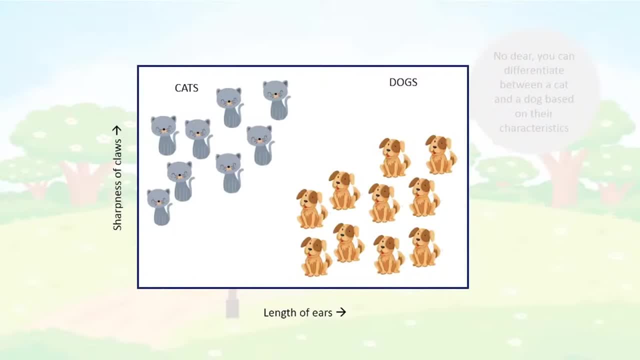 And we can look at these. We can evaluate the sharpness of the claws- How sharp are their claws- And we can evaluate the length of the ears, And we can usually sort out cats from dogs based on even those two characteristics. Now tell me if it is a cat or a dog. 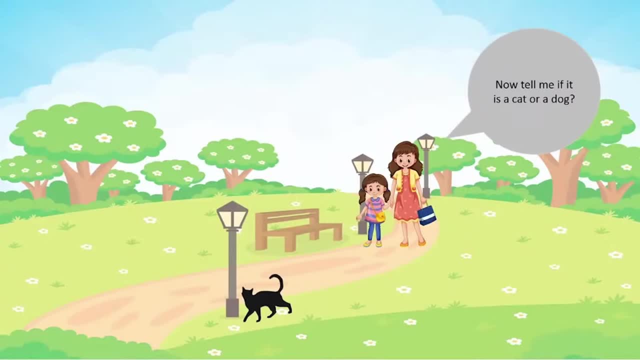 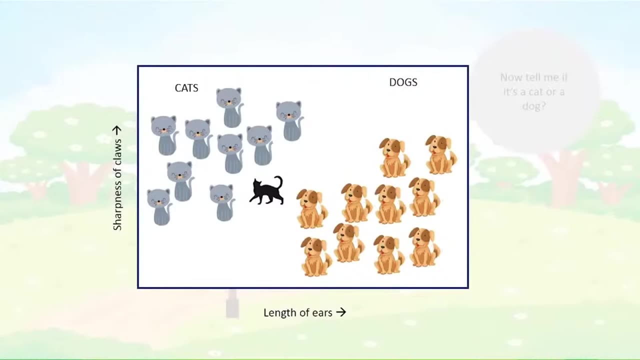 Not a question. Usually little kids know cats and dogs by now, Unless they live in a place where there's not many cats or dogs. So if we look at the sharpness of the claws, the length of the ears and we can see that the cat has smaller ears and sharper claws. 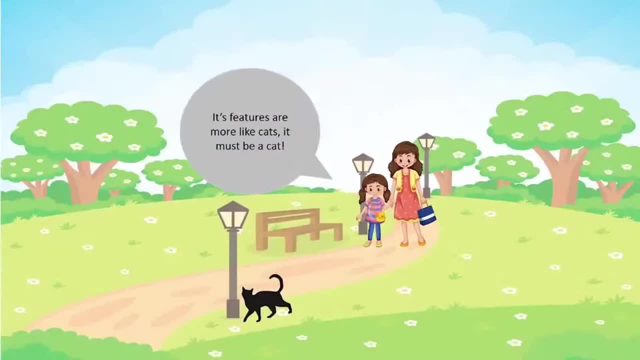 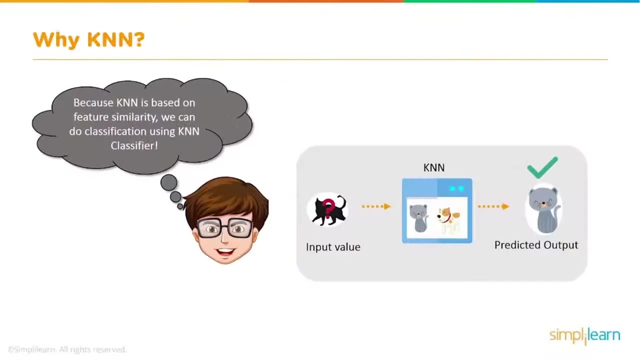 than the other animals. Its features are more like cats. It must be a cat- Sharp claws, Length of ears- And it goes in the cat group. Because KNN is based on feature similarity, we can do classification using KNN classifier. 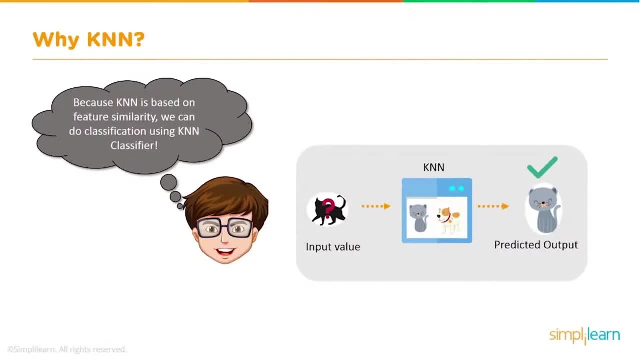 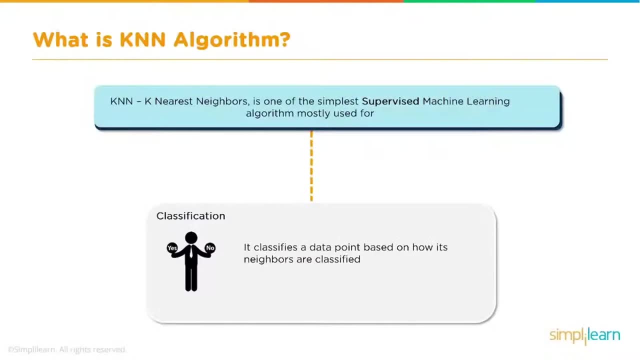 So we have our input value, the picture of the black cat. It goes into our trained model And it predicts that this is a cat coming out. So what is KNN? What is the KNN algorithm? K nearest neighbors is what that stands for. 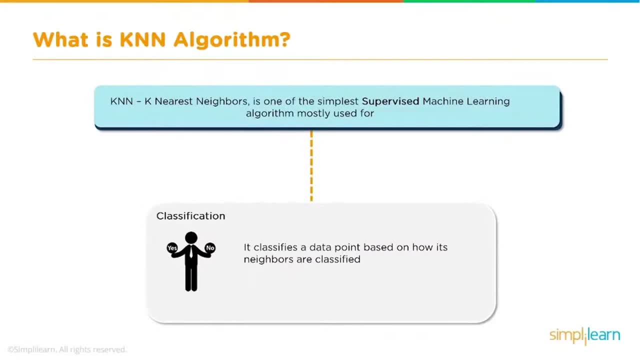 It's one of the simplest supervised machine learning algorithms mostly used for classification. So we want to know: is this a dog or it's not a dog? Is it a cat or not a cat? It classifies a data point based on how its neighbors are classified. 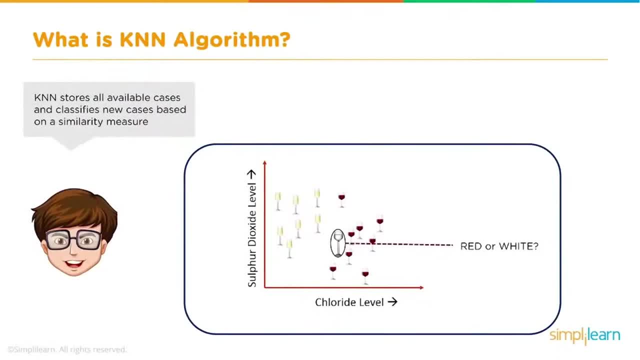 KNN stores all available cases and classifies new cases based on a similarity measure. And here we've gone from cats and dogs right into wine, another favorite of mine. KNN stores all available cases and classifies new cases based on a similarity measure. 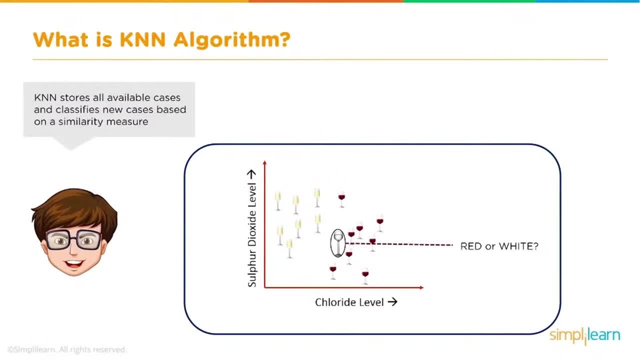 And here you see, we have a measurement of sulfur dioxide versus the chloride level And then the different ones, The different wines they've tested and where they fall on that graph, based on how much sulfur dioxide and how much chloride K, and KNN is a perimeter that refers. 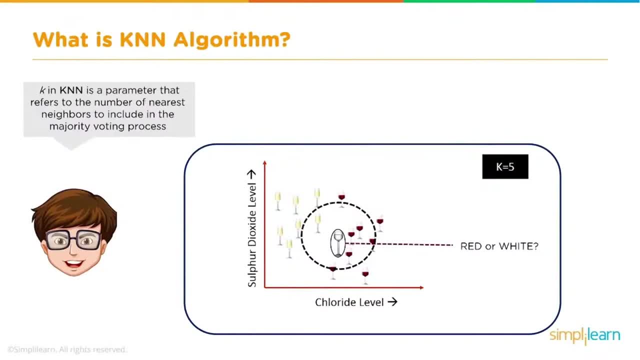 to the number of nearest neighbors to include in the majority of the voting process, And so if we add a new glass of wine there, red or white, we want to know what the neighbors are. In this case, we're going to put K equals 5.. 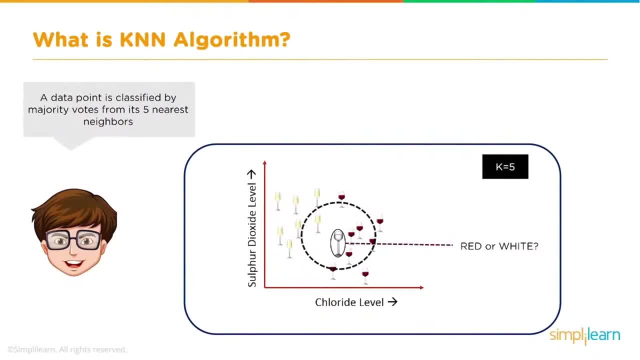 We'll talk about K in just a minute. A data point is classified by the majority of votes from its five nearest neighbors. Here, the unknown point would be classified as red, since four out of five neighbors are red. So how do we choose K? 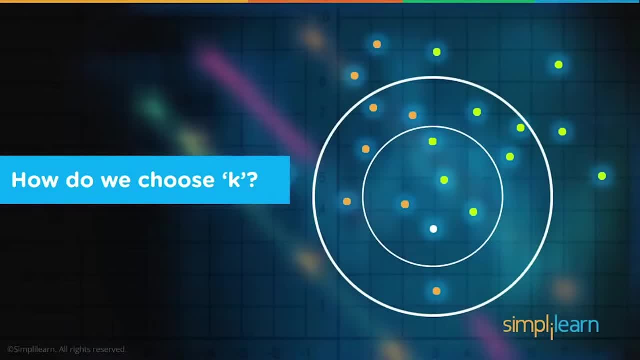 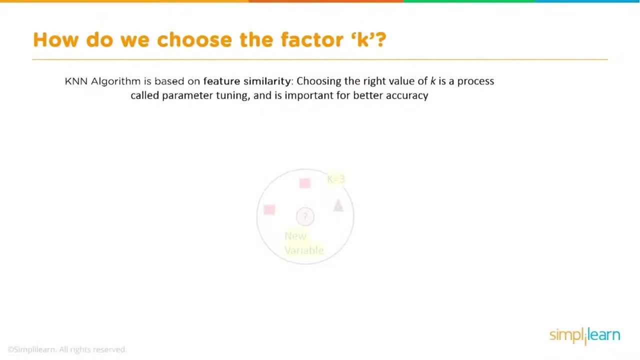 How do we know K equals 5?? I mean, that was the value we put in there, so we're going to talk about it. How do we choose the factor K? KNN algorithm is based on feature similarity. Choosing the right value of K is a process called parameter. 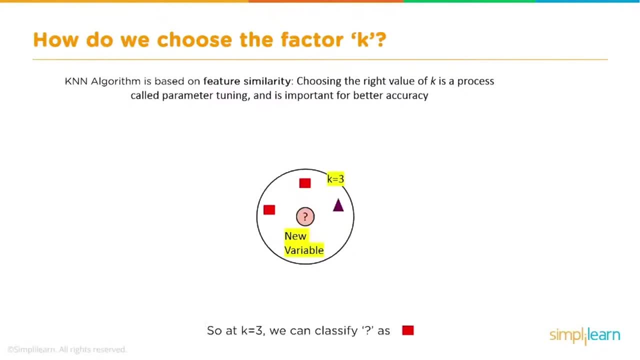 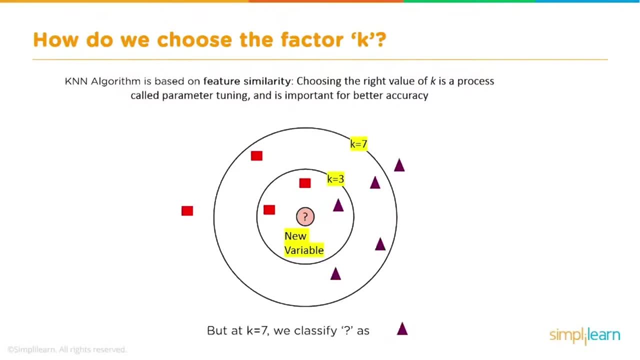 We're going to look at the three nearest neighbors. We're going to say this is a square And if we put K equals to 7, we classify it as a triangle, depending on what the other data is around it. And you can see as the K changes depending. 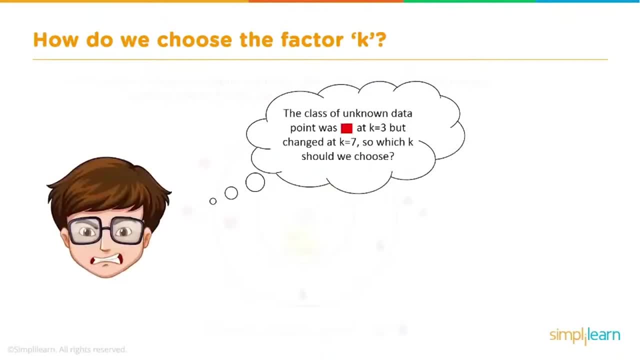 on where that point is. that drastically changes your answer And we jump, here We go. how do we choose the factor of K? You'll find this in all machine learning: Choosing these factors. that's the face you get. It's like: oh my gosh, did I choose the right K? 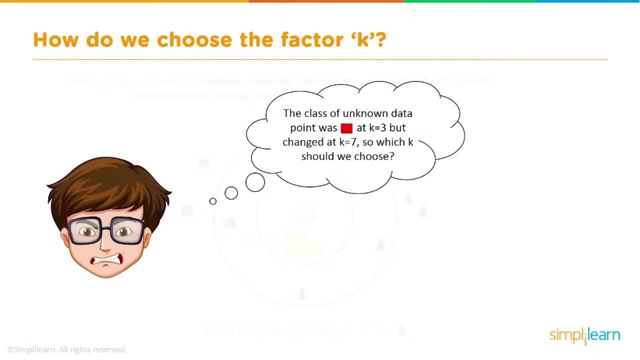 Did I set it right my values in whatever machine learning tool you're looking at, so that you don't have a huge bias in one direction or the other. and in terms of KNN, the number of K, if you choose it too low, the bias is based on- it's just too noisy. 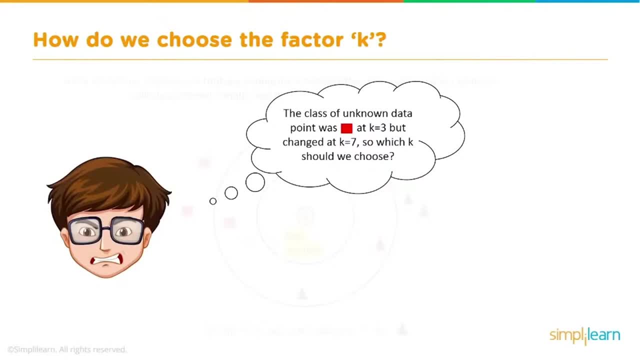 it's just right next to a couple things and it's going to pick those things and you might get a skewed answer and if your K is too big then it's going to take forever to process. so you're going to run into processing issues and resource issues. so what we do, the most common use and there's other options for. 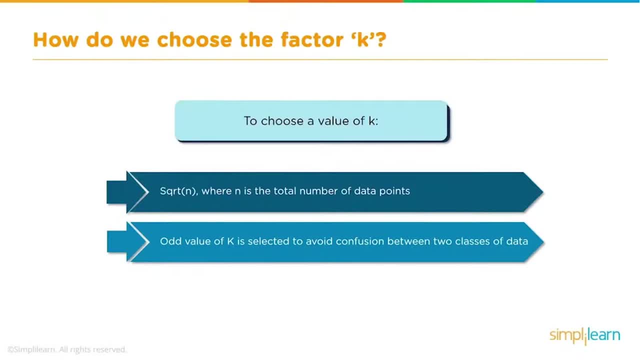 choosing K is to use the square root of in. so it is a total number of values you have. you take the square root of it. in most cases you also if it's an even number. so if you're using, like this case, squares and triangles, if it's even you. 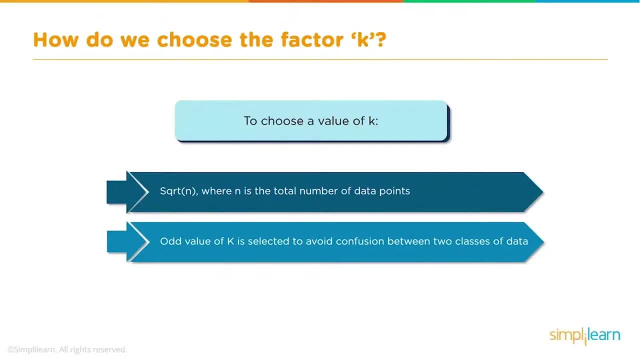 want to make your K value odd. that helps it select better. so, in other words, you're not going to have a balance between two different factors that are equal. so usually take the square root of in and, if it's even, you add one to it or subtract one from it, and that's where you get the K value from. that is the. 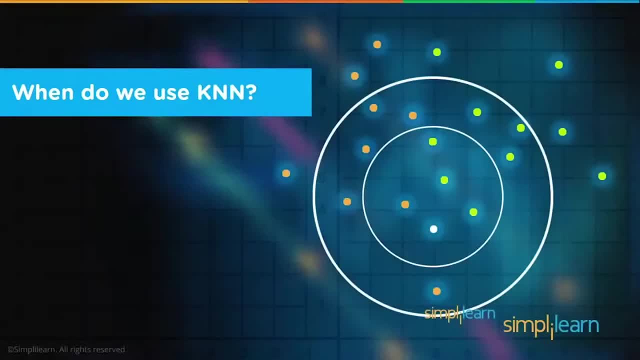 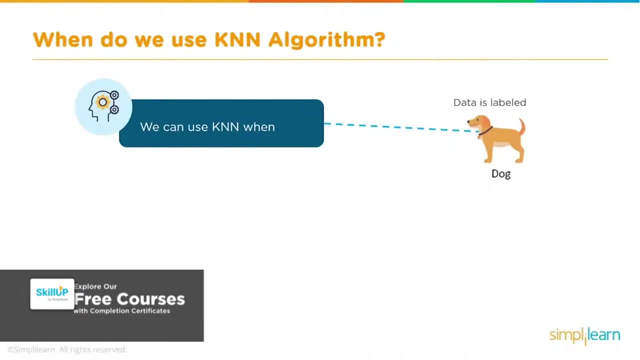 most common use and it's pretty solid. it works very well. when do we use KNN? we can use KNN when data is labeled, so you need a label on it. we know we have a group of pictures with dogs, dogs, cats, cats. data is noise free and so you can. 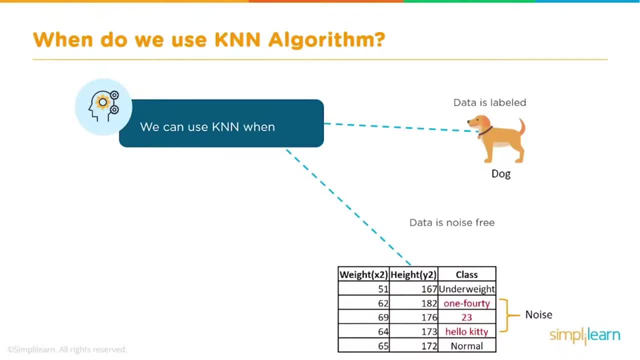 see here, when we have a class and we have, like, underweight 140, 23, Hello Kitty, normal, that's pretty confusing. we have a high variety of data coming in so it's very noisy and that would cause an issue. data set is small, so we're usually 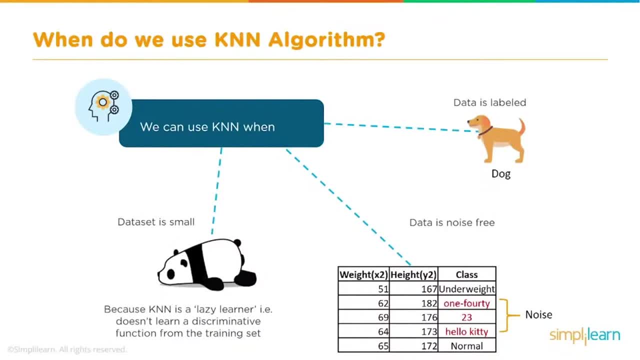 working with small data sets that are very noisy and that would cause an issue. data set is small, so we're usually working with small our data sets, where I mean you might get into gig of data if it's really clean, doesn't have a lot of noise, because KNN is a lazy learner, ie it doesn't learn a. 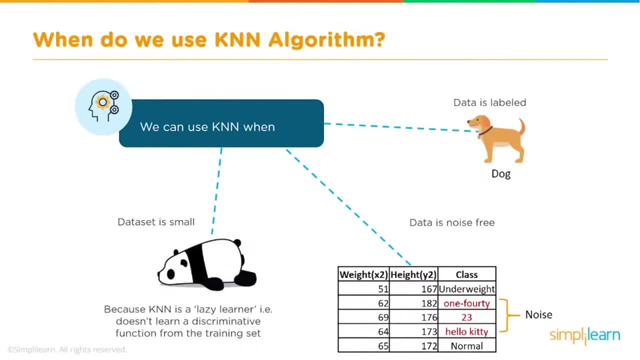 discriminative function from the training set, so it's very lazy. so if you have very complicated data and you have a large amount of it, you're not going to use the KNN, but it's really great to get a place to start, even with large data. 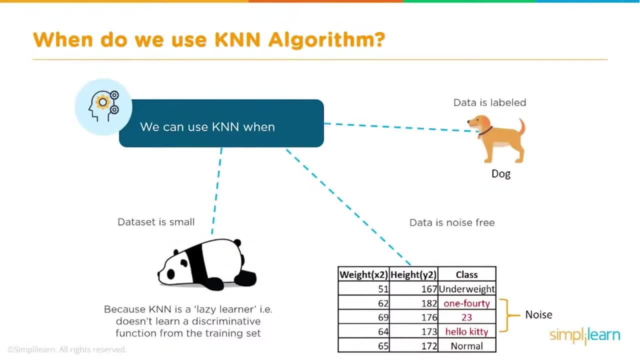 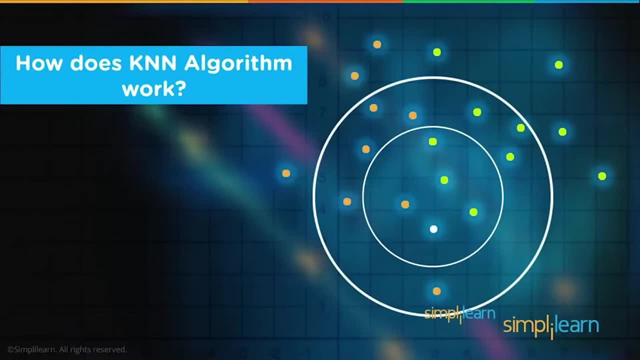 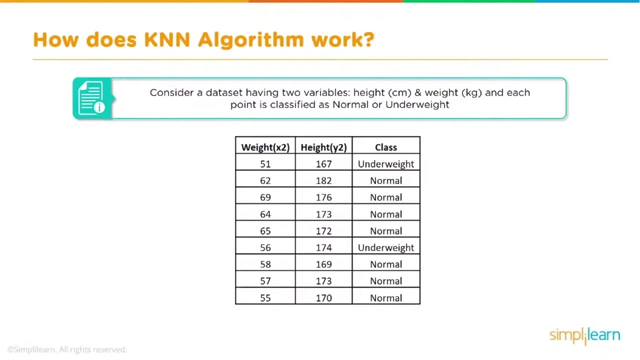 you can sort out a small sample and get an idea of what that looks like. using the KNN and also just using for smaller data sets, KNN works really good. how does a KNN algorithm work? consider a data set having two variables- height in centimeters and weight in kilograms- and each point is classified as normal or 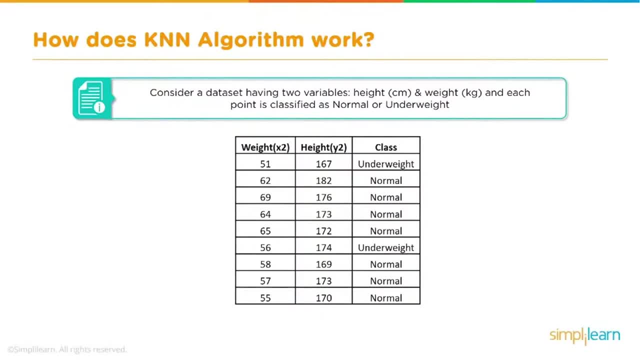 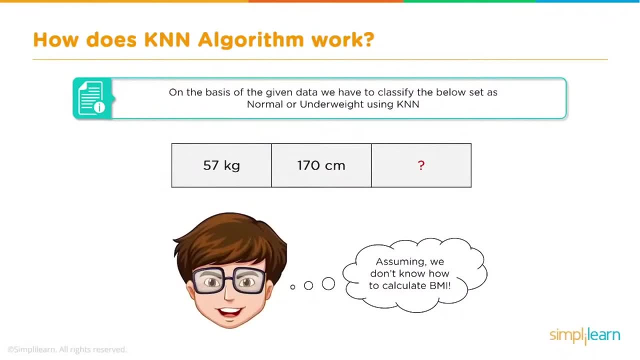 underweight. so we can see right here. we have two variables, you know, true, false, or either normal or they're not. they're underweight. on the basis of the given data, we have to classify the below set as normal or underweight using KNN. so if 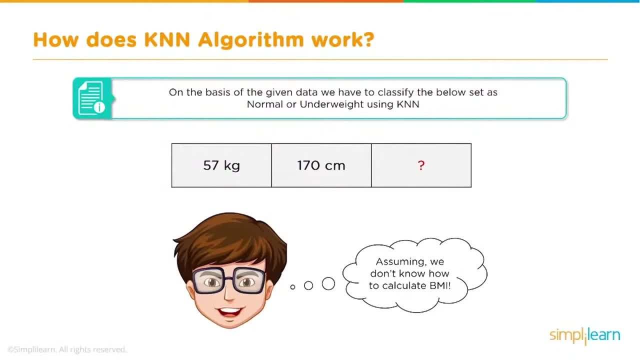 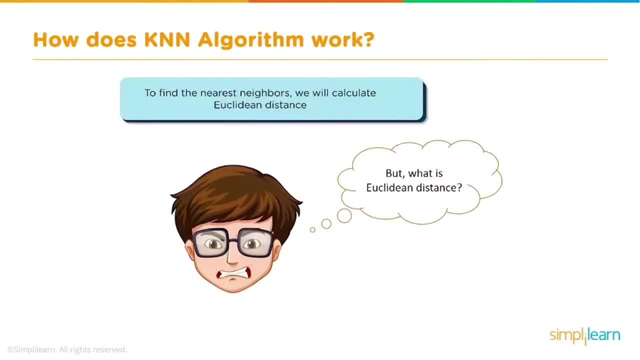 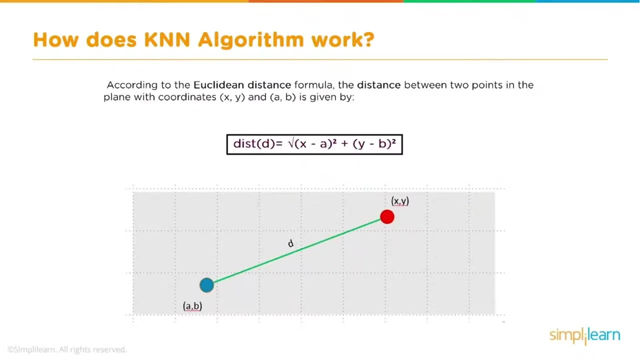 we have new data coming in this as 57 kilograms and 177 centimeters. is that going to be normal or underweight? to find the nearest neighbors will calculate the Euclidean distance according to the Euclidean distance formula: the distance between two points in the plane with the coordinates XY and. 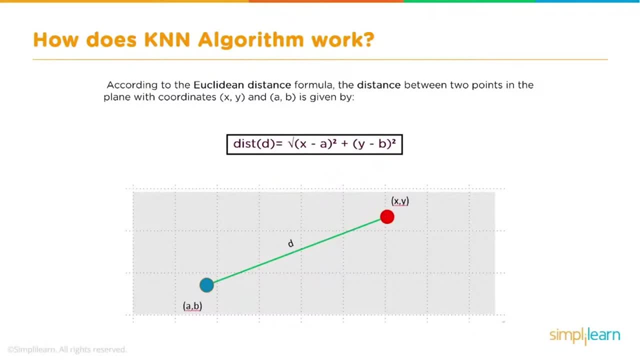 AB is given by distance, D equals the square root of X minus a squared, plus Y minus B squared. and you can remember that from the two edges of a triangle, computing the third edge, since we know the x side in the y side, let's calculate it to understand. 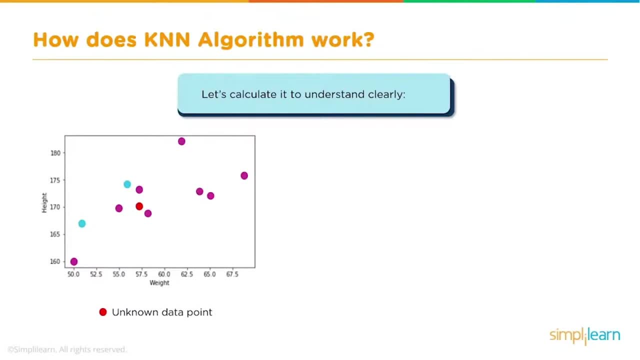 clearly. So we have our unknown point- We placed it there in red- And we have our other points where the data is scattered around. The distance d1 is the square root of 170 minus 167 squared plus 57 minus 51 squared, which is about 6.7.. And distance 2 is about: 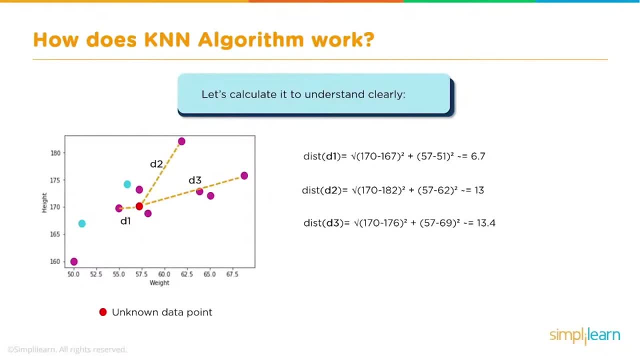 13. And distance 3 is about 13.4.. Similarly, we will calculate the Euclidean distance of the unknown data point from all the points in the data set And because we're dealing with small amount of data, that's not that hard to do, It's actually pretty quick- for. 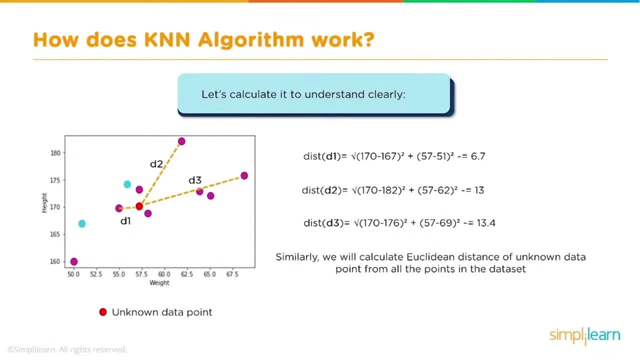 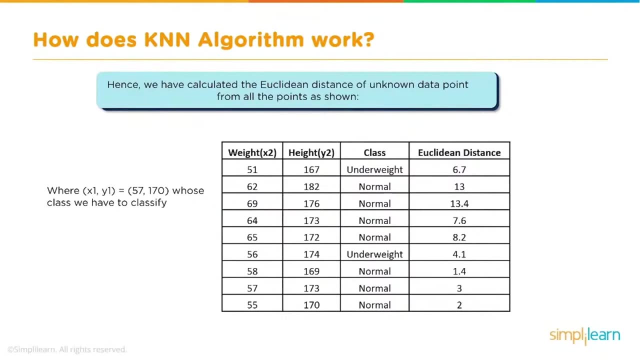 a computer And it's not really complicated math. So you can just see how close is the data based on the Euclidean distance. Hence we have calculated the Euclidean distance of unknown data point from all the points as shown, where x1 and y1 equal 57 and 170,. 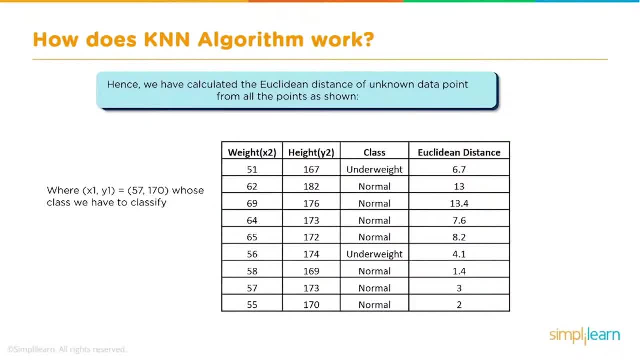 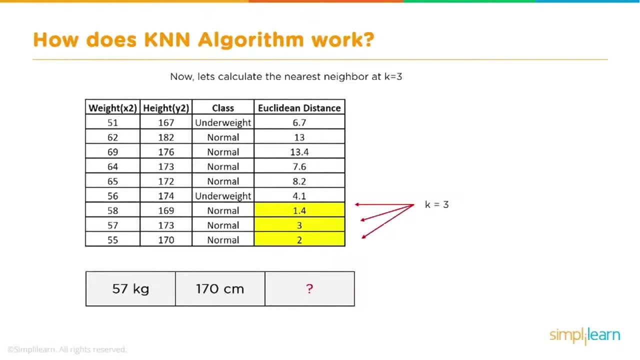 whose class we have to classify. So now we're looking at that, We're saying: well, here's the Euclidean distance. Who's going to be their closest neighbors? Now let's calculate the nearest neighbor at: k equals 3. And we can see the three closest. 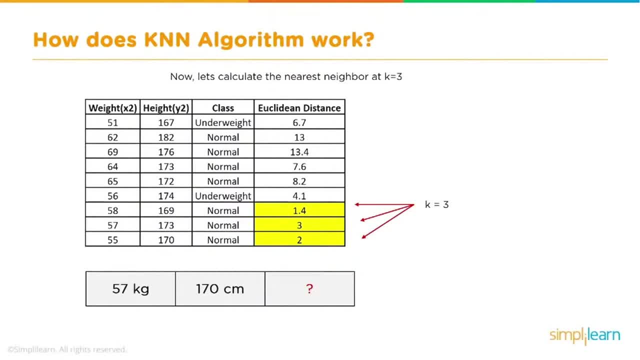 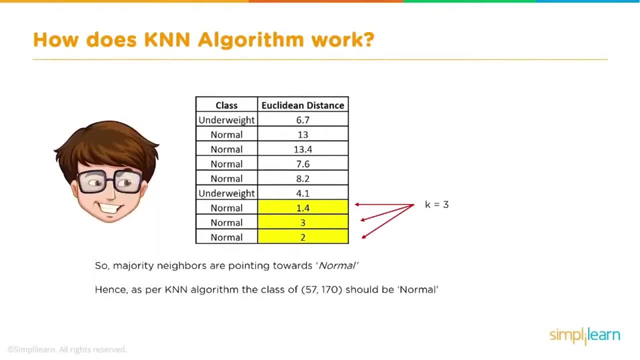 neighbors puts them at normal, And that's pretty self-evident. When you look at this graph, it's pretty easy to say: OK, we're just voting Normal, normal, normal. Three votes for normal. This is going to be a normal weight. So majority of neighbors are pointing. 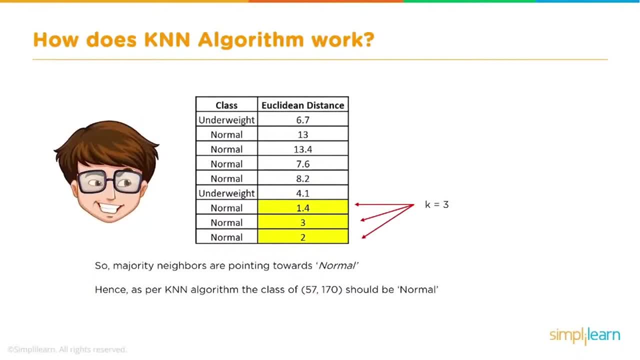 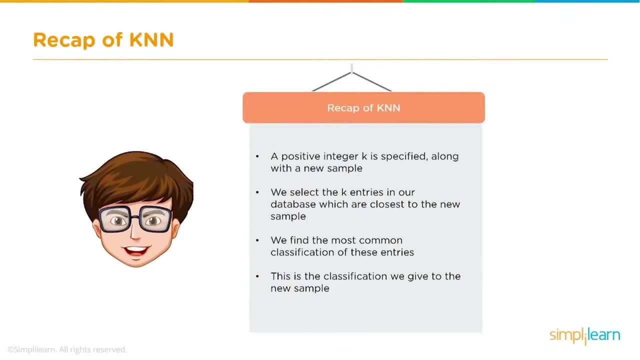 towards normal. Hence, as per KNN algorithm, the class of 57, 170 should be normal. So a recap of KNN Positive integer k is specified along with a new sample. We select the k entries in our database which are closest to the new sample. We find the most common classification. 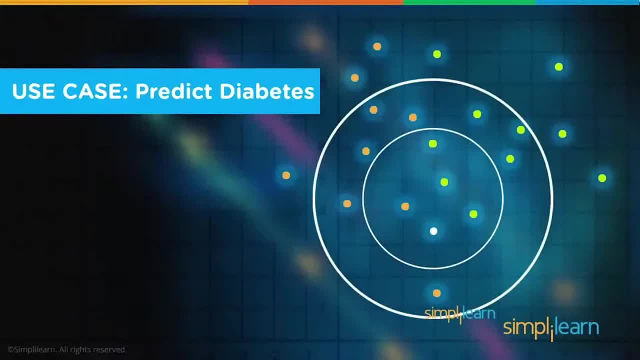 of these entries. This is the classification we give to the new sample. So, as you can see, it's pretty straightforward. We're just looking for the closest things that match what we got. So let's take a look and see what that looks like in a use case in Python. So let's dive. 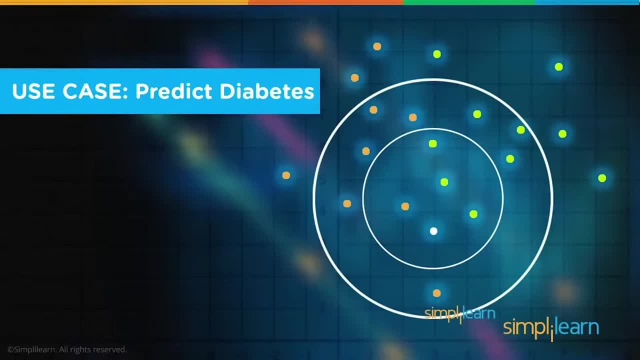 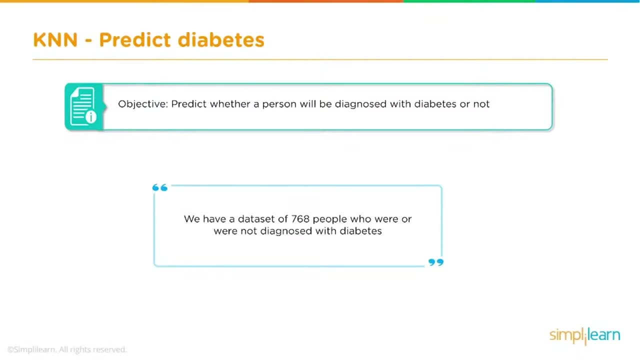 into the predict diabetes use case. So use case: predict diabetes. The objective: predict whether a person will be diagnosed with diabetes or not. There are 168 people who were or were not diagnosed with diabetes And let's go ahead and open that file and just take a look at that data. And this is in a simple spreadsheet. 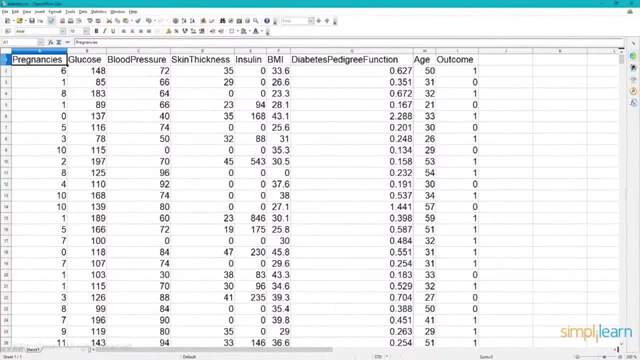 format. The data itself is comma separated, Very common set of data And it's also a very common way to get the data. And you can see here we have columns A through I. That's what: 1, 2,, 3,, 4,, 5,, 6,, 7,, 8.. Eight columns with a particular attribute And then the ninth. 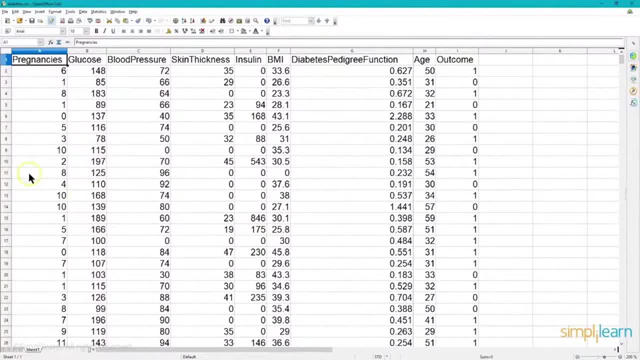 column which is the outcome is whether they have diabetes or not. And then we have the second column: We have diabetes. As a data scientist, the first thing you should be looking at is insulin. Well, you know, if someone has insulin, they have diabetes, because that's. 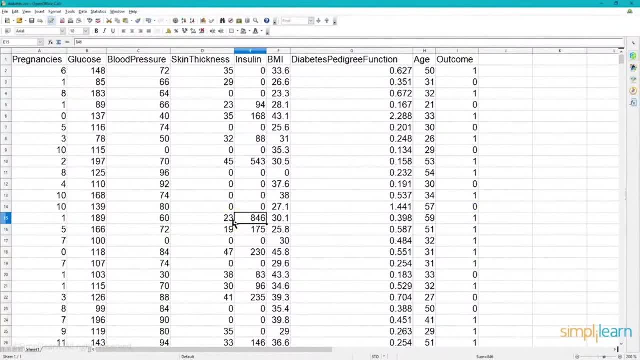 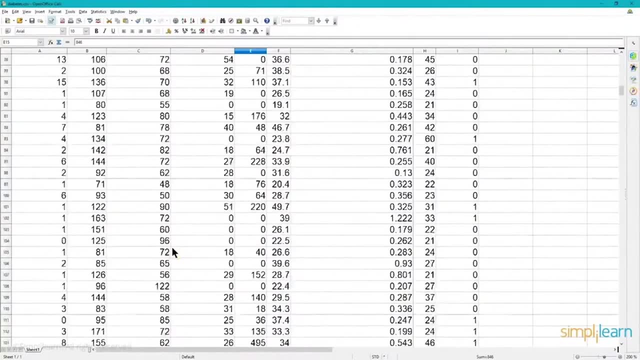 why they're taking it And that could cause issue in some of the machine learning packages, But for a very basic setup this works fine for doing the KNN And the next thing you notice is it didn't take very much to open it up. I can scroll down to the bottom of 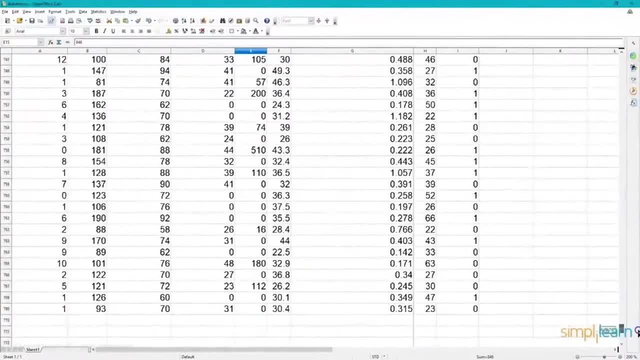 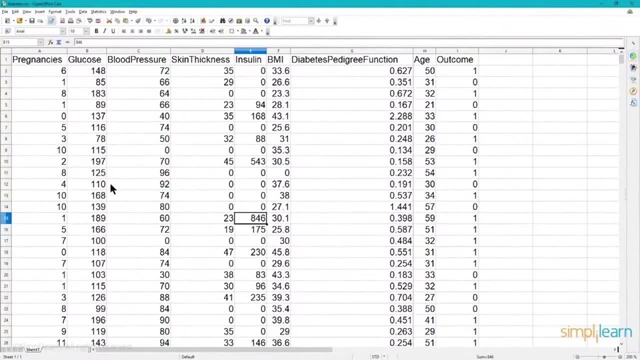 the data There's 768.. It's pretty much a small data set, You know, at 769, I can easily fit this into my RAM on my computer. I can look at it, I can manipulate it And it's not going to really tax, just a regular. 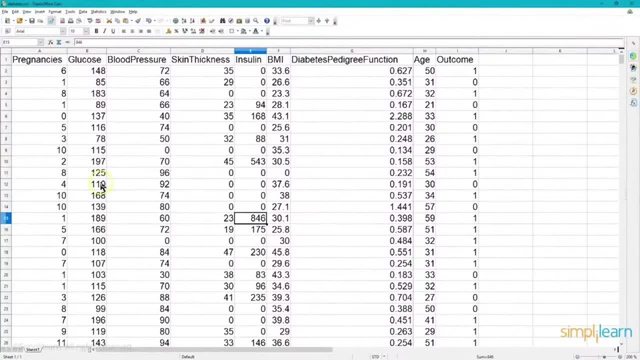 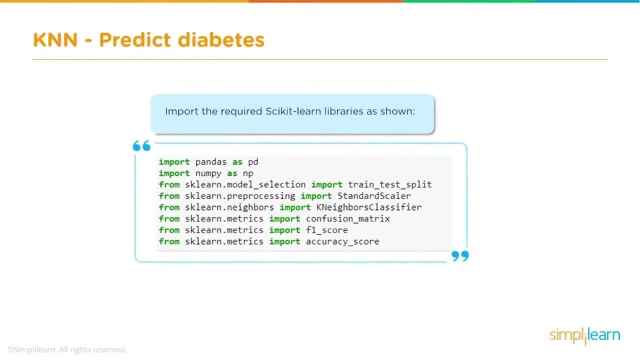 desktop computer. You don't even need an enterprise version to run a lot of this. So let's start with importing all the tools we need, And before that, of course, we need to discuss what IDE I'm using. Certainly, you can use any particular editor for Python. 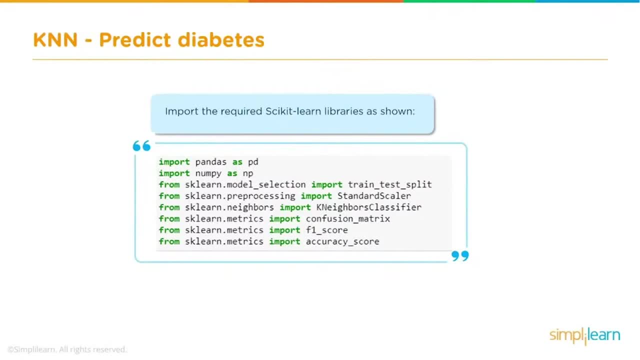 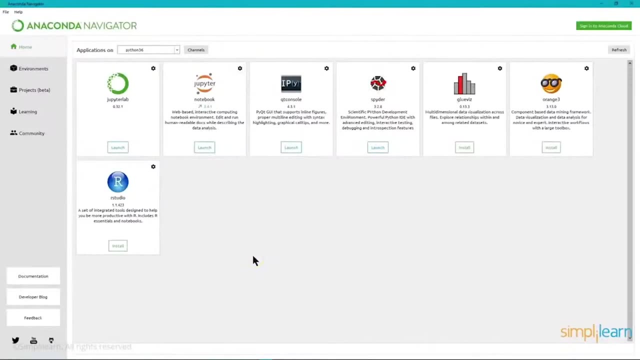 But I like to use for doing very basic visual stuff, the Anaconda, which is great for doing demos with the Jupyter Notebook, And just a quick view of the Anaconda Navigator, which is the new release. You can see under Home. I can choose my application. We're going to be using Python 3.6.. I have 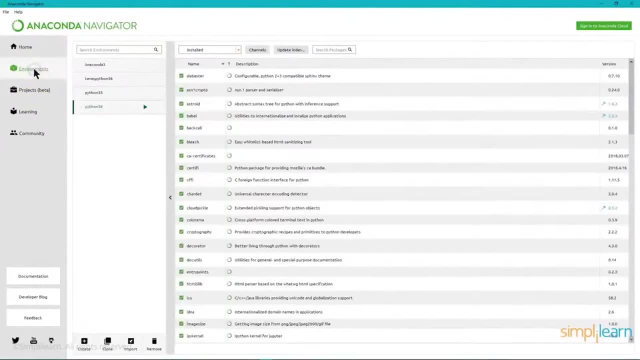 a couple of different versions on this particular machine. If I go under Environments, I can create a unique environment for each one, which is nice, And there's even a little button there where I can install different packages. So if I click on that button and open the, 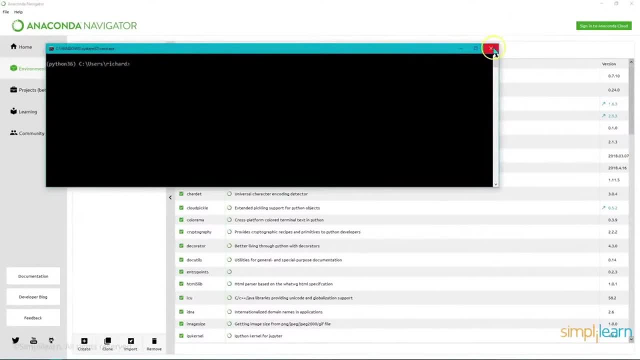 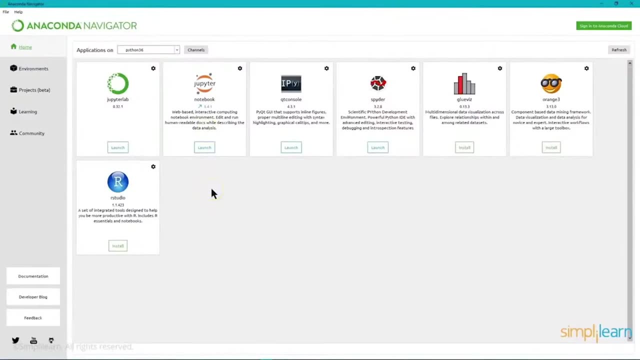 terminal. I can then use a simple pip install to install different packages I'm working with. Let's go ahead and go back under Home And we're going to launch our notebook And I've already- you know, kind of like the old cooking shows- I've already got my notebook And I'm 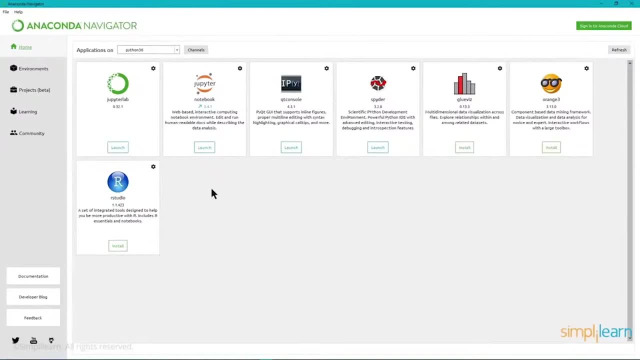 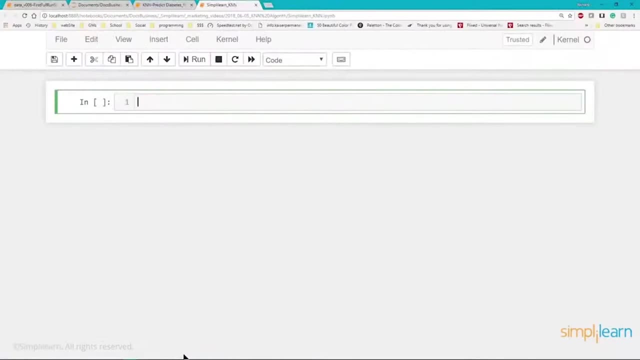 already prepared a lot of my stuff, so we don't have to wait for it to launch, because it takes a few minutes for it to open up a browser window. In this case, I'm going to. it's going to open up Chrome because that's my default that I use, And since the script 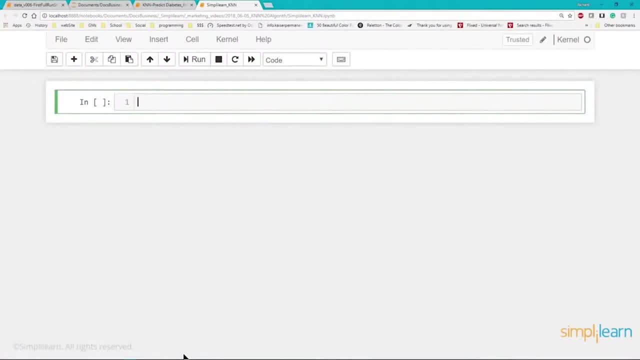 is pre-done. you'll see I have a number of windows open up at the top, The one we're working in, And since we're working on the KNN Predict whether a person will have diabetes or not, let's go ahead and put that title in there, And I'm also going to go up here. 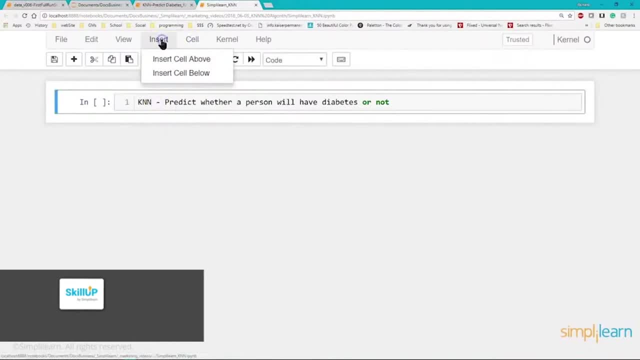 and click on cell. Actually, we want to go ahead and first insert a cell below And then I'm going to go back up to get a second one, And then that's the first one, And once we've got that, we're going to go ahead and go back down And I'm actually going to go into the. 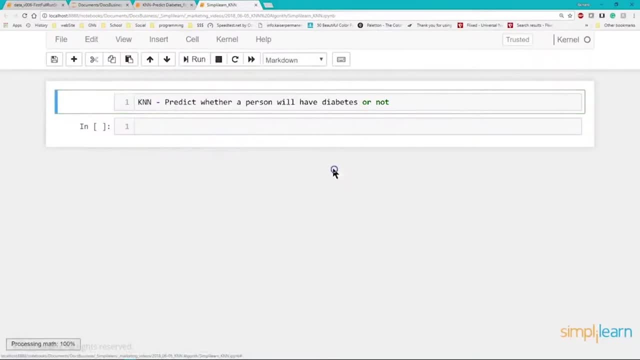 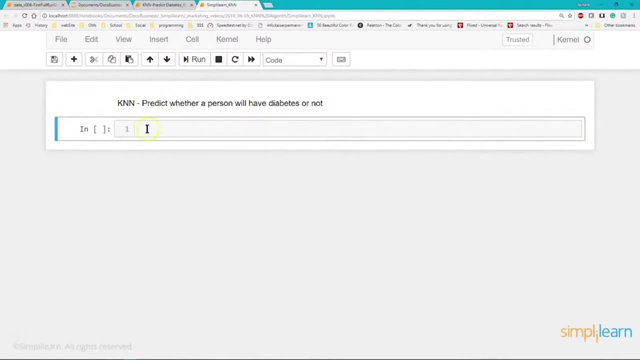 to the top cell and I'm going to change the cell type to markdown. That means this is not going to run as Python It's a markdown language, So if I run this first one it comes up in nice big letters, which is kind of nice. Reminds us what we're working. 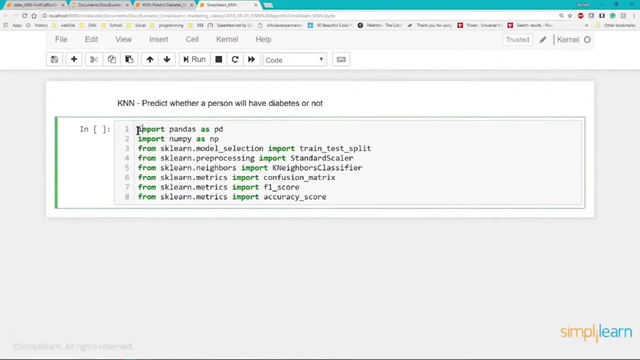 on And by now you should be familiar with doing all of our imports. We're going to import the pandas as pd import, numpy as np. Pandas is the pandas data frame and numpy is the number array- Very powerful tools to use in here. So we have our 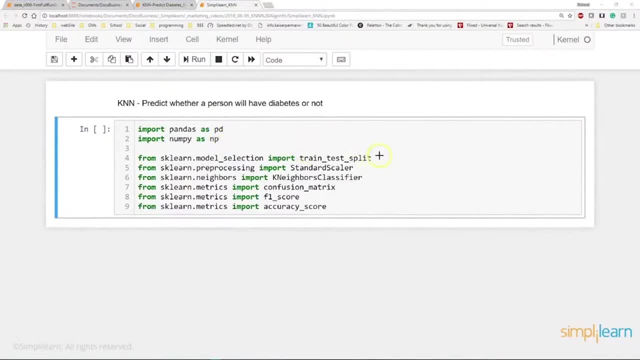 imports. So we've brought in our pandas, our numpy, our two general Python tools, And then you can see over here we have our train test split. By now you should be familiar with splitting the data. We want to split part of it for training our thing and then training our particular model. 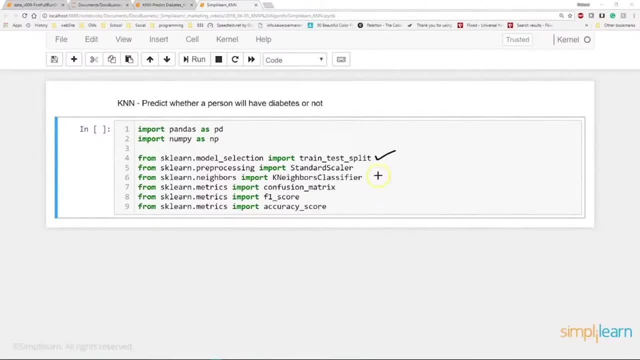 And then we want to go ahead and test the remaining data to see how good it is Pre-processing a standard scalar pre-processor so we don't have a bias of really large numbers. Remember, in the data we had like number pregnancies. 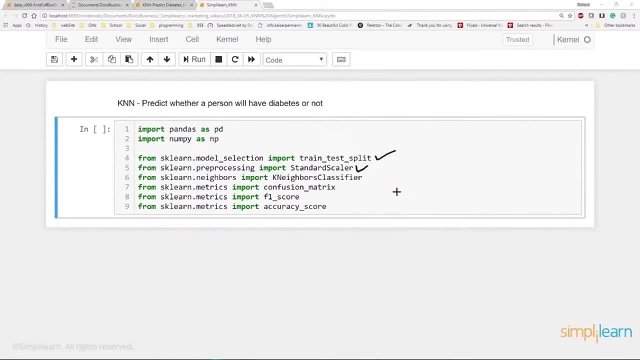 isn't going to get very large, Where the amount of insulin they take can get up to 256.. So 256 versus 6, that will skew results. So we want to go ahead and change that so that they're all uniform between minus 1 and 1.. And then the actual. 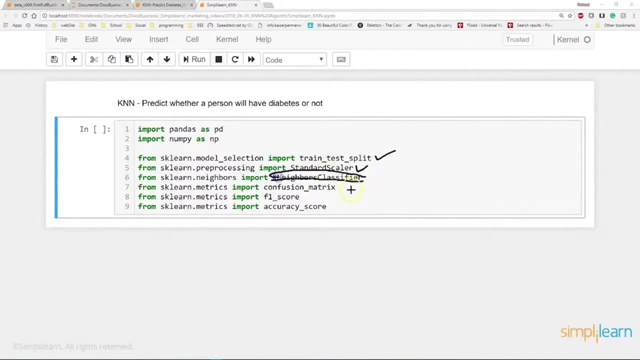 tool. This is the k-neighbors classifier we're going to use. And finally, the last three are three tools to test. All about testing our model. How good is it? Let me just put down test on there. And we have our confusion matrix, our F1 score and our accuracy. 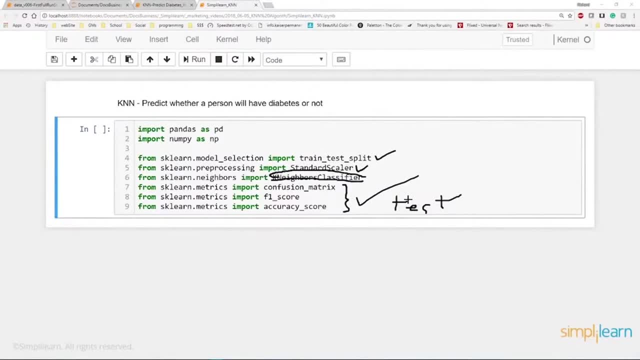 So we have our two general Python modules we're importing, And then we have our six modules specific from the sklearn setup, And then we do need to go ahead and run this. So these are actually imported. There we go, And then move on to the next step, And so in this, 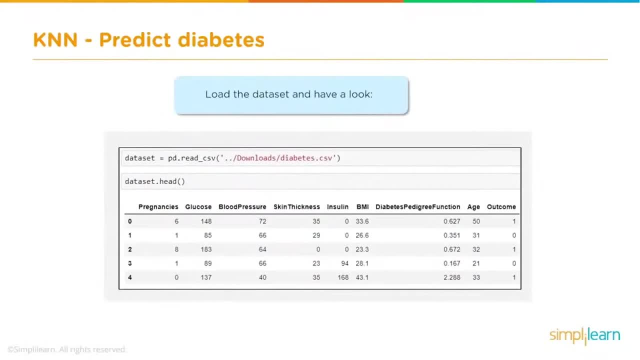 set. we're going to go ahead and load the database. We're going to use pandas. Remember, pandas is pd And we'll take a look at the data in Python. We looked at it in a simple spreadsheet, But usually I like to also pull it up so that we can. 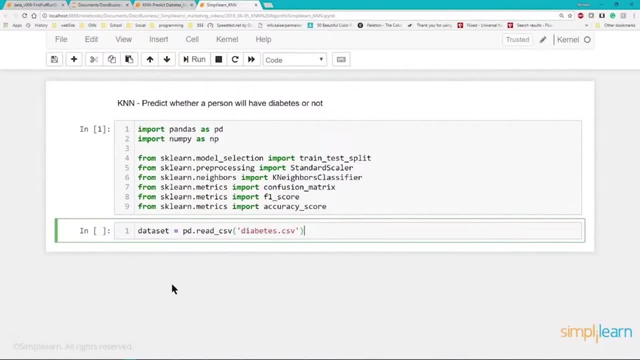 see what we're doing. So here's our data set equals pdreadcsv. That's a pandas command And the diabetes folder I just put in the same folder where my IPython script is. If you put it in a different folder you'd need. 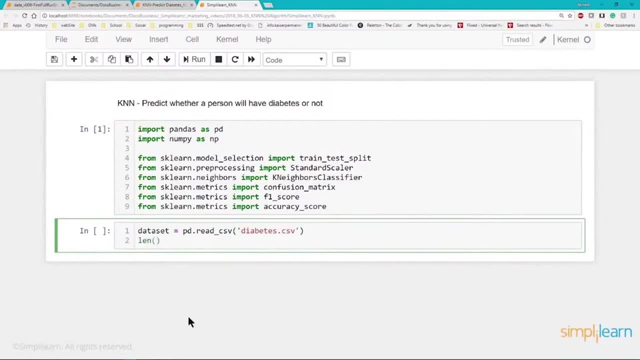 the full length on there. We can also do a quick length of the data set. That is a simple Python command, L-E-N for length. We might even let's go ahead and print that We'll go print. And if you do it on its own line, lengthdataset in the 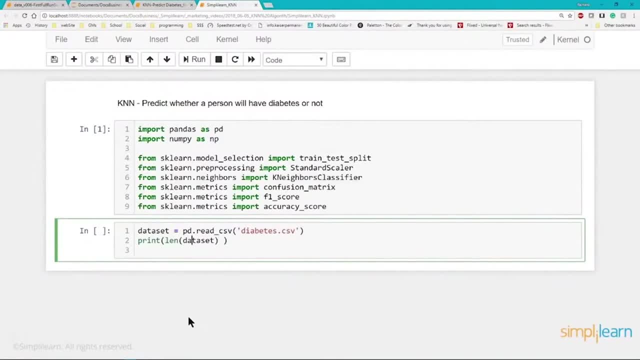 Jupyter notebook, it'll automatically print it. But when you're in most of your different setups, you want to do the print in front of there And then when you want to take a look at the actual data set- and since we're in pandas, we can. 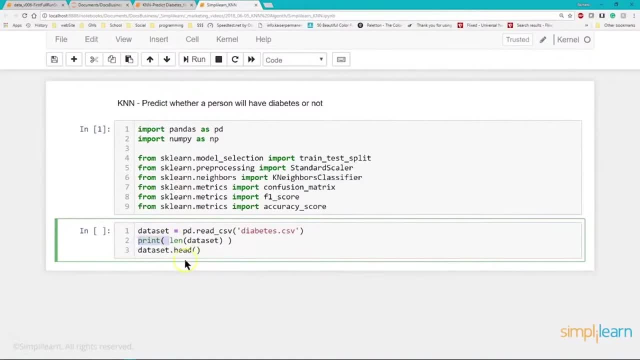 simply do data set head And again. let's go ahead and add the print in there. If you put a bunch of these in a row, you know the data set one head, data set two head. it only prints out the last one. So I usually always like to keep the print. 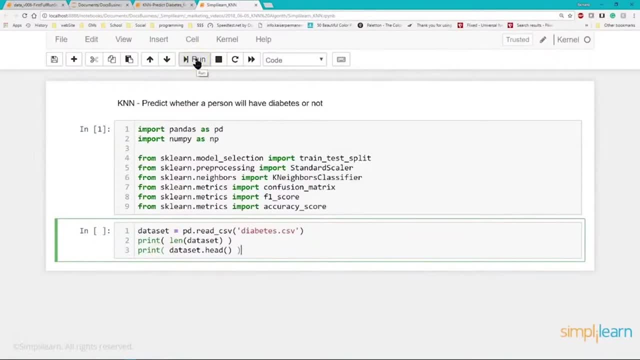 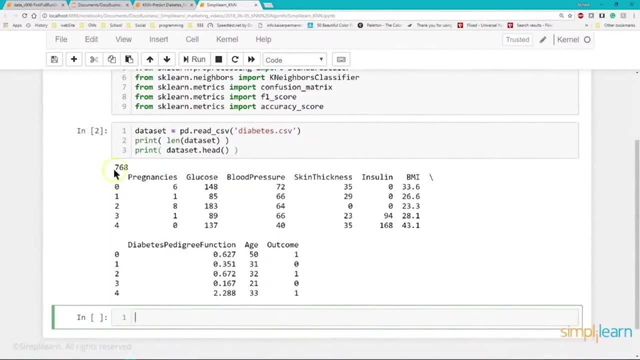 statement in there. But because most projects only use one data frame- pandas data frame- doing it this way doesn't really matter. The other way works just fine And you can see when we hit the run button we have the 768 lines which we've. 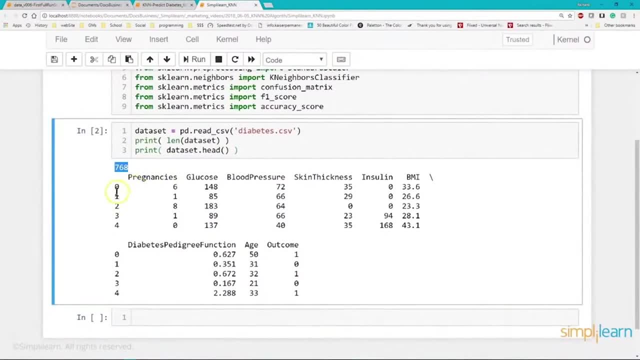 268 lines, which we knew, and we have our pregnancies. it's automatically given a label on the left. remember, the head only shows the first five lines, so we have zero through four and just a quick look at the data you can see it matches what we looked at before we have pregnancy: glucose blood pressure. 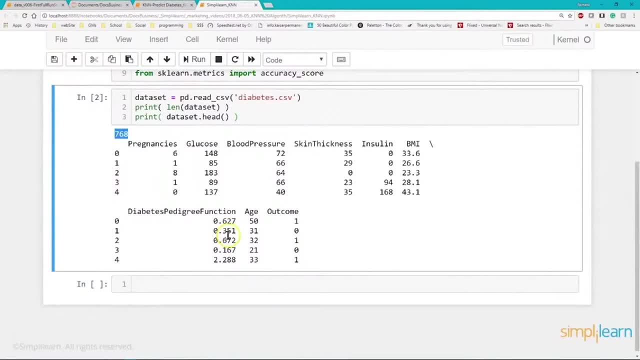 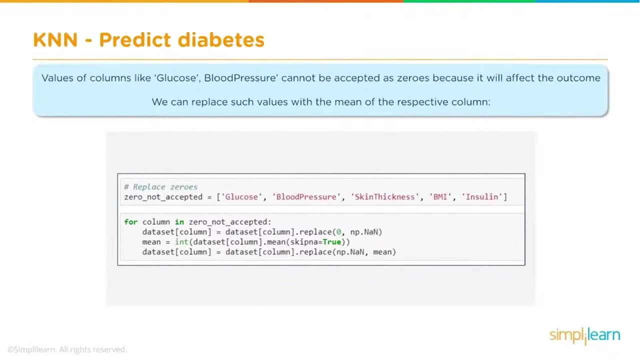 all the way to age, and then the outcome on the end, and we're going to do a couple things in this next step. we're going to create a list of columns where we can't have zero. there's no such thing as zero skin thickness or zero blood pressure, zero glucose- any of those, you'd be dead. so not a really. 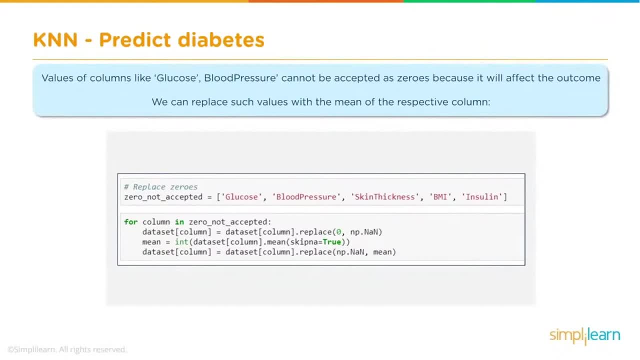 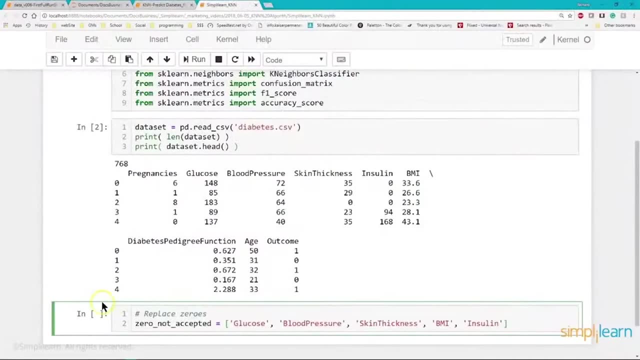 good factor if they don't, if they have a zero in there because they didn't have the data, and we'll take a look at that because we're going to start replacing that information with a couple of different things and let's see what that looks like. so first we create a nice list, as you can. 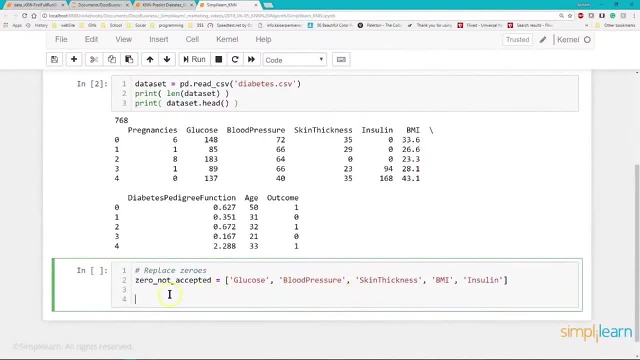 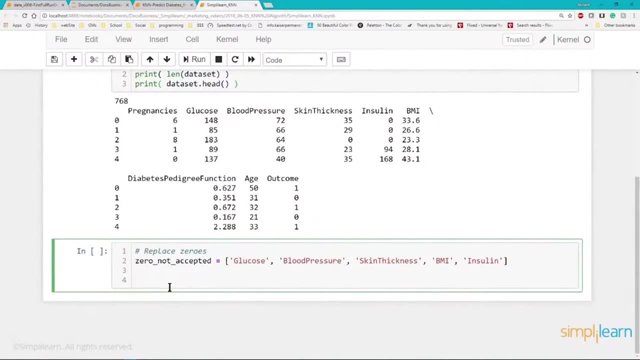 see, we have the values talked about: glucose, blood pressure, skin thickness, and this is a nice way when you're working with columns is to list the columns you need to do some kind of transformation on very common thing to do and then for this particular setup, we certainly could use the there's some. 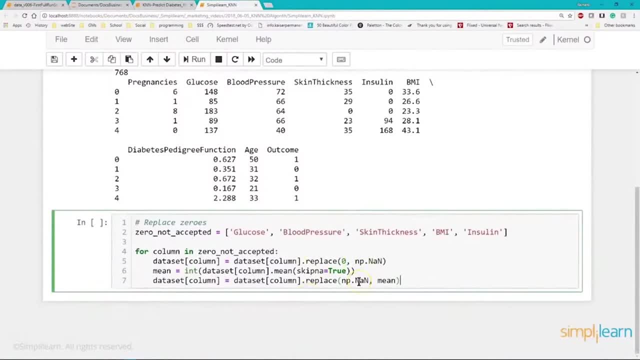 panda tools that will do a lot of this, where we can replace the NA, but we're going to go ahead and do it as a data set column equals data set column dot. replace this is- this is still pandas. you can do a direct. there's also one that's that you look for your NAN. a lot of different options. 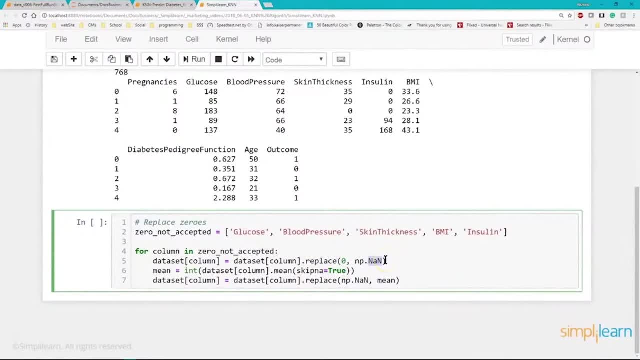 in here, but the NAN- numpy- NAN is what that stands for is- is none. it doesn't exist. so the first thing that's going to be doing is going to be replacing the zero with a numpy none. there's no data there. that's what that says. that's what this is saying right here. so put the zero in and we're going to. 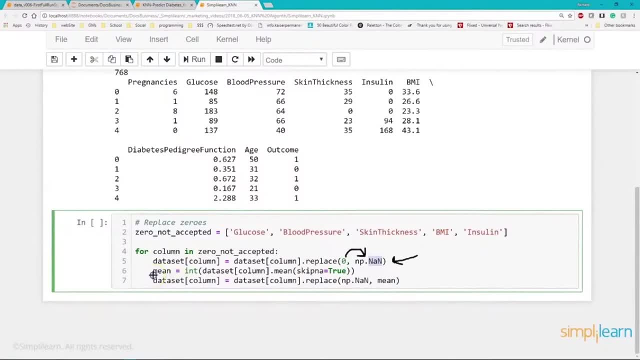 play zeroes with no data. so if it's a zero, that means a person's well, hopefully not dead. well, they just didn't get the data. the next thing they want to do is we're going to create the mean, which is the integer from the data set, from the column dot mean, where we skip in A's. we can do that is a. 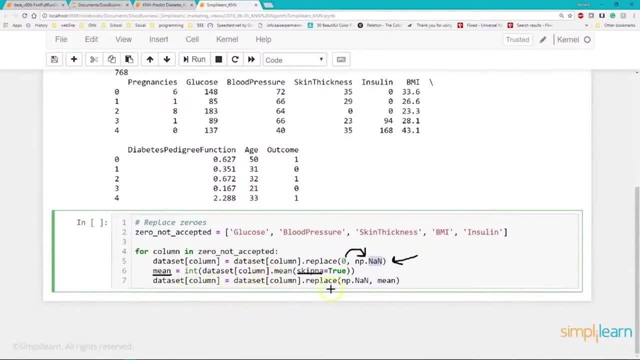 And then we're going to take that dataset column and we're going to replace all the NPNAN with the means. Why did we do that? We could have actually just taken this step and gone right down here and just replaced zero and skipped anything where except you could actually there's a way to skip zeros. 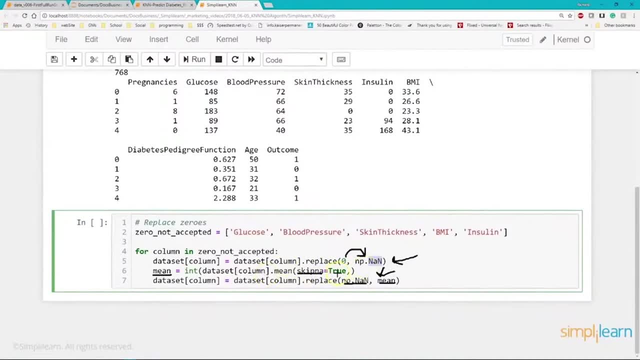 and then just replace all the zeros. But in this case, we want to go ahead and do it this way, so you can see that we're switching this to a non-existent value and we're going to create the mean. Well, this is the average person. 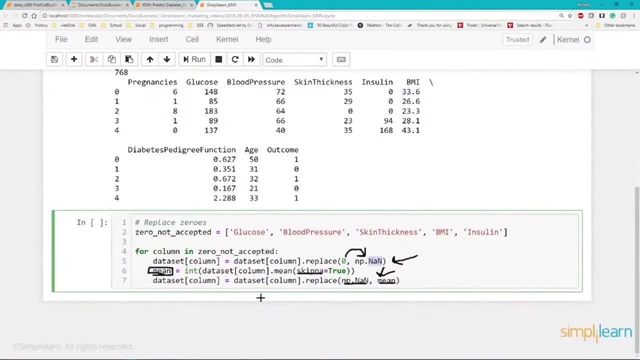 So if we don't know what it is, if they did not get the data and the data's missing, one of the tricks is you replace it with the average, What is the most common data for that. This way you can still use the rest of those values to do your computation, and it kind. 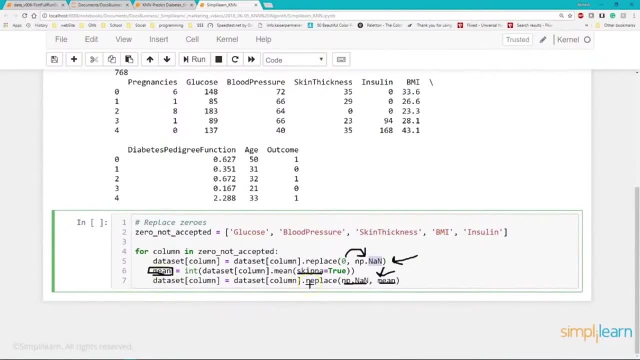 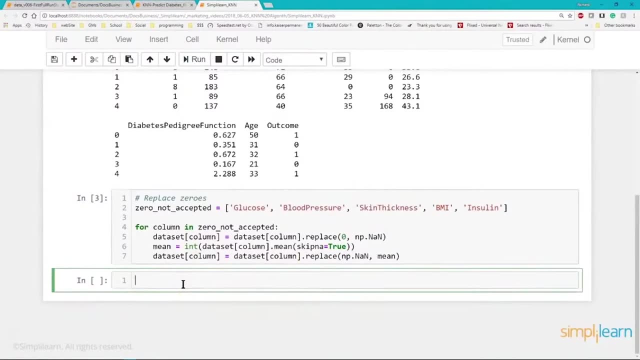 of just brings that particular value, those missing values, out of the equation. Let's go ahead and take this and we'll go ahead and run it. It doesn't actually do anything, so we're still preparing our data. If you wanted to see what that looks like, we don't have anything in the first few lines. 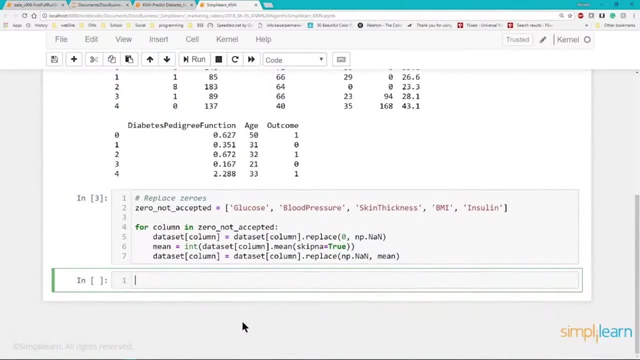 so it's not going to show up, But we certainly could look at a row. Let's do that. Let's go into our data set, let's print a data set And let's pick. in this case, let's just do glucose. 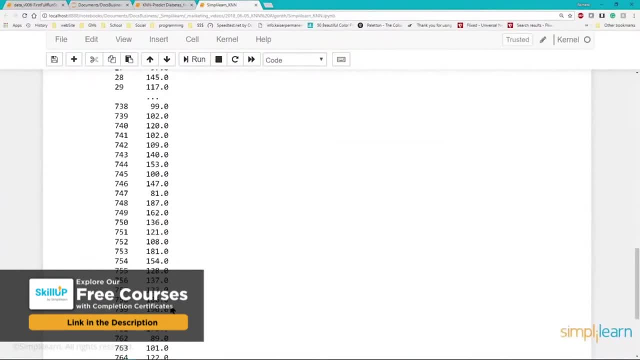 And if I run this, this is going to print all the different glucose levels going down And we thankfully don't see anything in here that looks like missing data. at least on the ones it shows You can see it skipped a bunch in the middle. 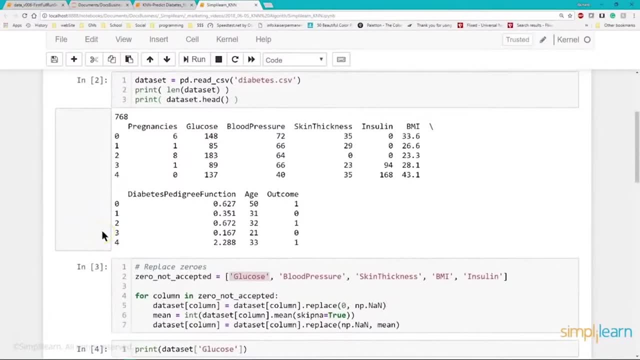 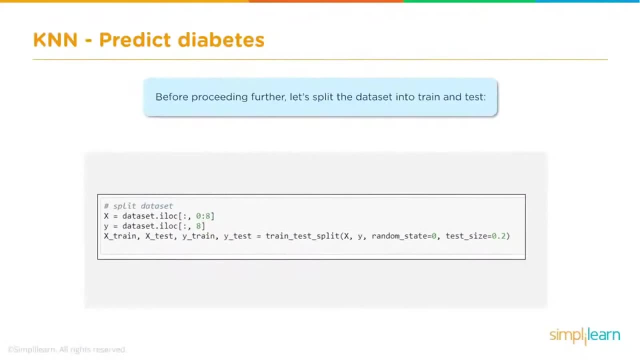 That's what it does. If you have too many lines in Jupyter Notebook, it'll skip a few and go on to the next in a data set. Let me go ahead and remove this And we'll just zero out that. And, of course, before we do any processing, before proceeding any further, we need to 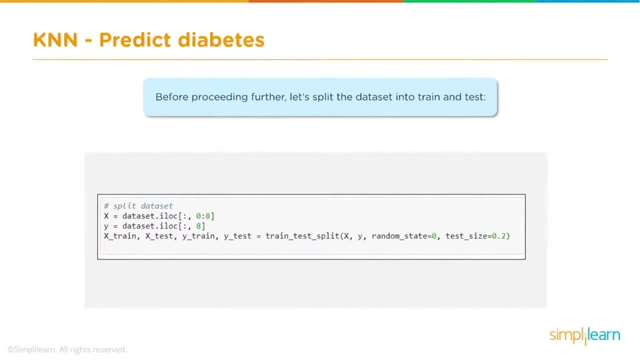 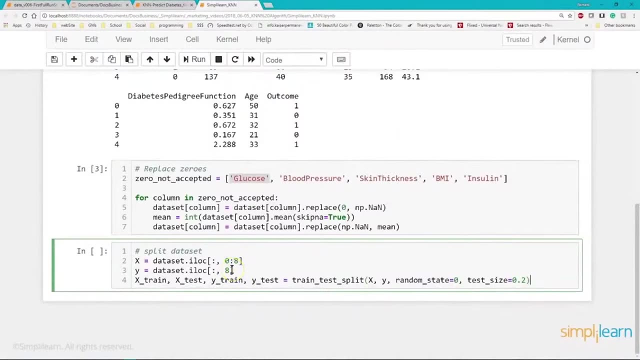 split the data set into our train and testing data. That way we have something to train it with and something to test it on. And you're going to notice we did a little something here with the Pandas database code. There we go, my drawing tool. 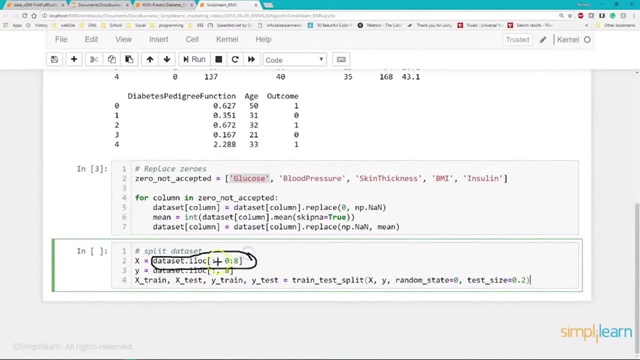 We've added in this right here off the data set, And what this says is that the first one in Pandas- this is from the PD Pandas- it's going to say, within the data set, We want to look at the I location and it is all rows. 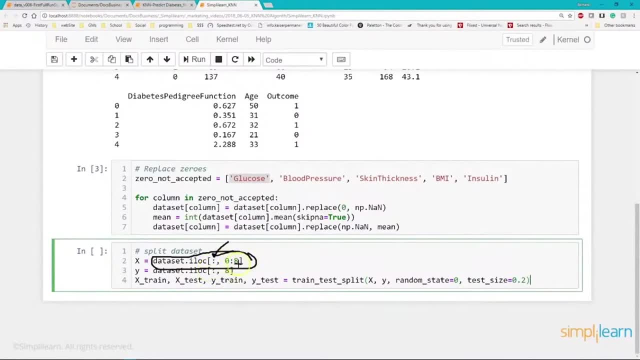 That's what that says. So we're going to keep all the rows, But we're only looking at zero, column zero to eight. Remember column nine? here it is, right up here, we printed it in. here is outcome. Well, that's not part of the training data. 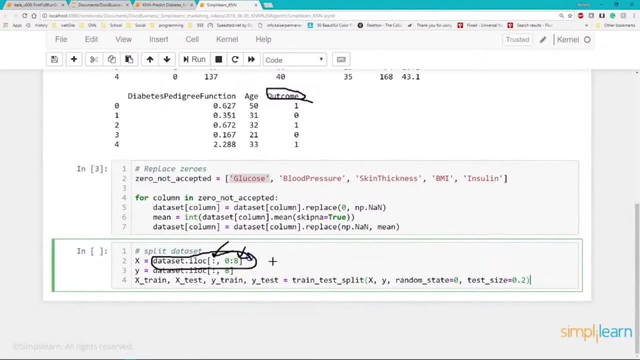 That's part of the answer. Yeah, it's column nine, but it's listed as eight number eight. So zero to eight is nine columns. So eight is the value And when you see it in here, zero. this is actually zero to seven. 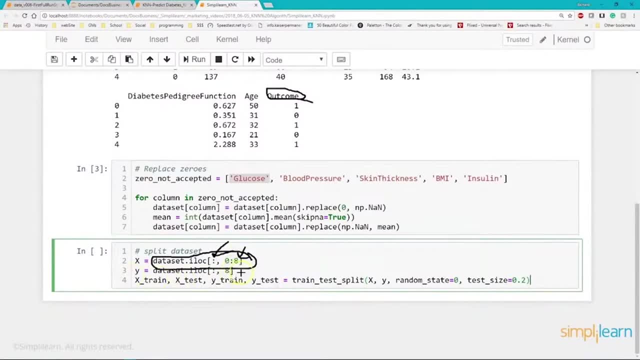 It doesn't include the last one. And then we go down here to Y, which is our answer, And we want just the last one, Just column eight, And you can do it this way with this particular notation. And then, if you remember, we imported the train test split. 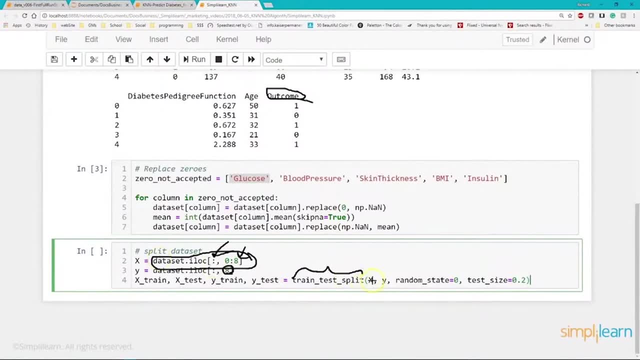 That's part of the sklearn right there And we simply put in our X and our Y. We're going to do random state equals zero. You don't have to necessarily seed it. That's a seed number. I think the default is one when you seed it. 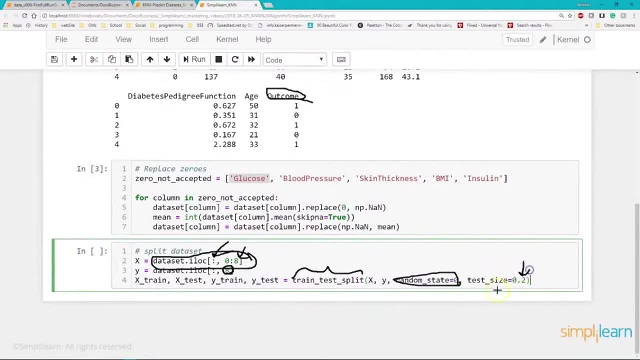 I'd have to look that up. And then the test size. Test size is 0.2.. That simply means we're going to take 20% of the data and put it aside so that we can test it later. That's all that is. 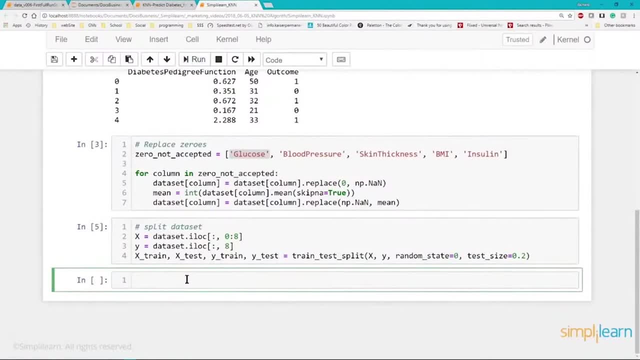 And again, we're going to run it. Not very exciting. So far we haven't had any printout other than to look at the data. But that is a lot of. this is prepping this data. Once you prep it, the actual lines of code are quick and easy. 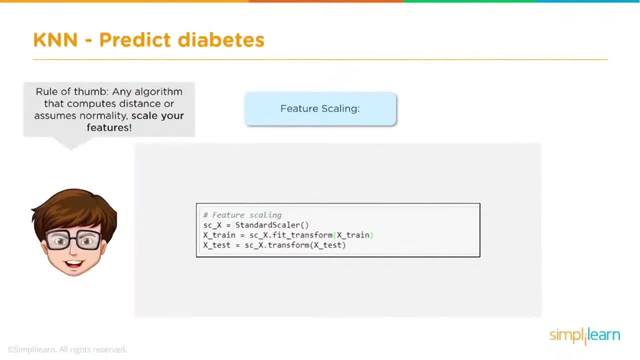 And we're almost there, But the actual running of our KNN. we need to go ahead and do a scale the data. If you remember correctly, we're fitting the data in a standard scaler, which means, instead of the data being from, you know, five to 303 in one column, and the next column is one. 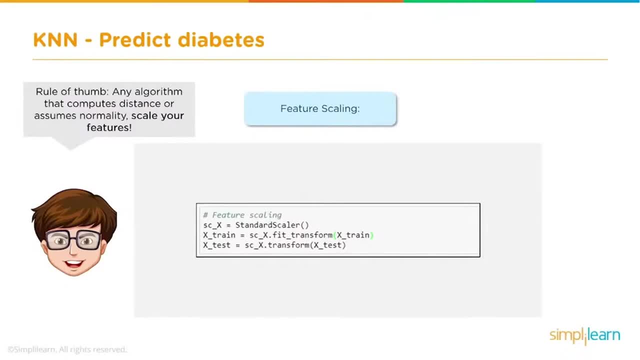 to six. We're going to set that all so that all the data is between minus one and one. That's what that standard scaler does, Keeps it standardized, And we only want to fit the scaler with the training set. But we want to make sure the testing set is the X test going in is also transformed. 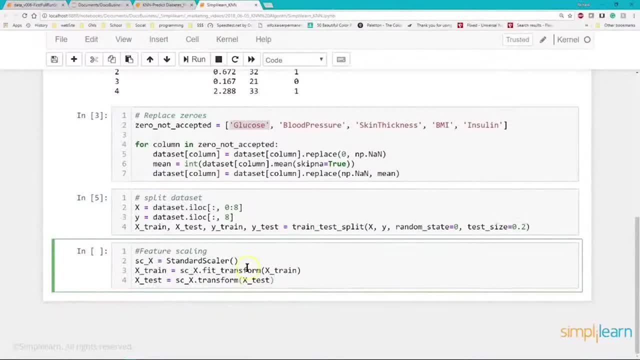 So it's processing it the same. So here we go with our standard scaler. We're going to call it SC underscore X for the scaler And we're going to import the standard scaler into this variable, And then our X train equals SC underscore X. 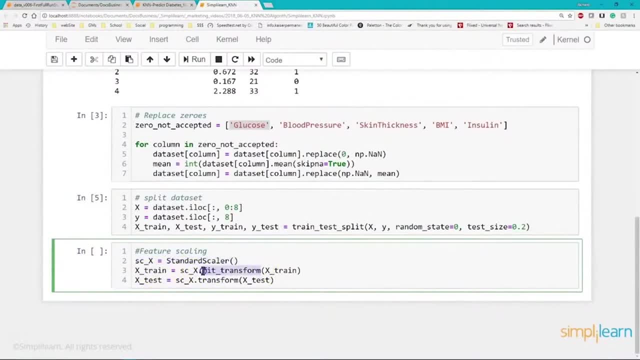 Okay, SC underscore X, dot fit, transform. So we're creating the scaler on the X train variable And then our X test. we're also going to transform it. So we've trained and transformed the X train and then the X test isn't part of that training. 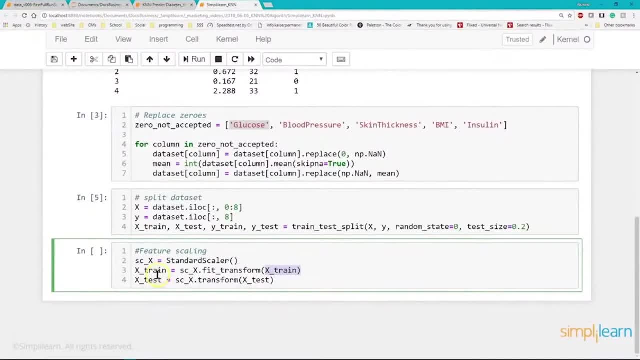 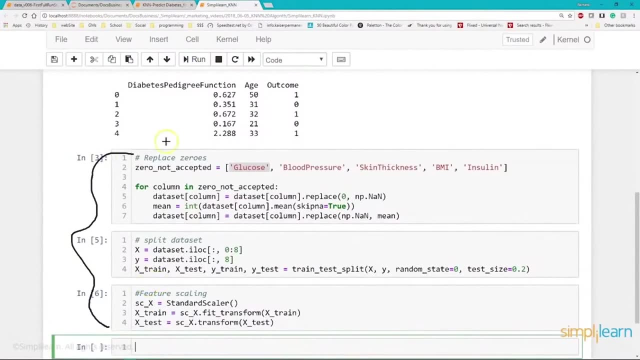 It isn't part of training the transformer. It just gets transformed. That's all it does. And again, we're going to go and run this. If you look at this, we've now gone through these steps, all three of them. 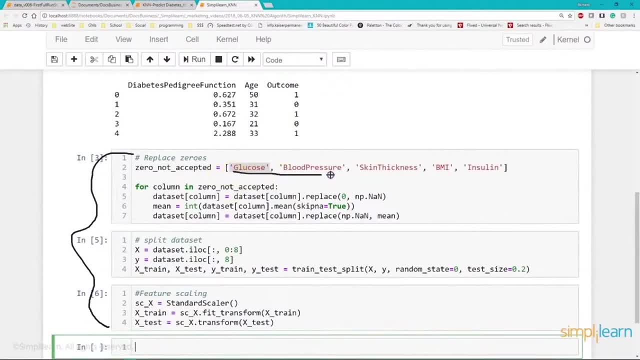 We've taken care of replacing our zeros for key columns. That shouldn't be zero And we've replaced that with the means of those columns, That way that they fit right in with our data models. We've come down here and we've split the data. 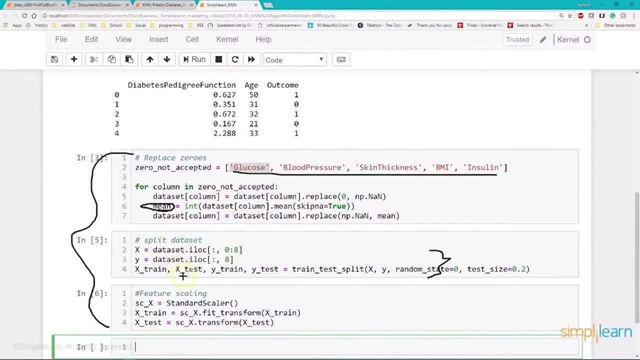 So now we have our test data and our training data And then we've taken and we've scaled the data, So all of our data going in Now. no, we don't train the Y part, The Y train and Y test. 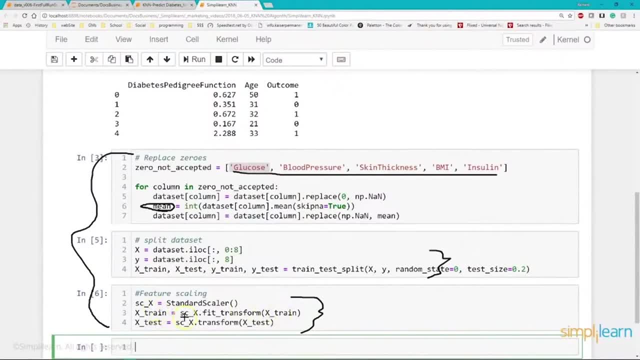 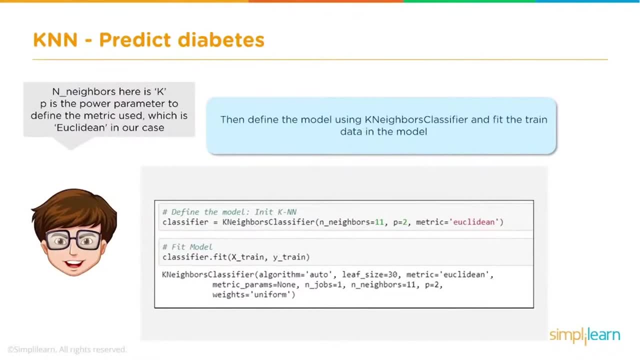 That never has to be trained, It's only the data going in. That's what we want to train in there. Then define the model using KNU, K, neighbors, classifier and fit the train data in the model. So we do all that data prep and you can see down here we're only going to have a couple. 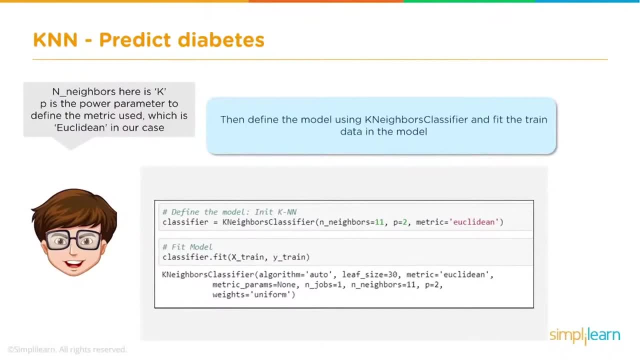 lines of code where we're actually building our model and training it. That's one of the cool things about Python and how far we've come. It's such an exciting time to be in machine learning because there's so many automated tools. Let's see. 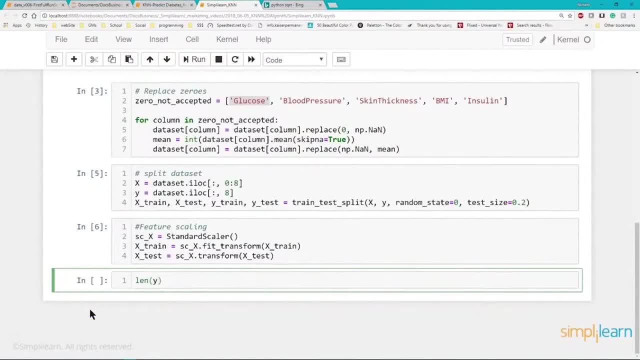 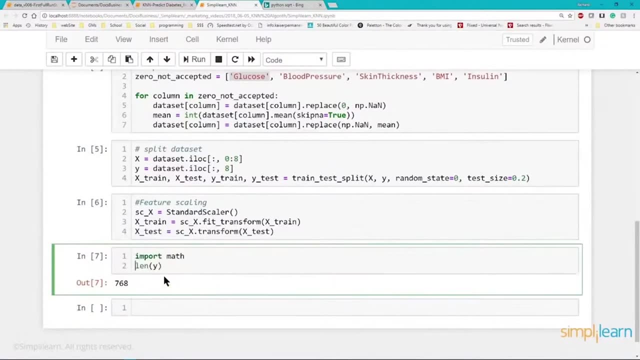 Before we do this, let's do a quick length of, and let's do Y. We want. let's just do length of Y and we get 768.. And if we import, We do math dot square root. Let's do Y train. 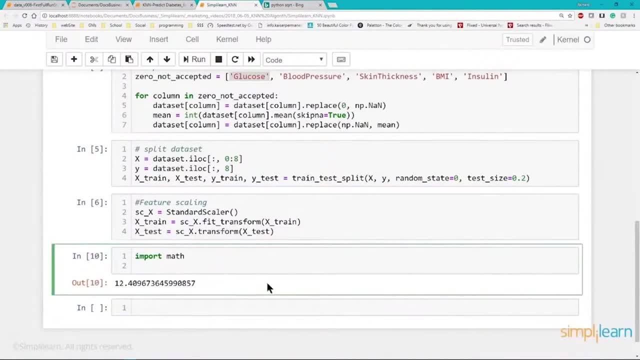 There we go. It's actually supposed to be X train. Before we do this, let's go ahead and do import math and do math square root length of Y test And when I run that, we get 12.409.. I want to show you where this number comes from. we're about to use 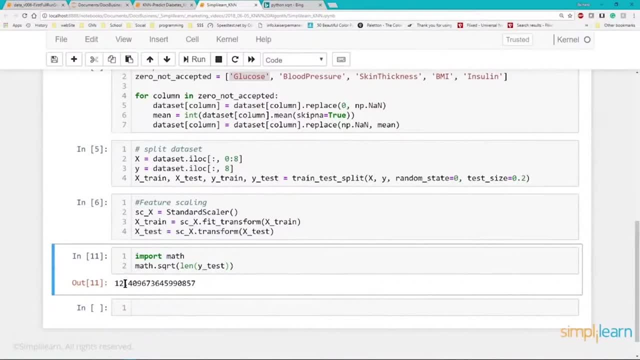 Twelve is an even number, So if you know, if you're ever voting on things, remember the neighbors all vote. Don't want to have an even number of neighbors voting, So we want to do something odd and let's just take one away. 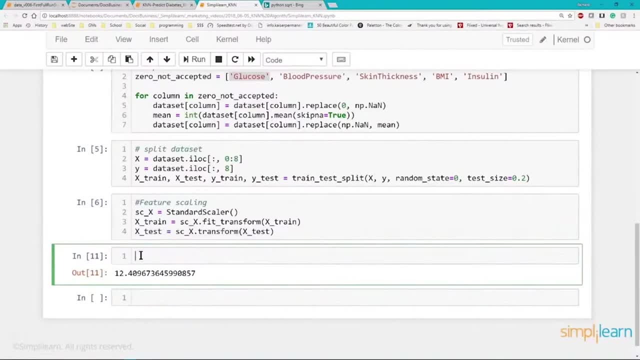 We'll make it 11.. Let me delete this out of here. That's one of the reasons I love Jupyter Notebook: because you can flip around and do all kinds of things on the fly. So we'll go ahead and put in our classifier. 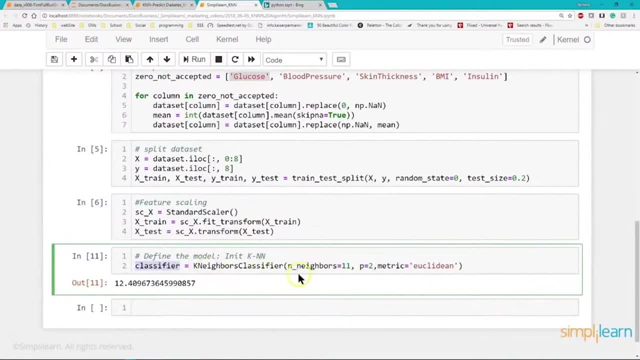 We're creating our classifier now and it's going to be the K neighbors classifier. N neighbors equal 11.. Remember we did 12 minus one for 11.. So we have an odd number of neighbors. P equals two, because we're looking for is it: are they diabetic or not? 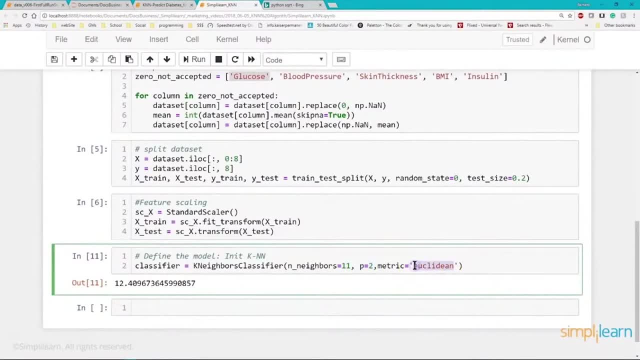 And we're using the Euclidean metric. There are other means of measuring The distance. you could do like square. square means values, all kinds of measure this, but the Euclidean is the most common one and it works quite well. It's important to evaluate the model. 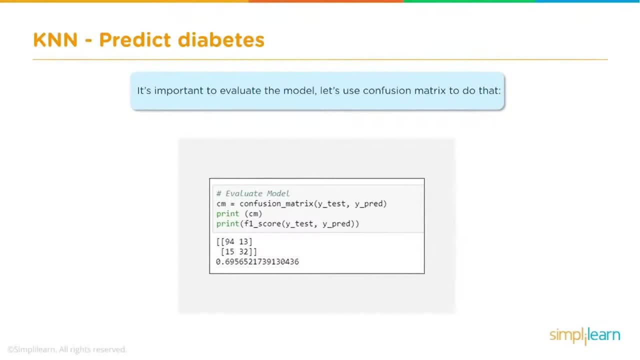 Let's use the confusion matrix to do that, and we're going to use the confusion matrix, Wonderful tool. And then we'll jump into the F1 score and finally, accuracy score, which is probably the most commonly used quoted number when you go into a meeting or something like that. 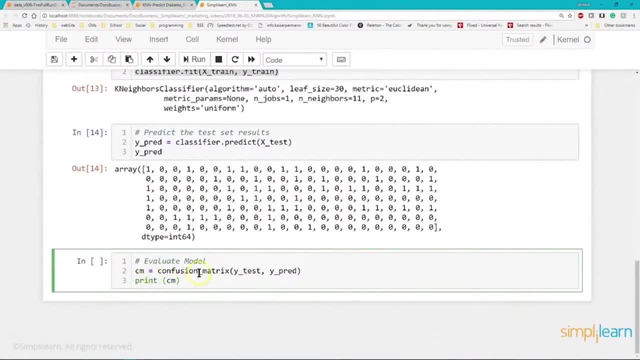 So let's go ahead and paste that in there And we'll set the CM equals one, Okay, And then we'll set the F1 score and finally, accuracy score: Okay, And then we'll set the CM equals one, Okay, And then we'll set the CM equals two. 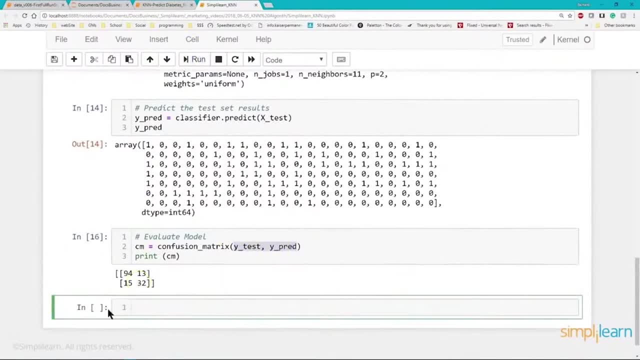 So those are the two values we're going to put in there, And let me go ahead and run that and print it out. The way you interpret this is: you have the Y predicted, which would be your title up here. We could do, let's just do PRED. 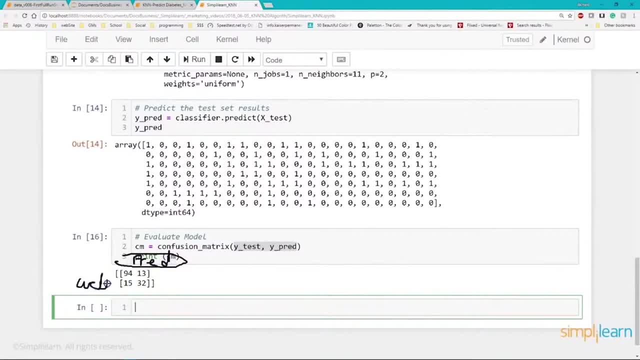 Predicted across the top and actual going down: Actual. It's always hard to write in here. actual That means that this column here down the middle, that's the important column column and it means that our prediction said 94 and prediction in the actual. 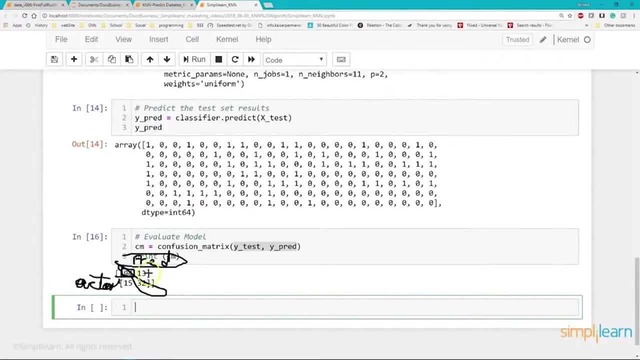 agreed on 94 and 32- this number here, the 13 and the 15. those are what was wrong, so you could have like three different. if you're looking at this across three different variables instead of just two, you'd end up with the third row down. 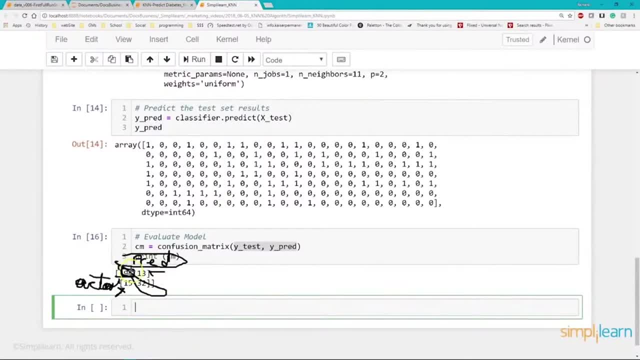 here and that column going down the middle. so in the first case we have the, the and I believe the zero is a 94 people who don't have diabetes. the prediction said to 13 of those people did have diabetes and were at high risk and the 32 that had diabetes it had correct, but our prediction said another. 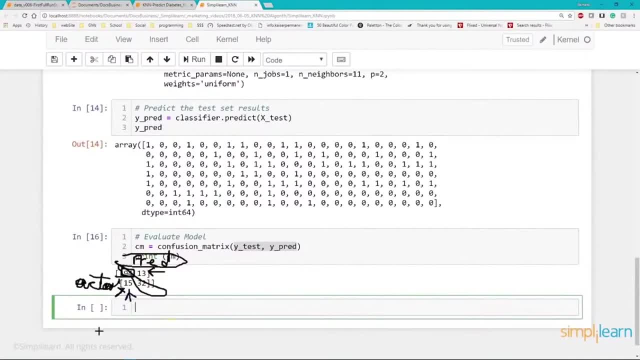 15 out of that 15. it classified as incorrect. so you can see where that classification comes in and how that works on the confusion matrix. then we're going to go ahead and print the f1 score. you just run that and you see we get a. 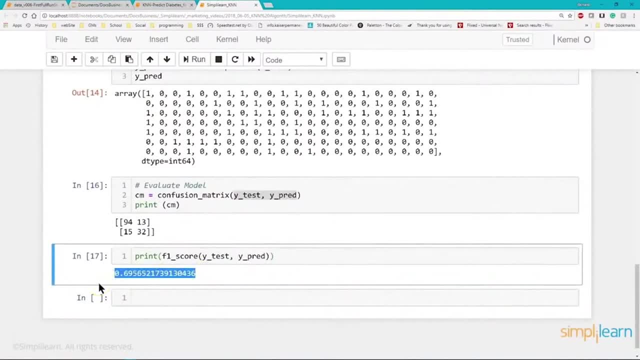 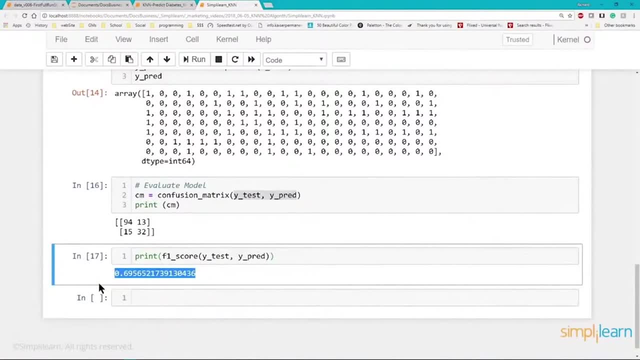 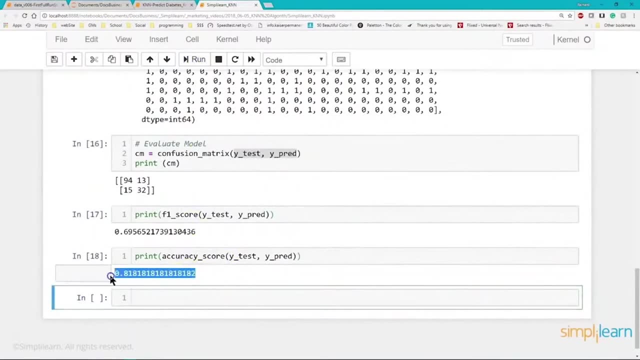 into account both sides of the balance of false positives, where, if we go ahead, just do the accuracy account- and that's what most people think of is- it looks at just how many we got right out of how many we got wrong. so a lot of people, when you're a data scientist and you're talking to other data scientists, they're 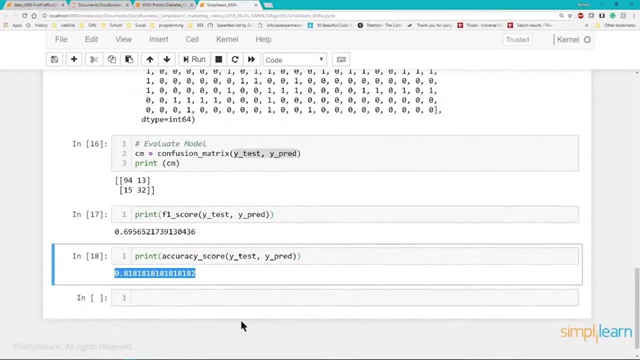 gonna ask you what the f1 score, the F score, is. if you're talking to the general public or the decision makers in the business, they're gonna ask what the accuracy is. and the accuracy is always better than the F1 score, but the F1 score is more telling. lets us know that there's more. 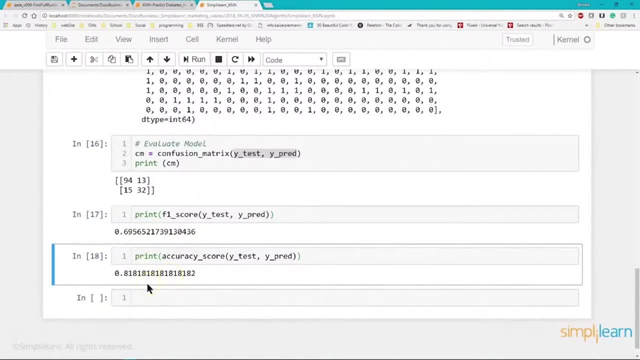 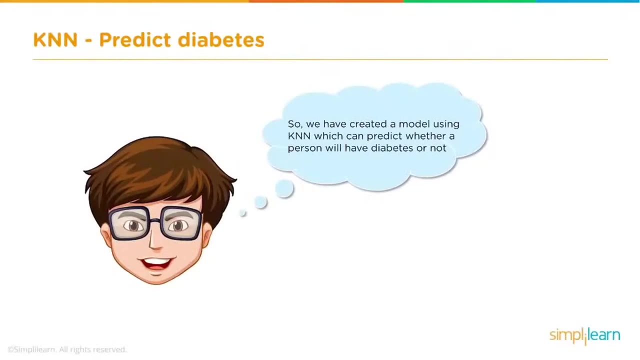 false positives that we would like on here, but 82%, not too bad for a quick flash look at people's different statistics and running an SK learn and running the K and in the K nearest neighbor on it. so we have created a model using KNN which can predict whether a person will have diabetes or 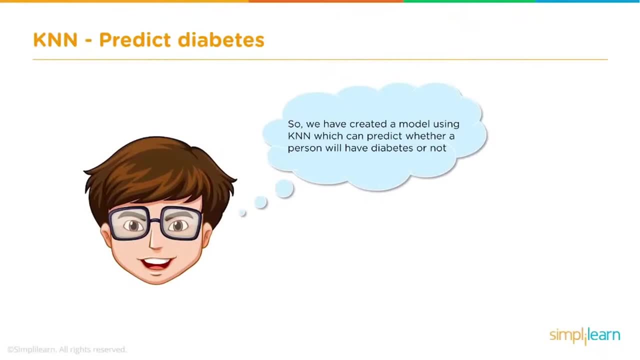 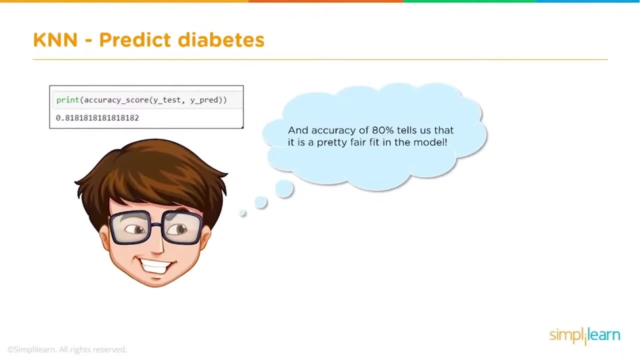 not, or at the very least, whether they should go get a checkup and have their glucose checked regularly or not. the print accuracy score is the same as the. We got the 0.818, which is pretty close to what we got, And we can pretty much round that off and just say we have an accuracy of 80%. 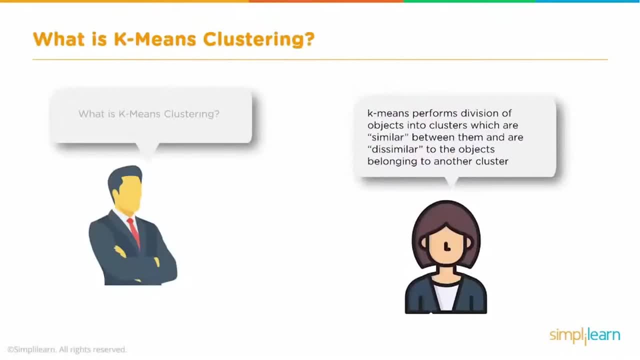 It tells us it is a pretty fair fit in the model. So what is K-means clustering? K-means clustering is an unsupervised learning algorithm. In this case you don't have labeled data, unlike in supervised learning. So you have a set of data and you want to group them. 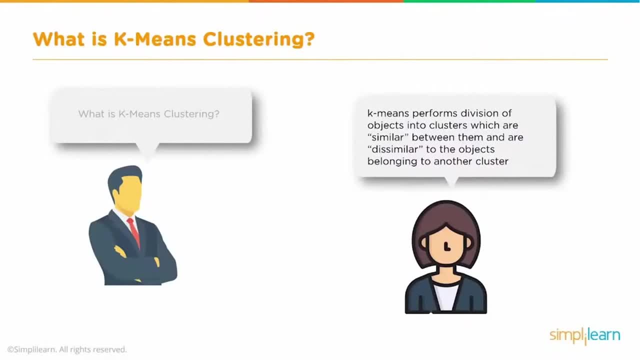 And, as the name suggests, you want to put them into clusters, which means objects that are similar in nature, similar in characteristics, need to be put together. So that's what K-means- clustering- is all about. The term K, basically, is a number. 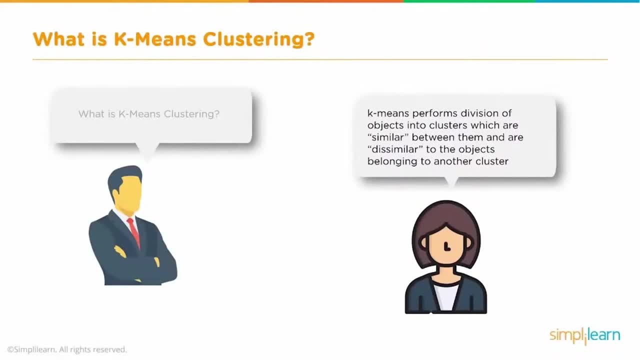 So we need to tell the system how many clusters we need to perform. So if K is equal to 2, there will be 2 clusters, If K is equal to 3, 3 clusters, and so on and so forth. That's what the K stands for. 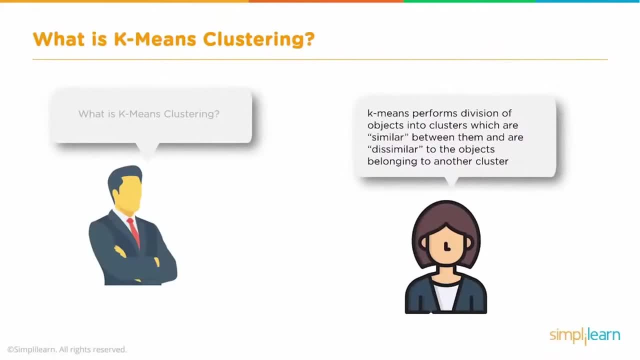 And, of course, there is a way of finding it: Finding out what is the best or optimum value of K for a given data. We will look at that. So that is K-means clustering. So let's take an example. K-means clustering is used in many, many scenarios. 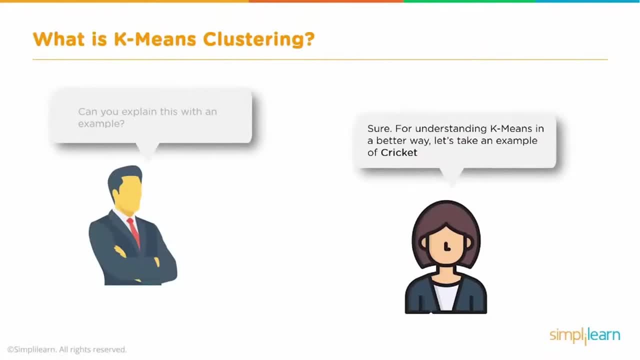 But let's take an example of cricket, the game of cricket. Let's say, you received data of a lot of players from maybe all over the country or all over the world, And this data has information about the runs scored By the people or by the player and the wickets taken by the player. 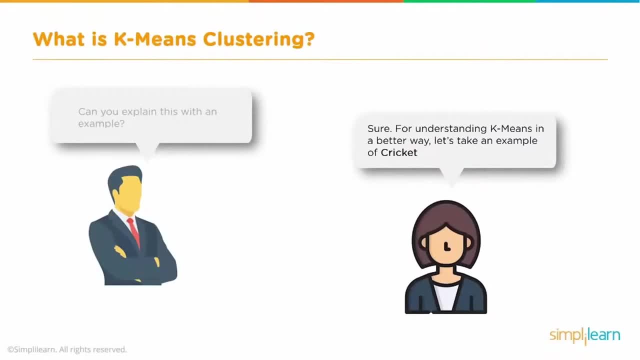 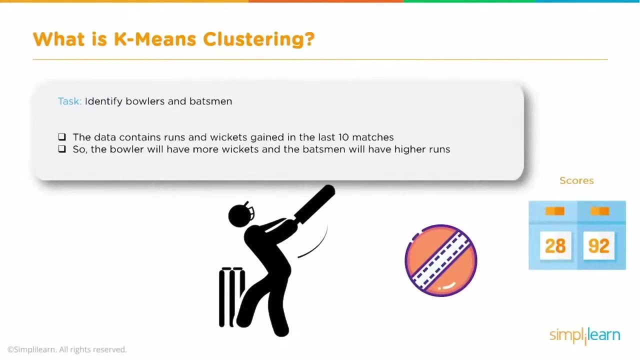 And, based on this information, we need to cluster this data into two clusters: batsmen and bowlers. So this is an interesting example. Let's see how we can perform this. So we have the data, which consists of primarily two characteristics, which is the runs and the wickets. 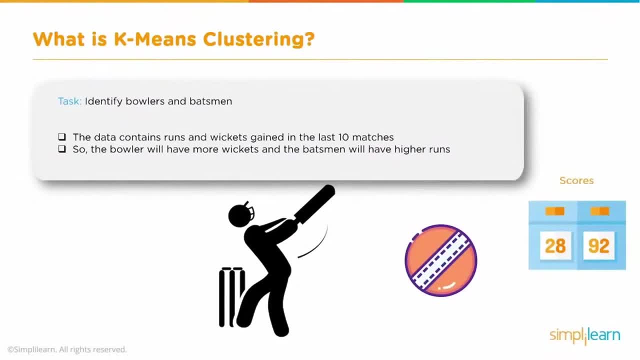 So the bowlers basically take wickets and the batsmen score runs. There will be, of course, a few bowlers who can score some runs And similarly there will be some batsmen who would have taken a few wickets. But with this information we want to cluster those players into batsmen and bowlers. 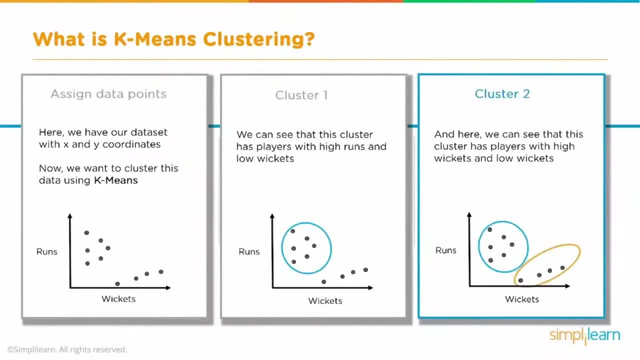 So how does this work? Let's say this is how the data is. So there is information on the y-axis about the runs scored and on the x-axis about the wickets taken by the players. So if we do a quick plot, this is how it would look. 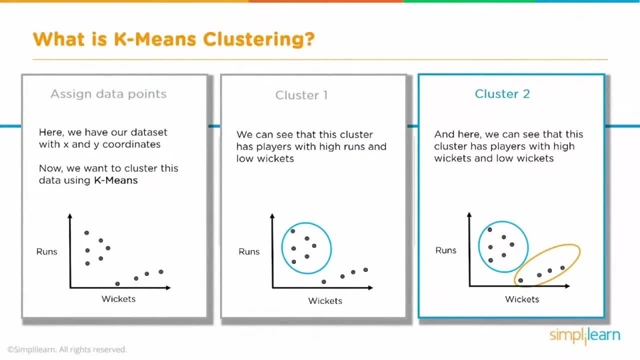 And when we do the clustering, we need to have the clusters, like shown in the third diagram out here. So we need to have a cluster which consists of people who have scored high runs, which is basically the batsmen, And then we need a cluster with people who have taken a lot of wickets, which is typically the bowlers. 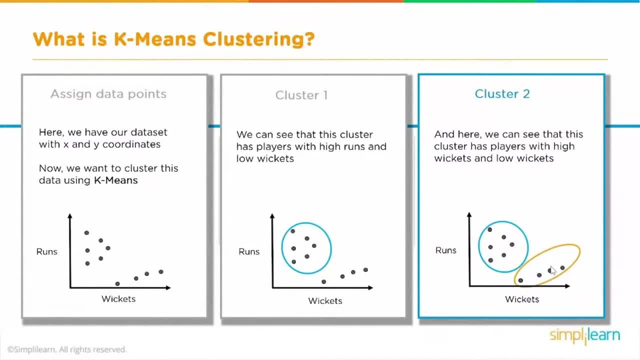 There may be a certain amount of overlap, but we will not talk about it right now. So with k-means clustering, we will have That means k is equal to two and we will have two clusters, which is batsman and bowlers. 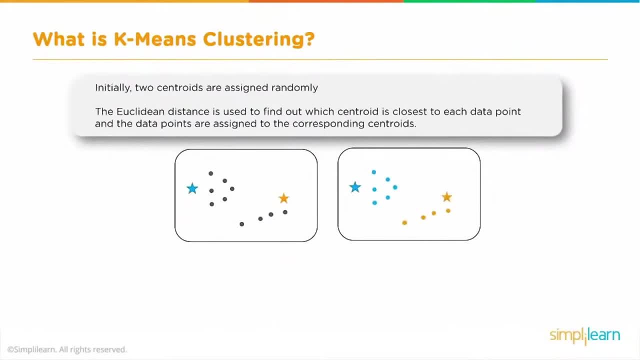 So how does this work? The way it works is: the first step in k-means clustering is the allocation of two centroids randomly, So two points are assigned as so called centroids. So in this case we want two clusters, which means k is equal to two. 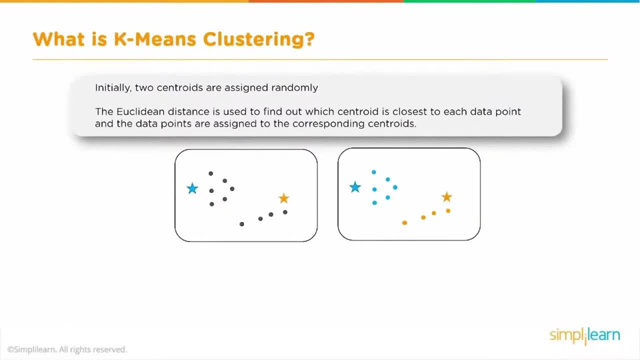 So two points have been randomly assigned as centroids. Look this: centroids, keep in mind. these points can be anywhere. there are random points. they are not initially, they are not really the centroids. centroid means it's a central point of a given data set, but in this case, when it starts off, it's not really the centroid. okay, so these points. 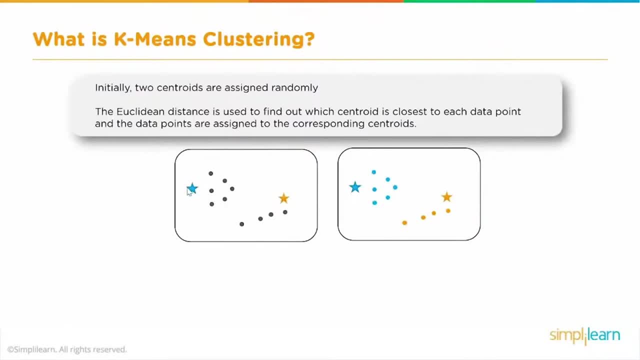 though, in our presentation here, we have shown them one point closer to these data points and another closer to these data points, they can be assigned randomly anywhere. okay, so that's the first step. the next step is to determine the distance of each of the data points from each. 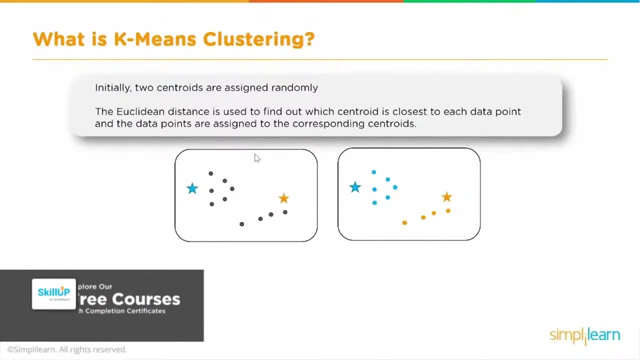 of the randomly assigned centroid. so, for example, we take this point and find the distance from this centroid and the distance from this centroid. this point is taken and the distance is found from this centroid and this and so on and so forth. so for every point the distance is measured from both the centroids and then whichever distance is less that point is. 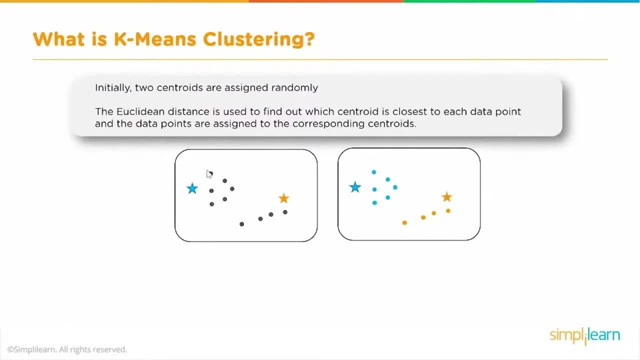 assigned to that centroid. so, for example, in this case, visually, it is very obvious that all these data points are assigned to this centroid and all these data points are assigned to this centroid, and that's what is represented here in blue color and in this yellow color. the next step is to 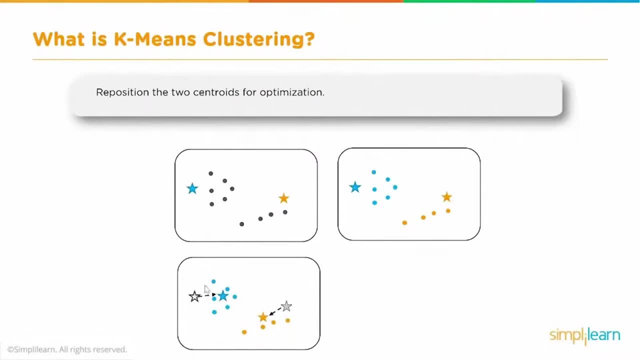 actually determine the central point or the actual centroid for these two clusters. so we have this one initial cluster, this one initial cluster, but, as you can see, these points are not really the centroid. centroid means it should be the central position of this data set, central position of this data set. so that is what needs to be determined as 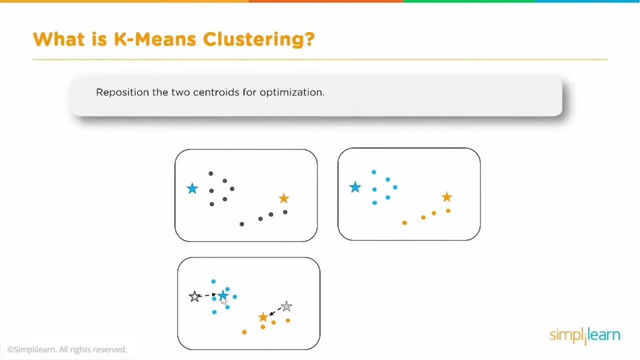 the next step. so the central point or the actual centroid is determined and the original randomly allocated centroid is repositioned to the actual centroid of these new clusters and this process is actually repeated. now what might happen is some of these points may get reallocated. in our example that is not happening probably, but it may so happen. 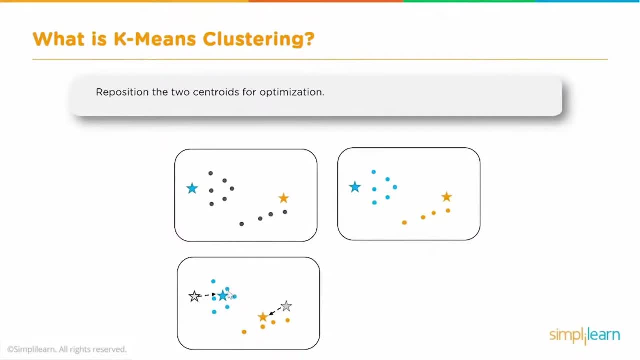 that the distance is found between each of these data points, once again with these centroids, and if there is, if it is required, some points may be reallocated. we will see that in a later example, but for now we will keep it simple. so this process is allowed till the centroid repositioning stops and that is our final cluster. so this is our. so after: 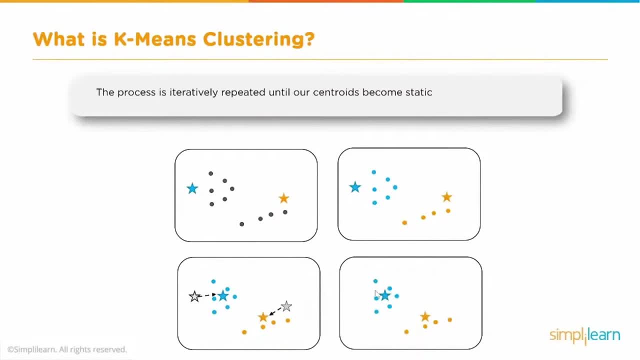 iteration, we come to this position, this situation where the centroid doesn't need any more repositioning and that means our algorithm has converged, convergence has occurred and we have the cluster, two clusters, we have the clusters with a centroid. so this process is repeated, the process of calculating the distance and repositioning the centroid is repeated till the repositioning. 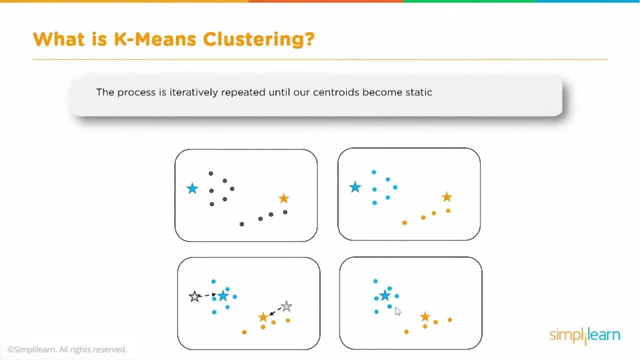 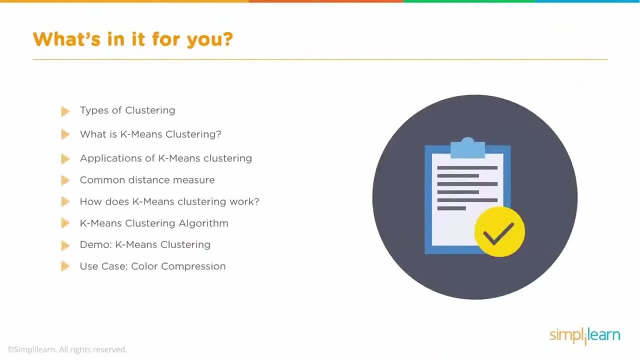 stops, which means that the algorithm has converged and we have the final cluster with the data points and the centroids. so this is what you're going to learn from this session. we will talk about the types of clustering. what is k-means clustering, application of k-means clustering, k-means clustering? 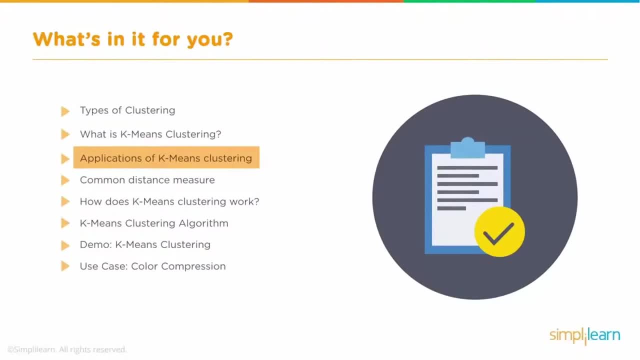 is done using distance measure. we will talk about the common distance measures and then we will talk about how k-means clustering works and go into the details of k-means clustering algorithm, and then we will end with a demo and a use case for k-means clustering. so let's begin. first of all, what are the types of clustering? 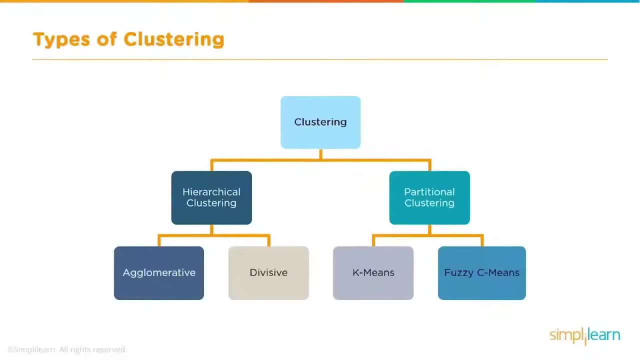 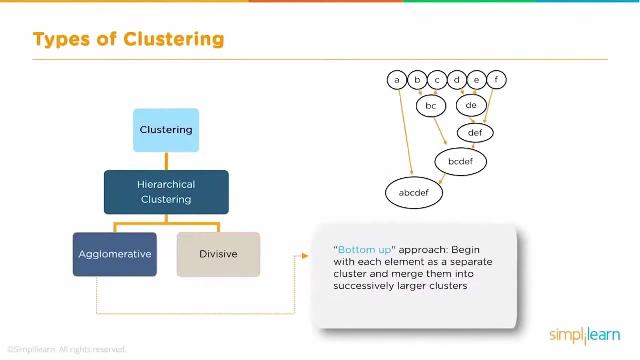 there are primarily two categories of clustering- hierarchical clustering and then partitional clustering- and each of these categories are further subdivided into agglomerative and divisive clustering and k-means and fuzzy c-means clustering. let's take a quick look at what each of these types of clustering are. in hierarchical clustering, the clusters have a tree-like structure. 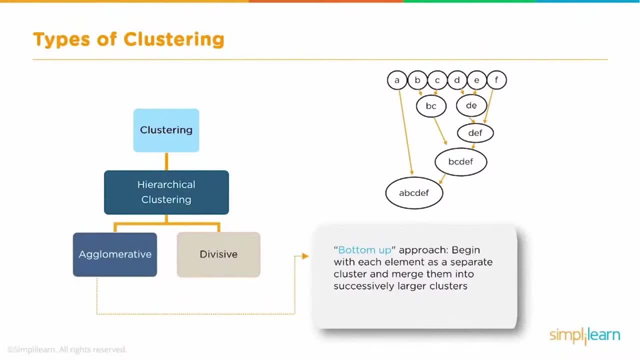 and hierarchical clustering is further divided into agglomerative and divisive. agglomerative clustering is a bottom-up approach. we begin with each element as a separate cluster and merge them into successively larger clusters. so, for example, we have a, b, c, d, e, f. we start by combining b and c form one cluster, d, e and e form one more. then we 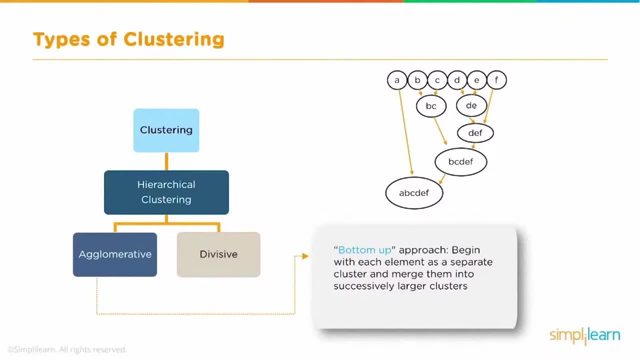 combine d, e and f- one more bigger cluster, and then add b, c to that and then finally a to it. compared to that, divisive clustering or divisive clustering is the top-down approach. we begin with the whole set and proceed to divide it into successively smaller clusters. so we have a, b, c, d, e, f. we first. 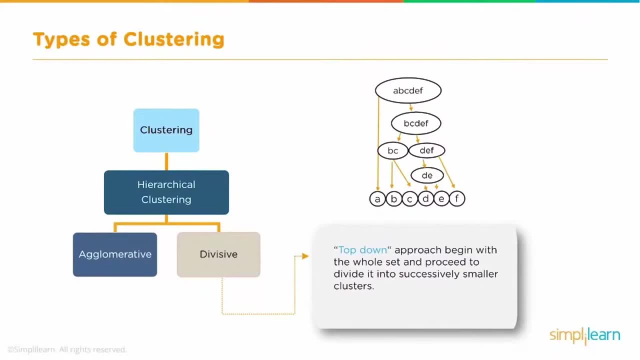 take that as a single cluster and then break it down into a, b, c, d, e and f. then we have partitional clustering, split into two subtypes: k-means clustering and fuzzy c-means. in k-means clustering the objects are divided into the number of. 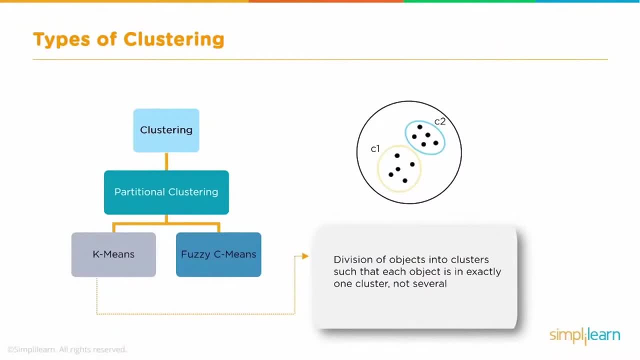 clusters mentioned by the number k. that's where the k comes from. so if we say k is equal to two, the objects are divided into two clusters, c1 and c2, and the way it is done is the features or are compared and all objects having similar characteristics are clubbed together. so that's. 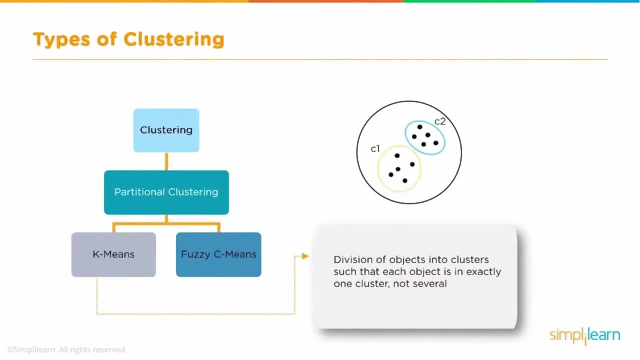 how k-means clustering is done. we will see it in more detail as we move forward. and fuzzy c-means is very similar to k-means in the sense that it clubs objects that have similar characteristics together, but while in k-means clustering two objects cannot belong to, or any object a single. 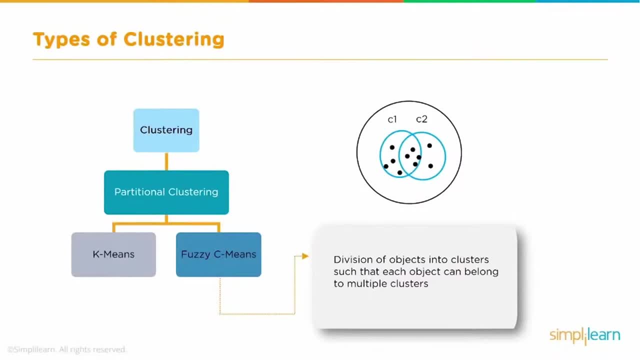 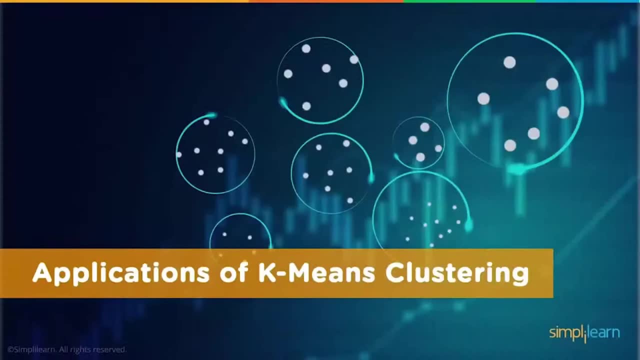 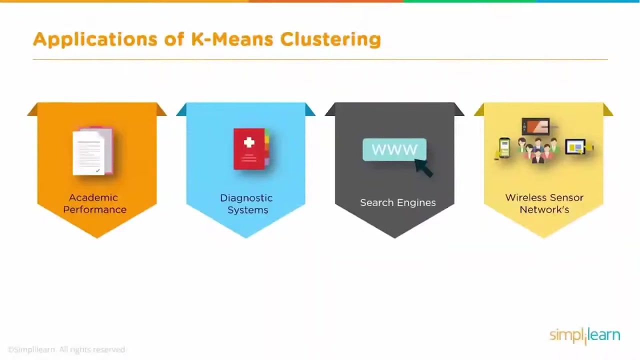 object cannot belong to two different clusters. in c-means objects can belong to more than one cluster. so that is the primary difference between k-means and fuzzy c-means. so what are some of the applications of k-means clustering? k-means clustering is used in a variety of examples. 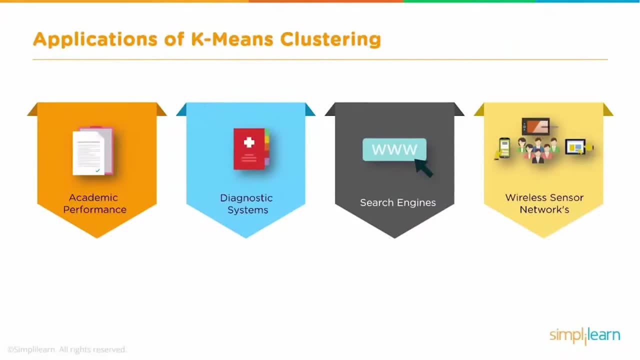 or variety of business cases in real life, starting from academic performance diagnostic systems, search engines and wireless sensor networks, and many more. so let us take a little deeper look at each of these examples. academic performance, so, based on the scores of students, students are categorized into a, b, c and so on. clustering forms a backbone of search engines. 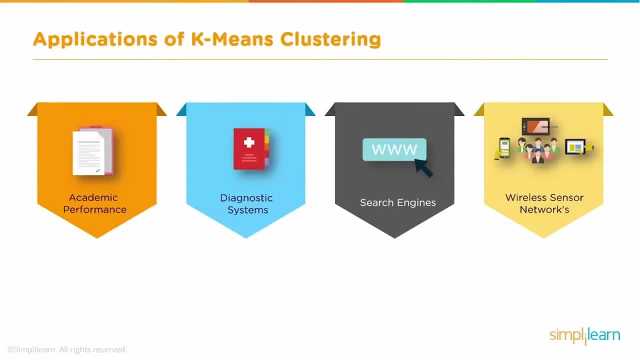 when a search is performed, the search results need to be grouped together. the search engines very often use clustering to do this and, similarly, in case of wireless sensor networks, the clustering algorithm plays the role of finding the cluster heads, which collects all the data in its respective cluster. so clustering, especially k-means. 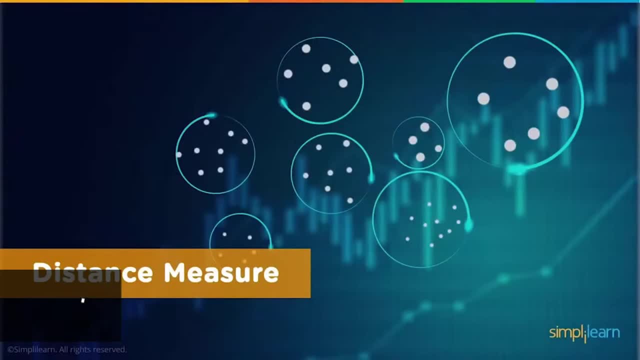 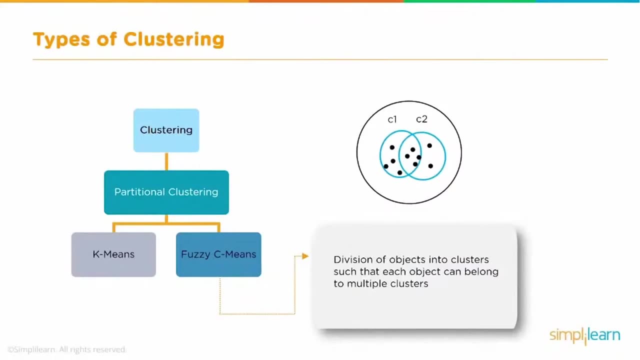 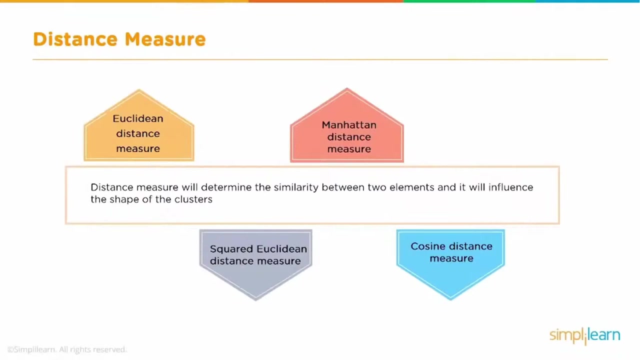 clustering uses distance measure, so let's take a look at what is distance measure. so, while these are the different types of clustering, in this video we will focus on k-means clustering. so distance measure tells how similar some objects are, so the similarity is measured using what is. 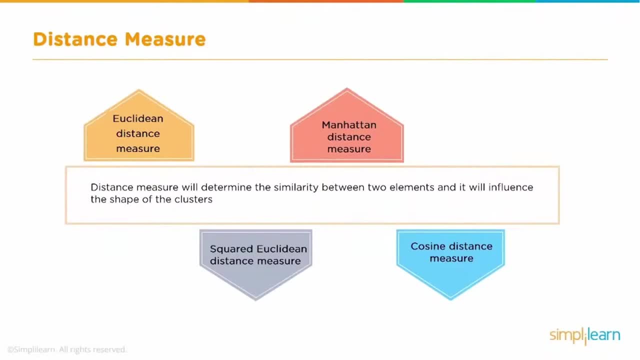 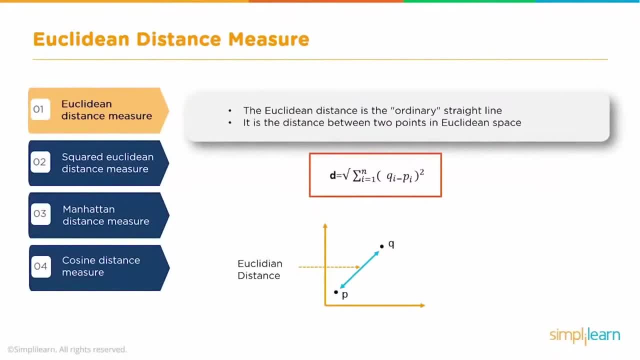 is Euclidean distance measure. this is nothing but the distance between two points. so we have learned in high school how to find the distance between two points. this is a little sophisticated formula: square plus x2 minus x1, whole square. so this is an extension of that formula. so that is the Euclidean 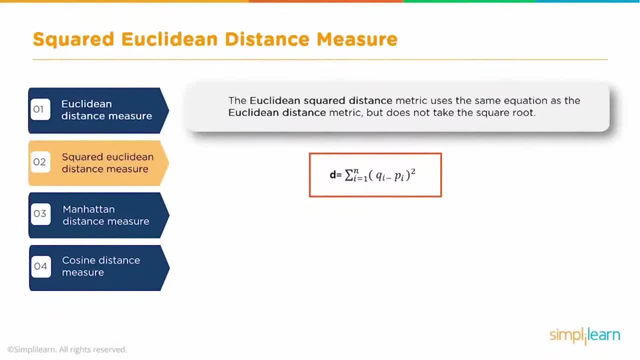 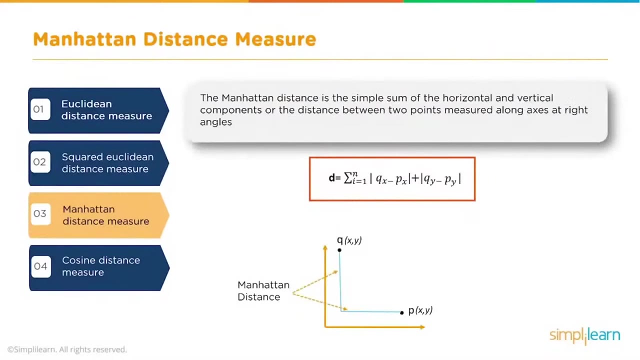 distance between two points. what is the squared Euclidean distance measure? it's nothing but the square of the Euclidean distance, as the name suggests. so instead of taking the square root, we leave the square as it is, and then we have Manhattan distance measure in case of Manhattan. 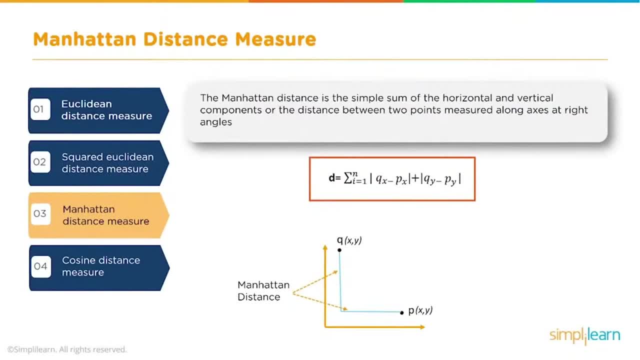 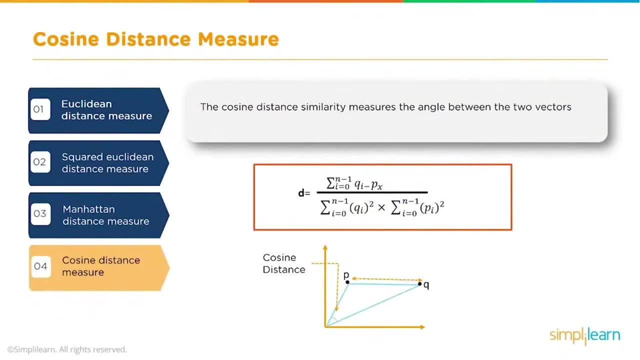 distance. it is the sum of the distances across the x-axis and the y-axis, and note that we are taking the absolute value so that the negative values don't come into play. so that is the Manhattan distance measure. then we have cosine distance measure. in this case we take the angle between the two vectors formed by joining. 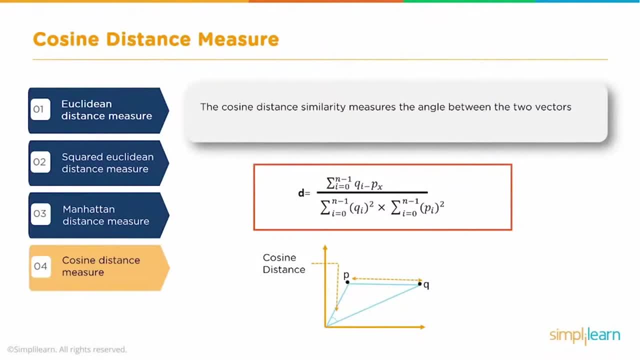 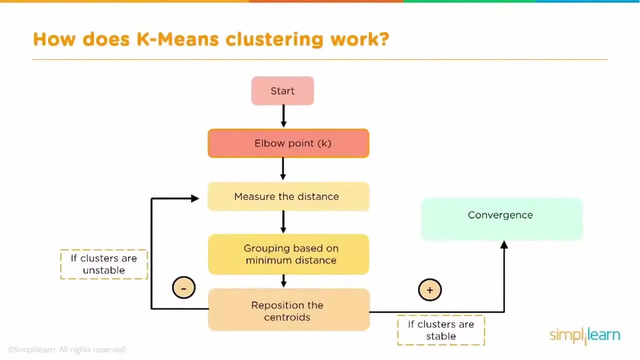 the points from the origin. so that is the cosine distance measure. okay, so that was a quick overview about the various distance measures that are supported by k-means. now let's go and check how exactly k-means clustering works. okay, so this is how k-means 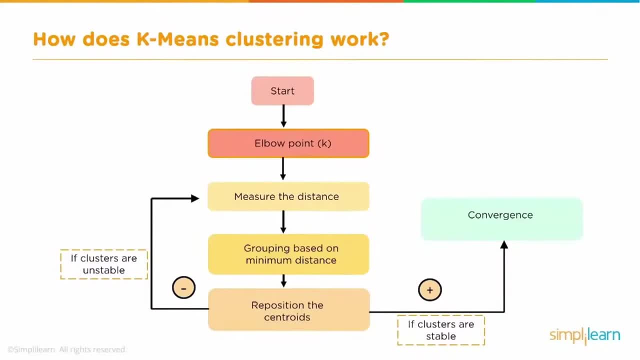 clustering works. this is like a flow chart of the whole process. there is a starting point and then we specify the number of clusters that we want. now there are a couple of ways of doing this. we can do by trial and error. so we specify a certain number. maybe k is equal to three or four or five. to start, 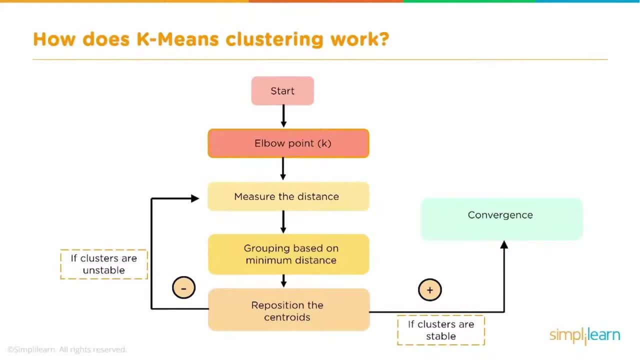 this. we keep changing until we get the best clusters. or there is a technique called elbow technique, whereby we can determine the value of k, what should be the best value of k, how many clusters should be formed? so once we have the value of k, we specify that and then the system. 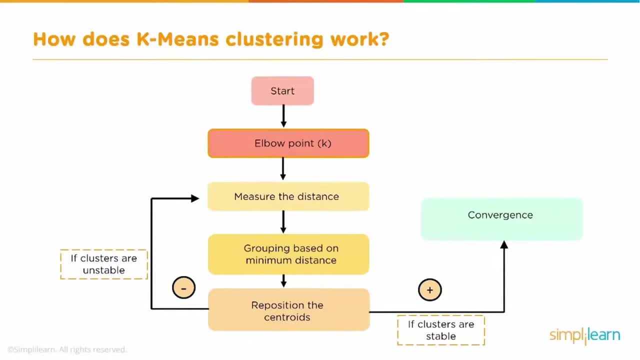 will assign that many centroids. so it picks randomly that to start with, randomly that many points that are considered to be the centroids of these clusters, and then it measures the distance of each of the data points from these centroids and assigns those points to the corresponding centroid from which the distance is minimum. so each data point will 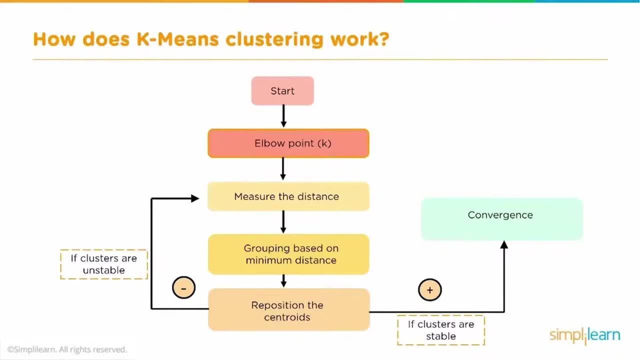 be assigned to the centroid which is closest to it, and thereby we have k number of initial clusters. however, this is not the final clusters. the next step it does is for the new groups, for the clusters that have been formed. it calculates the mean position, thereby calculates the new centroid position. the position of the centroid moves compared to the randomly 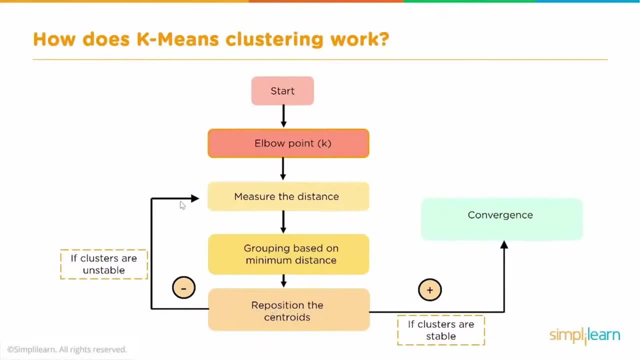 allocated one. so it's an iterative process. once again, the distance of each point is measured from this new centroid point and, if required, the data points are reallocated to the new centroids and the mean position or the new centroid is calculated once again. if the centroid moves, then the iteration continues, which means 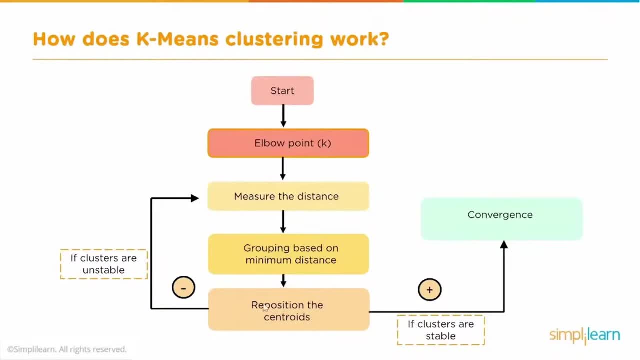 the convergence has not happened, the clustering has not converged. so as long as there is a movement of the centroid, this iteration keeps happening. but once the centroid stops moving, which means that the cluster has converged or the clustering process has converged, that will be the end result. so now, 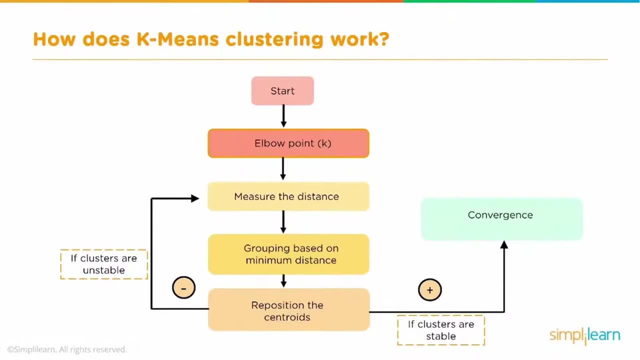 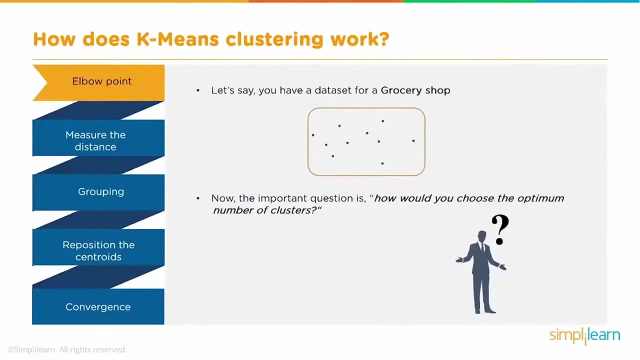 we have the final position of the centroid and now we finished. at the end the data points are allocated accordingly to the closest centroid. I know it's a little difficult to understand from this simple flow chart, so let's do a little bit of visualization and see if we can explain it better. let's take an example. if we have 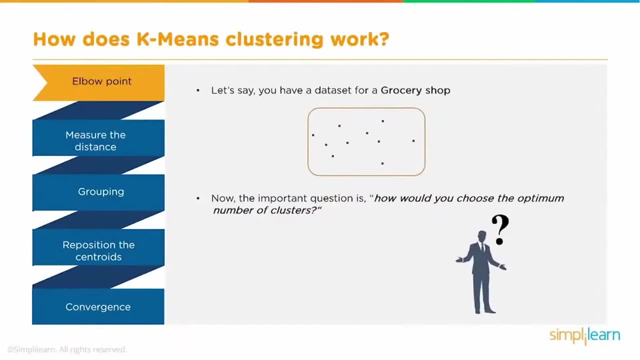 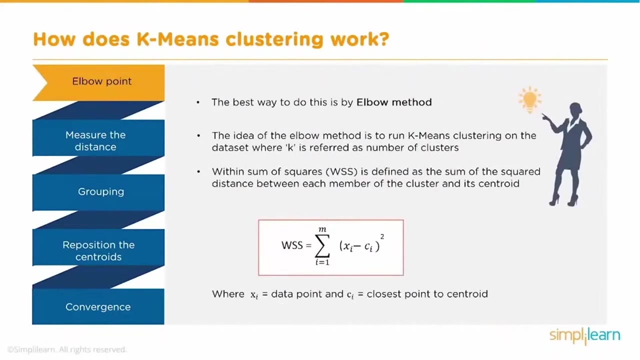 a data set for a grocery shop. so let's say we have a data set for a grocery shop and now we want to find out how many clusters this has to be spread across. so how do we find the optimum number of clusters? there is a technique called the elbow method. so when these 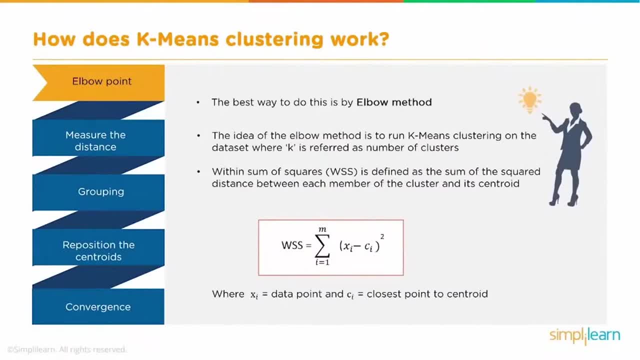 clusters are formed. there is a parameter called within sum of squares, and the lower this value is, the better the cluster is. that means all these points are very close to each other, so we use this within sum of squares as a measure to find the optimum number of clusters that can be formed. 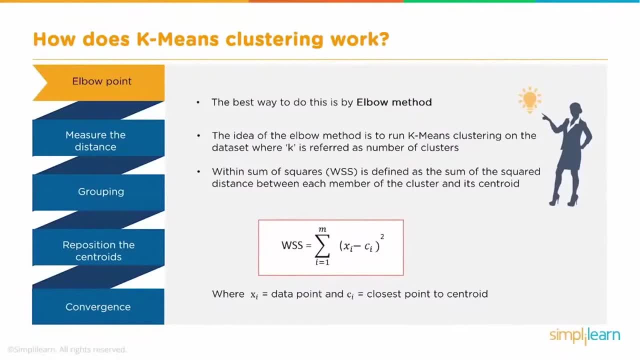 for a given data set. so we create clusters or we let the system create clusters of a variety of numbers, maybe of 10, 10 clusters, and for each value of k, the within ss is measured and the value of k which has the least amount of within ss or w. 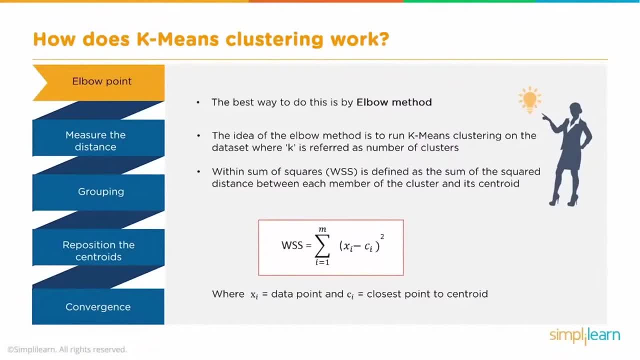 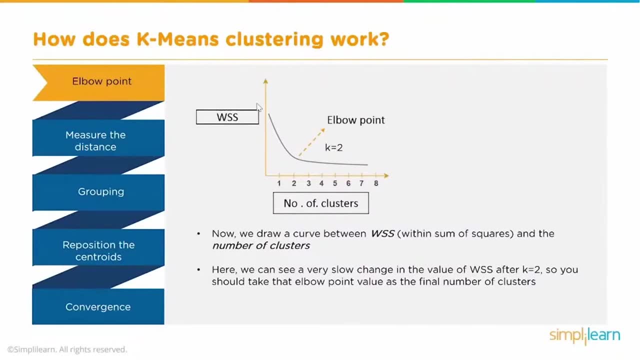 ss, that is taken as the optimum value of k. so this is the diagrammatic representation. so we have on the y-axis the within sum of squares, or wss, and on the x-axis we have the number of clusters. so, as you can imagine, if you have, k is equal to 1, which means all the data points are in a single. 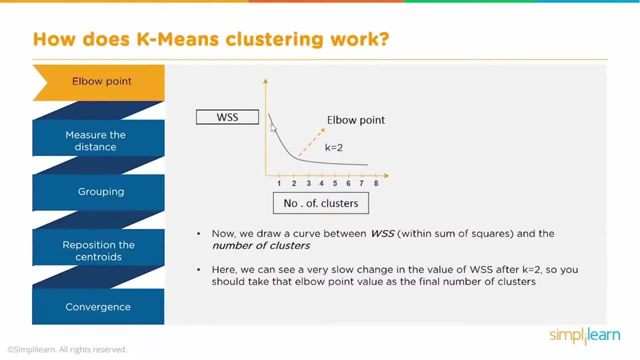 cluster, the within ss value will be very high because they are probably scattered all over. the moment you split it into you do, there will be a drastic fall in the within ss value. that's what is represented here. but then, as the value of k increases, the decrease, the rate of decrease, will not be so high. it will continue. 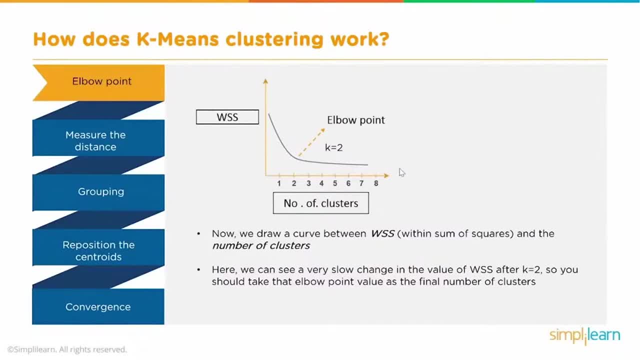 to decrease, but probably the rate of decrease will not be high. so that gives us an idea. so from here we get an idea. for example, the optimum value of k should be either 2 or 3 or at the most 4, but beyond that the value of k should be 2 or 3 or at the most 4, but beyond that the value of k should. 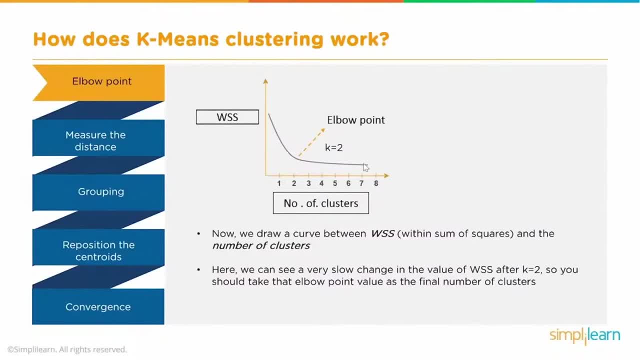 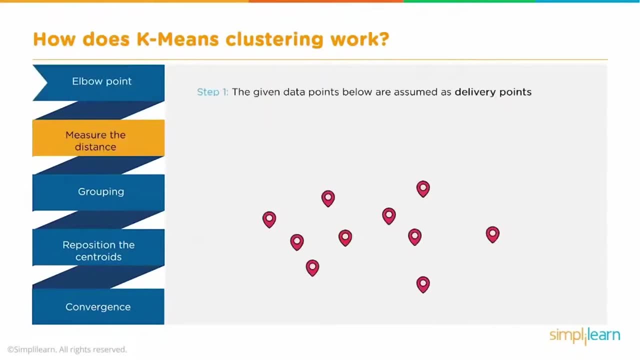 be 1 or 3 and from the start of the Leben Richter lambda m times k version of k. so we have a function r Ettling. so p somewhere between p1 of p, everyone's going to be the p function of p to the murder. p is a well known citation actually in chemistry. so the congress and 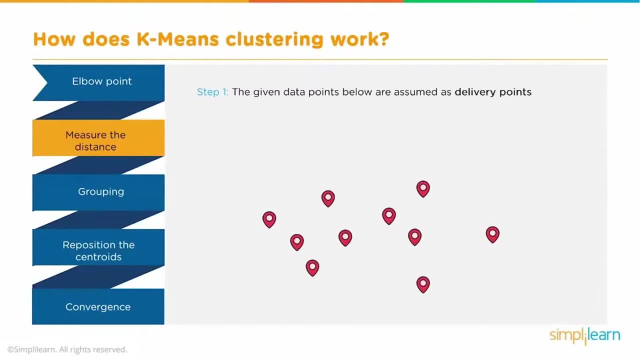 obviously, in mathematics of the acceleration that is going to be the addition, läh is bound to be the variation. Wow, but it's a little bit more complicated for some people to be able to. location from the centroid is measured and each point is assigned to the centroid which is closest. 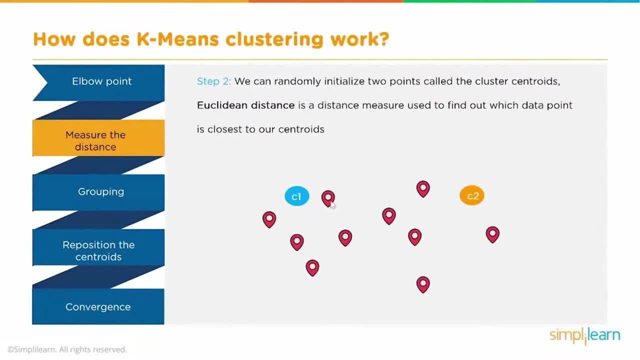 to it. So, for example, these points are very obvious that these are closest to C1, whereas this point is far away from C2.. So these points will be assigned. which are close to C1 will be assigned to C1, and these points or locations which are close to C2 will be assigned to C2.. 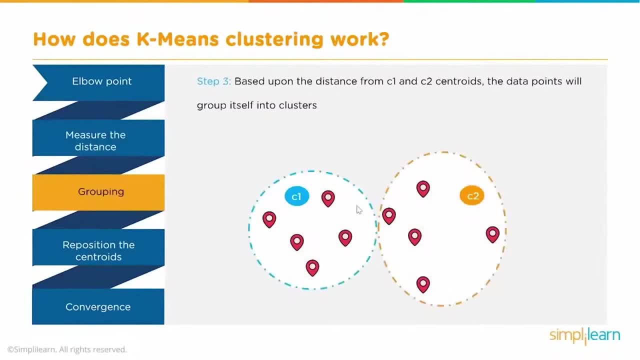 And then. so this is the how the initial grouping is done. This is part of C1 and this is part of C2.. Then the next step is to calculate the actual centroid of this data because, remember, C1 and C2 are not the centroids. They have been randomly assigned points and only thing that has been done. 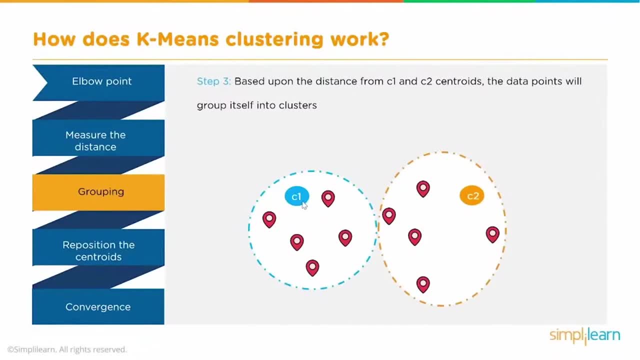 was the data points which are closest to them have been assigned to them. But now, in this step, the actual centroid will be calculated, Which may be, for each of these data sets, somewhere in the middle. so that's like the mean point that will be calculated And the centroid will actually be positioned or repositioned there. 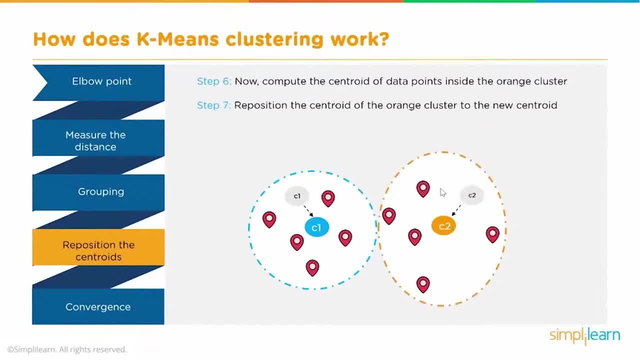 Same with C2, so the new centroid for this group is C2 in this new position and C1 is in this new position. Once again, the distance of each of the data points is calculated from these centroids. Now, remember, it's not necessary that the distance still remains, or each of these data points. 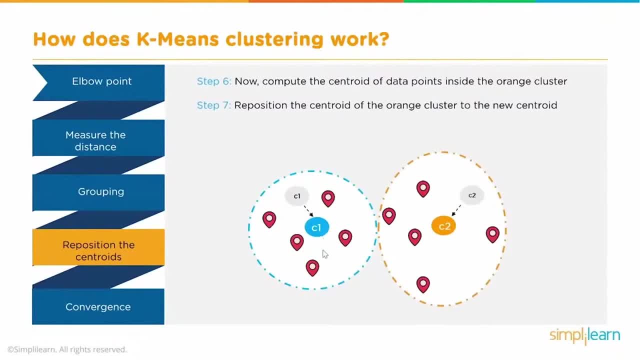 still remains. They are called that: last dozen points. This is the new position which happens. I know that if you're not familiar with this, information means that it's always'a bit of a haciendo in the same group. by recalculating the distance, it may be possible that some 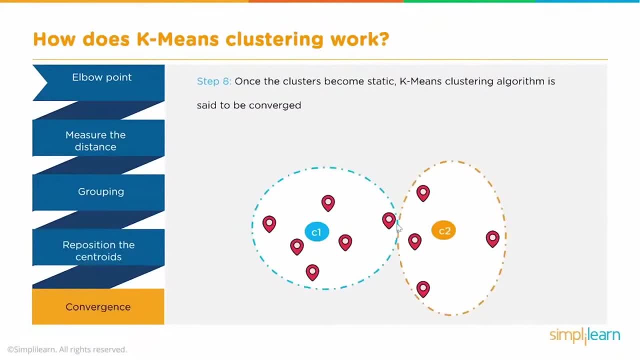 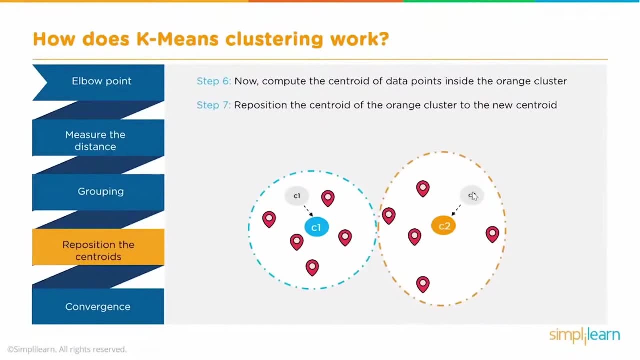 points get reallocated like. so you see this. so this point earlier was closer to c2 because c2 was here. but after recalculating, repositioning, it is observed that this is closer to c1 than c2. so this is the new grouping. so some 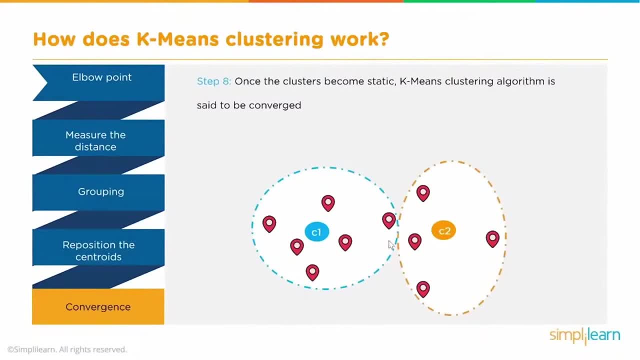 points will be reassigned and again the centroid will be calculated. and if the centroid doesn't change- so that is a repetitive process, iterative process- and if the centroid doesn't change, once the centroid stops changing, that means the algorithm has converged. and this is our final cluster, with this as the centroid. 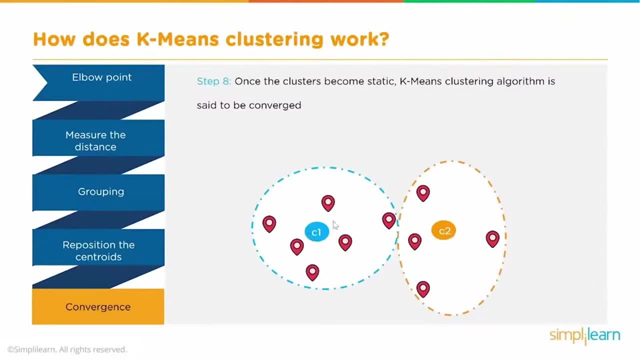 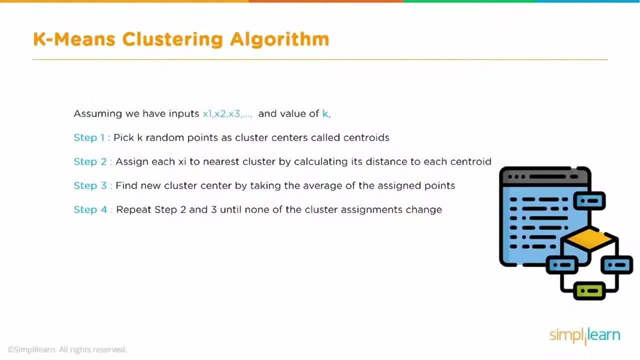 c1 and c2 as the centroids, these data points as a part of each cluster. so I hope this helps in understanding the whole process: iterative process, process of k-means clustering. so let's take a look at the k-means clustering algorithm. let's say we have x1, x2, x3, n number of points as our inputs and we want to 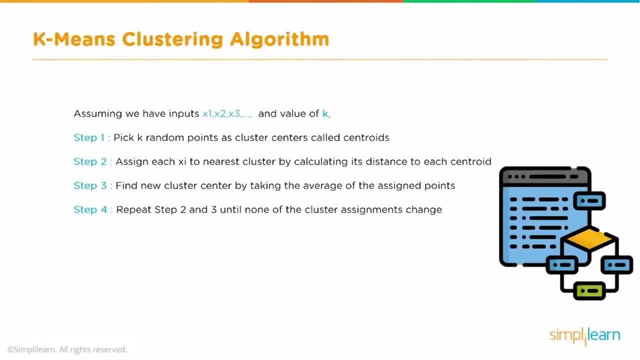 split this into k clusters, or we want to create k clusters. so the first step is to randomly pick k points and call them centroid. they are not real centroids, because centroid is supposed to be a centre point, but they are just changing around the circuit, which is more important, for isn't it? 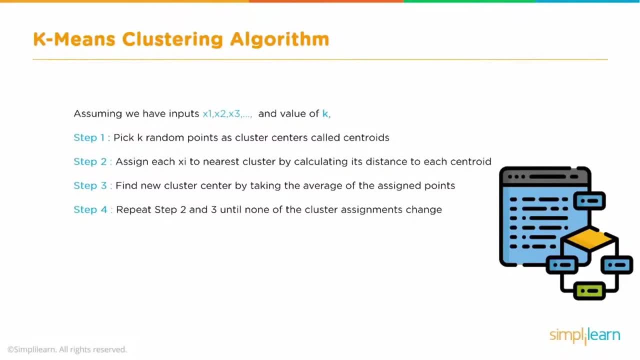 called centroids And we calculate the distance of each and every input point from each of the centroids. So the distance of x1 from c1, from c2, c3, each of the distances we calculate And then find out which distance is the lowest and assign x1 to that particular random centroid. Repeat that. 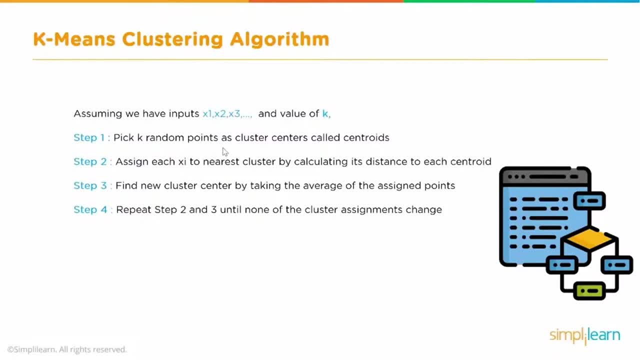 process for x2.. Calculate its distance from each of the centroids c1, c2, c3 to ck and find which is the lowest distance and assign x2 to that particular centroid, Same with x3, and so on. So that is the first round of assignment. that is done. Now we have k groups because there are 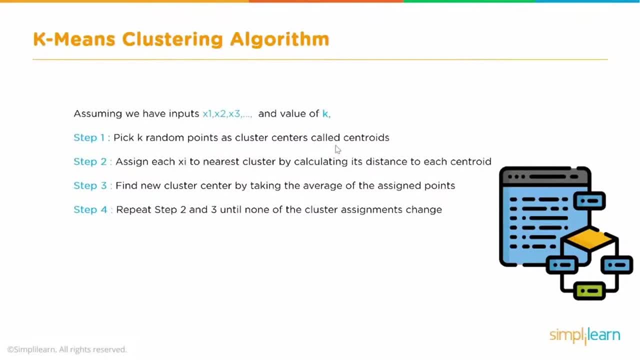 we have assigned the value of k, So there are k centroids and so there are k groups. All these inputs are assigned to the k centroids. So we have assigned the value of k, So there are k groups. All these inputs are assigned to the k centroids. All these inputs are assigned to the. 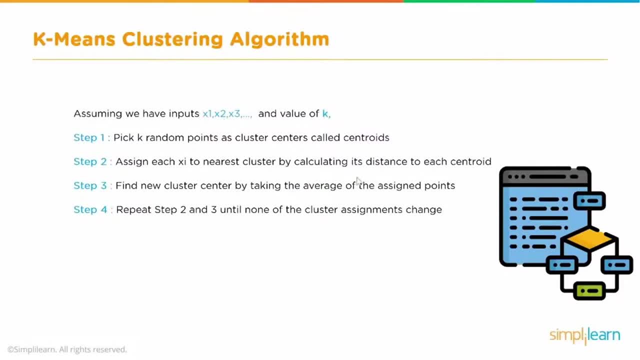 k groups. All these inputs have been split into k groups. However, remember we picked the centroids randomly, So they are not real centroids. So now what we have to do? we have to calculate the actual centroids for each of these groups, which is like the mean position, which means that 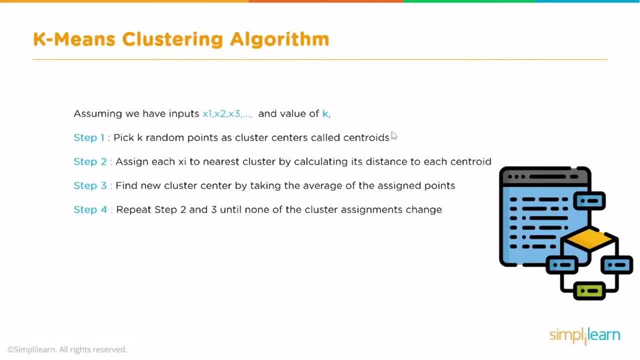 the position of the randomly selected centroids will now change and they will be the mean positions of these newly formed k groups. And once that is done, we once again repeat this process of calculating the distance right? So this is what we are doing. as a part of step four, We repeat step two and three, So we again calculate the distance of x1. 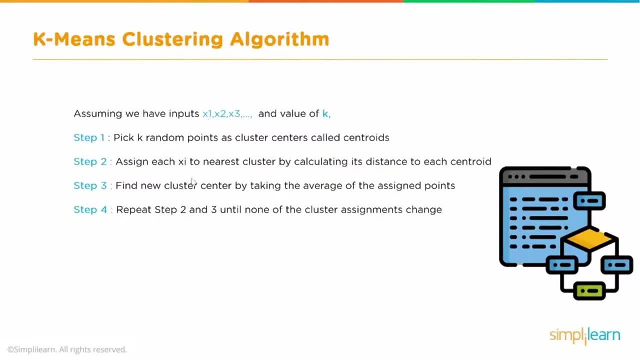 from the centroid c1,, c2,, c3, and then c, which is the lowest value, and assign x1 to that. Calculate the distance of x2 from c1,, c2,, c3 or whatever up to ck and find the distance of x1. 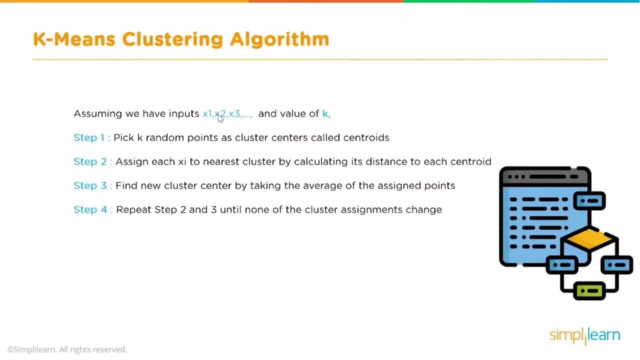 whichever is the lowest distance and assign x2 to that centroid and so on. In this process there may be some reassignment. x1 was probably assigned to cluster c2 and after doing this calculation maybe now x1 is assigned to c1. So that kind of reallocation may happen. So we repeat: 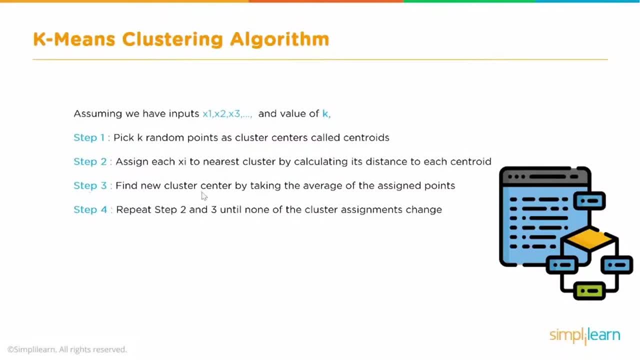 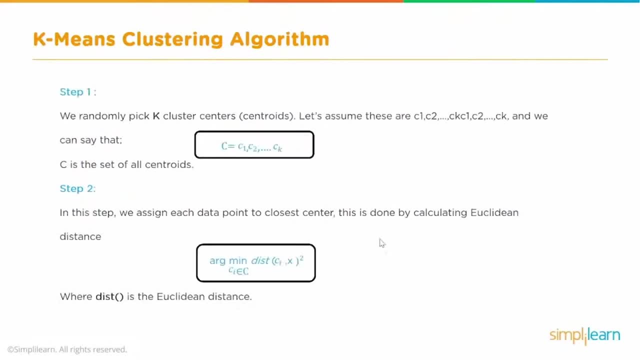 steps two and three till the position of the centroids don't change or stop changing, And that's when we have convergence. So let's take a detailed look at each of these steps. So we randomly pick k cluster centers. We call them centroids because they are not initially. they are not really the centroids, So we let us name. 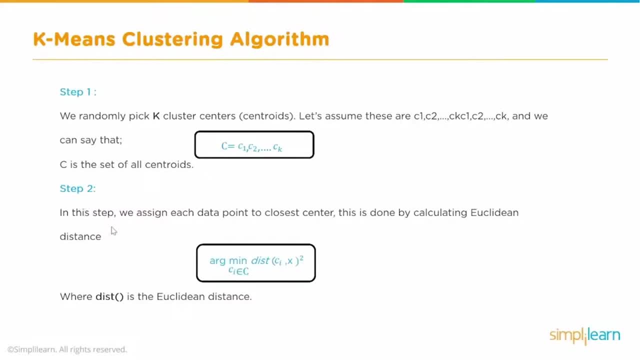 them: c1, c2, up to ck, And then step two, we assign each data point to the closest center. So what we do? we calculate the distance of each x value from each c value. So the distance between x1, c1,. 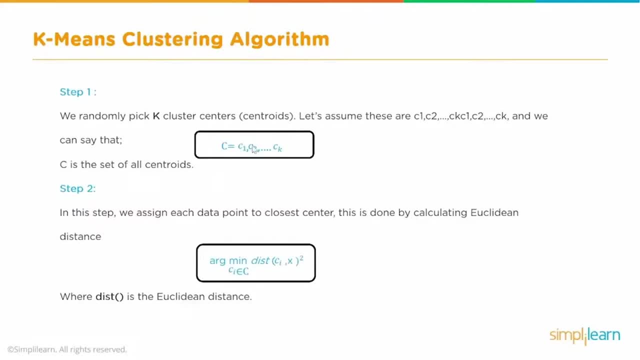 distance between x1, c2, c3, and c1.. So we calculate the distance of each x value from each c value, between x1, c2, x1, c3. And then we find which is the lowest value. right, That's the minimum value. 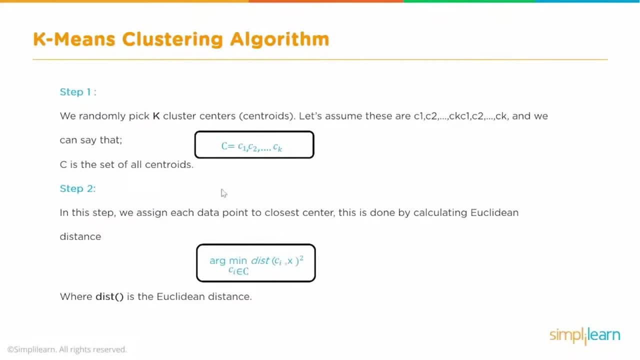 we find And assign x1 to that particular centroid, Then we go next to x2.. Find the distance of x2 from c1, x2 from c2, x2 from c3, and so on up to ck And then assign it to the point or to the centroid. 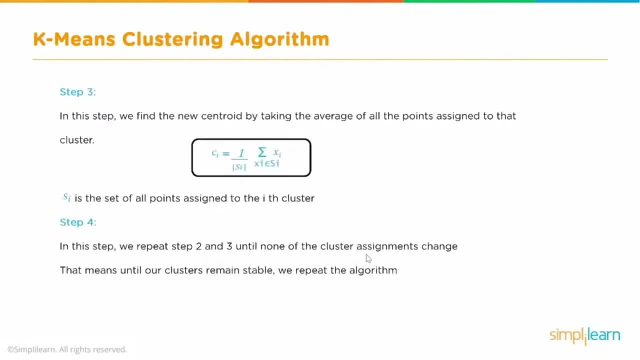 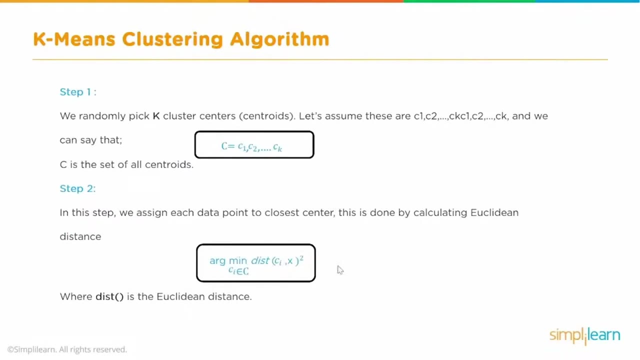 which has the lowest value, and so on. So that is step number two. In step number three, we now find the actual centroid for each group. So what has happened? As a part of step number two, we now have all the points, all the data points, grouped into k groups because we wanted to create 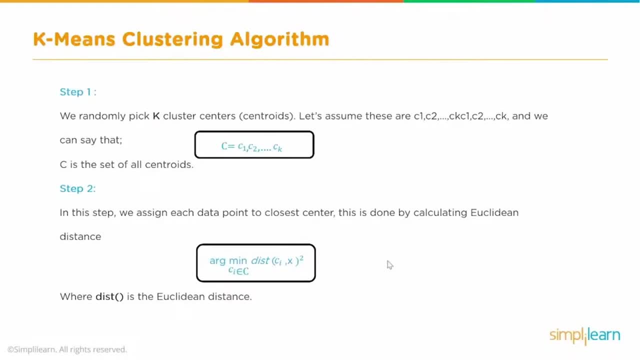 k clusters. right, So we have k groups. Each one may be having a certain number of input values. They need not be equally distributed. by the way, Based on the distance we will have k groups, But remember, the initial values of the c1, c2 were not really the centroids of these groups, right? We? 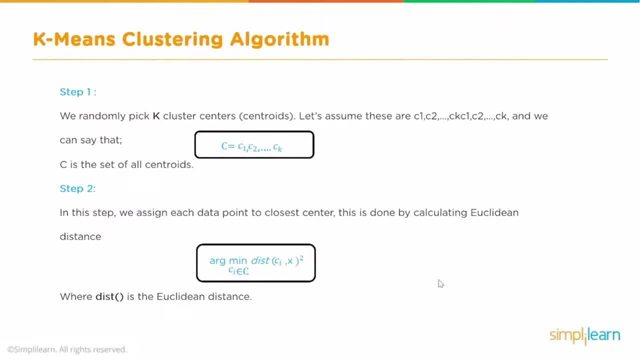 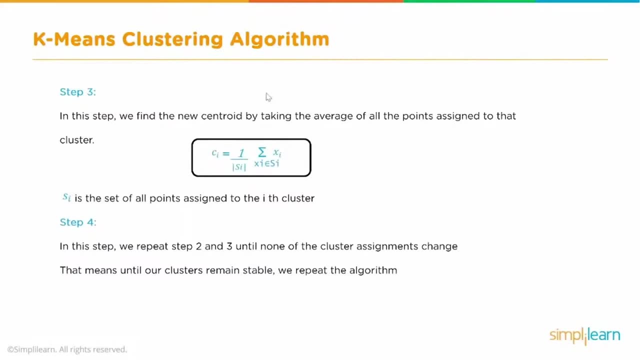 assigned them randomly. So now, in step three, we actually calculate the centroid of each group, which means the original point, which we thought was the centroid, will shift to the new position, which is the actual centroid for each of these groups. okay, And we again calculate the distance. 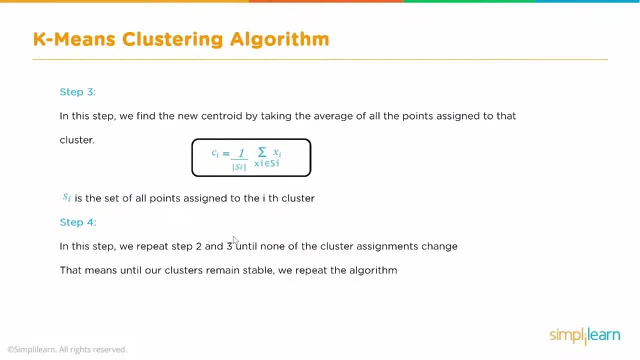 So we go back to step two, which is what We calculate again, the distance of each of these points from the newly positioned centroids And, if required, we reassign these points to the new centroids. So, as I said earlier, there may be a reallocation. So we now have a new set. 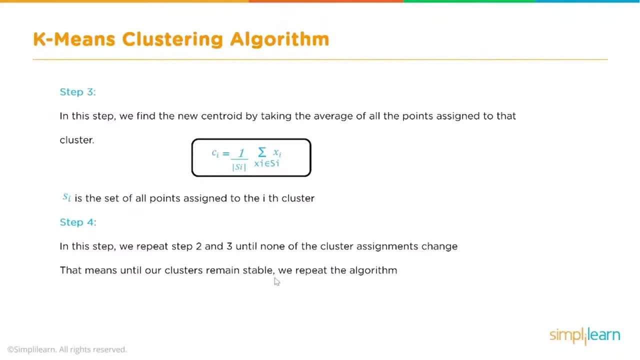 or a new group. We still have k groups, but the number of items and the actual assignment may be different from what was in step two here. okay, So that might change. Then we perform step three once again to find the new centroid of this new group. So we have again a new set of clusters. 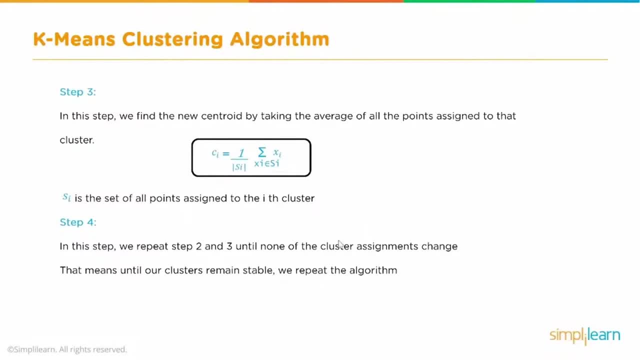 new centroids and new assignments. We repeat this, step two again. Once again we find: And then it is possible that after iterating through three or four or five times, the centroid will stop moving, in the sense that when you calculate the new value of the centroid, 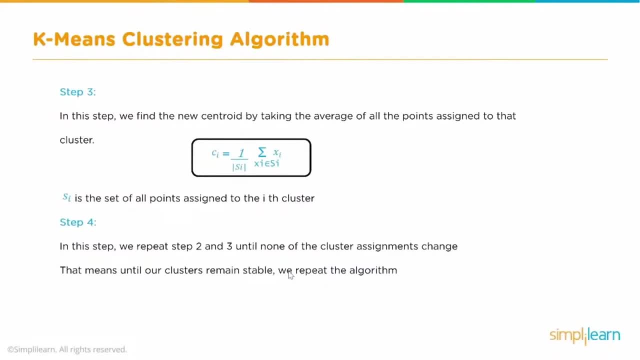 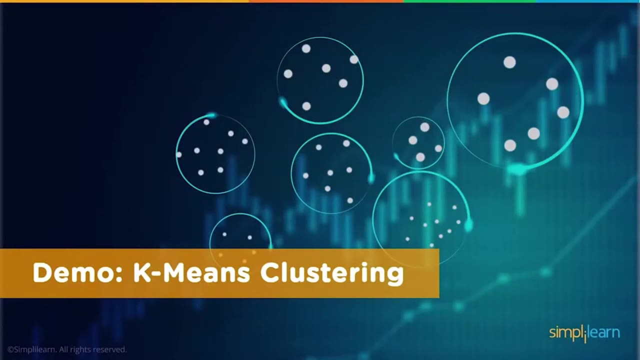 that will be same as the original value or there will be very marginal change. So that is when we say convergence has occurred And that is our final cluster. That's the formation of the final cluster, All right, So let's see a couple of demos of k-means clustering. We will actually see some. 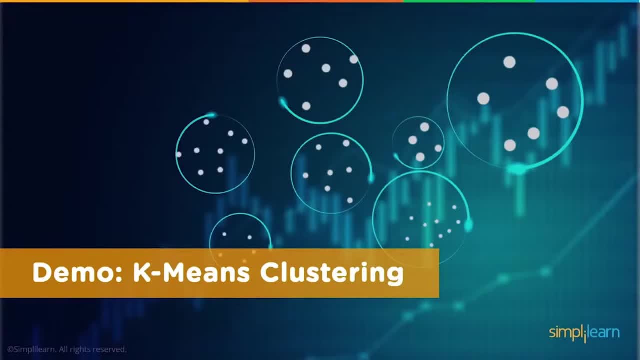 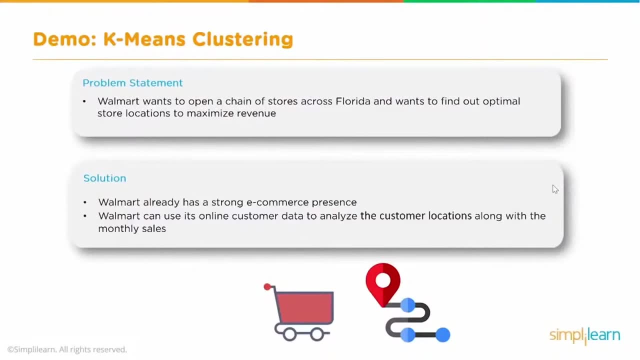 other demos of k-means clustering in a few minutes, But before that let's find out what's the problem that we are trying to solve. The problem statement is: let's say, Walmart wants to open a chain of stores across the state of Florida And it wants to find the optimal store locations. Now the 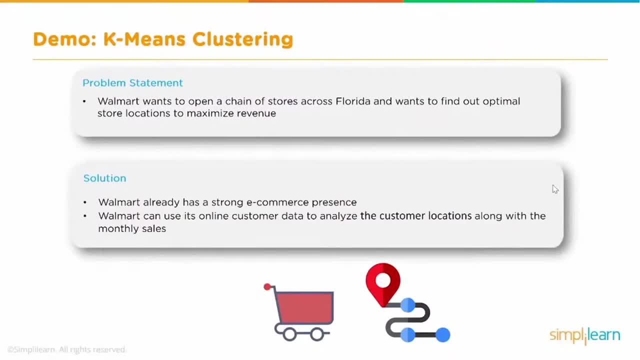 issue here is: if they open too many stores close to each other, obviously they will not make profit, But if they, if the stores are too far apart, they will not have enough sales. So how do they optimize this Now for an organization like 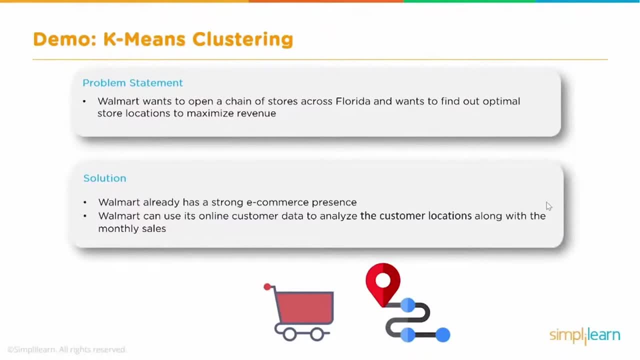 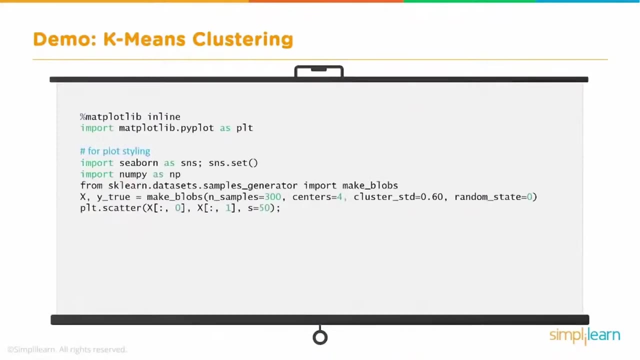 Walmart, which is an e-commerce giant. they already have the addresses of their customers in their database, So they can actually use this information or this data and use k-means clustering to find the optimal location. Now, before we go into the Python notebook and show you the live code, 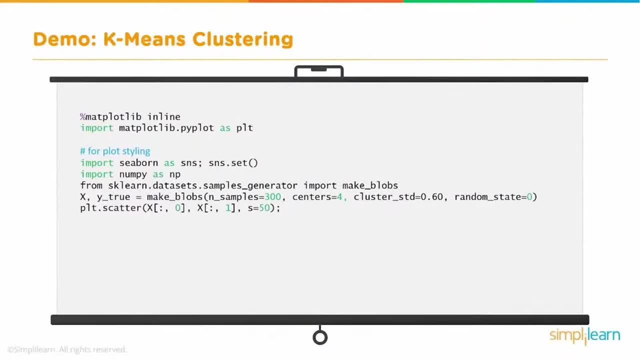 I wanted to take you through very quickly a summary of the code in the slides and then we will go into the Python notebook. So in this block we are basically importing all the required libraries like NumPy, matplotlib and so on, And we are loading the data that is available in the 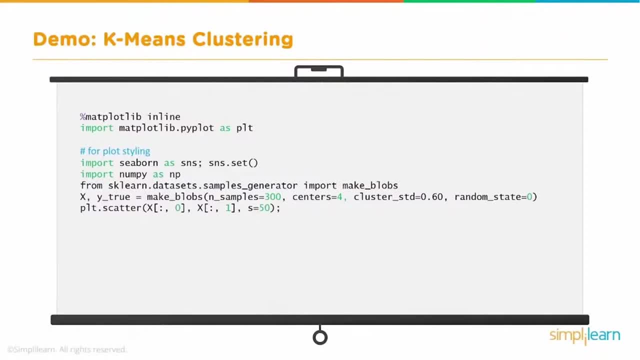 form of, let's say, the addresses. For simplicity's sake we will just take them as some data points. So what we do is quickly do a scatterplot to see how they are related to each other with respect to each other. So in the scatterplot we see that there are a few distinct groups already being 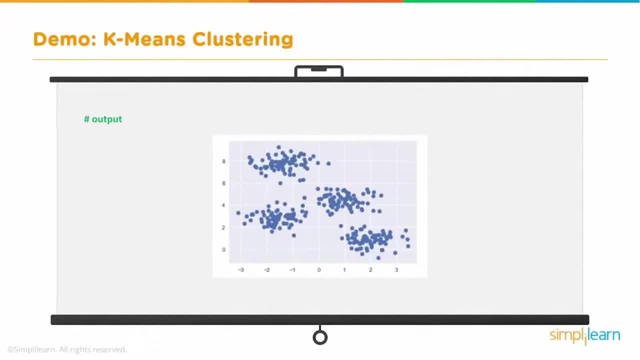 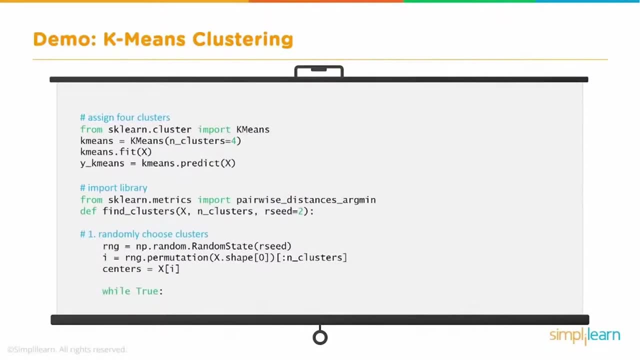 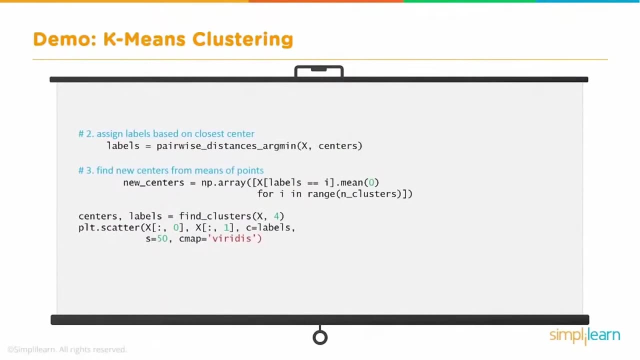 formed So you can actually get an idea about how the cluster would look and how many clusters, what is the optimal number of clusters? And then starts the actual k-means clustering process. So we will assign each of these to the centroids and then check whether they are the optimal distance, which is the shortest. 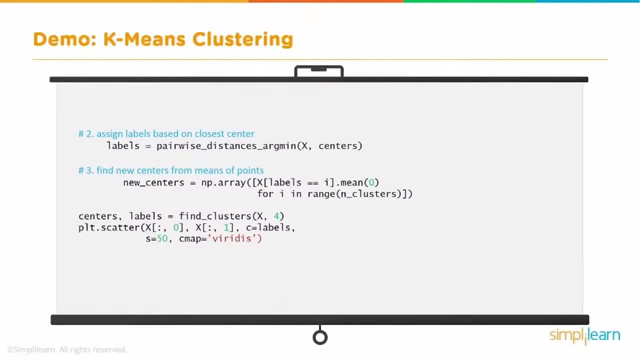 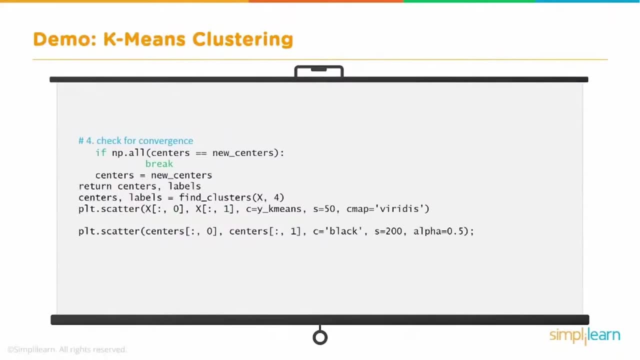 distance and assign each of the data points to the centroids and then go through this iterative process till the whole process converges And finally we get an output like this: So we have four distinct clusters, which is we can say that this is how the population is probably distributed. 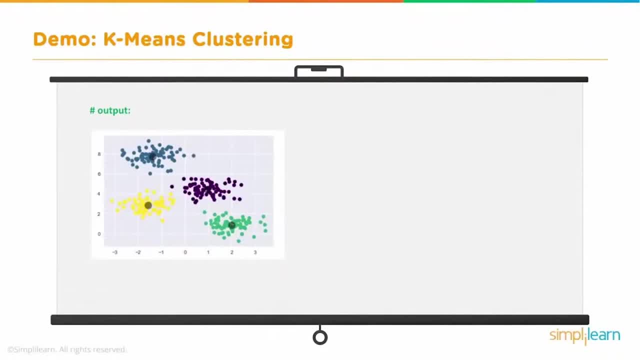 in the store. So we can say that this is how the population is probably distributed in the store. And then we can also say that this is how the population is probably distributed in the store. So we can say that this is how the population is probably distributed in the store. 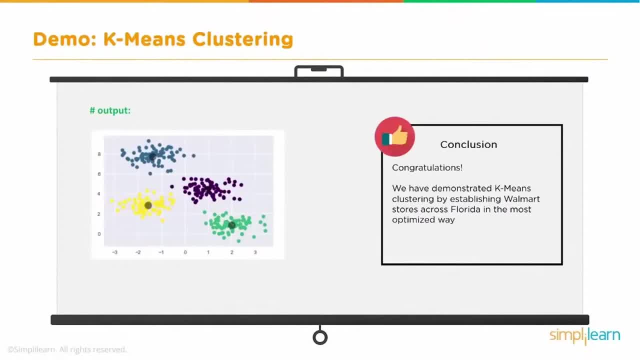 So that's the way we determine the best locations for the store and that's how we can help Walmart find the best locations for their stores in Florida. So now let's take this into Python Notebook. Let's see how this looks when we are running the code. live- All right. 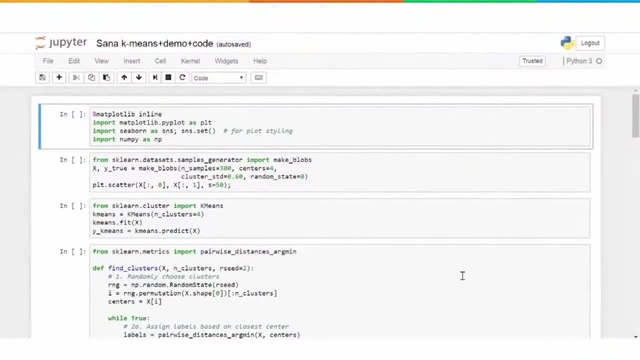 so this is the code for k-means clustering in Jupyter Notebook. We have a few examples here which we will demonstrate how k-means clustering is used, and even there is a small implementation of k-means clustering as well. Okay, so, let's get started. Okay, so this block is basically: 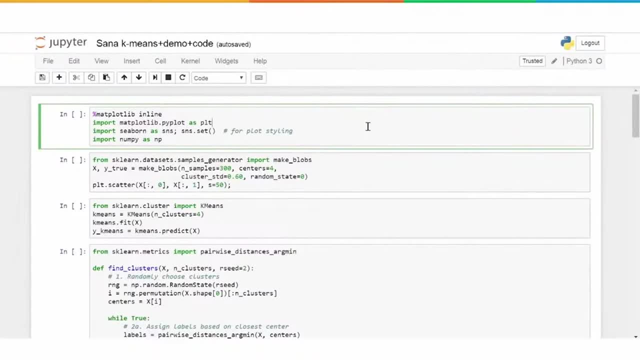 importing the various libraries that are required, like matplotlib and numpy and so on and so forth, which would be used as a part of the code. So let's say we are going and creating blobs which are similar to clusters. Now this is a very neat 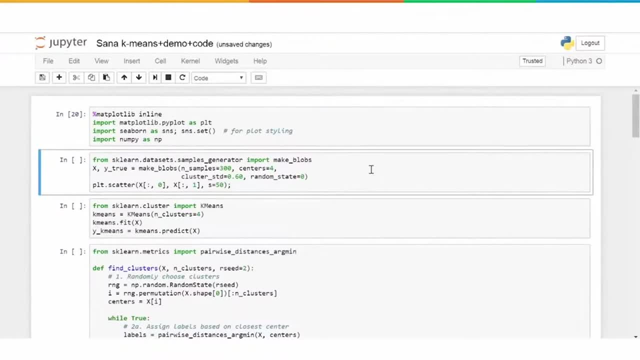 feature which is available in scikit-learn. Make blobs is a nice feature which creates clusters of data sets, So that's a wonderful functionality that is readily available for us to create some test data kind of thing. Okay, so that's exactly what we are doing here. We are using make blobs. 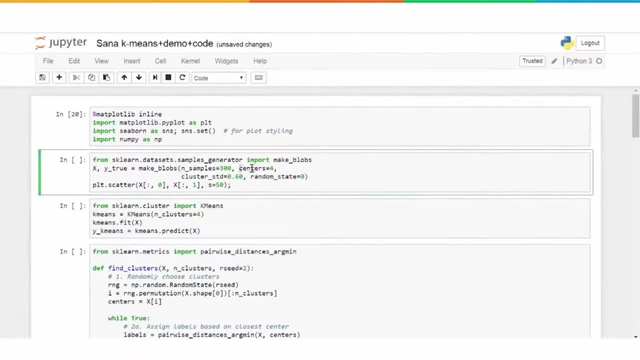 and we can specify how many clusters we want. So let's say we are going to make blobs and we can specify how many clusters we want to create. So we are going to make blobs and we can specify how many clusters we want to create. 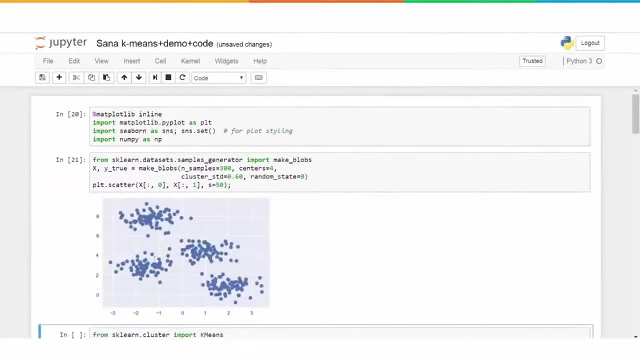 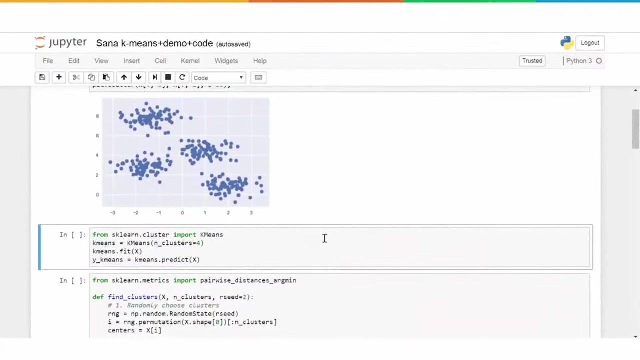 And this is how it looks. as you can see visually also, we can figure out that there are four distinct classes or clusters in this data set, And that is what make blobs actually provides. Now, from here onwards, we will basically run the standard k-means functionality. that is readily. 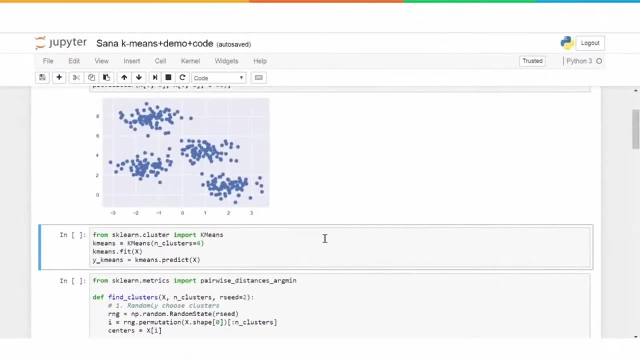 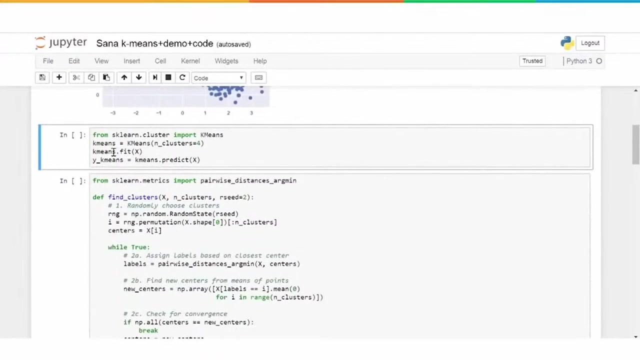 available. So we really don't have to implement k-means itself. the k-means functionality or the function is readily available. You just need to feed the data and we'll create the clusters. So this is the code for that: we import k-means and then we create an instance of k-means and we 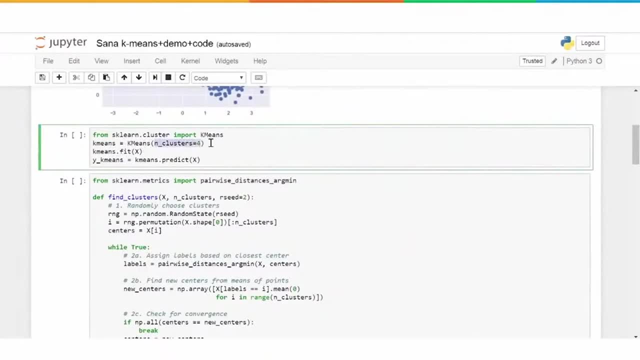 specify the value of k. this- n underscore clusters- is the value of k. Remember k-means. in k-means, k is basically the number of clusters that you want to create. So if I say I want to create a cluster to create and it is a integer value. so this is where we are specifying that. so we have k is. 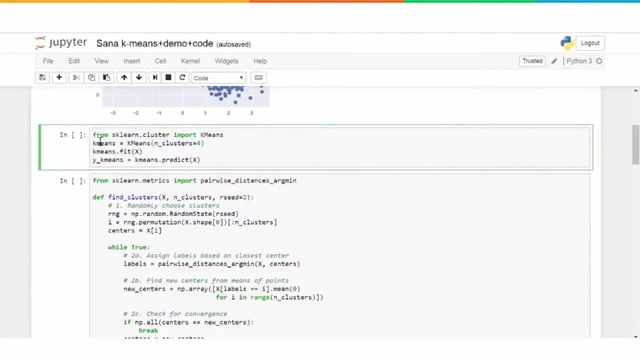 equal to 4, and so that instance is created. we take that instance and, as with any other machine learning functionality, fit is what we use, the function or, with the method, rather, fit is what we use to train the model. here there is no real training kind of thing, but that's the call, okay. 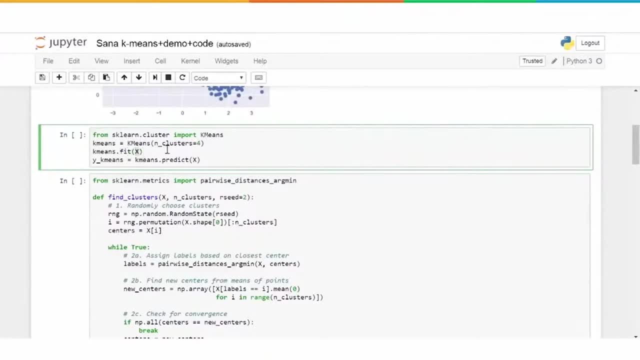 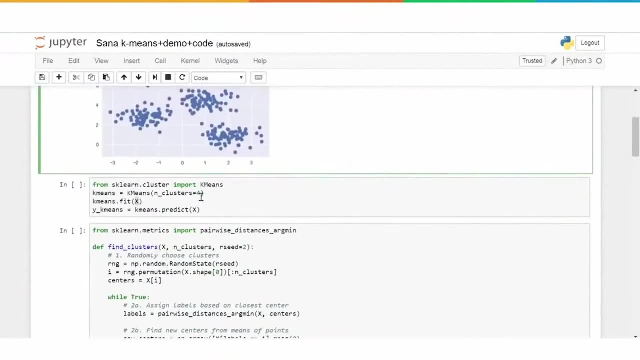 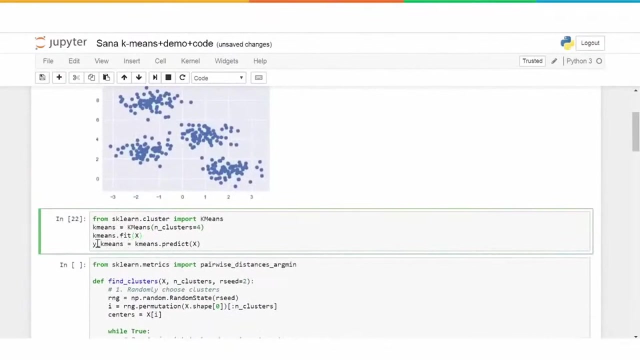 so we are calling fit and what we are doing here we are just passing the data, so x has these values, the data that has been created, right, so that is what we are passing here and this will go ahead and create the clusters and then we are using. 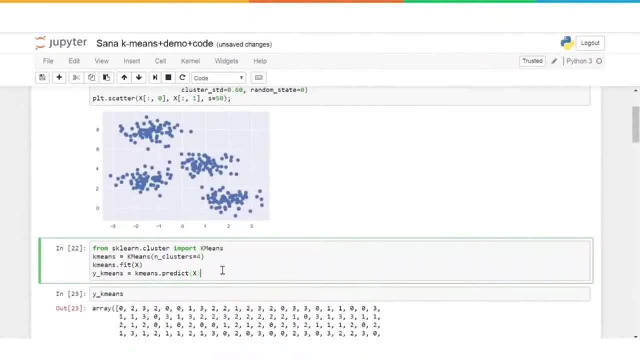 after doing fit, we run the predict, which basically assigns for each of these observations which cluster it belongs to. all right, so it will name the clusters. maybe this is cluster one, this is two, three and so on. or i will actually start from zero. cluster zero, one, two and three, maybe. 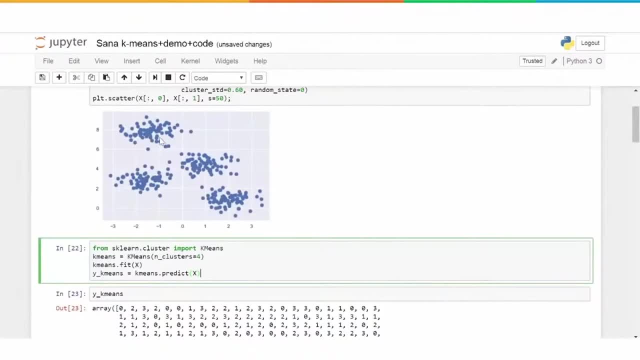 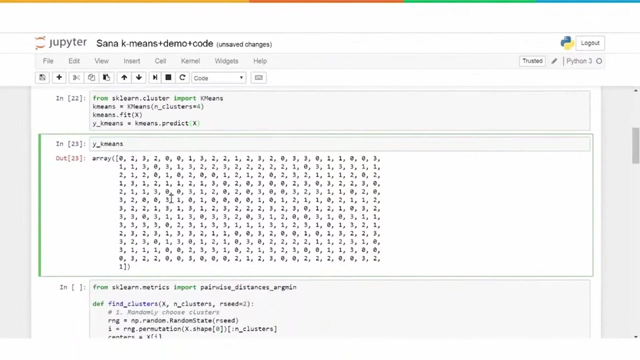 and then for each of the observations it will assign, based on which cluster it belongs to, it will assign a value. so that is stored in y underscore k means when we call, predict, that is what it does and we can take a quick look at these: uh y underscore k. 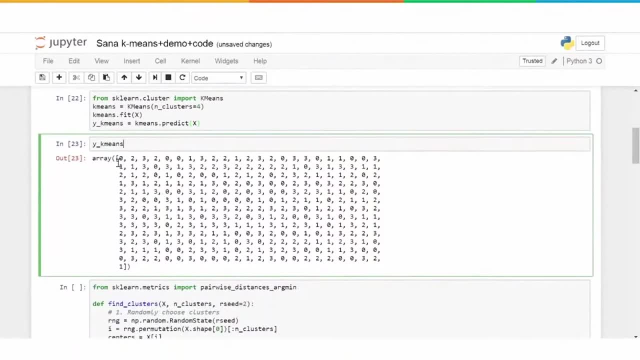 means all the cluster numbers that have been assigned for each observation. so this is the cluster number assigned for observation one. maybe this is for observation two, observation three and so on. so we have how many about? i think, 300 samples right. so all the 300 samples there. 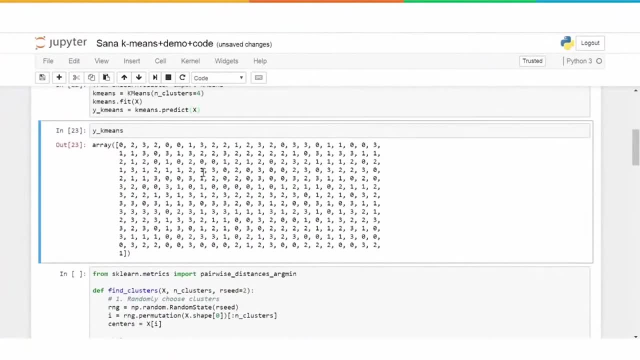 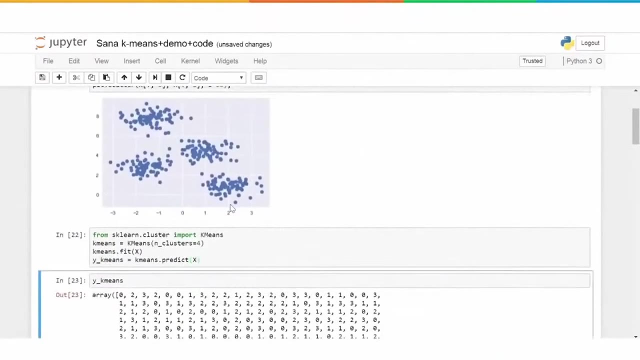 are 300 values here. each of them, the cluster number is given and the cluster number goes from zero to three. so there are four clusters, so the numbers go from zero, one, two, three. so that's seen here. okay now. so this was a quick example of generating some dummy data and then clustering. 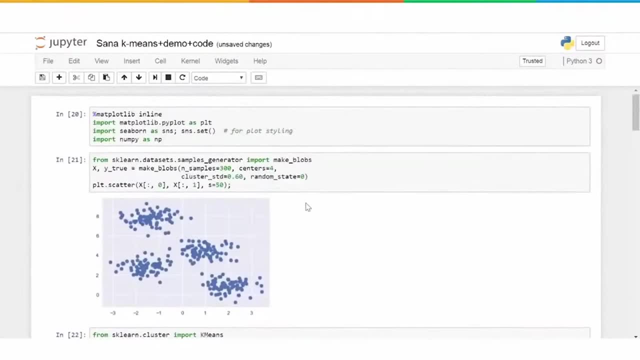 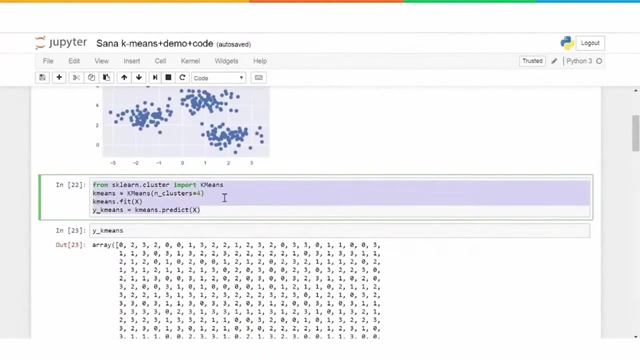 that okay and this can be applied. if you have proper data, you can just load it up into x, for example here, and then run the game. so this is the central part of the k means clustering program example. so you basically create an instance and you mention how many clusters you want by 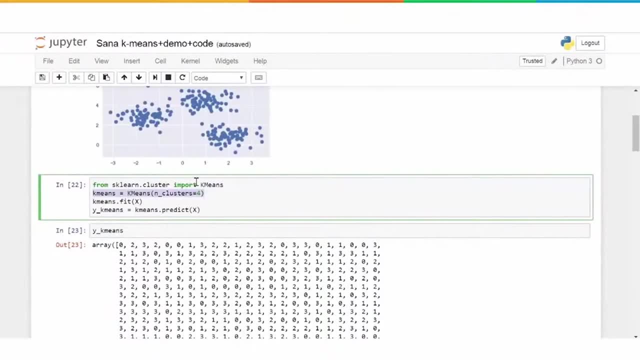 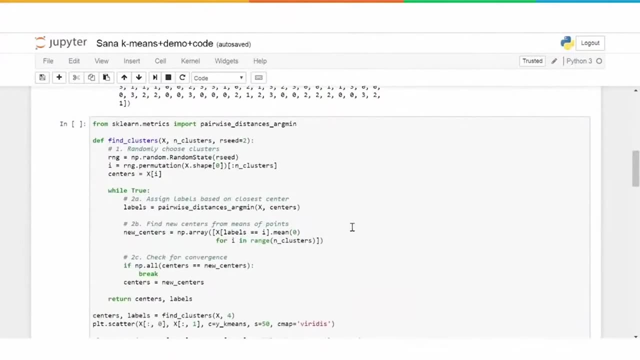 specifying this parameter and underscore clusters and that is also the value of k, and then pass it across the data to get the values. now the next section of this code is the implementation of a k-means. now this is kind of a rough implementation of the k-means algorithm. 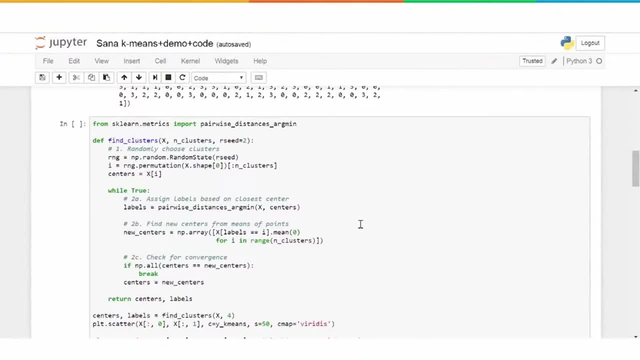 so we will just walk you through. i will walk you through the code at each step, what it is doing, and then we will see a couple of more examples of how k-means clustering can be used in. maybe some real life examples, real life use cases, all right, so in this case, 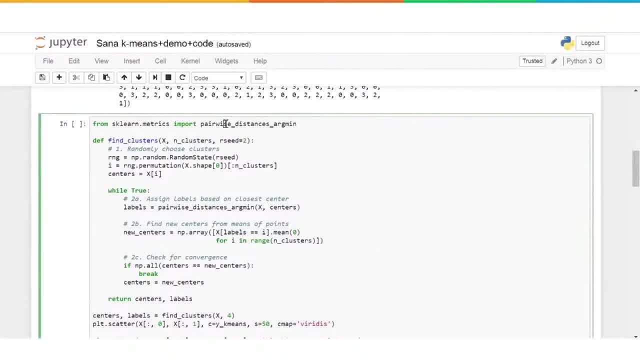 what we are doing is basically implementing the k-means clustering and there is a function for a library calculates for a given two pairs of points. it will calculate the, the distance between them and see which one is the closest, and so on. so this is like. this is pretty much like what. 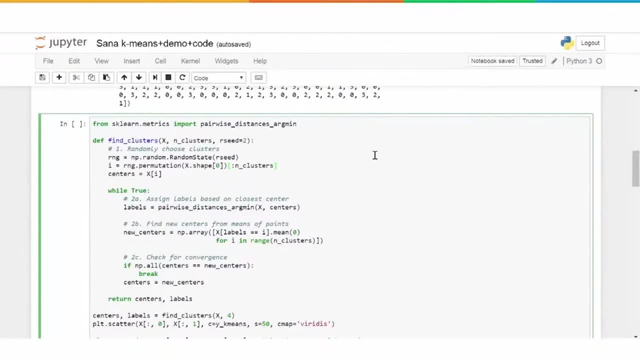 k-means does right. so it calculates the distance of each point or each data set from predefined centroid and then, based on whichever is the lowest data point, is assigned to that centroid. so that is basically available as a standard function and we will be using that here. so, as explained in the slides, the first step that is done in case of 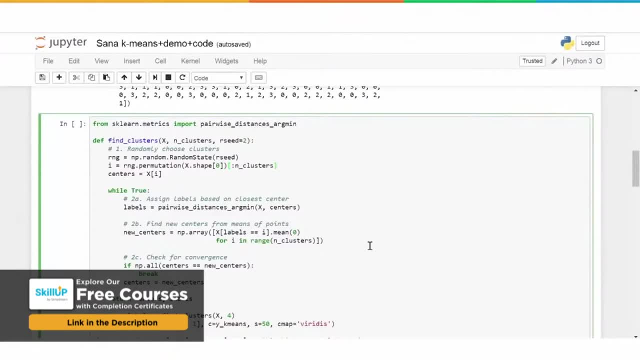 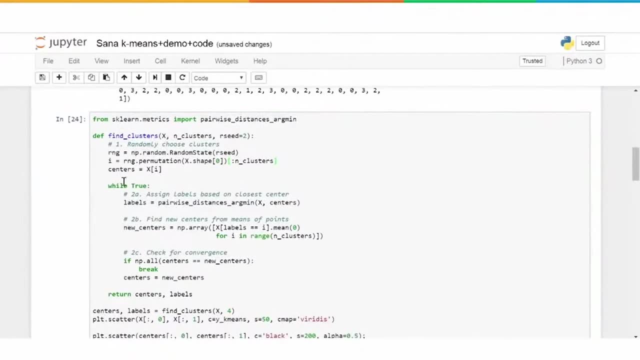 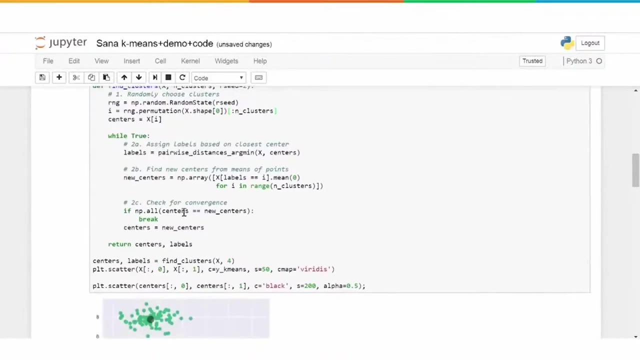 k-means. clustering is to randomly assign some centroids. so as a first step, we randomly allocate a couple of centroids which we call- here we are calling- as centers, and then we put this in a loop and take it through an iterative process for each of the data points we first find out using this: 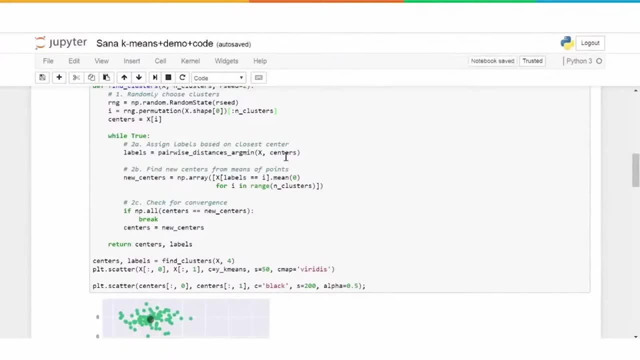 function pairwise distance argument. for each of the points, we find out which one- which center or which randomly selected centroid- is the closest and accordingly we assign that data on the data point to that particular centroid or cluster. and once that is done for all the data points, we 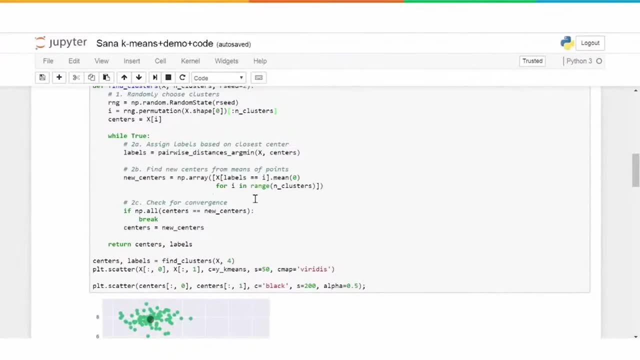 calculate the new centroid by finding out the mean position with the center position right. so we calculate the new centroid and then we check if the new centroid is the coordinates or the position is the same as the previous centroid. the positions we will compare and if it is the same, that means 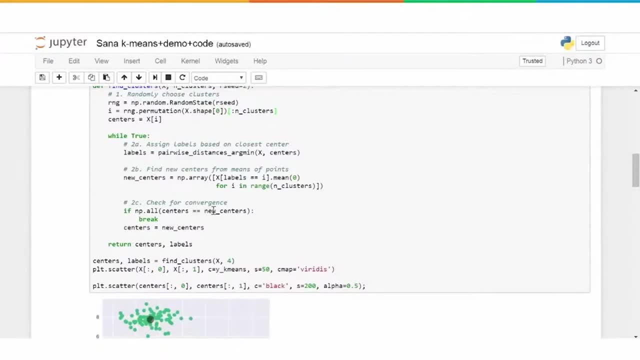 the process has converged. so remember, we do this process till these centroids or the centroid doesn't move anymore, right? so the centroid gets relocated each time this reallocation is done. so the moment it doesn't change anymore, the position of the centroid doesn't change anymore. we know that convergence has occurred. so till then. so you see here this is like an infinite. 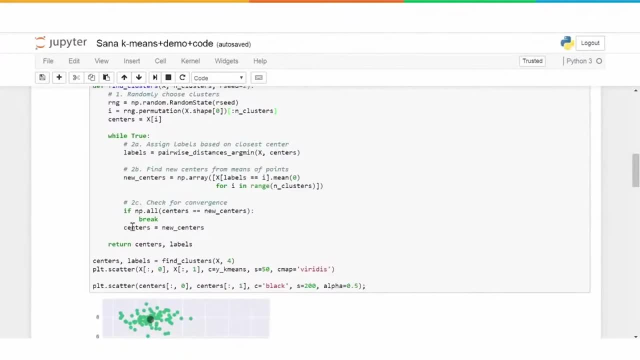 loop. while true is an infinite loop, it only breaks when the centers are the same, the new center and the old center positions are the same, and once that is done, we return the centers and the labels. now, of course, as explained, this is not a very sophisticated and advanced implementation. 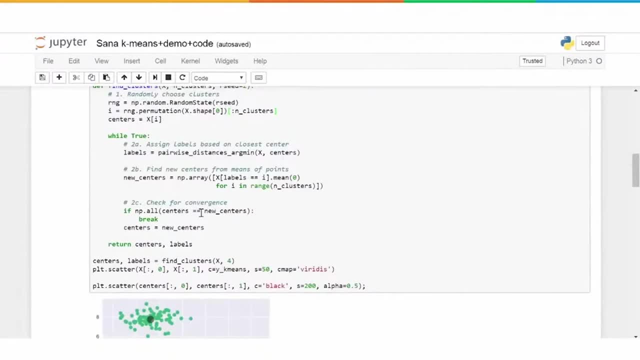 very basic implementation, because one of the flaws in this is that sometimes what happens is the centroid, the position, will keep moving, but in the change will be very minor. so in that case also with that is actually convergence right. so for example, the change is 0.0001. we can consider: 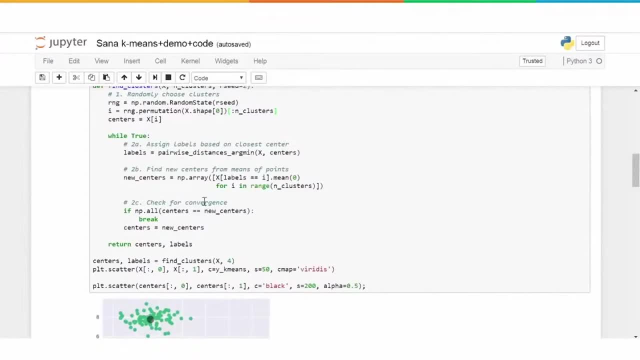 that as convergence. otherwise, what will happen is this will either take forever or it will be never ending. so that's a small flaw here. so that is something. additional checks may have to be added here. but again, as mentioned, this is not the most sophisticated implementation. this is like a kind of a rough implementation of the k-means clustering. okay, so if we execute this, 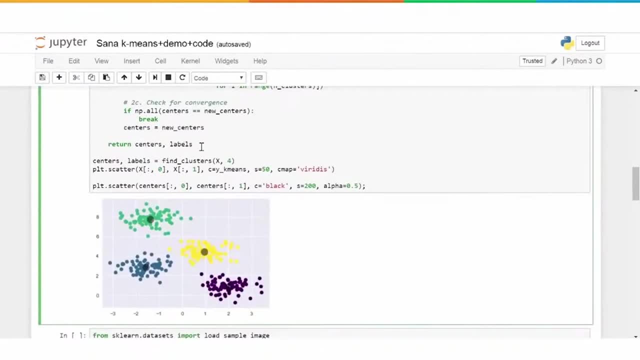 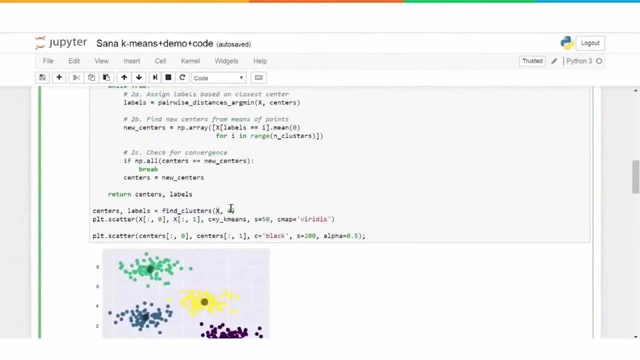 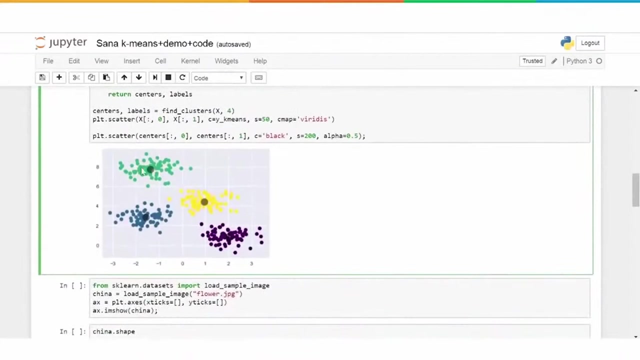 code. this is what we get as the output. so this is the definition of this particular function. and then we call that find underscore clusters and we pass our data, x, and the number of clusters, which is four, and if we run that and plot it, this is the output that we get. so this is, of course, each 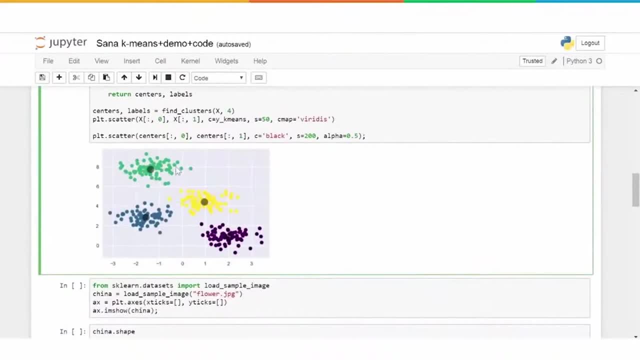 cluster is represented by a different color. so we have a cluster in green color, yellow color and so on and so forth, and these big points here, these are the centroids. this is the final position of the centroids and, as you can see, visually also, this appears like a kind of a center of all these. 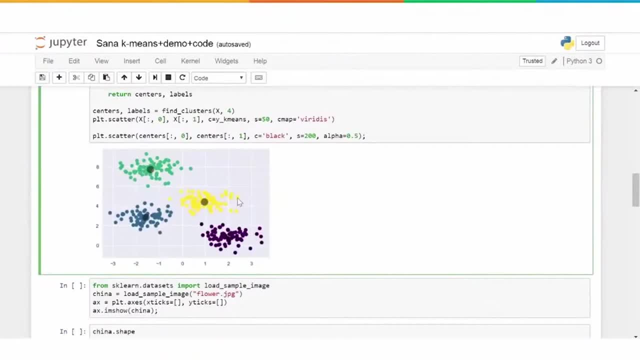 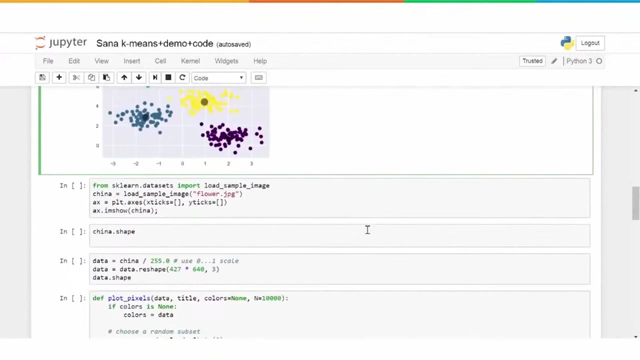 points here, right? similarly, this is like the center of all these points here, and so on. so this example, or this, is an example of a implementation of k-means clustering, and next we will move on to see a couple of examples of how k-means clustering is used in maybe some real-life scenarios or use. 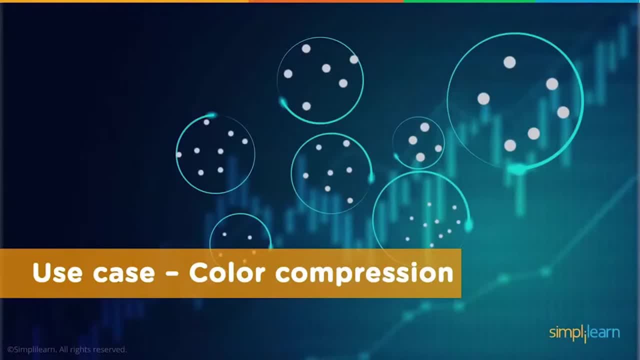 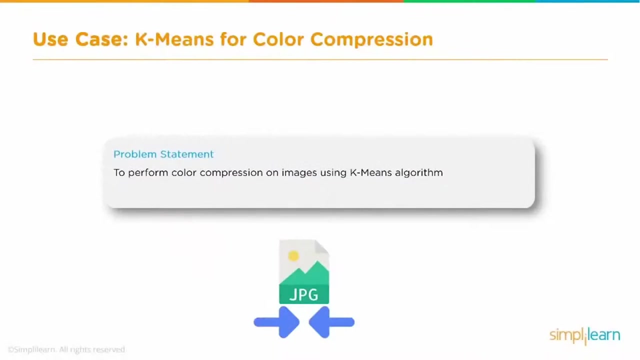 cases. in the next example or demo, we are going to see how we can use k-means clustering to perform color compression. we will take a couple of images, so there will be two examples and we will try to use k-means clustering to compress the colors. this is a common situation in image. 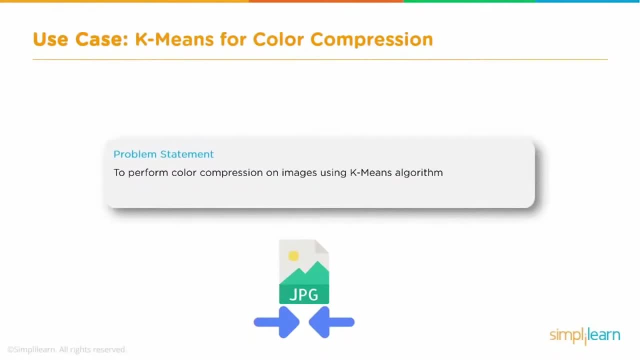 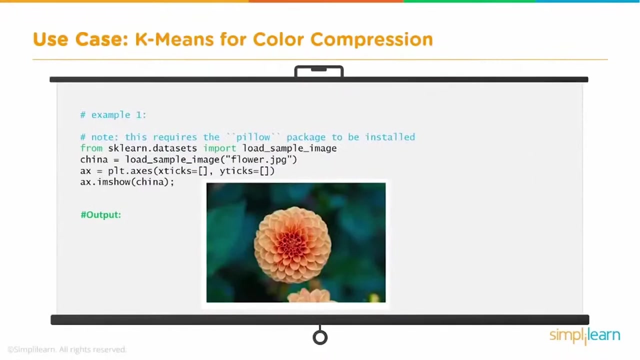 processing, when you have an image with millions of colors but then you cannot render it on some devices which may not have enough memory. so that is the scenario where where something like this can be used. so before again we go into the python notebook, let's take a look at quickly the the code. 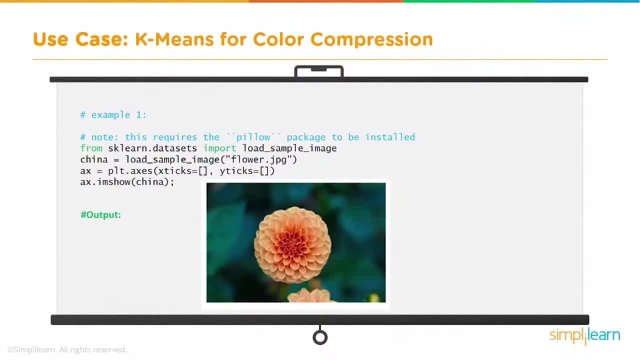 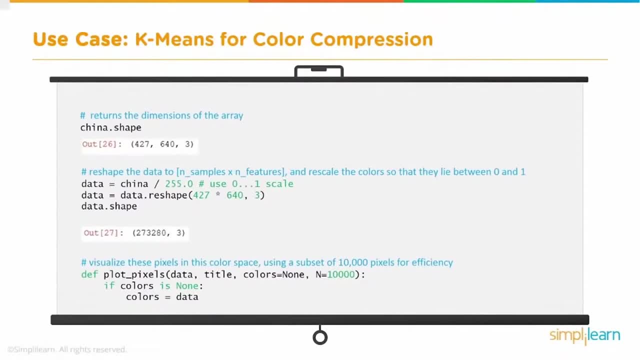 as usual, we import the libraries and then we import the image and then we will flatten it. so the reshaping is basically: we have the image, information is stored in the form of pixels and if the image is like, for example, 427 by 640, and it has three colors. so that's the overall. 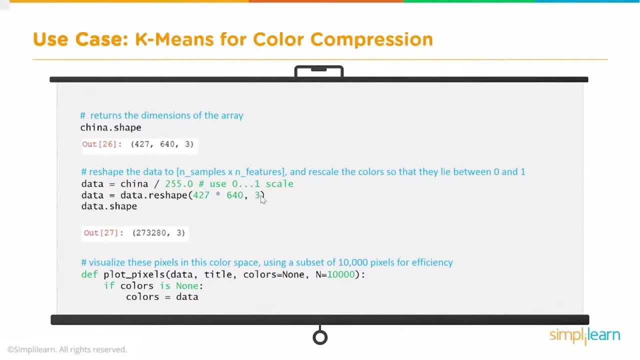 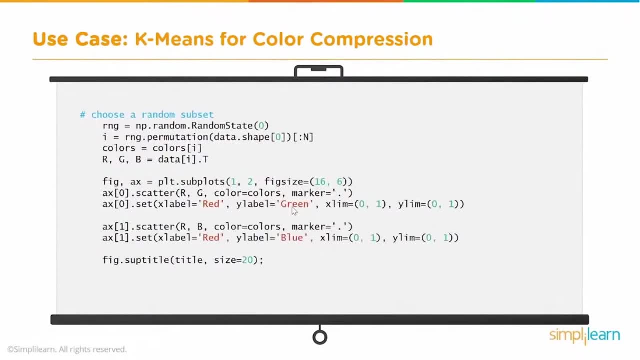 dimension of the of the initial image. we just reshape it and then feed this to our algorithm, and this will then create clusters of only 16 clusters. so this, this colors. there are millions of colors and now we need to bring it down to 16 colors, so we: 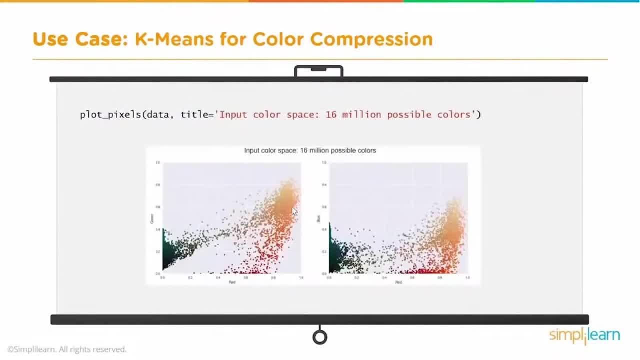 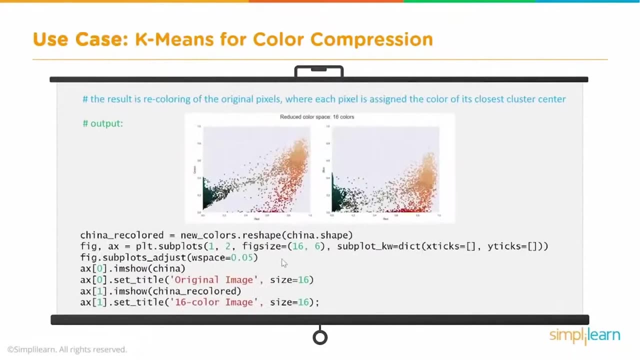 use k is equal to 16 and this is how, when we visualize, this is how it looks. there are- these are all about 16 million possible colors. the input color space has 16 million possible colors. so we just sub, compress it to 16 colors. so this is how it would look when we compress it to 16. 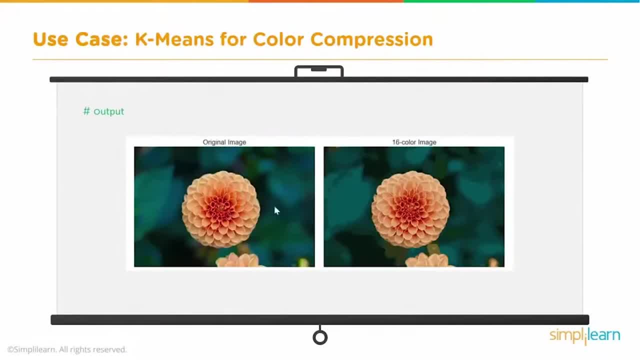 colors, and this is how the original image looks, and after compression to 16 colors, this is how the new image looks. as you can see, there is not a lot of information that has been lost, though the image quality is definitely reduced a little bit. so this is. 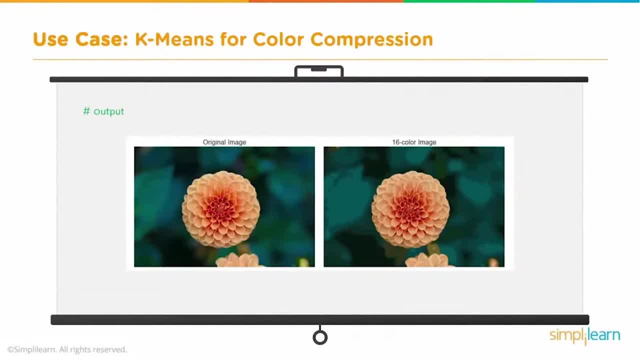 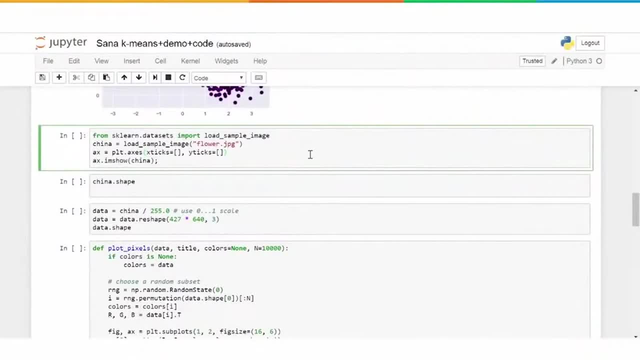 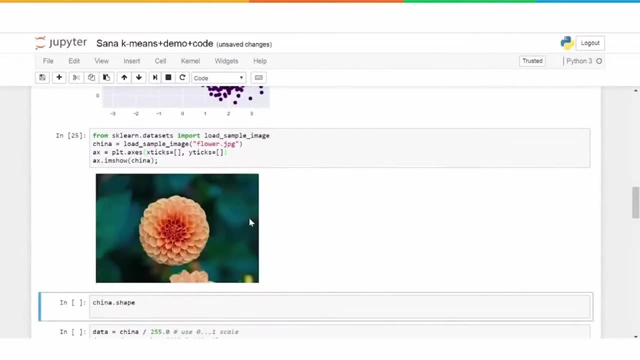 an example which we are going to now see in python notebook. let's go into the python and once again, as always, we will import some libraries and load this image called flowerjpg. okay, so let we load that and this is how it looks. this is the original image, which has, i think, 16 million colors and this: 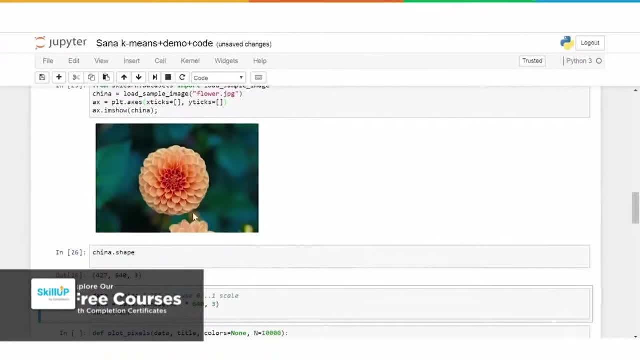 is the shape of this image, which is basically what is. the shape is nothing but the overall size, right? so this is 427 pixel by 640 pixel and then there are three layers, which is this. three basically is for rgb, which is red, green, blue, so color image will have that right. so that is the shape of this. 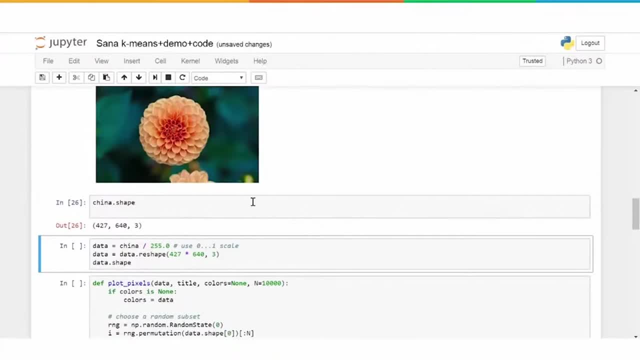 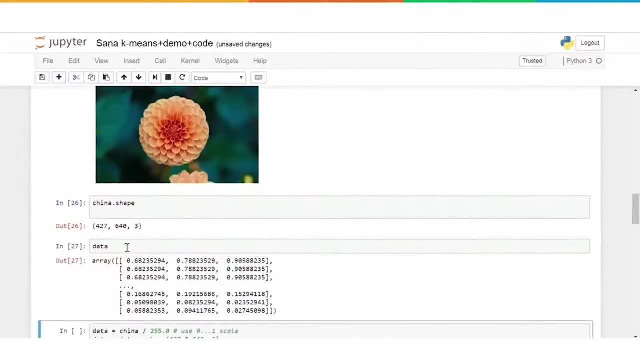 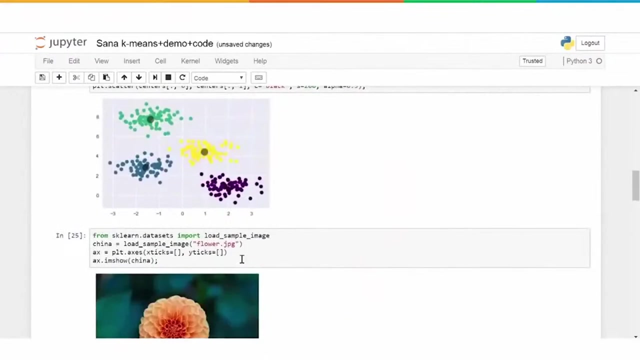 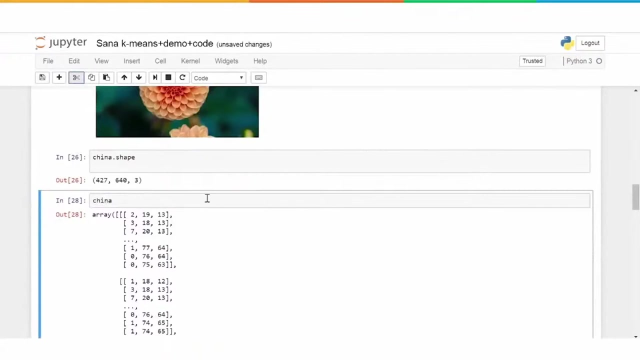 now what we need to do is data. let's take a look at how data is looking, so let me just create a new cell and show you what is in data. basically, we have captured this information, so data is what let me just show you here. all right, so let's take a look at china. what are the values in china? and if we see here, this is how. 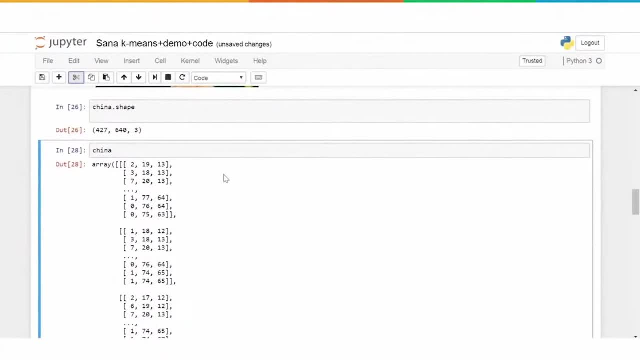 the data is stored. this is nothing but the pixel values. okay, so this is like a matrix, and each one has about for this, 427 by 640 pixels. all right, so this is how it looks. now, the issue here is: these values are large, the numbers are large, so we need to. 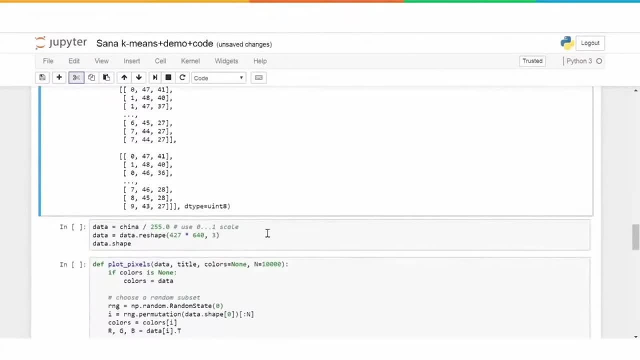 normalize them to between 0 and 1, right? so that's why we will basically create one more variable, which is data, which will contain the values between 0 and 1, and the way to do that is divide by 255. so we divide china by 255 and we get the new values in data. so let's just run this piece of. 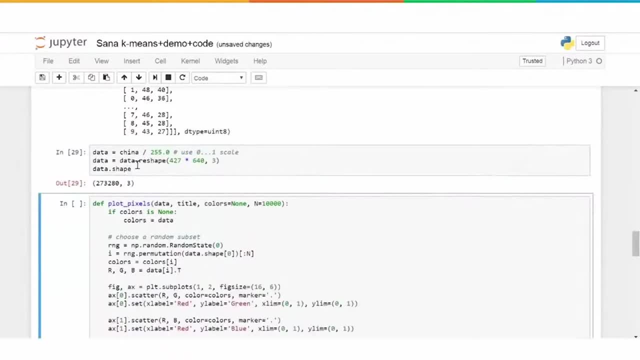 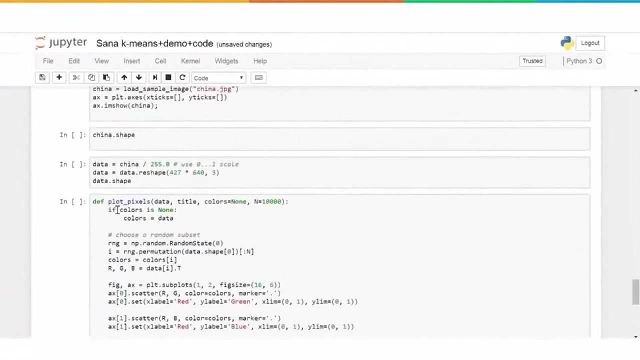 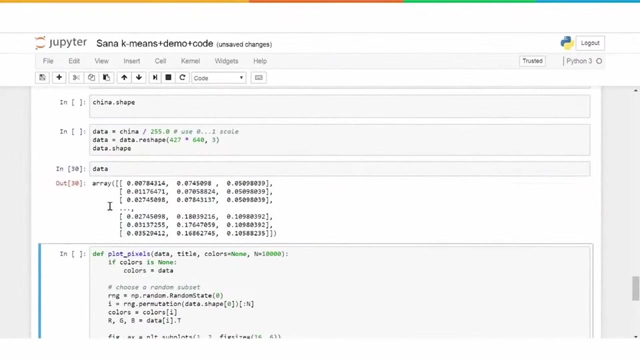 code and this is the shape. so we now have also. yeah, what we have done is we changed, using reshape, we converted into the three-dimensional, into a two-dimensional data set, and let us also take a look at how. let me just insert, probably, a cell here and take a look at how data is looking. all right. so this is how data is looking. 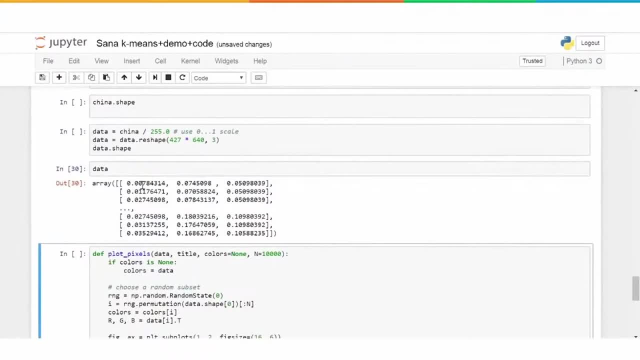 and now you see, this is: the values are between 0 and 1, right? so if you earlier noticed, in case of china, the values were large numbers. now everything is between 0 and 1. this is one of the things we need to do, all right? so after that, 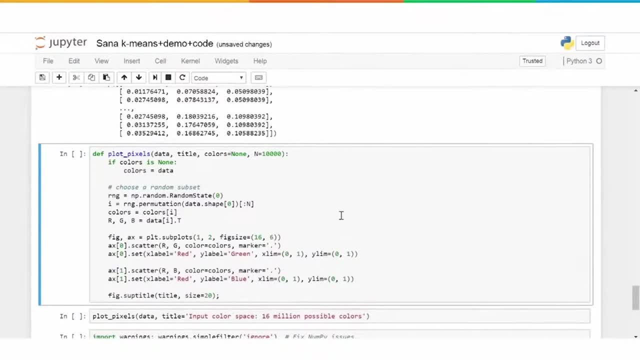 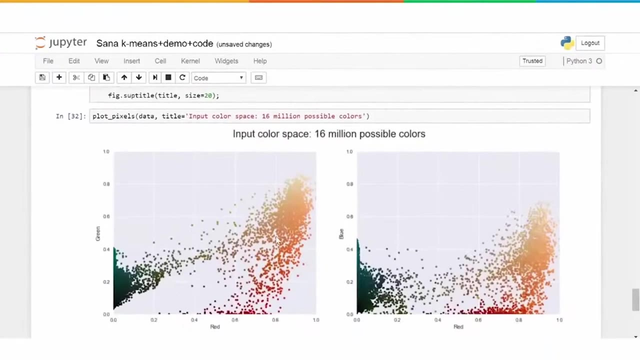 the next thing that we need to do is to visualize this, and we can take random set of maybe 10 000 points and plot it and check and see how this looks. so let us just plot this, and so this is how the original, the color, the pixel distribution is. these are two plots. one is red against green. 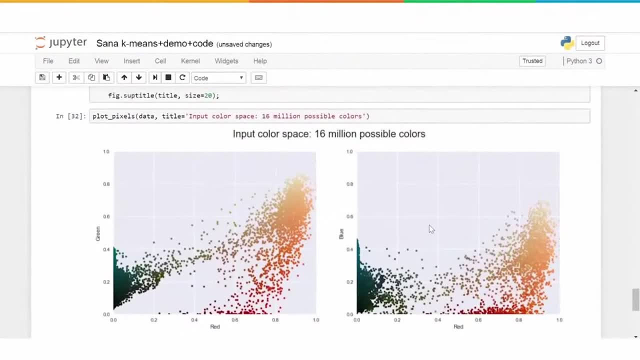 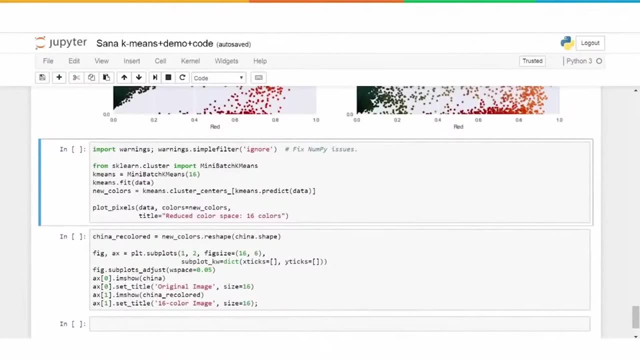 and another is red against blue, and this is the original distribution of the color. so, then, what we will do is we will use k-means clustering to create just 16 clusters for the various colors and then apply that to the image. now what will happen is, since the data is large, because there are millions of colors using 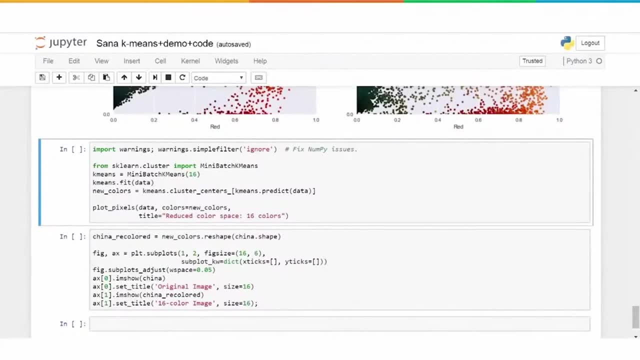 regular k-means may be a little time consuming, so there is another version of k-means which is called mini batch k-means, so we will use that, which is which processes in. the overall concept remains the same, but this basically processes it in smaller batches. that's the only thing, okay, so 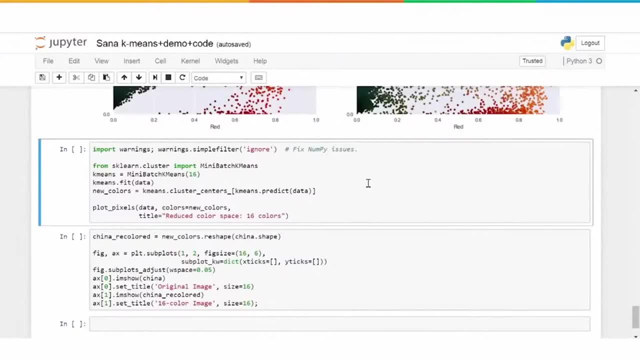 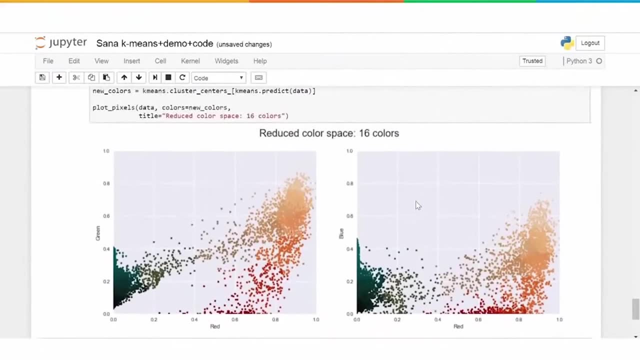 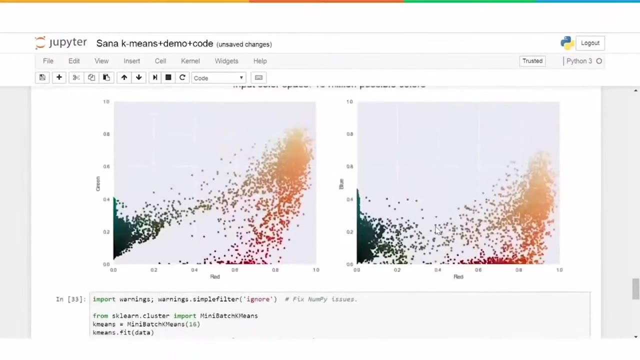 let's go ahead and execute this piece of code and also visualize this so that we can see that there are these. this is how the 16 colors, uh, would look. so this is red against green and this is red against blue. there is a quite a bit of similarity between this original color schema and the new one. 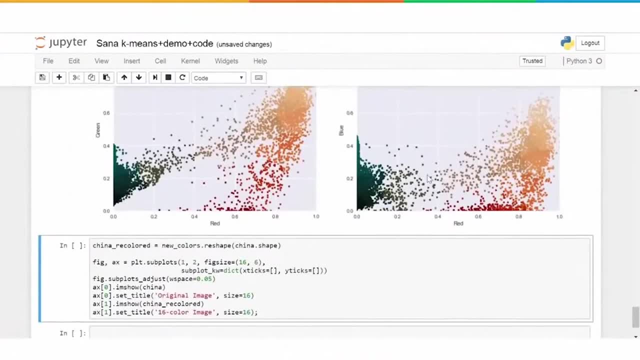 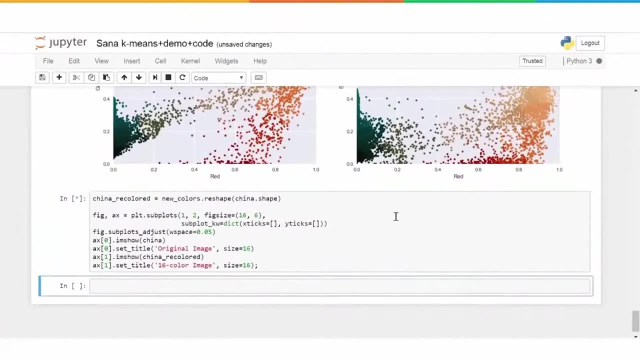 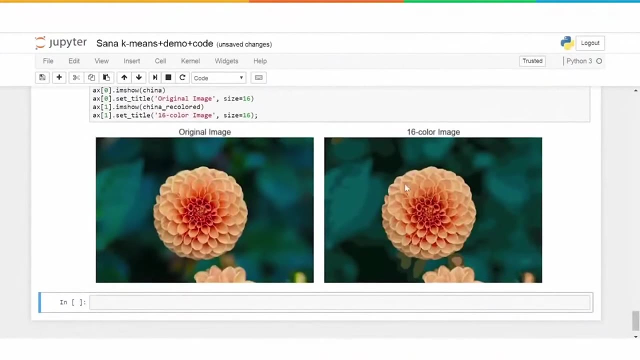 right, so it doesn't look very, very, completely different or anything like that. now we apply this to the image and we can take a look how this is looking. now we can compare both the images. so this is our original image and this is our new image. so, as you can see, there is not a lot of. 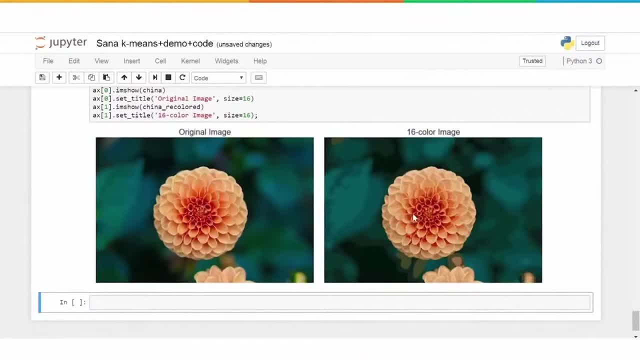 information that has been lost. it pretty much looks like the original image. yes, we can see that. for example, here there is a little bit- uh, it appears a little dullish compared to this one right, because we kind of took off some of the finer details of the color, but overall the high level information has been maintained at the same time, 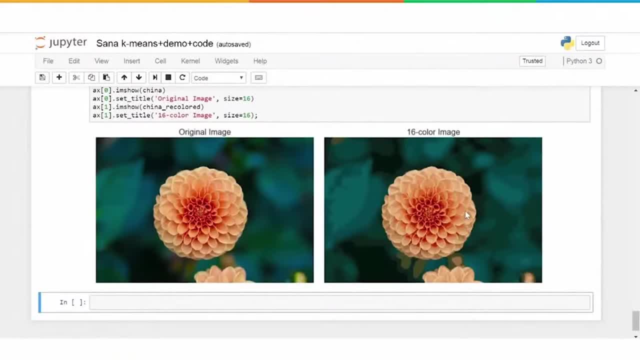 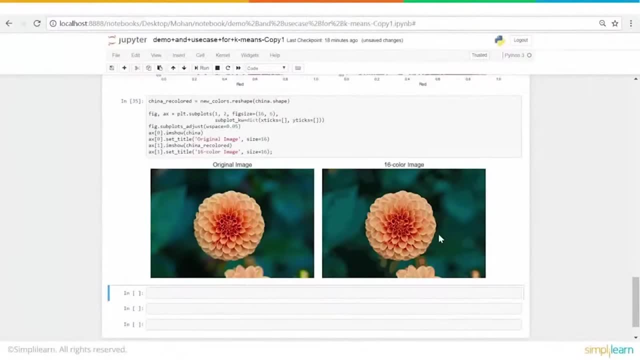 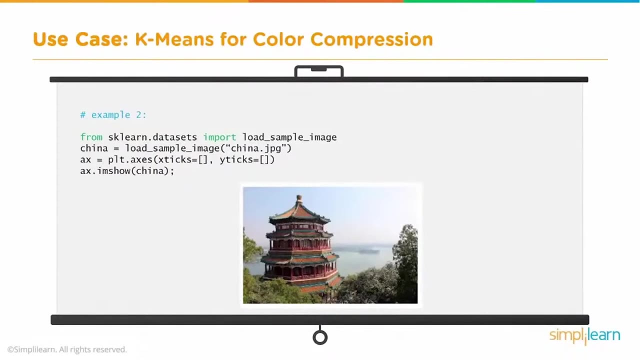 the main advantage is that now this can be. this is an image which can be rendered on a device which may not be that very sophisticated. now let's take one more example with a different image. in the second example, we will take an image of the summer palace in china and we repeat the same process. 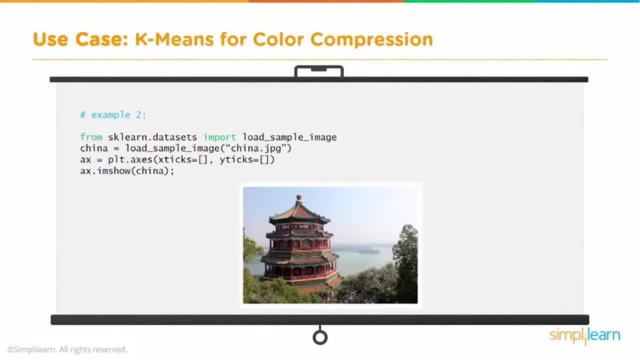 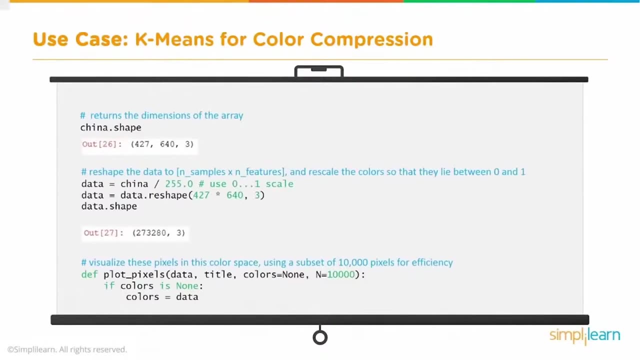 this is a high definition color image that also has different colors, such as black and white. a rich euh redish, we will have it. uh, a bunch of different colors would work in the same way. this image also has a huge anatomy, so, as you can see, the colors are very, very large. 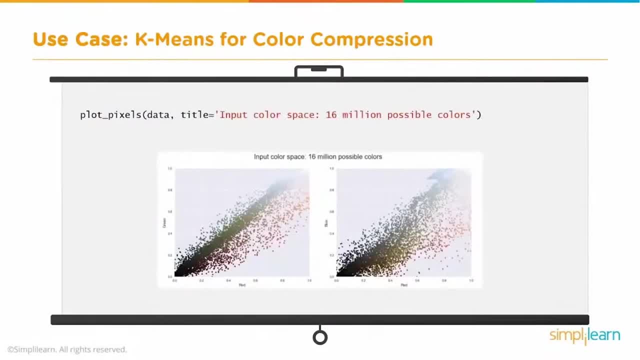 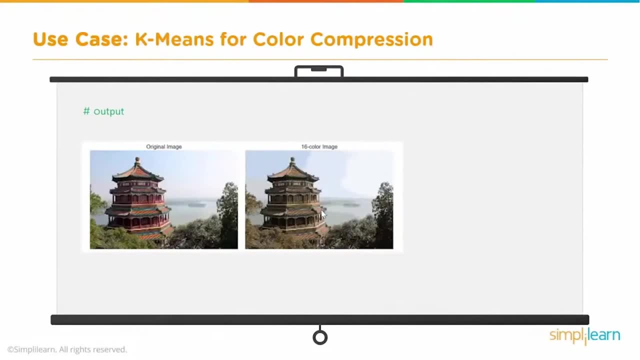 the image is very, very bright. mainly this image looked quite like with the large letters all color, and this image was made withtone. so if you move this city- Израël, i think- to the other side of this picture, um a little aggressive or details in this which are probably missing here. but then that's the compromise, because 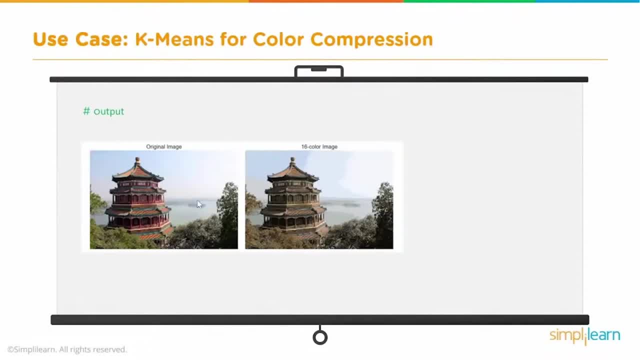 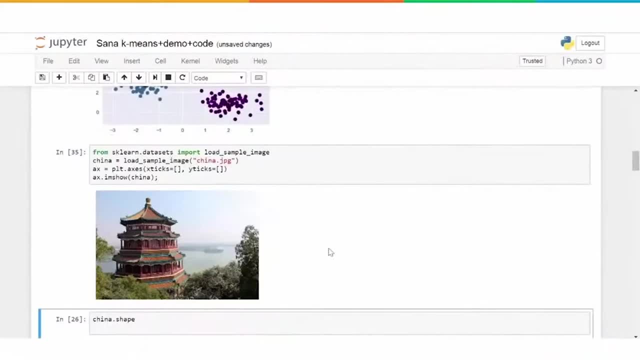 there are some devices which may not be able to handle this kind of high density images, so let's run this code in python notebook, all right. so let's apply the same technique for another picture which is even more intricate and has probably much complicated color schema. so this is the image now. 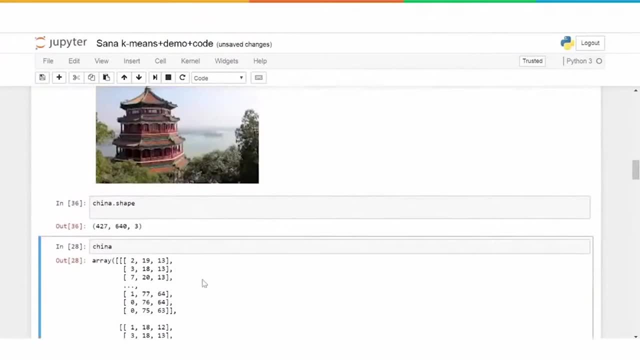 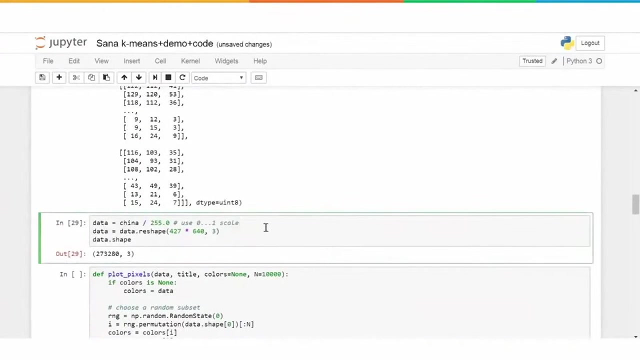 once again. we can take a look at the shape, which is 427 by 640 by 3, and this is the new data. would look somewhat like this compared to the flower image. so we have some new values here and we will also bring this. as you can see, the numbers are much big, so we will much bigger, so we will now. 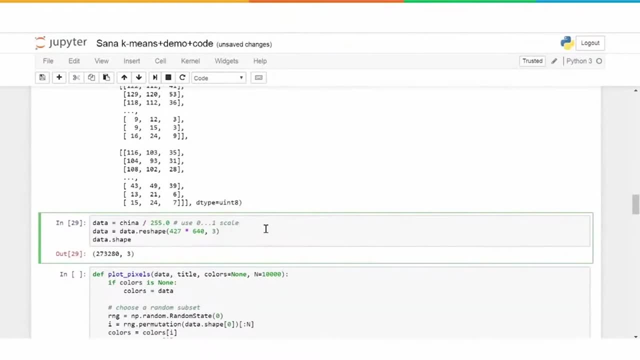 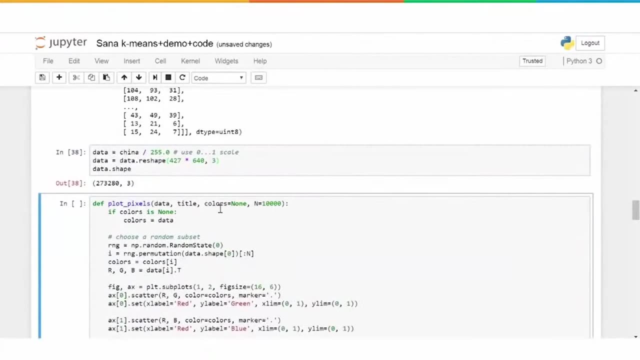 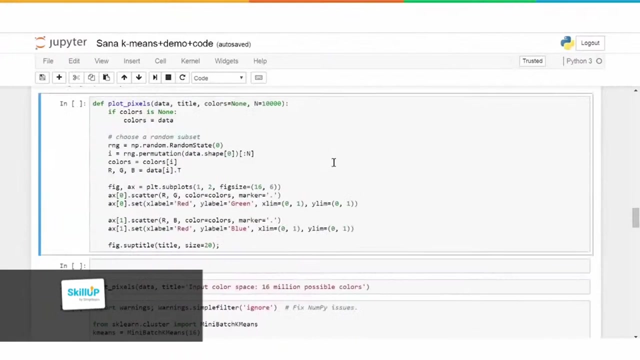 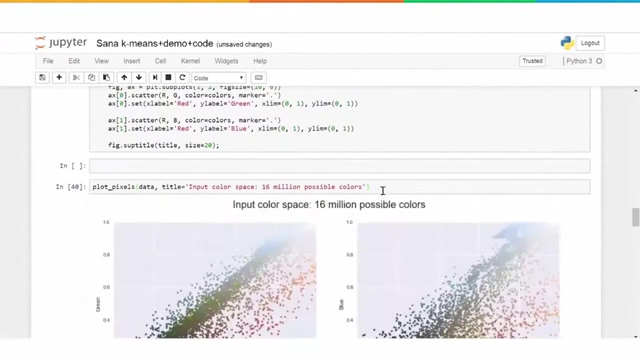 have to scale them down to values between 0 and 1, and that is done by dividing by 255. so let's go ahead and do that and reshape it. okay, so we get a two-dimensional matrix and we will then, as a next step, we will go ahead and visualize this how it looks: the 16 colors and this is. 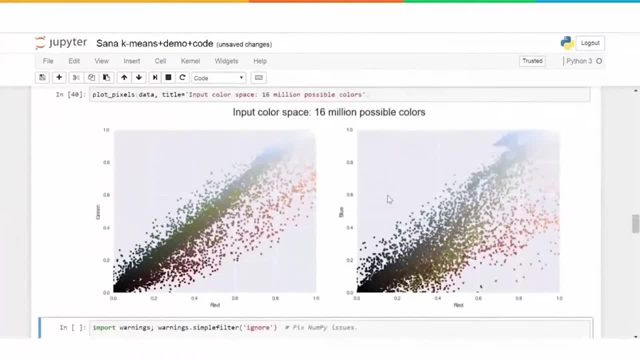 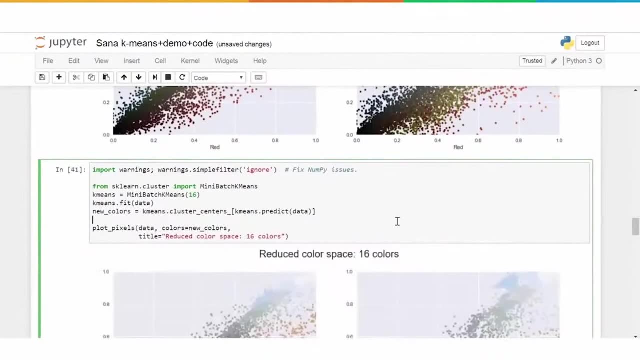 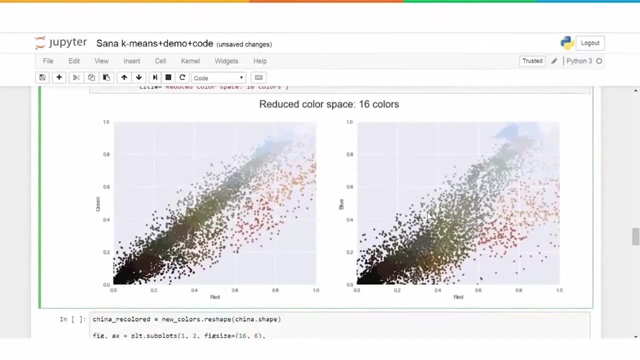 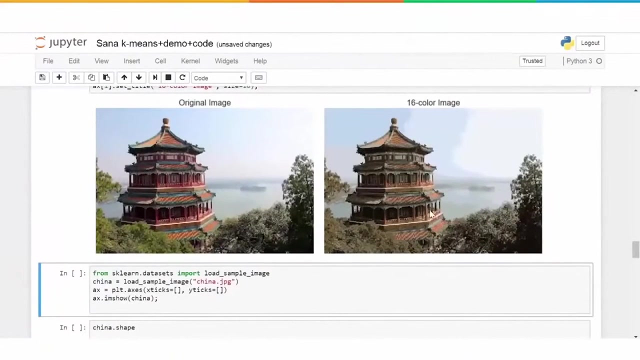 basically how it would look: 16 million colors, and now we can create the clusters out of this. the 16 k-means clusters we will create. so this is how the distribution of the pixels would look with 16 colors, and then we go ahead and apply this and visualize how it is looking for with the new, just the 16. 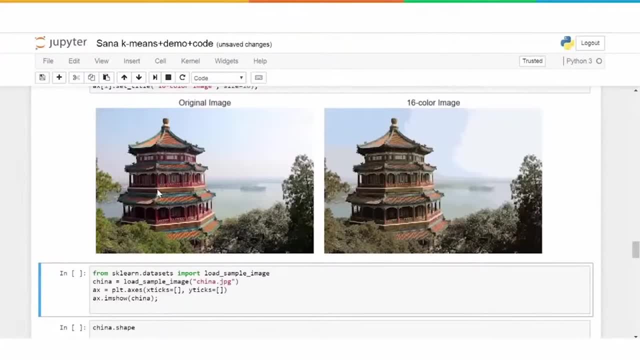 color. so, once again, as you can see, this looks much richer in color but at the same time- and this probably doesn't have, as we can see- it doesn't look as rich as this one, but nevertheless, the information is not lost. the shape and all that stuff, and this can be also rendered on a slightly a device, which 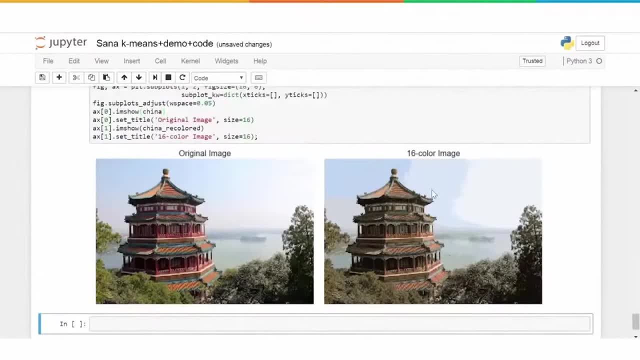 is probably not that sophisticated. okay, so that's pretty much it. so we have seen two examples of how color compression can be done using k-means clustering, and we have also seen, in the previous examples of how to implement k-means, the code to roughly how to implement k-means clustering, and we 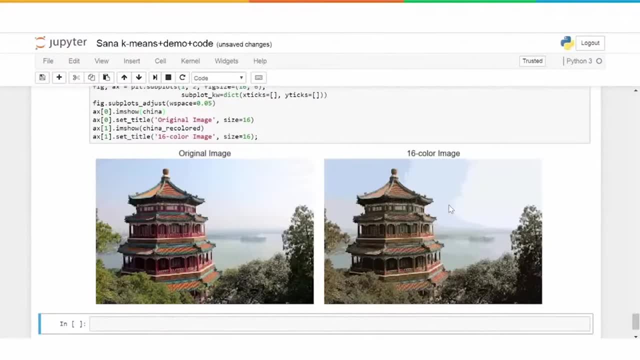 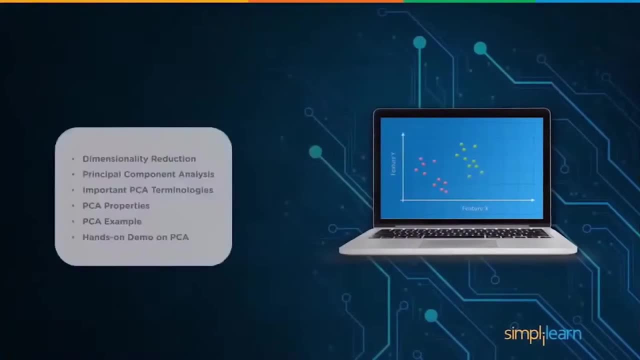 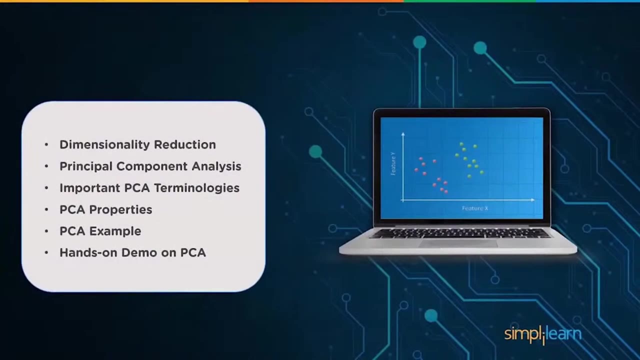 use some sample data using blob to just execute the k-means clustering. we talk about the principal component analysis. we're going to cover dimensionality reduction- principal component analysis. what is it important? pca terminologies, and you'll see it abbreviated normally as pca- principal component analysis, pca properties, pca example, and then we'll pull up some python code. 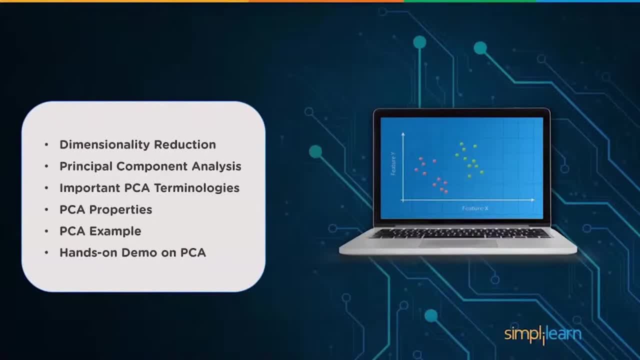 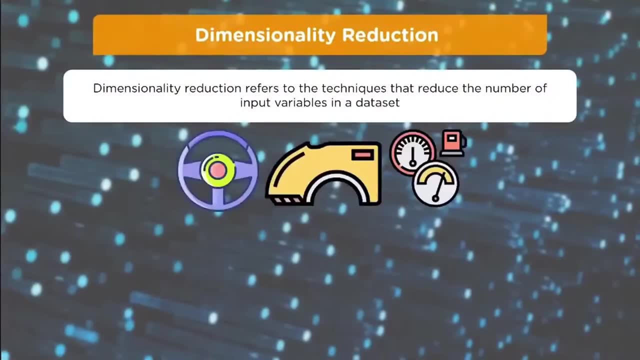 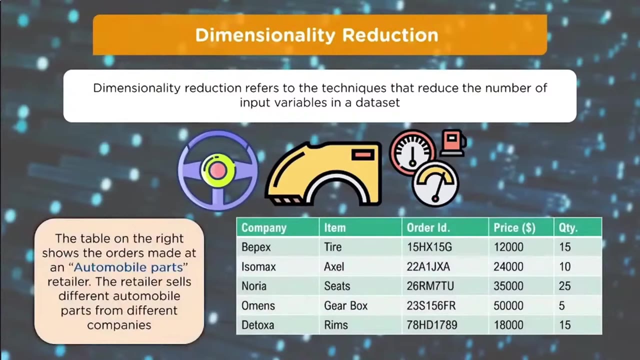 in our jupyter notebook, you and have some hands-on demo on the pca and how it's used. dimensionality reduction: dimensionality reduction refers to the technique that reduces the number of input variables in a data set, and so you can see on the table on the right shows the orders made at an automobile parts. 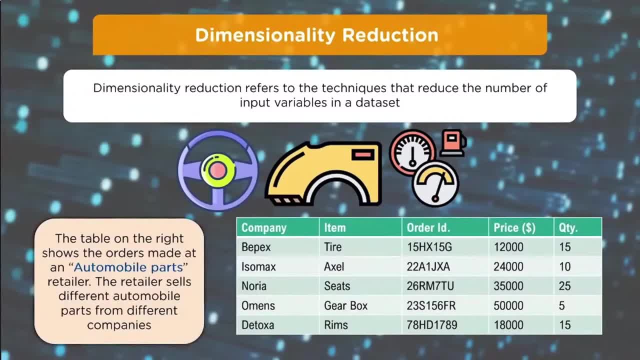 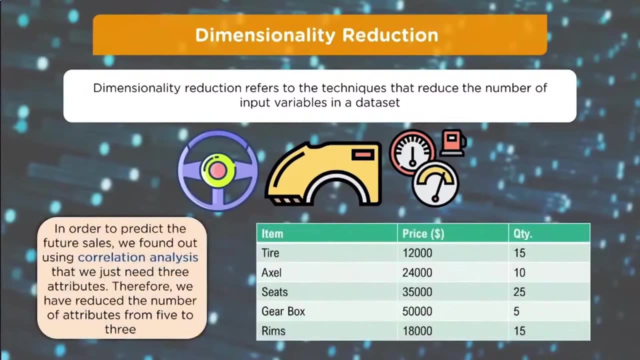 retailer. the retailer sells different automobile parts from different companies and you can see we have company bpacks, isomax, and they have the item, the tire, the axle, an order id, a price number and a quantity. in order to predict the future cells, we find out that using correlation. 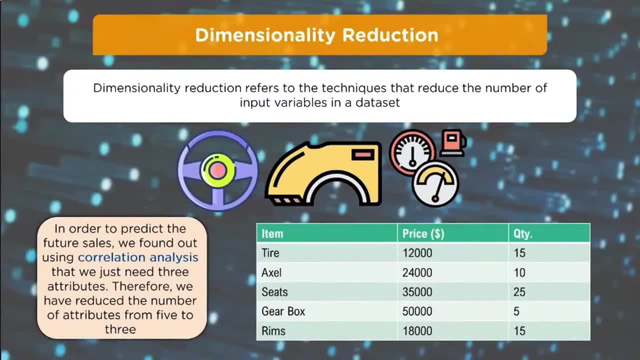 analysis that we just need three attributes. therefore, we have reduced the number of attributes from five to three and clearly we don't really care about the part number. i don't think the part number would have an effect on how many tires are bought and even the store who's buying them. 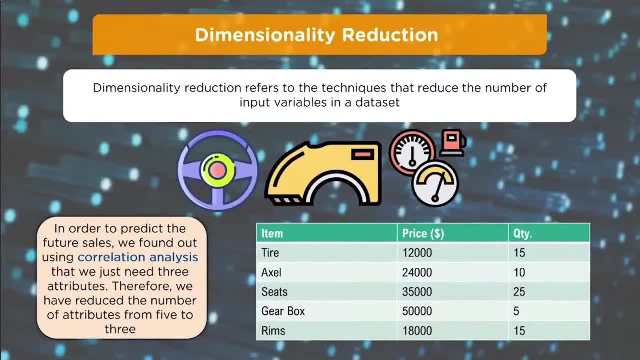 probably does not have an effect on that. in this case, that's what they've actually done is remove those and we just have the item, the tire, and we just need to get rid of those things that are, you know, tire, the price and the quantity. One of the things you should be taking away from this is in the scheme. 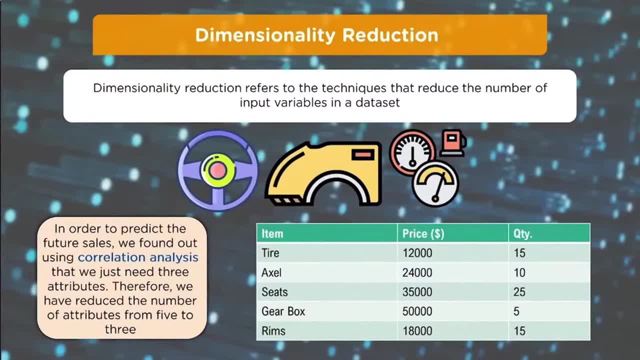 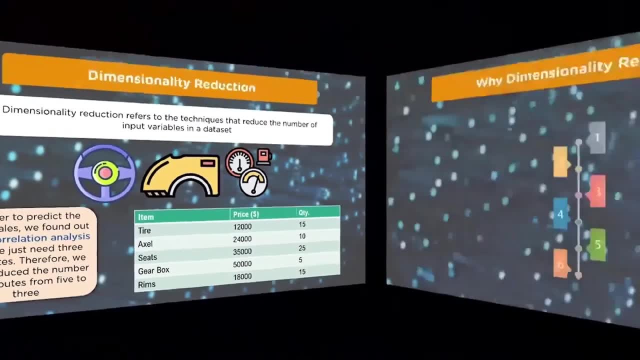 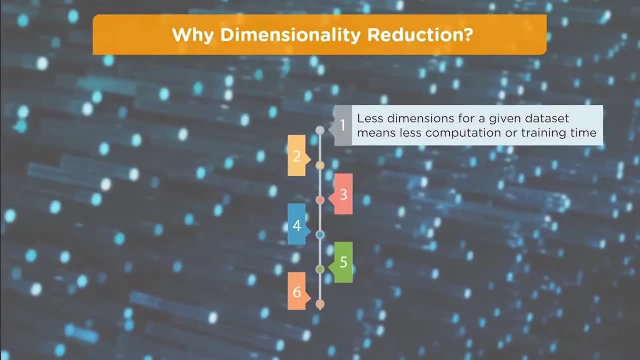 of things, we are in the descriptive phase. We're describing the data and we're pre-processing the data. What can we do to clean it up? Why dimensionality reduction? Well, number one: less dimensions for a given data set means less computation or training time. That can be really important if you're 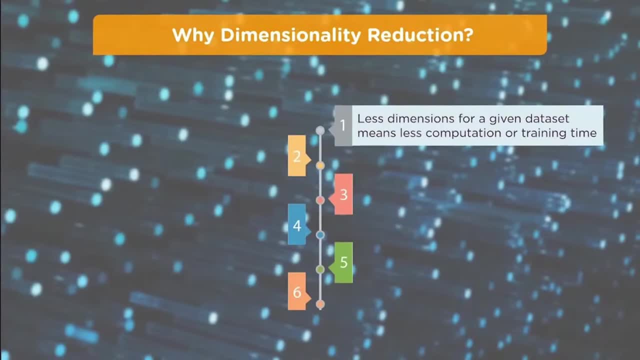 trying a number of different models and you're re-running them over and over again. And even if you have seven gigabytes of data, that can start taking days to go through all those different models. So this is huge. This is probably the hugest part as far as reducing our data set. 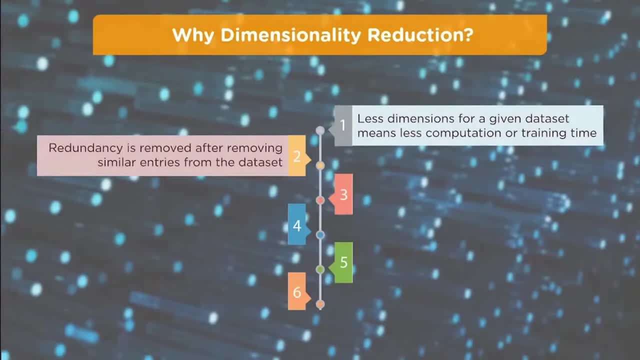 Redundancy is removed after removing similar entries from the data set, Again pre-processing some of our models. like a neural network, if you put in two of the same data it might give them a higher weight, And they would if it was just once. We want to get rid of that redundancy. 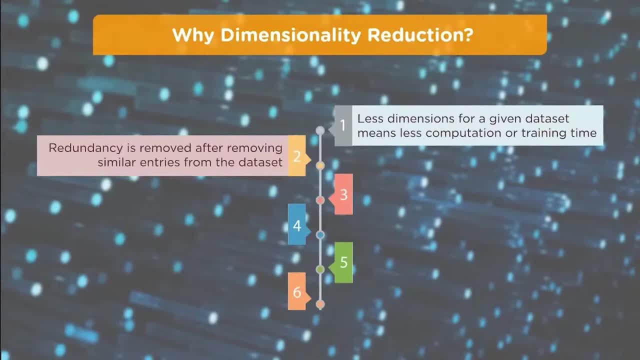 It also increases the processing time. if you have multiple data coming in, Space required to store the data is reduced. So if we're committing this into a big data pool, we might not send the company that bought it. Why would we want to store two whole extra columns when we add it into that pool? 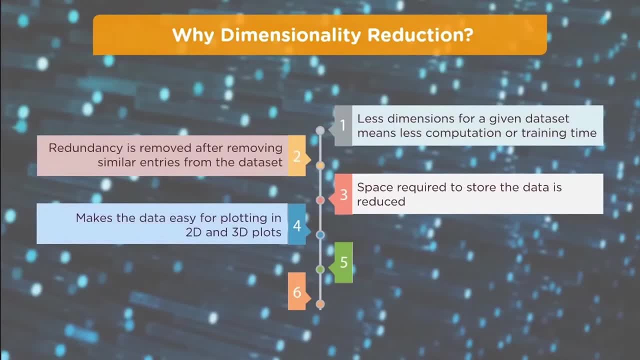 of data Makes the data easy for plotting in 2D and 3D plots. This is my favorite part, Very important. You're in your shareholder meeting. You want to be able to give them a really good, clear and simplified version. You want to reduce it down to something people can. 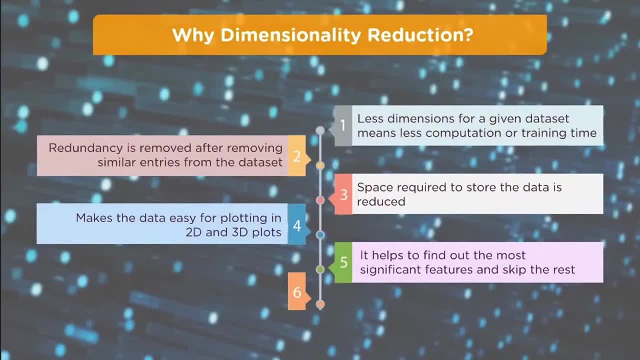 take in. It helps to find out the most significant features and skip the rest, which also comes in in postscribing. Leads to better human interpretation. That kind of goes with number four. what makes data easy for plotting, You have a better interpretation. 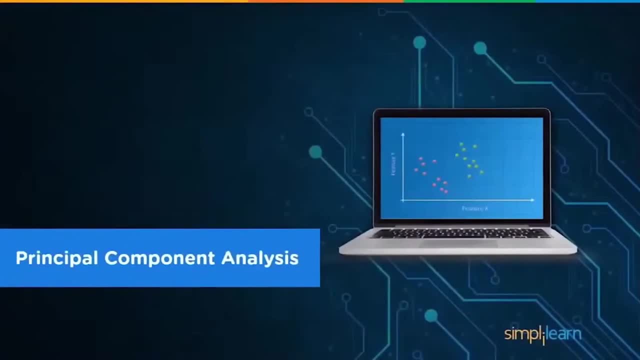 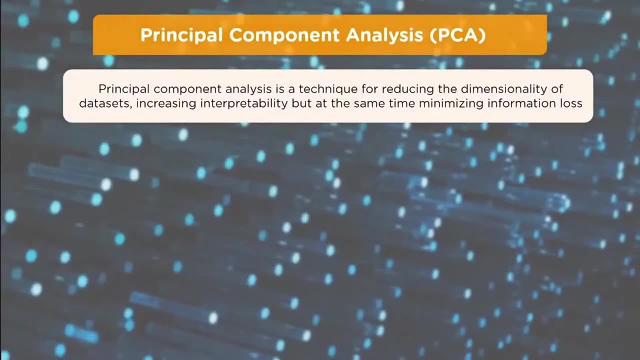 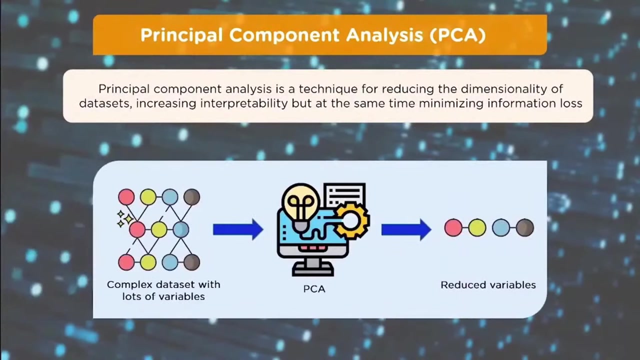 when we're looking at it, Principal component analysis. So what is it? Principal component analysis is a technique for reducing the dimensionality of data sets, increasing interpretability but at the same time minimizing information loss. So we take some very complex data set with lots of variables, We run it through the PCA, We reduce the variables, We 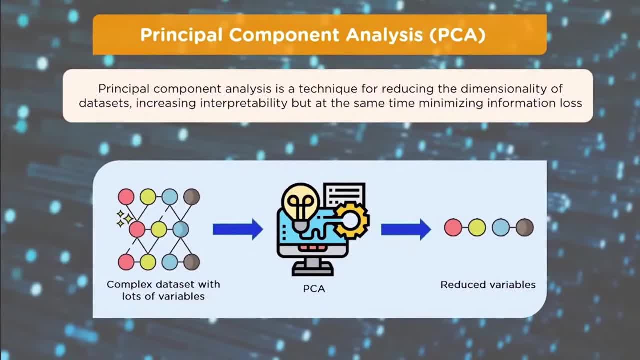 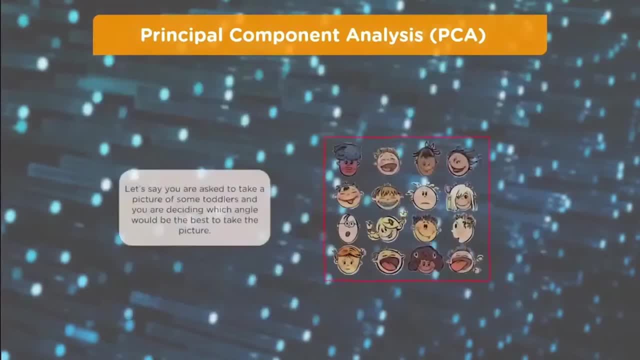 end up with a reduced variable setup. This is very confusing to look at because if you look at the end result, we have the different colors all lined up, So what we're going to take a look at is the same. We have a picture here. Let's say you are asked to take a picture of some toddlers and you 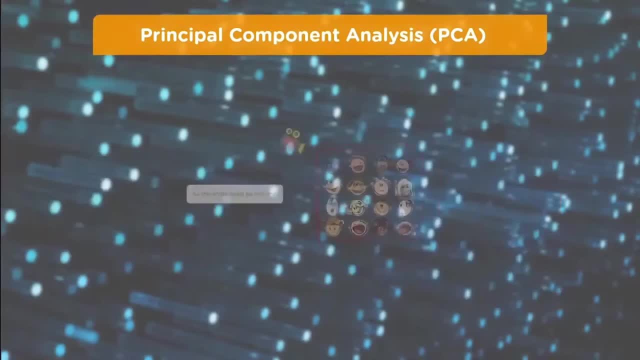 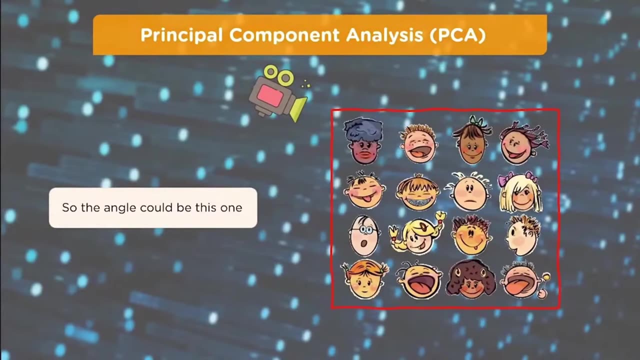 are deciding which angle would be the best to take the picture from. So if we come up here we look at this, We say, okay, this is one angle. We get the back of a lot of heads, not many faces, So we'll do it from here. We might get the one person up front smiling. A lot of the people in 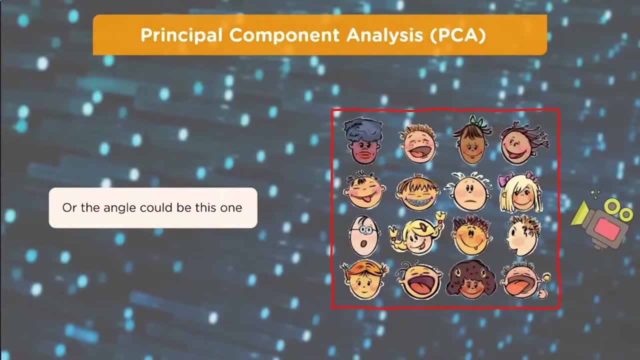 the class are missing, So we have a huge amount off to the right of blank space. Maybe from up here Again, we have the back of someone's head And it turns out that the best angle to click the picture from might be this bottom left angle. 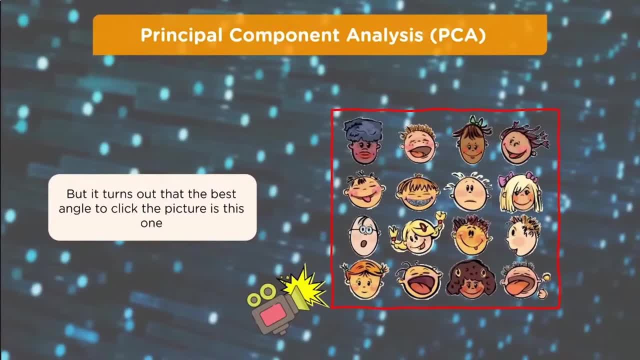 You look at it and you say, hey, that makes sense. It's a good configuration of all the people in the picture. Now, when we're talking about data, it's not. you really can't do it by what you think is. 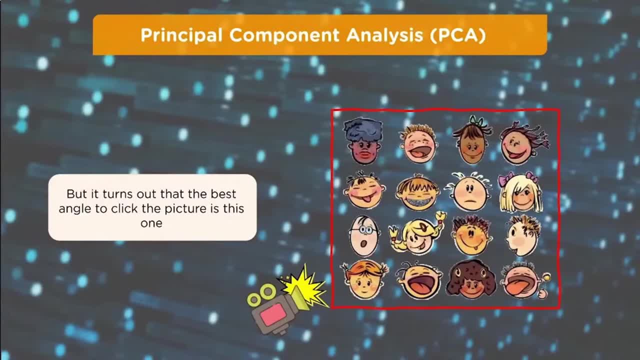 going to be the best. We need to have some kind of mathematical formula so it's consistent and so it makes sense in the back end. One of the projects I worked on many years ago has something similar to the iris. If you've ever done the iris data set, it's probably one of the most common ones out there. 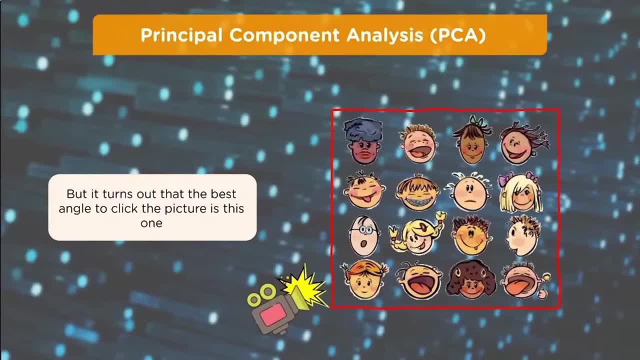 where they have the flower and they're measuring the stamen and the petals, and they have width and they have length of the petal. Instead of putting through the width and the length of the petal, we could just as easily do the width to length ratio. We can divide the width by the length and 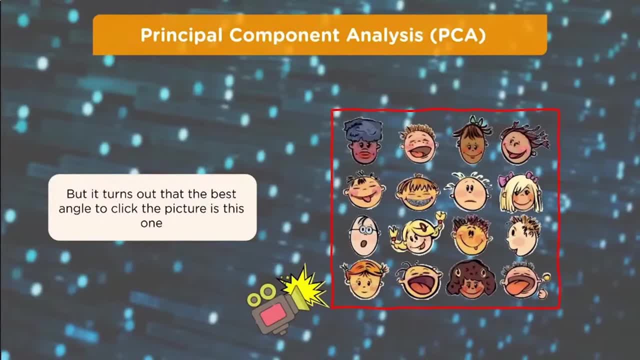 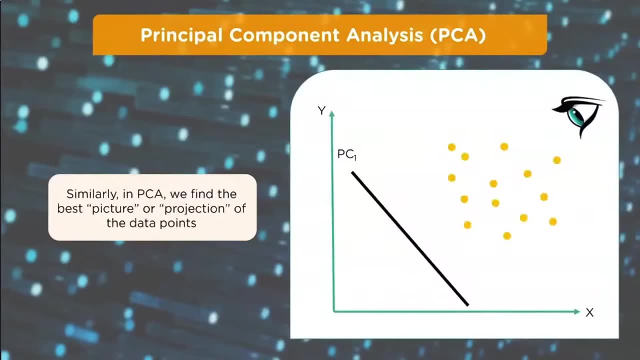 you get a single number where you had two. That's the kind of idea that's going on into this in pre-processing and looking at what we do, We can do to bring the data down. A very simplified example on my iris petal example: When we look at the 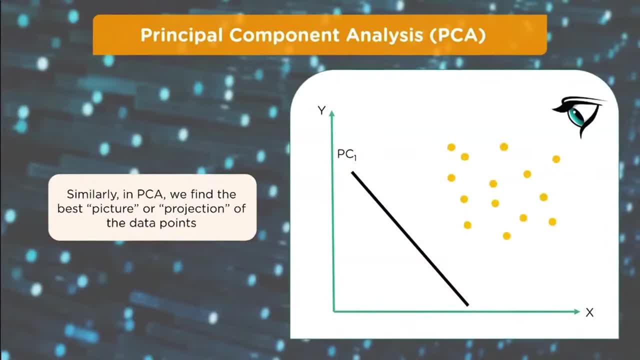 similarity. in PCA we find the best picture or projection of the data points, And so when we look down at from one angle- we've drawn a line down there- we can see these data points based on, in this case, just two variables. Now, keep in mind we're usually talking about 36,, 40 variables, Almost all of your. 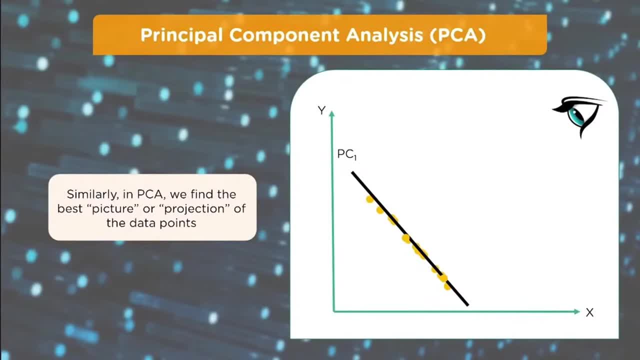 business models usually have about 26 to 27 different variables. they're looking at Same thing with, like, a bank loan model. We're talking, 26 to 36 different variables. they're looking at that are going in. So what we want to do is we want to find the best view. In this case, we're just looking at. 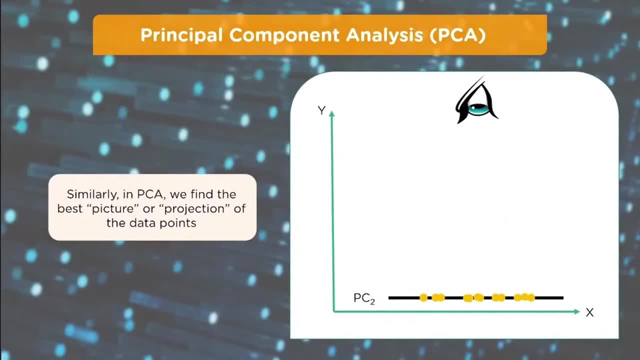 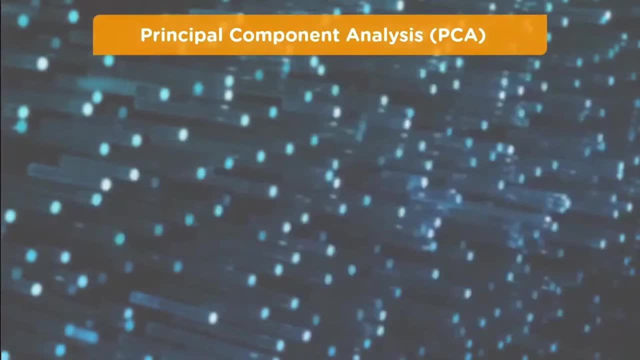 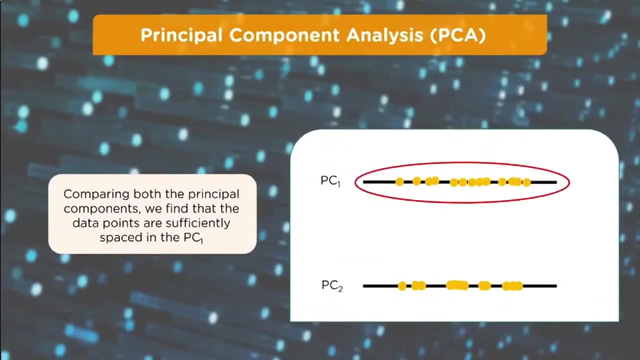 the XY. We look down at it and we have our second idea, PC2.. And again we're looking at the XY, this time from a different direction. Here, for our ease, we consider that we get two principal components, namely PC1 and PC2.. Comparing both the principal, 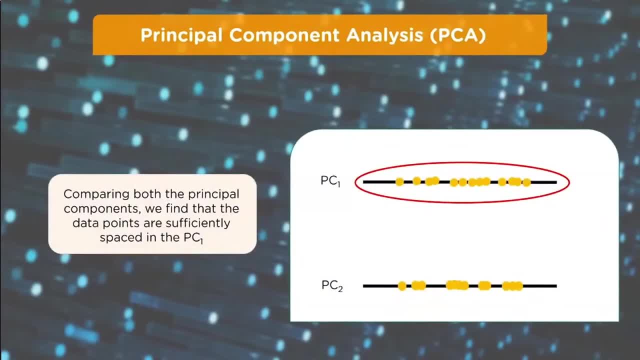 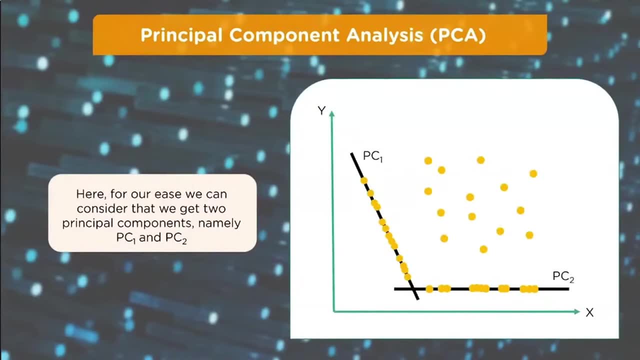 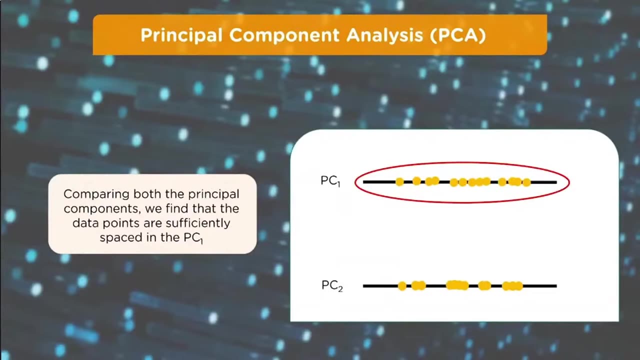 components, we find the data points are sufficiently spaced in PC1.. So if you look at what we got here, we have PC1. You can see along the line how the data points are spaced versus the spacing in PC2.. And that's what they're coming up with. What is going to give us the best look for these data points? 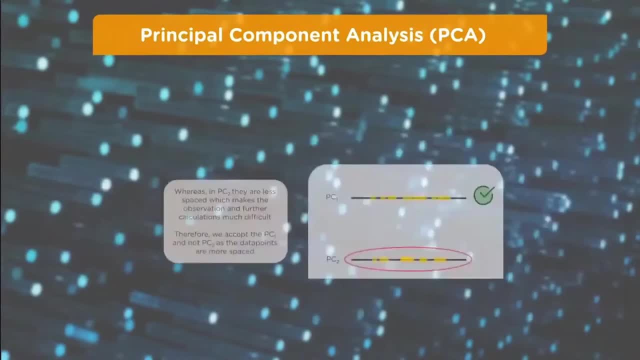 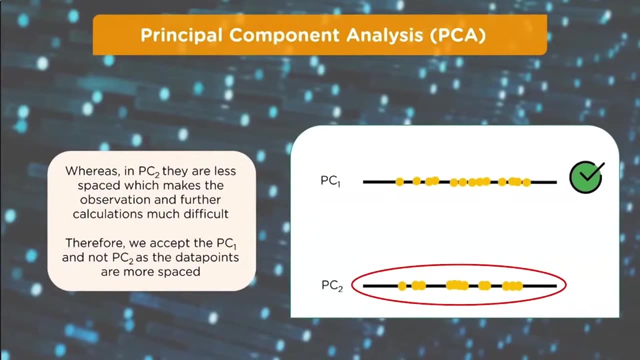 when we combine them And we're looking at them from just a single angle, Whereas in PC2, they are less spaced, which makes the observation and further calculations much more difficult. Therefore, we accept the PC1 and not the PC2, as the data points are more spaced. 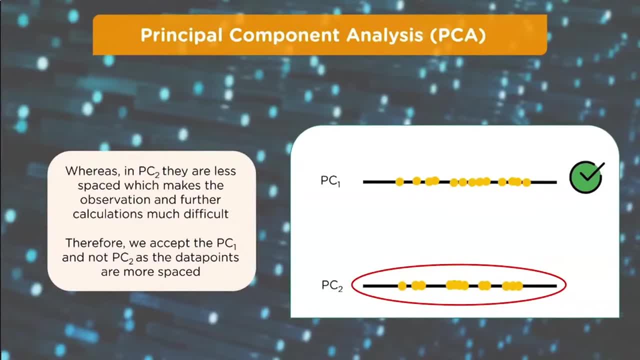 Now, obviously, the back end calculations are a little bit more complicated when we get into the math of how they decide what is more valuable. This gives you an idea, though, that when we're talking about this, we're talking about the perspective. 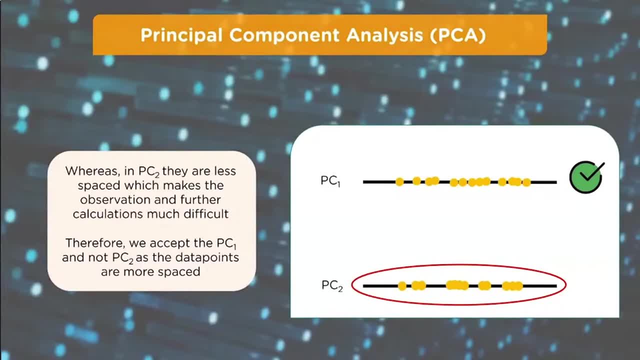 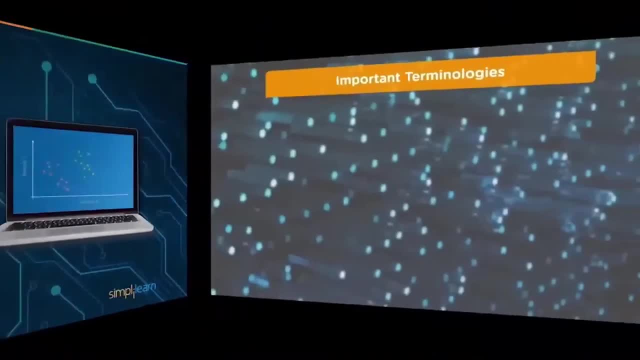 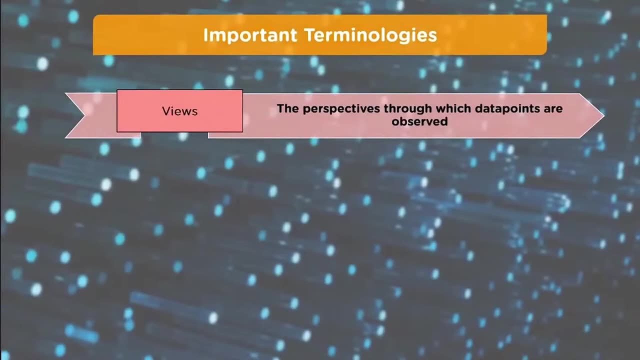 which would help in understanding how PCA analysis works. What we want to go ahead and do is dive into the important terminologies under PCA, And important terminologies are views, the perspective through which data points are observed, And so you'll hear that if someone's talking about a PCA presentation and they're not taking the time to reduce it to something. 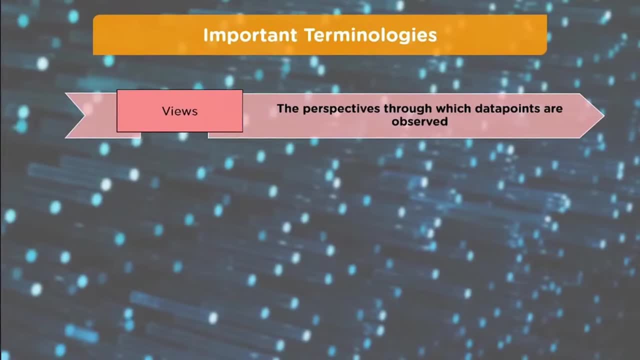 that the average person shareholders can understand. you might hear them refer to it as the different views. What view are we taking? Dimension number of columns in a data set are called the dimensions of that data set We talked about. you'll hear features, dimensions. 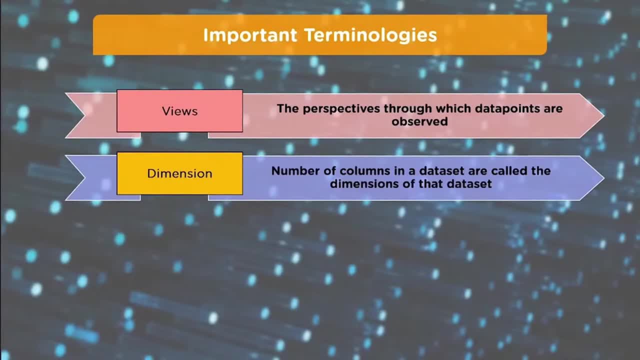 I was talking about features. There's usually, when you're running a business, you're talking 25,, 26,, 27 different features, minimal, And then you have the principal component: new variables that are constructed as linear combinations or mixtures of the initial variables. 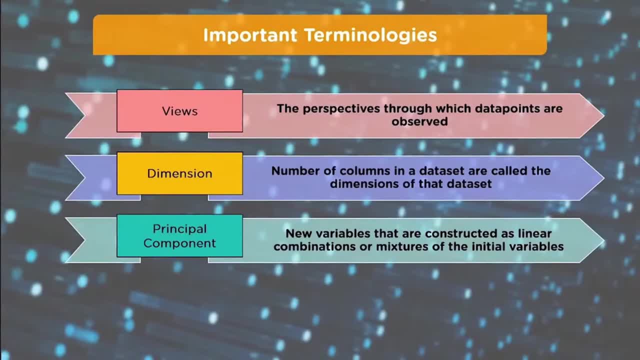 Principal component is very important. It's a combination. If you remember my flower example, it would be the width over the length of the petal, as opposed to putting both width and length in. You just put in the ratio instead, which is a single number versus two separate numbers. 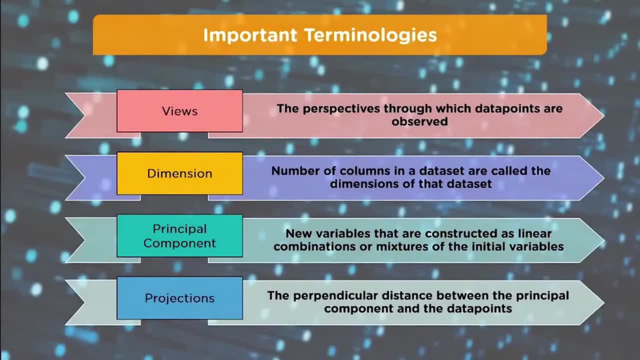 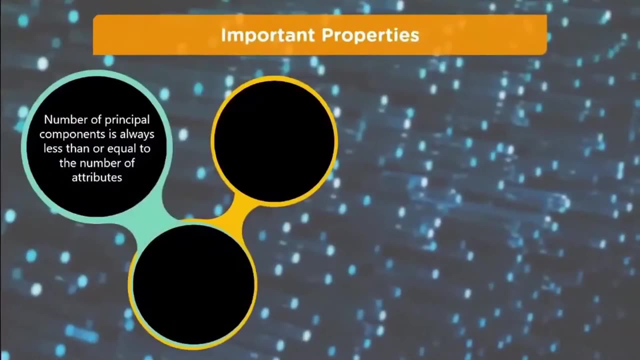 Projections, the perpendicular distance between the principal component and the data points. And that goes to that line we had earlier. It's that right angle line of where those points, how those points fall onto the line Important properties, important properties. Number of principal components is always less than the number of principal components. 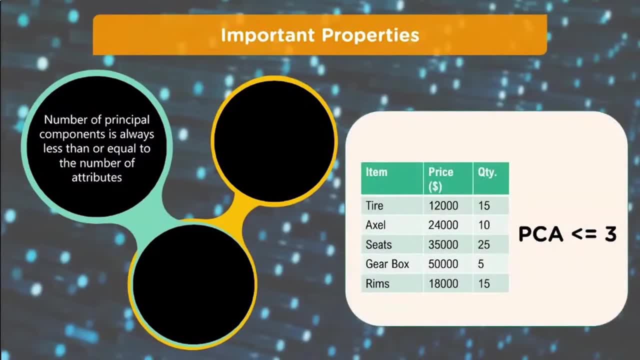 Number of principal components is always less than or equal to the number of attributes. That just makes common sense. You're not going to do ten principal properties with only three features. You're trying to reduce them. So it's just kind of goofy, but it is important to remember that. 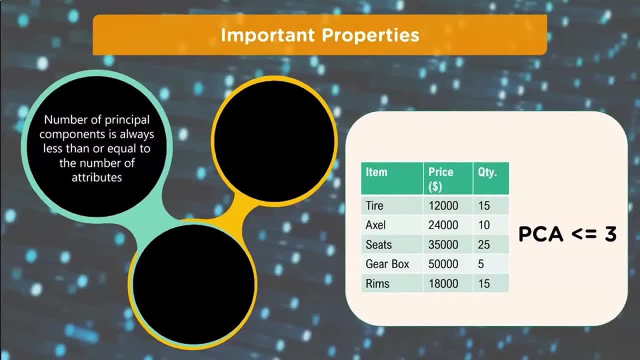 People will throw weird code out there and just randomly do stuff instead of really thinking it through. Principal components are orthogonal And this is what we're talking about- that right angle from the line when we do PC1.. We're looking at how those points fall onto that line. 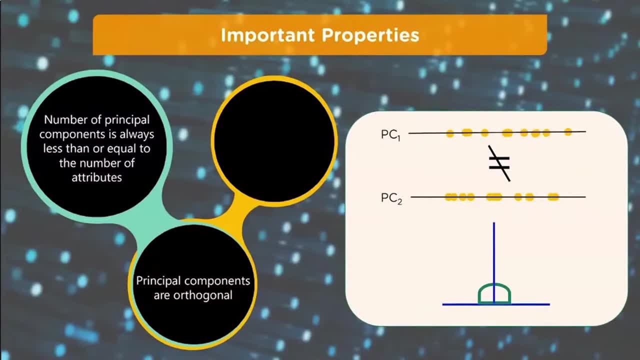 Same thing with PC2.. We want to make sure that PC1 does not equal PC2.. We don't want to have the same two principal points. when we do two points, The priority of principal components decreases as their numbers increase. This is important to understand. 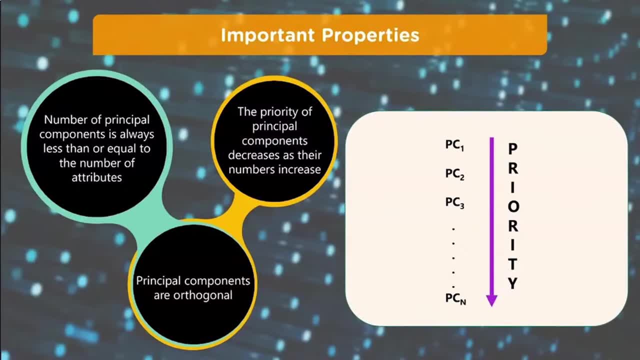 If you're going to create one principal component, everything is summarized into that one component. as we go to two components, the priority how much it holds value decreases as we go down. so if you have five different points, each one of those points is going to have less value than 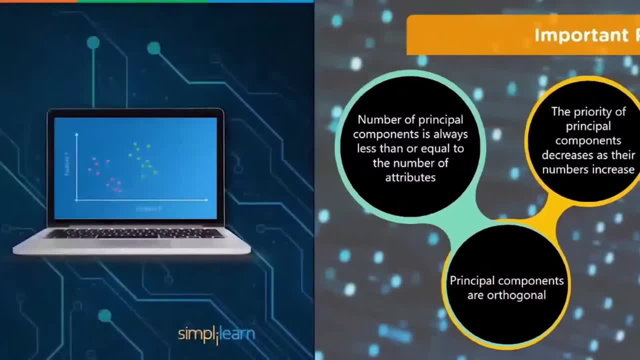 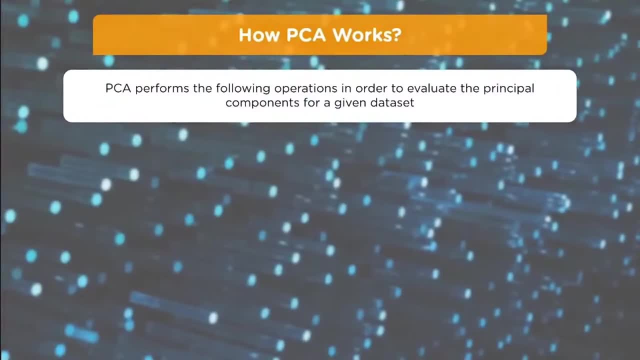 just the one point which has everything summarized in it: how PCA works. I said there was more in the back end. we talked about the math. this is what we're talking about is: how does it actually work? so now we have understanding that you're looking at a perspective. now we want to see how that math side works. PCA. 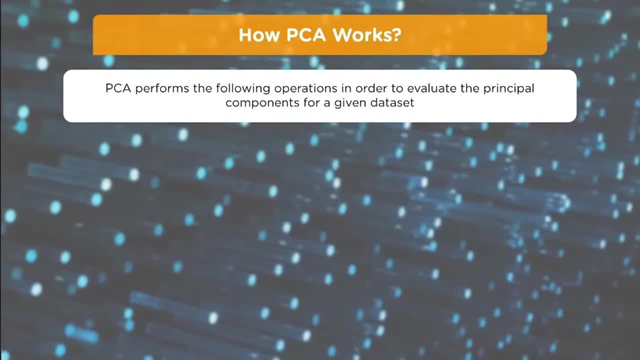 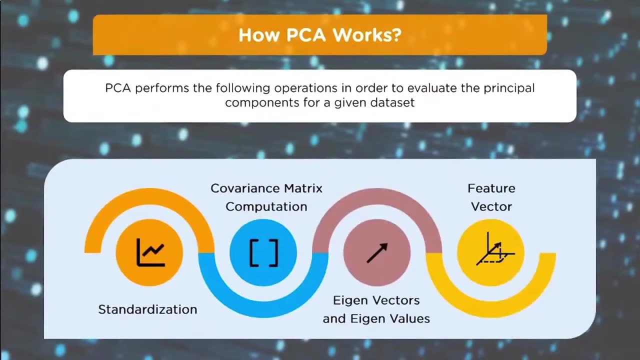 performs the following operations in order to evaluate the principal components for a given data set: first we start with the standardization, then we have a covariance matrix computation and we use that to generate our i gene vectors and i gene values, which is the feature vector. and if you remember, the i gene vector is like a. 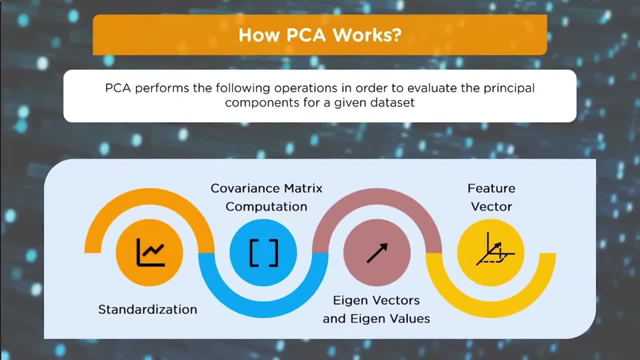 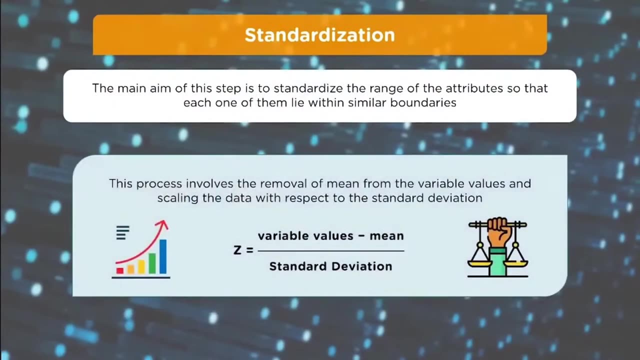 translation for moving the data from x equals 1 to x equals 2 or whatever altering it, and the i gene value is the final value that we generate. we talk about standardization. the main aim of this step is to standardize the range of the attributes so that each one of them lie within similar boundaries. this 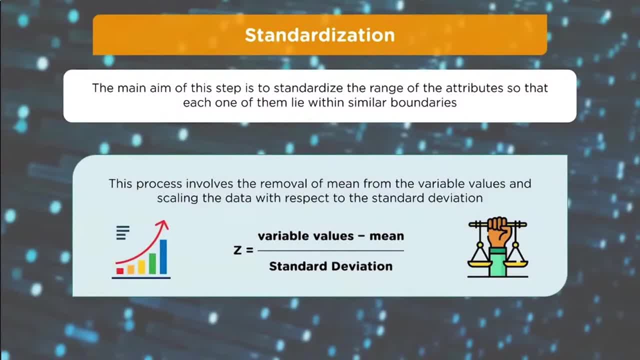 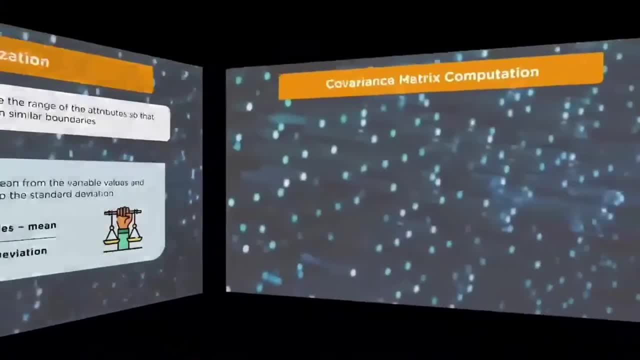 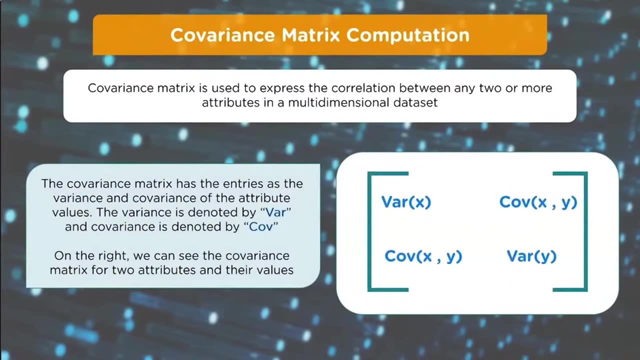 the standard deviation. the covariance matrix- computation covariance matrix is used to express the correlation between any two or more attributes in multi-dimensional data set. the covariance matrix has the entries as the variance and the covariance of the attribute values. the variance is denoted by var and the covariance is denoted by co. on the right we can see: 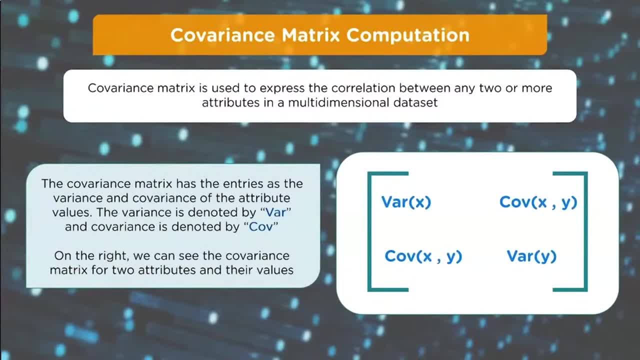 the covariance matrix for two attributes and their values. when we do a hands-on a look at the code, we'll do a display of this so you can see what we're talking about and what that looks like. for now, you can just notice that this is a. 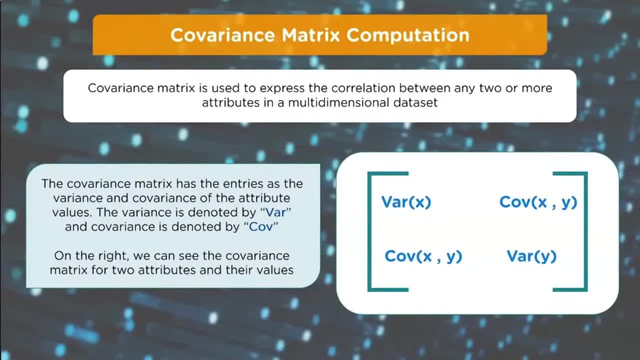 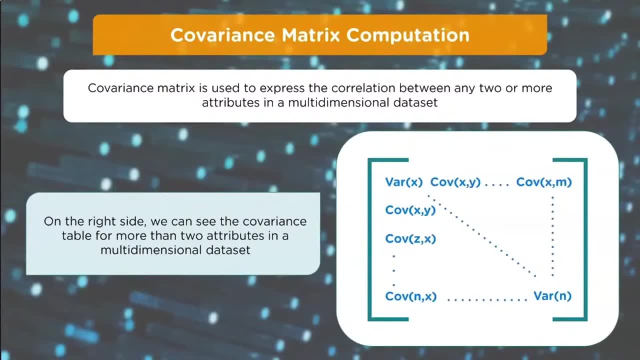 matrix that we're generating with the variance and then the covariance of x to y. on the right side we can see the covariance table for more than two attributes in a multi-dimensional data set. this is what I was talking about. we usually are looking at, not just one. 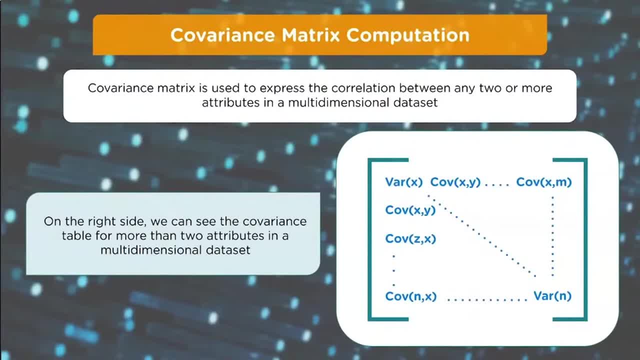 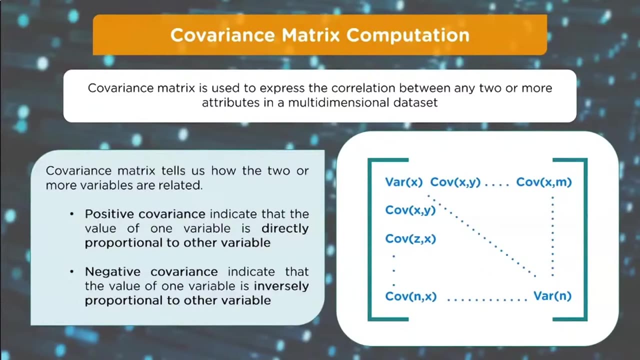 feature or two features. we're usually looking at 25, 30 features going on, and so if we do a setup like this, we should see all those different features as the different variables. covariance matrix tells us how the two or more variables are related. positive covariance indicate that the value of one variable is. 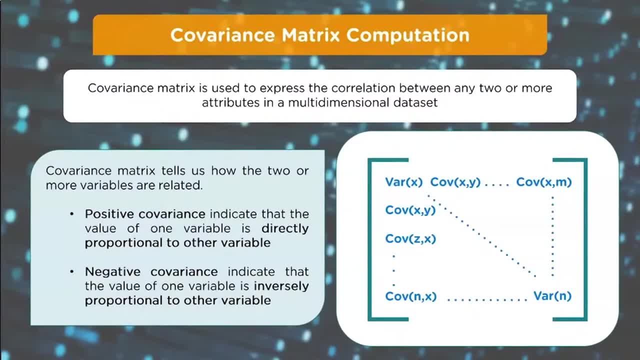 directly proportional to the other variable. negative covariance indicate that the value of one variable is inversely proportional to the other variable. that is always important to note whenever we're doing any of these matrixes that we're going to be looking at that positive and negative whether. 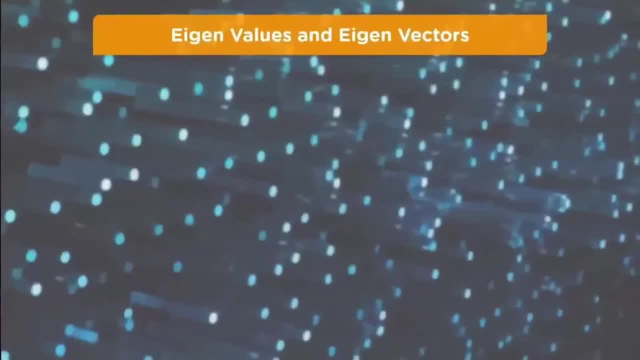 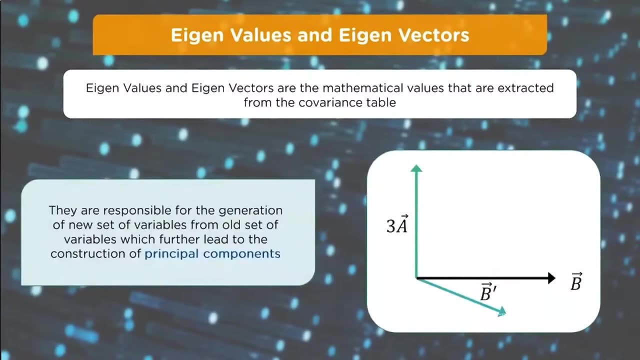 it's inverted or not. and then we have the i gene values and the i gene vectors. i gene values and i gene vectors are the mathematical value that are extracted from the covariance table. they are responsible for the generation of a new set of variables from the old set of variables, which further lead to the 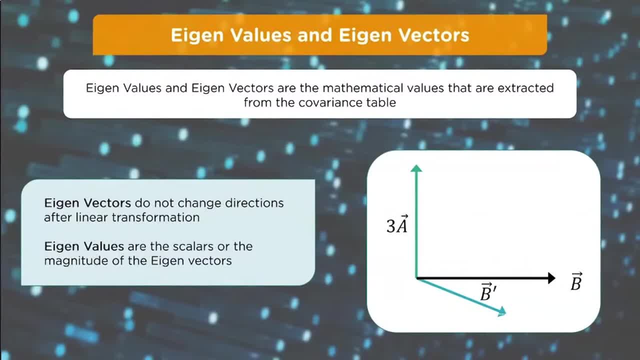 construction of the principal components. i gene vectors do not change directions after linear transformation. i gene values are the scalars or the magnitude of the i gene vectors and again this is just transforming that data. so we're going to change the vector B to the B prime as denoted on the chart. 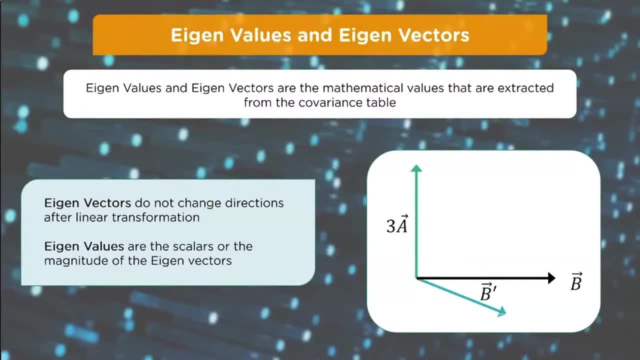 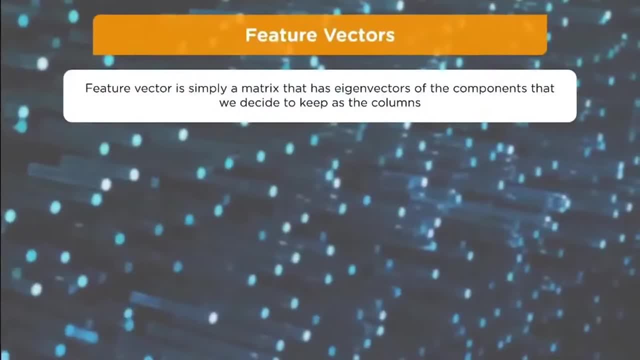 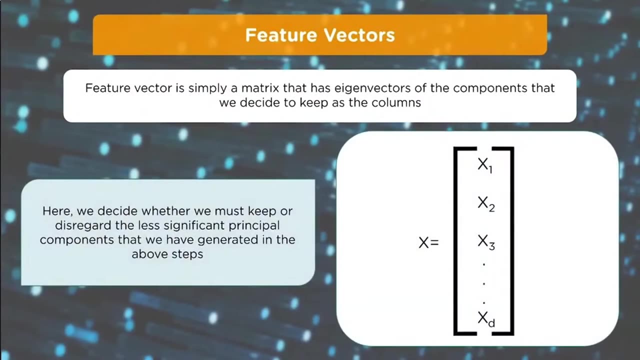 and so we have like multiple variables. how do we calculate that new variable? and then we have feature vectors. feature vectors is simply a matrix. it has i gene vectors of the components that we decide to keep as the columns. here we decide whether we must keep or discard. 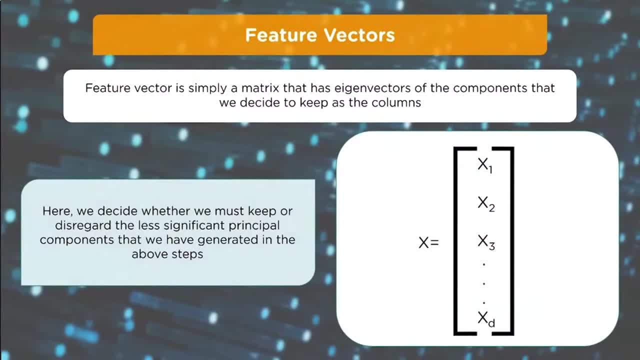 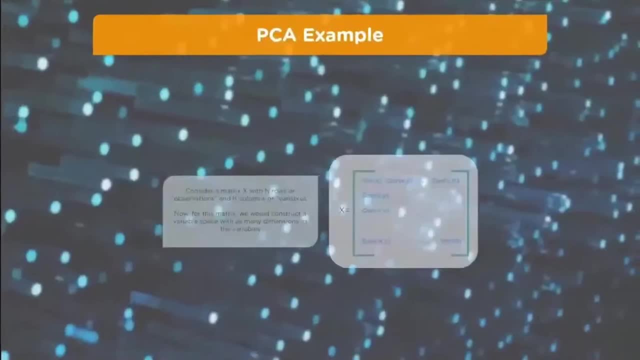 the less significant principal components that we have generated in the above steps. this becomes really important as we start looking at the back end of this, and we'll do this in the demo. but one of the more important steps to understand, and so we have the PC example. consider matrix X with 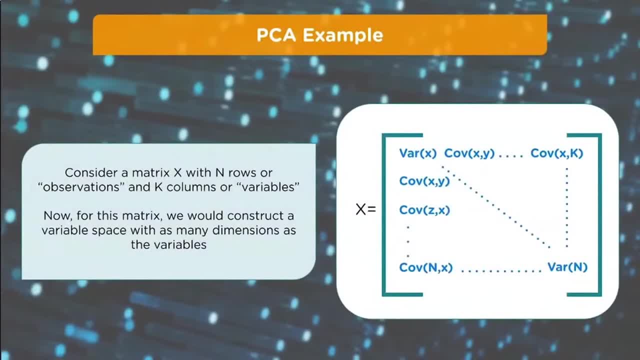 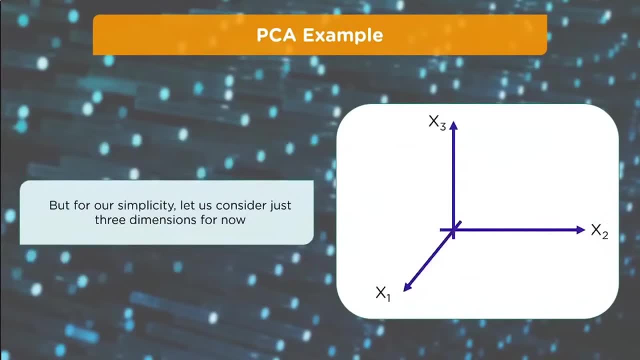 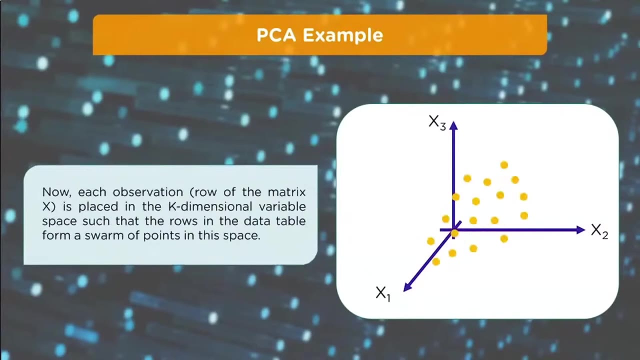 in rows or observations, and k columns or variables. Now for this matrix, we would construct a variable space with as many dimensions as the variable, But for our simplicity, let's consider this three dimensions for now. Now, each observation row of the matrix X. 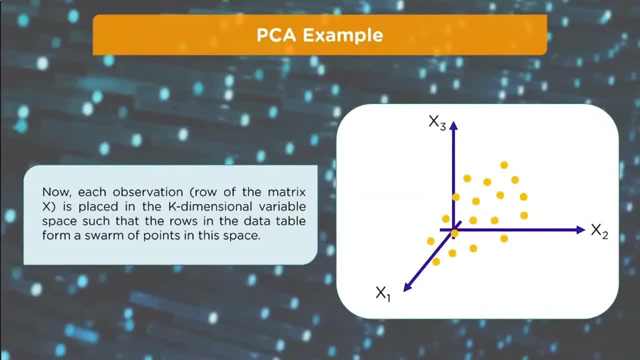 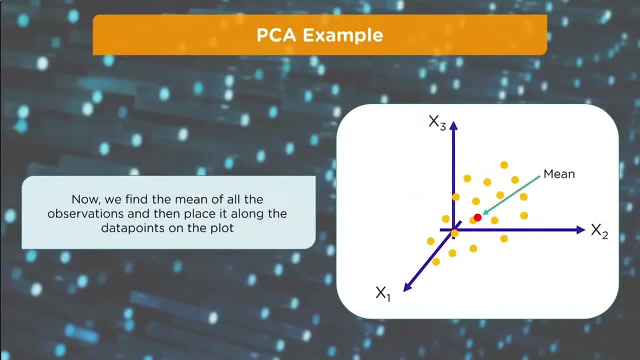 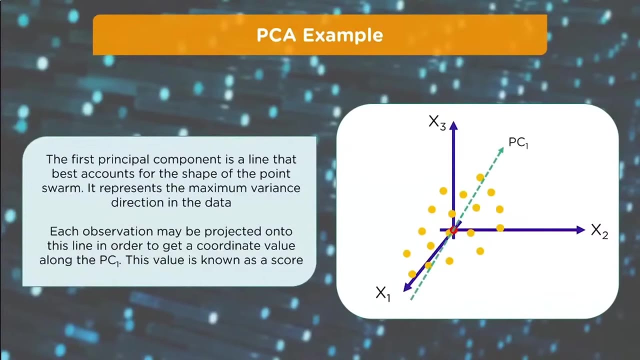 is placed in the k-dimensional variable space, such that the rows in the data table form a swarm of points in this space. Now we find the mean of all the observations and then place it along the data points on the plot. The first principal component is a line. 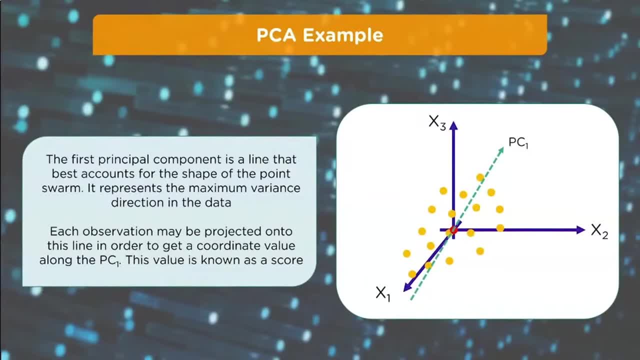 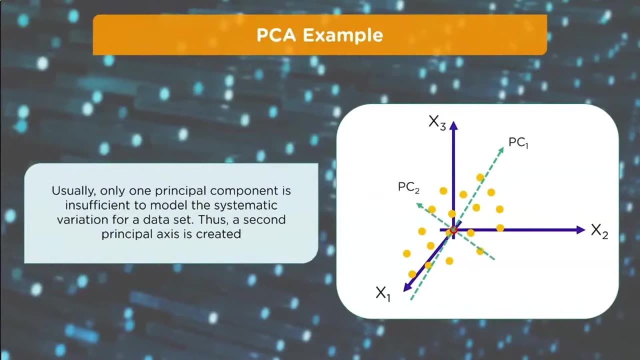 that best accounts for the shape of the point swarm. It represents the maximal variance direction in the data. Each observation may be projected onto this line in order to get a coordinate value along the PC1. This value is known as a score. Usually, only one principal component is insufficient. 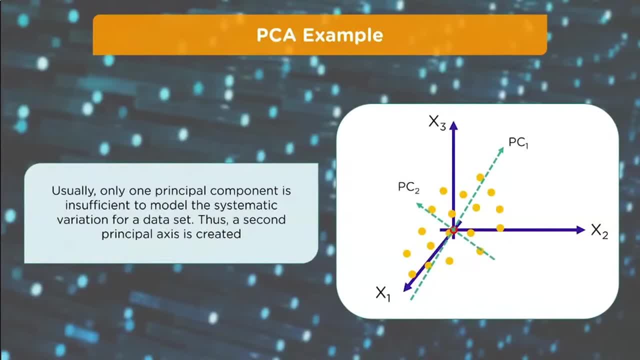 to model the systematic variation for a data set. Thus, a second principal axis is created. The second principal component is oriented such that it reflects the second largest source of variation in the data. While being orthogonal to PC1,, PC2 also passes through the average point. 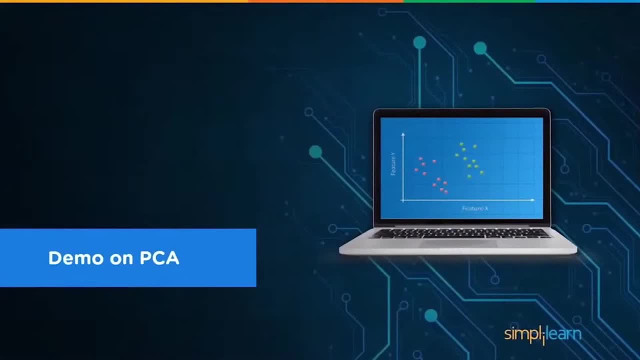 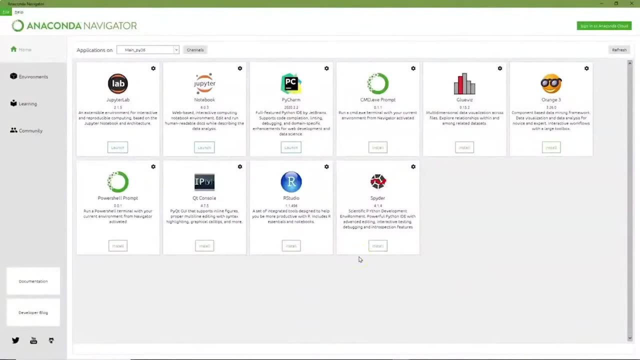 Let's go ahead and pull this up and just see what that means inside our Python scripting. I'm going to use the Anaconda Navigator and I will be in Python. I'm going to use Python 3.6 for this example. I believe there's even like a 3.9 out. 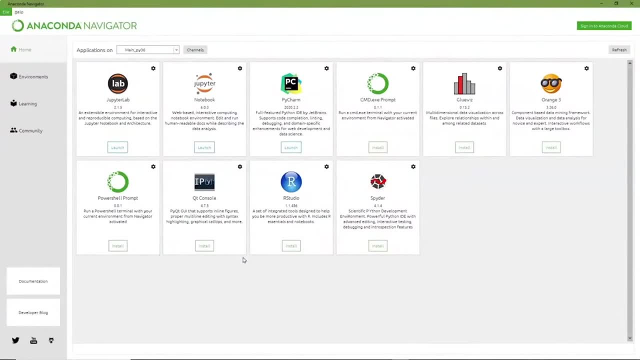 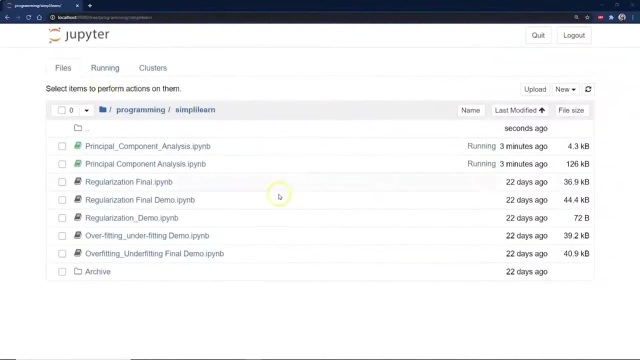 I tend to stay in 3.6 because a lot of the models I use, especially with the neural networks, are stable in 3.6.. And then we open up our Jupyter. I'm in Chrome. I'm going to go ahead and create a new Python 3.. 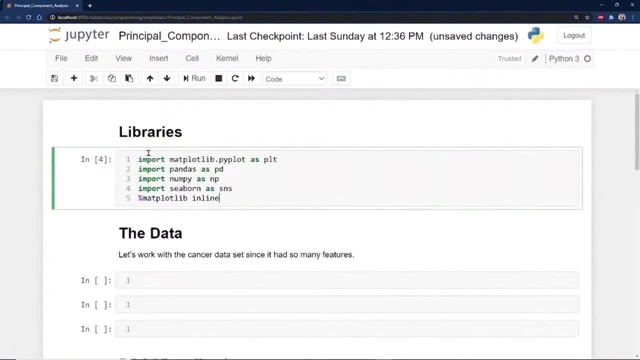 And for ease of use. our team in the back was nice enough to put this together for me, And we'll go ahead and start with the libraries, The first thing I like to do whenever I'm looking at any new setup. well, you know what? let's do the libraries first. 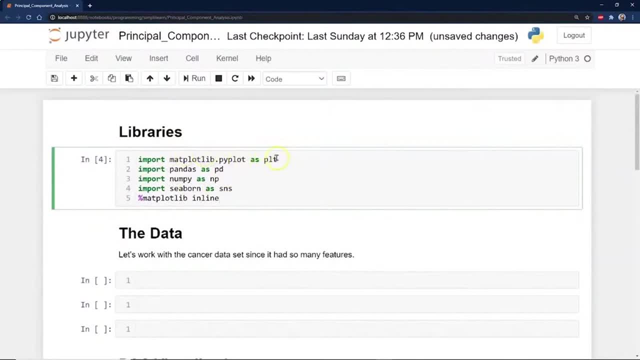 We're going to do our basic libraries, which is matplotlibrary, the PLT for the matplotlibrary, pandas, our data frame, PD numpy, our numbers array, NP, seaborn for graphing SNS. that goes with the plot that actually sits on matplotlibrary. 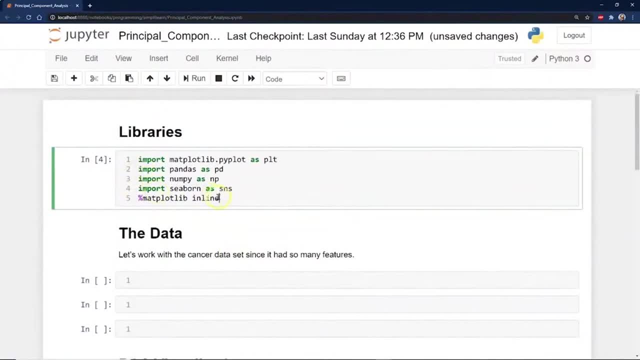 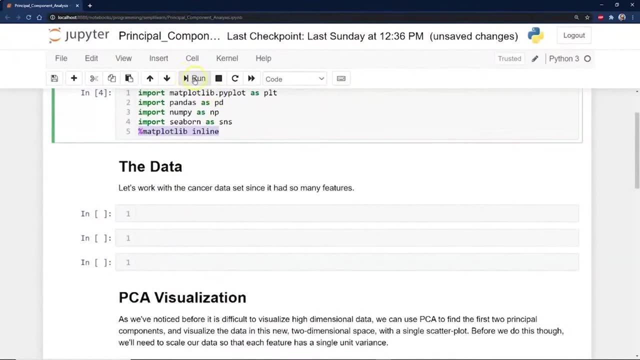 So the seaborn sits on there And then we have our amber sign because we're in Jupyter Notebook matplotlibrary in line. The newer version actually doesn't require that, but I put it in there either anyway, just because I'm so used to it. 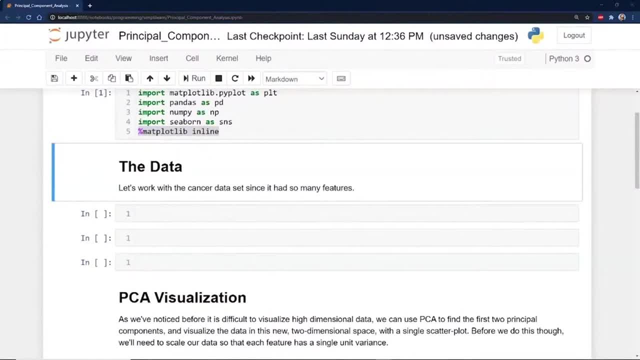 And then we want to go ahead and take a look at the data And in this case, we're going to pull in. certainly, you can have lots of fun with different data, but we're going to use the cancer data set, And one of the reasons the cancer data set is 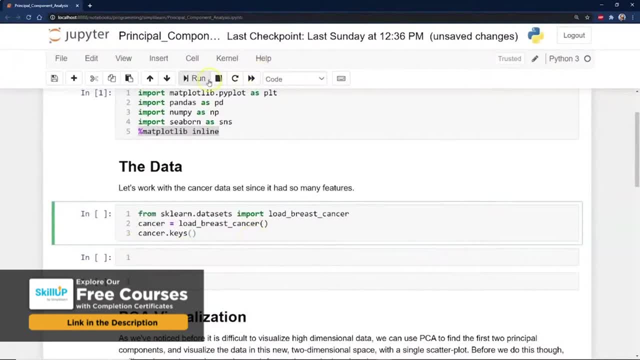 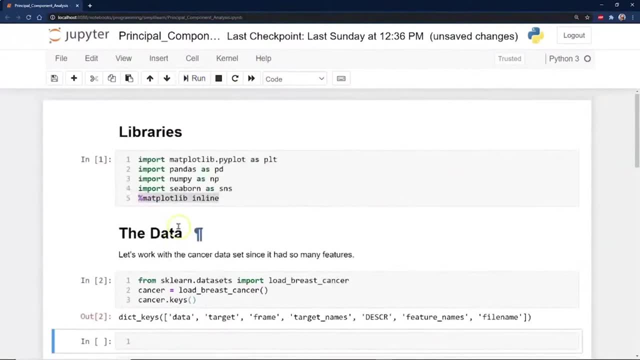 is it has like 36, 35 different features. So it's kind of fun to use that as our base for this. Then we'll go ahead and run this and look at our keys And the first thing we notice in our keys for the cancer data set. 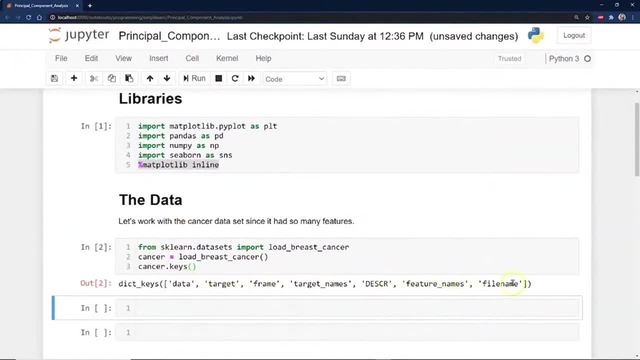 is: we have our data, we have our target, our frame, target names, description, feature names and file name. So what we're looking for in all this is: well, let's take a look at the description. Let's go in here. 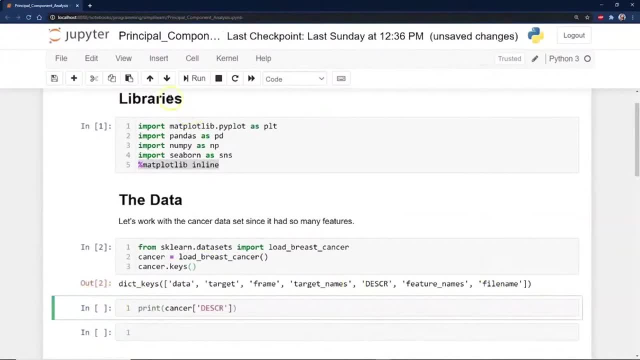 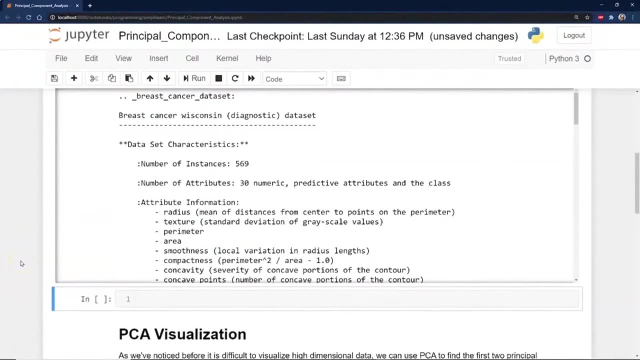 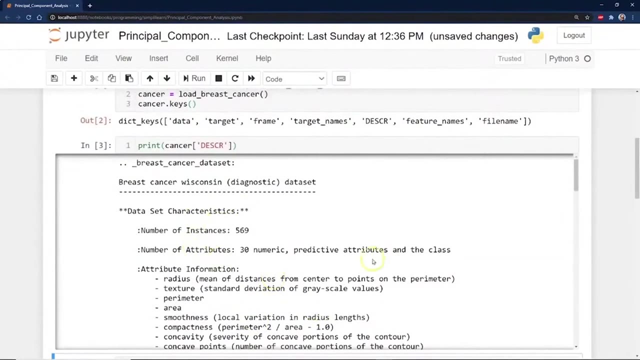 and pull up the description on here. I'm not going to spend a huge amount of time on the description, because this is. we don't want to get into a medical domain. We want to focus on our PCA setup. What's important is you start looking at. 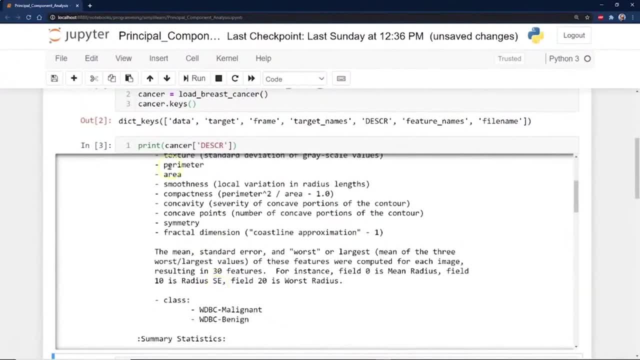 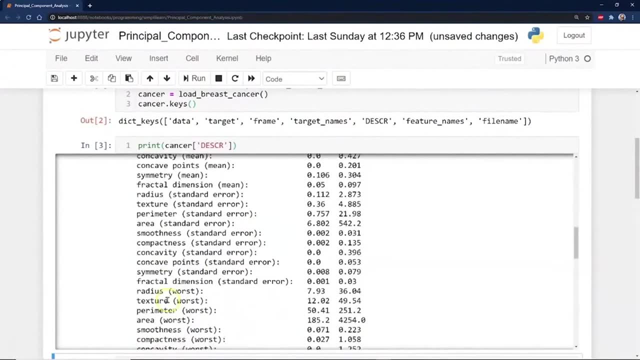 what the different attributes are, what they mean. If you were in the medical field, you'd want to note all these different things, whether what they're measuring, where it's coming from. You can actually see the actual different measurements, what the difference are taking. no missing attributes. 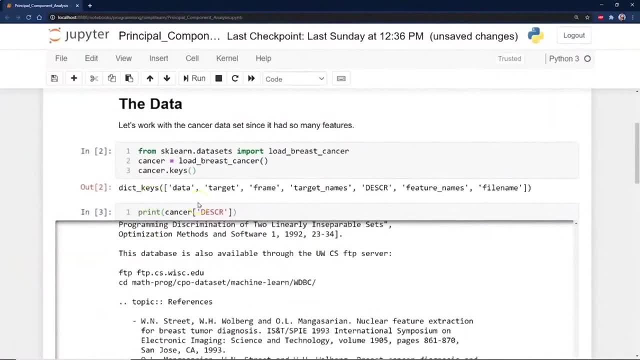 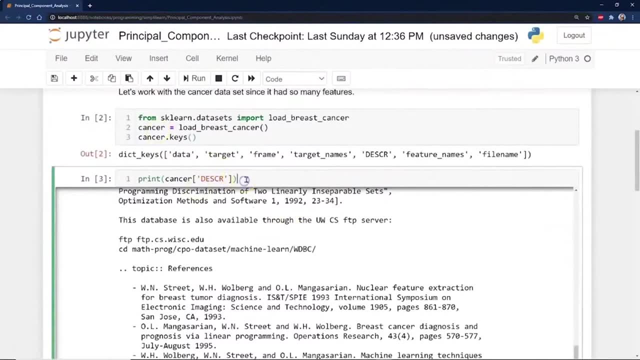 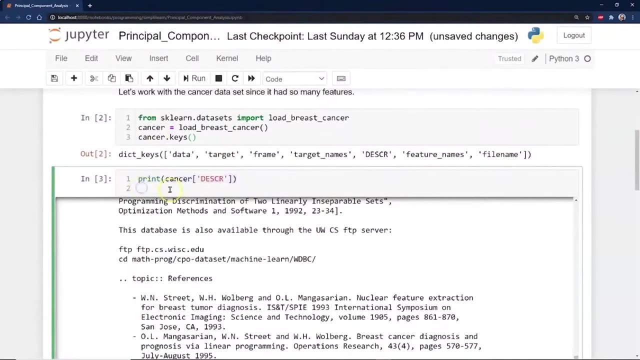 We page all the way to the bottom And you're going to have your data, in this case our target- And if you dig deep enough to the target, let's actually do this. Let's go ahead and print target names A little quick here. 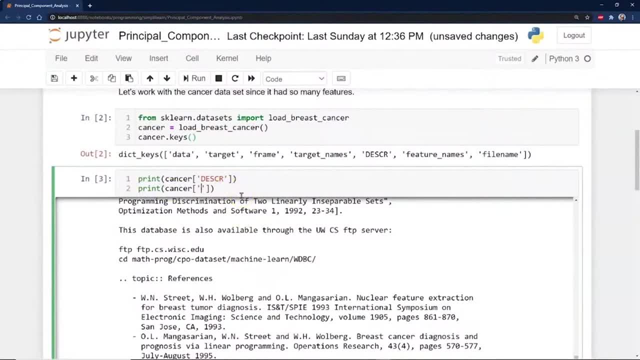 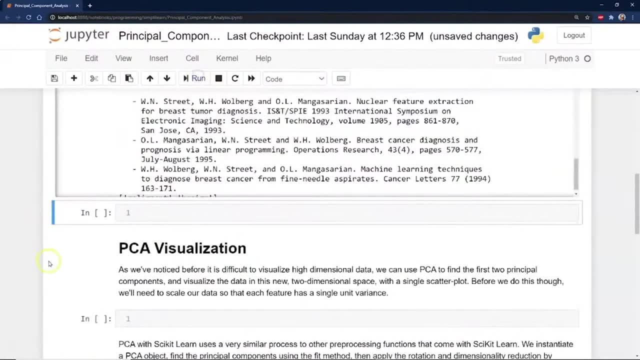 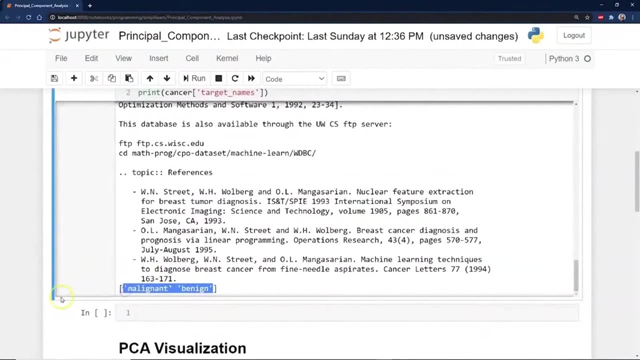 I always like to just take a look and see what's on the other end of this. Target names run that. So the target name is: is it malignant or is it benign? So in other words, is this dangerous growth or is it something we don't have to worry about? 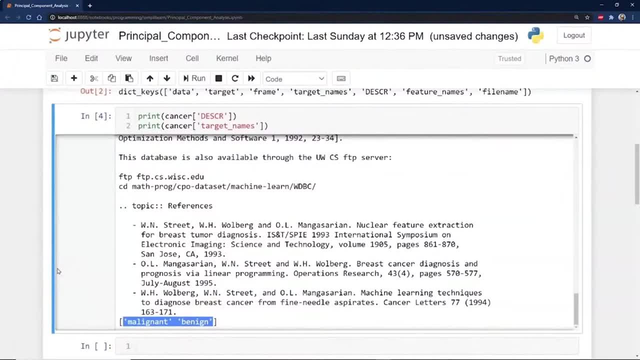 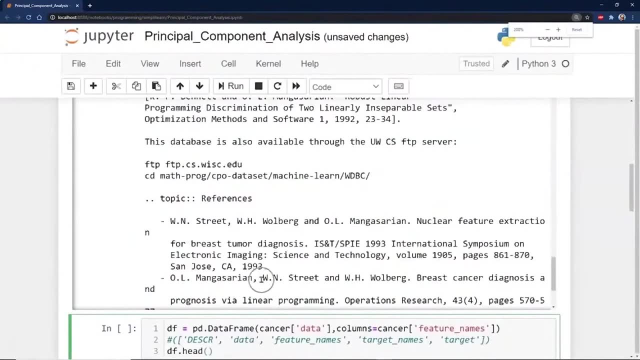 That's the bottom line with the cancer in this case. And then we can go ahead and load our data, And you know what? let me go up just a notch here so we're easy of reading. It's hard to get that just right. 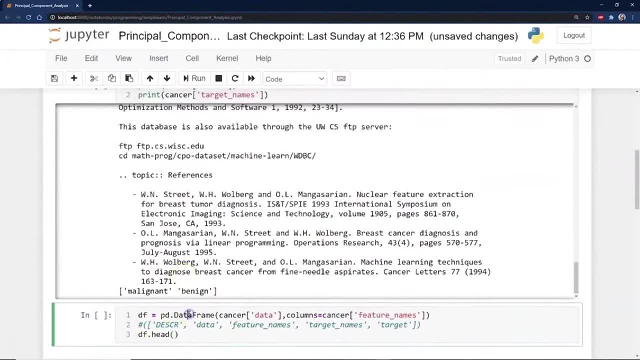 I guess I'll be able to do So. let's go ahead and look at our data. We're going to use our pandas and we're going to go ahead and do our data frame. It's going to equal cancer data Columns, equals cancer feature, equals feature names. 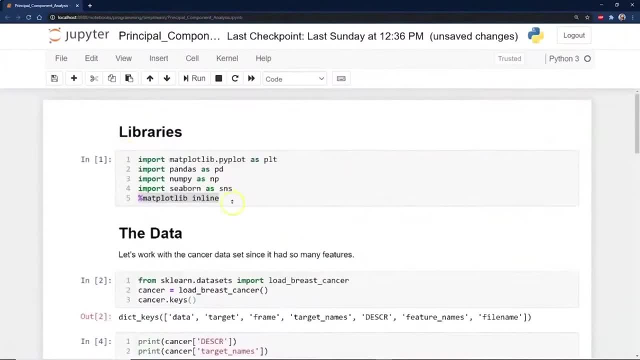 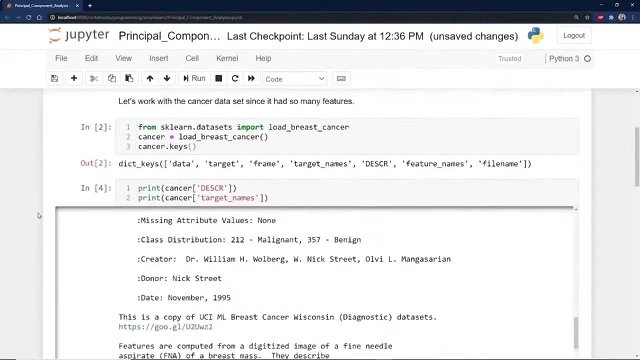 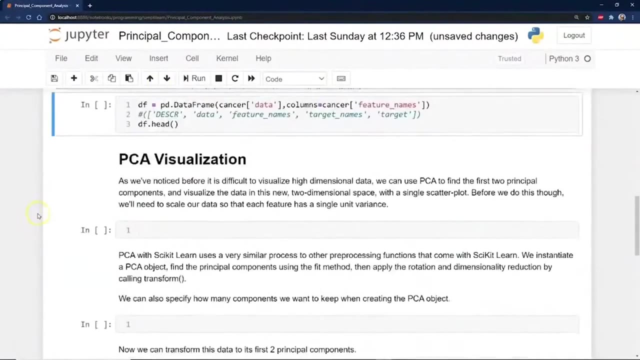 So remember up here we already loaded the names up of the features in there. What is going to come out of this? Let me just see if I can get to that. It's at the top of target names. That's just this list of names here in the setup. 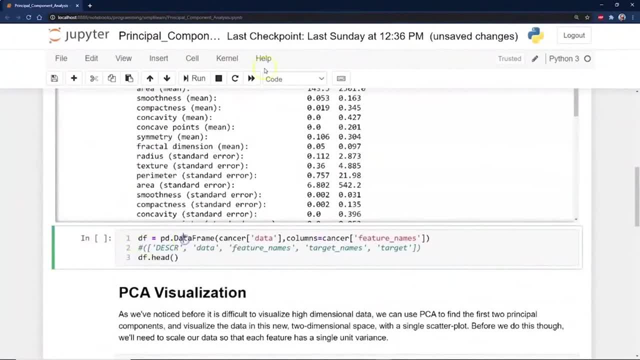 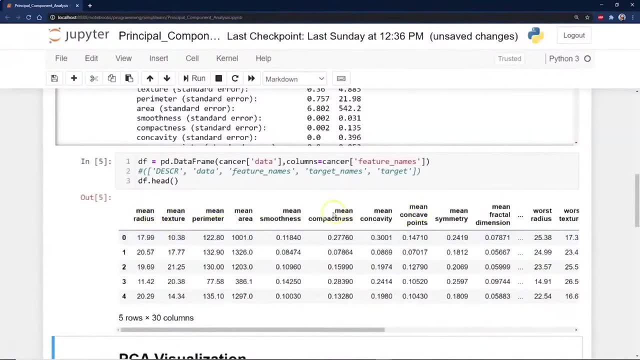 And we can go ahead and run this code and it'll print the head And you can see, here we have the mean radius, the mean texture, mean perimeter. I don't know about you. this is a wonderful data set, if you're playing with it, because, like many of the data, 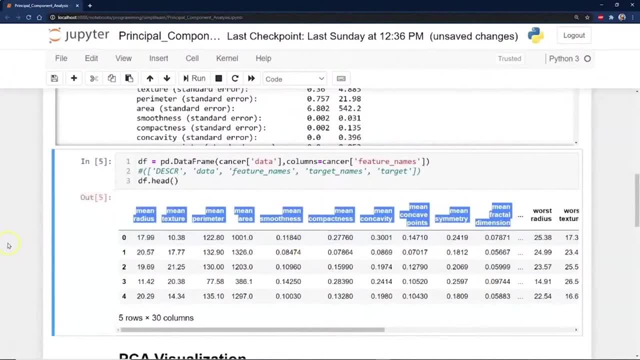 most of the data that comes in. half the time we don't even know what we're looking at. We're just handed a bunch of stuff as a data scientist going what the heck is this? And so this is a good place to start. 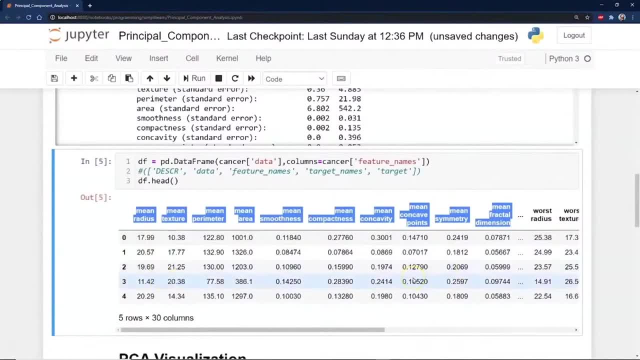 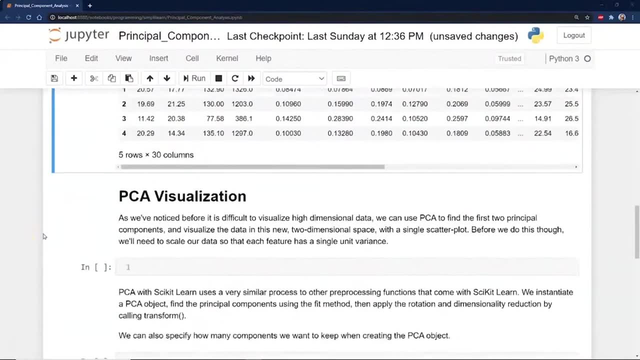 because this has a number of different features in there and we have no idea what these feature means or where they come from. We want to just look at the data and figure that out, And now we actually are getting into the PCA side of it. 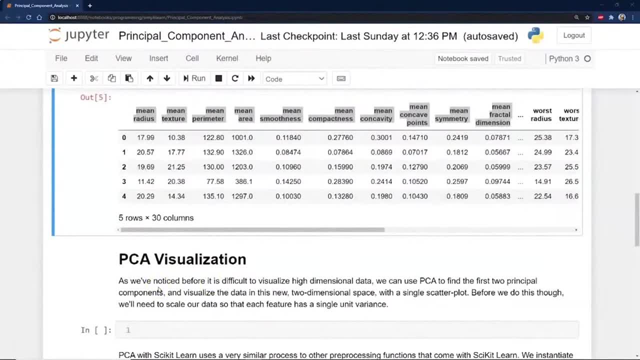 As we've noticed before, it is difficult to visualize high dimensional data. We can use PCA to find the first two principal components and visualize the data, this new two-dimensional space with a single scatter plot. Before we do this, we need to go ahead and scale our data. 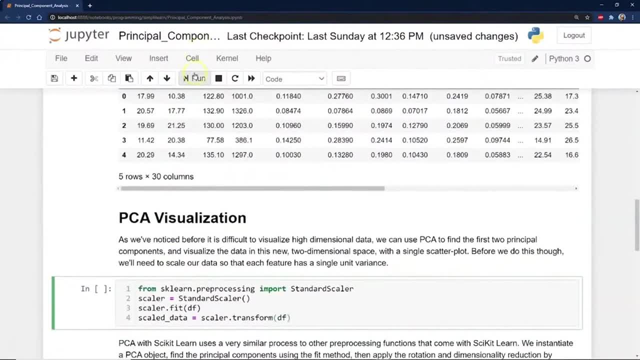 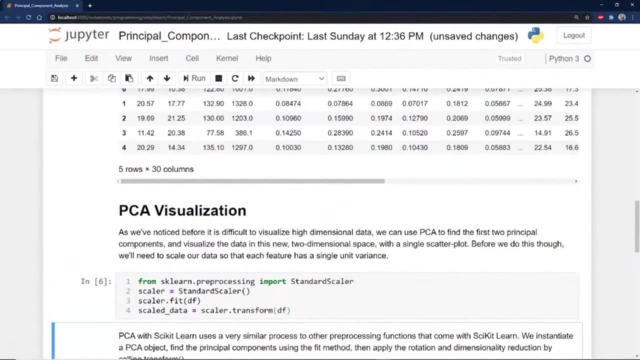 Now, I haven't run this to see if you really have to scale the data on this, but as just a general run time. I almost do that as the first step of any modeling, even if it's pre-modeling, as we're doing here. 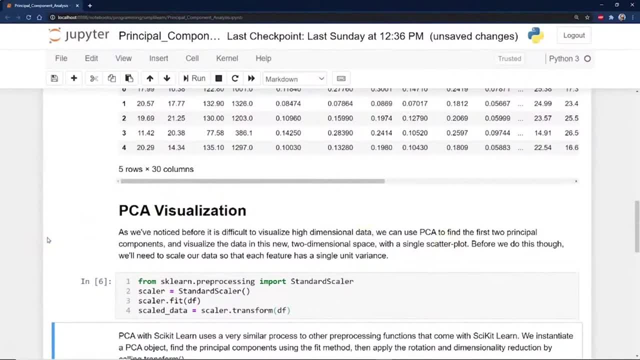 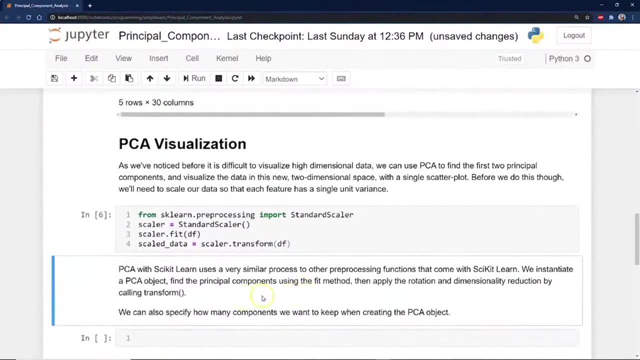 In neural networks that is so important With PCA visualization. it's already going to scale it when we do the means and deviation inside the PCA, But just in case, it's always good to scale it. And then we're going to take our PCA with the scikit-learn. 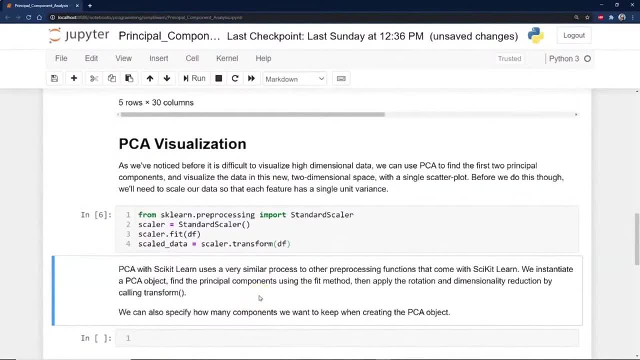 uses very similar process to other pre-processing functions that come with scikit-learn. We instantiate a PCA object, find the principal components using the fit method, then apply the rotation and dimensionality reduction. by calling transform We can also specify how many components we want to keep. 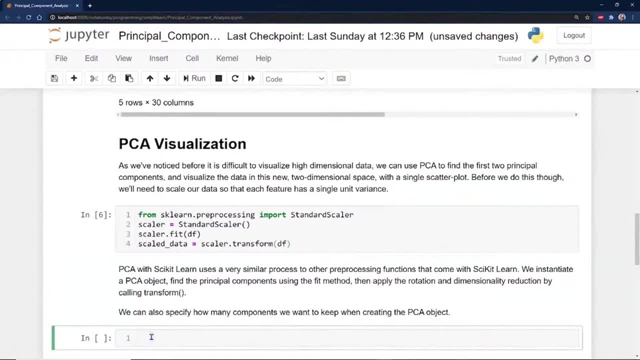 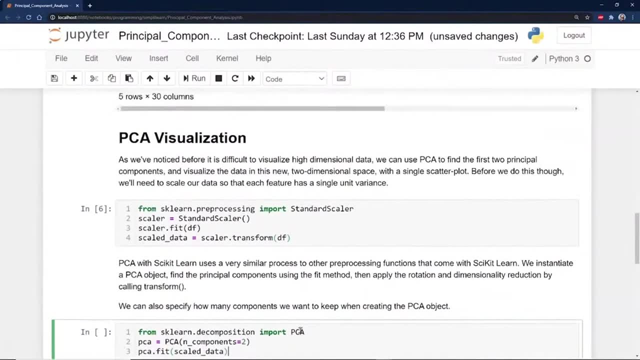 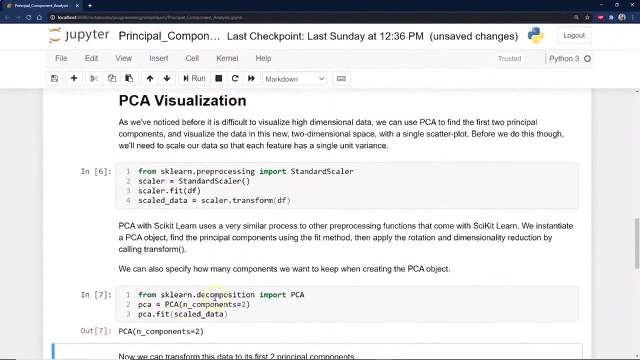 when creating the PCA object, And so the code for this Ops getting a little bit ahead. Let me go ahead and run this code. So the code for this is: from sklearn decomposition: import PCA. PCA equals PCA and components equals 2.. 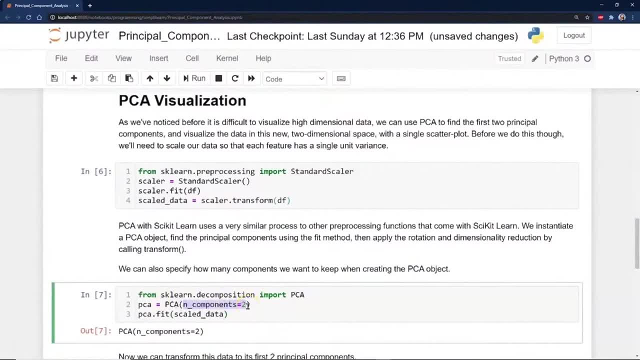 And that's really important to note that, because we're only going to want to look at two components, I would never go over four components. I'll show you how to do that in a minute, especially if you're going to demo this with somebody else. 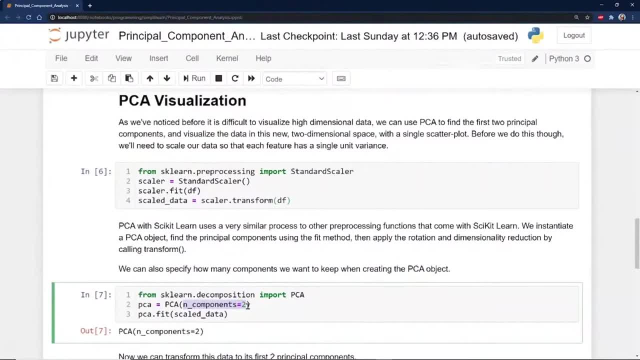 If you're showing this to the shareholders, the whole idea is to reduce it to something people can see, And then the PCA fit. we're going to take the scaled data that we generated up here and then you can see we've created our PCA model with: in components equals 2.. 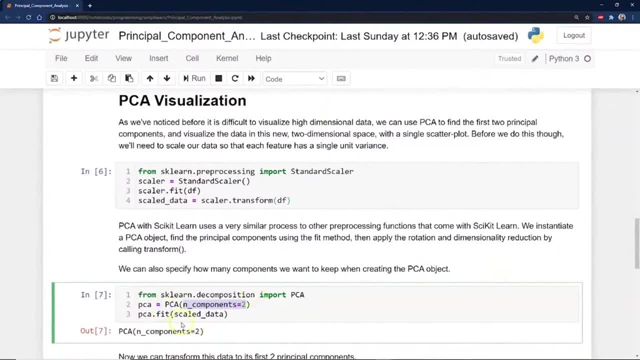 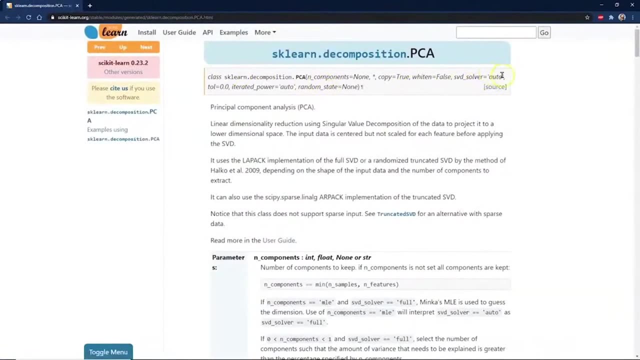 Now, whenever I use a new tool, I like to go in there and actually see what I'm using. So let's go to the Scikit web page for the PCA And you can see in here. here's our call statement. It describes what all the different setups you have on there. 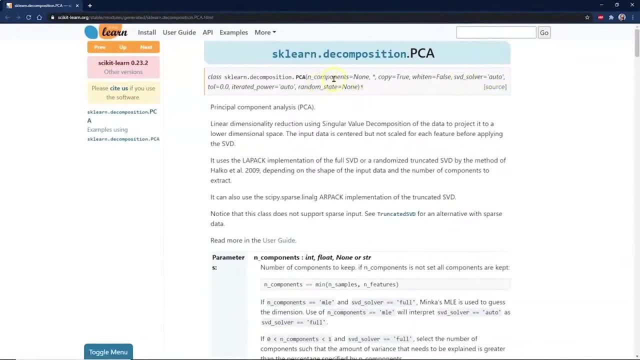 Probably the biggest one to look at would. be well, the biggest one is your components. how many components do you want which you have to put in there pretty much. And then you also might look at the SVD solver. It's on auto right now, but you can override that. 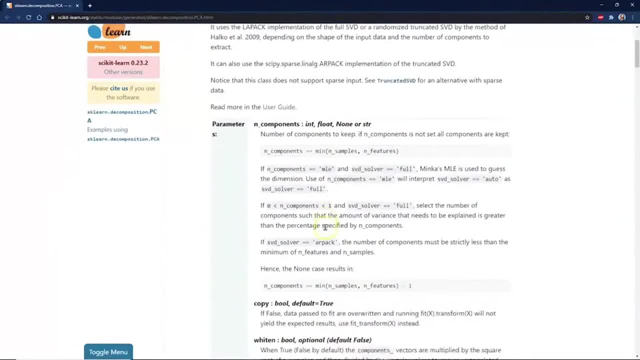 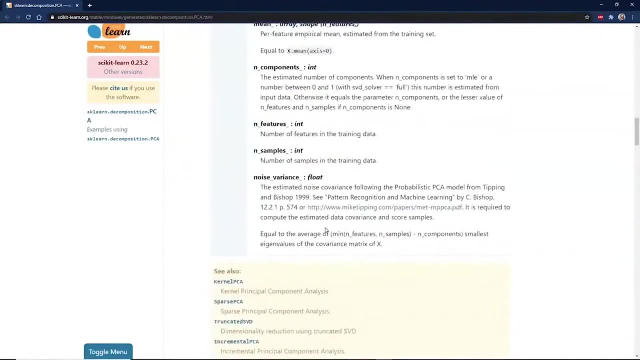 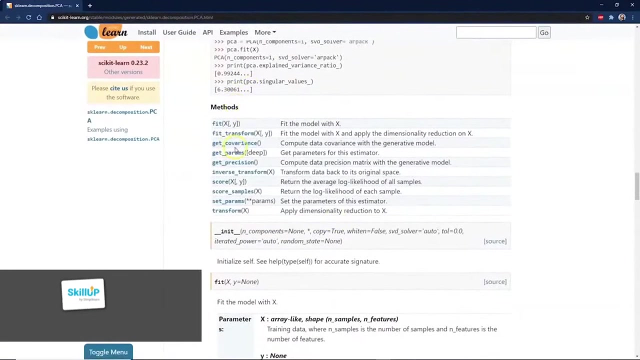 and do different things with it, It doesn't matter. It does a pretty good job as it is. And if we go down all the way down to our methods, if you notice we have fit and we have fit transform. Nowhere in here is predict. 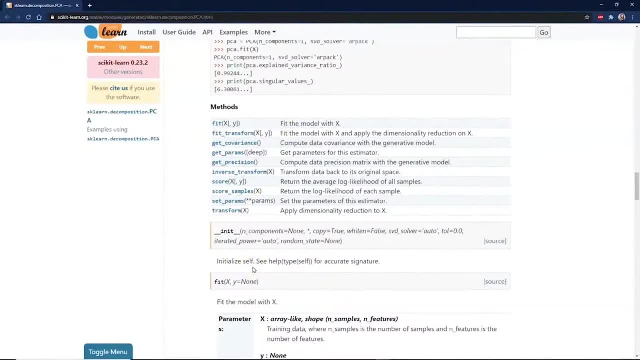 because this is not used for prediction. It's used to look at the data. Again, we're in the describe setup. We're fitting the data, We're taking a look at it. We've already looked at our minimum maximum. We've already looked at what's in each quarter. 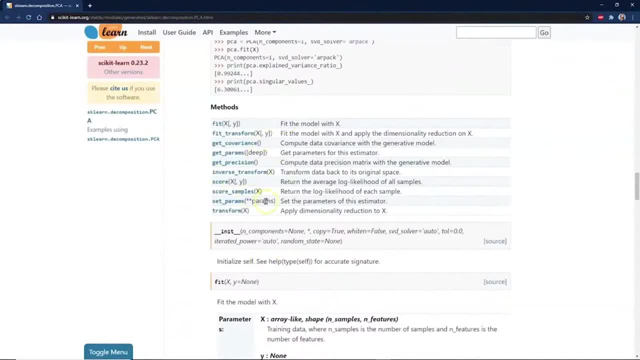 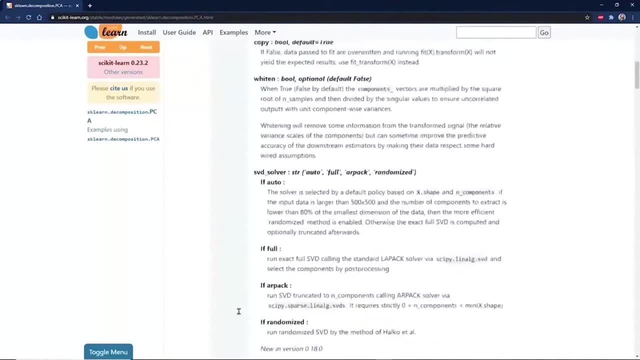 We've done a full description of the data. This is part of describing the data. That's the biggest thing I take away when I come zooming in here- And of course they have examples of it down here if you forget- And the biggest one, of course, is the number of components. 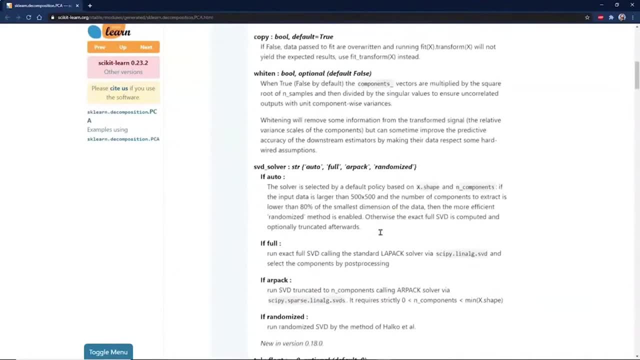 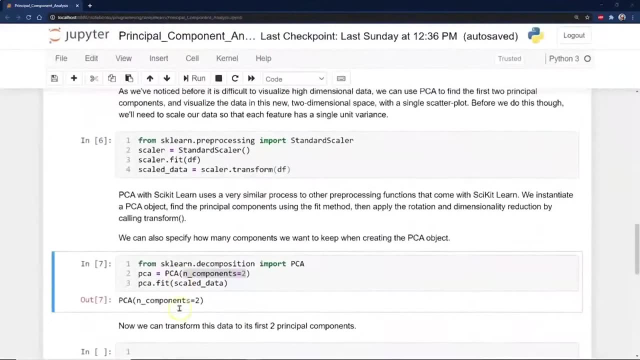 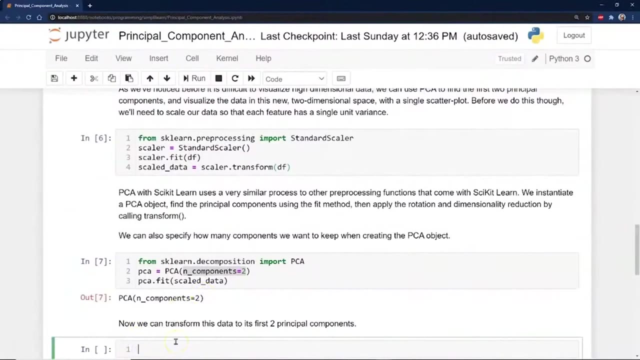 And then I mean the rest. you can play with The actual solver, whether you're doing a full or randomized. there's different things. It does pretty good on the auto, And now we can transform this data to its first two principal components. 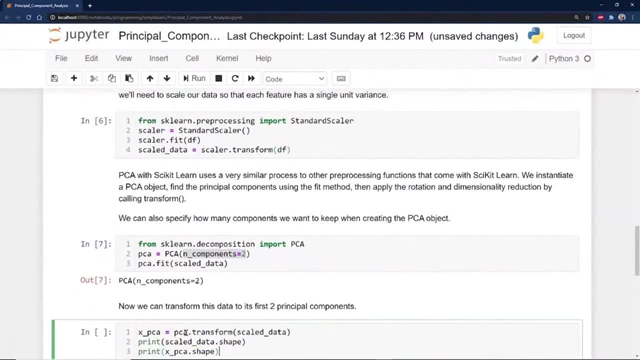 And so we have our XPCA. We're going to set that equal to PCA transform scaled data. So there we go, There's our first transformation, And let's just go ahead and print the scaled data shape and the XPCA data shape. 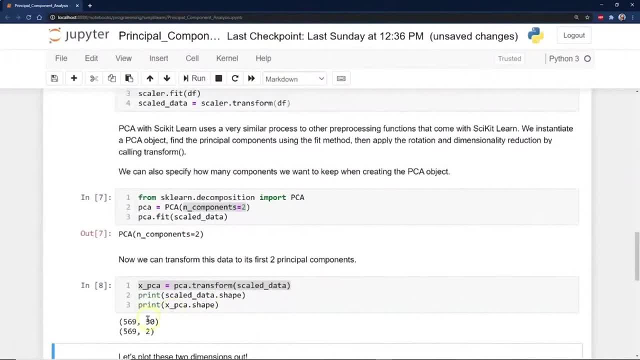 And the reason we want to do this is just to show us what's going on here. We've taken 30 features. I think I said 36 or something like that, but it's 30. And we've compressed it down to two features. 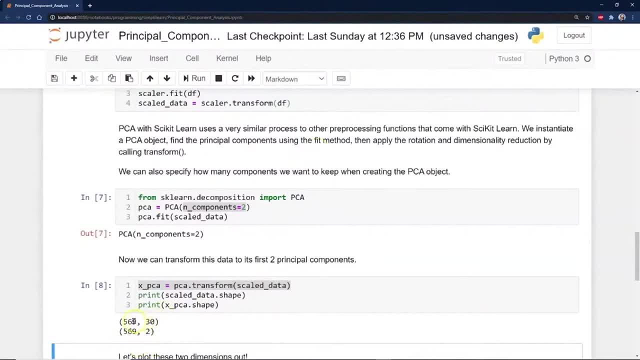 And we decided we wanted two features. And that's where this comes from. We still have 569 data sets. I mean data rows, not data sets. We still have 569 rows of data, But instead of computing 30 features, we're now only doing our model on two features. 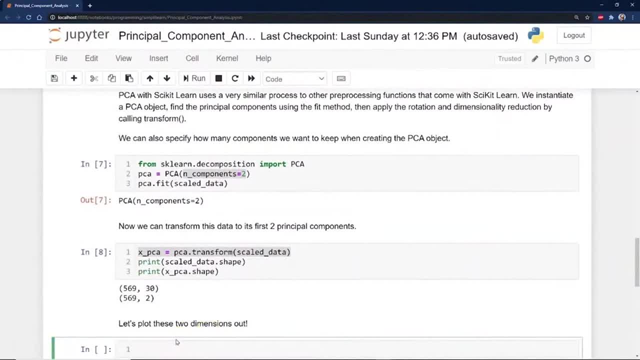 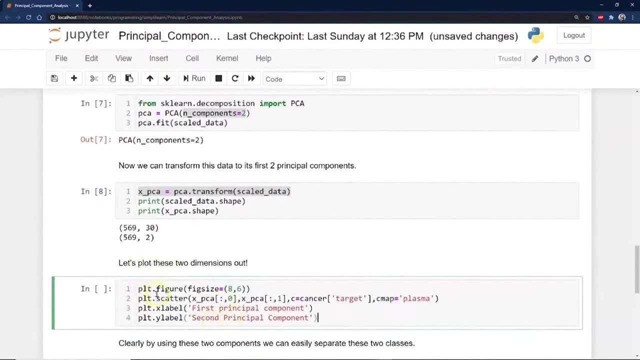 So let's go ahead and plot these and take a look and see what's going on, And we're just going to use our PLT figure. We're going to set the figure size on here. Here's our scatter plot: XPCA. 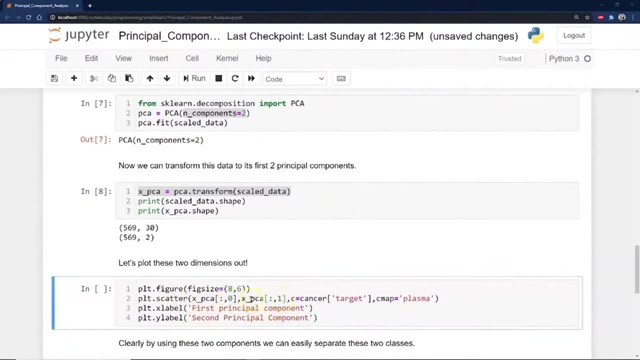 X underscore PCA of one. These are two different perceptions we're using, And then you'll see right here: C for color cancer equals target, And so remember, we have zero, We have one And, if I remember correctly, zero was malignant. 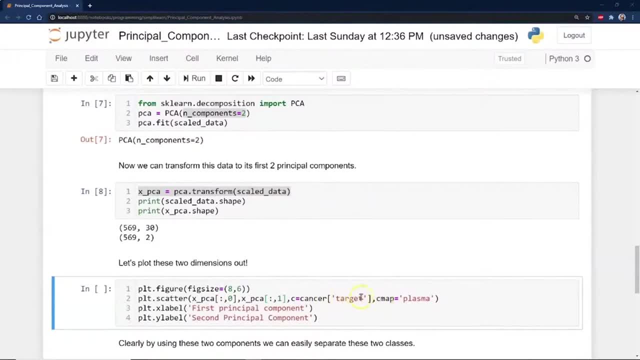 One was benign. So everything in the zero column is going to be one color And the other color is going to be one. And then we're going to use the plasma map just kind of telling you where it is, add some labels. 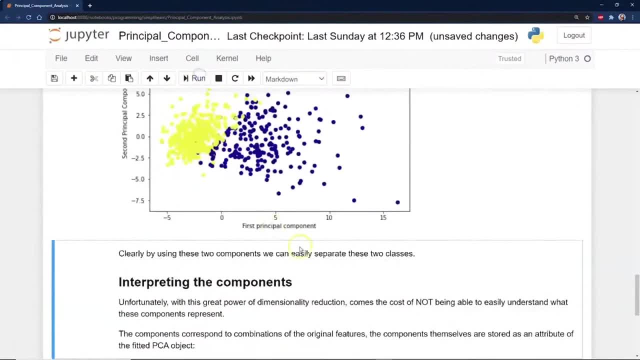 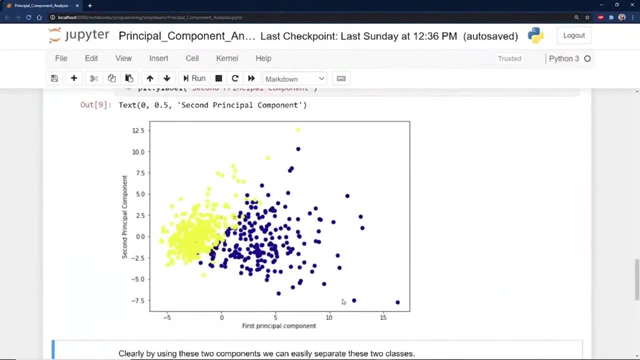 first principal component. second principal component: And we'll go ahead and run this And you can see here, instead of having a chart, one of those heat maps with 30 different columns in it, we can look at this and say, hey, this one actually did a pretty good job. 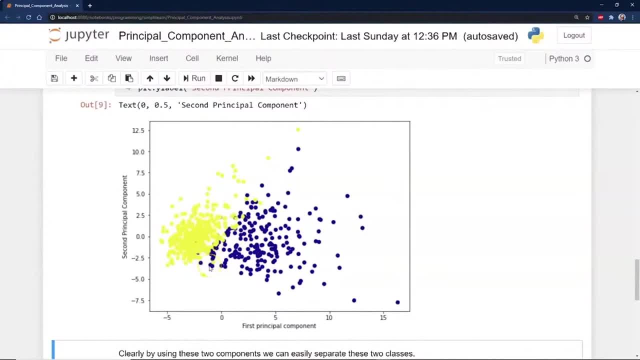 of separating the data And a couple things. when I'm looking at this that I notice is: first, we have a very clear area where it's clumped together, where it's going to be benign, And we have a huge area. 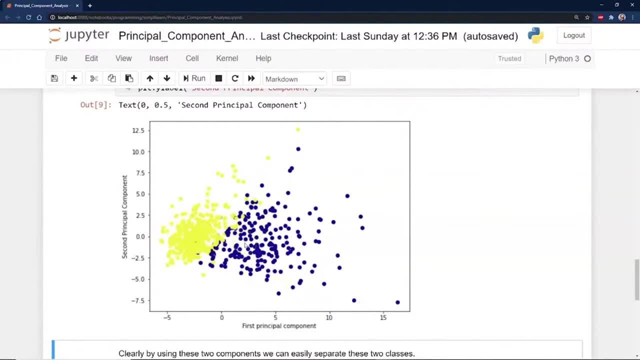 it's still clumped together, more spread out where it's going to be malignant, or I think I had that backwards And then in the middle, because we're dealing with something, in this particular case cancer, we would try to separate. 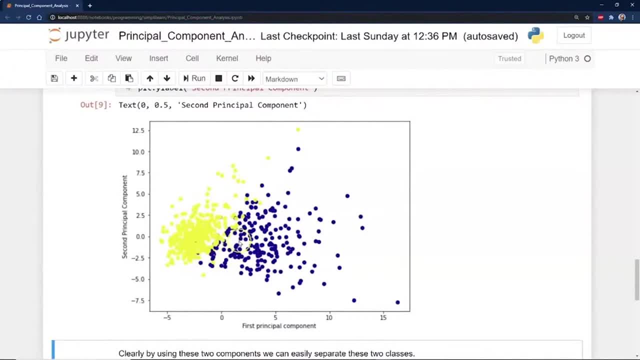 I would be exploring how to separate this middle group out. In other words, there's an area where everything overlaps and we're not going to have a clear result on it Just because those are the people. you want to go in there and have extra tests. or treat it differently, versus going in and saying just cutting into the cancer so the body absorbs it and it dissipates, versus actively going in there, removing it, testing it, going through chemo and all the different things. That's a big difference. 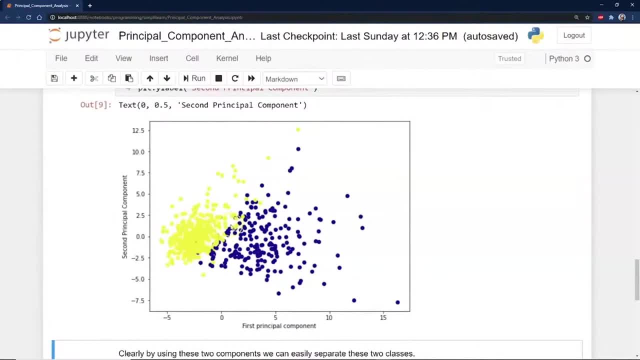 as far as what's going to happen here, And that middle line where they overlap is going to be huge. That's domain specific. Going back to the data we can see here clearly, by using these two components we can easily separate these two classes. 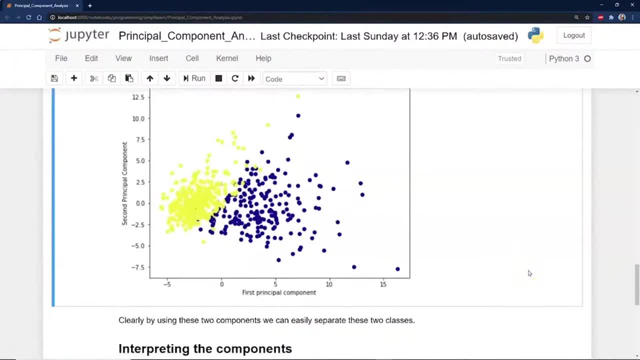 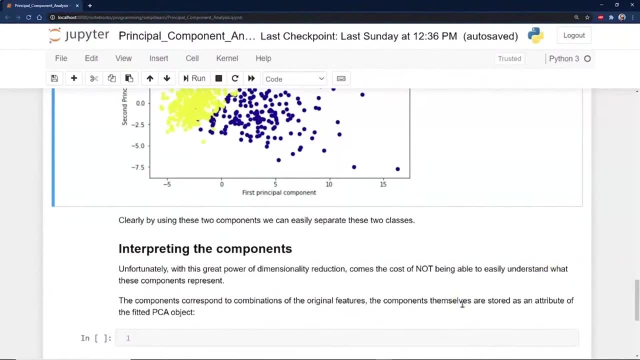 So the next step is: what does that mean? Interpreting the components. Unfortunately, with this great power of dimensionality reduction comes the cost of not being able to easily understand what these components represent. I don't know what principle component one represents. 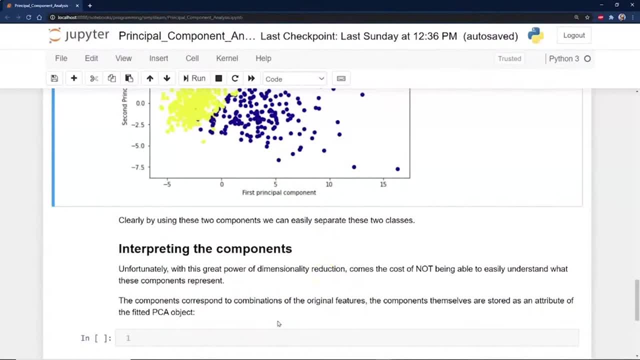 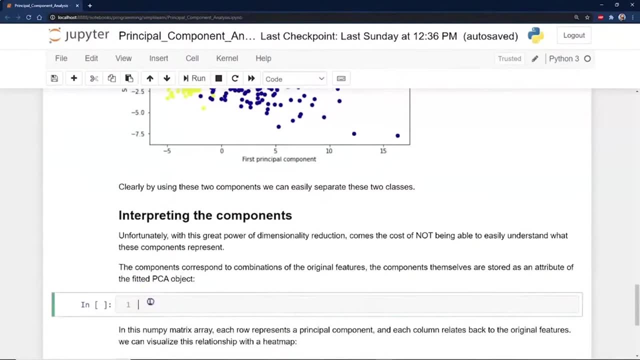 or second principle, The components correspond to combinations of original features. The components themselves are stored as an attribute of the filtered PCA object And so when we look at that, we can go ahead and do look at the PCA components. This is in our model we built. 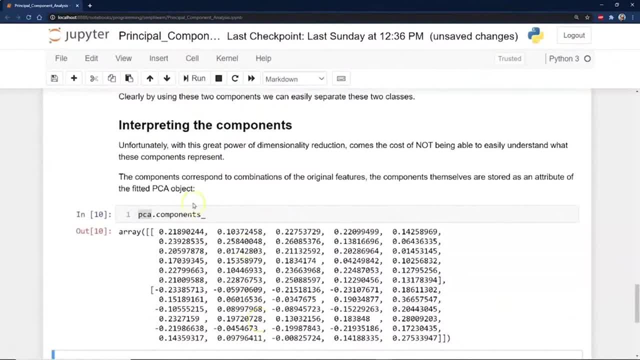 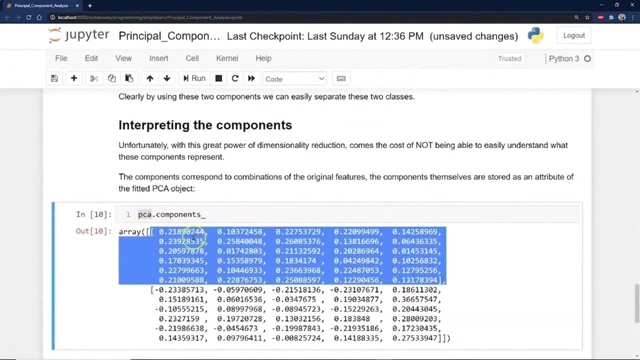 We've trained it. We can run that and you can see. here's the actual components. It's the two components. they each have their own array And within the array you can see the what, the scores they're using. 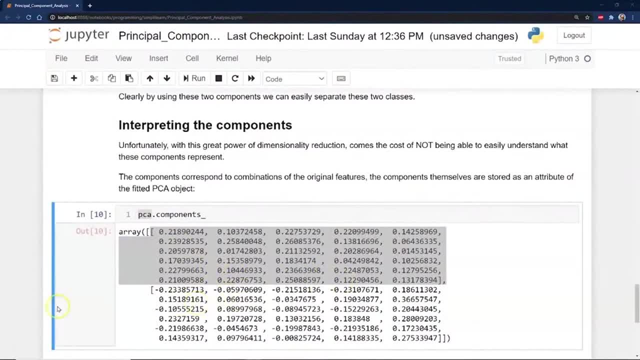 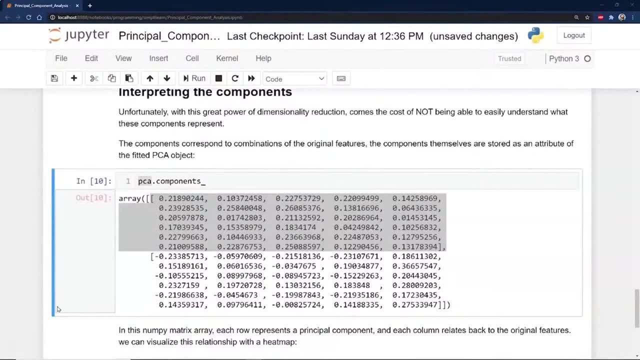 And these actually give weight to what features are doing what. So in this numpy matrix array, each row represents a principle component and each column relates back to the original features. What's really neat about this is we can now go in reverse. 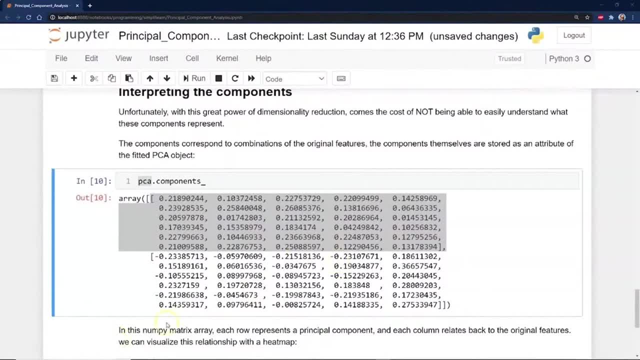 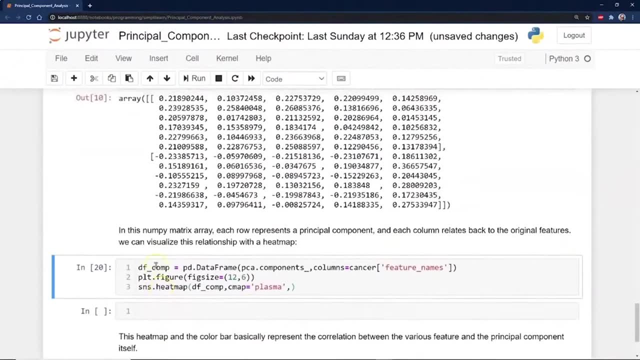 and drop this onto a heat map and start seeing what this means. And so let me go ahead and just put this down. I already got it down here. We go ahead and put this in here. We're going to use our 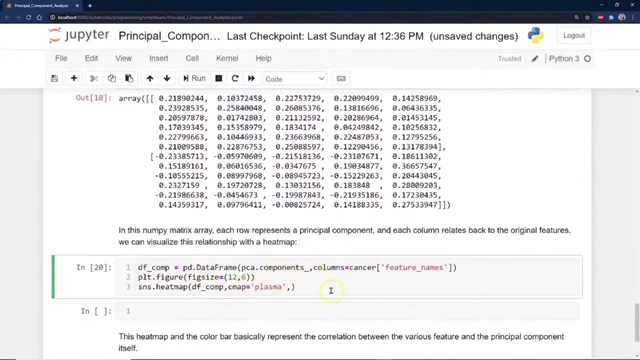 dfcomp data frame and we do our PCA components. And I want you to notice how easy this is. We're going to set our columns equal to cancer feature names. That just makes it really easy. And we're dumping it into a data frame. 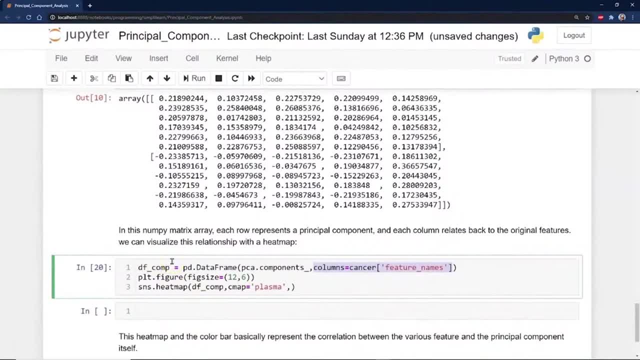 What's neat about a data frame is when we get to seaborn, it will pull that data frame apart and set it up for us what we want, And so we're just going to do the seaborn heat map of our data frame composition. 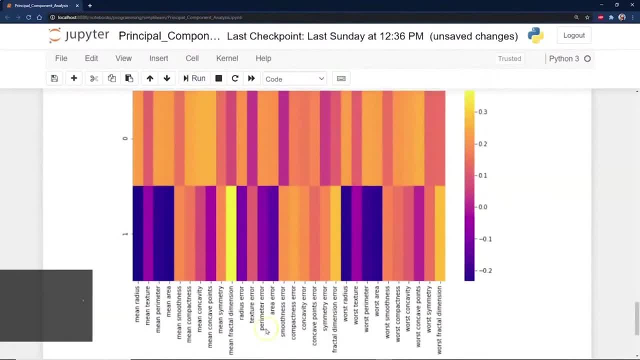 and we'll use the plasma coloring And it creates a nice little color graph. here You can see we have the mean radius and all the different features. along the bottom On the right we have a scale, So we can see we have the dark colors. 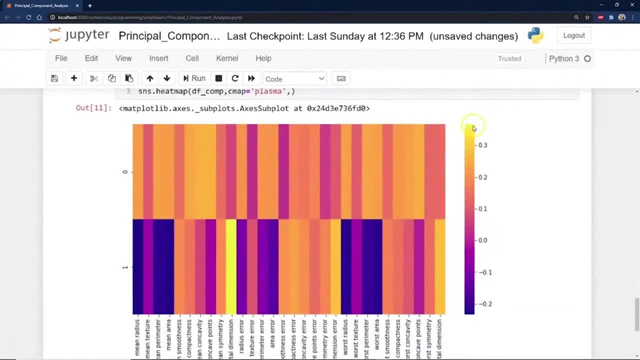 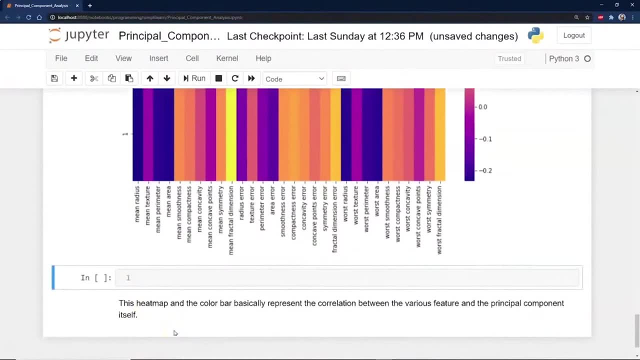 all the way to the really light colors which are what's really shining there. This is like the primary stuff we want to look at. So this heat map and the color bar basically represent the correlation between the various features and the principal component itself. 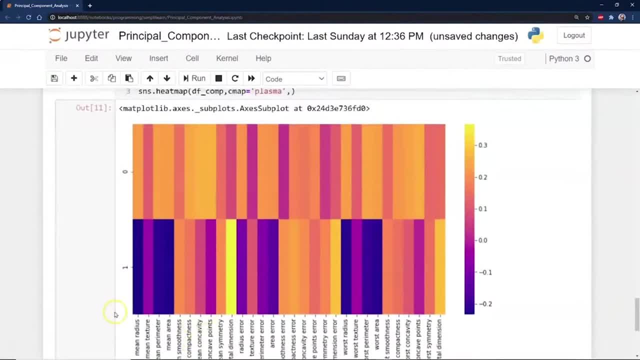 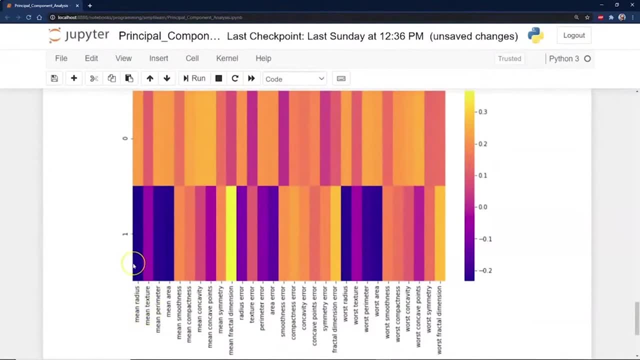 So you know very powerful map to look at And then you can go in here and we might notice that the mean radius. look how on the bottom of the map it is on some of this. So you have some interesting correlations here. 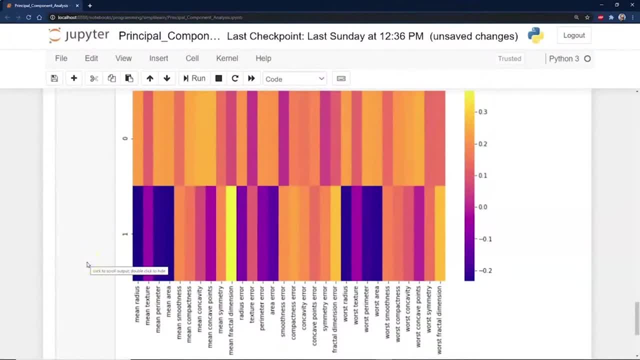 that change the variations on that and what means what? This is more, when you get to postscribe, you can also use this to try to guess, as what these things mean, what you want to change to get a better result. Regularization in machine learning. 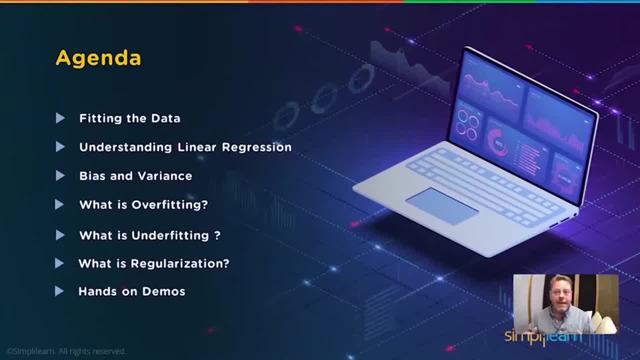 So our agenda on this one is fitting the data: understanding, linear regression, bias and variance. what is overfitting, what is underfitting- and those are like the biggest things right now in data science- is overfitting and underfitting. 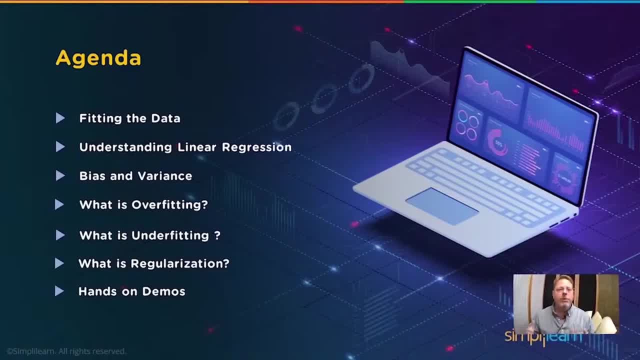 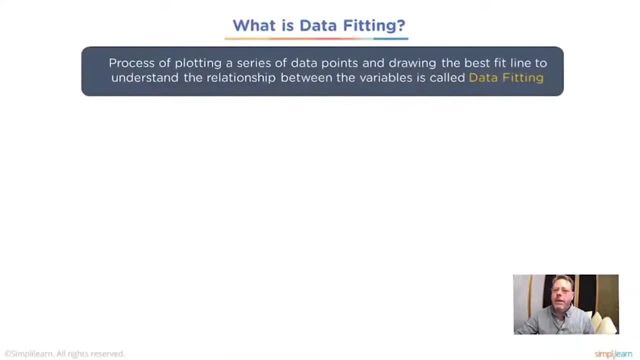 What does that mean And what is regularization? And then we'll do a quick hands-on demo to take a look at this. So, fitting the data. Let's start with fitting the data, And we talk about what is data fitting? It's a process of plotting a series of data points. 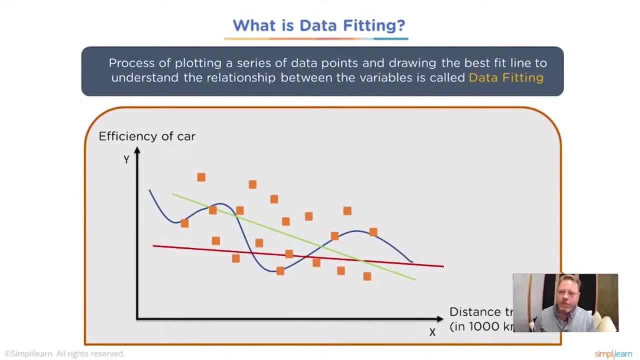 and drawing the best fit line to understand the relationship between the variables. And this is what we call data fitting. And you can see here we have a couple of lines we've drawn on this graph. We're going to go in a little deeper on there. 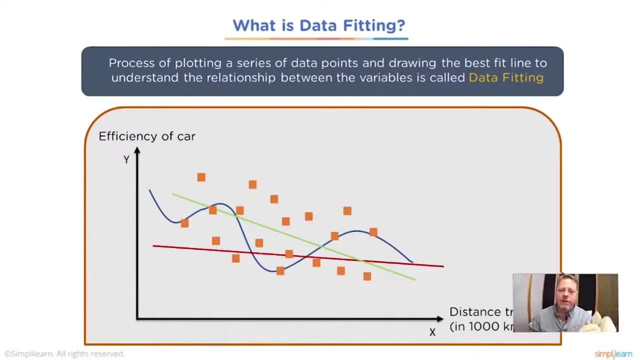 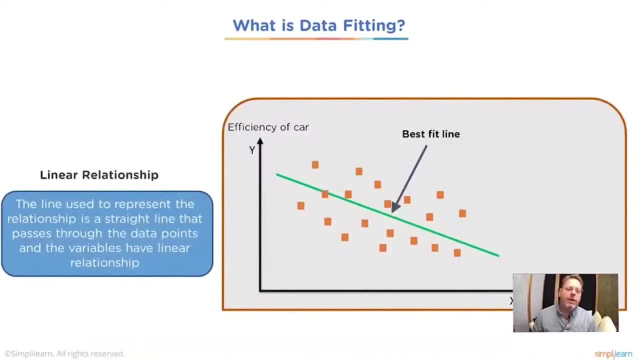 So we might have, in this case, just the two dimensions. We have an efficiency of the car and we have the distance traveled in 1,000 kilometers. And so what is data fitting? Well, it's a linear relationship And a linear relationship. 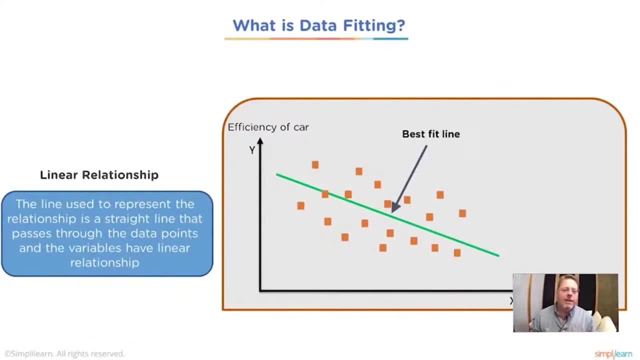 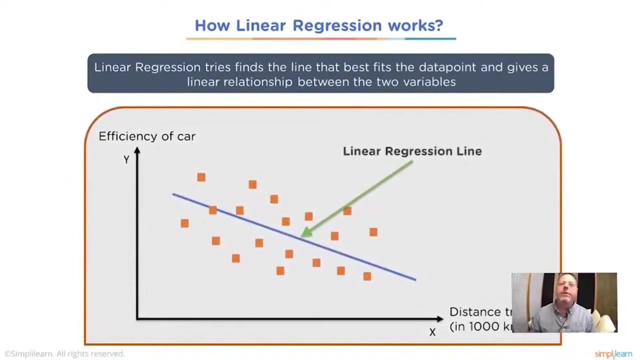 very specifically, linear means line. The line used to represent the relationship is a straight line that passes through the data points, and the variables have a linear relationship, Linear regression. So let's start with how linear regression works. A linear regression finds a line that best fits the data point. 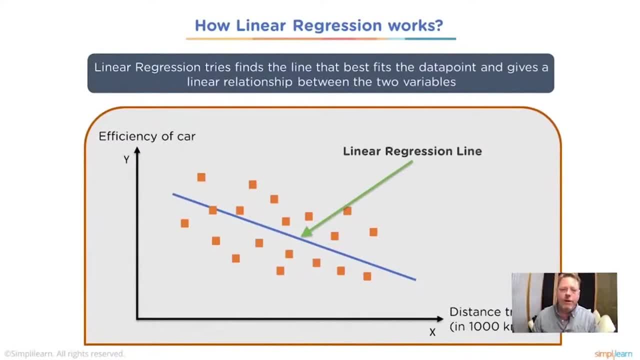 and gives a relationship between the two variables, And so you can see, here we have the efficiency of the car versus the distance traveled, And you can see this nice straight line drawn through there. And when you talk about multiple variables, all you're doing is putting this: 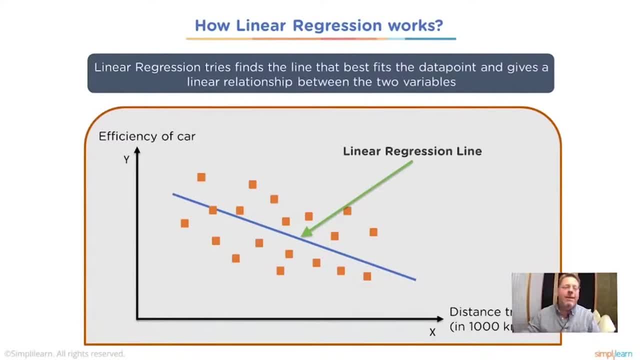 instead of a line it now becomes a plane. It gets a little more complicated with multiple variables, but they all come down to this linear kind of drawing a line through your data and finding what fits the data the best, And so we can consider an example. 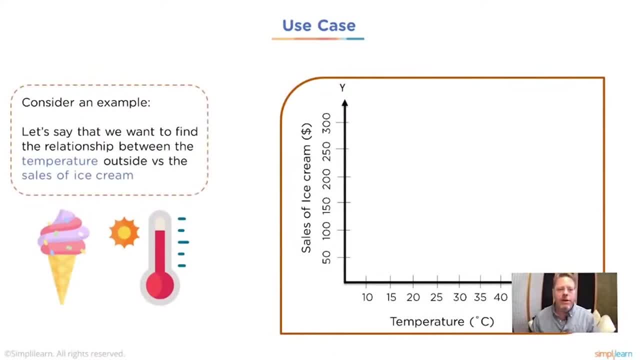 Let's say that we want to find the relationship between the temperature outside versus the sales of ice cream, And so we start looking at that. We're looking at how many ice cream cones we're selling or how much money we sold on ice cream. 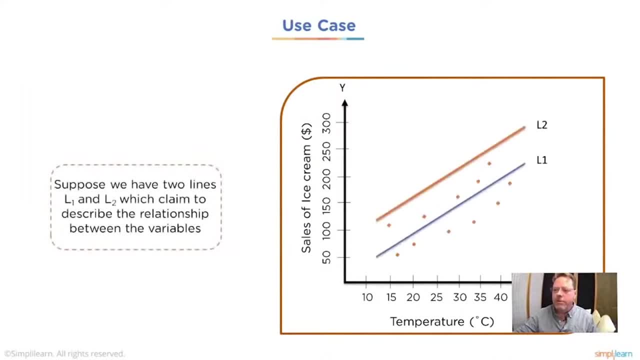 And we're looking at how warm it is outside, which would hopefully draw a lot of people into the ice cream store, And suppose we have two lines. We're going to draw L1 and L2. And we're going to kind of guess which one we think is the best fit. 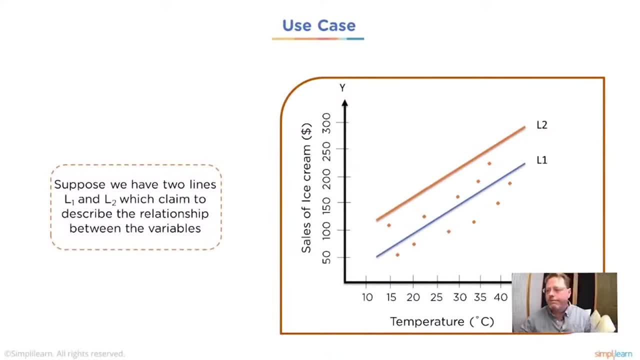 which claim to describe the relationship between the variables. And so first we find the square of the distance between the line L1 and each data point and add them all and find the mean distance. And I want you to think about that when we square something. 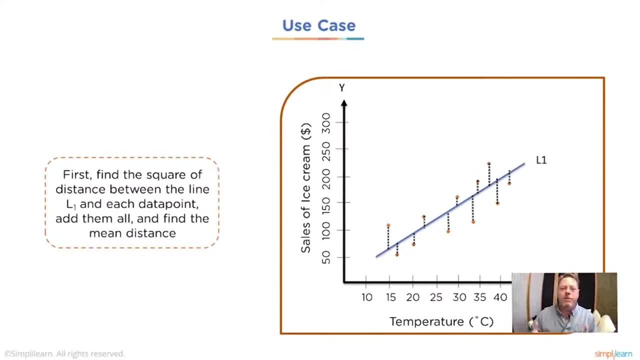 If it's a negative or positive number, it no longer matters, because a minus 2 squared is 4.. 2 squared is 4.. So we're removing what side of the line it's on, and we're just looking for the error. 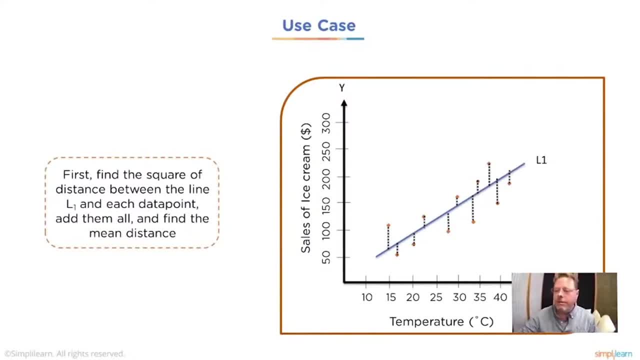 In this case the mean distance of each of the little dotted lines you see here. This way of calculating the square of the distance, adding them and then taking the mean, is called mean square, error or loss function, And we talk about loss. 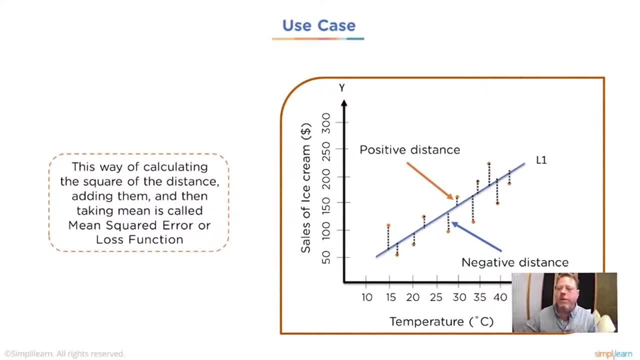 How far off are we? That's what we're really talking about. What did we miss? And we have a positive distance and a negative distance And, of course, when we square it, neither of it just becomes a positive error, And so we take the mean square error. 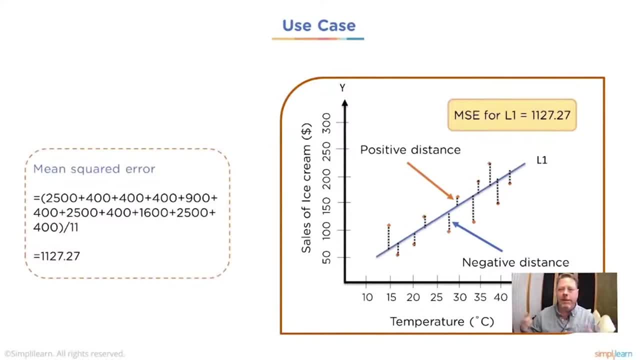 and a lot of times you'll see it referred to as MSE. If I look in a code and I'm going through my Python code and I see MSE, I know that's the mean squared error And we take all the dotted lines and we calculate this error. 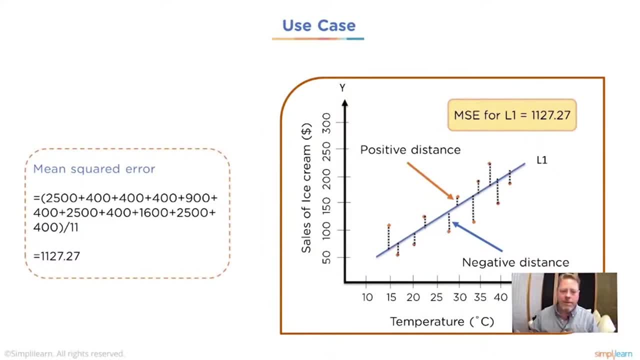 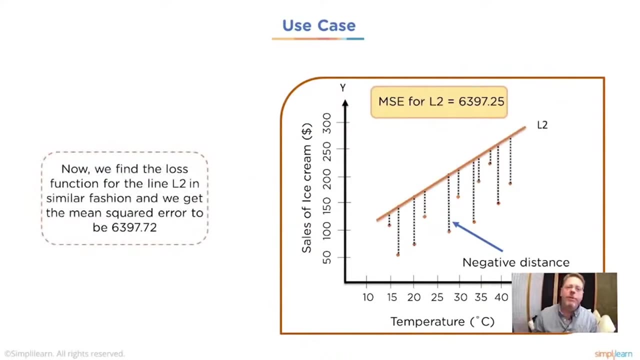 and we add them all together and then we average it or find the means, And in this case they ran a demo on this and it was 1,127 points. So that's 1.27 for our L1 line. Now we find the loss function for line L2 in a similar fashion. 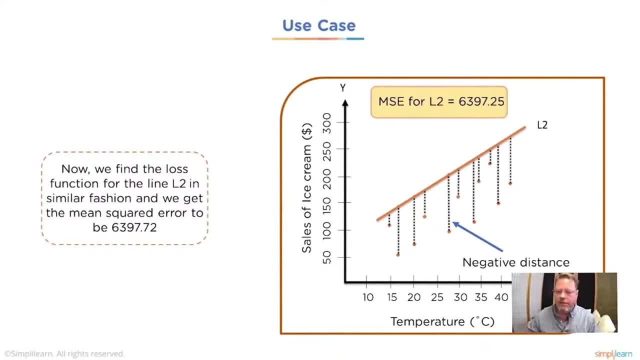 And we get the mean square error to be 6,397.. And it's computed the same way. So maybe you put this line just way outside the data range and this is the error you get. By analyzing our results, we find that the loss function. 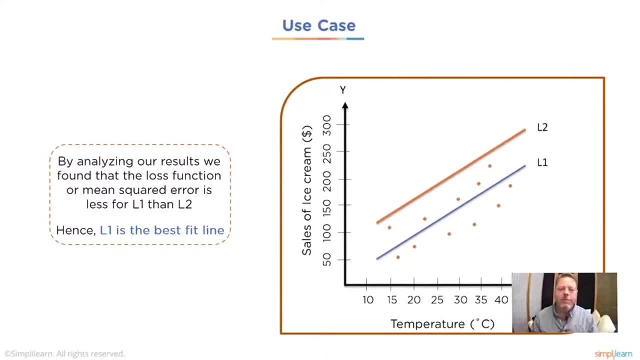 or the mean square error is less for L1 than L2. Hence L1 is the best fit line. This process describes a lot of machine learning processes. We're going to keep guessing and get as close as we can to find the right answer. 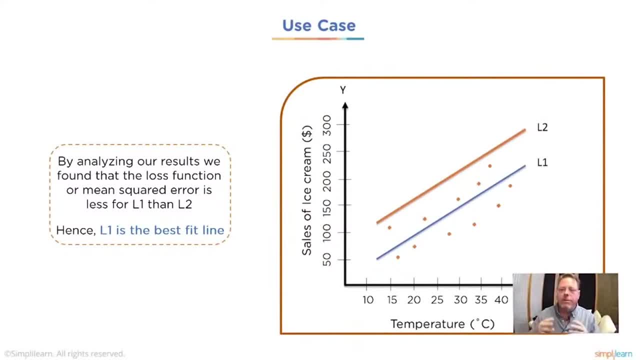 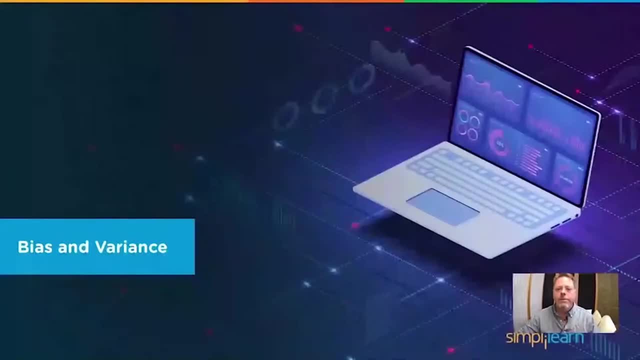 We have to have some way to calculate this and figure out which one is the best, And the mean square error is one of the better fits for doing this and most commonly used. We really want to talk about bias and variance. These are important terms to know in machine learning. 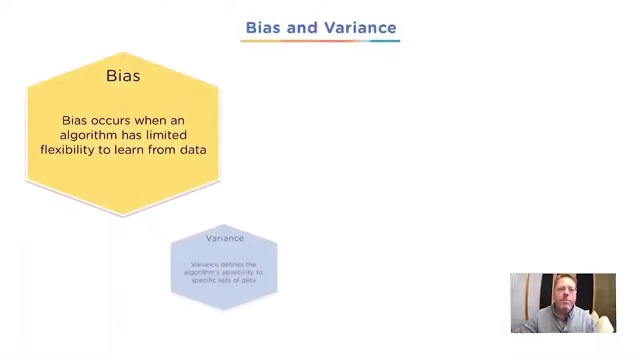 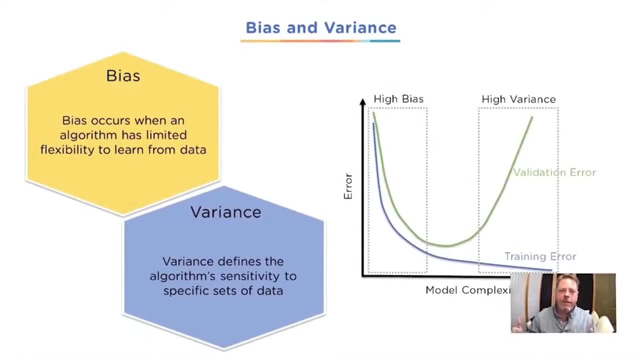 and with linear regression. So bias: Bias occurs when an algorithm has limited flexibility to learn from data. Variance defines the algorithm's sensitivity to specific sets of data. Let's start with bias and variance. You can see here we have the two different setups. 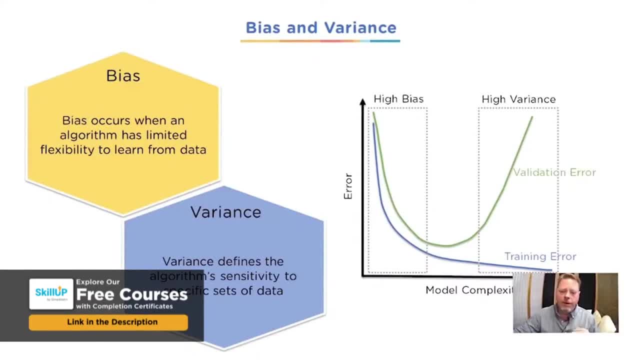 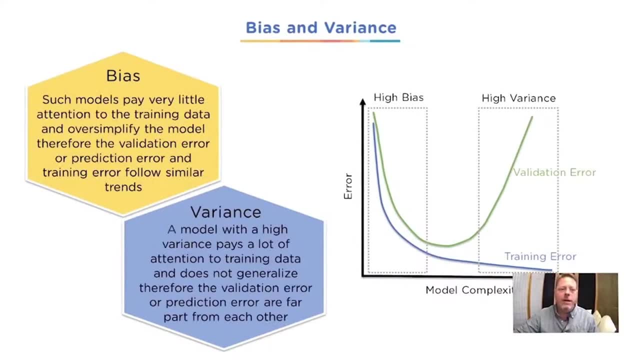 Bias you can think is very generalized, Where variance is very specific, And so when we talk about bias, such models pay very little attention to the training data and oversimplify the model. Therefore, the validation error or prediction error and training error follow similar trends. 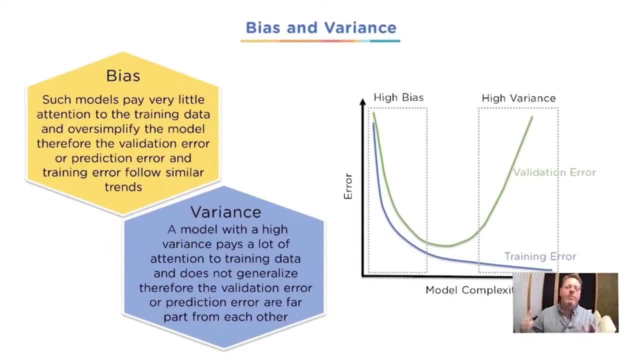 And with bias. if you oversimplify it so much, you're going to miss your local. if you have a really good fit, you're going to miss it. You're going to just kind of guess what the average is and that's what your answer is going to be. 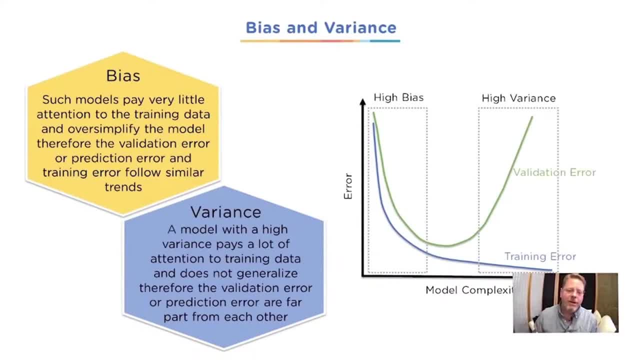 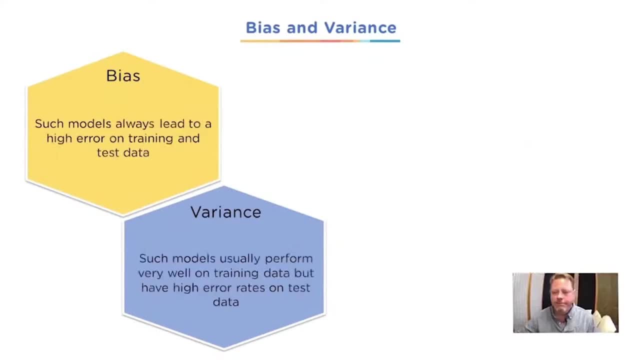 With variance. a model with a high variance pays a lot of attention to training data and does not generalize. Therefore, the validation error or prediction error are far apart from each other. Such models always lead to a high error on training and test data, as a bias does. 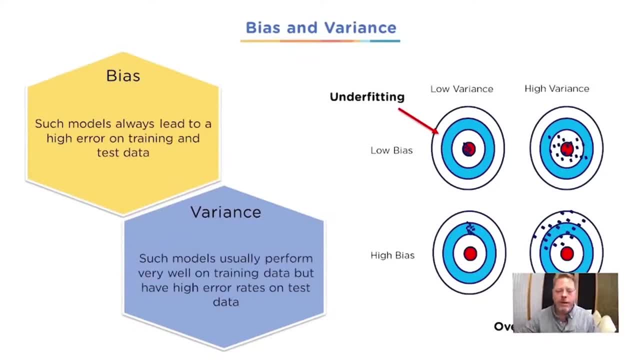 Where variance. such models usually perform very well on training data, but have high error rates on test data, And I want you to think about this: When we're talking about a bias, the error is going to be high both when you're training it and you're testing it. 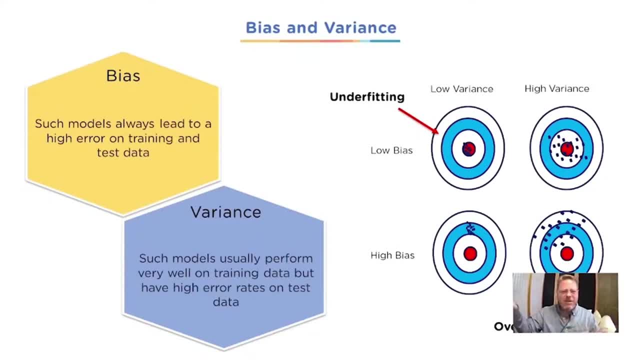 Why? Because we're just kind of getting an average. We're not really fitting it close With variance. we're fitting it so close that the test data does really good. It's going to nail it every time If you're doing categorical testing. 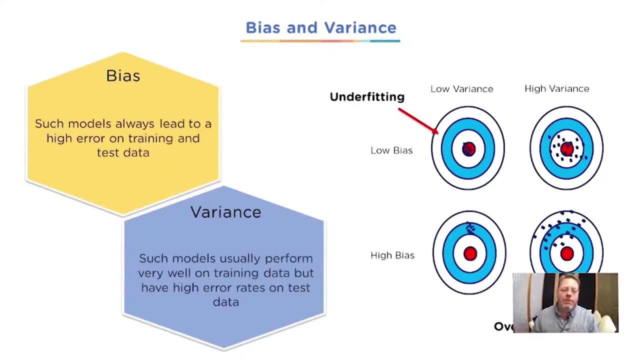 that's a car, that's a truck, that's a bicycle, But with variance. suddenly a truck has to have certain features and it might have to be red, because you had so many red pictures. So if it's an 18-wheeler, it has to be red. 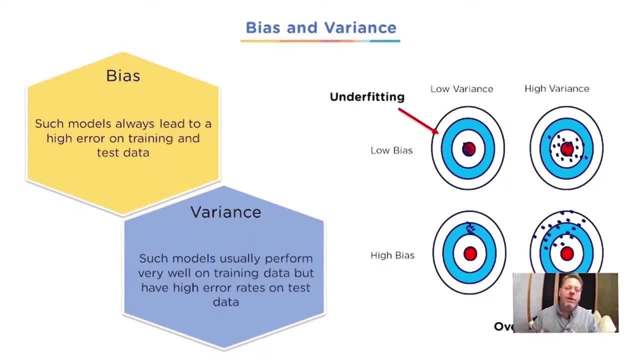 If it's blue, then it has to be a bicycle. That's the kind of variance we're talking about, where it picks up on something and it cannot get the right answer unless it gets a very specific data. And we see that so that, as you're testing it in your models, 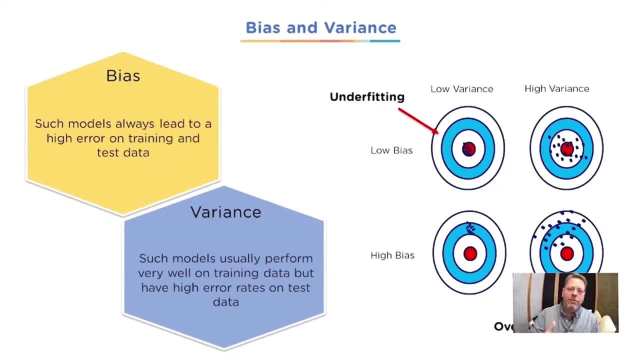 and you've programmed it. you've got to look for how I trained it, what is coming out, and if it's not looking good on either bias or if it's not looking good on the training or on the test data, then you're biasing your data. 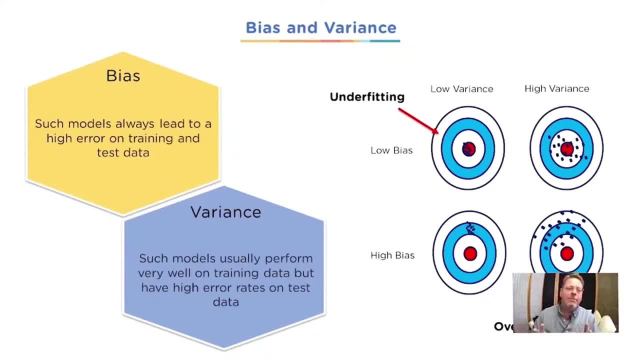 If it really looks good on the training data, then that's going to be your variance. You've overfitted the data, And those are very important things to know when you are building your models in regression of any kind or any kind of setup for predicting. 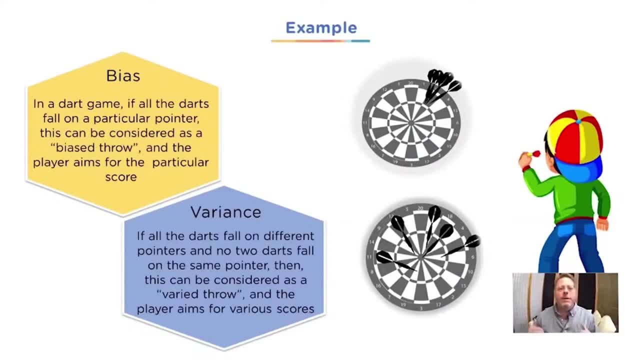 So in dart games, if all the data fall on a particular pointer, this can be considered as a biased throw and the player aims for the particular score For variance if all the darts fall on different pointers and no two darts fall on the same pointer. 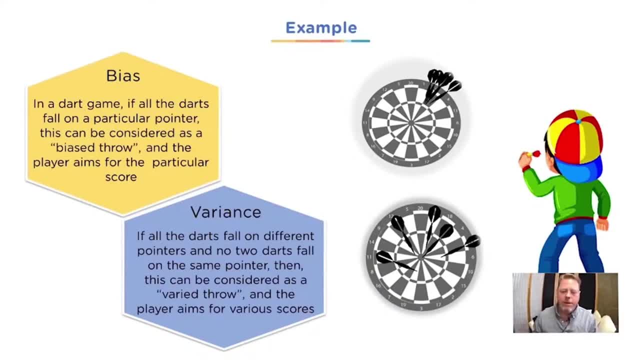 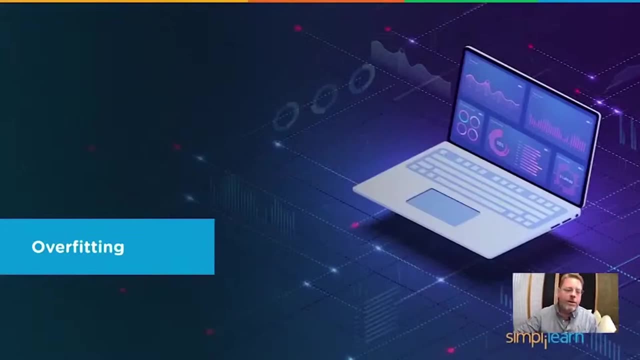 then this can be considered as a varied throw and the player aims for various scores. Again, the bias sums everything up in one point, kind of averages it together, where the variance really looks for the individual predictions coming out. So let's go ahead and talk about overfitting. 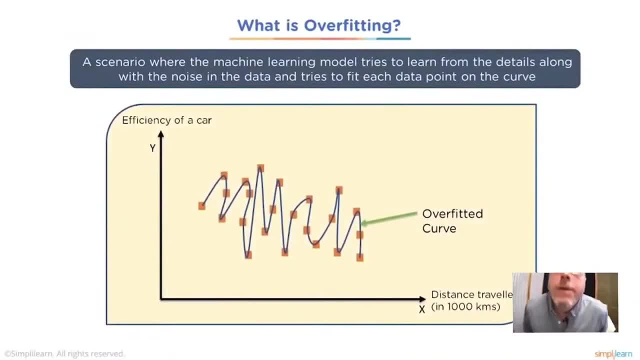 When we talk about overfitting, it's a scenario where the machine learning model tries to learn from the details, along with the noise and the data, tries to fit each data point on the curve. You can see that if you plug in your coordinates. 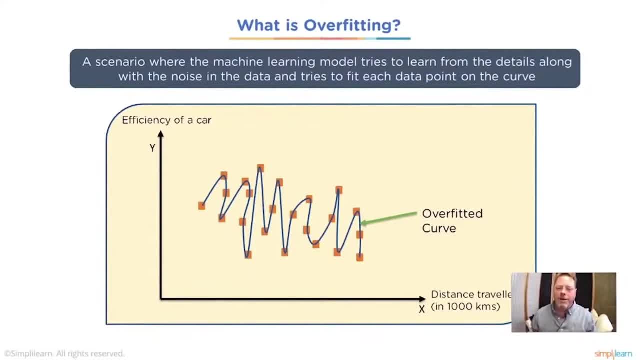 you're just going to get the whatever is fitted, every point on the data stream. There's no average, There's no two points that might have the. you know you have two different answers because if the wind blows a certain way and the efficiency of your car, 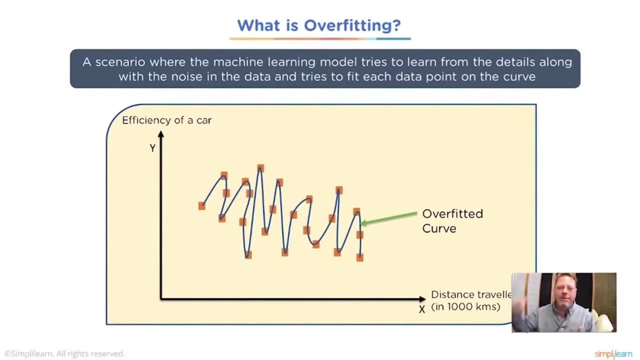 maybe you have a headwind, so your car might alter how efficient it is as it goes, And so there's going to be this variance on here and this says no, you can't have any variance with. you know, it's going to be exactly this. 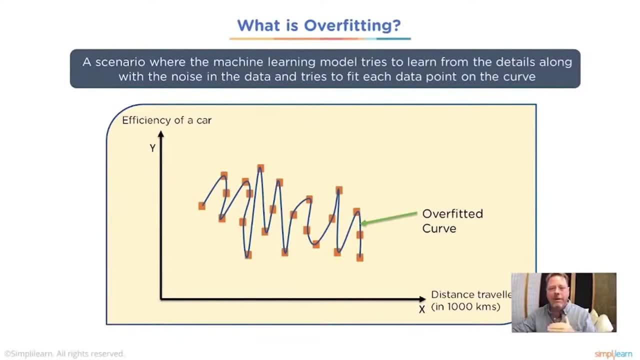 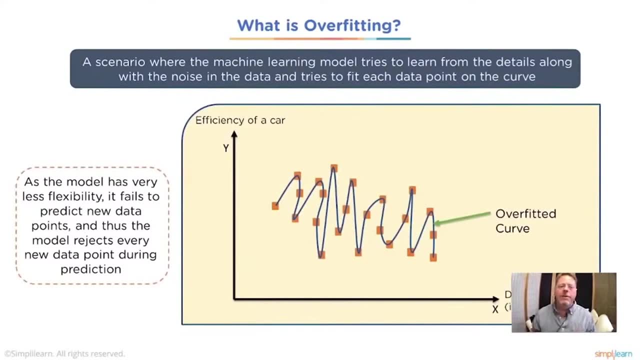 You can't be the same speed or the same car and have a slightly different efficiency. So as the model has very less flexibility, it fails to predict new data points and thus the model rejects every new data point during the prediction. So you'll get like a really high error on here. 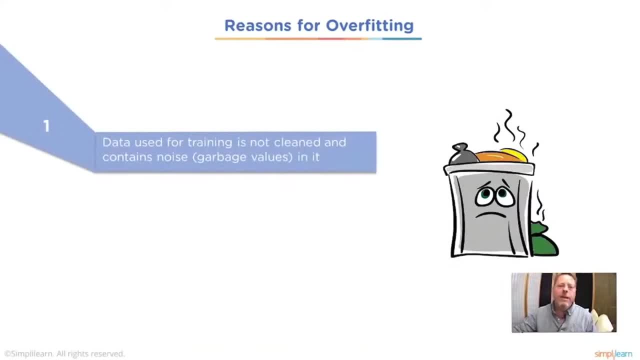 And so reasons for overfitting. Data used for training is not cleaned and contains noise garbage values in it. You can spend so much time cleaning your data and it's so important. It's so important that if you have, if you have some kind of 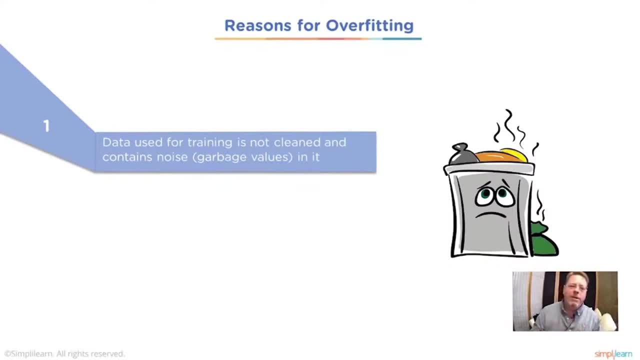 something wrong with the data coming in. it needs to be addressed whether it's the source of the data. maybe they use in medical different measuring tools, So you now have to adjust for data that came in from hospital A versus hospital B or even off of machine A and machine B. 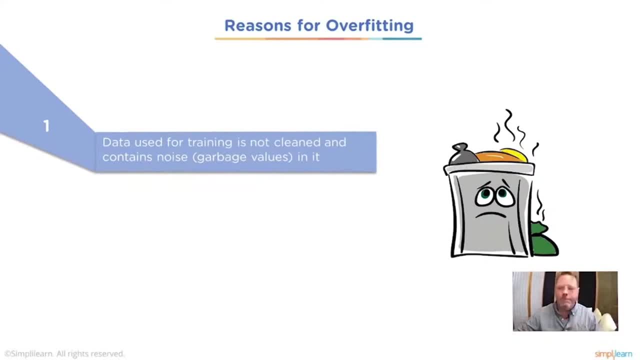 that's testing something and those numbers are coming in wrong. The model has a high variance. Again, wind is a good example. I was talking about that with the car. You may have a hundred tests, but because the wind's blowing, it's all over the place. 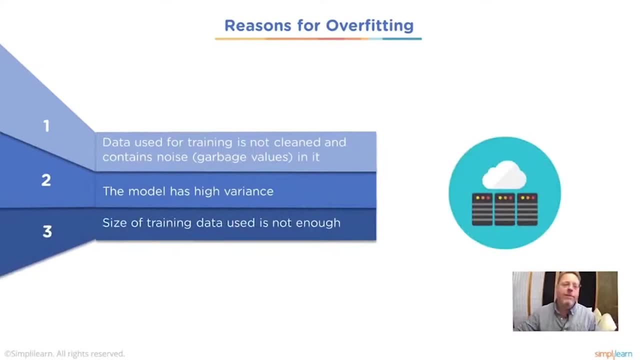 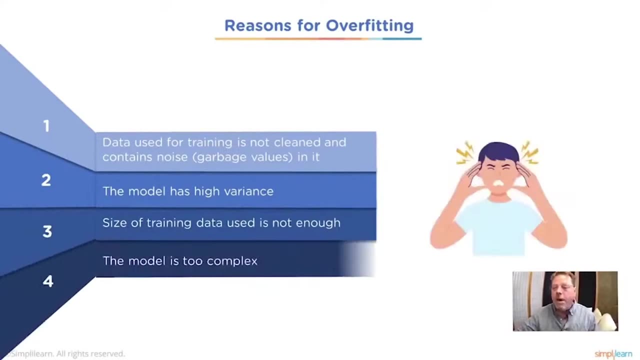 Size of training data used is not enough, So a small amount of data is going to also cause this problem. You only have a few points and you try to plot everything. The model is too complex. This comes up a lot. We put too many pieces together. 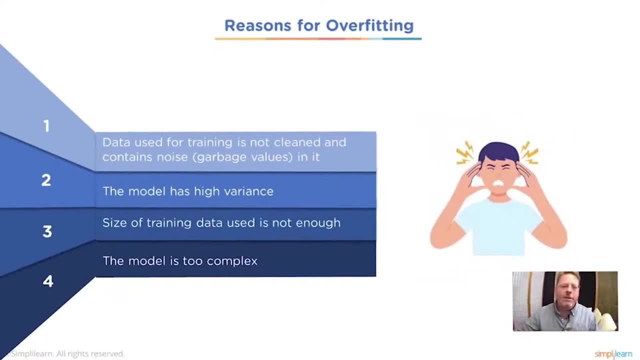 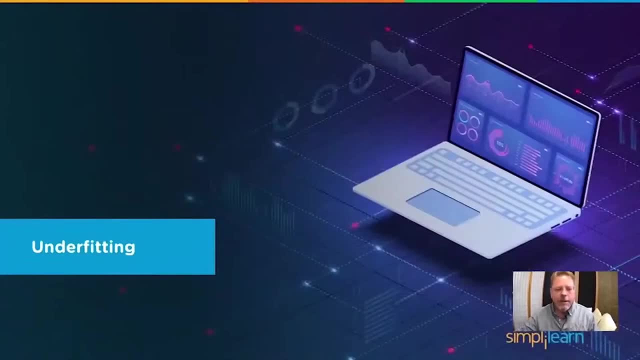 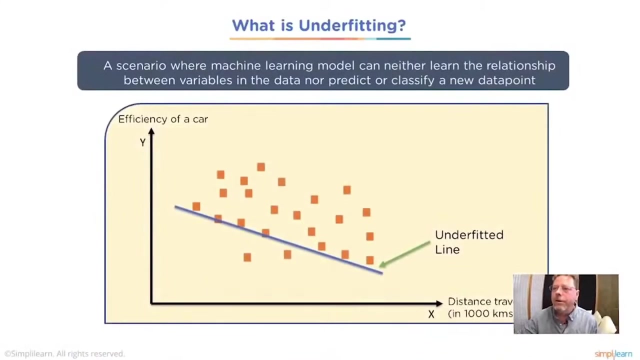 and how they interact can't even be tracked, And so you have to go back, break it up and find out actually what correlates and what doesn't. So what is underfitting A scenario where machine learning models can either learn the relationship between the data points? 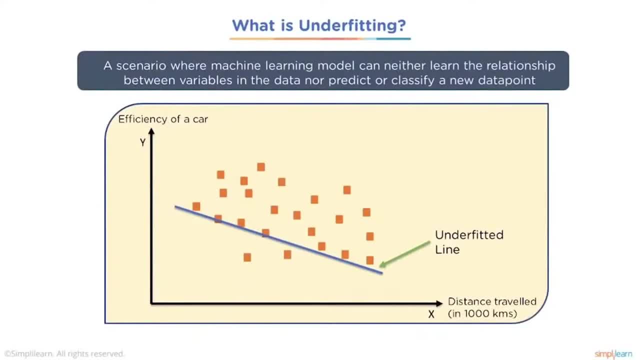 nor predict or classify a new data point. And you can see, here we have our efficiency of our car and our line drawn and it's just going to be way off for both the training and the predicting data, As the model doesn't fully learn the patterns. 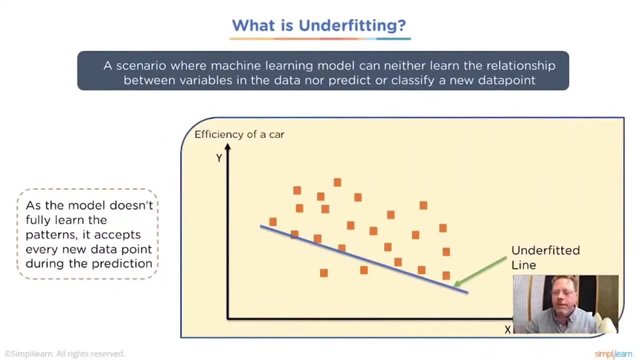 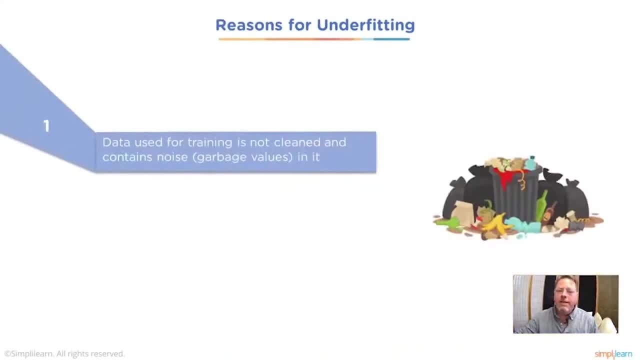 it accepts every new data point during the prediction. So instead of looking for a general pattern, we just kind of accept everything. Data used for training is not cleaned and contains noise, garbage and values- Again underfitting and overfitting same issue. 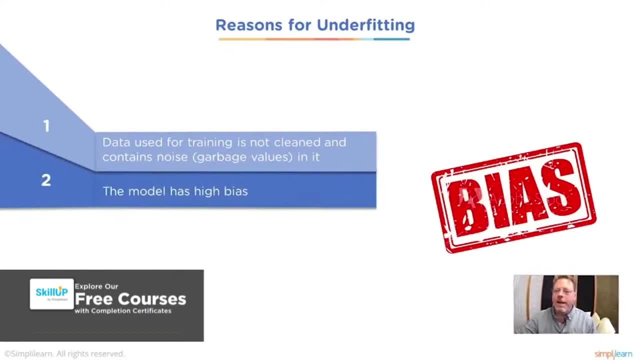 You've got to clean your data. The model has a high bias. We've seen this in all kinds of things, from the most common is the driving cars to facial identification or whatever it is. The model itself, when they build it might have a bias towards one thing. 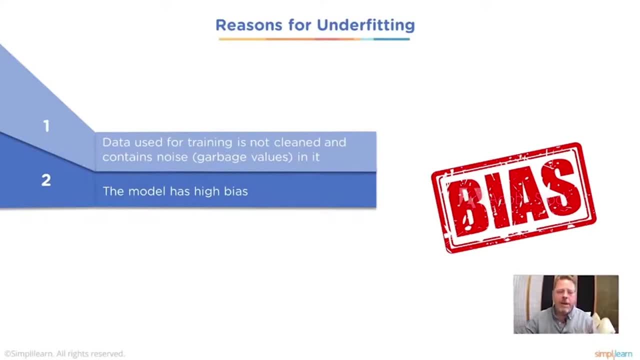 And this would be an underfitted model- would have that bias because it's averaged it out. So if you have five people from India and 10 people from Africa and 20 people from the US, you've created a bias because it's looking at the 20 people. 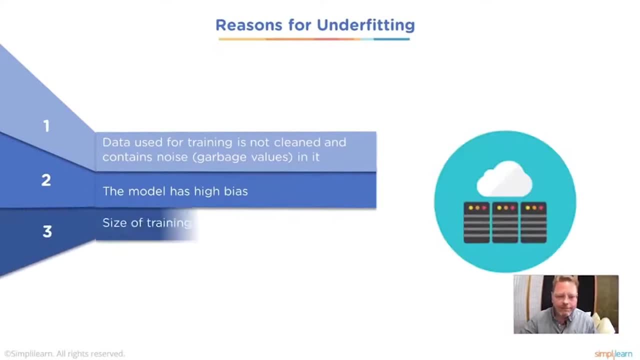 and you only have a small amount of data to work with. Size of training data used is not enough. That goes with the size I was just talking about. So we have a model with a high bias. We have size of training. data used is not enough. 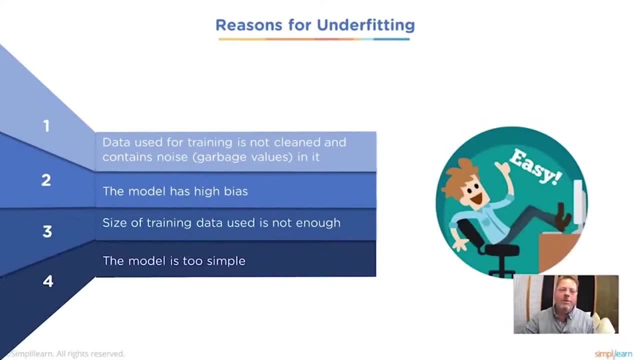 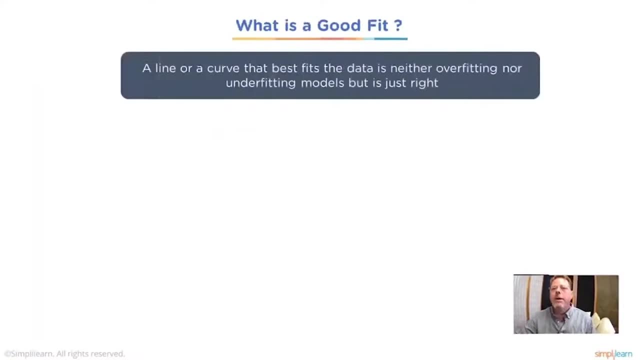 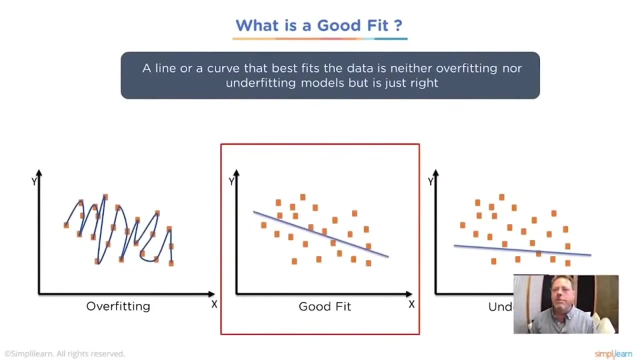 The model is too simple. Again, this is one straight line through all the data when it has a slight shift to it for other reasons. So what is a good fit? A linear curve that best fits the data is neither overfitting or underfitting models. 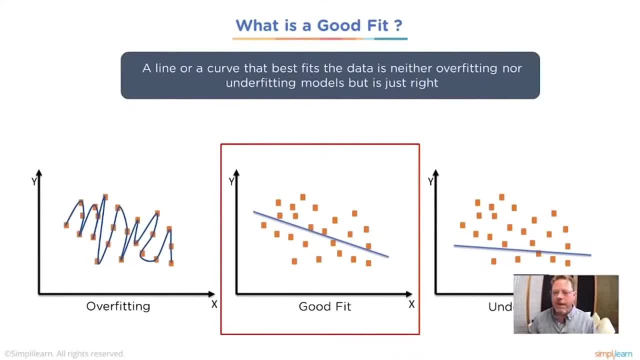 but is just right. And of course we have the nice examples here where we have overfitting lines going up and down. every point's trying to be included. underfitting the line really is off from where the data is and then a good fit is got to get rid of that. 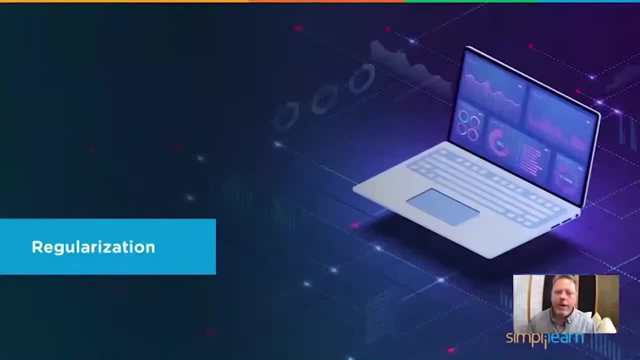 minimize that error coming through. Regularization is taking the guesswork out. You're looking at this graph and you're going, oh, which one? is that really overfit or is that underfit? That's pretty hard to tell. So we talk about regularization. 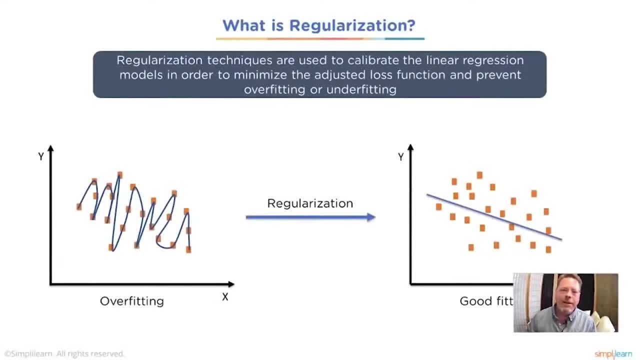 Regularization techniques are used to calibrate the linear regression models and to minimize the adjusted loss function and prevent overfitting or underfitting. So what that means in this case, we're going to go ahead and take a look at a couple different things. 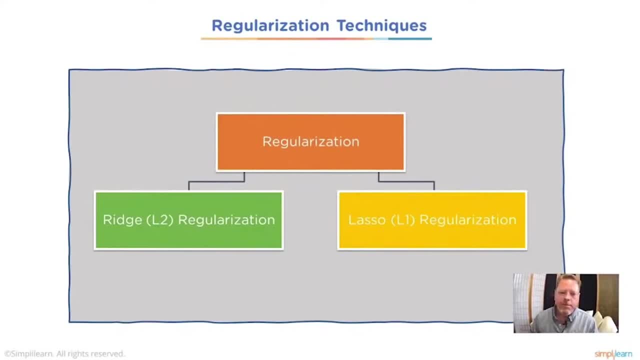 We're going to look at regularization, which we'll start with a linear model. We'll look at the ridge regularization and the lasso regularization And these models are just like, just like we did the MLP, the multi-layered positron in the sklearn module. 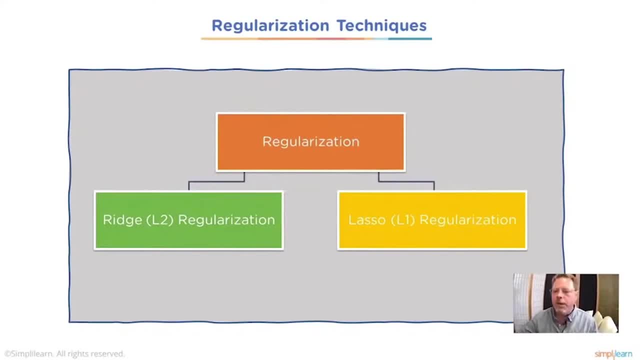 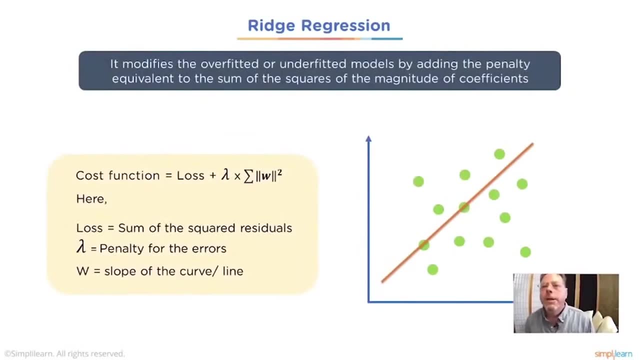 You could bring in the ridge module and you can bring in the lasso module. So when we talk about ridge regression, it modifies the overfitted or underfitted models by adding the penalty equivalent to the sum of the squares or the magnitude of the coefficients. 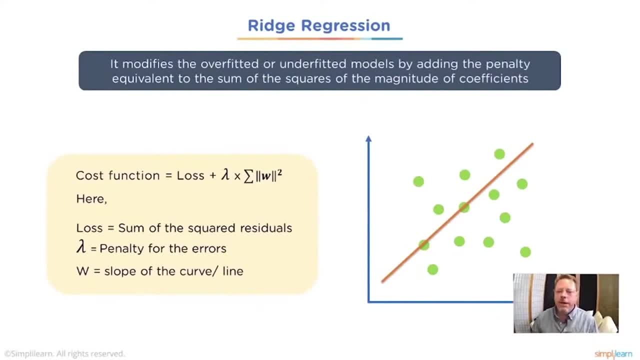 And so we have a cost function equals loss, equals lambda times the sum of w squared or the absolute value of w squared. So that's the absolute value, depending on how you're doing it. Now, remember we talked about error, whether we either square it or we absolute value it. 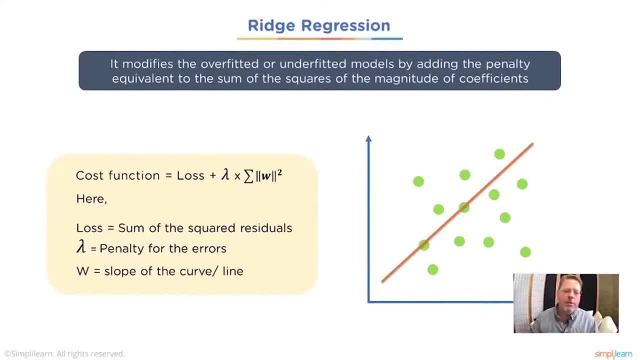 because that removes the plus or minus sign on there, And there's reasons to do it either way, but it is more common to square the value And then we have our. in this case, the lambda is going to be the penalty for the errors. 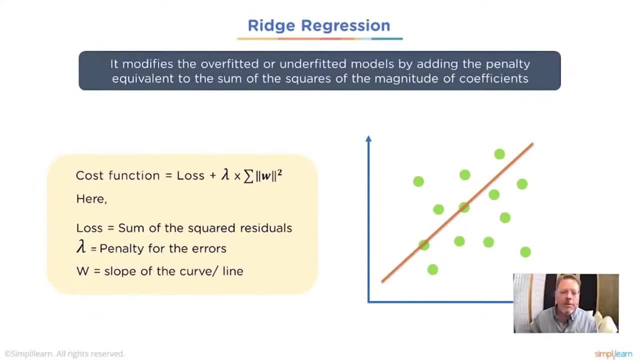 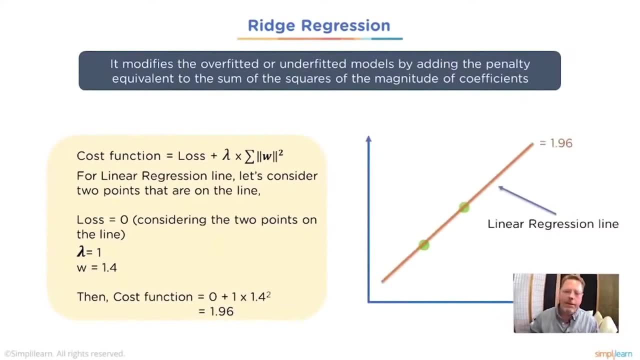 We've thrown in a Greek character for you just to confuse everybody. And w is the slope of the curve of the line. So we're going to look at this and this is going to be like a linear regression model. So if you had in sklearn- 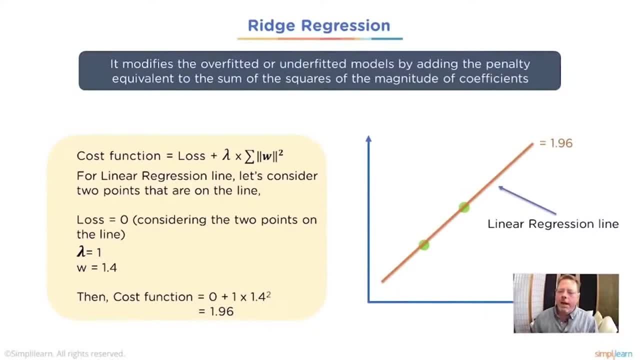 you could import just a standard linear regression model. It would plot this line across whatever data we're working on And we look at this and of course, we're just extrapolating this. I know they use some specific data, but don't want to get into the actual domain. 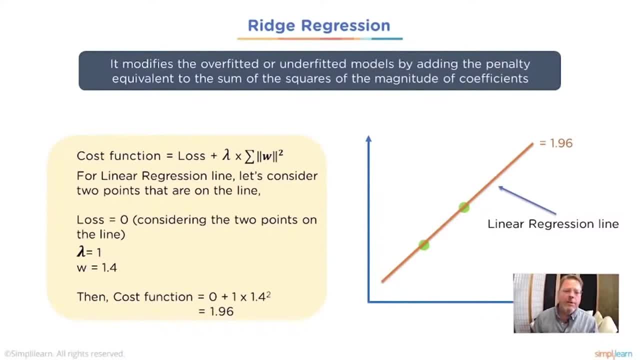 And so, for a linear regression line, let's consider two points that are on the line, And we'll go ahead and have a loss equals zero. considering the two points on the line, We'll go ahead and do lambda equals one. We'll set our w is going to be one point four. 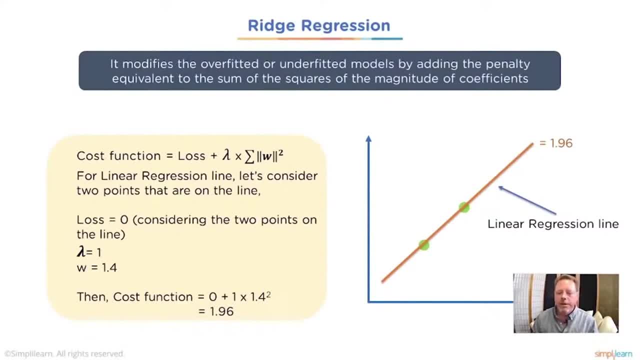 Then the cost function equals zero plus one times one point four squared, which equals one point nine six. So really don't get caught up too much in the math on this, other than understanding that this is something that's very easy for a computer to calculate. 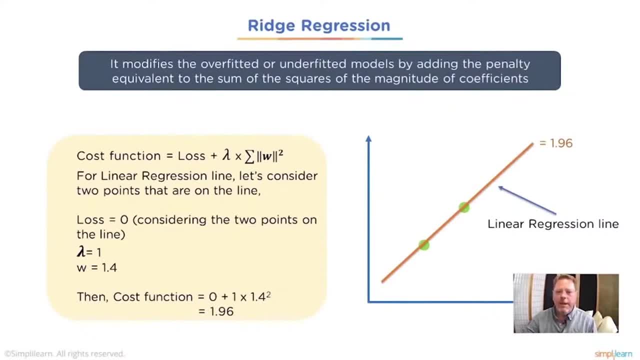 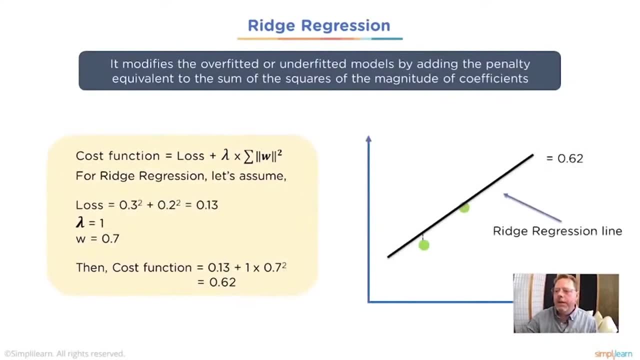 And if you ever see the loss plus the lambda times, the sum of w squared, the sum of w squared. And then let's say we have a ridge regression line and we go ahead and plot it and we do the calculations on the data And for the ridge regression, 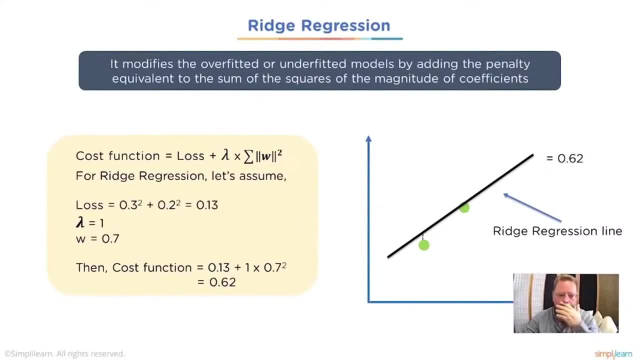 let's assume a loss equals point three squared plus point two squared equals point one three. So when we put all the calculations through of the two points, we end up with a point six two. So we've now had a linear regression model. We now had a ridge regression model. 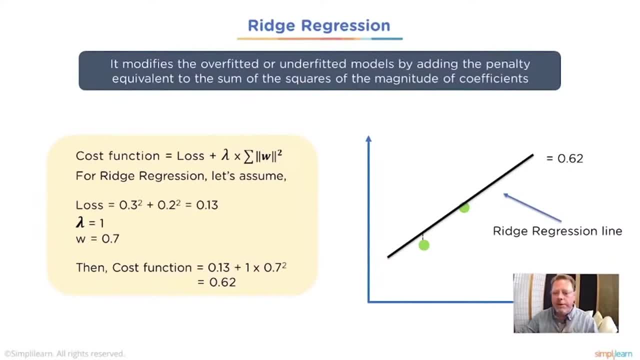 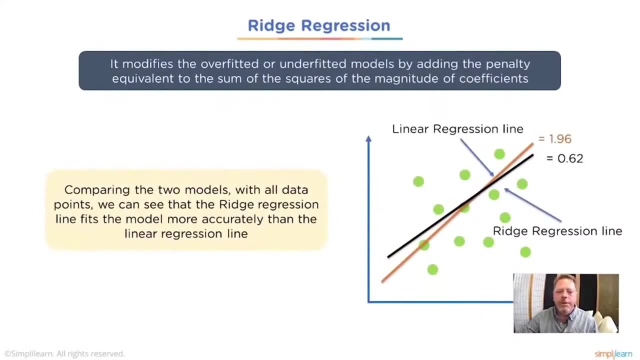 And the ridge regression model. it plots a little differently than the standard linear regression model And comparing the two models with all the data points, we can see that the ridge regression line fits the model more accurately than the linear regression line And I find this true on a lot of data I work with. 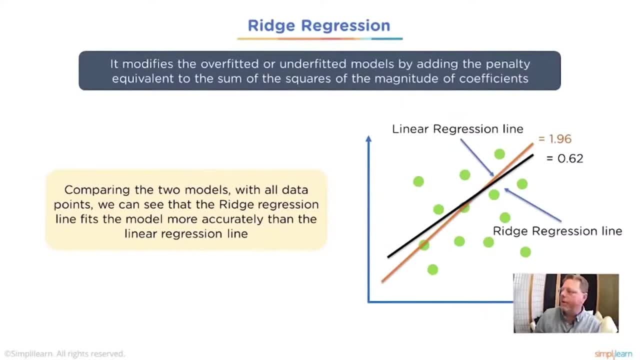 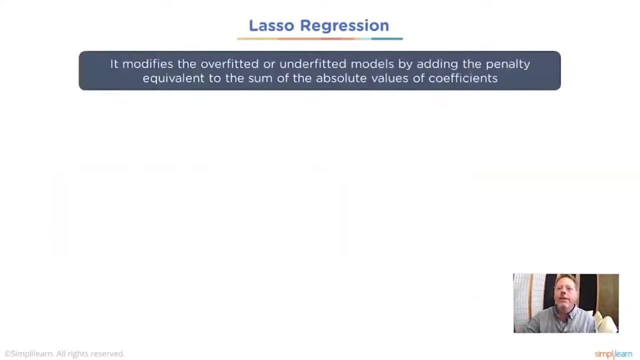 I'll end up using either the ridge regression model or the lasso MARS regression model for fitting, especially dealing with a lot of like stock markets, which is a little bit more expensive, And so we have our lasso. We just talked about lasso coming in here. 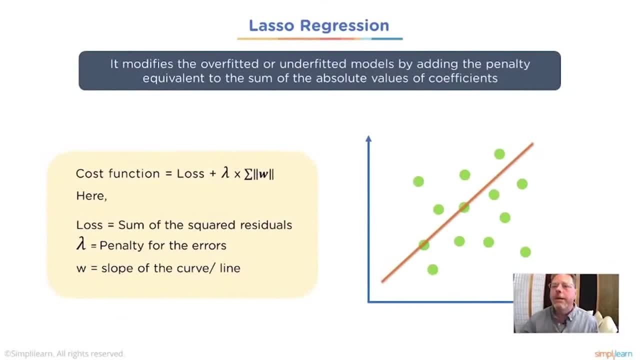 And the cost function equals. instead of doing a squared, we're just going to do the absolute value. And so, if you remember, this is where ridge regression changes. Where's my ridge regression model? We're squaring the value here, And if you look at this, 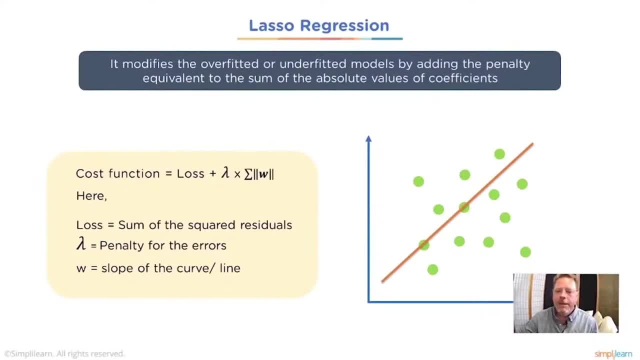 we're not squaring the value, We're just finding the absolute value. And so, if you remember, this is where ridge regression changes. We're squaring the value, We're just finding the absolute value on here, And so the loss of the squared individuals. 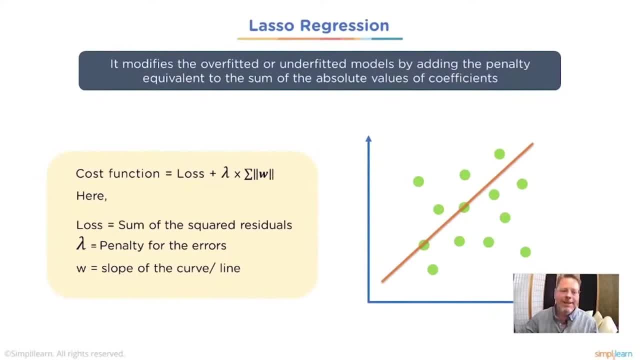 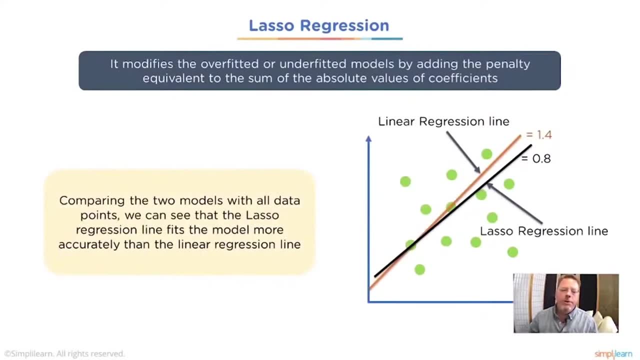 and here is our lambda symbol again: penalty for errors. and w equals the slope of the curve. And comparing the two models with all the data points, we can see that the lasso regression line fits the model more accurately than the linear regression line. 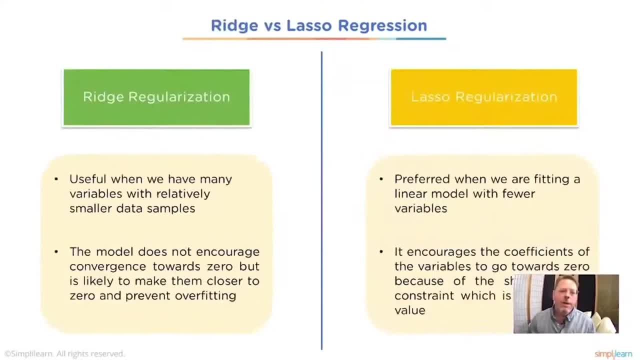 And this is like I said. I use these two models a lot: The ridge, and this is important. This is kind of the meat of the matter. How do you know which one to use? Some of it is. you just do it a bunch of times. 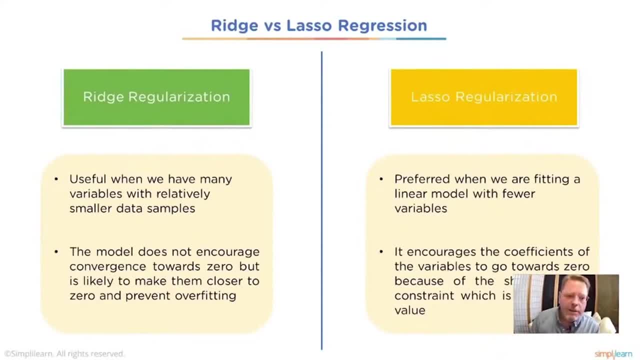 and then you figure it out. Ridge regularization is useful when we have many variables with relatively smaller data samples. The model does not encourage convergence towards zero, but is likely to make them closer to zero and prevent overfitting The Lasser regularization model. 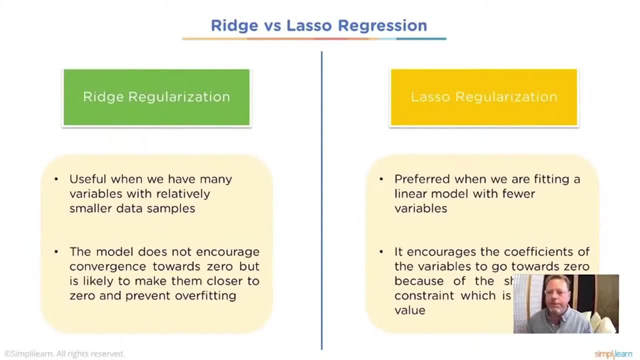 is preferred when we are fitting a linear model with fewer variables. So in the iris thing we had four or five variables as we measured the different leaf pieces. You might be doing the measurements on the cancer project which has 36 different variables. 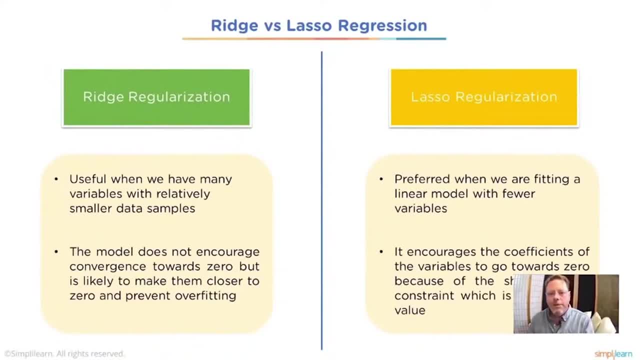 So, as we get down to the iris with four variables, lasso lar will probably work pretty good, where you might use the ridge regularization with more model if you have something significantly larger, And in this case it encourages the coefficients of the variables to go towards zero. 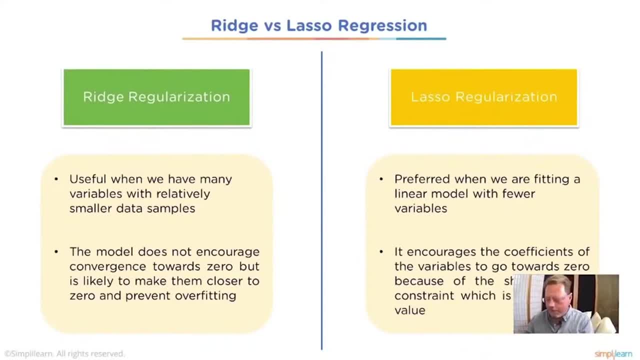 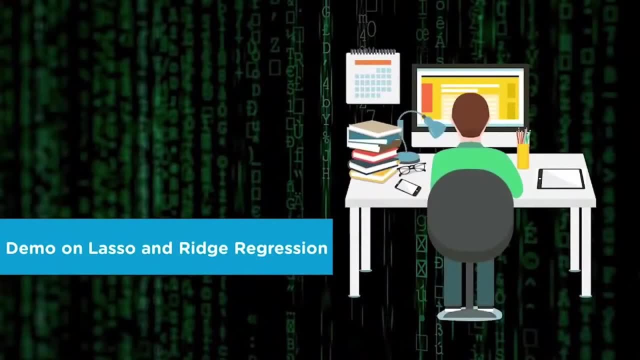 because of the shape of the constraint, which is an absolute value. And with any of this, we want to go ahead and do a demo in lasso and ridge regression. So let's take a look and see what that looks like in our code. 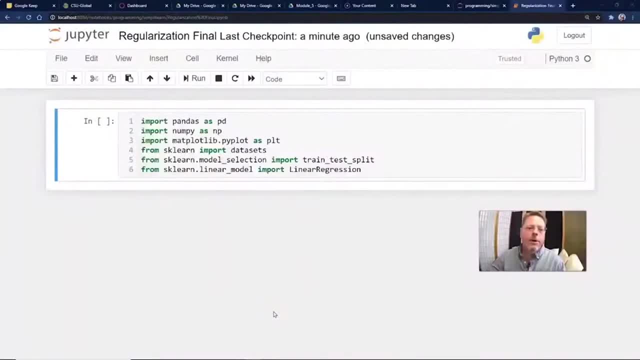 and bring up our Jupyter notebook. We'll start with our imports. Pandas is PD Import. numpy is NP Import. matplotlib is PLT. SKlearn- we're going to import our data sets. It's kind of more generic. We usually just import one data set. 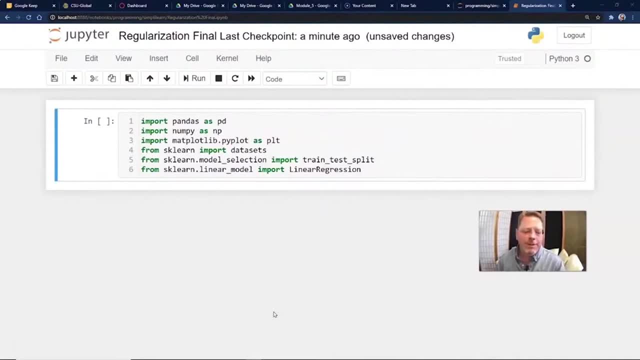 instead of all of them, but you know quick and dirty when you're putting some of these together. We have our SKlearn model selection. We're going to import our train test split for splitting our data up, And then we'll bring in our linear regression model. 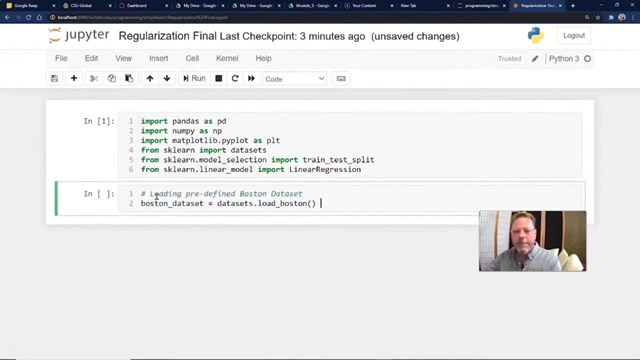 And we'll go ahead and run these just to load them up and then load our data set. We were just talking about that. You could just have imported the load Boston and Boston data set in there, instead of loading all the data sets And then, once we've loaded our data set. 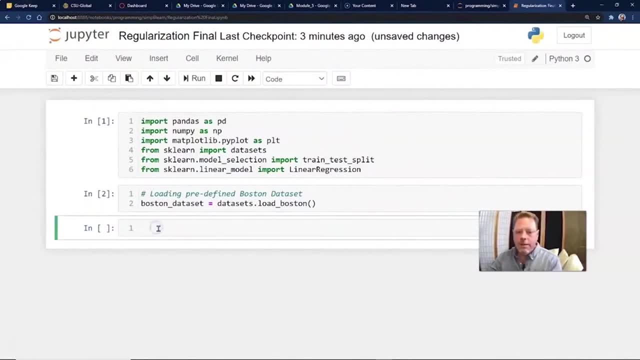 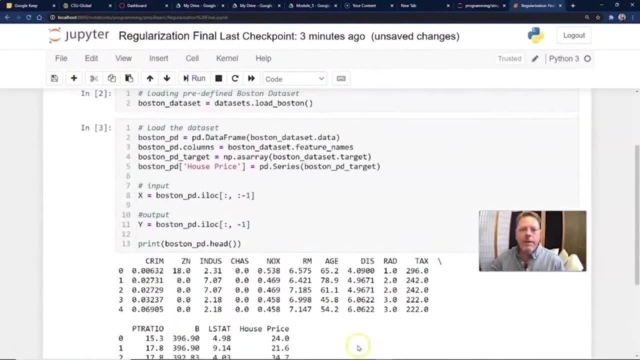 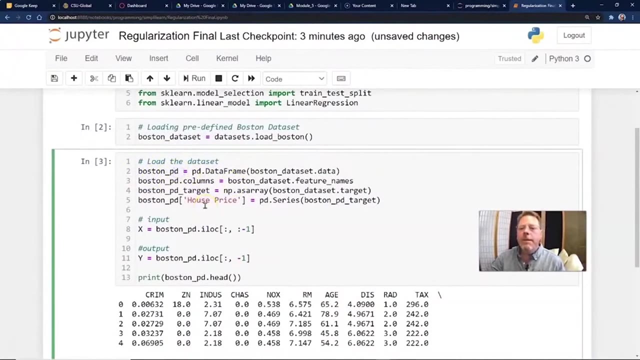 we want to go ahead and take a look at that data and see what we got here. Let me just go ahead and pop that down there and go ahead and run it. And so we've gone ahead and taken our Boston data. We put it into our Pandas data frame. 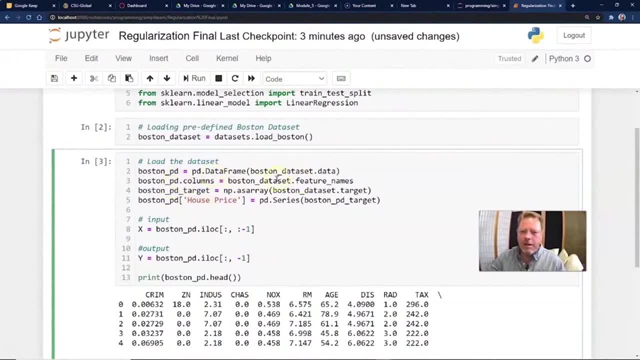 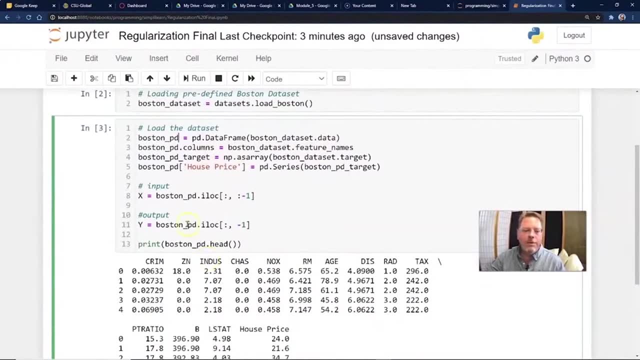 the Boston data set and then the Boston columns. So we want to see what's going on with them. We have our target, We have the house price, et cetera, And so our X equals Boston. I location Now, remember, in Pandas. 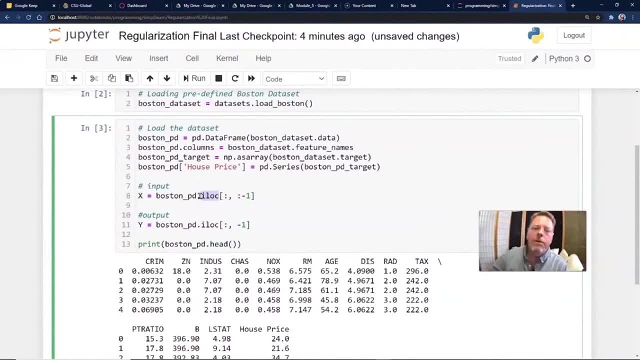 the new updates to Pandas. they want I location if you're going to pull data. We used to be able to leave this off, but it does something different. It creates a slice versus a direct setup, So make sure you're using that I location. 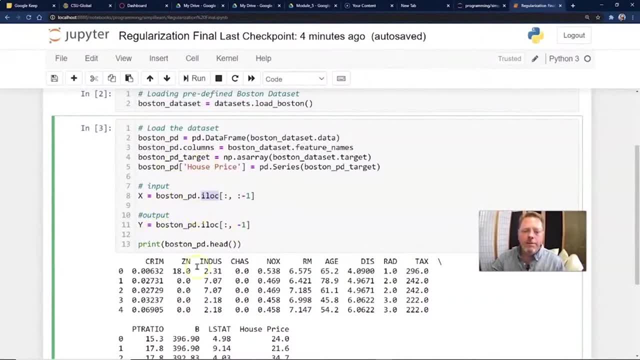 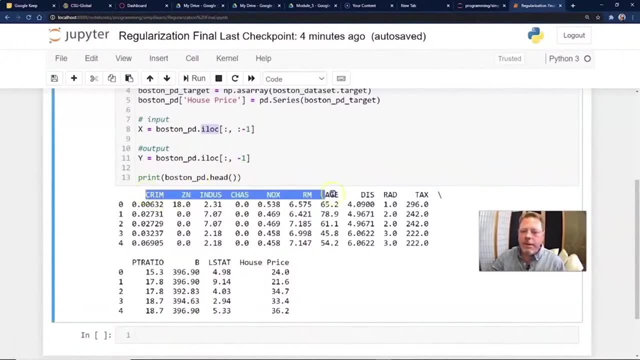 and the output. So this is all just bringing our data together And we can see here, if we do, we print the Boston Pandas head. we can see here all of our different aspects we're looking for And if you're following the X and the Y, 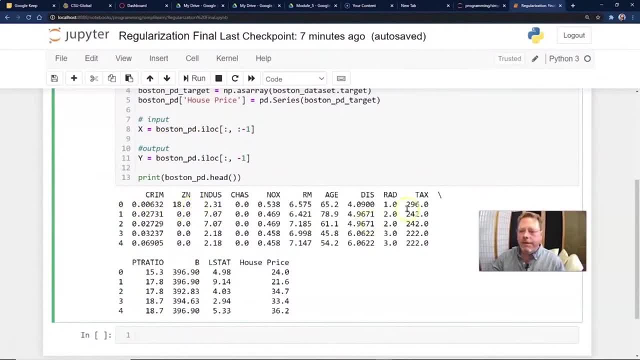 the X is everything except for the last column, where Y is all the. that's what this means: all the rows except for the last column. And then Y is all the rows but just the last column. So Y is our house price and the X is the CRIM. 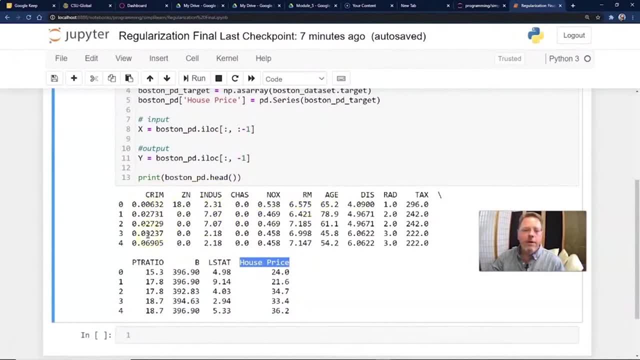 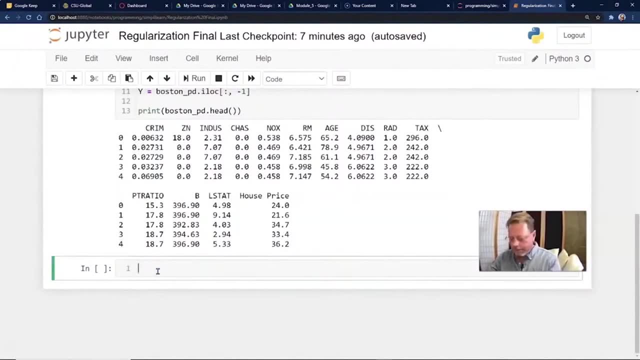 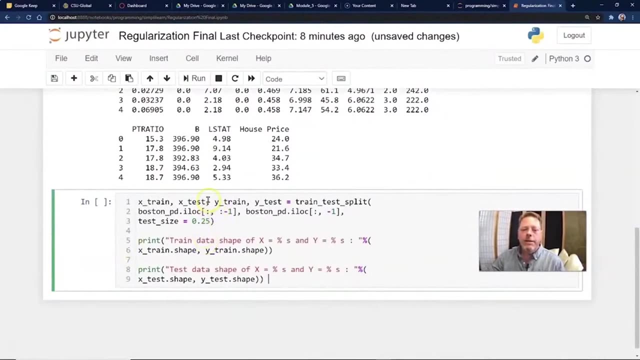 ZN industry, CHAZ Knox and all these other different statistics they've collected for house sales in Boston. There we go, Oops control. So we'll go ahead and split our data X train and our X test Y train. 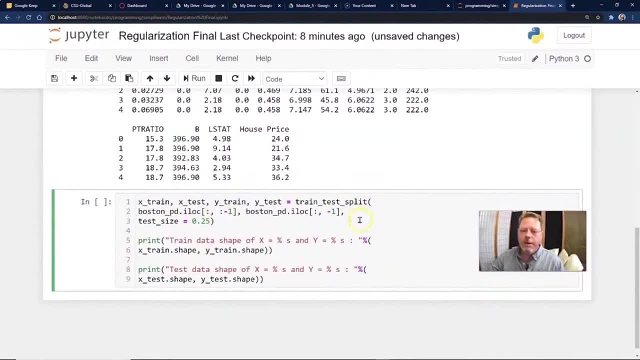 Y test equals the train test split which we imported, And we have our Boston. you could have easily used the X and Y on here as opposed to Boston I location, And we'll create our test size. We're going to take 25% of the data. 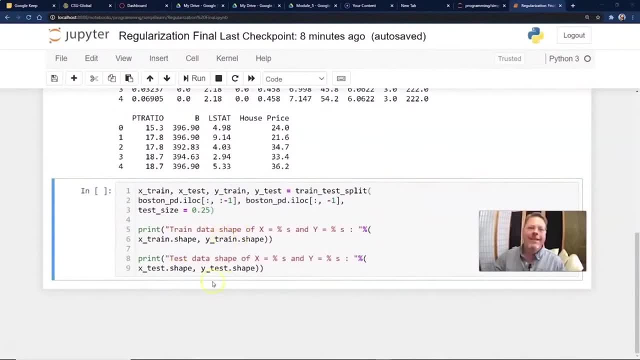 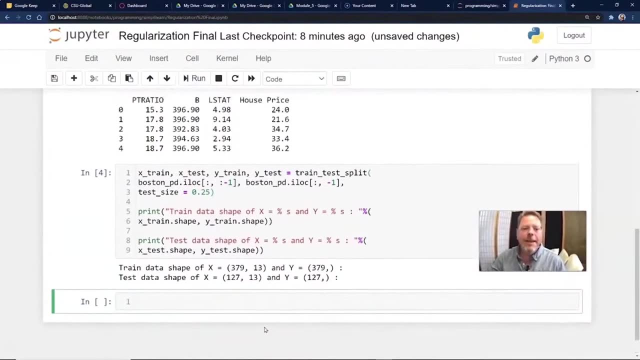 and put it in as a test, And then we'll go ahead and run. this Need an extra drink there. So we have our train and test and then, of course, the print, the train data shape. I love doing this kind of thing Whenever I'm working with this data. 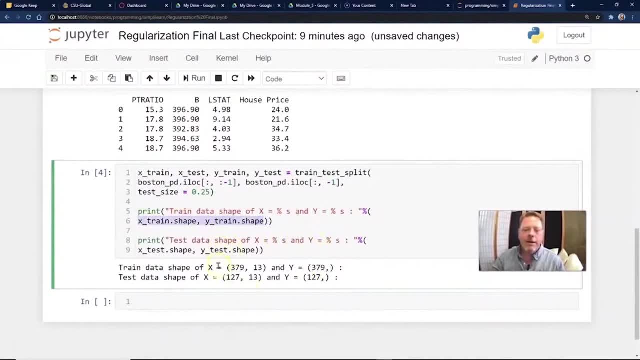 print out the shape. make sure everything looks correct so that we have 127 by 13 and 127 by one, 379 by 13. They should match, And if the data sets are not quite matching, then you know something's wrong. 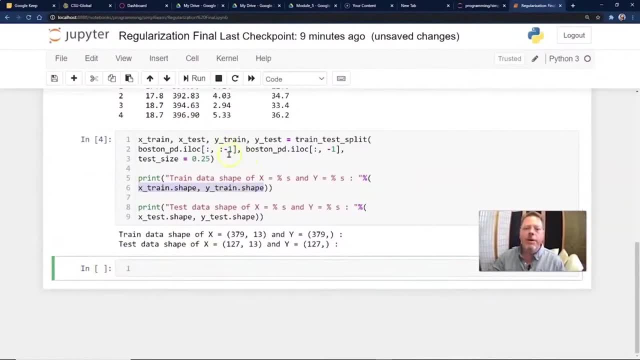 and you're going to get all those errors. I don't know how many times I've gone through here and it's dropped a row on one of them and not on the other, or something weird is happening When I'm cleaning the data. This is pretty straightforward and simple. 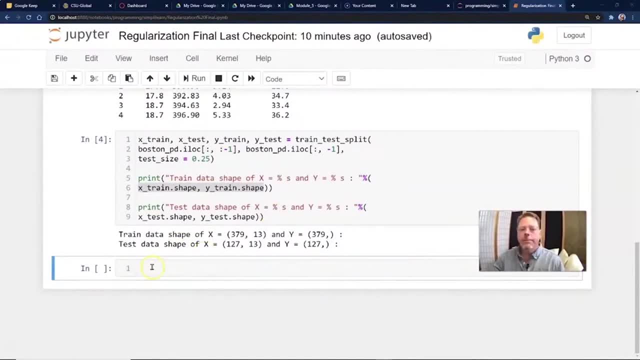 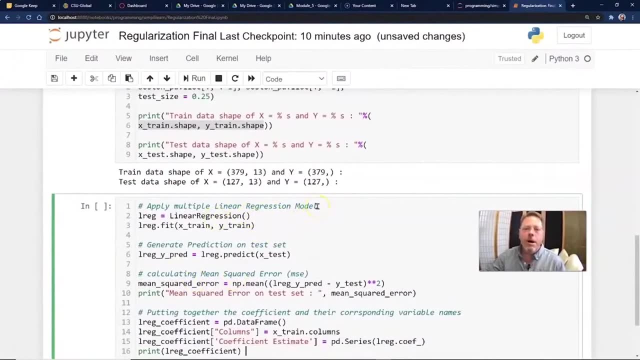 because the data comes in a nice prepacket and is all clean for you. So let's go ahead and apply the multiple linear regression model And we'll call this LREG- Lreg- Linear Regression. We're going to go ahead and fit that linear regression model. 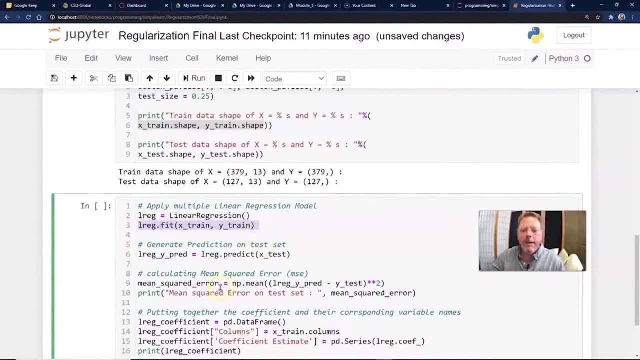 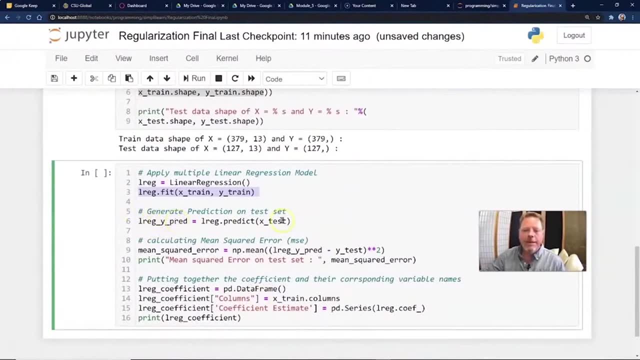 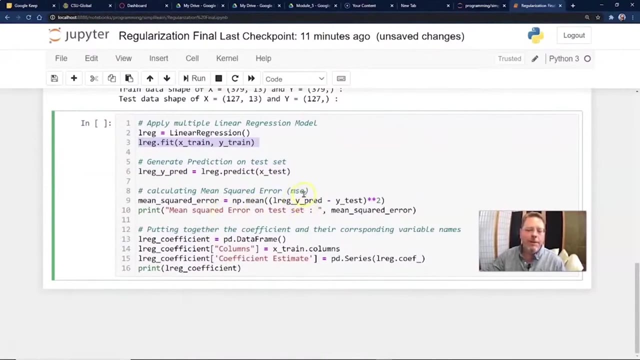 to X train and Y train. Then we'll generate the prediction on the test set. So here's our LREG Y predict with our X test going into the prediction And let's calculate that mean square error, MSE. I told you you'll see MSE used a lot. 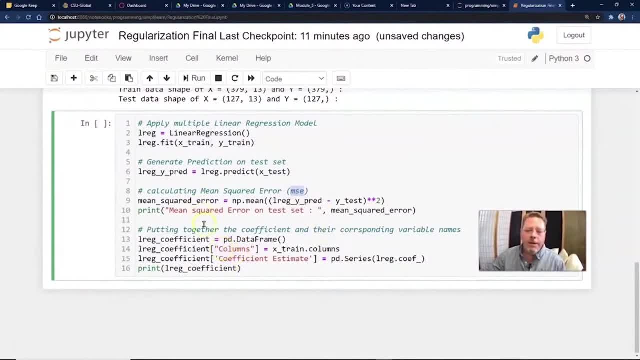 People use it in variables and things like that. It's pretty common And we get our mean squared error equals. this is just the basic formula. we've already been talking about. What's the difference squared? Then we look for the average of that. 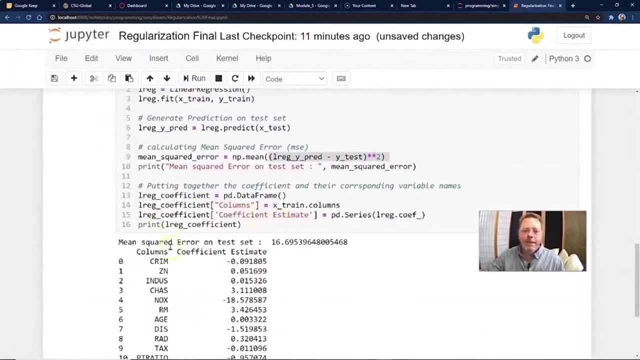 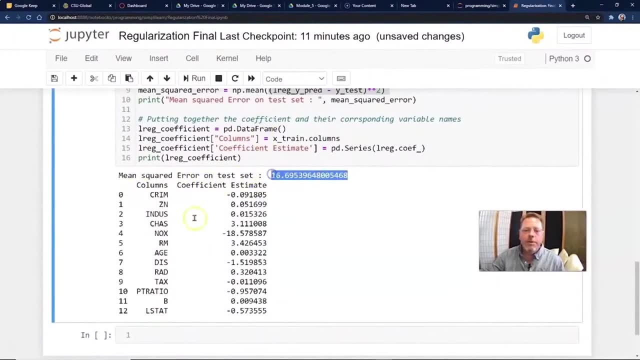 We'll go ahead and just run this And you can see when we get through the end of this. we have our mean square error on test, We have our total and then we have each column coming down And at this point, unless you really know the data, 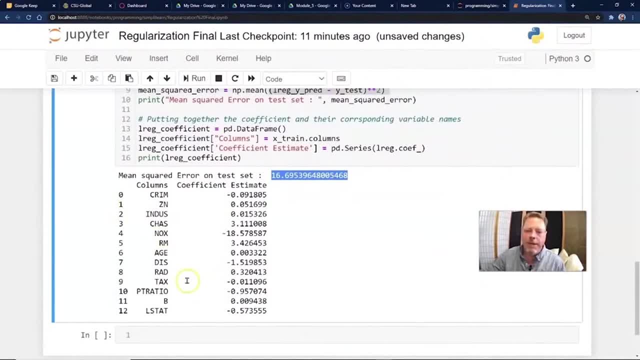 you're working with, it's not going to mean a whole lot. So if it's in your domain, you might know what you're looking at when you see these kinds of numbers coming up. But if it's not, it's just a bunch of numbers. 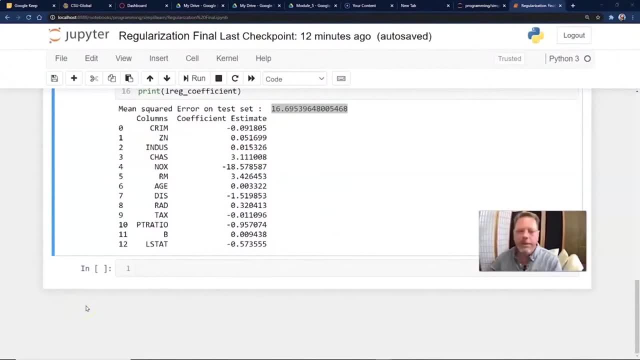 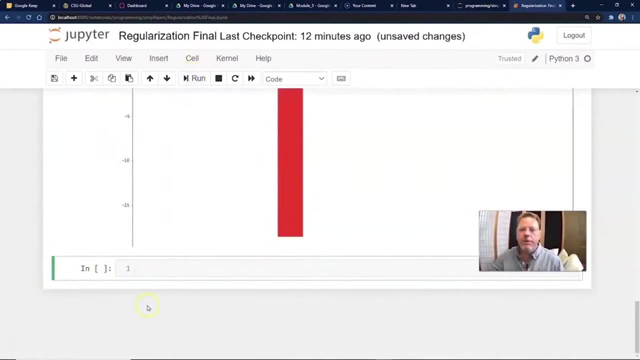 and that's okay- At least that's okay for this demo. And then we're going to go ahead and plot these so we can see what's going on, And this is always kind of fun. It's always nice to have a nice visual. 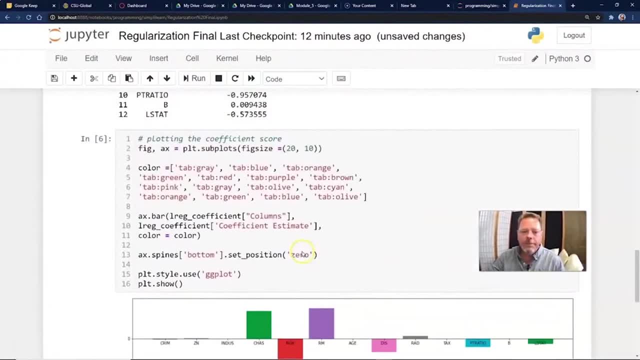 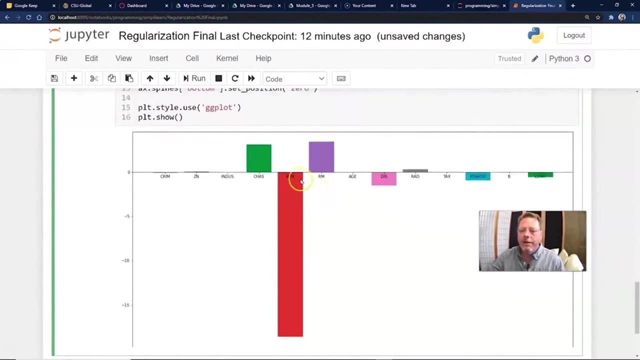 of what you're looking at And you can see here when we plot the coefficient scores on here. the guys in the back did a great job putting some pretty colors together and making it look nice and setting up the columns. You can see here: your NOX has just a huge coefficient. 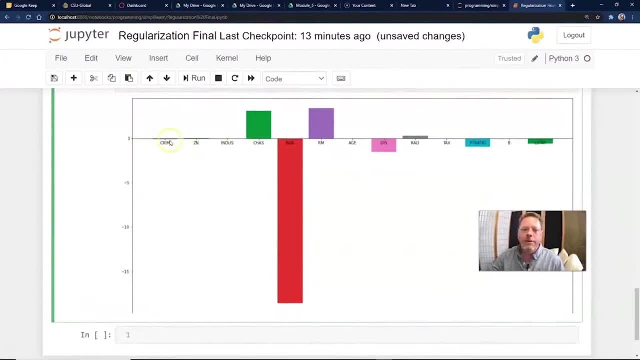 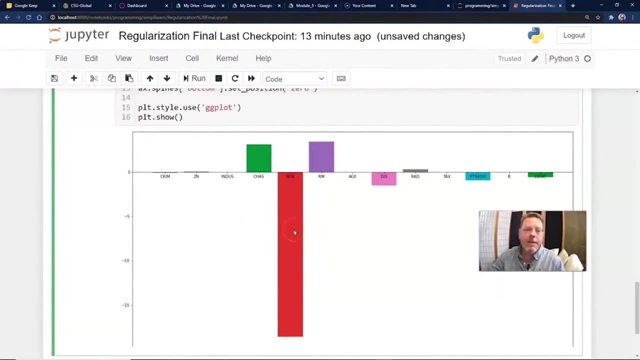 When I look at a table like this, I look for what has very little different coefficients- They're not using a huge change- and what has huge changes And that flags you for all kinds of things as you're working with the data, But it depends so much. 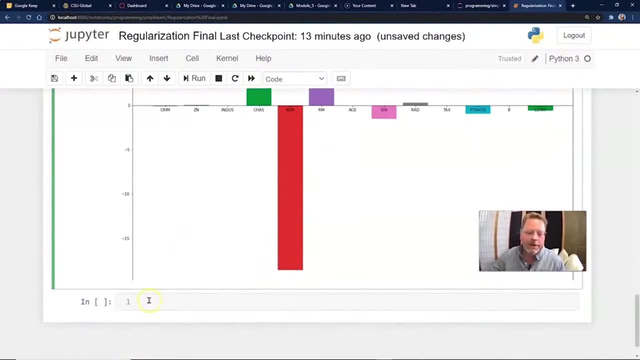 on the domain you're working with. These are great things, though, as just a quick look to see what's going on with your data and what you're looking for, And, of course, once we look at this now, our motive is to reduce. 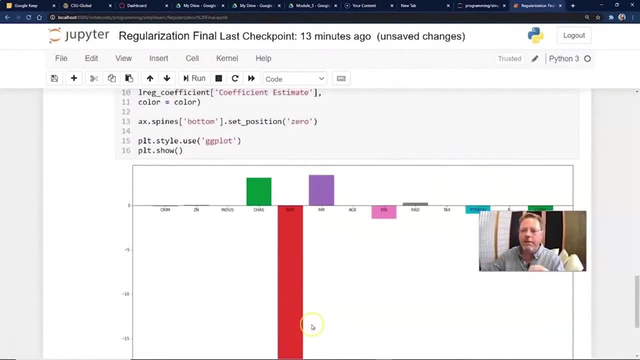 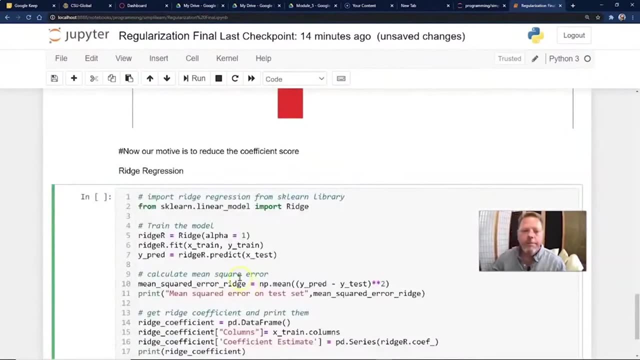 the coefficient score. So now we want to take these and bring them down as much as we can, And for that we're going to work with the ridge regression on here. So let's start by going ahead and we're going to import our ridge model. 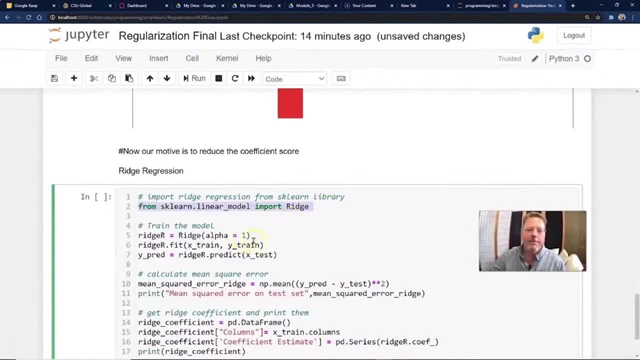 the ridge regression from the sklearn library or the scikit And we're going to go ahead and train the model. So here's our ridge: r equals alpha equals 1. And I mentioned that earlier When I work with the ridge model. 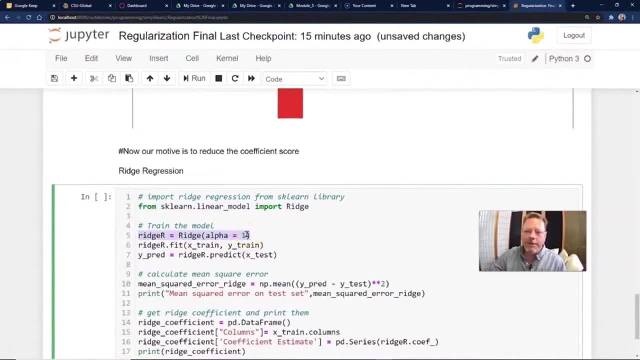 you'll see: alpha equals 1.. If you set alpha equal to 0, that's a standard linear regression model. So you have alpha equals 1,, 2,, 3,, 4, and you usually use 1,, 2, or 3, 4. 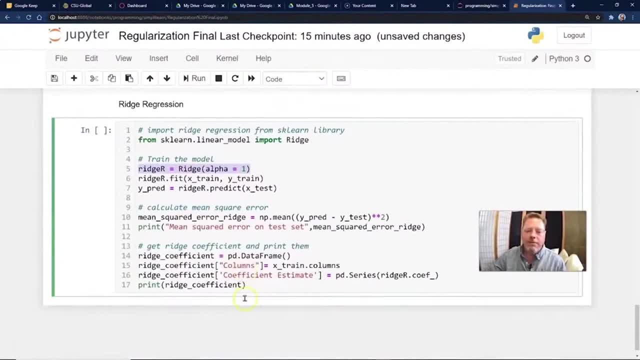 in a standard integer on there And we'll go ahead and fit the ridge model on there with our x-train and our y-train data, generate a prediction for that for our x-test, and we'll calculate the mean square error just like we did before. 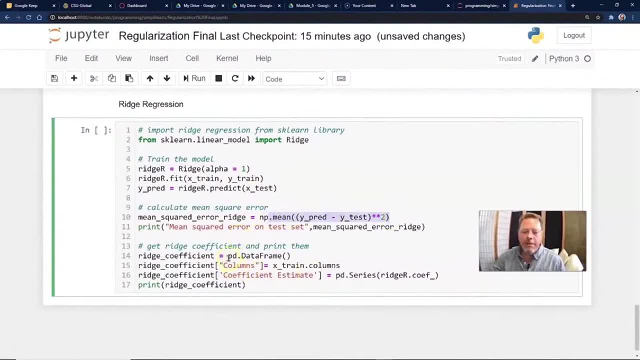 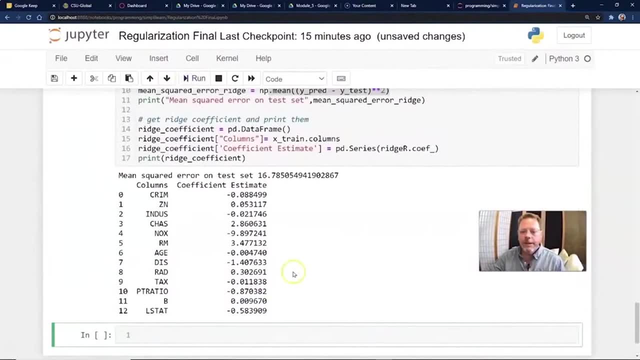 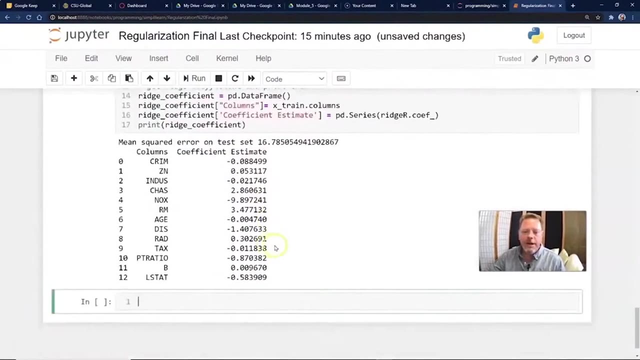 This should all look familiar And we'll go ahead and print that out and we'll look at the ridge coefficient for our data and see what that looks like. Now, if I jump up and down between these two, you'll get a headache. 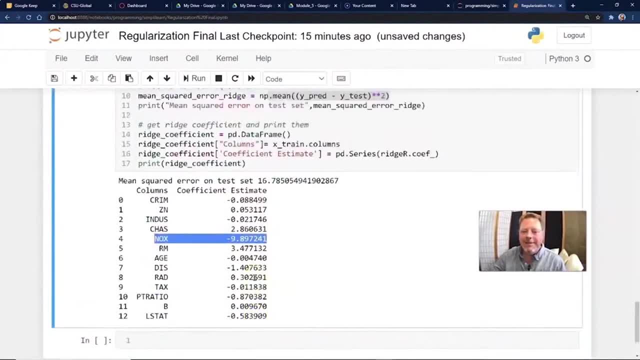 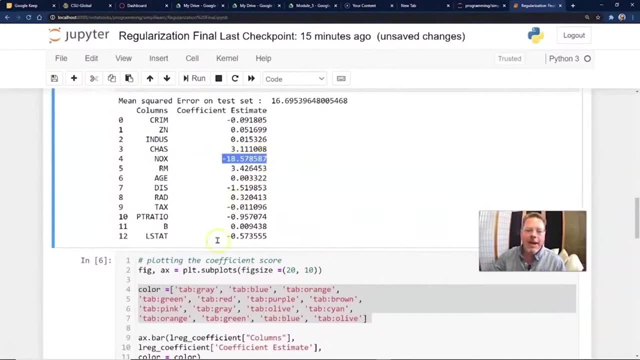 You'll still see the Nox value. Let's just look at the Nox, because that was the biggest value. It's a minus 9 here, And if we go back up here, the Nox value is a minus 18.. So right off the bat, 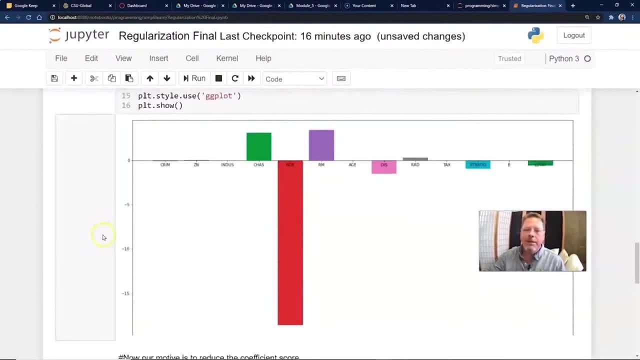 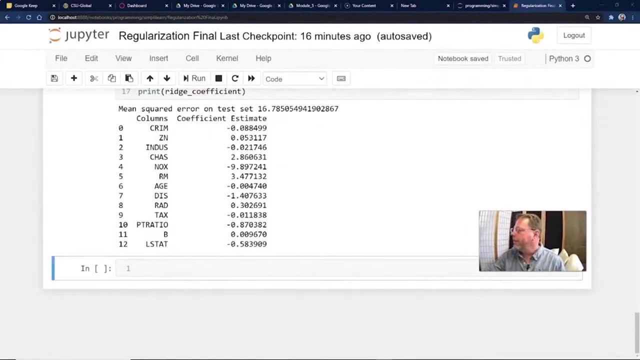 I'm seeing a huge change in the biggest coefficient there. So if we're going to do that nice setup, we want to go ahead and just print it and see what that looks like. There we go And we've set up our plots- subplots. 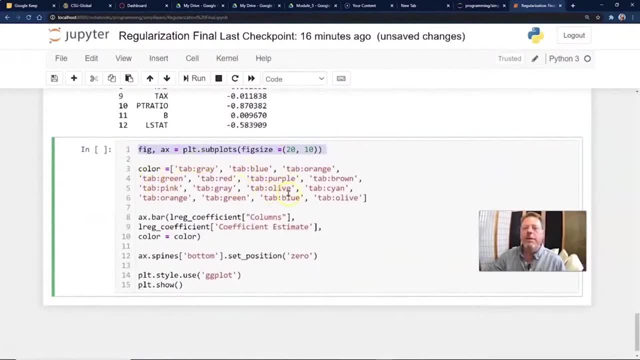 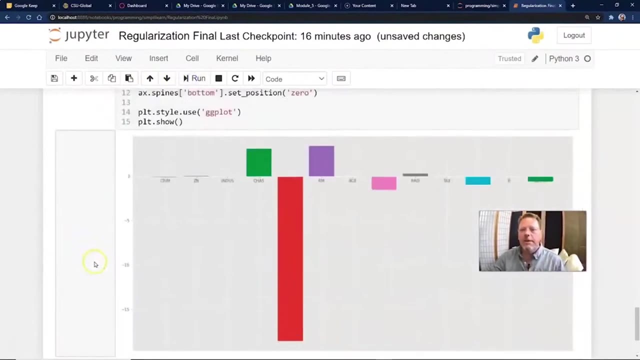 and again the team put together some nice colors so it makes it look good. We're doing an x-bar based on the columns and our L-regress coefficients: color equals color x, spine bottom and so forth, So it just puts together a nice little graph. 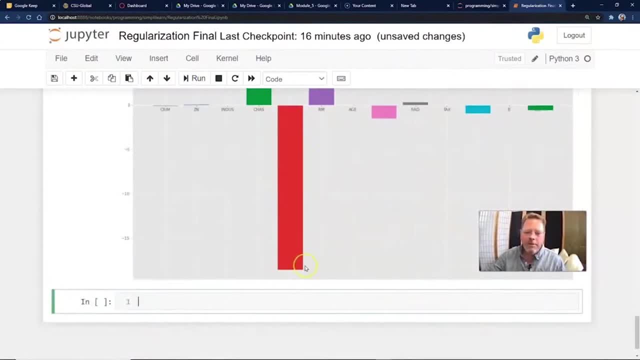 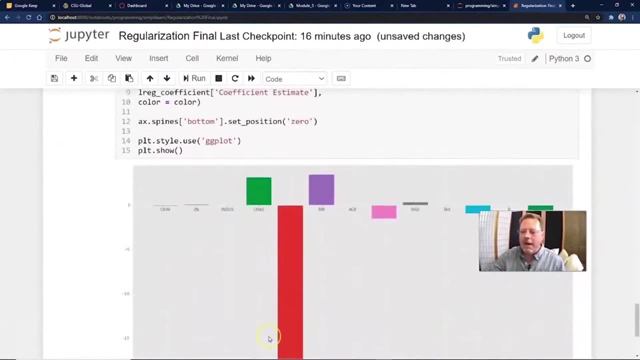 And you're starting to see one when you compare this, if you put it on the same graph as this one up here, this is up here at minus 18.. This is at minus 9.. And so this graph is half the size of the graph above. 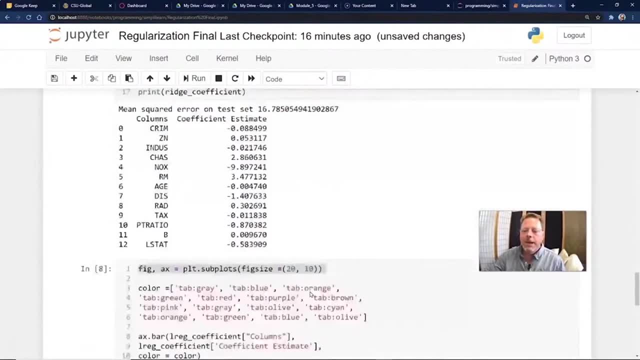 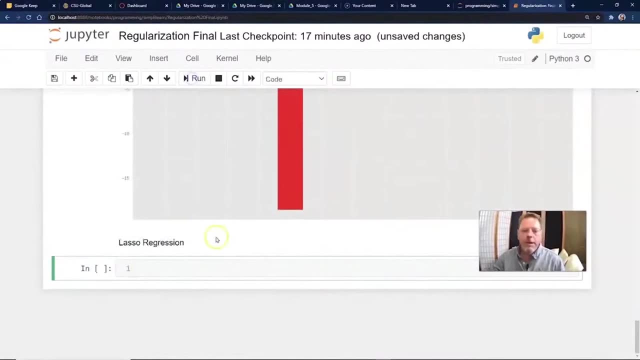 The same thing with these values here. They might look the same, but they're actually all almost half the value on here. And then, finally, you can do the same thing for the lasso regression. This will all look very similar as far as what we worked on before. 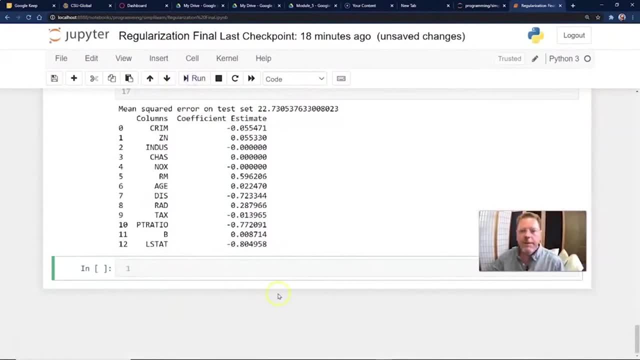 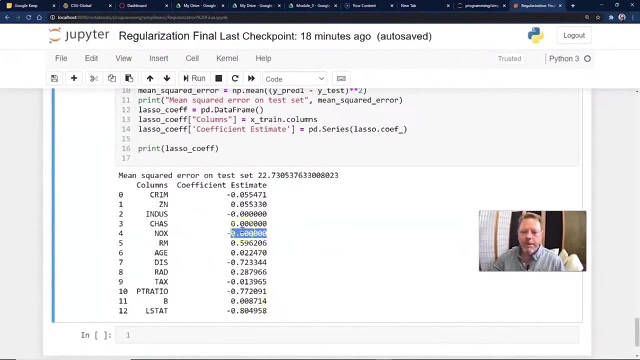 And I'm just going to go ahead and print that on here and run it. And again, let's go up to NOX. Look where NOX is. It's all the way down to 0.. And if we look at our next biggest coefficient, 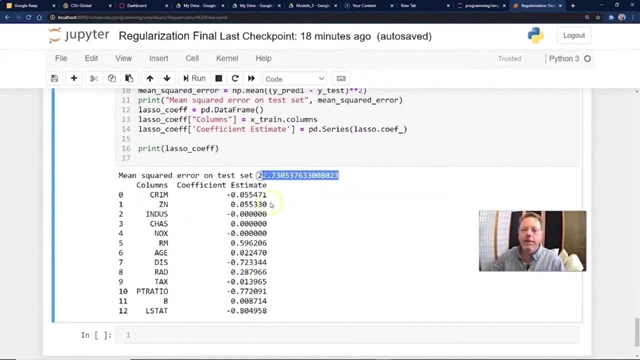 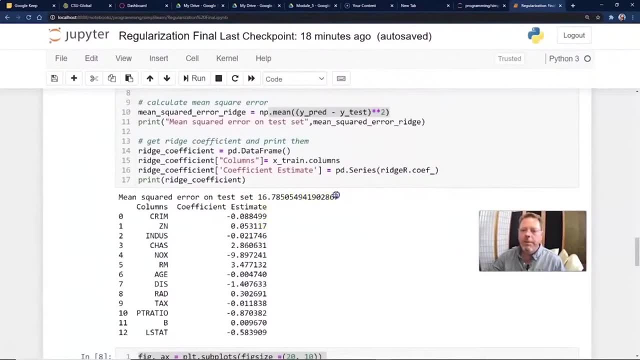 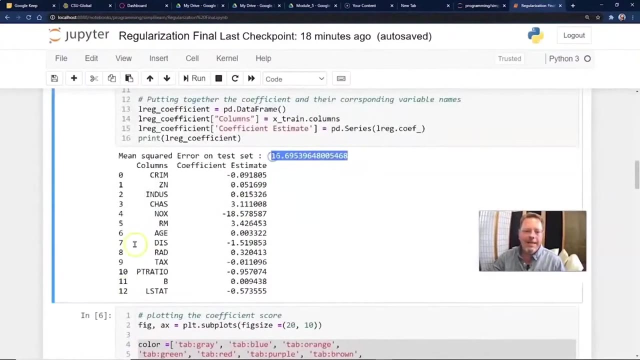 it's minus 0.8.. And really here's our 22.73.. We go up here: 16.7.. And we go up here and we look at the same number, 16.69.. And so we look at this: 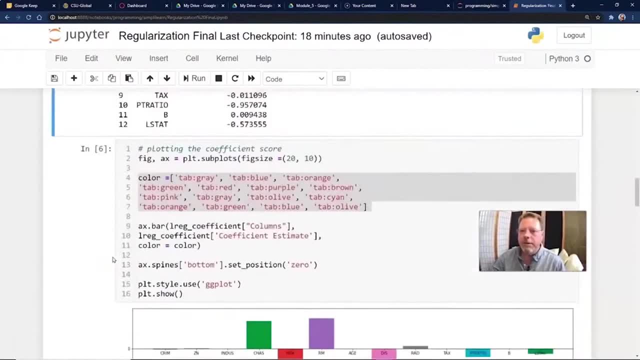 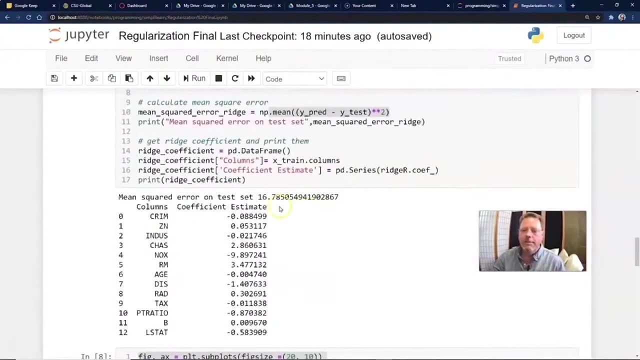 If I was running this and working on a project with this, I would look at these numbers. I'd start with the 16.69, come down here and compare it to 16.78.. 69 is better than 78. So from the very beginning, 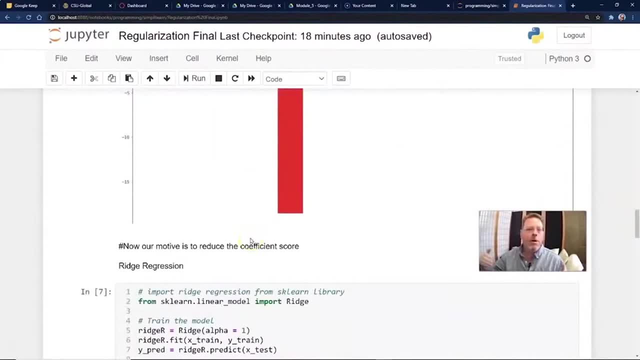 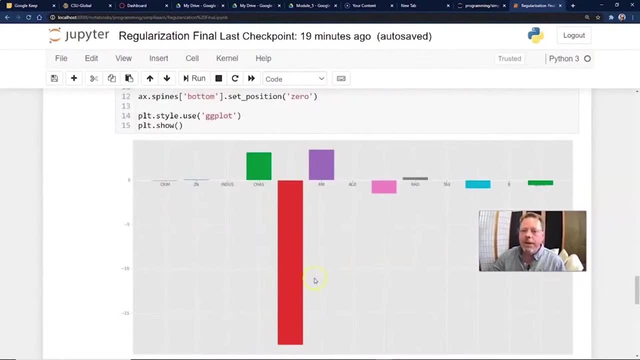 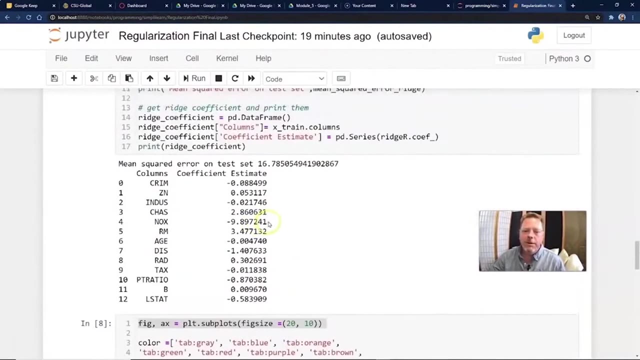 we might start looking at this first model for overall predicting, But there's other factors involved. We might know that the NOX value is central and the other ones aren't quite as good, And so we might start looking at just certain setups like what is this particular coefficient? 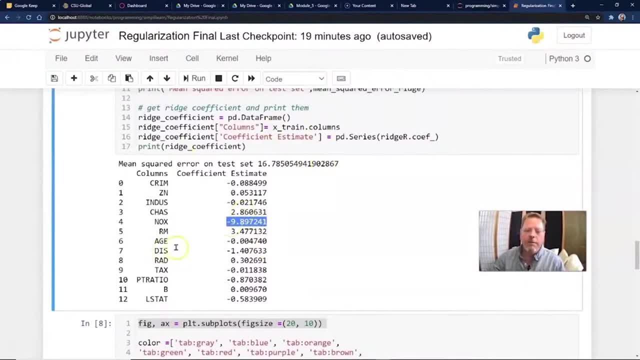 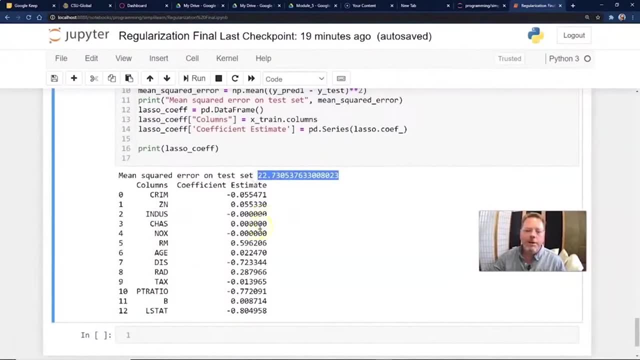 because it might have a certain meaning to us and so forth, And so you can look at all those different items in there Again. but the bottom dollar is our first model did better than our other two models. Our mean square error on the test set. 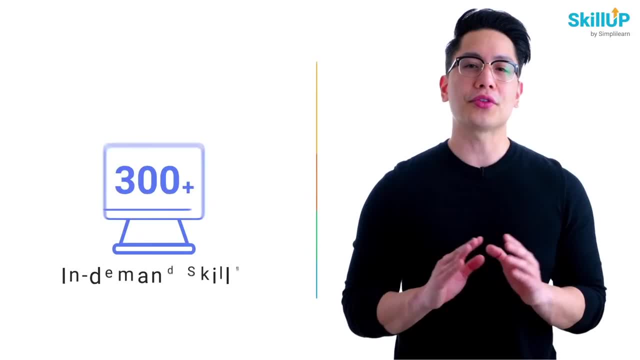 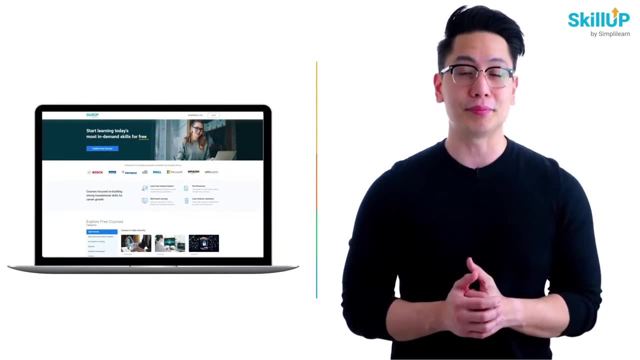 continues to come down on this. Choose from over 300 in-demand skills and get access to 1,000 plus hours of video content for free. Visit SkillUp by SimplyLearn. Click on the link in the description to know more In this video. 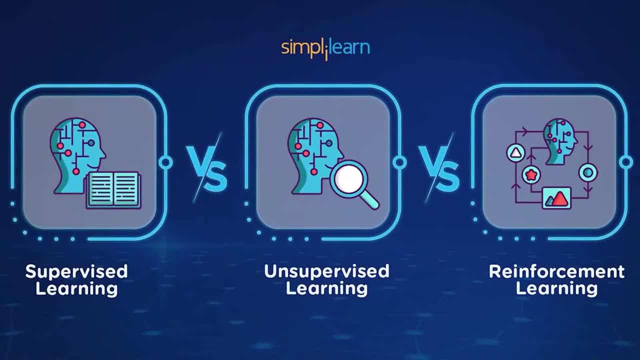 you will learn about an interesting machine learning topic, that is, supervised versus unsupervised, versus reinforcement learning. Let's discuss each of them in detail and understand when to use these algorithms, along with their applications. Now, there are a number of algorithms used in the field of machine learning. 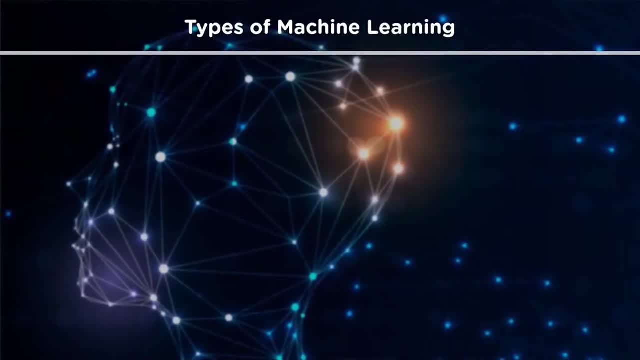 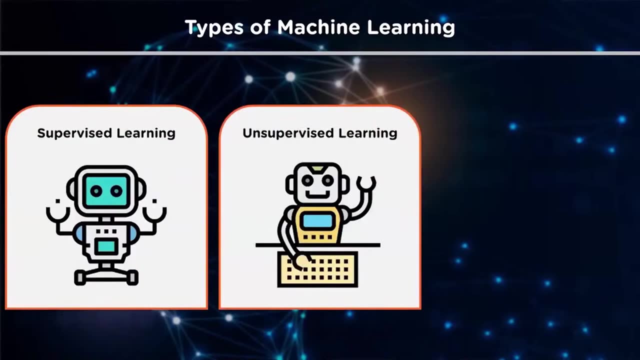 to solve complex problems. Each of these algorithms can be classified into a certain category, So the different types of machine learning algorithms are: supervised learning, unsupervised learning and reinforcement learning. Now let's look at the definition of each of these learning techniques. 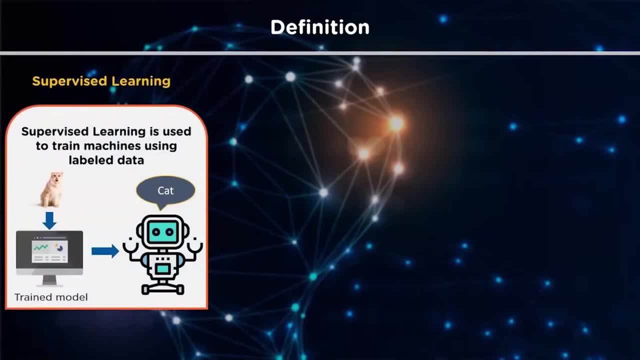 Supervised learning uses labeled data to train machine learning models. Labeled data means that the output is already known to you. The model just needs to map the inputs to the outputs. An example of supervised learning can be to train a machine that identifies the image of an animal. 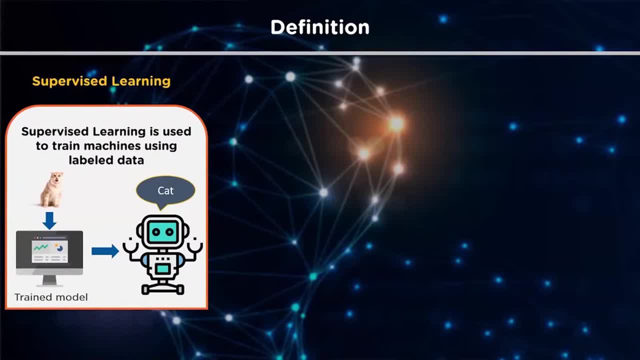 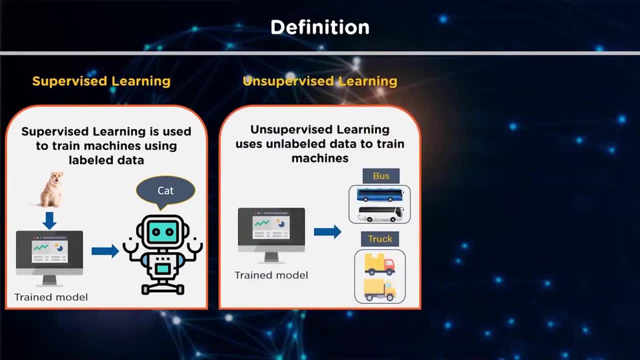 Below you can see we have a trained model that identifies the picture of a cat. Unsupervised learning uses unlabeled data to train machines. Unlabeled data means there is no fixed output variable. The model learns from the data, discovers patterns and features in the data. 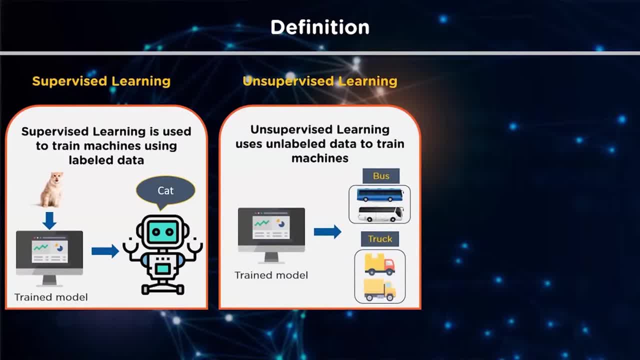 and returns the output. Here is an example of an unsupervised learning technique that uses the images of vehicles to classify if it's a bus or a truck. So the model learns by identifying the parts of a vehicle, such as the length and width of the vehicle. 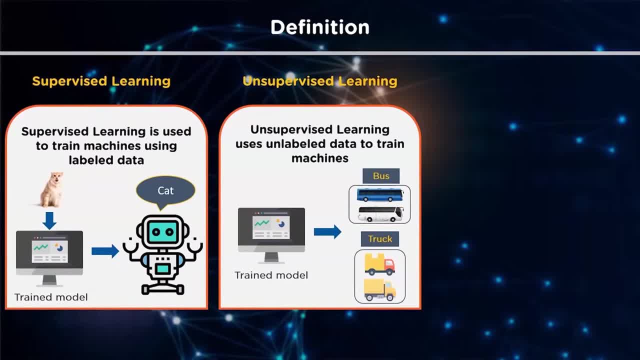 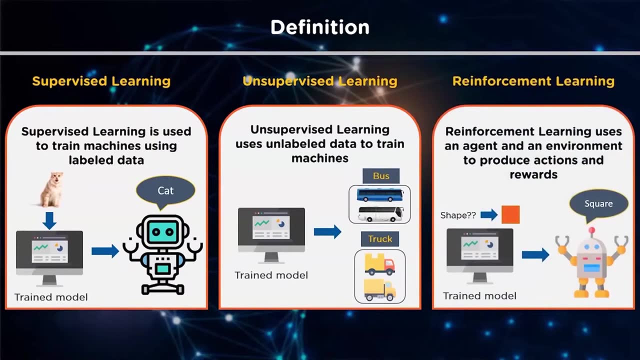 the front and rear end covers, roof hoods, the types of wheels used, etc. Based on these features, the model classifies if the vehicle is a bus or a truck. Reinforcement learning trains: a machine to take suitable actions and maximize reward in a particular situation. 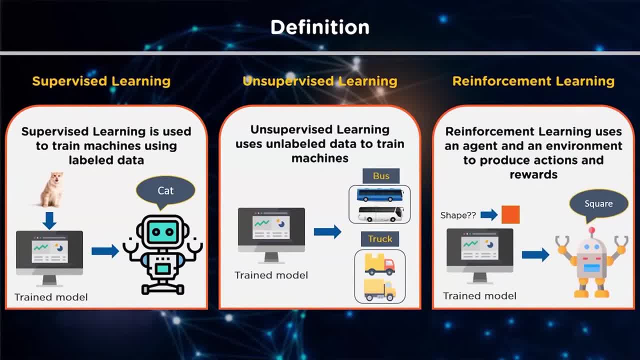 It uses an agent and an environment to produce actions and rewards. The agent has a start and an end state, but there might be different paths for reaching the end state, like a maze In this learning technique. there is no predefined target variable. 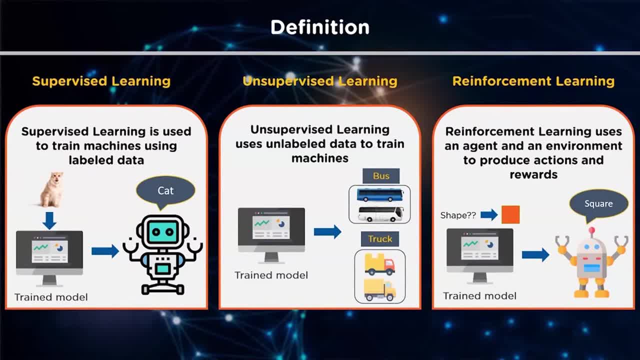 An example of reinforcement learning is to train a machine that can identify the shape of an object. given a list of different objects, such as square, triangle, rectangle or a circle, In the example shown, the model tries to predict the shape of the object. 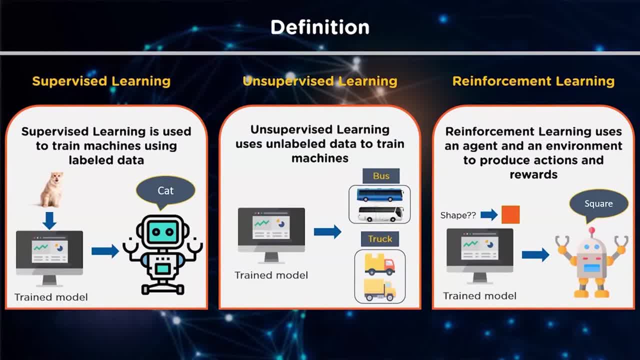 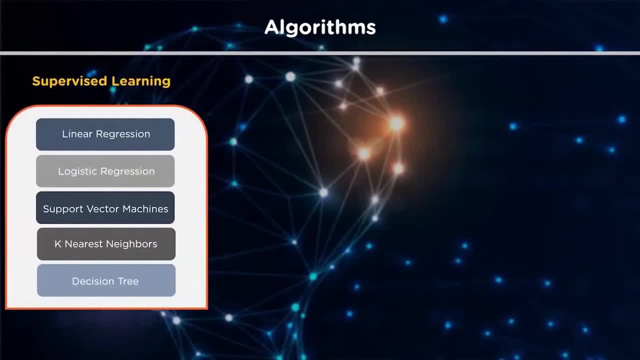 which is a square here. Now let's look at the different machine learning algorithms that come under these learning techniques. Some of the commonly used supervised learning algorithms are linear regression, logistic regression, support vector machines, k-nearest neighbors, decision tree, random forest and naive Bayes. 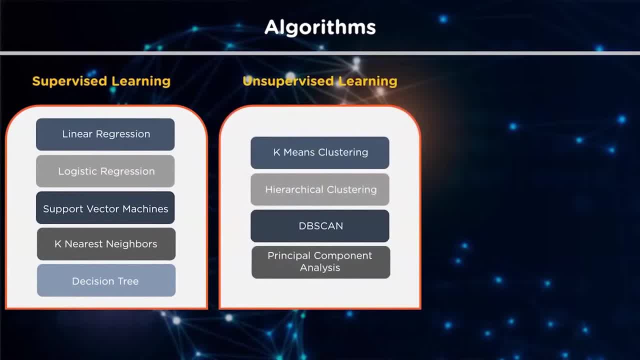 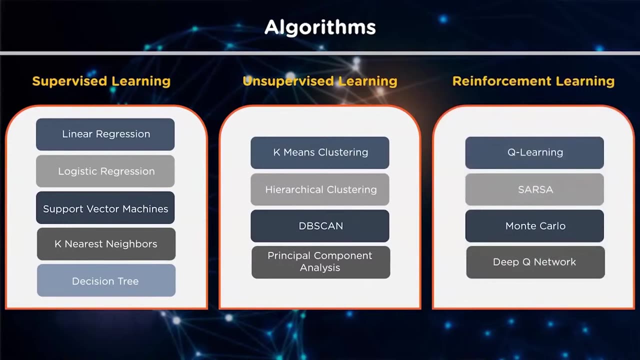 Examples of unsupervised learning algorithms are k-means clustering, hierarchical clustering, db-scan, principal component analysis and others. Choosing the right algorithm depends on the type of problem you are trying to solve. Some of the important reinforcement learning algorithms are Q-learning, Monte Carlo. 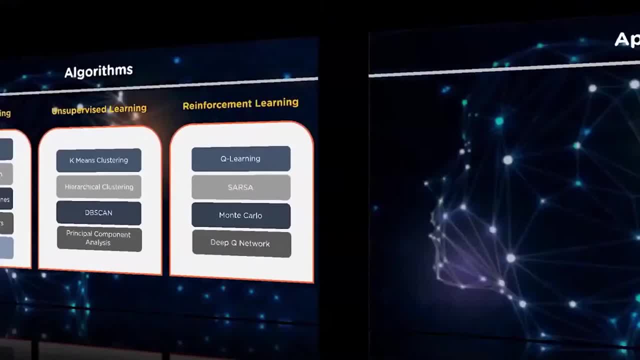 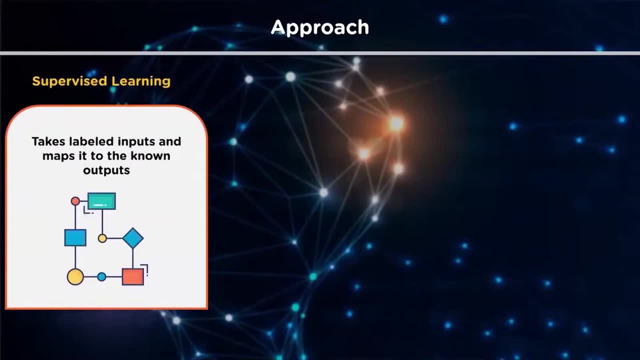 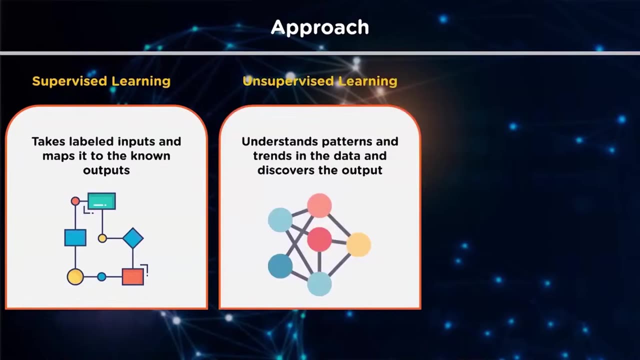 SAR-SAR and deep Q-network. Now let's look at the approach in which these machine learning techniques work. Supervised learning takes labeled inputs and maps it to known outputs, Which means you already know the target variable. Unsupervised learning finds patterns. 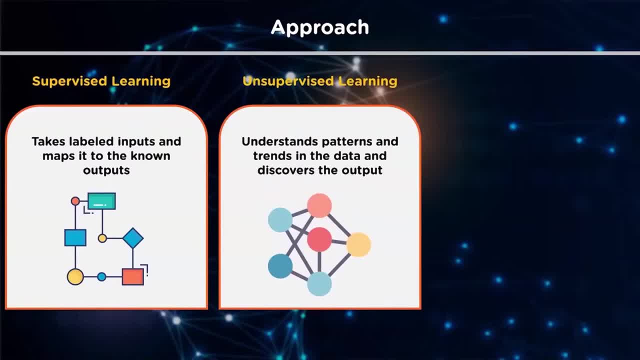 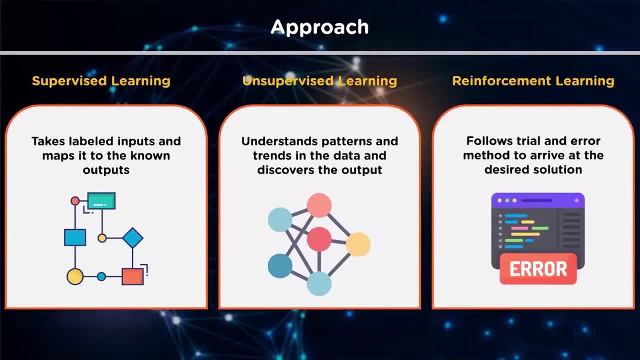 and understands the trends in the data to discover the output. So the model tries to label the data based on the features of the input data, While reinforcement learning follows trial and error method to get the desired solution. After accomplishing a task, the agent receives an award. 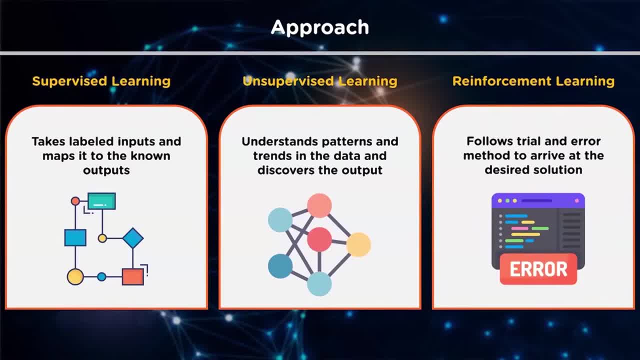 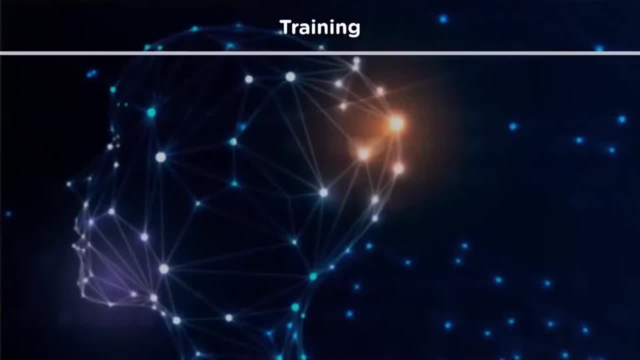 An example could be to train a dog to catch the ball. If the dog learns to catch a ball, you give it a reward, such as a biscuit. Now let's discuss the training process for each of these learning methods. So supervised learning methods. 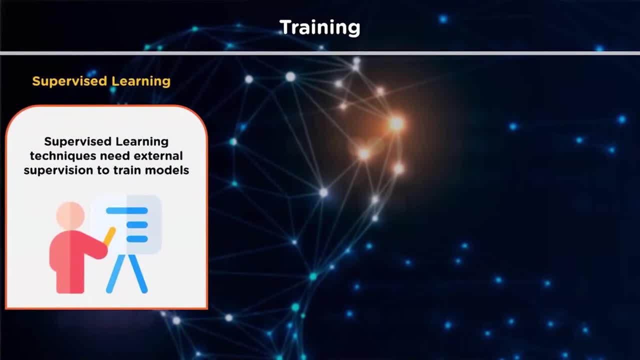 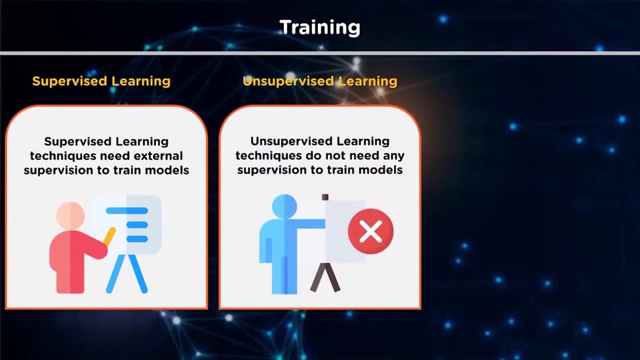 need external supervision to train machine learning models, and hence the name supervised. They need guidance and additional information to return the result. Unsupervised learning techniques do not need any supervision to train models. They learn on their own and predict the output. Similarly, reinforcement learning methods. 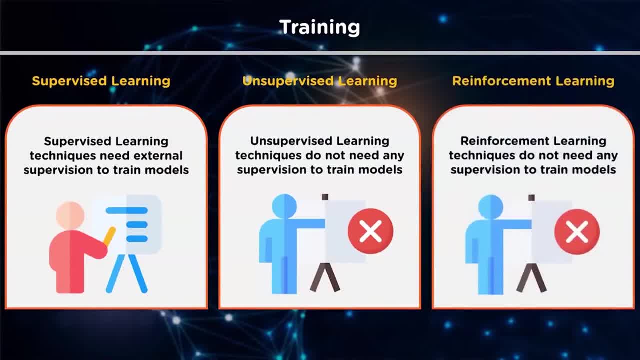 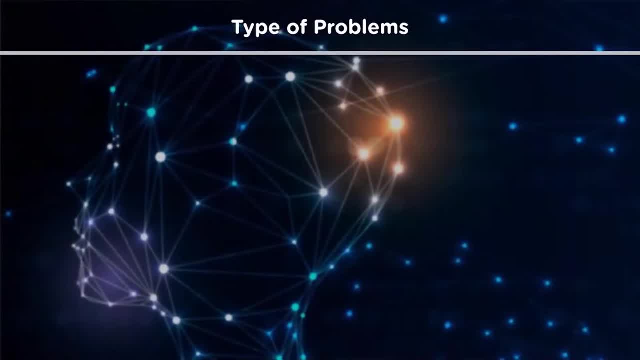 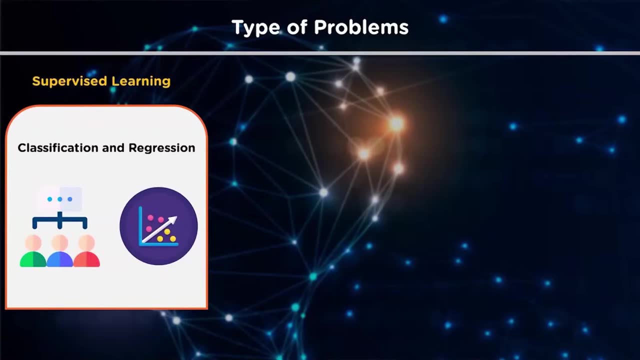 do not need any supervision to train machine learning models, And with that let's focus on the types of problems that can be solved using these three types of machine learning techniques. So supervised learning is generally used for classification and regression problems. We'll see the examples in the next slide. 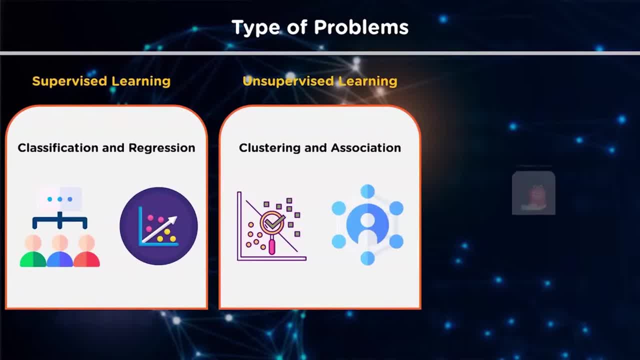 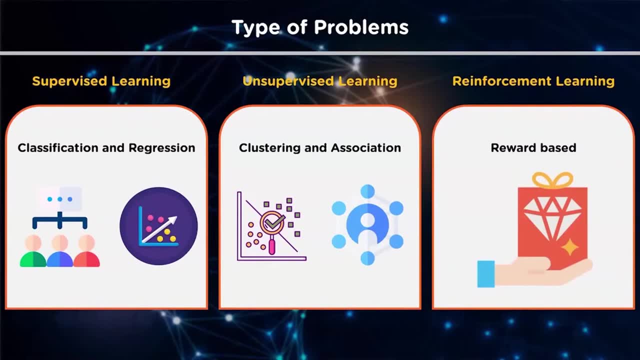 And unsupervised learning is used for clustering and association problems, While reinforcement learning is reward-based. so for every task or for every step completed, there will be a reward received by the agent, And if the task is not achieved correctly, there will be some penalty used. 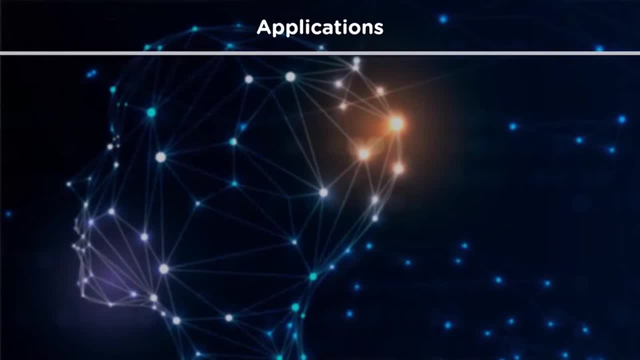 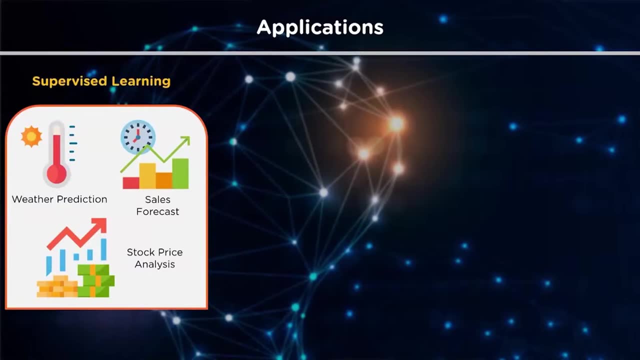 Now let's look at a few applications of supervised, unsupervised and reinforcement learning. As we saw earlier, supervised learning are used to solve classification and regression problems. For example, you can predict the weather for a particular day based on humidity, precipitation, wind speed. 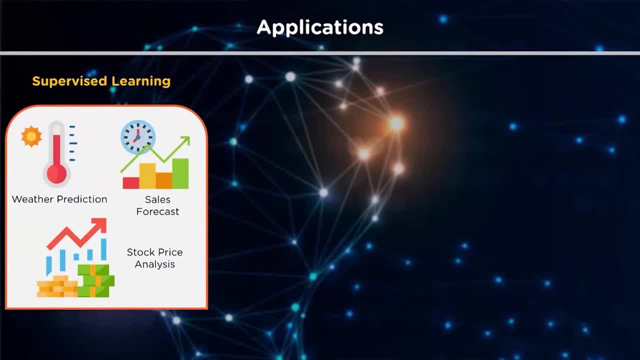 and pressure values. You can use supervised learning algorithms to forecast sales for the first month or the next quarter for different products. Similarly, you can use it for stock price analysis or identifying if a cancer cell is malignant or benign. Now talking about the applications. 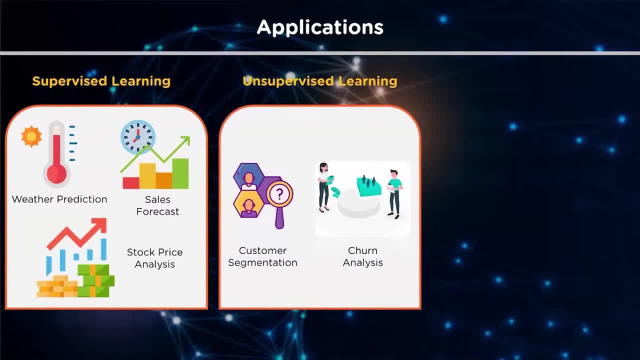 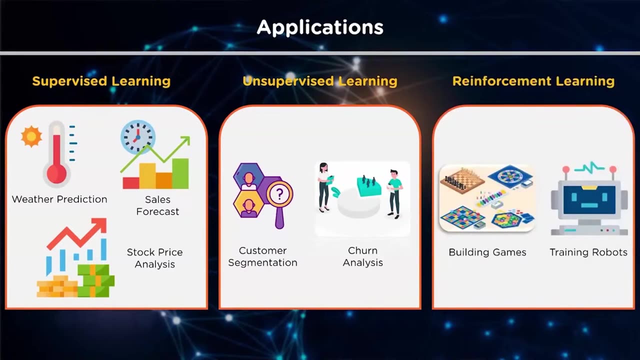 of unsupervised learning. we have customer segmentation. So based on customer behavior, likes, dislikes and interests, you can segment and cluster similar customers into a group. Another example where unsupervised learning algorithms are used is customer churn analysis. Now let's see. 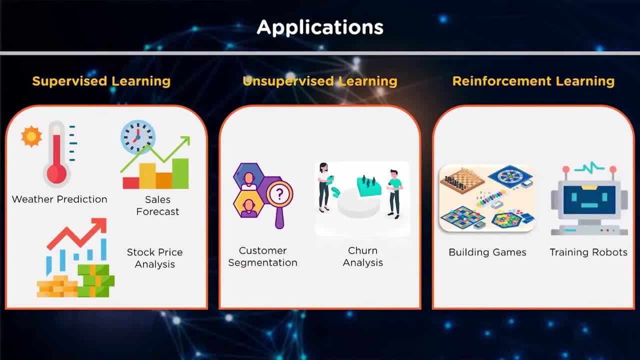 the applications we have in reinforcement learning. So reinforcement learning algorithms are widely used in the gaming industries to build games. It is also used to train robots to perform human tasks. If getting your learning started is half the battle, what if you could do that for free? 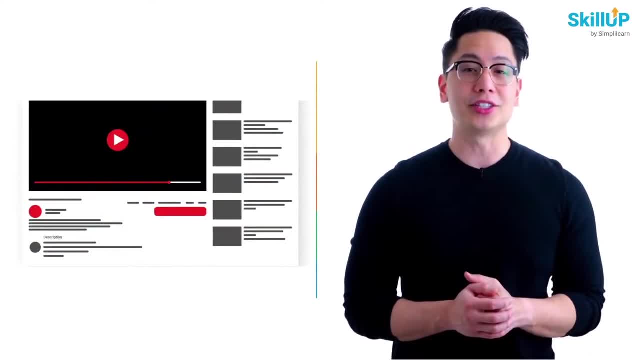 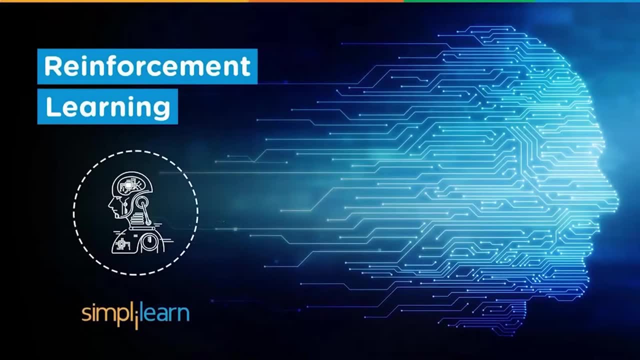 Visit SkillUp by SimplyLearn. Click on the link in the description to know more Reinforcement learning by SimplyLearn. My name is Richard Kirschner, with the SimplyLearn team. That's wwwsimplylearncom. Get certified, Get ahead. 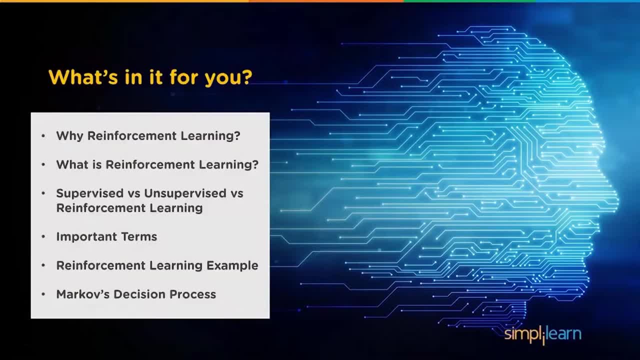 We're going to cover reinforcement learning today And what's in it for you. We'll start with why reinforcement learning. We'll look at what is reinforcement learning. We'll see what the different kinds of learning strategies are that are being used today in computer models. 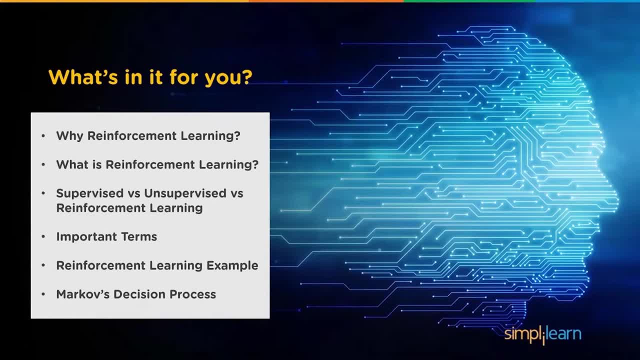 under supervised versus unsupervised, versus reinforcement. We'll cover important terms specific to reinforcement learning. We'll talk about Markov's decision process and we'll take a look at a reinforcement learning example, while we'll teach a tic-tac-toe how to play. 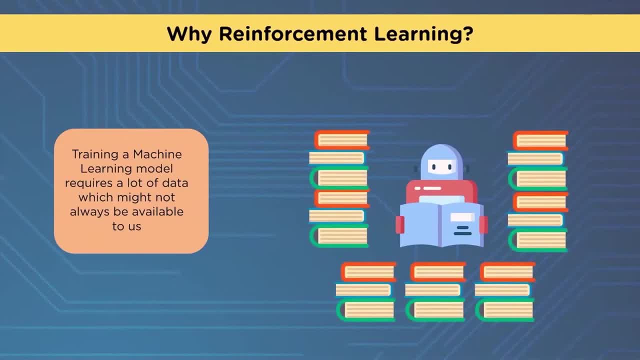 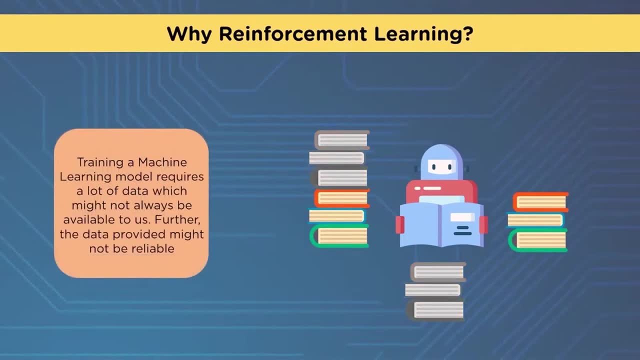 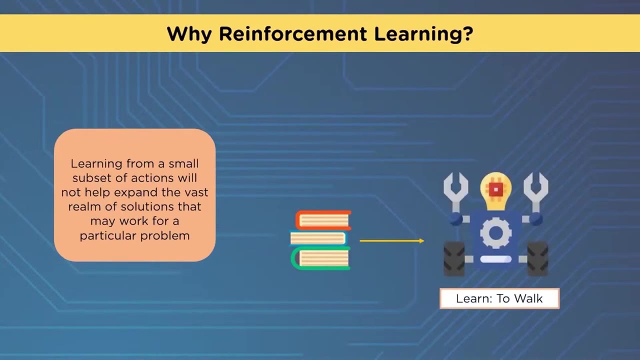 Why reinforcement learning Training? a machine learning model requires a lot of data, which might not always be available to us. Further, the data provided might not be reliable. Learning from a small subset of actions will not help expand the vast realm of solutions that may work. 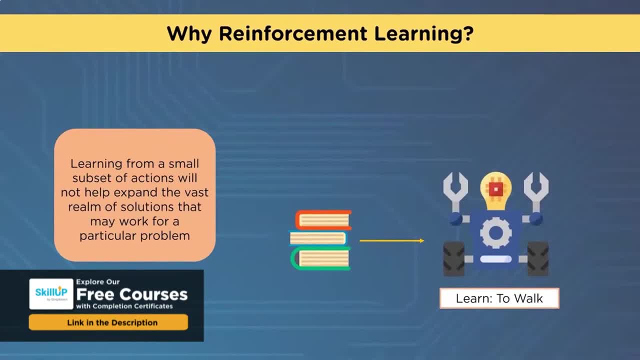 for a particular problem. You can see here we have the robot learning to walk- Very complicated setup. when you're learning how to walk, You'll start asking questions like: if I'm taking one step forward and left, what happens if I pick up a 50 pound object? 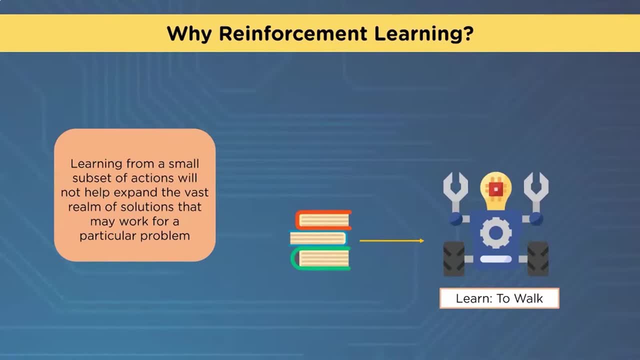 How does that change how a robot would walk? These things are very difficult to program because there's no actual information on it until it's actually tried out. Learning from a small subset of actions will not help expand the vast realm of solutions that may work for a particular problem. 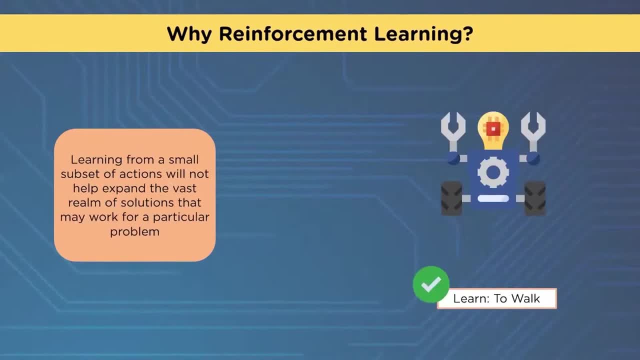 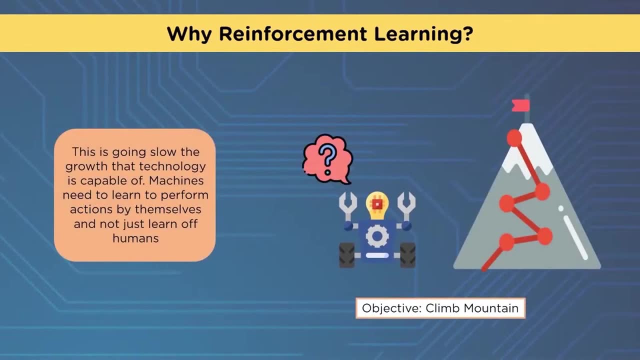 And we'll see here. it learned how to walk. This is going to slow the growth that technology is capable of. Machines need to learn to perform actions by themselves and not just learn off humans. And you see the objective climb a mountain. A real interesting point here. 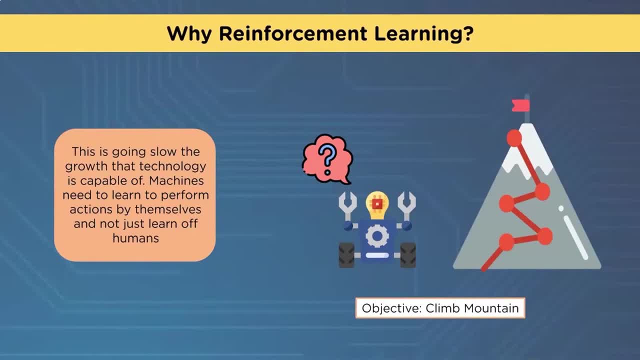 is that as human beings we can go into a very unknown environment and we can adjust for it and kind of explore and play with it. Most of the models, the non-reinforcement models in computer machine learning, aren't able to do that very well. 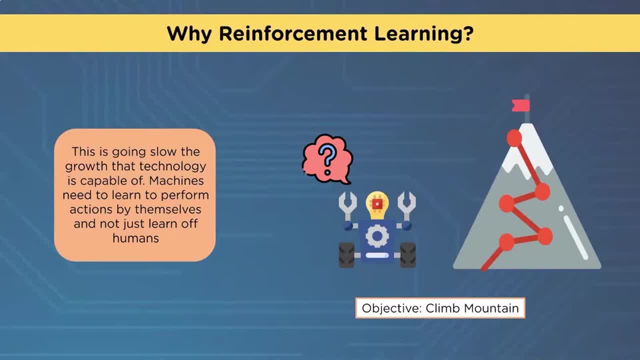 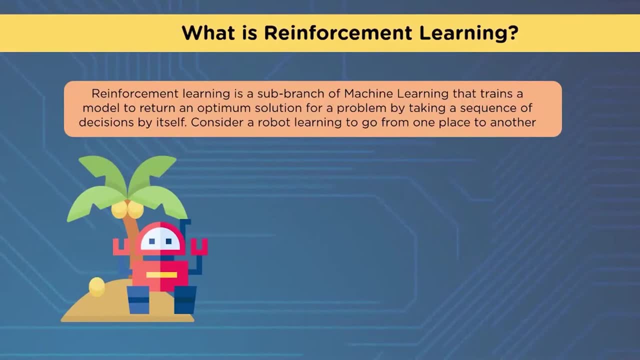 There's a couple of them that can be used or integrated to see how it goes is what we're talking about with reinforcement learning. So what is reinforcement learning? Reinforcement learning is a sub-branch of machine learning that trains the model to return an optimum solution for a problem. 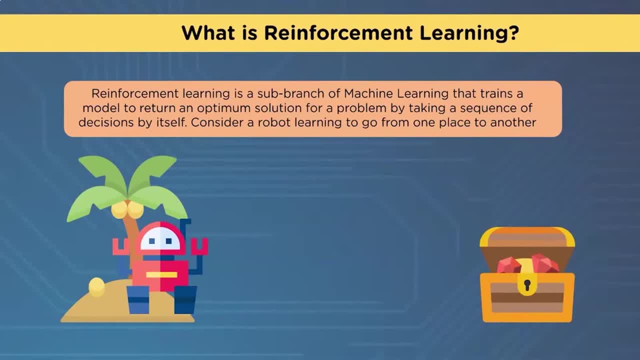 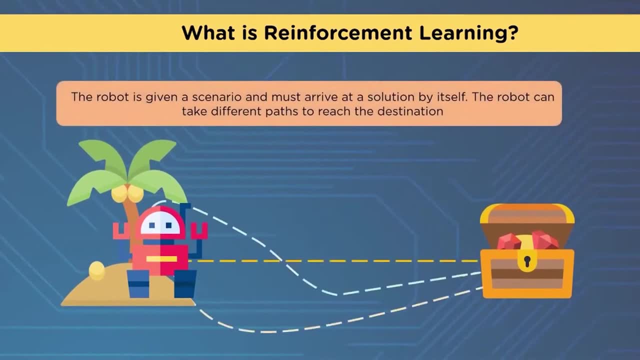 by taking a sequence of decisions by itself. Consider a robot learning to go from one place to another. The robot is given a scenario and must arrive at a solution by itself. The robot can take different paths to reach the destination. It will know the best path. 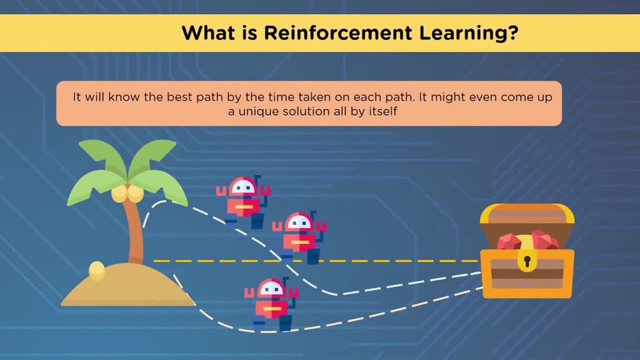 by the time taken on each path. It might even come up with a unique solution all by itself, And that's really important, as we're looking for unique solutions. We want the best solution, but you can't find it unless you try it, So we're looking at our different. 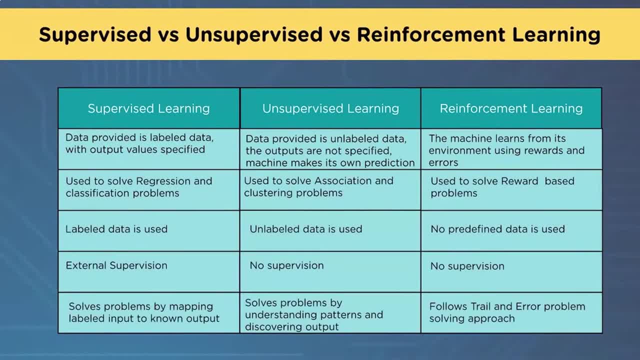 systems, our different model. We have supervised versus unsupervised, versus reinforcement learning, And with the supervised learning that is probably the most controlled environment. We have a lot of different supervised learning models, whether it's linear, regression, neural networks- there's all kinds of things in between. 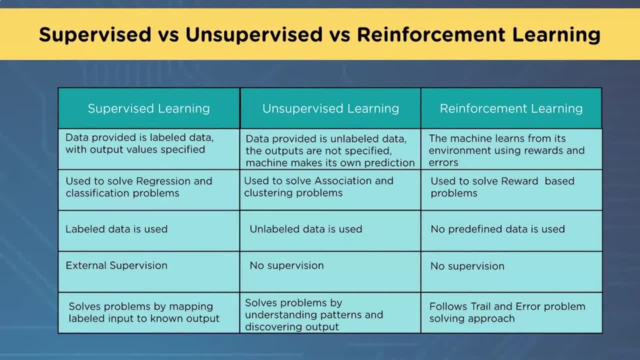 decision trees. The data provided is labeled, data with output values specified, And this is important because when we talk about supervised learning, you already know the answer for all this information. You already know the picture has a motorcycle in it, So you're supervised learning. 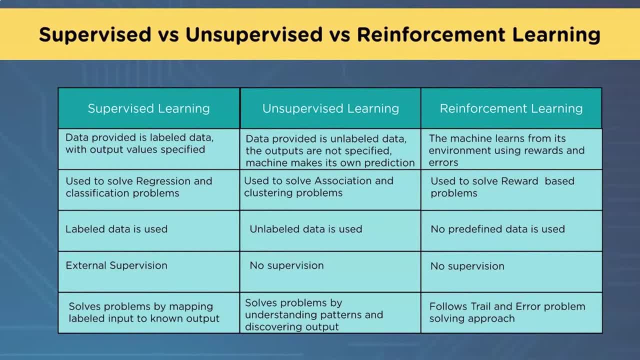 You already know that the outcome for going back a week. you're looking at stock. you have the graph of what the next day looks like, So you have an answer for it And you have labeled data which is used. You have an external supervision. 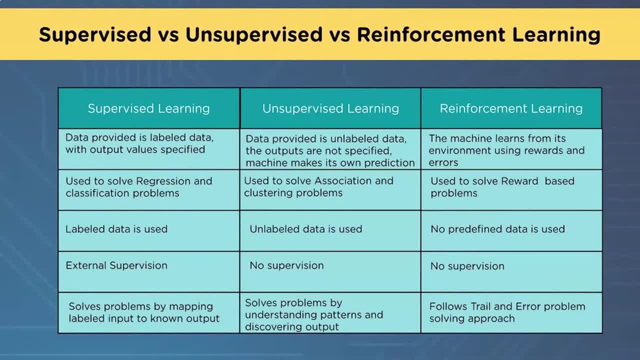 and solves problems by mapping labeled input to known output. So very controlled Unsupervised learning is really interesting because it's now taking part in many other models. You can actually insert an unsupervised learning model in almost either supervised or reinforcement learning models. 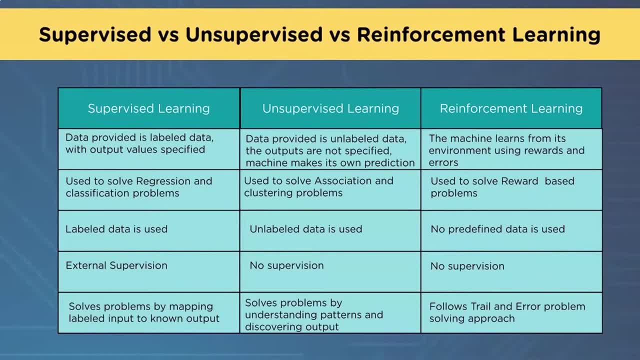 As part of the system, Which is really cool. Data provided is unlabeled data. The outputs are not specified. Machine makes its own predictions. Used to solve association with clustering problems. Unlabeled data is used. No supervision. Solves problems by. 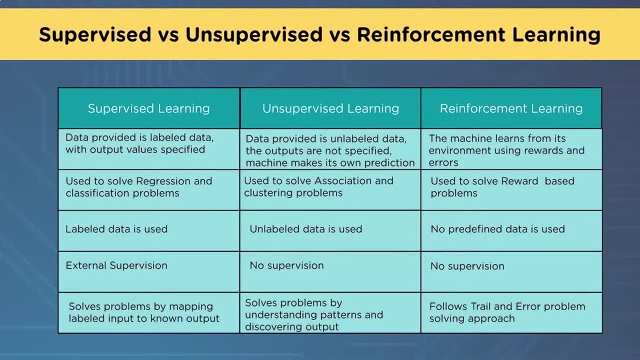 understanding patterns and discovering output. So you can look at this and you can think some of these things go with each other. They belong together. So it's looking for what connects in different ways And there's a lot of different algorithms that look at this. 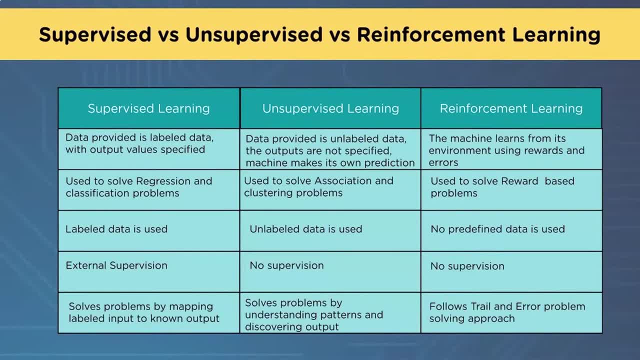 When you start getting into those, there's some really cool images that come up of what unsupervised learning is, How it can pick out, say, the area of a donut. One model will see the area of the donut and the other one will divide it into three sections. 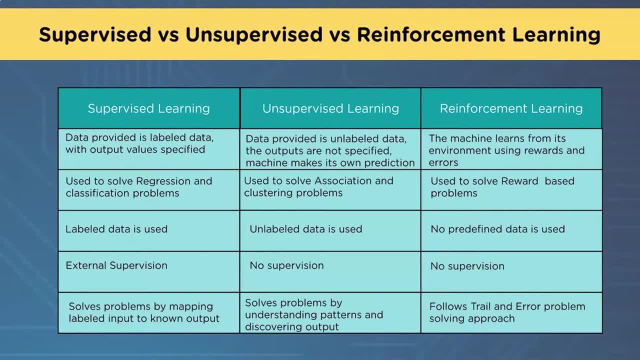 based on its location versus what's next to it. So there's a lot of stuff that goes in with unsupervised learning, And then we're looking at reinforcement learning, Probably the biggest industry in today's market or growing market. It's very infant stage. 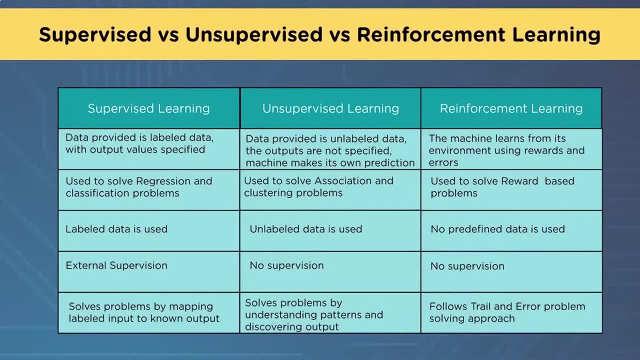 as far as how it works and what it's going to be capable of. The machine learns from its environment, using rewards and errors, Used to solve reward based problems. No predefined data is used, No supervision Follows trail and error problem solving approach. 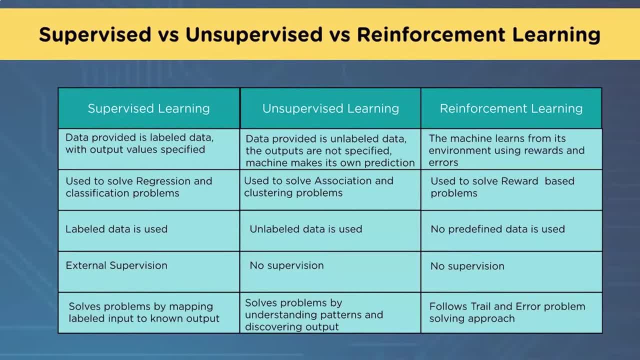 So again we have a random. at first you start with a random- I try this, It works and this is my reward. Doesn't work very well, maybe Trying to get it to do, And you get your reward back. and then it looks at that and says: 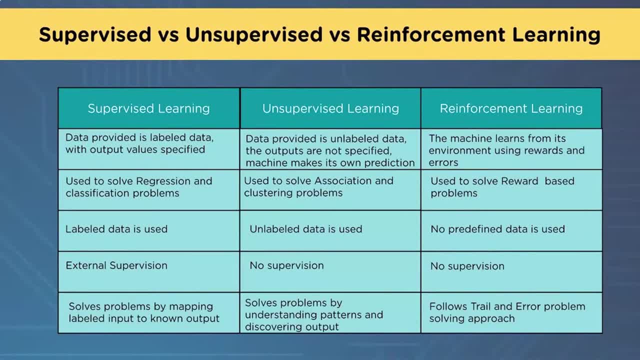 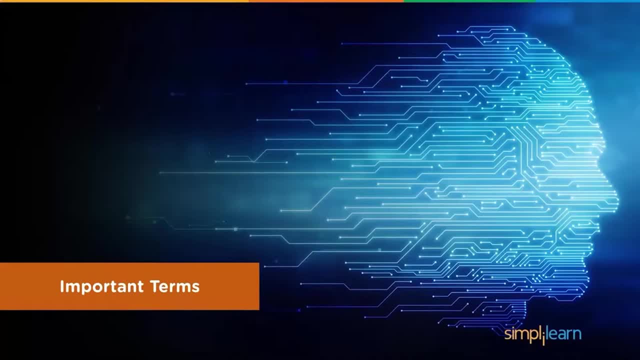 well, let's try something else, And it starts to play with these different things, finding the best route. So let's take a look at important terms in today's reinforcement model, And this has become pretty standardized over the last few years, So these are really good to know. 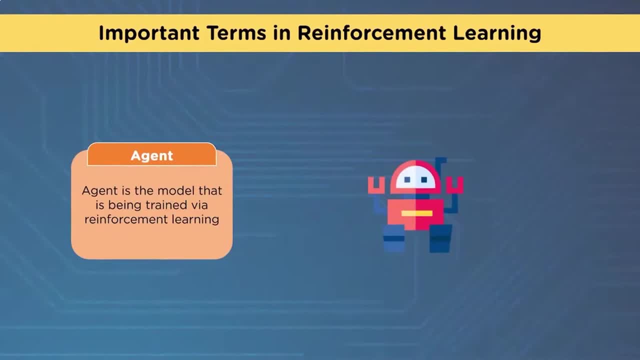 We have the agent. Agent is the model that is being trained via reinforcement learning. So this is your actual entity using a neural network or cue table or whatever Combination thereof. This is the actual agent that you're using. This is the model. 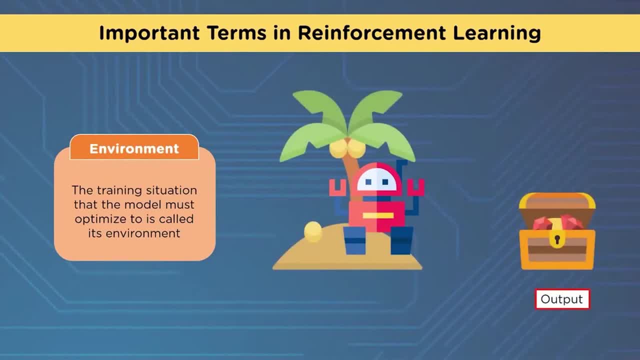 And you have your environment. The training situation that the model must optimize to is called its environment, And you can see here, I guess we have a robot who's trying to get a chest full of gems or whatever, and that's the output, And then you have your action. 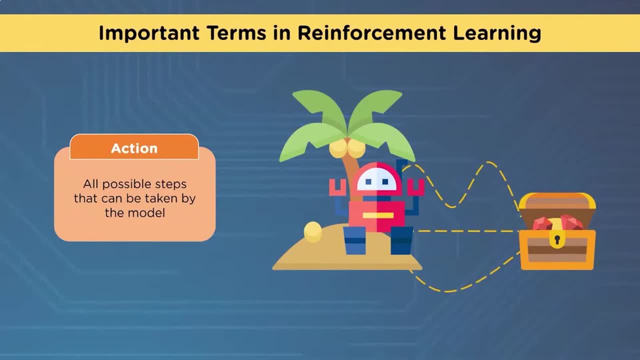 This is all possible steps that can be taken by the model and it picks one action. So we have different routes to get to the chest of diamonds and gems. We have a state, The current position, condition returned by the model, And you could look at this. 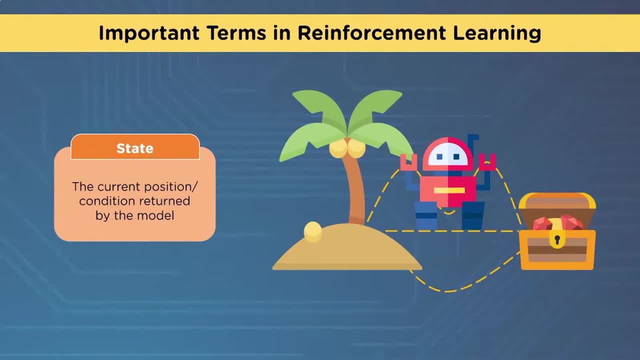 if you're playing like a video game, this is the screen you're looking at. So when you go back here, the environment is the whole game board. So if you're playing one of those Mobius games, you might have the whole game board going on. 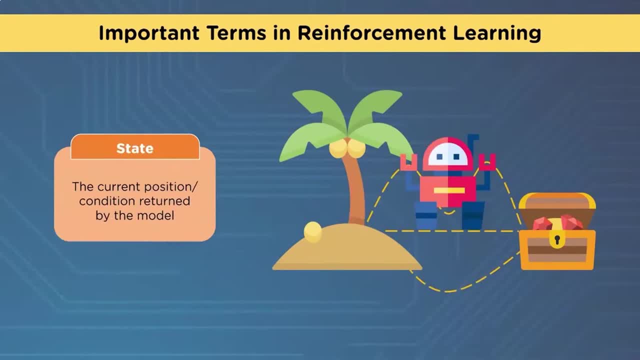 but then you have your current position. Where are you on that game board? What's around that? What's around you? If you were talking about a robot, the environment might be moving around the yard. where it is in the yard and what it can see. 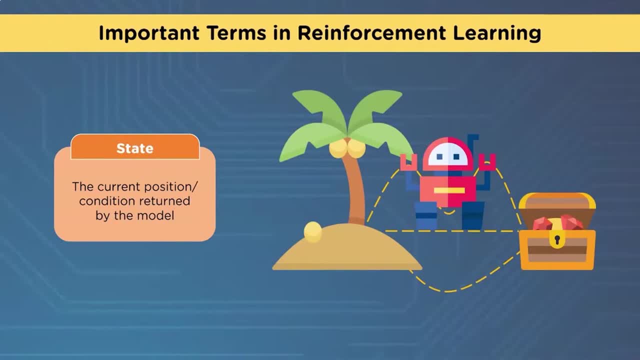 what input it has in that location. that would be the current position condition returned by the model. And then the reward: To help the model move in the right direction, it is rewarded. Points are given to it to appraise some kind of action. So yeah, you did good. 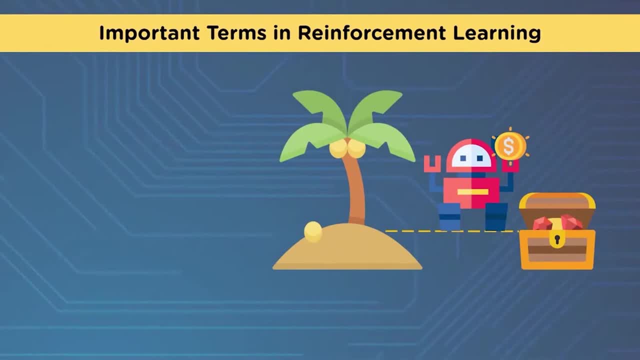 or if it didn't do, as good reward possible. And then policy. Policy determines how an agent will behave at any time. It acts as a mapping between action and present state. This is part of the model. What is your action that you're going to take? 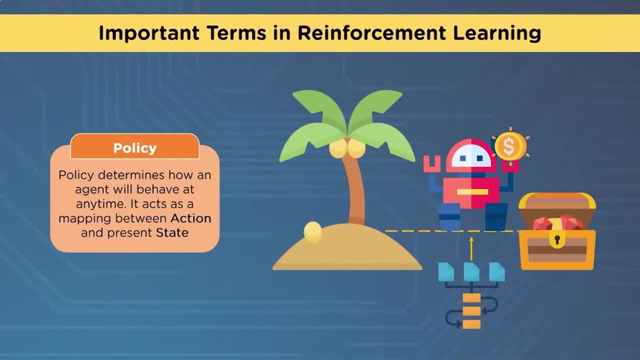 What's the policy you're using to have an output from your agent? One of the reasons they separate policy as its own entity is that you usually have a prediction of different options and then the policy. well, how am I going to pick the best based on those predictions? 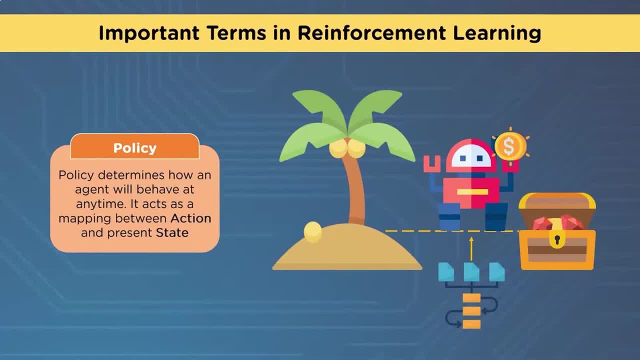 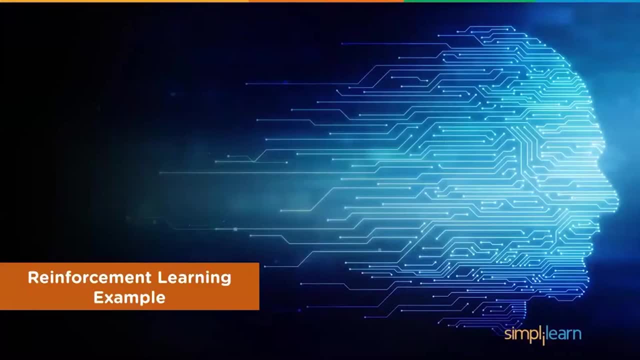 I'm going to guess at different options and we'll actually weigh those options in and find the best option we think will work. So it's a little tricky, but the policy thing is actually pretty cool how it works. Let's go ahead and take a look at a reinforcement learning example. 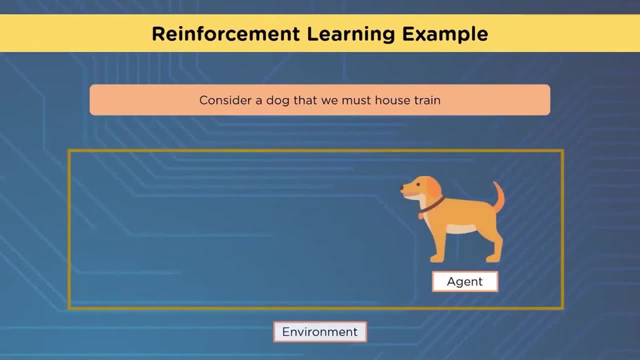 And just in looking at this, we're going to take a look, consider what a dog that we want to train. so the dog would be like the agent puppy or whatever, and then your environment is going to be the whole house or whatever it is where you're training them. 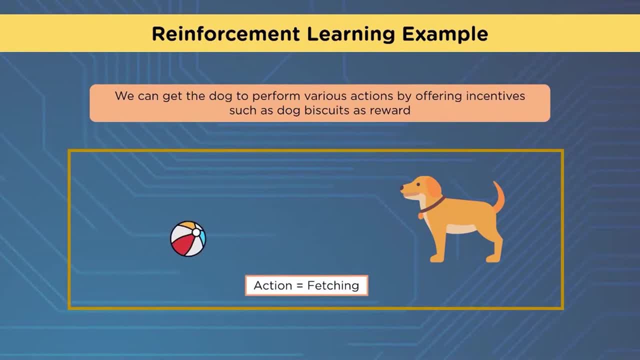 and then you have an action. we want to teach the dog to fetch, so action equals fetching. and then we have a little biscuit so we can get the dog to perform various actions by offering incentives such as a dog biscuit as a reward. the dog will follow a policy. 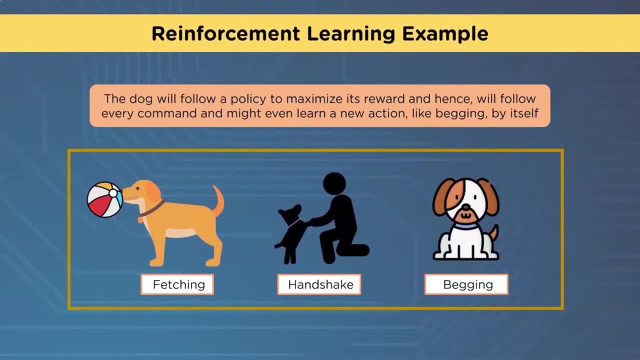 to maximize this reward and hence will follow every command and might even learn new actions. so we start off with fetching. it goes: oh, I get a biscuit for that. it tries something else, and you get a handshake or begging or something like that and it goes: oh, this is also reward based. 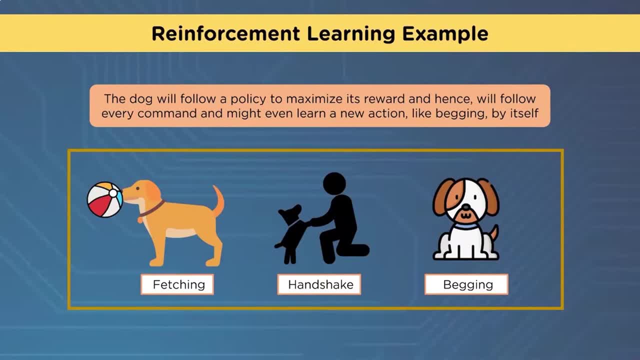 and so it kind of explores things to find out what will bring it his biscuit. and that's very much like how a reinforced model goes, is it looks for different rewards. how can I try different things and find a reward that works? the dog also will want to run around and play. 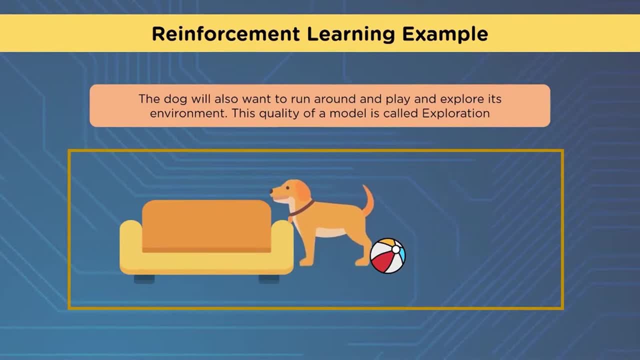 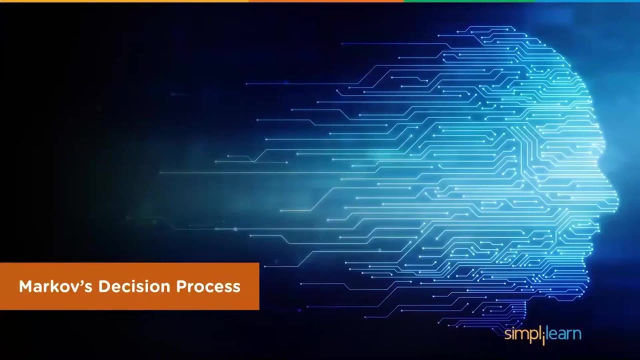 in an explorers environment and the other quality of a model is called exploration, so there is a little randomness going on in exploration. it explores new parts of the house. climbing on the sofa doesn't get a reward. in fact, it usually gets kicked off the sofa. so let's talk a little bit about 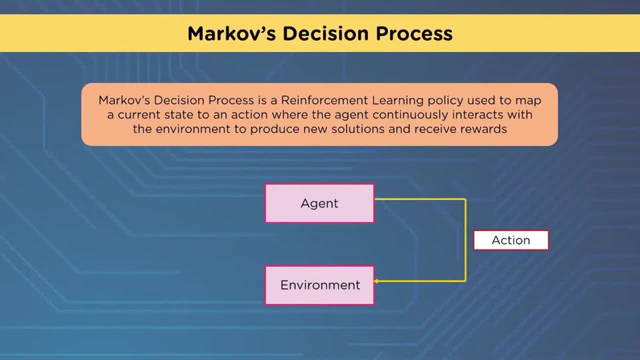 Markov's decision process. Markov's decision process is a reinforcement learning policy used to map a current state to an action where the agent continuously interacts to produce new solutions and receive rewards. and you'll see, here's all of our different vocabulary. we just went over 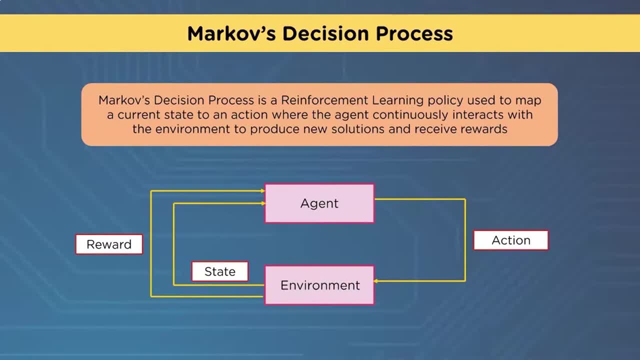 we have a reward or state or agent or environment interaction, and so, even though the environment kind of contains everything, you really, when you're actually writing the program, your environment is going to put out a reward in state that goes into the agent. the agent then looks at this state. 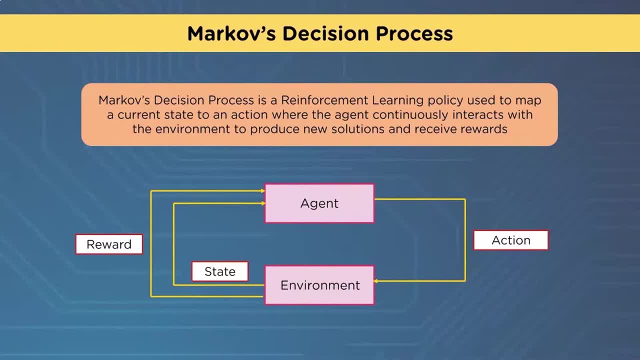 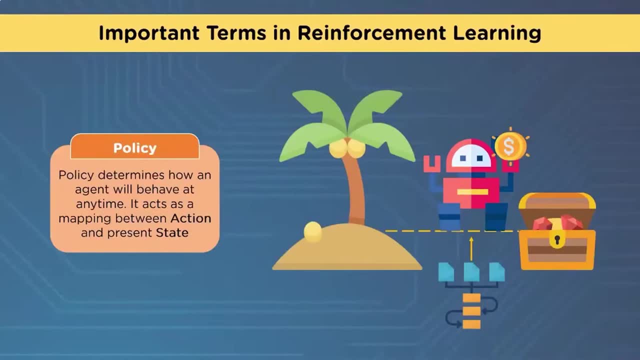 or looks at the reward first and it says, okay, I got rewarded for whatever I just did, or I didn't get rewarded. and then it looks at the state and then it comes back and if you remember from policy, the policy comes in and then we have a reward. 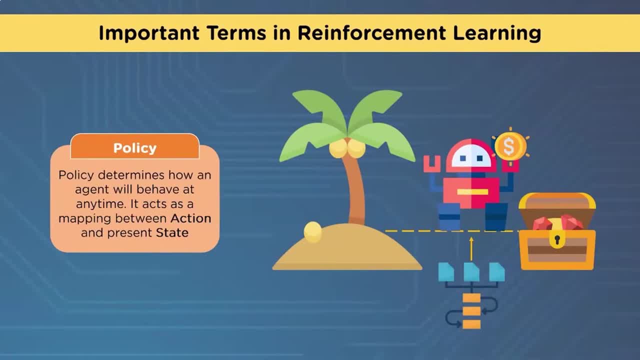 the policy is that part that's connected at the bottom. and so it looks at that policy and it says, hey, what's a good action? that will probably be similar to what I did, or sometimes they're completely random, but what's a good action that's going to bring me? 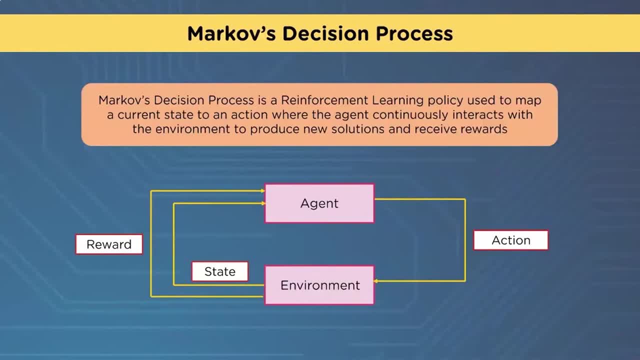 a different reward. so taking the time to just understand these different pieces as they go is pretty important in most of the models today, and so a lot of them actually have templates based on this that you can pull in and start using pretty straight forward as far as 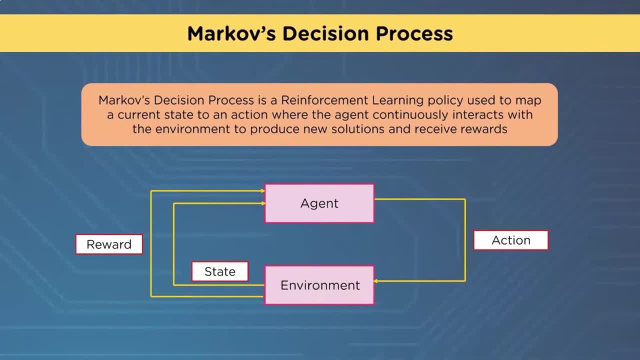 once you start seeing how it works, you can see your environment. it says, hey, the agent did this. if you're a character in a game, this happened. and it shoots out a reward in a state. the agent looks at the reward, looks at the new state and then takes a little guess and says: 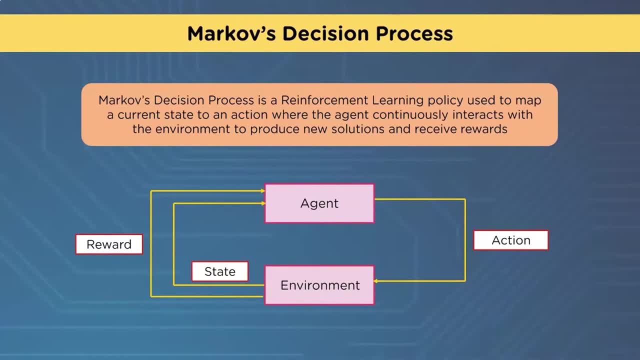 I'm going to try this action and then that action goes back into the environment. it affects the environment. the environment then changes depending on what the action was, and then it has a new state and a new reward that goes back to the agent. so in the diagram shown, 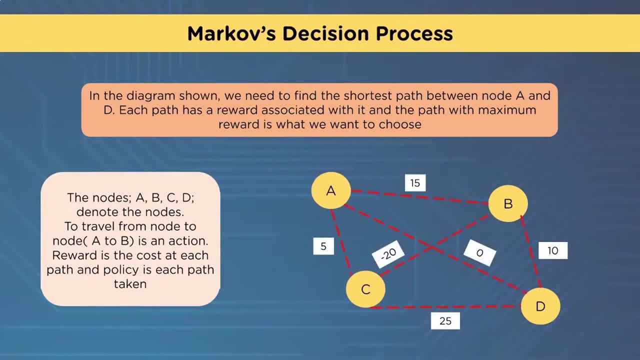 we need to find the shortest path between node A and D. each path has a reward associated with it, and the path with the maximum reward is what we want to choose: the nodes A, B, C, D- to note the nodes that travel from node A to B. 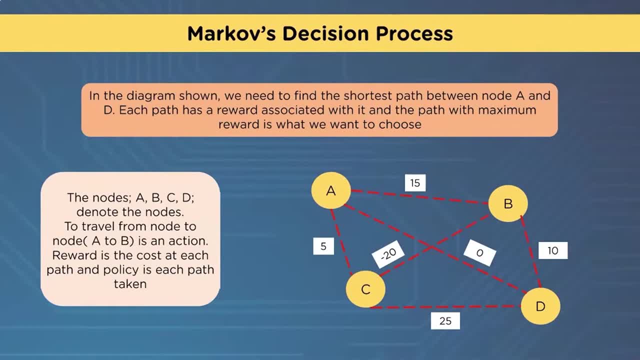 is an action. reward is the cost of each path and policy is each path taken. and you can see here: A can go to B, or A can go to C right off the bat, or it can go right to D. and if you explored all three of these, 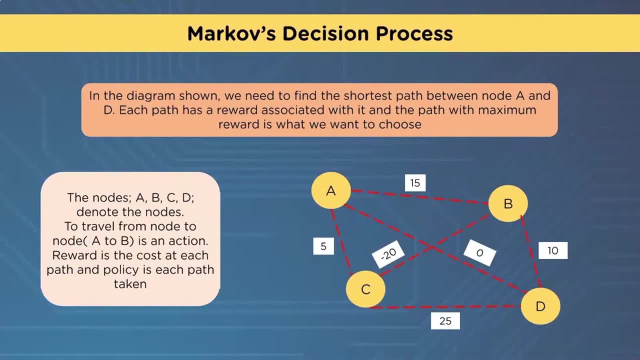 you would find that A going to D was a zero reward. A going to C and D would generate a different reward. or you could go A, C, B, D. there's a lot of options here, and so when we start looking at this diagram, you start to realize. 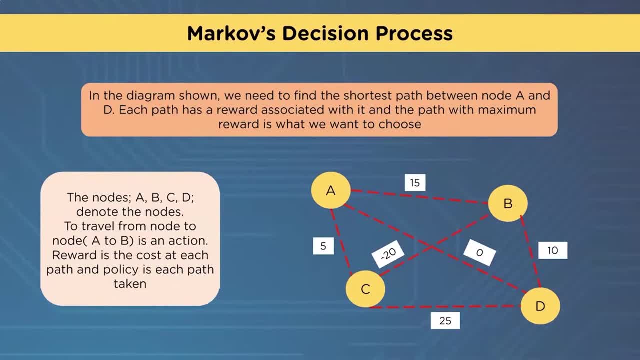 that even though today's reinforced learning models do really good at finding an answer, they end up trying almost all the different directions, you see, and so they take up a lot of work or a lot of processing time for reinforcement learning. they're right now in their infant stage. 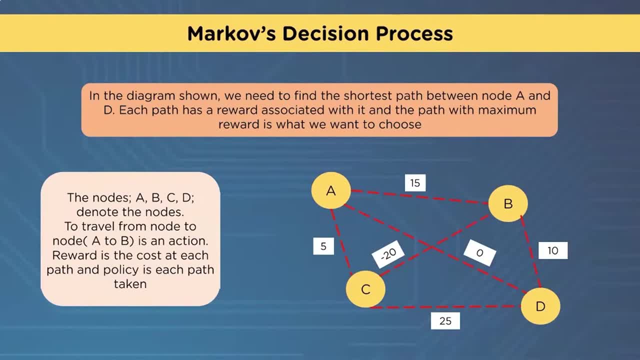 and they're really good at solving simple problems. so we'll take a look at one of those in just a minute, in a tic-tac-toe game, but you can see here. once it's gone through these and it's explored, it's going to find the A, C, D. 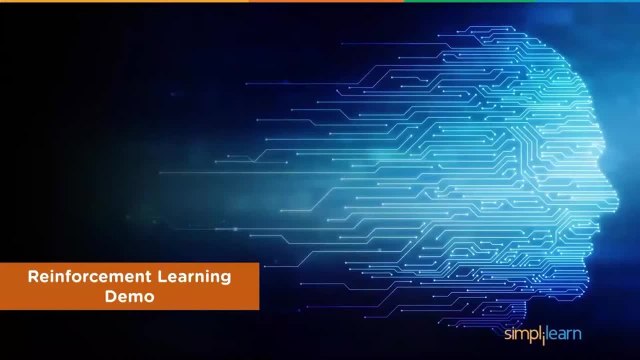 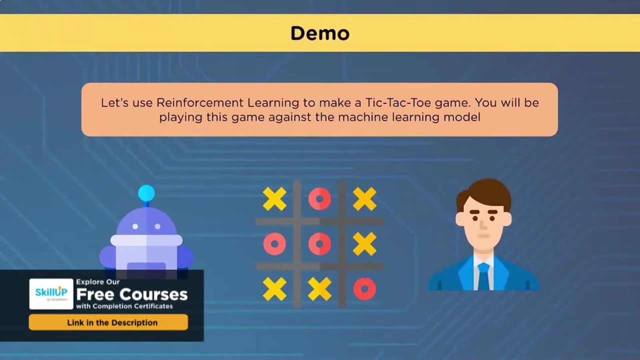 is the best reward. it gets a full 30 points for it. so let's go ahead and take a look at a reinforcement learning demo. in this demo, we're going to use reinforcement learning to make a tic-tac-toe game. you'll be playing this game against the machine learning model. 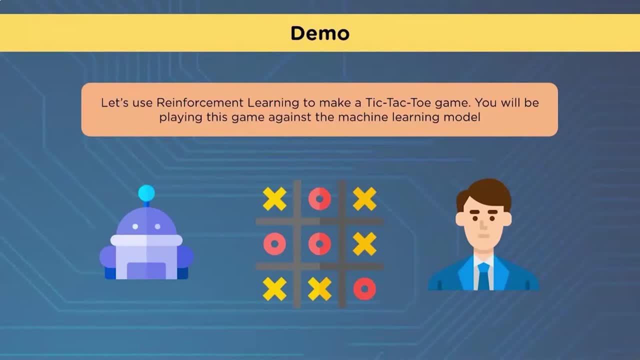 and we'll go ahead. we're doing it in Python, so let's go ahead and go through. not always I actually have a lot of Python tools. let's go through Anaconda, which will open up a Jupyter notebook. seems like a lot of steps, but it's worth it to keep all my stuff separate. 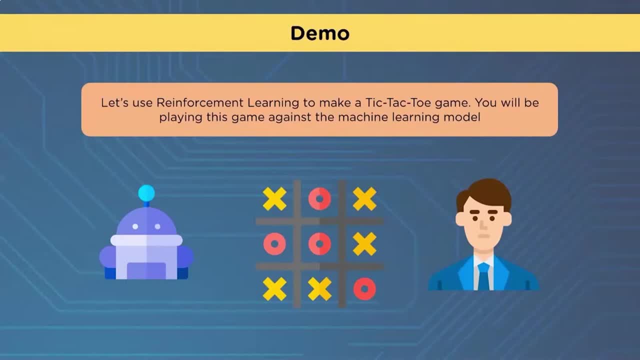 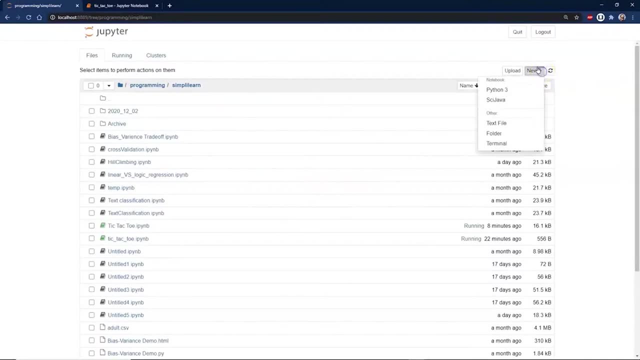 and it also has a nice display when you're in the Jupyter notebook for doing Python. so here's our Anaconda navigator. I open up the notebook, which is going to take me to a web page, and I've gone in here and created a new Python folder. 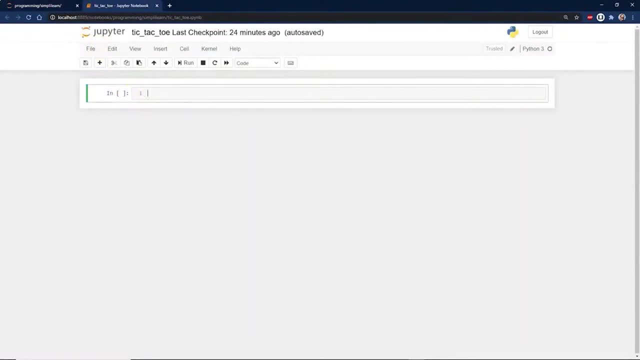 in this case, I've already done it and enabled it to change the name to tic-tac-toe. and then, for this example, we're going to go ahead and import a couple things. we're going to import numpy, as in p. we'll go ahead and import pickle. 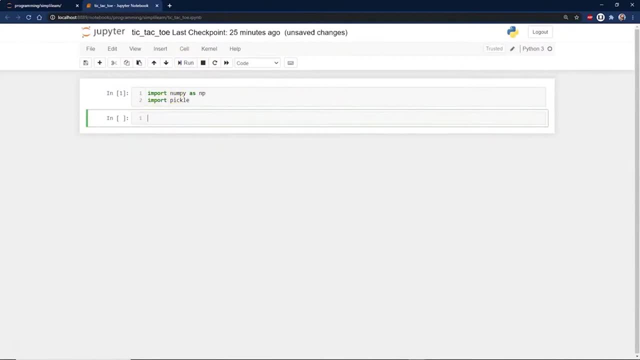 numpy, of course, is our number array, and pickle is just a nice way sometimes for storing different information, different states that we're going to go through on here, and so we're going to create a class called state. we're going to start with that and there's a lot of 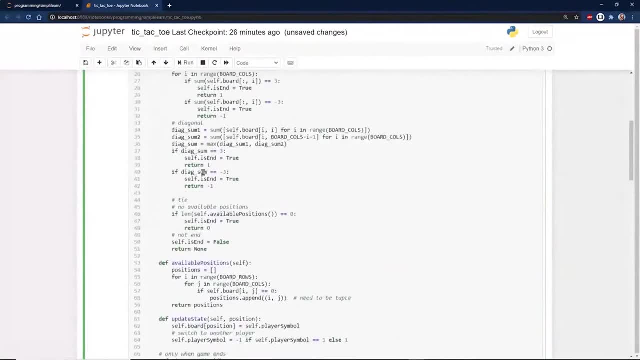 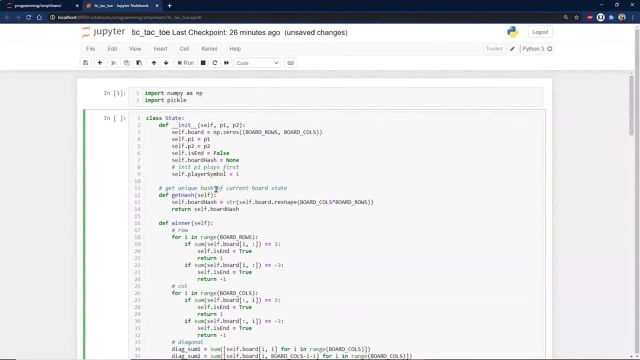 lines of code to this class that we're going to put in here. don't let that scare you too much. there's not as much here. it looks like there's going to be a lot here, but there really is just a lot of setup going on in our class state. 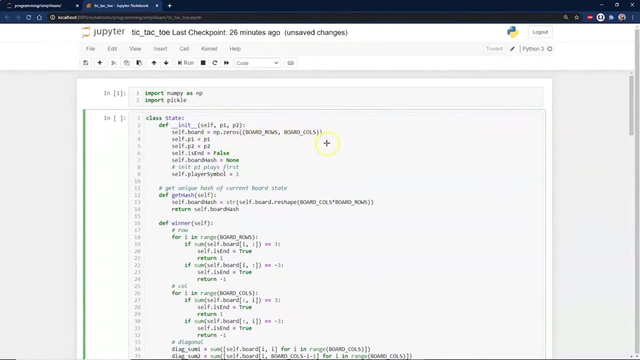 and so we have up here. we're going to initialize it. we have our board. it's a tic-tac-toe board, so we're only dealing with nine spots on the board. we have player one. player two is in. we're going to create a board hash. 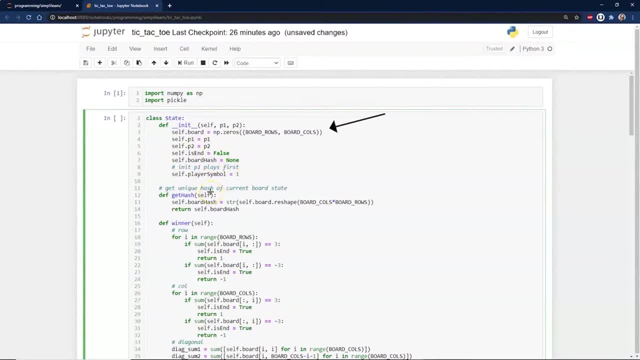 we'll look at that in just a minute. we're just going to store some information in there. symbol of player equals one, so there's a few things going on. as far as the initialization, then something simple. we're just going to get the hash of the board. 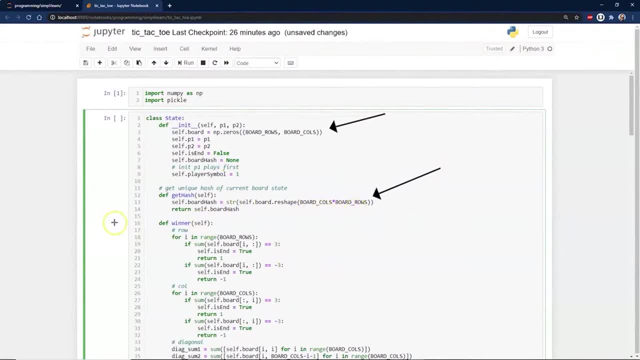 get the information from the board on there, which is columns and rows. we want to know when a winner occurs, so if you get three in a row, that's what this whole section here is for. let me go ahead and scroll up a little bit and you can get a copy of this code. 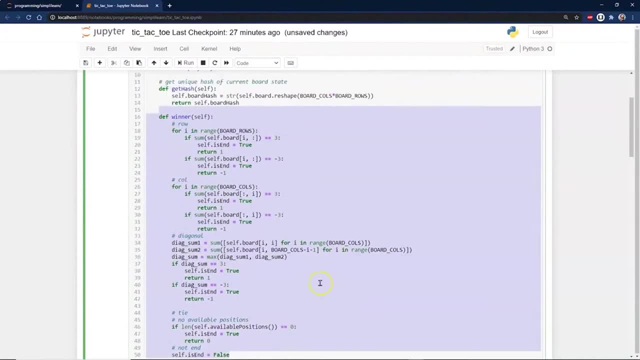 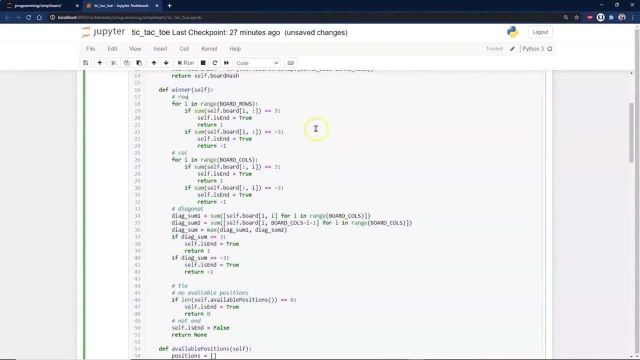 if you send a note over to simplylearn, we'll send you over this particular file and you can play with it yourself and see how it's put together. I don't want to spend a huge amount of time on this, because this is just some real general python coding. 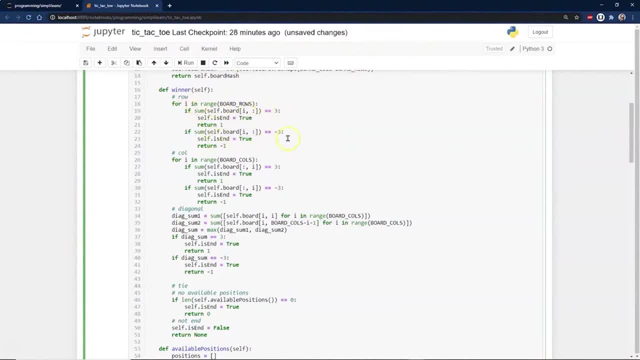 but you can see, here we're just going through all the rows and you add them together and if it equals three, three in a row, same thing with columns, so you've got to check the diagonal. that's what all this stuff does here. it just goes through the different areas. 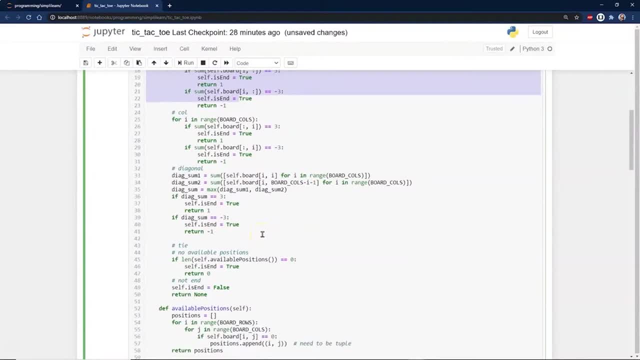 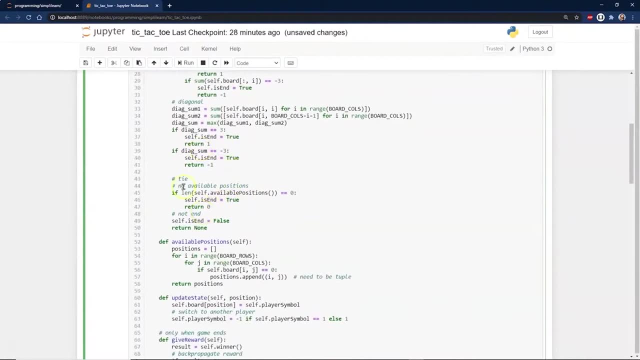 actually let me go ahead and put there we go, and then it comes down here and we do our sum and it says true minus three. it just says: did somebody win or is it a tie? so you've got to add up all the numbers on there anyway. 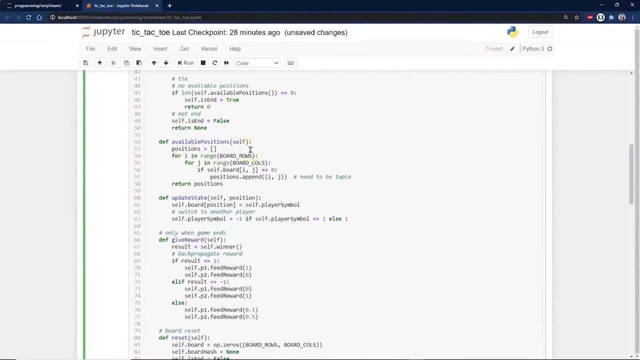 just in case they're all filled up. and next we also need to know available positions. these are ones that no one's ever used before, so if somebody tries something, or the computer tries something, it's not going to give it an illegal move. that's what the available positions is doing. 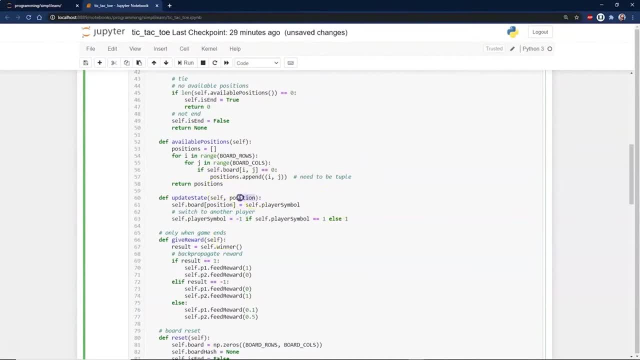 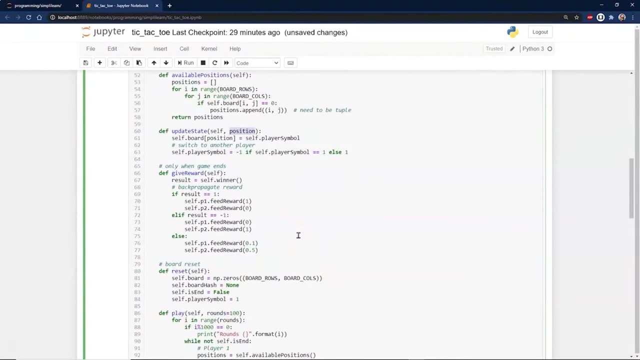 then we want to update our state so you have your position going in. we're just sending in the position that you just chose and you'll see there's a little user interface we put in there where you can pick the row and column in there and again, 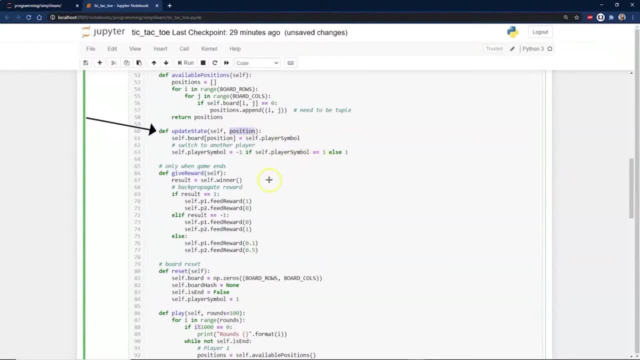 this is a lot of code, so really it's kind of a thing you'd want to go through and play with and just read through it and get a copy of it- a great way to understand how this works. and here is a given reward, so we're going to give a reward. 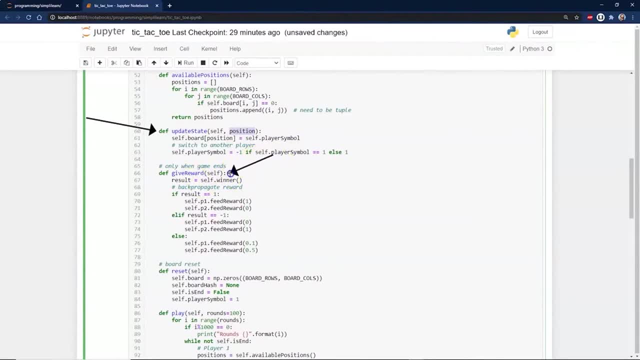 result equals self winner. this is one of the hearts of what's going on here. we have a result selfwinner, so if there's a winner, then we have a result. if the result equals one, here's our feedback. if it doesn't equal one, then it gets a zero. 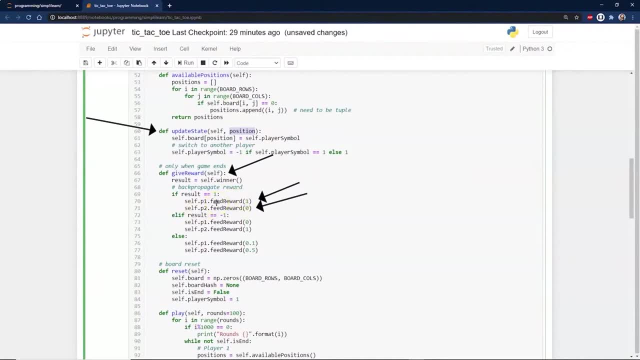 in this particular case, if it wins- and that's important to know, because different systems of reinforced learning do rewarding a lot differently depending on what you're trying to do. this is a very simple example with a 3x3 board, imagine if you're playing a video game. 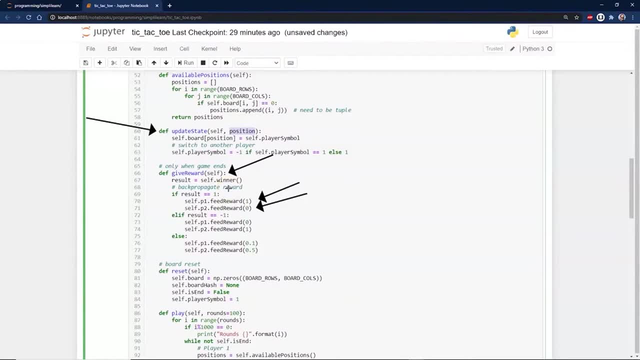 certainly you only have so many actions, but your environment is huge. you have a lot going on in the environment and suddenly a reward system like this is going to be. it's going to have to change a little bit. it's going to have to have different rewards. 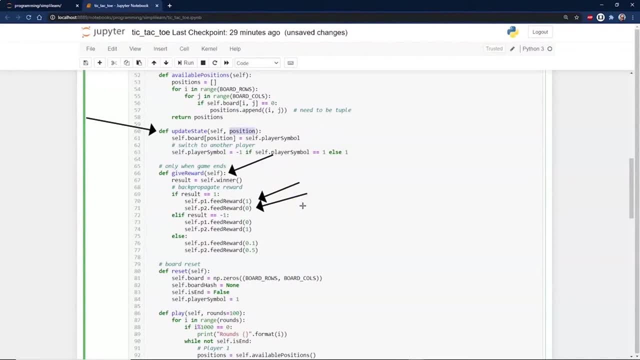 and different setup, and there's all kinds of advanced ways to do that. as far as weighing, you add weights to it, and so they can add the weights up, depending on where the reward comes in. so it might be that you actually get a reward. in this case, you get the reward. 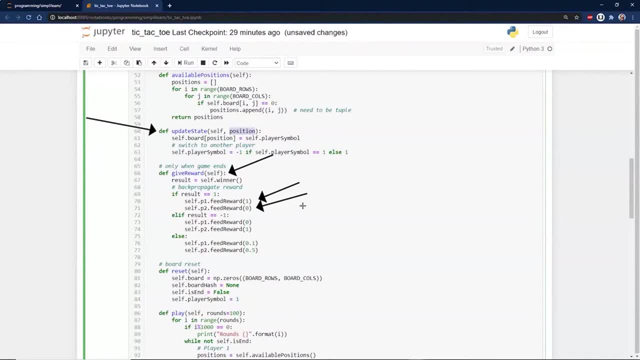 at the end of the game. I'm spending just a little bit of time on this because this is an important thing to note, but there's different ways to add up those rewards, so if you're on the same path, the first reward is going to be weighed a little bit less. 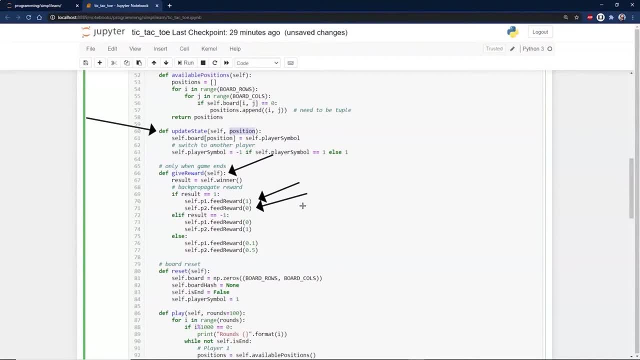 than the last reward, because the last reward is actually winning the game, or scoring, or whatever it is, so this reward system gets really complicated in some of the more advanced setups. in this case, though, you can see right here that they give a .1 and a .5 reward. 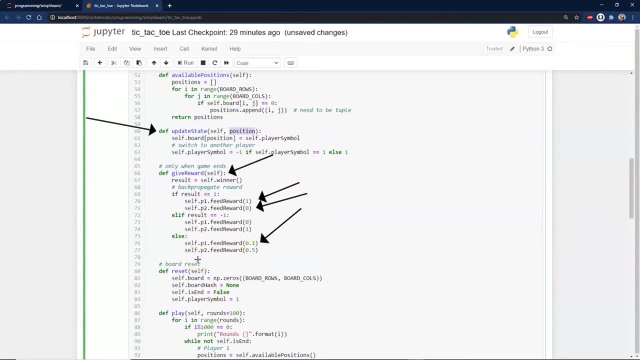 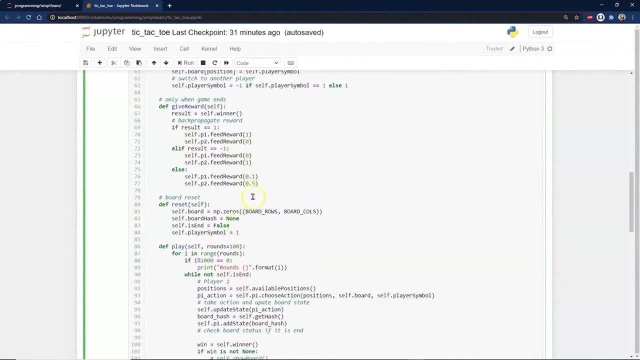 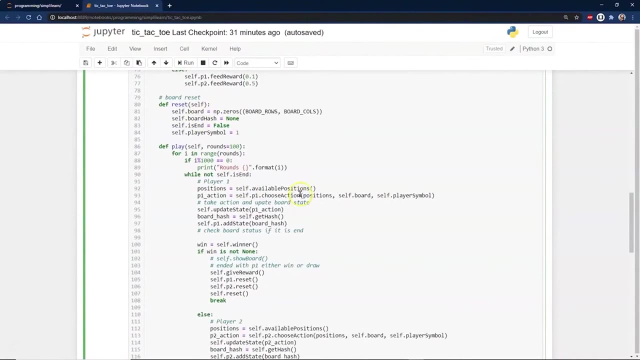 just for getting picking the right value and something that's actually valid. so rewards again, that's like key, it's huge. how do you feed the rewards back in? then we have a board reset. that's pretty straight forward. it just goes back and resets the board to the beginning. 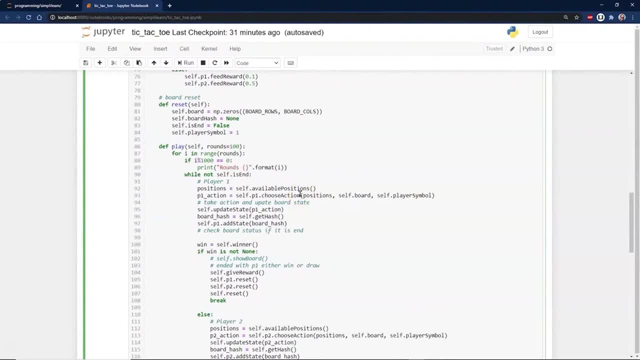 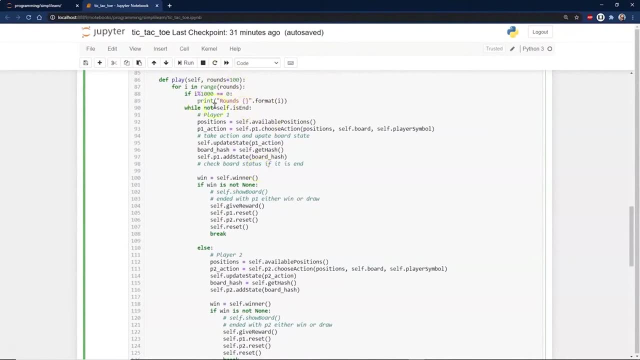 because it's going to try out all these different things while it's learning. it's going to do it by trial and error, so you have to keep resetting it. and then, of course, there's the play. we want to go ahead and play. rounds equals 100. 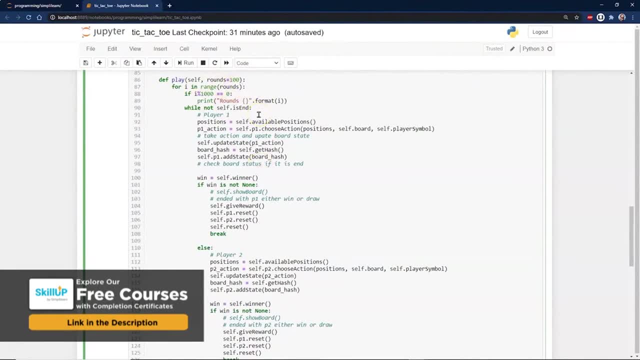 depends on what you want to do on here to higher level, but this is just going to go through and you'll see in here that we have player 1 and player 2. this is the computer playing itself, one of the more powerful ways to learn to play a game. 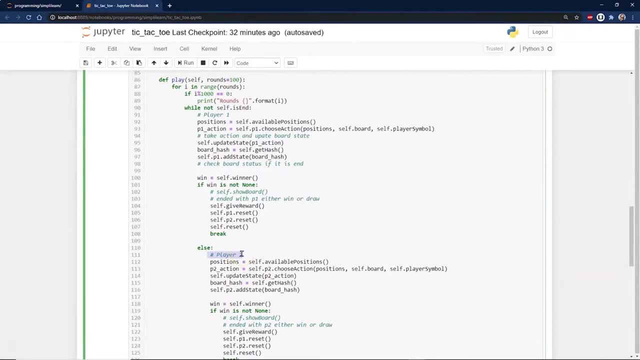 or even learn something. that isn't a game is to have two of these models that are basically trying to beat each other and so they keep finding, explore new things. this one works for this one, so this one tries new things. we've seen this in chess. I think it was a big one. 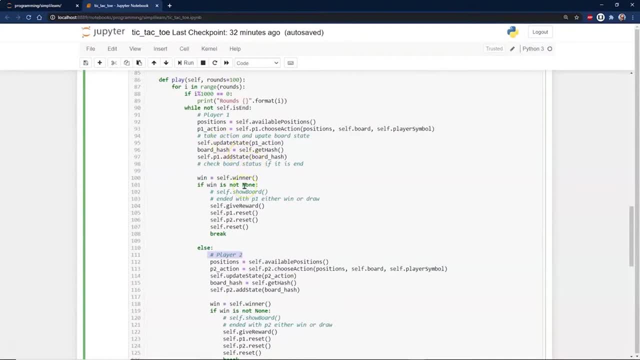 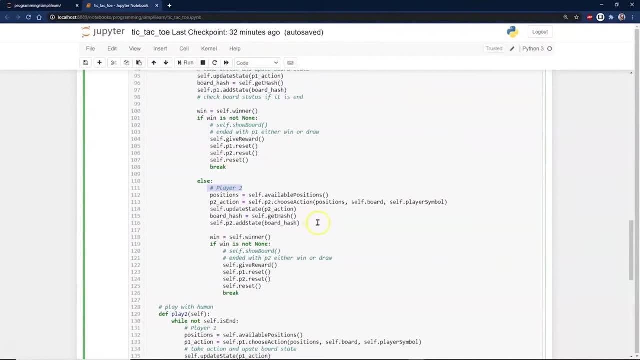 where they had the two players in chess with reinforcement learning. it was one of the ways they trained one of the top computer chess playing algorithms. so this is just what this is: it's going to choose an action, it's going to try something, and the more it tries stuff. 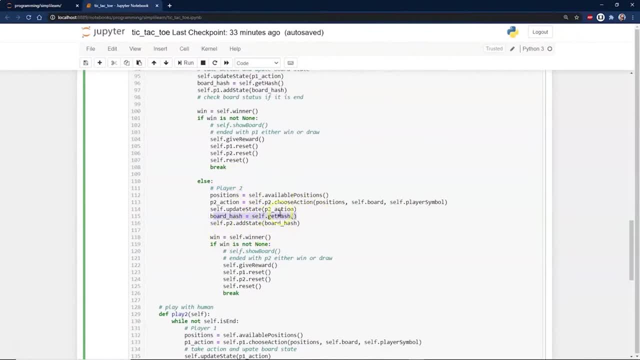 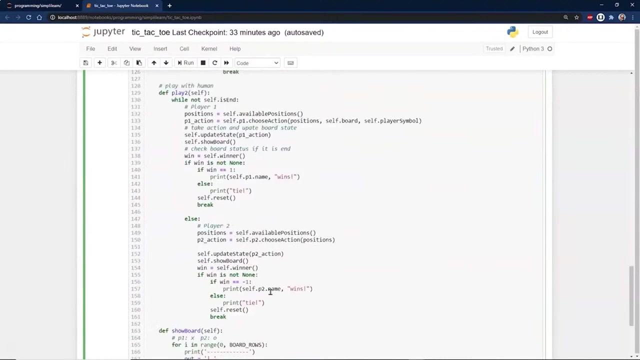 the more we're going to record the hash. we actually have a board hash where you can get the hash set up on here where it stores all the information and then once you get to it, you do a win. one of them wins, it gets the reward. then we go back and reset and try again. 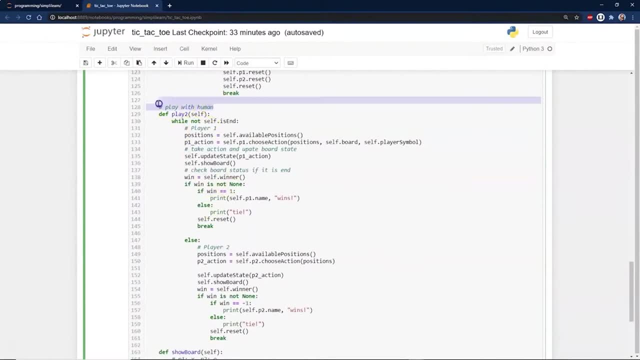 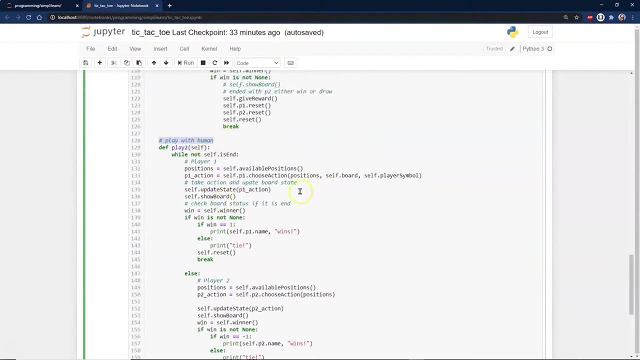 and then kind of the fun part we actually get down here is we're going to play with a human, so we'll get a chance to come in here and see what that looks like when you put your own information in and then it just comes in here. 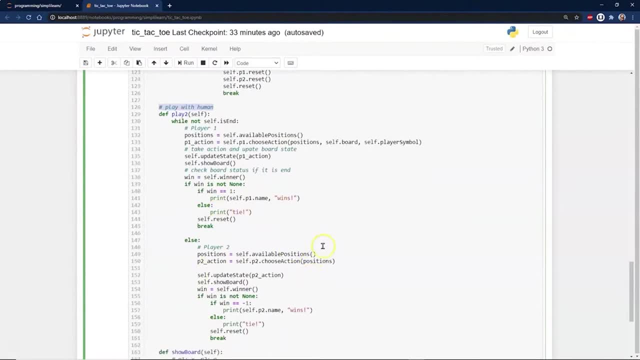 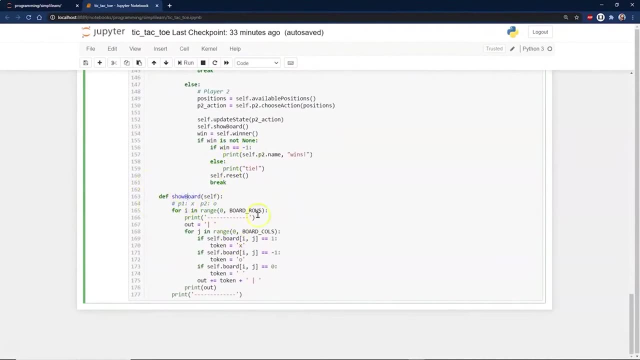 and does the same thing it did above. it gives it a reward for its things, or sees if it wins or ties, looks at available positions. it's going to show the board, so it's going to print the board out each time. really, as an integration, it's not that exciting. 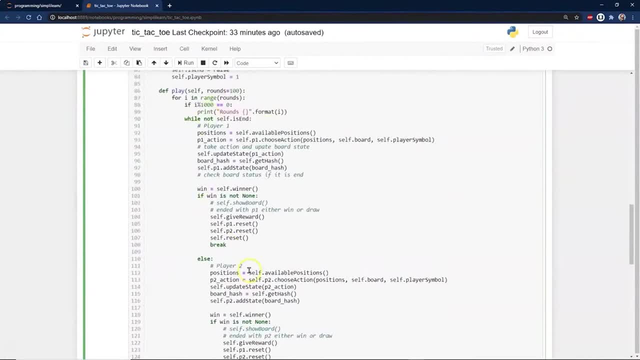 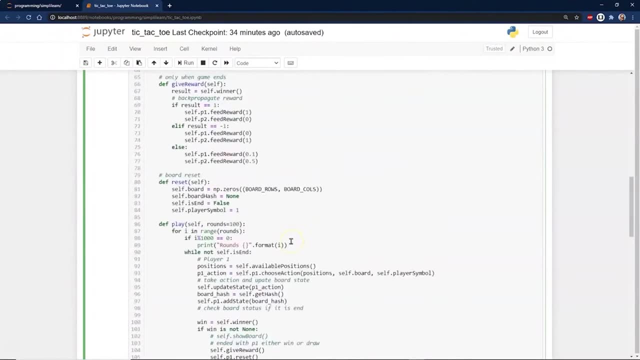 what's exciting in here is one looking at this reward system. whoops play one more up. the reward system is really the heart of this. how do you reward the different set up? and the other one is when it's playing. it's got to take an action. 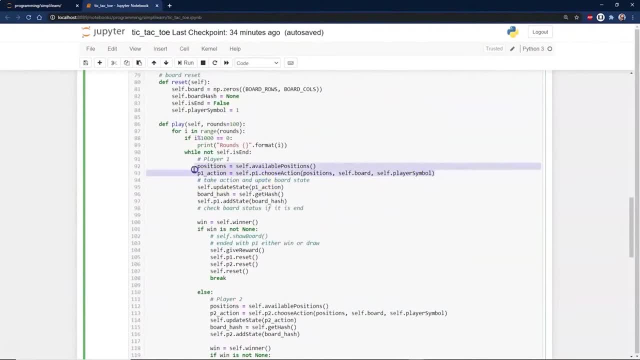 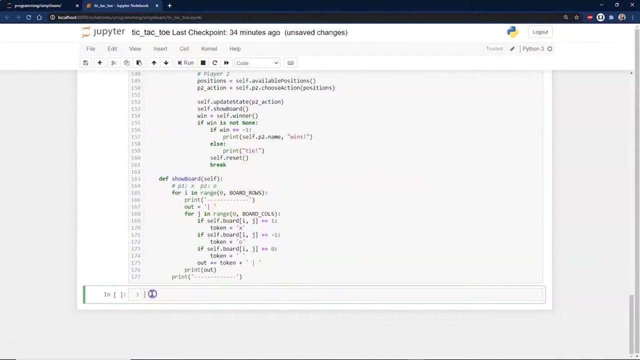 and so what it chooses for an action is also the heart of reinforcement learning. how do we choose that action? and those are really key to right now where reinforcement learning is in. today's technology is figuring this out, how do we reward it and how do we guess the next best action? 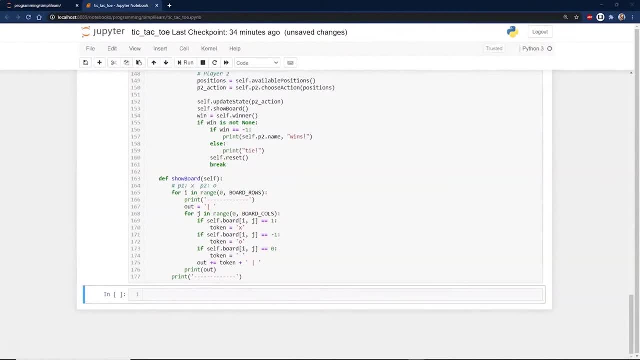 so we have our environment and you can see the environment or the state which is kind of like what's going on. we're going to return the state, depending on what happens. we can create our agent, in this case our player. so each one is grab that and so we look at a class player. 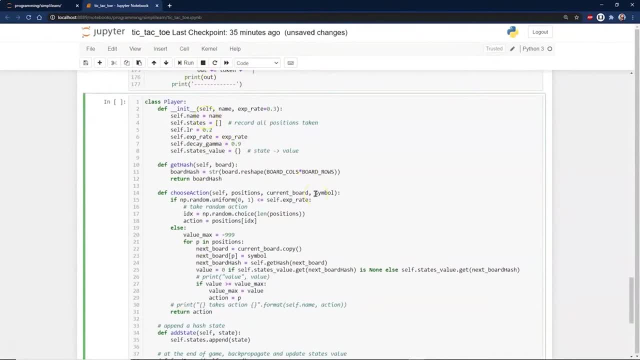 this is where a lot of the magic is really going on. how is this player figuring out how to maneuver around the board? and then the board, of course, returns a state that it can look at and reward. so we want to take a look at this. we have name self state. 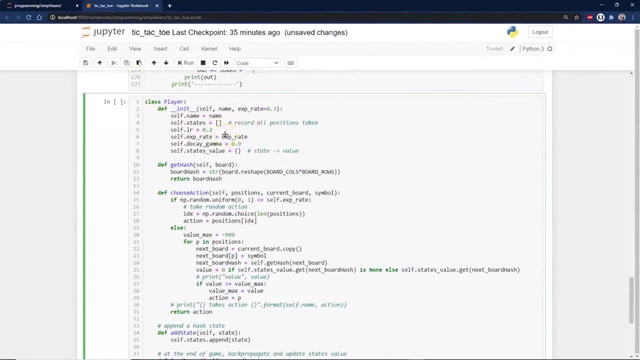 this is class player. when we say class player, we're not talking about a human player, we're talking about just the computer players, and this is kind of interesting. so remember I told you, depending on what you're doing, there's going to be a decay gamma explore rate. 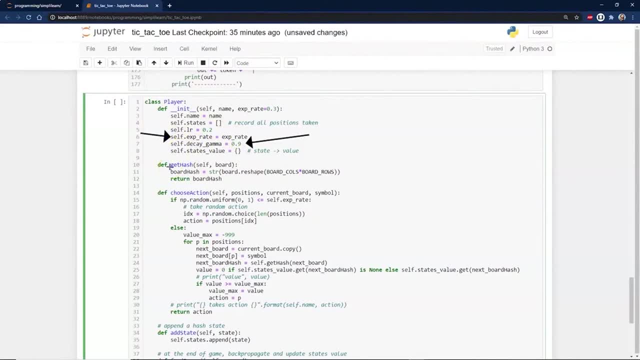 these are. what I'm talking about is how do we train it. as you try different moves, it gets to the end. the first move is important, but it's not as important as the last one, and so you could say that the last one has the heaviest weight. 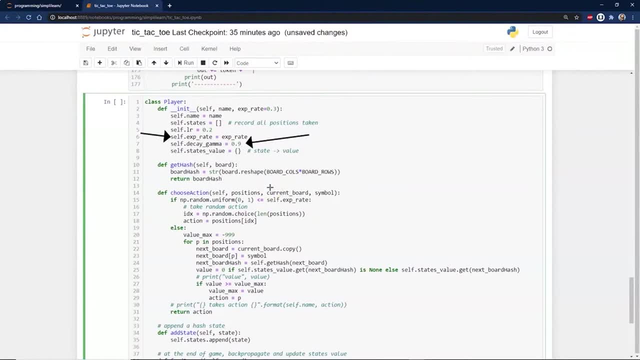 and then, as you get there, the first move gives you a 5 reward, the second gives you a 2 reward and the third one gives you a 10 reward, because that's the final ending. you got it. the 10 is going to count more than the first step. 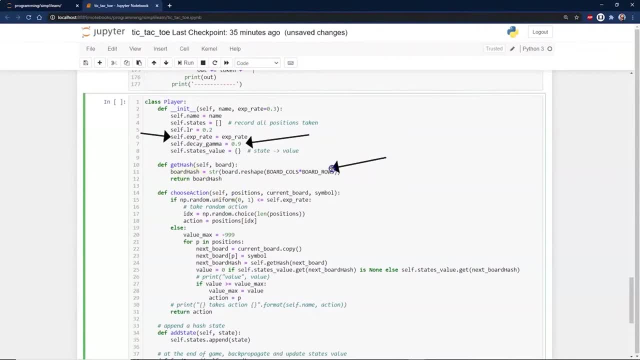 and here's our: we're going to get the board information coming in and then choose an action. this was the second part that I was talking about. that was so important. so once you have your training going on, we have to do a little randomness: our NP random uniform. 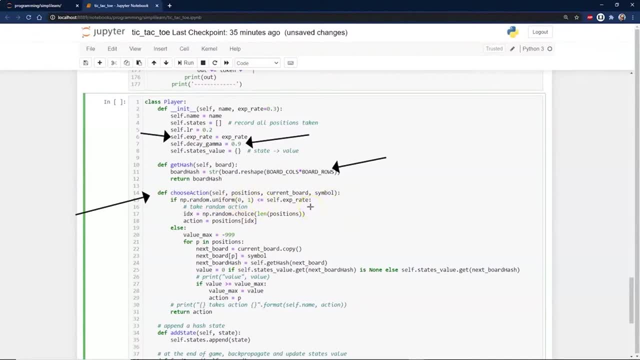 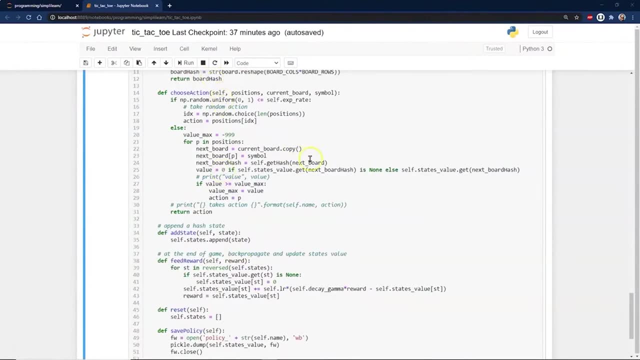 so it's picking out a random number, take a random action. this is going to just pick which row and which column it is, and so choosing the action, this one. you can see we're just doing random states, choice, length of positions, action position and then it skips in there. 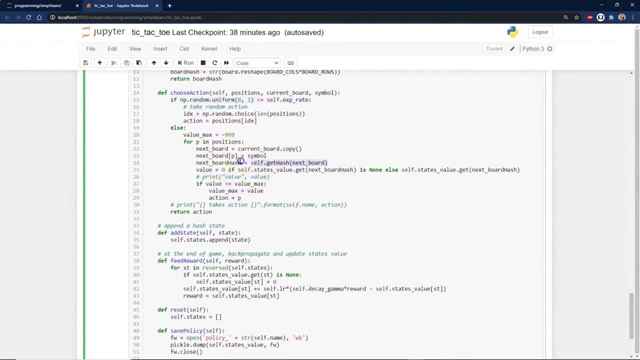 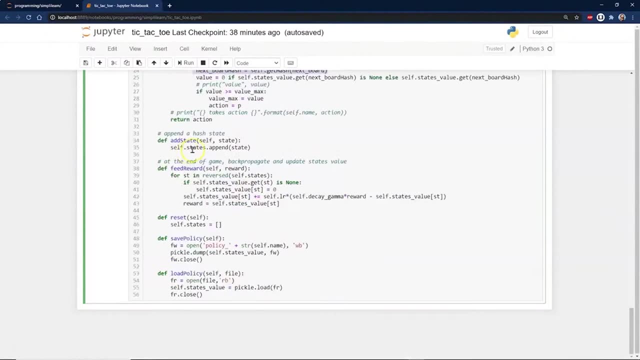 and takes a look at the board for P and positions. it's actually storing the different boards each time you go through and see what it did so it can properly weigh the values, and this simply just appends a hash state. what's the last state? append it to our states on here. 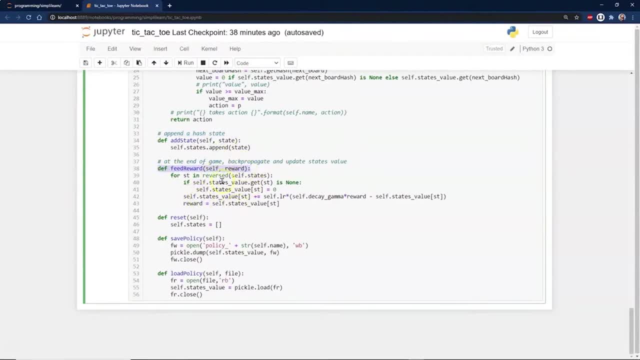 here's our feedback rewards. the reward comes in and it's going to take a look at this and say: is it none? what is the reward? and here is that formula. remember I was telling you about up here. that was important because it has decay gamma times the reward. 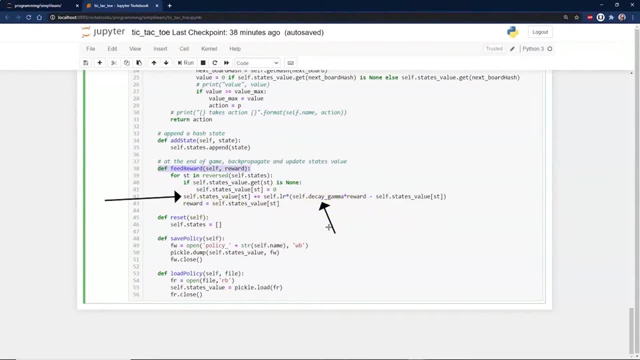 as it goes through each step, and this is really important. this is kind of the heart of this, of what I was talking about earlier. you have step 1 and this might have a reward of 2. you have step 2. I probably should have done ABC. 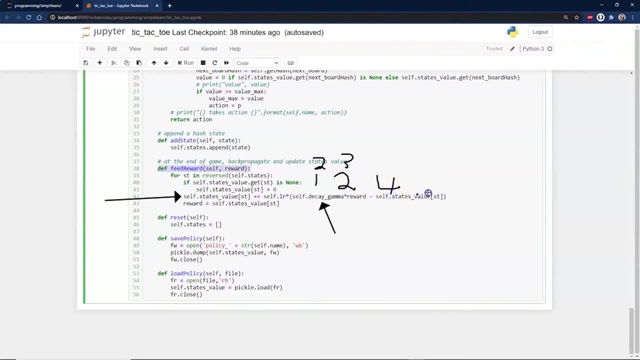 this has a step 3, step 4 and so on, until you get to step in and this might have a reward of 10. so, reward of 10, we're going to add that, but we're not adding. let's say this one right here. let's say this reward here: 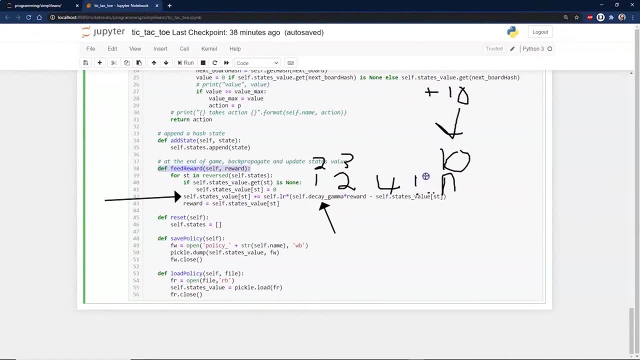 right before 10 was. let's say it's also 10. that just makes the math easy. so we had 10 and 10, we had 10. this is 10 in whatever it is, but this time it's .9, so instead of putting a full 10 here, 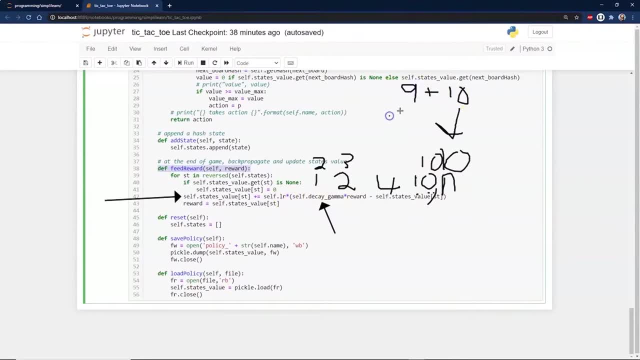 we only do 9, that's .9 times 10, and so this formula, as far as the decay times the reward minus the cell state value, it basically adds in. it says here's 1 or here's 2. I'm sorry, I should have done this ABC. 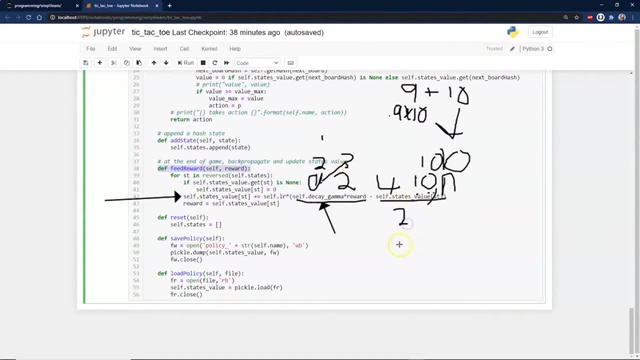 it would have been easier. so the first move goes in here and it puts 2 in here. then we have our self set up on here and we have the answer in the math. but this is really the key: how do we train our states and we want the final state? 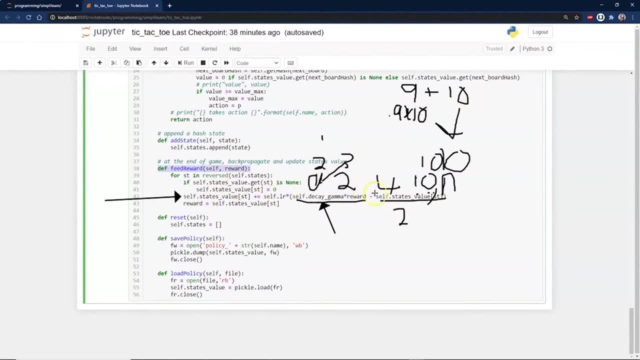 the win to get the most points. if you win, you get the most points and the first step gets the least amount of points. so you're really training this almost in reverse. you're training it from the last place where you have, like it says: this is now where I need to sum up my rewards. 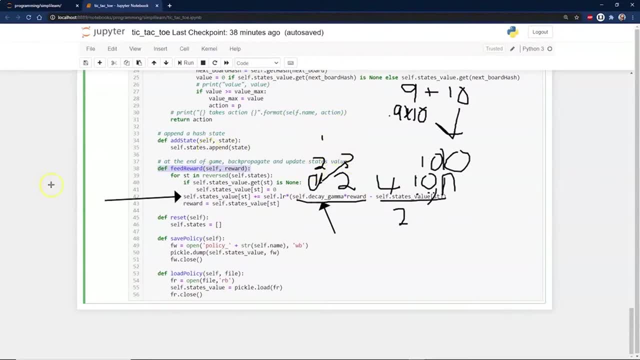 and I want to sum them up, going in reverse, and I want to find the answer in reverse- kind of an interesting play on the mind when you're trying to figure this stuff out- and of course we want to go ahead and reset the board down here. save the policy. 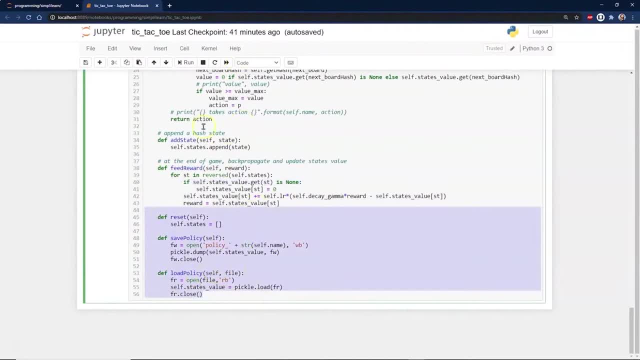 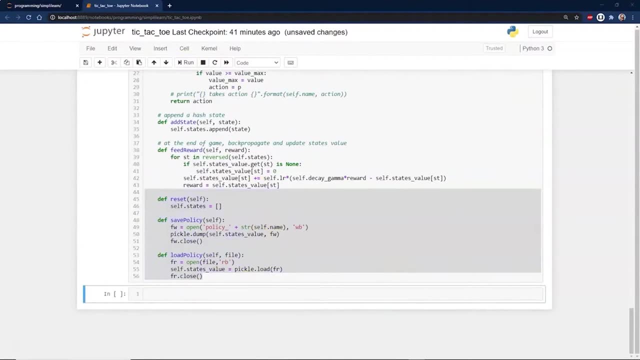 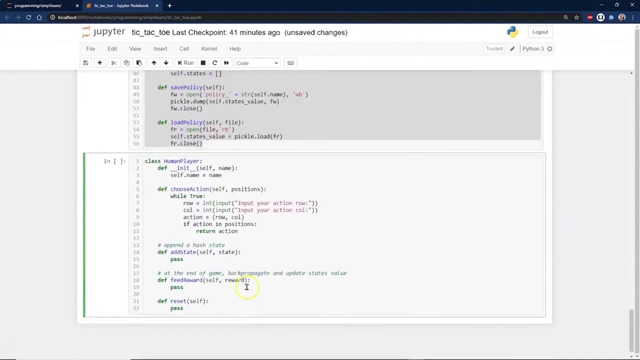 load policy. these are the different things that are going in between the agent and the state. to figure out what's going on, let's go ahead and load that up and then, finally, we want to go ahead and create a human player, and the human player is going to be a little different. 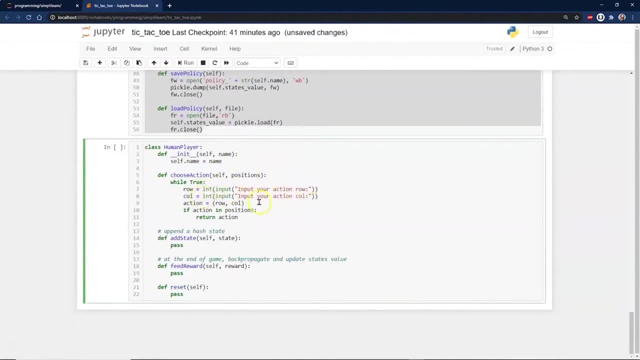 in that you can choose an action row and column. here's your action. if action is, if action in positions- meaning positions that are available- you return the action. if not, it just keeps asking you until you get the action that actually works, and then we're going to go ahead. 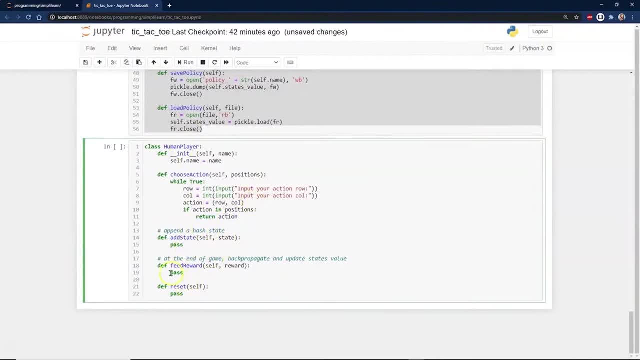 and append to the hash state, which we don't need to worry about because it returns the action up here and feed forward again. this is because it's a human at the end of the game: bat, propagate and update state values. this part isn't being done because 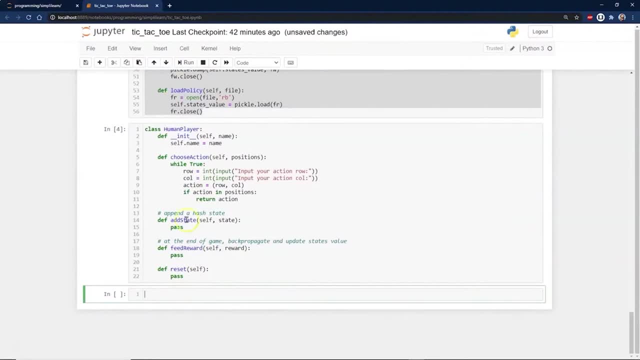 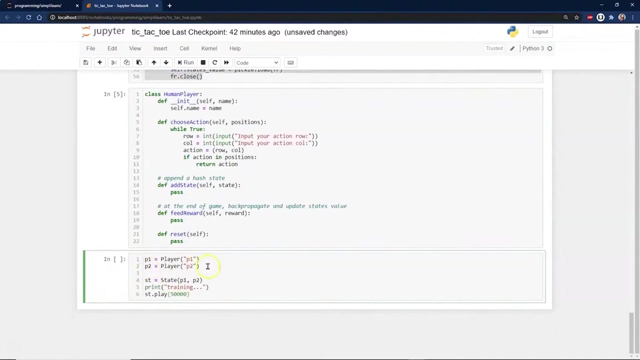 it's not programming the model. the model is getting its own rewards. so we've gone ahead and loaded this in here. so here's all our pieces, and the first thing we want to do is set up p1 player1, p2 player2, and then we're going to send our 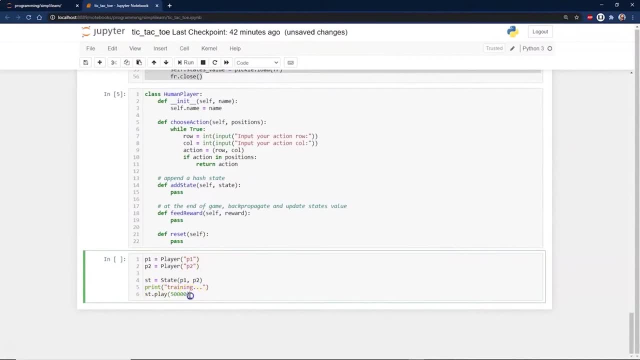 players to our state. so now it has p1, p2 and it's going to play 50,000 rounds. now we can probably do a lot less than this and it's not going to get the full results. in fact, you know what? let's go ahead and just do 5. 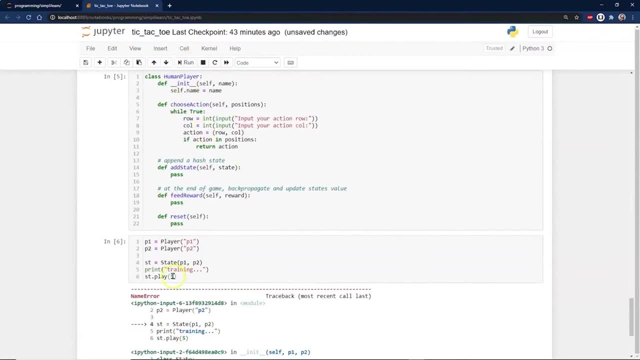 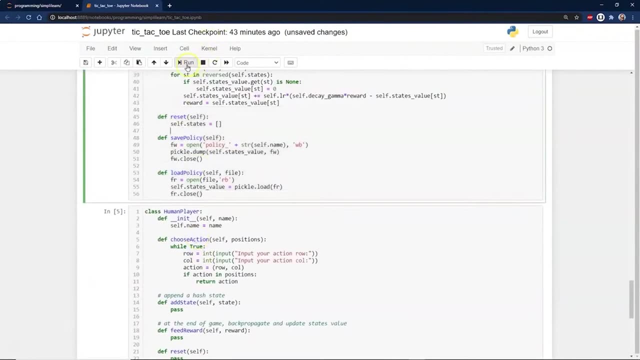 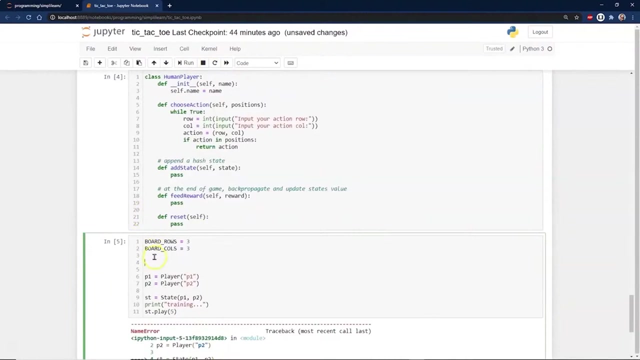 just to play with it, because I want to show you something here. oops, somewhere in there I forgot to load something. there we go. I forgot to run this. oops, forgot a reference there for the board rows and columns 3x3. there's actually in the state. 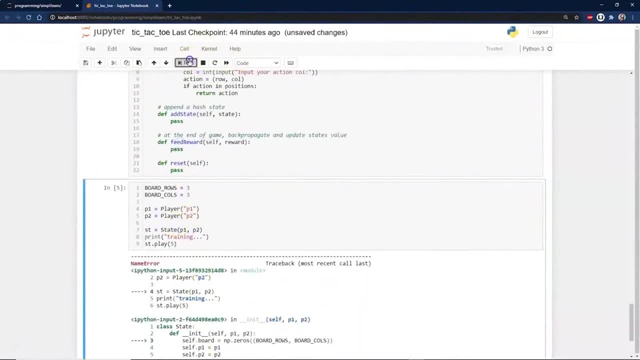 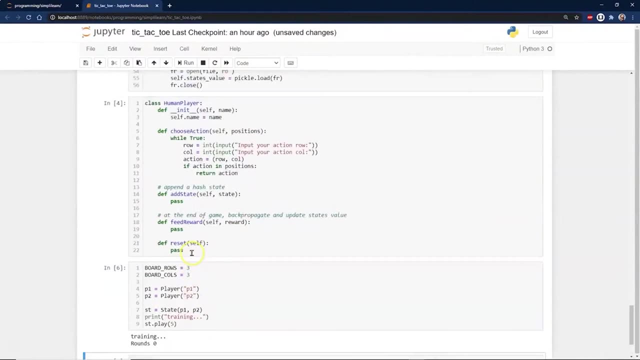 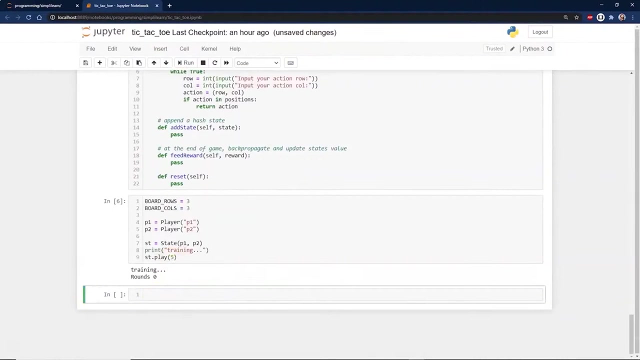 it references that we can just tack it on on the end. it was supposed to be at the beginning, so now I've only set this up with let's see where are we going here. I've only set this up to train 5 times, and the reason I did that 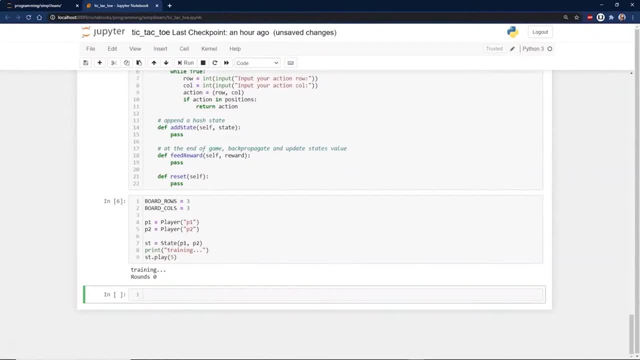 is we're going to come in and actually play it and then I'm going to change that and we can see how it differs on there. there we go. I didn't even make it through a run and we're going to go ahead and save the policy. 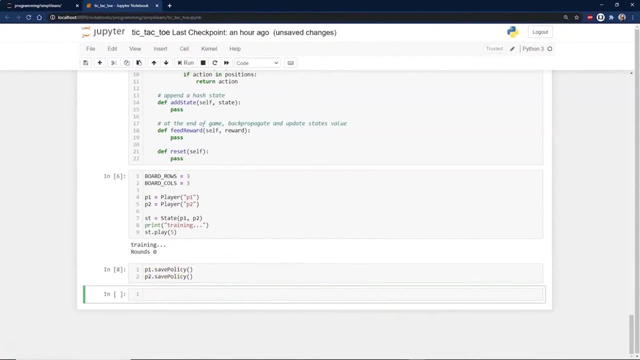 so now we have our player 1 and our player 2 policy. the way we set it up, it has two separate policies loaded up in there, and then we're going to come in here and we're going to do: player 1 is going to be the computer. 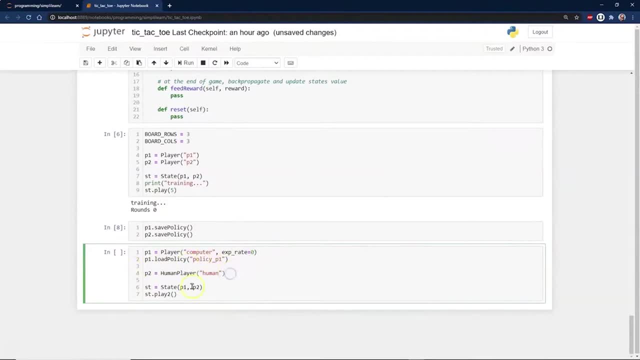 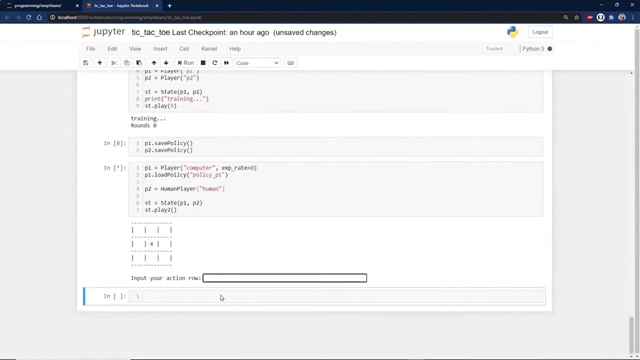 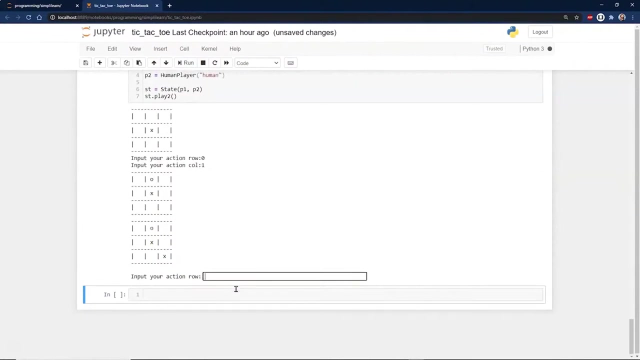 experience rate 0. load policy 1: human player: human, and we're going to go ahead and play this. just one round of training, in fact minimal training, and so it puts an x there and I'm going to go ahead and do. row 0, column 1. 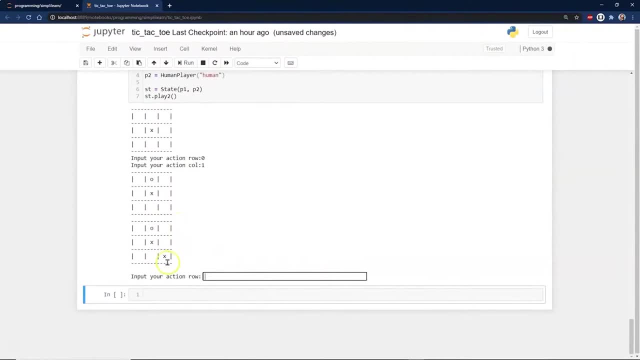 and you can see this is very basic on here, and so I put in my 0 and then I'm going to go 0, block it 0, 0 and you can see right here it. let me win. just like that I was able to win. 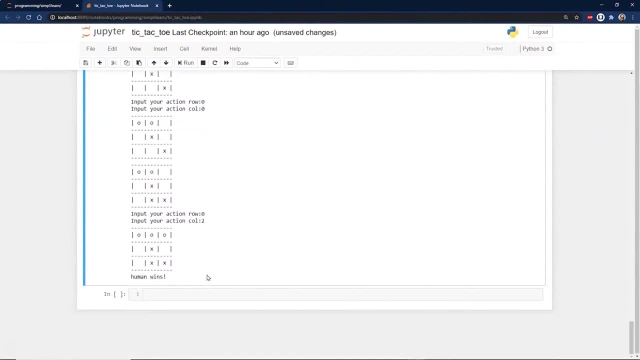 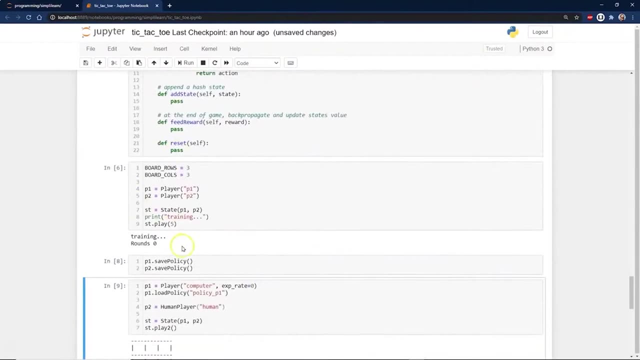 0, 2 and woo 7 wins. so I only trained it 5 times. we're going to run this again, and this time, instead of 5, let's do 5,000 or 50,000. I think that's what the guys in the back had. 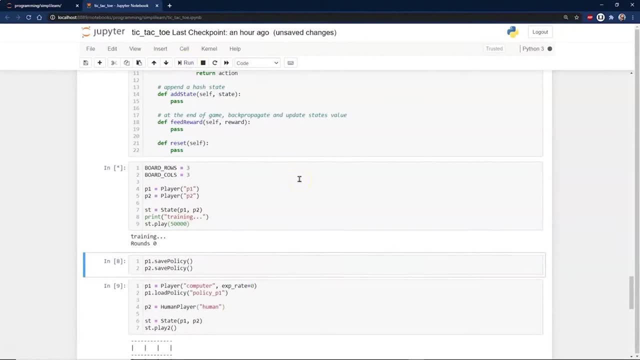 and this takes a while to train it. this is where reinforcement learning really falls apart. look how simple this game is. we're talking about a 3 by 3 set of columns, and so for me to train it on this, I could do a Q table, which would go much quicker. 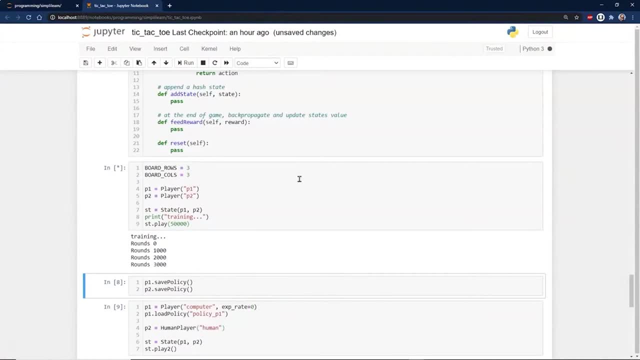 you could build a quick Q table with almost all the different options on there and you would probably get the same result much quicker. we're just using this as an example. so when we look at reinforcement learning, you need to be very careful what you apply it to. 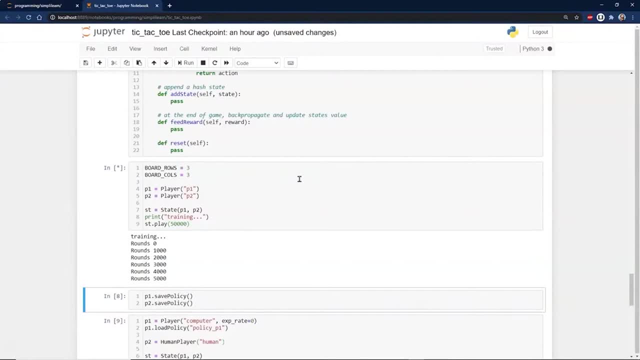 it sounds like a good deal until you do like a large neural network where you're doing a network to a learning increment of 1, so every time it goes through it learns and then you do your action. so you pick from the learning set up and you actually try. 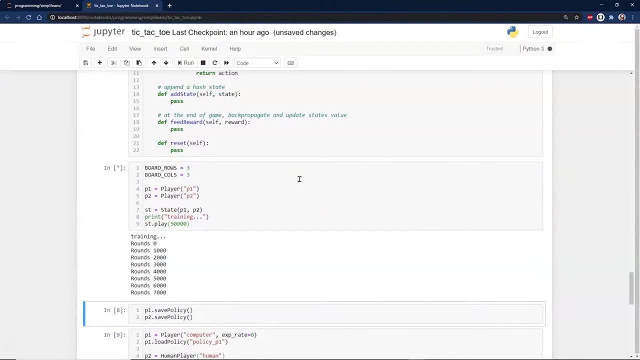 actions on the learning set up until you get what you think is going to be the best action. so you actually feed what you think is right back through the neural network. there's a whole layer there which is really fun to play with, and then it has an output. 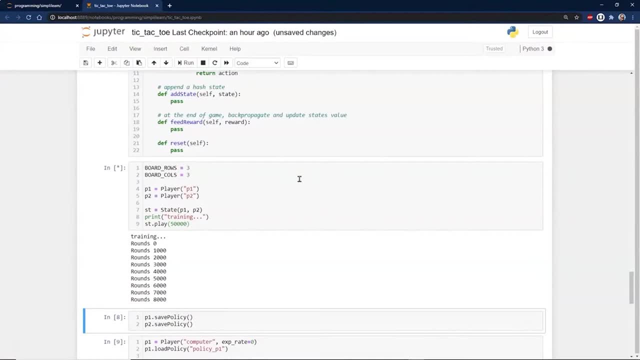 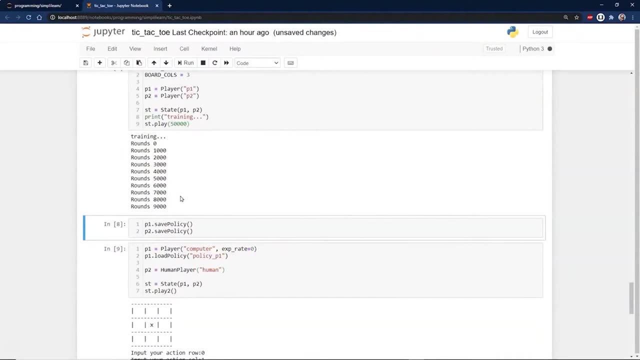 well, think of all those processes. I mean that is just a huge amount of work it's going to do. Let's go ahead and skip ahead here. give it a moment. it's going to take a minute or two to go ahead and run now to train it. 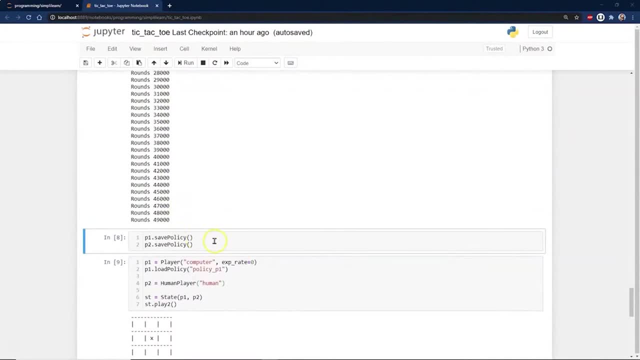 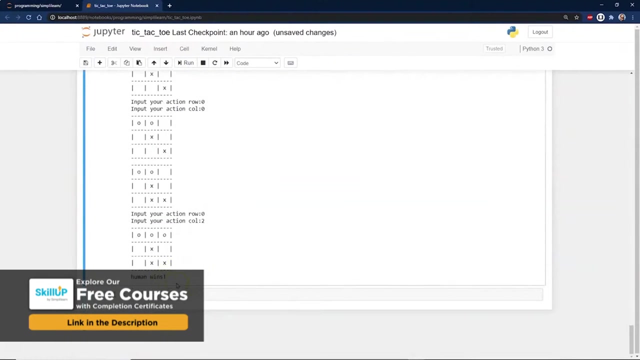 we went ahead and let it run and it took a while. this took. I got a pretty powerful processor and it took about 5 minutes plus to run it and we'll go ahead and run our player set up on here. whoops, it brought in the last. 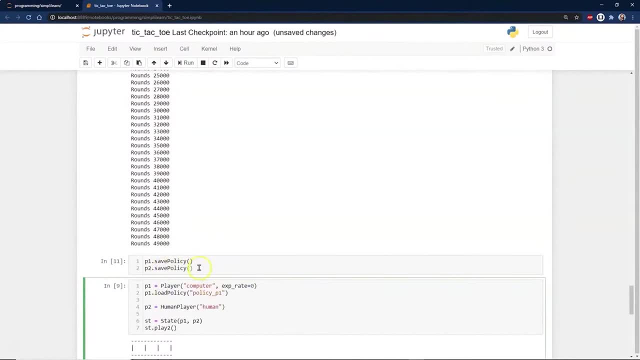 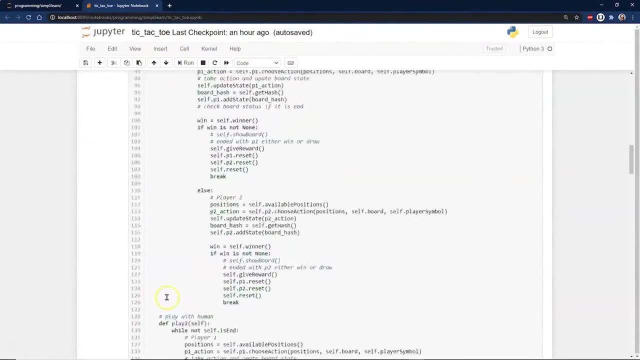 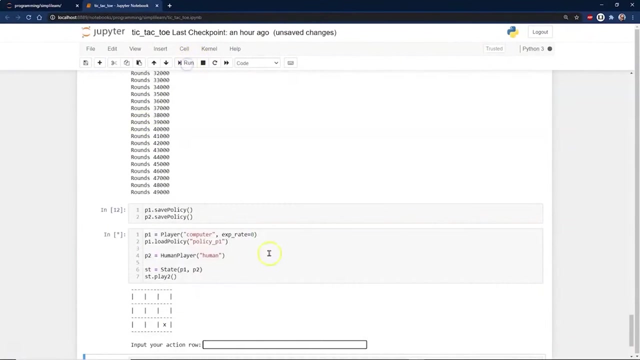 whoops it brought in the last round. so give me just a moment to redo the policy. save there we go. I forgot to save the policy back in there and then go ahead and run our player again. so we've saved the policy and then we want to go ahead and load the policy. 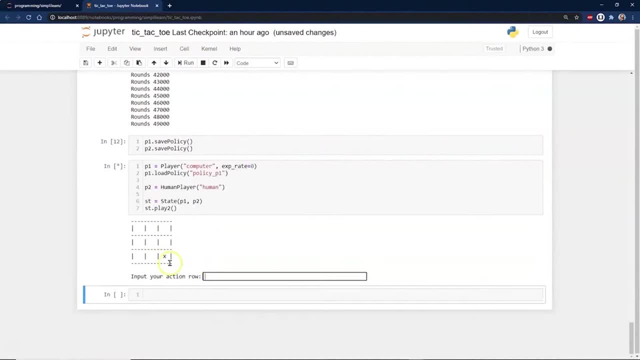 for P1 as the computer, and we can see the computer has gone in the bottom right corner. I'm going to go ahead and go 1: 1, which is the center, and it's gone right up the top. and if you have ever played tic-tac-toe- 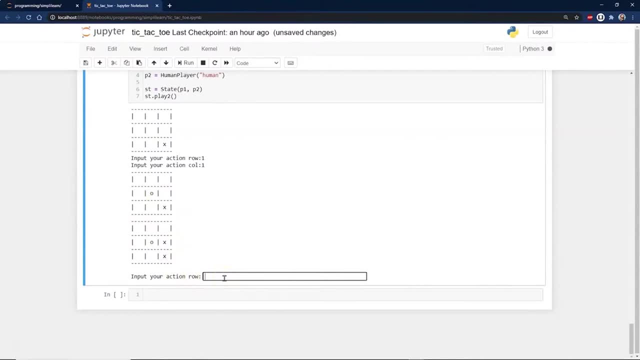 you know the computer has me, but we'll go ahead and play it out. row 0, column 2: there it is, and then it's gone here, and so I'm going to go ahead and go. row 0, 1, 2, no 0, 1. 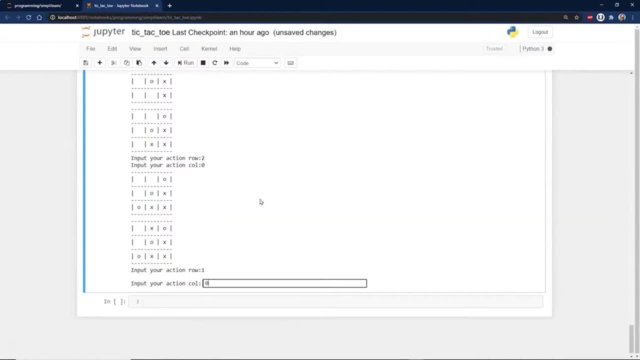 there we go and column 0, that's where I want it. and it says: okay, your action, there we go, boom. so you can see, here we didn't catch the win on this. it said tie. kind of funny, they didn't catch the win on there. but if we play this a bunch of times, 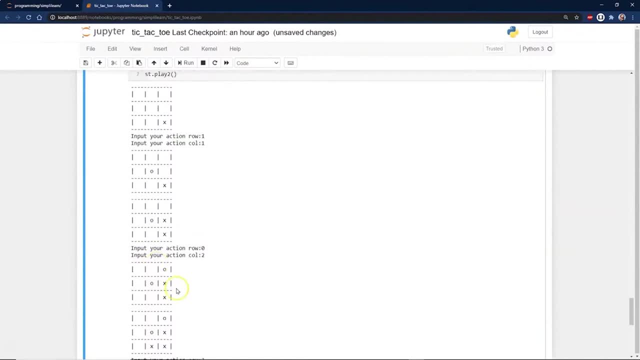 you'll find that it's going to win more and more. the more we train it, the more the reinforcement happens. this lengthy training process is really the stopper on reinforcement learning. as this changes, reinforcement learning will be one of the more powerful packages evolving over the next decade or two. 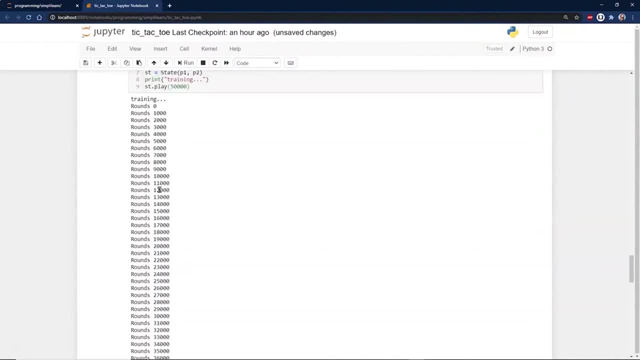 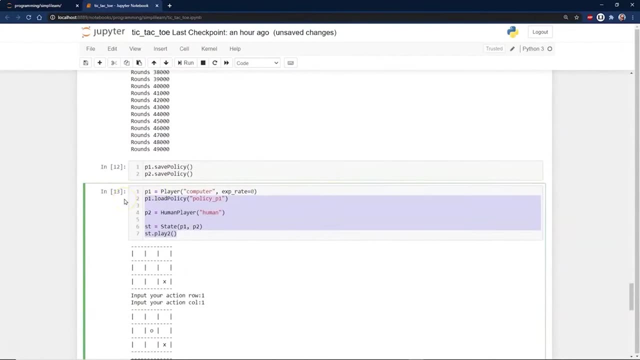 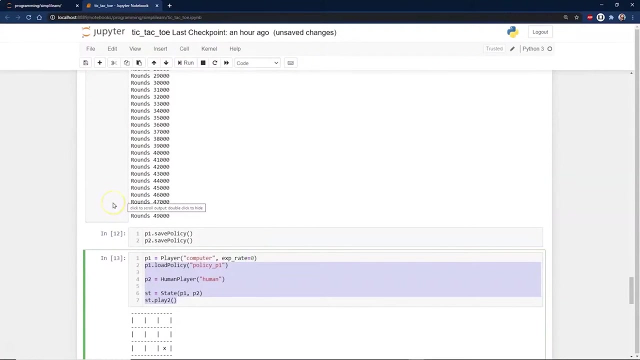 in fact, I would even go as far as to say it is the most important machine learning tool and artificial intelligence tool out there, as it learns. not only a simple tic tac toe board, but we start learning environments, and the environment would be like a language if you're translating a language or something from one language to the other. 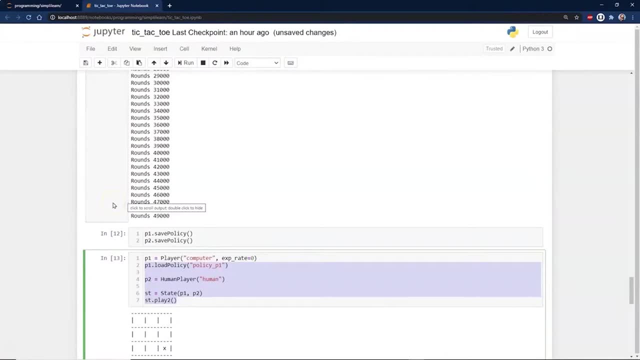 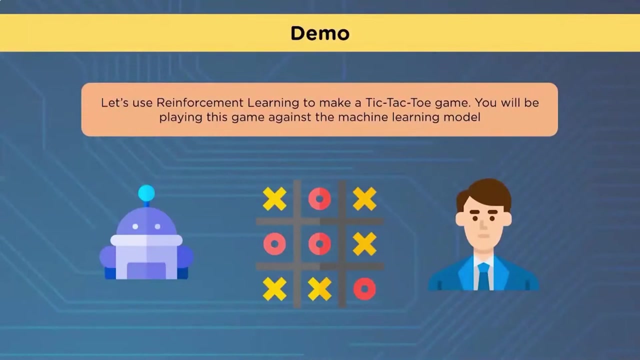 so much of it is lost if you don't know the context it's in, what's the environments it's in, and so being able to attach environment and context and all those things together is going to require reinforcement, learning to do so. again, if you want to get a copy of the tic tac toe board, 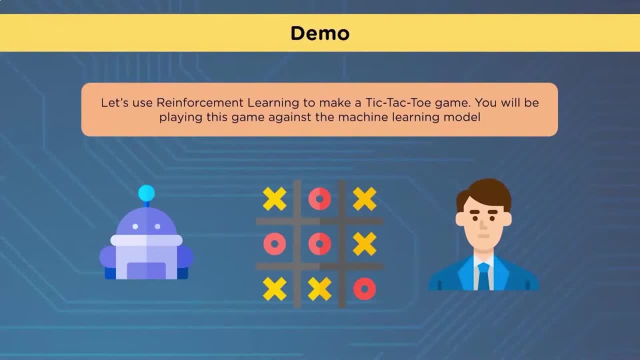 it's kind of fun to play with. you can run it, you can test it out, you can test it for different values. you can switch from p1 computer where we loaded the policy 1 to load the policy 2 and just see how it varies. there's all kinds of things you can do on there. 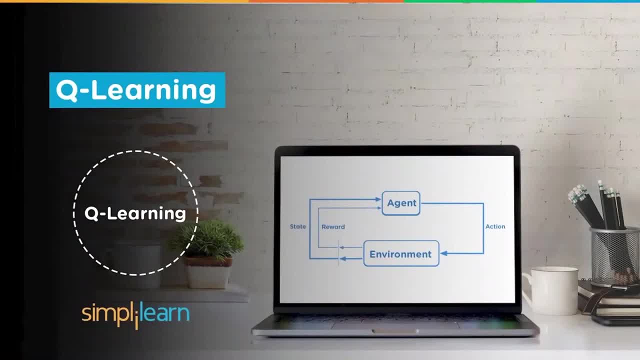 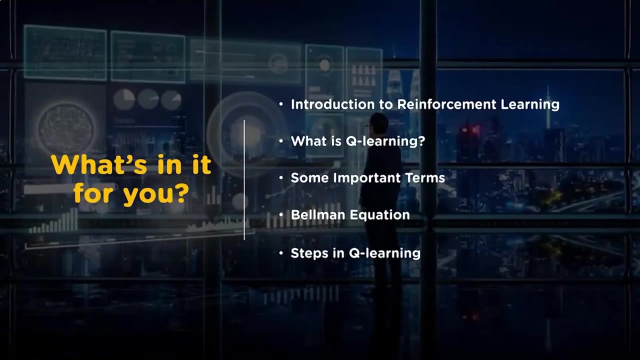 welcome to QLearning. my name is Richard Kirschner, with the SimplyLearn team, wwwsimplylearncom. get certified, get ahead. what's in it for you today? an introduction to reinforcement learning. what is QLearning? some important terms: Bellman equation, steps in QLearning. 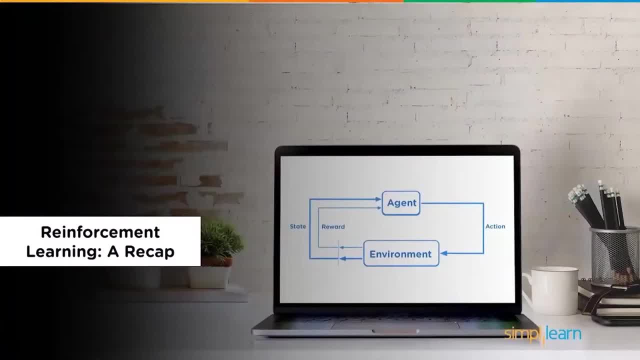 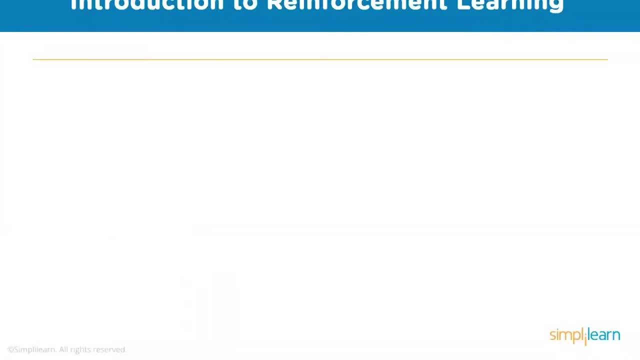 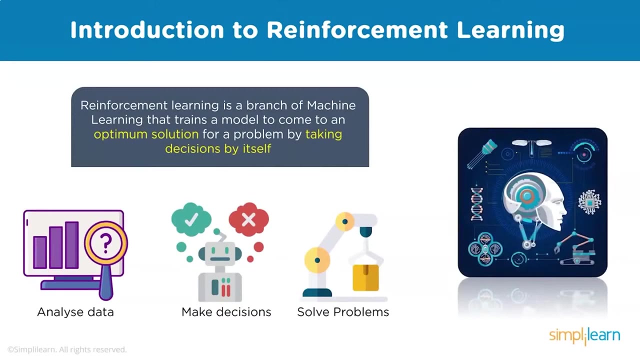 a quick recap. so we're going to go back and do a reinforcement learning recap and you'll remember we have our agent, our action, our environment and our reward and the state, and so reinforcement learning is a branch of machine learning that trains a model to come to an optimum. 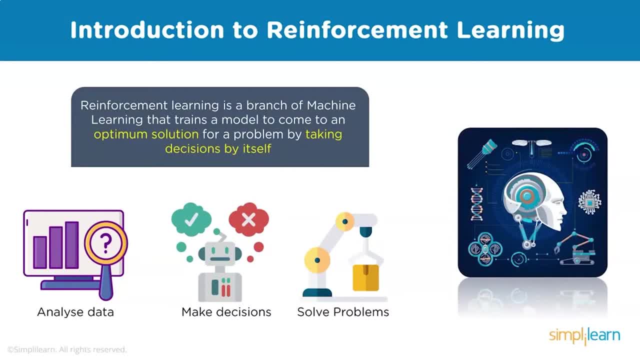 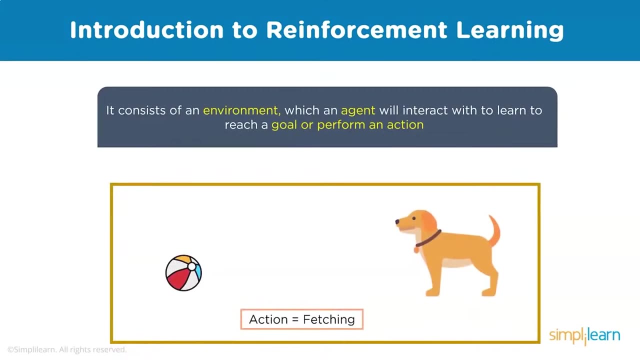 solution for a problem by taking decisions by itself. so we look at it, we analyze the data, make decisions, solve problems. it consists of an environment which an agent will interact with to learn, to reach a goal or perform an action. and you see, here we have the dog. 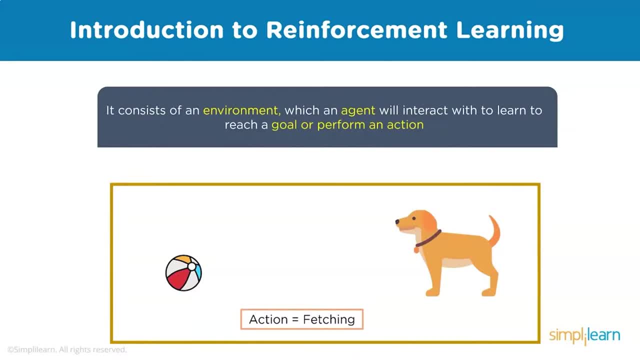 and the action equals fetching. and the first thing you're going to notice here- and I'll talk a little bit more about this- is that our action is kind of a singularity. the action isn't a regression type model where we're looking at float numbers or we're trying to predict something. 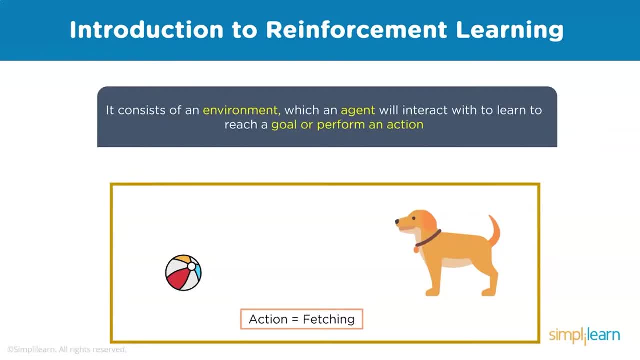 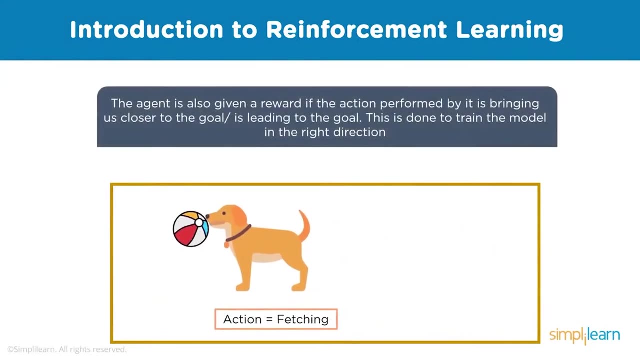 or doing a reinforcement learning, where we're trying to guess the value of the stock market, where you have 5.33, $5.33. this is very, a little bit different and you'll see why QLearning is so powerful. but also where falls short. the agent is also given a reward if the 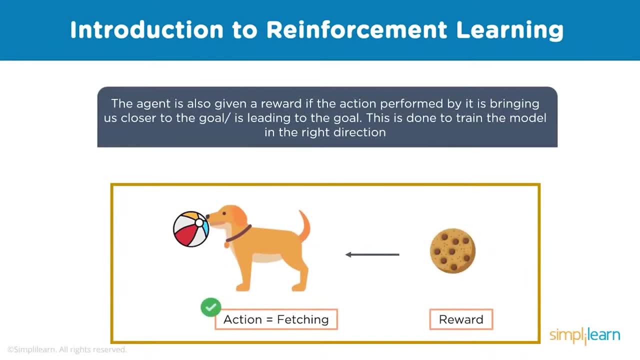 action performed by it is bringing, is closer to the goal, is leading to the goal. this is done to train the model in the right direction. you have a reward of a- hopefully a doggy cookie, and action equals fetching, so it gets a reward. it gets to go fetch. 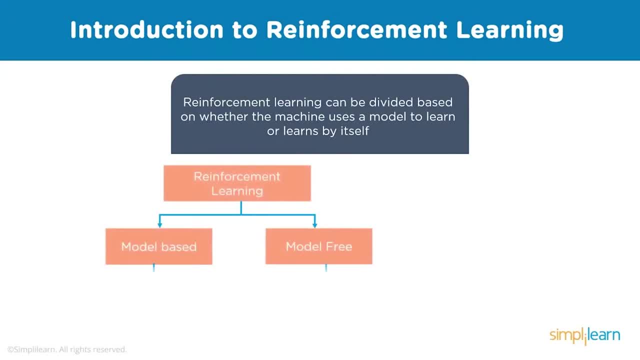 the ball. reinforcement learning can be divided based on whether the machine uses a model to learn or learns by itself. so reinforcement learning it's model based. learn the model given model, and you can think of neural networks, I think are the most common right now used for reinforcement learning there. 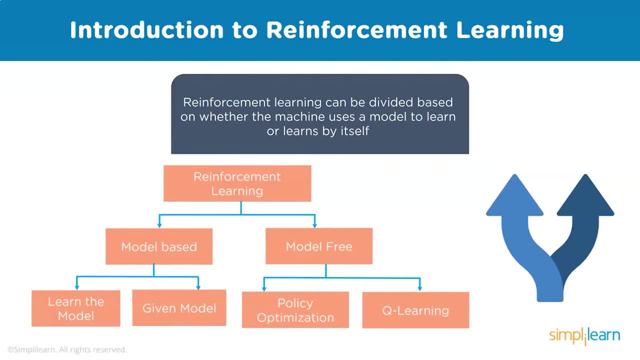 certainly are a lot of other options out there. but you have this black box and you go back and you send the error back up and it trains it based on how much of an error. the error could be computed based on, maybe a maximum reward subtraction or something like that. 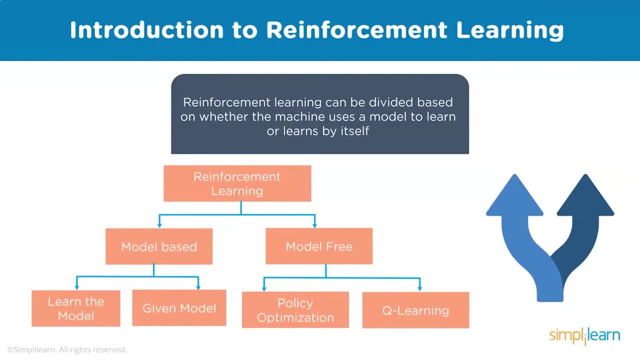 so the closer you get to the maximum reward, the better, and so we talk about a model free. you have your policy optimization and your QLearning, and this is kind of the cool thing about QLearning is it can do, it's very powerful on certain things, making it very 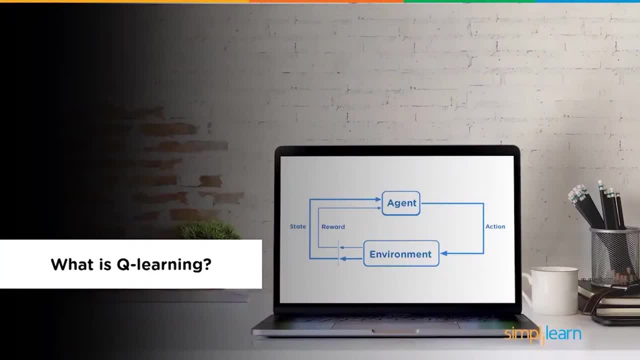 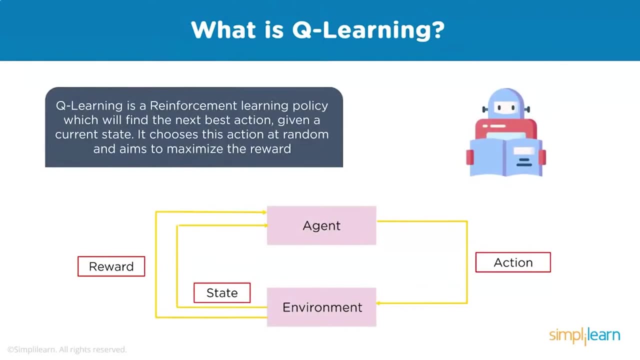 quick and easy to do, a reinforcement learning. so what is QLearning? QLearning is reinforcement learning policy which will fill the next best action given a current state. it chooses this action at random and aims to maximize the reward. and so you can see, here's our standard reinforcement. 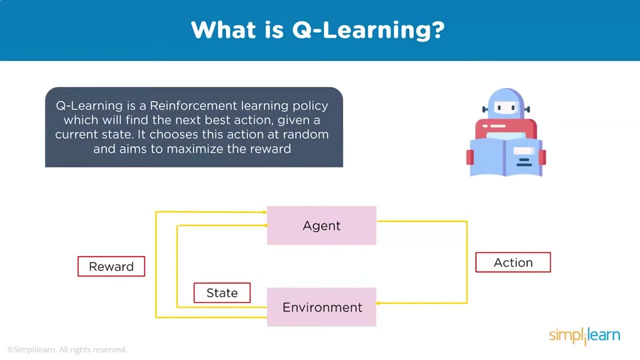 learning graph by now. if you're doing any reinforcement learning, you should be familiar with this. where you have your agent, your agent takes an action, the action affects the environment and then the environment sends back the reward or the feedback and the state, the new state, the agent's in. where is it at? 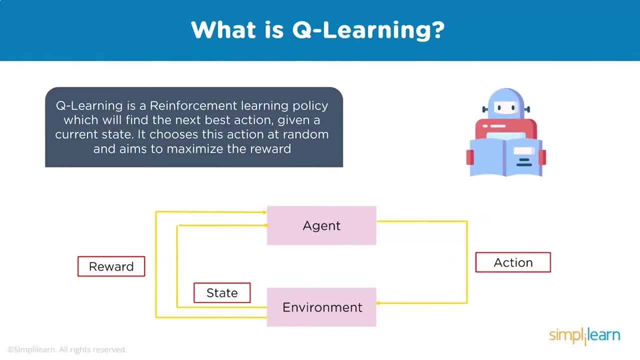 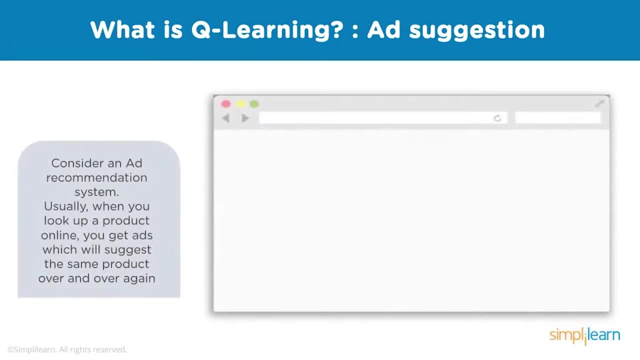 on the chessboard? where is it at in the video game? if your robot's out there picking trash up off the side of the road, where is it at on the road? consider an ad recommendation system. usually when you look up a product online, you get ads which will suggest. 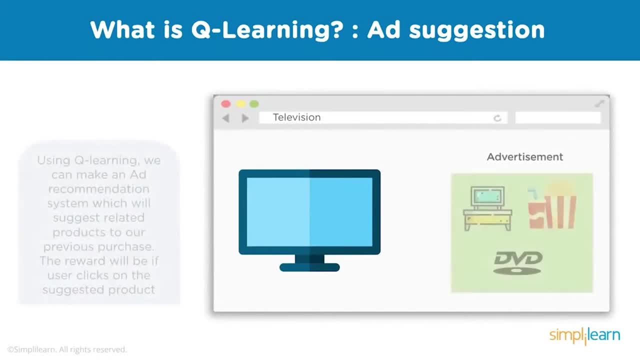 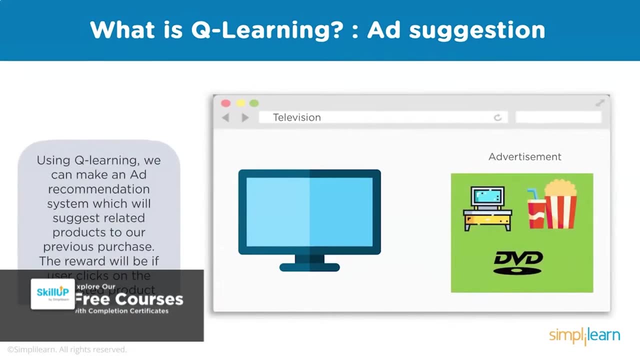 the same product over and over again. using QLearning we can make an ad recommendation system which will suggest related products to our previous purchase. the reward will be if user clicks on the suggested product and again you can see you might have a lot of products on your. 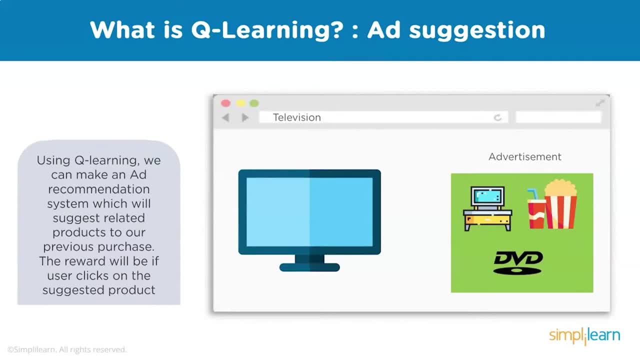 web advertisement or your pages. but it's still not a float number, it's still a set number and that's something to be aware of when you're using QLearning. and you can see here that if you have a hundred people clicking on ads and you click on one of the ads, 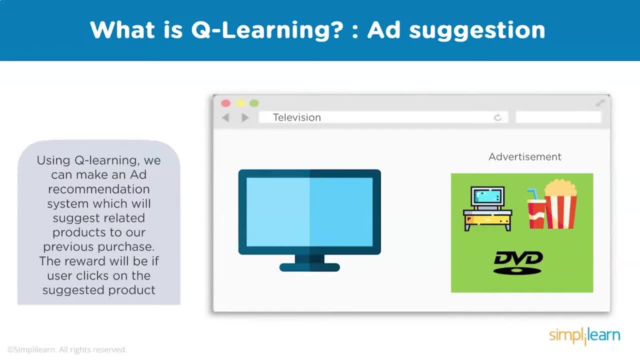 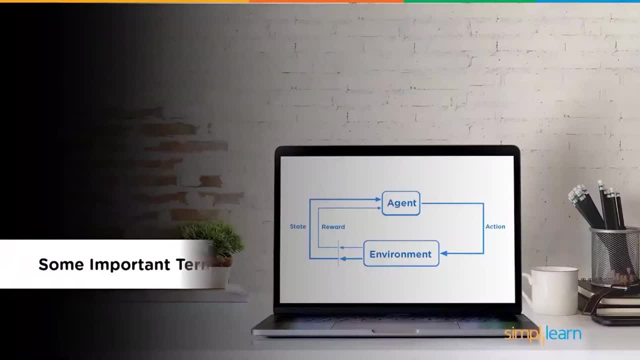 it might go in there and say, okay, this person clicked on this ad. what is the best set of ads, based on clicking on this ad or these two ads afterwards, based on where they are browsing? so let's go ahead and take a look at some important terms when we talk about QLearning. 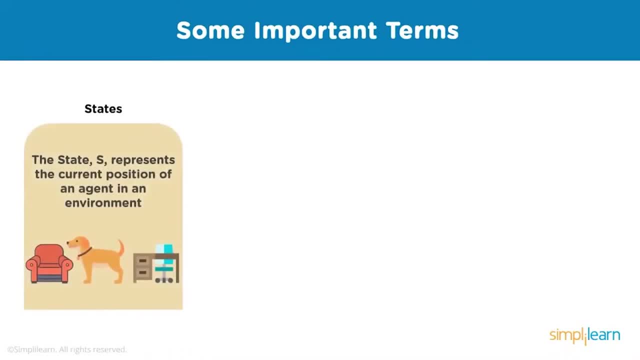 we have states. the state S represents the current position of an agent in an environment. the action- the action A is the step taken by the agent when it is in a particular state- rewards: for every action the agent will get a positive or negative reward. and again, when we talk about 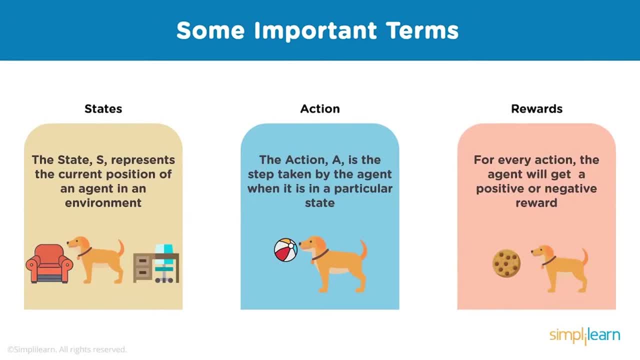 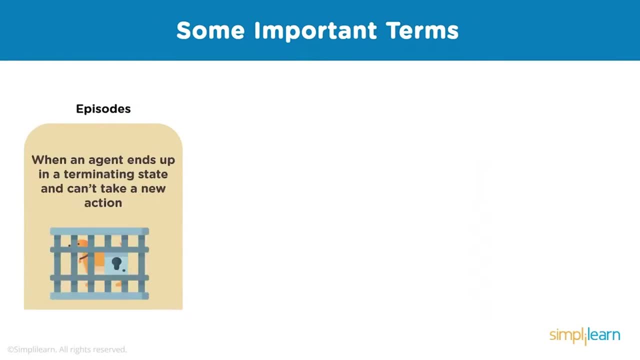 states. we're usually not. when you're using a Q table, you're not usually talking about float variables, you're talking about true, false- we'll take a closer look at that in a second- and episodes when an agent ends up in a terminating state and can't take a new action. 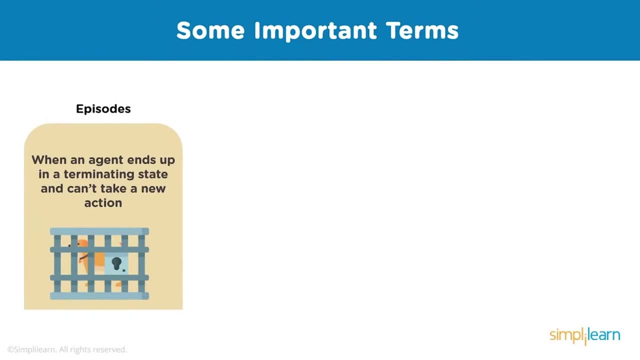 this might be if you're playing a video game character stepped in and is now dead, or whatever. Q values used to determine how good an action A taken at a particular state. S is QA of S and temporal difference, a formula used to find the Q value by using the value of the current. 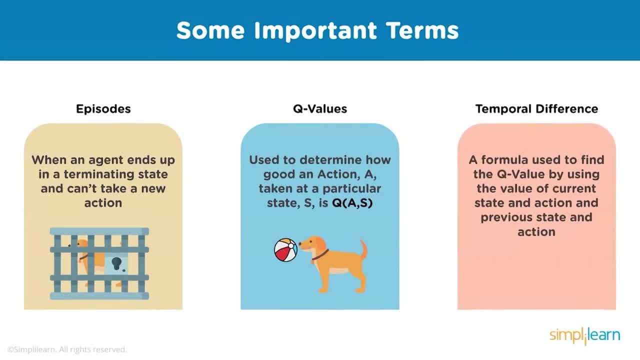 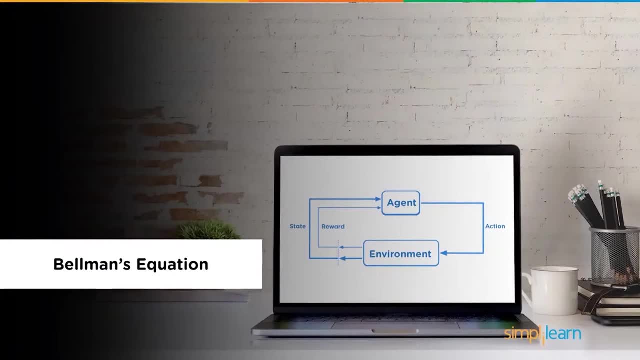 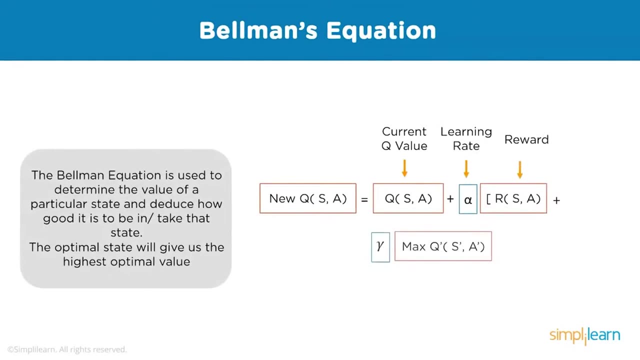 state and action and previous state and action and there's Bellman's equation, which basically is the equation that kind of covers what we just looked at in all those different terms. the Bellman equation is used to determine the values of a particular state and deduce how good it is. 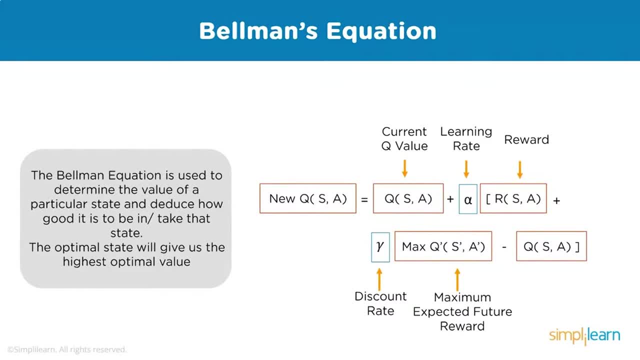 to be in. take that state. the optimal state will give us the highest optimal value factor influencing Q values. the current state and action, that's your SA, so your current state and your action. then you have your previous state and action, which is your S, I guess prime. 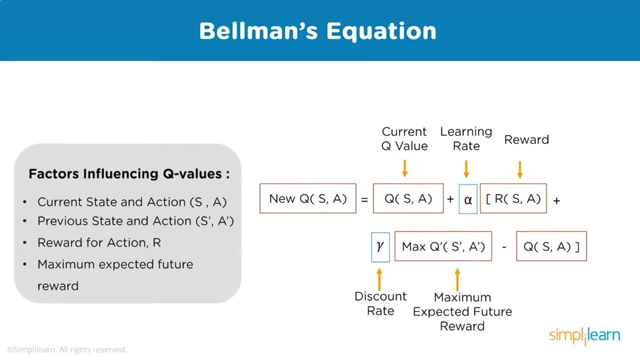 I'm not sure how they reference that S prime A prime. so this is what happened before. then you have a reward for action, so you have your R reward and you have your maximum expected future reward and you can see there's also a learning rate put in there. 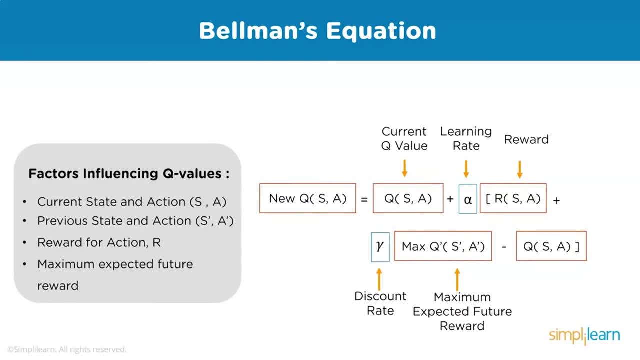 and a discount rate. so when we're looking at these, just like any other model, we don't want to have an absolute final value on here. if you do absolute values instead of taking smaller steps, you don't really have that approach to the solution, you just have a jump. 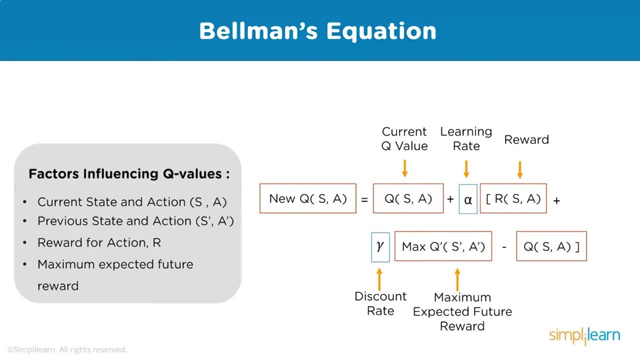 and then pretty soon, if you jump one solution out, that's what's going to be the new solution, whichever one jumps up really high first, kind of ruining the whole idea of doing a random selection, and I'll go into the random selection in just a second steps in Q learning. 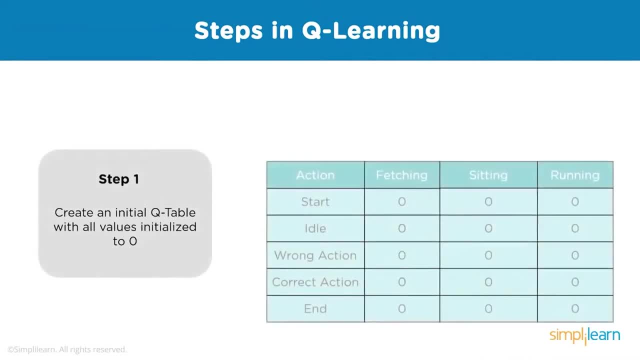 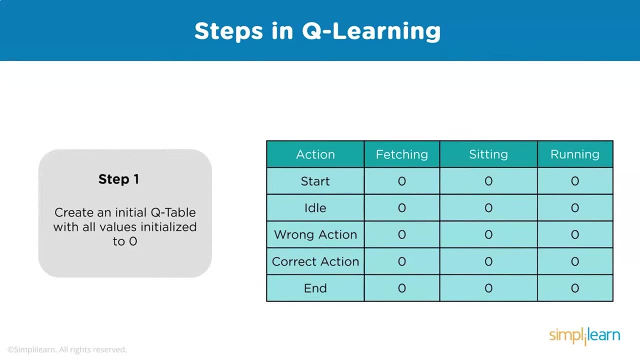 step one: create an initial Q table with all values initialized to zero. again, we're looking at zero one. so you know, here's our action. we start, we're in idle, we took a wrong action, we took a correct action and end, and then we have our actions. 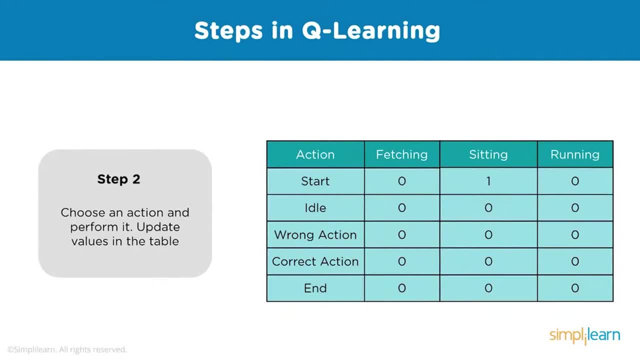 fetching, sitting and running. of course we're just using the dog example and choose an action and perform it, update values in the table and of course, when we're choosing an action, we're going to kind of do something random and just randomly pick one. so you start out and you sit. 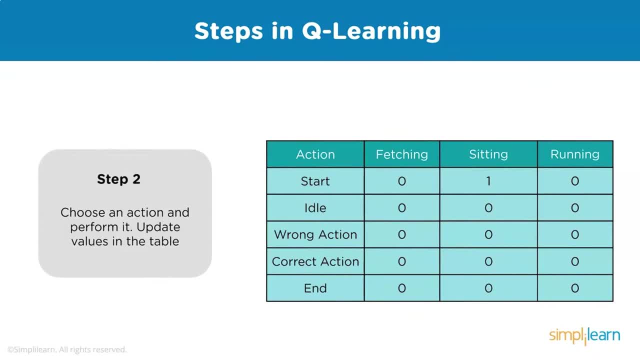 and you have. then. then, depending on that action you took, you can now update the value for sitting after you start from start to sitting, get the value of the reward and calculate the value- Q value- using the Bellman equation. and so now we attach a reward to sitting. 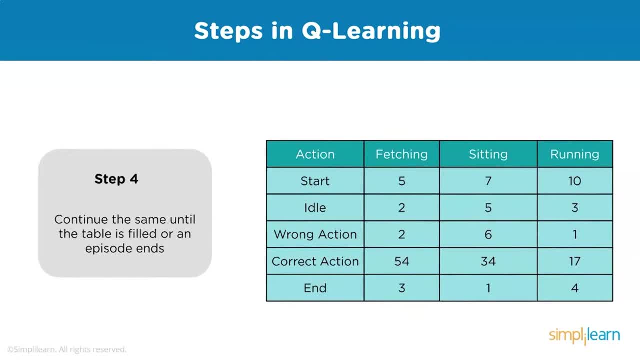 and when we attach all those rewards, we continue the same until the table is filled with or an episode ends- and I mentioned I was going to come back to the random side of this- and there's a few different formulas they use for the random set up to pick it. I usually look. 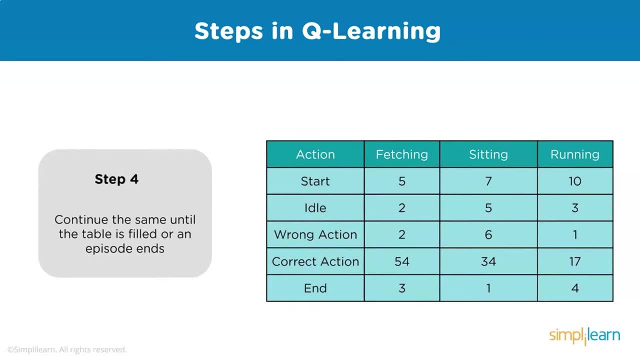 whatever Q model I'm using, do their standard one, because someone's usually gone in and done the math for the optimal spread. but you can look at this: if I have, running has a reward of 10, sitting has a reward of 7, fetching has a reward of 5. 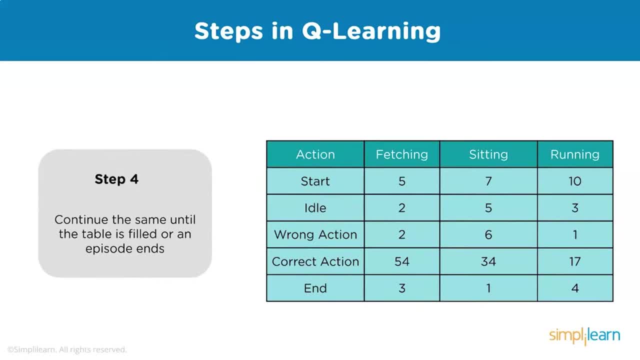 just kind of without doing like a means, using the bell curve for the means value and, like I said, there's some math you can put in there to pick so that you're more likely, so that running has even a higher chance. but even if you were just going to do an average on this, 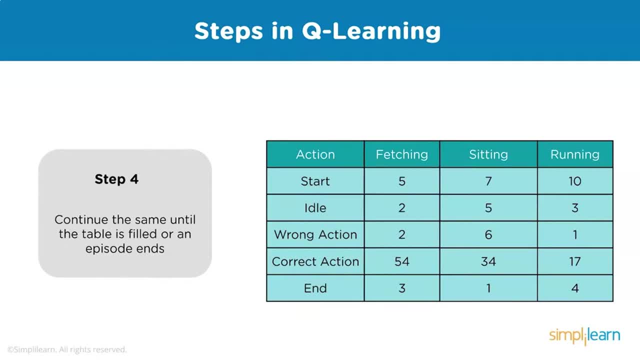 you could do an average, a random number, by adding them all together. so you get 10 plus 7 plus 5 is 22. you could do 0 to 22 or 0 to 21, but 1 to 22, 1 to 5 would be fetching. 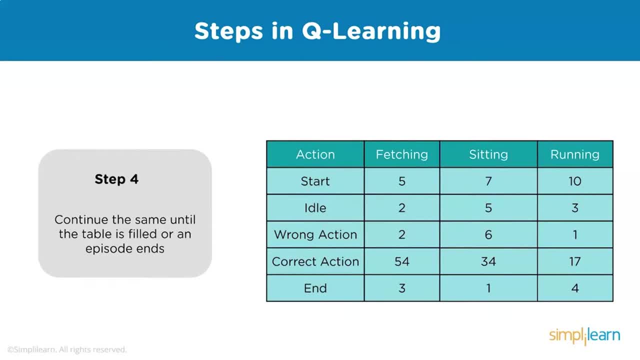 and so forth. you know the last 10, so you could just look at this as what percentage are you going to go for that particular option? and then that gets random set up in there and then, as you slowly increment these up, you see that if you're idle, 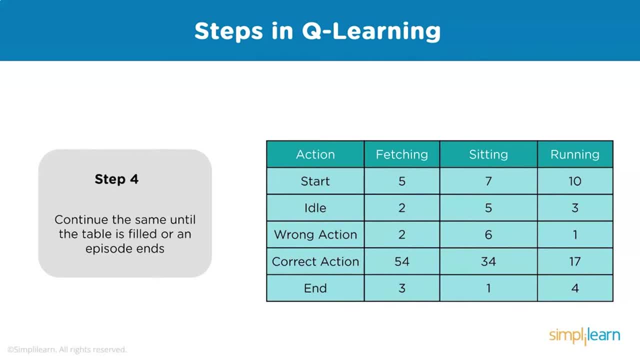 where's one? here? we go sitting at the end. if you're at the end of wherever you're at sitting gets a reward of 1. where's a good one on here? oh, wrong action, running for a wrong action gets almost no reward, so that becomes very, very less. 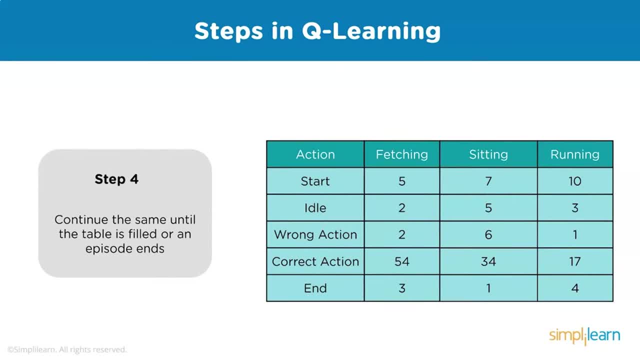 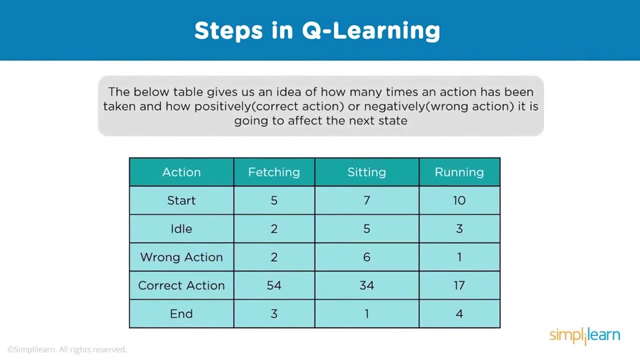 likely to happen, but it still might happen. it still might have a percentage of coming up, and that's where the random programming in Q-learning comes in. the below table gives us an idea of how many times an action has been taken and how positively correct action or negatively wrong action. 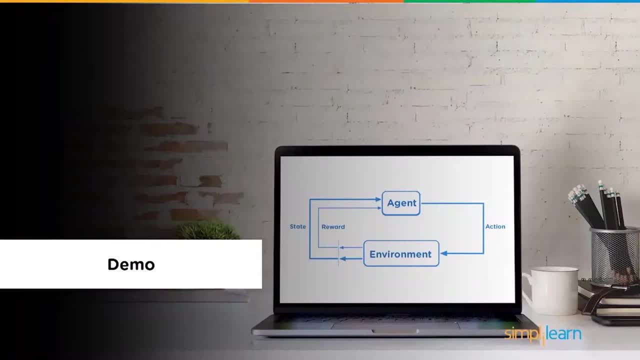 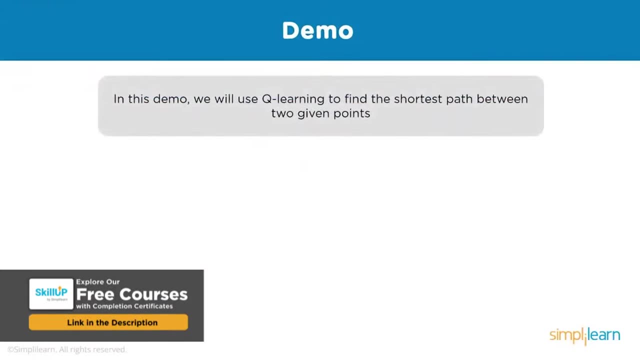 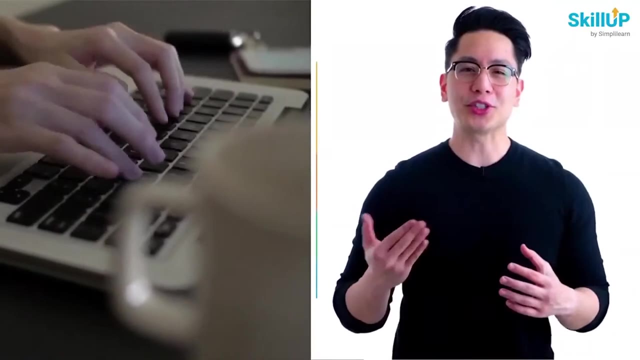 it is going to affect the next state. so let's go ahead and dive in and pull up a little piece of code and see what this looks like in Python. in this demo, we'll use Q-learning to find the shortest path between two given points and scale up by simply learn. 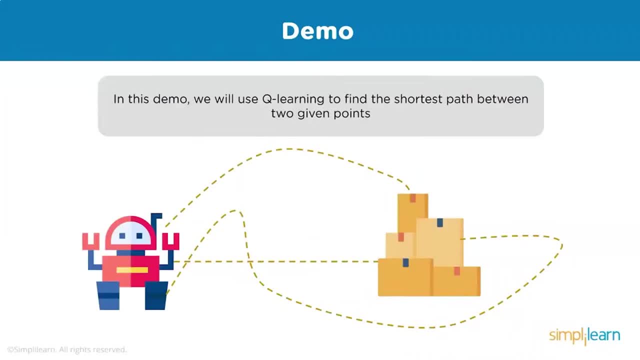 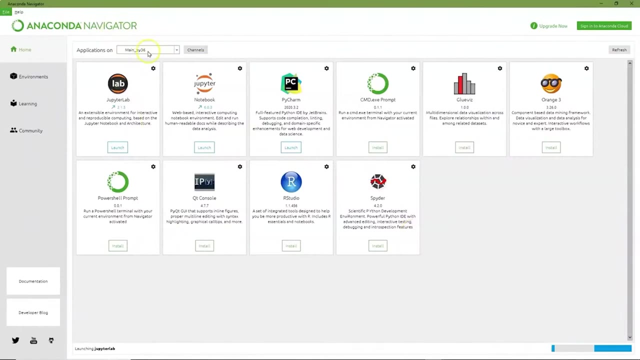 click on the link in the description to know more. if you've seen my videos before, I like to do it in the Anaconda Jupyter Notebook setup, just because it's really easy to see and it's a nice demo. so here's my Anaconda. this one, I'm actually using Python 3.6. 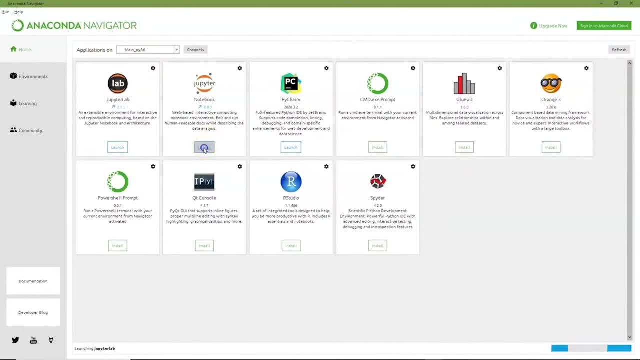 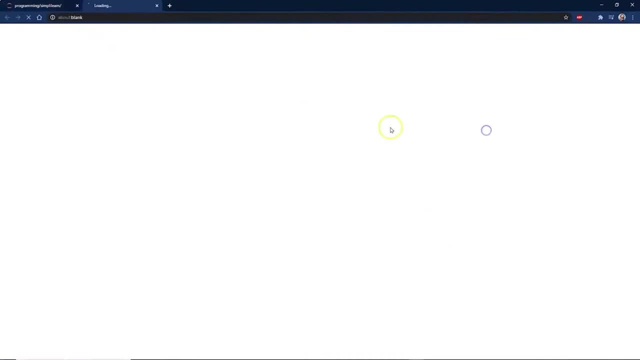 environment that I set up in here and we'll go ahead and launch the Jupyter Notebook on this. and once we're in our Jupyter Notebook there's a kernel loaded with Python 3. we'll go ahead and create a new Python 3 folder in here. 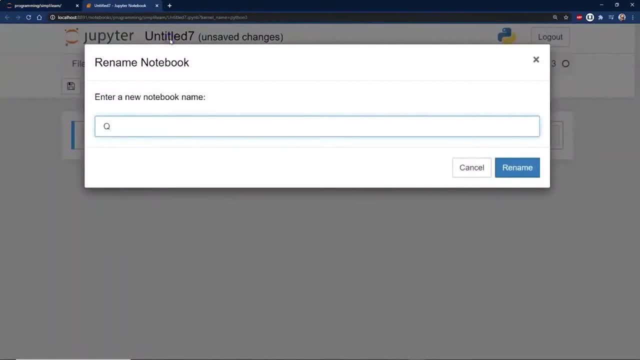 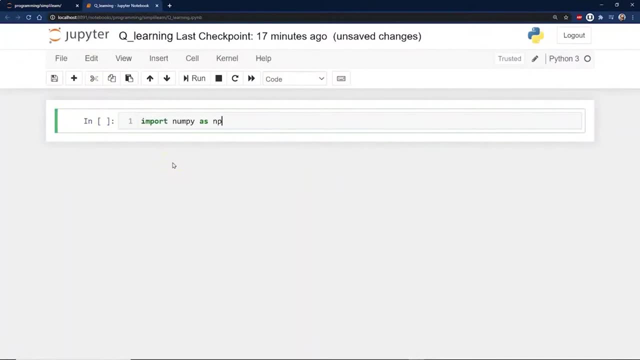 and we'll call this Q-learning. and to start this demo, let's go ahead and import our numpy array. we'll just run that, so it's imported. and, like a lot of these model programs, when you're building them, you spend a lot of time putting it all together. 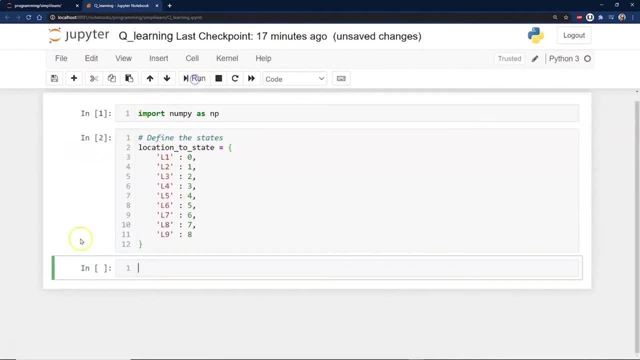 and then you end up with this really short answer at the end, and we'll take a look at that as we come into it. so we go ahead and start with our location to state. so we have L1, L2. these are our nine locations, one to nine. 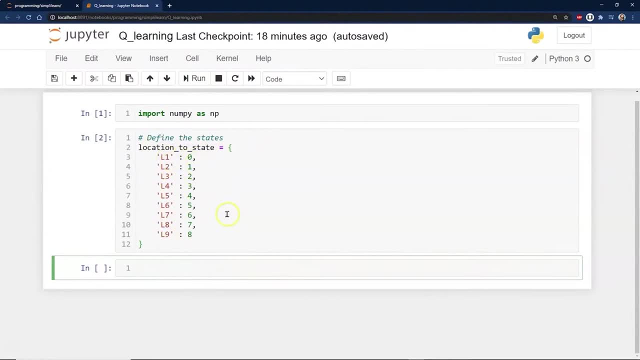 and then, of course, the state is going to be 0,, 1,, 2,, 3,, 4. it's just a mapping of our location to an integer on there, and then we have our actions. our actions are simply moving from one location. 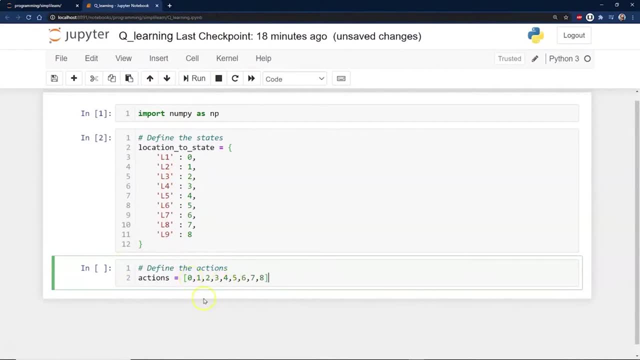 to another. so I can go to location 0. I can go to location 1,, 2,, 3, 4, 5,, 6,, 7, 8. so these are my actions. I can choose. these are the locations of our state. 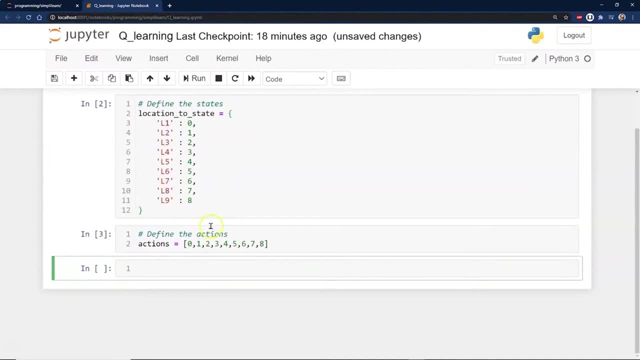 and if you remember earlier I mentioned that the limitation is that you don't want to put in a continually growing table, because you can actually create a dynamic Q table where you continually add in new values as they arise, because when you have float values it just becomes infinite. 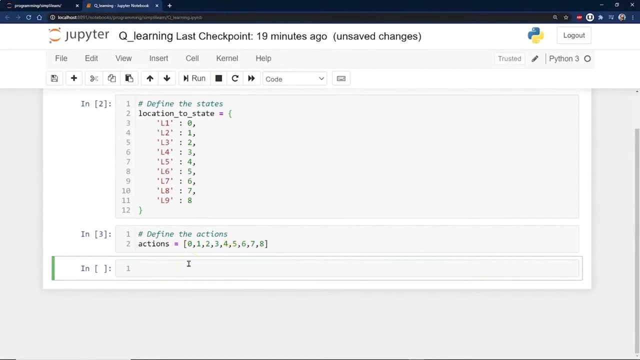 and then your memory in your computer is gone or it's not going to work. at the same time you might think: well, that kind of really limits the Q learning setup, but there are ways to use it in conjunction with other systems, and so you might look at. 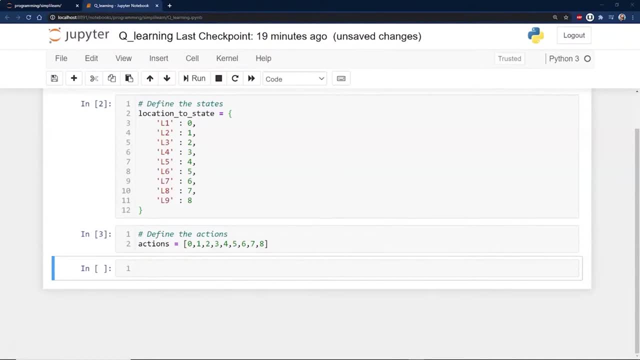 well, I do. I've been doing some work in stock and one of the questions that comes out is: to buy or sell the stock and the stake coming in might be. you might take it and create what we call buckets, where anything that you predict is going to return. 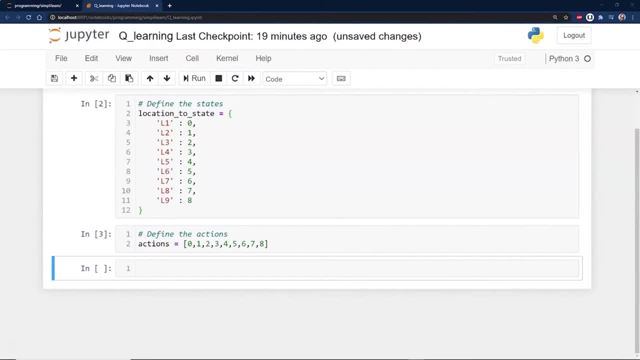 more than a certain amount of money, the error for that stock that you've had in the past. you put those in buckets. and suddenly you start creating these buckets, you realize you do have a limited amount of information coming in. you no longer have a float number. you now have bucket 1, 2. 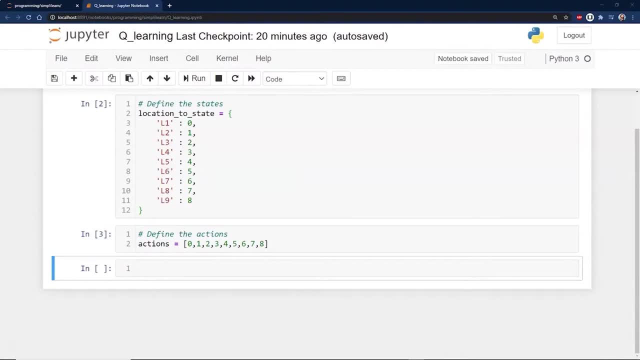 3 and 4, and then you can take those buckets, put them through a Q learning table and come up with the best action. which stock should I buy? it's like gambling. stock is pretty much gambling. if you're doing day trading, you're not doing long term investments. 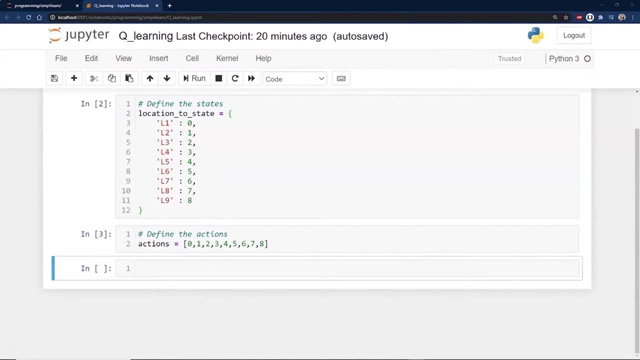 and so you can start looking at it like that. a lot of the current feeds say that the best algorithms used for day traders, when you're doing it on your own, is really to ask the question: do you know? and now you have it in a Q learning table. 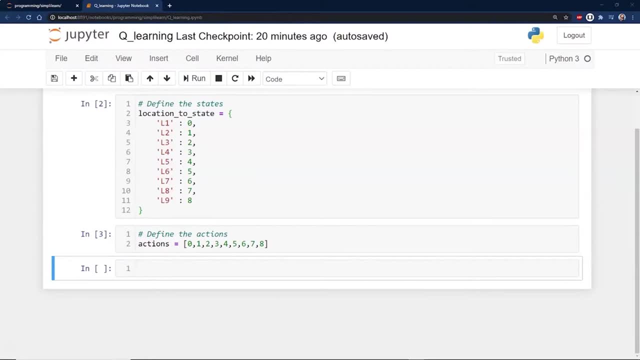 and now you can take it to that next level and you can see where that can be a really powerful tool. at the end of doing a basic linear regression model or something, what is the best investment? and you start getting the best reward on there, and so if we're going to have rewards, 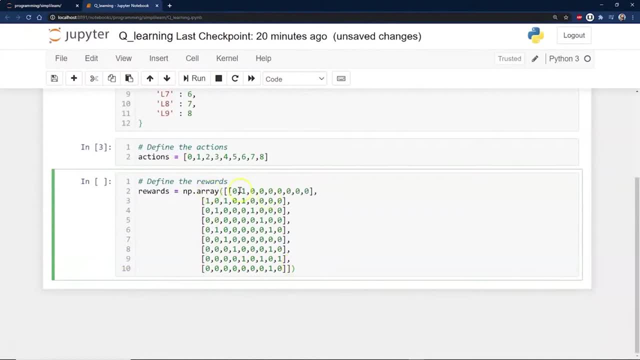 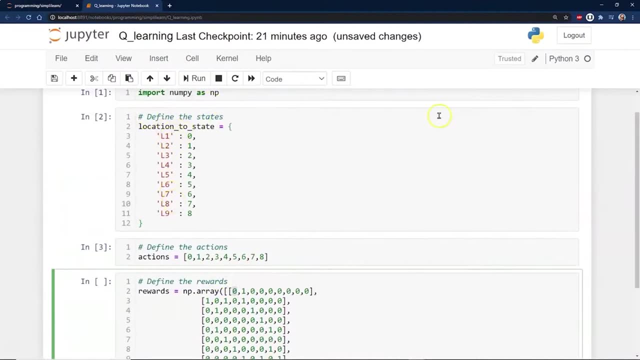 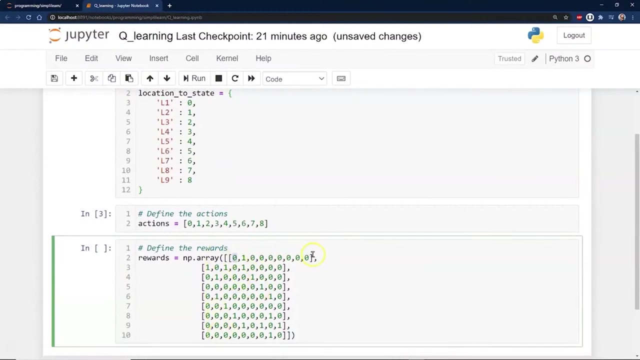 these rewards we just create. it says basically, if you're, this should match our Q table because it's going to be, you have your state and you have your action, if you remember from the dog. and so we have whatever state we're in, going down and then the next action. 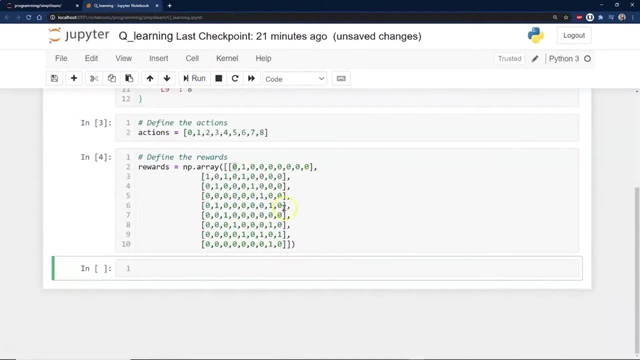 and what the reward is for it. and, of course, if you were actually doing something more connected, your reward would be based on the actual environment it's in. and then we want to go ahead and create a state to location so we can map the indexes. so, just like we defined our rewards, 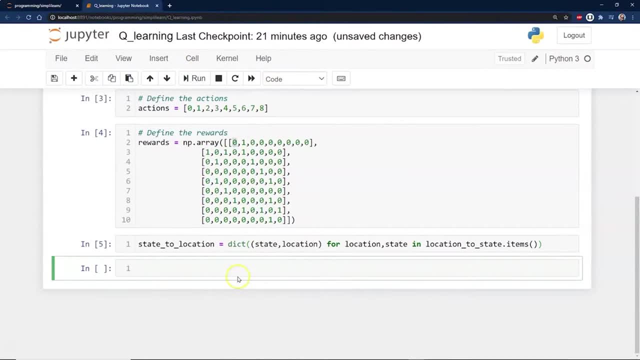 we're going to go ahead and do state to location and you can see here it's a dictionary set up for location, state and location to state with items, and we also need to define what we want for learning rates. you remember we had our two different rates. 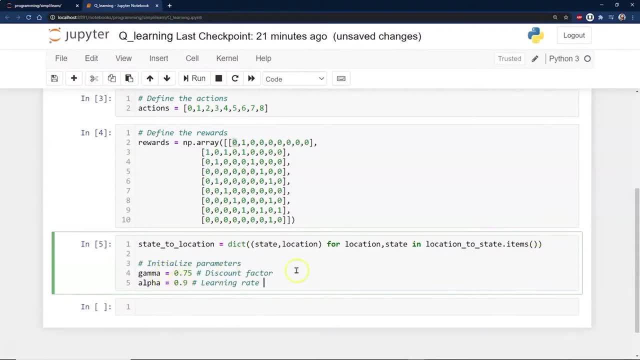 as far as like learning from the past and learning from the current. so we'll go ahead and set those to .75 and the alpha set to .9 and we'll see that when we do the formula and, of course, any of this code. send a note to our Simply Learn team. 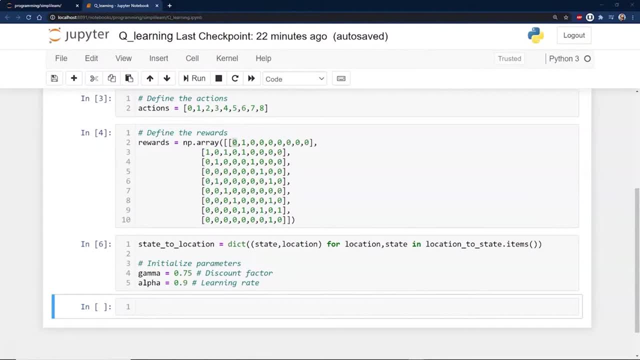 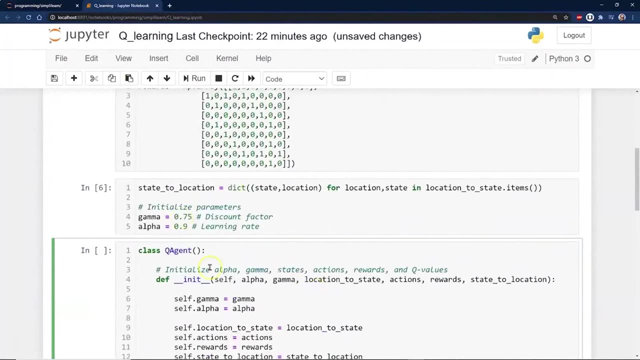 they'll get you a copy of this code on here. let's go ahead and pull. there we go the next two sections. since we're going to keep it short and sweet, here we go. so let's go ahead and create our agent. so our agent is going to have our initialization. 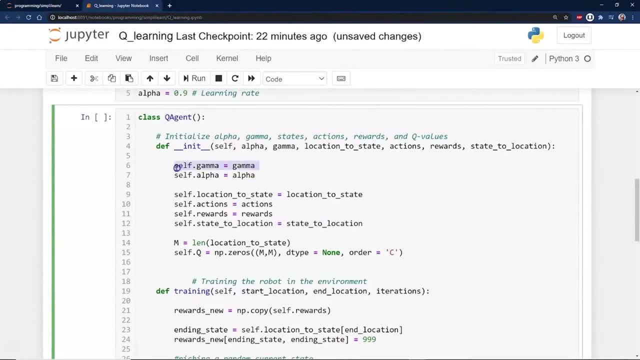 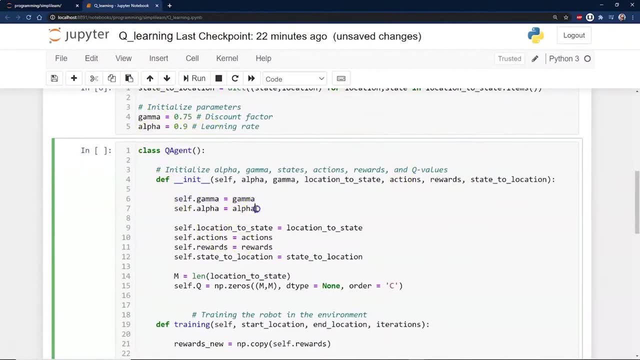 where we send it all the information we define our self. gamma equals gamma. we could have just set the gamma rate down here instead of submitting it. it's kind of nice to keep them separate, because you can play with these numbers: our self alpha. then we have our location state. 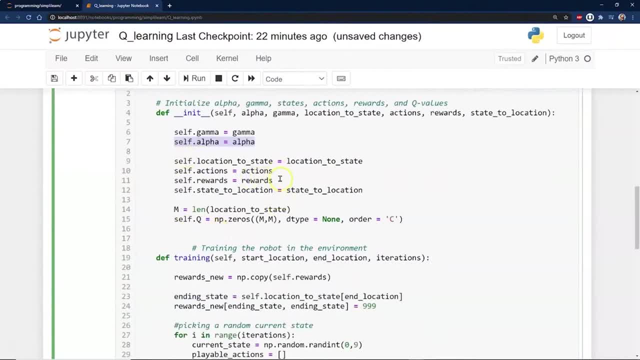 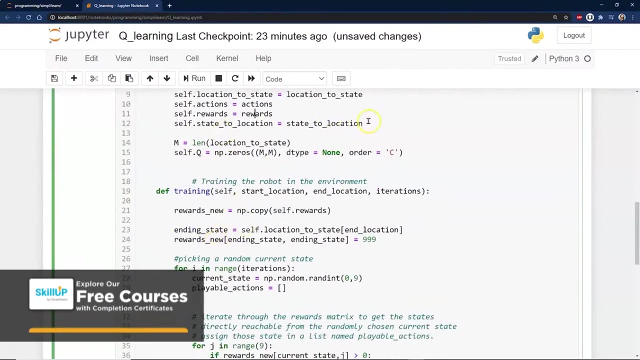 we'll set that in here. we have our choice of actions. we're going to go ahead and just embed the rewards right into the agent, so obviously this would be coming from somewhere else instead of from self generated, and then a self state to location equals our state to location. 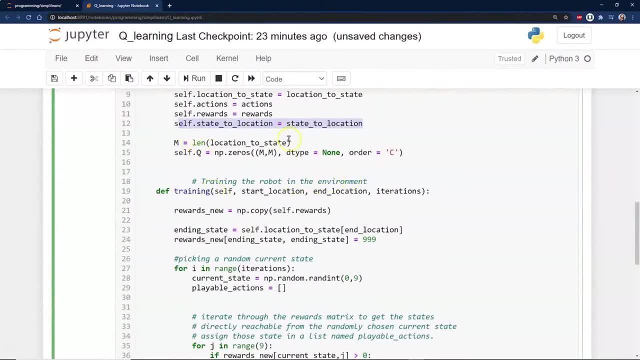 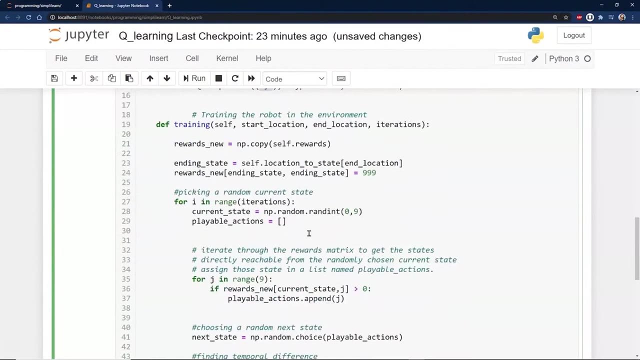 dictionary and we go ahead and create a queue learning table and I went ahead and just set the queue learning table up to zero to zero what the setup is, location to state how many of them are there. this just creates an array of zero to zero setup on there. 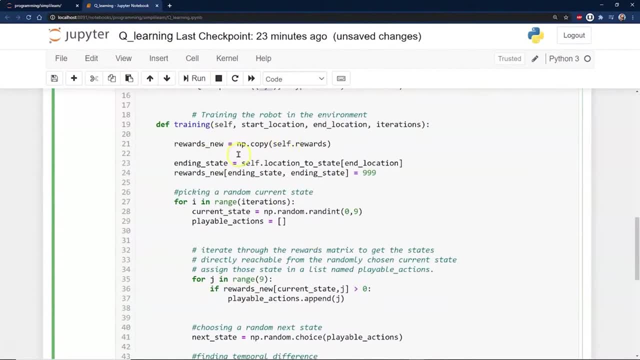 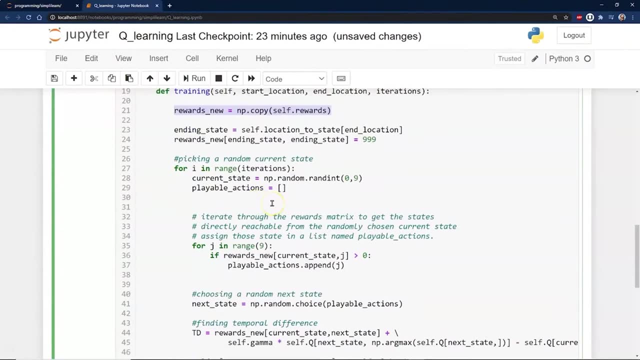 and then the big part is the training. we have our rewards new equals a copy of self dot. rewards: ending state equals the self location state in location. so this is whatever we end up at: rewards new equals ending state plus ending state equals nine, nine, nine, just kind of goes. 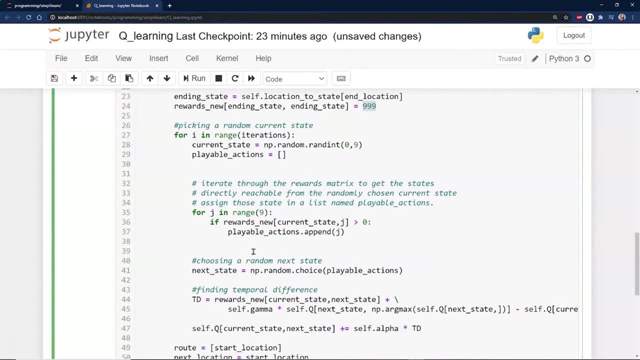 to a dead end and we start going through iterations and we'll go ahead. let's do this. so this we're going to come back and we're going to call it on here. let me just erase that. switch it to an arrow. there we go. so what we're doing is: 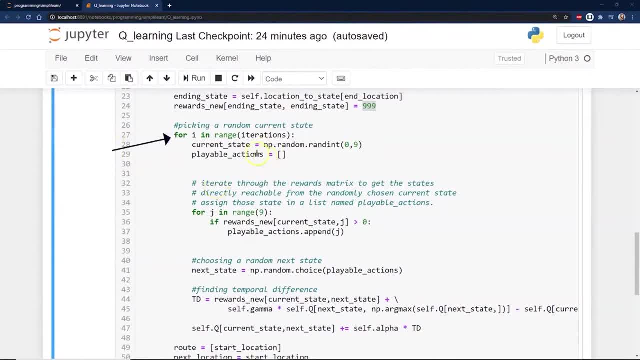 we're going to send in here to train it. we're going to say, hey, I want to iterate through this a thousand times and see what happens. now this part would actually be: instead of iterating, you might have your external environment, and they're going back and forth. 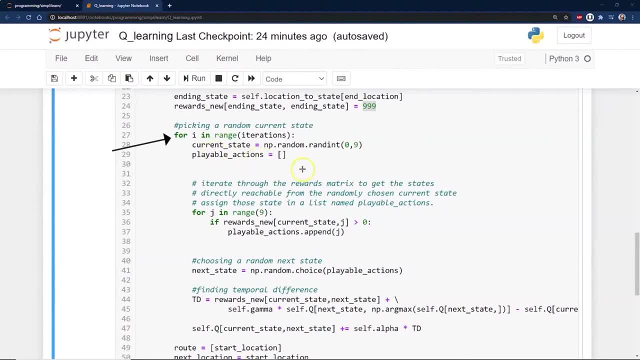 and you iterate through outside of here. but just for ease of use, our agent is going to come in here and iterate through this sometimes. I'll put this iteration in here and I'll have it call the environment and say, hey, this is what I did. what's the next state? 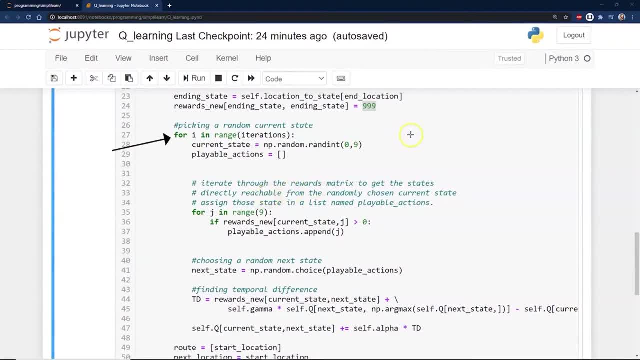 and the environment does its thing right in here as I iterate through it, and then we want to go ahead and pick a random state to start with. that's what's going on here. you have to start somewhere, and then you have your playable actions. we're going to start with just. 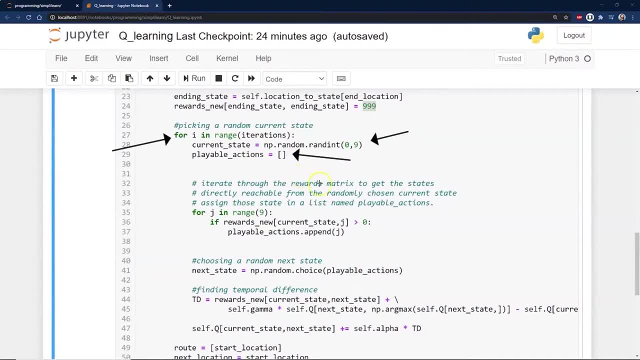 an empty thing for playable actions, and we'll fill that up. so that's what choices I have, and so we're going to iterate through the rewards matrix directly reachable from the randomly chosen current state, assign those states to a list named playable actions, and so you can see here. 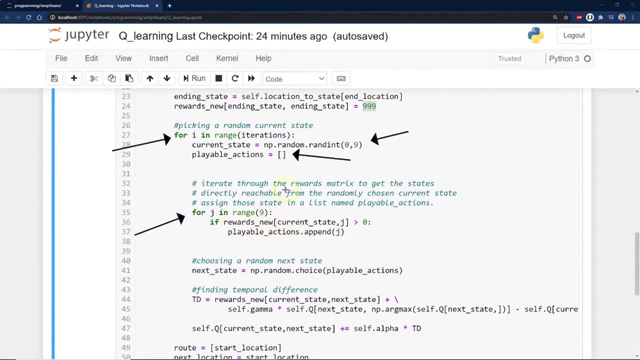 we have range 9. I usually use lengths of whatever I'm looking at, which is our locations or states as they are. we have a reward, so we want to look at the current the rewards. the new reward is our is in our chart here of rewards, underscore new. 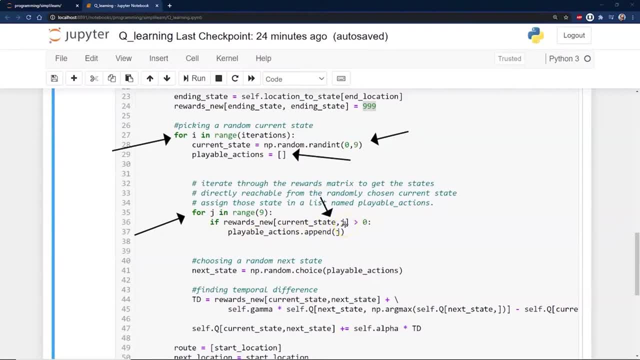 so we have our current state plus j, j being what is the next state we want to try, and so we go ahead and do our playable actions and we append j, and so what we're doing is we're randomly trying different things in here to see what's going to generate a better reward. 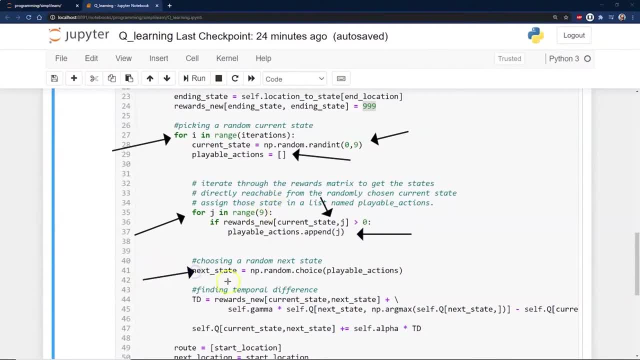 and then, of course, we go ahead and choose our next state. so we have our random choice, playable actions and if you remember, I mentioned on this- let me just go ahead and let's do a free form- when we were talking about the next state. this right here. 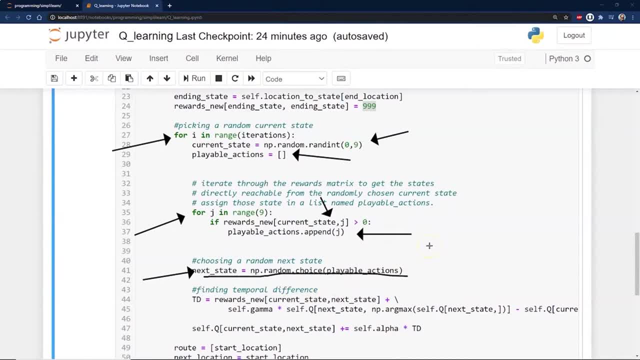 just does a random selection. instead of a random selection, you might do something where, whatever the best selection is, which might be option 3 here and then, so you can see that it might use a bell curve, and then option 2 over here might have a bell curve. 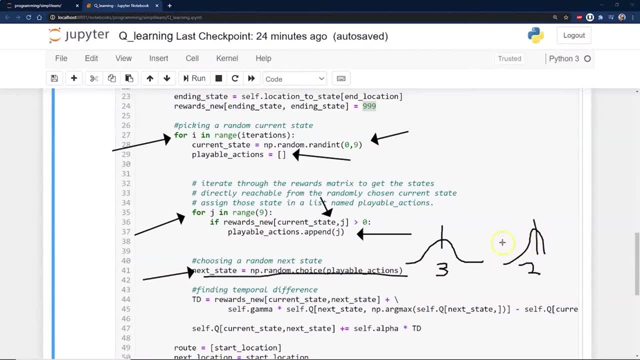 like this and we start looking at these averages and these spreads, or we can just add them all together and pick the one that kind of goes in all of those. so those are some of the options we have in here. we just go with the random choice. that's usually where you start to play with it. 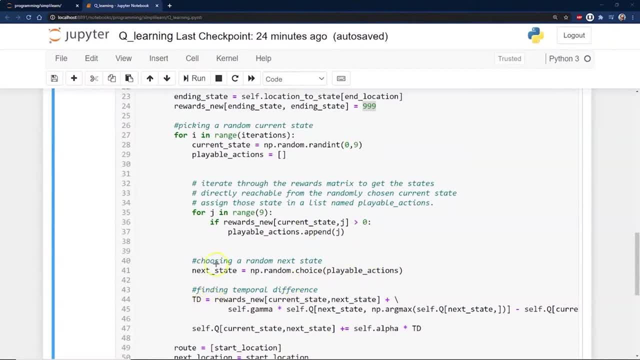 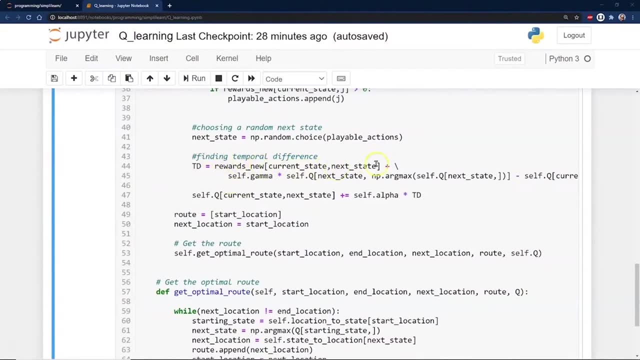 and then we have our rewards section down here, and so we want to go ahead and find- well, in this case the temporal difference. so you have your rewards new plus the self gamma, and this is the formula we were looking at. this is Bellman's equation here. 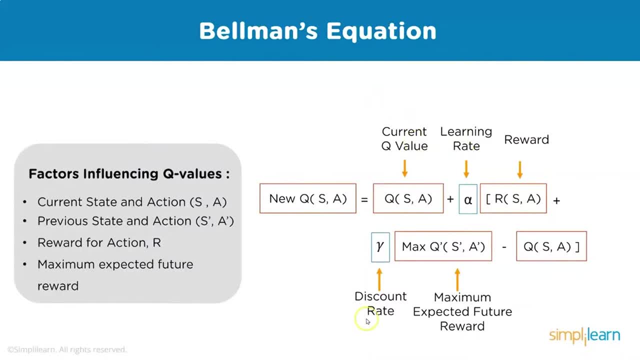 so we have our current value, our learning rate, our discount rate involved in there, the rewards system coming in for that, and we can add it all together. this is, of course, our maximum expected future set up in here. so this is all of our Bellman's equation. 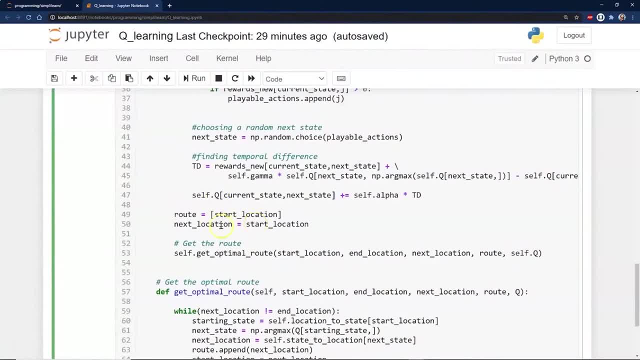 that we're looking at here, and then we come up in here and we update our queue table. that's all. this is on this one. that's right. here we have self queue- current state, next state- and we add in our alpha because we don't want to. 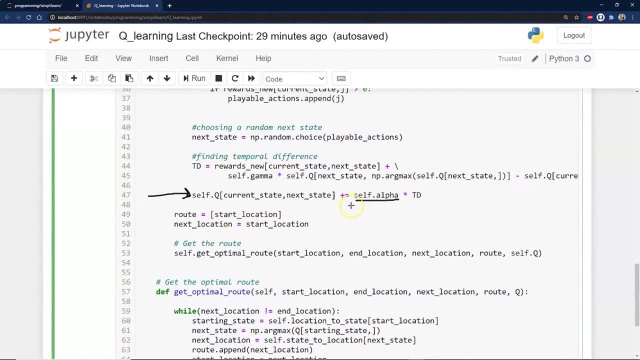 train all of it at once, in case there's slight differences coming in there. we want to slowly approach the answer and then we have: our route equals the start location and next location equals start location. so we're just incrementing. we took a step forward and then finally, 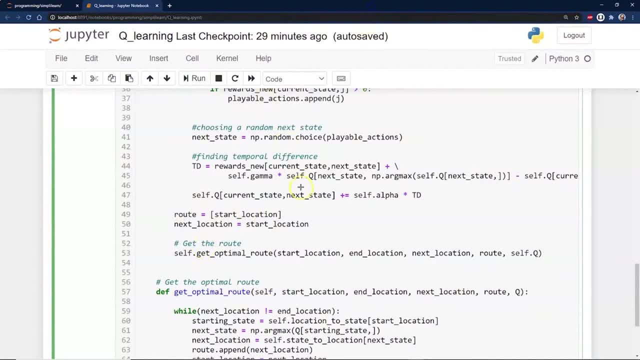 remember I was telling you how we're going to do all this and just have some simple thing at the end or just generates a simple path. we're going to go ahead and get the optimal route. we want to find the best route in here, and so we've created a definition for the optimal. 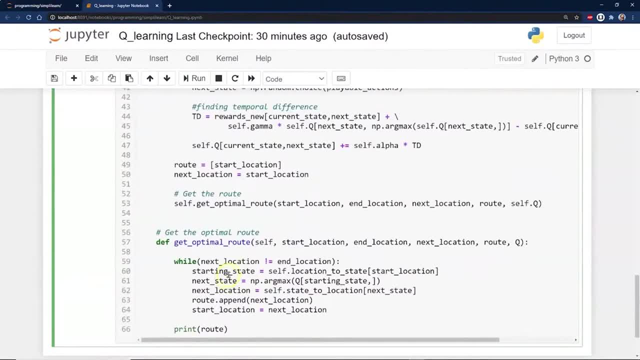 route down here. just scroll down for that and we get the optimal route. we go ahead and put the information in, including the queue table: self start location in location, next location- route queue and it says while next location is not equal to in location. so while we can still go. 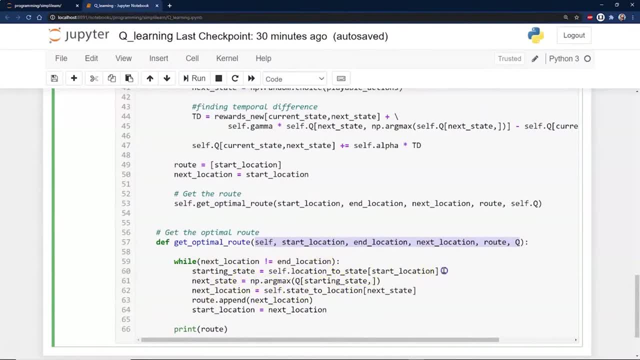 our start location equals self location to state start location. so we already have our best value for the start location. the next state looks at the queue table and says, hey, what's the next one with the best value? and then the next location. we go ahead and pull that in and we just append it. 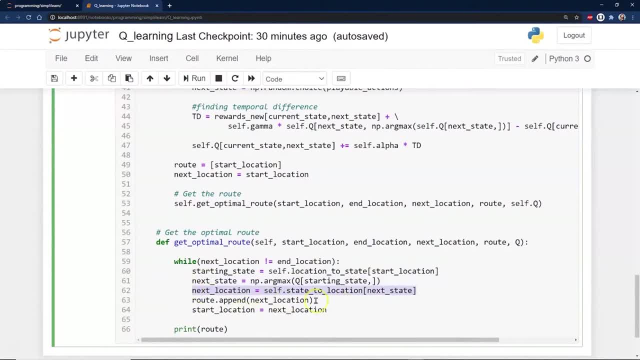 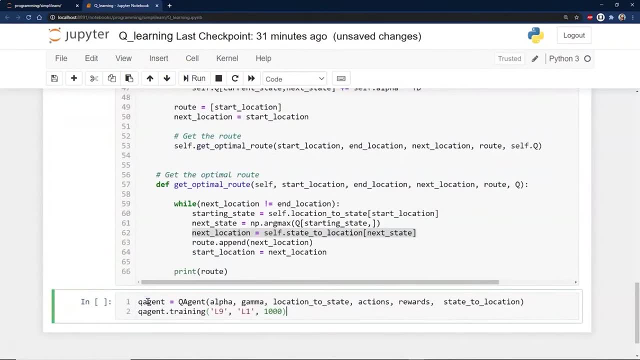 that's what's going on down here. and then our start location equals the next location and we just go through all the steps and we'll go ahead and run this and now that we have our queue table, queue agent loaded, we're going to go ahead and take. 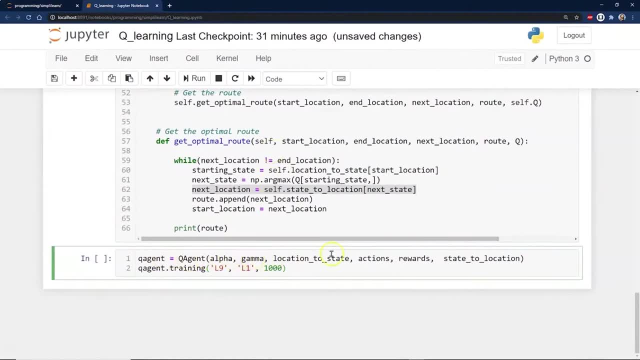 our queue agent, load them up with our alpha gamma that we set up above, along with the location step action, reward, state to location, and our goal is to plot a course between L9 and L1, and we're going to go through a thousand iterations on here, and so when I run that 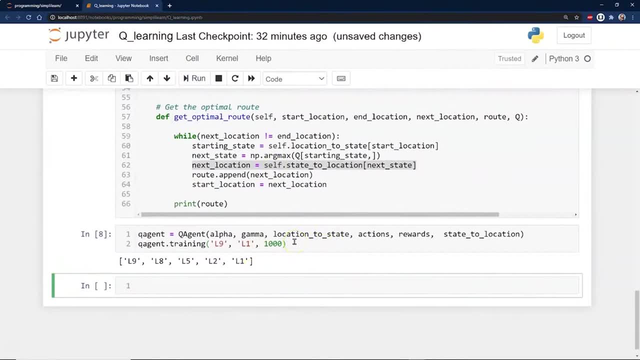 it runs pretty quick. why is this so fast? if you've been running neural networks and you've been doing all these other models, you sit here and wait a long time for a very small amount of data. these are all integers. these aren't float values. the math is not heavy on the processing end. 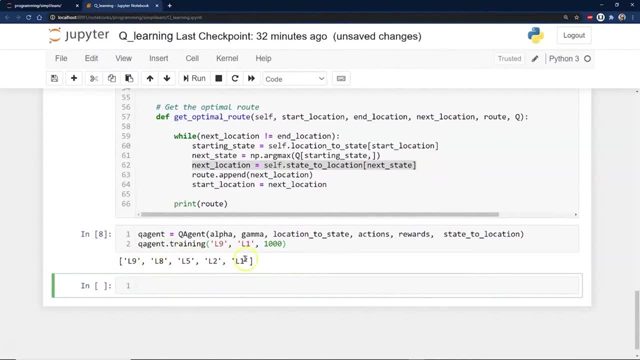 and this is where queue tables are so powerful. if you have a small amount of information coming in, you very quickly get an answer off of this, even though we went through it a thousand times to train it and you'll see. here we have L9,, 8,, 5. 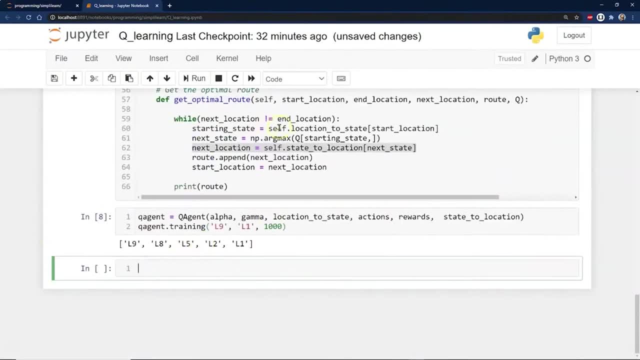 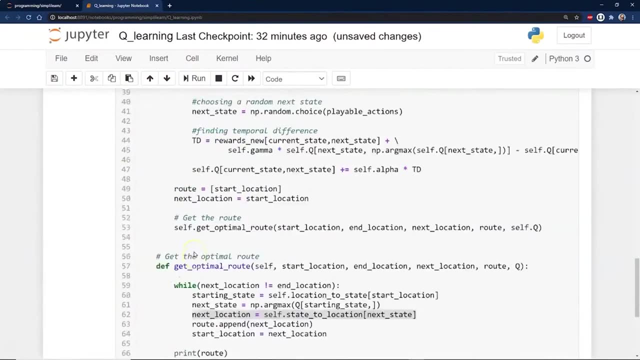 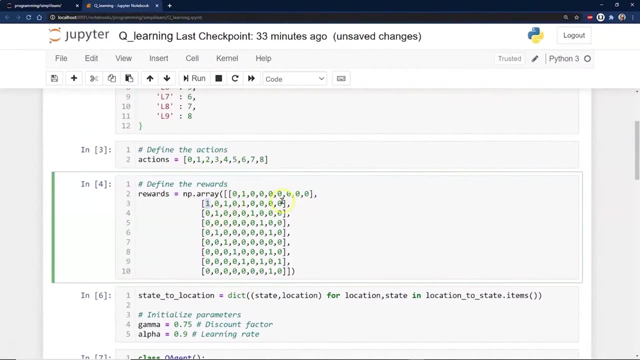 2 and 1 and that's based on our reward table we had set up on there and this is the shortest path between these different setups in here and if you remember on our reward table, you can see that if you start here, there's places you can't go. 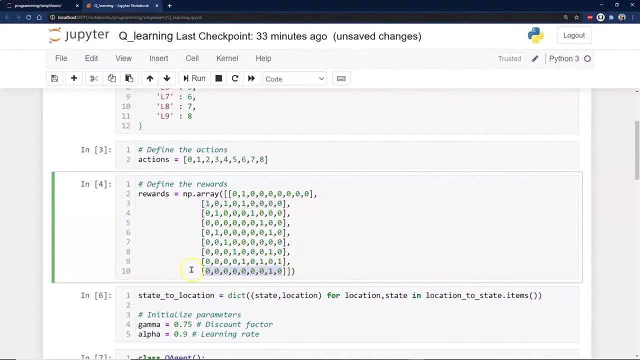 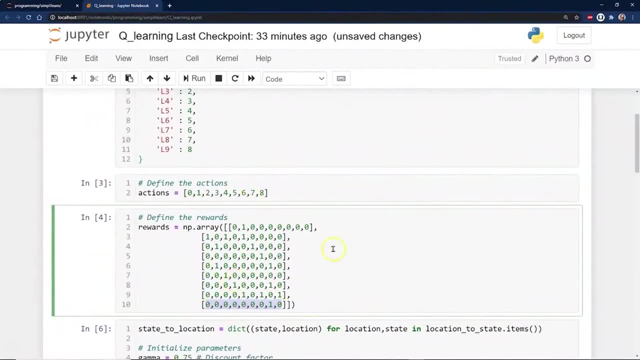 that's how this reward table was set up, so I can only go to certain places. so kind of a little maze setup in there and you can play with it. this is a really fun setup to play with and you can see how you can take this whole code and you can. 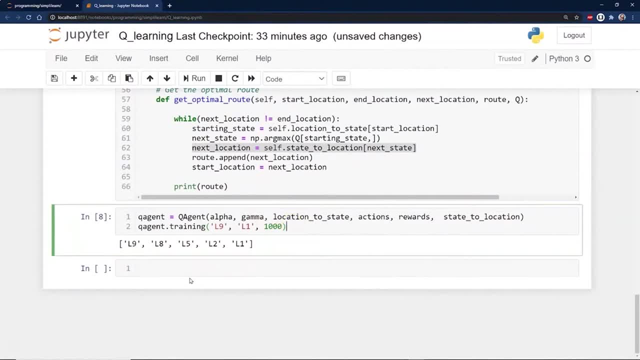 like I was saying earlier, you can embed it into another setup. you can model predictions where you put things into buckets and you're trying to guess the best investment, the best course of action, as long as you can take that course of action and reduce it down to a yes, no. 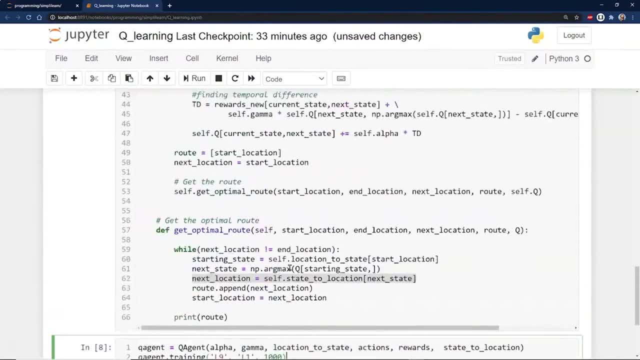 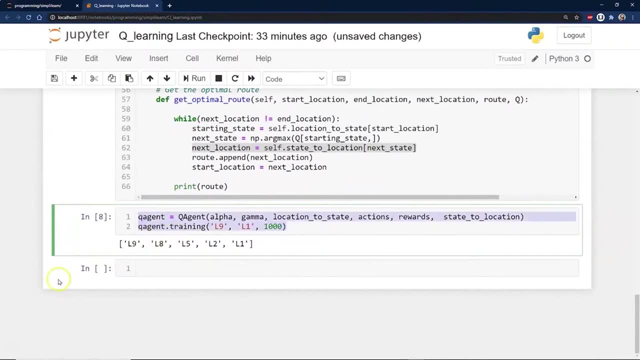 or if you're using text, you can use one hot encoder. which word is next? there's all kinds of things you can do with a queue table, depending on just how much information you're putting in there. so that wraps up our demo. in this demo, we've found the shortest distance. 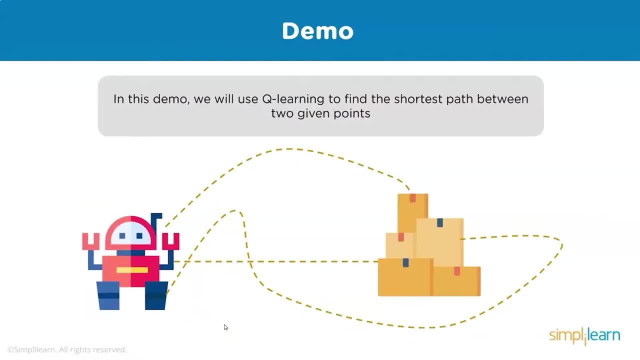 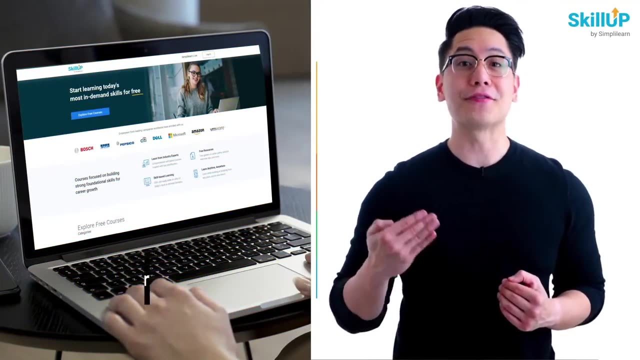 based on whatever rules or state rewards. we have to get from point A to point B and what available actions there are. if getting your learning started is half the battle, what if you could do that for free? visit SkillUp by SimplyLearn. click on the link in the description to know more. 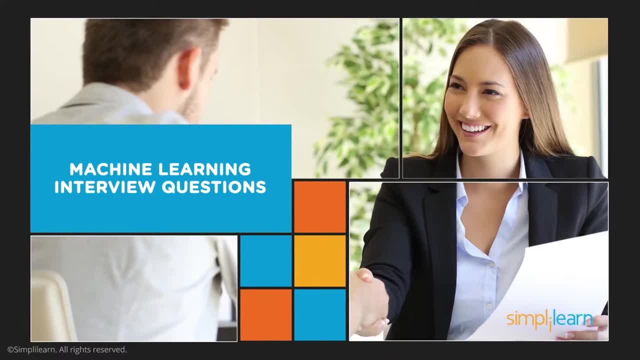 this video will probably help you when you're attending interviews or machine learning positions, and the attempt here is to probably consolidate 30 most commonly asked questions and to help you in answering these questions. we tried our best to give you the best possible answers but, of course, what is more important- 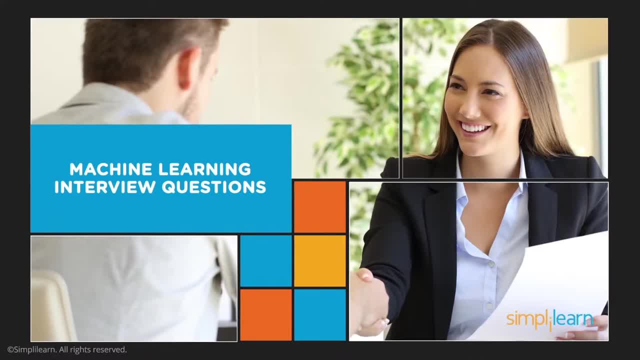 here is rather than the theoretical knowledge you need to kind of add to the answers or supplement your answers with your own experience. so the responses that we put here are a bit more generic in nature, so that if there are some concepts that you're not clear, this video will help you in kind of. 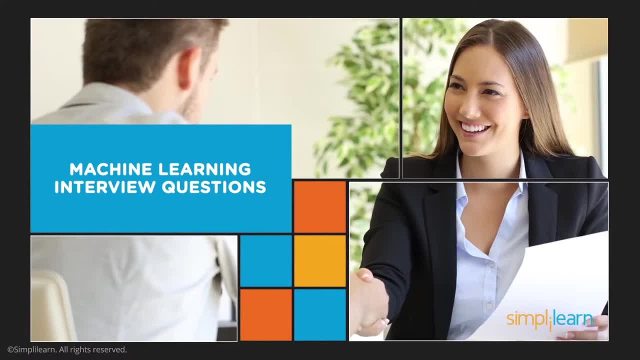 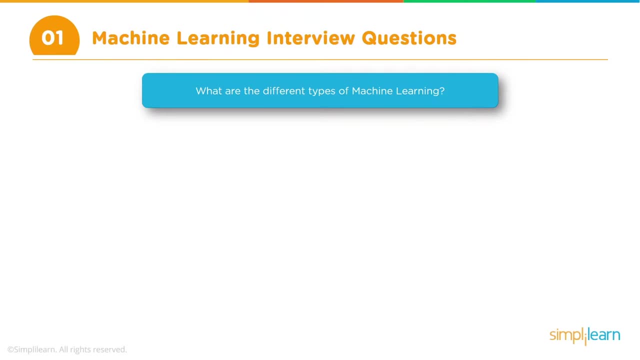 getting those concepts cleared up as well, but what is more important is that you need to supplement these responses with your own practical experience. okay, so with that, let's get started. so one of the first questions that you may face is: what are the different types of machine learning? 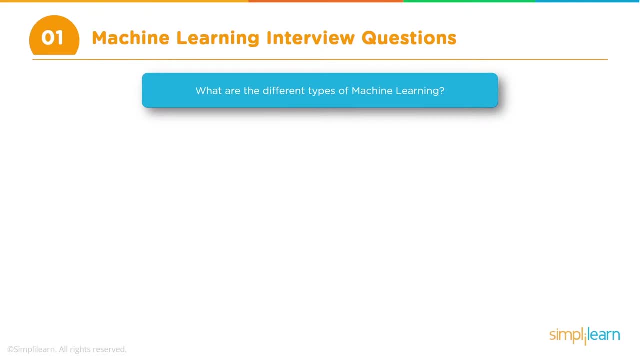 now what is the best way to respond to this? there are three types of machine learning. if you read any material, you will always be told there are three types of machine learning. but what is important is you would probably be better of emphasizing that there are actually two main. 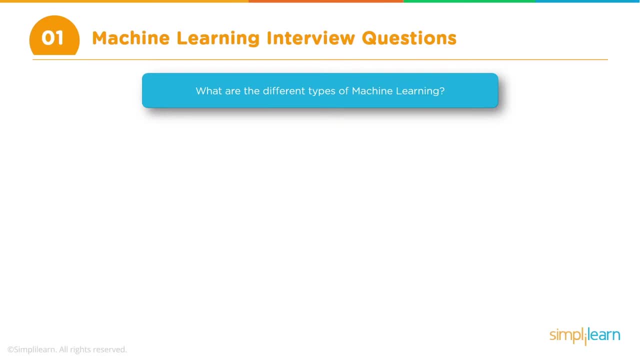 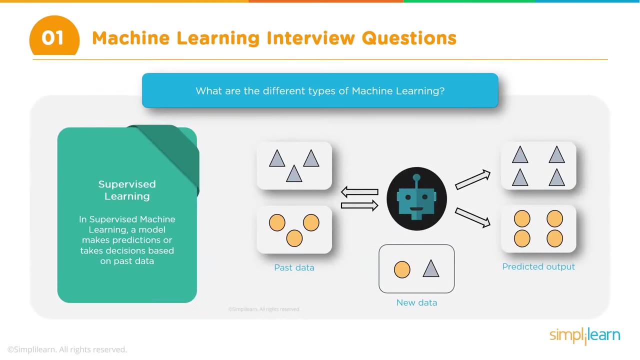 types of machine learning, which is supervised and unsupervised. and then there is a third type, which is reinforcement learning. supervised learning is where you have some historical data and then you feed that data to your model to learn. now you need to be aware of a key word: that 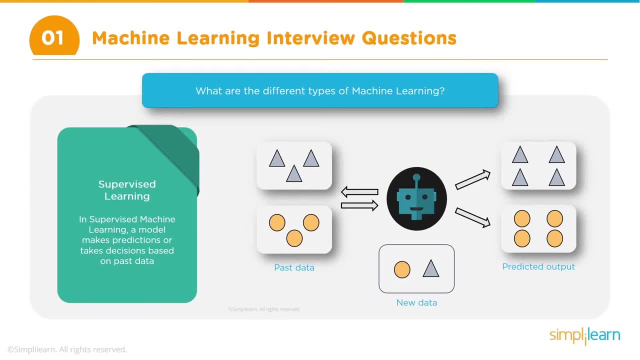 they will be looking for. which is labeled data? right? so if you just say past data or historical data, the impact may not be so much. you need to emphasize on labeled data. so what is labeled data basically? let's say, if you are trying to do training model, 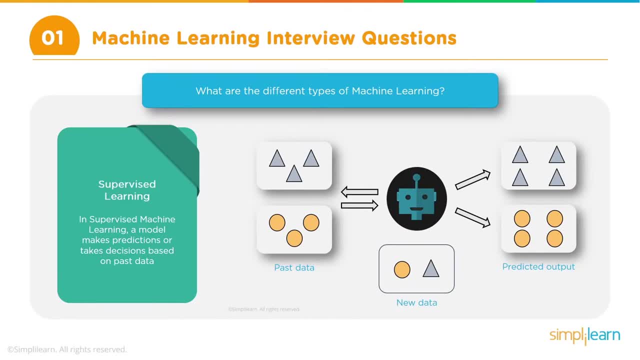 for classification you need to be aware of for your existing data. which class each of the observations belong to right. so that is what is labeling. so it is nothing but a fancy name, but just make it a point to throw in that key word labeled, so that will have the 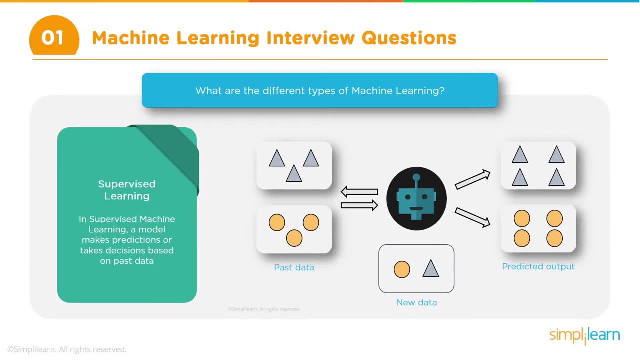 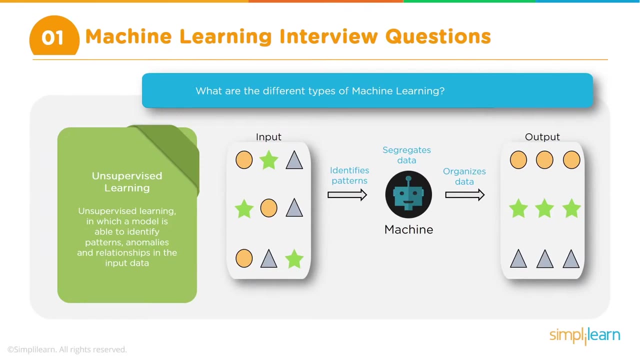 right impact. okay, so that is what is supervised learning: when you have existing labeled data which you then use to train your model. that is known as supervised learning, and unsupervised learning is when you don't have this labeled data. so you have data, it is not labeled, so the system 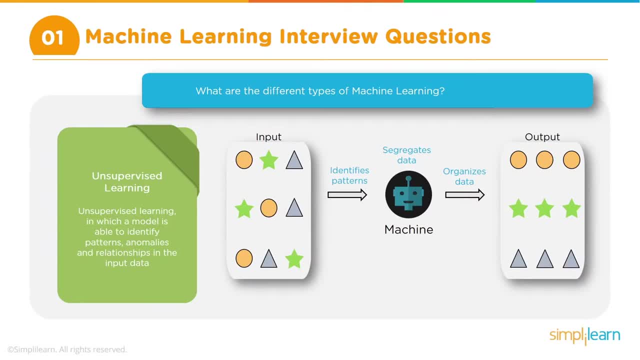 has to figure out a way to do some analysis on this. okay, so that is unsupervised learning, and you can then add a few things like what are the ways of performing supervised learning and unsupervised learning, or what are some of the techniques. so supervised learning, we. 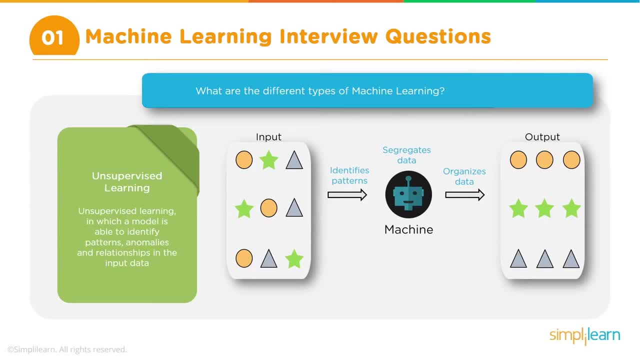 perform, or we do, regression and classification and unsupervised learning. we do clustering, and clustering can be of different types. similarly, regression can be of different types, but you don't have to probably elaborate so much if they are asking for just the different types. you can just mention. 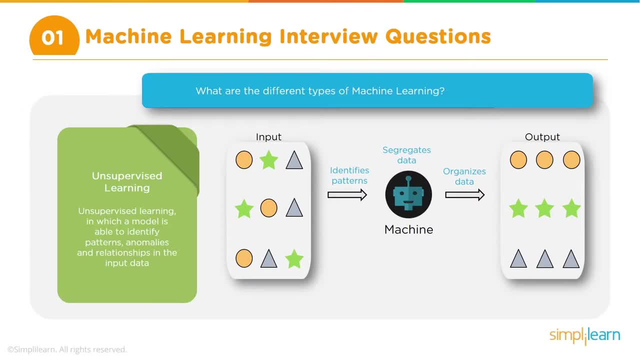 these, and just at a very high level. if they want you to elaborate, give examples, then of course. if nothing, there is a different question for that. we will see that later. then the third: so we have supervised, then we have unsupervised, and then reinforcement: you need to provide a 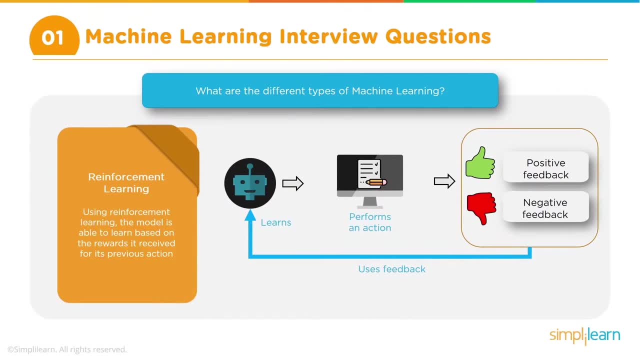 little bit of information around that as well, because it is sometimes a little difficult to come up with a good definition for reinforcement learning, so you may have to a little bit elaborate on how reinforcement learning works right. so reinforcement learning works in in such a way that it basically has: 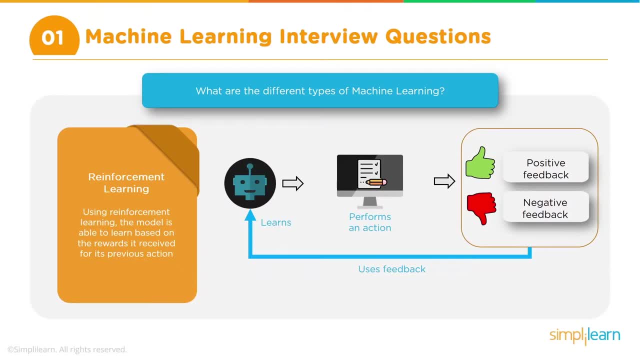 two parts to it. one is the agent and the environment. and the agent basically is working inside of this environment and it is given a target that it has to achieve and every time it is moving in the direction of the target. so the agent basically has to take. 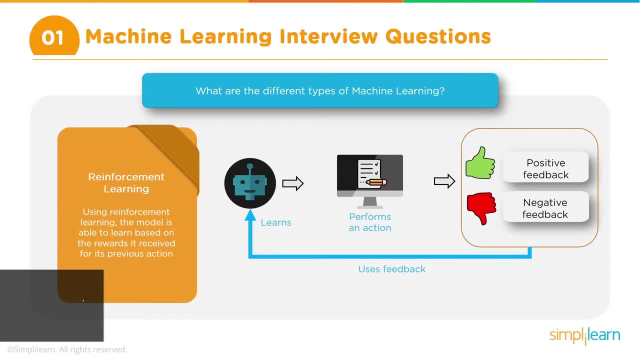 some action and every time it takes an action which is moving the agent towards the target, right towards a goal- a target is nothing but a goal- okay, then it is rewarded. and every time it is going in a direction where it is away from the goal, then it 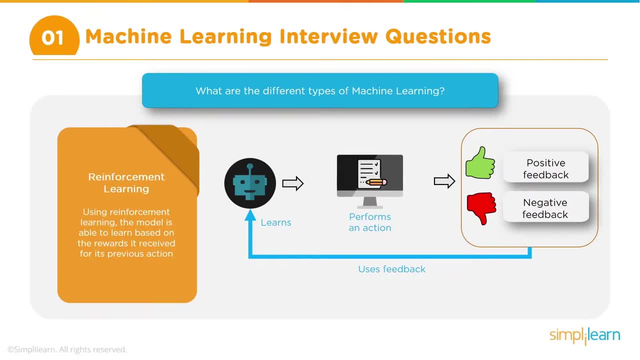 is punished. so that is the way you can a little bit explain. and this is used primarily or very, very impactful for teaching the system, to learn games and so on. examples of this are basically used in alpha go. you can throw that as an example where alpha go. 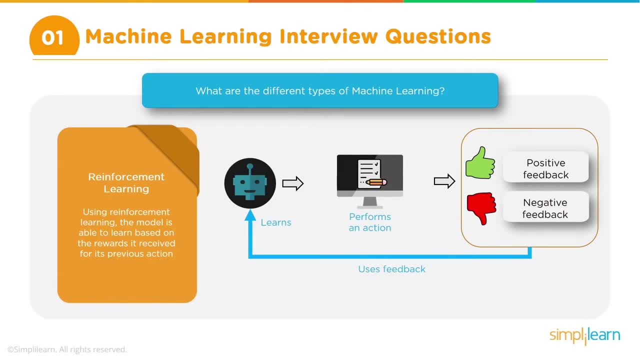 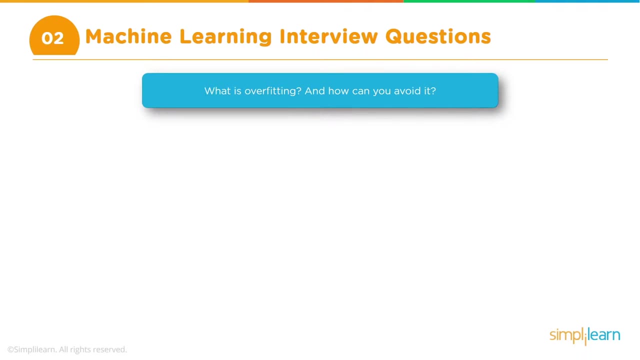 used reinforcement learning to actually learn to play the game of go and finally it defeated the go world champion. right? this much of information? that would be good enough. okay, then there could be a question on overfitting. uh, so the question could be: what is overfitting and how can you? 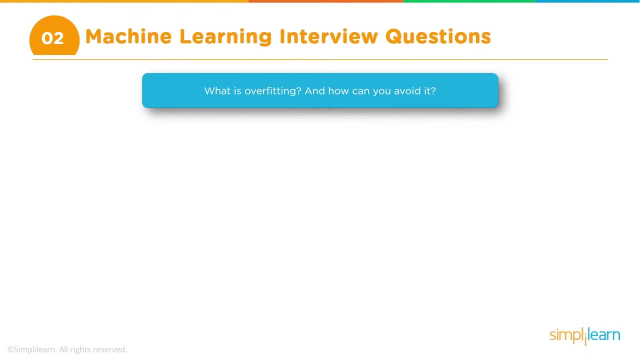 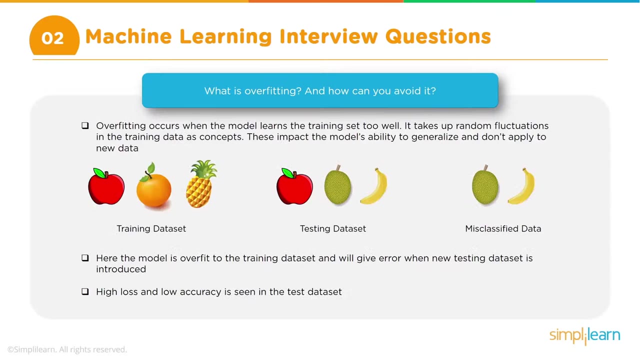 avoid it. so what is overfitting? let's first try to understand the concept, because sometimes overfitting may be a little difficult to understand. overfitting is a situation where the model has kind of memorized the data. so this is an equivalent of recognizing the data, so we can draw an. 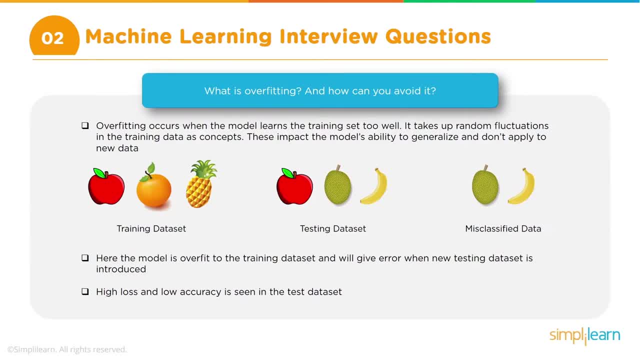 analogy so that it becomes easy to explain this. now, let's say, you're teaching a child about recognizing some fruits or something like that- okay. and you're teaching this child about recognizing, let's say, three fruits: apples, oranges and pineapples- okay. so this is a small child and for the first, 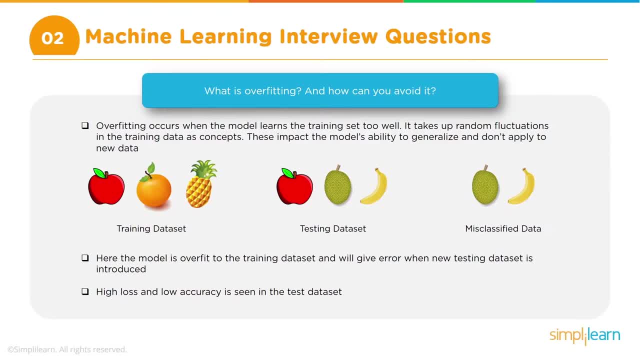 time you're teaching the child to recognize fruits, then. so what will happen? so this is very much like that is your training data set. so what you will do is you will take a basket of fruits which consists of apples, oranges and pineapples, okay, and you take this basket to this child and 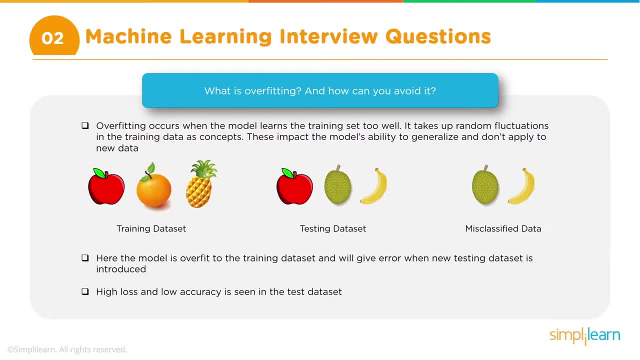 there may be, let's say, hundreds of these fruits. so you take this basket to this child and keep showing each of this fruit and then first time, obviously, the child will not know what it is. so you show an apple and you say, hey, this is apple. then you show maybe an orange and say: 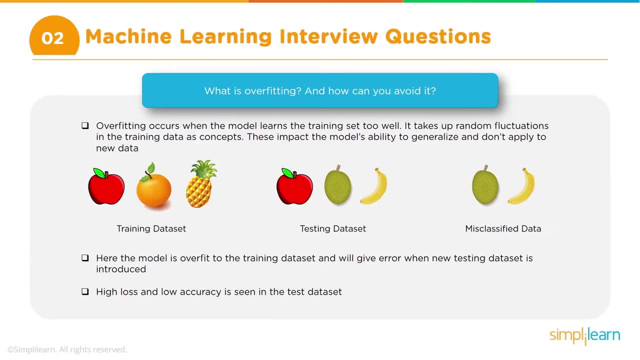 this is orange, and so on and so forth, and then again you keep repeating that right. so until that basket is over. this is basically how training work. in machine learning also, that's how training works. so till the basket is completed- maybe 100 fruits- you keep showing this child. 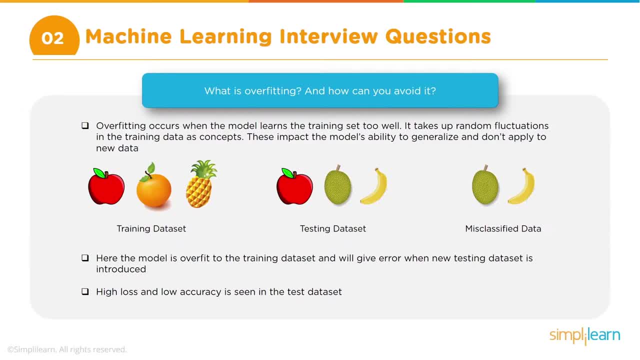 and then in the process, what has happened? the child has pretty much memorized these. so even before you finish that basket right by the time you are halfway through, the child has learned about recognizing the apple, orange and pineapple. now what will happen after halfway through? initially, you remember 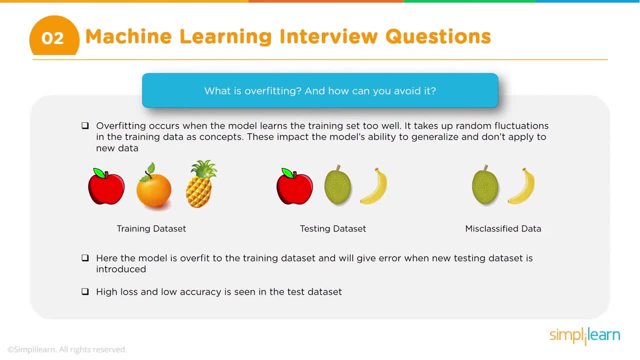 it made mistakes in recognizing but i'm sure halfway through now it has learned. so every time you show a fruit, it will exactly 100 accurately it will identify. it will say: the child will say: this is an apple, this is an orange. and if you show a pineapple it will say: 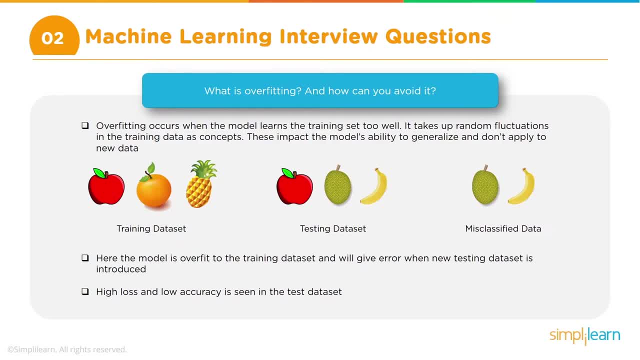 this is a pineapple right, so that means it has kind of memorized this data. now, let's say, you bring another basket of fruits and it will have a mix of maybe apples, which were already there in the previous set, but it will also have in addition to apple it will. 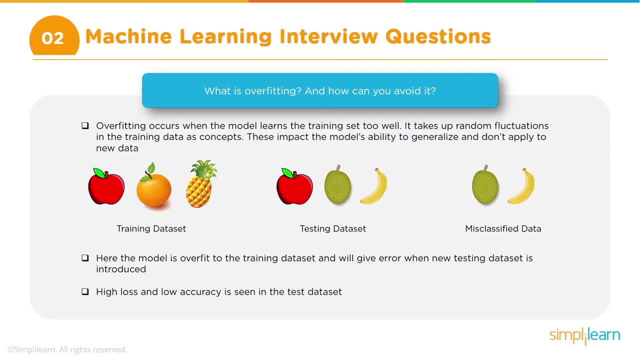 have a banana or maybe another fruit like a jackfruit, right. so this is an equivalent of your test data set, which the child has not seen before. some parts of it it probably has seen, like the apples it has seen, but this banana and jackfruit it has not seen. so 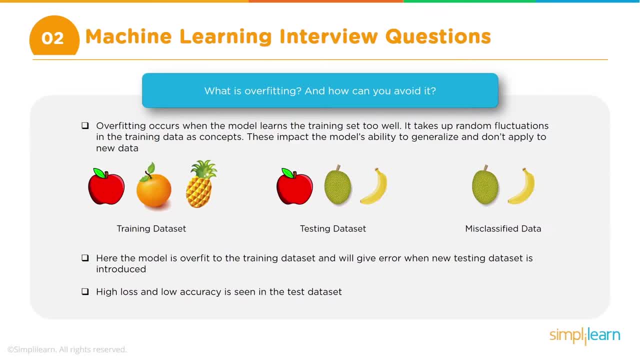 then what will happen in the first round, which is an equivalent of your training data set. towards the end it has 100. it was telling you what the fruits are right: apple was accurately recognized, orange was accurately recognized and pineapples were accurately recognized, right. so that is like a hundred percent. 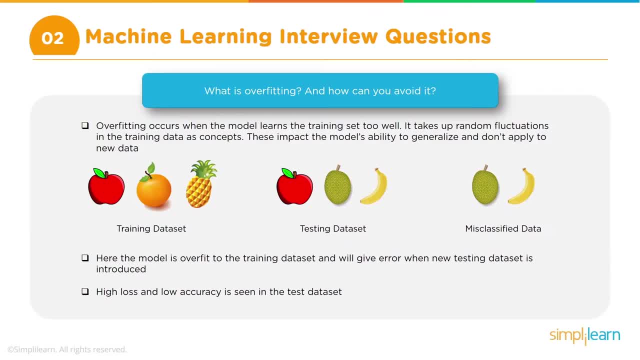 accuracy. but now, when you get another, a fresh set, which were not part of the original one, what will happen? all the apples maybe it will be able to recognize correctly, but all the others, like the jackfruit or the banana, will not be recognized by the child, right? 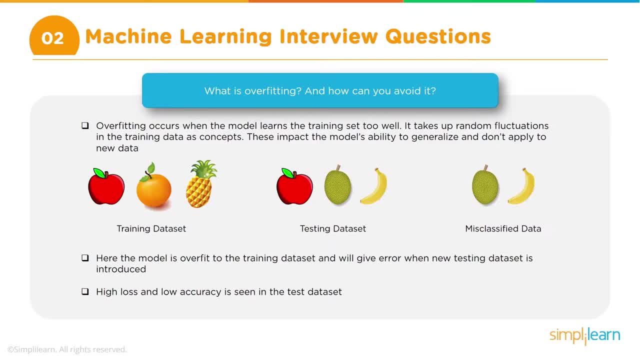 so this is an analogy, this is an equivalent of overfitting. so what has happened during the training process? it is able to recognize or reach 100 accuracy, maybe very high accuracy, okay, and we call that as very low loss, right, so that is the technical term. so the loss is pretty. 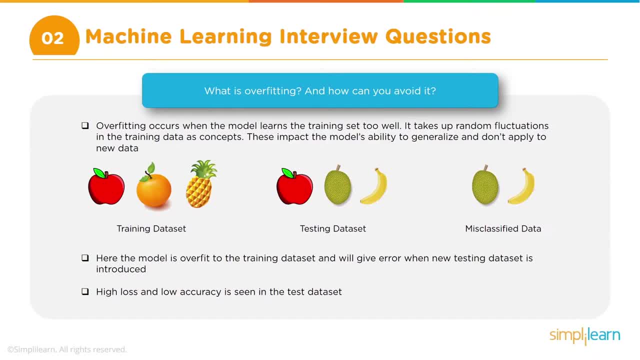 much zero and accuracy is pretty much 100, whereas when you use testing, there will be a huge error, which means the loss will be pretty high and therefore the accuracy will be also low. okay, this is known as overfitting. this is basically a process where training is done. training processes it. 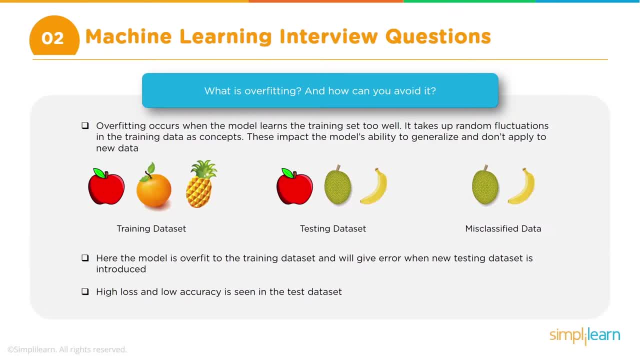 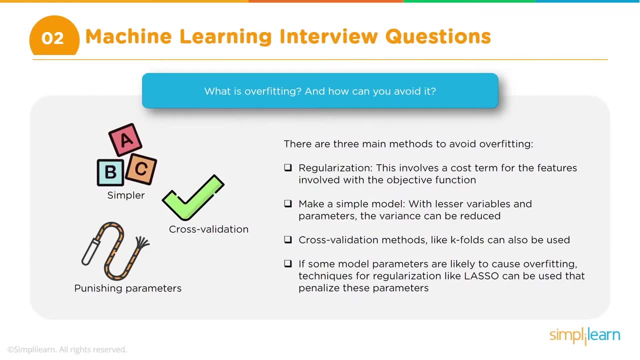 goes very well, almost reaching 100 accuracy, but while testing it really drops down. now how can you avoid it? so that is the extension of this question. there are multiple ways of avoiding overfitting. there are techniques like what you call regularization. that is the most common technique, that 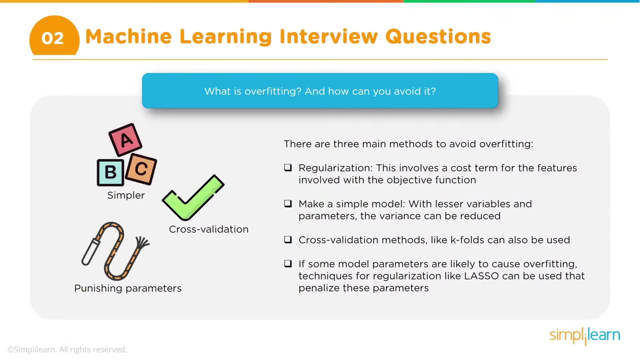 is used for avoiding overfitting and within regularization there can be a few other subtypes, like drop out in case of neural networks and a few other examples. but i think if you give example or if you give regularization as the technique, probably that should be sufficient. 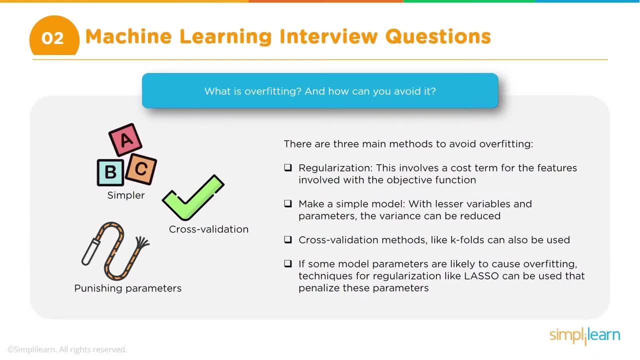 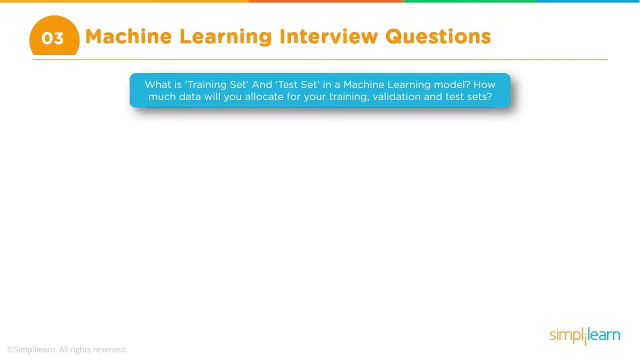 so. so there will be some questions where the interviewer will try to test your fundamentals and your knowledge and depth of knowledge and so on and so forth, and then there will be some questions which are more like quick questions, that will be more to stumble. okay, then the next question is around. 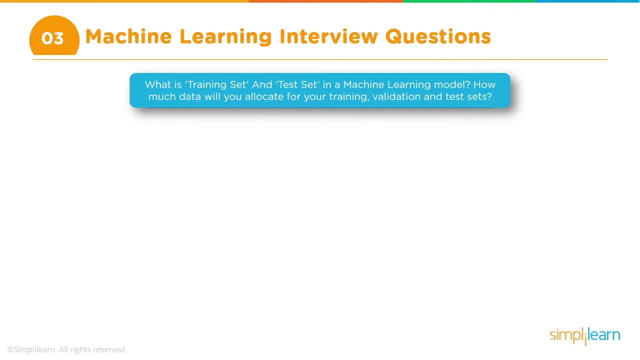 the methodology. so when we are performing machine learning training, we split the data into training and test, right? so this question is around that. so the question is: what is training set and test set in machine learning model and how is the split done? so the question can be like: 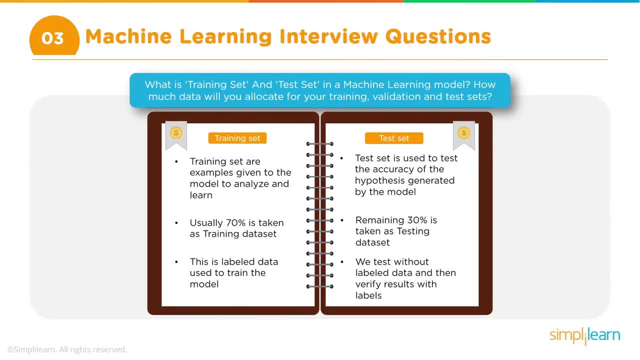 that. so in machine learning, when we are trying to train the model. so we have a three-step process: we train the model and then we test the model and then, once we are satisfied with the test, only then we deploy the model. so what happens in the train and test is that you. 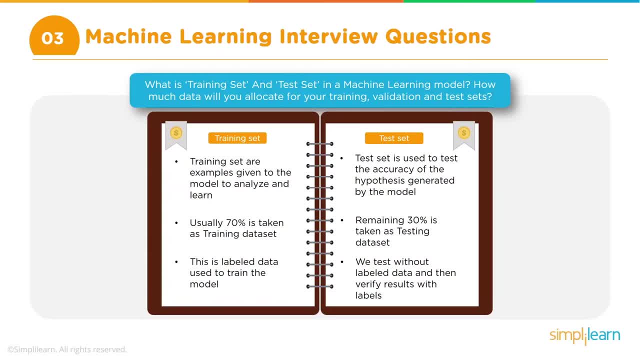 remember the labeled data. so let's say a, you have thousand records with labeling information. now, one way of doing it is you use all the thousand records for training and then maybe right, which means that you have exposed all these thousand records during the training process, and then you take. 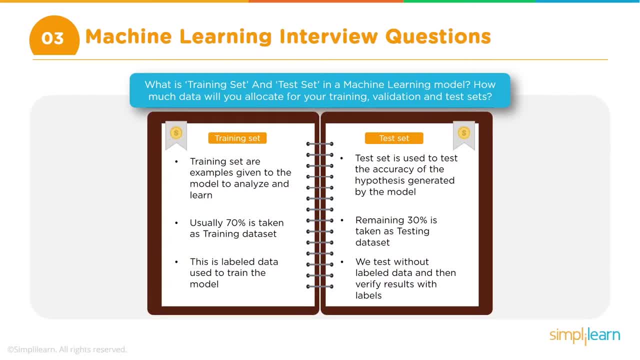 a small set of the same data and then you say, okay, i will test it with this, okay, and then you probably what will happen? you may get some good results right, but there is a flaw there. what is the flaw? this is very similar to human beings. it is like. 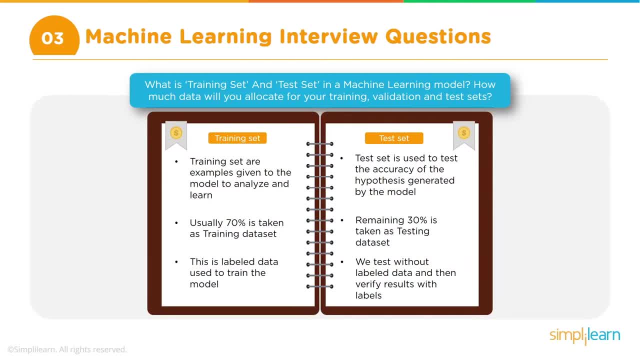 you are showing this model, the entire data, as a part of training. okay, so obviously it has become familiar with the entire data. so when you are taking a part of that again and you are saying that i want to test it, obviously you will get good results. so 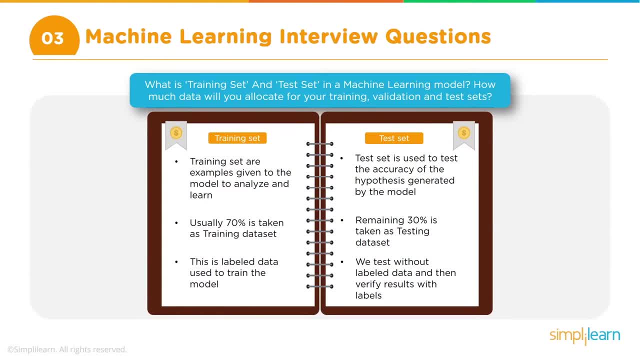 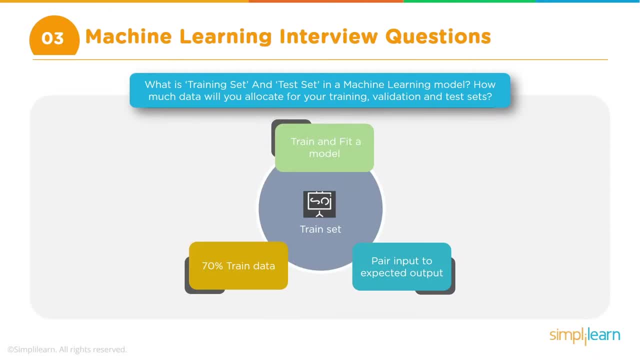 that is not a very accurate way of testing. so that is the reason what we do is we have the label data of this thousand records or whatever we set aside before starting the training process. we set aside a portion of that data and we call that test set and the 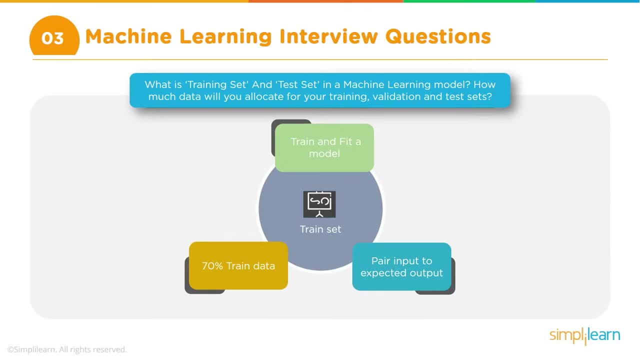 remaining we call as training set and we use only this for training. our model now the training process, remember- is not just about passing one round of this data set. so let's say, now your training set has 800 records. it is not just one time you pass this. 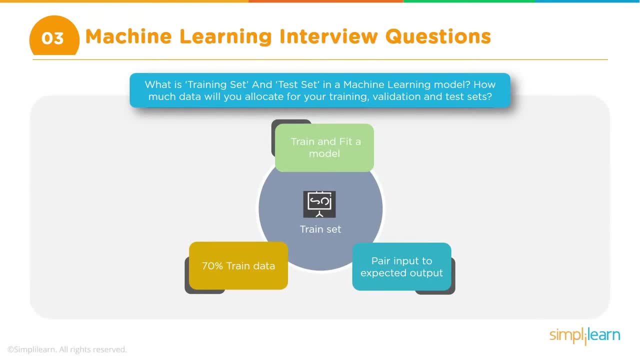 800 records. what you normally do is you actually, as a part of the training, you may pass this data through the model multiple times. so this thousand records may go through the model, maybe 10, 15, 20 times, till the training is perfect, till the accuracy is high. 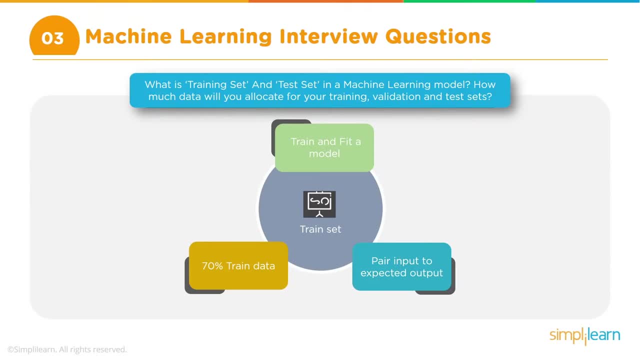 till the errors are minimized. okay, now so, which is fine, which means that your- that is what is known as the model- has seen your data and gets familiar with your data. and now, when you bring your test data, what will happen is: this is like some new data, because that is. 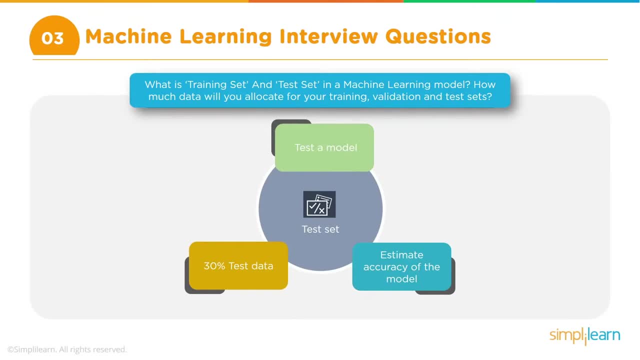 where the real test is. now you have trained the model and now you are testing the model with some data which is kind of new. that is like a situation like like a realistic situation, because when the model is deployed, that is what will happen. it will receive some new data, not the 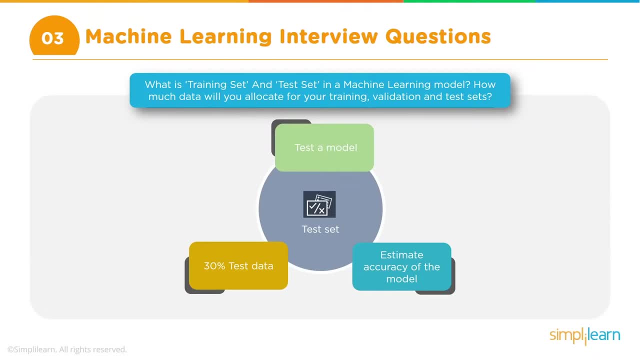 data that it has already seen right. so this is a realistic test. so you put some new data. so this data which you have set aside is for the model. it is new and if it is able to accurately predict the values, that means your training has worked. okay, the model got. 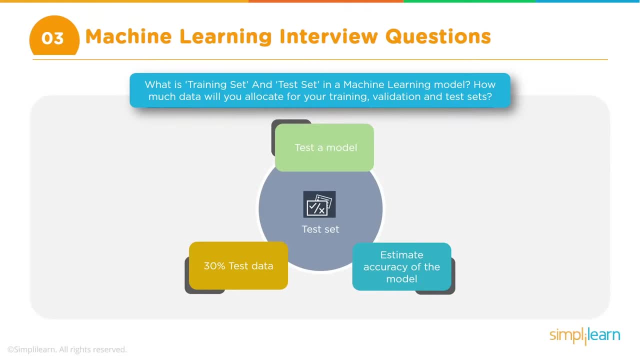 trained properly. but let's say, while you're testing this with this test data, you're getting a lot of errors. that means you need to probably either change your model or retrain with more data and things like that. now coming back to the question of how do you split this? what should be the 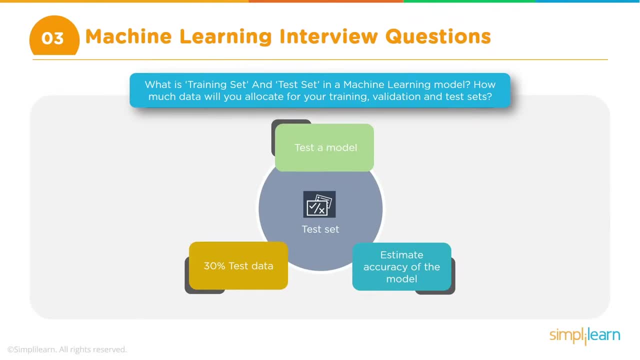 ratio. there is no fixed number. again, this is like individual preferences. some people split it into 50- 50, 50 test and 50 training. some people prefer to have a larger amount for training and a smaller amount for test, so they can go by either 60, 40 or 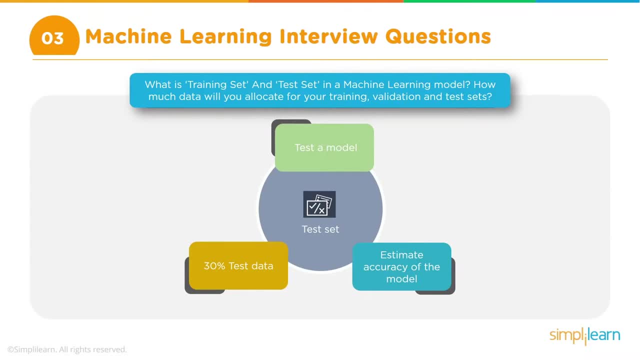 70, 30 or some people even go with some odd numbers like 65, 35 or 63.33 and 33, which is like one-third and two-thirds. so there is no fixed rule that it has to be something. the ratio has to be this. you can go by. 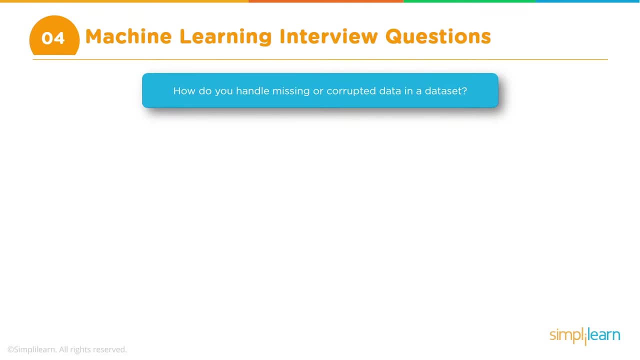 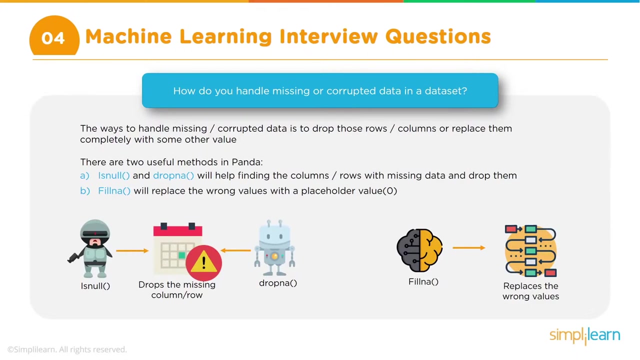 your individual preferences, all right. then you may have questions around data handling, data manipulation or what do you call data management or preparation. so these are all some questions around that area. there is, again, no one answer, one single good answer to this. it really varies from situation to 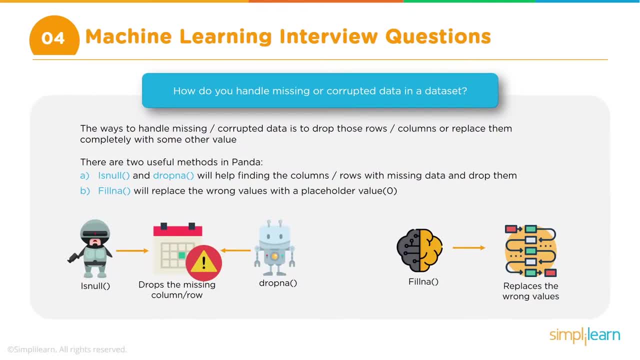 situation and depending on what exactly is the problem, what kind of data it is, how critical it is, what kind of data is missing and what is the type of corruption. so there are a whole lot of things, which is a very generic question and therefore you need to be a little. 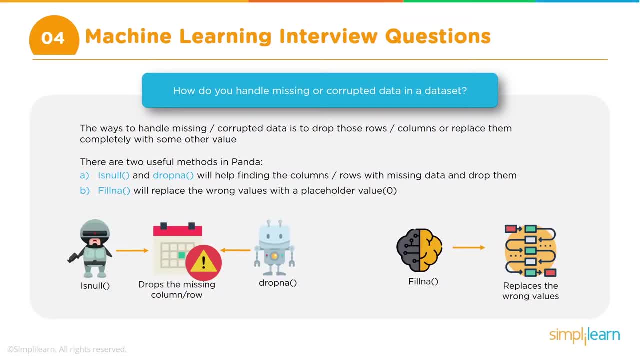 careful about responding to this as well, so probably have to illustrate this again. if you have experience in doing this kind of work in handling data, you can illustrate with examples, saying that i was on one project where i received this kind of data. these were the columns where data was not filled or 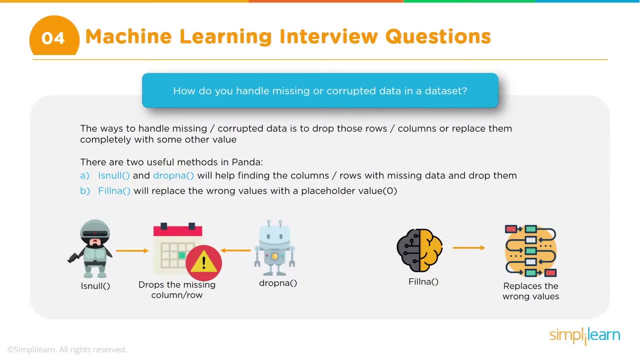 these were the, this many rows where the data was missing. that would be, in fact, a perfect way to respond to this question, but if you don't have that, obviously you have to provide some good answer. i think it really depends on what exactly the situation is, and there are multiple ways. 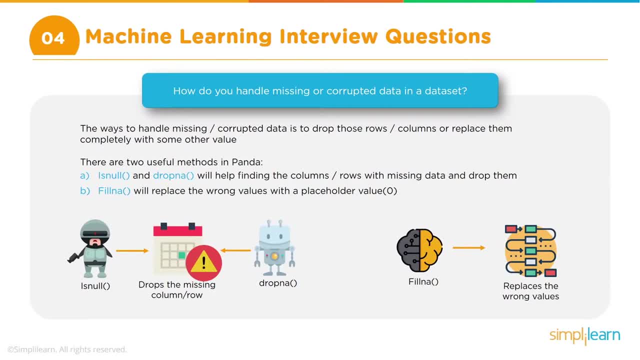 of handling the missing data or corrupt data. now let's take a few examples now. let's say you have data where some values in some of the columns are missing and you have pretty much half of your data having these missing values in terms of number of rows. 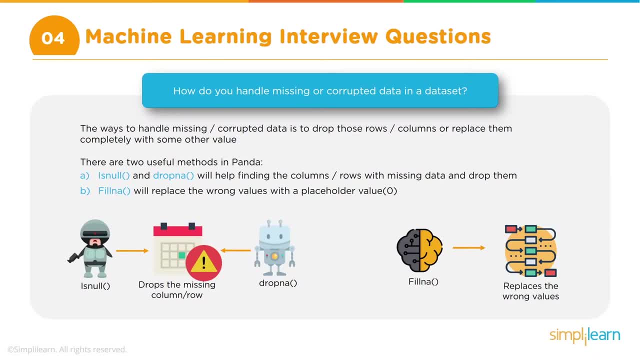 okay, that could be one situation. another situation could be that you have records or data missing, but when you do some initial calculation, how many records are corrupt, or how many rows or observations, as we call it, has this missing data? let's assume it is very minimal, like. 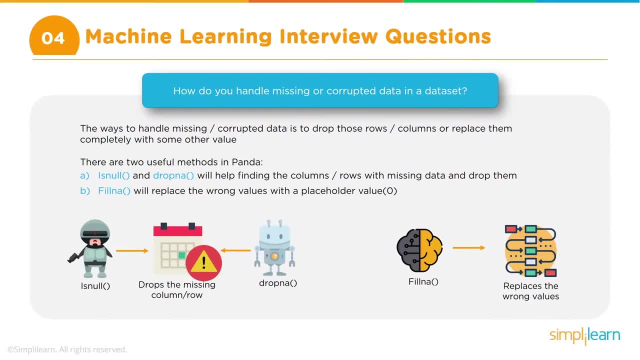 10 percent. okay, now, between these two cases, how do we so? let's assume that this is not a mission critical situation and in order to fix this 10 of the data, the effort that is required is much higher, and obviously effort means also time and money, right? so 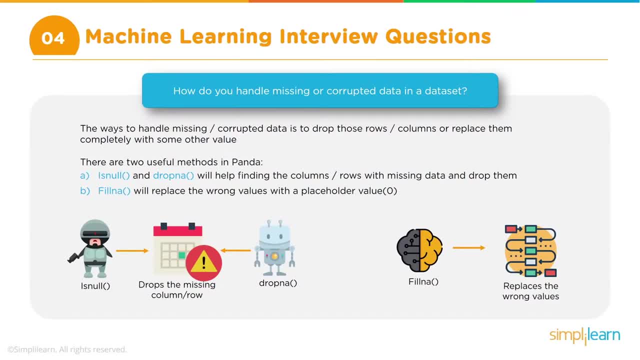 it is not so mission critical and it is okay to, let's say, get rid of these records. so obviously one of the easiest ways of handling the data part or missing data is remove those records or remove those observations from your analysis. so that is the easiest way to do. 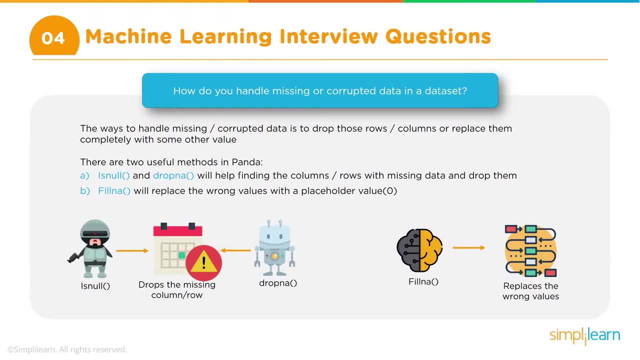 but then the downside is, as i said in as in the first case, if, let's say, 50 of your data is like that, because some column of the other is missing, so it is not like every in every place, in every row, the same column is missing. 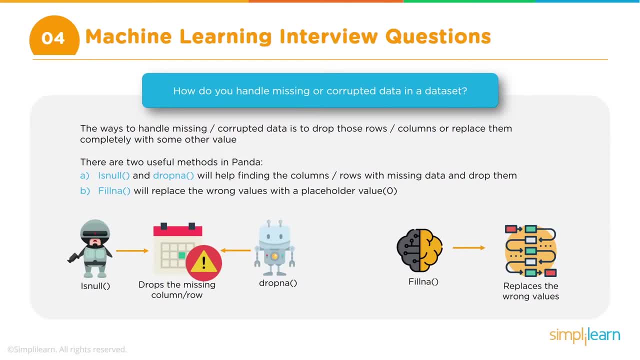 but you have in maybe 10 percent of the records. column one is missing and another 10, column two is missing, another 10 column three is missing, and so on and so forth. so it adds up to maybe half of your data set. so you cannot completely. 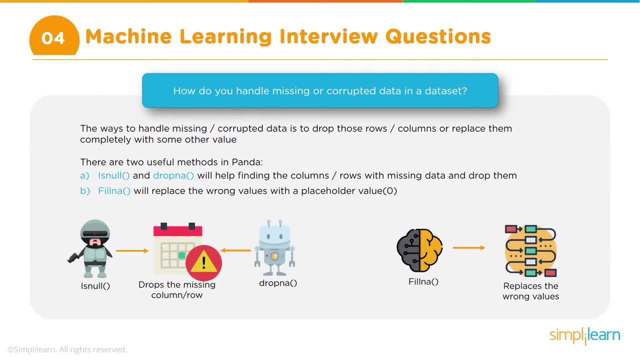 remove half of your data set, then the whole purpose is lost. okay, so then, how do you handle? then you need to come up with ways of filling up this data with some meaningful value. right, that is one way of handling. so when we say meaningful value, what is? 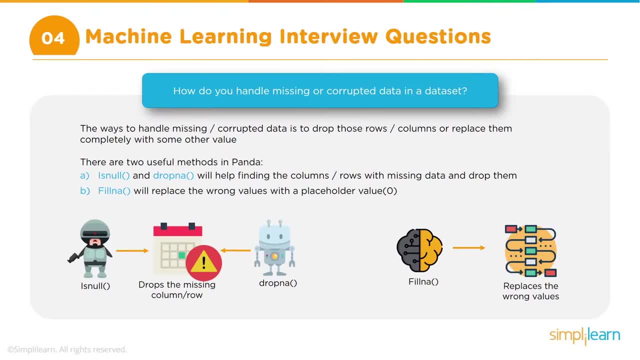 that meaningful value, let's say for a particular column. you might want to take a mean value for that column and fill wherever the data is missing. fill up with that mean value so that when you're doing the calculations your analysis is not completely way off, so you have values which are not missing. 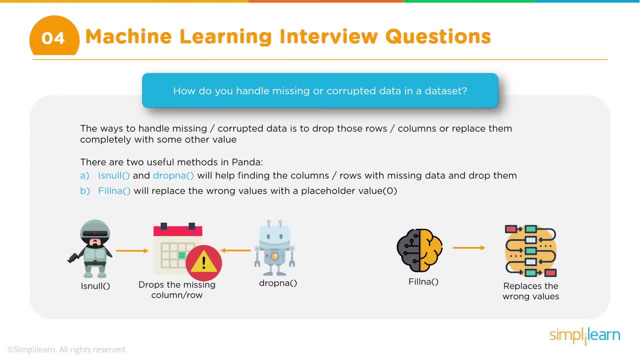 first of all, so your system will work. number two: these values are not so completely out of whack that your whole analysis goes for a toss right. there may be situations where, if the missing values, instead of putting mean, maybe a good idea to fill it up with the. 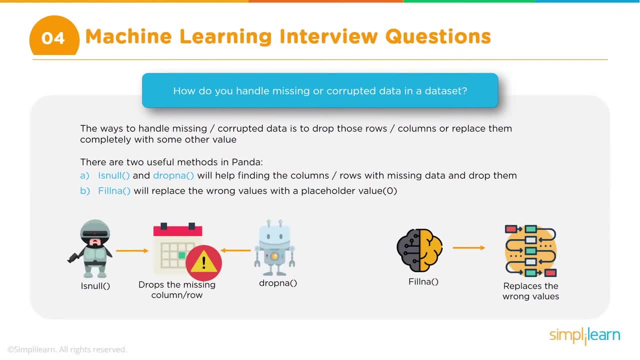 minimum value, or with a zero. so or with the maximum value. again, as i said, there are so many possibilities, so there is no like one correct answer for this. you need to basically talk around this and illustrate with your experience. as i said, that would be the best. otherwise, this is how you need. 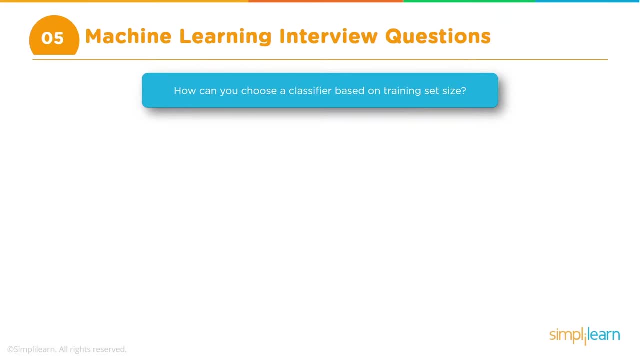 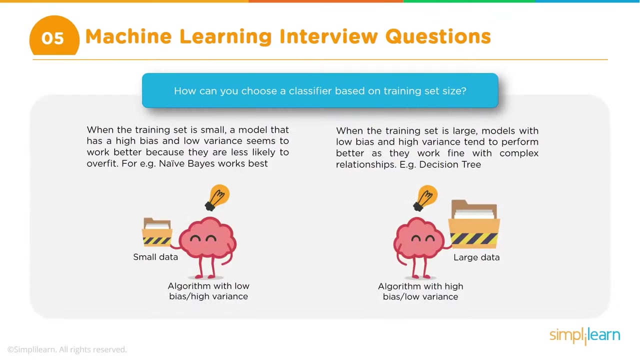 to handle this question. okay. so then the next question can be: how can you choose a classifier based on a training set data size? so, again, this is one of those questions where you probably do not have like a one size fits all answer. first of all, you may not, let's say, decide your. 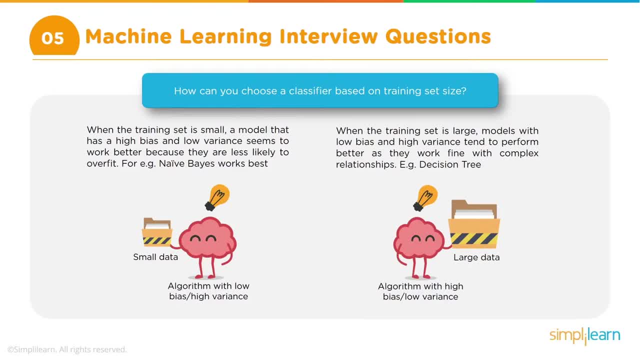 classifier based on the training set size. maybe not the best way to decide the type of the classifier and even if you have to, there are probably some thumb rules which we can use, but then again every time. so, in my opinion, the best way to respond to this. 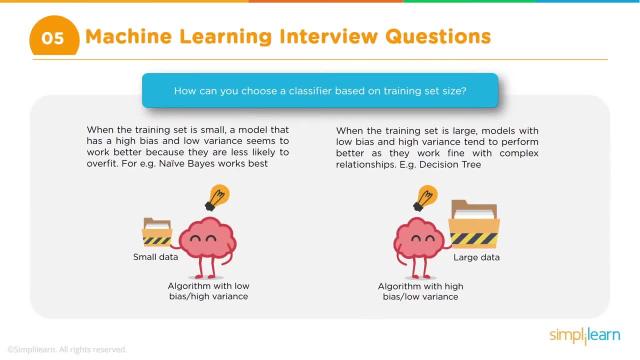 question is: you need to try out few classifiers, irrespective of the size of the data, and you need to then decide, on your particular situation, which of these classifiers are the right ones. this is a very generic issue, so you will never be able to just by if somebody defines a problem to you and 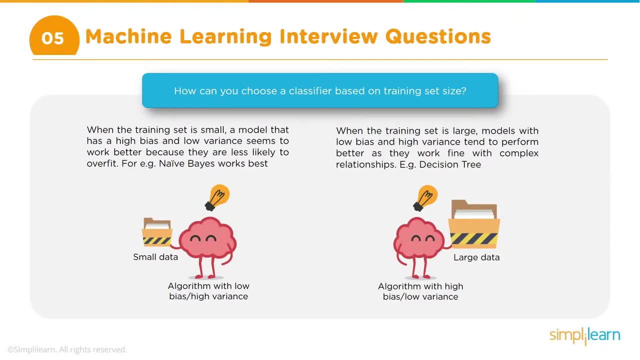 somebody, even if you, if they show the data to you or tell you what is the data or even the size of the data. i don't think there is a way to really say that, yes, this is the classifier that will work here. no, that's not the right way, so you need. 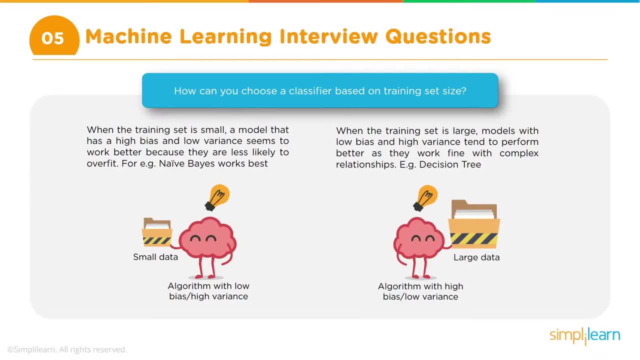 to still. you know, test it out, get the data, try out a couple of classifiers, and then only you will be in a position to decide which classifier to use. you try out multiple classifiers, see which one gives the best accuracy, and only then you can decide. then you 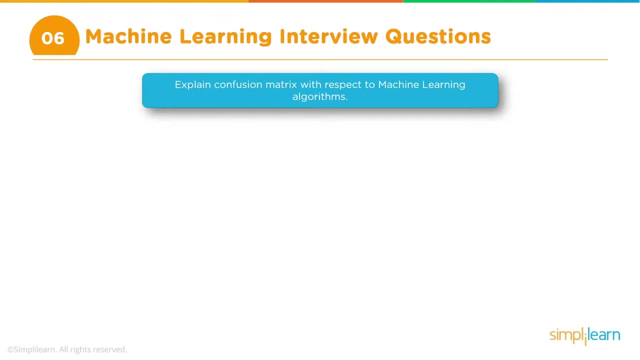 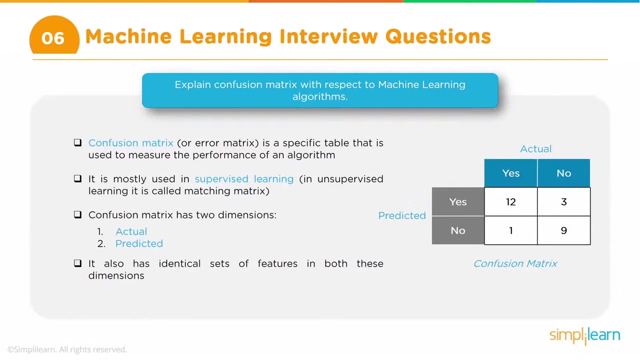 can have a question around confusion matrix, so the question can be explained: confusion matrix, right, so confusion matrix? i think the best way to explain it is by taking an example and drawing like a small diagram. otherwise it can really become tricky. so my suggestion is to take a 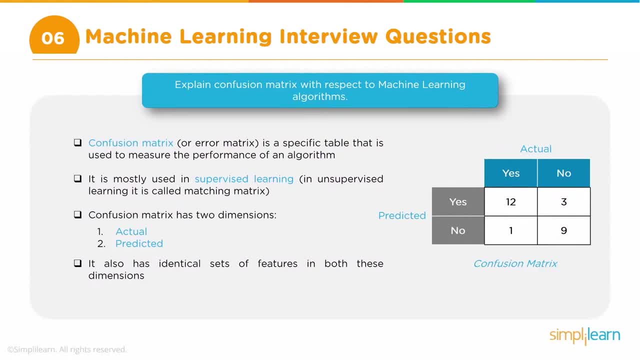 piece of pen and paper and explain it by drawing a small matrix and confusion. matrix is about to find out. this is used especially in classification, uh learning process, and when you get the results, when the our model predicts the results, you compare it with the actual value and try to find out what is the accuracy. 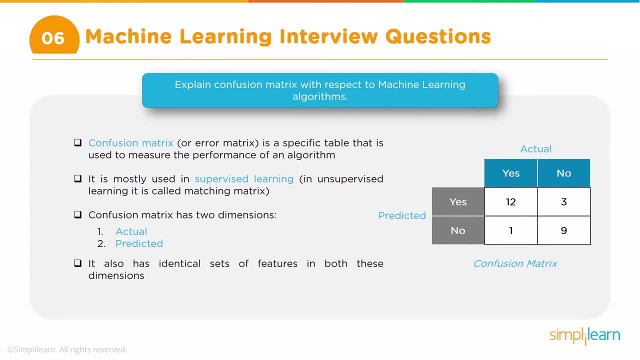 okay. so in this case, let's say this is an example of a confusion matrix and it is a binary matrix, so you have the actual values, which is the labeled data right and which is so you have how many yes and how many no. so you have that information. 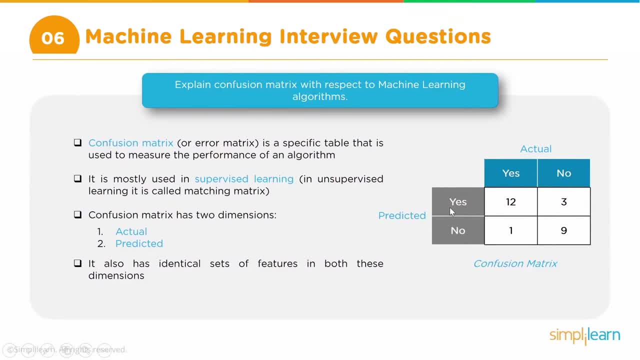 and you have the predicted values. okay, how many yes and how many no? right? so the total actual values: the total yes is 12 plus 1- 13, and they are shown here, and the actual value no's are 9 plus 3- 12. okay, so that is. 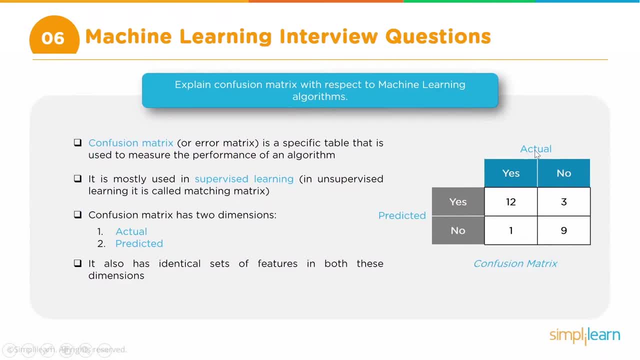 what this information here is. so this is about the actual and this is about the predicted. similarly, the predicted values there are: yes are 12 plus 3- 15 yeses and no are 1 plus 9 10 no's. okay, so this is the way to. 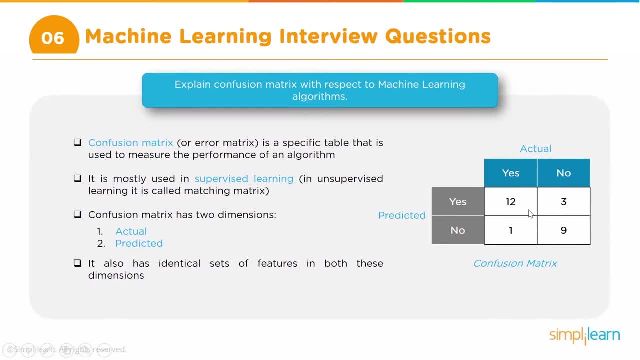 look at this confusion matrix, okay, and out of this, what is the meaning conveyed? so there are two or three things that needs to be explained outright. the first thing is: for a model to be accurate, the values across the diagonal should be high, like in this case. right, that is one. 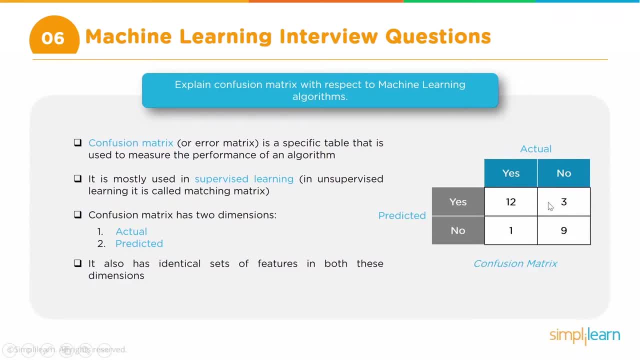 number two. the total sum of these values is equal to the total observations in the test data set. so in this case, for example, you have 12 plus 3, 15 plus 10, 25, so that means we have 25 observations in our test data. 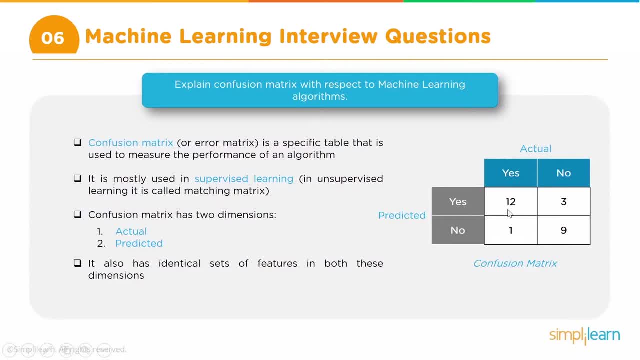 set. okay, so these are the two things. you need to first explain that the total sum in this matrix, the numbers, is equal to the size of the test data set and the diagonal values indicate the accuracy. so by just by looking at it, you can probably have an idea about. is this: 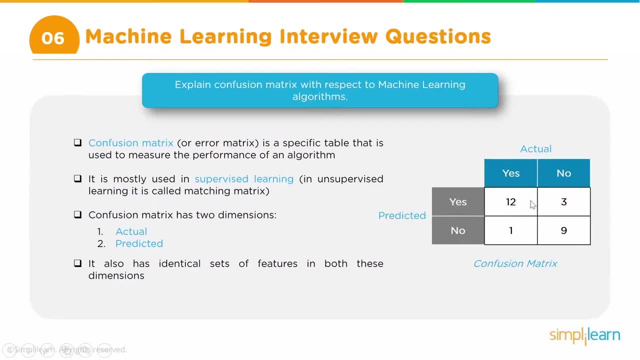 an accurate model? is the model being accurate if they're all spread out equally in all these four boxes? that means probably the accuracy is not very good. okay now, how do you calculate the accuracy itself? right? how do you calculate the accuracy itself? so it is a very simple. 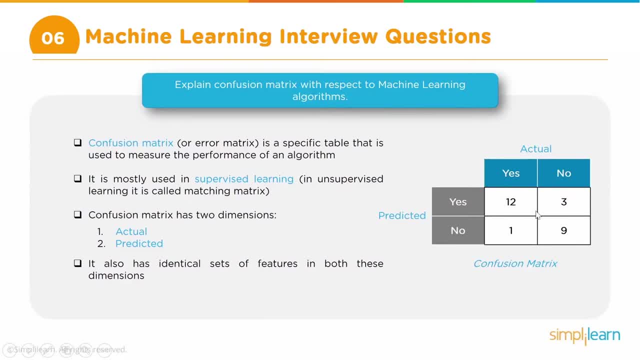 mathematical calculation. you take some of the diagonals right, so in this case it is 9 plus 12, 21, and divide it by the total. so in this case, what will it be? let's me take a pen. so your, your diagonal values is equal to. if i say d is equal. 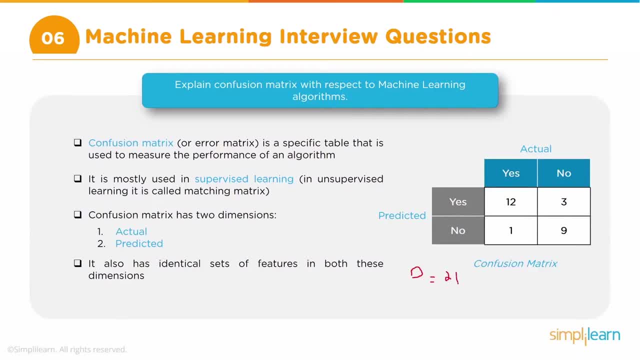 to 12 plus 9, so that is 21, right, and the total data set is equal to right. we just calculated it is 25.. so what is your accuracy? it is 21 by your accuracy is equal to 21 by 25, and this turns out to be: 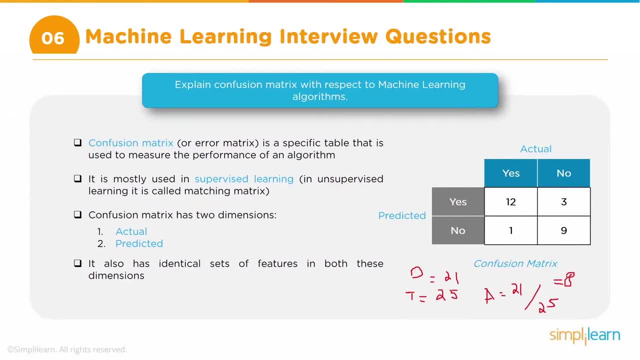 about 85 percent, right? so this is 85 percent. so that is our accuracy. okay, so this is the way you need to explain. draw diagram. give an example. maybe it may be a good idea to be prepared with an example so that it becomes easy for you. you. 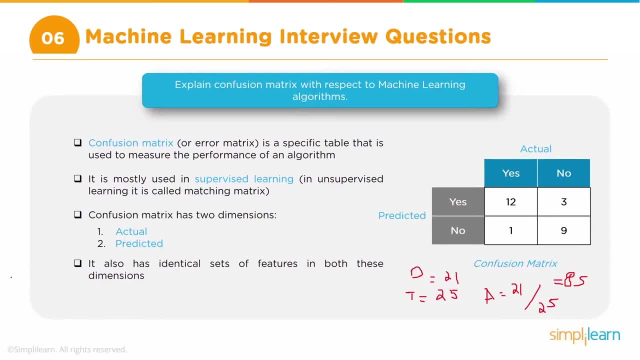 don't have to calculate these numbers on the fly, right? so a couple of uh hints are that you take some numbers which are with, which add up to 100. that is always a good idea, so you don't have to really do this complex calculations. so the total value will be: 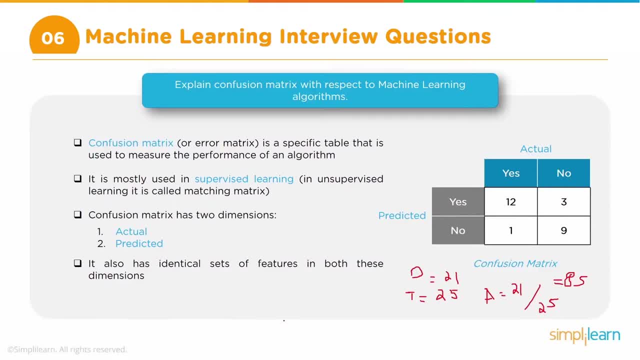 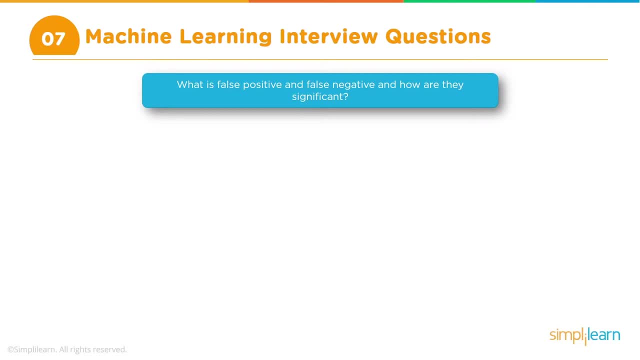 100 and then diagonal values. you divide. once you find the diagonal values, that is equal to your percentage. okay, all right. so the next question can be a related question about false positive and false negative. so what is false positive and what is false negative? now, once again, the best way to explain this. 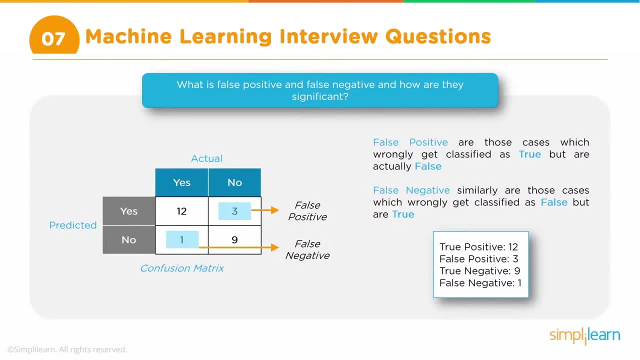 is using a piece of paper and pen, otherwise it will be pretty difficult to explain this. so we use the same example of the confusion matrix and we can explain that. so a confusion matrix looks somewhat like this, and when we just, yeah, it looks somewhat like this, and we continue with the previous. 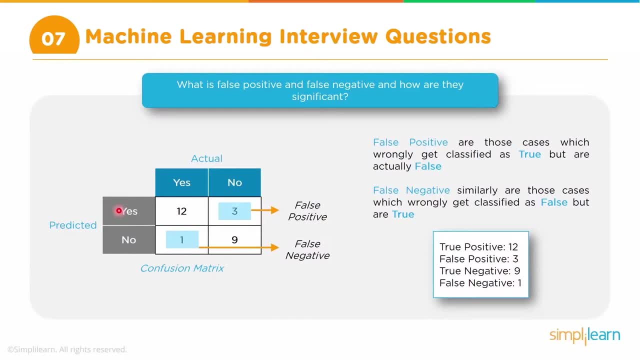 example, where this is the actual value, this is the predicted value and in the actual value we have 12 plus 1: 13 yeses and 3 plus 9: 12 no's, and the predicted values there are 12 plus 3: 15 yeses. 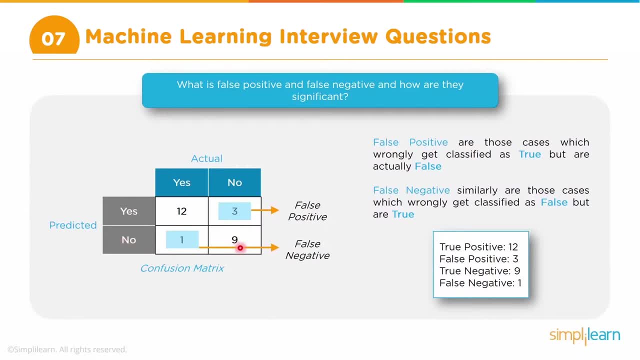 and 1 plus 9, 10, no's okay. now this particular case, which is the false positive. what is a false positive? first of all, the second word which is positive, okay, is referring to the predicted value. so that means the system has predicted it as a positive, but the 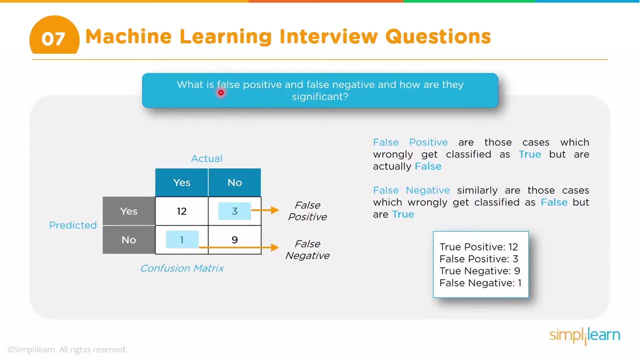 real value. so this is what the false comes from, but the real value is not positive. okay, that is the way you should understand this term: false positive or even false negative. so false positive, so positive is what your system has predicted. so where is that system predicted? this is the one positive is. 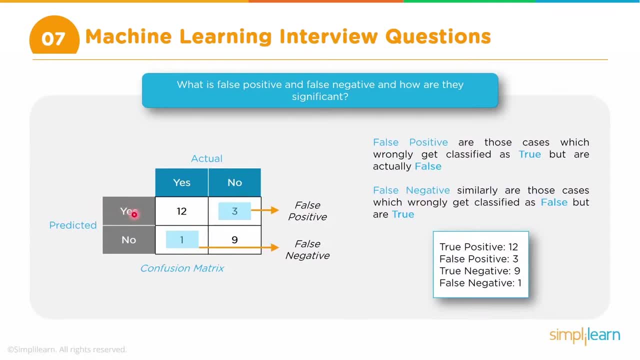 what? yes, so you basically consider this row. okay. now, if you consider this row, so this is, this is all positive values, this entire row is positive values. okay now, the false positive is the one which where the value- actual value is negative, predicted value is positive, but the 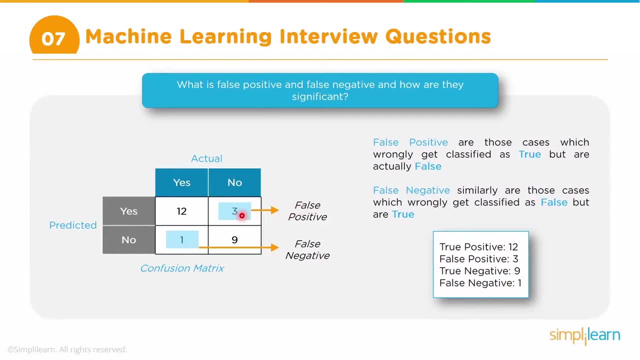 actual value is negative. so this is a false positive, right, and here is a true positive. so the predicted value is positive and the actual value is also positive. okay, i hope this is making sense. now let's take a look at what is false negative, false negative, so negative. 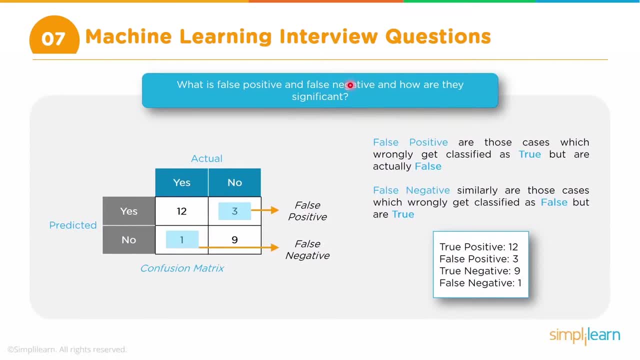 is the second term. that means that is the predicted value that we need to look for. so which are the predicted negative values? this row corresponds to predicted negative values. all right, so this row corresponds to predicted negative values. so this number, it think this is the row for. so for predicted negative values. 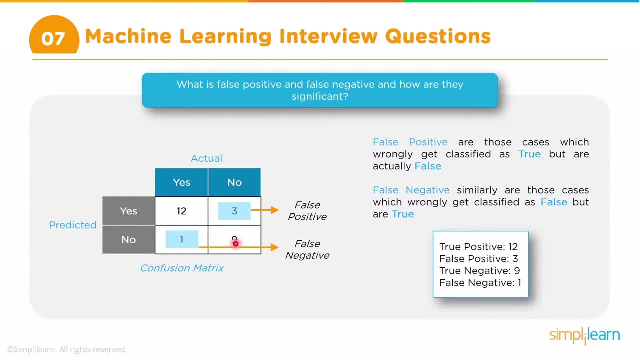 so yours, and this is the first row, right, so the first row. so the fø punto of, say, f is negative. the right row, this is the row for predicted negative values and what they are asking for false. so this is the row for predicted negative values and this one. 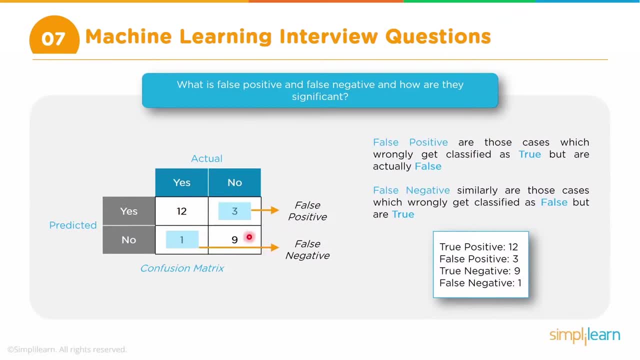 and false negative. Same way there can be true positive and true negative as well. So, again, positive, the second term you will need to use to identify the predicted row right. So if we say true, positive, positive we need to take for the predicted part. So predicted positive is here. 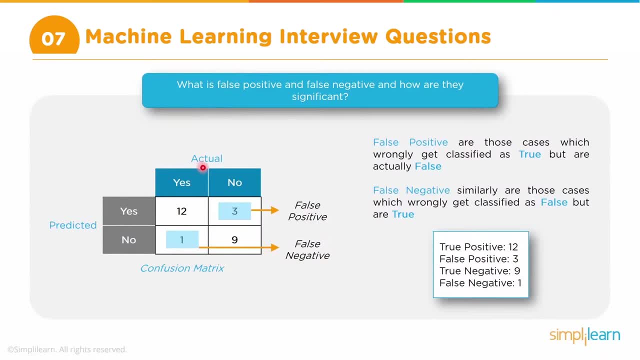 okay. and then the first term is for the actual, So true, positive. so true, in case of actual is yes, right. So true, positive, is this one okay. and then, in case of actual, the negative. Now we are talking about, let's say true, negative, true, negative, Negative is this one and the true comes from here. 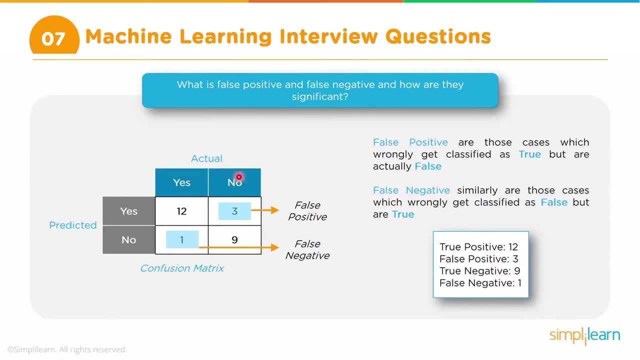 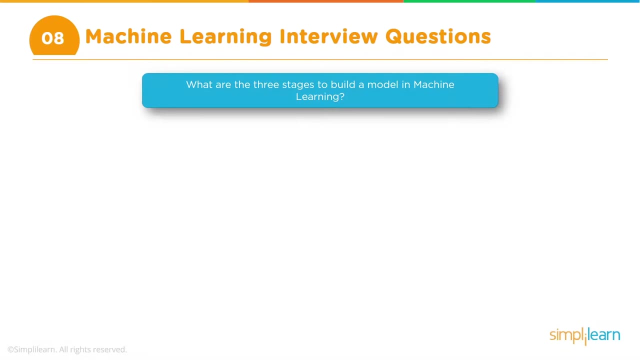 So this is true, negative. right, 9 is true negative. The actual value is also negative and the predicted value is also negative. okay, So that is the way you need to explain this: the terms false positive, false negative and true positive, true negative. Then you might have a question like: what are the? 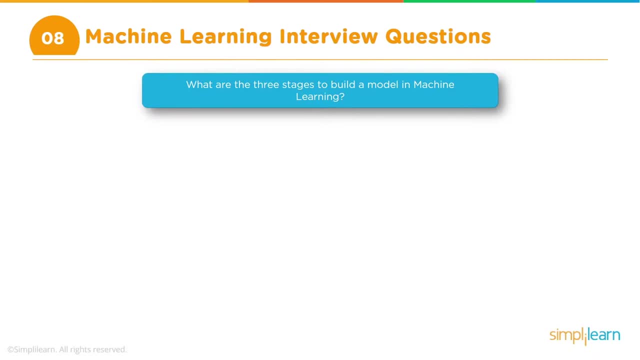 steps involved in the machine learning process, or what are the three steps in the process of developing a machine learning model? right, So it is around the methodology that is applied. So basically, the way you can probably answer in your own words, but the way the model development of the 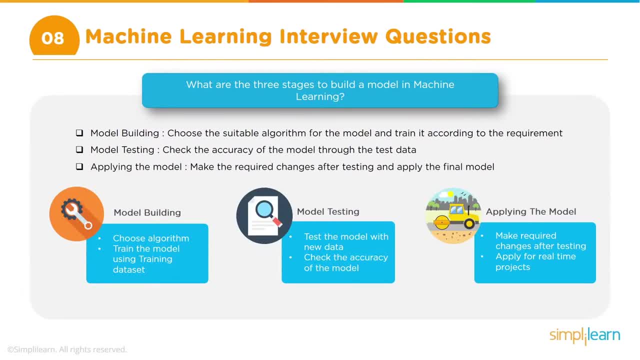 machine learning model happens is like this. So first of all you try to understand the problem and try to figure out whether it is a classification problem or a regression problem. Based on that, you select a few algorithms and then you start the process of training these models. okay, So you can. 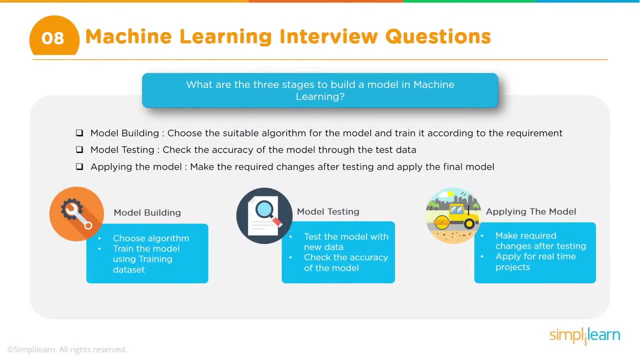 either do that or you can. after due diligence, you can probably decide that there is one particular algorithm which is most suitable. Usually it happens through trial and error process, but at some point you will decide that, okay, this is the model we are going to use. okay, So in that case, 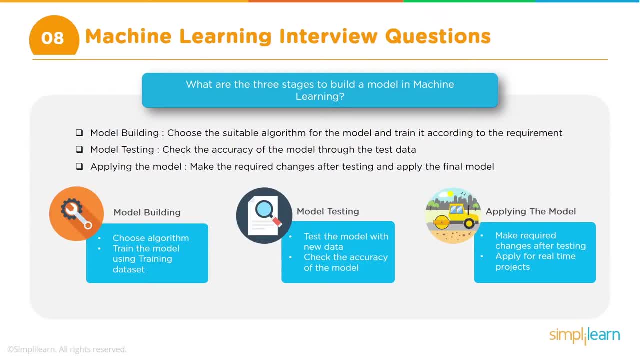 we have the model algorithm and the model decided and then you need to do the process of training these models. okay, So you can either do that or you can, after due diligence, you can start the process of training the model and testing the model. and this is where, if it is, 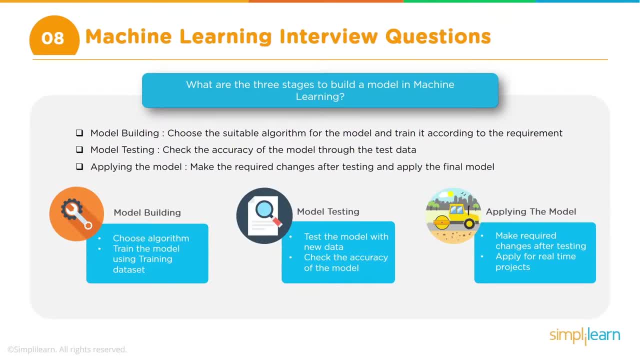 supervised learning. you split your data, the label data, into training data set and test data set, and you use the training data set to train your model. and then you use the test data set to check the accuracy, whether it is working fine or not. So you test the model before you actually put it into. 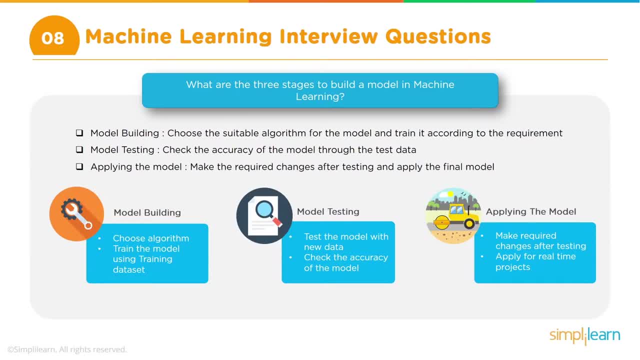 production right. So once you test the model, you're satisfied it's working fine. then you go to the next level, which is putting it for training the model, and then you use the test data set to check the accuracy, whether it is working fine or not. So you test the model before you actually put it into. 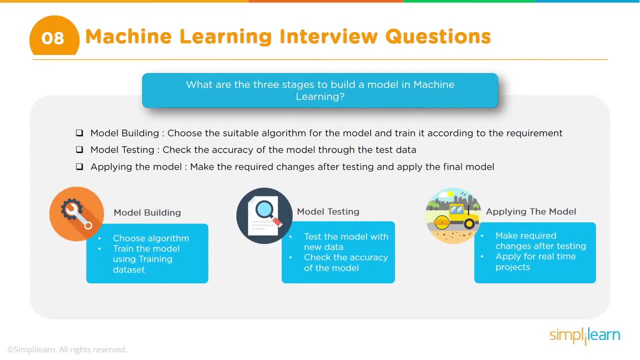 production and then in production, obviously new data will come and the inference happens. So the model is readily available and only thing that happens is new data comes and the model predicts the values, whether it is regression or classification Now. so this can be an iterative process. so it is. 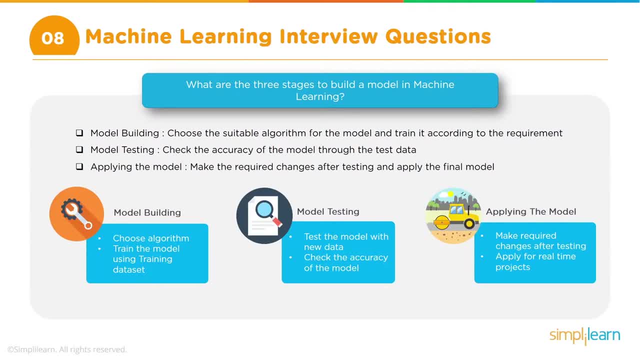 not a straightforward process where you do the training through the testing and then you move it to production Now. so during the training and test process, there may be a situation where, because of either overfitting or things like that, the test doesn't go through. 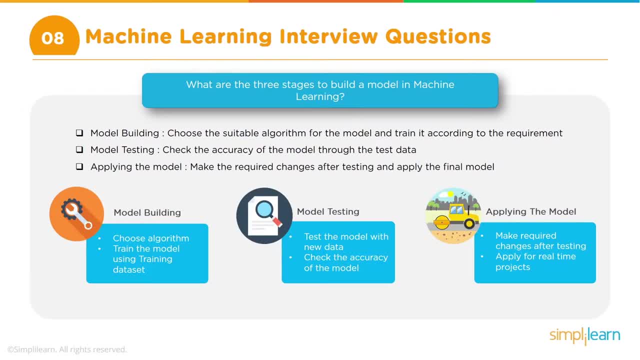 Which means that you need to put that back into the training process, So that can be an iterative process. not only that: even if the training and test goes through properly and you deploy the model in production, there can be a situation that the data that actually comes, the real data that 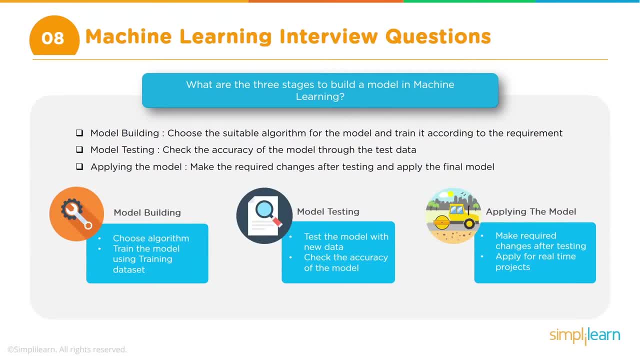 comes with that this model is failing, So in which case you may have to once again go back to the drawing board, or initially it will be working fine, but over a period of time, maybe due to the change in the nature of the data- once again the accuracy will deteriorate. 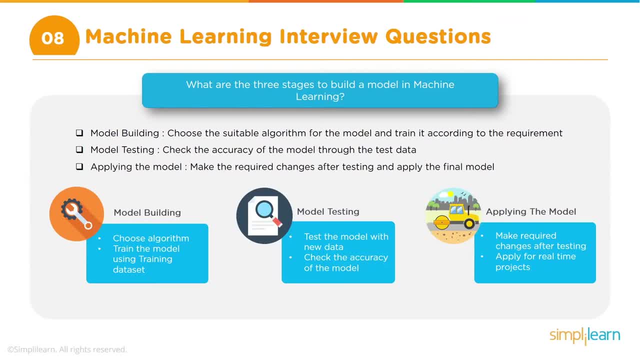 So that is again a recursive process. so once in a while you need to keep checking whether the model is working fine or not and, if required, you need to tweak it and modify it, and so on and so forth. So net, net. this is a continuous process of tweaking the model and testing it and making sure it is up. 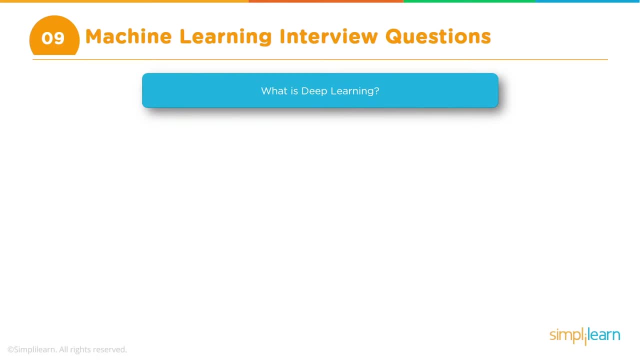 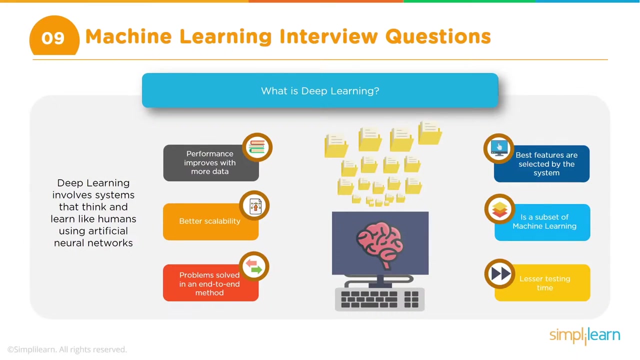 to date. Then you might have question around deep learning. so because deep learning is now associated with AI, artificial intelligence and so on, so can be as simple as what is deep learning? So I think the best way to respond to this could be: deep learning is a part of machine learning and then 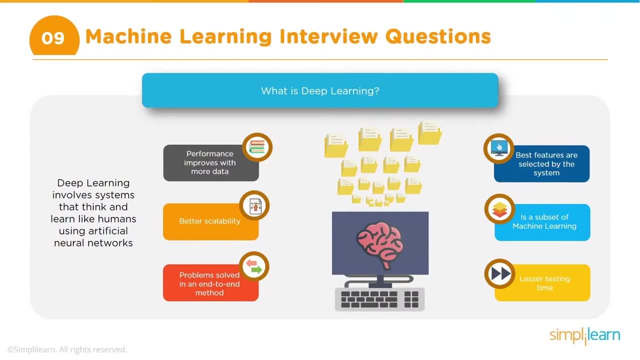 then obviously the question would be: then what is the difference, right? So deep learning, you need to mention there are two key parts that interviewer will be looking for when you are defining deep learning. So first is, of course, deep learning is a subset of machine learning. So machine learning, 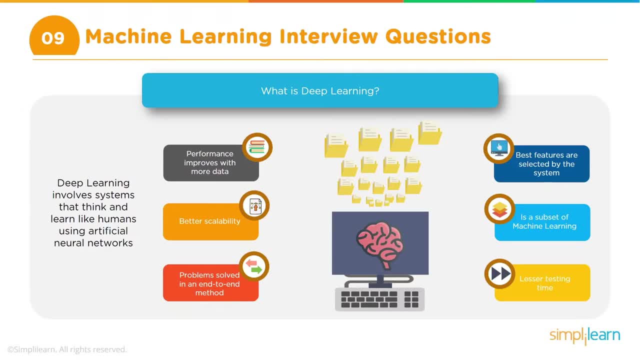 is still the bigger, let's say, scope, and deep learning is one part of it. So then, what exactly is the difference? Deep learning is primarily when we are implementing these, our algorithms, or when we are using neural networks for doing our training and classification and regression and all that right. So when we use neural network, then it. 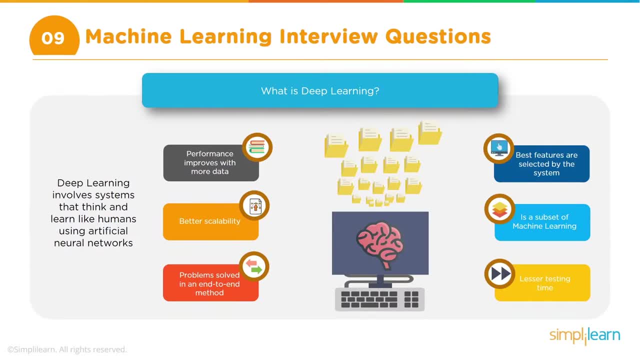 is considered as deep learning and the term deep comes from the fact that you can have several layers of neural networks and these are called deep neural networks and therefore the term deep. you know, deep learning. The other difference between machine learning and deep learning, which the interviewer may be wanting to hear, is that, in case of machine 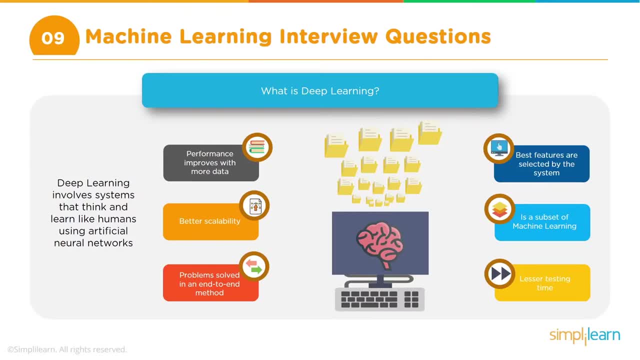 learning, the feature engineering is done manually. What do we mean by feature engineering? Basically, when we are trying to train our model, we have our training data right. So we have our training label data and this data has several and, let's say, if it is a regular table, it has several columns. 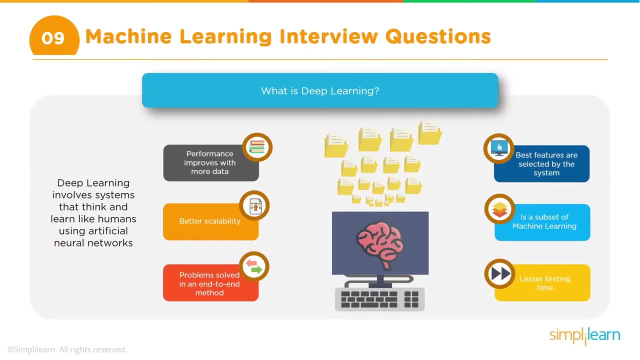 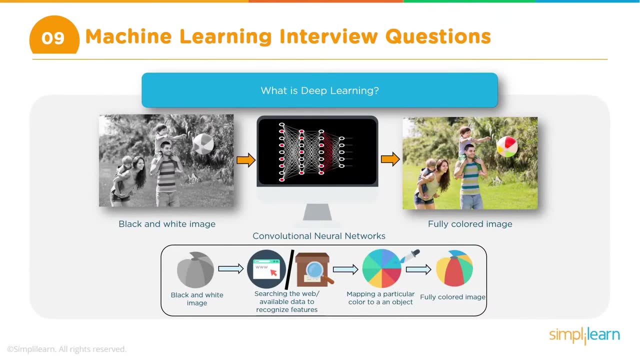 Now each of these columns actually has information about a feature, right? So we are trying to predict the height, weight and so on and so forth. So these are all features of human beings. let's say we have census data and we have all. So those are the features Now there. 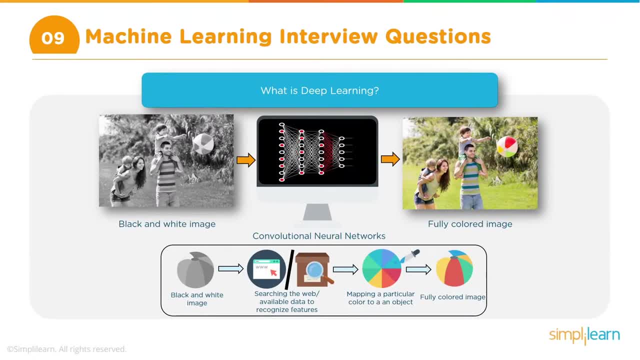 may be probably 50 or 100. in some cases there may be 100 such features. Now all of them do not contribute to our model, right? So we, as a data scientist, we have to decide whether we should take all of them, all the features, or we should throw away some of them. because, again, if we take 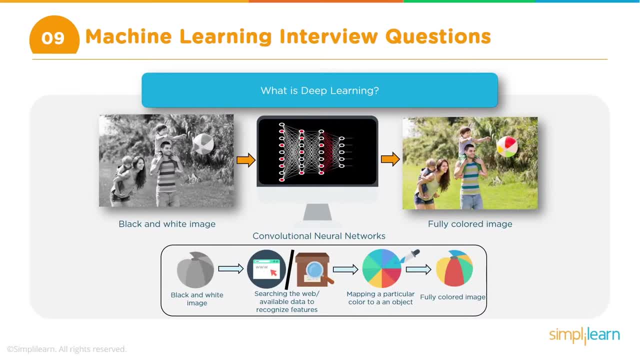 all of them number one. of course accuracy will probably get affected, but also there is a computational part. So if you have so many features and then we have so much data, it becomes very tricky. So in case of machine learning, we manually take care of identifying the features that do not contribute to the learning process. 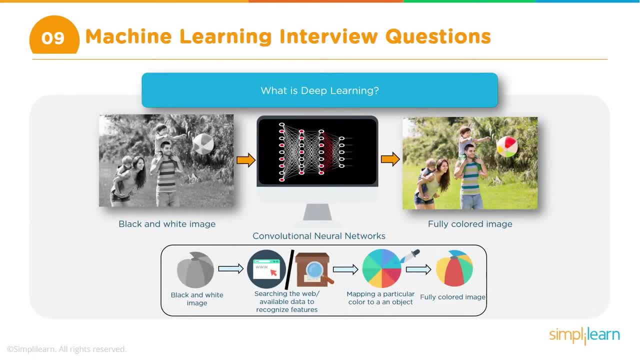 and thereby we eliminate those features and so on. right, So this is known as feature engineering, and in machine learning we do that manually, Whereas in deep learning, where we use neural networks, the model will automatically determine which features to use and which to not use, and therefore feature engineering. 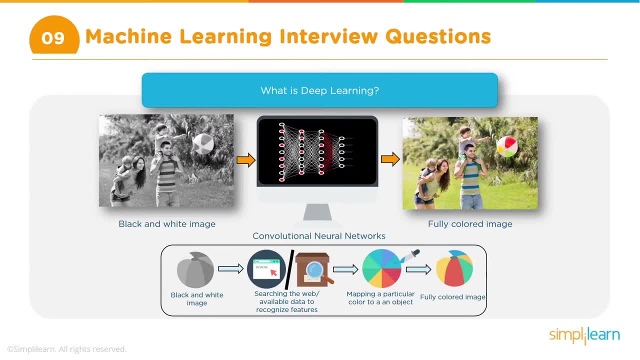 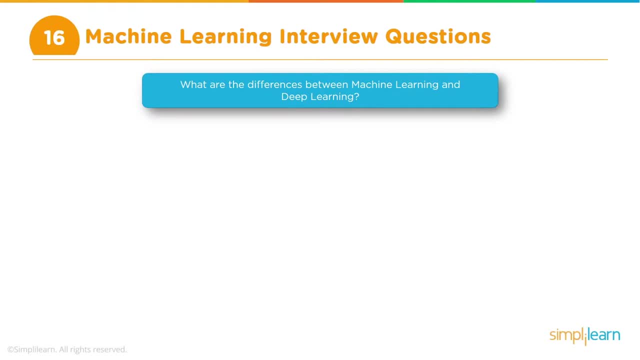 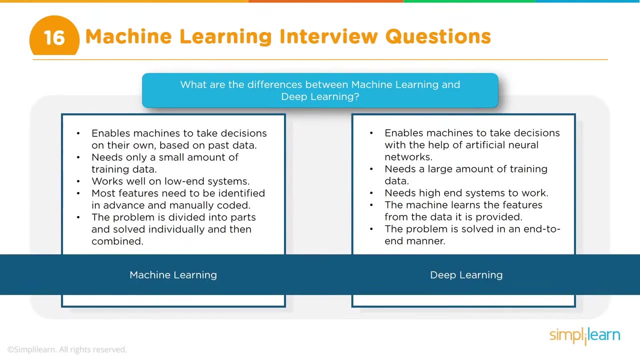 is also done automatically. So this is a explanation. these are two key things probably will add value to your response. All right, so the next question is: what is the difference between, or what are the differences between, machine learning and deep learning? So here this is a quick comparison. 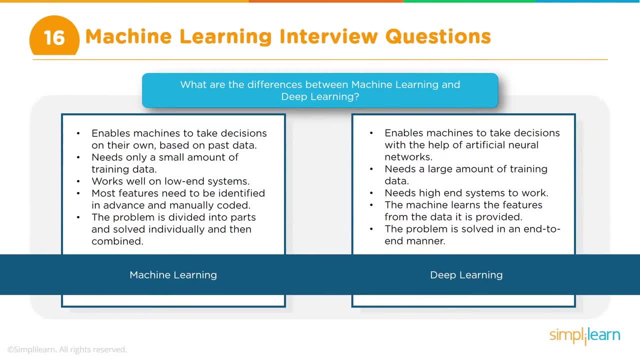 table between machine learning and deep learning, and in machine learning enables machines to take decisions on their own based on past data. So here we are talking primarily of supervised learning, and it needs only a small amount of data for training and then works well on low-end systems. 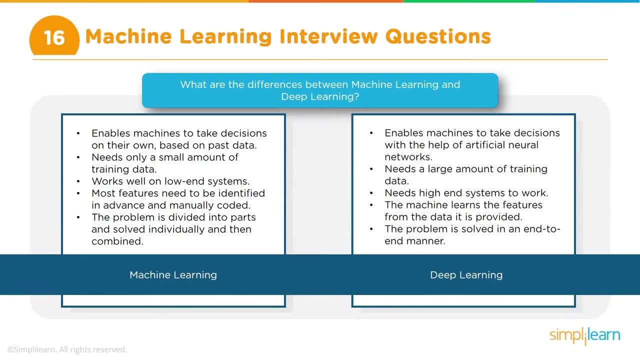 so you don't need large machines and most features need to be identified in advance and manually coded. So basically the feature engineering part is done manually and the problem is divided into parts and solved individually and then combined. So that is about the machine learning part In deep. 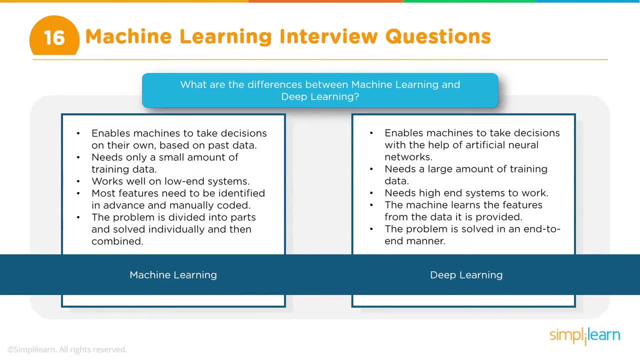 learning, deep learning- It basically enables machines to take decisions with the help of artificial neural networks. So here in deep learning we use neural networks. So that is the key differentiator between machine learning and deep learning. and usually deep learning involves a large amount of data and 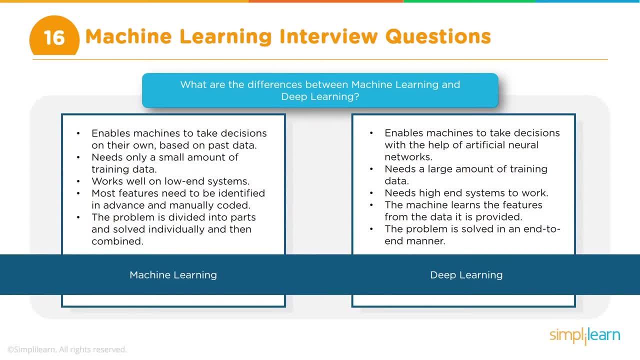 therefore the training also requires. usually the training process requires high-end machines because it needs a lot of computing power and the machine learning features are the or the feature engineering is done automatically, So the neural networks takes care of doing the feature engineering as well, and in case of deep learning, therefore, it is said that the problem is handled. 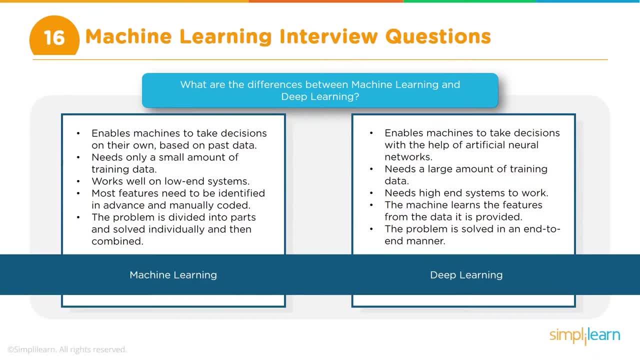 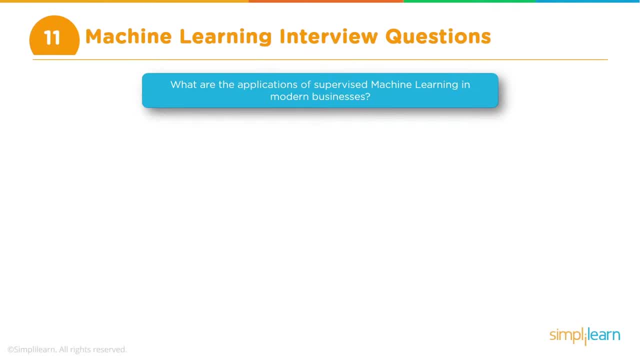 end-to-end. So this is a quick comparison between machine learning and deep learning. in case you have that kind of a question, Then you might get a question around the uses of machine learning or some real-life applications of machine learning in modern business. The question may be worded. 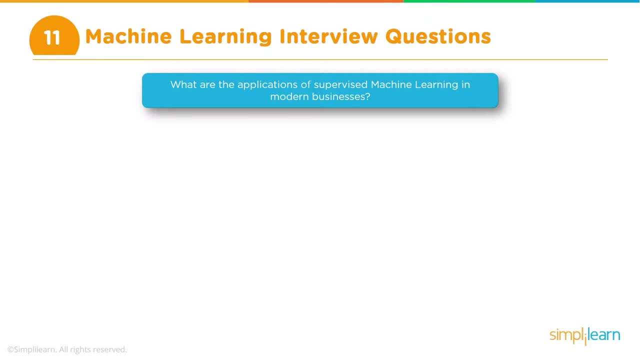 in different ways, but the meaning is: how exactly is machine learning used, or actually supervised machine learning? It could be a very specific question around supervised machine learning. So this is like give examples of supervised machine learning, use of supervised machine learning in modern business. So that could be the next question. So there are quite a few examples. 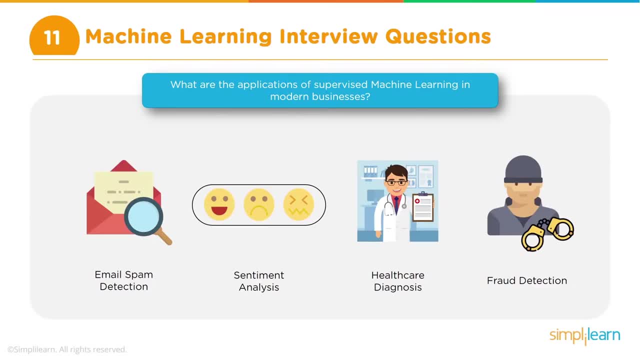 or quite a few use cases, if you will, for supervised machine learning. The very common one is email spam detection, So you want to train your application or your system to detect between spam and non-spam. So this is a very common business application of supervised machine learning. So how does this work? 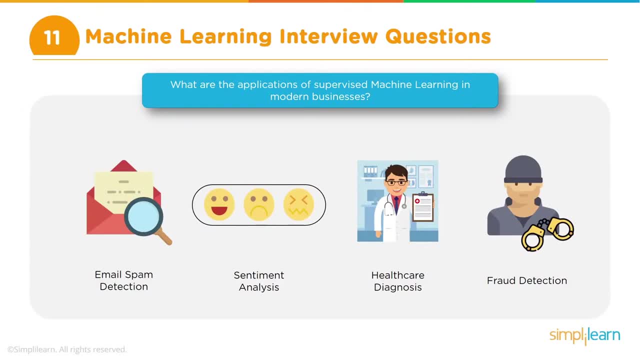 The way it works is that you obviously have historical data of all of your emails and they are categorized as spam and not spam, So that is what is the labeled information, and then you feed this information or all these emails as an input to your model- right, and the model will then get. 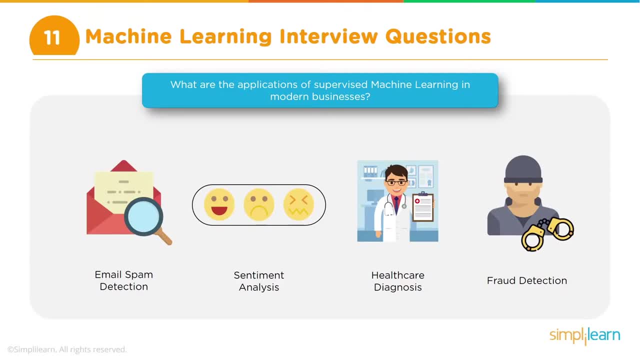 trained to detect which of the emails are, to detect which is spam and which is not spam. So that is the training process and this is supervised machine learning, because you have labeled data, You already have emails which are tagged as spam or not spam and then you use that to train your model right. So this is one. 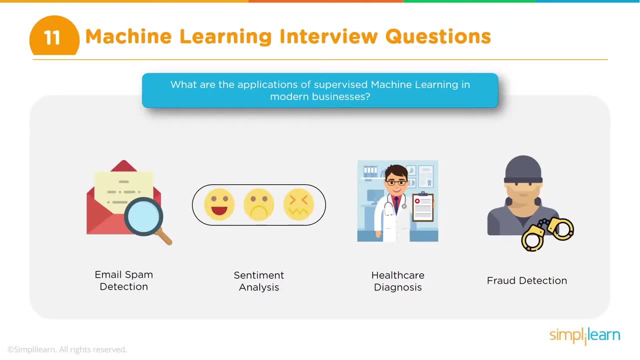 example. Now there are a few industry specific applications for supervised machine learning. One of the very common ones is in healthcare diagnostics. In healthcare diagnostics you have this: two images- and you want to train models to detect whether from a particular image, whether it can find out if the person is sick or not, whether a person has cancer or not, right? So this is a very 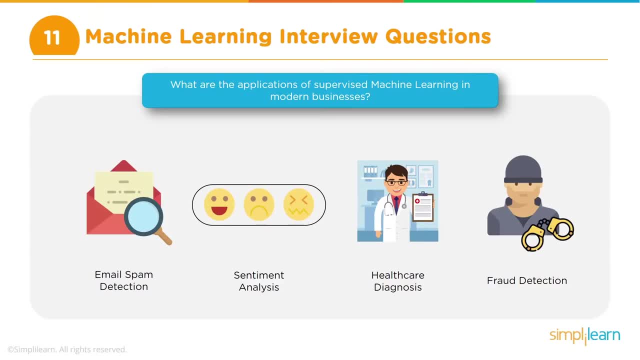 good example of supervised machine learning. Here the way it works is that existing images- it could be x-ray images, it could be MRI or any of these images- are available and they are tagged saying that, okay, this x-ray image is defective of the person. 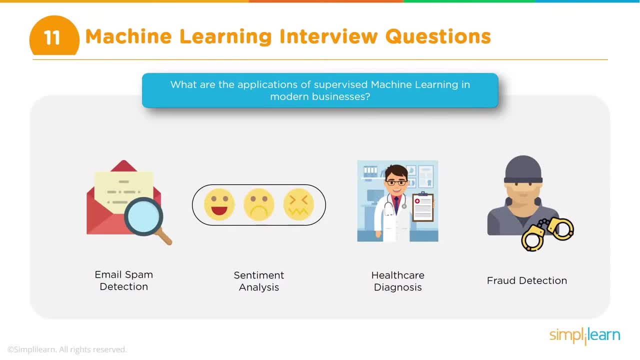 Guardianship of other humans, an illness, or it could be cancer, which have an illness right. So it is tagged as defective or clear or good image and defective image, something like that. so we come up with the binary- or it could be multi class as well- saying that this. 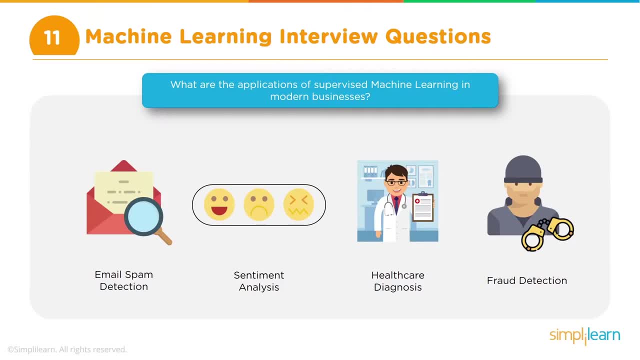 is defective to 10%, this is 25% and so on. But let's keep it simple. you can give an example of just a binary classification. that would be good enough. So you can say that in healthcare diagnostics. You can day that in healthcare diagnostics, using image, we need to detect whether a person is ill or whether a person is sick. 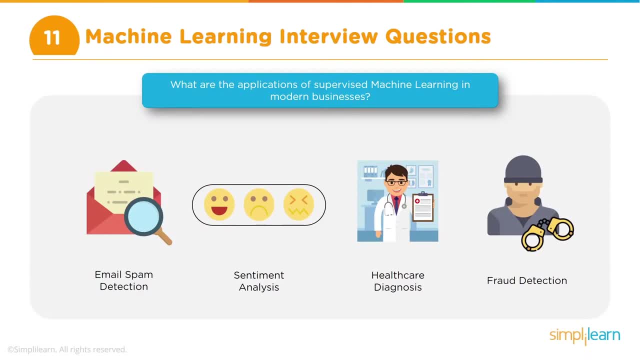 or if one is ill, whether a person is ill this one. so, saying that this is the simple, this is what I recommend, whether a person is having cancer or not. so here, the way it works is you feed labeled images and you allow the model to learn from that so that when new image is fed, it will be able to predict. 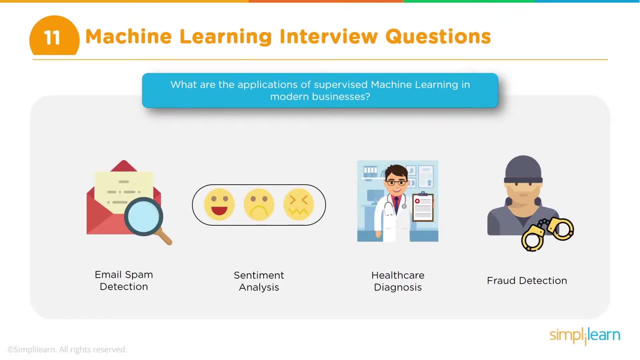 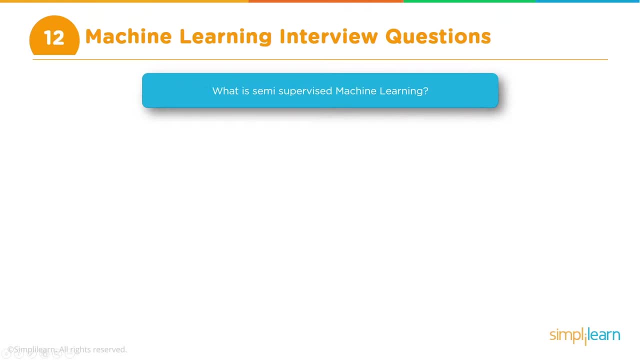 whether this person is having that illness or not, having cancer or not, right? so i think this would be a very good example for supervised machine learning in modern business. all right, then we can have a question like: so we've been talking about supervised and unsupervised, and so there 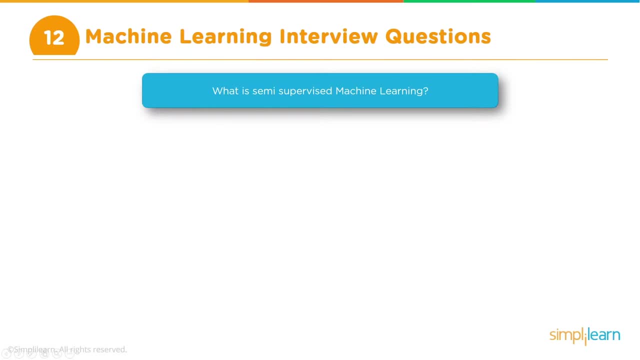 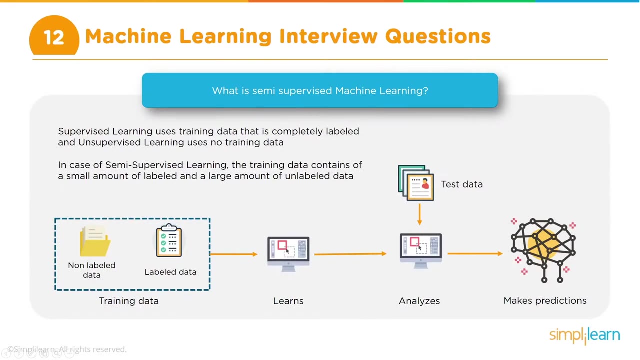 can be a question around semi-supervised machine learning. so what is semi-supervised machine learning now? semi-supervised learning, as the name suggests, it falls between supervised learning and unsupervised learning, but for all practical purposes it is considered as a part of supervised learning, and the reason this has come into existence is that. 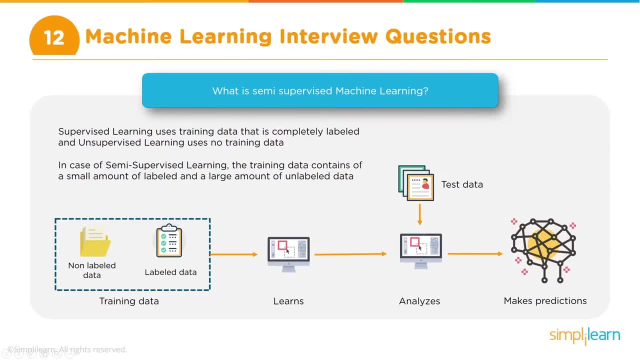 you can have a question like: so we've been talking about supervised and unsupervised. in supervised learning, you need labeled data. so all your data for training, your model, has to be labeled. now this is a big problem in many industries or in many under many situations. 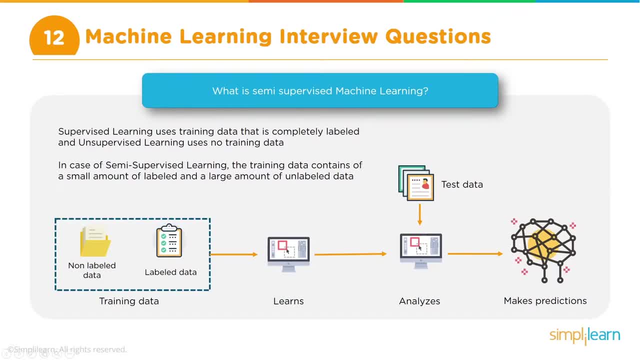 getting the labeled data is not that easy because there's a lot of effort in labeling this data. let's take an example of diagnostic images. we can just, let's say, take x-ray images. now there are actually millions of x-ray images available all over the world, but the 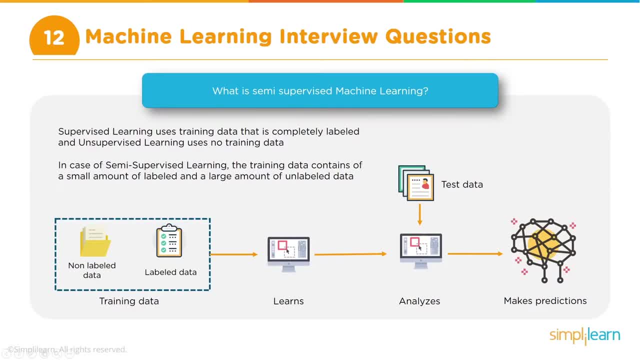 problem is they are not labeled, so their images are there, but whether it is defective or whether it is good that information is not available along with it, right in a form that it can be used by a machine, which means that somebody has to take a look at these images, and usually it should be like: 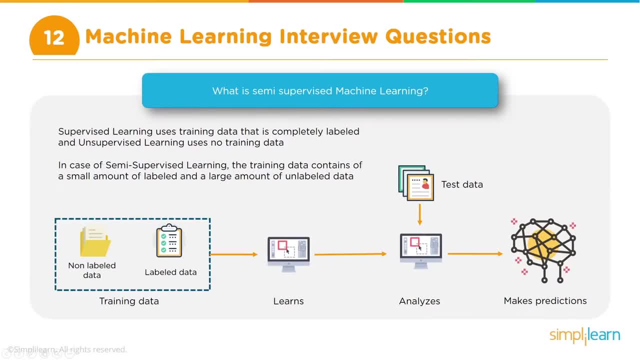 a doctor and then say that okay, yes, this image is clean and this image is cancerous, and so on, and so now that is a huge effort by itself. so this is where semi-supervised learning comes into play. so what happens is there is a large amount of data, maybe a part. 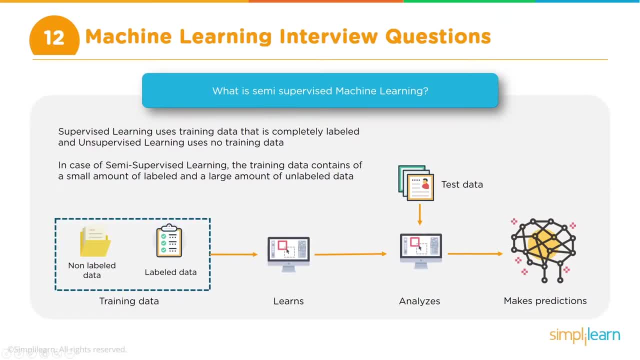 of it is labeled, then we try some techniques to label the remaining part of the data so that we get completely labeled data and then we train our model. so i know this is a little long winding explanation, but unfortunately there is no quick and easy definition for semi-supervised machine. 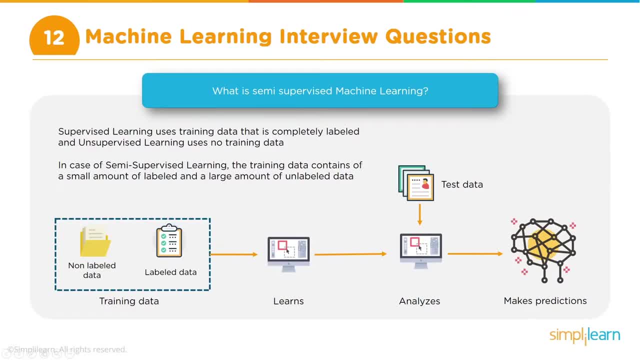 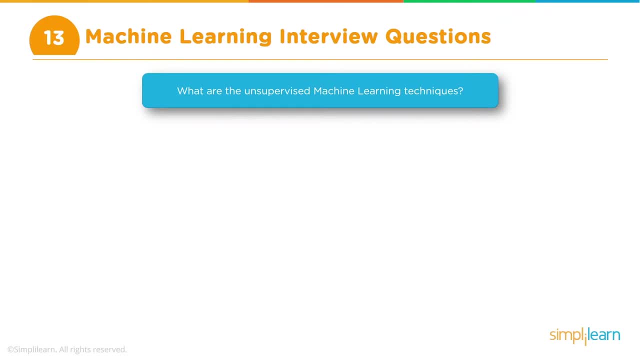 learning. this is the only way, probably, to explain this concept. we may have another question, as: what are unsupervised machine learning techniques, or what are some of the techniques used for performing unsupervised machine learning? so it can be worded in different ways. so how do we answer this question? so, unsupervised learning, you can say that there are two types. 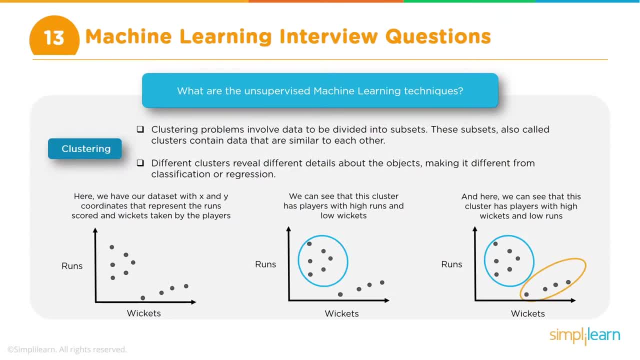 clustering and association. and clustering is a technique where similar objects are put together. there are different ways of finding similar objects, so their characteristics can be measured and if they have, in most of the characteristics, if they are similar, then they can be put together. this is clustering, then. 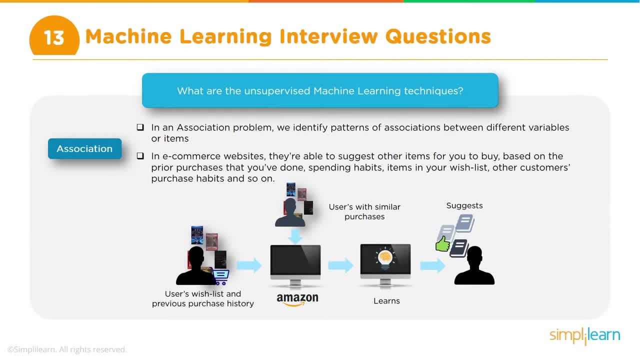 association you can. i think the best way to explain association is with an example. in case of association, you try to find out how the items are linked to each other. so, for example, if somebody bought, maybe, a laptop, the person has also purchased a mouse. So this is more in an e-commerce scenario, for example. 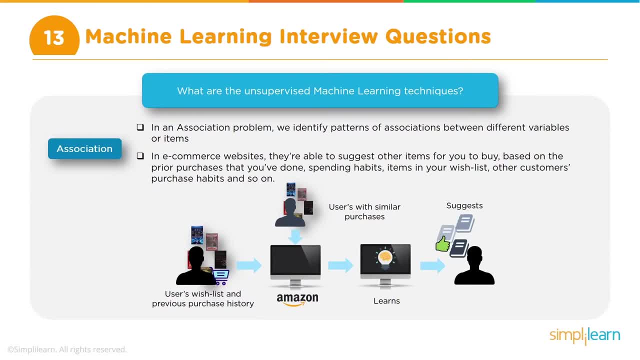 So you can give this as an example. So people who are buying laptops are also buying a mouse, So that means there is an association between laptops and mouse. or maybe people who are buying bread are also buying butter, So that is a association that can be created. 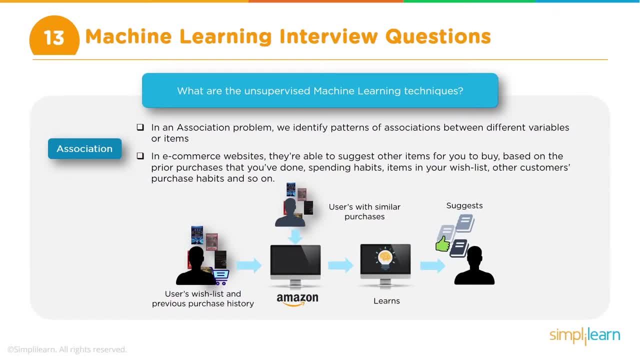 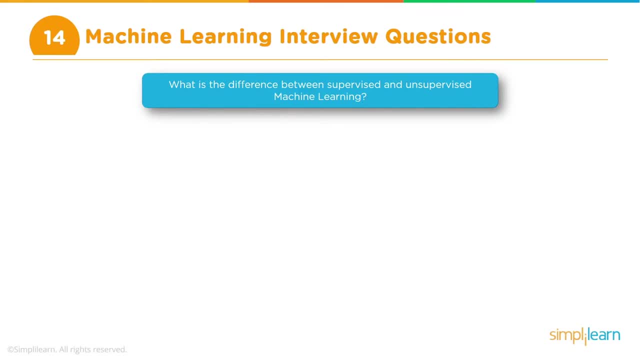 So this is unsupervised learning, one of the techniques. Okay, All right, Then we have a fundamental question Then: what is the difference between supervised and unsupervised machine learning? So machine learning, these are the two main types of machine learning: supervised and. 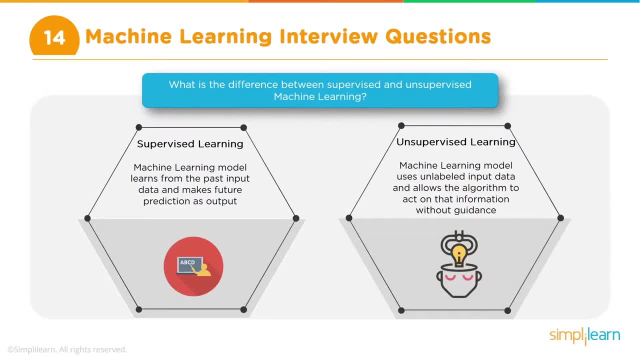 unsupervised. And in case of supervised- and again here, probably the keyword that the person may be wanting to hear is labeled data. Very often people say, yeah, we have historical data and if we run it, it is supervised. And if we don't have historical data, yes, but you may have historical data, but if it, 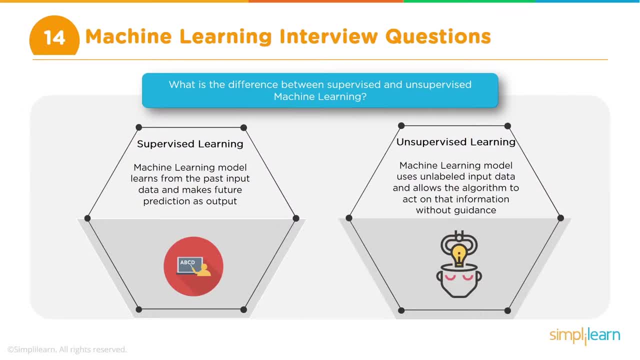 is not labeled, then you cannot use it for supervised learning. So it is. it's very key to understand that we put in that keyword labeled Okay. So when we have labeled data for training, our model, then we can use supervised learning. 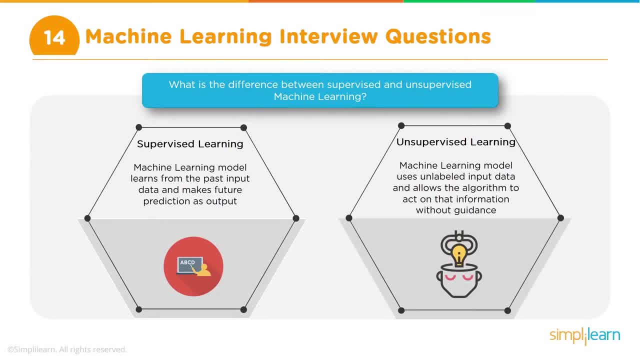 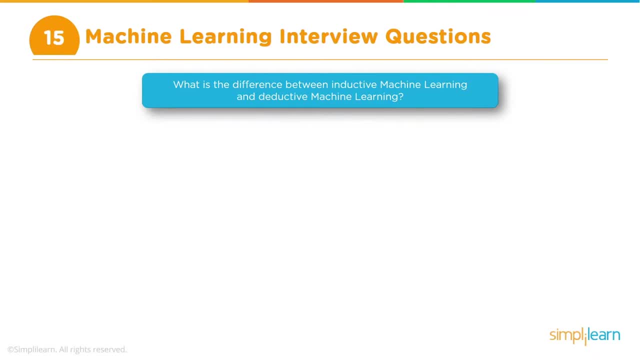 And if we do not have labeled data, then we use unsupervised learning And there are different algorithms available to perform both of these types of trainings. So there can be another question a little bit more theoretical and conceptual in nature. This is a 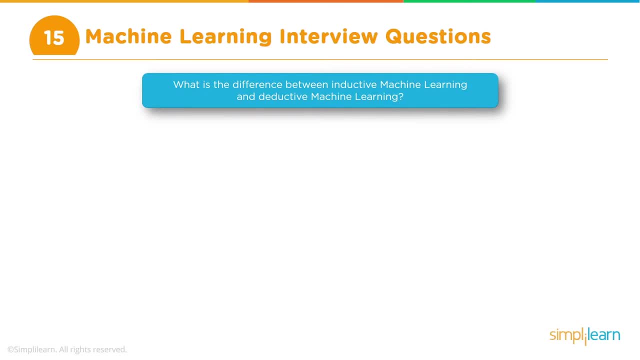 About inductive machine learning and deductive machine learning. So the question can be: what is the difference between inductive machine learning and deductive machine learning? or somewhat in that manner, So that the exact phrase or exact question can vary and they can ask for examples and 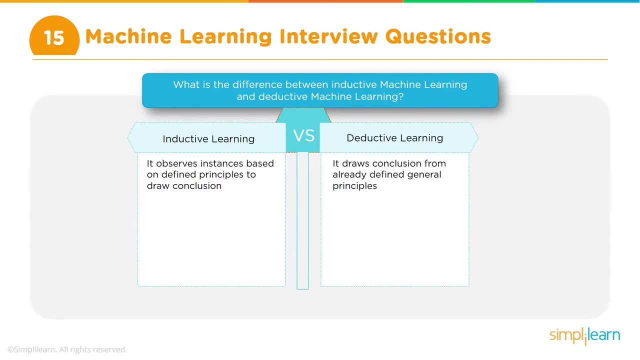 things like that, but that could be the question. So let's first understand what is inductive and deductive training. Inductive training is induced by somebody, and you can illustrate that with a small example. I think that always helps. So whenever you're doing some 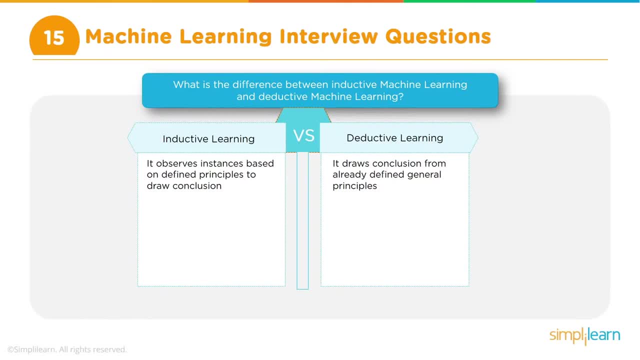 Explanation. try as much as possible, as I said, to give examples from your work experience or give some analogies, and that will also help a lot in explaining as well And for the interviewer also to understand. So here we'll take an example, or rather we will use an analogy. 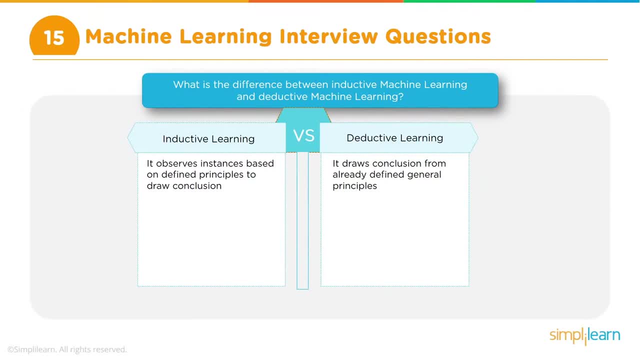 So inductive training is when we induce some knowledge or the learning process into a person without the person actually experiencing it. What can be an example? So we can probably Tell the person, or show a person a video, that fire can burn the thing, burn his finger or fire can cause damage. 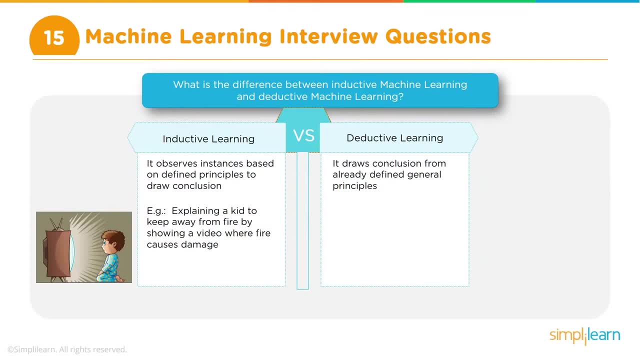 So what is happening here? This person has never probably seen a fire or never seen anything getting damaged by fire, but just because he has seen this video, he knows that, okay, fire is dangerous and if a fire can cause damage, right. 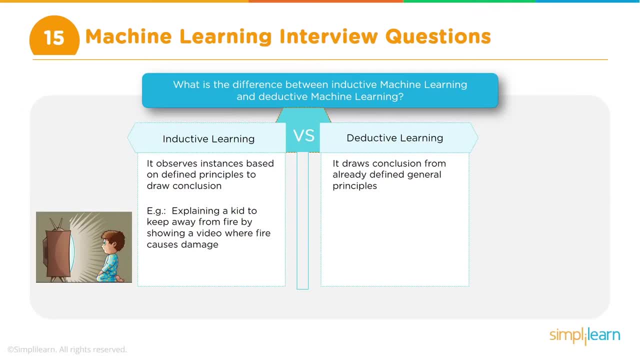 So this is inductive learning. compared to that, What is deductive learning? So here you draw conclusion, or the person draws conclusion out of experience. so we will stick to the analogy. so, compared to the showing a video, let's assume a person is allowed to play with fire, right, and then he figures out that if he puts his finger it's burning, or if throw something into the fire it burns. so he is learning through experience. so this is known as deductive learning. 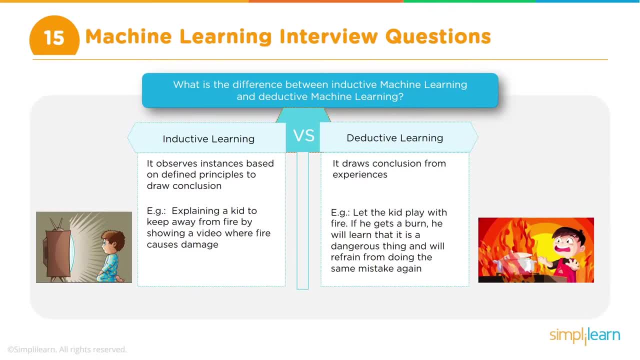 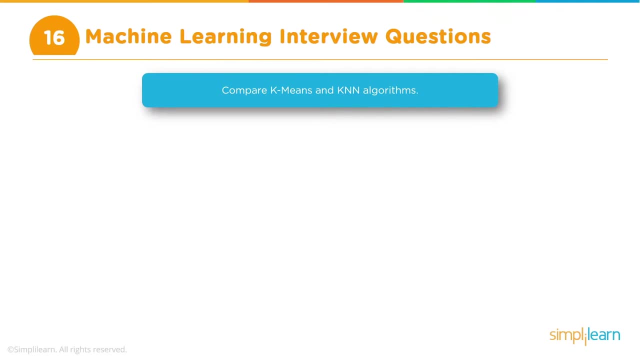 Okay, so you can have applications or models that can be trained using Inductive learning or deductive learning. All right, I think probably that explanation will be sufficient. The next question is: are KNN and K-means clustering similar to one another, or are they same right? 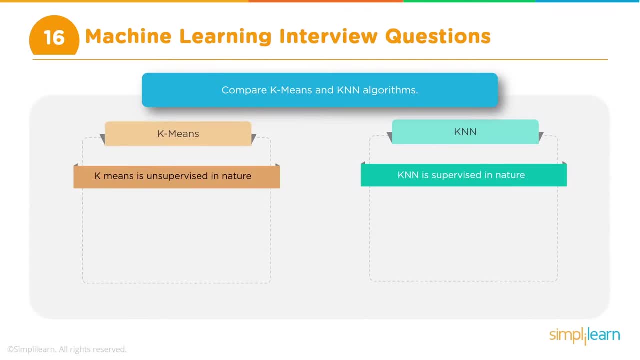 Because the letter K is kind of common between them, okay, So let us take a little while to understand what these two are. One is KNN and another is K-means. KNN stands for K-nearest neighbors and K-means, of course, is the clustering. 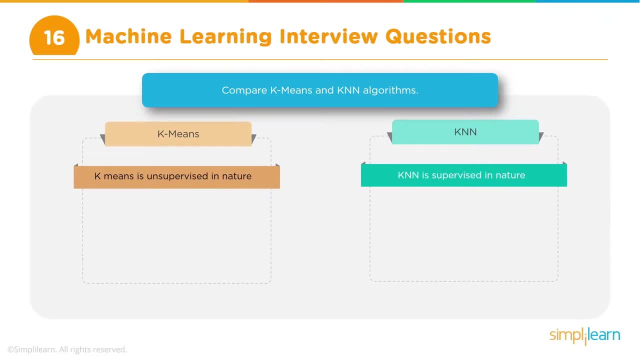 Now, these two are completely different except for the letter K being common between them. KNN is completely different. K-means clustering is completely different. KNN is a classification process and therefore it comes under supervised learning, whereas K-means clustering is actually unsupervised. okay, 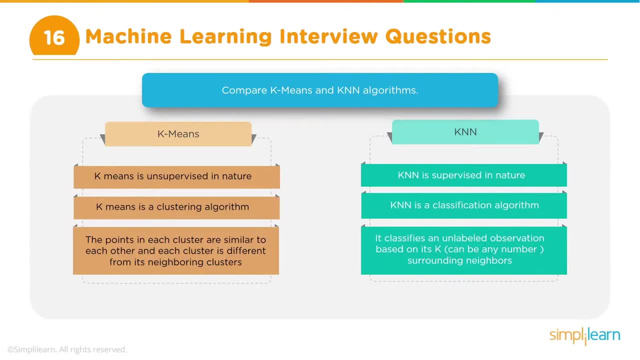 When you have KNN, when you want to implement KNN, which is basically K-nearest neighbors, the value of K is a number, So you can say K is equal to 3.. You want to implement KNN with, K is equal to 3.. 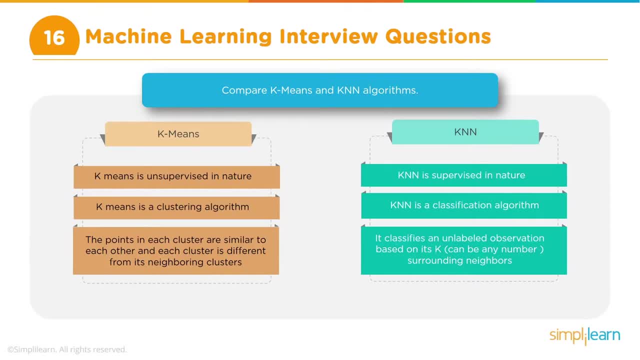 So, which means that it performs the classification in such a way that: how does it perform the classification? So it will take three nearest objects and that is why it is called nearest neighbor. So basically, based on the distance, it will try to find out its nearest objects. that are, let us say, three of the nearest objects. 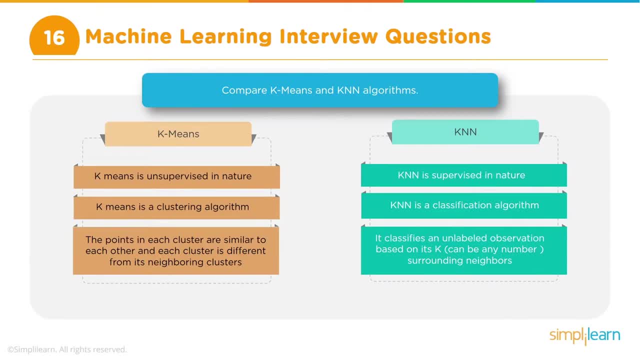 And then it will check whether the class they belong to which class, right? So if all three belong to one particular class, then obviously this new object is also classified as that particular class. but it is possible that they may be from two or three different classes, okay. 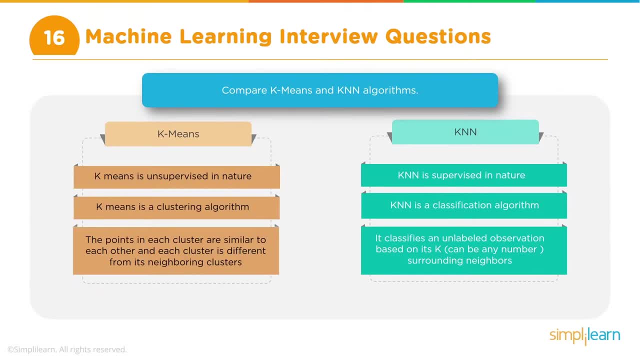 So let us say they are from two classes. and then if they are from two classes, now usually you take an odd number, you assign an odd number to it. So if there are three of them, and two of them belong to one class and then one belongs to another class, 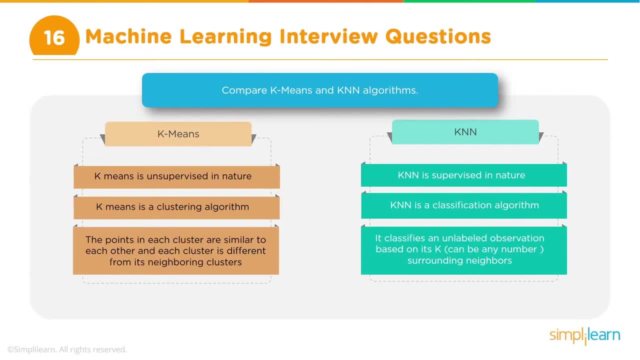 So this new object is assigned to the class to which the two of them belong. Now the value of K is sometimes tricky: Whether should you use KNN, Should you use three? Should you use five? Should you use seven? That can be tricky, because the ultimate classification can also vary. 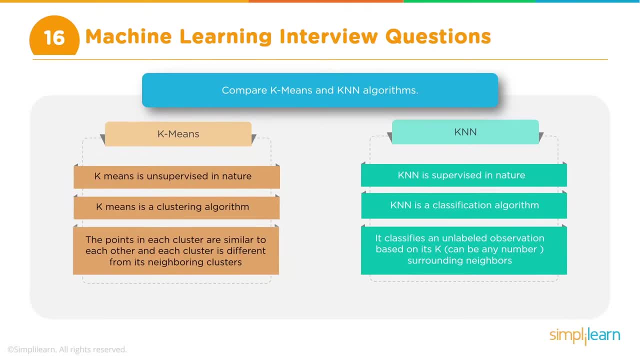 So it's possible that if you're taking K as three, the object is probably in one particular class, But if you take K is equal to five, maybe the object will belong to a different class, because when you're taking three of them, probably two of them belong to class one and one belong to class two. 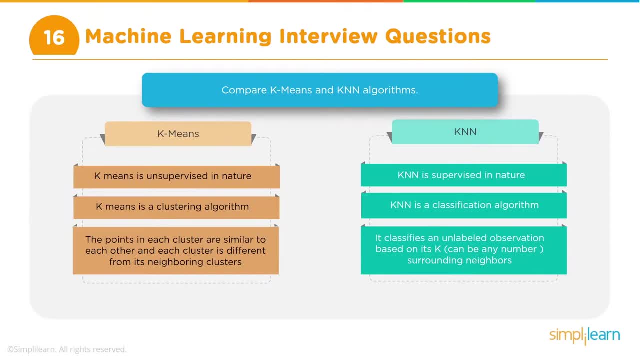 Whereas when you take five of them, it is possible that only two of them belong to class one and three of them belong to class two, So which means that this object will belong to class two. So you see that. So it is. the class allocation can vary depending on the value of K. 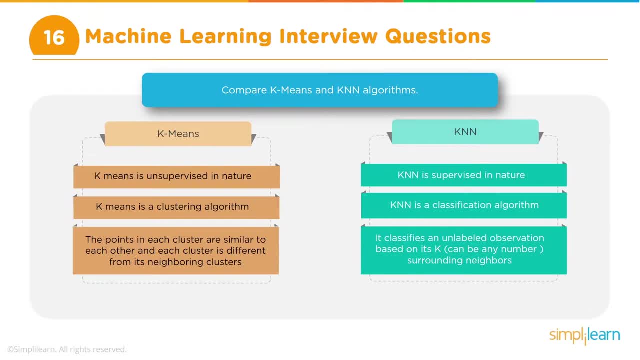 Now K means, on the other hand, is a clustering process and it is unsupervised, Where what it does is the system will basically identify how the objects are, how close the objects are with respect to some of their features. OK, 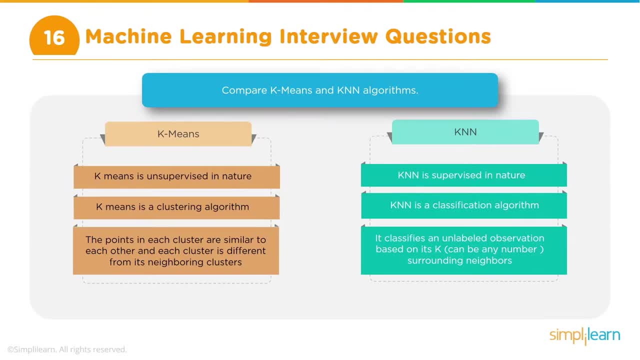 But the similarity, of course, is the letter K, And in case of K means also we specify its value, and it could be three or five or seven. There is no technical limit as such, but it can be any number of clusters that you can create. 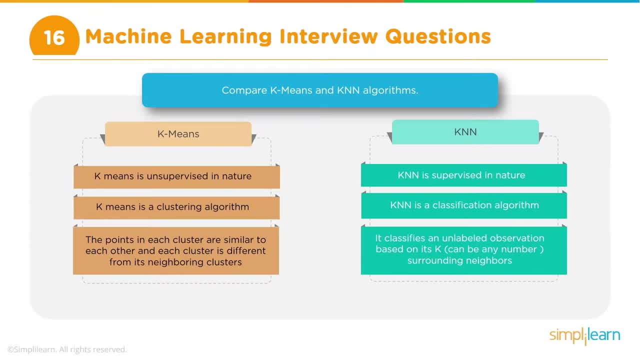 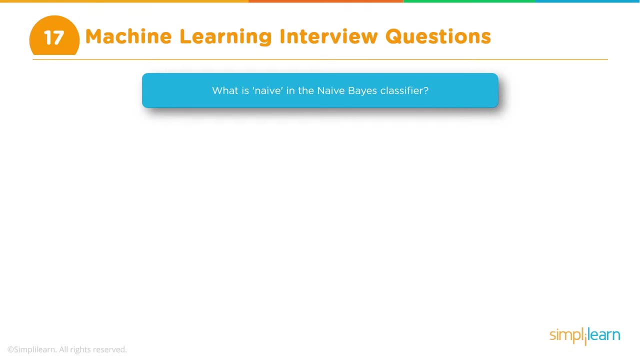 OK, So based on the value that you provide, the system will create that many clusters of similar objects. So there is a similarity to that extent that K is a number in both the cases, But actually these two are completely different processes. We have what is known as naive based. 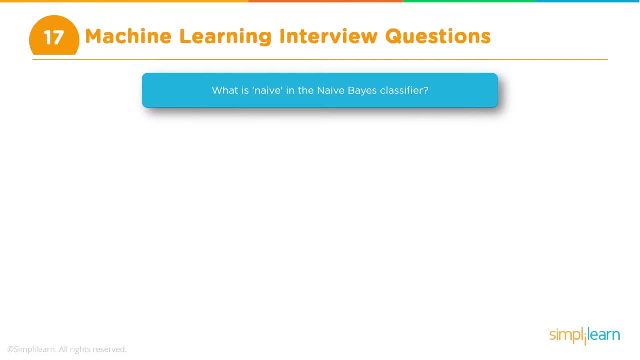 classifier and people often get confused, thinking that naive based is the name of the person who found this classifier or who developed this classifier, which is not 100 percent true. Base is the name of the person. B-A-Y-E-S is the name of the person, but naive is not the name of the person. 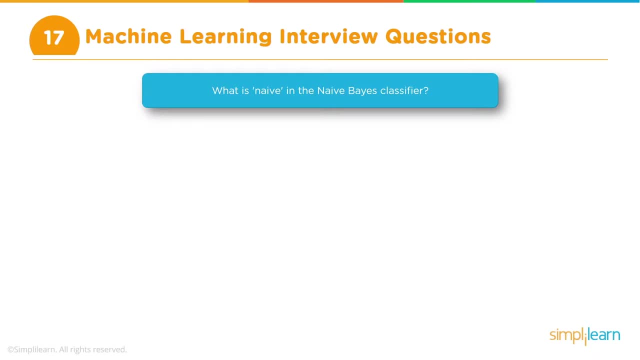 Right, So naive is basically an English word And that has been added here because of the nature of this particular classifier. Naive based classifier is a probability based classifier And it makes some assumptions that the presence of one feature of a class is not related to the presence of any other feature of maybe other classes. 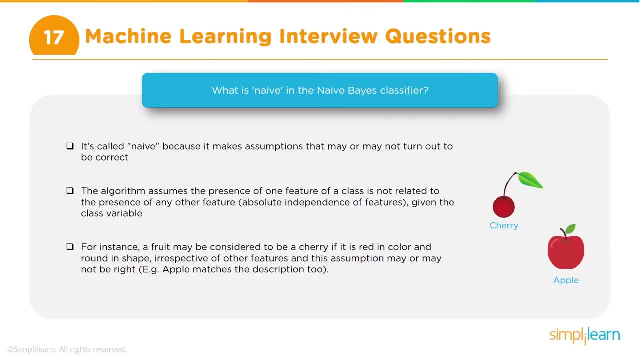 Right, So which is not very strong or not a very- what do you say? accurate assumption, because these features can be related and so on. But even if we go with this assumption, this whole algorithm works very well, even with this assumption. 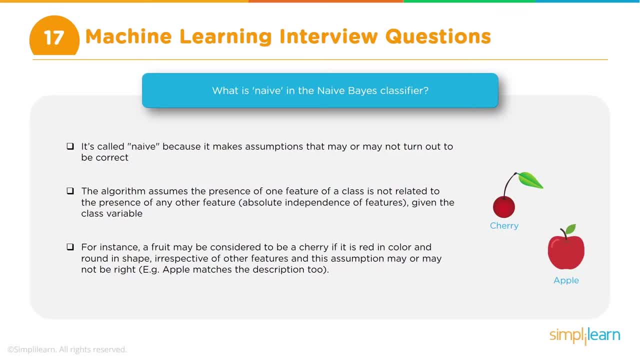 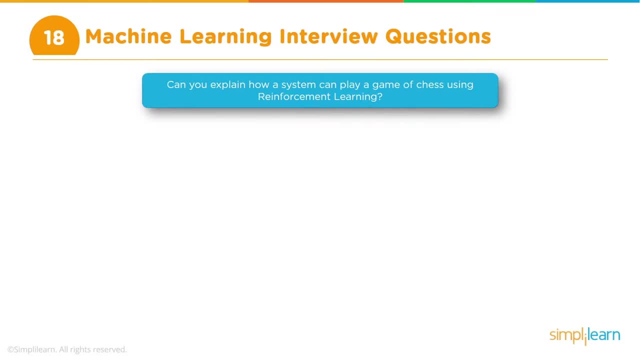 And that is the good side of it, But the term comes from that, So that is the explanation that you can get. Then there can be question around reinforcement learning. It can be paraphrased in multiple ways. One could be: can you explain how a system 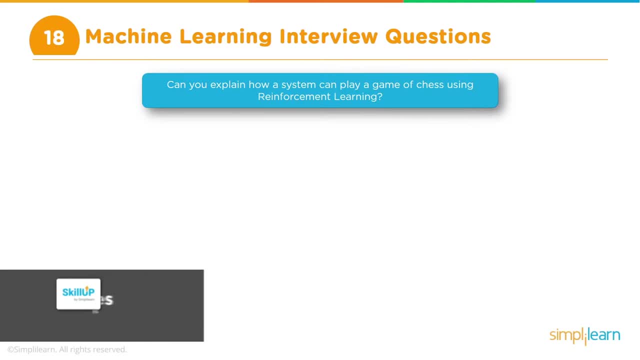 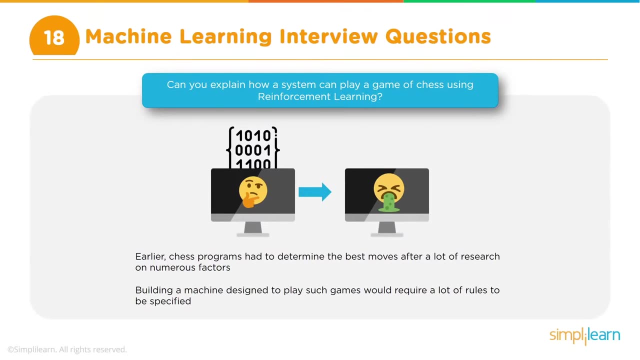 can play a game of chess using reinforcement learning, or it can be any game. So the best way to explain this is again to talk a little bit about what reinforcement learning is about and then elaborate on that to explain the process. So, first of all, reinforcement learning has an environment and an agent and 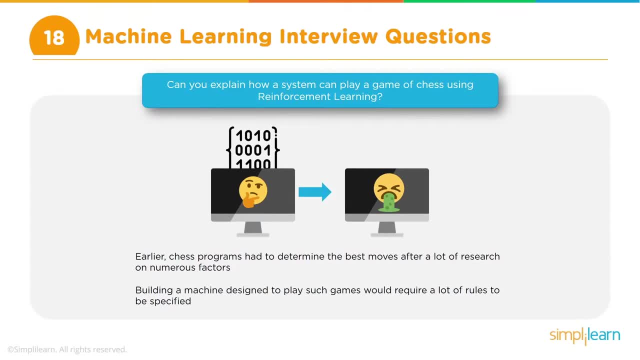 the agent is basically performing some actions in order to achieve a certain goal, And these goals can be anything either. if it is related to game, then the goal could be that you have to score very high score a high value, high number, or it could be that your number of lives should be as high as possible. 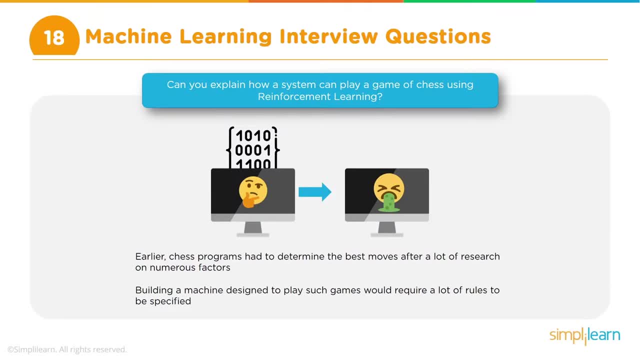 Don't lose life. So these could be some of them. More advanced examples could be for driving the automotive industry: self-driving cars. they actually also make use of reinforcement learning to teach the car how to navigate through the roads, and so on and so forth. That is also another example. 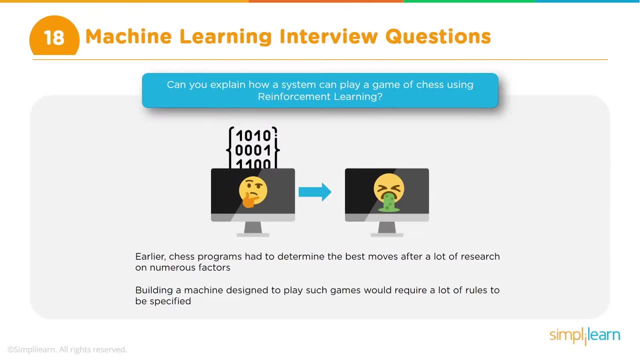 Now, how does it work? So if the system is basically there is an agent and environment, and every time the agent takes a step or performs a task which is taking it towards the goal, the final goal, let's say, to maximize the score or to minimize the number of lives. 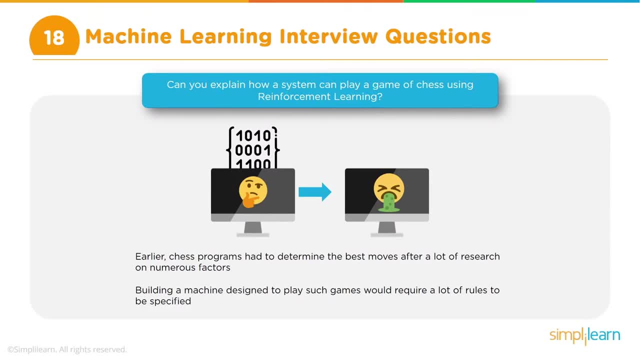 and so on, or minimize the debts, for example, it is rewarded. And every time it takes a step which goes against that goal and contrary or in the reverse direction, it is penalized. OK, so it is like a carrot and stick system. 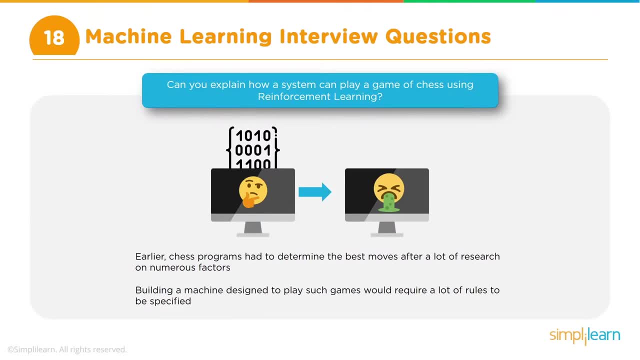 Now, how do you use this to create a game of chess or to create a system to play a game of chess? Now, the way this works is- and this could probably go back to this AlphaGo example, where AlphaGo defeated a human champion- 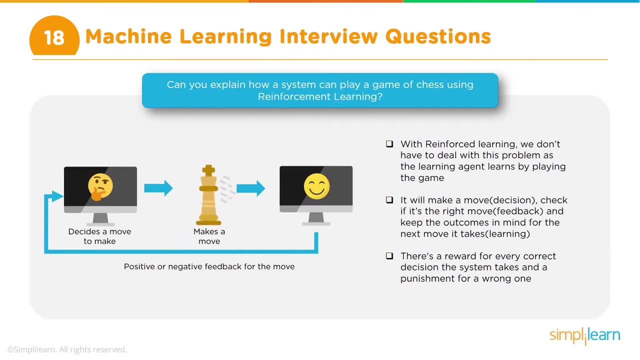 So the way it works is in reinforcement learning, the system is allowed, For example, in this case we are talking about chess, So we allow the system to first of all watch playing a game of chess. So it could be with a human being, or it could be the system itself. 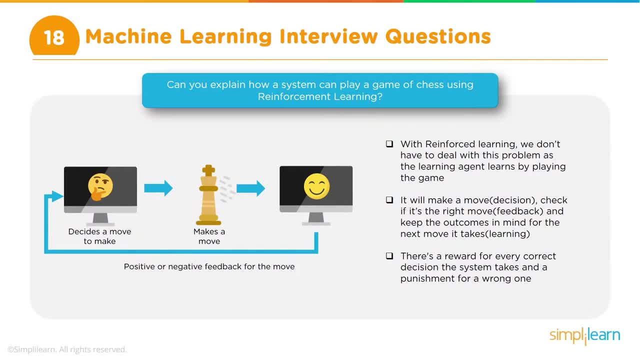 There are computer games of chess, So either this new learning system has to watch that game or watch a human being play the game, because this is reinforcement. learning is pretty much all visual, So when you are teaching the system to play a game, the system will not actually. 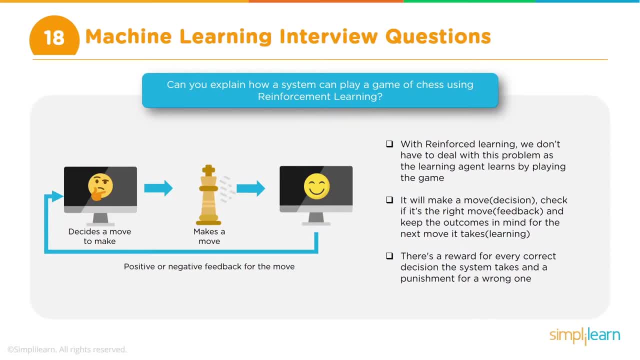 go behind the scenes to understand the logic of your software, of this game or anything like that. It is just visually watching the screen and then it learns. OK, so reinforcement learning to a large extent works. So you need to create a mechanism whereby 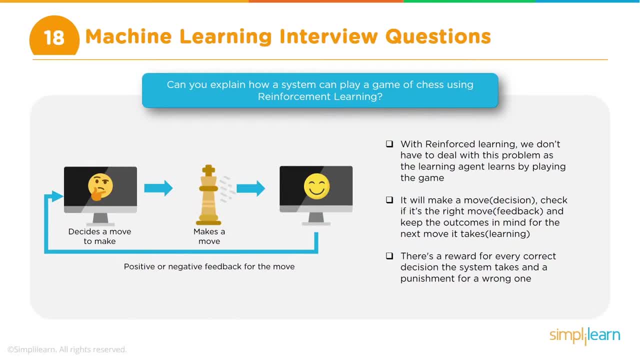 your model will be able to watch somebody playing the game, and then you allow the system also to start playing the game, So it pretty much starts from scratch. OK, And as it moves forward, right at the beginning the system really knows nothing about the game. 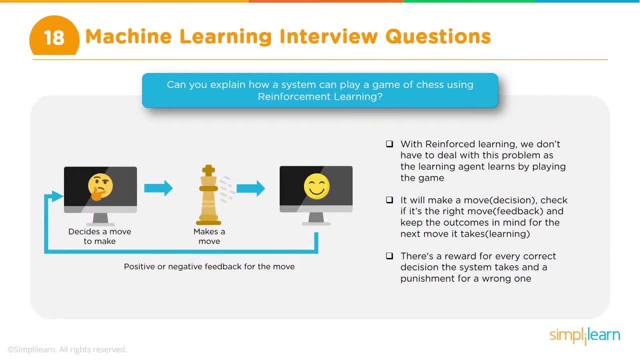 of chess. OK, so initially it is a clean slate. It just starts by observing how you're playing, So it will make some random moves and keep losing badly, But then what happens is over a period of time. So you need to now allow the system or you need to play with the system, not just one. 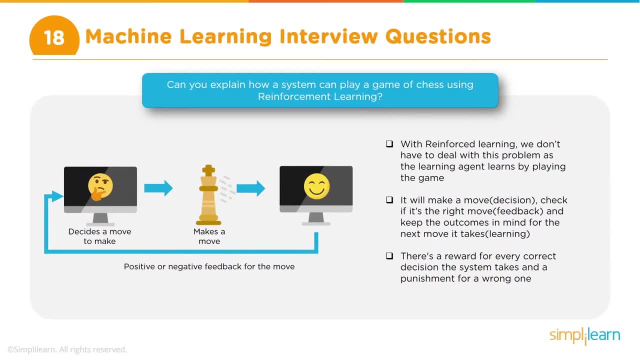 two, three, four or five times, but hundreds of times, thousands of times, maybe even hundreds of thousands of times. And that's exactly how AlphaGo has done. It played millions of games between itself and the system. So for the game of chess also, you need to do something like that. 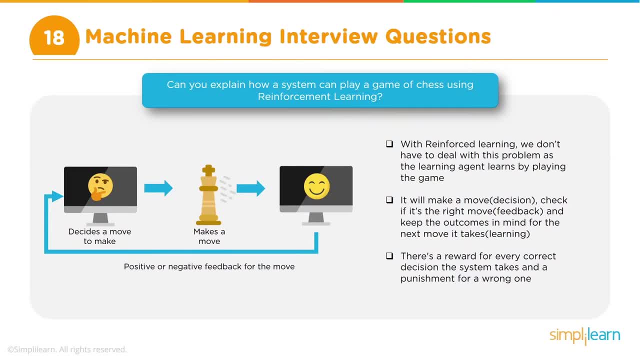 You need to allow the system to play chess and learn on its own over a period of repetition. So I think you can probably explain it to this much, to this extent, And it should be sufficient. Now this is another question which is again somewhat. 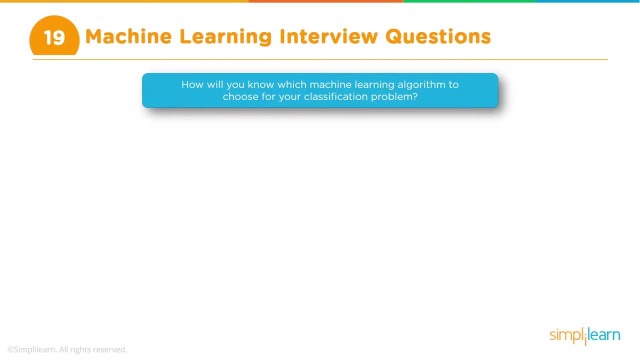 similar, but here the size is not coming into picture. So the question is: how will you know which machine learning algorithm to choose for your classification problem? Now, this is not only classification problem. It could be a regression problem. I would like to generalize this question. 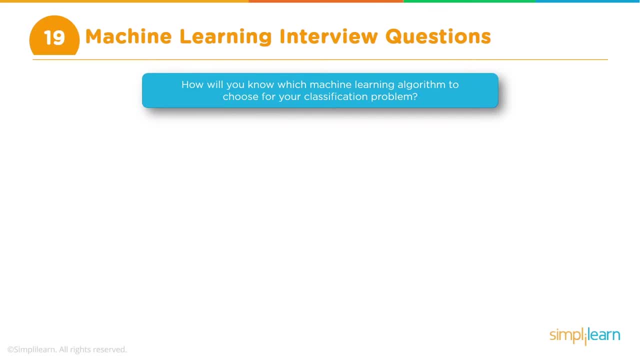 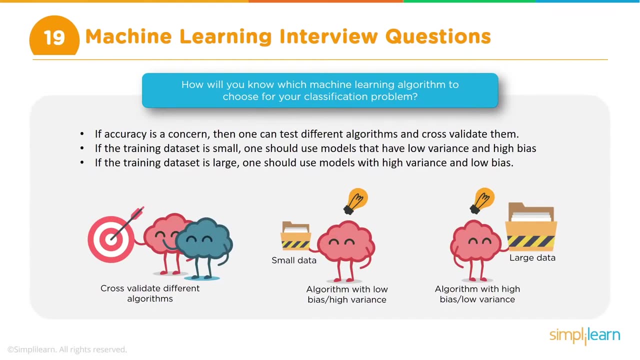 So if somebody asks you, how will you choose, How will you know which algorithm to use, The simple answer is: there is no way you can decide exactly saying that this is the algorithm I'm going to use in a variety of situations. There are some guidelines, like, for example, you will obviously 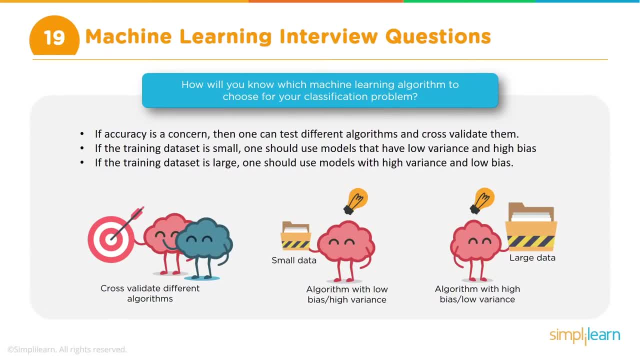 depending on the problem, you can say whether it is a classification problem or a regression problem, and then in that sense you are kind of restricting yourself to: if it is a classification problem There are, you can only apply a classification algorithm to that extent. 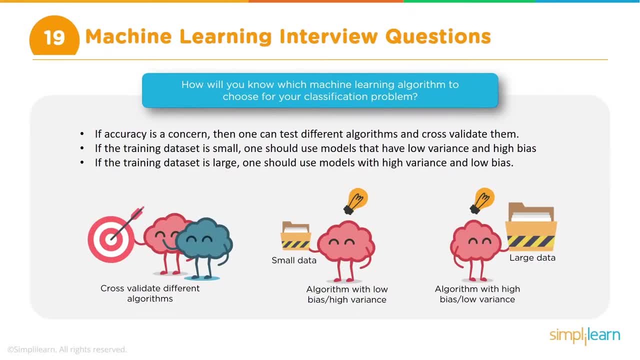 You can probably, let's say, limit the number of algorithms. But now, within the classification algorithms, you have decision trees, you have SVM, you have logistic regression. Is it possible to outright say yes, But for this particular problem, since you have explained this now? 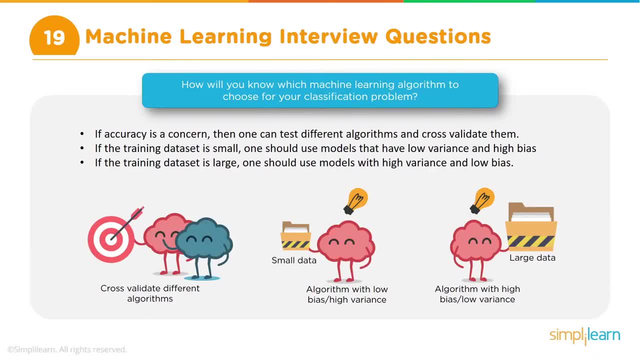 this is the exact algorithm that you can use. That is not possible. So you have to try out a bunch of algorithms, see which one gives us the best performance, best accuracy, and then decide to go with that particular algorithm. So in machine learning a lot of it happens through trial and error. 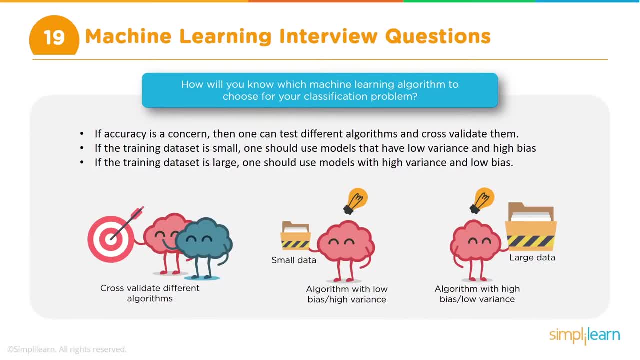 There is no real possibility that anybody can, just by looking at the problem or understanding the problem, tell you that OK, in this particular situation, this is exactly the algorithm that you should use. Then the questions may be around application of machine learning. 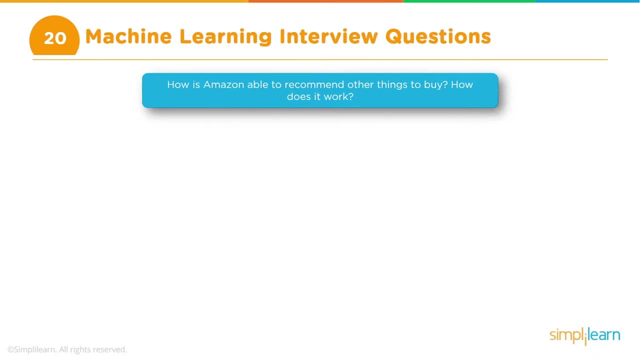 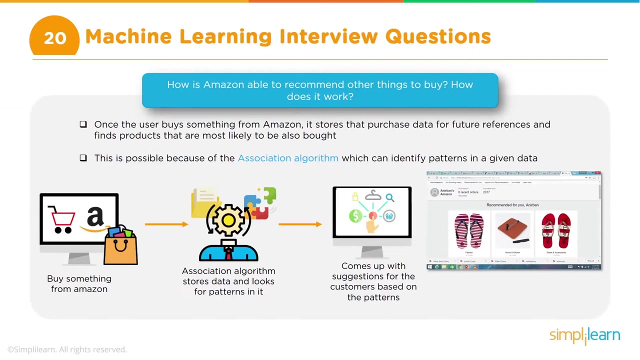 And this question is specifically around how Amazon is able to recommend other things to buy. So this is around recommendation engine: How does it work? How does the recommendation engine work? So this is basically the question is all about. So the recommendation engine again works based on various inputs that are provided. 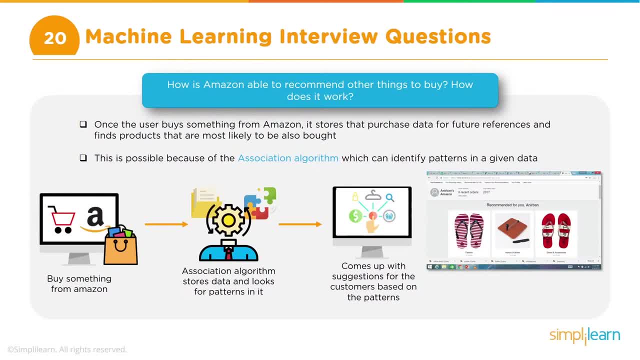 Obviously something like, you know, Amazon. a website or e-commerce site like Amazon collects a lot of data around the customer behavior: who is purchasing what, and if somebody is buying a particular thing, they're also buying something else. So this kind of association. 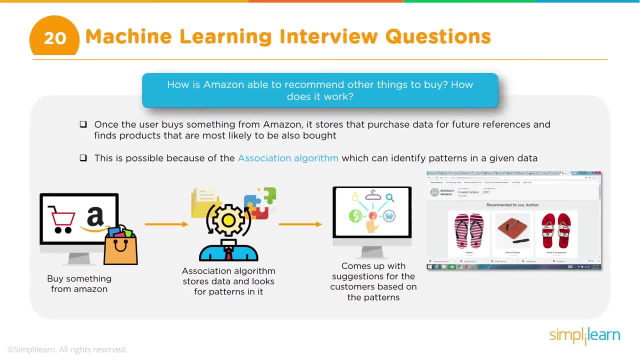 So this is the unsupervised learning we talked about. They use this to associate and link or relate items, And that is one part of it. So they kind of build association between items, saying that somebody buying this is also buying this. That is one part of it. 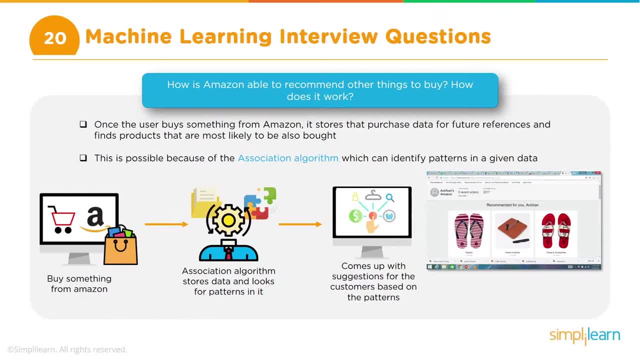 Then they also profile the users based on their age, their gender, their geographic location. They will do some profiling And then when somebody is logging in and when somebody is shopping, kind of the mapping of these two things- are done. They try to identify, obviously, if you have logged in. 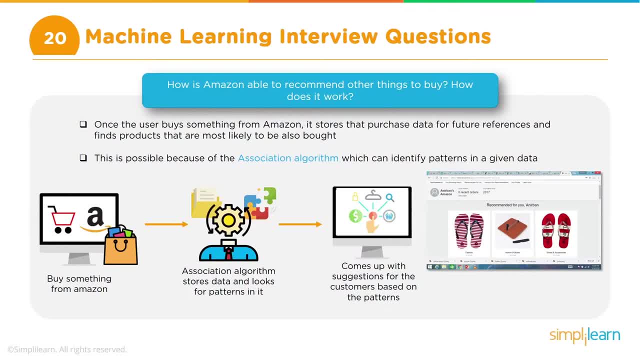 then they know who you are and your information is available, Like, for example, your age, maybe your gender, and where you're located, what you purchased earlier. Right, So all this is, And the recommendation engine basically uses all this information and comes up. 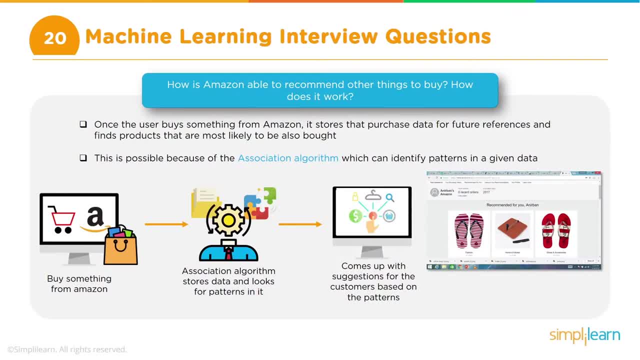 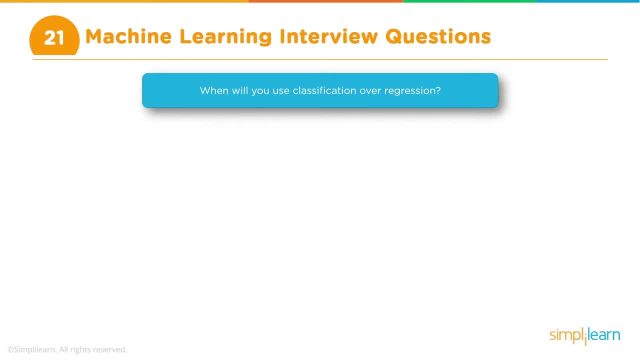 with recommendations for a particular user. So that is how the recommendation engine works, All right. Then the question can be something very basic like: when will you go for classification versus regression, And when do you do classification instead of regression, or when do you use classification instead of regression? 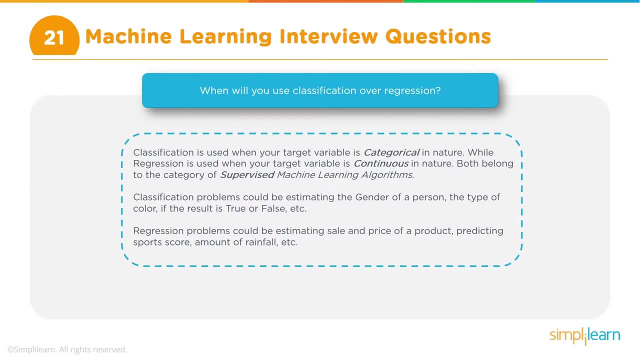 Now, yes, So this is basically going back to the understanding of the basics of classification and regression. So classification is used when you have to identify or categorize things into discrete classes. So the best way to respond to this question is to take up some examples and use it. 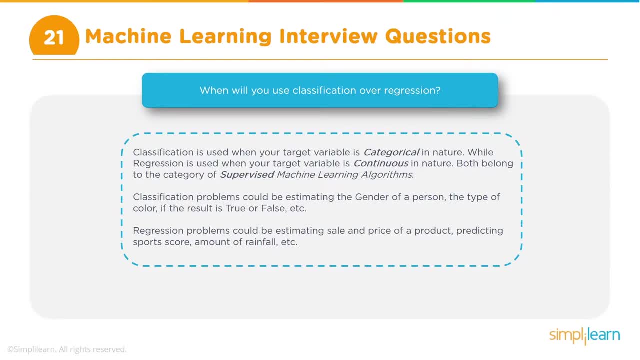 Otherwise it can become a little tricky. The question may sound very simple, but explaining it can sometimes be very tricky. In case of regression we use, of course there will be some keywords that they will be looking for, So just you need to make sure you use those keywords. 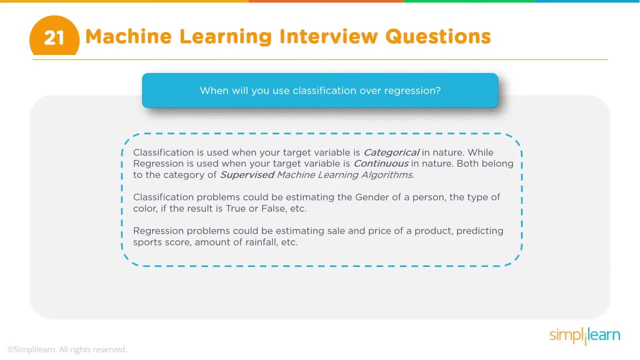 One is the discrete values, Another is the class, Another is the continuous values. So, for regression, if you are trying to find some continuous values, you use regression, whereas if you are trying to find some discrete values you use classification. and then you need to illustrate what are. 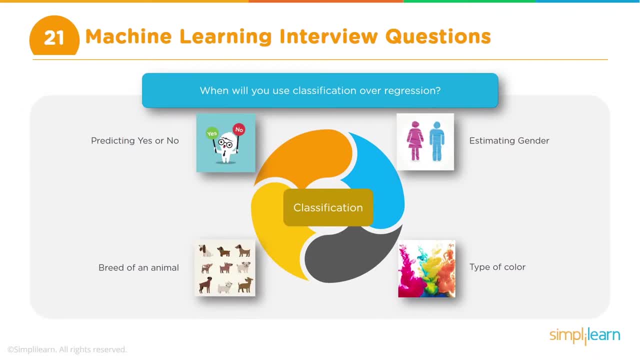 some of the examples of classification is like, let's say, there are images and you need to put them into classes like cat, dog, elephant, tiger, something like that. So that is a classification problem, or it can be that is a multiclass classification problem. 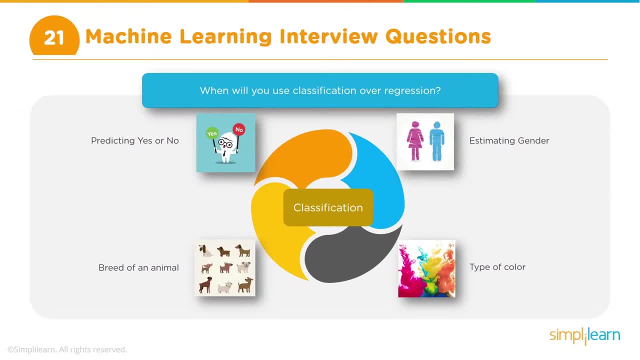 It could be binary classification problem, Like, for example, whether a customer will buy or he will not buy. That is a classification, binary classification. It can be in the weather forecast area. Now weather forecast is again a combination of regression and classification. 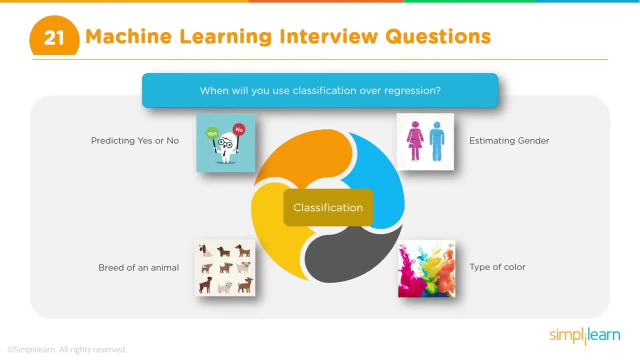 because, on the one hand, you want to predict whether it's going to rain or not. That's a classification problem, That's a binary classification right, Whether it's going to rain or not rain. However, you also have to predict what is going to be the temperature tomorrow. 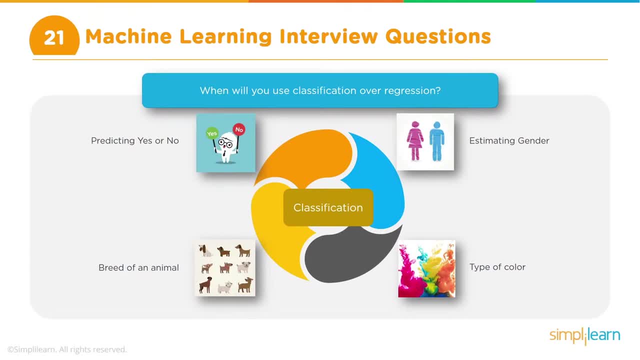 Now, temperature is a continuous value. You can't answer the temperature in a yes or no kind of a response, Right? So what will be the temperature tomorrow? So you need to give a number which can be like 20 degrees, 30 degrees or whatever. 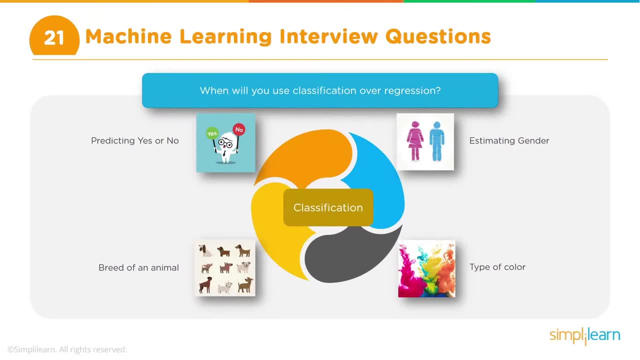 Right, So that is where you use regression. One more example is stock price prediction, So that is where, again, you will use regression. So these are the various examples. So you need to illustrate with examples and make sure you include those keywords like discrete and continuous. 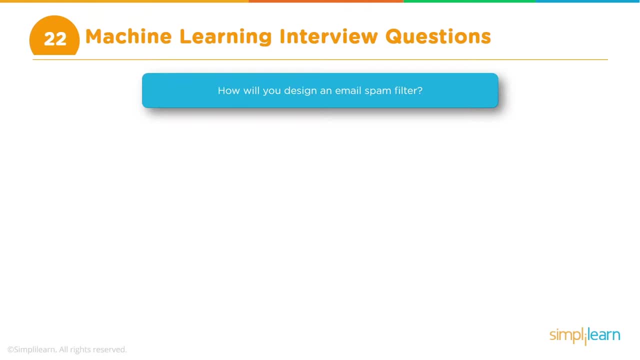 The next question Is more about a little bit of a design related question to understand your concepts and things like that. So it is: how will you design a spam filter? So how do you basically design a spam filter? So I think the main thing here is he's. 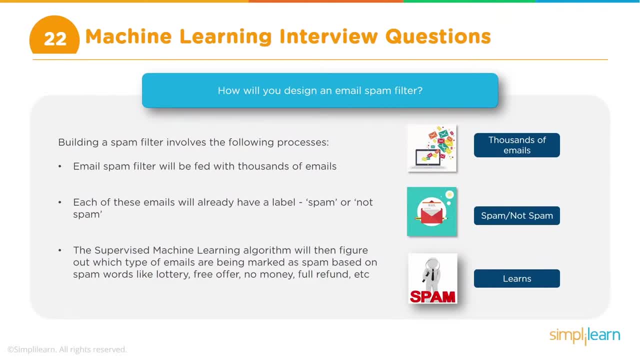 looking at, probably understanding your concept in terms of what is the algorithm you will use or what is your understanding about difference between classification and regression and things like that, and the process, of course. So the best way to go about responding to this is we say that OK. 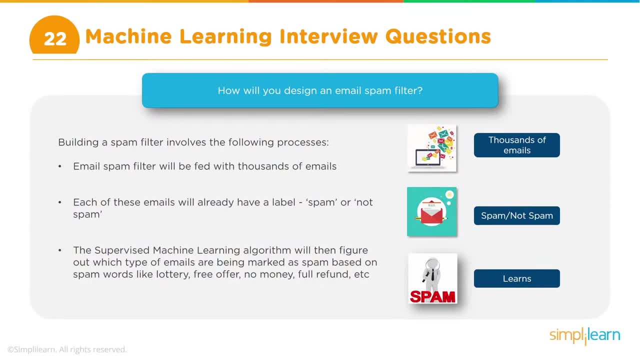 this is a classification problem, because we want to find out whether an email is a spam or not spam so that we can apply the filter accordingly. So first thing is to identify what type of a problem it is. So we have identified that it is a classification. 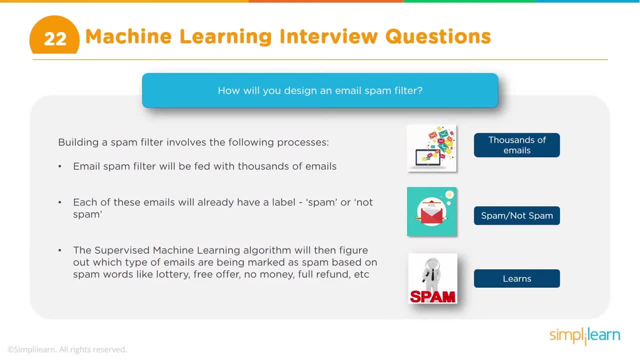 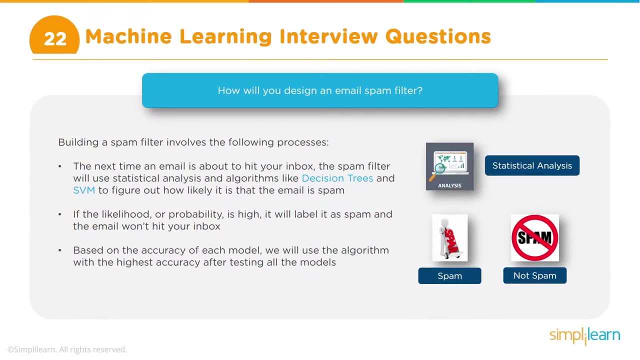 Then the second step may be to find out what kind of algorithm to use Now, since this is a binary classification problem. logistic regression is a very common, very common algorithm, But however, as I said earlier also, we can never say that OK. 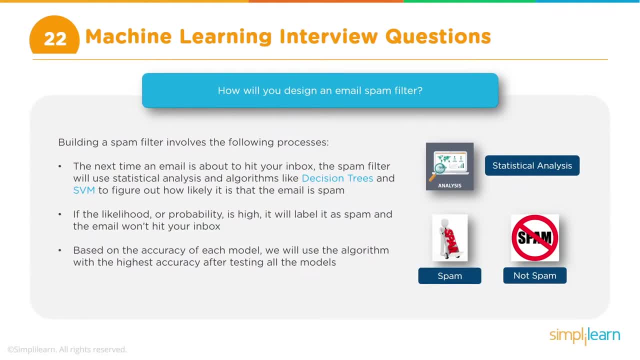 for this particular problem. this is exactly the algorithm that we can use. So we can also probably try decision trees or even support vector machines, for example SVM. So we will kind of list down a few of these algorithms and we will say, OK, we want to, we would like to try out these algorithms. 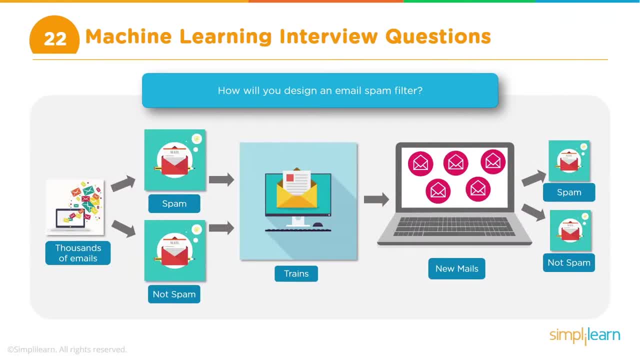 And then we go about taking your historical data, which is the labeled data Which are marked, So you will have a bunch of emails, and then you split that into training and test data sets. you use your training data set to train your model, that or your algorithm. 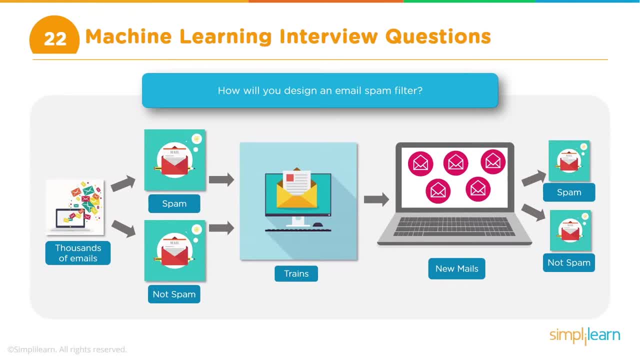 that you've used, or rather the model actually So, and you actually will have three models. Let's say you are trying to test out three algorithms, So you will obviously have three models. So you need to try all three models and test them out as well. 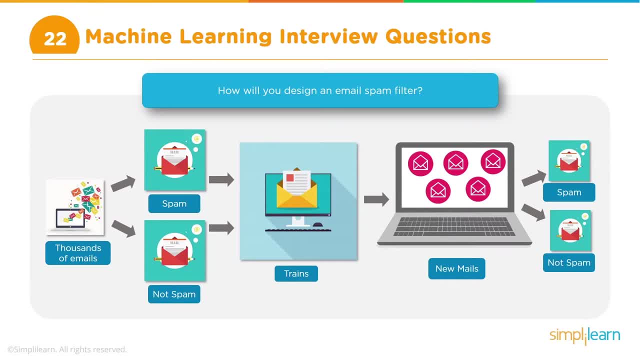 See which one gives the best accuracy, And then you decide that you will go with that model. OK, so training and test will be done. and then you zero in on one particular model And then you say, OK, this is the model we will use. 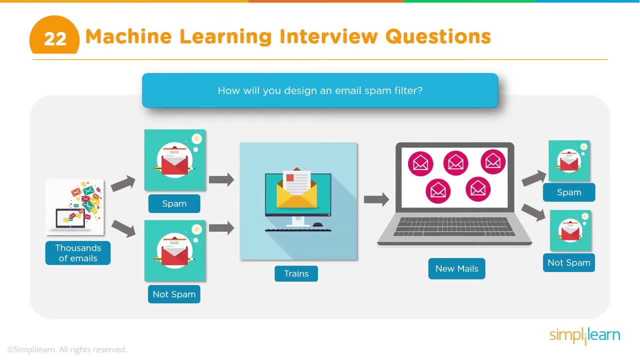 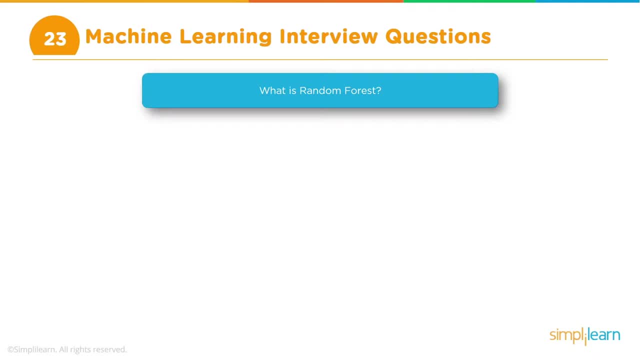 We will use and then go ahead and implement that or put that in production. So that is the way you design a spam field. The next question is about random forest. What is random forest? This is a very straightforward question. However, the response: you need to be again a little careful. 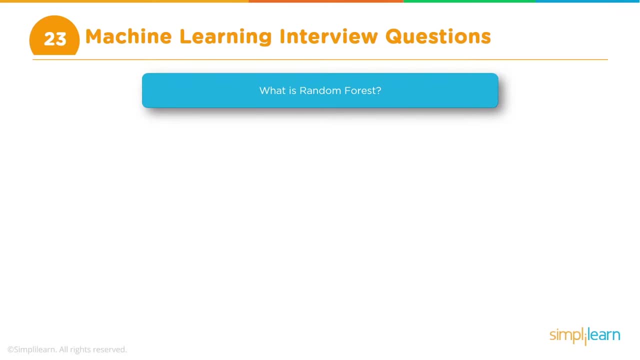 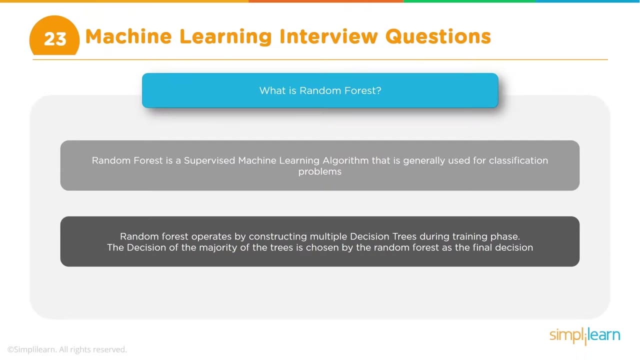 While we all know what is random forest, explaining this can sometimes be tricky. So one thing is random: forest is kind of, in one way it is an extension of decision trees, because it is basically nothing but you have multiple decision trees and trees will basically be used for doing, if it is, classification. 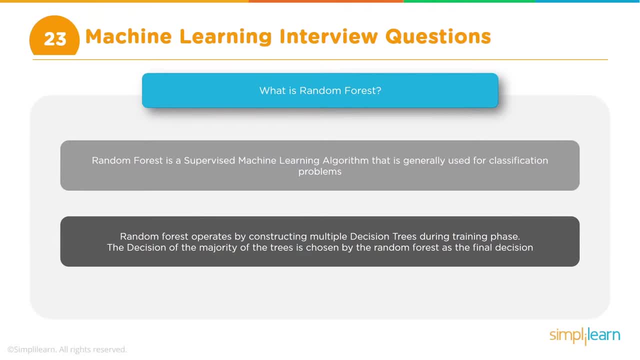 Mostly it is classification. You will use the trees for classification and then you use voting for finding the final class. So that is the underlines. But how will you explain this? How will you respond to this? So, first thing, obviously we will say that random forest is one. 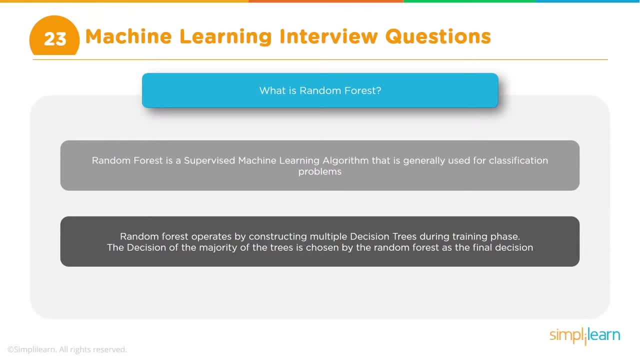 of the algorithms and the more important thing that you need to- probably the interviewer is waiting to hear- is ensemble learner. So this is one type of ensemble learner. What is ensemble learner? Ensemble learner is like a combination of algorithms, So it is a learner which consists of more. 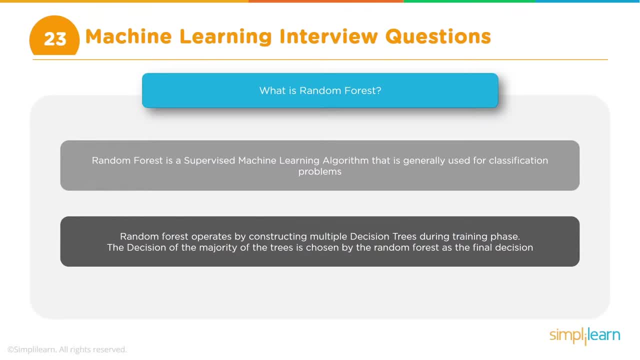 than one algorithm, or more than one, maybe models. So, in case of random forest, the algorithm is the same, But instead of using one instance of it, we use multiple instances of it, and we use So in a way that is a random forest is an ensemble. 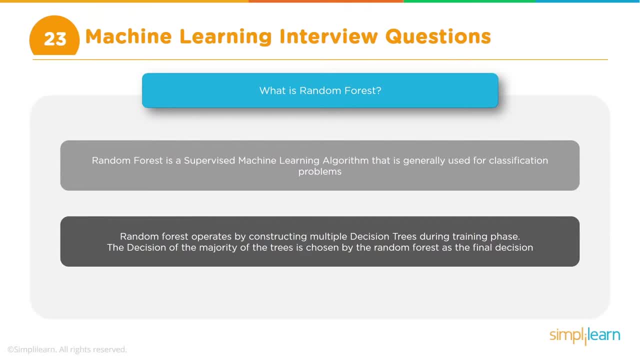 There are other types of ensemble learners where we have, like we use different algorithms itself, so you have one, maybe logistic regression and a decision tree combined together, and so on and so forth. or there are other ways like, for example, splitting the data in a certain way, and so on. 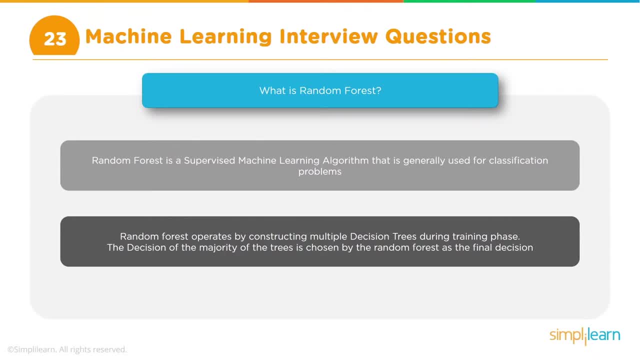 So that's all about ensemble. We will not go into that, But random forest itself. I think the interviewer will be happy to hear this word: ensemble learner. And so then you go and explain how the random forest works. So if the random forest is used, 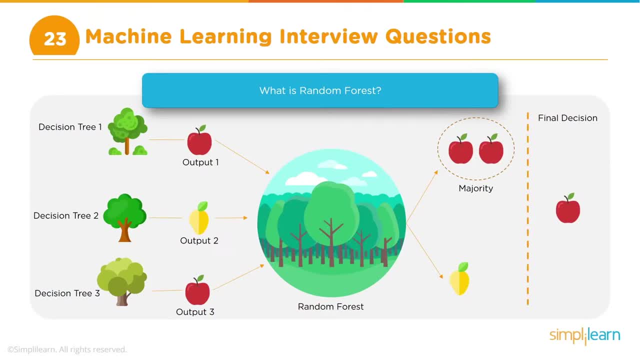 for classification, then we use what is known as a voting mechanism. So basically, how does it work? Let's say your random forest consists of 100 trees and each observation you pass through this forest and each observation. let's say it is a classification problem. 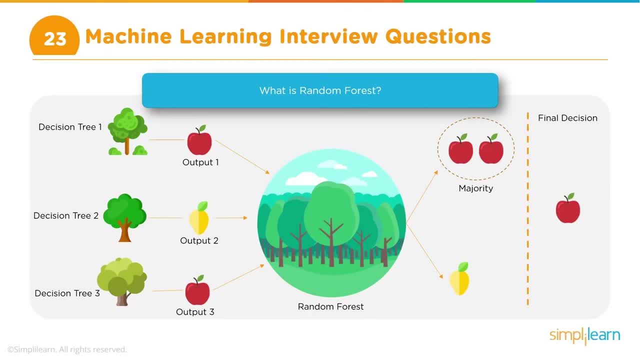 binary classification- zero or one, and you have 100 trees. Now if 90 trees say that it is a zero and 10 of the trees say it is one, then you take the majority, You may take a vote And since 90 of them are saying zero, you classify this as zero. 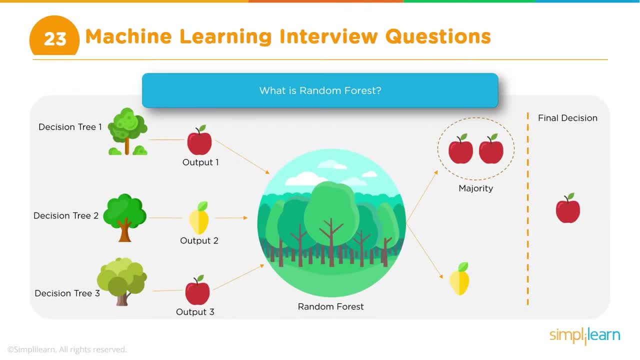 Then you take the next observation, and so on. So that is the way random forest works for classification. If it is a regression problem, it's somewhat similar, But only thing is, instead of vote, what we will do is regression. Remember what happens. 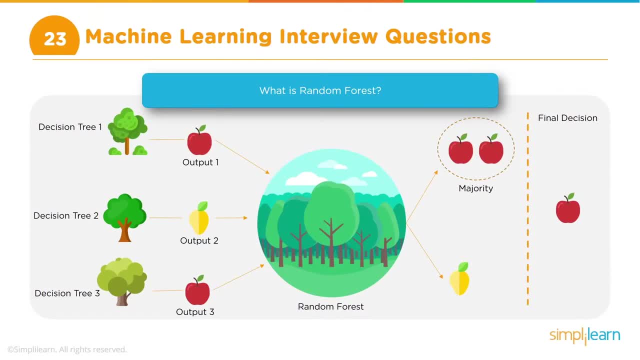 You actually calculate a value right. So, for example, you're using regression to predict the temperature and you have 100 trees and each tree, Obviously, we'll probably predict a different value of the temperature. They may be close to each other, but they may not be exactly the same value. 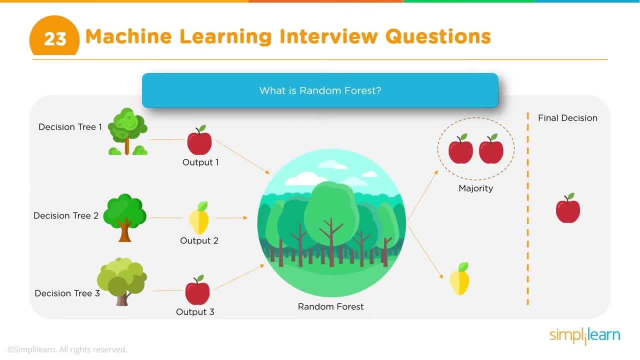 So these 100 trees. So how do you now find the actual value, the output for the entire forest? So you have outputs of individual trees which are a part of this forest, But then you need to find the final output of the forest itself. 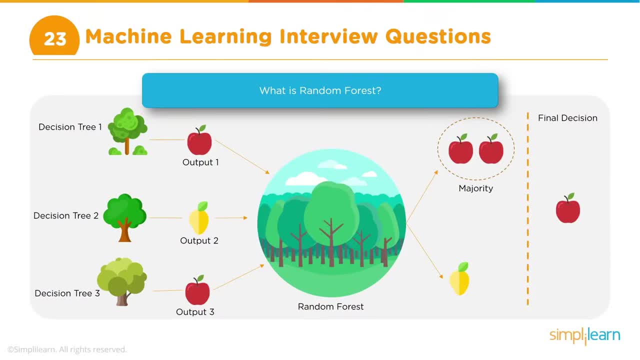 So how do you do that? So in case of regression, you take like an average or the mean of all the 100 trees, Right? So this is also a way of reducing the error. So maybe if you have only one tree and if that one tree makes an error, 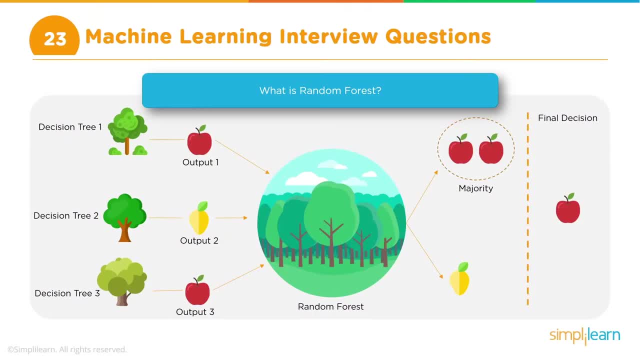 it is basically 100 percent wrong or 100 percent right. But if you have, on the other hand, if you have a bunch of trees, you are basically mitigating that error, reducing that error. OK, so that is the way random forest works. 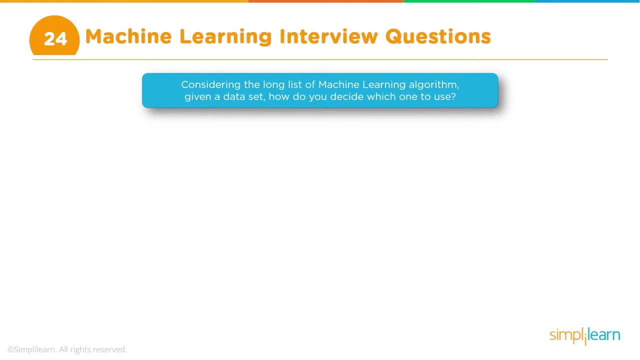 So the next question is: considering the long list of machine learning algorithms, How will you decide on which one to use? So once again here, there is no way to outright say that this is the algorithm that we will use for a given data set. 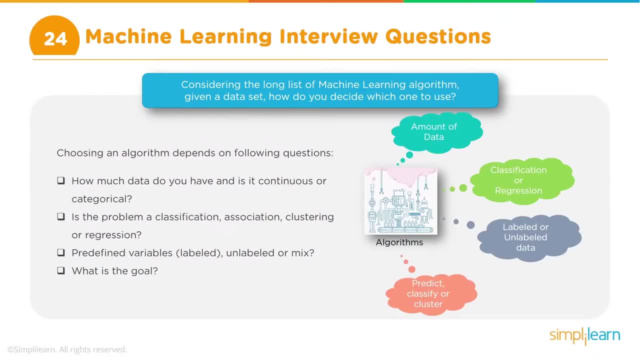 This is a very good question, But then the response has to be like again: there will not be a one size fits all, So we need to. first of all, you can probably shorten the list in terms of by saying, OK, whether it is a classification problem or it is a regression problem. 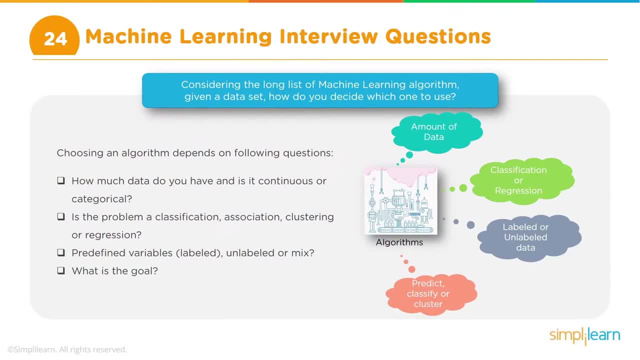 To that extent you can probably shorten the list because you don't have to use all of them. If it is a classification problem, you only can pick from the classification algorithms. So, for example, if it's a classification, you cannot use linear regression algorithm. 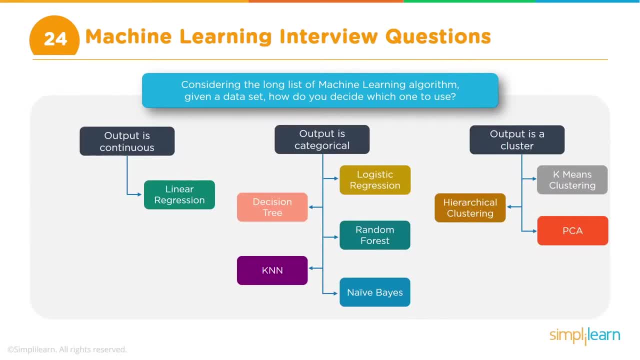 or if it is a regression problem, you cannot use SVM. or maybe you can use SVM, but maybe a logistic regression. So to that extent you can probably shorten the list, but still you will not be able to 100 percent decide on saying that this is the exact algorithm that I'm going to use. 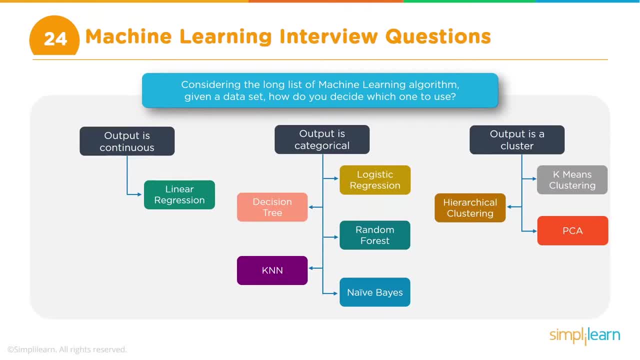 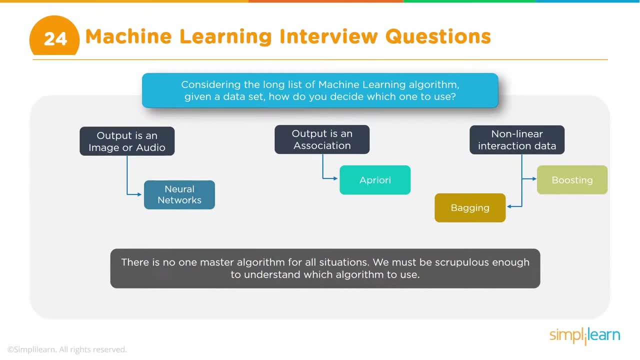 So the way to go about is you choose a few algorithms based on what the problem is. You try out your data, You train some models of these algorithms, Check which one gives you the lowest error or the highest accuracy, And based on that you choose that particular algorithm. 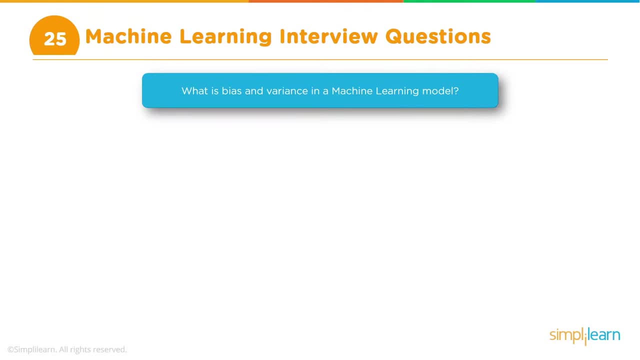 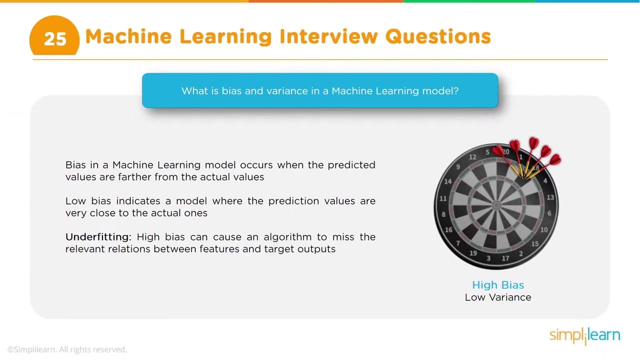 OK, All right. Then there can be questions around bias and variance. So the question can be: what is bias and variance in machine learning? So you just need to give out a definition for each of these. For example, bias in machine learning: it occurs when the predicted values are far. 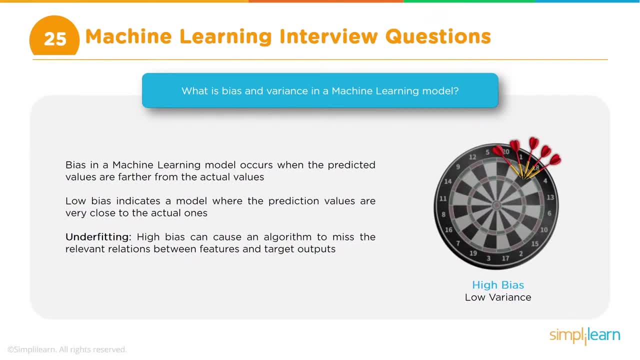 from the actual value. So that is a bias, And whereas they are all, all the values are probably. they are far off, but they are very near to each other, though the predicted values are close to each other, while they are far off from the actual value. 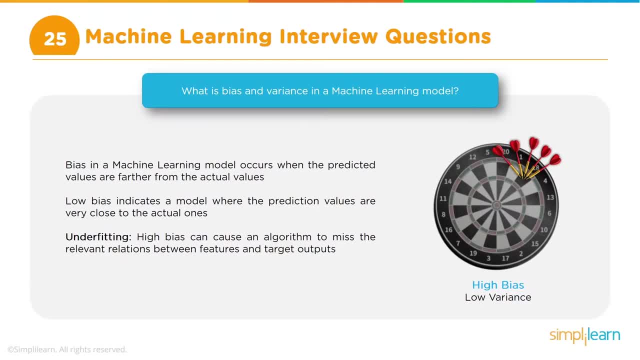 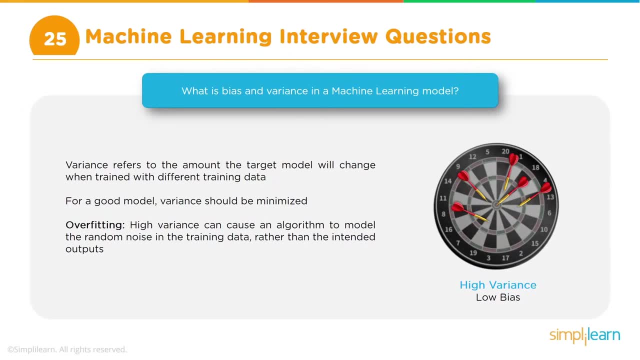 But they are close to each other. You see the difference. So that is bias. And then the other part is your variance. Now, variance is when the predicted values are all over the place, So the variance is high. That means it may be close to the target, but it is kind of. 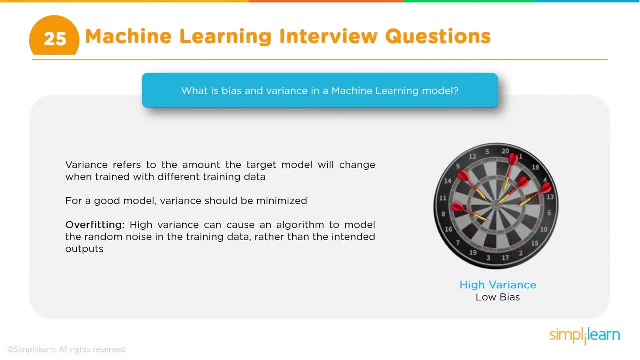 very scattered, to the point, the predicted values are not close to each other. Right, In case of bias, the predicted values are close to each other, but they are not close to the target. But here, they may be close to the target, but they may not be close to each other. 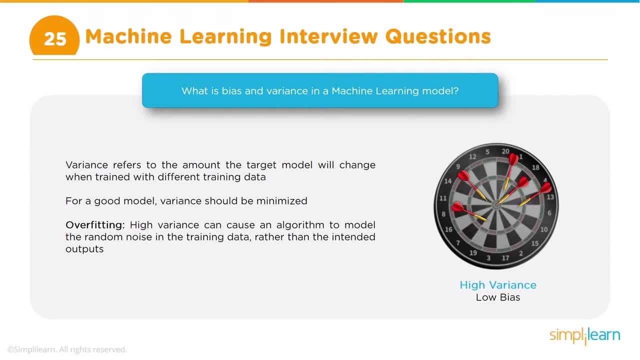 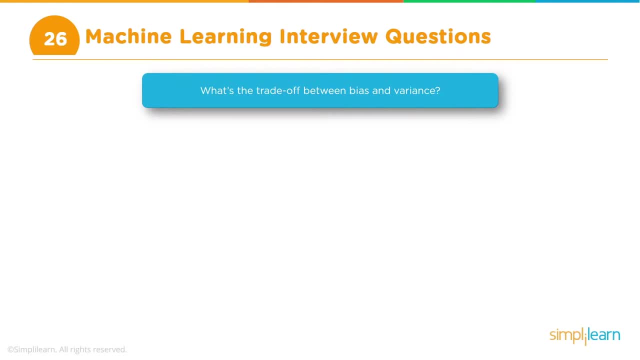 So they are a little bit more scattered. So that is what case of variance? OK, then the next question is about, again related to bias and variance. What is the trade off between bias and variance? Yes, I think this is an interesting question because these two are. 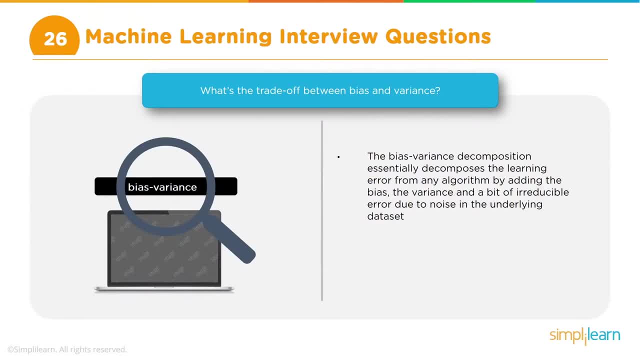 heading in different directions. So, for example, if you try to minimize the bias, variance will keep going high And if you try to minimize the variance, bias will keep going high And there is no way you can minimize both of them. 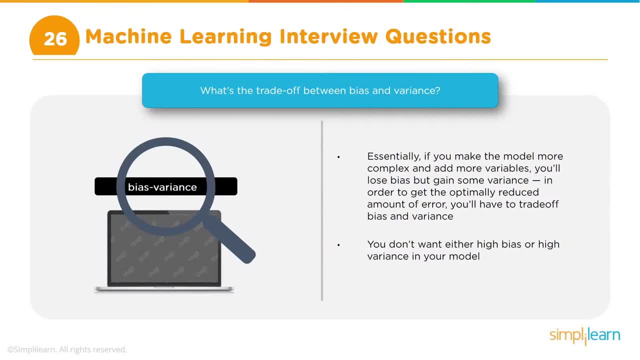 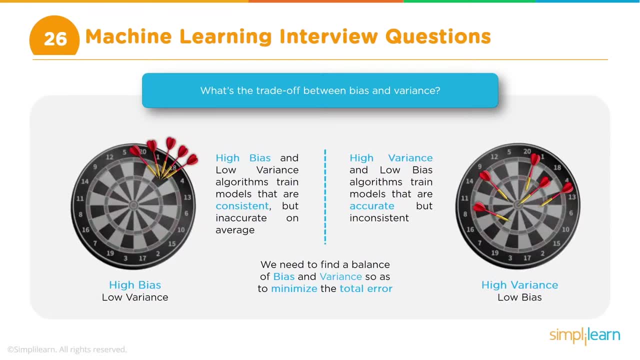 So you need to have a trade off saying that, OK, this is the level at which I will have my bias and this is the level at which I will have variance. So the trade off is that pretty much, that you decide what is the level you will. 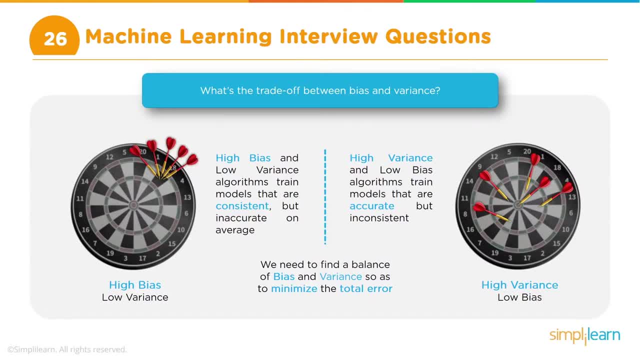 tolerate for your bias and what is the level you will tolerate for variance and a combination of these two in such a way that your final results are not way off, and having a trade off will ensure that the results are consistent. So that is basically: the output is consistent, and which means that they are. 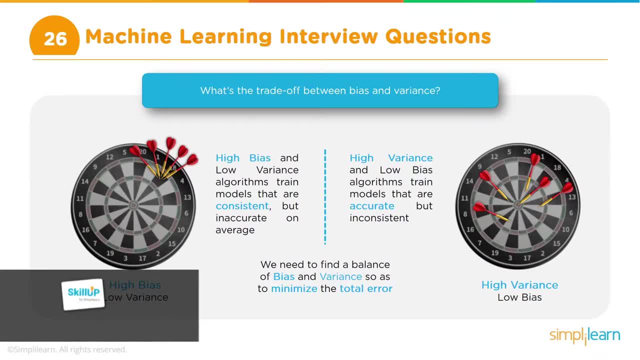 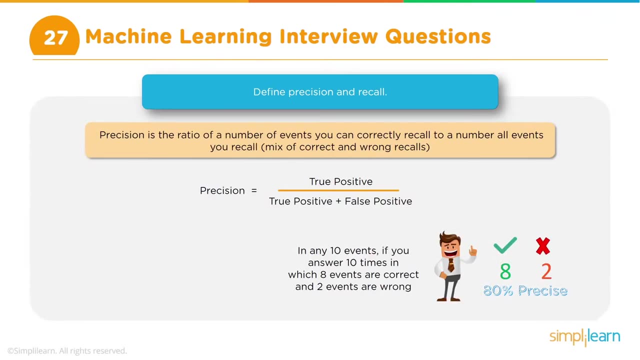 close to each other and they are also accurate. That means they are as close to the target as possible. So if either of these is high, then one of them will go off the track. Define precision and recall. Now again. here I think it would be best to draw a diagram and take the confusion matrix. 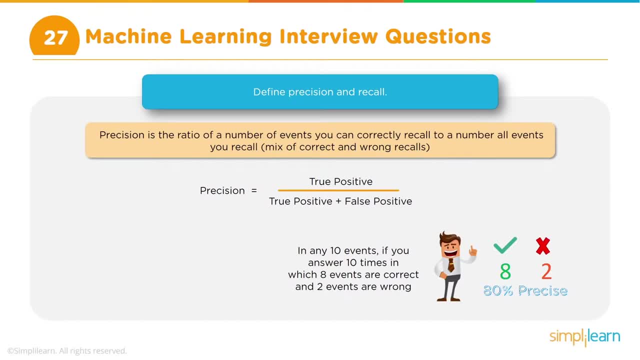 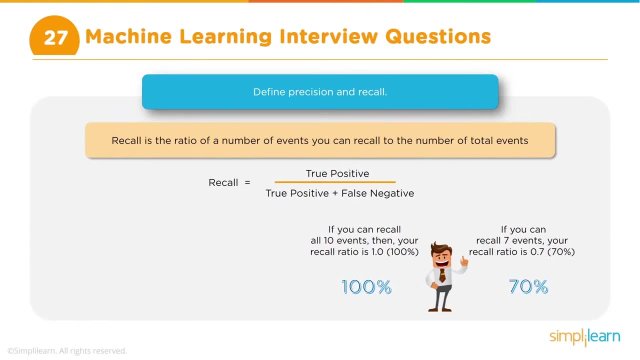 And it is very simple. The definition is like a formula. Your precision is true positive by true positive plus false positive, And your recall is true positive by true positive plus false negative. OK, so that's, you can just show it in a mathematical way. 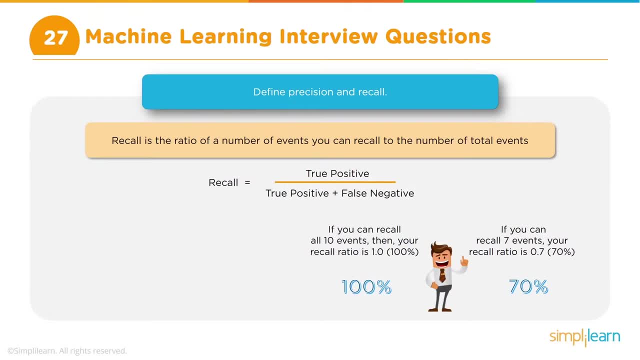 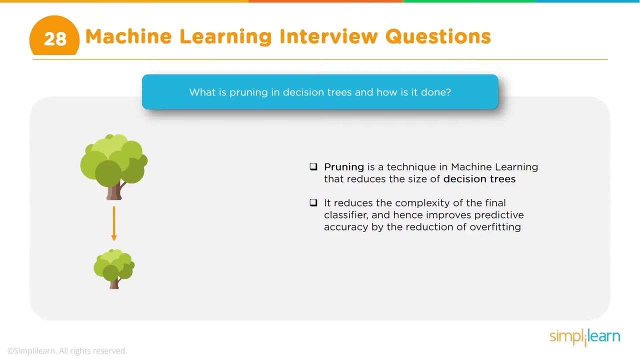 That's pretty much that can be shown. That's the easiest way to define, So the next question can be about decision tree. What is decision tree pruning and why is it So? basically, decision trees are really simple to implement and understand, But one of the drawbacks of decision trees is that it can become highly complicated. 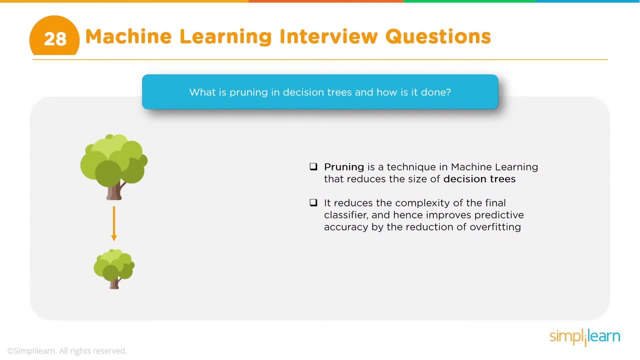 as it grows and the rules and conditions can become very complicated, And this can also lead to overfitting, which is basically that during training you will get 100 percent accuracy, But when you're doing testing you'll get a lot of errors. 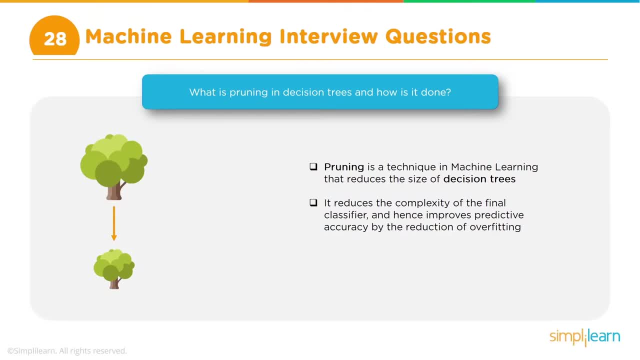 So that is the reason pruning needs to be done. So the purpose or the reason for doing decision tree pruning is to reduce overfitting or to cut down on overfitting. And what is decision tree pruning? It is basically that you reduce the number of branches because, as you may be aware, 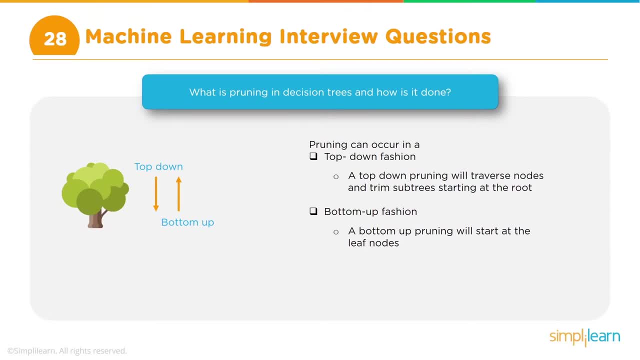 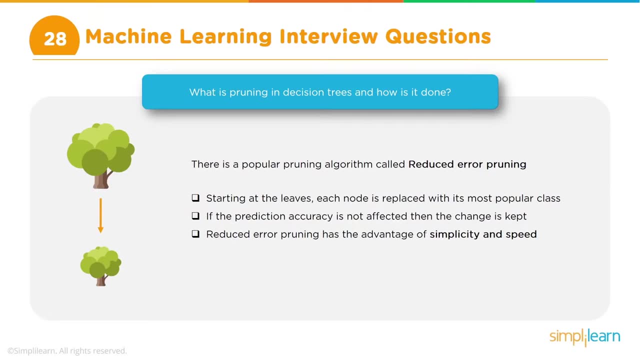 a tree consists of the root node and then there are several internal nodes, and then you have the leaf nodes. Now, if there are too many of these internal nodes, that is when you face the problem of overfitting, and pruning is the process of reducing those internal nodes. All right, 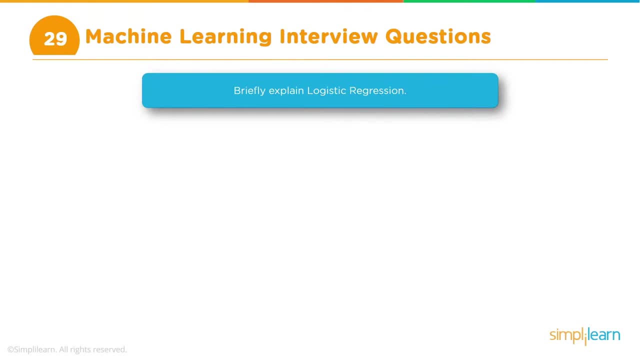 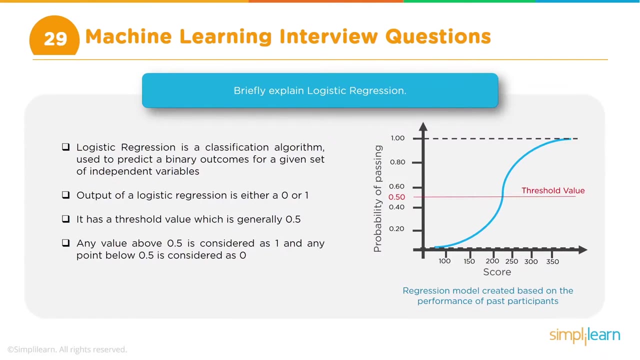 So the next question can be: what is logistic regression? So, basically, logistic regression is one of the techniques used for performing classification, especially binary classification. Now, there is something special about logistic regression and there are a couple of things you need to be careful. 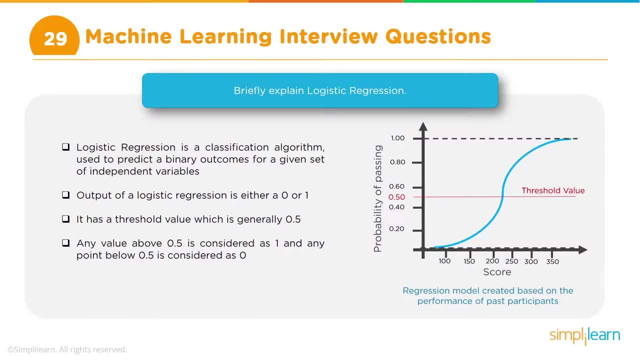 about. First of all, the name is a little confusing. It is called logistic regression but it is used for classification, So this can be sometimes confusing, So you need to probably clarify that to the interviewer, if it's really you know. 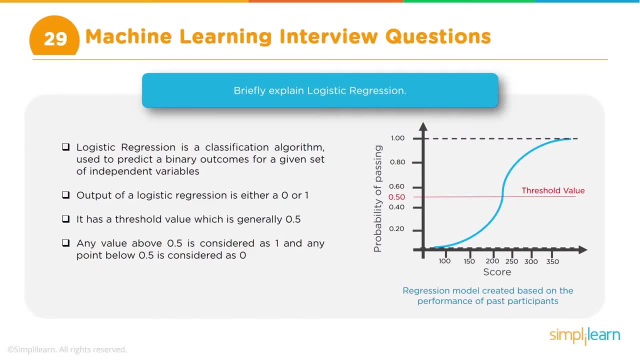 if it is required, and they can also ask this like a trick question, Right? So that is one part. Second thing is the term logistic has nothing to do with the usual logistics that we talk about, but it is derived from log, so that the mathematical derivation was log. 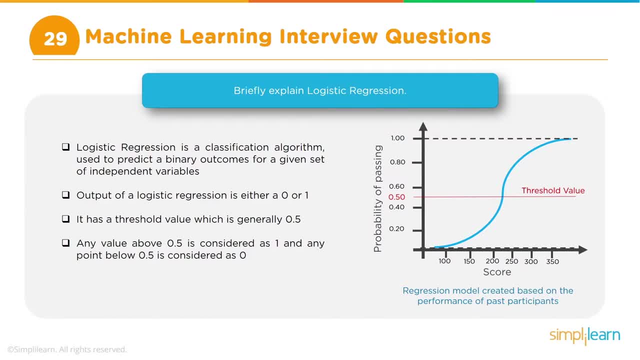 and therefore the name logistic regression. So what is logistic regression and how is it used? So logistic regression is used for binary classification and the output of a logistic regression is either a zero or a one, and it varies. So it's basically: it calculates a probability between zero and one. 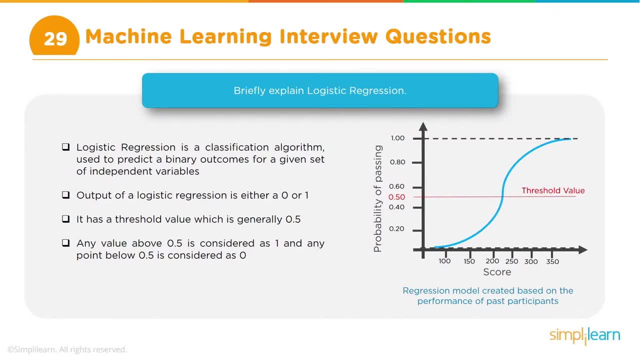 And we can set a threshold that can vary. Typically it is point five, So any value above point five is considered as one, And if the probability is below point five it is considered as zero. So that is the way we calculate the probability, or the system calculates. 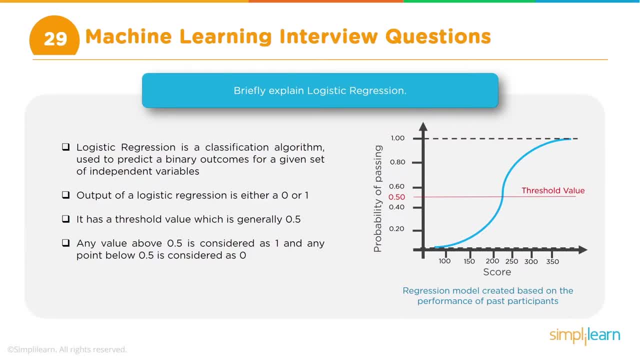 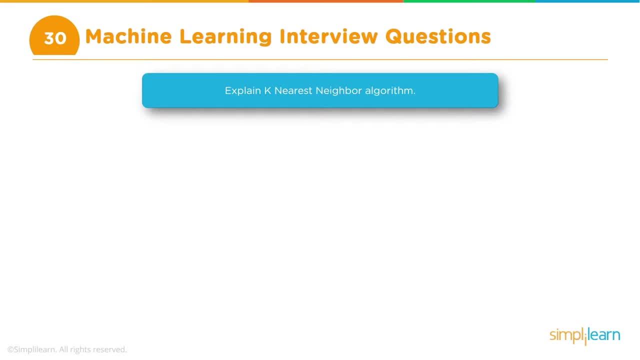 the probability and, based on the threshold, it sets a value of zero or one which is like a binary classification: zero or one. OK, then we have a question around k nearest neighbor algorithm. So explain k nearest neighbor algorithm. So, first of all, what is a k nearest neighbor algorithm? 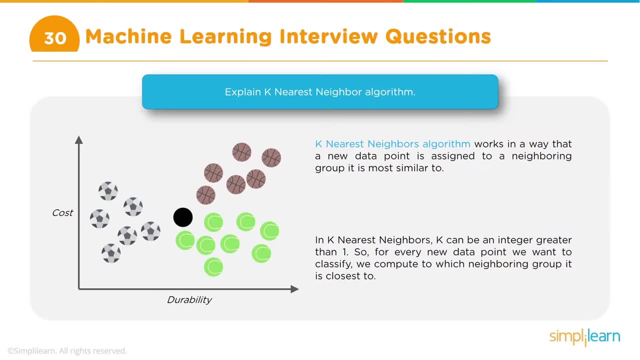 This is a classification algorithm, So that is the first thing we need to mention, And we also need to mention that the k is a number, It is an integer, and this is variable And we can define what the value of k should be. 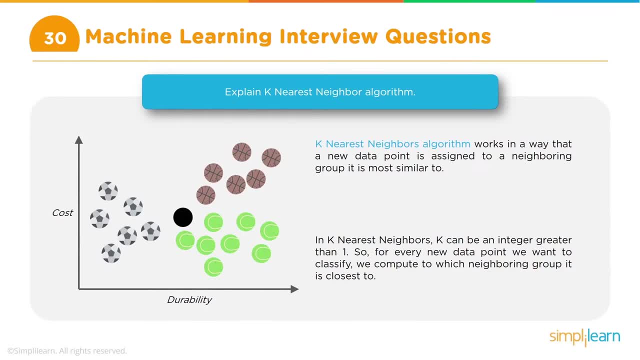 It can be two, three, five, seven, and usually it is an odd number. So that is something we need to mention. Technically it can be even number also, but then typically it would be odd number, and we will see why that is. 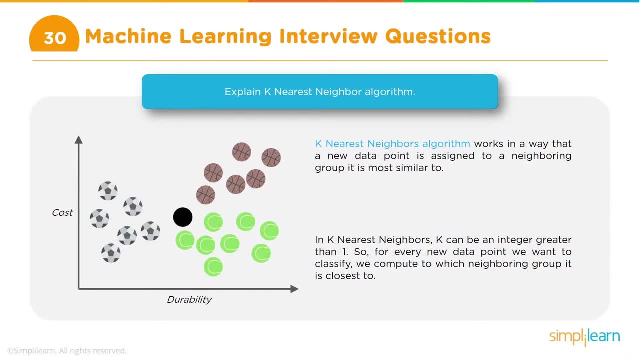 OK, so based on that, we need to classify objects. OK, we need to classify objects. So, again, it will be very helpful to draw a diagram. You know, if you're explaining, I think that will be the best way. 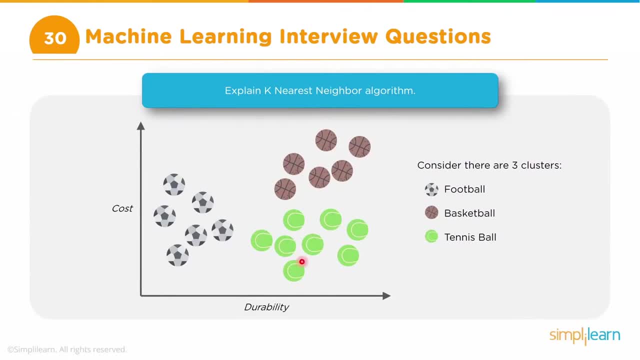 So draw some diagram like this and let's say we have three clusters or three classes existing and now you want to find for a new item that has come. you want to find out which class this belongs to, Right? So you go about as the name suggests. 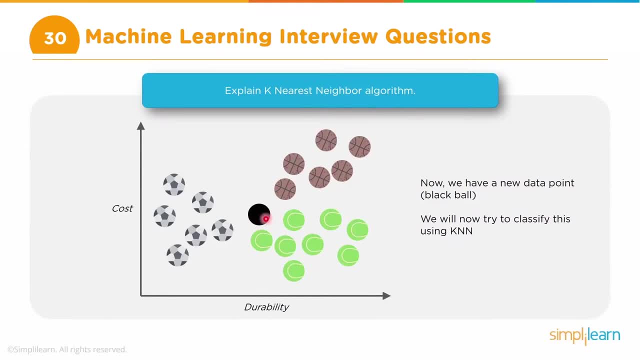 you go about finding the nearest neighbors and the points which are closest to this, and how many of them you will find. That is what is defined by k. Now, let's say our initial value of k was five, So you will find the k, the five nearest data points. 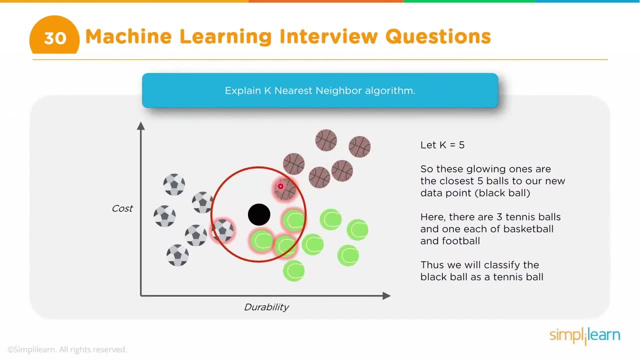 So, in this case, as it is illustrated, these are the five nearest data points, But then all five do not belong to the same class or cluster. So there are one belonging to this cluster, one, the second one belonging to this cluster, two, three of them belonging 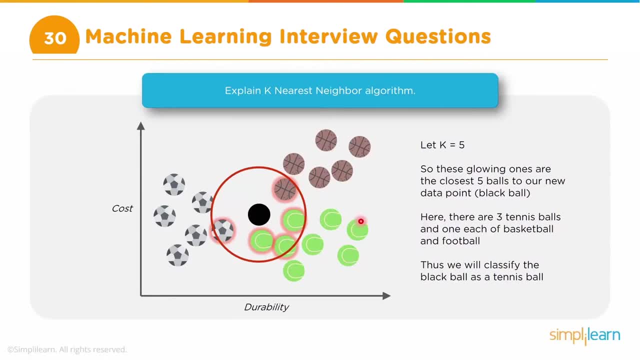 to this third cluster. OK, So how do you decide? That's exactly the reason we should, as much as possible, try to assign an odd number, so that it becomes easier to assign this. So in this case, you see that the majority actually. 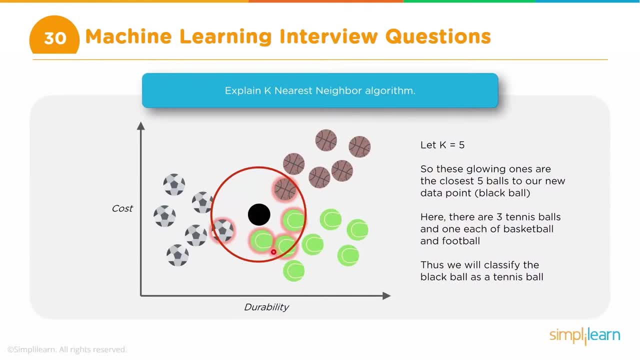 if there are multiple classes, then you go with the majority. So, since three of these items belong to this class, we assign which is basically the, in this case the green, or the tennis, or the third cluster, as I was talking about. 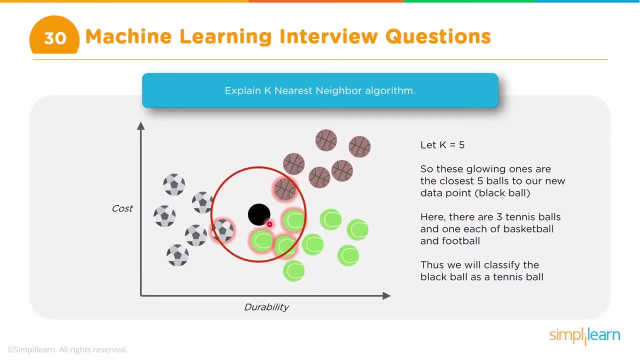 So we assign it to this third class. So in this case it is. that's how it is decided. So k: nearest neighbors. The first thing is to identify the number of neighbors that are mentioned as k. So in this case it is: k is equal to five. 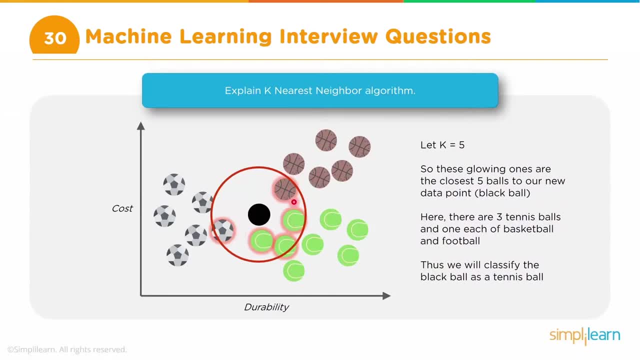 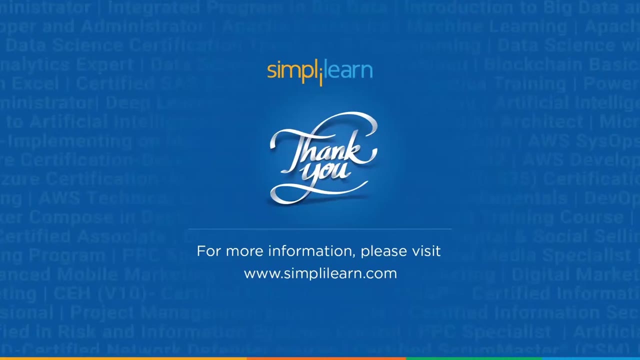 So we find the five nearest points and then find out out of these five which class has the maximum number in that, and then the new data point is assigned to that class. So that's pretty much how k nearest neighbors work, And with that we come to the end of this video. 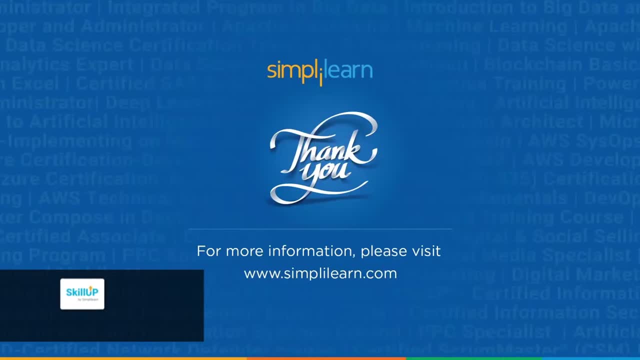 On supervised, unsupervised and reinforcement learning. We hope you enjoyed this video. If you did, a thumbs up would be really appreciated. Also, here's your reminder to subscribe to our channel and click on the bell icon. Thank you for watching and stay tuned for more from SimplyLearn.